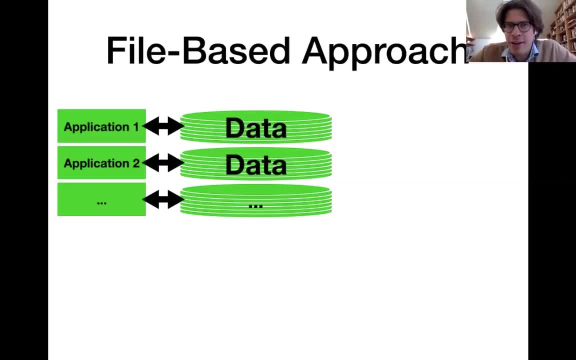 Now if those applications are running in the same organization, for instance, it can create a couple of problems. For instance, here at Cornell we might have multiple applications that all need to store data about students, And if they store the data independently, it means that we are wasting space. 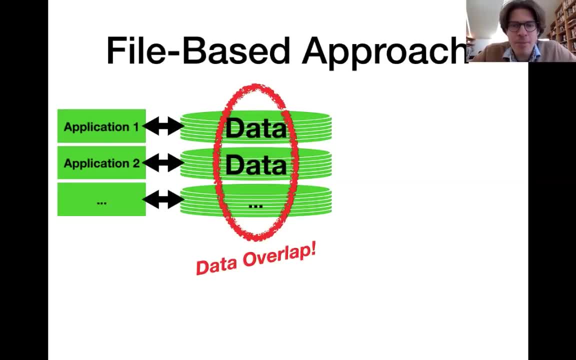 Because we don't have enough data. We don't have enough data Because we are storing the same data redundantly. And what's even worse, if you are updating data like the address of a student, for instance, then if you are not careful, if the data is stored redundantly, you might introduce inconsistencies between different copies of the data, which of course we want to avoid. 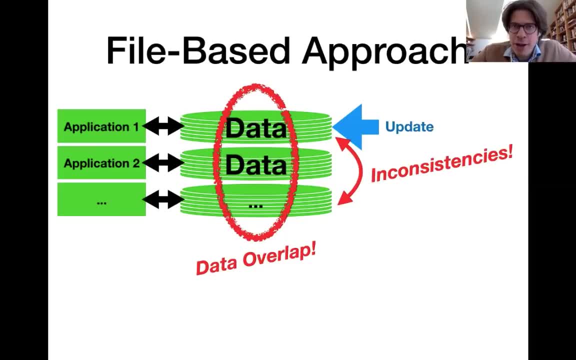 And then, on the other side, if you are managing data- pretty much independently from what specific data you are managing- There's a couple of things that you always want to do. For instance, you want to have some kind of mechanism that recovers your data if you are in the process of editing it and then suddenly your system crashes, for instance because you lose power. 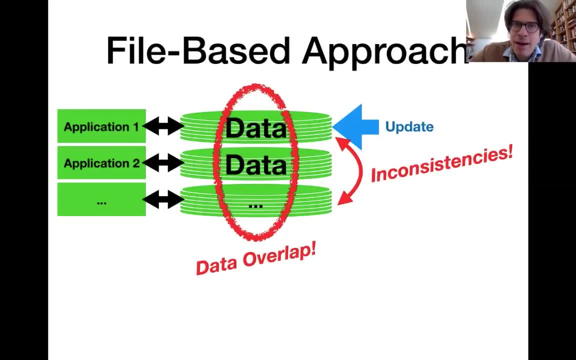 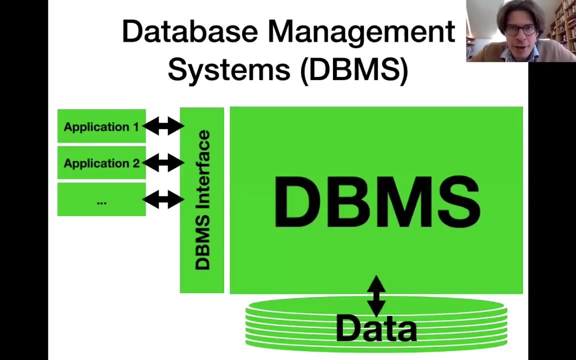 And if we store and manage data independently in each application, it would mean that we might have to reimplement that functionality for each specific application, which is also bad, of course. This is why people came up With a database management system which looks like you see here there is one system managing all the data from the organization, at least for a certain domain. 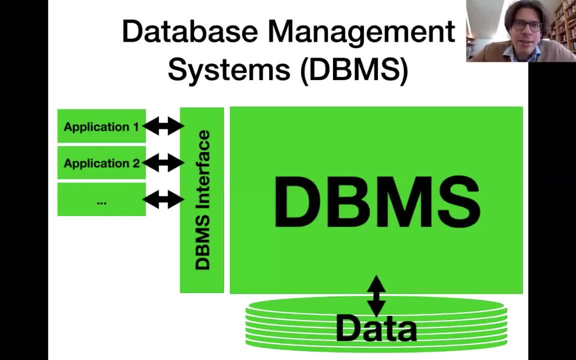 And then those applications. they access this data via the database management system by a unified interface. So those applications. they don't manage their data themselves and separately anymore. Now, for most of this course, we will be discussing About a specific type of data which is very common in practice, which is relational data. 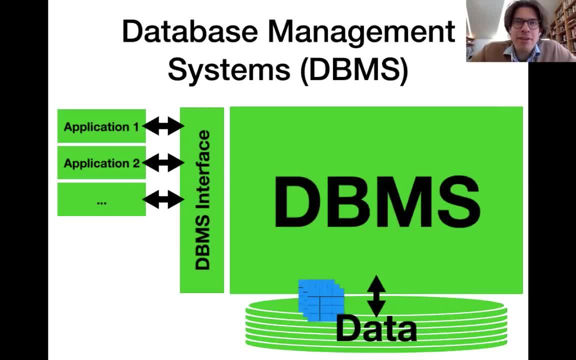 And for the moment, you can think of relational data simply as a collection of tables. Now, in the first part of this course, we're going to discuss about a language for inserting data of this type, for modifying it and for deriving insights from that data. 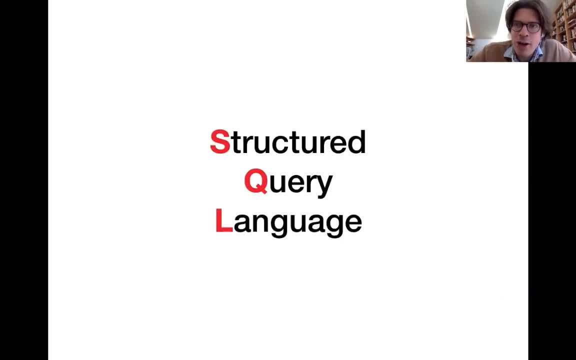 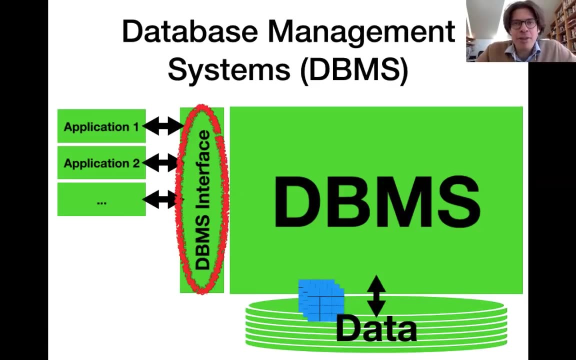 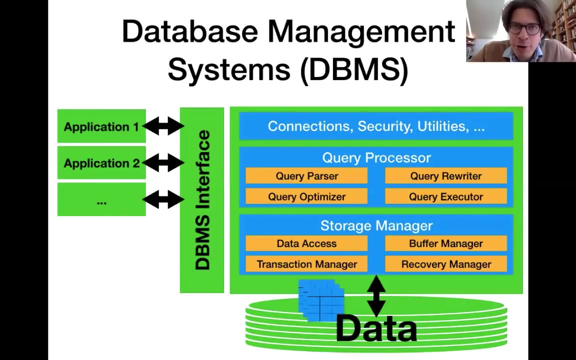 And this language is called the structured query language And it is supported by most relational database management systems. After discussing about the interface, we're essentially going to open up the database management system and we're going to look at the different components that allow it to manage and to process your data. 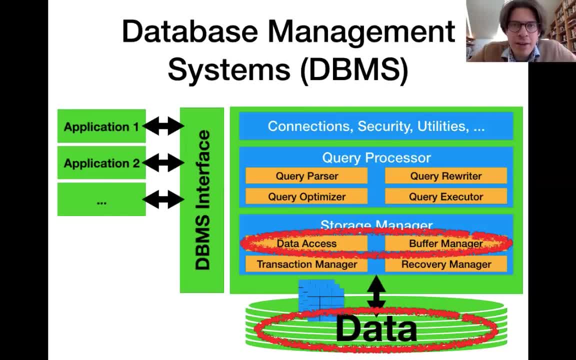 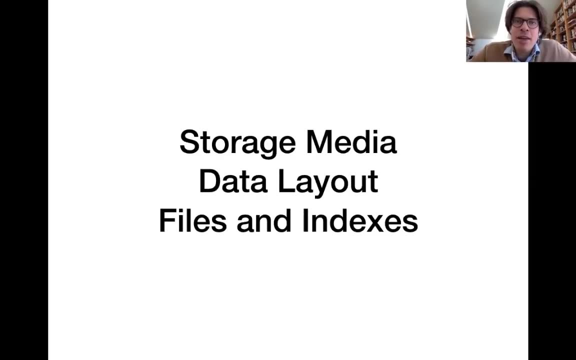 First of all, we're going to discuss about the way in which your data is stored and about how we can access that data efficiently By the database management system. So we're going to discuss first of all, about storage media, such as hard disks, and about the properties and about the way in which we want to store our data on them in order to make access efficient. 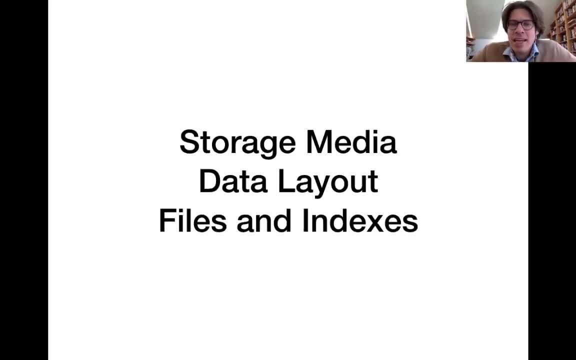 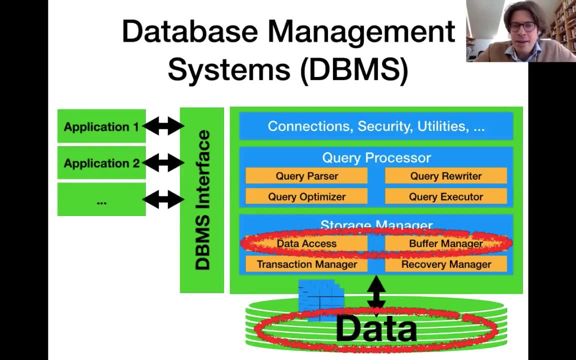 We're also going to discuss about specific access methods, such as indexes, which allow you to very efficiently find specific data that you're looking for. Next, we're going to discuss about how we can process the data and derive A new insights from it. 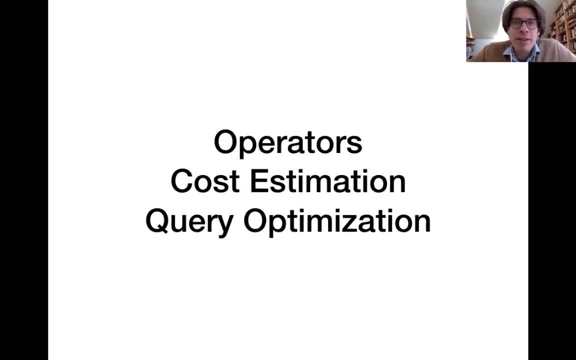 So here we're going to discuss about a standard operators, for instance, operators for filtering data or for combining different data sources. Yes, who called a joins? We're going to discuss about how to implement those operators and about how to connect to multiple operators in a query processing plans. 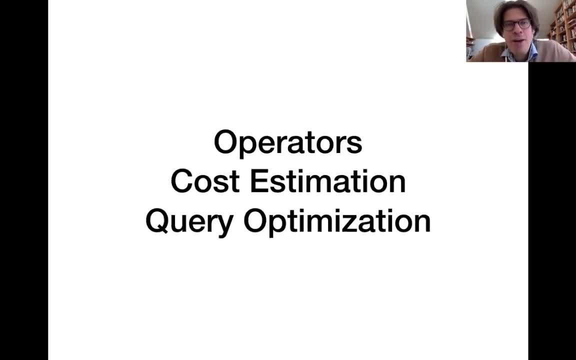 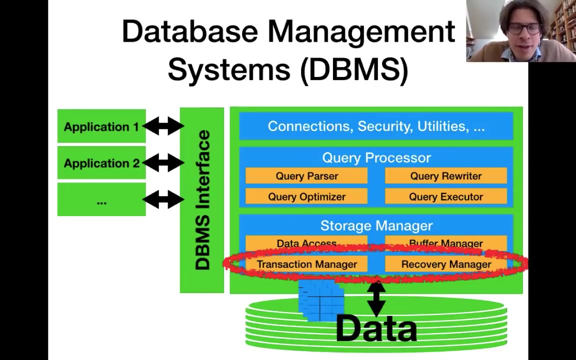 You also got to discuss about how we can estimate processing costs for operators and entire query plans before actually Executing them, which allow us to choose the most efficient plan for an incoming query by a process called query optimization. After that, we're going to talk about how we can process transactions, and transactions are groups of commands that either read or modify your data, which are semantically related to. typically, you either want to execute all operations of a transaction or none of them. 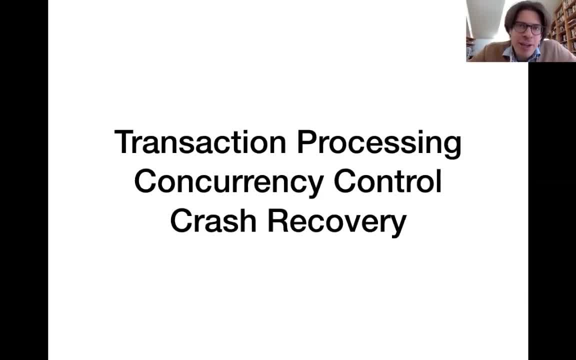 So we are going to discuss about it from sections In particular, we're going to discuss about how we can ensure that transactions are executed properly, especially in cases where multiple users are using the database management system concurrently, which is the Common case, and we will see how we can use a process called concurrency control in order to ensure that multiple users on the same database 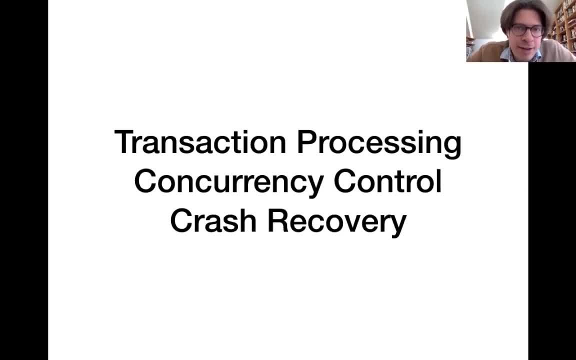 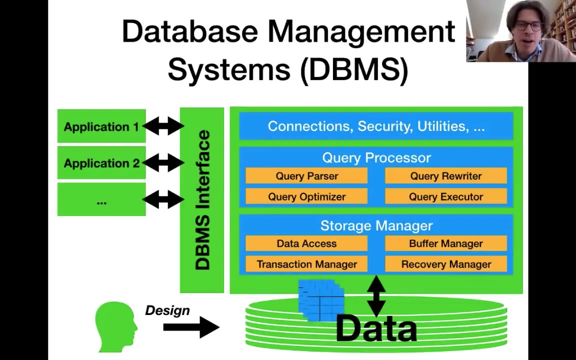 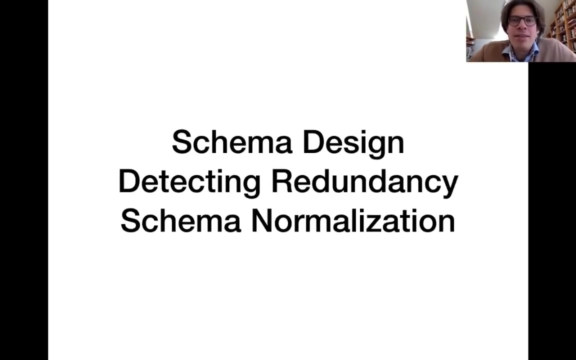 Don't interact In a bad way, which might lead to inconsistent data. and also we're going to discuss about crash recovery, about how we can bring your database back into consistent state after a system crash. Now, after that, we're going to discuss a little bit more about how we can design a good a database. We're going to see a tools that allow you to design the schema of a database for a specific use case. 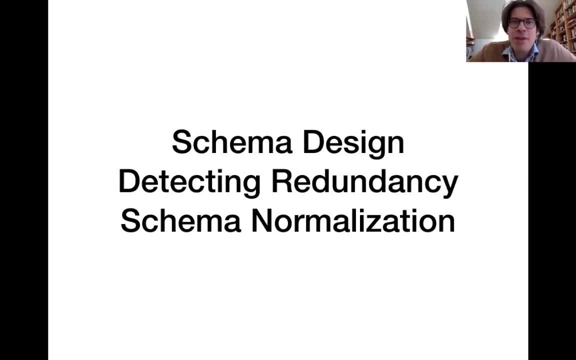 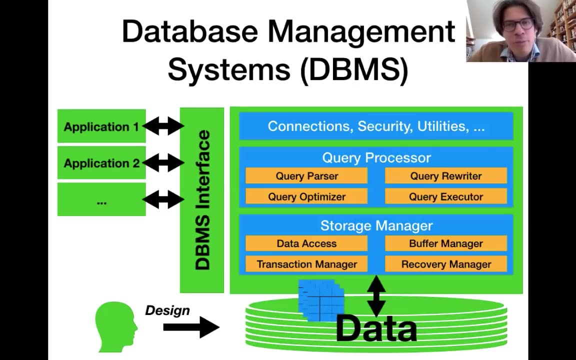 We're going to see how we can detect the redundancy In those as key matter and how we can optimize those as key matter by normalization and at this partially get rid of that redundancy. Now, if you want to serve a large number of users or if you're dealing with a lot of data and typically you don't want to run your database on one single machine but you want to distribute it and run multiple instances on multiple machines, So in the next part of the course, 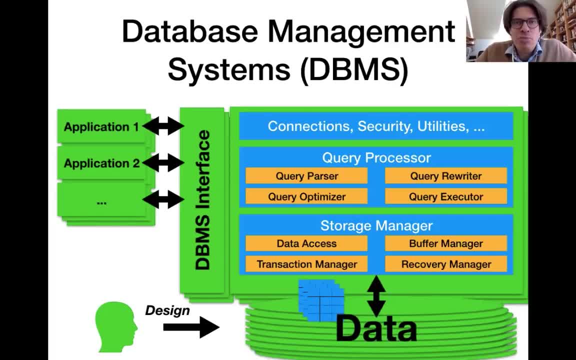 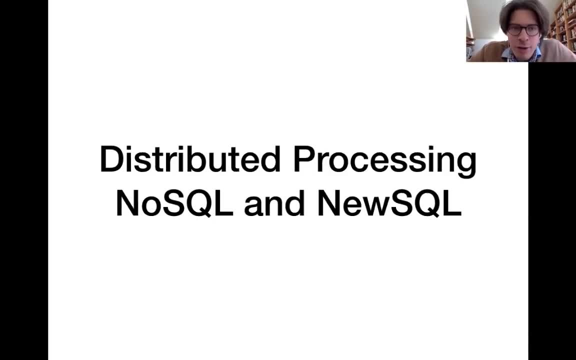 Next part of the course, we're gonna discuss about distributed data processing. We're gonna discuss about corresponding challenges and how we can solve them. We're also gonna discuss about terms such as NoSQL and NewSQL, which are some recent trends in data processing. 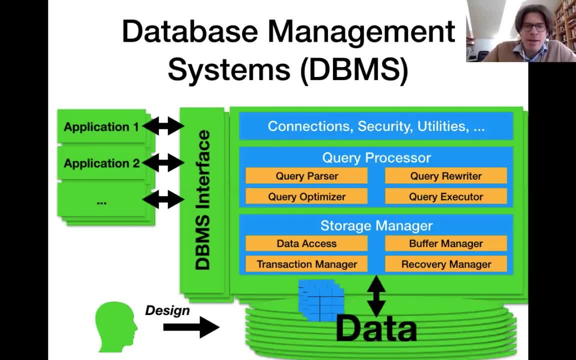 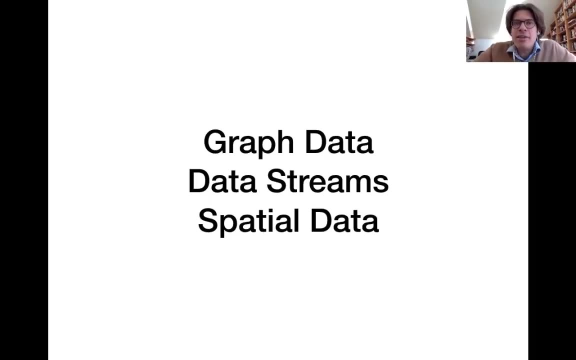 We're also gonna see a couple of corresponding systems. Now, in the final part of the course, we're gonna broaden our scope beyond relational data. We're gonna look at different types of data, for instance, graph data, spatial data and data streams. 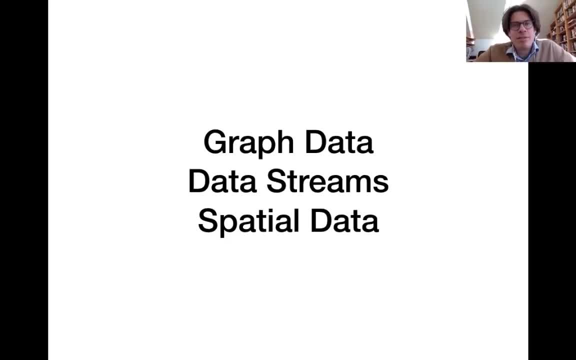 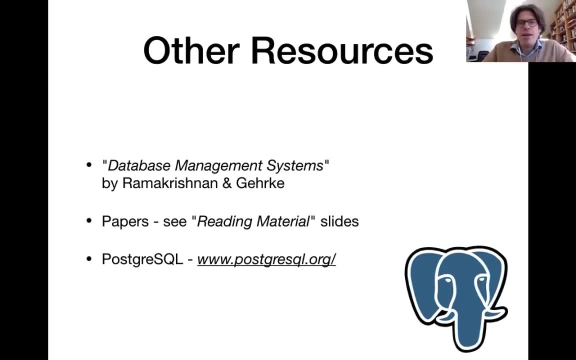 And we're gonna discuss about specific systems that have been tailored in order to store and to process those different data types. Now, in order to follow this lecture- you can follow it without additional material, but it can be helpful to look into the book. 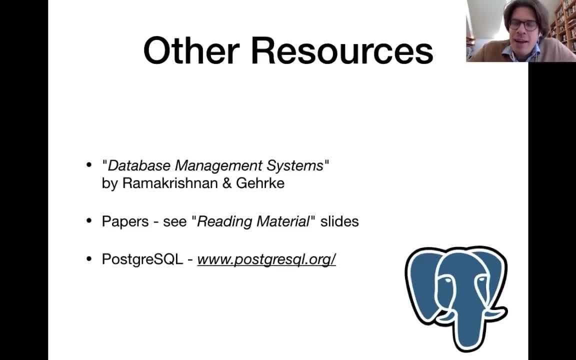 Database Management Systems by Ramakrishnan and Gerke. Often at the beginning of my slides I will have the abbreviation RG, followed by a section number, and that refers to the corresponding section in this book, in case you want to read up more details. 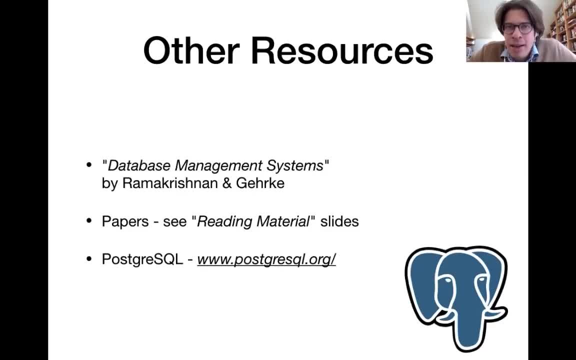 Also, especially for some of the more recent systems that we are discussing, I will give you references to specific papers that provide you specific references to specific papers that provide you with more details, And those references are typically at the beginning of my slides, titled reading material. 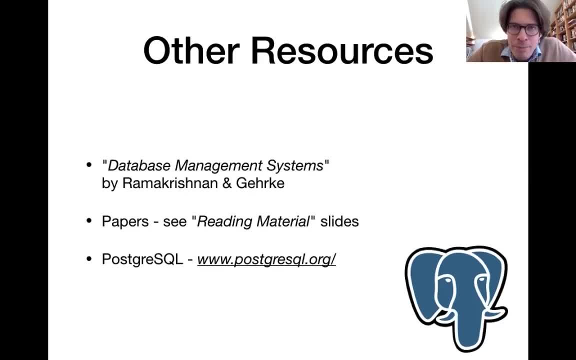 And then in this lecture I'm gonna make a lot of examples. I want to show you what it is like to use one of those database management systems in practice and how to get some impression for what's happening inside And for those examples. 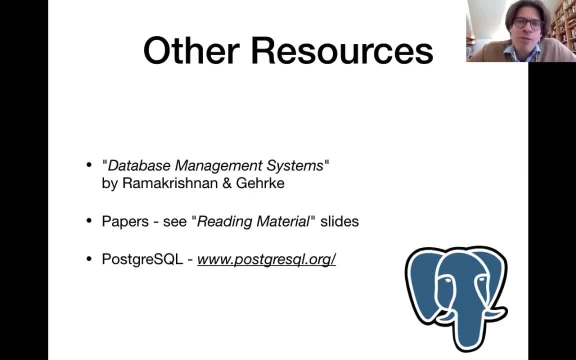 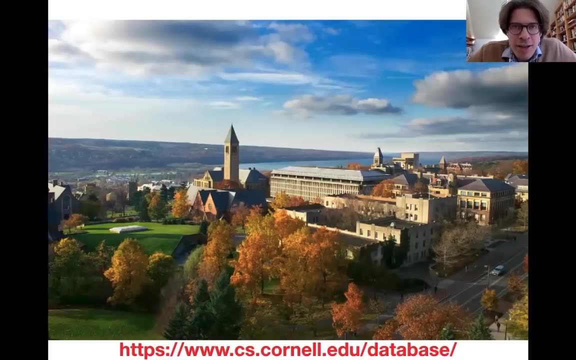 I'm gonna use the Postgres Database Management System, one of the most popular open source database management systems. one of the most popular open source database management systems. you can find it, download it and install it at the web address that you see below. Now, this course was given at Cornell as an online course. 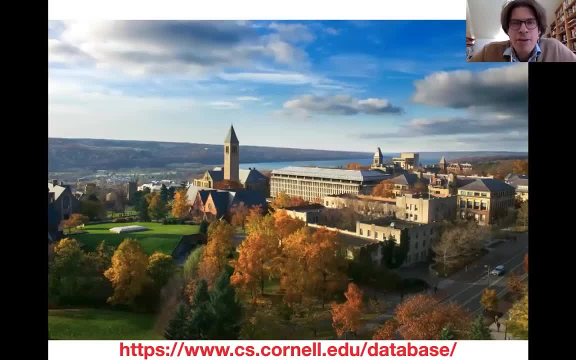 in fall semester 2020.. Students were able to interact with me via the chat. Sometimes I'm getting questions on the chat which you will not be able to see because we want to keep the students anonymized, but I typically read out the question and the course. 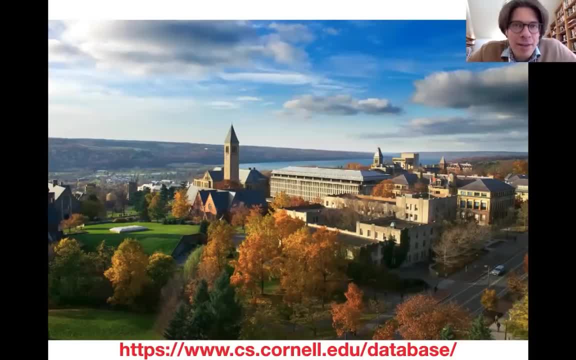 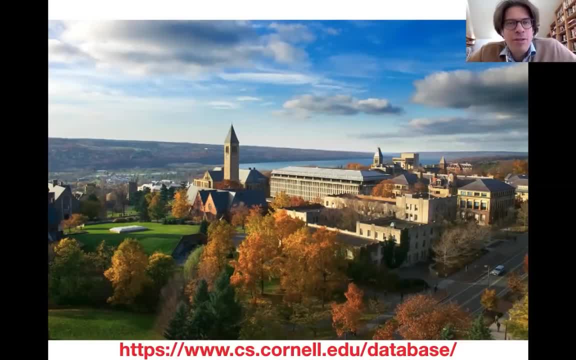 that ask you, for instance, to write a queries in order to solve specific tasks. I encourage you to do those exercises with me. Typically, I give you a couple of minutes to solve them. I'm from the Cornell Database Group, So if you get interested, 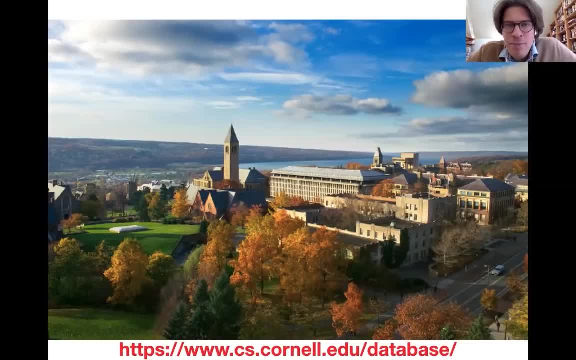 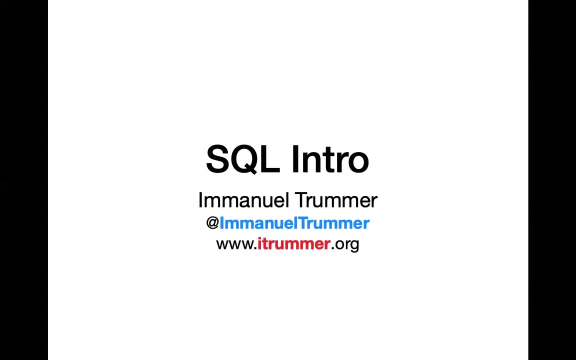 buy this course in database systems in general and perhaps become interested in database systems research. please check out our website. You'll see the URL below. And now I wish you good luck and have fun with the course. The last time we have been talking about database. 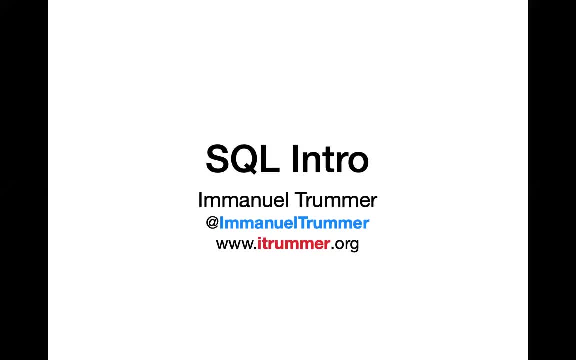 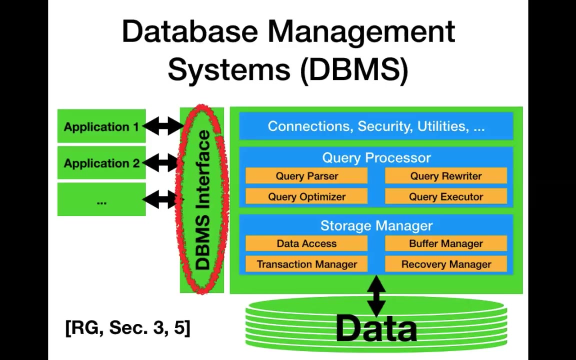 management systems, which is a system that essentially manages the data- all the data that you are interested in- and then different applications can access the data by a unified interface. Thank you. Here you see the high-level architecture that we have discussed the last time. 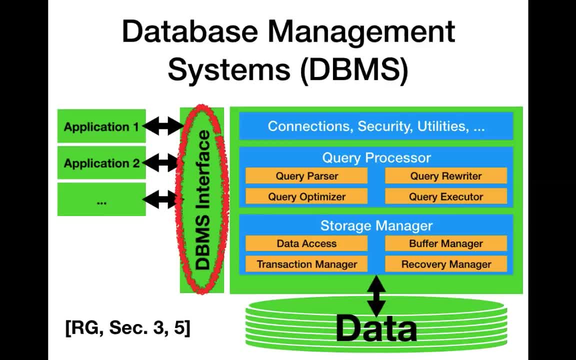 I gave you a quick overview. in the coming lectures We're going to look at different components within the architecture and we're going to discuss in more detail what is behind that. Now, in this lecture, and also in the following lectures, we'll be looking at the interface to the database. 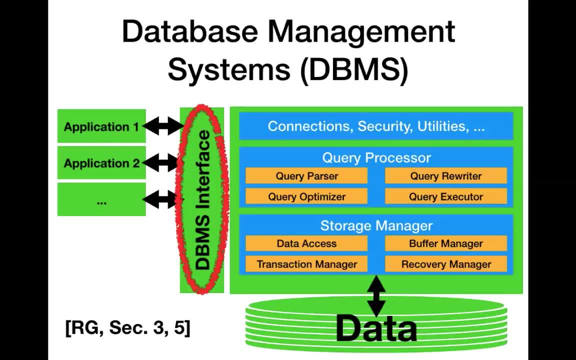 system. So that is essentially the interface that either you as users are directly using or that the application is using. Thank you, Thank you. Thank you very much. Thank you for the questions about database management and where to begin and how the help can be given. 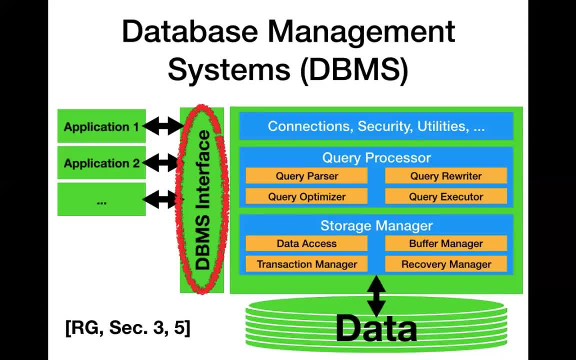 to help combat the overall space we call database management, Thank you. Thank you for among the questions related to getting the data in the database to ant. I hope that the Q&A went smoothly. It was very good. courtesy of line are COVID общation. 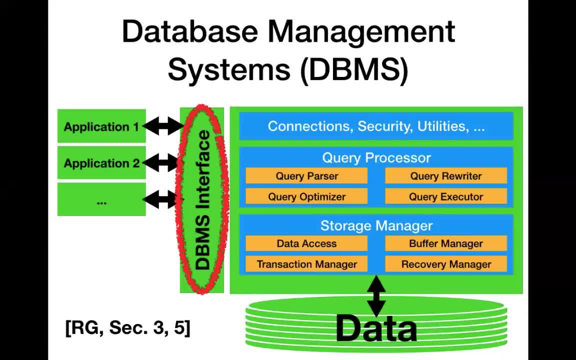 on the server. I'm happy to talk with you. See you later And we will have time for discussion. Bye, bye. our G that stands for Ramakrishnan and Gerke and the relevant sections. it's primarily section 3 and section 5. the question last time was whether you actually need the book and you don't need the. 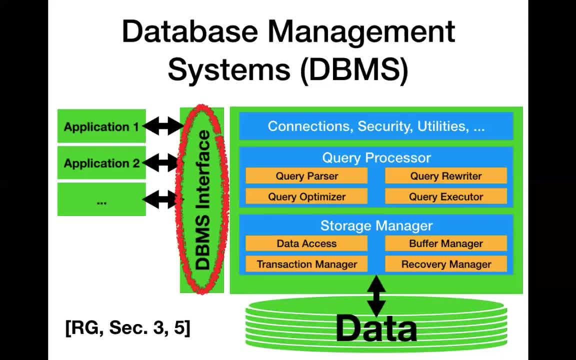 book, if you understand everything that I point out here in the course. so for the homeworks, the relevant material is what we are covering in the course, but if you want additional information, then it might make sense to have a look at the book. all right, so now we are talking about the database. 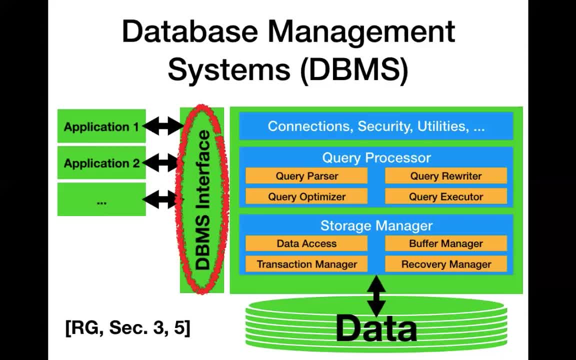 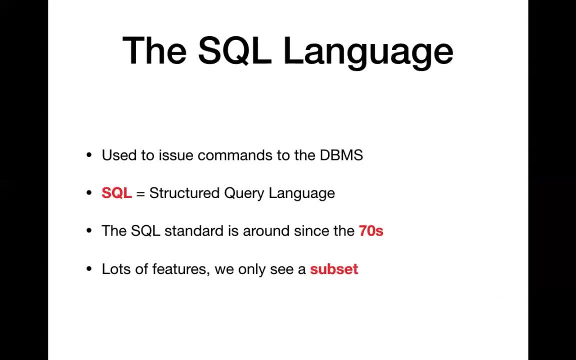 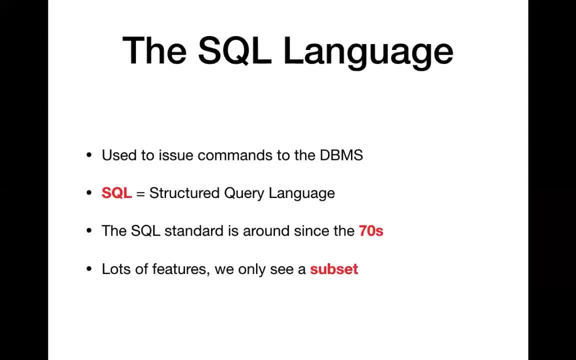 data in some way. it's a very old standard already. I mean, the first version of it appeared in the 70s and currently the latest version has a couple of hundred pages. so you're not gonna cover all of SQL. it's a very powerful language, but you're gonna see a subset of features which are sufficient for. 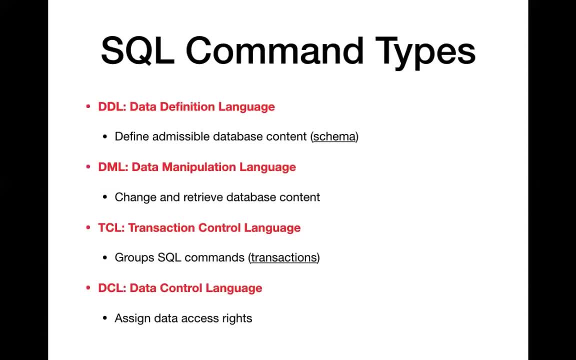 most use cases now, people decide to use the database as a way to use the database as a way to use the database. so you can distinguish different types of SQL commands depending on what they do. first of all, you have the so-called DEL data definition language, and that one essentially allows you to define what 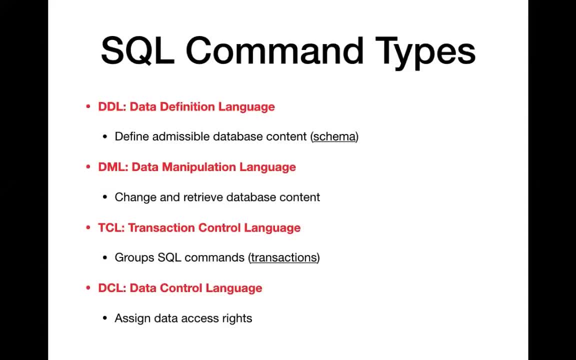 the structure of your database looks like. so you can essentially tell the database management system what kind of data entries are admissible. you can set constraints, and then the database management system will reject any changes to the data that would not comply with those constraints. then, beyond defining constraints, of course you can also: 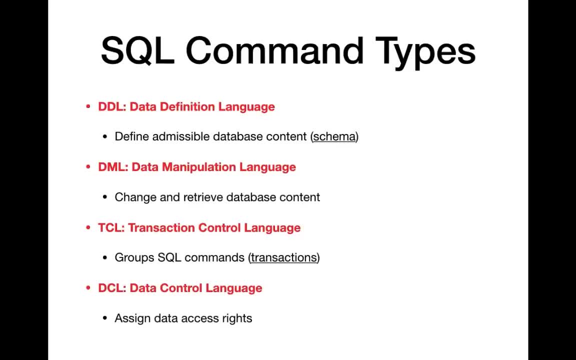 insert and manipulate and retrieve data. that is the DML, the data manipulation language. you also have the transaction control language- that one is discussed a little bit later- which allows you to group SQL commands into so-called transactions, which have several nice properties that we'll discuss in a few minutes. 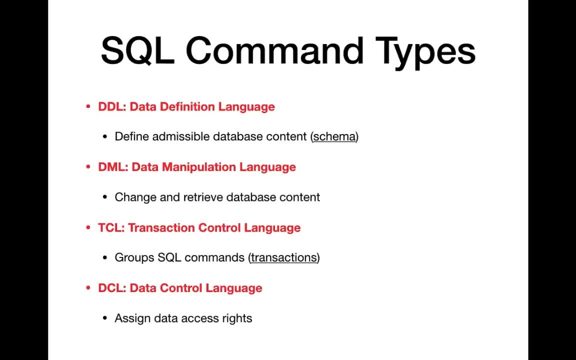 later. Also, you have a couple of commands in order to assign data access rights, for instance, which are controlled by the database system, but that we won't go into detail in this course. All right Now. in the following, we will first of all discuss about the data definition language. 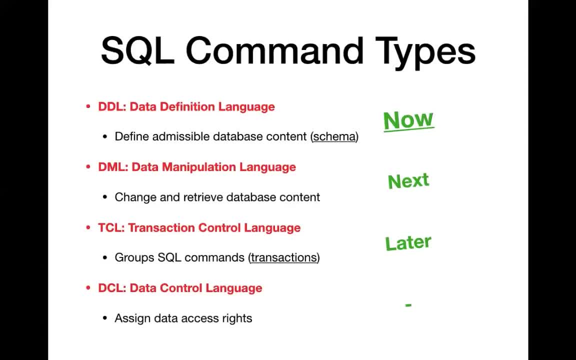 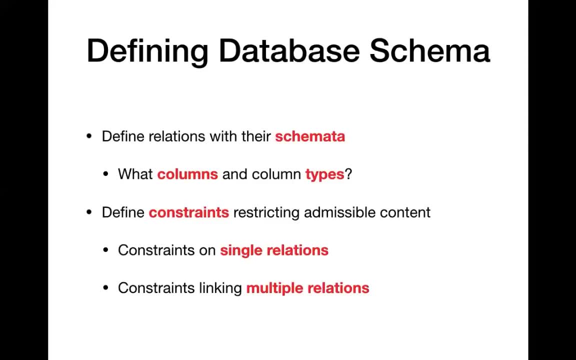 After that we cover the data manipulation language. The TCL is covered a couple of lectures later, not immediately. So let's start with the data definition language. You are defining a so-called database schema which essentially describes the content that you can insert into your database. Now we have heard last time that those relational databases 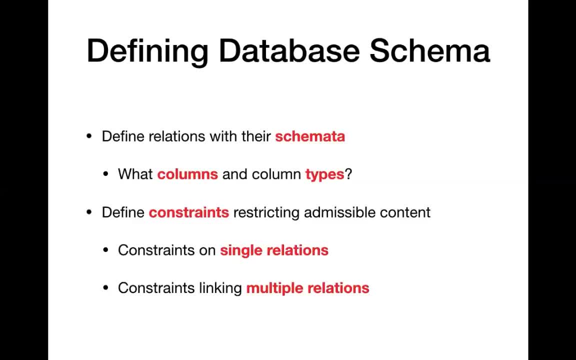 that we are focusing on here. they consist of a collection of relations, where each relation essentially looks like a two-dimensional table, essentially a little bit like a spreadsheet, And one first thing that you can define for each relation is: what are its columns? 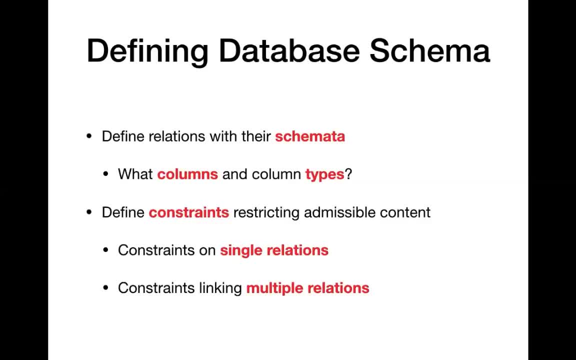 what are the names of the columns and what are the data types of the columns? Because each column of a relation is associated with a data type and once you insert data entries into that relation, they actually have to comply with those data types. We're going to see some concrete examples. 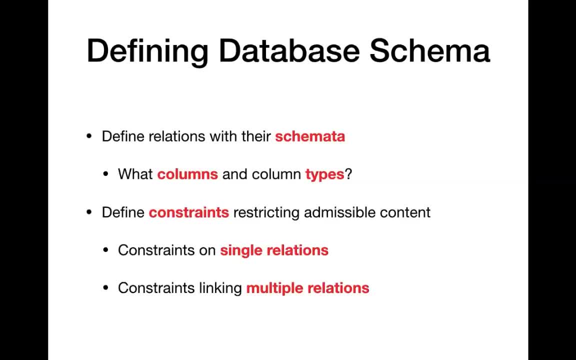 later You can generally introduce more constraints beyond the data type. You can put constraints on single relations. You can also define constraints that link multiple relations. You're going to see some specific examples for constraints in the following slides. Now, in order to 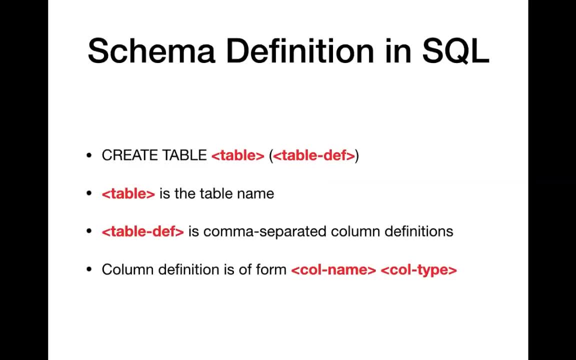 create one relation. this is the command that you use in SQL. In SQL, you're going to need a table. We are essentially. we are actually not talking about relations, but we're talking about tables. So, strictly speaking, there's a couple of fine differences between relations in the. 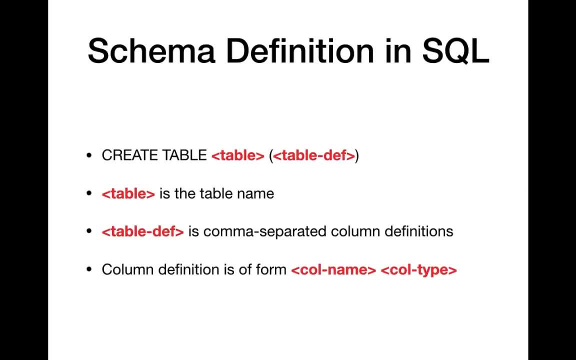 relational data model and tables in the SQL language, But for the moment I'm not going to go into detail here. You can assume that what is called table in SQL is meant to represent what I called relation in the context of the relational data model. And this is the command. 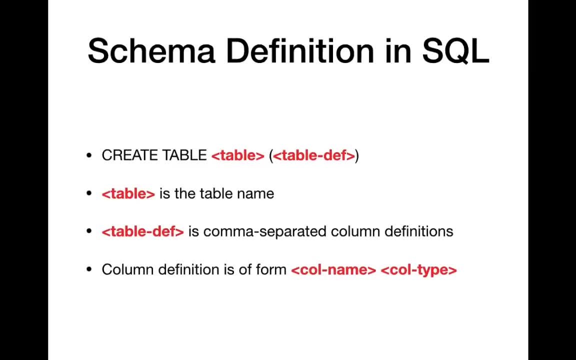 that you use when you create a table and when you write the table, you have to write the name of the table And then, between parentheses, you have a comma-separated list of column definitions, where each of those column definitions consists of the column name and the column data type. 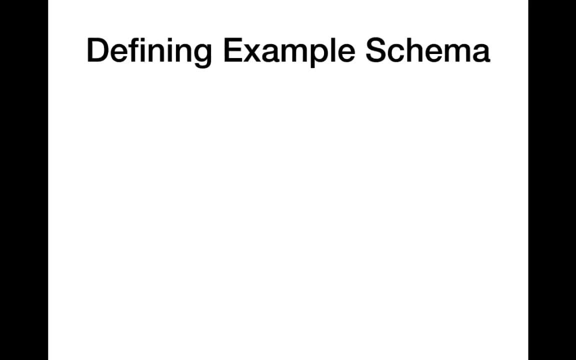 Now let's make things a little bit more concrete. So in the following, we are going to use a very simple university database with information about students as a running example. So First of all, it might make sense to introduce a table. 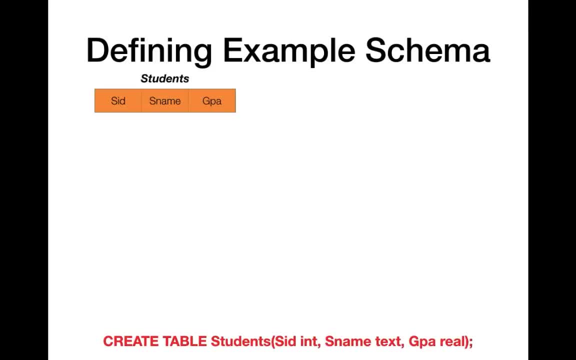 in order to store information on students, And you can do this with the command that you see here. I am telling the database system. I want to create a table named students which has an SID, a student ID of type integer, then an S name- student name- of type text. 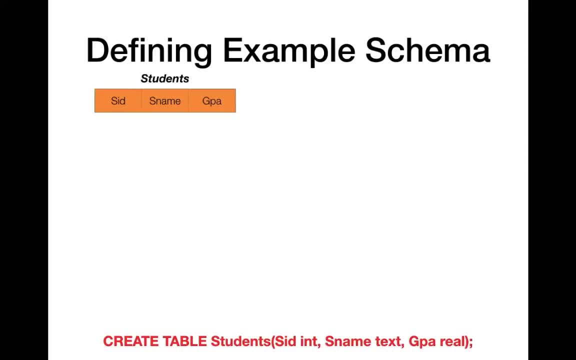 and the GPA of type real, All right, and maybe I also want to keep track of which courses those students are enrolled in. So I might want to introduce a table enrollment which essentially links student IDs to course IDs. So the content of this table that you see. 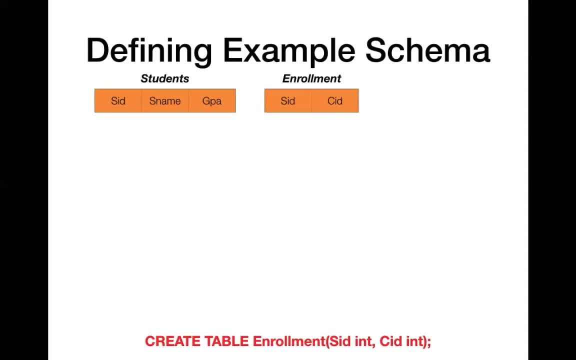 in the middle enrollment would be pairs of student IDs and course IDs, with the semantics that the corresponding student is enrolled in the corresponding course, And maybe the course ID alone. that's not very informative, So ideally we also want something which links the course ID to the course name. 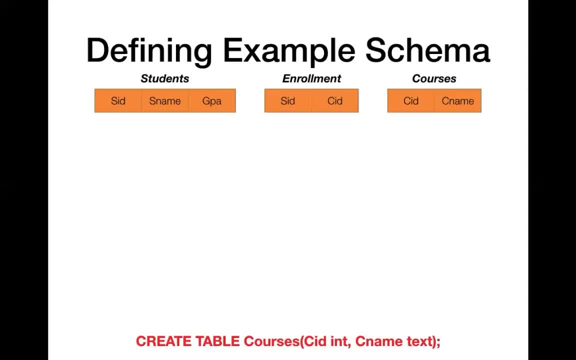 So we can introduce one more table which is doing this, which has the course ID and the corresponding course name as columns. All right, So that is a very simple database with three tables and you can create that relatively quickly with SQL commands. Now 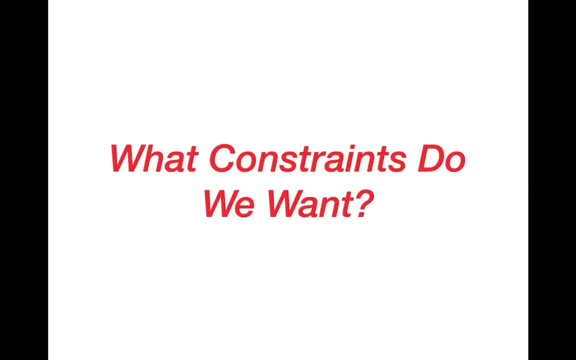 beyond specifying that certain columns have certain data types. perhaps we want a couple of other constraints. Is there any kind of constraints on that database that anyone can think of? constraints that essentially ensure that the database content will make sense. So if you have an idea for a constraint, 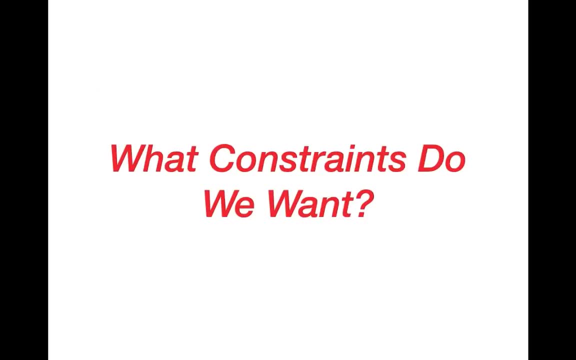 please write it into the chat. All right, here comes already like the. okay, very good, Very good. Okay, there's a couple of very nice propositions here. Thank you, Okay, please feel free to still type something if you have another idea. 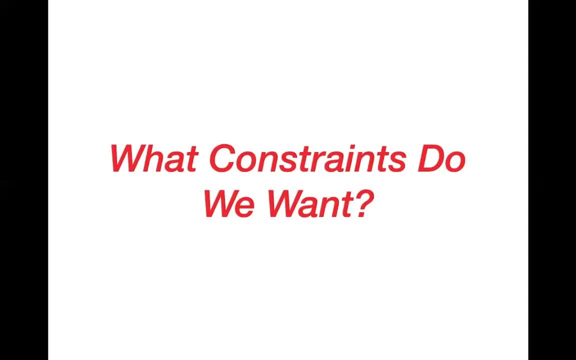 Right. So there's a couple of propositions about restricting, for instance, the value range for the GPA, And that makes a lot of sense, because right now it could be any kind of any kind of, you know, a real number. 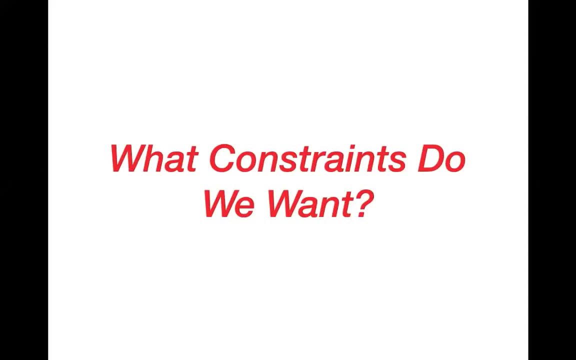 So restricting the value domain further by, for instance, setting a non negativity constraint. that is good, And the other thing that I see here in different variations- there's many very good ideas here, Thank you, That's amazing- Is to enforce some kind of uniqueness constraints. 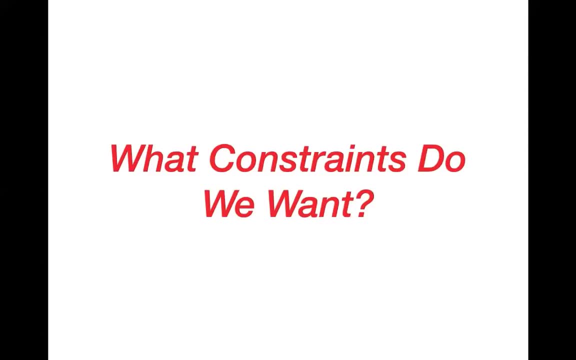 For instance, we have all those IDs in our database And typically, in order to make sense, we have to have, you know, we have to have a number of values. We have to have a number of values. So to make sense, an ID should be unique. 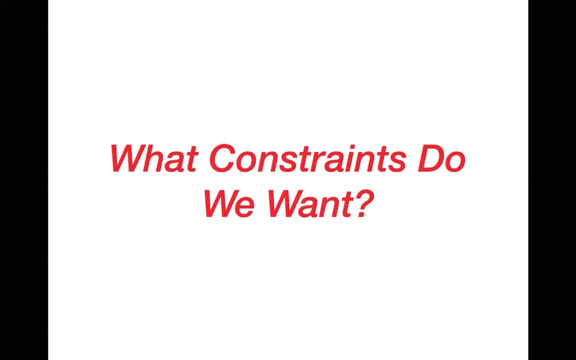 So you shouldn't have, for instance, two students with the same net ID, because that would create all kinds of confusion. So the proposition here is to add some constraints which enforce a uniqueness in certain columns when it comes to the IDs, for instance. 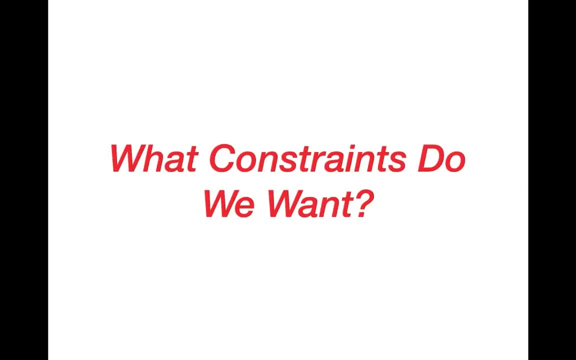 And another group proposition is, for instance, that if you look at the enrollment table, the enrollment table links students, Students- to courses. So what we want is that the student in the course that are linked, that they actually Exist and that a corresponding entry has been inserted into the corresponding other table. 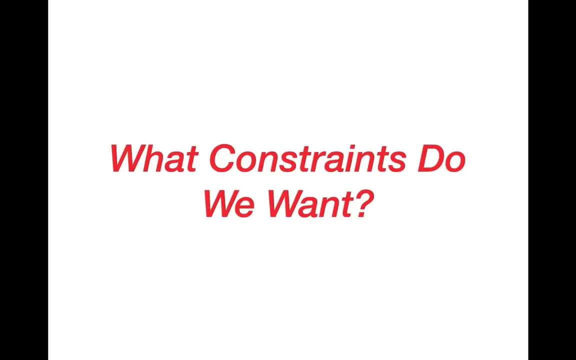 So you don't want to store enrollments for a student for which you don't have the name entered, and you don't want to store An enrollment for a course that doesn't exist in your database. So it makes a lot of sense to link those different tables together. 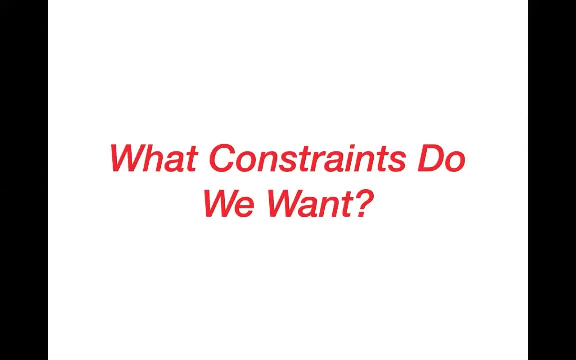 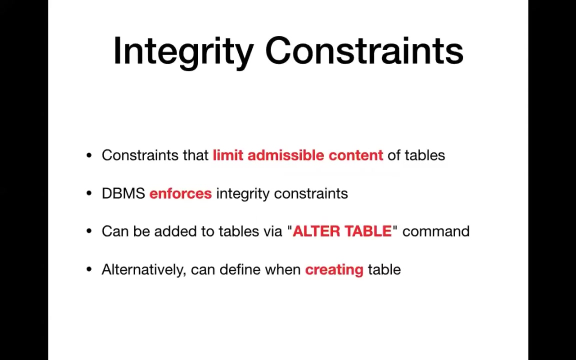 Mm-hmm. So very good propositions, and this essentially Covers already the things that we will see in a little bit more detail in the following. So very good. now. General term here is called integrity constraints. they generally add, like limits, the content that you can insert into the database and 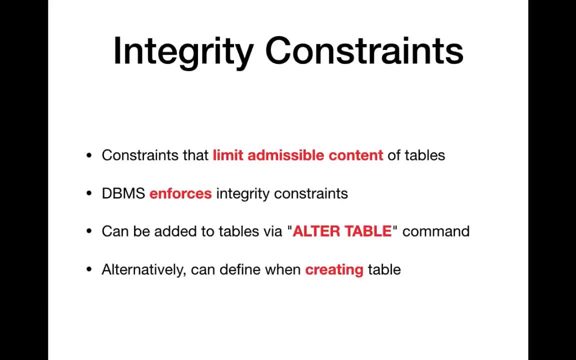 the database System takes care of enforcing those constraints. So if you try to change the data in a way that violates one of those constraints, then typically the database system will tell you to that the update cannot be done, or What we will see later. There's also possibility that the database system 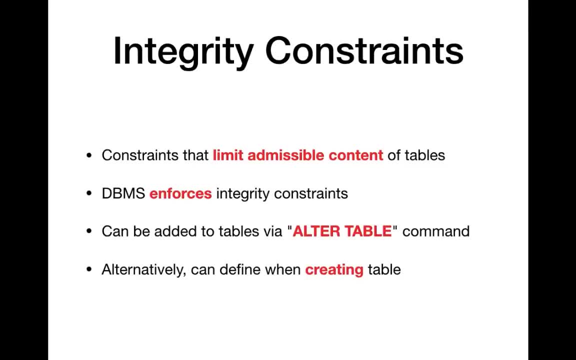 Essentially tries to fix things itself, But in the most typical case it would just essentially tell you: no, This update is rejected because it violates one of those constraints. alright, yes, different ways of adding those constraints to the table schema that we have defined before in general in SQL. 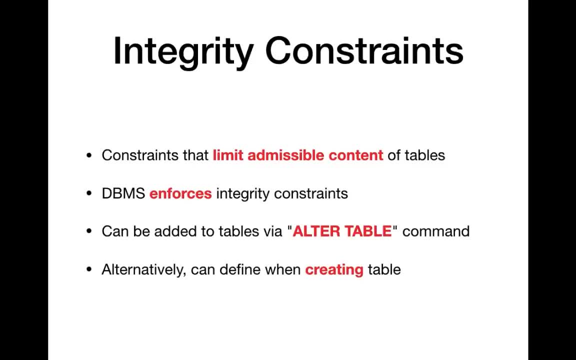 There's always many, many different ways of expressing the same thing. So if you are using seek for over a while, then you will learn about different variants and you will typically figure out what what variant of Of the commands you prefer. So in the following we're gonna see one way of writing those constraints, for instance: 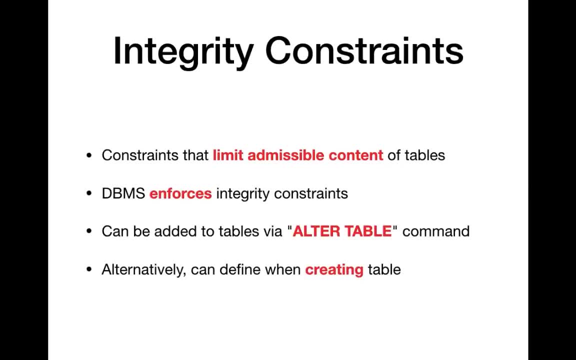 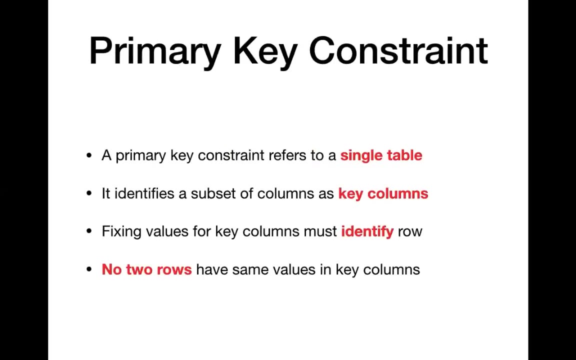 But just so you know, there's many different ways of writing the same thing. alright, so We can add constraints, for instance by using the alter table command and this first type of constraint that we will be looking at. those are the primary, a key constraints, and I have already seen somewhere here in the 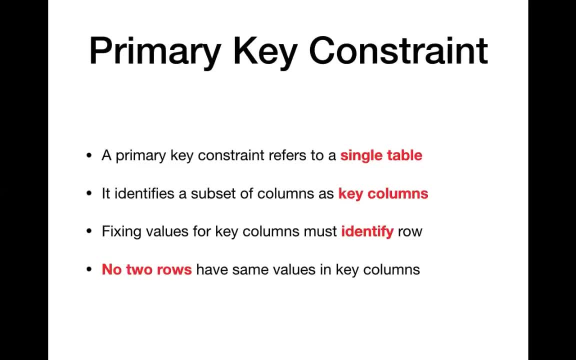 Chat, the key word, the catch word, primary keys are very good. That essentially is a constraint By which you say that one column or a combination of columns corresponds to an ID, a unique identifier. so Those primary key constraints are placed on the single tables and they identify a subset of columns generally that are key corners and 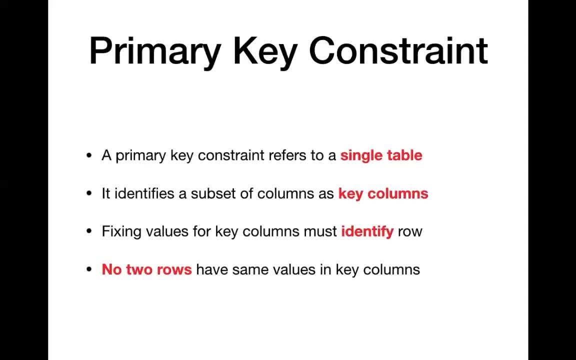 The semantics is that no two entries in the same table Can have exactly the same value combination in those a key column. so that means that if you fix the values in the key columns then you Automatically you narrowed it down to one single note, Like for the students. if you have the net ID, you narrow it down to one specific student. 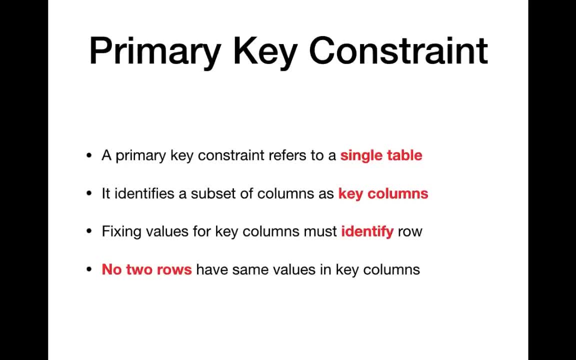 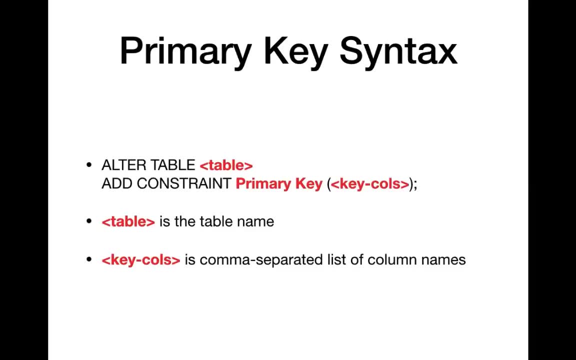 Because no two students can have the same net. So this is the general Syntax of the command. you write alter table and the table name add Constraint make sense, and then here we want to add a primary key constraint. So here between the parentheses you have comma separated list of the columns that you want to become the key. 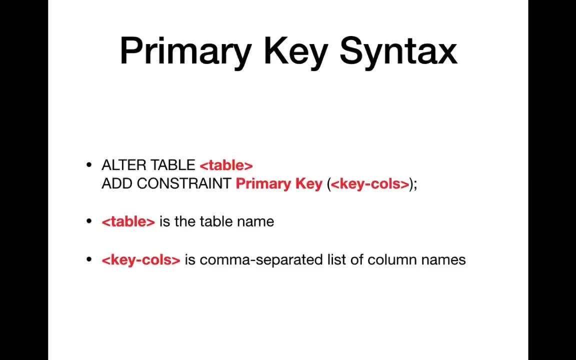 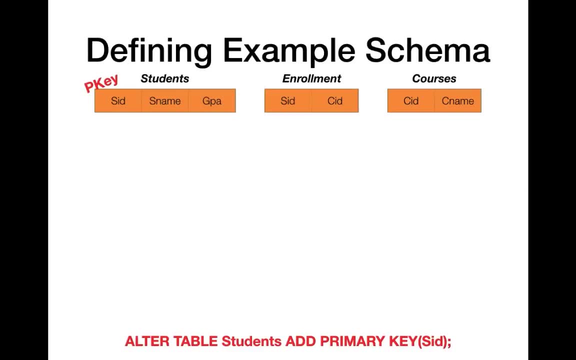 So those columns must exist in the table that you're altering. for instance, here you're altering the students table by adding the constraint that the student ID should be a Key, so it should be unique, and you must have a value entered there Also for the enrollment. 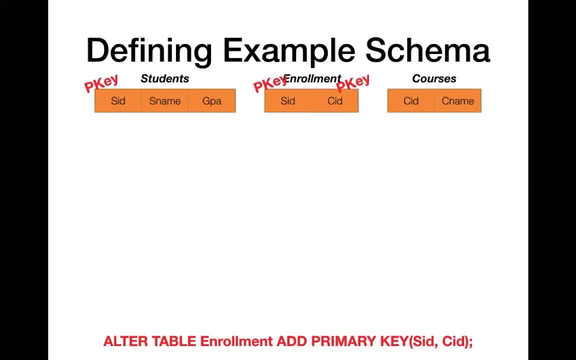 It is. maybe it is a little bit more difficult because for the enrollment The same student could be enrolled in two different courses, So then would have two entries in the enrollment tables with the same student ID, Also for the same course you might have. you typically have many students. 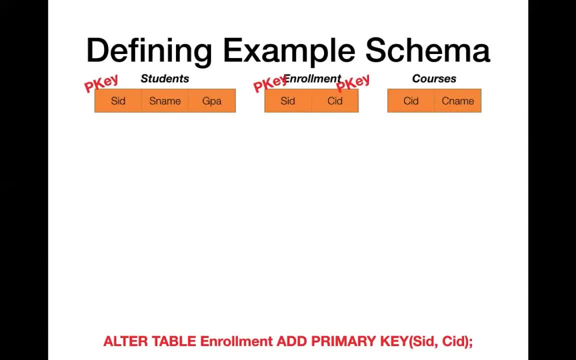 That are enrolled in the same course, Which would be represented as multiple entries in the enrollment table with the same course ID. So in separation, we cannot say that either the student ID or the course ID forms a key for the enrollment table, Right? So what we do instead is that we take the combination of the two. we say that: 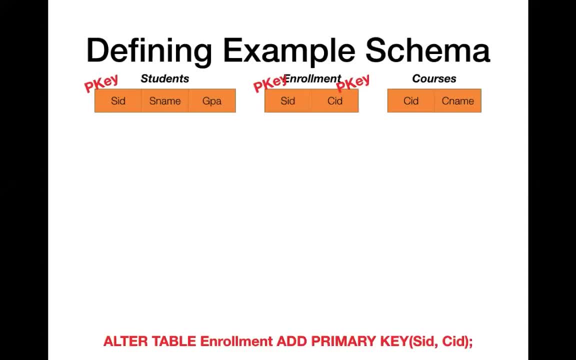 The student is not unique by the core in the course is not unique, But the combination of a student a course should be unique because otherwise he would be storing enrollment information twice. that seems redundant and unnecessary. Now might change, by the way, if we Add, for instance, a year. call him in the enrollment if we say that we don't keep track of the current state. 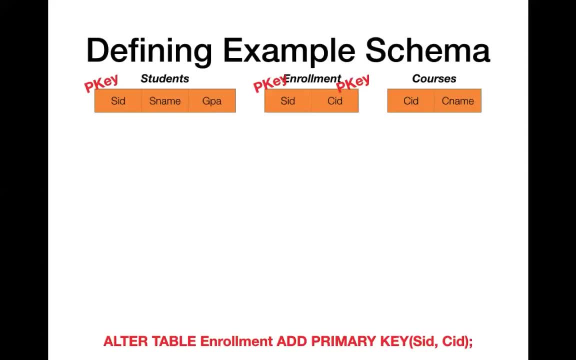 But also of the state in past years that it might make sense somebody is taking the same course twice, then you would have to extend it. but for this value, very simple database, we can say that a combination of the student and the course is unique. finally, with regards to the courses table, we have said that the course id should be unique. 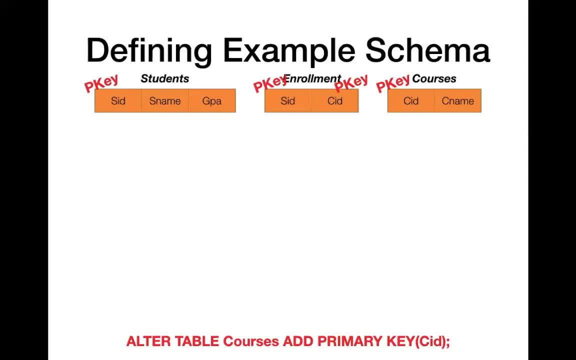 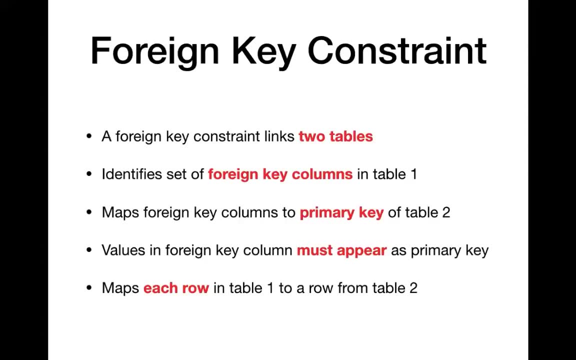 and this is the constraint in order to express that. so now, a different type of constraint is the foreign key constraint. this one links together two tables and in one of those tables it identifies a set of foreign key columns, and then it links those foreign key columns to the primary columns in another table. 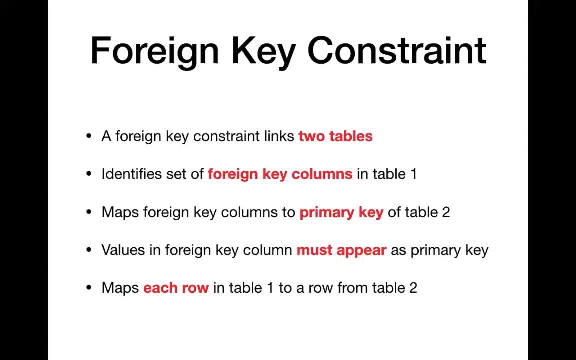 and the semantics is that you are essentially stating that any value combination that appears in the foreign key columns must also appear in the primary key columns, because you are essentially linking each entry in the table with the foreign key to one entry in the table with the primary key. so if we fix the values in the foreign key columns, 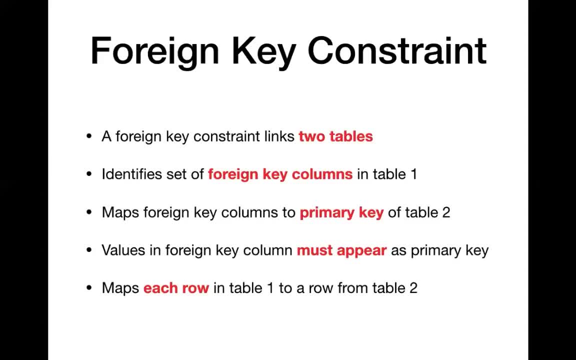 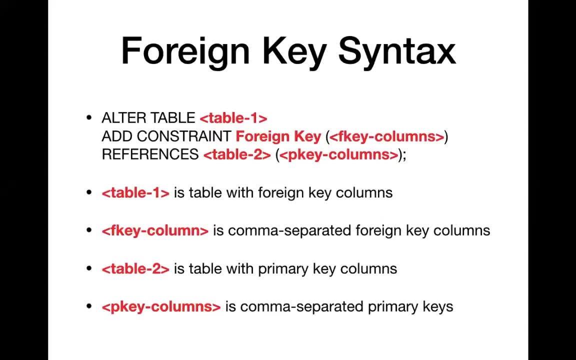 then that should narrow it down to one single row, to one single associated row in the table with the primary key constraint. all right, let's make it more concrete. so here you see the syntax for the command by which i add foreign key constraints. we are altering a table again and we add a constraint of type foreign key where we specify: 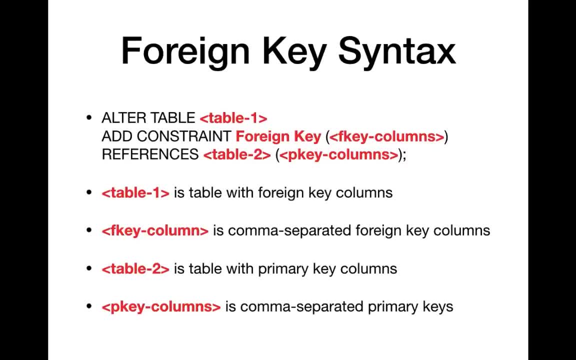 the foreign key columns between those parentheses. and then we reference another table and the course that allows you to divide the column in a restaurant organized in our собственноicação in Google thatisen newspaper and we add thatmark from the text code in order. we recall that generally performed in this: 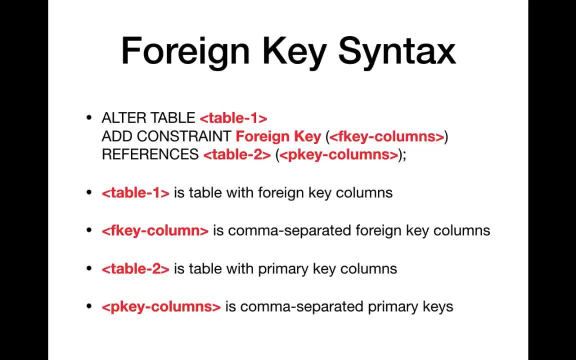 owner, run or helpnorms table. we are also altering the column by adding an element on each of the main Search results, the80 columns and inside the pool menu right now, so that now we can have available command trois times on each side as a free foreign key tag departments are given as functional controls, depending on the database system, sometimes our there is additional restrictions about what type of foreign key constraints. uh, you can define um and the syntax might always vary between different database systems a little bit, but this is the command that should work in the Postgres database system a bit, but this is the command that should work in the postgres data support system. all right, so here we have some. 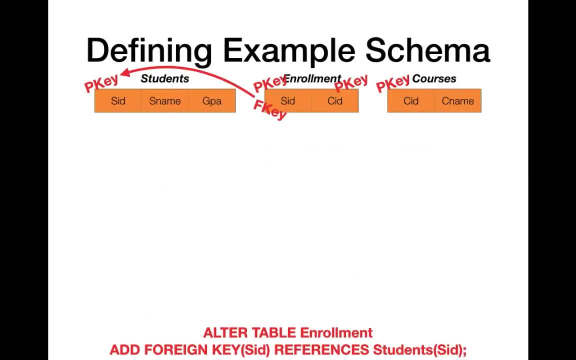 So here we are extending our running example database and we already had that in the chat. People suggested that there should be a link from the enrollment table to the students table and also to the course table. Now here we are taking care of the link to the students table, linking the student ID column in the enrollment table to the primary key student ID column in the students table. 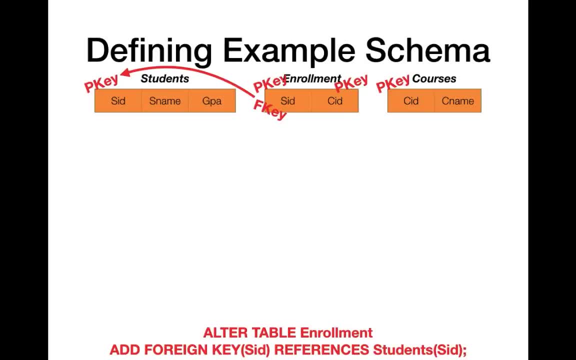 And so if you try to insert an enrollment for a student that hasn't been entered, then, for instance, the database system would give you an error. Same principle for the courses. Here we are adding a link between the course ID column and enrollment to the primary key constraint in the courses table. 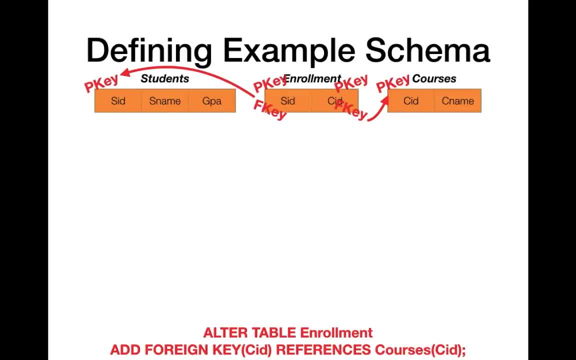 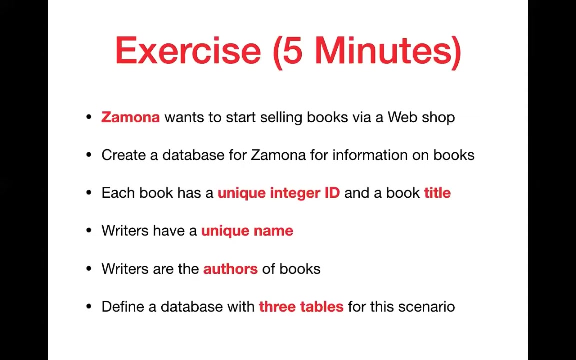 And here we essentially ensure that you're not inserting any enrollments for courses that don't exist. All right, All right, So, and now I'm going to give you a little exercise which links to the example that we have just seen, just to get a hang of it a little bit. while you're working on the exercise, I will also look for questions in the chat. 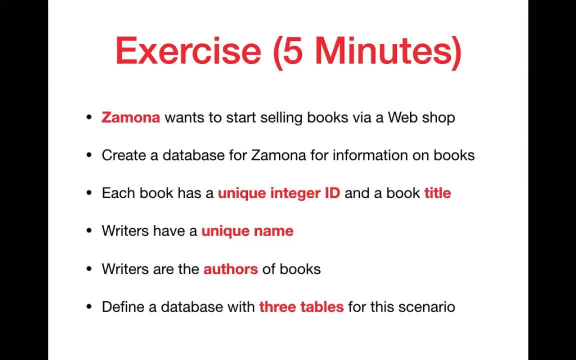 And the exercise is the following: So we are considering a bookseller- let's call it Samona- who wants to start selling books via a web portal. So your goal for the moment is to create a database schema for Samona in order to store information on books, So each of those books has a unique integer ID and a book name. 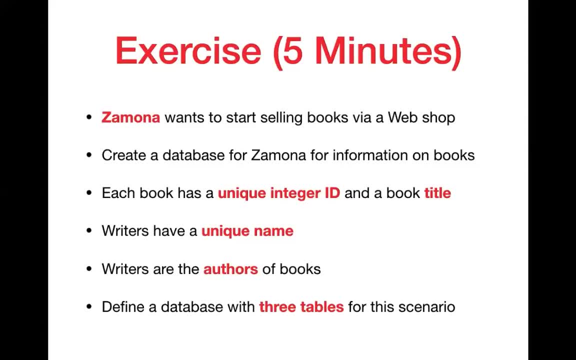 You also have writers on the other side which have unique names, and those writers are linked to books as authors. So your goal is to come up with the commands. to be fine, A database with three tables for this scenario, And You can either do it just by writing down the comment or, if you have already Postgres installed, then you can try it out yourself. 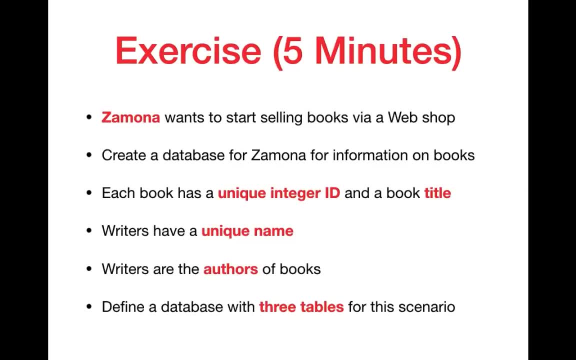 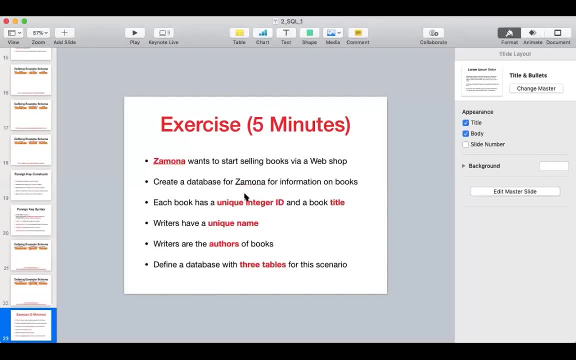 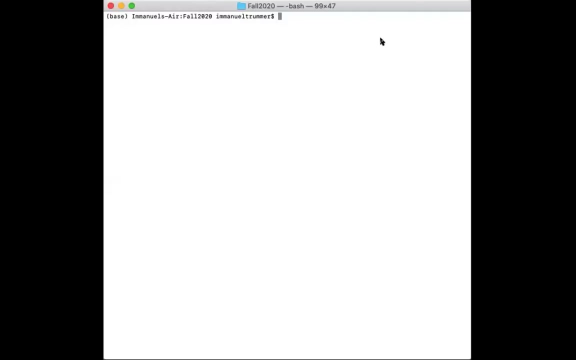 I will very quickly demonstrate to you What that it looks like using Postgres for once, that we quickly share my console here, right? so at this point you should be seeing the console window. if that is not the case, please let me know in the chat. here is some first. 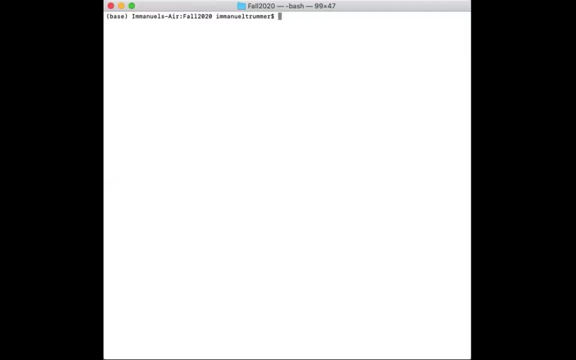 questions. on the example: yes, there can be more than one writer for a single book, and one book can also be written by multiple authors. very good questions. okay, quickly gonna demonstrate how using Postgres looks like. maybe some of you have already experienced with Postgres, so you can skip that and already start. 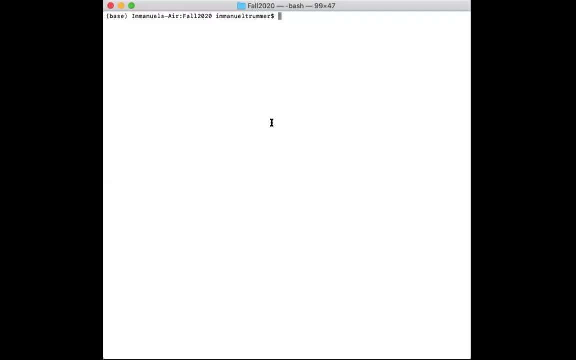 working on the example for the other, as it might be interesting to have a look, and after that I'm gonna give you a few minutes to try out, to try coming up with a solution for the example. all right, okay. so first of all, there's many different ways of accessing Postgres. 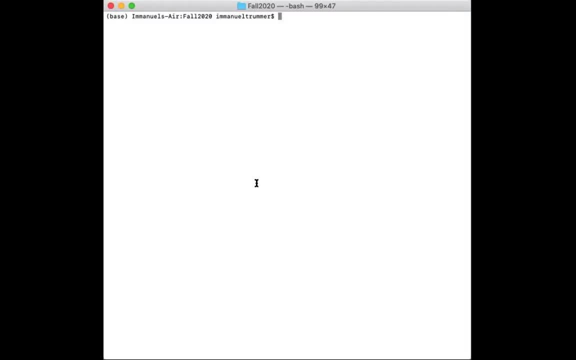 there's different interfaces and also depends a bit on which operation system and which version of Postgres you're using. the following: I'm going to show you how to use Postgres in a few minutes. I'm going to show you how to use Postgres in a few minutes. I'm going to show you how to use Postgres in a few minutes. I'm 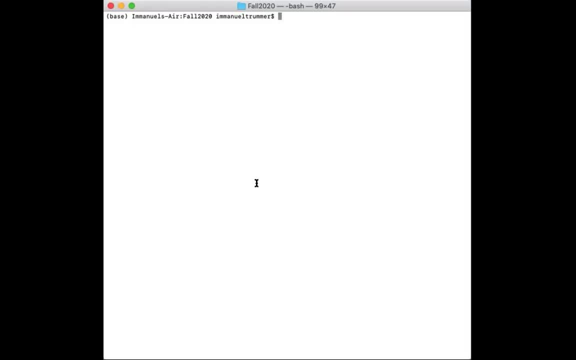 going to use one of the most basic tools to access Postgres, which is the psql tool. now, before I am accessing a database, I first of all have to create it. so in this example that we have seen before, we have been talking about students and courses, so this should be a university database. so I'm entering the 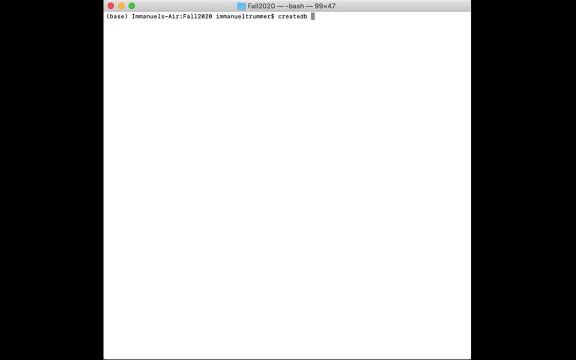 command: create DB. create database and what we call it university, for instance. all right, so now the database has been created, but right now it's not populated yet. so now I'm gonna log into that database with psql. I don't know. we are in the database and can issue a sequel commands. now some of the, so you can. 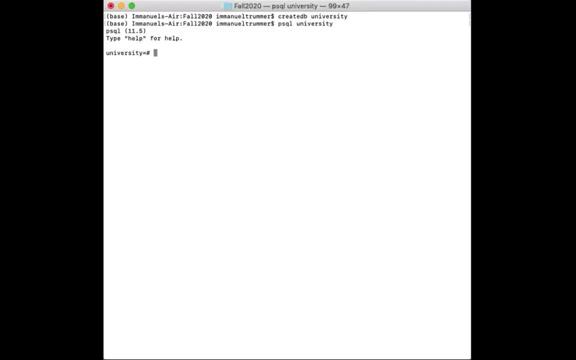 try out the example that we have seen. I'm not gonna do the entire example, just a few command just to see what it looks like. a using Postgres, for instance, we have created a table about students. so, um, what we can do here, we can create a table with the student IRA and the student name, right? and if we 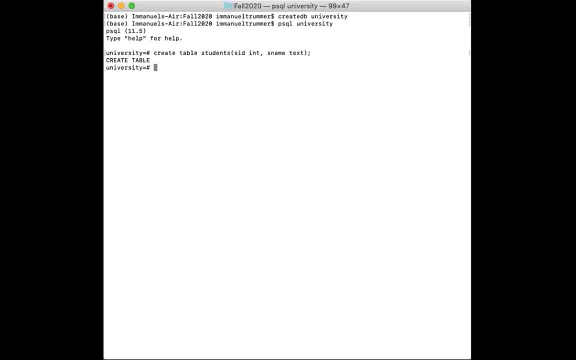 do that, then the database tells us it has successfully created this table and we can also create the table- Roman, for instance- which has the student ID and it also has the course ID. right, all right and okay. and so, depending on your postgres setup, you have to- essentially you have- to make sure that you have installed 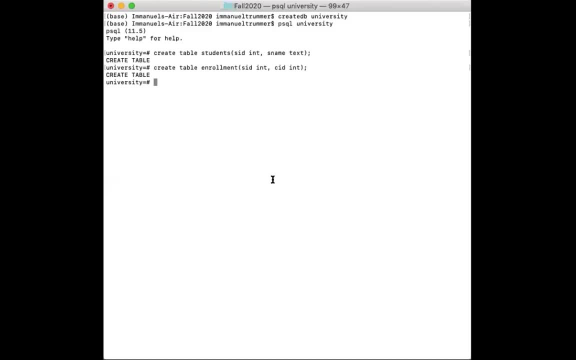 it properly, otherwise you might see some some error messages here. you don't necessarily have to do the example with me here, so I'm just giving you a little glimpse of what using postgres looks like. to make sure they have seen the console at least once, and then you can try setting it up and maybe doing the course example or the. 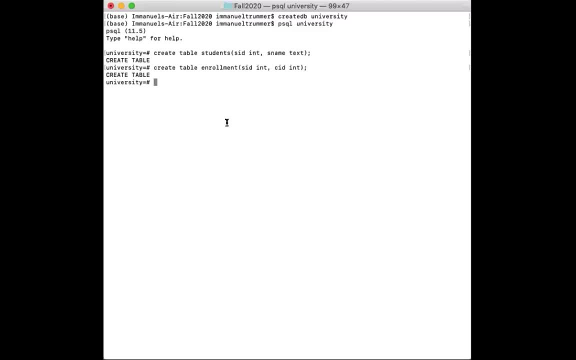 exercise that we have now. you can try to do that with the database. one good question: how do you list? list all the tables? the command for that says backslash D in postgres, and here you see all the tables that we have introduced so far. all right, so I'm gonna go back to that example later. what? 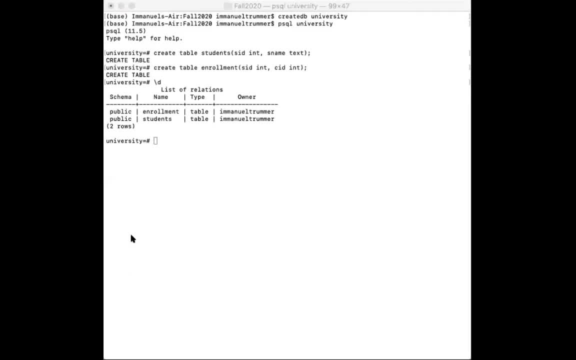 was the last table that we had. it had. yeah, all right, I can just add this one. I can give you an idea here. this one, for example: you want to use the oh, Oh, yeah, and here, for instance, I'm adding one of those constraints, right, all right, and so. 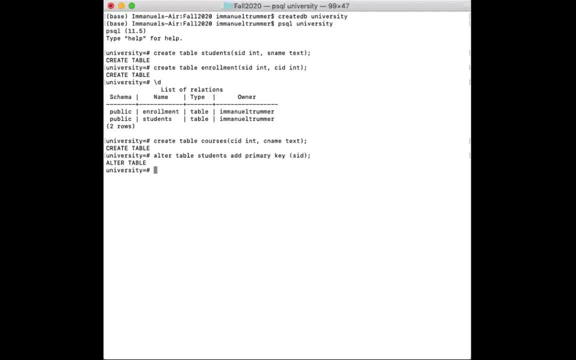 I'm not gonna go through the entire example here, but this is the principle. you issue those secret commands, for instance in a console like this one here in the database system gives you feedback about better executing. the command was successful, all right. so either with the terminal, if you have. 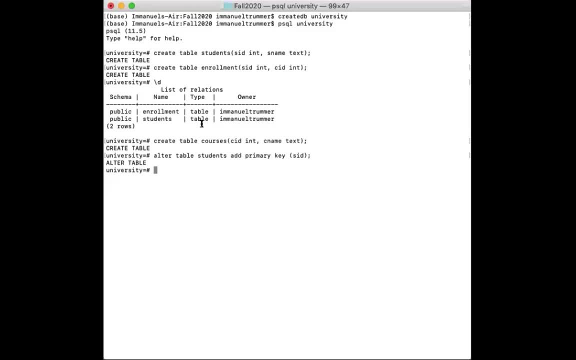 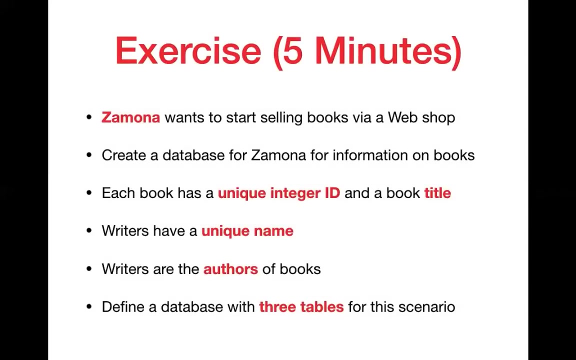 already installed it, or if you just write down the commands. I give you a couple of minutes in order to do this example here. let me quickly share the slides again. yeah, they are you all. right, here you go. you have the slides, so I'm gonna give you just a few more minutes in order to 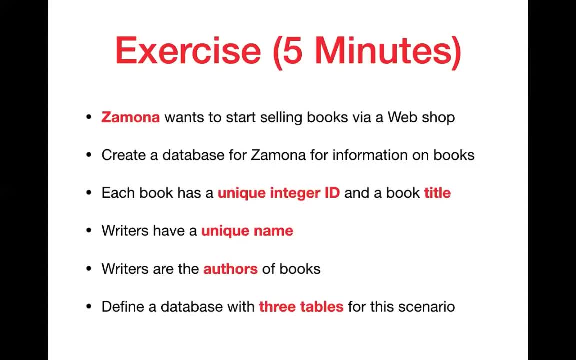 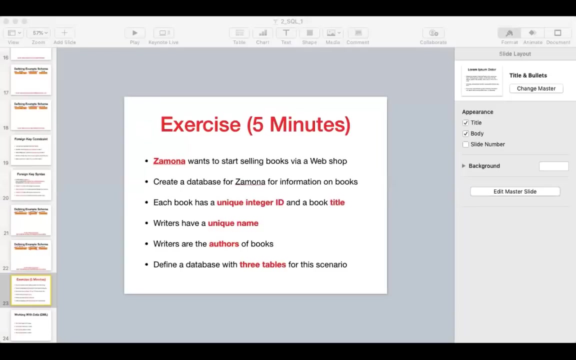 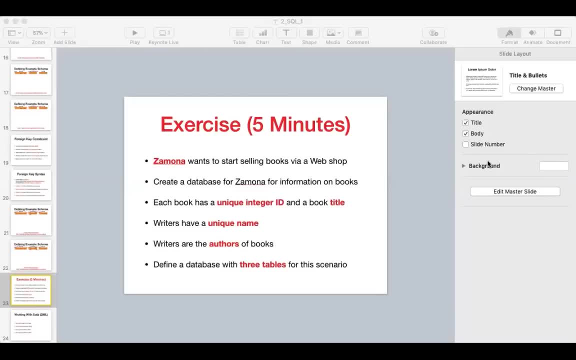 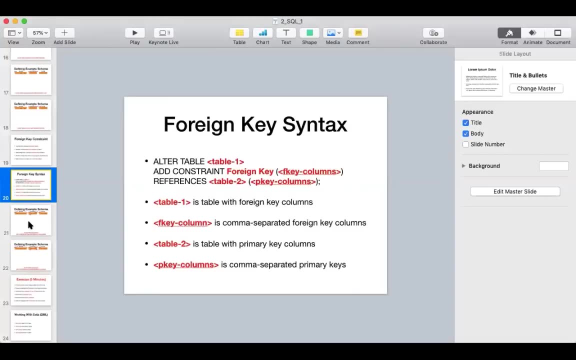 That is a typo. It should just say: add foreign key or add primary key. This is what we use. Okay, Let's look at the examples. Okay, Let's do this exercise. So there is no exam in this course. There was one question about an exam and there is no exam in this course. 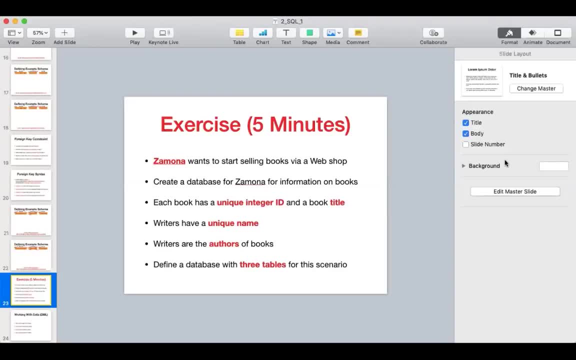 And for the homeworks in general, the syntax should be so, basically, whatever syntax works in Postgres, there's slightly different SQL dialects for different database systems and for the homework submissions, Okay, Okay, So in this case I'm going to use the one that is supported by Postgres. 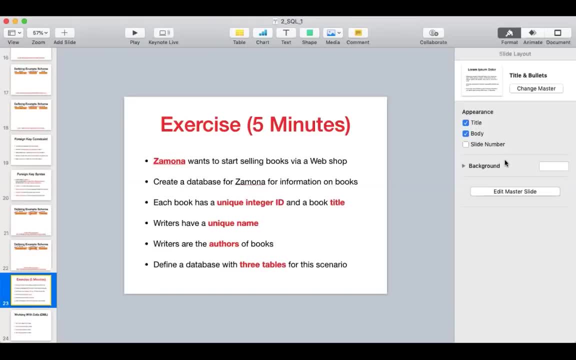 In most cases it doesn't matter. so SQL database systems: they implement the SQL standard quite tightly typically, but every once in a while there is one detail which is a little bit different in different SQL versions supported by different database systems. so in case, 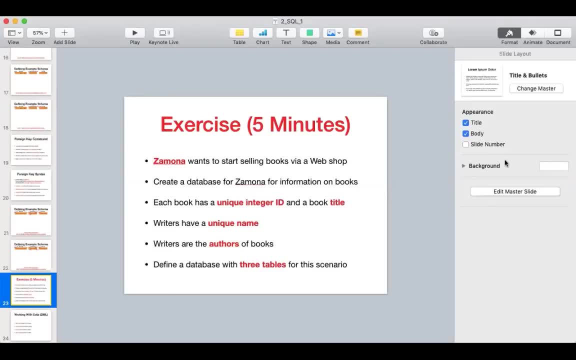 of doubt. So I suggest to go with the Postgres syntax, which is also the syntax that we will see here in the slides. Okay, So we're grading. Okay, Okay, Okay, Okay, Okay, Okay Okay. 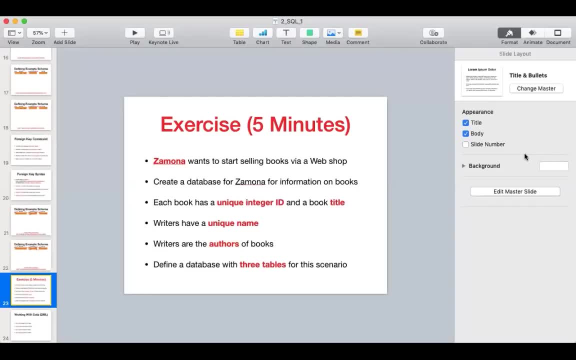 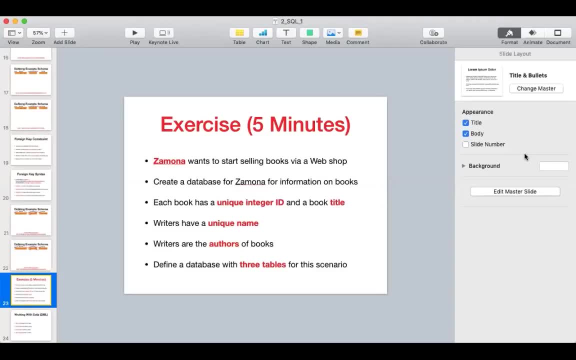 do it temporarily. If you want to go ahead and인 the very next day, we can. so you can use the tool we used to do itами, so this is not same for us. into this code we need only a string priceodi that we're choosing. 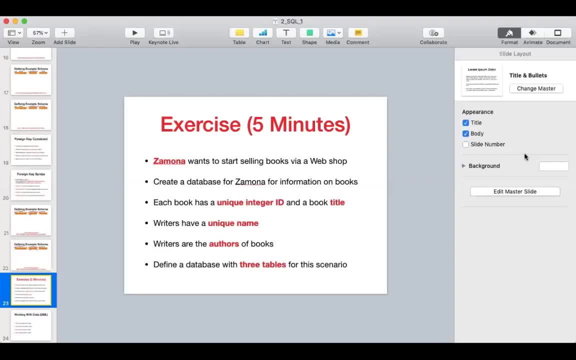 a great one. then we can directly set the primary key and foreign key, whether we can set them directly when creating tables- and yes, you absolutely can do this. you use the primary key keyword in creating the table, for instance. then you can make a column directly the primary. 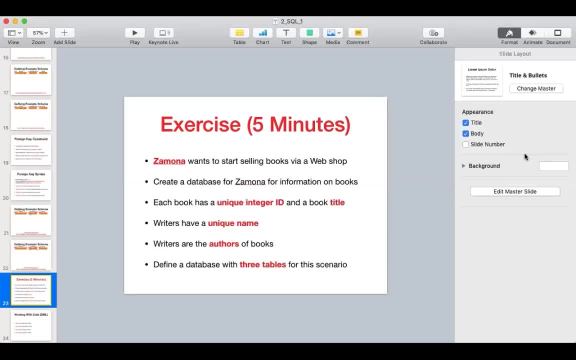 key um. there's different ways of setting those constraints um here we have seen how we can add them um afterwards, but you can also add them directly when creating the corresponding table. very good, all right, i think now you had a little bit of time to look into this, so we're gonna. 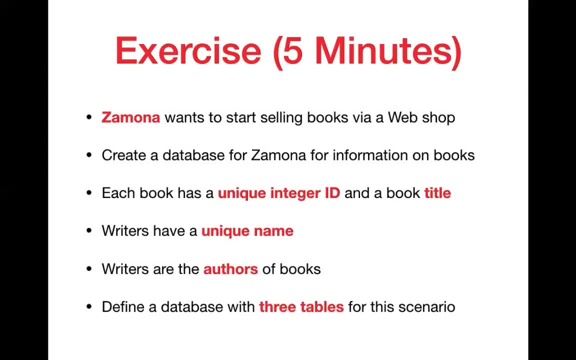 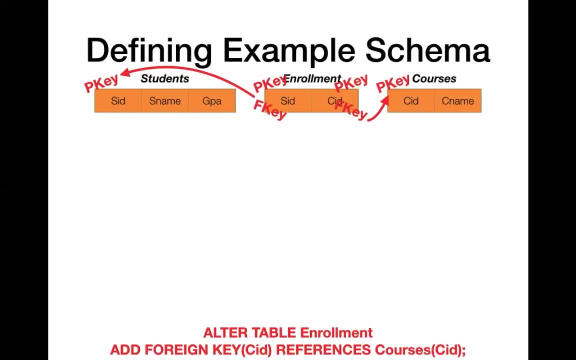 publish the complete solution um on the website. but the high level idea here is that you essentially have again database with three tables. you have one table about the books, you have one table about the writers and then you have one table linking the books to the writers, like the. here you have this. 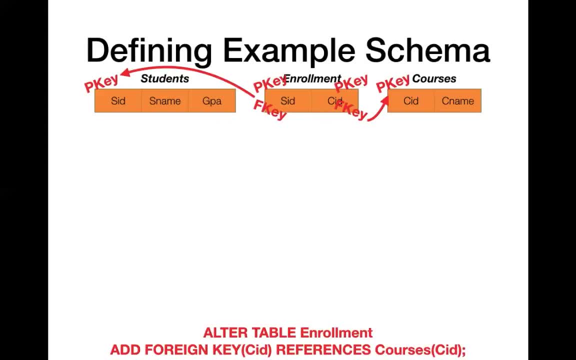 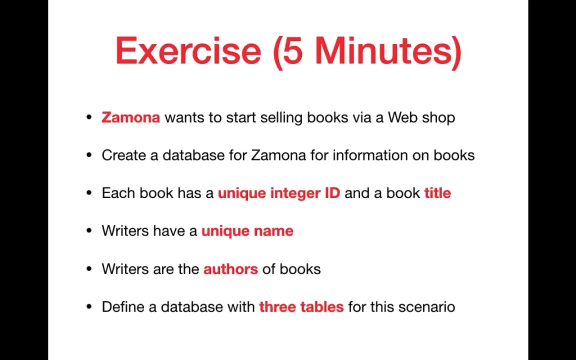 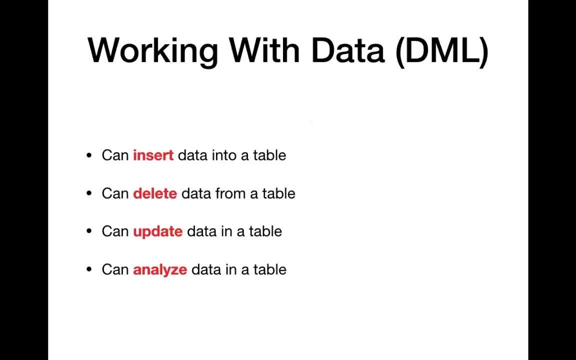 table in the middle which links the students to the courses that they are involved in, and in a similar way, you can link the authors to the books that they have written. so it's the same principle as here, just with a different scenario. all right now, um, beyond just defining the schema of the database, of course you can. 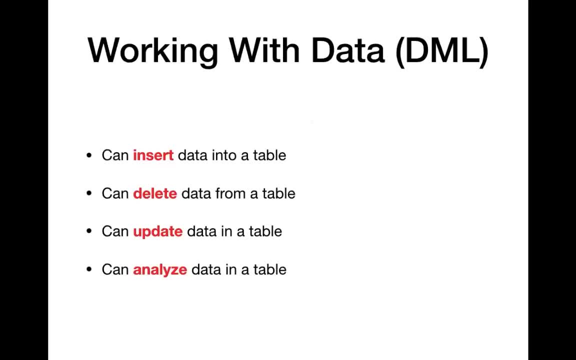 also insert data that complies with the schema. you can delete data, you can update it and you can analyze it in various ways, and in the following we're gonna see it um commands for doing all of those uh things. so now this is the data manipulation language. um. first of all, we want to 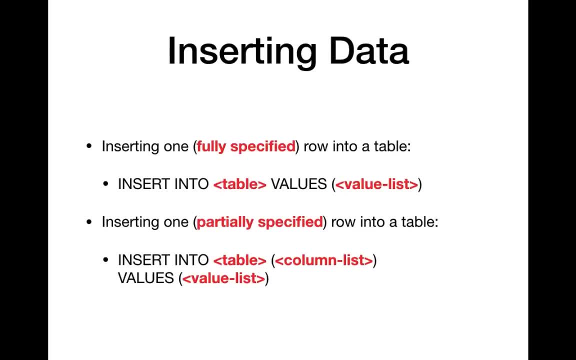 insert data into our database, and here you see, first of all, the command for inserting the one fully specified row into a table in a database. so here we have this: insert into table name values, uh, and here you specify the values for different columns for one single row. 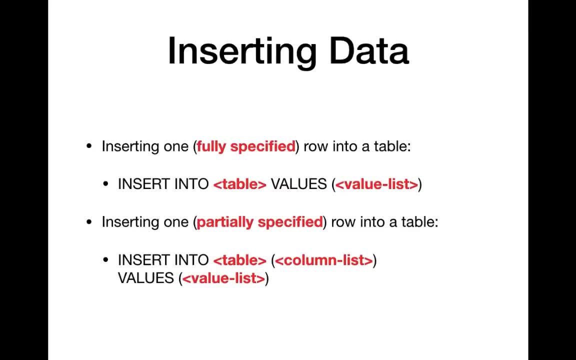 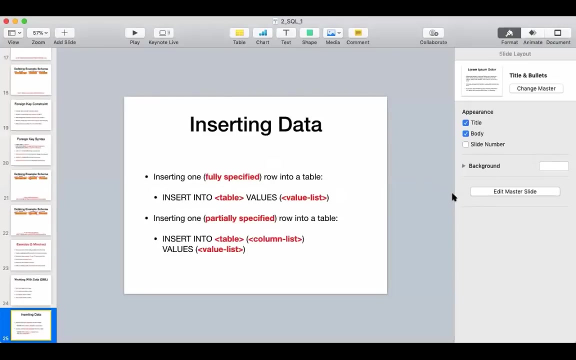 right, um, here i'm saying, uh, fully specified. um. one feature of sql is that it allows you to uh handle cases where some parts of your data are unknown. let me quickly mute everyone. i can do something in the background here, all right? so, um, i will show you how to get into the database. 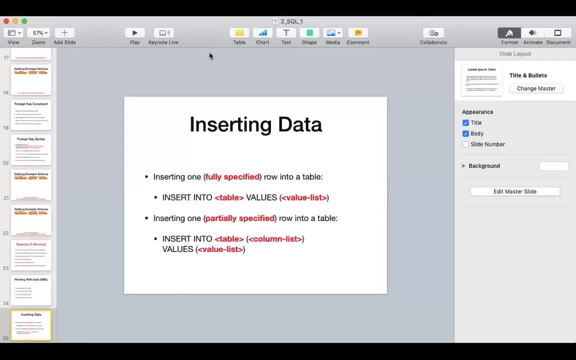 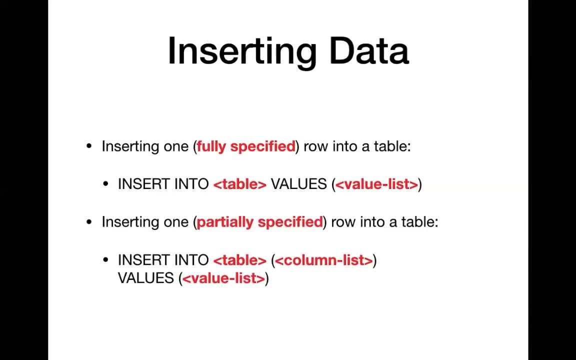 okay, um, good, all right. so here we first of all see a command for inserting a fully specified row, which means that you are, but you do not have to do that. sql has a way of representing fields where you don't actually know the value. currently it is called an sql null value. we will see this more detail later, but here. 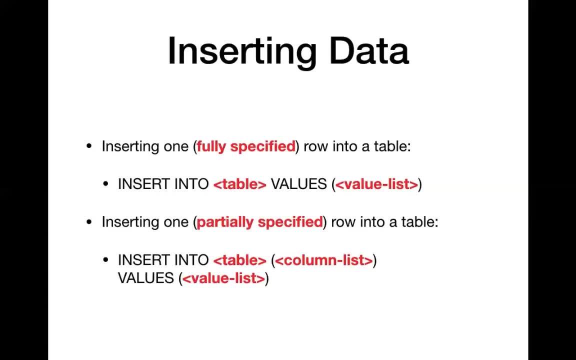 we already connected that a little bit because the second command that you see here, it allows you to specify values only for a subset of the columns, and the remaining columns they will be filled up with null values automatically. so in the second case you have to specify for which columns you actually want to set a value. all right, now what we can. 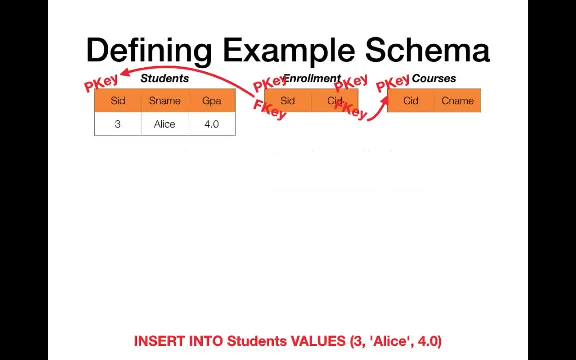 do here? first of all, we want to store information on some students, so it makes sense. we want to insert an entry tree for a student named alice, and here you can see how we do this. we want to insert something into the students table with the values s3 for the student id, alice for the student name and 4.0 for 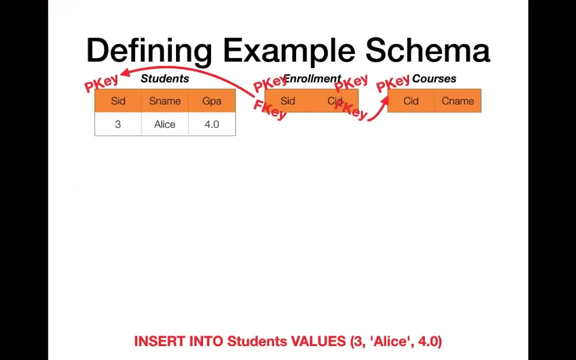 the gpa. all right, and as you see, the corresponding table- the row appears here on the left upper side. all right, now let's also insert a student named bob, but this time we're only specifying values for the student id and the student name. perhaps we currently don't quite know the gpa when entering. 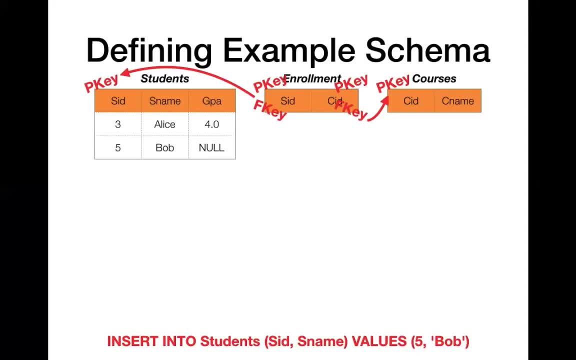 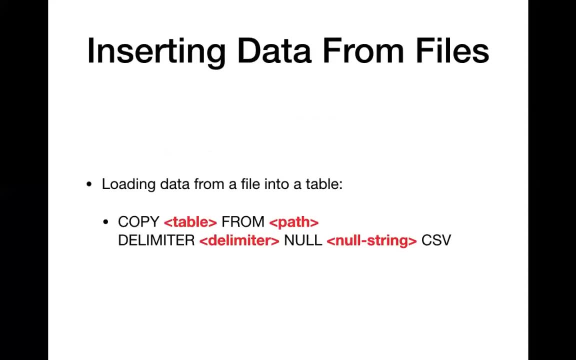 the data and it will be automatically replaced by this null value placeholder. okay, so this is how you can insert data, but in practice, if you're using an sql database system, then, um, if you want to analyze data, you're typically loading it from a file, and postgres also supports the 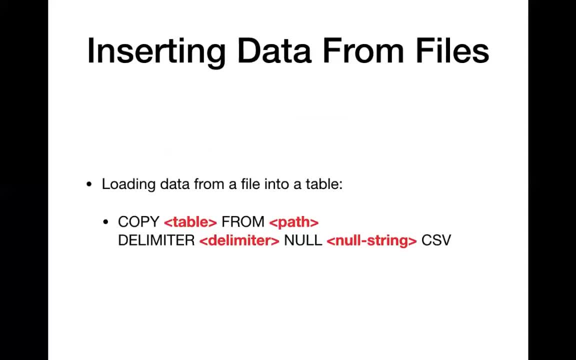 commands for that um, you can load the content of a table from a file by using the command that you see here: copy some table from some file specified as a pass, with specific delimiters and with a specific representation of null values, for instance. so it's many versions of this command, but it tends 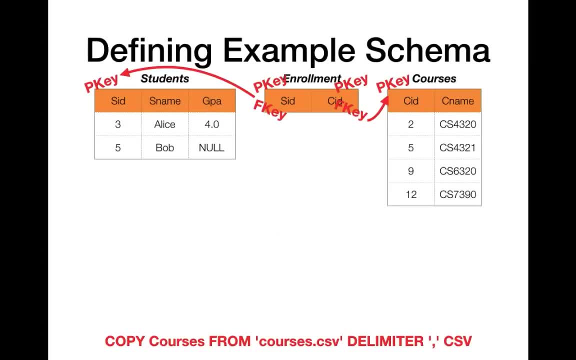 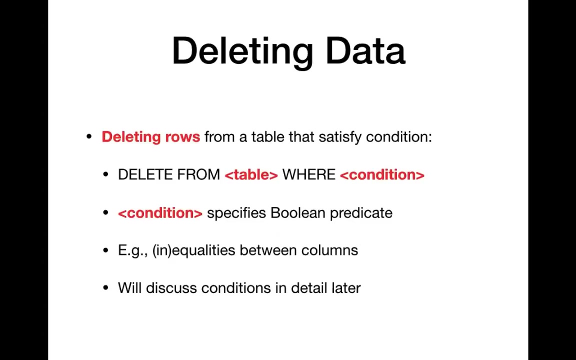 to be very useful in practice. all right, so here, for instance, we might be loading the information, all the courses, from some comma separated value file, which we could do by a command like the one that you see here. okay, we can insert data. of course. we can also delete data. you can delete. 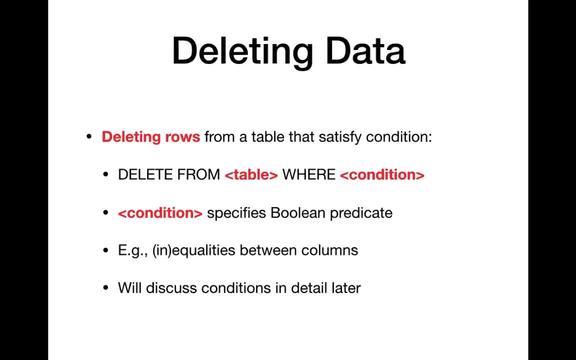 rows from a table which satisfies certain conditions. with the command that you're using you see here: delete from table name where some condition holds and that condition essentially specifies which rows in a table you want to delete. you will see in more detail later which syntax you can use for those conditions. that sql supports- very rich conditions, but for instance you could 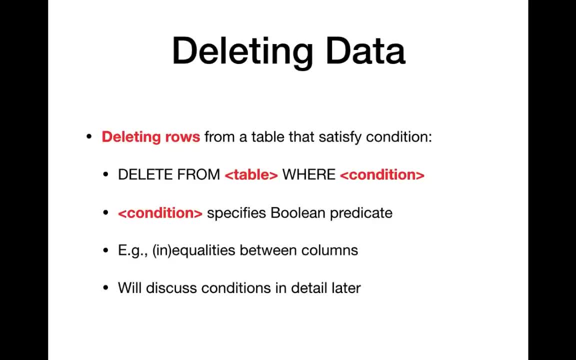 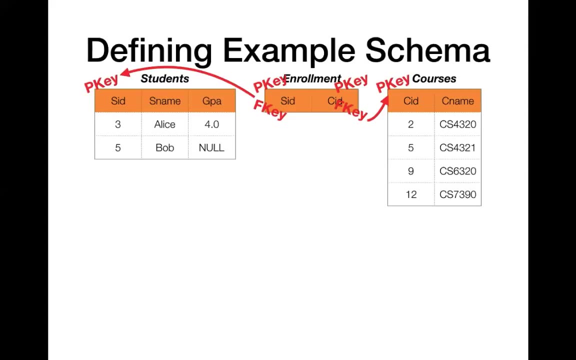 use some inequalities between columns and constants, and we will discuss all the different types of conditions that you can use here in more detail later. for instance, a course database we might want to delete at the 6320 course because that one is not given the semester. so if you here observe the original course table after the command, it will. 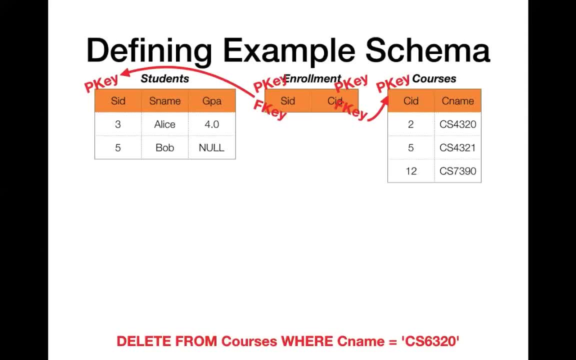 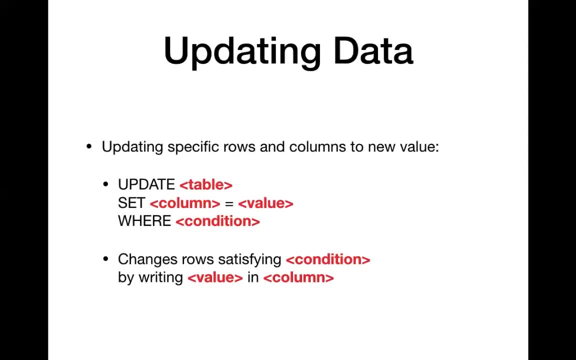 shrink by one row because we delete the one where the condition cname equals. here 6320 is satisfied. beyond inserting and deleting data, you can also update it. you can update the specific rows and like the values in specific columns or specific rows using the command that you see here. 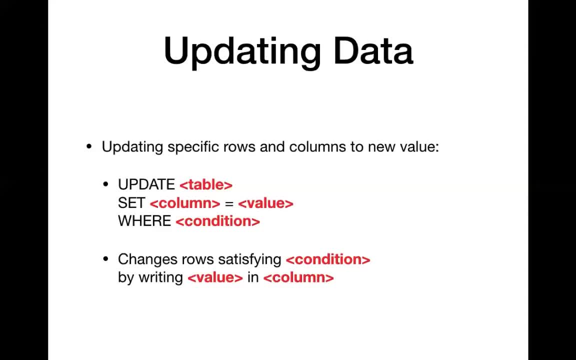 we are simply writing, we are updating a table, we are setting a specific columns to specific values for all the rows where this condition here is satisfied. so this command is present, valid to all the values, and so that means we get nothing in this part. we just need tovalue the value of the table. this is the value, but effectively every column functions in c, those values. in a table we get 0 and no interval. so that means we can only get something р, as usual on any table. let that be wrong. it's Kamera. that means we get the domain name. that is. 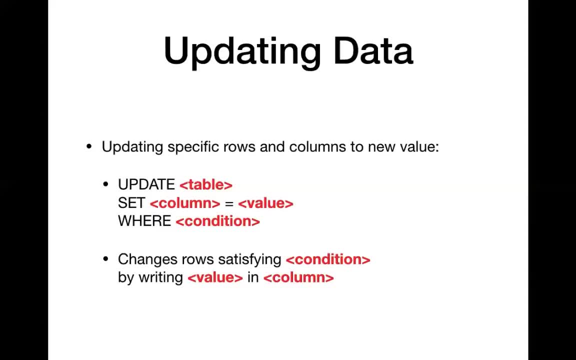 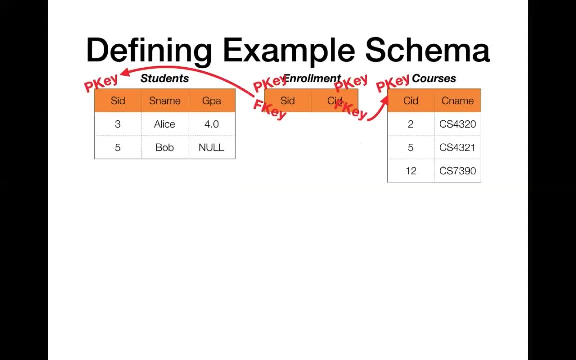 and changes those rows satisfying the condition by writing the given value into the given column. Here, for instance, maybe we want to change the course ID to number seven, where the name is 4320.. And here you can see the table changing after we run the corresponding command here. 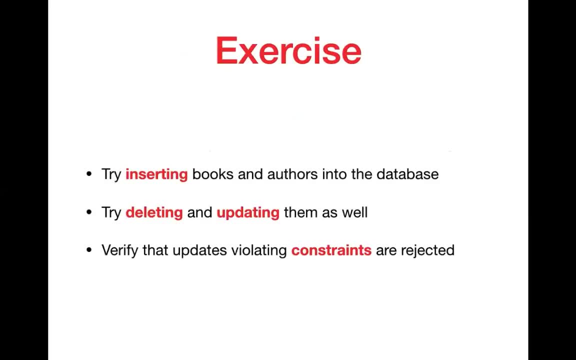 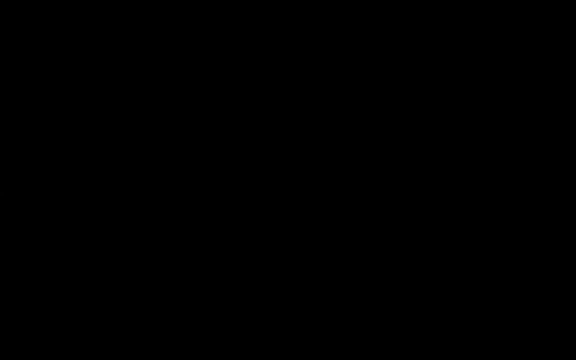 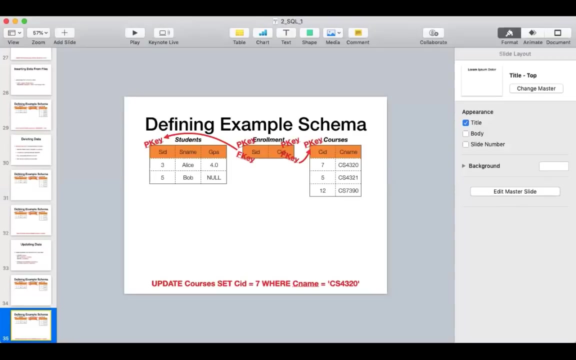 All right now, this is an exercise that you can do at home, or at home anyway, but an exercise we can do after the lecture. And for the moment, I can show you again how those examples work in Postgres, just to make sure that you have seen that once. 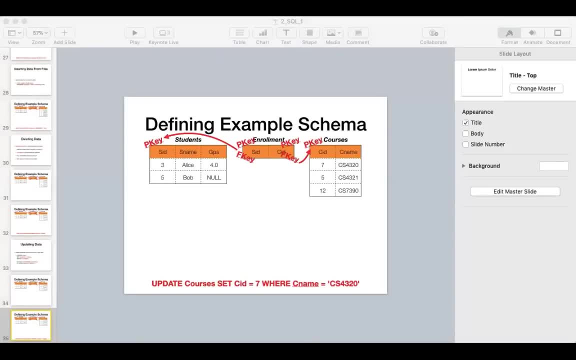 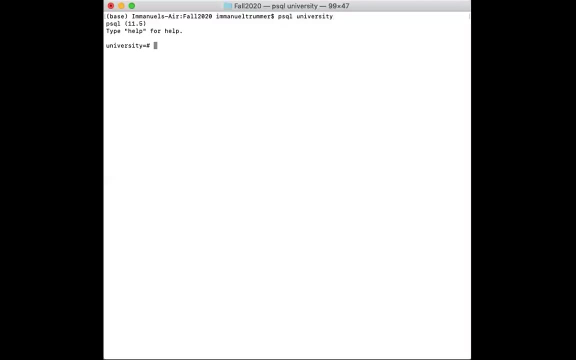 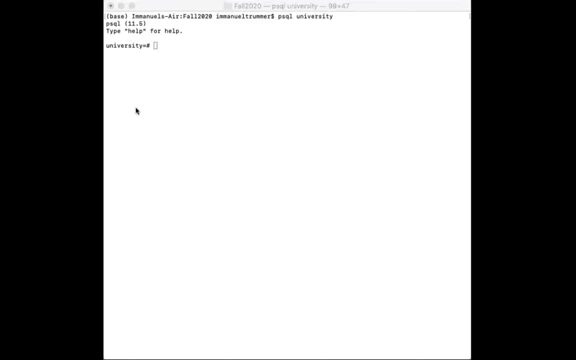 All right, and I'm about to be inside here. For instance: okay, we inserted student name Elizabeth. Okay, and I think they actually didn't define the GPA column. Okay, and I think they actually didn't define the GPA column. 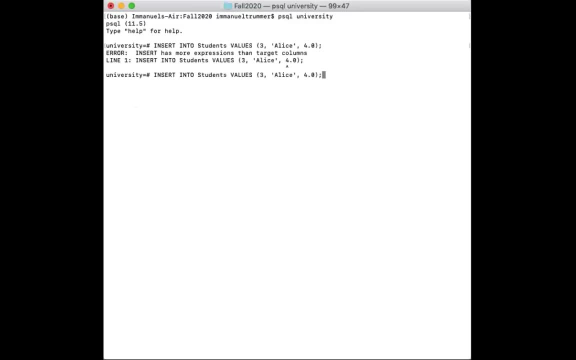 Okay, and I think they actually didn't define the GPA column When I made the example before. Let me quickly verify that. So here, with the backslash D command, you can show all the tables. And this is my example And this is the German example. 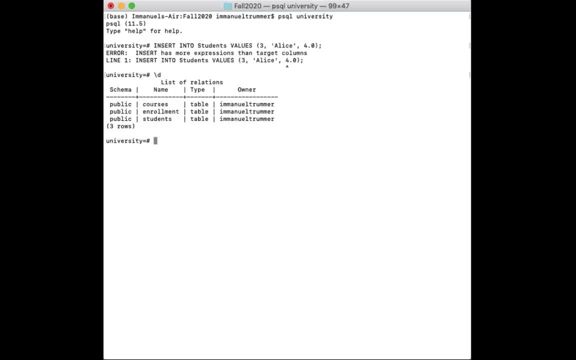 This is my example. So this is the German version of the student tables that are currently defined. So at least I defined the students table. but let's see which columns I have in that table specifically And with the syntax here- a backstrash d and the name of a table, you can actually find the 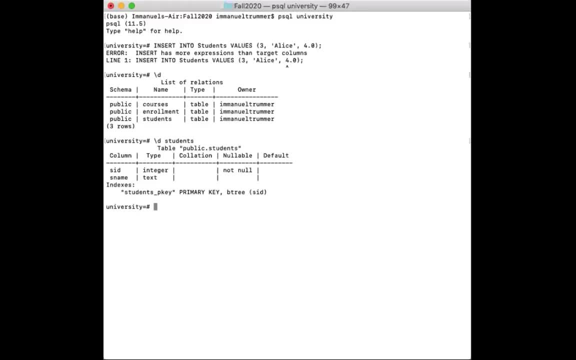 different columns of the table. And here, indeed, I made a mistake because I didn't- or I mean it is inconsistent with the example slightly- because I didn't- introduce the GPA column. So what I can do in those cases is that I delete the. 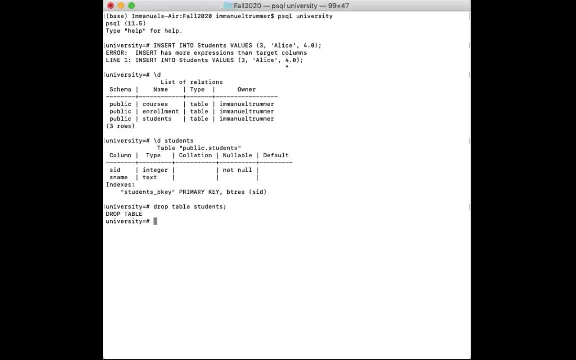 students table again with this command. So now I only have two tables left, And now I'm creating the students table again. What did we have? We have the student ID, we have the student name and we have the old table. Now, when I'm doing this, newề table should be or this group, but now hice th Beau samples And i had the student name and you have the. 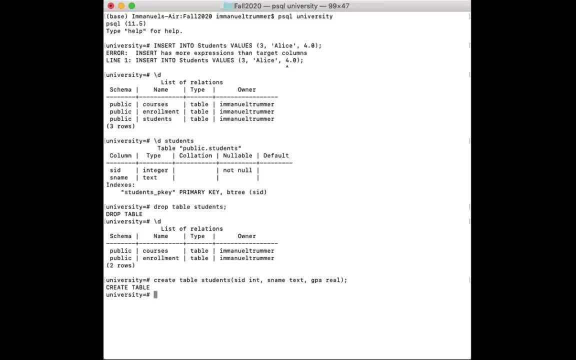 gpa and it's different versions that i can be using, all right, um, okay, and i'm quickly gonna finish this. i see there's a couple of questions popping up in the chat. i'm gonna take care of them in a minute and, uh, what i just wanted to show you here is how we insert one more row for the. 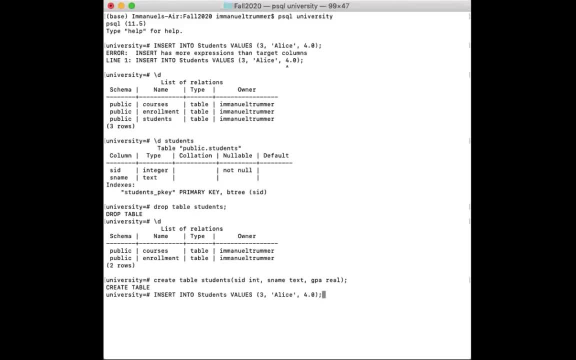 students some first row here. um, i'm inserting the student others and the database system now gives me a feedback. um, the um, the first number that you see here. that one will be typically, uh, zero. that is only used if um a postgres assigns a so-called oids. but this is not going to be part of this. 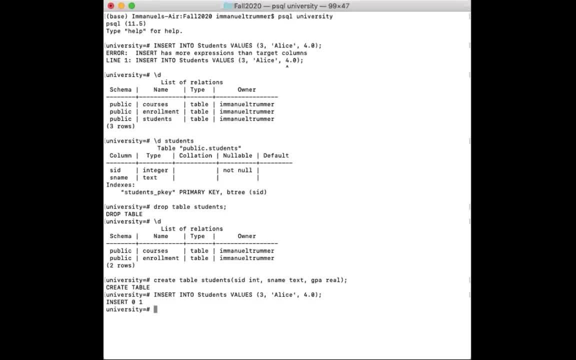 lecture. the second number is more interesting. it tells us that one row has been inserted into the table, and here somebody is already proposing the correct command. very good, somebody is proposing a command to say to essentially show the content of that table, which we will see more detail later. but i can. 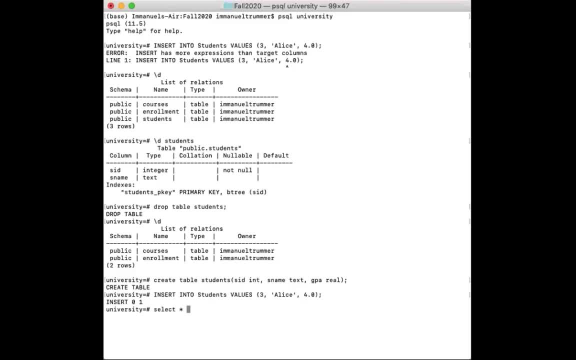 already give you the command here we are doing: select the star, which means we are. we want to know something about all the columns from the students table, right? and now it shows me this one single entry in the students table. all right, so yeah, i'm just. i want to give you a little bit of a feeling for what it is like to use one of those. uh. 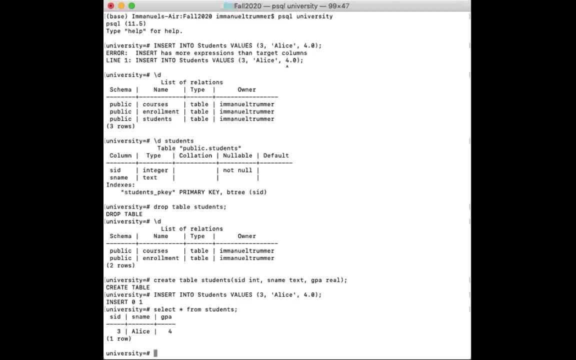 database management systems. i should also say that this interface is, of course, very simplistic. depending on which version, which tool and which operating system you're using. you might have some nicer graphical interface, um, but the sql commands, they uh, remain the same, and i mean, in many cases you would actually 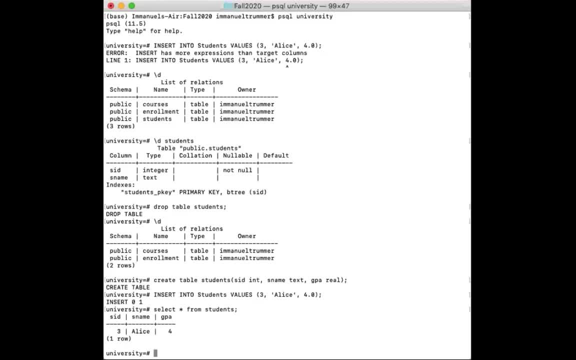 in practice, you might not be using sql directly, except if you are developing an application, like in many cases, the end user is actually shielded from uh issuing sql commands. um, you use some kind of interface which, in the background, it generates sql queries that are sent to some data. 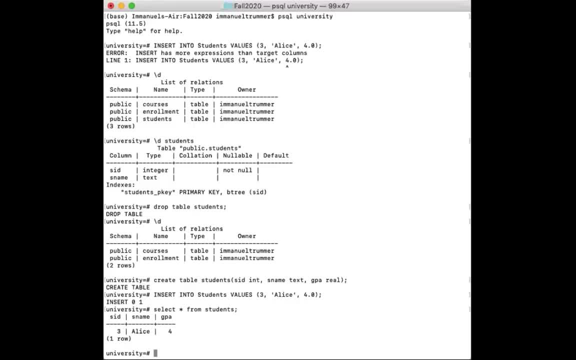 base, but of course, if you want to develop this interface, then you need to know about sql. okay, a couple of questions, so all right. so some questions already refer to advanced concepts, some of which we will not necessarily cover in this course, even though it's very interesting questions. 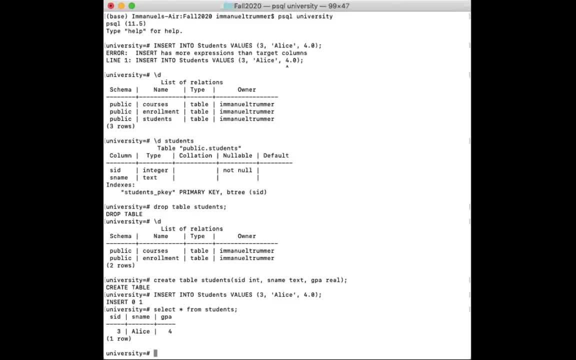 um, okay, here one question about the previous book exercise, so i quickly sketched out the solution, which uses three tables, in analogy to the example that we did with students here. the question is whether we couldn't have done it with two tables, like simply one table about books and one table about authors. 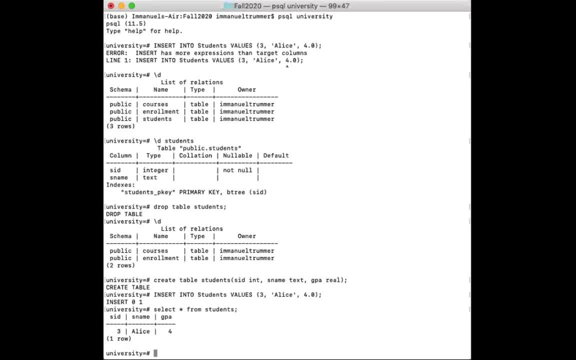 ideas in the author's table and have an area of also ideas in the books table. um so, um, in principle, um, so, in principle, you can use arrays, but let's say the proper way. uh, the most secret way of doing things is that you uh, yeah, not too bad, i should formulate it that way, but uh, 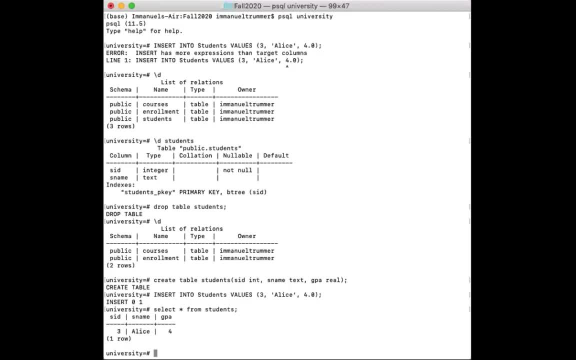 for this course. um, we are only working with uh scenarios where we have a single values, scalar values, single integers, strings and so on in one field of your tables. but, depending on which database management system you're using, there might be some advanced features that allow you to do things differently. 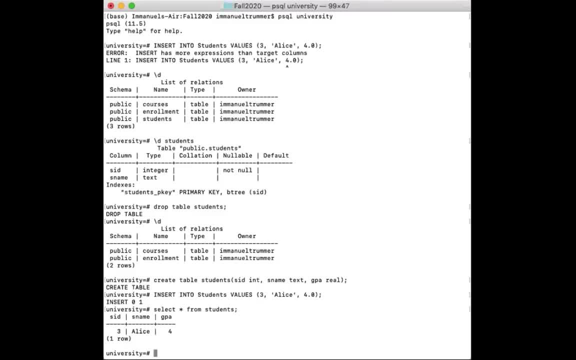 sorry messages. okay, one quick question about the first number in the insert statement. so that number is not um, that number is not relevant for this. uh, for this course it basically um. if postgres would assign something called an object id, then this in during the insert command, then this object id would replace the zero for this. 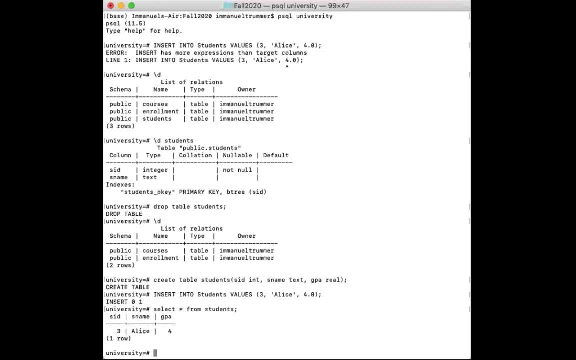 first of the two numbers, but since this didn't happen in this case, we have the zero number and um for the purpose of um, this course, um, we will assume that one column and one row only has one single value, like one integer or one string, and we have to say, uh, but maybe one of these two values is also not relevant. 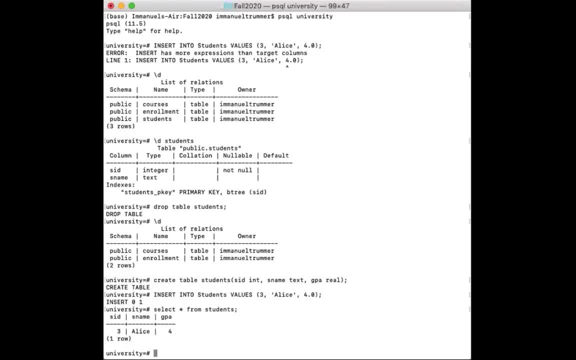 it must be one two, three or one two or one four. so we have to say that the two values are same, but because of this particular- uh, this is a correct distribution. so we're only gonna say one column and one row, and that means you have one value. 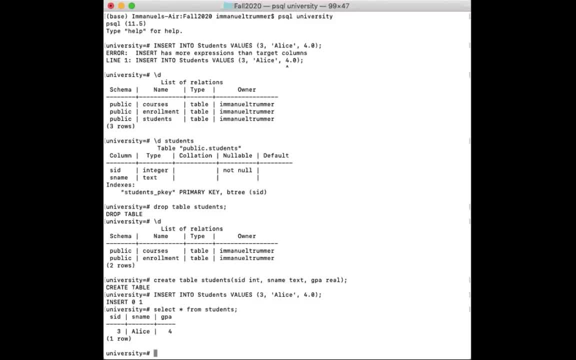 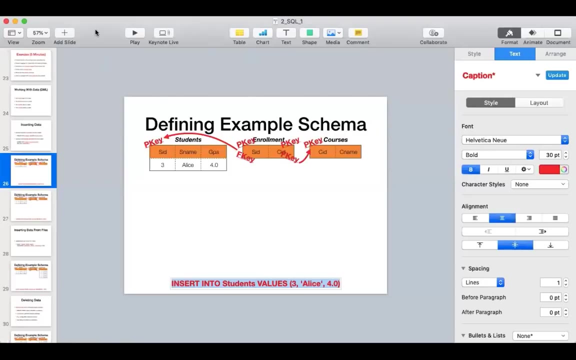 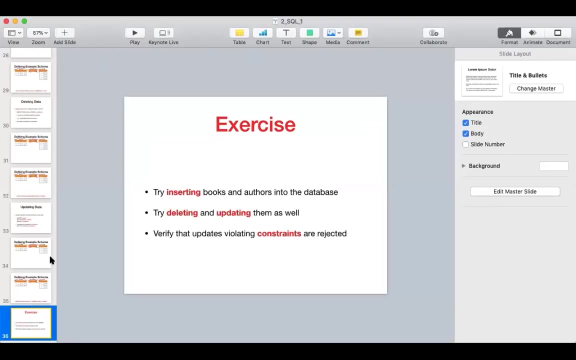 okay, okay, so there we go, so, so all right. good, so we are at the end of our time frame. um, i recommend you to have another look at the examples that we have seen. um, we had one in class exercise and, until the next lecture, you might want to play a little bit with this example database and think about how you would insert or 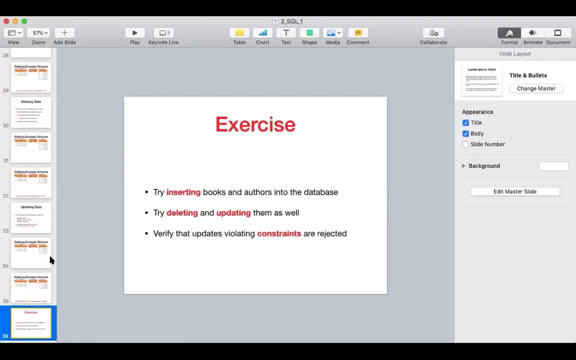 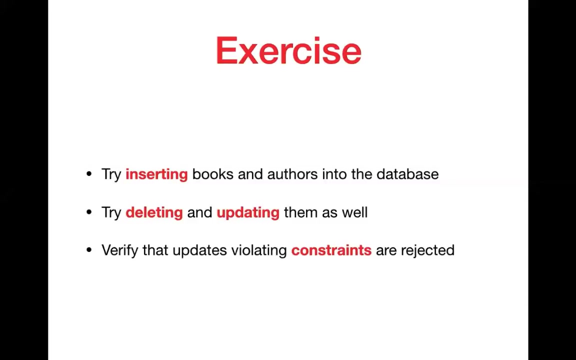 update uh specific books and authors in this database and perhaps make one example where you insert data which doesn't comply with certain constraints and so the database system might reject your updates. in the next lecture on monday, we will continue seeing some more sql features. we are going to essentially discuss about the interface to sql first and then afterwards we 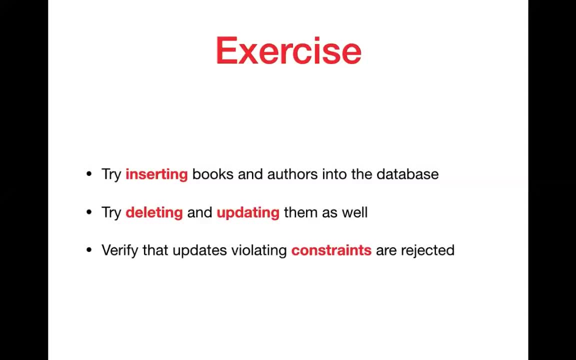 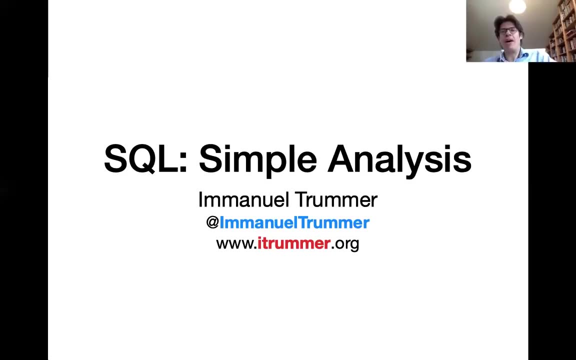 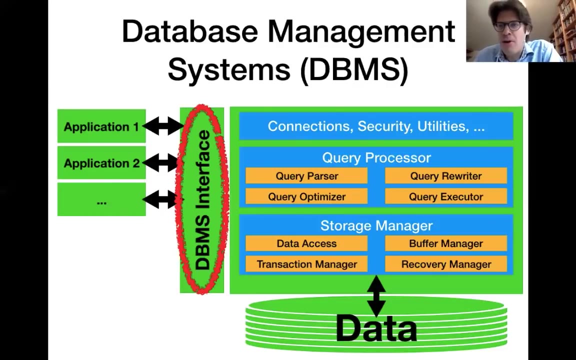 will start discussing about how the database management system actually internally processes your sql commands. all right, so, um, the last time we have been talking about the interface to the database system and um, today we are going to continue talking about that. you're learning a language called sql, the. 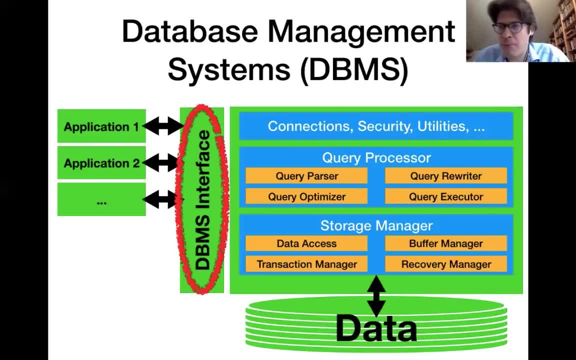 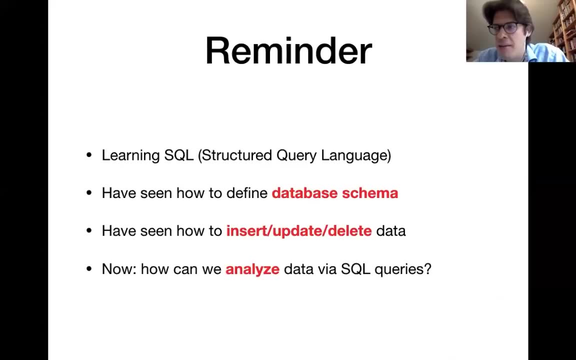 structured carry language um. the relevant book chapters are still the ones that i had in my last slides from the ramakrishna nagarka book, the sections three and five. now, the last time, we have seen how you can define the structure of a database in sql, meaning you can define what are. 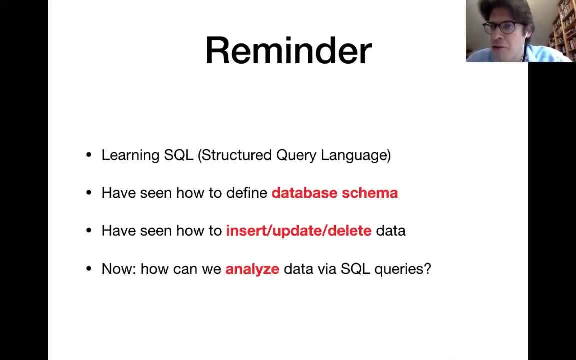 the tables and what are the columns, those tables, and you can define constraints, like the primary and foreign key constraints that we have seen last time, and we have also seen how we can insert and delete and update uh content that you have in those tables. now, of course, ultimately, once you put data into a database, then at some 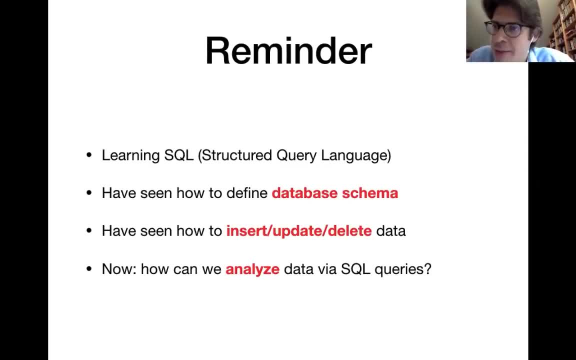 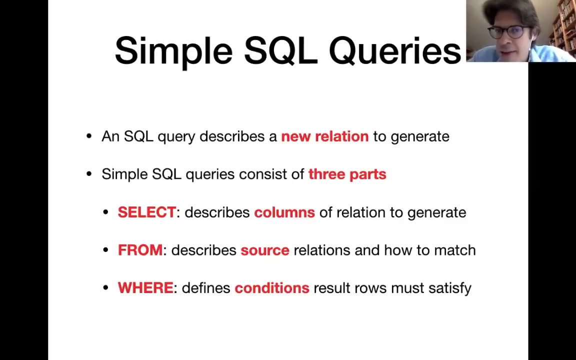 point. you want to actually retrieve it or analyze it. in some days, and today, we will start discussing about sql queries, which analyze the content of your database. now, generally, such an sql query describes a new relation or a new table to generate, and this new table is generated from the content that you have in your database. so this new 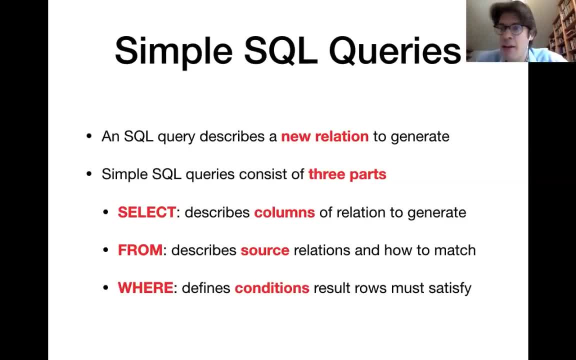 table that can consist of one single value can also have multiple rows and multiple columns, And in the SQL query you define what that table should look like and what content you want inside. So very important. we quickly mention that in one of the previous lectures. SQL is. 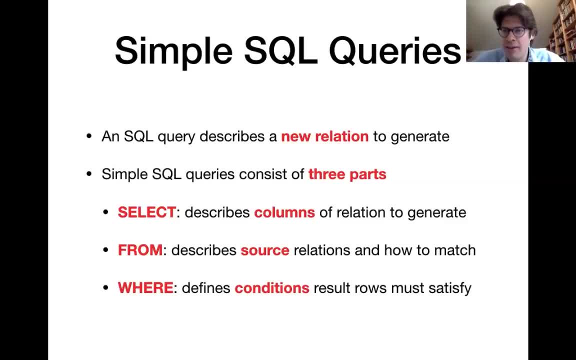 a declarative language, so you do not instruct the database management system, which steps to execute in order to analyze your data. You just describe a desired result and you leave it to the database management system to figure out what is the best way of generating that result. 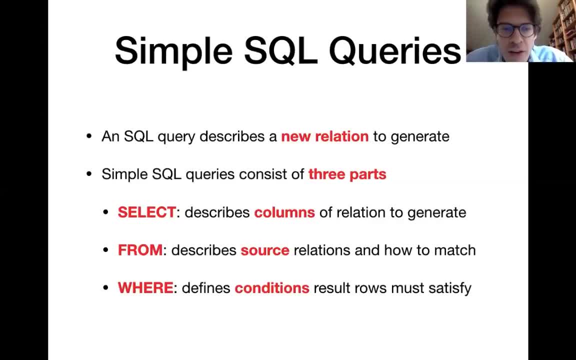 Now we're going to start with a simple class of SQL queries which consists of three parts which describe the desired result relation. Now, in the from part of the query, you are specifying the tables from which you want to generate something. So this is essentially the data sources for your analysis. 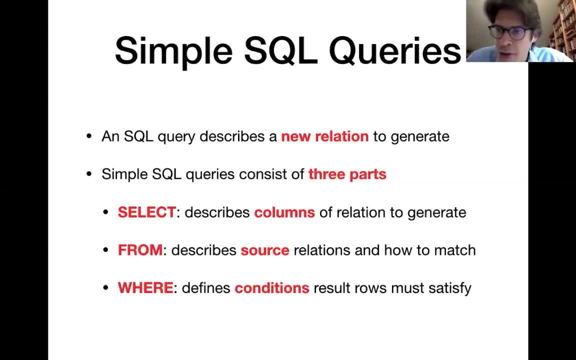 Then in the where condition, you specify certain predicate, certain conditions that the rows in your result relation must satisfy, And in the select part of the query you specify the columns of the result relation that you want to see. So we are discarding the other columns. 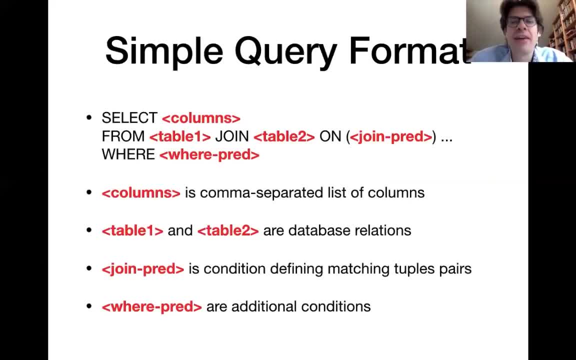 All right, the syntax for the simple class of queries is as you see here: In the from clause you specify the data sources, In the where clause you specify conditions for row filtering, and in the select clause you specify the columns that you're interested in. Now, most of that. 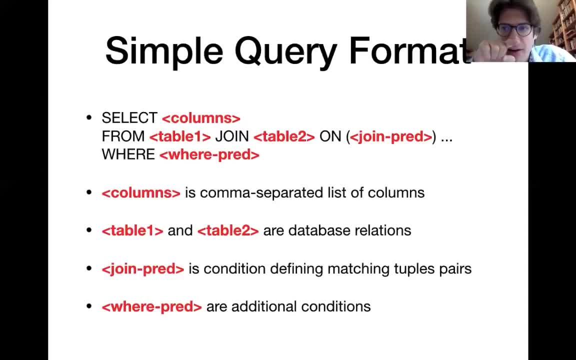 is pretty intuitive. Perhaps the from clause that one looks a little bit more complicated. So let me say a few words on that. So here in the from clause we are essentially combining two data sources, two tables, and we are using the join keyword to do that. So the semantics of what you see. 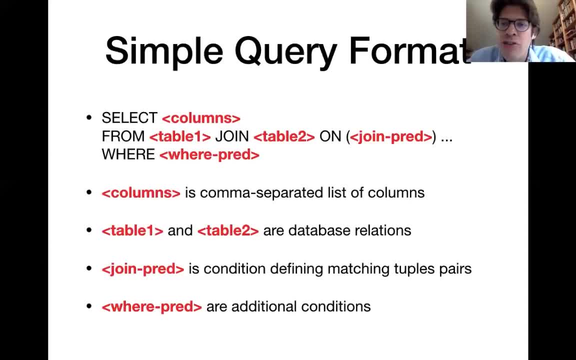 here is that I essentially retrieve a path of rows containing one row from table one and one row from table two, And I only want to retrieve those paths which match, which satisfy a certain condition together, And that condition is specified as the join predicate. So we are only 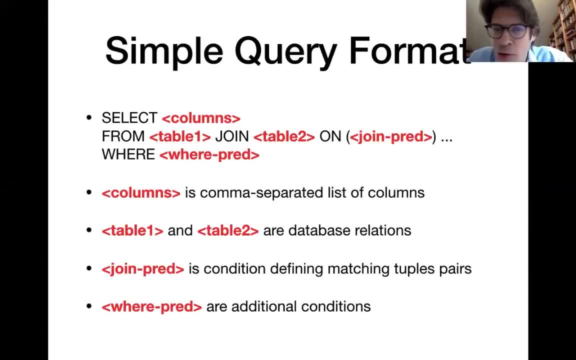 retrieving those tuple paths, those row paths which satisfy together the join condition. Also, you see those little dots on the right hand side of the from clause. This indicates that you can add more tables. You can join with a third table on some join condition and with a fourth table on some join condition. and 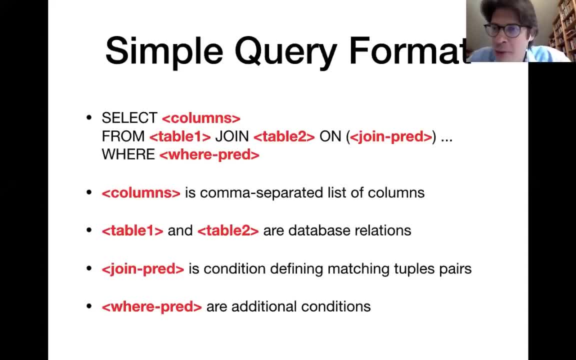 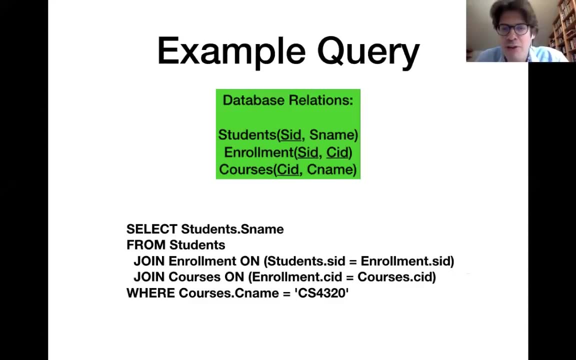 so on. So you essentially you can choose how many data sources you want to combine. Of course, if you are dealing with large data sources, then the more data sources you combine, the longer processing could take. Let's make things more concrete by an example query. Now. this example query refers to the database that you see on 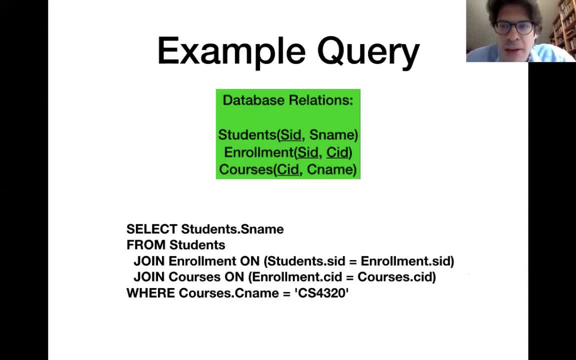 the top marked in green. It is pretty much the database that we have seen last time. It's a database containing information on students and the courses they're taking. There's one table, one relation, for the students with a student id and a student name. Then there is a table storing the 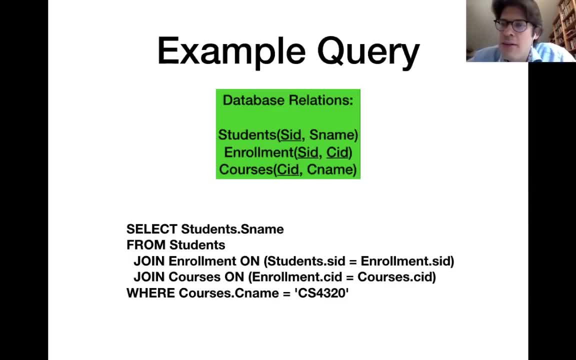 courses with the course id and the course name. And then there's this enrollment table which connects the students table to the courses table And essentially stores pairs of a student id and the course id with the semantics that the corresponding student is enrolled in the corresponding course. On the lower half of the slide you see a 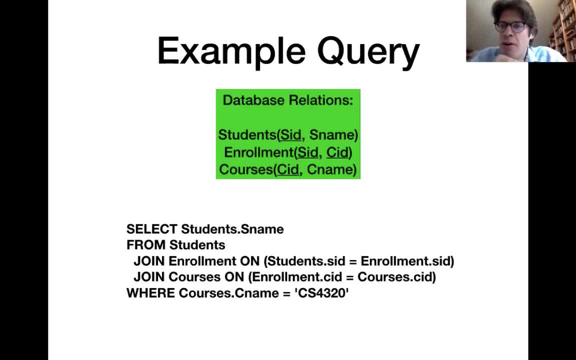 corresponding query. And perhaps one last thing I should point out about the database, and you might notice that I have underlined some of those columns in those relations And that typically means that the corresponding columns are primary key. So this is what it means in this case. 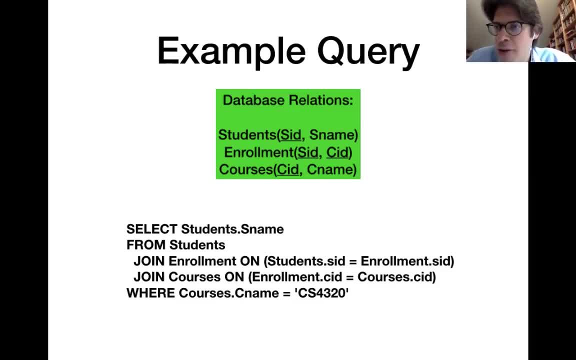 In some other books on databases you might find slightly different notations, but this is a typical notation in order to indicate which are the primary key columns. All right, now you see this a query- on the lower part of the slide and perhaps on the first side. we're not being used to those. 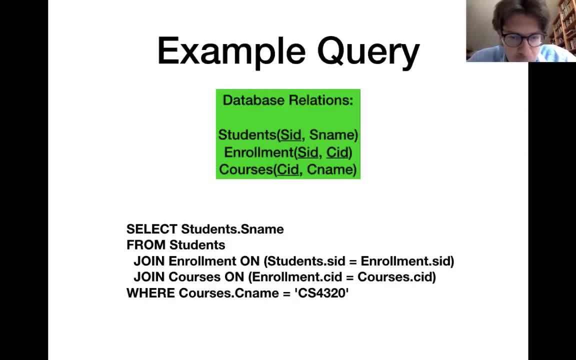 queries and sometimes look a little bit complex. So if you want to understand what one of those SQL queries is doing, it's typically good to essentially decompose it and look at the different parts. So if I try to understand what a SQL query is doing, 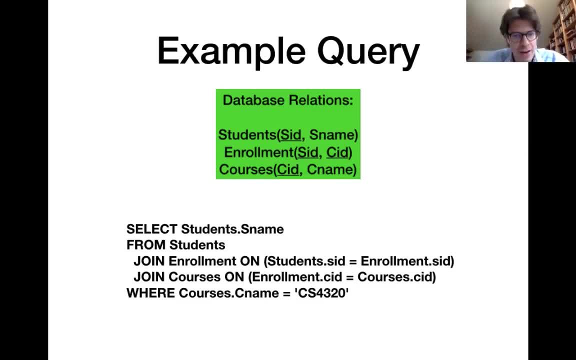 I typically start by looking at the from clause. So let's do that. And if you look at this first part of the from clause, then what we're doing here is you're essentially pairing up students with their enrollment, So we are selecting a path of one row from the students representing one student. 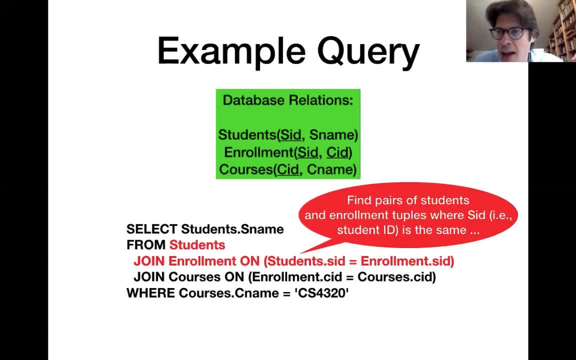 and we want to retrieve a matching path in the enrollment relation, which is essentially one tuple, with a student id and a course id, where the student id matches the student id that I have selected in my students table. So this essentially combines each student with the related enrollment information. The second part of this from clause over: 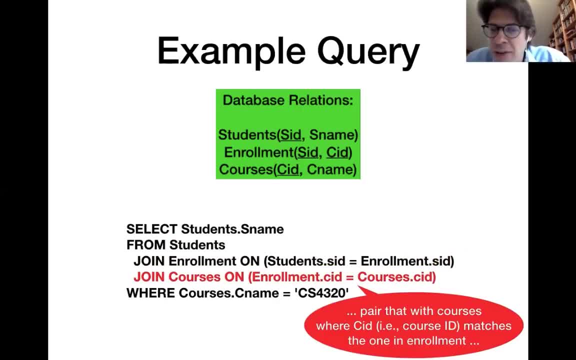 here combines that with the information in the courses table. So, after having matched the students with the enrollments, the enrollment relation only gives me the course id, but I might also need the course id. So here I'm therefore matching the tuple paths from the student and the 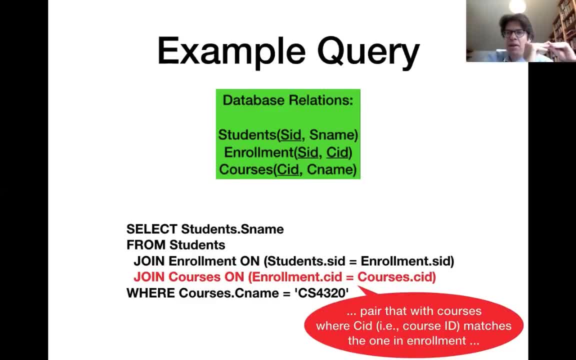 enrollment table that match on the student id and pairing that with a third tuple from the courses relation which matches on the course id. So the result of this entire from clause those are triples of tuples, One from the students, one from the enrollment and one from the courses. 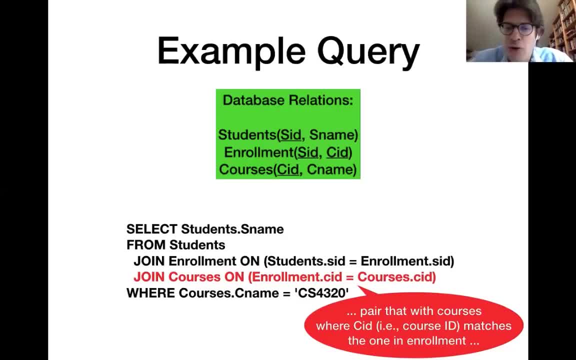 That match on the student id and on the course id, because those are the two joint conditions you see here. So the next step I'm doing here is that I filter the rows in my recirculation using this predicate, and in this predicate we are essentially restricting the course name to CS4320.. 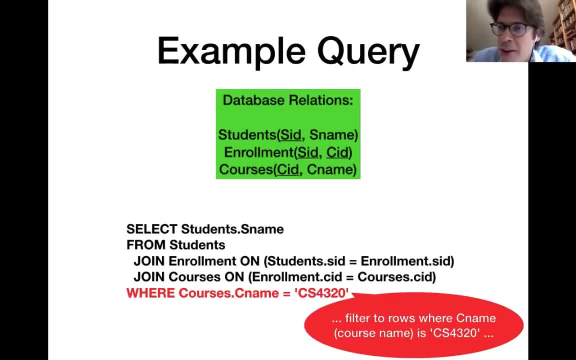 So I want to know something about course enrollments for that specific course. All right, so we will discard the rows which don't satisfy this condition in the where clause. Now, finally, we look at the select clause, and here I'm essentially specifying the columns that I want to keep in my recirculation. 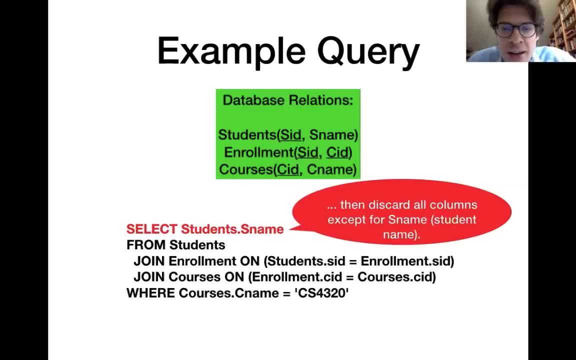 So I will discard those columns which don't appear in the select clause And, as you see, throughout this entire query we have always referred to columns by this notation that you see here. Here I'm selecting the s name, the student name column in the students. 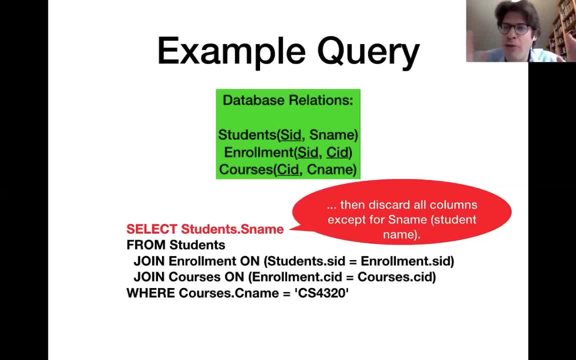 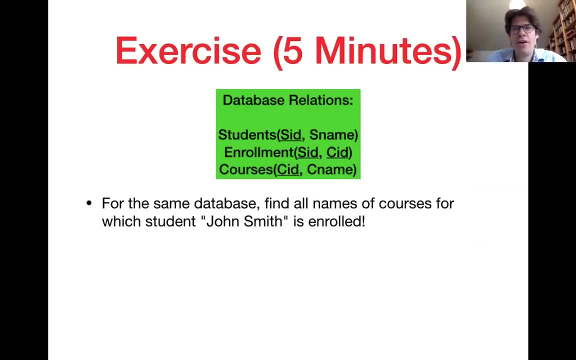 relation. So if you want to refer to one column of one specific relation, we use the notation relation, aka table name, dot column name. We also see a couple of alternatives, a couple of simplifications in the following Now. so now you have seen your first. 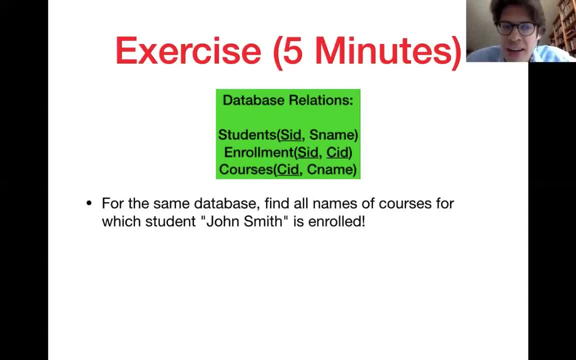 SQL query In order to get the hang of it. I think it's good to make a little example here. I give you a couple of minutes- maybe five is maybe even a little bit much- And here I ask you to find the names of courses. 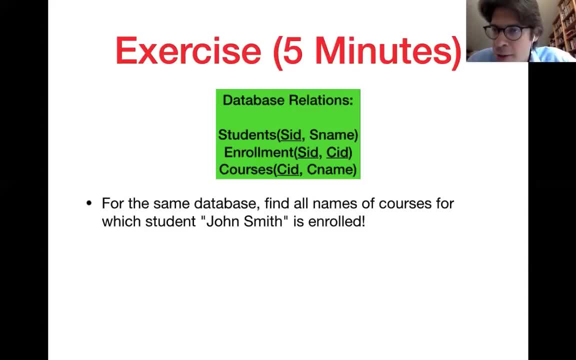 in which one specific student named John Smith is enrolled. So give it a try to formulate that SQL query. You can either do it on paper, or you can do it in Postgres, if you have it installed, or you can go to this website that I have shown you. 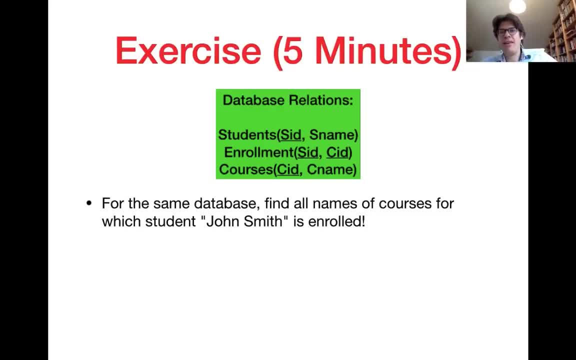 at the beginning. And here there is one question: whether by doing the select we create a new relation or whether we modify the old one. So in general, this entire SQL query together, all clauses together, is defining one new relation to create. So you cannot say that the select clause alone is creating that relation. 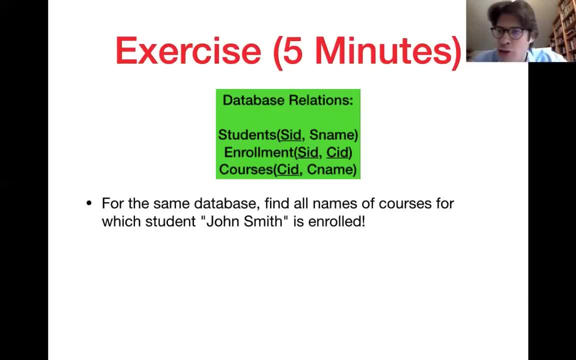 but the query in its entirety is essentially creating one temporary result relation that will be shown to the user. All right, so I'll give you a couple of minutes to make that example and in the meantime I'll show you how to do it. I'm answering questions that appear in the chat here. 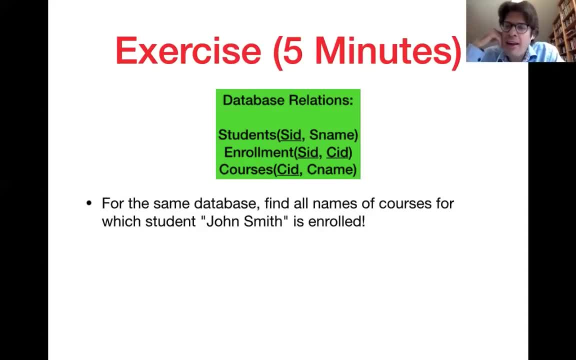 Okay, and this is a very good question. Somebody's asking whether we can only join using columns that appear in foreign key constraints. So you might remember from last time we've seen that we can link the columns from different tables by those foreign key constraints. We essentially specify that. 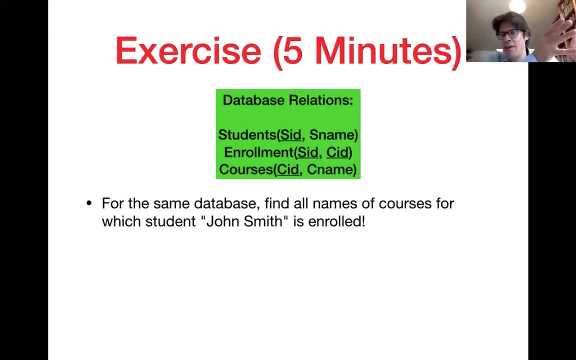 value of the column is equal to the value of the column. So you can see that the columns that appear in the columns of one relation must appear as primary key in the columns of in another relation. So you're essentially matching rows from one relation with the foreign key on the columns. 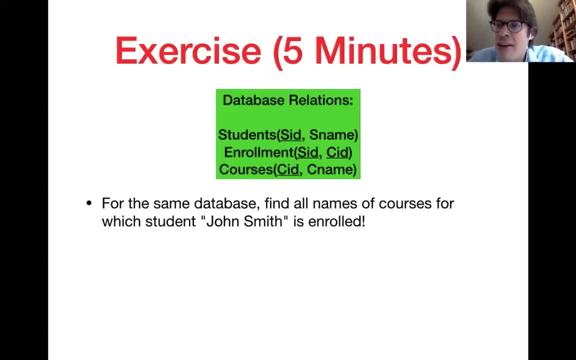 to rows in another relation And in those examples here I have indeed used joins that connect relations which are linked by foreign key. Now, in general, this is not necessary. In general, you can formulate arbitrary join conditions and you can formulate arbitrary joins. You can join arbitrary relations Having. 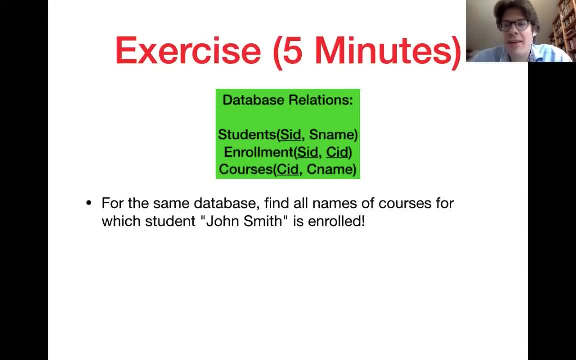 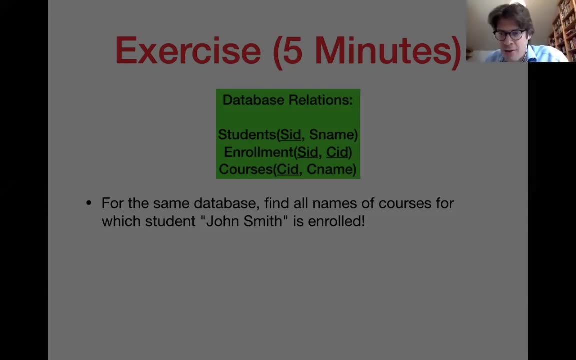 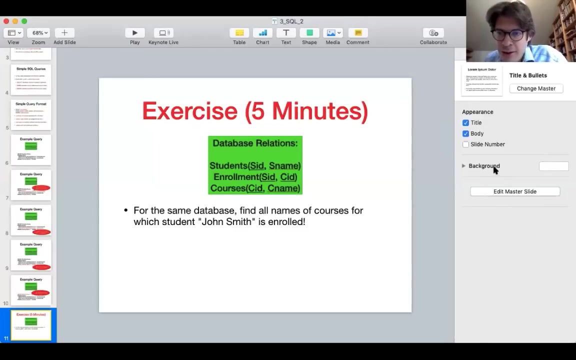 said that the most typical join is actually, so in practice, the most common case is that you join tables with foreign key conditions, but that is not required, Right, and here I'm just accessing the chat, All right, and that is another a great question here. 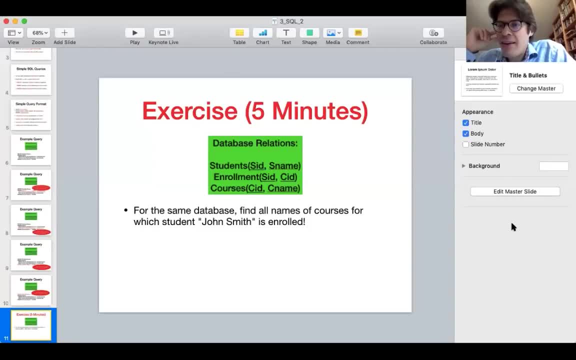 Question is whether the order of the tables in the joins matter. Now, the order of the tables does not matter for the query result. Also, internally, the database system might freely choose the order in which it internally executes the operations for joining a table, So it typically does that to. 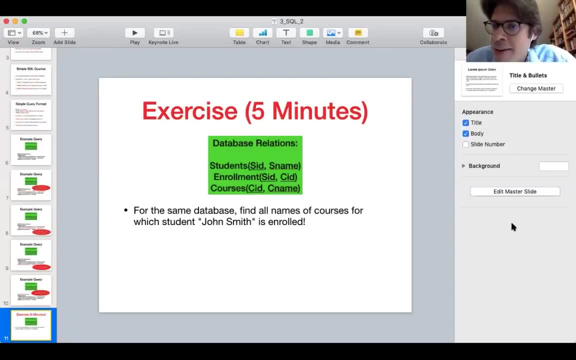 optimize the expected running time for answering your queries. So for the final result of the query, the order of your tables in the join does not matter, And if you have a reasonably sophisticated database system, then the order of the tables does not matter for performance either. 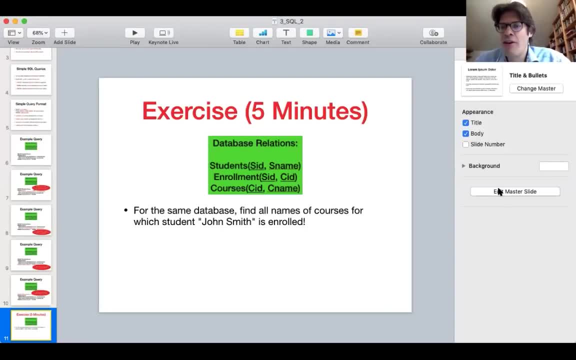 because the database system internally chooses the order in which it does the joins. We will talk much more about performance later. And left outer joins and right outer joins that, as you mentioned here, we will discuss about them later. And yes, so once we come to those left outer joins and right outer joins, 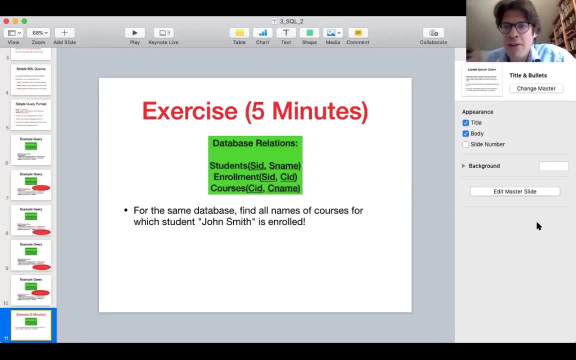 which I haven't introduced yet, then the order will matter. But I mean for the joins that we have discussed so far, the order does not matter. Not for the query result- All right, okay, and for the solution of the exercise. please currently don't discuss it in the chat, yet I'm gonna show that to you. 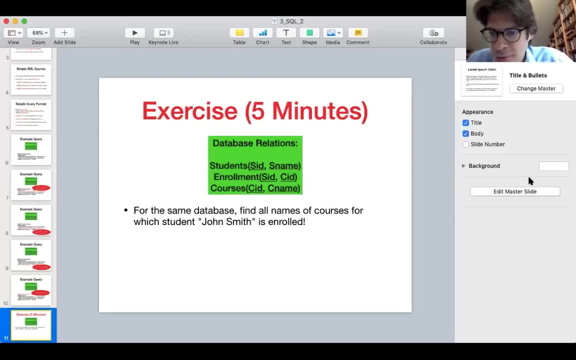 in a minute. If there's questions left after I quickly go over how to approach this exercise, then please feel free to ask them in the chat. Okay, and here another great question Now. we only selected the studentss name, but in the rest of the query we mentioned. 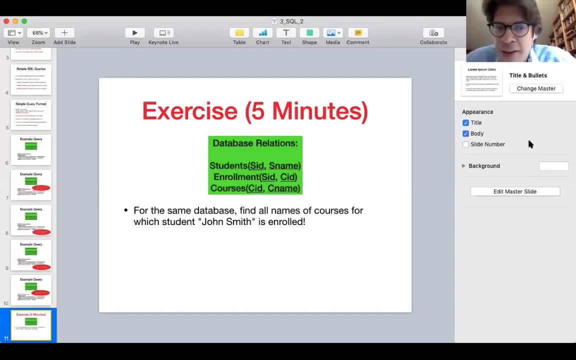 many other columns, for instance in the where condition and so on In the join conditions, But since we only write the student name column in the select class, it means that this is the only one that we as users will see afterwards. Okay, All right, I think now we had a couple of minutes. 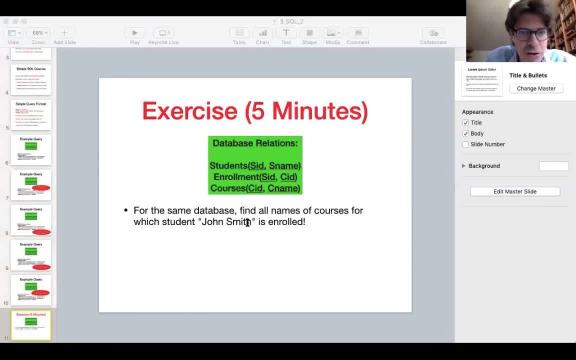 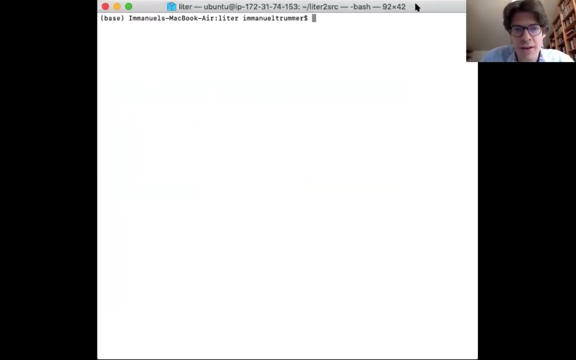 and we answered a few questions. So let me actually quickly enter the solution here in postgres, Quickly share my terminal here. Okay, so I still have the database that we created a last time. If I call the university here, you see the names of the tables that we have here. 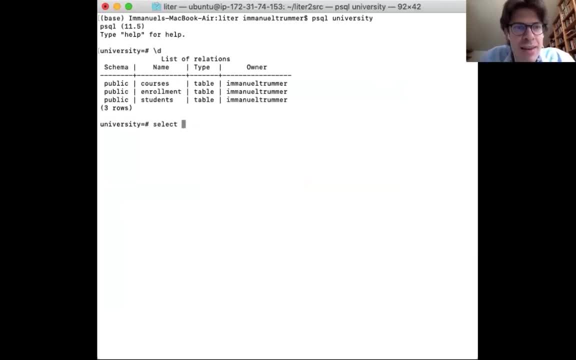 And the goal was to select the names of the courses in which student john smith is enrolled. So we want to find course names. that's why we, as that's what the column, that we finally want to see it, And as data sources, we need, of course, the students, because we want to 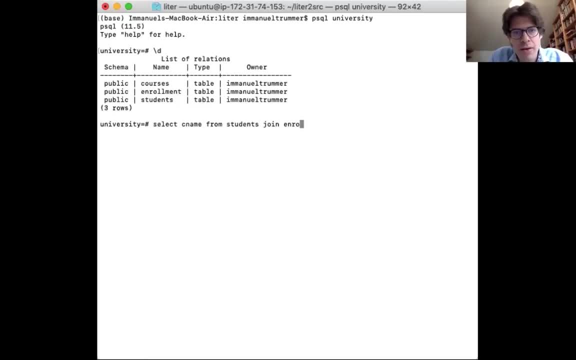 check something about the student name. We need to combine that with enrollment information, And here I'm Using a shortcut that we have not officially introduced yet, So let me write out the name of the students table before the column name. The joint condition is that the students 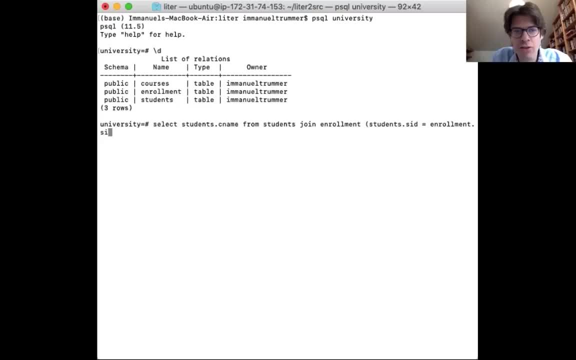 student id must match the enrollment student id And I'm also combining that with the data source and here we must have that enrollment course id matches the courses course id. and now we want to filter to: oh, let's take thank you, and here I want to have the student name. 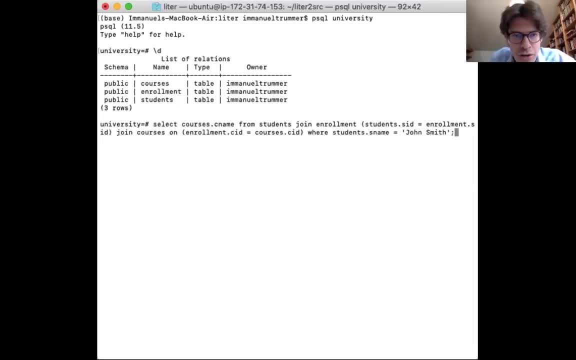 match John Smith. so here we are selecting the courses that curse them from. the students join the enrollment, join the courses that a student name matches at John Smith. so oh, okay, and here a little mistake, now we got it. so here we see that the student is a student name match and here we see that the student is. 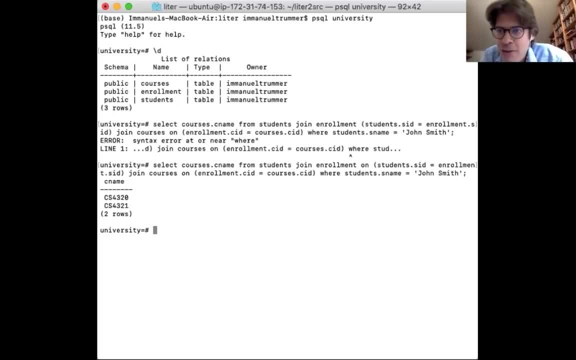 a student name match, and here we see that the student is enrolled in two courses: cs4320 and cs4321. all right, so, and the order of the joint relations for the joints that we are considering right now does not matter. all right, so. this is how we can solve this exercise. it is very close to the 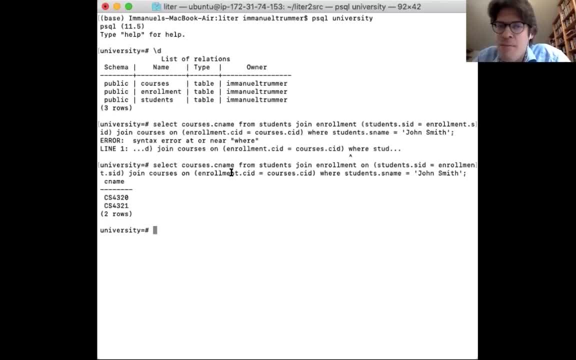 initial query that we have seen. we are featuring by the course name and we are retrieving the students. all right, okay. all right, yes, and from course, indeed, yeah, the states are different. yeah, L� you find in the street. all right, yes, and the front cause indeed includes, yes, all the joints, so that is products. 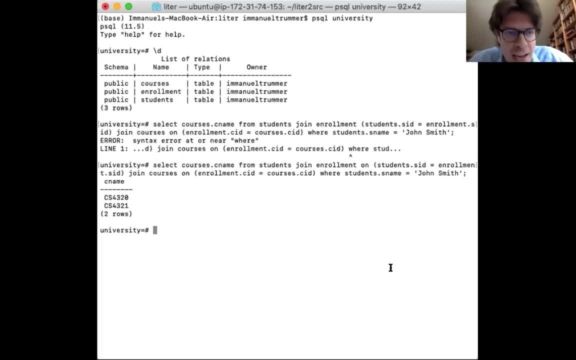 something that you find in the front, clausecraft, and the source, meaning the data source. this combines multiple paper. do not answer this query. this from one of the high schools table table, since you need, for instance, information about normal knowledge of to solve it from base and crushed where the school, where it is based again. 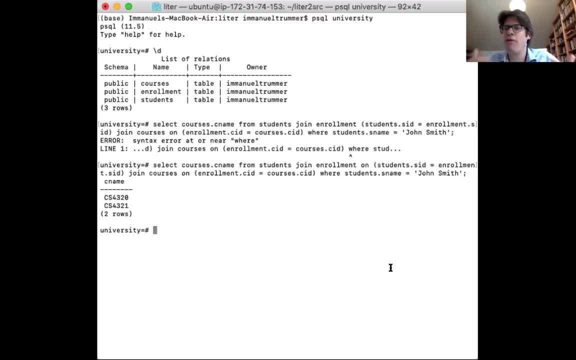 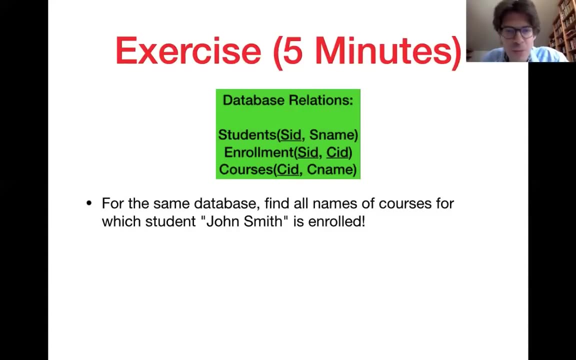 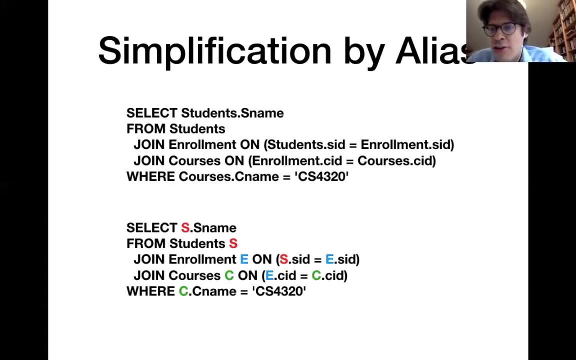 organizations in russia. this leaves you with no solution but the experience of the course name, but also information about the student name that you don't find in the same table. all right now, sql allows you to write the same sql query in many different ways. there's many possibilities to reduce writing overheads, and which one you prefer just might. 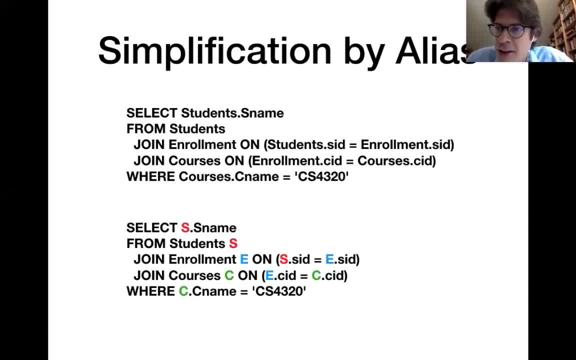 differ from one person to another one. so i'm introduce, i'm going to introduce in the following, a couple of shortcuts that you may choose to use if you find it easier. now, one first thing here is that some of those tables in the database, they can have pretty long names and it quickly gets tedious. 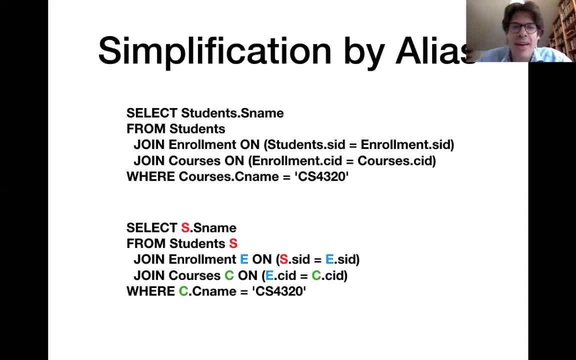 to write out those names multiple times in the multiple times in the same query. so this is why sql gives you the opportunity to introduce so-called aliases, which are essentially a shortcut for the names of tables in the from course. so here you see the same query, but written in two different ways. 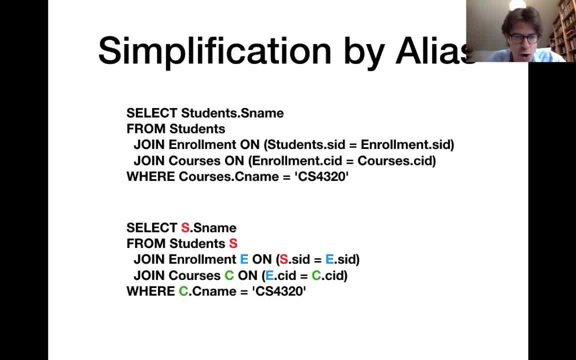 um. in the query on the lower half of the slide, you're essentially assigning the shortcut s to the students table here, and then we are using that shortcut in the other parts of the query, for instance once we are referring to the column that we want to select. then, once we are referring to 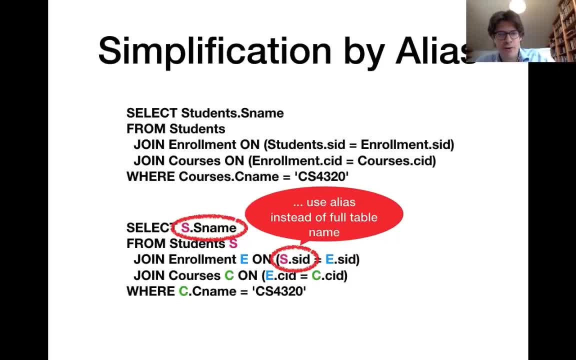 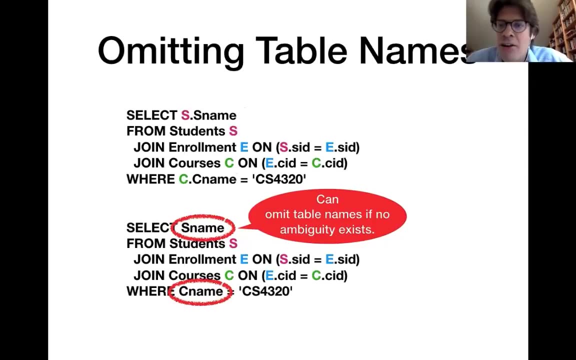 columns in join conditions right. so this simply saves you typing a little bit when writing the query and you can even simplify further if column names are unique among the tables that you use in your from clause. so for instance, the student name and the course name columns. the student name column. 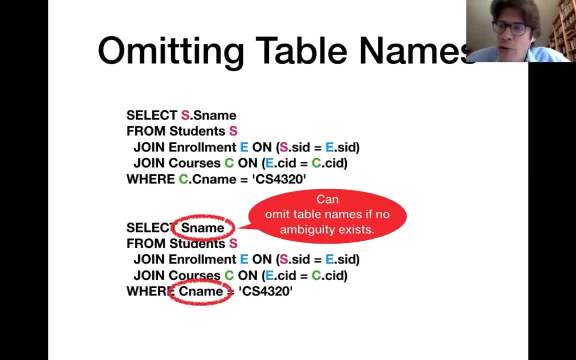 only appears in the students table and the course name column only appears in the courses table. so if you just write the name of the colon, then the database management system should be able to infer the associated table automatically. because there's no ambiguity in those cases, sql allows you to simply omit the name of the corresponding table. 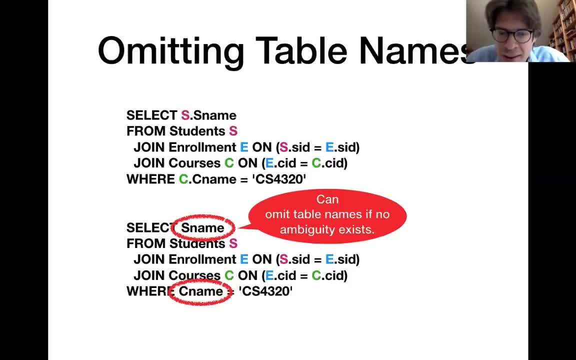 the other side, if you have something like the student id or the course id, the student id, for instance, appears in the students table, but also in the enrollment table. so if you just just write student ID, the database management system does not know which table you are referring to. 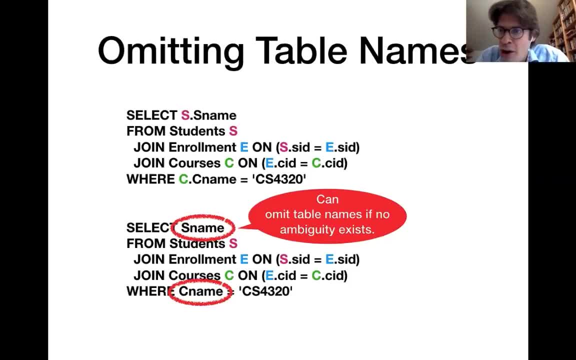 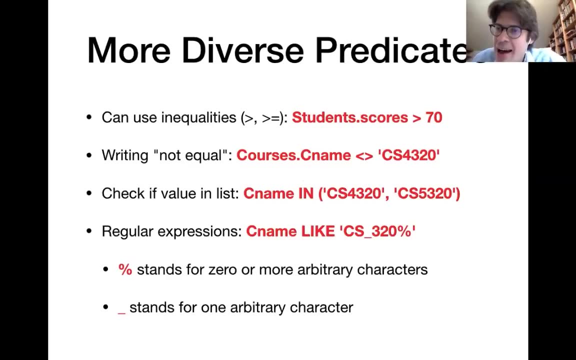 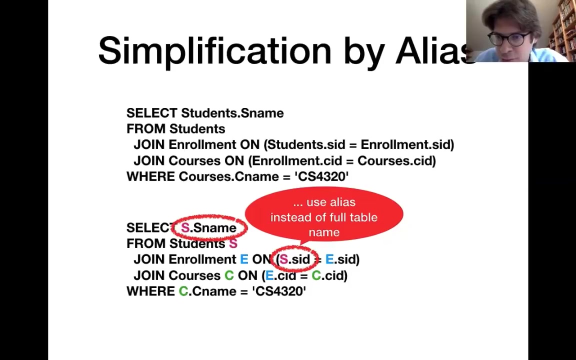 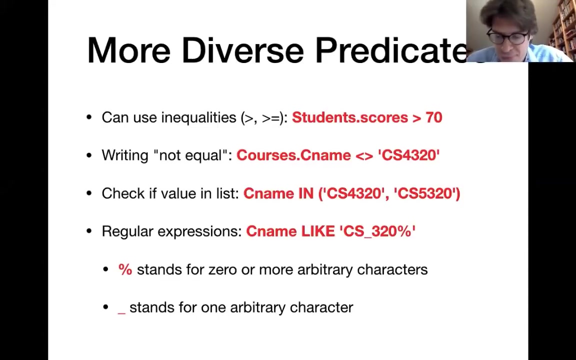 And that's why, for those columns, you have to add the table name or the alias name, All right. And for the alias- both works- You can also use the AS keyword, All right. so these are some shortcuts that you can use in order to simplify. 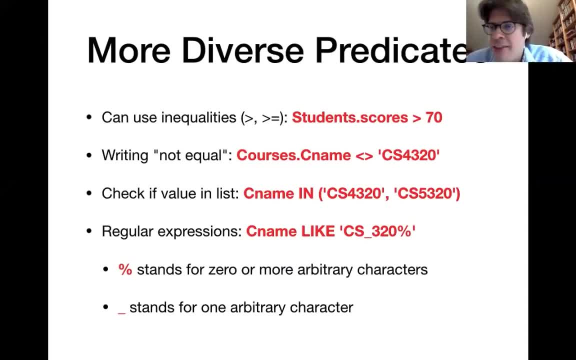 the SQL queries that you write, The predicates, for instance in the where clause that we have seen so far. they have been relatively simple, but SQL supports a very rich set of predicates that you can use And you can use them to formulate. 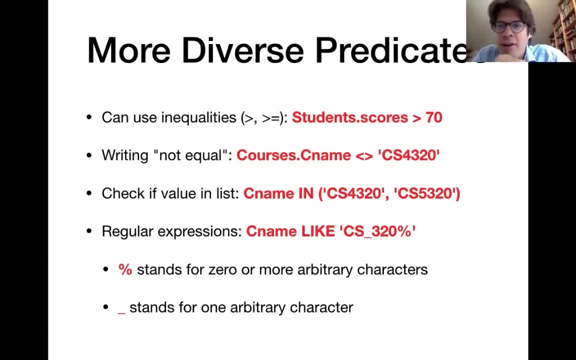 Of course, you can use quantities and inequalities. You can, for instance, check if the value in one column is within a list of allowed values, And you can even formulate regular expressions. For instance, here I'm checking whether the course name. 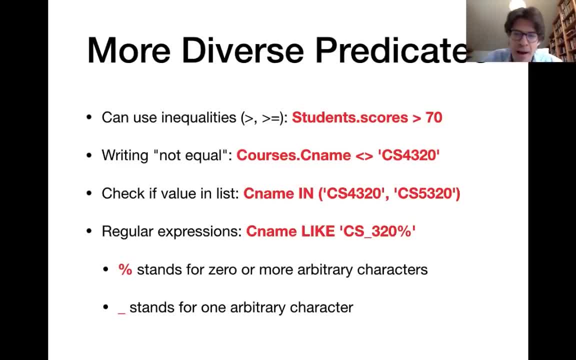 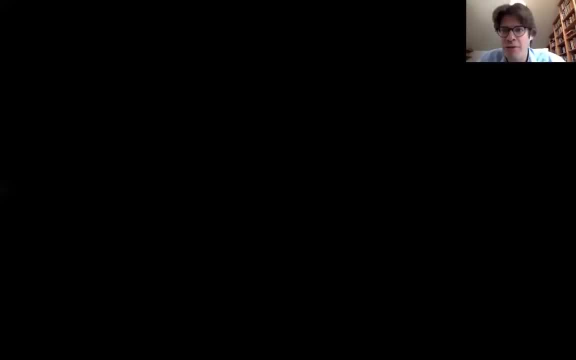 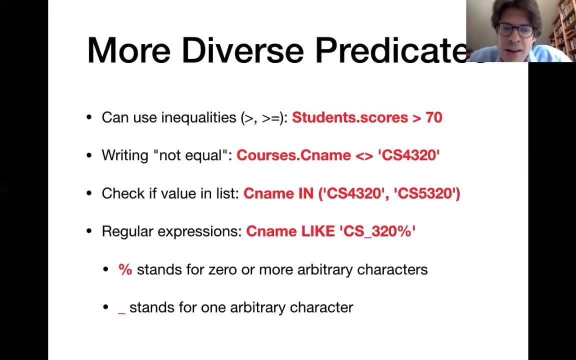 matches the expression CS. All right. so here I am, I'm taking a look at with the and I'm taking a look at with the SS logo here. you're gonna see that as well. So let's take a look at some of this. 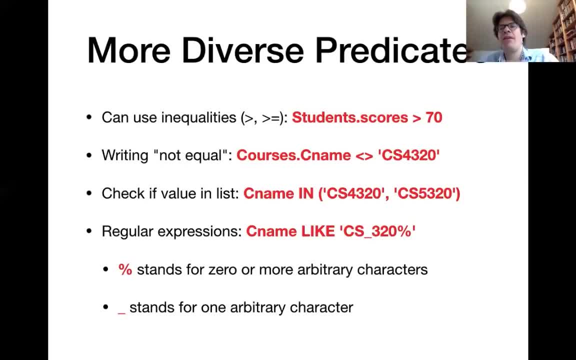 So if we go back to the start button here, that's where we get the first tab, That's where we get the first page, and SQL supports many more types of predicates. but let's say the things that I'm showing you here. in my experience, those are perhaps the things. 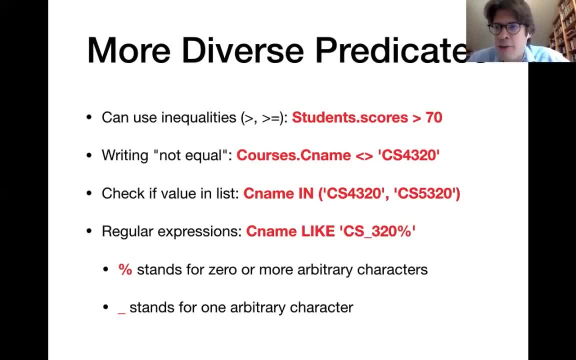 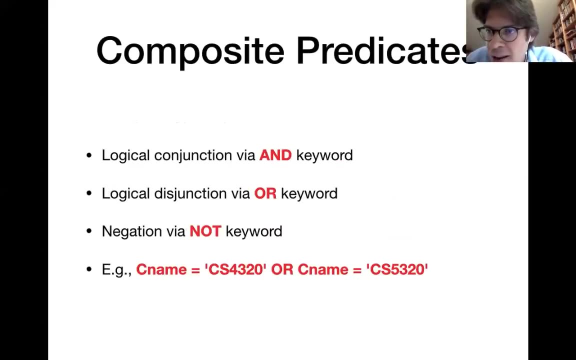 that you use most frequently in a practice. So if you learn those things, then you should already. you should be able to treat most cases that arise in practice. Of course, you can also compose predicates using the typical operators. You can formulate a logical conjunction. 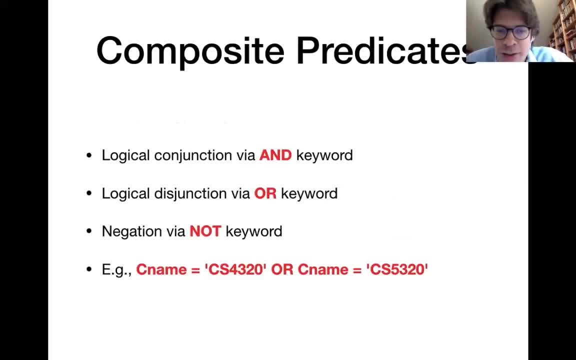 by using the and keyword or a disjunction. by using the or keyword, You have the not negation and for instance, here you could check whether the course name is CS 4320, or whether it's 5320.. An alternative way of writing that would be: 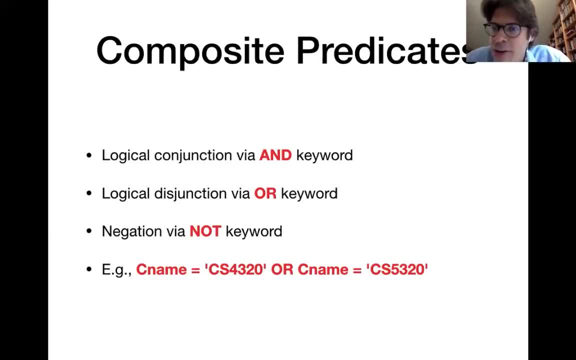 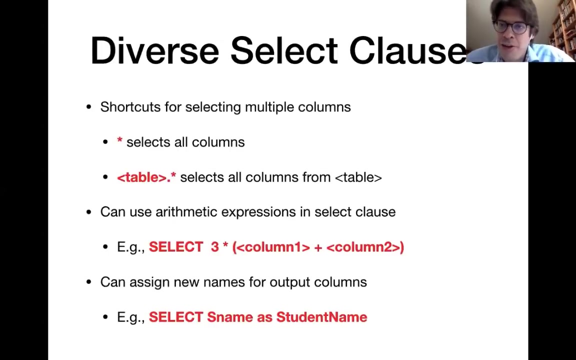 by using the in list, the in keyword, the in keyword that we have seen on the previous slide. All right, Good. Okay, couple of questions here in the chat. All right, So beyond the predicates, there's also many more features that you can use. 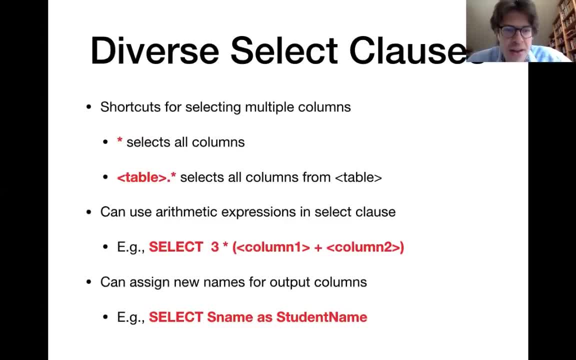 in order to write your select classes, For instance, the tables that you will be working with in practice. often they have a lot of columns and it can become very tedious to write out all the columns names if you just want to retrieve all the information in a table. 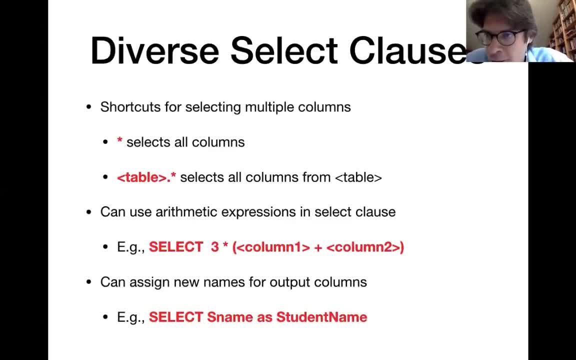 So the star operator in the select class. so when you use the table, the star operator in a select class clause essentially means that you want to retrieve all the columns that you have in your tables, in all the tables that you selected in the 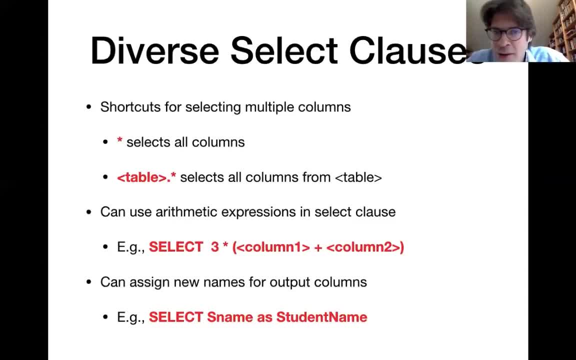 front clause You can make it more specific by writing a table name, dot, star, and then you retrieve only the columns for one specific table. You can also formulate arbitrarily complex arithmetic expressions in the select clause. You can for instance here: you can sum up values in two columns and 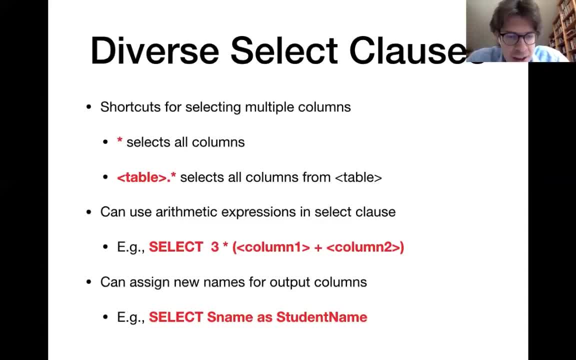 then you can multiply by some constant and so on. That is fine And, especially if you do this, if you use some complex expressions instead of single column names in the select clause, then in order to not get confused by the output of the query, you probably want to probably want to. 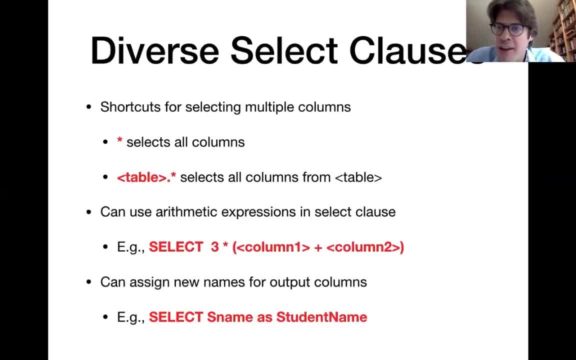 integrate all the columns that you have in the select clause And then you can introduce some readable name for the corresponding column, and SQL allows you to do that simply by writing the name that you want for the column after here the column name after the AS keyword. So here, for instance, I'm renaming the. 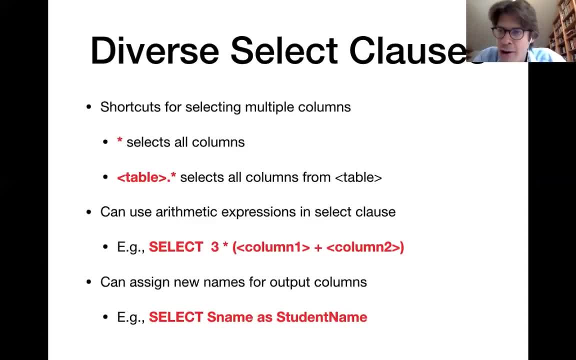 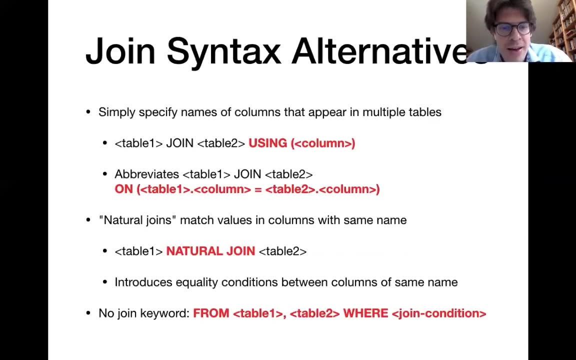 student name column at the S name column to the more readable student name. I could also use the student name column to the more readable student name. I could also use the immersed undercitleshelcom, but in order to assign some name to the expression that you see above. There's also a couple of alternative ways of. 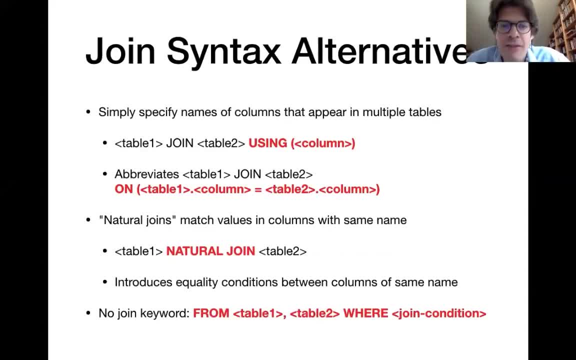 of writing those joint conditions that you have seen so far. So far we have been explicitly formulating the joint condition, but there is a couple of frequent cases of for which people have introduced shortcuts in sql for instance. often those joint conditions, they are actually equality conditions between columns of different tables. here, for instance: 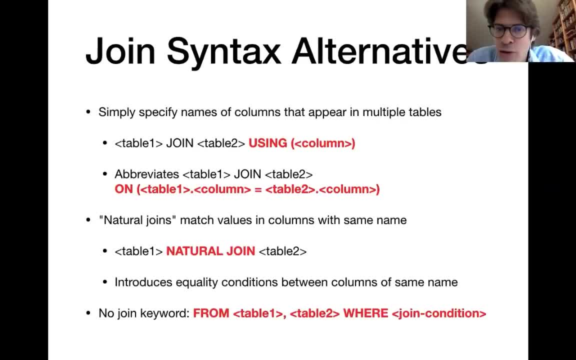 you can use the using keyword and simply you write the name of the column that should be equivalent, and then it is automatically expanded into this equality condition. also quite useful in practice is the natural join. a natural join between two tables simply means that you want the values in all columns that have the same name to be equal. so instead of 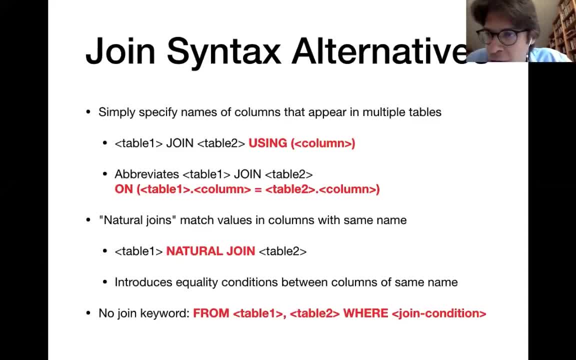 actually typing out the names of all the columns on which you want to match. this one will be expanded automatically. it can be a little bit dangerous because every once in a while if you're dealing with large tables with many columns, then you know that they have one column of the same name in common. but 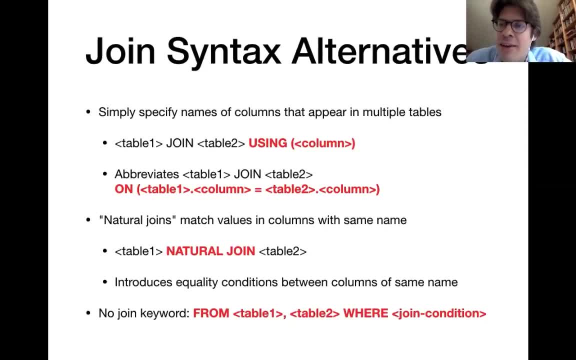 there might be other columns of the same name that you are not aware of. so the natural join is sometimes a little bit dangerous, because every once in a while you will overlook that there is other column paths than you intend which also have the same name, and then they get automatically added to the join condition. so table one: natural join. table two: 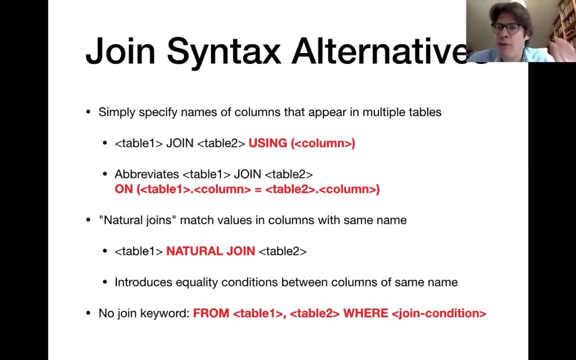 means i'm retrieving all the paths of couples from the first table and the second table which have the same value in all columns that have the same name. i'm gonna go to show you some examples in a second. finally, just so you know, you will sometimes find um, you will sometimes. 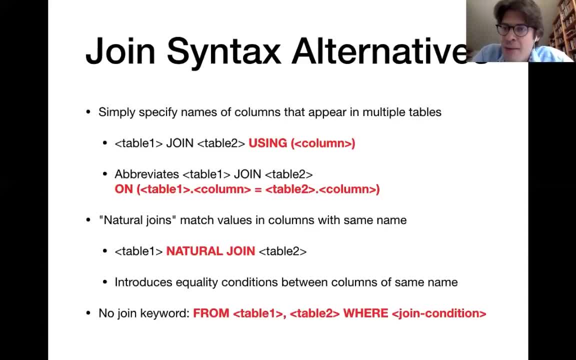 find um queries where somebody doesn't use the join keyword at all. that is also admissible. if you write something from table one comma table two, where join condition, the semantics is basically the same as if you had written table one join, table two on join condition, right, okay? 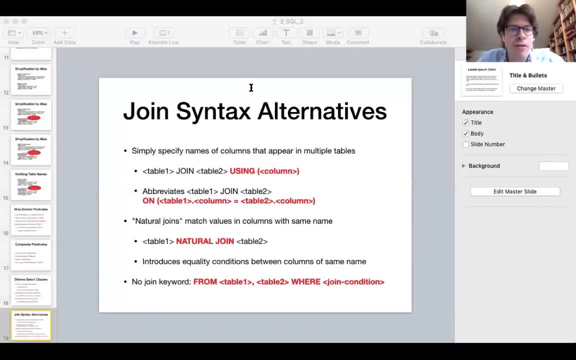 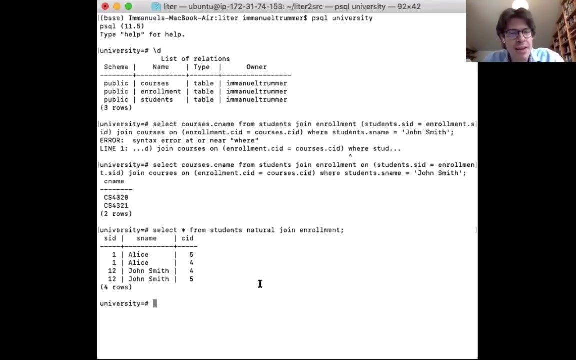 so let me throw this one for just a second, because i have never written any formula in table one, so what i'm going to do is i'm going to read out from the follow-upacji: all right, and now? Now you should be able to see my screen again. 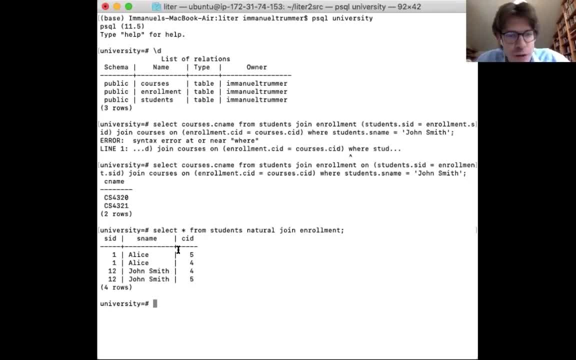 So here, just to show you one example with the natural join, I see that somebody tried it and it gave an error. but I mean the principal, you do it like this. it should work. So here we have the students table and the enrollment table. 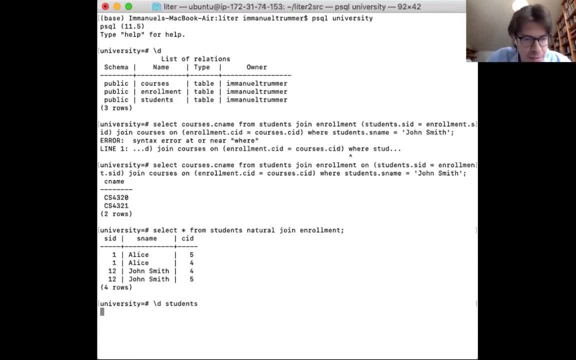 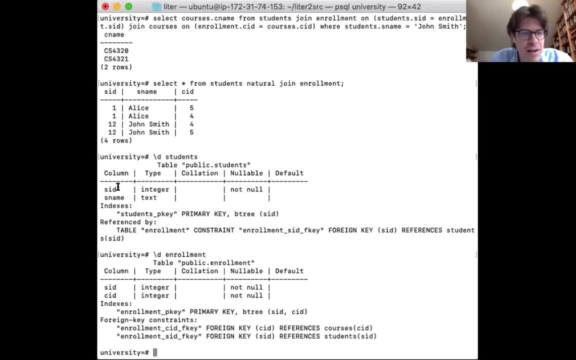 They have one column of the same name. Let me show you this Right. so the students table has the student ID and the enrollment table also has the student ID. So if I do the natural join between the two, then that will automatically match them. 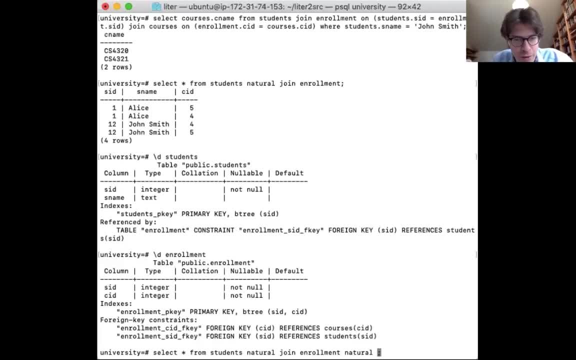 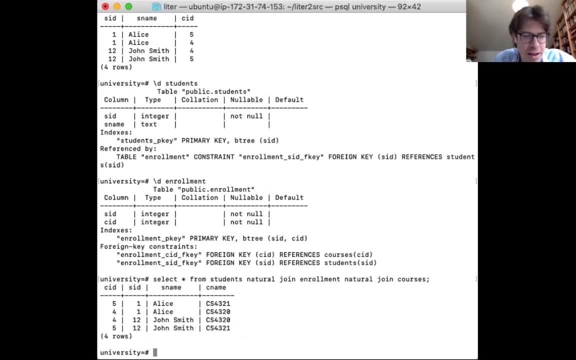 And you can also do a natural join on multiple tables, as one of you is asking us a good question. So here, for instance, if I joined with the courses table in addition, then here implicitly I'm adding a match condition for the course ID. 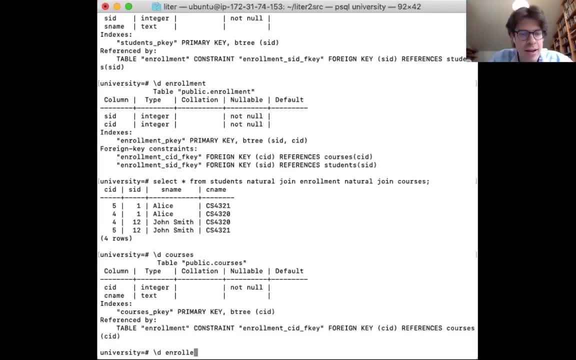 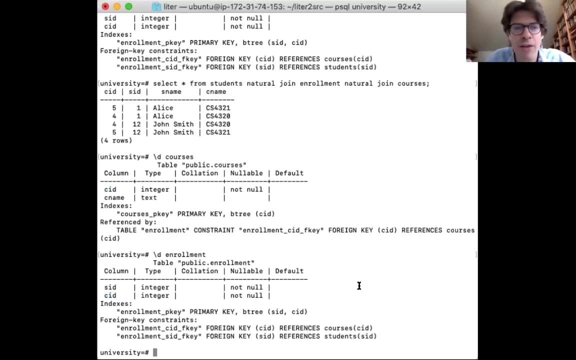 which appears in a courses and it also appears in enrollment. Okay, so that is one way of writing this query And, as you see, I'm using the star notation and select clause in order to retrieve all the columns of the result. Okay, 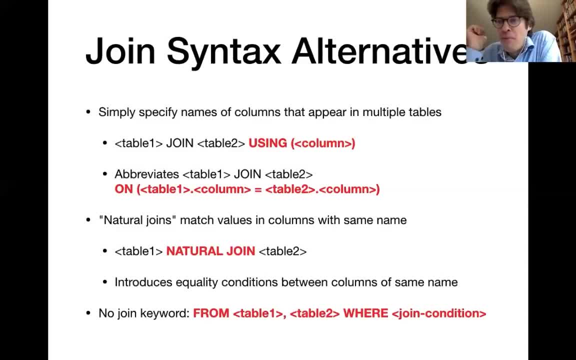 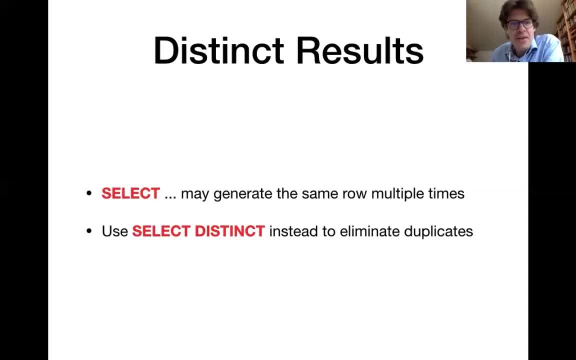 All right. so those are a couple of alternatives about how you can formulate your SQL queries. encourage you to play with it a little bit and try out different formulations. one last point: so far we have been using the select clause, and if you do this then in principle, you might get the same row in your reside multiple times. 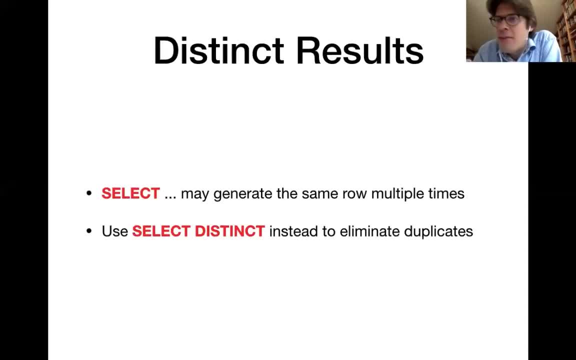 sometimes that's maybe even what you want. often it's not what you want, and in order to eliminate duplicate reside rows, which are kind of boring, you can also use the select distinct notation and then the database management system and automatically eliminate all the duplicates. now, so far we have been 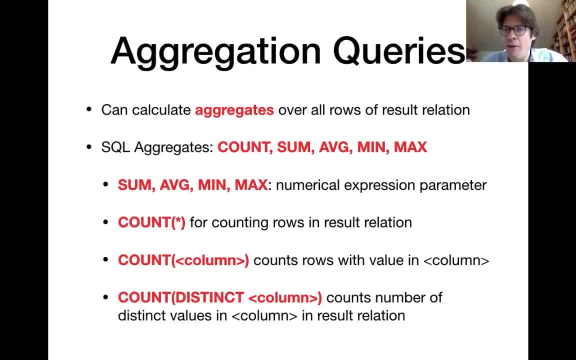 generating resides that consists of a single Rose. but if you're dealing with a lot of data, then often you rather want to learn something about aggregates. for instance, you want to count the rows that satisfy up conditions, and SQL gives you a rich set of aggregates that you can use. here you 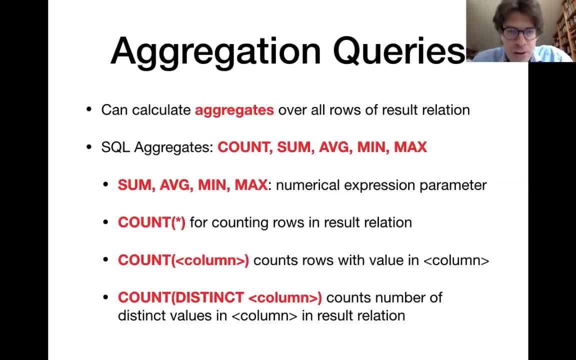 see the aggregates that are supported by default. you can count things, you can sum up things, you can average things, you can calculate minima and you can calculate maxima. now we will see a concrete example in a second. just if you a broad overview of different aggregates that you can use, you use those. 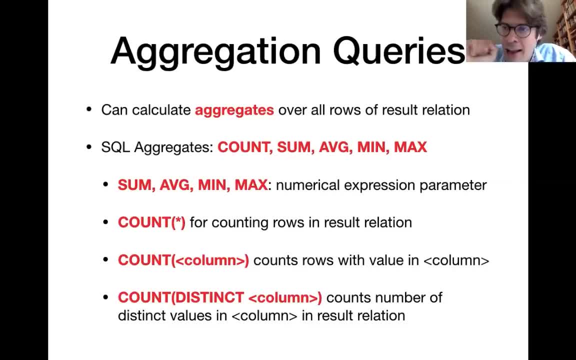 aggregation functions typically in the select clause. instead of getting all the different rows as a result, you would rather get the number of rows, for instance, or the maximum in one specific column on. those aggregates typically have some parameters, for instance for summing or averaging. you need to 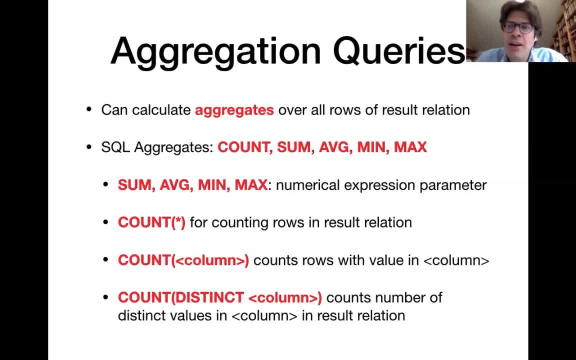 indicate which column or which expression you want to sum or average over one common annotation is. if you want to simply count the number of recited rows, then you typically use this count and star between parentheses sometimes. we have already quickly discussed, and we will discuss this in more detail, that a SQL 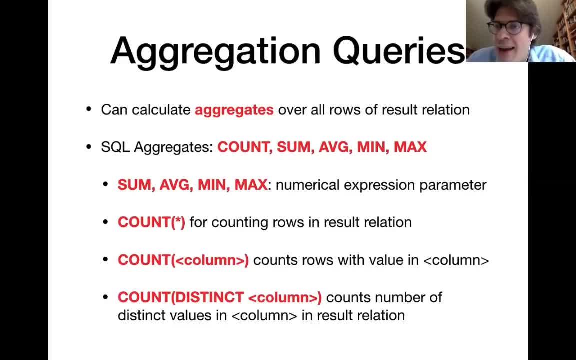 allows you to replace unknown values in a certain row in the column by placeholders, which are called null values. sometimes you want to count how many reside rows you have for which the value in one specific column is unknown, and you can do this by writing this count and then, as parameter, within parentheses, you write the name of the column in which. 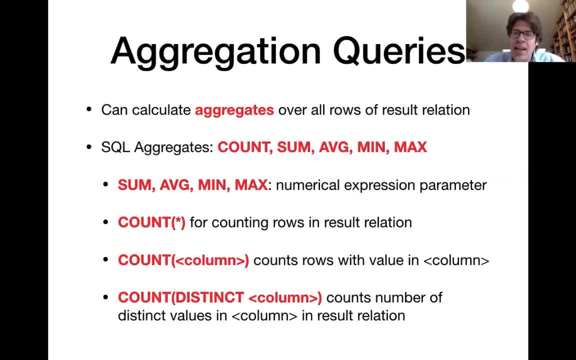 you need to have a value. you can also count the distinct, the number of distinct values that appear in certain columns of the syntax. and this is just some of the most common commonly used features. if you're interested and explore a bit, then you would find many more, but this is what. 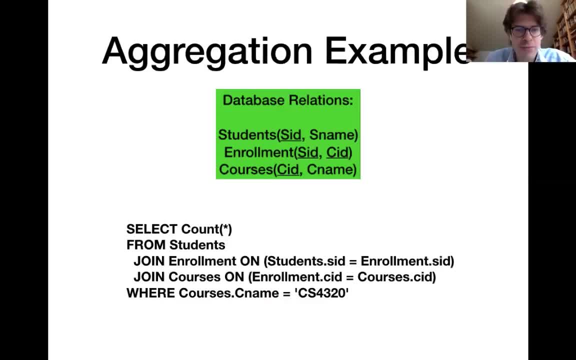 you need. in most cases, in my experience, this is how we can use that in this example query over here. this is nearly the same query as before, but no, I actually don't want to retrieve a specific student names anymore now. I just want to count how many students are enrolled. so, in order to understand what, 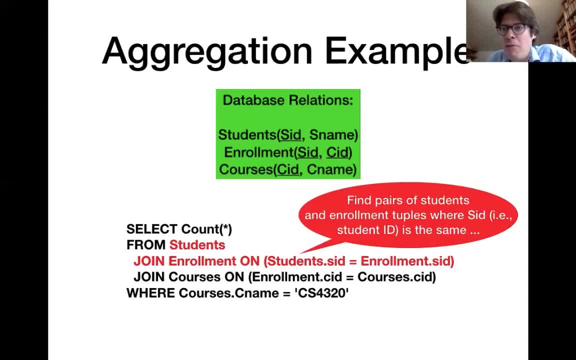 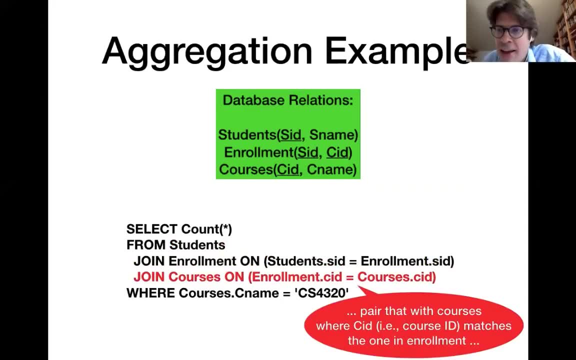 the query does. we can again look at the from clause first, which hasn't changed. so here I'm still pairing up students with enrollment information and combining that with information about courses. then I'm throwing away all the rules that are not about the CS 4320 course. and now- and this has changed compared to before, finally- I simply 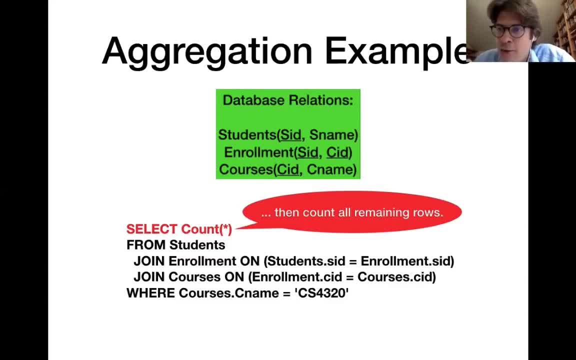 count the number of remaining rows, and so the result of this query would be one single number, which is the number of people enrolled in, as he is 4320. all right, we can check whether there's any questions. you in the chat? yes, okay, and this is an interesting question which already relates to a performance. 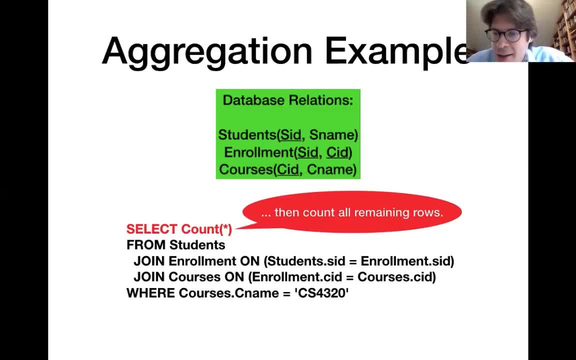 question is, if you have really large tables, whether it makes a difference for performance whether we use the count star syntax or the count in one specific column syntax. so the semantics of the two is slightly different, so you might not be able to use both of them interchangeably. but 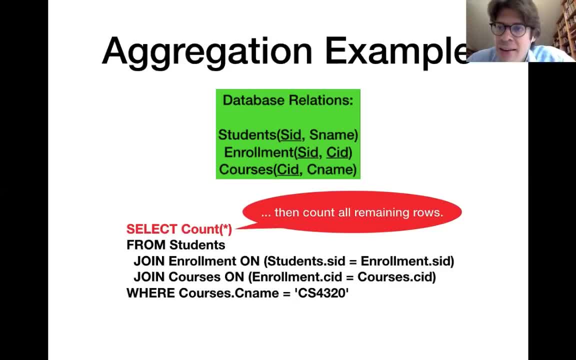 it's a landed question and it depends a little bit on your database management system. so there's- we will see that in more detail much later in this course. there's database systems which are efficient at retrieving data only from specific columns, and they could potentially benefit from that. there's. 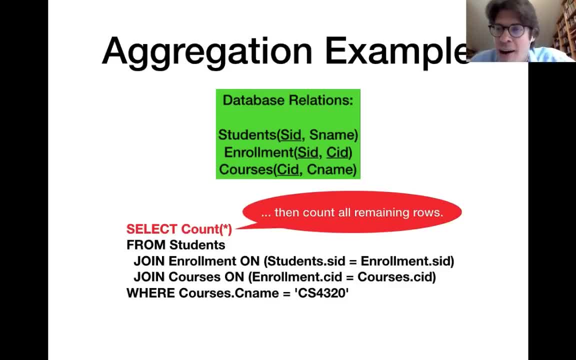 other database management systems which are not efficient at retrieving data in specific columns separately, but they always retrieve all the information about one row in your table together, so they could benefit and that so it depends a little bit on the type of database system that we are talking about. 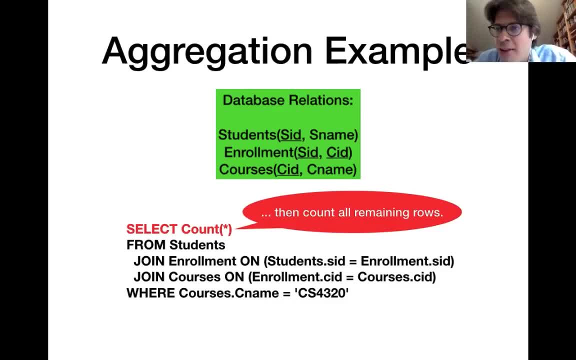 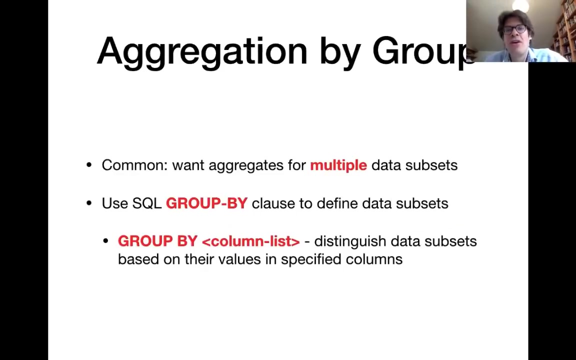 but that is already a topic that we will discuss later in this course. but great question, all right. now, here we are aggregating over the entire query. we cite your counting, all the rows in the result. often, in practice, you actually want to break down things. you want to calculate aggregates for different data subsets. 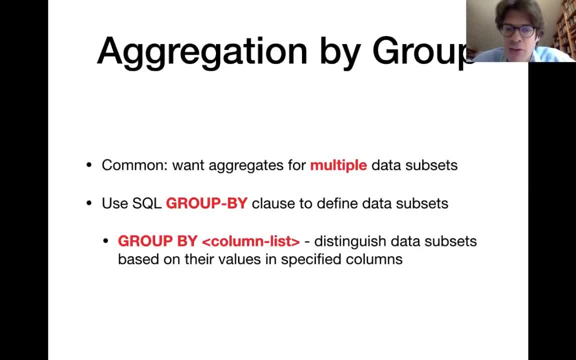 and sequel also allows you a function order to do that. it's called the group, by course, and there you can see that the results are also very, very useful if you, you essentially specify a list of columns that is used in order to partition your data and then for 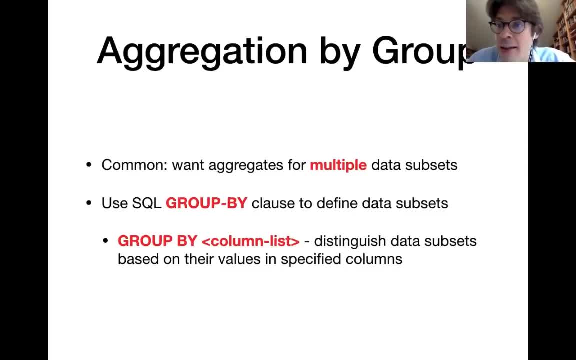 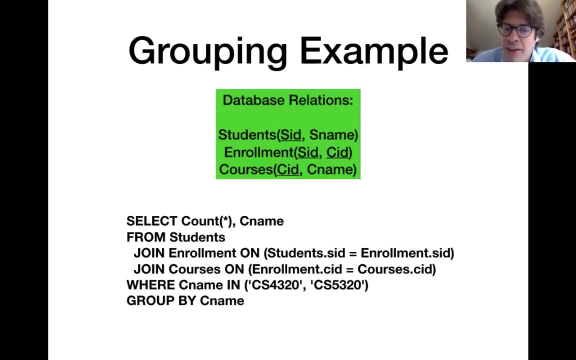 each partition of your data for each group. you are calculating, for instance, aggregates separately. So, for instance, if I want to know how many students have been enrolled in CS4320 and how many students have been enrolled in CS5320, like the second listing of the course, 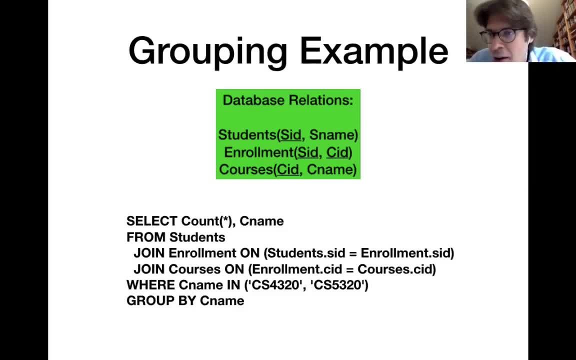 then I could, in this case, issue two separate queries where once I filter to CS4320 and once I filter to CS5320. but it is of course more efficient if I can do that just with one single query, and that is the query that you see here. So the beginning is again, I'm pairing students. 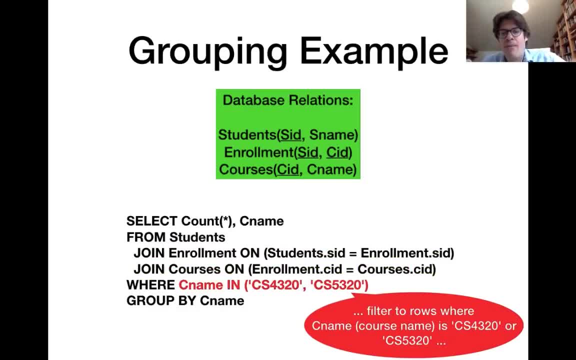 with enrollments and parents. Then I'm filtering to the rows that either concern CS4320 or CS5320. and now comes one- a new aspect, because now I am partitioning the data based on the value in the course name. So I'm separating the rows for CS4320 from the rows for CS5320 and finally I calculate a group specific row count. 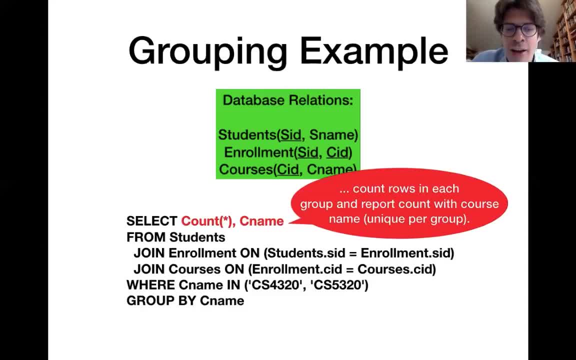 and display that together with the course name, and I could also leave out the condition in the back clause, and then I would get a breakdown for the enrollment number for all courses that are listed in my database. Of course, writing one query like that is much more efficient than to write separate aggregate queries for each specific course. 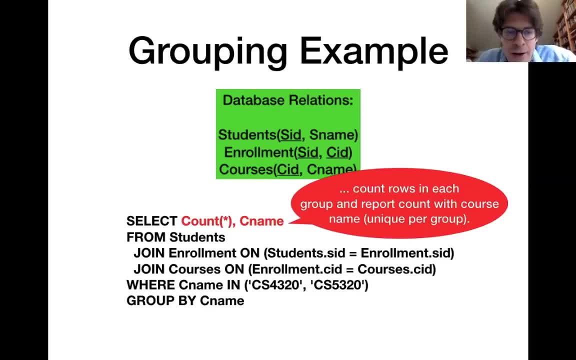 All right. So now you see here that in the select clause I'm selecting the count, which is the count of the rows for each group. I'm also selecting the course name. That makes sense, because I want to know which group a specific count refers to. 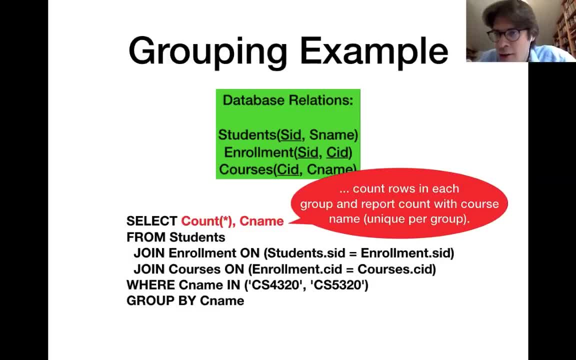 But I have to be a little bit careful in general about what I put into the select clause if I am using a group-by-group, Because the result to a group-by-query must always contain one single row for each group, only one row per group. 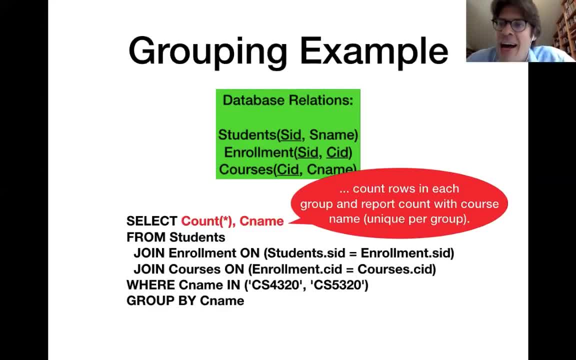 And that means that in the select clause I can only ask for columns and aggregates and general expressions that have one value for each of the groups. For instance, here for the same course I could have multiple students enrolled, So for one specific group of results that share the same course name, I might still have different. 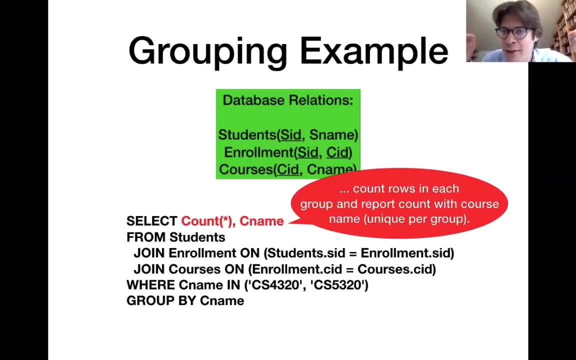 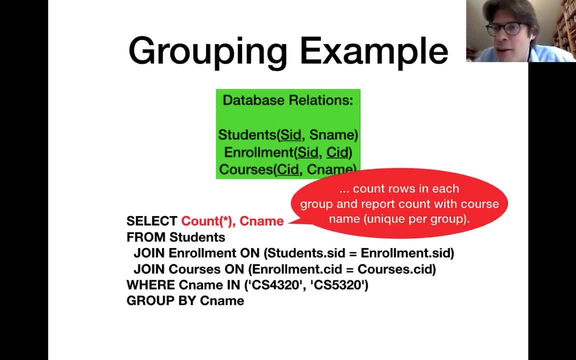 So I can add a new one. So I can add a new one, So I can add a new one. So I can do that. and if it is a unique value per group, then the database management system will throw an error. here. I am respecting that, because the count is, of course, something which is unique. 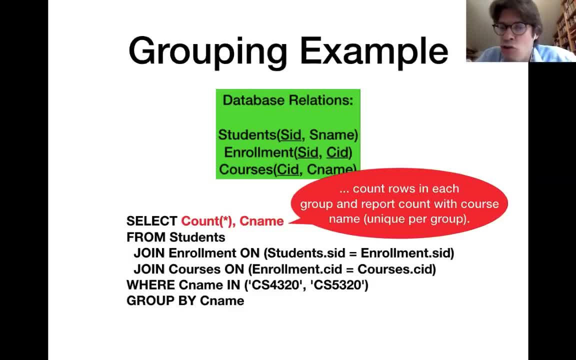 for each group and the course name is also unique for each group, because that is precisely the column that I use in order to define the groups. So, by definition, if two rows have different values in the course name column, then it would be in different groups. 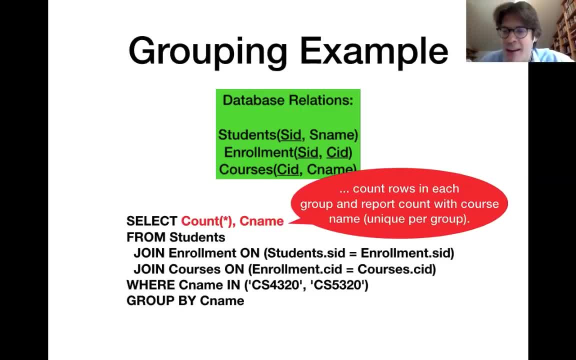 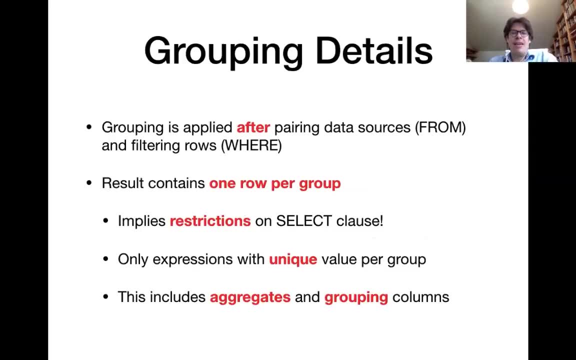 So within the same group, I only have one specific value: you in the group by column. all right, here you see essentially what I just explained laid out in a little bit more detail. so, first of all, in terms of evaluation order, as we have seen in this example, grouping is applied after we. 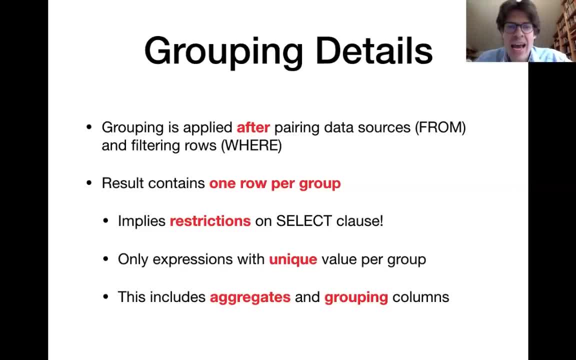 have filtered by the where clause and what I also introduced in this example. you have this constraint that the result can only contain one row for each group, and that implies some restrictions on what you can put into the select clause once you are running a group by queries. all right, now one last feature that I 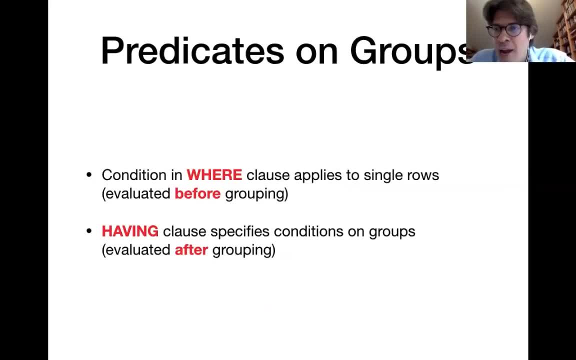 wanted to mention here. sometimes in practice, you also want to put some condition on groups as opposed to conditions on single rows. so the where clause is where you put conditions on single rows and that is evaluated before doing the grouping. then, after the grouping has happened, you might still want to have some condition for filtering. 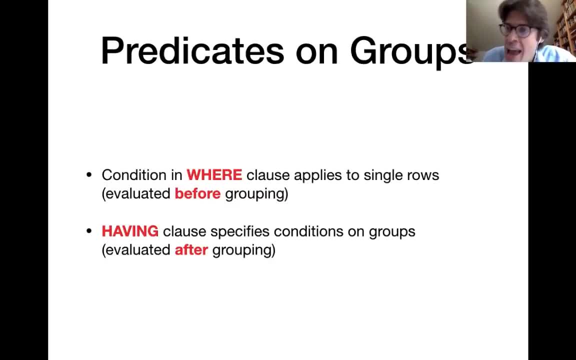 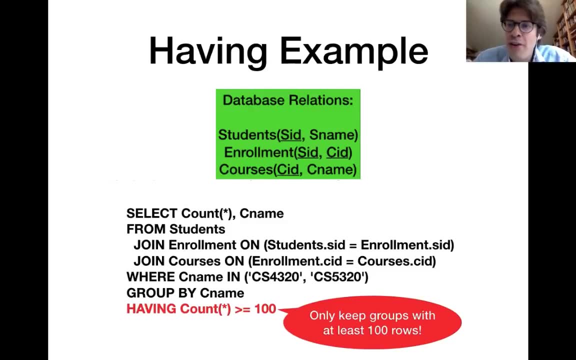 out entire groups. you can do that using the having clause, for instance, in this example that we have added the having clause in order to only show the results for those courses where we have a count of at least 100- which incidentally is the case for those courses here- and then in your query result you're only shown those. 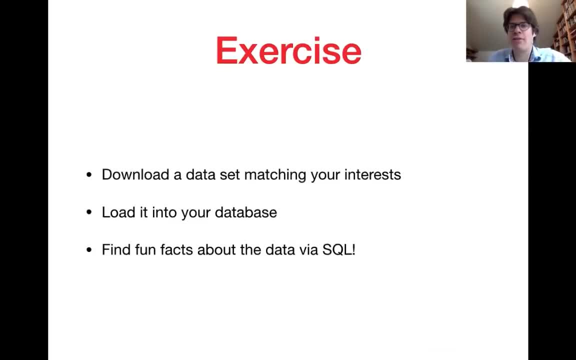 groups which satisfy those conditions. so this is it for some first intro to SQL queries. we want to discuss some more advanced features and then we will go to the next slide. so I recommend you to revise the material that we have seen today and also to experiment a little. 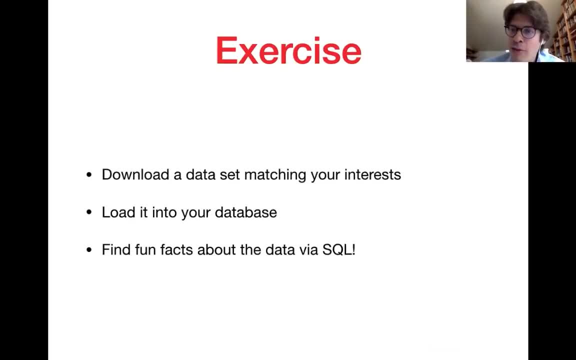 bit. so we have seen different ways in which you can experiment, installing postgres or using this public website. for instance, you might either create a database yourself using the commands we have seen last time, or you might download some data set from Kaggle, for instance, which matches your interest, and then you load it into a database and then you export to this client. on these two, 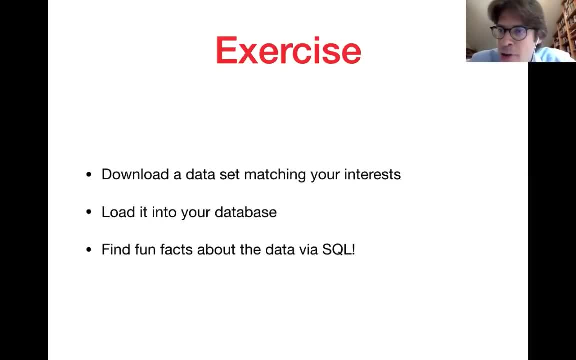 and experiment a little bit with it. So please explore a little bit with those queries And if you find out something interesting about the data set, then please feel free to share your insight and the associated SQL query and data set on Piazza so others might also benefit from that. 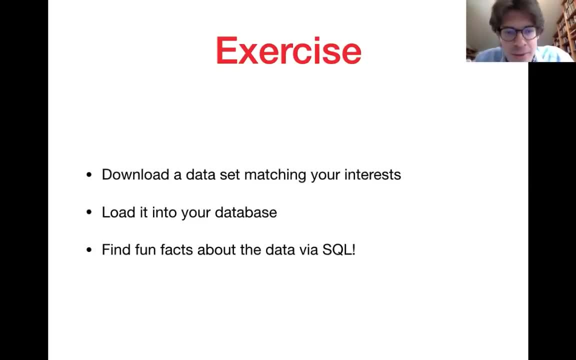 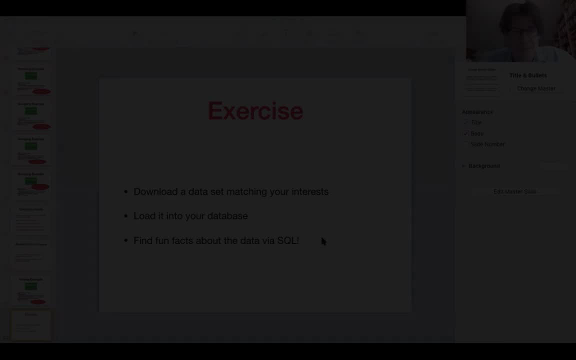 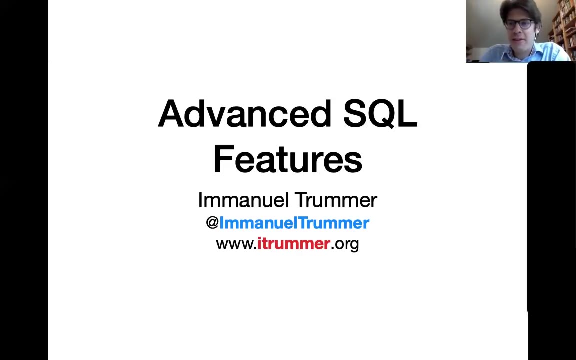 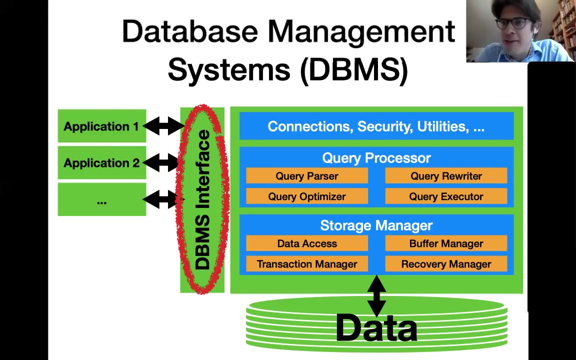 All right, good, Then, have a great day and see you on Wednesday. Bye, All right, let's get started. Hello everyone, Good morning. So today we are still discussing about the interface to a database management system. The relevant chapters are still number three and five. 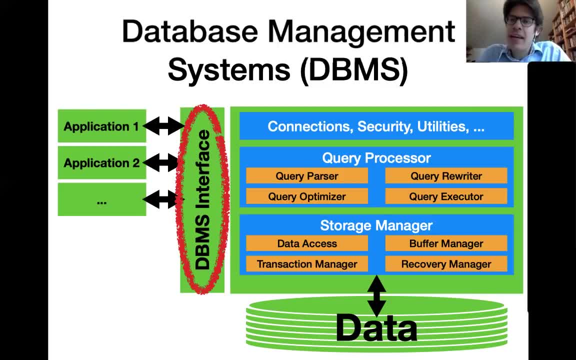 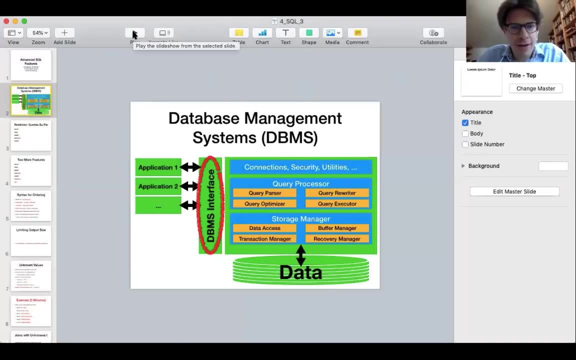 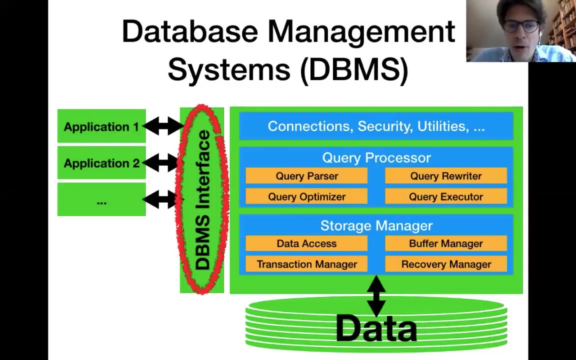 in the Ramakrishnan and Gerke book. So in the last lecture we have seen a couple of ways how we can analyze data in our database via SQL varies quickly. fix that, Yes. So today we're gonna see a couple of more advanced queries. 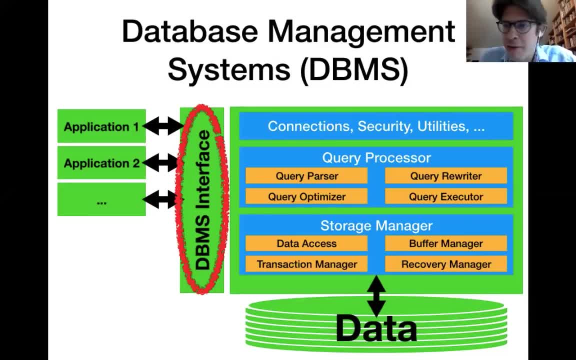 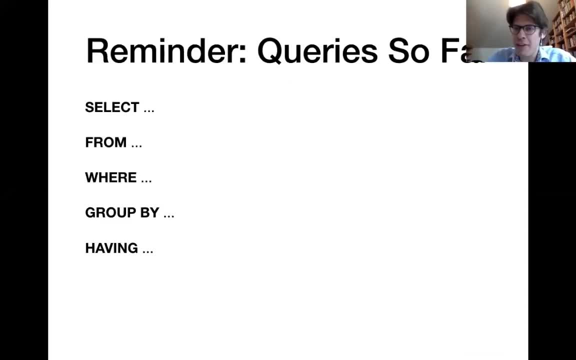 But before we do this, a little reminder about what we have seen last time. Last time we have seen queries that correspond to the format that you see here. We are specifying data sources from which we want to use data in the FROM clause. 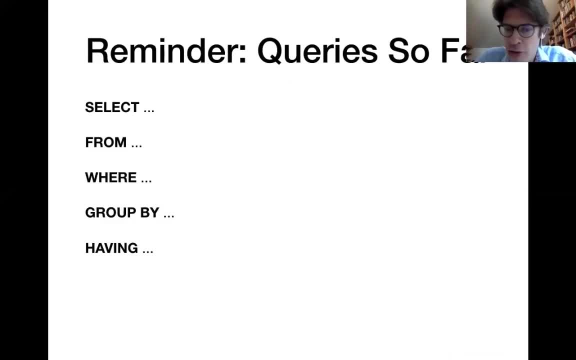 Then we specify conditions that the result rows should satisfy in the WHERE clause. Then we specify how we want to partition our data into groups in the GROUP BY clause, And in the HAVING clause we can specify conditions that those groups should satisfy. All right, and finally in the SELECT clause, 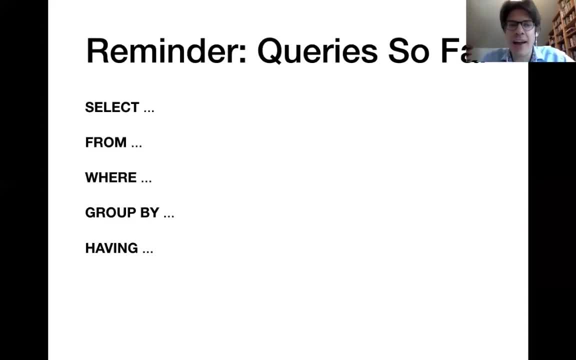 we are specifying which are the columns that we want to see in our result. So many of those parts of the query are actually optional, but this is the things that we have seen in the last lecture. All right now, before we go any further. 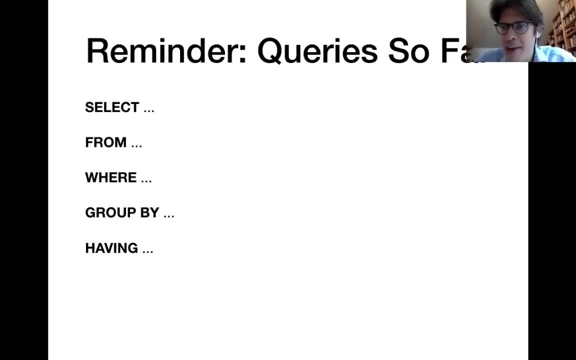 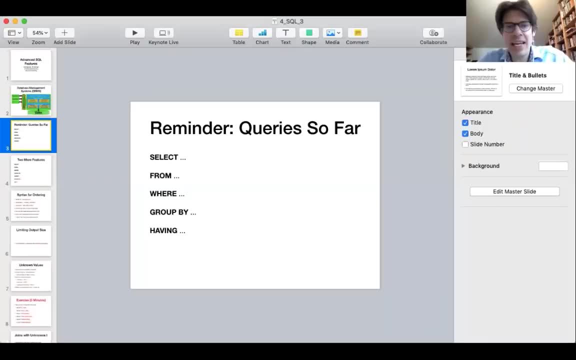 because we haven't seen many examples yet for this type of query. we're gonna get a bit closer to it first. Now let me show you one more thing: do a little bit of data exploration, and if you do data exploration, then you first of all want: 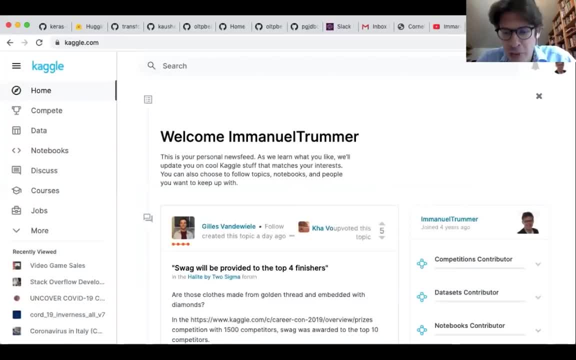 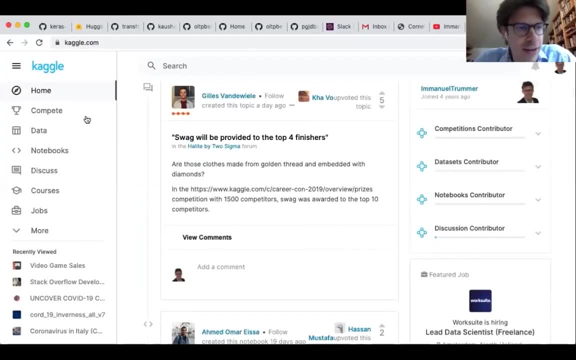 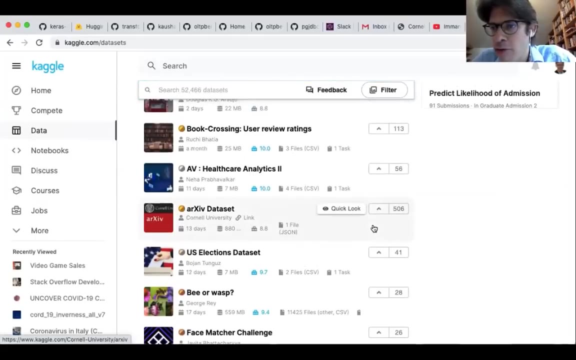 to have a data set. so one possibility to download such data sets is the cackle website, for instance, and if you look under the data attack, then here you have data sets about various topics. so I recommend you to perhaps choose one or two of them, download them and run a couple of secret. 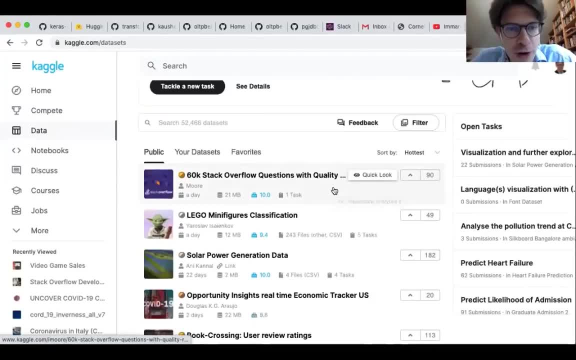 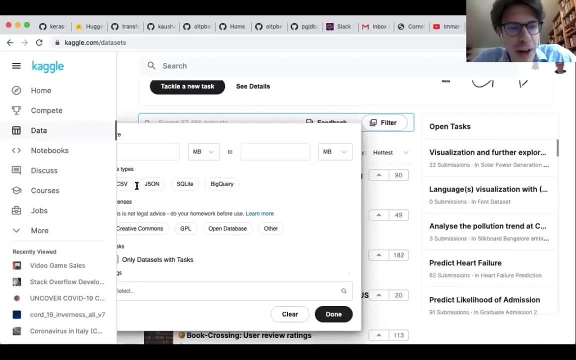 queries over them to get the hang of it, which is what we are about to do now. all right, and here, specifically, since we want to load those files into a database, we can, for instance, with strict things to comma separators, value files that we can easily import into our data set, and 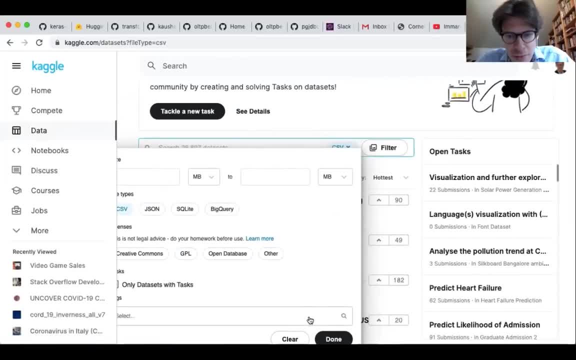 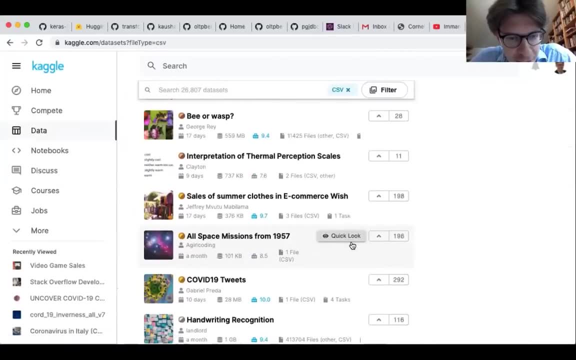 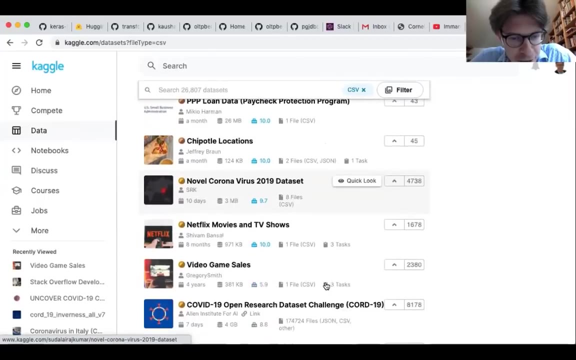 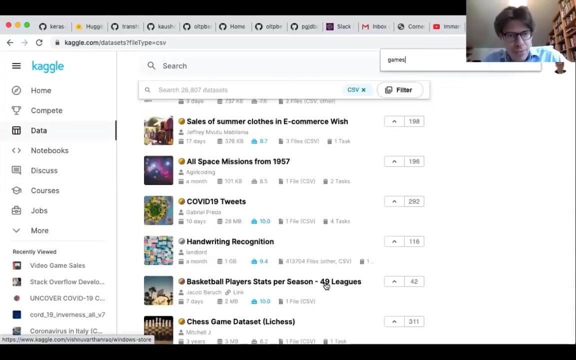 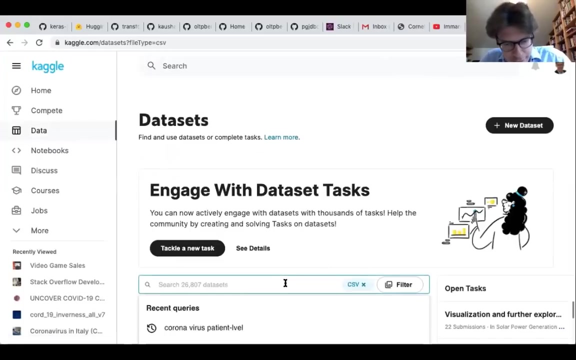 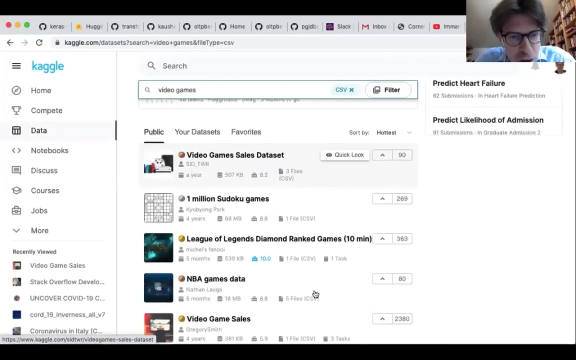 seems to be. it's a light problem with the interface here. okay, all right now. I spotted on a slide, but it's not true. there is a lot to pleaur actually. let me just sort this out. we, just before the lecture, I spotted a data set that I wanted to use for this demonstration, and here. it is All right. that is a data set about video game sales and we're going to use it. going to run a couple of simple twisting Investor rein. ¡'re modest insight E Certes our data is that we are going to take ask of our reforms and it is products over and over again. there has been a doublehedged lobbying agreement in here so that it's first thing, because if we go and see how many people actually want an emergency bitty economy. 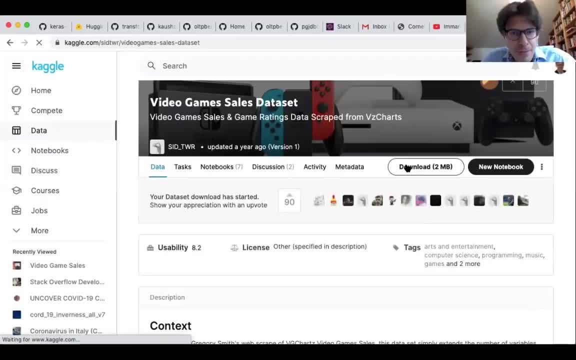 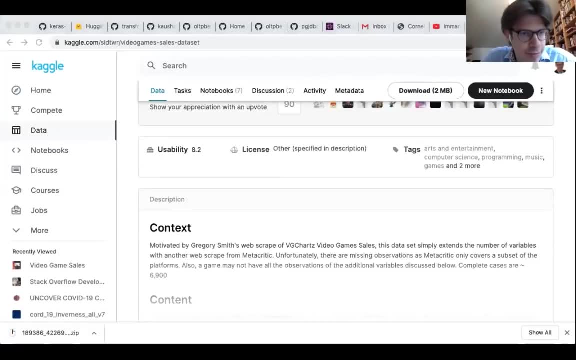 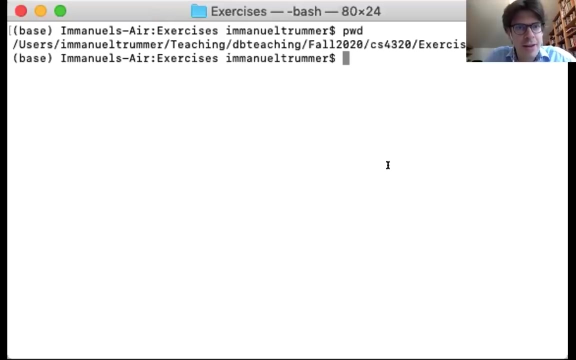 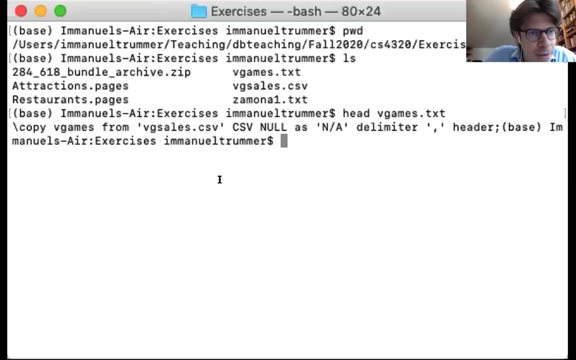 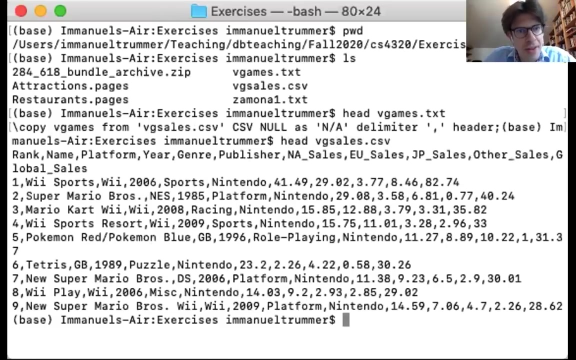 Here, not the corresponding data. all right, we have downloaded it. now i'm copying that's data. here you can see my console and the data set, um that we are looking at. it looks like you see here. so we basically we have values separated by comma term, the first row of the data set that you. 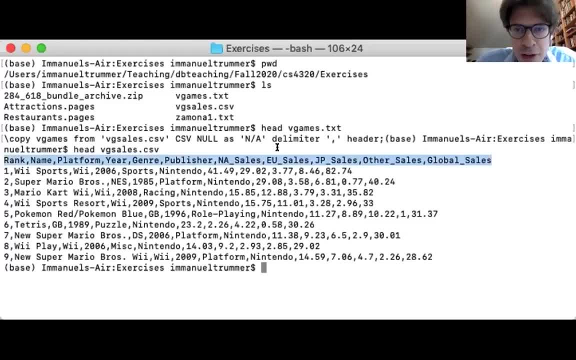 see here. that is essentially the um- the headers of the different columns, and after that you have the associated data set that you see here. that is essentially the um- the headers, associated data rows. so i just want to guide you through the um analysis of one simple data set, um. so after we downloaded it. 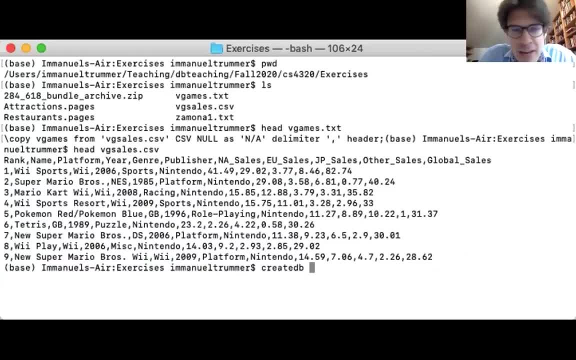 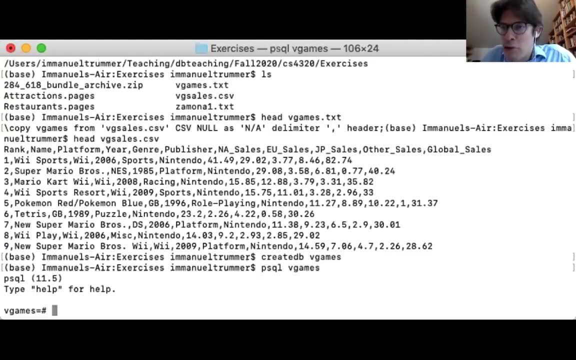 we want to create a database in order to import the data um. so, for instance, we can create this database over here. now we log into the database, and so the first thing that we would do in order to end the analysis of such a data set is to create a table in order to 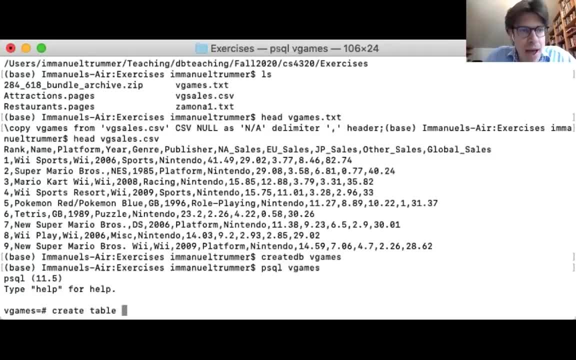 import the data, and we have already seen the command for that. so let's create this table over here. um, we have the columns that we want in the table, essentially given in this, uh, in this file over here. so, for instance, here we first of all have a sales rank which is apparently of type integer. then we have 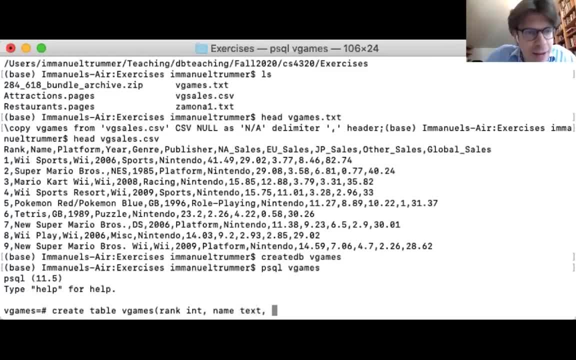 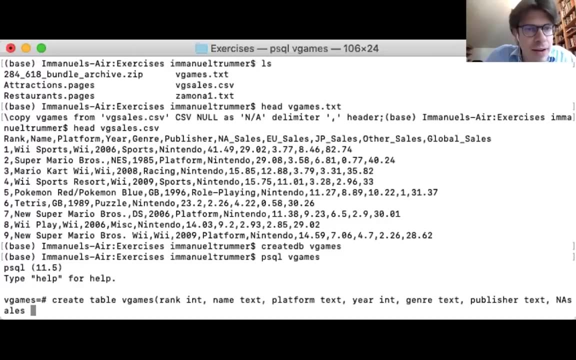 a game name which is of type text. it seems there's the platform of type text, the year of type, integer game. genre of type text. the publisher: um, then first sales column, which seems to be of type numeric sales. in the new, this is in millions of units, by the way. um, that is. 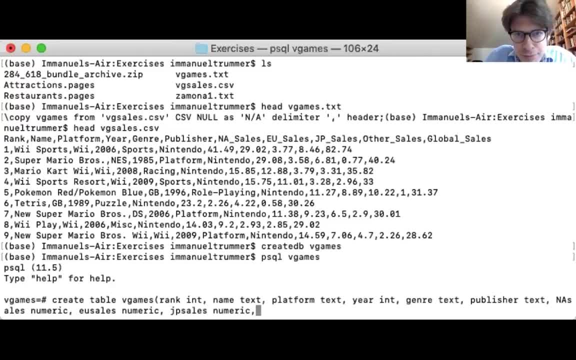 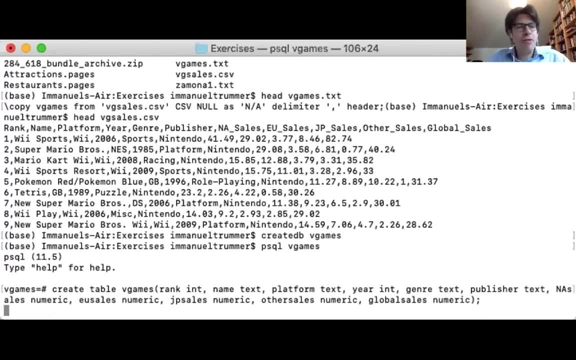 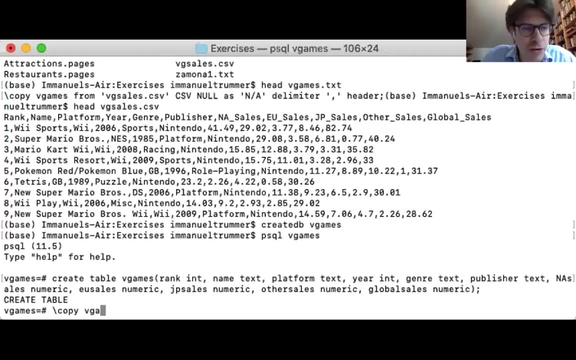 also numeric sales in japan. all right, and now we have created this, a table into which we want to import the data, and we have already seen the command for that. so if i want to import the data from a file, um, i simply write this copy command with the name of the table. 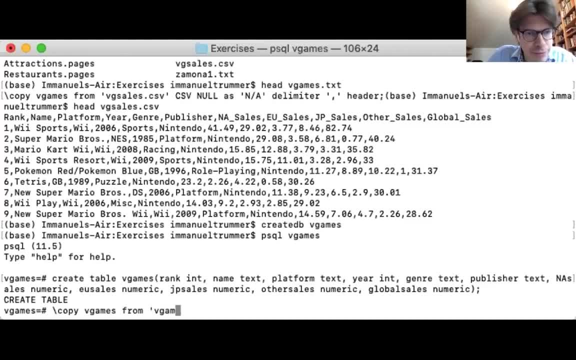 and then the name of the file, which is vg salescsv. now we are telling the database that here we want to import a csv file and, um, we tell database that values are separated by comma type, could be a different character and um, what you also often want to specify is how those uh, null values that we will 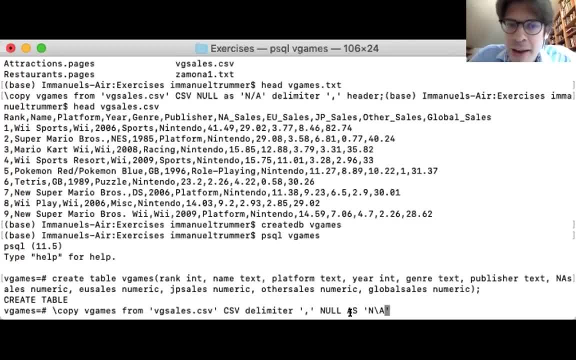 talk more about today. null value essentially means a value that is unspecified, and you need to know how those null values are specified and then you need to tell the database about it. i believe in this data set it should be one. null value should be represented as n and a. 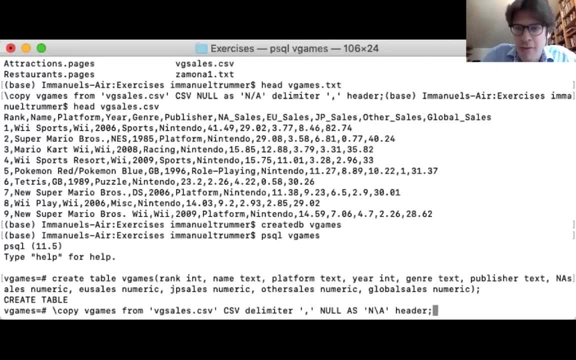 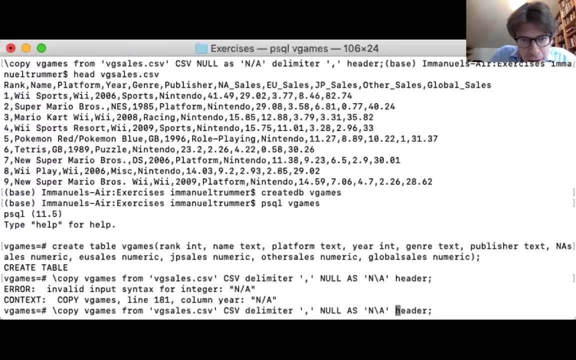 and also here we have one header row and that is also important for the database management system to know. so i'm writing, uh that here and now let's load that data into the table and i think maybe the main, which now values, are represented. it might be this way around with the backslash. 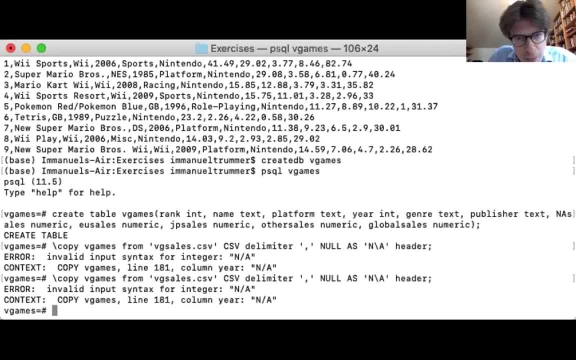 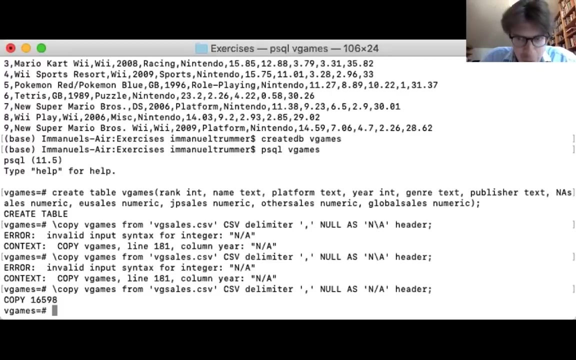 um, let me quickly check there, all right. all right, so that was the right representation for the null values. i got it wrong. um, now we have loaded the data. the database management system tells us that we have loaded about 17 000 rows, and if we want to first of all inspect what we have just 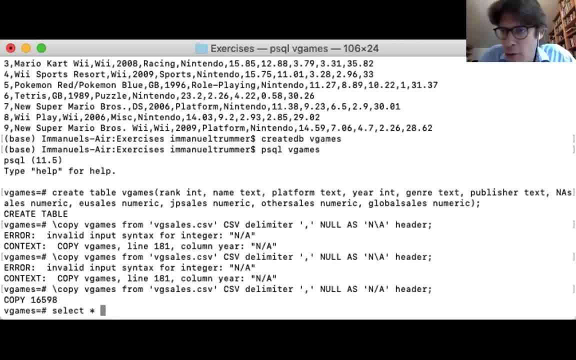 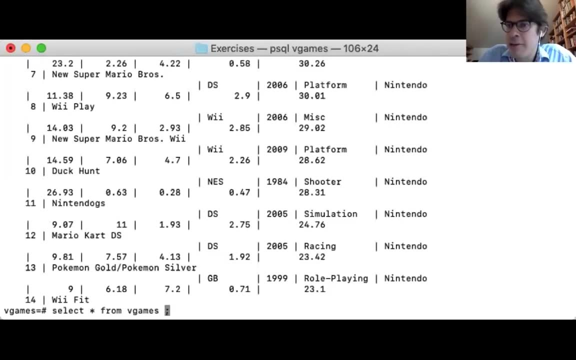 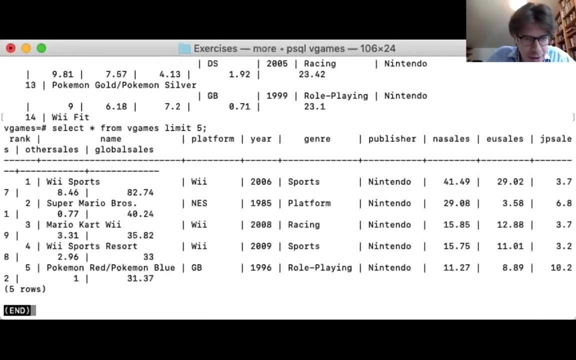 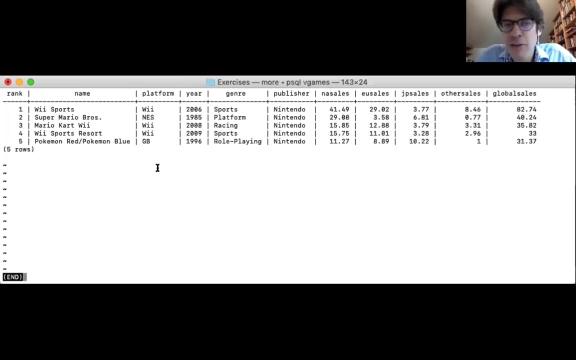 loaded. we would write something like select all columns from that table and loading all the rows. that can be a little bit too much data. so 羽 Tuning, absolutely all right, that is kind of what we would expect, and then we would end this like this. so first i did express everything. one small new feature that i wanted to introduce today, that is the limit clause. Gotta Limit Clause, which works by specifying how many rows you want to show in the result of a query server. write this, then i get a much more reasonable output and on first view that looks okay. let me quickly increase the size of this window a little bit, then it becomes easier to see. so just a quick increase in the size of this window a little bit, then it becomes easier to see. so, all right, this seems to be a data we got more use of. we got to anxious. 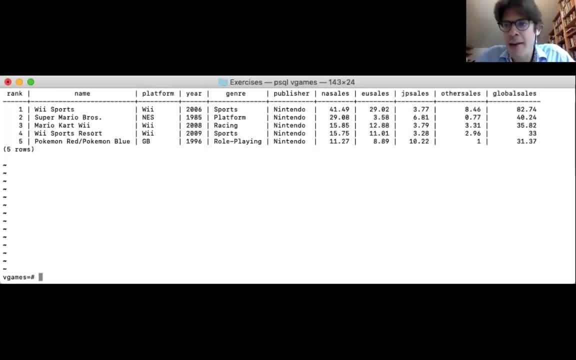 but I wanted to load everything. fine, All right. and now, the last time, we have seen different queries for aggregation and grouping and so on. So now I can perhaps apply some of that to this data set over here, perhaps the first thing that I might be generally interested in. 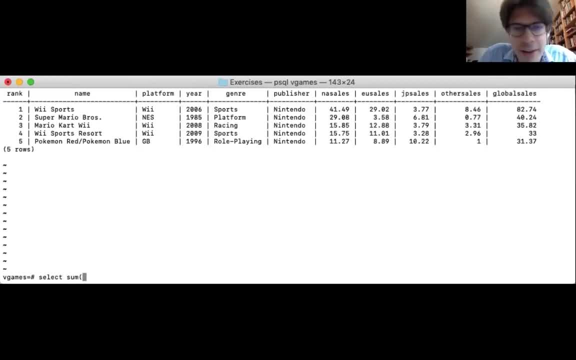 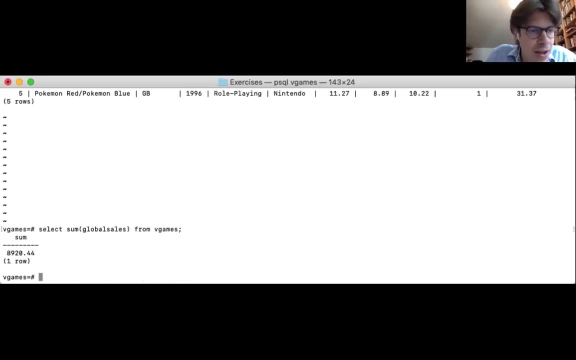 is how many of those games people sell in total, And I could express this as a query where I'm summing over the global sales of those games, And the data source is, of course, still the VGames table. Now, if I do this, then I find that in total, 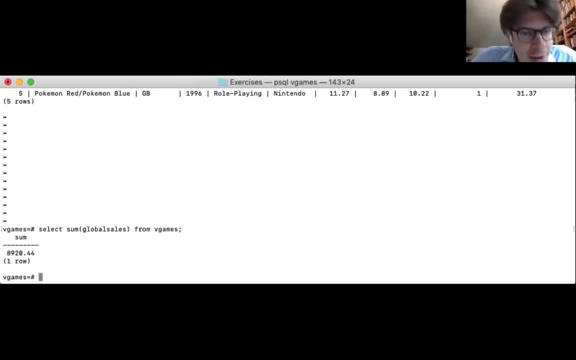 about 900 billion units are sold here. That is interesting, but perhaps I want to make it a little bit more precise. I want to break down those sales into different categories, And you can do this exactly with the group by query that we have seen last time. 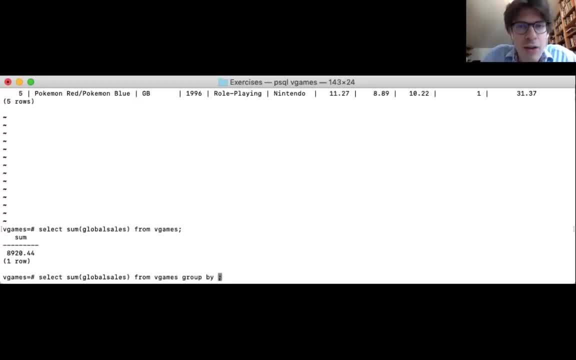 So perhaps what I want you to do here is that I group by the genre in order to see which types of games sell better than others, And if I do this, then that's not gonna be very useful here. If I do this, then essentially just would get the numbers. 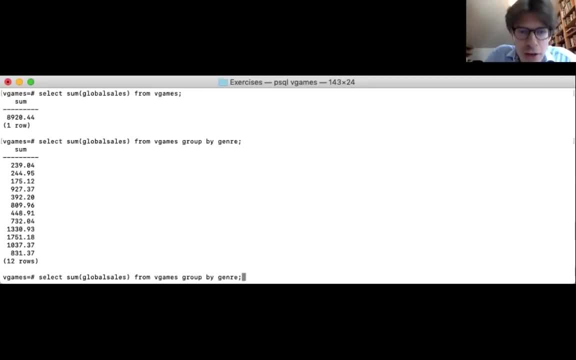 here, but I wouldn't get which genres those numbers are associated with. So what I probably want to do is that I also put the genre into the select course here. All right, and here I have the different categories Of games, with the number of units sold in millions. 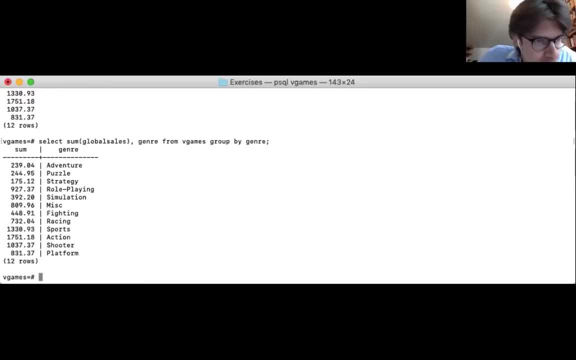 And, yeah, it seems that certain categories of games there are significantly more popular than others. Particular sports and action games seems to be quite popular. All right now. another thing that I could do is to group those games, for instance by the platform. 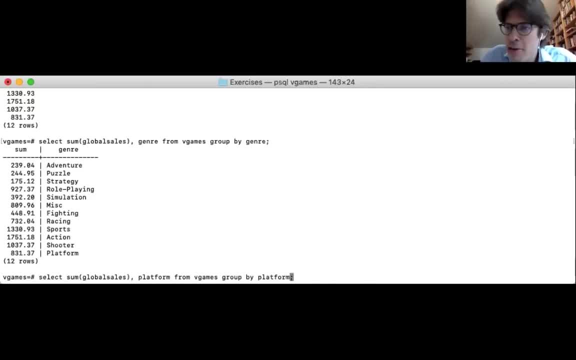 for which they have been produced, And I want to you know how many units have been sold for different platforms, So I can do this. like you see here. Perhaps this is a little bit more data than I actually wanted. I see there's like data for 31 platforms. 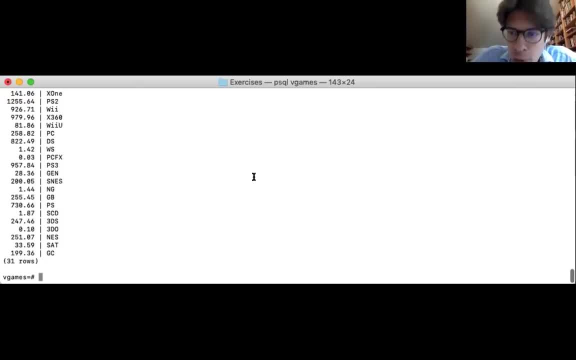 And maybe I want to focus more on the important ones. And here there is a great question. in the chat Somebody is proposing to order them And you can absolutely do this, And that is the second feature that I wanted to introduce. All right, let's see. 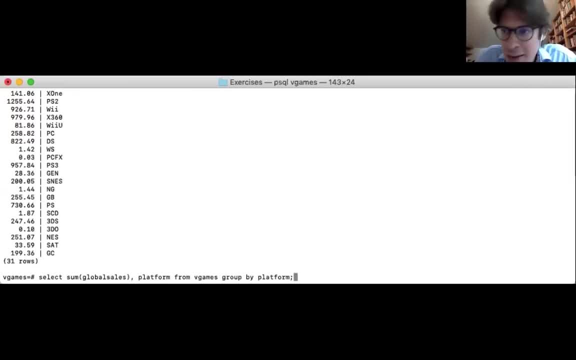 Let's see what I can introduce today. Let me do this in a second. For the moment, I wanted to propose a different solution to how I can reduce the number of platforms for which I retrieve data. For instance, here I could introduce account statement. 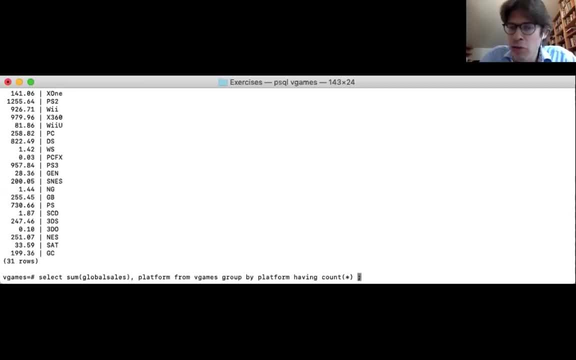 And only retrieve data for those platforms where the number of titlers is above a certain threshold. Now here, essentially, since we use the group by clause, this query is grouping data by the platform, So one group is defined by one specific platform. 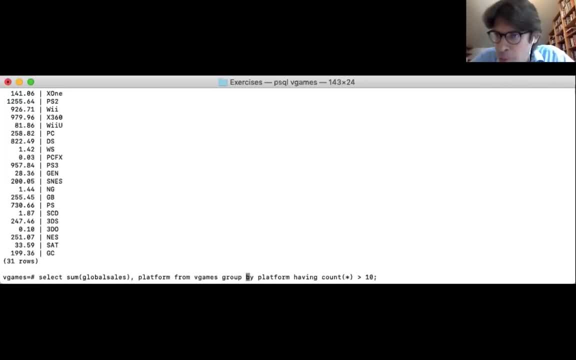 And if I want to narrow it down to platforms that have certain properties, that is a condition on the groups. So I must put that condition into the having clause. And now let's experiment a little bit. For instance, if I set this threshold that might 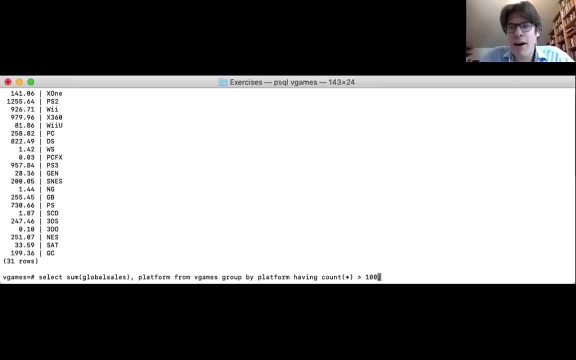 be too restrictive, But here, essentially, I narrow it down to platforms for which we have at least over 100 titles. All right, and now this narrows it down already quite a bit, from 31 to 20 rows. Maybe I can narrow it down even further. 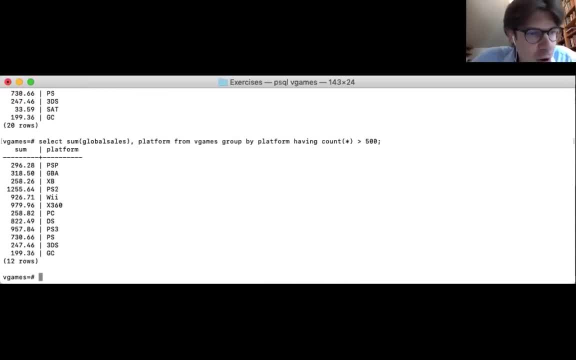 to only the most common platforms. Yes, and now we have only relatively common platforms, So that is how I can narrow down things, by the different possibilities that I have to think about. So the next thing I want to do is to know what the results look like for each of the platforms. 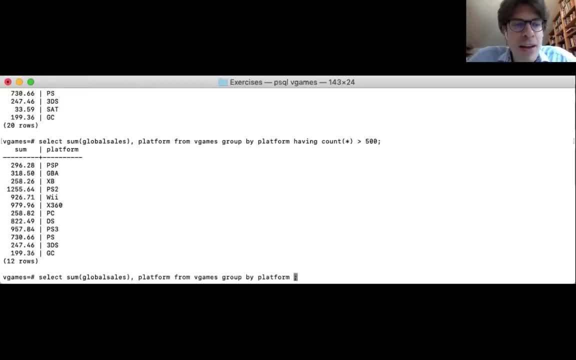 And the answer to that would be to order things. So, instead of using this conditional to prune out groups associated with platforms that are less commonly used, I could also say that I simply order the results by the number of sales, for instance, And then I would know where in the result to look. 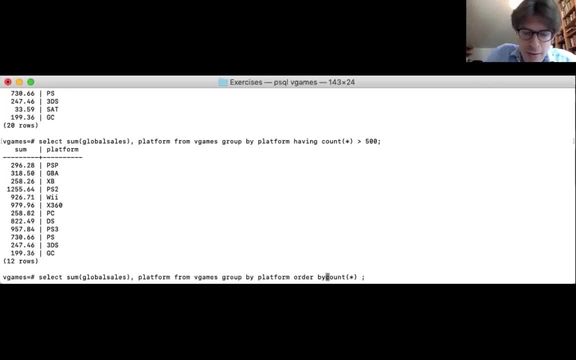 for those platforms that sell more titles. So here, for instance, I could also read the results of these platforms right order by count, and I want to order in ascending order. so I'm putting this ask abbreviation here. so if you do this then, as you see, here I tend to get the 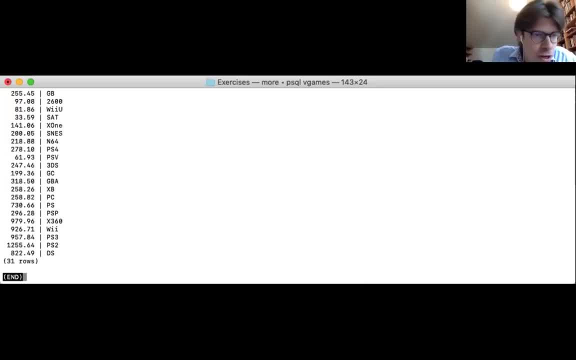 platforms that have more titles and are also associated with more sales: more units old rather later in the query, and if I want to get them first instead, then I can use the desk keyword instead. so yeah, now we are starting with those platforms for which attempt to have more titles and as opposed to the count here, 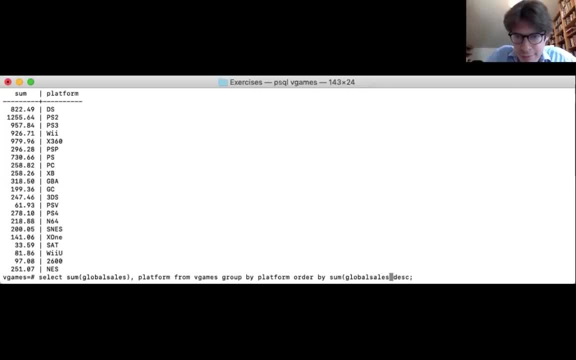 I could also use the sum again, and now I will get first those platforms for which I have lots of global sales, and here another proposition is whether it wouldn't be better to first to first sort and then to limit the number of output rows. right, you can also do this. 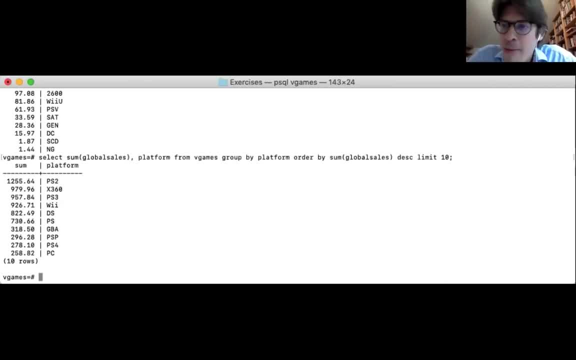 and that works perfectly. that is a good suggestion. so here I'm first sorting and then later I'm narrowing it down to only the most common platforms. so the advantage of this one over the query with the having cost that I used before is that with the having clause I have to decide what kind of threshold I should set, and a purely I 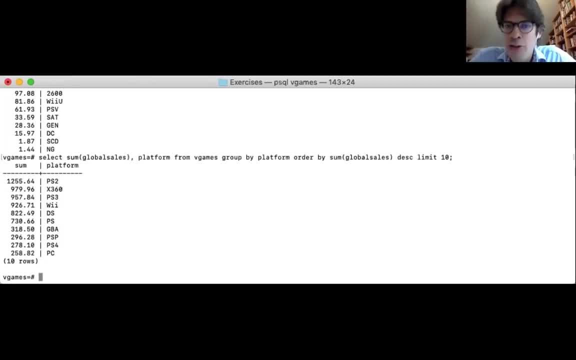 might not know what makes a good threshold. so if I want to narrow it down to a fixed number of rows at most, then this type of query- here we are first sought by something and then a limit to something that is probably preferable. all right, and here is a couple of questions, and so 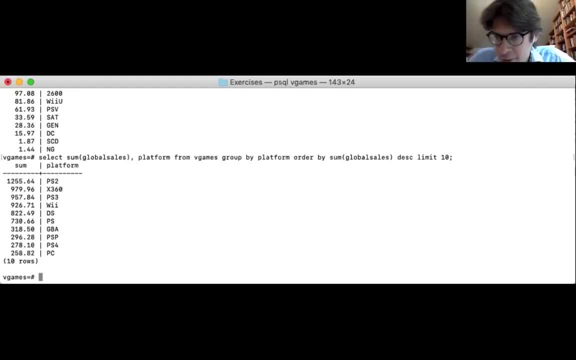 the limit clause is applied at the very end. that was a question here, and people have also posted a link to the data set. thanks, that is the correct one and the best- версion is positive because relat aspect is how to vary theotted data set. contar secondны is because it is. 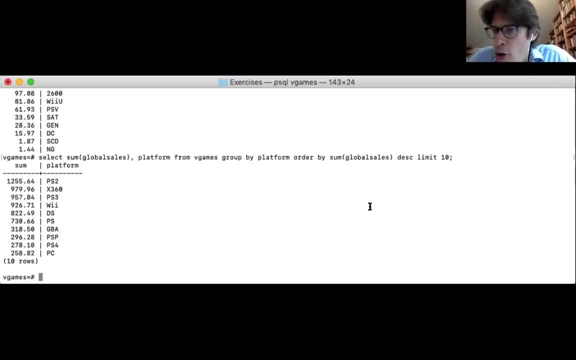 booklet, but do like which order you're talking about. how do you fun through it? and width, because at the very end it's been listed over an actual quantity of data. there is a block here for over a day using the second order flow method- lots of choice and cackle- or on similar websites. 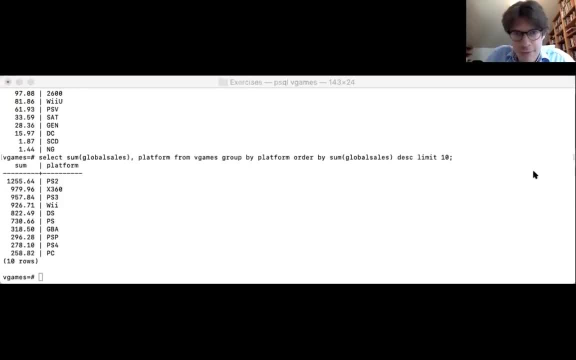 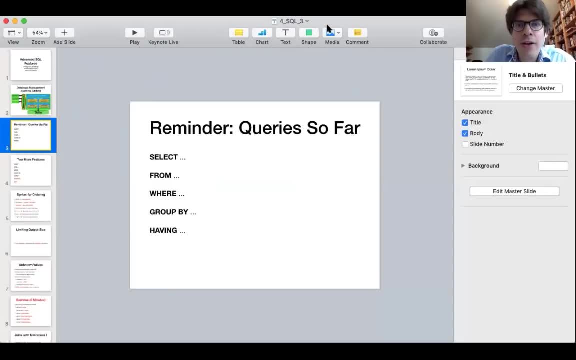 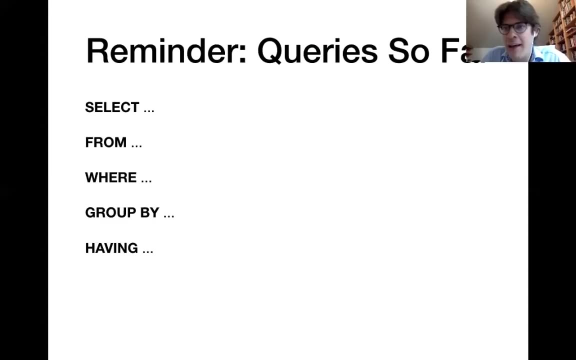 all right now you should be able to see my slides again. all right, so we have started with a reminder for the type of queries that we have seen last time and we have applied that. we have also added two new features now. the first feature that we added is: 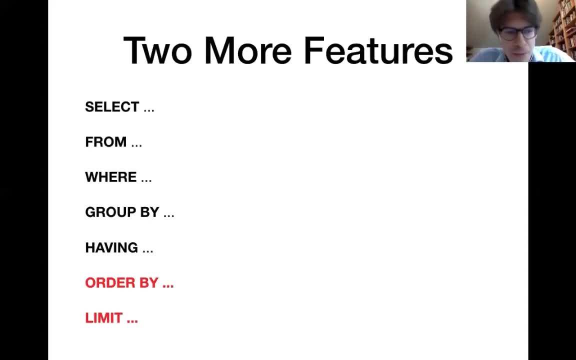 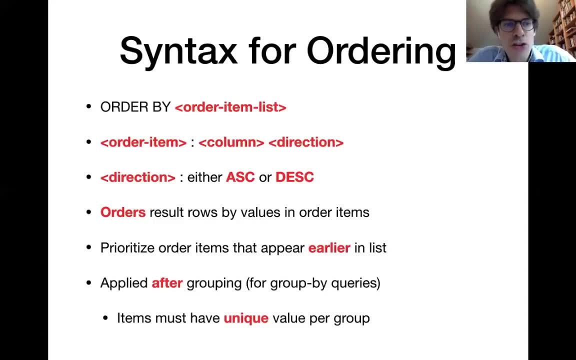 the order by clause and then we added the limit clause. i have already demonstrated how that works, but here is a little bit more details about the syntax. so the order by clause- and as you see it comes after the having clause- is right now with the other wePartnLOB, so the order by clause comes. 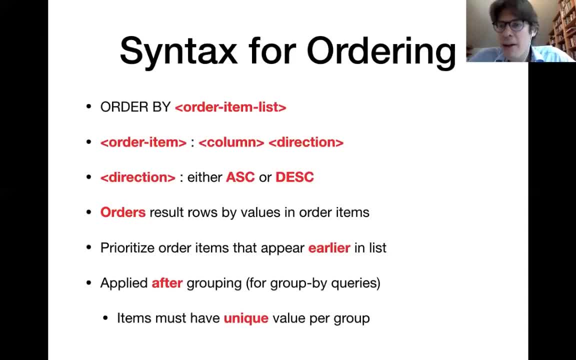 if you have any. The order by clause allows you to specify a list of order items, and each order item consists of a column according to which you want to sort and a sorting direction, which can be ascending or descending. Now this statement ensures that the output of your query is sorted by those columns. 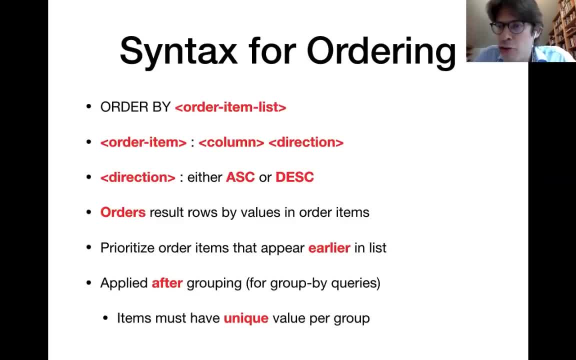 that you specify here. So in order to determine the sorting order between different reside rows, the database management system, we first look at the first order item that appears in your order by clause, and then, for those rows which have the same value in the first order by item, if we look at the second, 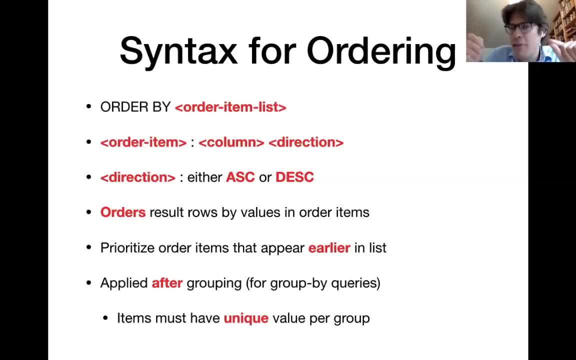 order by item and solve by that, and if it also has the same value there, then it will look at the third one, and so on. So the priority for sorting is on the items that appear earlier in your order by clause, And there was some question about in which order things are applied. 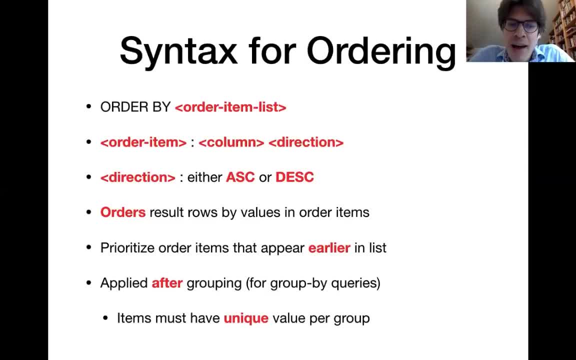 in general For the order by clause, it is applied after the wear condition, for instance, is evaluated and also after grouping has happened. And that is important because if you have a group by query, then into the order by clause you can only put columns that are guaranteed. 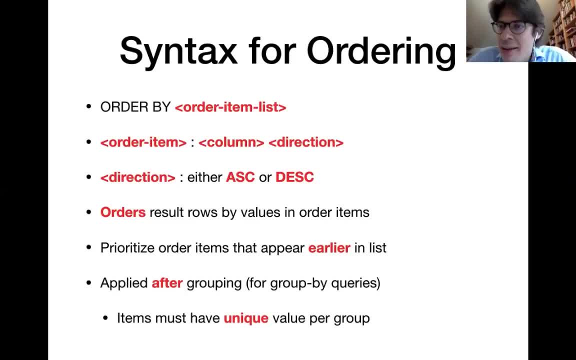 to have the same value for any group. So basically you can only use a columns in the order by clause where all rows in the same group are guaranteed to have the same value. And that means that as long as we're talking about columns, those essentially must be columns that appear also. 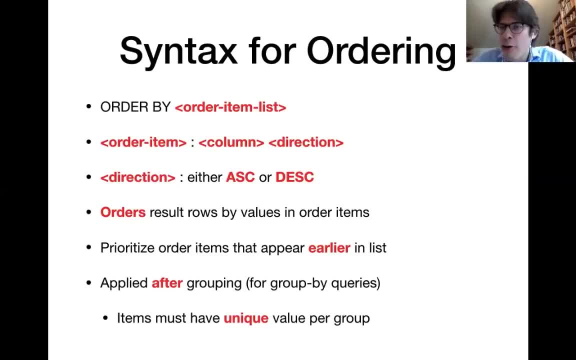 in the group by clause, because if a column appears in a group, by clause it is guaranteed that all rows in a group have the same value for that column, because that column is used in order to define groups. so this is a bit similar to the restrictions that we had for the exact clause. 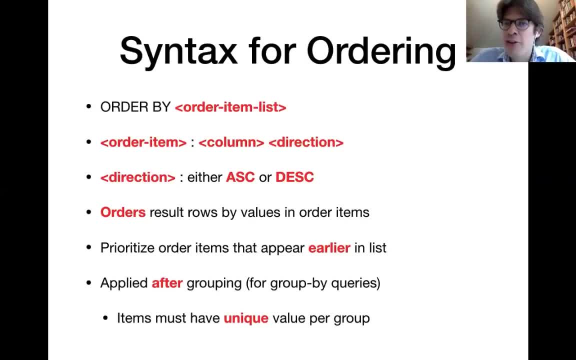 once we have a group by query, then there's also certain constraints on what you can put into the select clause. you can also only put columns into the select clause, for instance, that are guaranteed to have the same value for all rows within a group, and that also means that in practice, 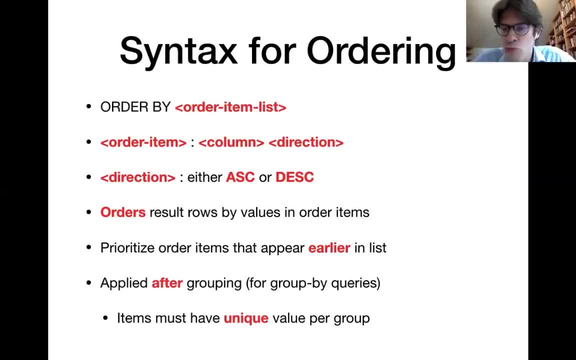 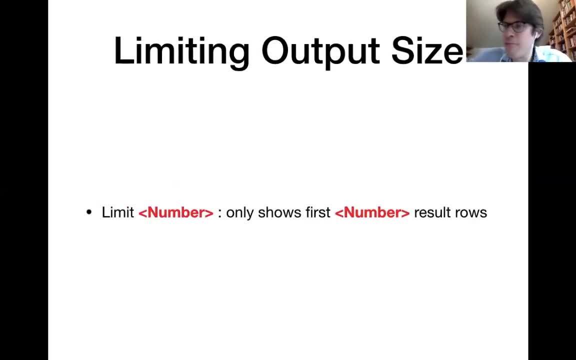 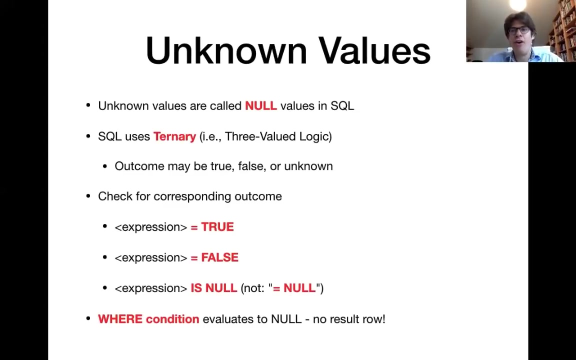 we want to restrict it to columns that appear in the group by call- all right now, the limit operator. that is a pretty intuitive. I simply give the database system the maximum number of results rows and then this limit toss is applied at the very end of query evaluation. all right now. in a following we're gonna discuss more and more. 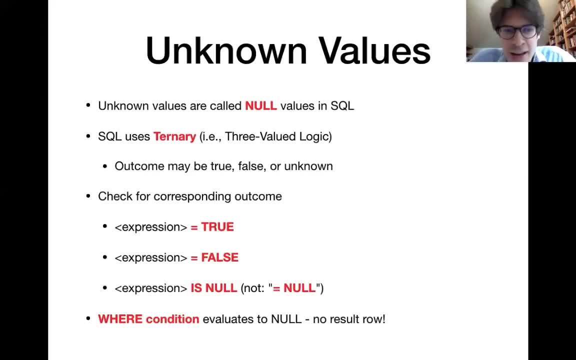 advanced features of SQL queries. first of all, I want to discuss a little bit more about null values now. we have already quickly mentioned null values a couple of times. another in SQL simply means a value that is currently unspecified, for instance, because it is unknown now those null values for. 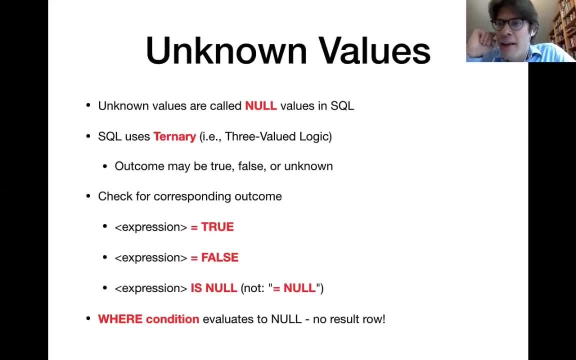 instance, influence the way in which SQL evaluates boolean conditions. typically, you would think of those boolean conditions as evaluated as non-evaluable values, but that's not the case in the case of SQL, which you that you true or false. but if one of those conditions contains, 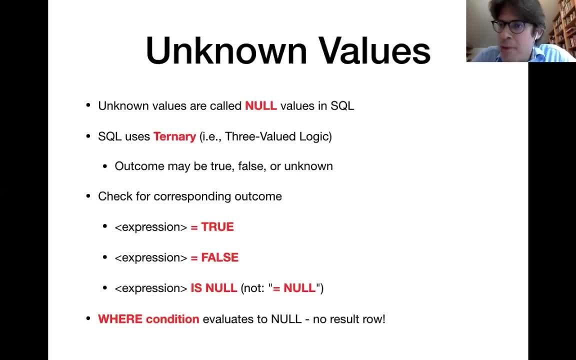 contains now value, then the overall result of the expression could also be unknown, and we will see a couple of more concrete examples for that in the following. now this is how you can essentially check for the evaluation result of one of those Boolean expressions. You can check whether it is true or whether it is. 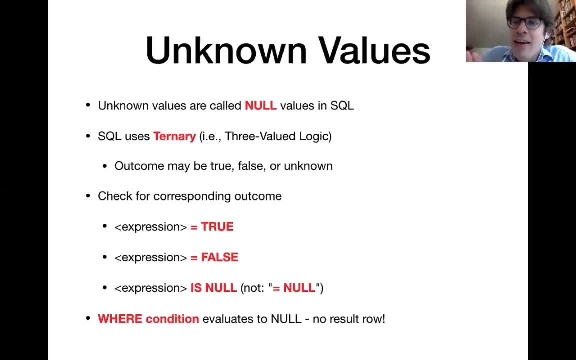 false, Careful. if you want to check whether the evaluation result is null, whether the evaluation result is unknown, you cannot simply write equal to null, but you need to write is null in order to check for that. And then, if you have any rows in your data, that where the condition in the 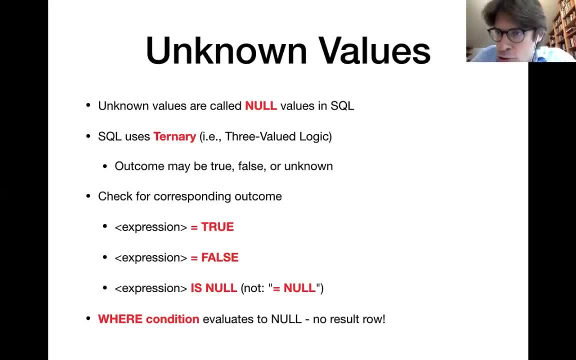 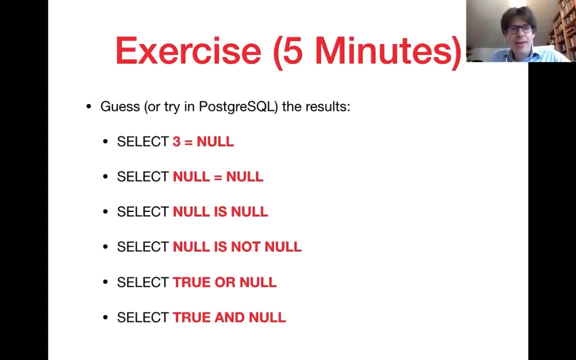 where clause, for instance, whether it's true, null as opposed to true, then those rows will not be contained in your query result. Now let's make a couple of concrete examples. I encourage you to try out at least some of those examples, either in your local Postgres installation or using the 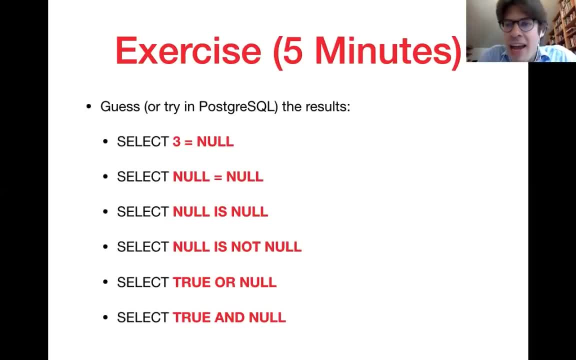 website that I have shown you last time, which doesn't require any local setup- Perhaps the first one. we can do it together. If we have a query of the form that you see here, where we want to know whether 3 equals null, does anyone have propositions for what the result of this query could be? 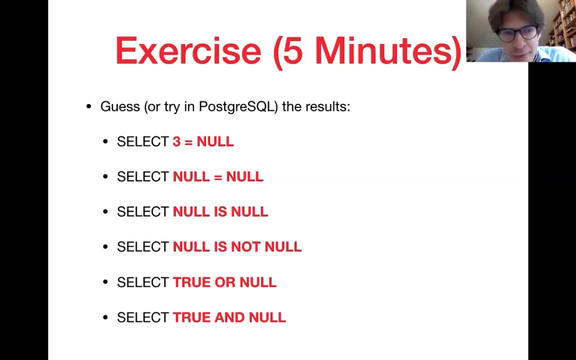 Syntactic error. Okay, That would be one possibility. It's a little bit more permissive than that actually. Okay, there's different propositions, Null empty. Okay, So does anyone want to explain in the chat, please? why do you think, for instance, that the 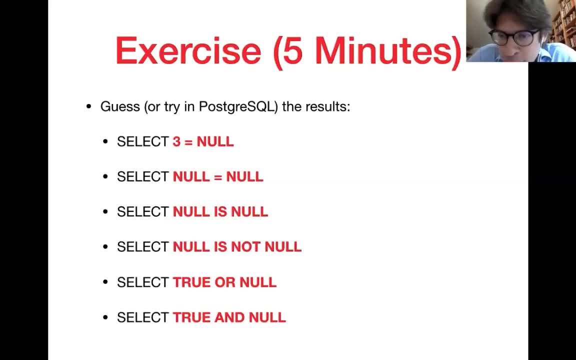 results could be syntactic error. Okay, So does anyone want to explain in the chat please, why do you think, for instance, that the results could be syntactic error? Okay, So does anyone want to explain in the chat, please, why do you think, for instance, that the results could be syntactic error? 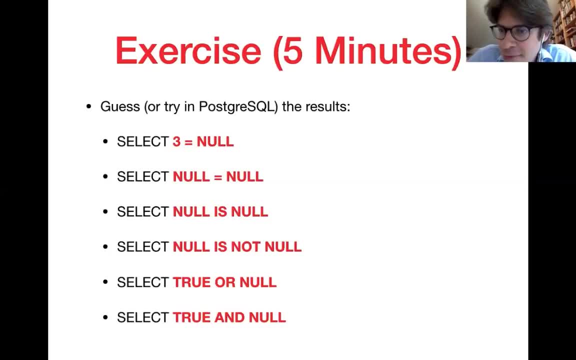 Or why the result could be null, for instance. Okay, Perhaps typing out an explanation like that it takes a little bit more time, So let me resolve that. So the correct answer here would actually be 0.. Okay, Perhaps typing out an explanation like that it takes a little bit more time, So let me resolve that. 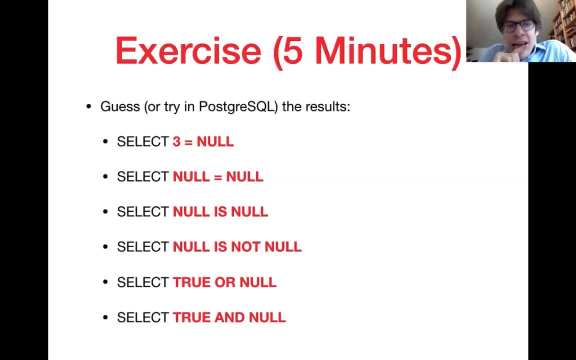 So the correct answer here would actually be 0.. would actually be null, And I expected that perhaps some people write false as a proposition, but that has not happened. I guess one could at first view think that the result here could be false because I have an equality condition and I have different things on the left side of it. 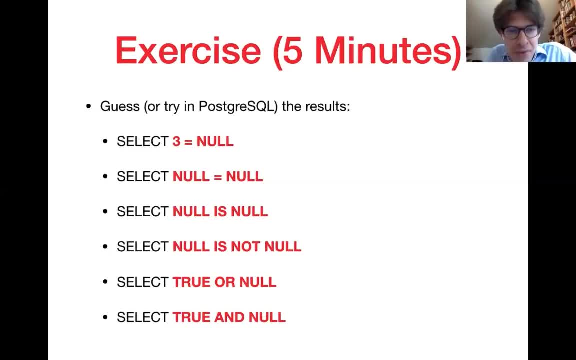 and on the right side of it. Now the problem is this: Those null values represent an unknown value, so they are placeholders, so to speak. That means if I write a 3 equals null, it essentially asks whether 3 is equal to some unspecified placeholder. But the placeholder 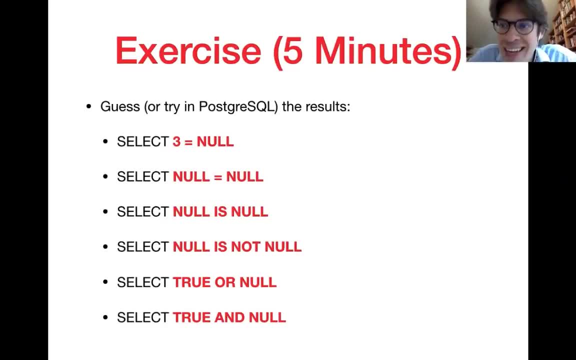 as it is unspecified, we cannot be 100% sure that it isn't 3 by coincidence. So here I'm essentially asking whether 3 equals to some unknown value, and whether that is the case depends on that unknown value. And since we cannot decide whether this is true or false, the answer: 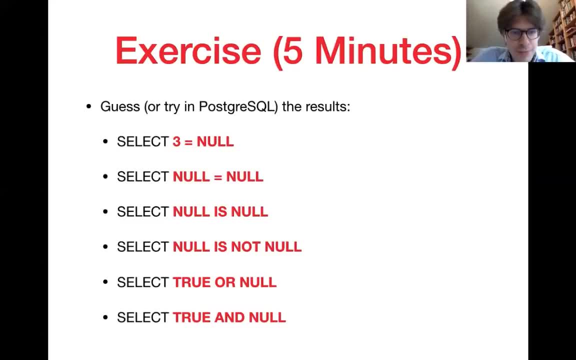 to this query would indeed be null. Okay, and there's a couple of other examples here. Yeah, and somebody is posting how that looks like in Postgres into the chat. So those null values, in Postgres they're just represented as empty spaces. So here you have one row, but you don't see. 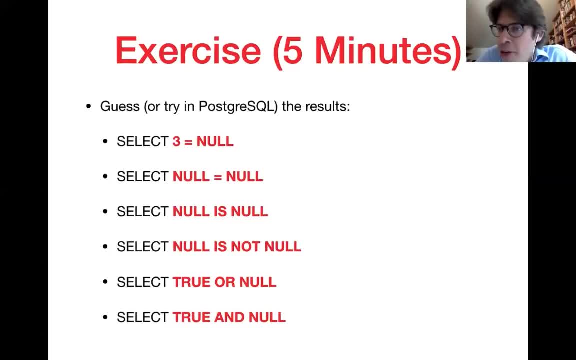 any content, and that's because this row only contains one null values, So null isn't a value like in other languages like Java. So there is some differences between a Java null value and a SQL null value And, in particular, you couldn't perform certain operations with Java. 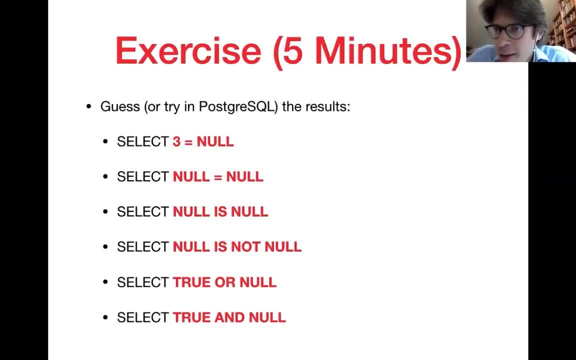 null values because at some point you might get an exception, a null pointer exception- from the Java system. So here in SQL, in principle you can use null values wherever you can use other values as well. The only thing is that if you have a null value somewhere, it might mean. 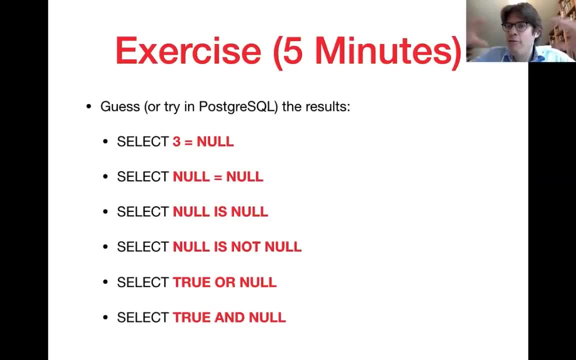 that if the null value is contained within one expression, it might make the result of the entire expression unknown, meaning null in the end as well, And null is false in this case. so that depends on which case you are referring to. So, in some cases, if you are referring to the semantics, if you have a method of downloading, then null value is even false in this case. Well, it's just also true in SEO, right? So I guess I just have one question before we get to some of these questions, And the answer is: if we can recover the null value and we use, so, we're doing at least one. 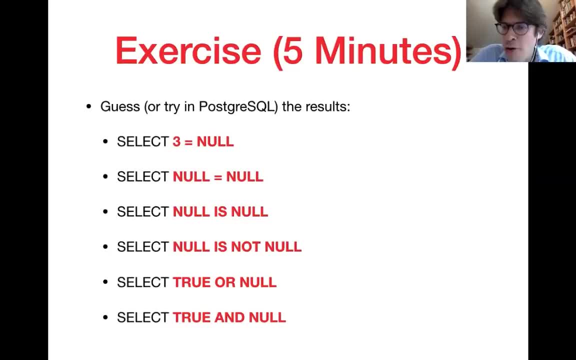 sort of automatic Honeycomb question from Jill daemon of free SERVICE. Okay, Um huh, if we have a null value as a result in the where clause for one specific row, then I fully agree. having a null there is treated in the same way as if the result had been false. So if the 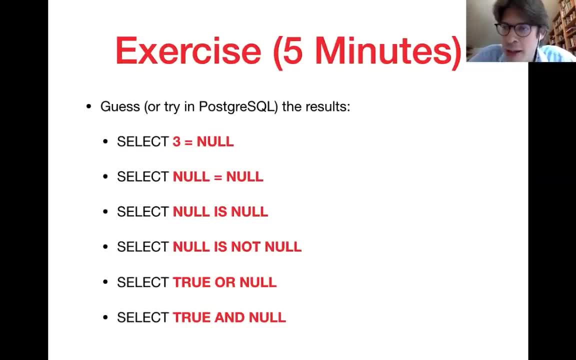 entire condition in the where clause evaluates to null, then the corresponding row will not be included into the query result. All right, So okay. so now, maybe you had a little bit of time to try out some of those examples. I believe it is relatively quick to try because you don't need to type a lot, And 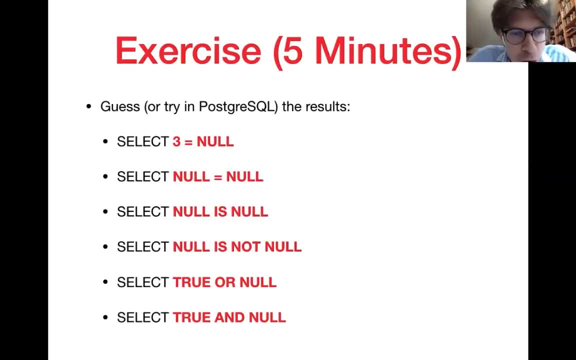 yes, so we have already discussed about the first one. The second one is also null as a result, because we are essentially asking: is one first unknown value the same as one second unknown value? And of course, that depends on the unknown value. The third query: null is null. That is always true. because is null is? 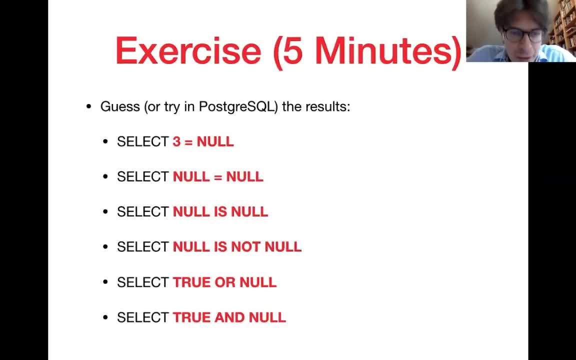 checking whether something is unknown, and in this case it is indeed unknown. The next query is the opposite of that and therefore false. Now perhaps the last two queries are still interesting. We have true or null, and in this expression we do have a null value appearing. However, an or expression is. 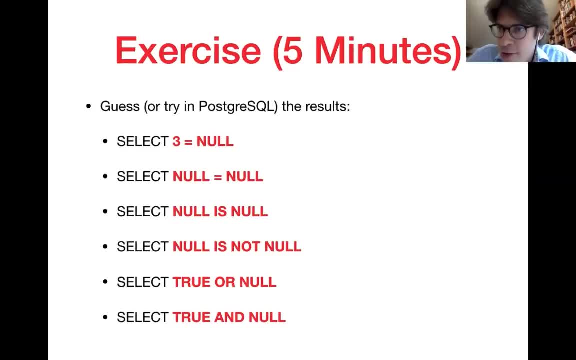 true as soon as at least one of the components is true, And in this case, one of the components definitely is true. Therefore, the end result does not really depend on the unknown value and therefore the end result of this should also be true On the other side. for the last query, we have true and null. 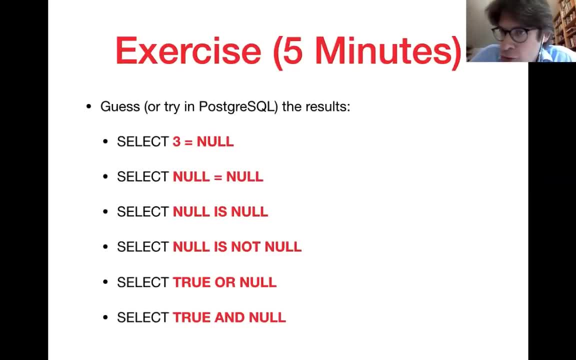 That means if the unknown value is also true, it makes the entire expression true. But if the unknown value is false, it makes the entire expression false. So the result depends on the unknown value and therefore the result is also unknown. So this is what is called SQL's ternary logic, because all 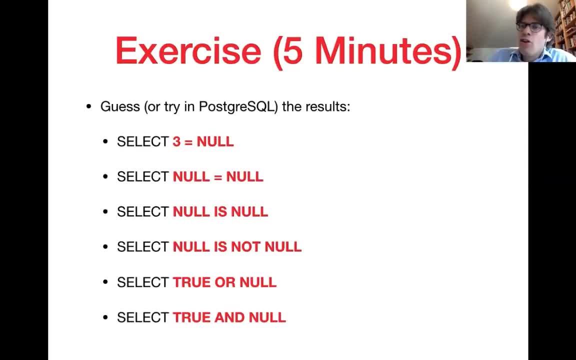 logical expressions can have a three-result values- true, false and unknown- And the question is: what should select? null is null due if the predicate is true. So this query, frankly, is not very useful, admittedly. So this is just for the sake of an example. In practice. 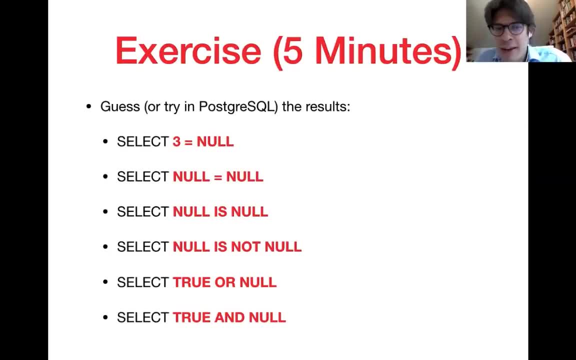 this query. it's not interesting. It essentially has a constant result, right? And, by the way, also note that here we are not using any data source in order to calculate the result of our query, So we don't have a FROM clause. Depending on the database management system, some of them disallow that You always need a FROM clause. 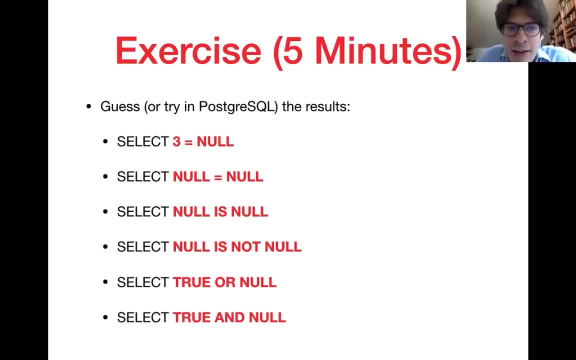 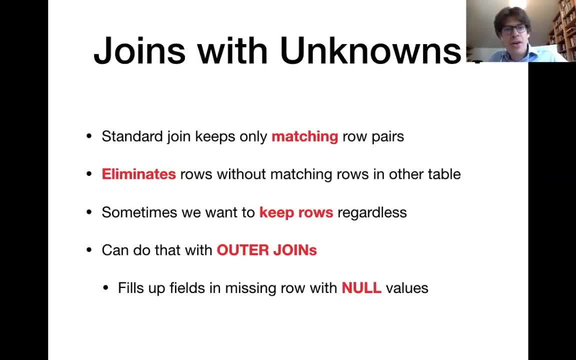 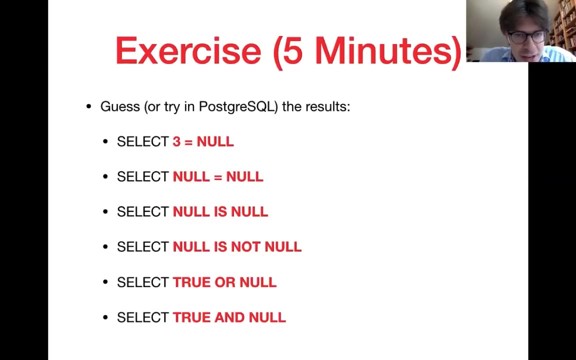 But in Postgres you can write queries like that that do not depend on only data in your database, but just evaluate constant expressions. All right Now. and the IS keyword? Quick question here. still So, the IS keyword. it is a more precise expression. 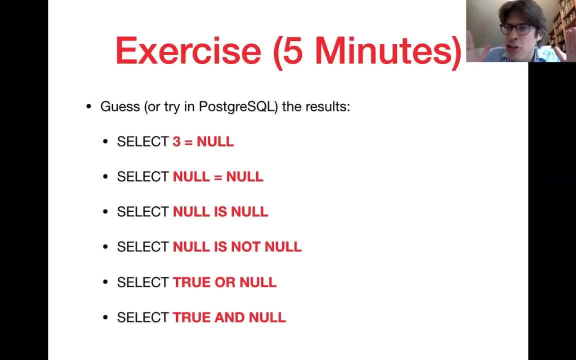 It is actually the ISNULL expression. So that essentially checks whether the expression on the left hand side of it evaluates to null or not, And it is true only if the left hand expression evaluates to null. So null equals, null is null, but null is null. that is true. 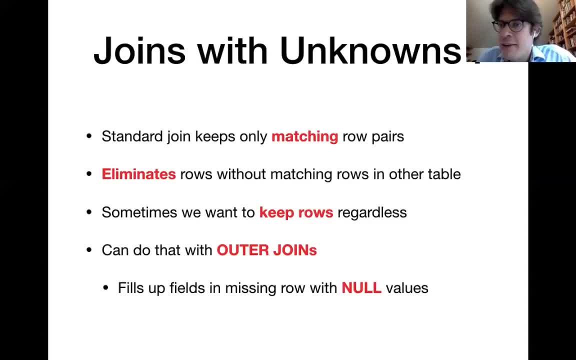 All right. So it is basically not only the single IS keyword, but it is ISNULL, that is, a fixed command. Both words together, All right. So now that we have discussed in more detail about null values, we can discuss more about some. 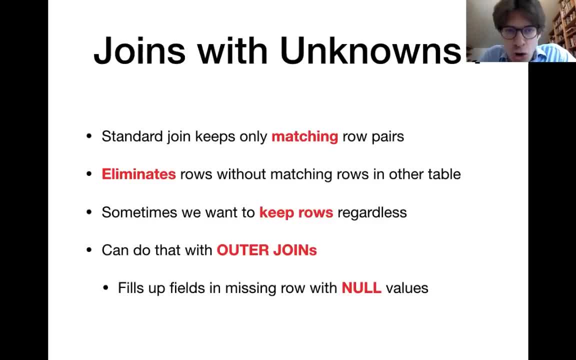 extended variants of the join. So far we have been looking at joins that essentially retrieve pairs of rows from two tables that match together, meaning that they satisfy some kind of join conditions. For instance, we have seen the example where I'm pairing up the students with the 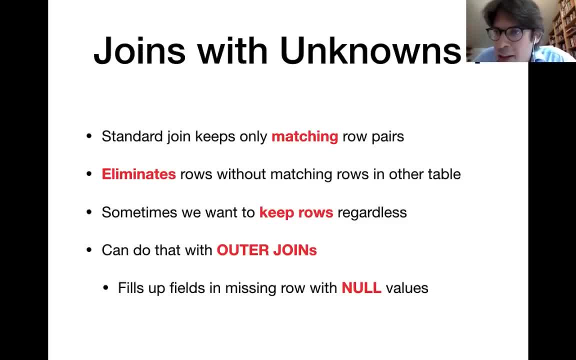 enrollment information for the courses that they are enrolled in, and I'm always matching together those rows which have the same student ID. Now, one problem with that is that it eliminates rows in a table which don't find any matches in the other table. Those rows will not appear in the join result. 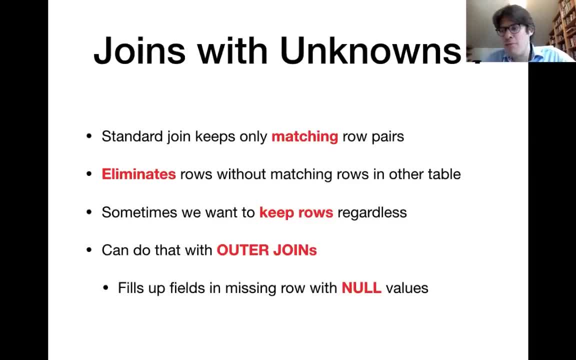 So if I'm, for instance, joining students with enrollment information, then a student who hasn't enrolled into any courses yet will not appear in the join result at all, And this is not what I want. in some cases, Perhaps I want to, for instance, encourage students to enroll for courses who have not enrolled yet. 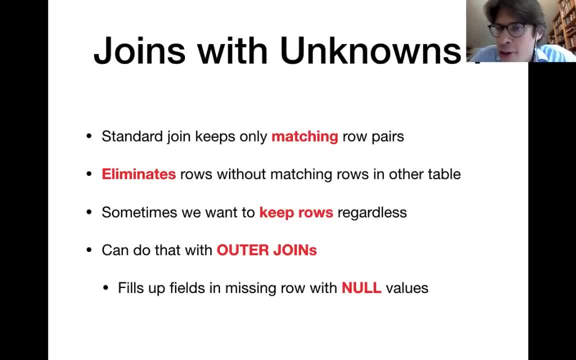 But in order to do that, I first of all need to make sure that those students remain in the join result, such that I can see that they haven't enrolled in any courses yet. And SQL offers you some specialized syntax in order to make sure that the result of a join 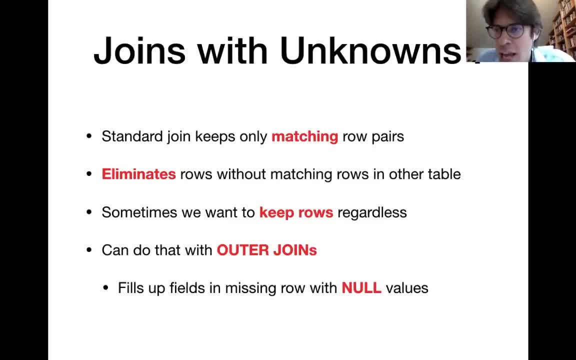 keeps all the rows that appear in the input tables, Even those rows which do not have any matching rows in the other table, And that is called an outer join. Now, for instance, for students and enrollment, the recirculation of the join between students and enrollment. 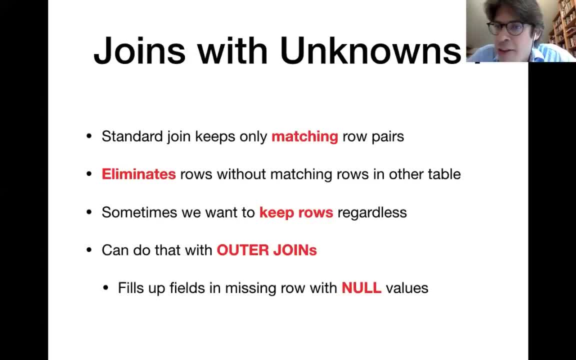 contains columns for the student ID, for instance, but also columns for the course ID for the enrollment. And the question is: if you want to keep those students without enrollment in our join result, what should we fill in as values for the course ID column? 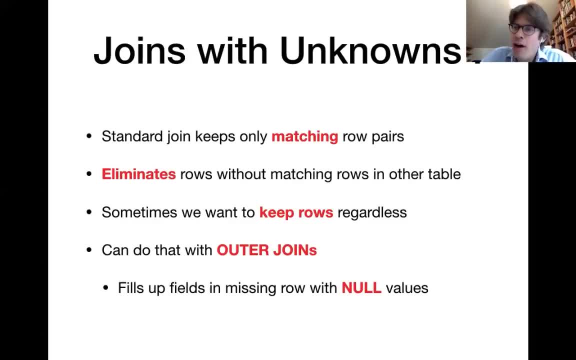 And this is where null values come into play, because those outer joins will fill in the values for rows without matching rows in the other tables. They will fill in those missing values with null values again. So if you have those students who haven't enrolled into any courses yet, 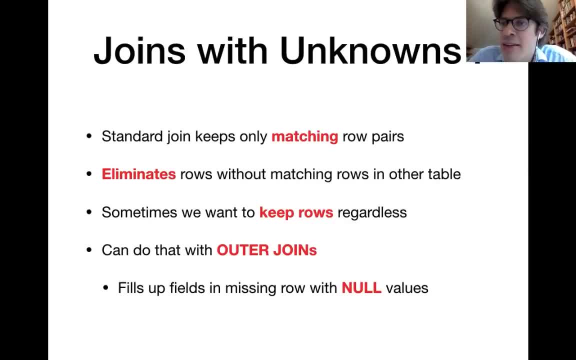 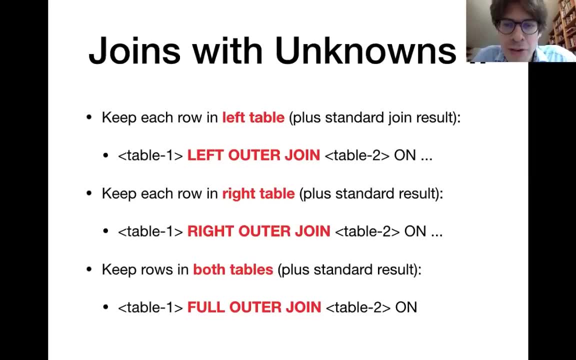 then the course ID and the corresponding join result will be set to the null value. This is the syntax that you can use here. You can write in the from clause of the query: some first table left outer join. some second table on some join condition. 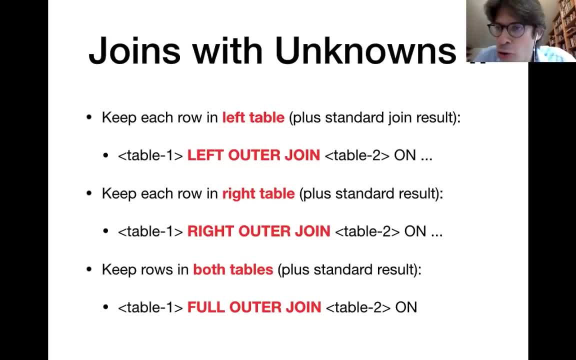 And that is guaranteed to keep all the rows of the table on the left side of this join. There's also the complement, the right outer join, where we say that all the rows on the right hand side of the table are kept in the join result. 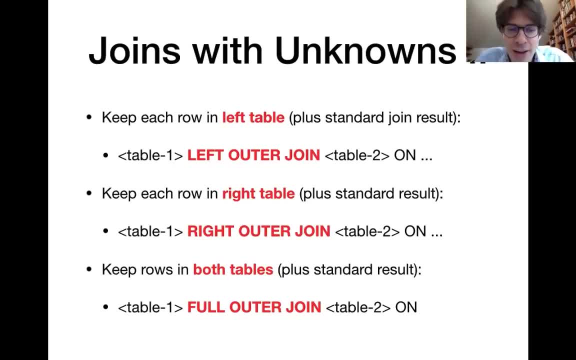 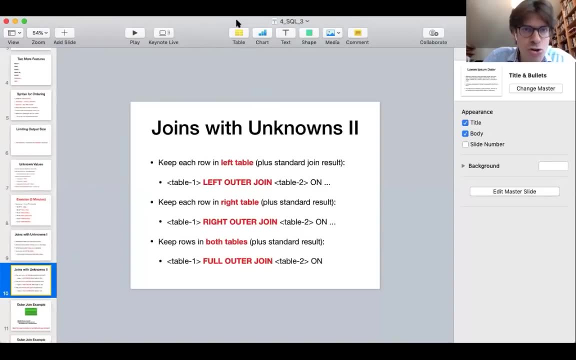 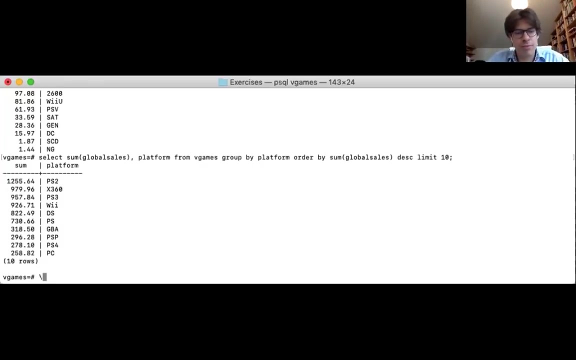 And if you're interested in keeping the values, the rows for both tables, you can also use the so-called full outer join And very quickly I'm going to show that to you. So if we have, for instance, So if you log into the university database where we have those tables with students, courses and enrollment, 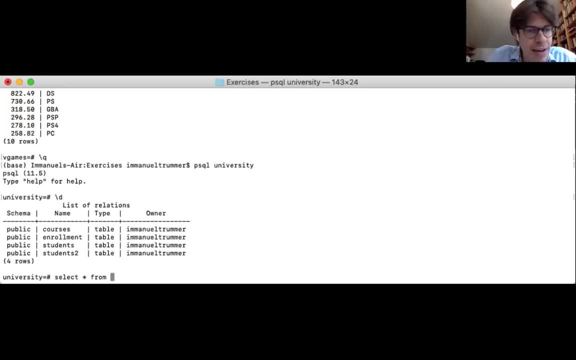 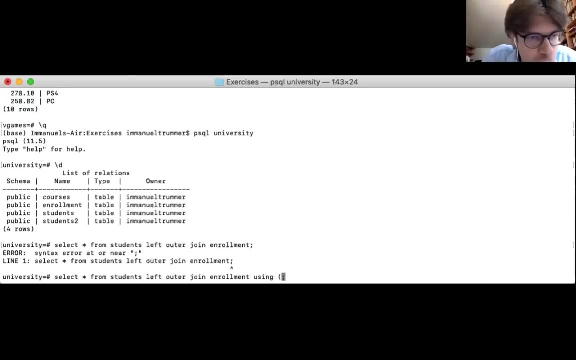 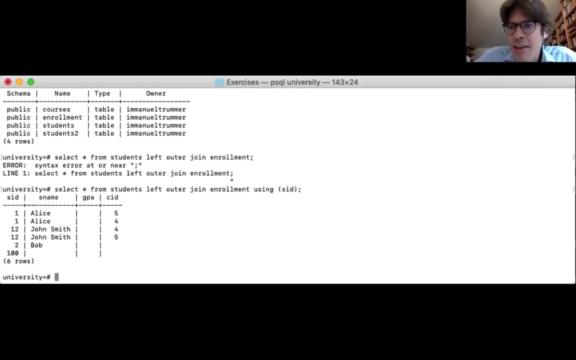 then we can for instance select all columns from the students, For example the topics, So that says left outer join with the enrollment information, And here I should still add the join condition which is on the student ID. And here you see the result of this join. 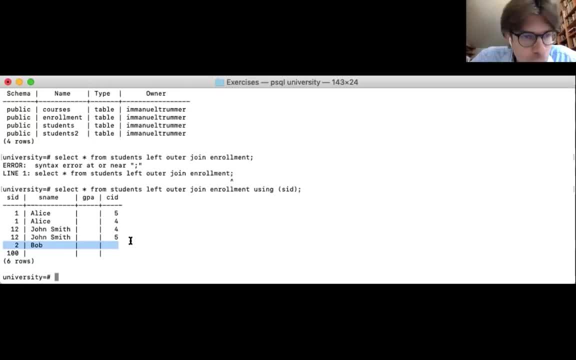 Now here, for instance, a student Bob. that is why the course ID is left empty in Postgres and that always indicates a null value Here. by the way, I had also inserted before a student with unspecified a student name, so that's why here we have the student ID for that. 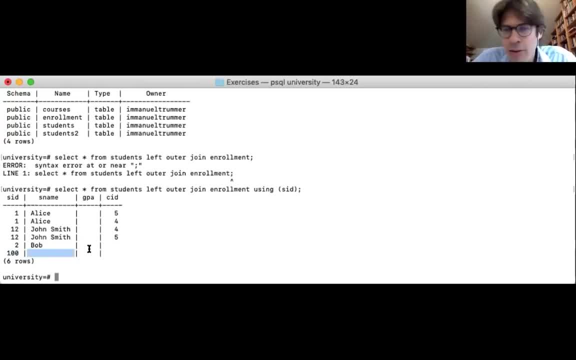 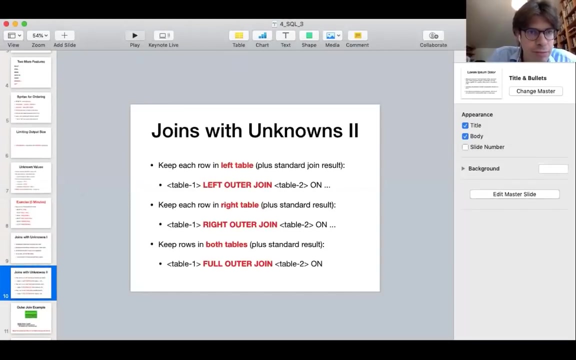 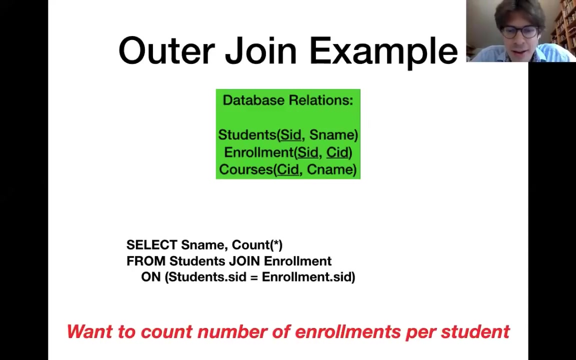 student, but the name has not been assigned yet, and also that student has not been enrolled in any courses. that is why we have empty fields here as well. So this is how the results to an outer join looks like in Postgres. Now back to the slides here. So let's also see a little example here in the 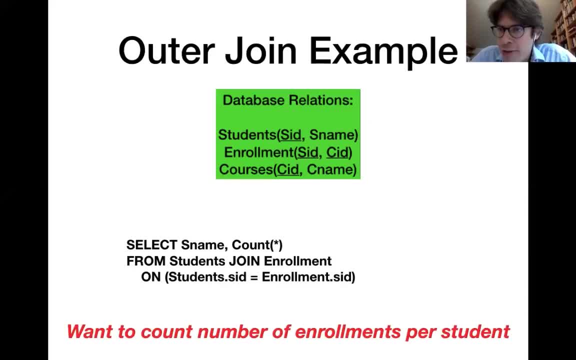 slides, One thing that I might want to do, for instance- I mean especially. for instance, I want to remind students we have not enrolled in any courses yet, that we have not enrolled in any courses yet, that we have not enrolled in any courses yet. what I want to do is perhaps to count the number of enrollments for each. 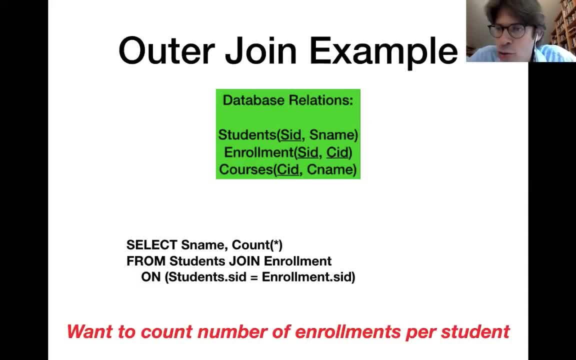 student and in the following we will see how we can do that with an outer join. So here, for the moment, we are using the same database that we have used in the previous lectures of students with enrollment information and courses and, as you see, for the moment you're not using any outer join, we are using a. 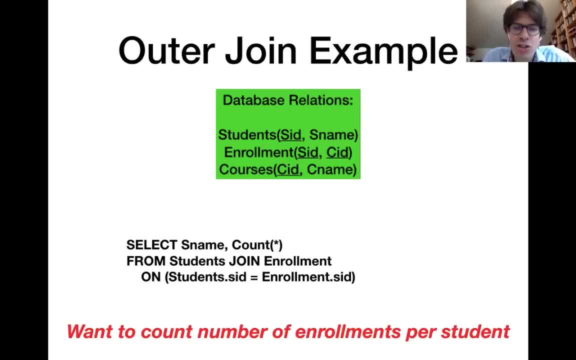 standard join, And that means that students without any enrollment would be filtered out by this query, which is not what we want. So already we probably want to replace this join by a left outer join that is guaranteed to keep information about each student. but now the problem is that we have currently- we are currently- 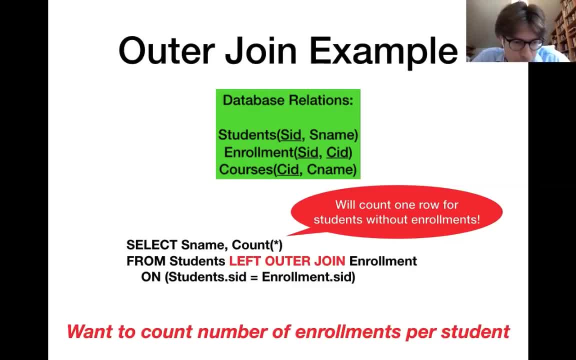 using a counter statement and I just see that some group by statement in this query has been left. so here I actually want to add a group by statement for the corresponding query. so that unfortunately has dropped. So here we want to group by by the student name. 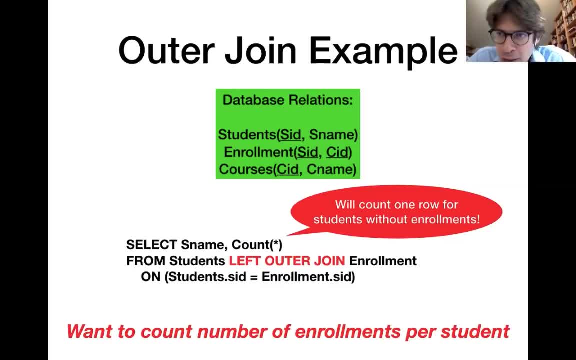 In order to count the number of enrollments for each student, and the problem that we still have here is that, for the moment, we are counting the number of reside rows. that means, for those students for which we don't find any matching enrollment information, we will still count a one reside row for those. 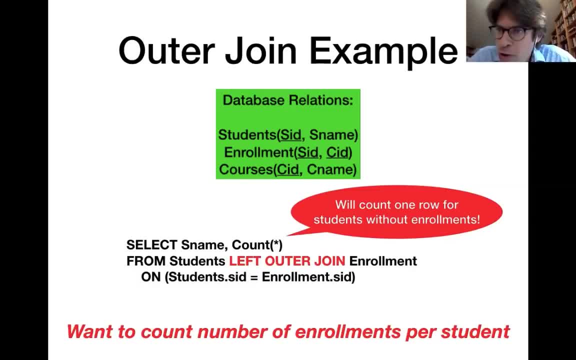 students, which is not what we want, because for those students, we want to count zero enrollments. So the last thing that we need to do in order to make this work is that we replace the count star, which counts any reside row, by count C ID, which only 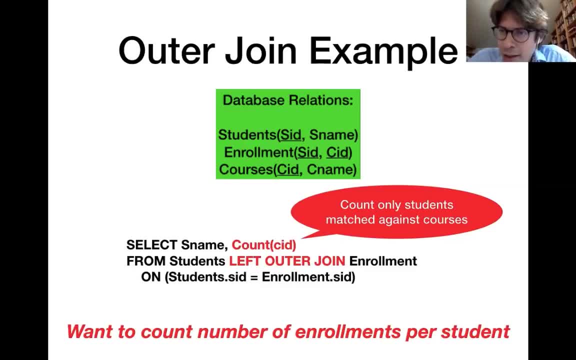 counts those reside rows that have a non null- meaning a noun- value in the count star course ID column. So if a student doesn't have any associated enrollment information then after the outer join that student will have null values in the course ID column. And if we use 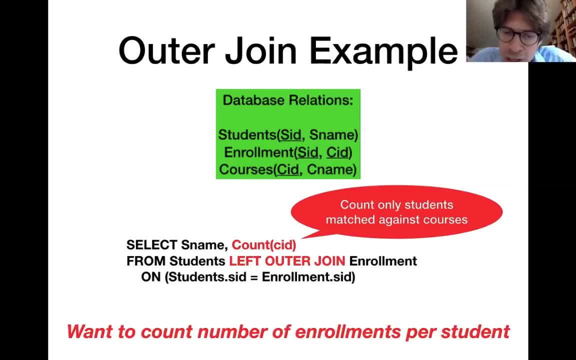 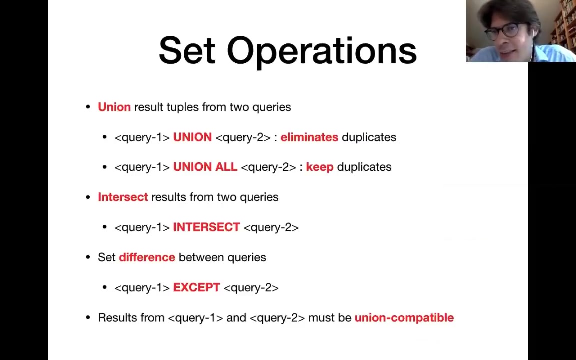 this counting variant. then those rows with null value for the course ID will not get counted, So I will get a count of a zero for those students who have no enrollments yet. All right, So this is some useful join syntax that, in practice, every once in a while you might need some of that. I'm. 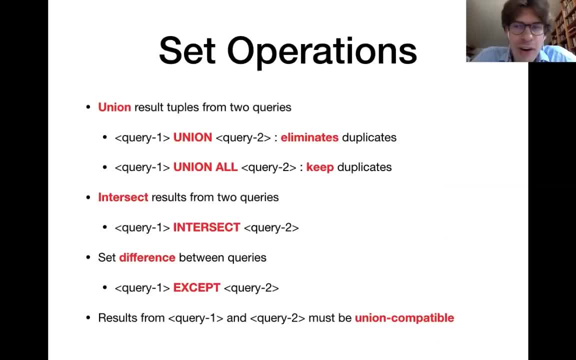 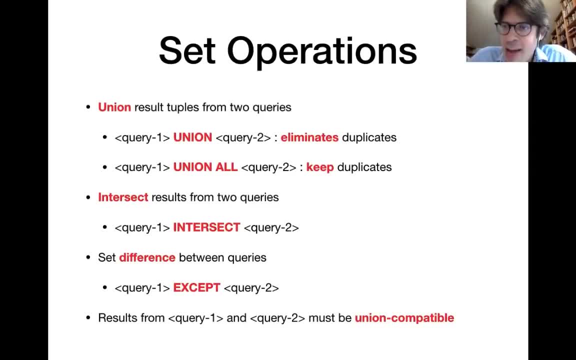 in the following we're going to look at some examples. So in this video we're going to look at a little bit more advanced SQL features. and one powerful feature of SQL is that you can write queries which combine multiple other queries together, So you can essentially write composite queries that essentially combine. 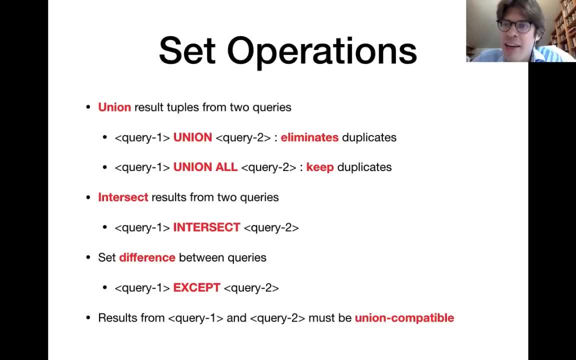 multiple smaller secret queries in one way or in another one. And the easiest way probably of is with the sql set operations. so if you have a result of the queries then, for instance, sometimes you might want to take a union of the result of two queries and with sql you can do this using. 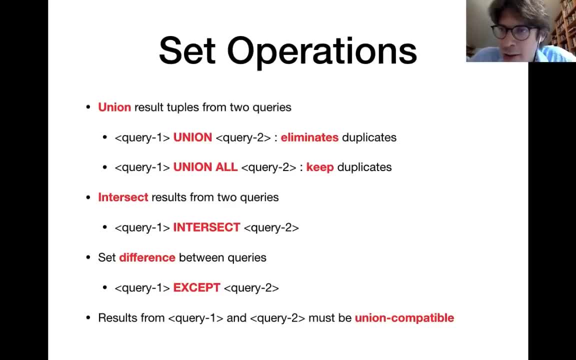 the union or union, all keywords, and essentially here, um, in this specification, uh, query one, query two refers to a queries, for instance, like the ones that we have seen so far, but then you can compose them, using the union keyword, for instance, into a larger query and the result of that query is: 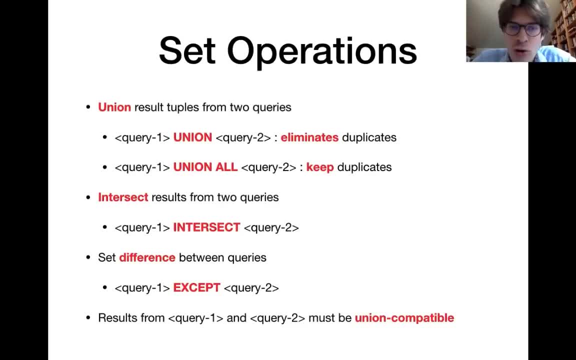 essentially the union of the results of the two contained queries. what is important here is that those two queries, query one and query two, they must be compatible, meaning that their results have the same structure, so it has to have the same number of columns and also the same column types. 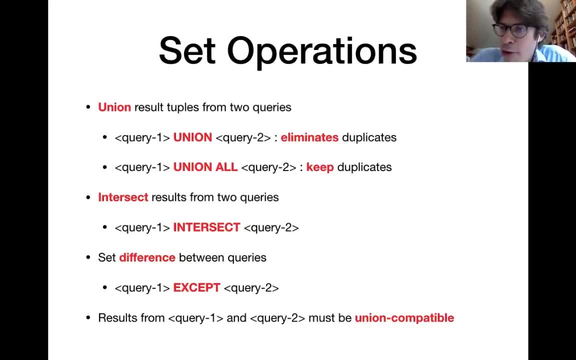 there's a couple of different variants. if you use the union a keyword, for instance, then sql will automatically eliminate a duplicate rows that appear in the union result. if you use union or, for instance, then it will keep any duplicate rows. you might have the same result. row. 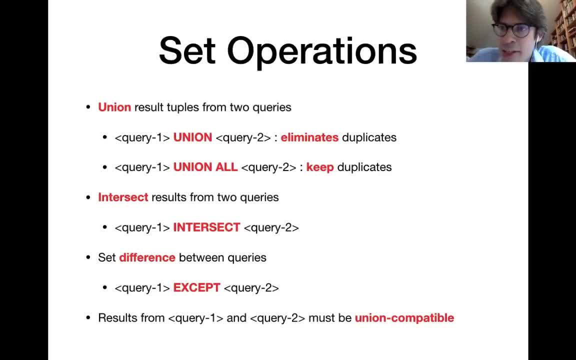 that appears in the union result, for instance, in a result, and it will have the same number of columns. so that means you have multiple types. you also have operations for intersecting the results of queries and for taking the set difference between two uh trail resides. but in all of those 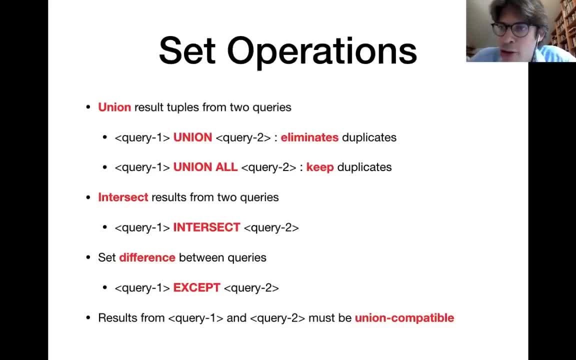 cases you must be careful because the um, the result structure of those different queries that you are combining with the set operations, must be compatible, all right be kept when using a union. so in general, without putting the order by clause, you are not guaranteed anything about the reside order. so if you want a specific reside order then you can still use the. 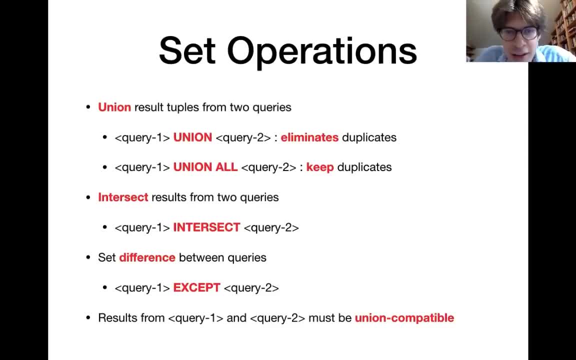 order by clause. by the way, some of those operations here, some of those set operations, they are, for instance, not supported in some other common database systems, but if you tried the sql or with the website that i have shown, then you will be able to run those operations. 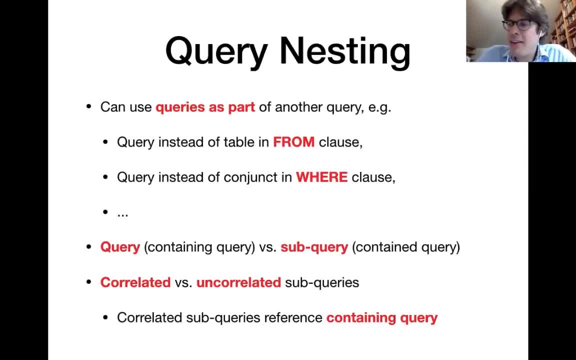 all right now. another thing that we will start discussing today, and finish at next time probably, is that we can essentially not only combine queries for set operations, but we can essentially use a so-called nested query in many other parts of a query as well. for instance, so far we have seen that in the from. 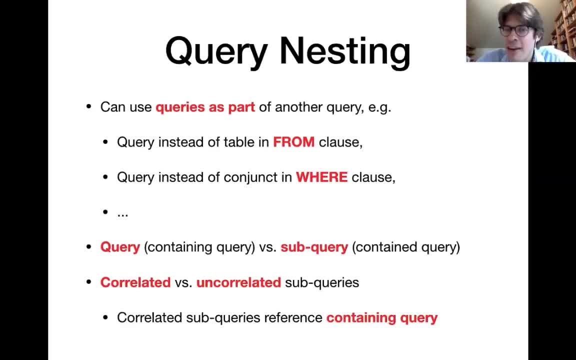 clause of a query, we can refer to tables that appear in your database, but instead of that, you could also write a new query inside of the, from course, and we will see some examples on that also. for instance, you might use a queries as part of a condition in the where clause, and so on, and 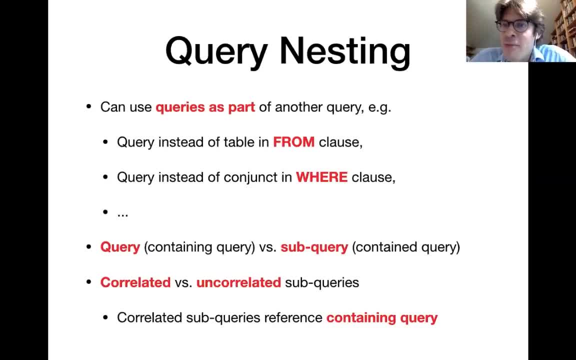 so on. so, in general, since queries take sql relations as input and produced sql relations as output, you can compose them together in a various interesting ways. now if we have the situation that we have one large query which is containing a smaller query, so to speak, then we 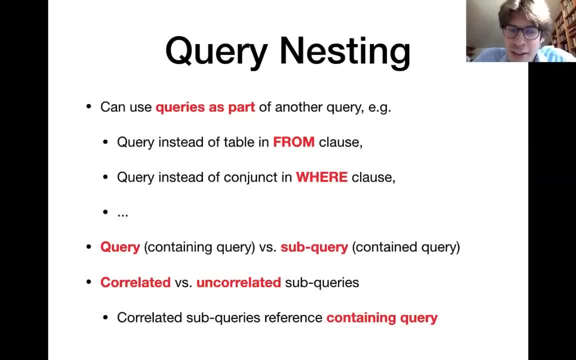 also call that a contained query, the sql query, so to speak, and we also call that a contained query, the subquery, as opposed to the containing a query. it has different variants of that containment. in the simplest case, the contained, the subquery is essentially self-contained. so you: 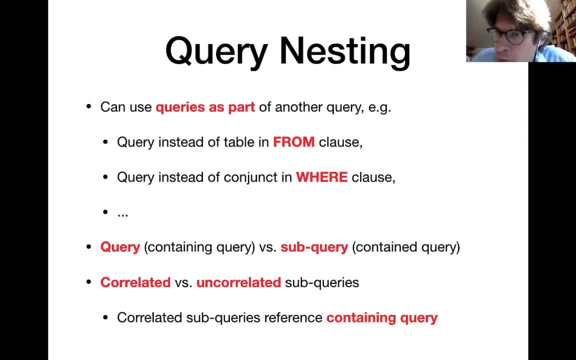 could run this query independently and it would work with your database management system. that is what we call an uncorrelated subquery. but for more complex expressions you can actually make the subquery refer to elements outside, to elements of the containing query, and those cases are a little bit more difficult to understand. that is what we call. 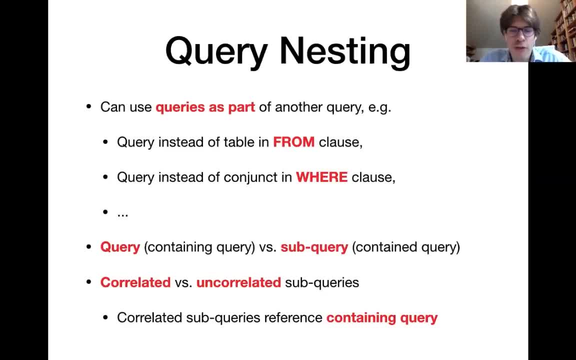 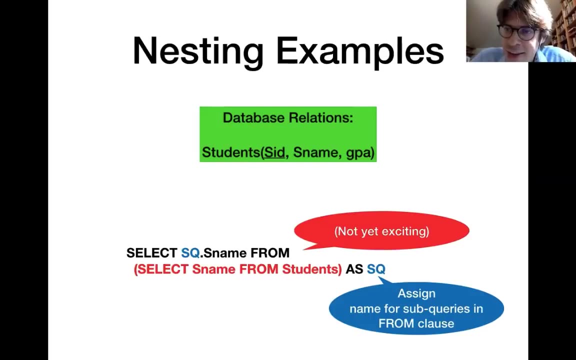 correlated subqueries. now, in the following we're going to first discuss about the uncorrelated subqueries, which are a little bit easier to understand, and we start with a rather trivial and, frankly, not very useful example here. so we simply want to select the names of all students. then i can, of course, simply use the 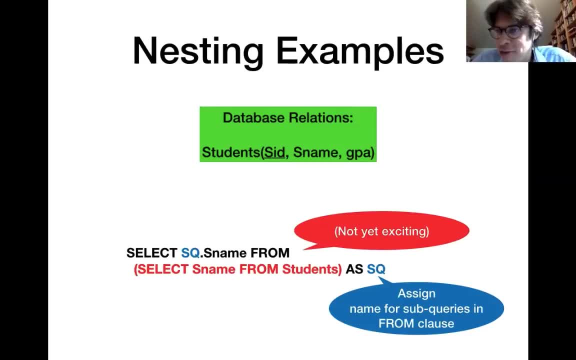 students table in the from course. but just to illustrate the principle of subqueries, i can also put a new, a subquery into the from cause, as you see here. so here, essentially, i have one entry in the from cause which corresponds to a subquery. it's an. 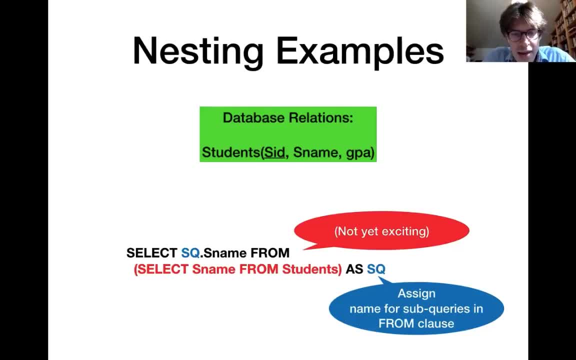 entire query right there and what it does is essentially just selecting the student names from the students and then the resize of that subquery is named sq for a subquery and, as you see in the select clause of the query, for instance, i can refer to the name for the subquery. 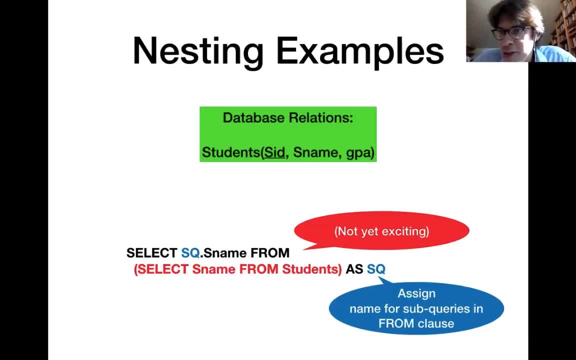 that i have just introduced. so that is important. uh, postgres actually will force you to assign names for subqueries that appear in the from clause, because typically if you use a tables in the from course, then you always have a name and i can use that name in order to refer to specific. 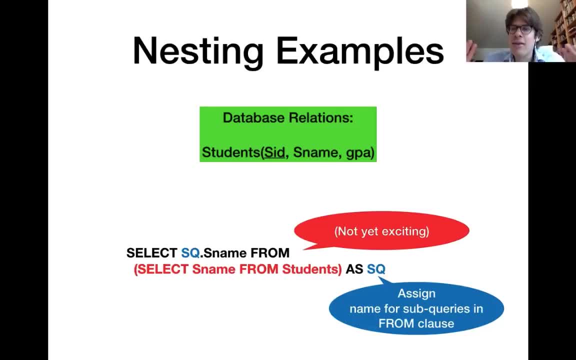 elements from other parts of the query. but if i write a new subquery then a theory- it doesn't have a name yet. so postgres forces you to specify a corresponding name and that. so how that is handled depends a little bit on the database management system in each case. 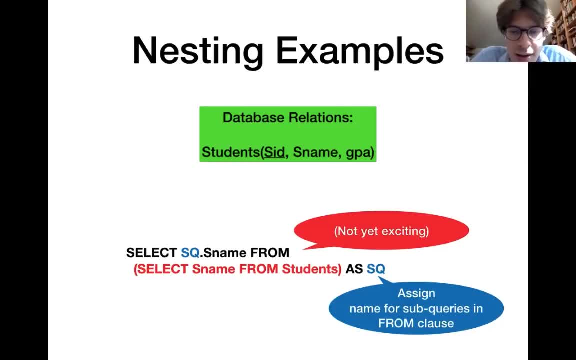 this query is not yet a very interesting, admittedly. so let's see something a little bit more useful, and here we have a subquery in the where clause, for instance, and what we are doing here is that we are selecting the names of students where the gpa is greater or equal to the 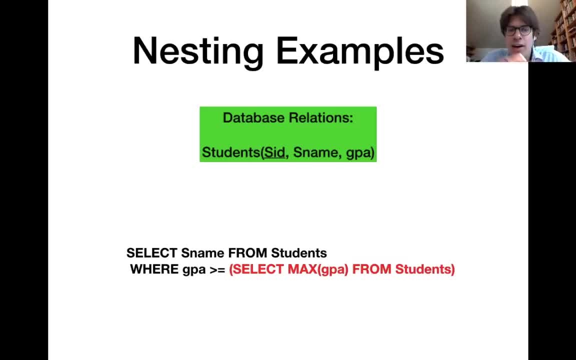 maximum gpa among all students. so here we are selecting the students with the highest gpa, and here we essentially we use one subquery in order to calculate the largest gpa over all students with the maximum aggregation function, and then we are using the result of that query within a condition. 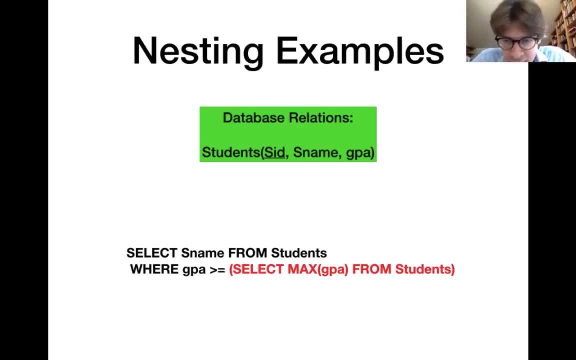 in the their course, and here the question is whether the result of that query would not be just one student. that depends, actually, because multiple students might have the same gpa and very good. as he said, that's the whole point of thisاف, which is that more question than one kind of a category. 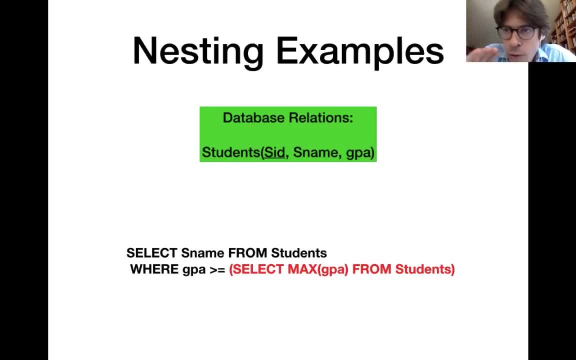 at least that's warm up, but that wanted to. showedelic example: quick for a darryin. before anything else, i want to introduce a of the following one: students, we just added to our website and in this particular using segue, use, for example, play, play bran. you can go through its version and see how many questions we can add. 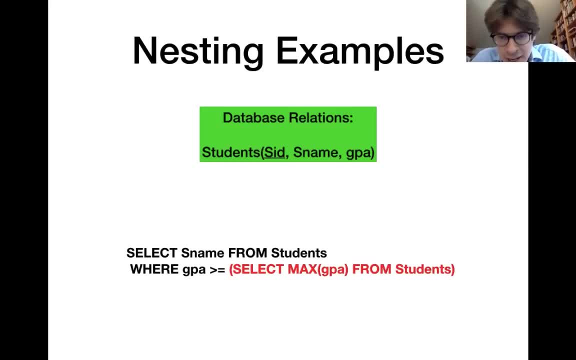 example for sub queries, and here things are already becoming a little bit more useful. So today I wanted to take a little bit of time to show you how to apply SQL in order to actually analyze. do some at least some simple analysis of a data set in. 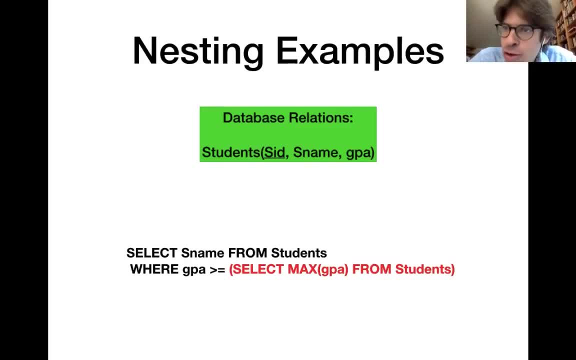 practice the full cycle. basically, I encourage you to try it out yourself. So I mean SQL. it's something which is a little bit like a programming language, in that it is much easier to understand it if you are experimenting with it yourself. So I encourage you to do that Now the next time we're going to. 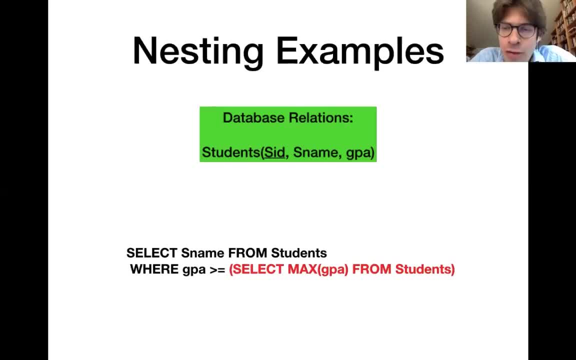 see a little bit more advanced features of SQL, in particular when it comes to sub queries, And then we are going to start with a new chapter. we're going to start looking at how the database management system internally processes your queries Right? Thank you and have a nice day. 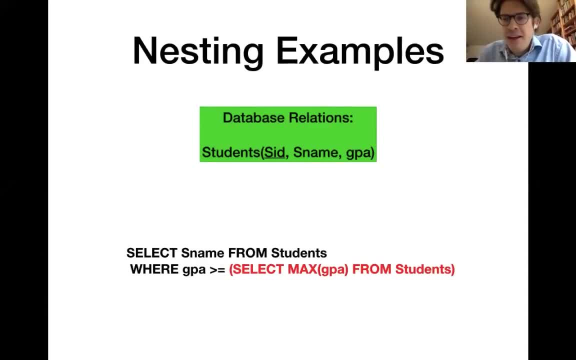 Good, So hello everyone. Today we are first gonna talk a little bit more about SQL, And probably we will still have enough time to start with a new topic, which is about looking at how your data is actually stored on the computer. 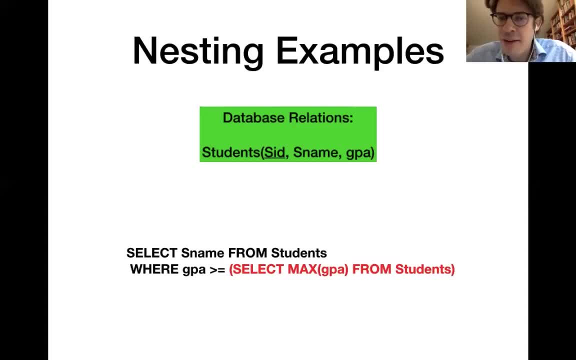 Now, last time we have seen one very important feature of SQL, which is that you can essentially nest SQL queries, so called sub queries, within a larger surrounding query, So you can use a SQL query as part of a SQL query, basically, And the 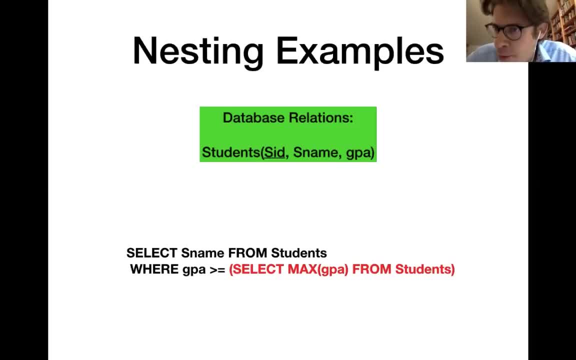 last time. we've seen a couple of very simple examples for that Here. you see one of them here, And this is actually quite a good and relatively easy to use. So what we're actually doing is we're selecting the student names from the students table where the GPA is greater or equal. 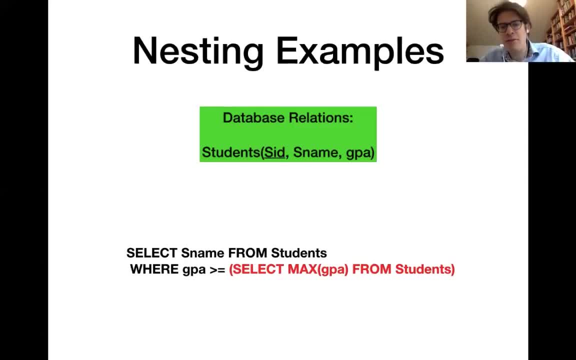 to the maximum GPA across all students And in order to calculate this maximum GPA, we are actually using a sub query. So here we have FON. a query is used as an operand within the where condition of the surrounding query. So that is one possible use case for sub queries. You can also use them in other 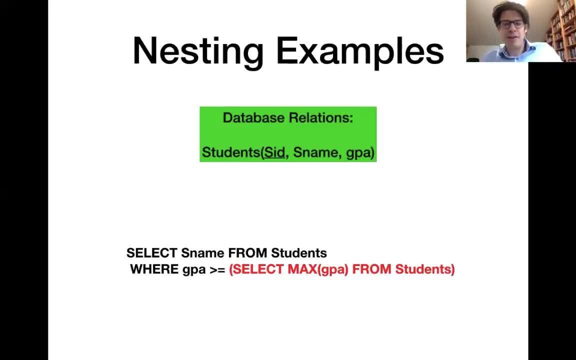 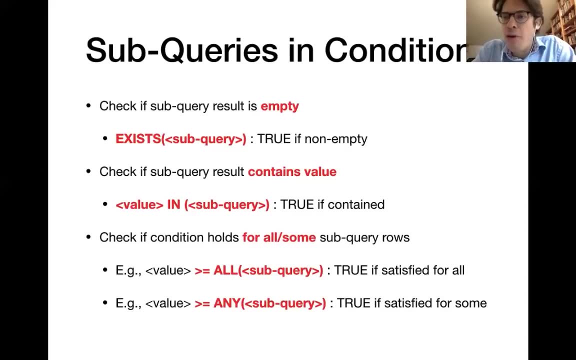 parts of a query. All right now. in the last example, we have seen one possibility to include a subquery into a launcher query. There's many more ways in which you can do that. Here you see a couple of more ways in order to integrate sub queries into the where condition or into conditions in general. 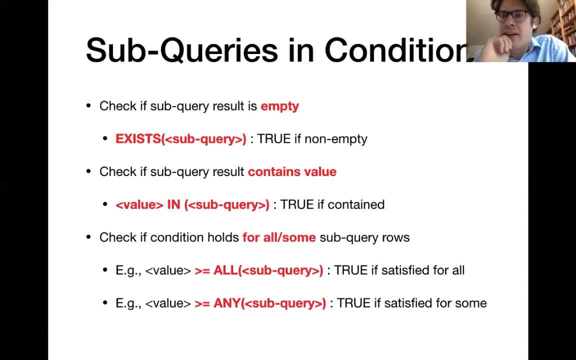 of your query, And one operation that you commonly use in the context of sub queries is the one that you can use in the context of the, that is, this exists expression here, and that essentially checks whether the result of a subquery is empty, And you also see some more examples on that. So 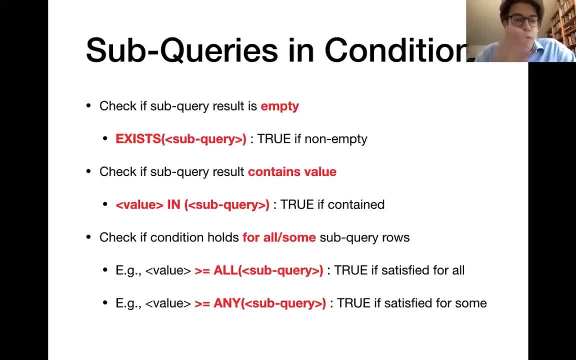 that is commonly used. Or, for instance, you could check whether one specific value is within the result values produced by a subquery, And you can do this using the in keyword that we have already seen. And you can do this using the in keyword that we have already seen. And you can do this using the in keyword that we have already seen. 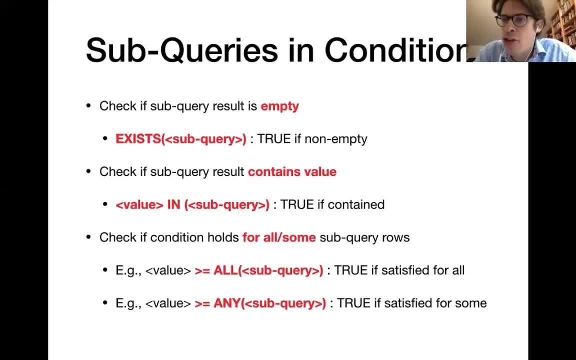 But so far we have seen it for checking whether one value is within a list of constant values, And here we are using it to check whether one value is within the results returned by a subquery. Another thing that you can use is the all and any keywords, And here, essentially, you use that in order to 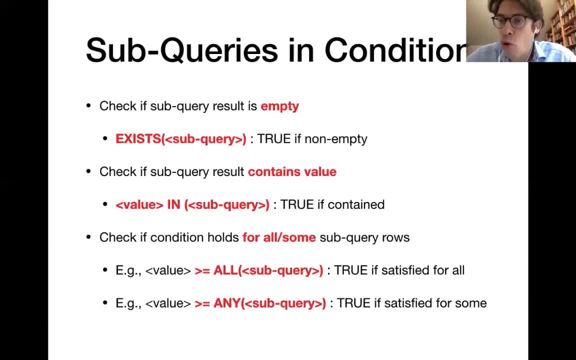 test whether some condition is satisfied, either for all result rows of a subquery or for any meaning for at least some of them, And in that case the corresponding condition returns true. Let's perhaps see one more example for the last possibility here. What we are doing here is we are selecting the 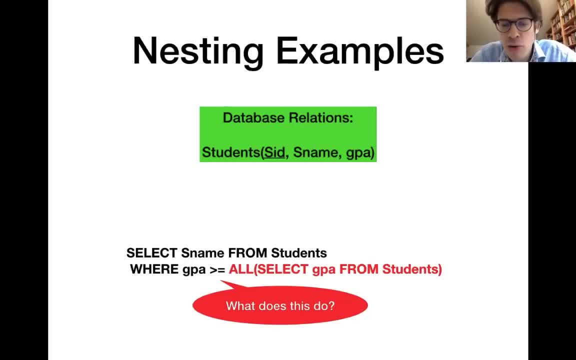 student name from the students where GPA is greater or equal. all result rows from this subquery that selects GPAs from students, And can anyone tell me in the chat what you believe that this query is doing? Anyone any ideas? Yeah, exactly So. yeah, I have multiple propositions. Yeah, so multiple. 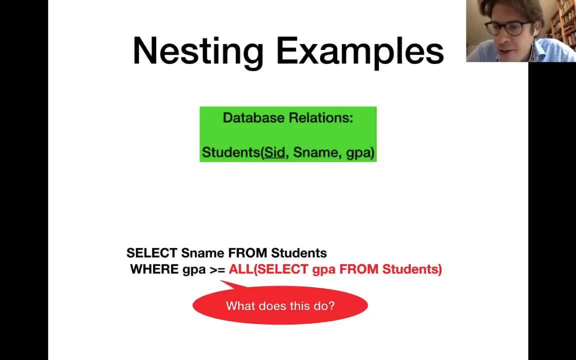 times the same propositions actually. So that is correct. So here we are again essentially checking the subquery, Having asked whether this is2014еч it is not Based on. the result can be false or null. So here I mean it could be null if we have. 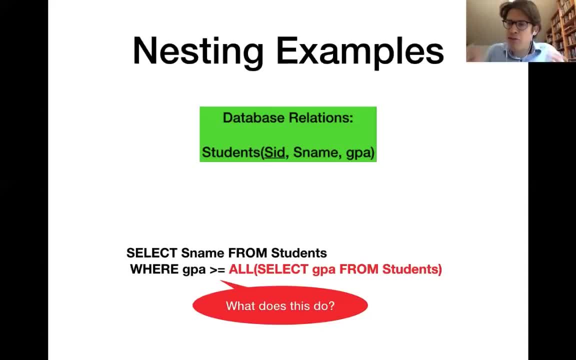 for instance, some null values for the GPA. If there are some students that don't know the GPA, I cannot verify that one specific student has the highest GPA because I don't know the GPA of some of the other students. right, And I mean for this to be false. 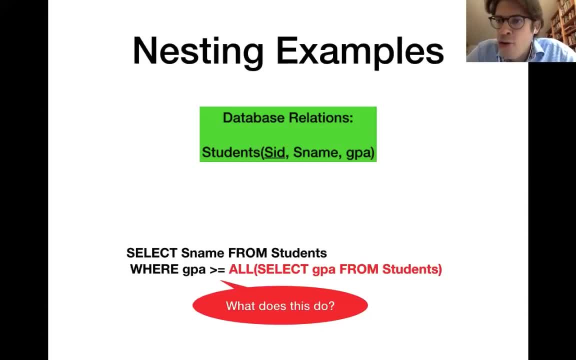 that is the case if there is another student who has a higher GPA than the currently examined students. So you can imagine that here we are iterating over the students that are stored in a student table. We are picking one, Then we check whether this condition- that student's GPA- 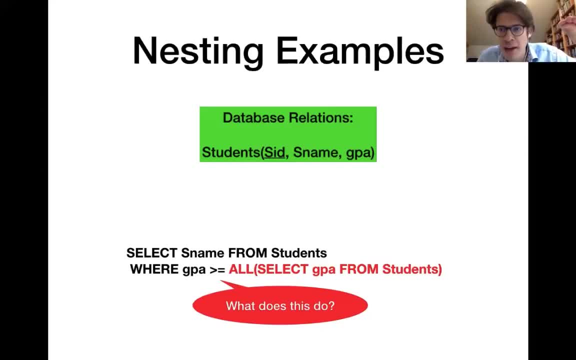 is greater or equal The list of all GPAs. So we have the GPAs from all students for each of them And if that is the case, I'm going to include it into the recite. If that is not the case, I'm not going. 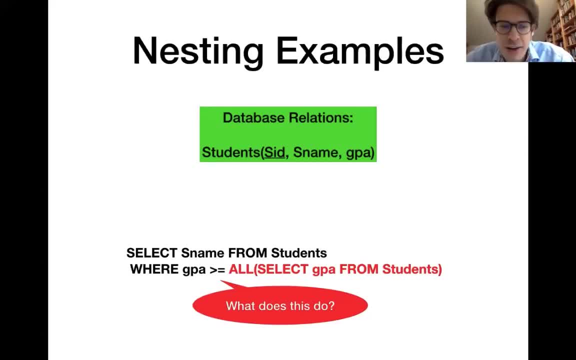 to include it into the query recite, right? So we can essentially imagine that we have a for loop, pretty much, where we iterate over the students, And then the subquery would essentially correspond to another for loop. So we have essentially two nested for loops. 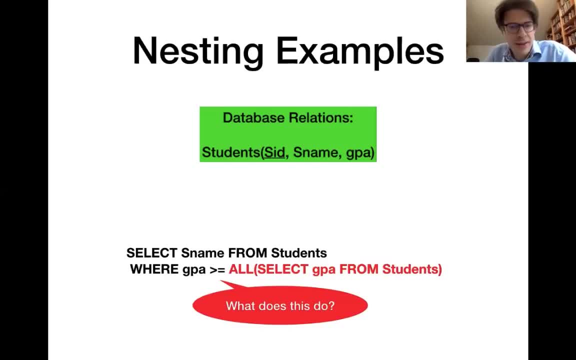 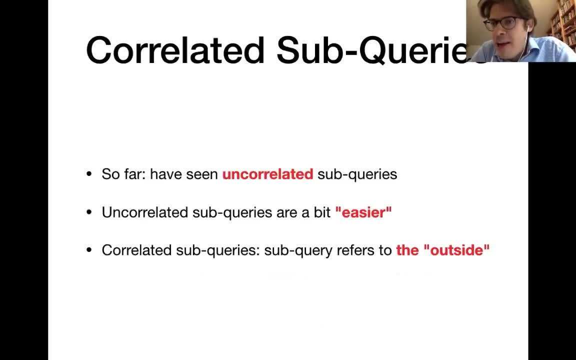 And then we have a for loop for the students, right, OK, All, right. Now those are a couple of examples for subqueries. Essentially, you just evaluate the subqueries first for the examples that we have seen, And then you get some kind of return value. 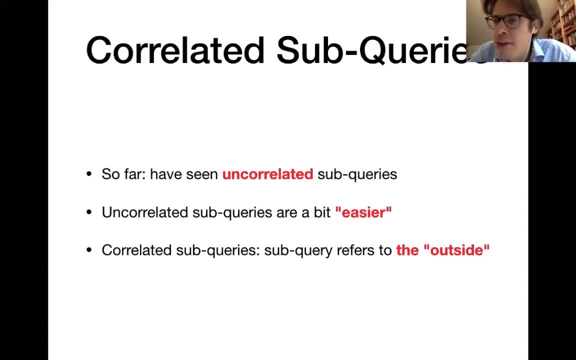 Then you insert that return value into the surrounding query. Now, what we have seen so far, This is what we call uncorrelated subqueries, And that means essentially that you could run the subquery all by itself and the database management system would not complain. 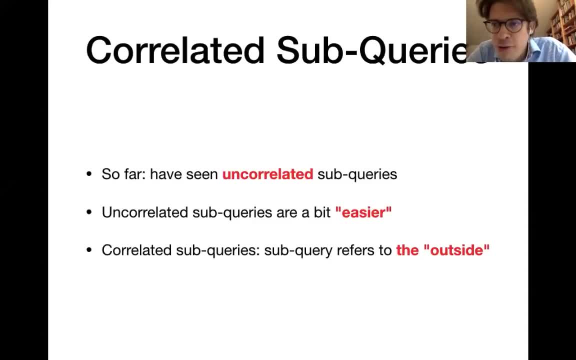 Correlated subqueries are a little bit more difficult. This is why we are doing them now And we started with the other ones. For correlated subqueries, the nested query, the subquery, is not independent from the surrounding query. So here the subquery is not independent. 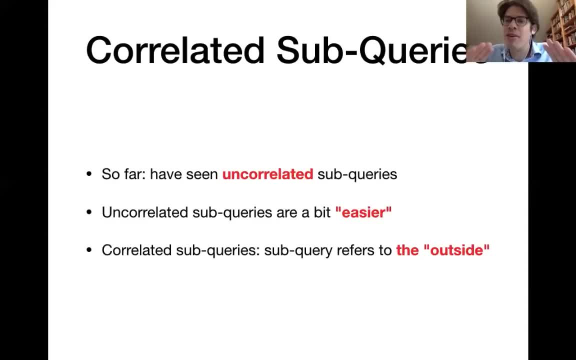 And then we have the subquery. query would essentially reference some elements that appear in the surrounding query, which means that a subquery all by itself is not viable because it would include references to something that only exists in the outer query. So here, by the way, I see some interesting discussion. 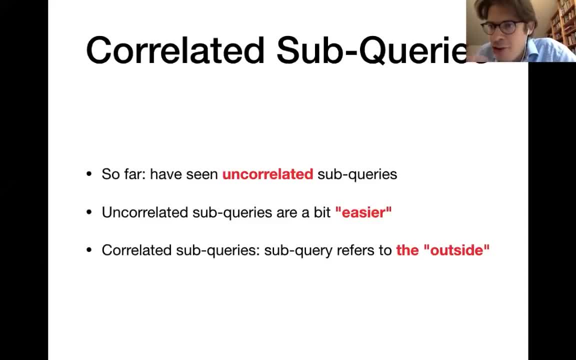 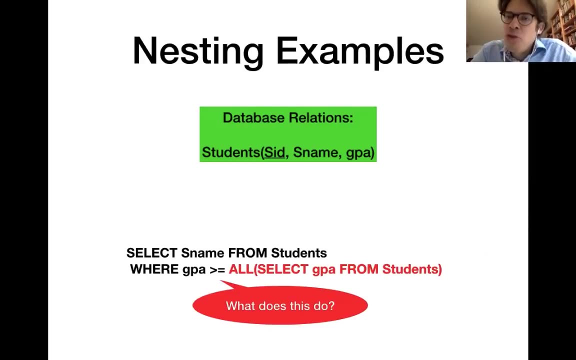 going on and I encourage you to generally answer the questions of your classmates also in the chat. And just because I see that here, let me say one last thing about the evaluation of this subquery that I have shown here. I told you that you can imagine that this is evaluated. 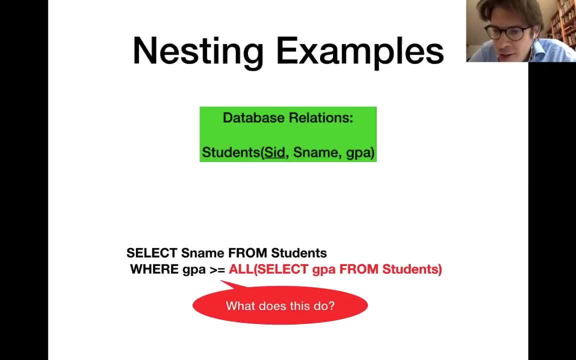 by two nested for loops. And here one of the questions is: wouldn't that be inefficient? And I actually agree with that. So if I say that you could evaluate it with two nested for loops, I just mean conceptually. this is how you can imagine what the query result is going to be. 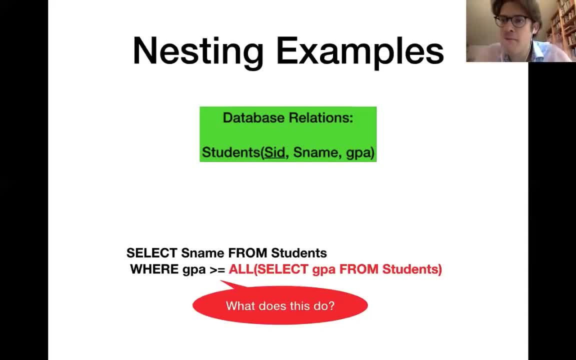 You can. essentially, in order to understand what the result of this query is, you can imagine that we would have two nested for loops, But internally, the database management system is probably doing something more efficient, or could be doing something more efficient, And the way in which you're going, 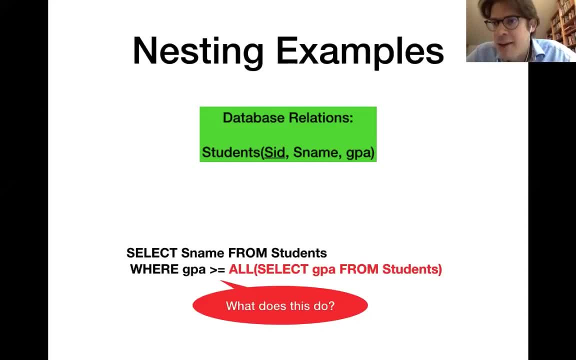 to write your query generally is independent of how the database management system evaluates your query. So the two for loops. this is not necessarily what's happening inside, But this is what you can imagine is happening in order to understand what the result of this query is. 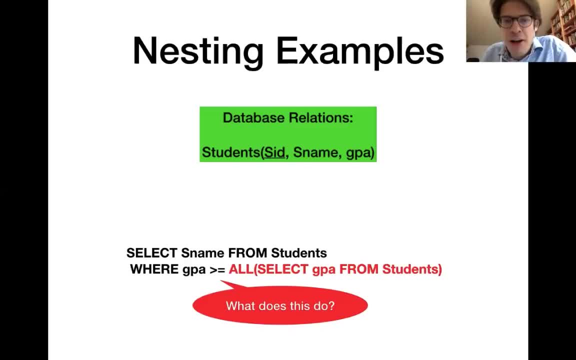 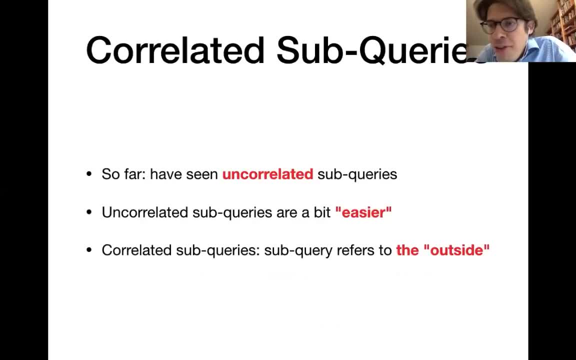 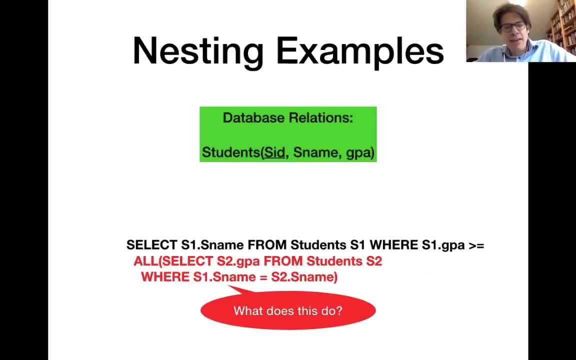 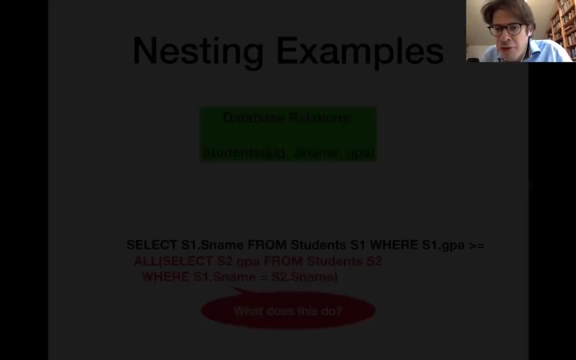 OK, very good points here in the chat. All right, and now we are switching to correlated sub-query which reference some things outside of the sub-query and in the surrounding query. Now let's see the first example. You need to move the chat. 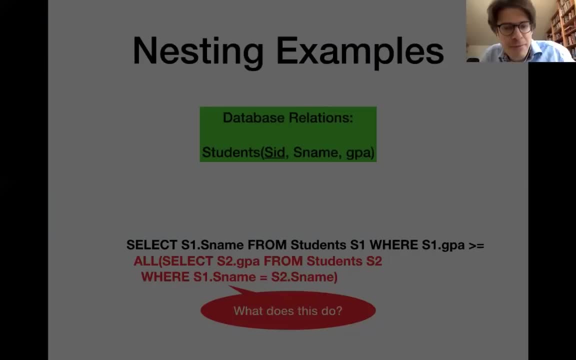 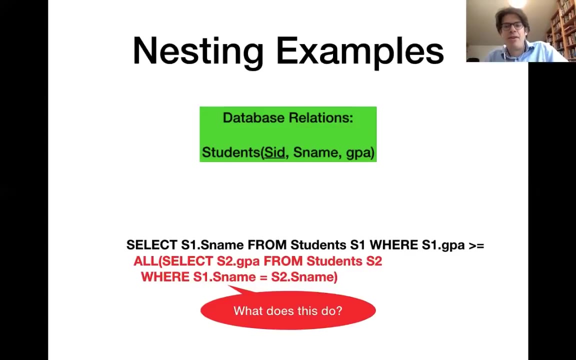 so I can see the example fully. So here we are again, selecting the student names from the students table and we assign the alias s1 to it in the outer query, and the condition to be included in the result is that the s1.gpa must be greater or equal to all. and here comes 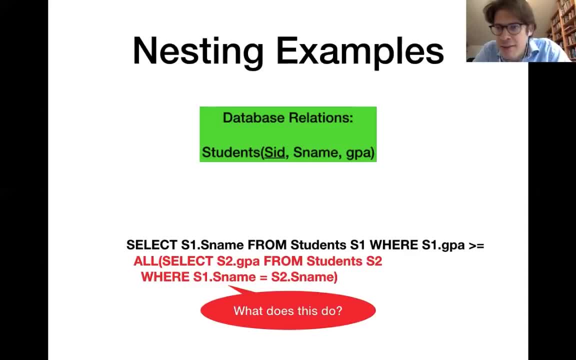 a select over students. again, This time we assign a different alias, s2, and we require that s1.sname equals s2.sname. So can anyone first of all tell me why this is a correlated subquery Looks kind of similar to the ones that we have seen already. so what makes this? 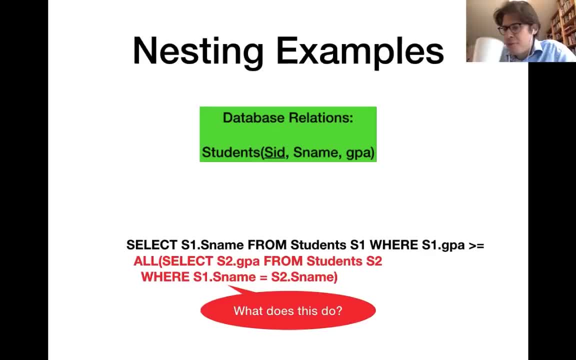 one specific. Oh yes, very good, and here is the reference to, in hurtic, such as two. so we find the, in particular s 1. Right, here we find a subquery. we are referencing tableNot axle s2 and table Verdict. Now, table added. aleias Matters s tool is not particularly exciting, because that is defined as table, unsere. 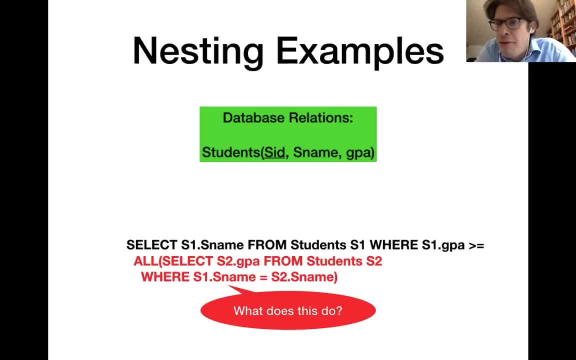 tablealeye the s2 is is not particularly exciting because that is defined as table Very important to know. when we define S1, it is because we define rhymes, like we gave it name before and character within the same sub-query, Table-alias S1,. on the other hand, 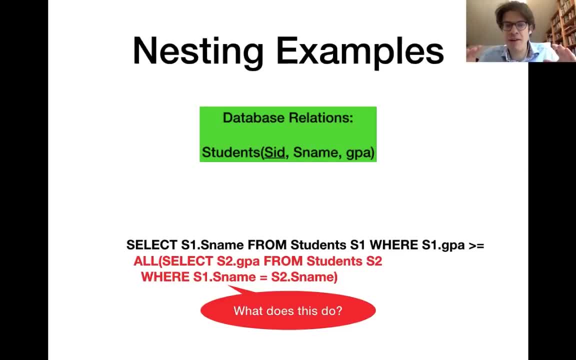 that one is actually not defined within the sub-query, but it is defined outside. It is defined in the outer query. That means if you take the sub-query, select S2.gpa from students S2, where S1.sname equals S2.sname. 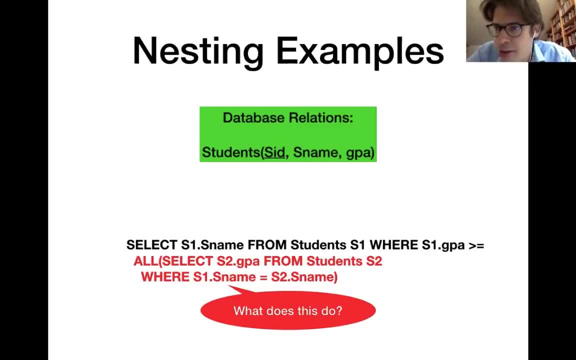 That's sub-query marked in red And you run it all by itself in a database management system. You will actually not be able to do that because the database system will complain to you that there is some undefined identifier S1. That's why it is a correlated sub-query. 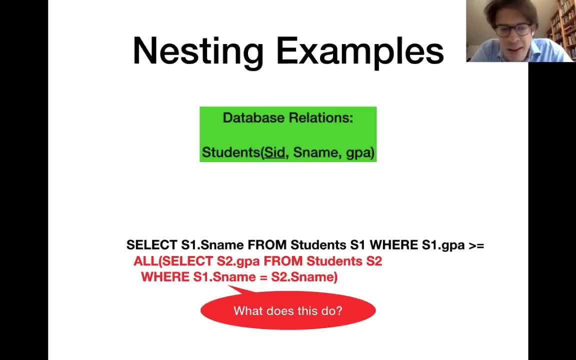 So, yes, So this is why it is a correlated sub-query, And can anyone guess as to what this query is actually doing? So, strictly speaking, we have not yet discussed in detail how to evaluate those correlated sub-queries, but maybe anyone has a hunch. 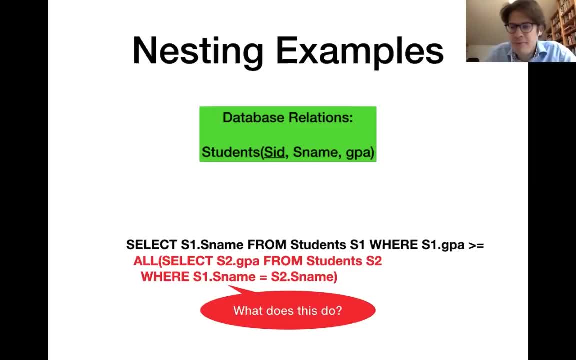 about what this could be. Hmm, Hmm, Very good, And here I see the right solution popping up. So what it does is actually the following. So I'm again going to tell you how we can imagine that this query is evaluated, even though internally inside the database system. 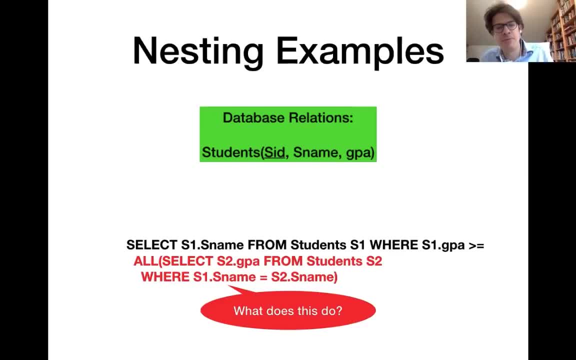 it might be evaluated in a more efficient manner. But what you can imagine here is that we are iterating in the outer query, We're iterating over the students again, And for each of those students that we are iterating over in the outer loop, so to speak. 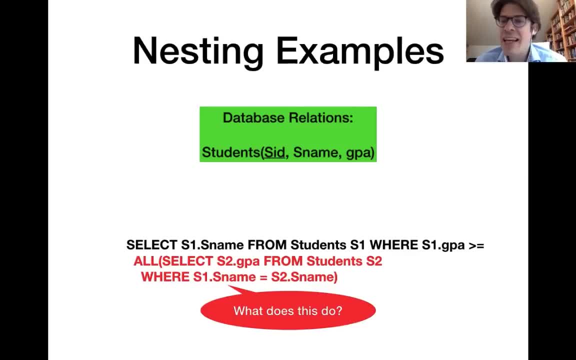 we are iterating over the students in an inner loop And within that inner loop you're only considering students which have the same name as the currently selected student in the outer loop, And then we check whether for all of those students which have the same name as the students in the outer loop. 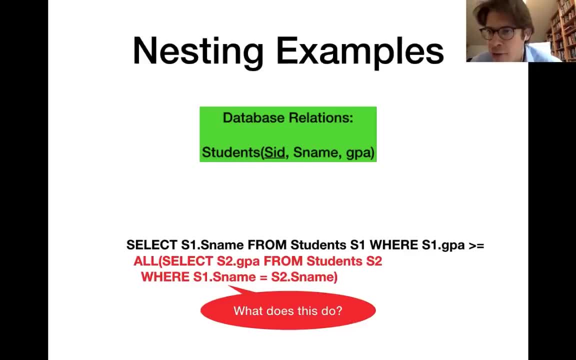 the GPA from the outer loop student is greater or equal to the GPA of the inner loop student. That's one and that's two. basically, Those are like two iterator variables. Okay, And because of that, as suggested here by one of your peers, you can see that the GPA of the inner loop student is greater or equal to the GPA of the outer loop student And because of that, as suggested here by one of your peers, you can see that the GPA of the inner loop student is greater or equal to the GPA of the outer loop student. 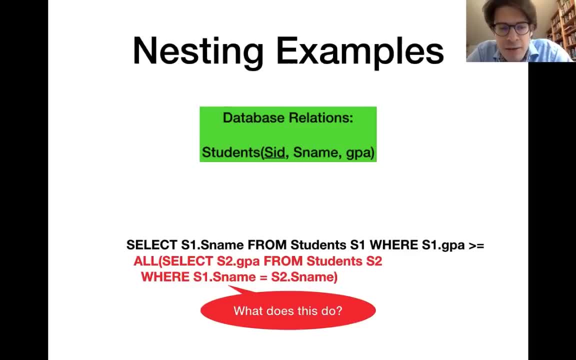 And because of that, as suggested here by one of your peers, we do indeed retain those students- the name of students- which have the maximum GPA among all the students with the same name. So that's maybe a little bit of an artificial example. 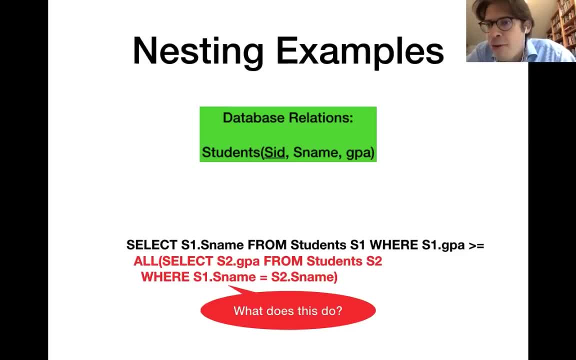 but of course, in principle you can have students with the same name even though not the same net ID, And here we are keeping the maximum GPA student among all groups of students with the same name. One thing that I used here: 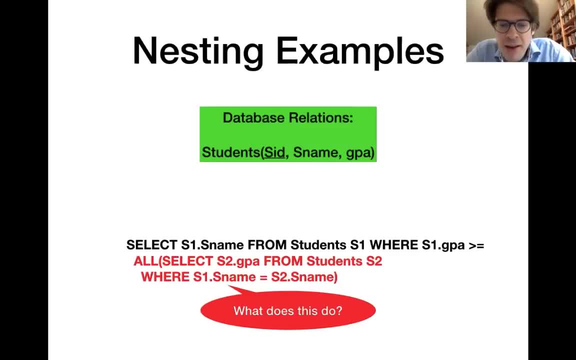 by the way, besides introducing correlated subqueries, I have one query where the same table appears multiple times. You have already seen that before, but just to point your attention towards that. So in general, you can have the same table appear multiple times in a query. 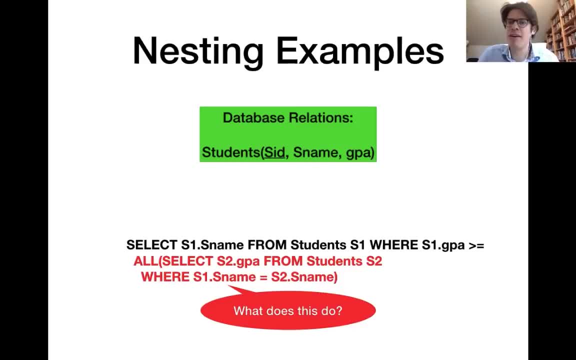 either within different subqueries or even like within the same query. but what you often want to do is to assign different aliases to that same table. So here I have the students table, one's appearing with S1, and one's appearing with S2.. 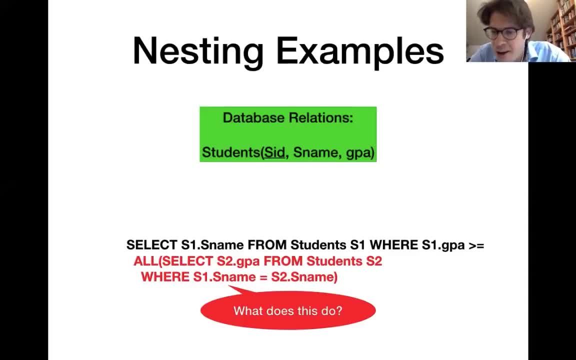 And one interesting question that I see here is that so better disclose the query would be possible with our two aliases to students, And here I mean if you want to. I mean you could probably reformulate the query in quite a different way. 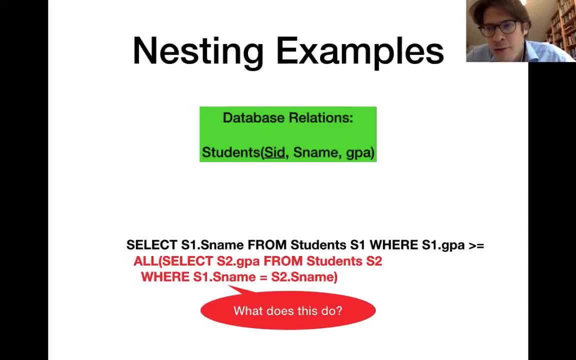 And maybe you could get around that, but I mean definitely as long as you stay with this structure of the query. here you need to compare students of the same name, so you need to compare two students And in order to distinguish between those two students, 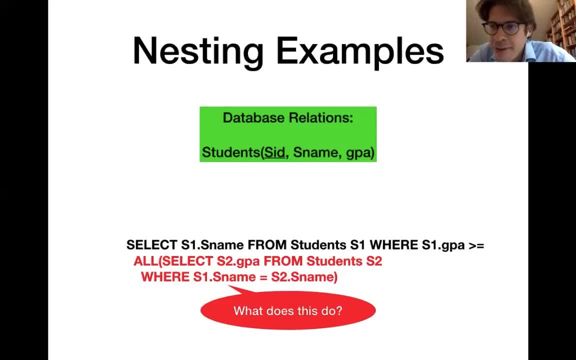 you need to use an alias here. Yes, exactly. So that's why I'm saying that if you keep the same structure, then you need to do this. It would also be ways, for instance, to group by the names, get the maximum GPA in each group. 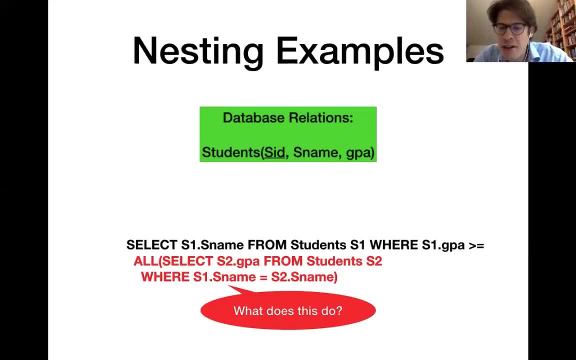 That's a good thing, is a great suggestion. and then joining that with the um, and then joining that in order to um get the student associated with the maximum gpa within each of those as student groups, or you could, for instance, um use a subquery in the front course. 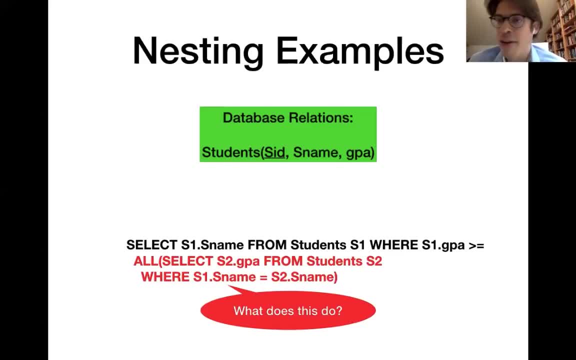 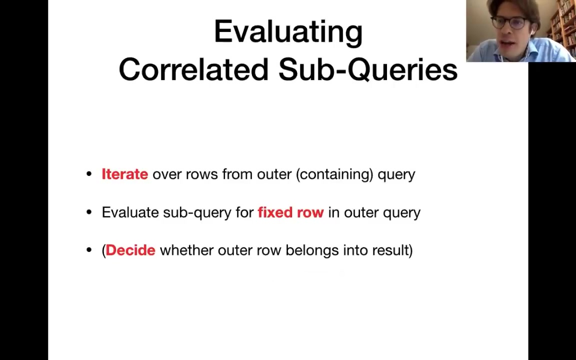 and then you would have to introduce an alias for that subquery, but, strictly speaking, not for the table alone. okay, so there's many ways of writing this, but you need some some way of correlating different students in order to make this comparison. all right, so the general principle, um, in order to imagine how the result of 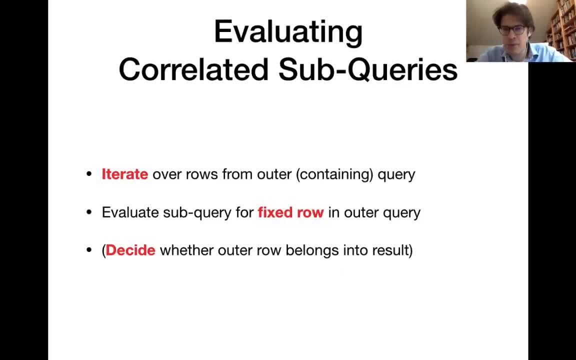 those correlated subqueries is generated. i find it quite convenient to imagine nested loops being evaluated, even though that might be inefficient. it's not that the database management system is doing in the background, but it can help to imagine that, and then you would generally iterate over the 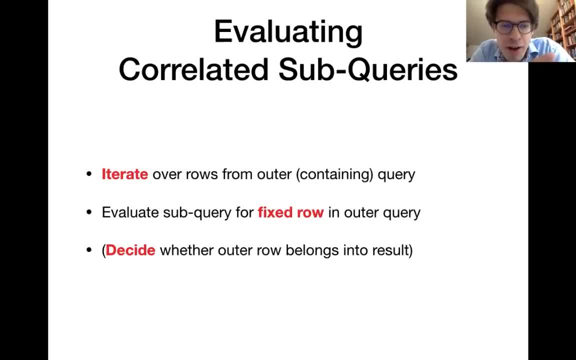 rows in some outer containing query, and for a fixed row you would evaluate the inner query. now, here the result of the inner query might depend on which row is currently selected in the outer query. that is why, at least conceptually, we would have to re-evaluate the correlated subquery for each different row in the outer. 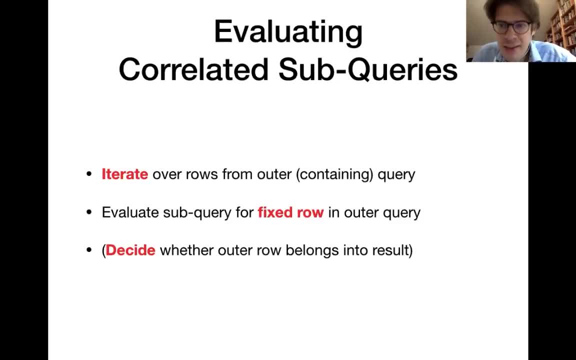 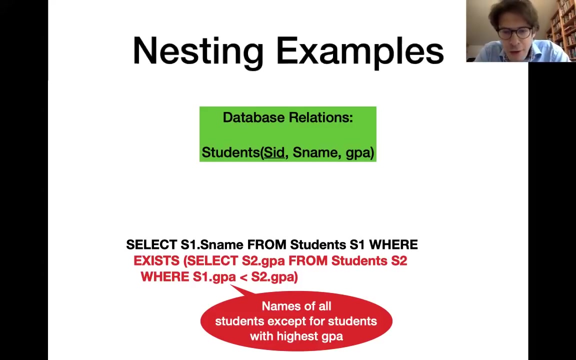 query and then if the better, if the where condition in the outer query uses a subquery, then finally you would decide for the currently selected row in the outer query, better to include it into the result set or not. now, here, for instance, we have another example. so here again we are comparing students and we use a correlated. 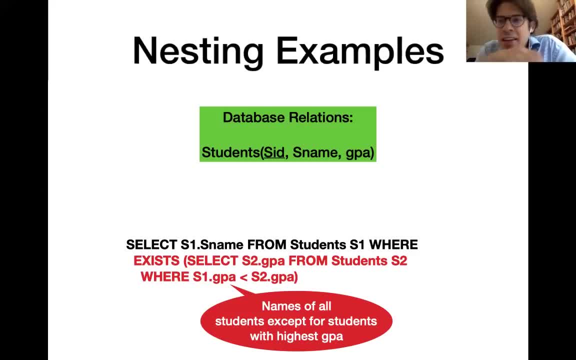 subquery. so here we in the outer loop iterate over the students again, and then for each fixed student in the outer loop we check whether the result of this correlated subquery is non-empty. that is what the exists keyword is doing. there exists some result. and for a fixed student in the outer loop, 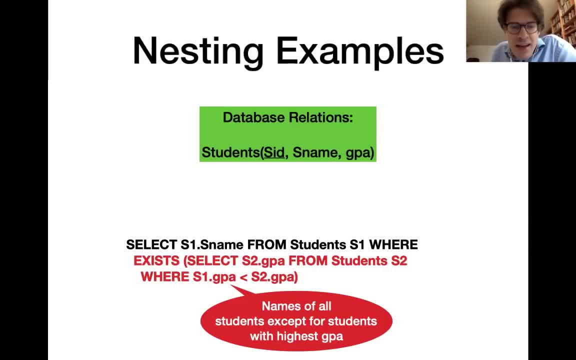 in the inner query, i'm iterating over the students again and i check whether there is another student who has a higher gpa now, and if such a student exists, then the outer loop student will be included into the result set. so what is this basically doing? is that? 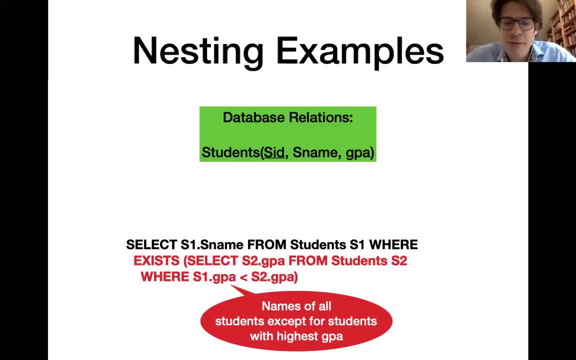 here. this time we're selecting the names of all the students except for the students with the highest gpa, because for each student we test whether there's another student with a higher gpa. right, so those are the results that we have here. so we have a couple of simple correlated subqueries that you see here. 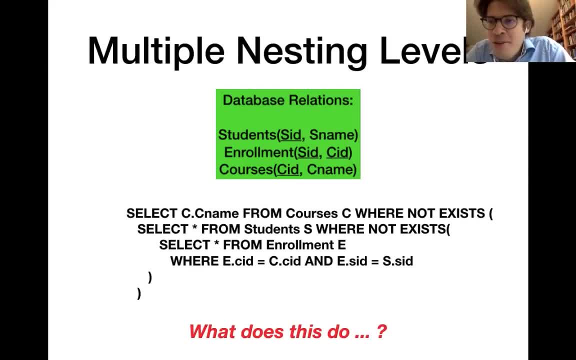 now take a look at this one. now, what i'm exploiting here is the fact that actually your subqueries can also have subqueries, so you can have multiple levels of nesting here. in this query we are first iterating over courses, then next you're iterating over students. 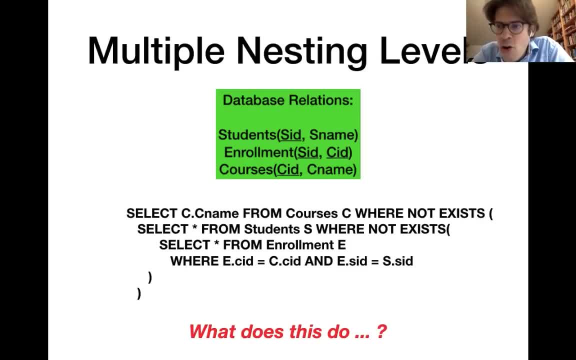 then next we are iterating over enrollments. um, does anyone have an idea what this query is doing? any propositions, okay. first. first proposition: find courses that have no students enrolled in them. or find the courses that have no enrollment. okay, other propositions in order to break that down. so that is perhaps the most complex query we have. 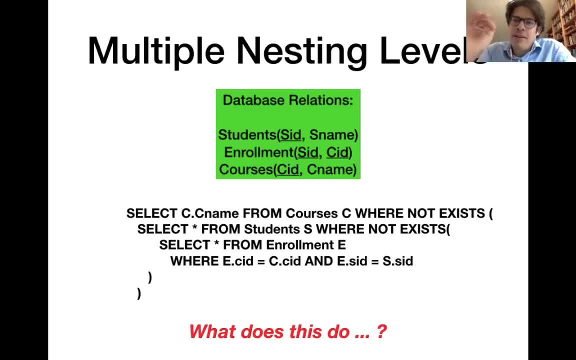 seen so far. okay, so let's break it down a bit. so let's make it simpler by imagining that we have already fixed one course in the loop. now can anyone tell me, but the result of this select star from students and so on, what a result of this query is gonna be? so we have fixed the course and 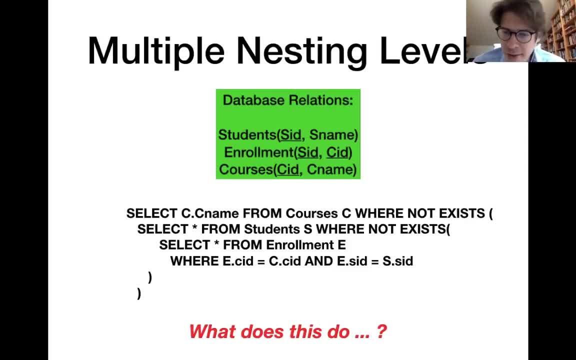 now we have this query: select star from students, as we're not exists. select star from enrollment: eat where course ID matches and student ID matches. find courses with at least one student enrolled. okay, that is all right. this is the writer direction here. okay, I'm gonna give it a second because I think it's. 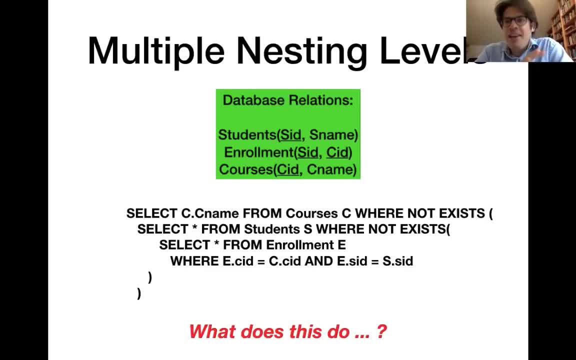 a nice example and make sense to think about this for a few seconds. okay, good propositions here. okay, I'm gonna resolve it in a minute. just the okay. people are agreeing- that's green- to the solution perhaps? okay, all right, so I give it one more minute and just think about it a little bit more. 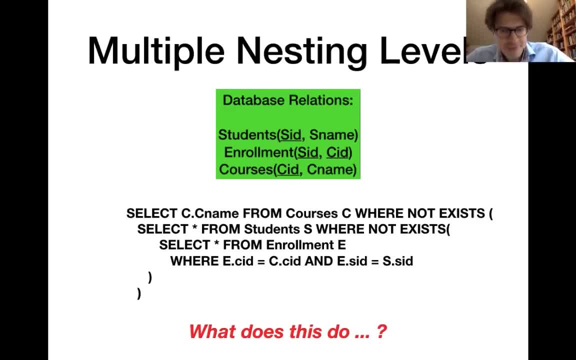 and clearly, as the exists keyword tests whether the result of a subquery is correct or not. okay, okay, okay, okay, all right. so let me try to please show you again. okay, all right. so let me try to try to go into an example and see if there is where. 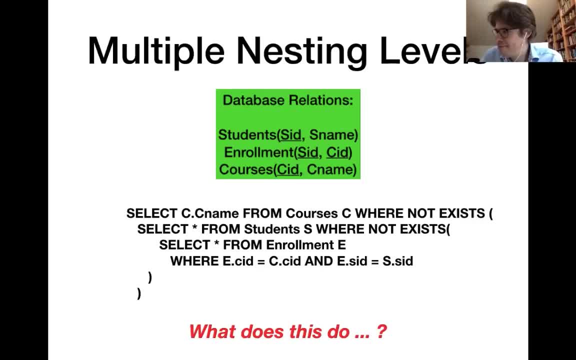 it says non, empty, not exists, essentially tests whether the result of a sub query is empty, and it is true only in that case. you, you, all right, so all right. so let's have a look at this, so let's maybe start with the innermost a sub query, so 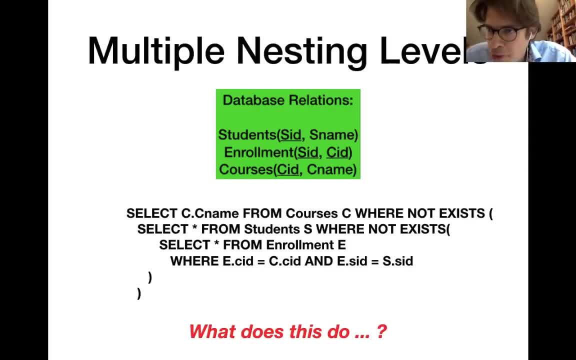 what we're doing here is that we are looking at the enrollment information which links students to the courses that they are enrolled in- okay- and the student as well as the course they have been fixed in the outer queries currently. so here I'm essentially checking whether some enrollment 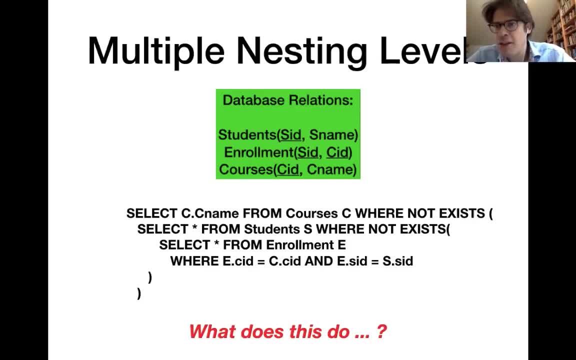 information exists for the currently selected course and for the currently selected student. now, this innermost subquery is contained within a not exists class in that middle query which selects from the students table right. and so basically, um, here in that middle query, I am producing a students which are not 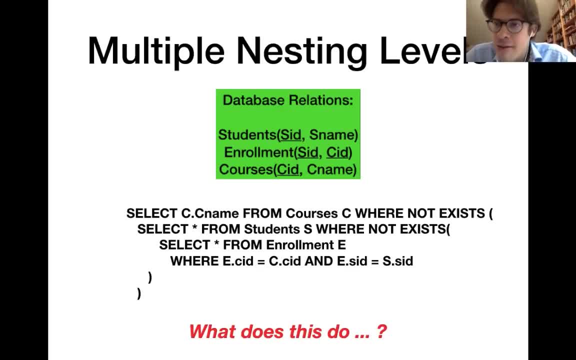 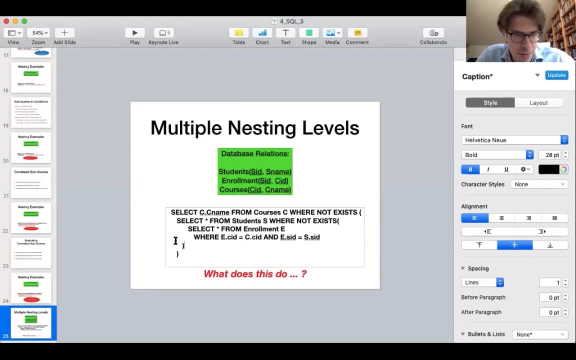 enrolled in a specific course because the enrollment information for this student with the currently selected course in the outer query is empty. okay, so here let me essentially- let me maybe mark that here this query essentially looks for students that are not enrolled in the currently selected course. and now I'm looking for courses where the result of 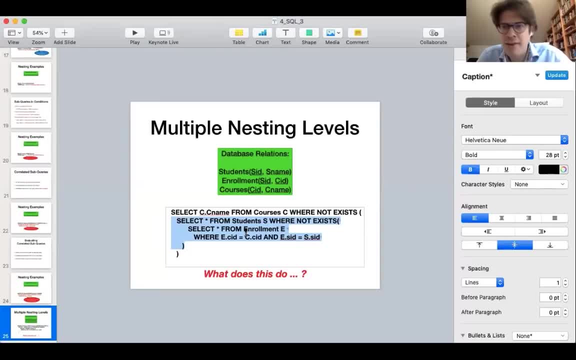 this sub query is empty. so I'm essentially looking for courses where no student is not enrolled. so that, formulated differently, means that here I'm looking for the students for the courses where all the students are enrolled, which most likely is empty. the reside of that query, but that is. 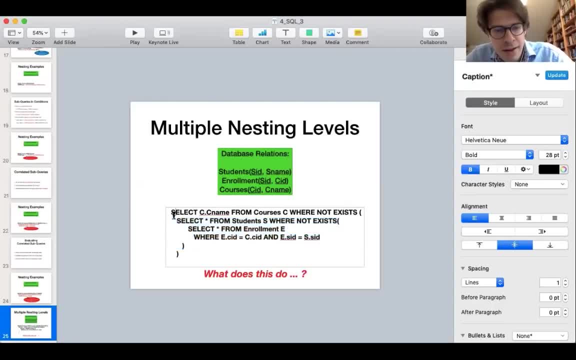 what the query is looking for here. I am fixing a course, then I'm looking for students which are not enrolled in that course, and then I'm checking better. that list is empty, so no student is not enrolled in the course, and if so, I'm including the name of this course into the reside set. that's what this. 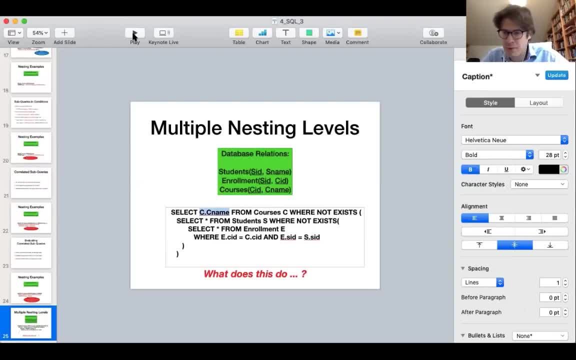 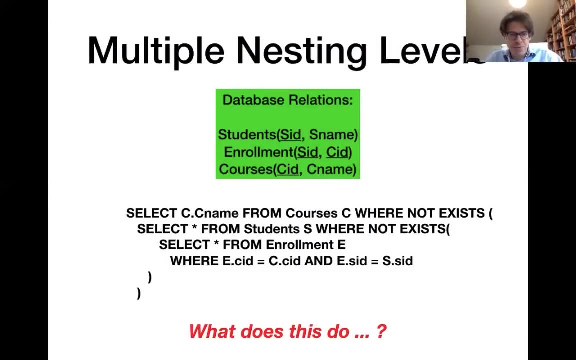 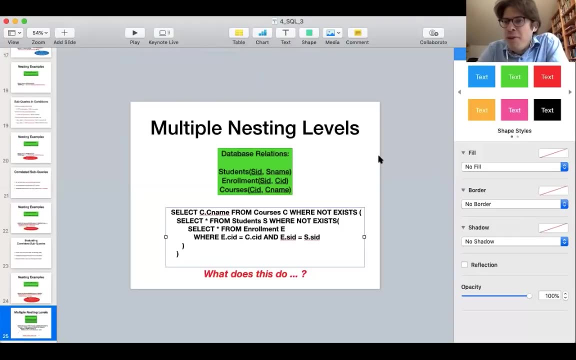 query is doing. I'm looking for students which are not enrolled in the course and, if so, I'm including the name of this course into the reside set. that's what this query is doing, all right, so that is what we will see about a sequel now. this is the probably. 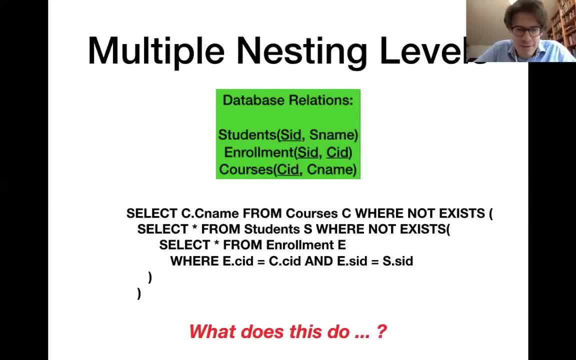 the most difficult query that we have seen in the course, and I encourage you to think a little bit more about it and to make sure that you understand what's going on there, and also perhaps to experiment a little bit. there's some, there's some nested queries yourself, for instance, in one of the data set that we 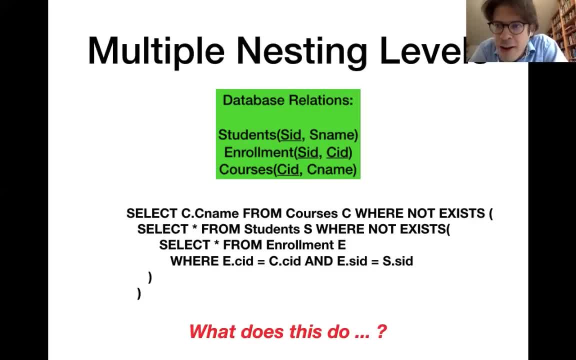 of the in the data set that we have recently downloaded or in some other data set of your choosing. we have seen a couple of examples, but in the end, to really get the hang of it, you probably want to write some queries like this yourself, and I encourage you to look at this and maybe send some other queries and I will looks like reading for you concerning some of the queries yourself, but you know, just no, it doesn't want to focus on this ones. the sake and weren't any query ones are clear are, if you have it, this one in your listening, related questions겠어. 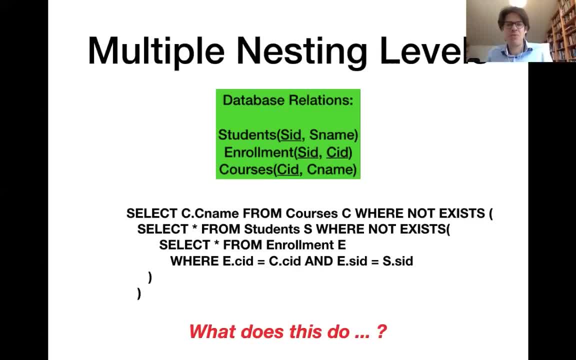 you probably want to count and write some queries like this yourself, and I encourage you to take a minimum if you can get some of these works and the answers within the topic on your own disappointment dot com. faster record action related issues and also, if you need, your tasks include further supplement projects. 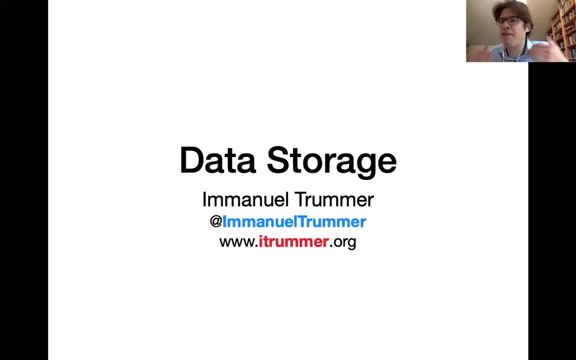 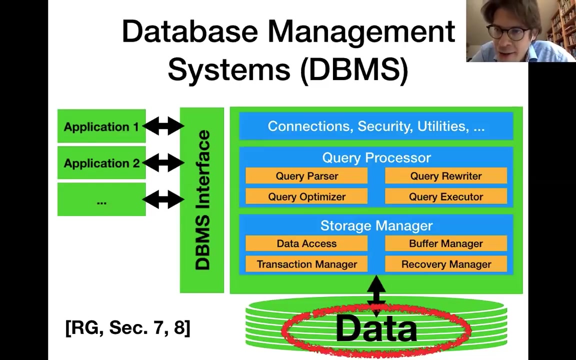 I encourage you to do that. so now we have seen essentially what is the interface of database management systems, and now we will see in the following a little bit more of what is going on inside of the database management system. so first of all, we're going to talk more about how the data of your database 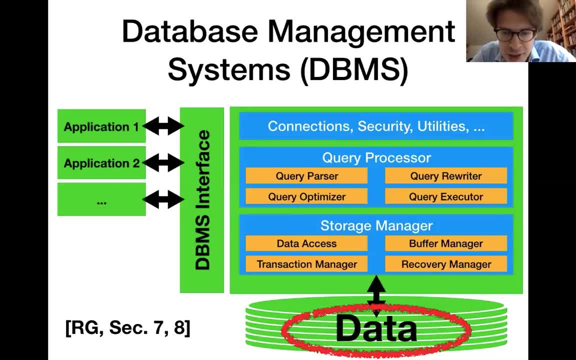 management system is organized and stored. so here we are at the lower part of this diagram that I have introduced in the first vector and the relevant chapters in the Ramakrishnan and a gap the book. those are chapters 7 and 8 in particular, and what we are going to do in the following is that we are first 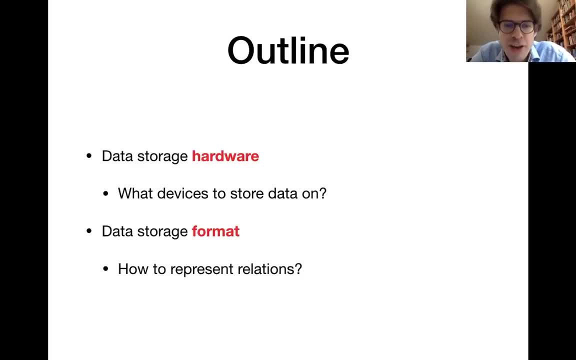 going to discuss about the hardware on which a data is stored and then we're going to discuss a little bit about the format according to which data is stored on that hardware. so in the following, we're going to first discuss about the hardware on which your data is stored and the properties of that hardware. 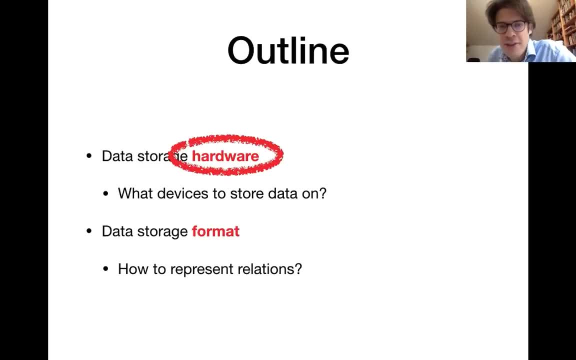 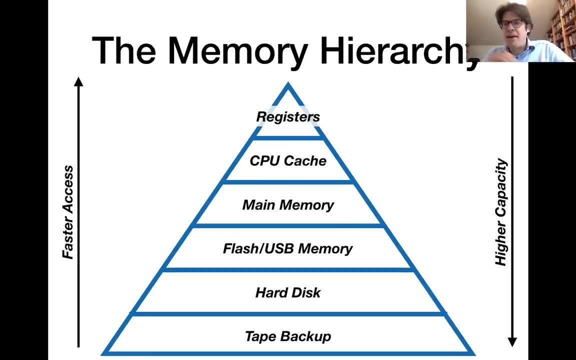 will motivate certain design decisions in the database management system. now, data on your computer is generally stored on different locations and typically those possible locations are represented as this memory hierarchy that you see here. it's often represented, and in this pyramid shape in all the order to illustrate that the capacity of the storage layers decreases once you go. 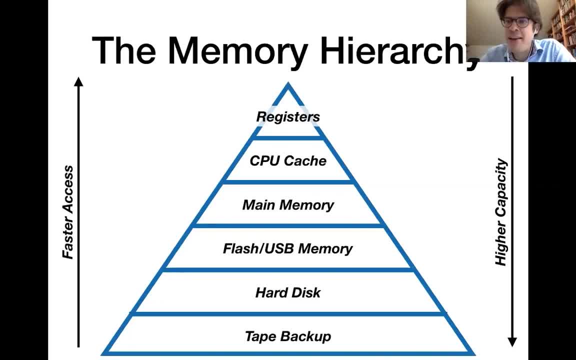 up that pyramid. so typically the storage layers towards the upper part of this pyramid. they have faster access times but they also have fewer kept like less capacity, so you can store less data there. another important distinction between the different layers of the memory hierarchy is that some of them are volatile, meaning that data there is. 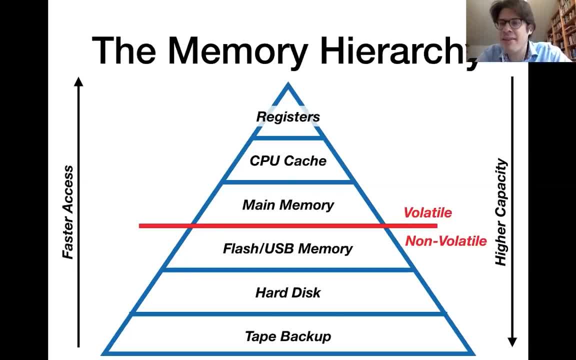 erased once your computer switches off, while others are permanent, meaning that even if your server switches off, then they will still keep the data stored and, at least traditionally, database management systems. they consider, for instance, updates to your data only a secure once those updates reach stable storage, at the very top of that pyramid, so to speak. 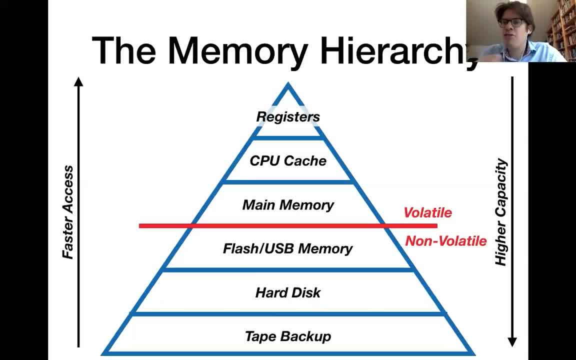 sits the cpu which is doing the actual processing. so what needs to happen in order to do any useful complication over the data is that you move the data through the memory hierarchy up to the processor registers where the processor can access it. now, in the following we're going to go through those different layers of the memory hierarchy. 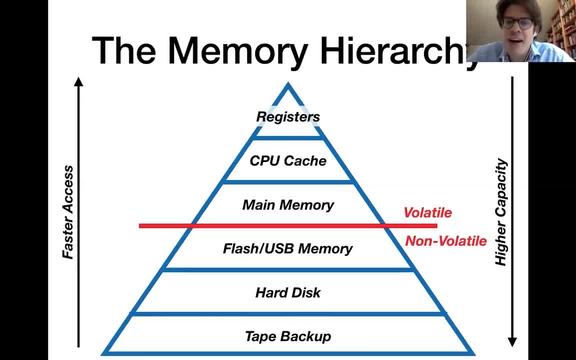 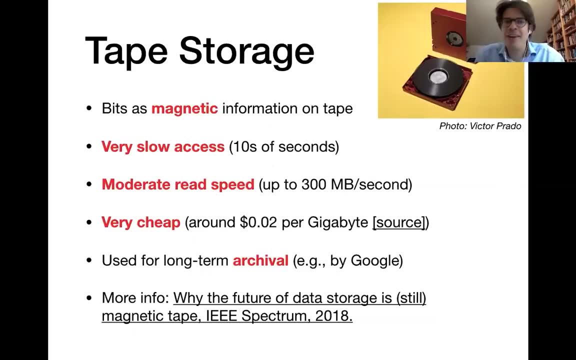 and get a sense a little bit for what those storage devices look like and what kind of properties they are featured. all right, so at the very bottom of that memory hierarchy we have a typically those tape storage devices and you see one of them in the right upper corner. now, those tape storage devices, they work according to. 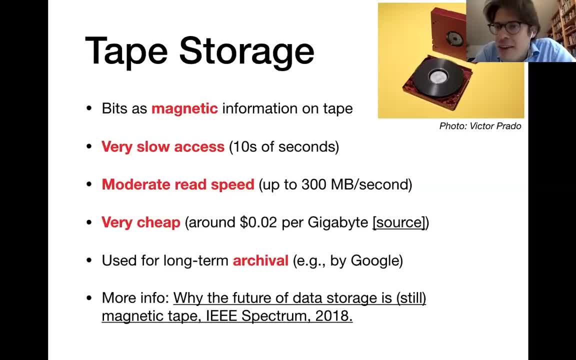 the same principle, basically, as those music tapes that are not very common anymore. but the problem- you have seen one already. they, those tapes, generally store information. they store bits as a magnetic information on that tape. now, once you have positioned your tape at the correct position where the data you're interested is, 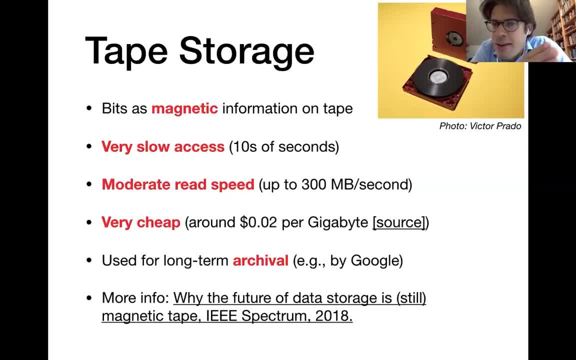 are that you are interested in is located at. in that case, you can get quite reasonable speeds for reading and writing data. it's not going to be fast, but it's. it's not going to be terrible either. the problem is that it might take quite some time until you bring your tape into the position. 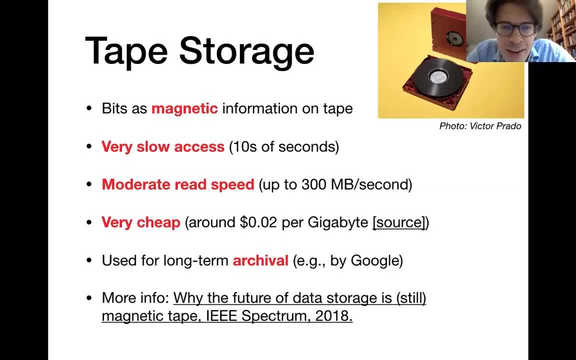 where the data you're interested in is located at. so that might take seconds, tens of seconds even, which, in the context of data processing, is completely awful, of course, but on the pro side, those tapes are extremely cheap. so i have put a couple of numbers here and please take those numbers. 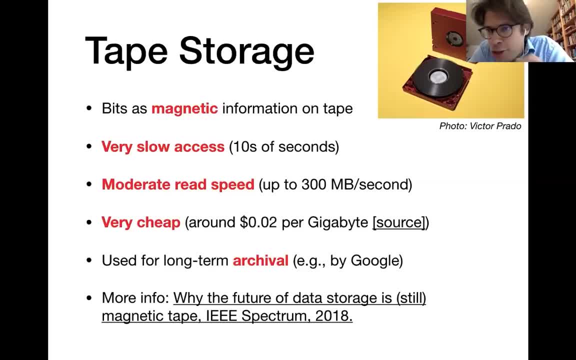 with a grain of salt because, um, they keep changing over time and it also depends on which specific devices you are considering. but i think that those numbers, they give you some intuition for how the different layers of the memory hierarchy relate to each other. for that the numbers are useful, but don't take them too serious either. so the 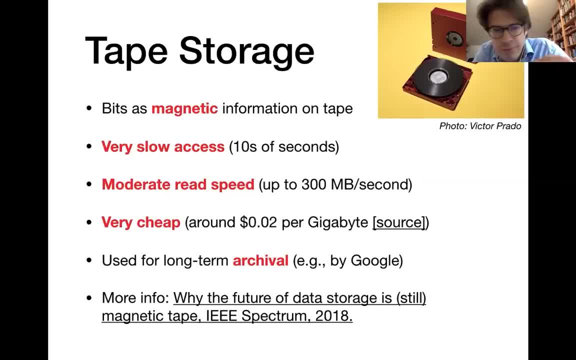 nice thing about tape storage is that it is very cheap. you can store a lot of data for um without paying too much money, and that's why it is quite popular for long-term archival storage. so also cloud providers like google, for instance, they um they would use tape in order to, in order to store backups. so we are not going. 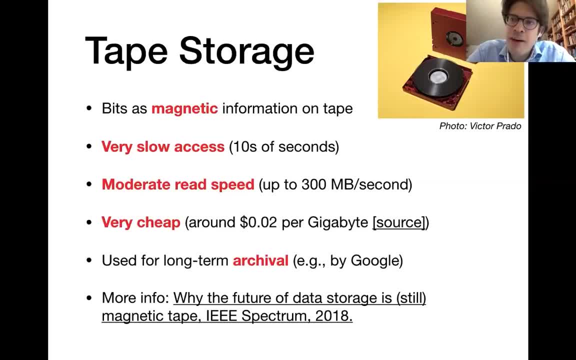 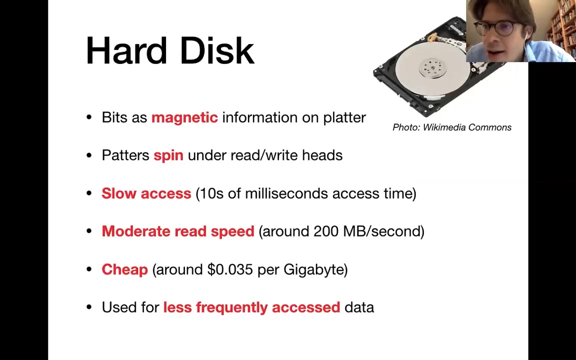 to discuss that much about a tape storage, because um, the database management system, typically assumes that you can access data faster than this. but if you're interested in reading up more, then here i have a link to a corresponding article in the slides. now the next higher level of the memory hierarchy, that is hard disk, and hard disk that is. 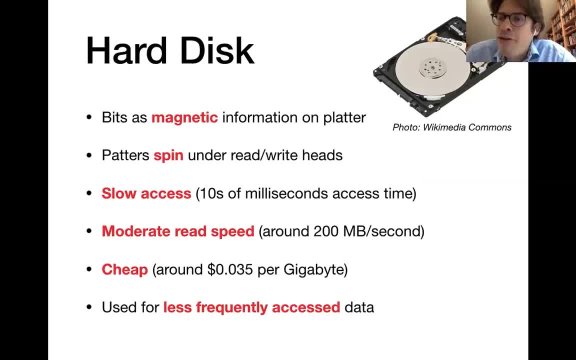 a popular storage medium and, uh, a large part of traditional database management systems. they have been designed under the assumption that the bulk of your data is actually stored on heart disc. hard disk represents bits in a similar manner as the previous storage medium- as magnetic information again, but this time we are writing this magnetic. 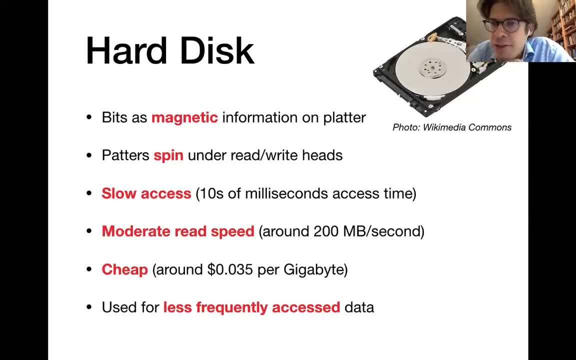 information on a round disk such as the one that you see on the right upper side. so you see, here there is indeed a round disk, or even multiple stack disks, in the middle of that heart disk, and in order to access data you're interested in, you have to do two. 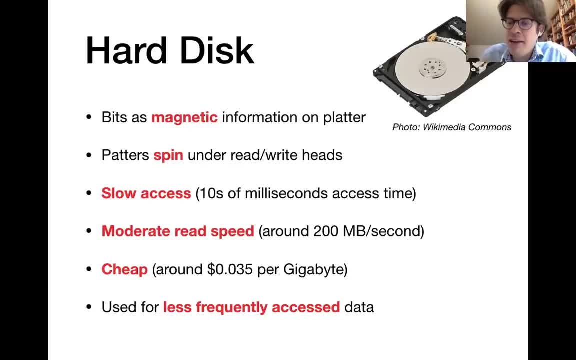 things. so, first of all, this disk containing the magnetic information. it is spinning with a very high frequency, thousands of spins per minute, and you're reading and writing data on that disk with so-called heads for which you can choose the distance between the middle of that disk and the head, So you can move that head into one direction in. 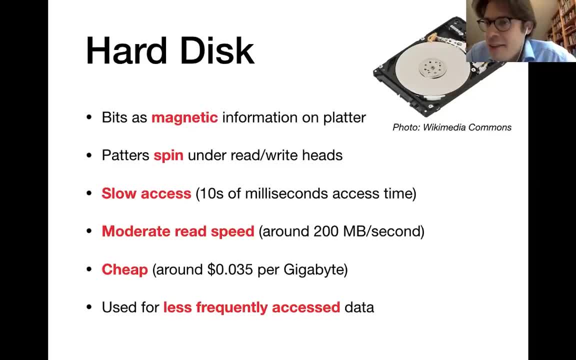 order to access different parts of the disk. and as the disk is already spinning, once you have positioned your head properly, you just have to wait, essentially until the data you're interested in comes rushing by as the disk turns. So once we have positioned those heads properly, then 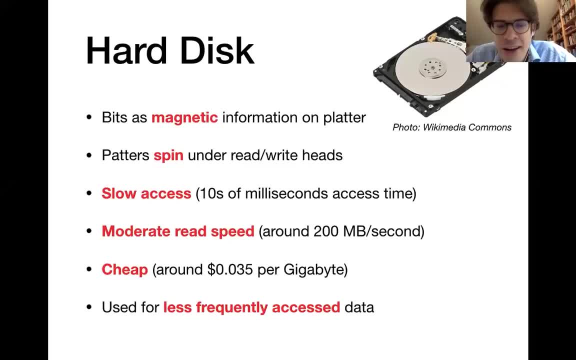 again, we can read data at reasonable speeds and write it at reasonable speeds. Again, one problem is that it can take a little bit of time to position that read write head properly. It can take some tens of milliseconds, which is, of course, much faster than before, but still. 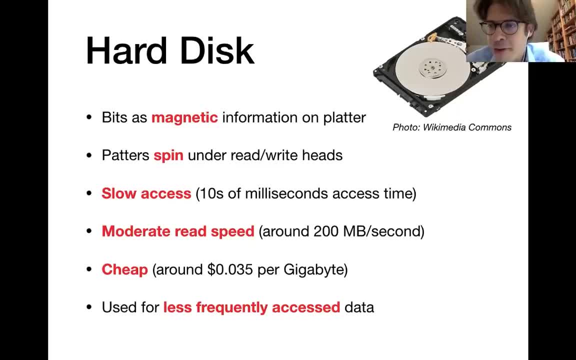 in the context of data processing it is kind of long. so hard disk is not considered a very efficient, high-performance, at least in terms of speed. let's say it's not considered the medium of choice On the pro side. again, it is more expensive than tape, but it is still quite cheap. so that's why you. 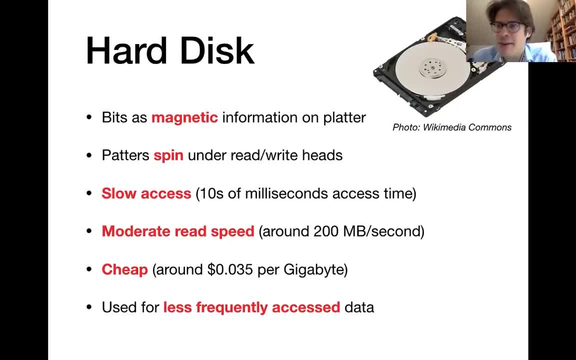 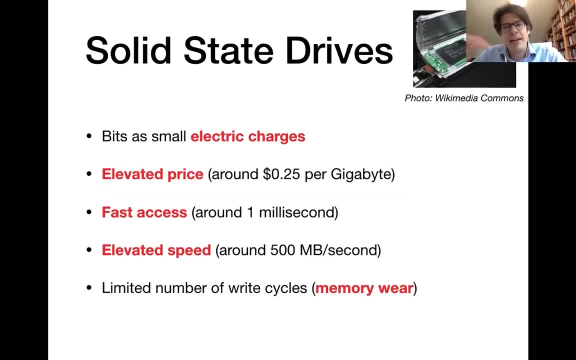 might want to use it for less frequently accessed data and indeed traditional data management systems. they assume that you typically store the data that is not immediately used on hard disk. A little bit over the hard disks are those solid-state drives which use a different technology to store bits using a small electric charges. They have a 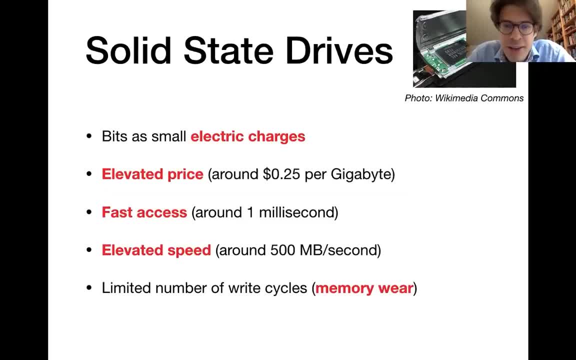 comparatively elevated price Here. those numbers are already slightly outdated, but you see they are significantly higher than for a hard disk. You have in exchange a pretty fast access because we don't have any moving parts. you don't have any mechanical parts that you need to reposition, like the disk heads for instance, and you can also. 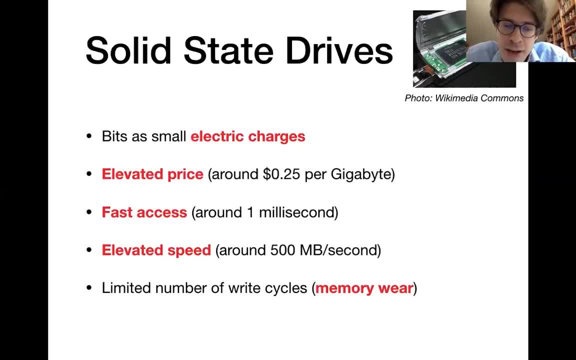 at least read speeds at quite an elevated rates, let's say. One problem with those devices is that the number of write cycles that you can do is limited. They wear out. but people have been looking into techniques in order to at least partially overcome that, in order to, for instance, have some spare capacity. 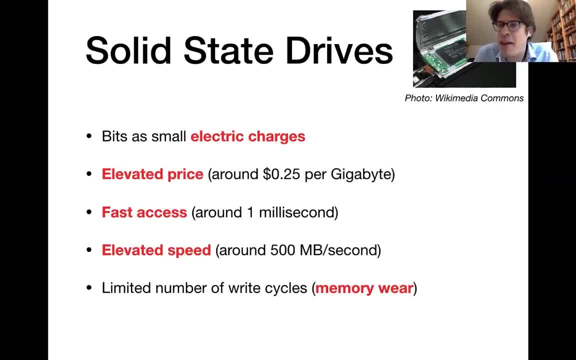 in order to replace cells that fail because you have too many writes on them and to try to partition the writing load equally on those devices. We're not gonna discuss it into much detail, but just to give you some little overview of the pros and cons of that as storage technology. 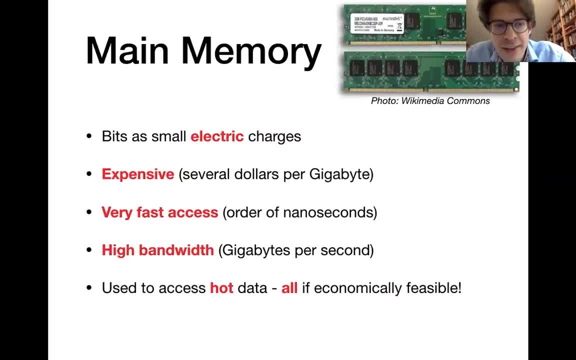 Main memory. that is the next level of the memory hierarchy and here we have a big jump in terms of access speed. again, you're storing bits as a small electric at charges and compared to the other storage media, main memory is quite expensive for storage methods. 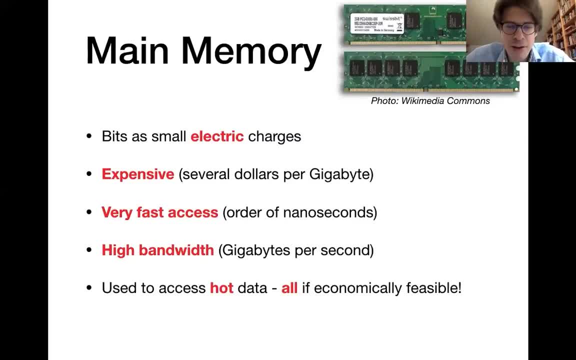 For storage, if you look at the price per gigabyte, for instance. but on the other side you have some very fast access times. You can read and write data at a relatively high bandwidth. So this is a very significant difference to the storage media that we have seen before. 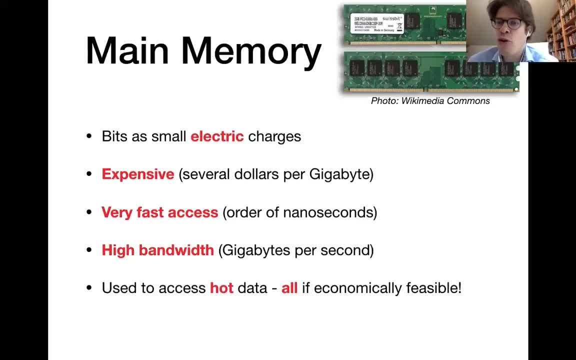 So traditionally, main memory is used in order to hold data that you're immediately Working with, and if you can afford it nowadays and want more, people are even able to fit entire databases into main memory. if you have Hundreds of gigabytes or terabytes of main memory, that might be feasible. Of course, you have to pay a little bit for it. 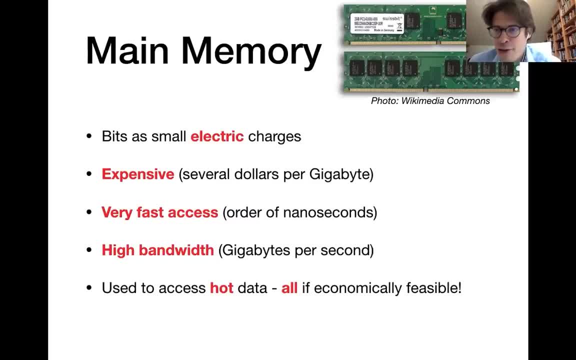 so there's a big jump in terms of access efficiency between Hard disk- in particular also SSDs- and main memory. so in traditional database management system design we are actually assuming that that The main overhead when it comes to data movements is for moving data From hard disk into main memory. and, as we will see in much more detail later, 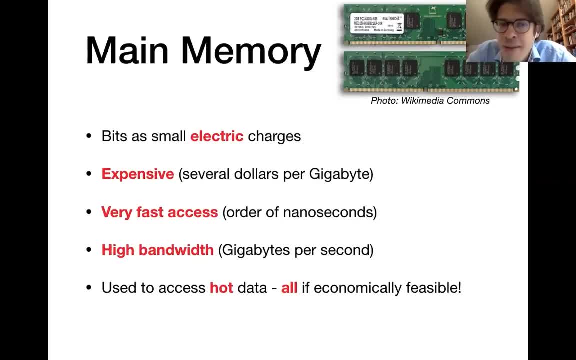 therefore, We try to be efficient about When and what data we move from hard disk into main memory. So Main memory and a hard disk- Those are typically Considered one for storing the bulk of your data once, for storing the data that is immediately relevant, Even if nowadays, more often, you can fit significant parts of your database into main memory. 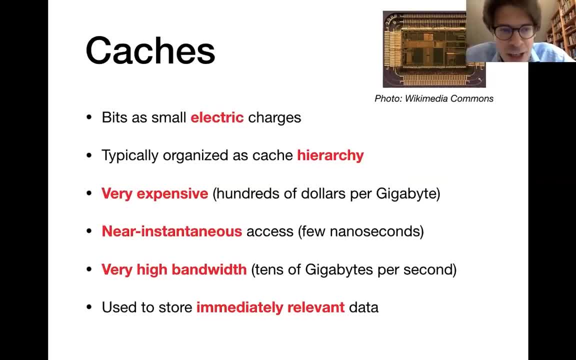 finally, you have the CPU caches, and they are typically organized as a, So you have not only one cache, but you have L1, L2, and L3 caches, and from L1 to L3, typically we increase the capacity, but access time increases as well. 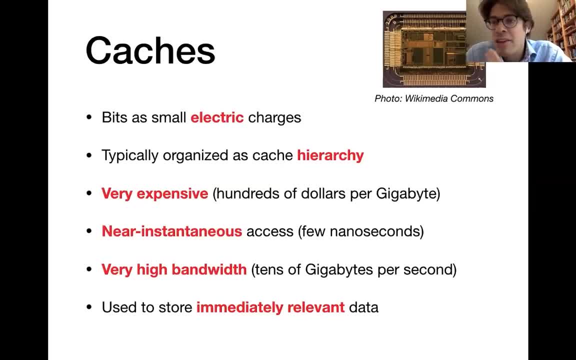 Now, clearly those caches are very expensive per gigabyte so we cannot make them all too much. but on the pro side they offer essentially near instantaneous access and very high bandwidth. So that data is typically currently being used for some operation, or it has at least. 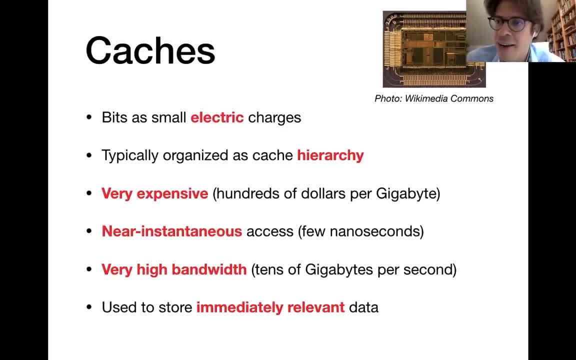 been used recently or it is close to data that has been used recently. So you cannot fit that much data into those caches. but if you can fit data into it then you have extremely high access times And that makes it very efficient. 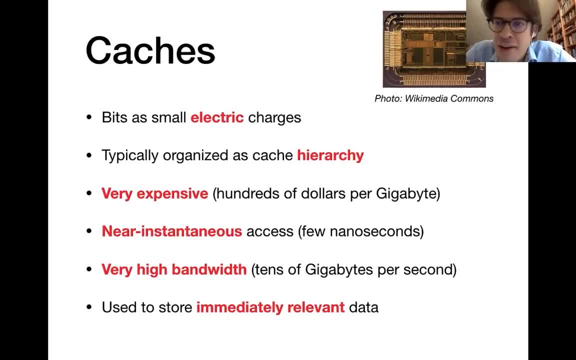 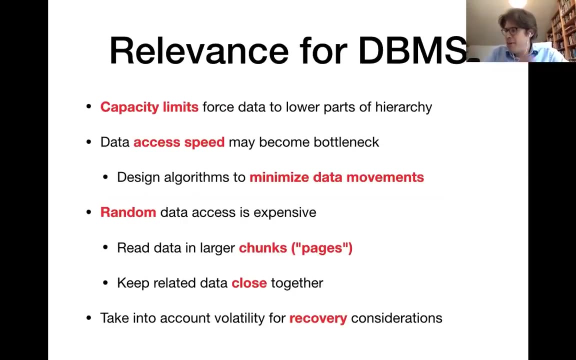 Now the final layer of the memory hierarchy, that would be the registers. but I mean the registers. they are basically what the processor can access immediately, So I'm not going to discuss this in detail. So now we have seen a little overview of the different storage layers in your database. 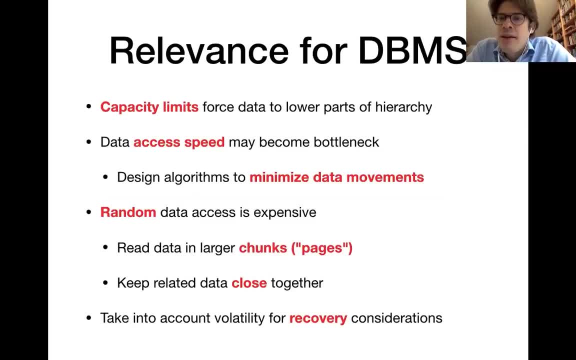 management system. But we want to discuss about database management systems. it's not a hardware code, right? So I mean, how does the properties of those storage layers relate to design decisions that we make in a database management system? And it will turn out that during for the next couple of weeks, many of the things that 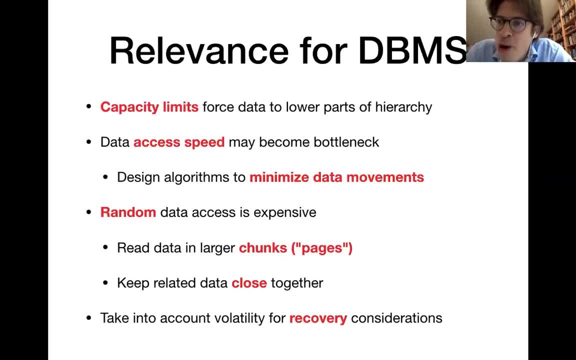 we will be discussing. they only make sense due to the property of those storage layers, And so I want you to internalize those high-level points that I'm noting down here, which illustrate a little bit how those storage media properties influence the design of database management. 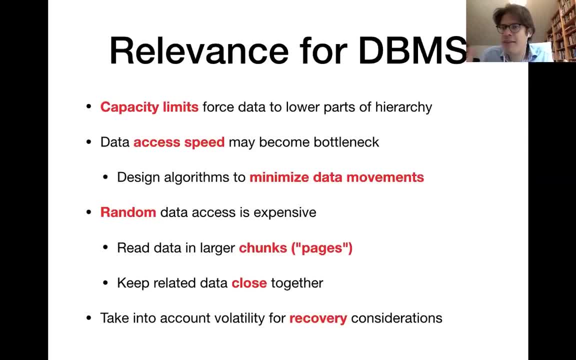 systems. I mean generally. what we have seen is that the capacity of those upper layers of your memory hierarchy is limited, And that means that you have a lot of data, You have a lot of data, You have a lot of data. Since we are generally dealing with large datasets, we have to assume that at least. 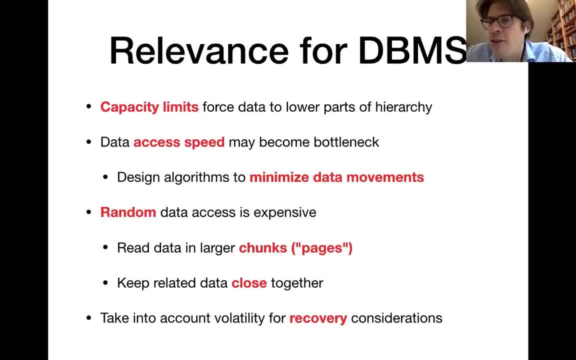 one part of our dataset is stored on one of the lower parts of that hierarchy where we have some significant access times. And that is important because typically, if you have been looking at algorithms like sorting algorithms, for instance, you have been looking at the number of computational steps that 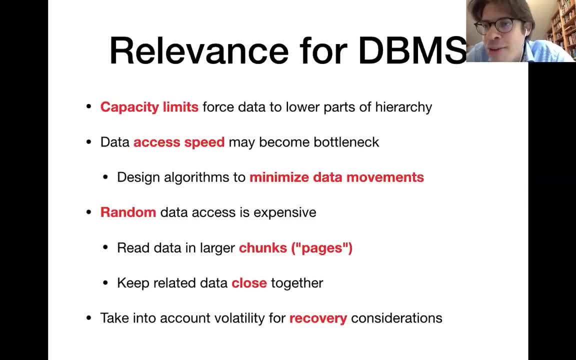 they are performing. We have compared different algorithms by how many computational steps we are performing. But in the case of databases, if you're dealing with very large datasets, then because you often cannot fit them into the efficient layers of the memory hierarchy, you have to account. 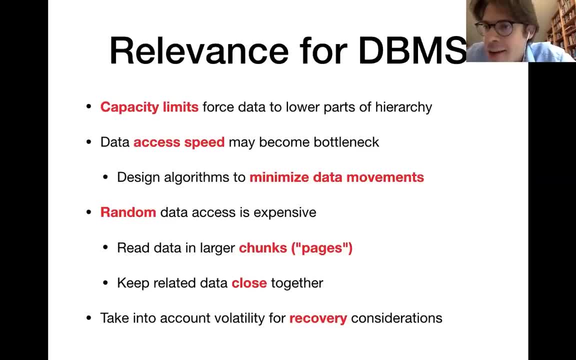 for overheads, just for accessing data, not even doing the computation. If you have, for instance, your data located mostly on hard disk, then just the time for accessing that data is limited. But if you have a lot of data, for moving data through the memory hierarchy, that often 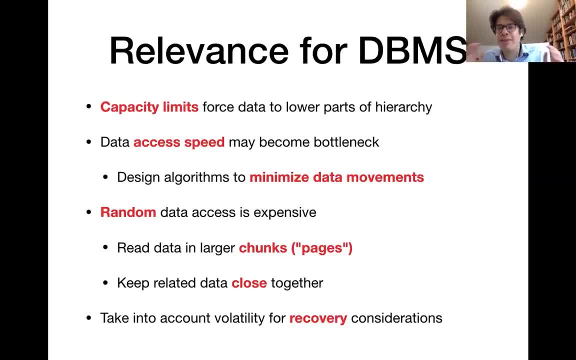 dominates your total execution time, And this is why many of the algorithms that we will see in the following that are used by database management systems. they are not optimized for minimizing the number of comparisons, for instance, But instead they are really optimized for minimizing how often I need to load data. 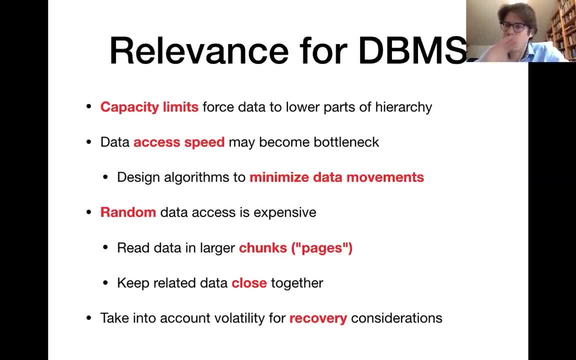 for instance, from hard disk. Right, So we want to design our algorithms in order to minimize the number of comparisons. Right, So we want to minimize data movements, Another property of those devices. we have often separated the bandwidth for reading and writing data and the time for accessing data that was located, for instance, somewhere. 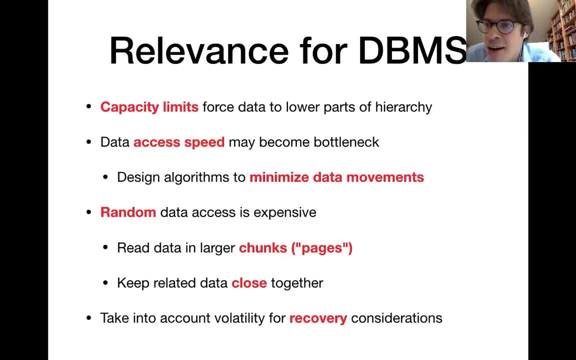 on the disk And then in order to access some random location in your data you have to do things like rewinding the tape or like repositioning Your disk head and those things. they cause quite some overheads. So random data access is often very expensive with those storage media. 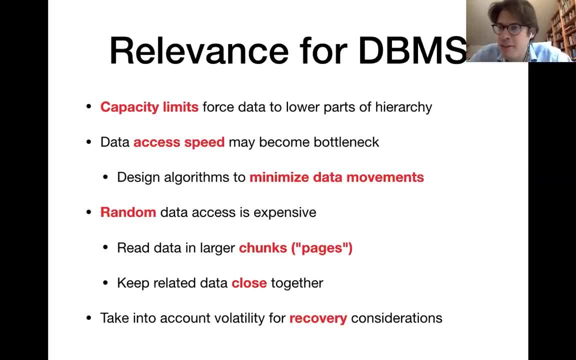 So that's why, once you have already repositioned your disk head, you don't want to read one single bit, but you want to read a reasonable chunk of data to make it worth your while to pay for all that overhead. That is why we will see in the following that we are 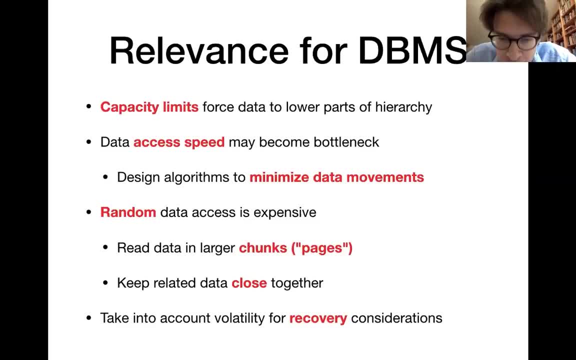 We are generally accessing data in chunks of data, which we will also call pages in the following, And the reason is that doing that is often more efficient than accessing a very small units of data. Another thing that we will see later is that, because we can quite cheaply read data, that 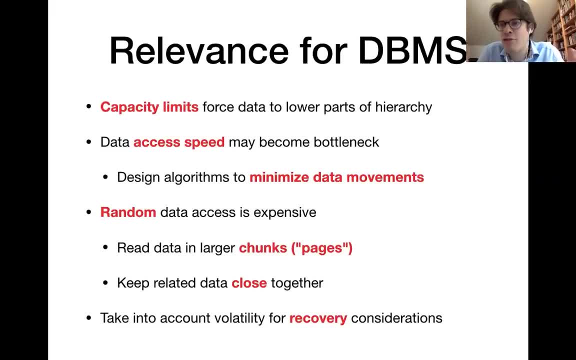 is close together. for hard disk, it doesn't require you to reposition your disk head, for instance Right, So you can read close by data quite efficiently. And that motivates us to design data structures that keep related data close together in order. 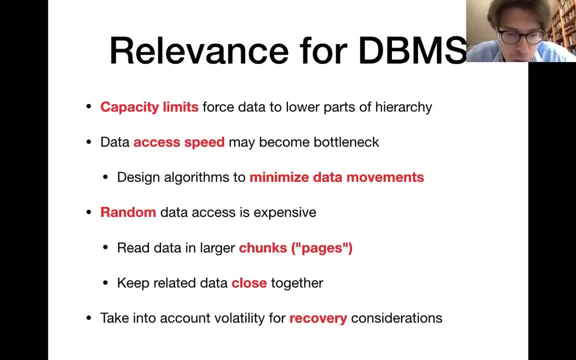 to make the access more efficient. That's also something that we will see in the following, And one topic that we will discuss about much more in later lectures of this course is the topic of volatility, because once a database processes updates, as long as those updates. 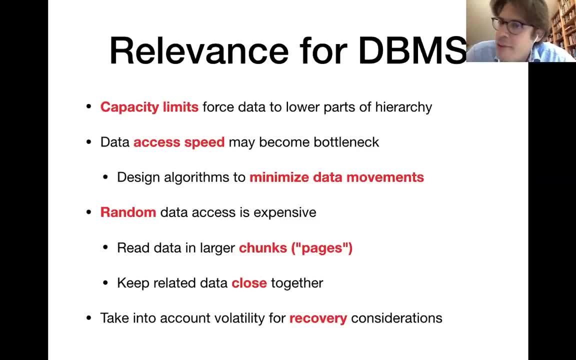 are only written in main memory. They could get lost if your server suddenly loses power, for instance, And database management systems. they use quite sophisticated strategies to make sure that your updates are secure and that, even if you suddenly lose power or some other catastrophe. 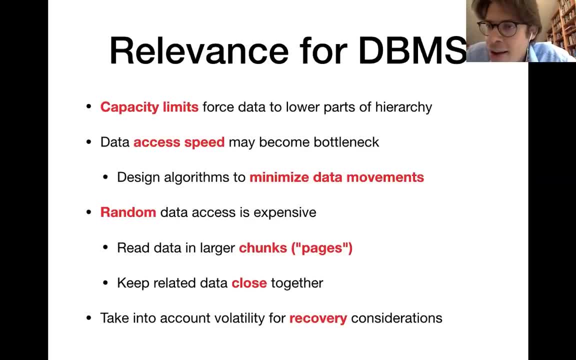 happens that your database remains in a consistent state, And those strategies need to be very aware about which level of the memory hierarchy your data currently resides on, Whether that level is volatile- meaning it loses data once the power switches off- or not. So I want to end with those high level points. 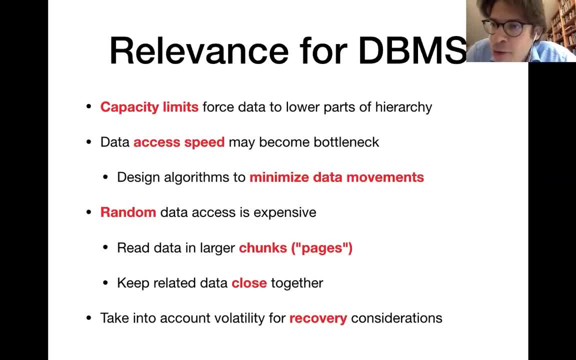 Please internalize them, because without them many of the things that we will do in the following lectures, they won't make that much sense. So I often get questions about why we do things in a certain way, which could be answered by those high level points here. 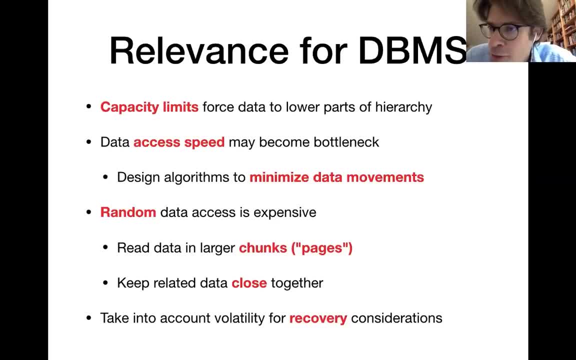 The next time we're going to look more into data storage formats and we're going to start with indexing over the week, And I encourage you to revise the material that we have seen about secret queries, because on Monday next week the homework which focuses on secret queries will come out. 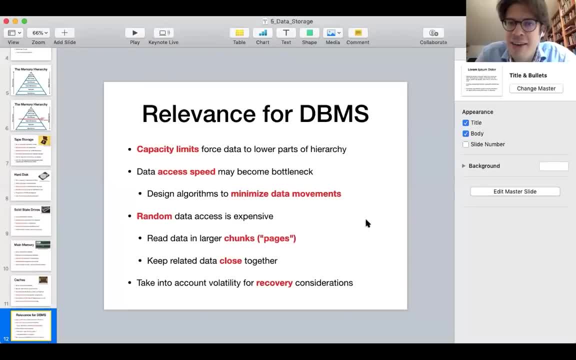 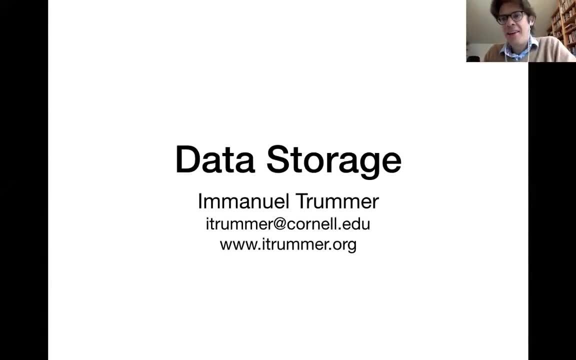 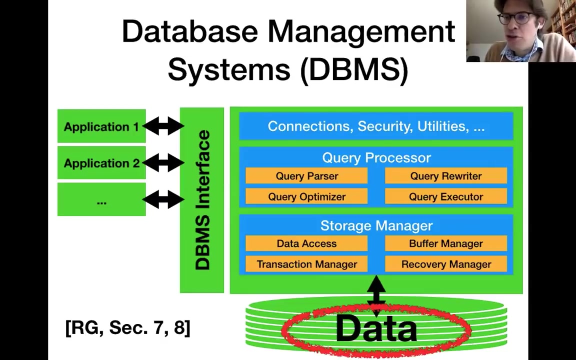 All right, have a nice day, and I wish you a nice weekend, and then we'll see you again on Monday. Hello everyone, Bye, Let's get started here. And the last time we have been talking about data storage, Last time we have mostly focused on the hardware on which your data is stored. 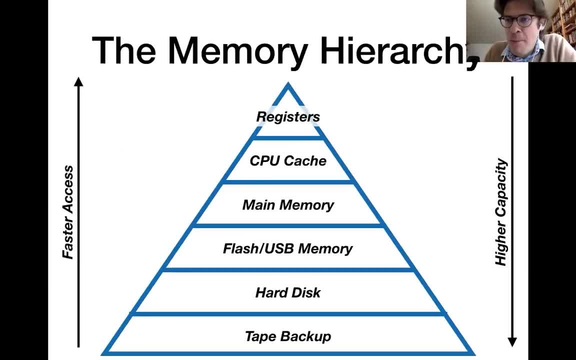 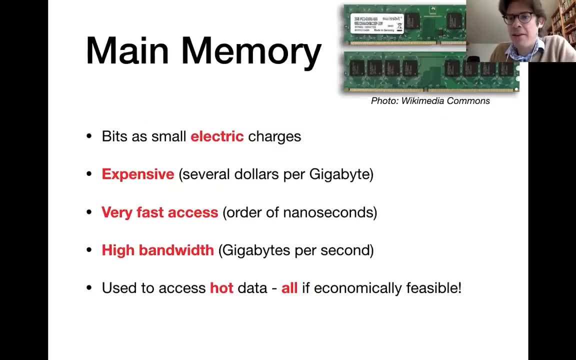 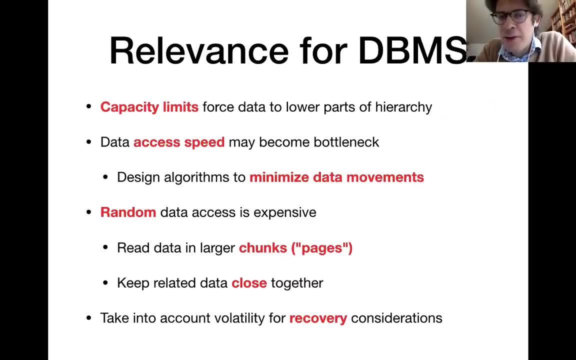 We have quickly seen the memory hierarchy and we have discussed about a couple of different common data storage devices and their pros and cons and use cases. I have ended with this light over here, where I summarize certain common properties of those data storage devices and summarize points that will become important when we discuss. 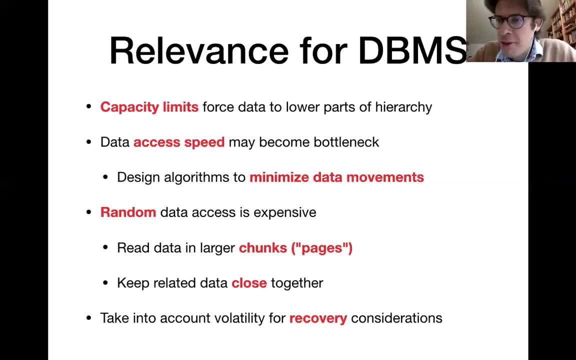 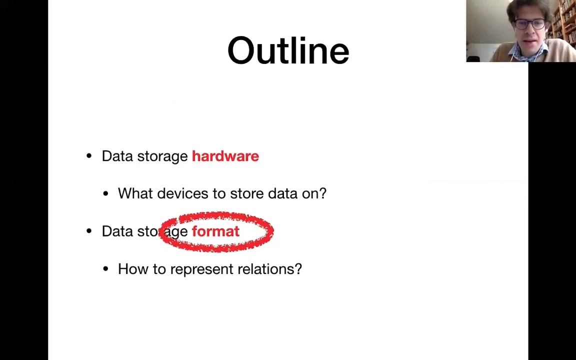 about the design of database management systems, because a lot of that design is motivated by properties of the data storage hardware. This time I want to discuss little bit more about not where the data is stored, but how the data is stored. We're going to discuss about different data storage formats Now so far, when we 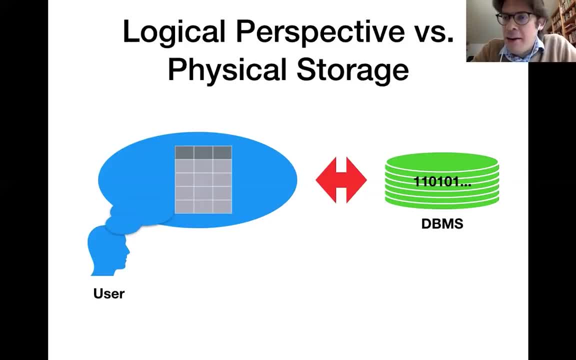 have been learning SQL, then you have thought about your data in the form of tables, with different columns and rows stored in those tables. Of course, internally we use a more low-level format. You have to somehow map this high-level perspective on the data to how those, to the bits and bytes that are. 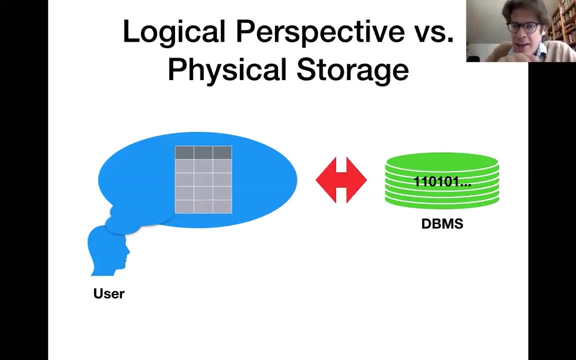 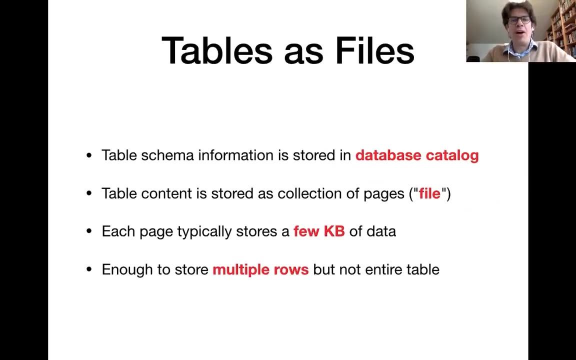 actually stored. So in the following we're going to discuss about this connection, about how we can map those, this logical perspective, to the physical storage reality. All right, So generally, for a given table, there's two things that we want to store. So 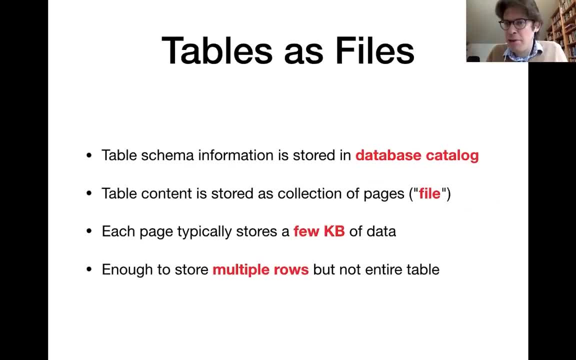 first of all, we have the structure of the table, the schema meaning, like the column types and the constraints on the table. Now this kind of information is stored in something called the database catalog, So that is a central repository of the database. This is where it maintains certain metadata about all the data, that is. 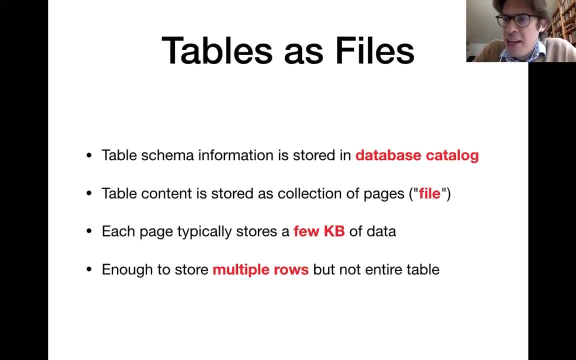 stored. The actual content of a table is stored as a collection of pages, And one of those pages typically fits a few kilobytes of data, So one page essentially corresponds to a chunk of data stored at one specific location on your storage device. 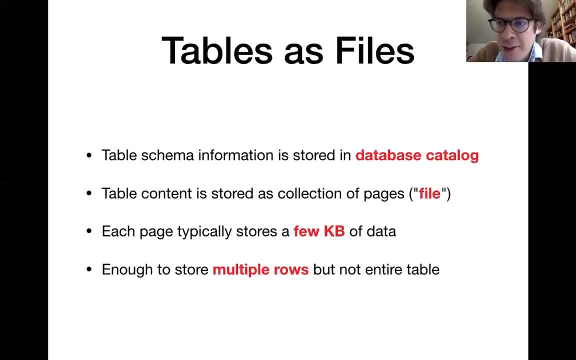 And the size of those pages is chosen in order to maximize a retrieval efficiency from the corresponding storage device. We have, for instance, seen for hard disks there's a certain overhead in repositioning your read and write head. So once you have repositioned that you don't want to read only a single bit or 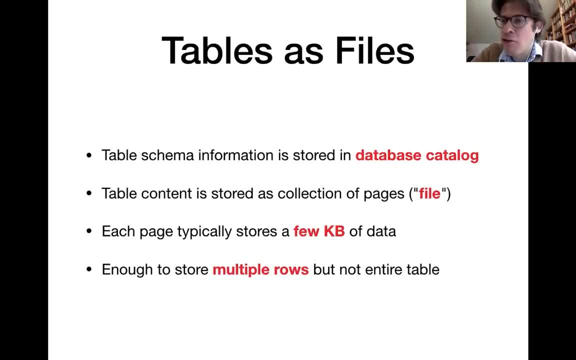 byte, but you want to read a little bit more data in order to make it a worth it, And so those pages they are. they have a granularity that makes it somewhat efficient to retrieve and store a data at those quantities, right? So one of those pages is typically not large enough to fit all the data from a 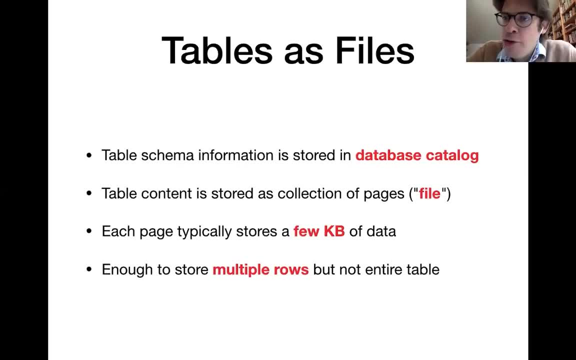 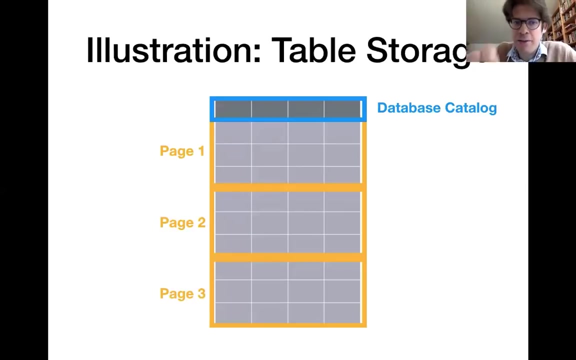 relation, but it is typically large enough in order to store multiple rows from one relation. So that means that in order to store one table, we have multiple pages where each page stores multiple rows and we have to somehow keep track. So this is an illustration of what we have just discussed. So the metadata about the table. 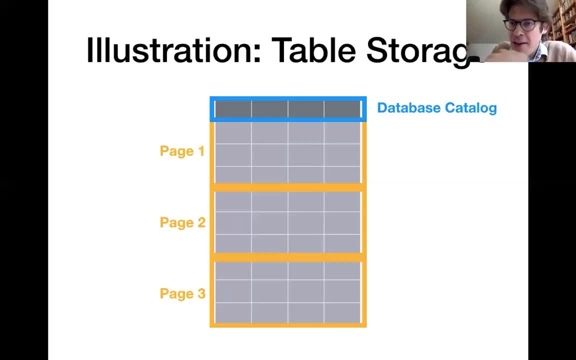 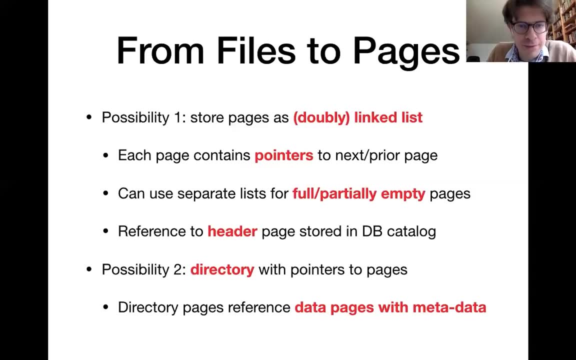 schema which I associate with the table columns. that is stored in a database catalog and then the content is stored as a collection of pages. All right, So we have multiple pages that store rows from the same table. we have to somehow keep track which pages store information for a given table. 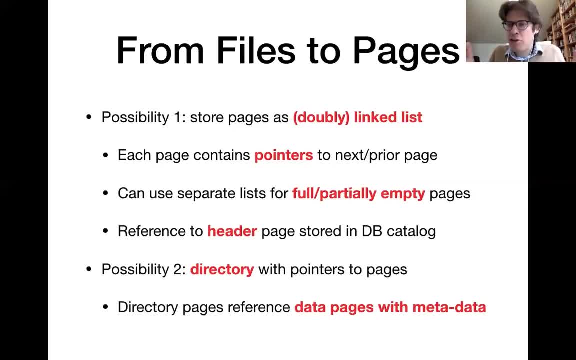 so all those pages together which contain data from the same table. they are called a file. which pages belong to a certain file? there's multiple ways of doing that now. one first possibility is that we store those pages that belong to the same table as a linked list, meaning that one page essentially contains pointers. 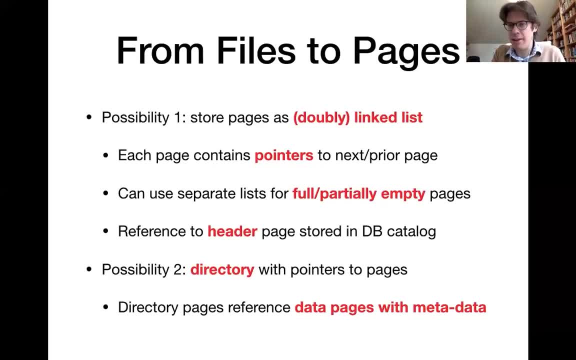 pointing to the next and to the previous page, and so if I want to retrieve the data within a table, I just follow those pointers and read all the associated pages. now, that's the first possibility. a second possibility is to rather store a directory, which essentially are pages, again that store references to those 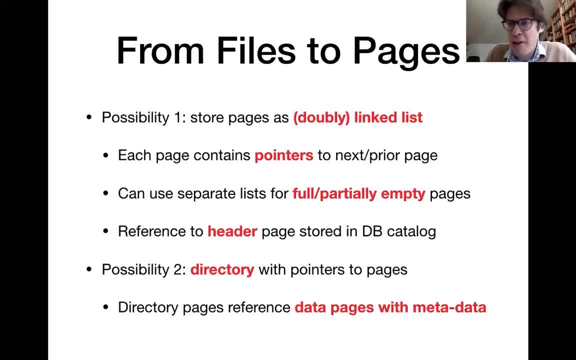 data pages. when I'm following, I'm gonna illustrate those pages and then I'm going to show you how to do that, and then I'm going to show you how to do that, and then I'm going to do that, and then I'm going to show you how to do that, and then I'm going to. 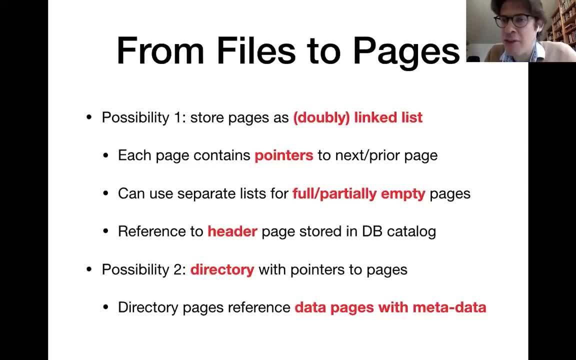 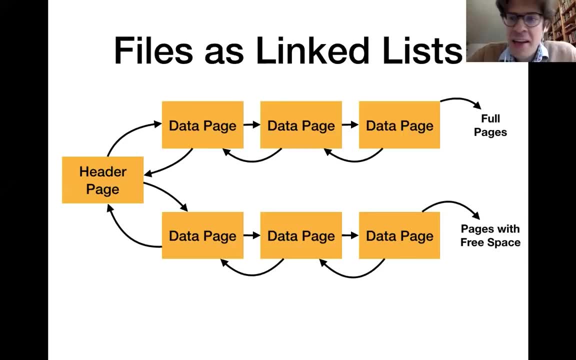 two possibilities. so the first possibility was that we store a linked list of pages. this is how that would look like. so we have so called header page, which essentially that's the starting page if I want to retrieve data from the table, and then, in order to make things more efficient, I can actually 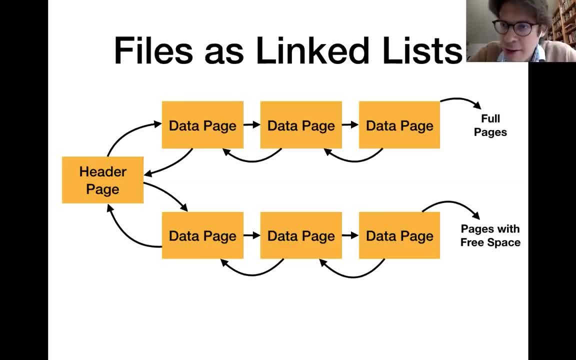 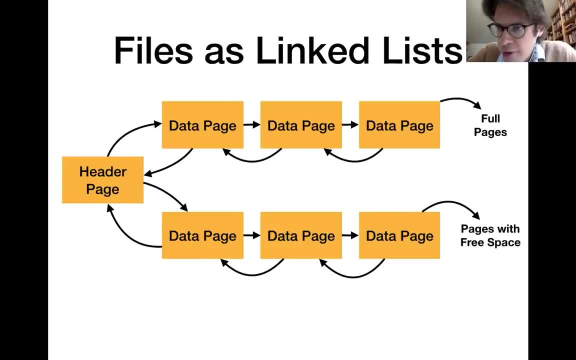 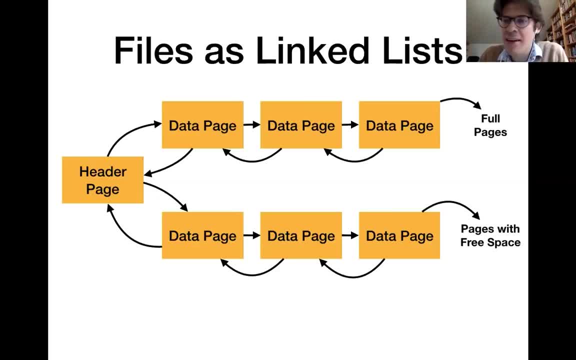 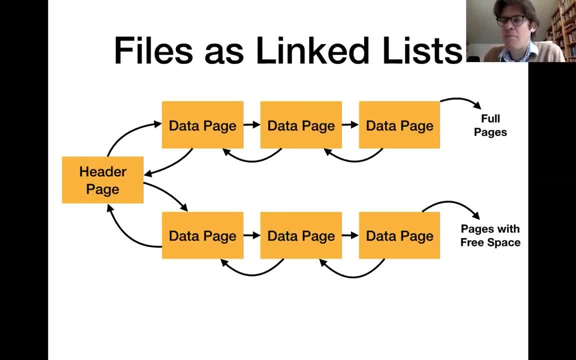 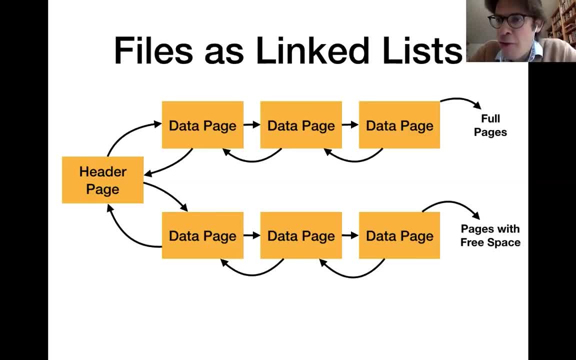 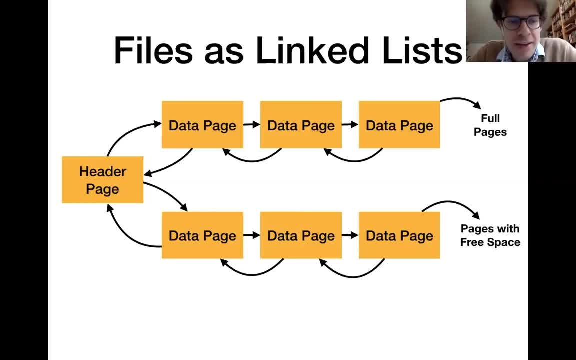 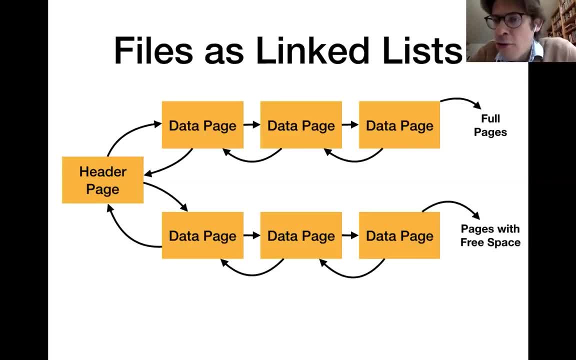 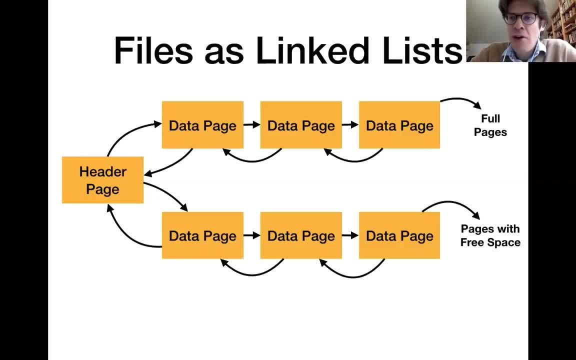 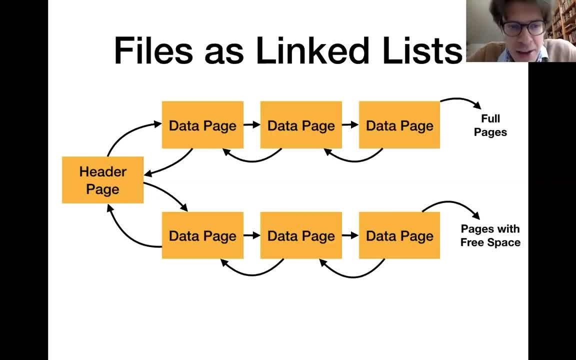 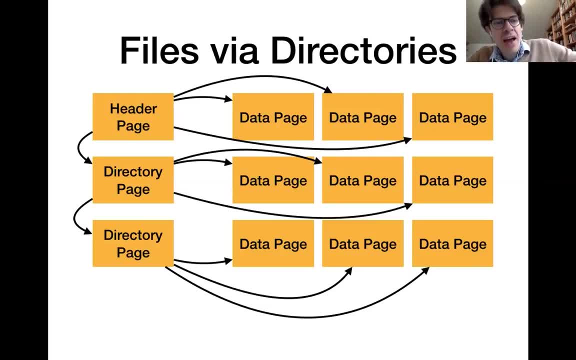 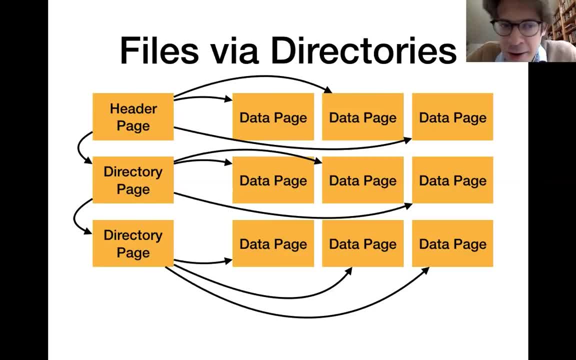 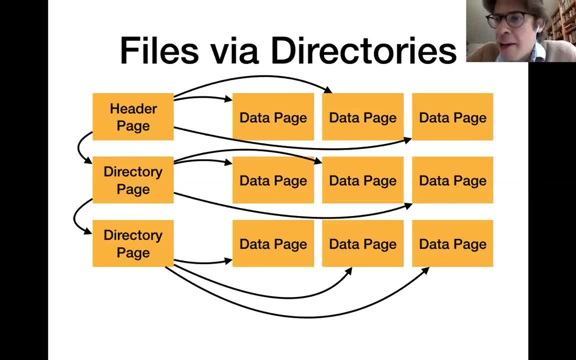 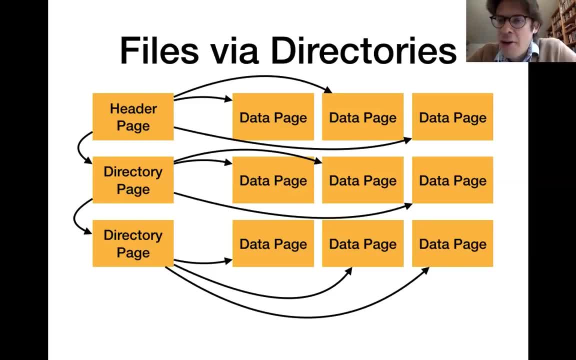 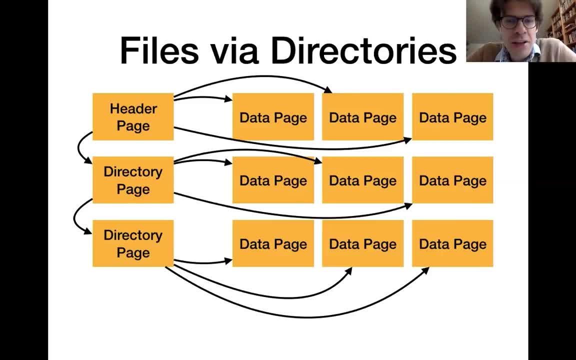 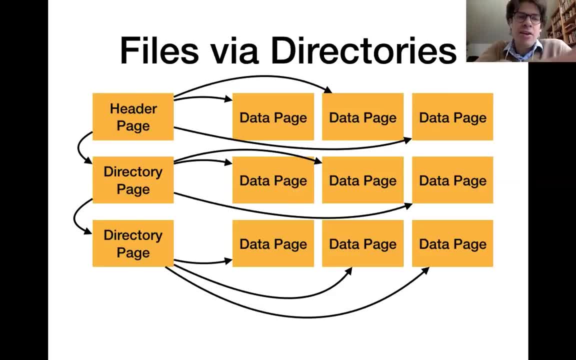 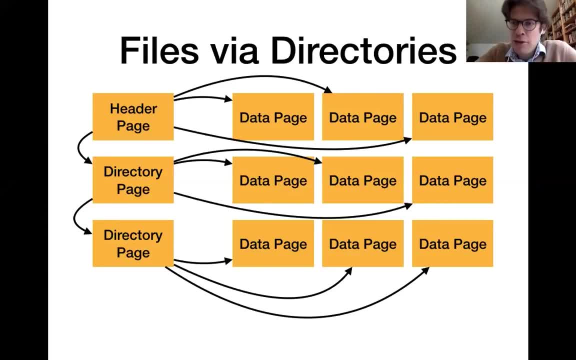 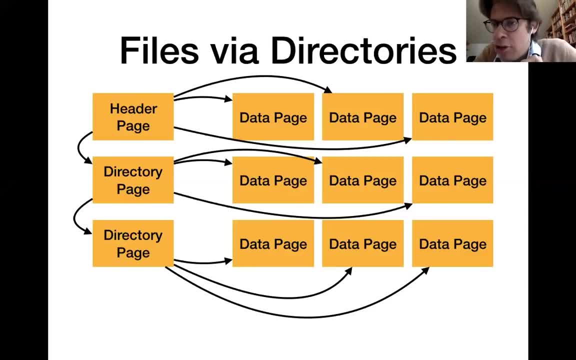 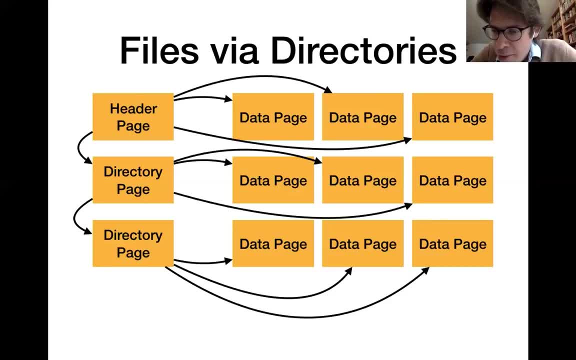 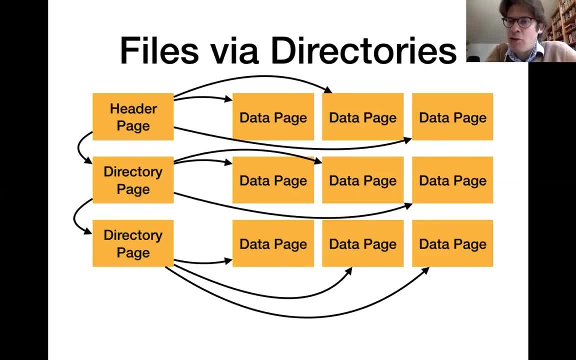 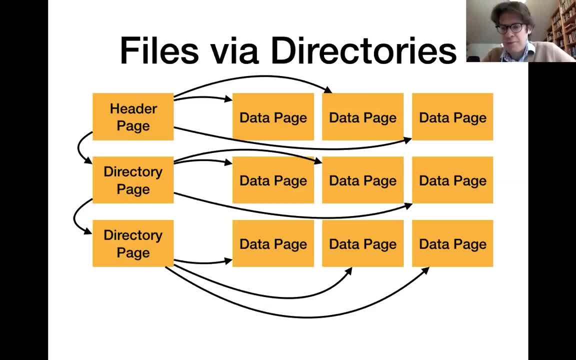 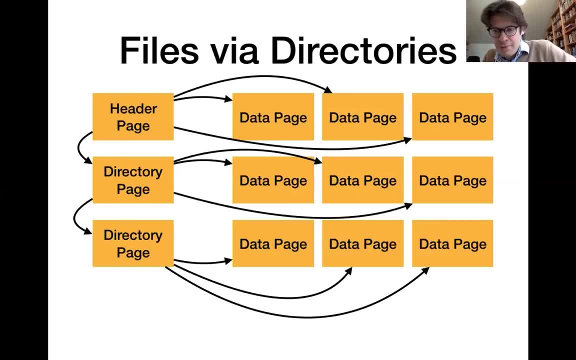 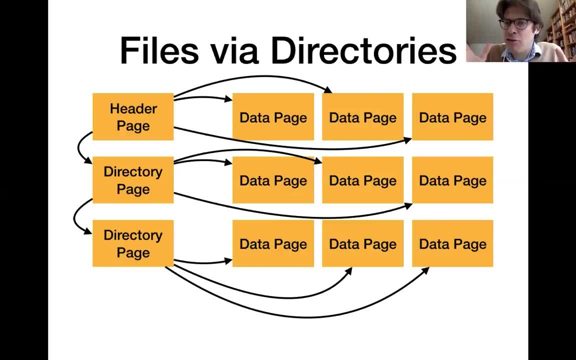 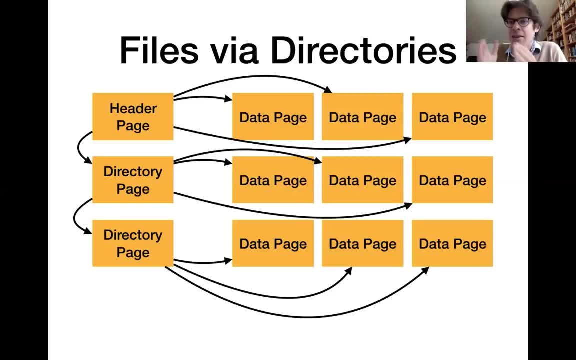 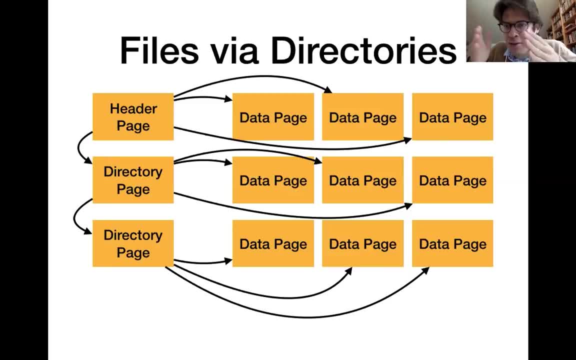 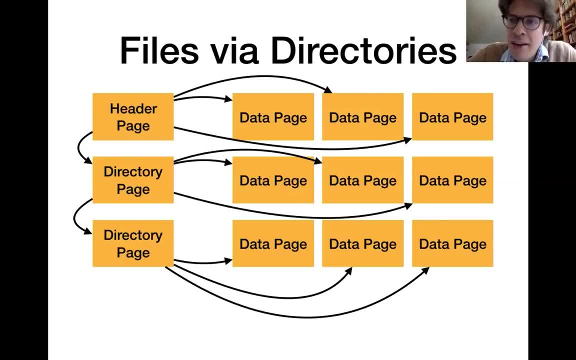 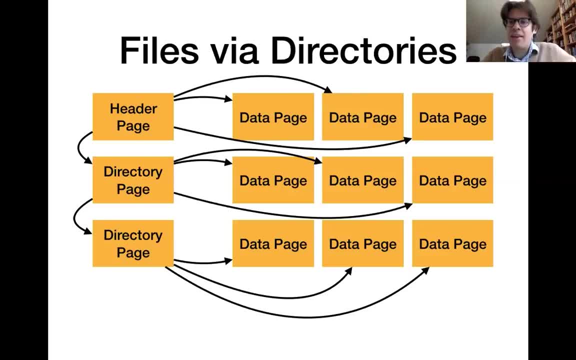 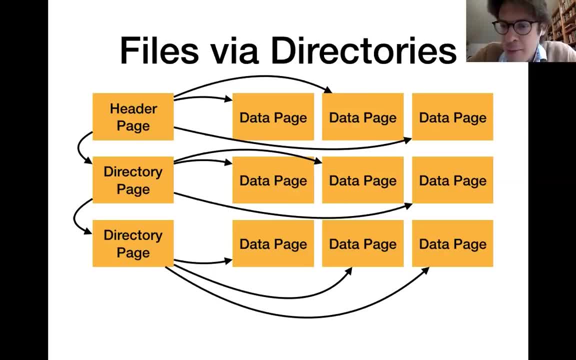 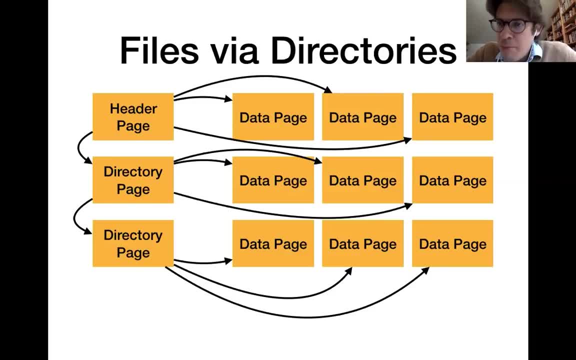 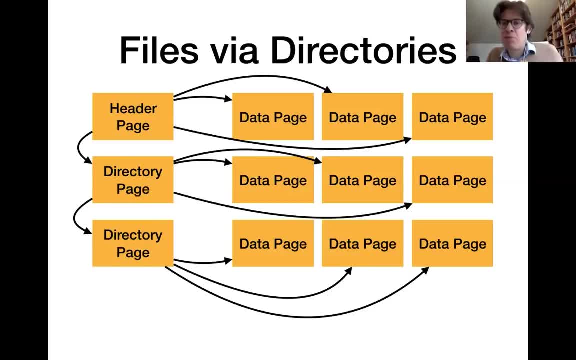 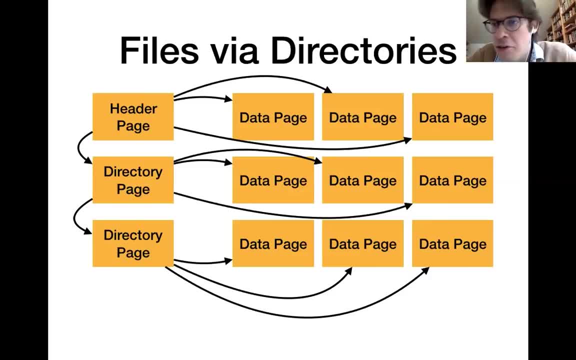 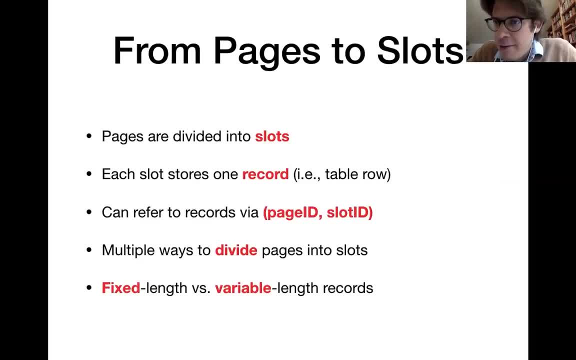 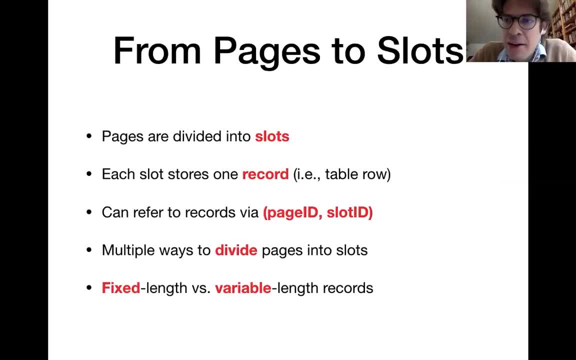 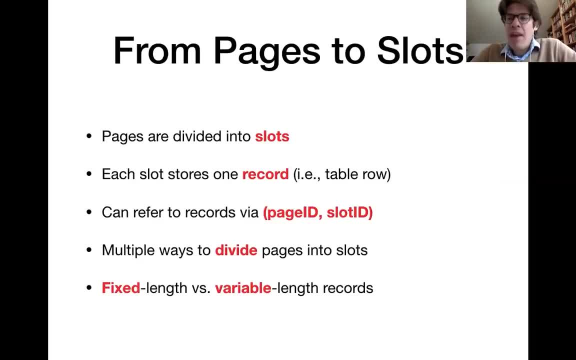 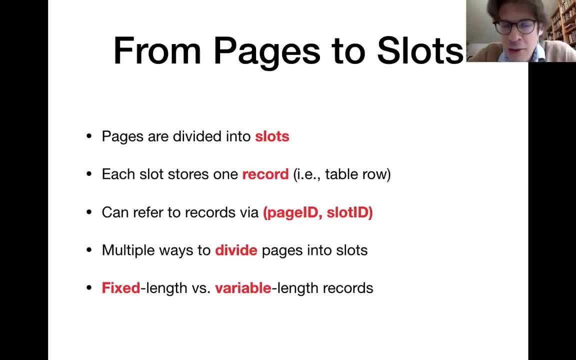 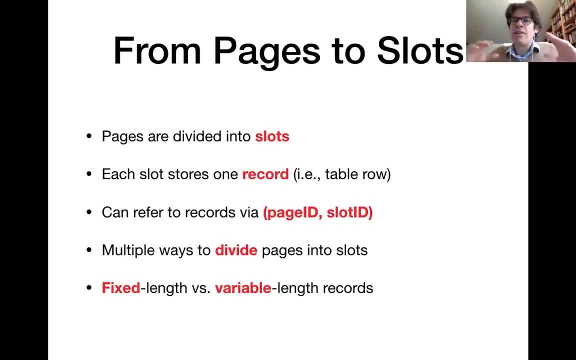 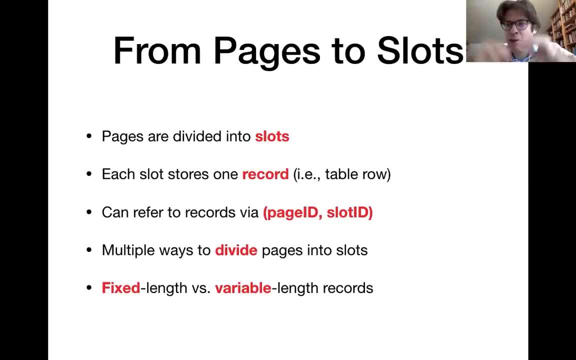 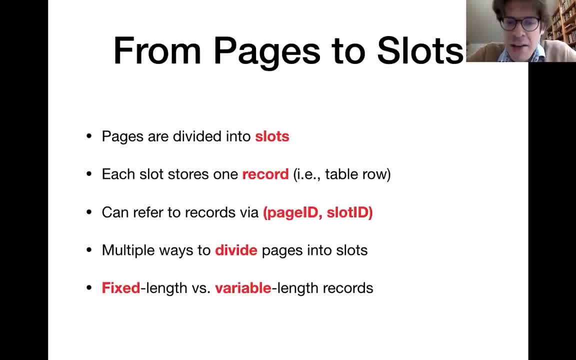 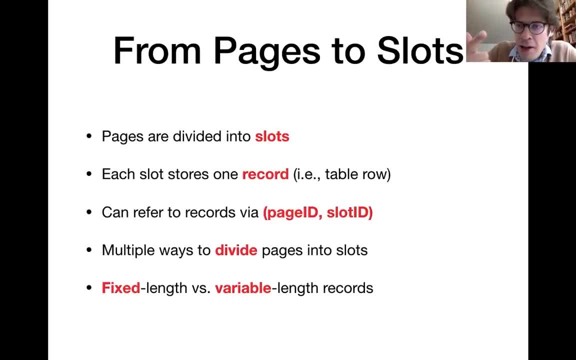 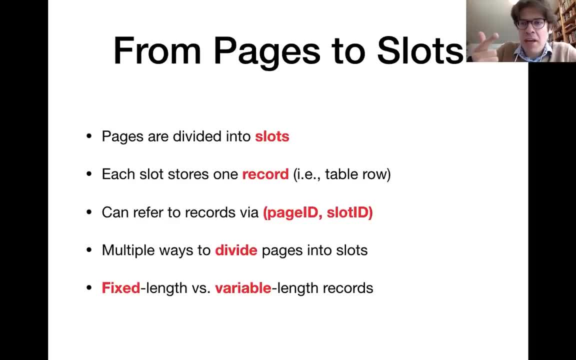 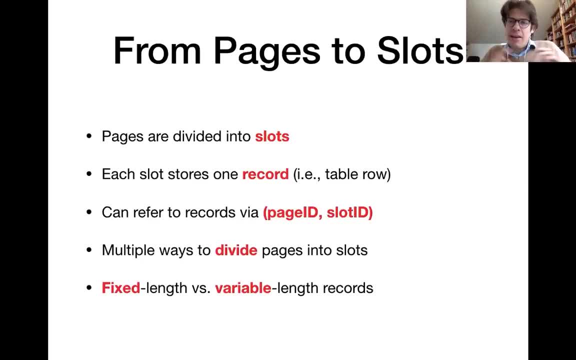 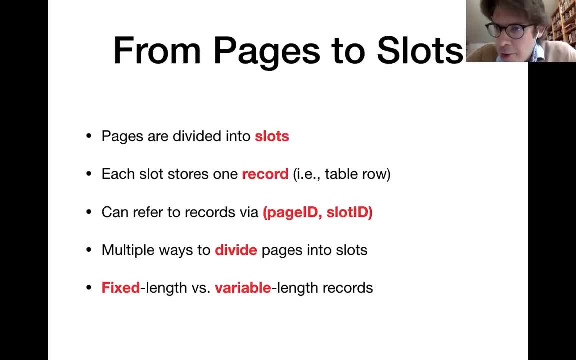 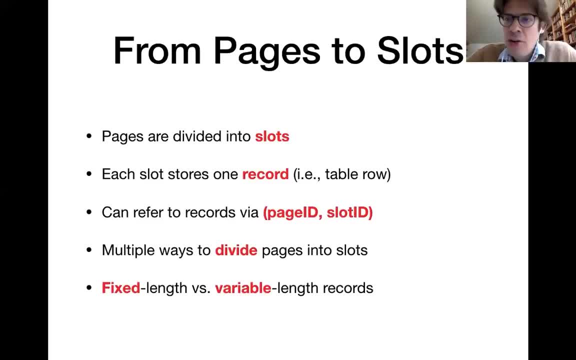 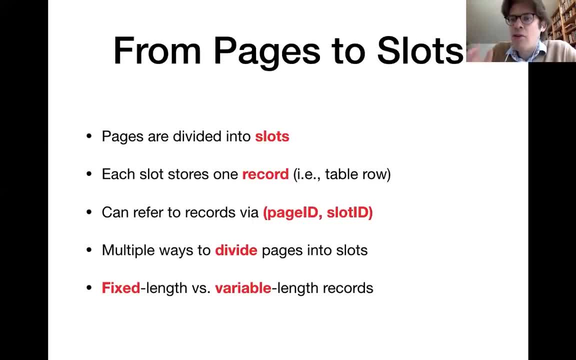 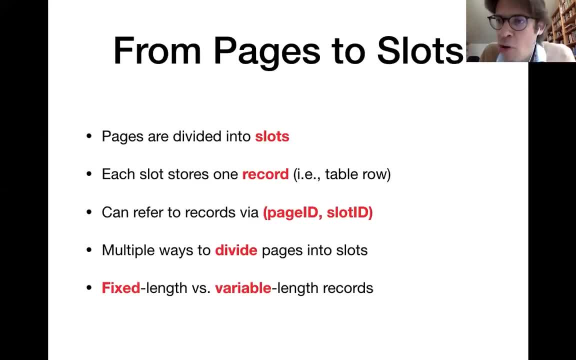 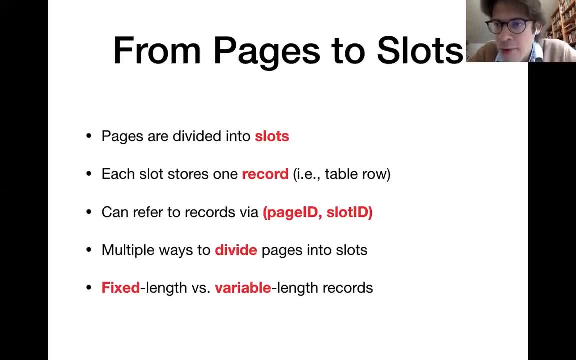 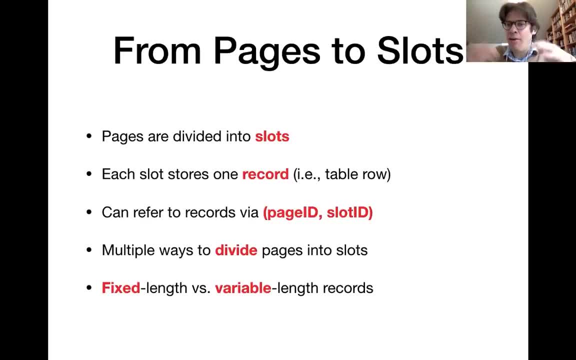 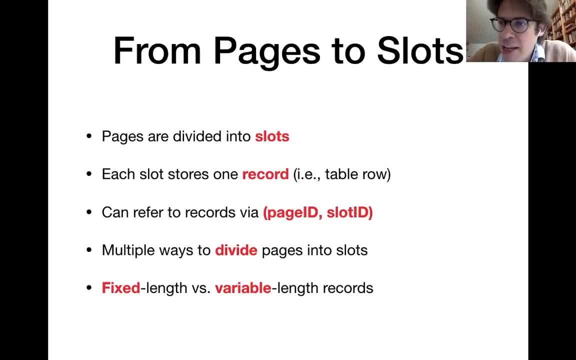 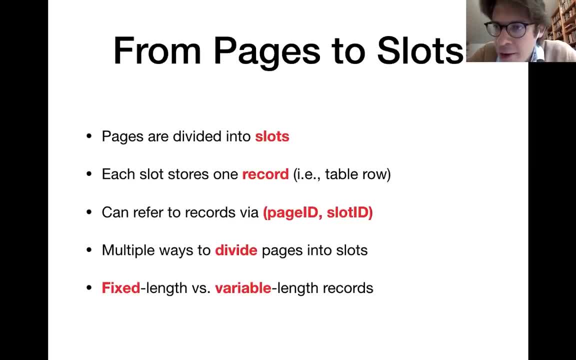 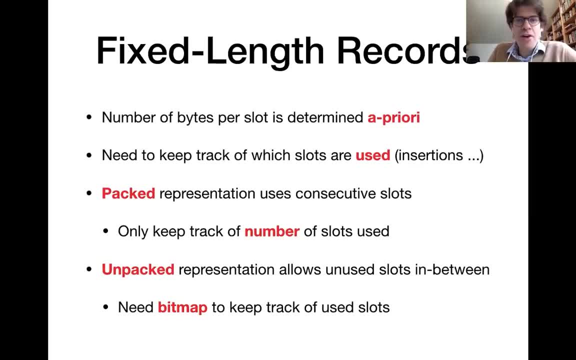 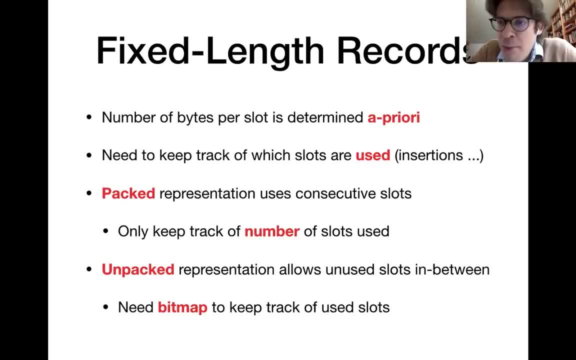 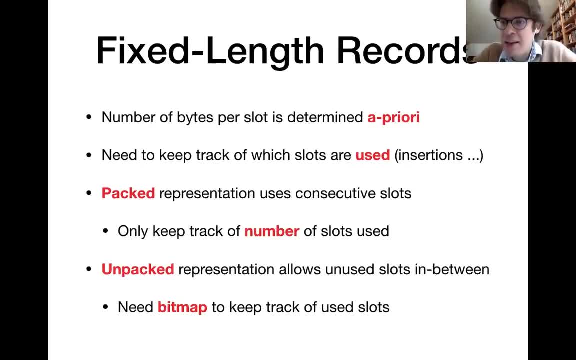 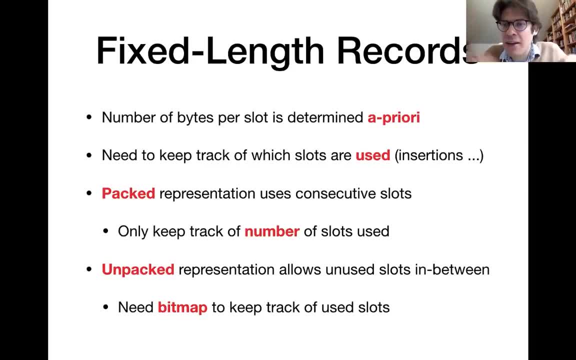 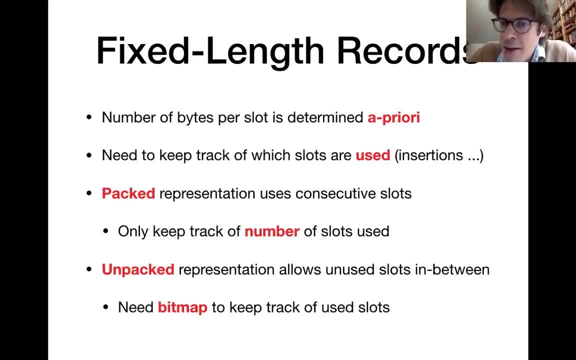 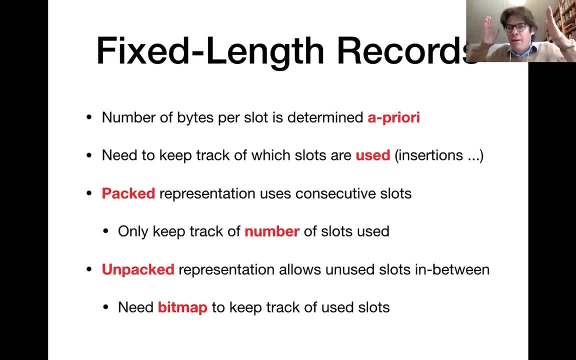 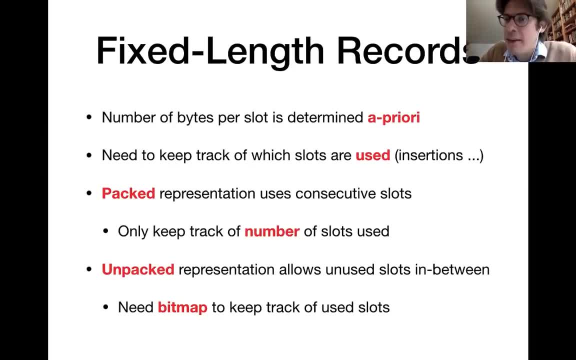 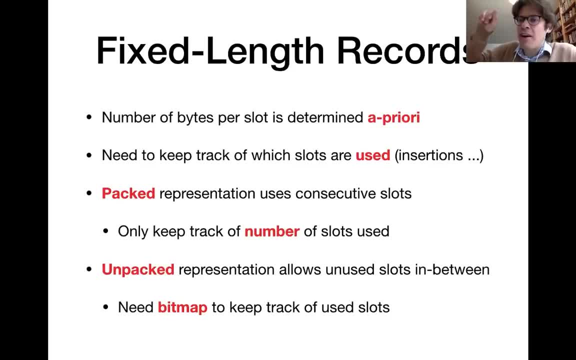 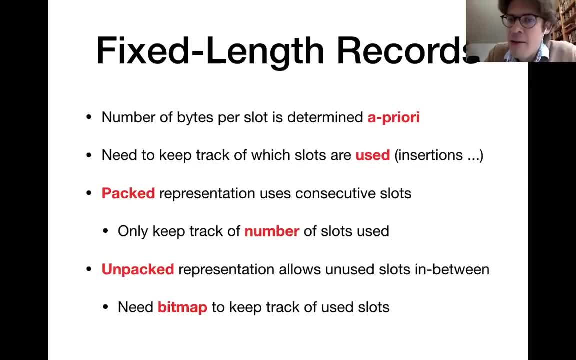 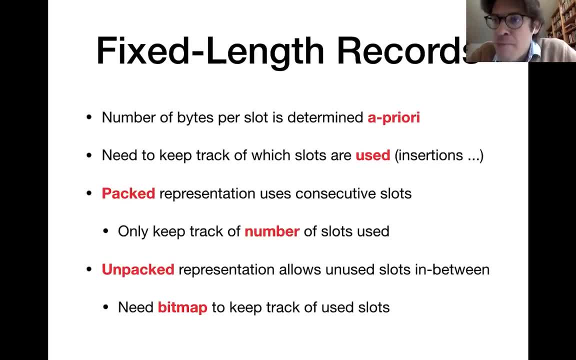 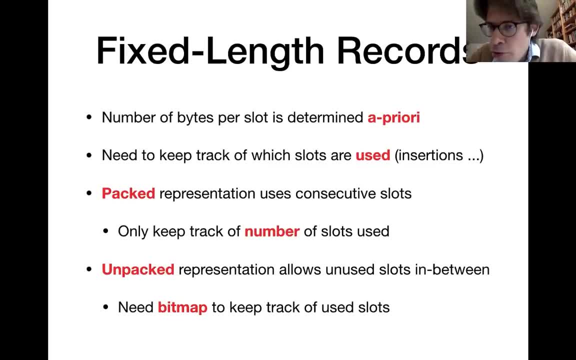 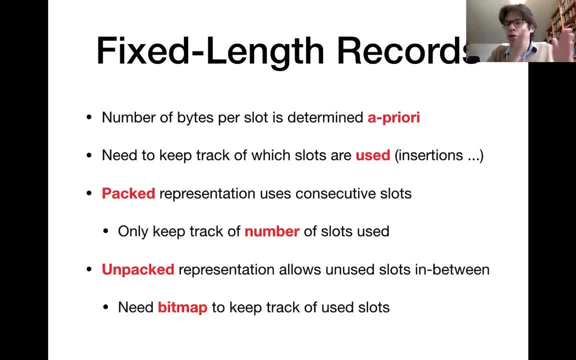 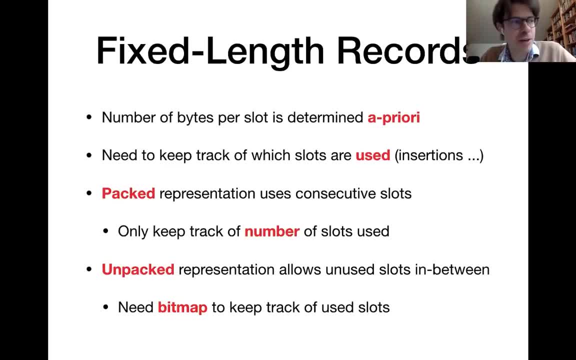 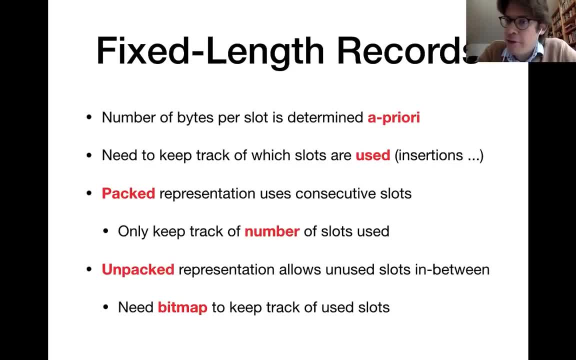 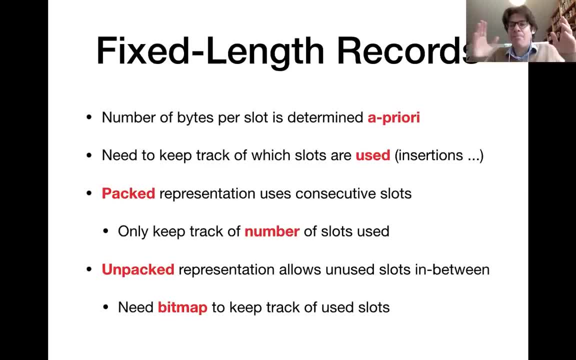 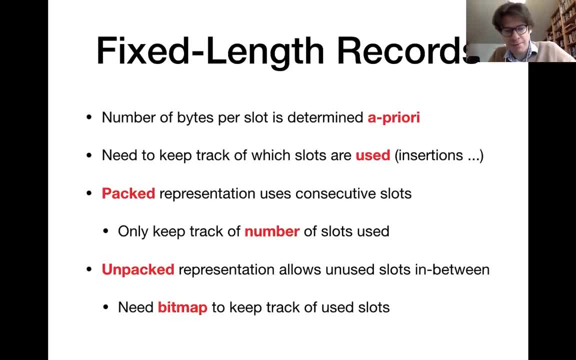 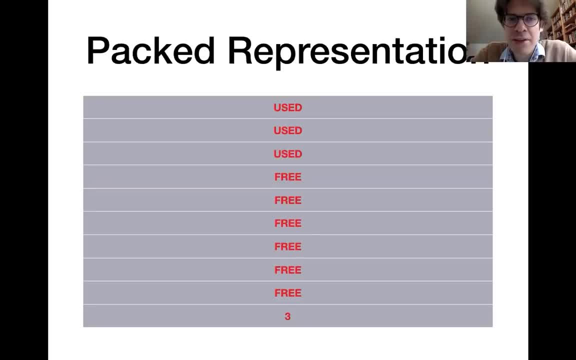 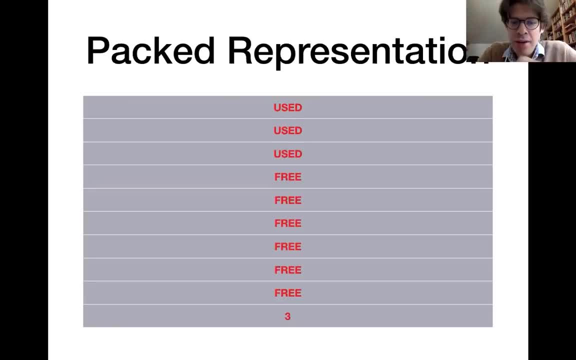 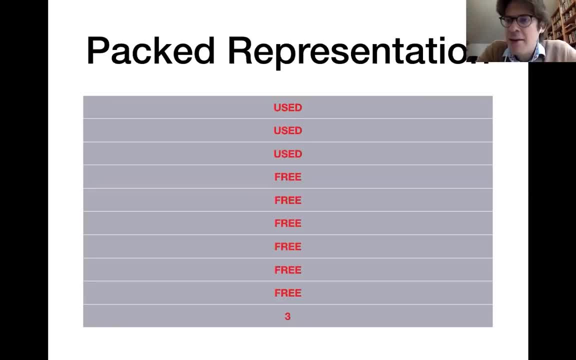 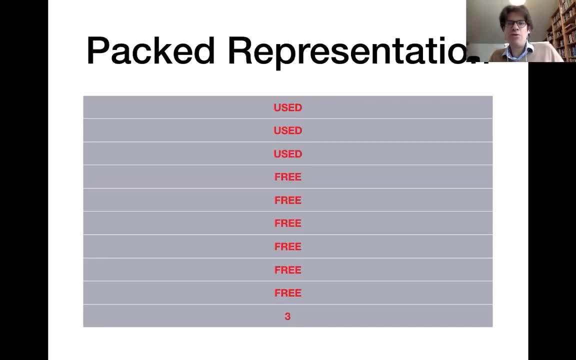 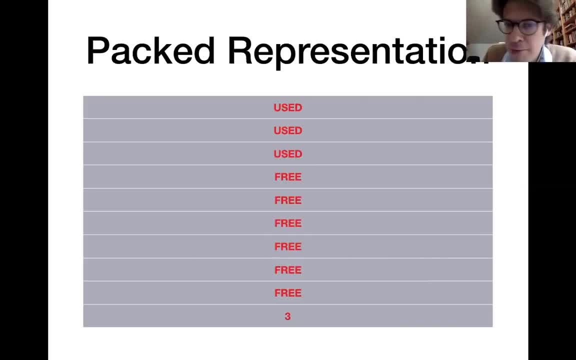 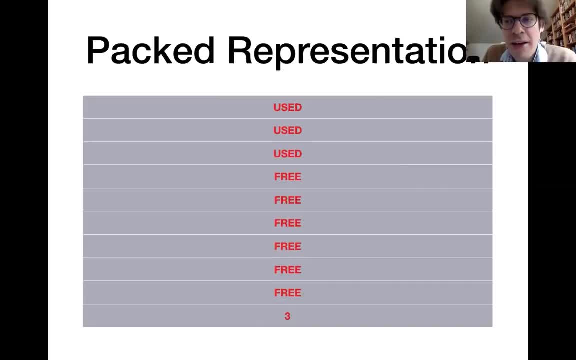 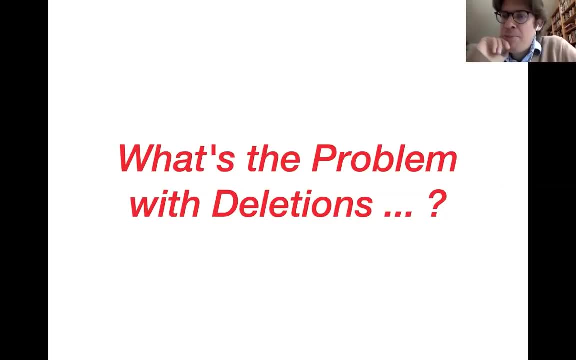 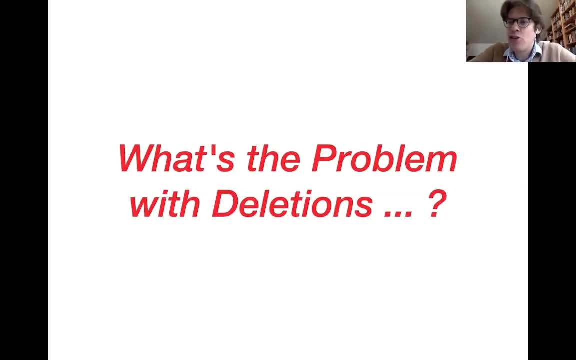 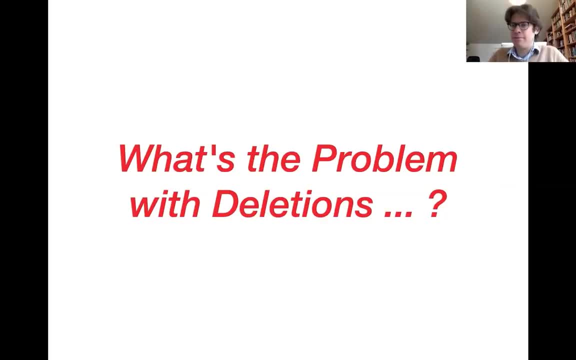 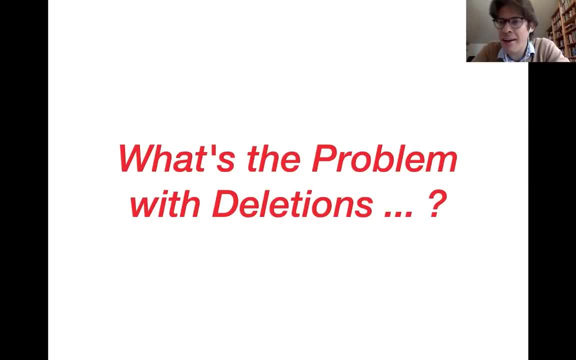 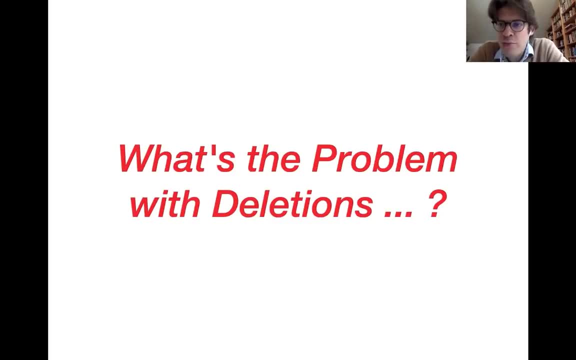 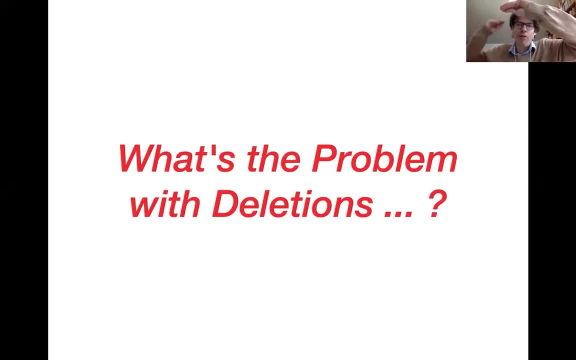 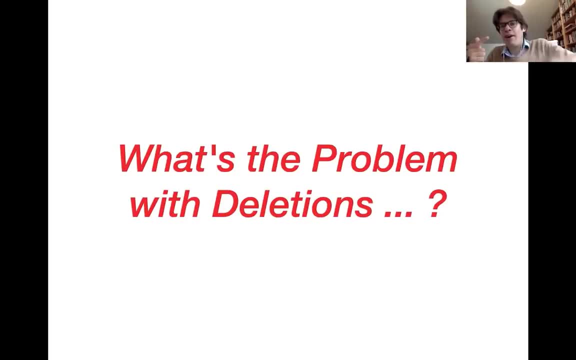 ID. Now, if I move around the records on a page in order to fill gaps, it doesn't change the page ID, but it does change the slot ID, And so if I have external references, then I would need to update them in order to get back to the packed representation. So it would. 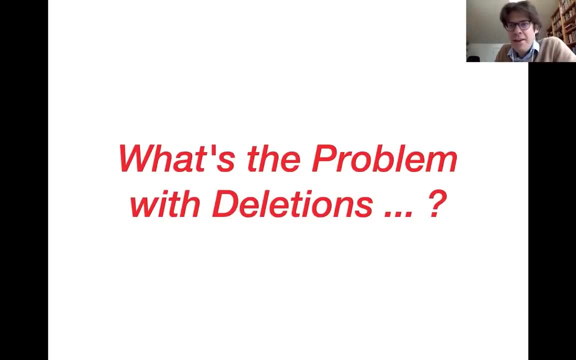 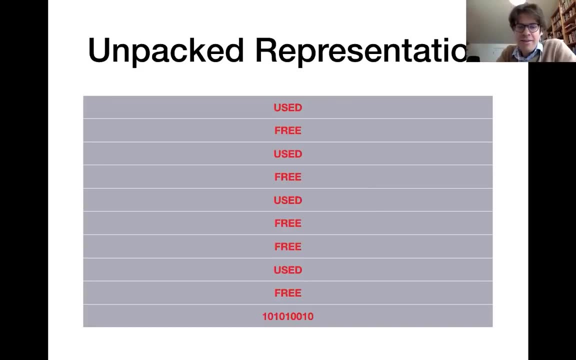 make things difficult. So an alternative way of doing this is the unpacked representation that you see here, And very good answers to the questions, by the way. So the unpacked representation allows gaps between different records, as you see here, And then you need 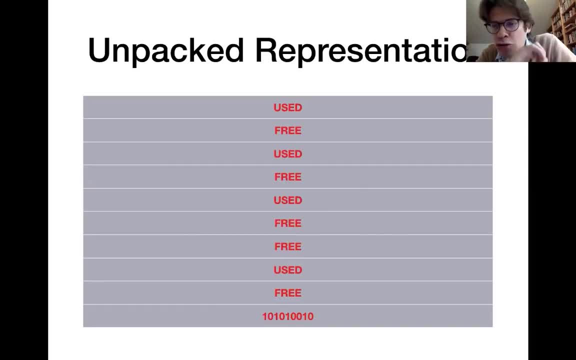 a bitmap in order to keep track of which of those slots occur in use and which ones are available. So here in the bottom row, you see the bitmap, together with the flags indicating whether the slot is already used. Okay, Okay, thank you. 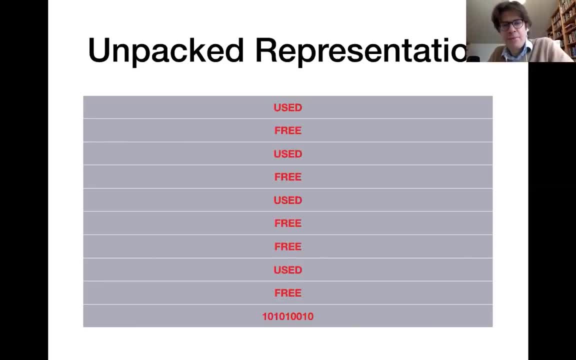 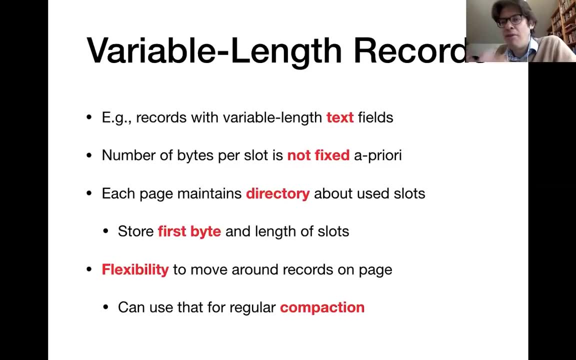 in use or not. all right, now, that was the little bit easier case where we have a fixed number of bytes per slot. now, if I have text columns, for instance, then the number of bytes I need per entry will vary across different, across different records, across different rows. so, yeah, in the variable lengths case. now in 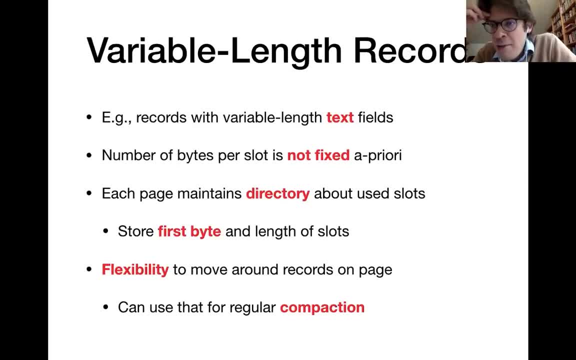 order to do this I need the way of keeping trap track. there on my page, specific records start and end, so typically you would store the starting position together with the lengths of the corresponding record and restore the information you in that way, and that's the way to store all of the data so I can store it. 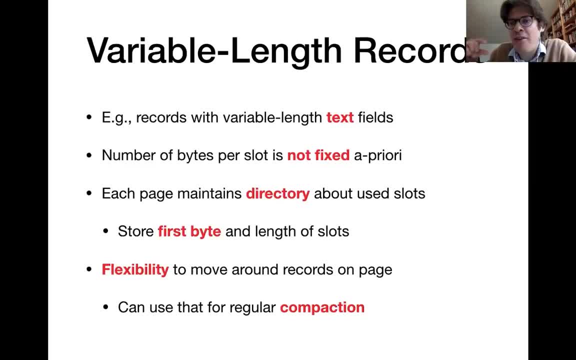 again in a directory, but here they're talking about that directory that is stored on each page and keeps track of their specific record. on that page are located right now. that creates a couple of opportunities for space optimizations. deleting by slots can become a problematic if I start moving, like 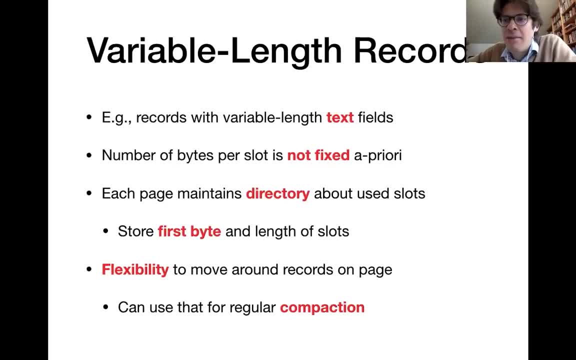 copying around records on my page, then that might destroy external references. now, if I use those on page directories, yeah, that is not a problem anymore because I can freely move around records on my page. the only thing that I need to update is this director, which is directly stored on the page and which 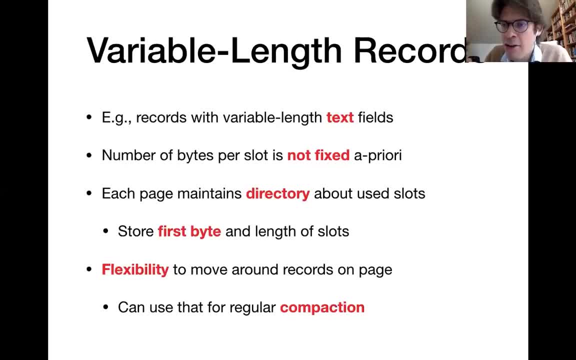 maps a slot IDs to the corresponding positions. so, since I have this additional layer of interaction in the form of the on page directory, moving records around on my page doesn't destroy the external references right, and I can exploit that in order to regularly compact the. This way, I'm maximizing my used space on a page by filling holes that have been. 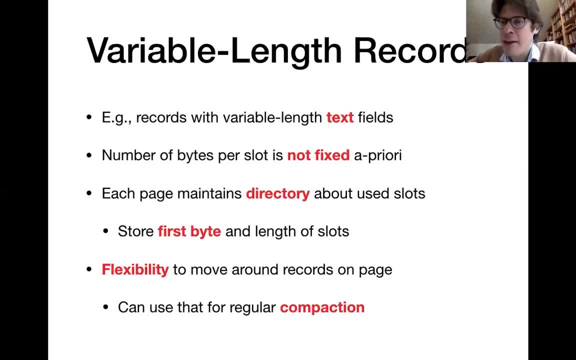 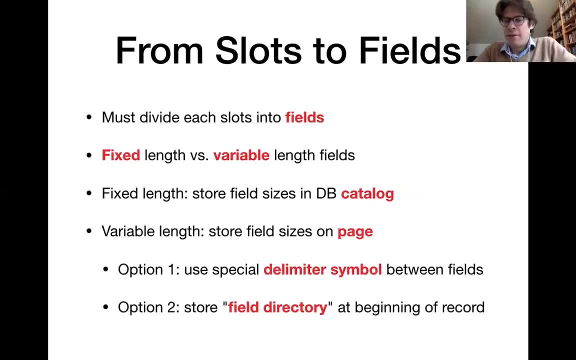 left by deletions, for instance, and thereby I'm maximizing the consecutive free space that I have on my page. We have to decompose things even further, because one row, one record, typically stores data from multiple fields, from multiple fields. If I make a request for an object, I have to cut this off of the list. 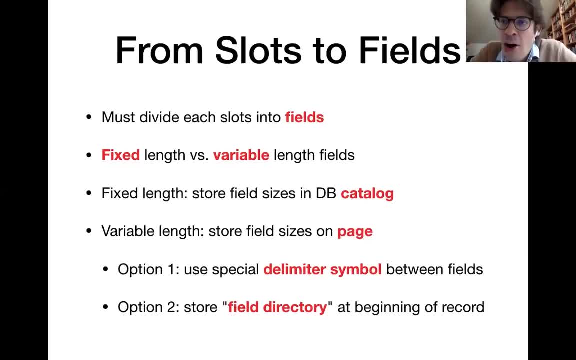 I have to make a request for a lot of space. I have to cut this off of the list, So that's a really important component: to maximize that data in order to create columns, and that is why we need to think about how we can divide. 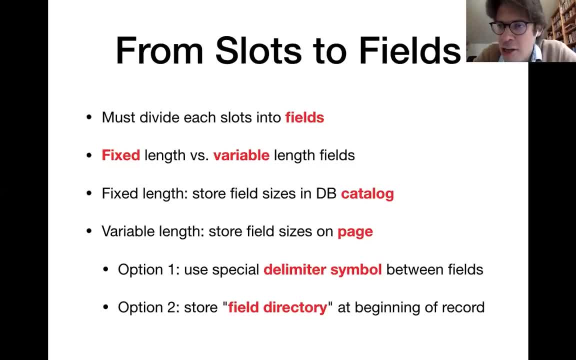 the space of a slot into space associated with different fields within that slot. And again you're facing at those challenges. If my fields have variable lengths as opposed to a fixed length For fixed length fields, for instance, if all of your fields, 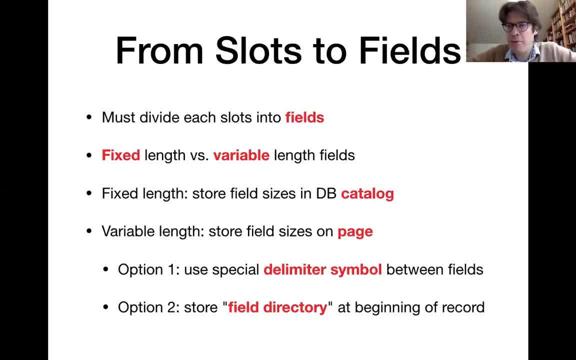 are integers, because all the columns in your table are integer columns. then we can just store the fixed length per column in our database catalog and we don't need to store any additional metadata on the page itself in order to divide the slot into fields. Variable length entries make things a little bit more. 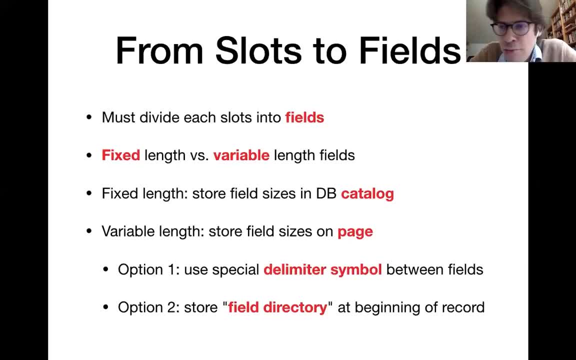 complicated Again, and here we have two possibilities. The first one would be to use some kind of specialized delimiter symbol in order to separate the data from different fields. So that is one possibility. Another possibility is to use again the directories here, essentially directories at the 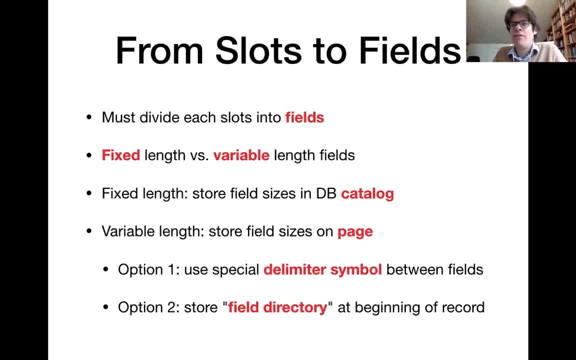 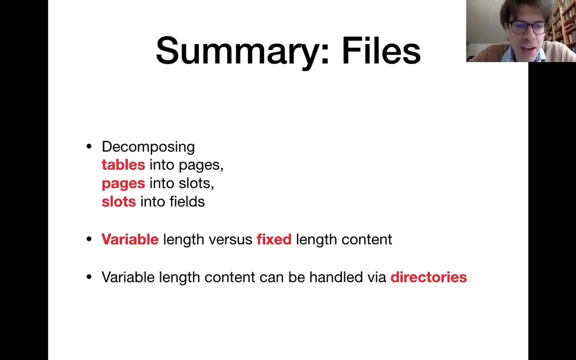 beginning of each record, which tells you which part of the slot space is reserved for the data that you have for storing data in specific fields. So this is how we decompose everything down from pages to slots and to fields Here. that is the summary of what we have. 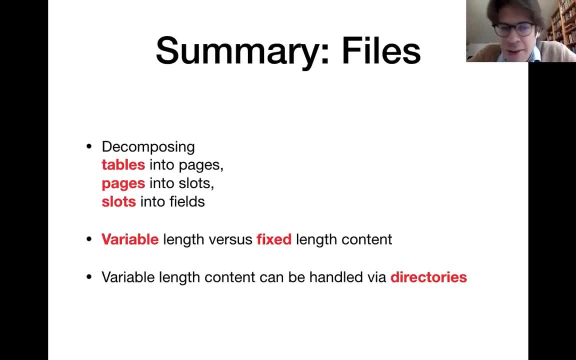 been doing One topic that keeps coming up, that is the topic of fixed length versus variable length content. Fixed length content is often easier to handle. If you have variable length content, then we need some kind of directory, whether that is a directory of pages, a directory of slots. 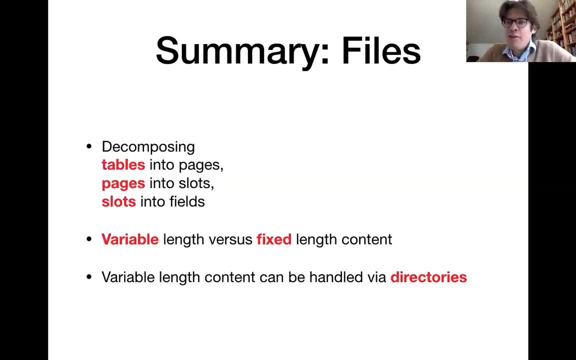 or a directory of fields. So here we have a reuse, the certain common ideas at multiple granularities. All right, And one question that I see here currently in the unanswered question is: in the unpacked representation do we still use slot ids? 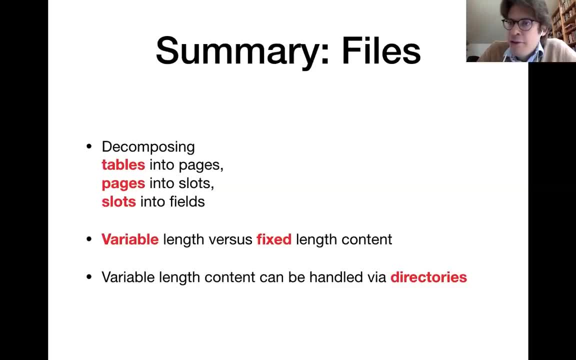 Yes, we always use slot ids So in the unpacked representation. so that doesn't essentially. that doesn't change anything. You still have slot ids for the different slots, just that now you might have empty slots between consecutive used slots. So the slot is essentially the space. 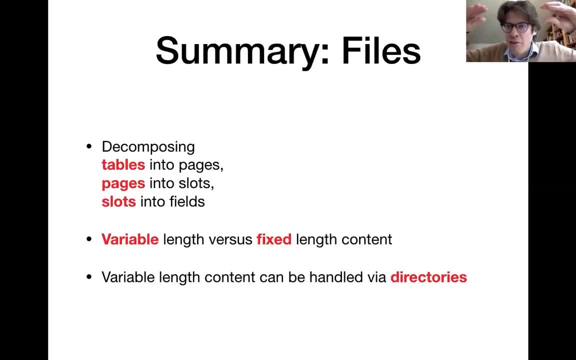 reserved on the page for storing one specific record, And that space can either be used occupied by a record currently or not. So just because one of the slots is empty doesn't mean that it loses its ID. Okay, All right. Now one last remark on how we store data. 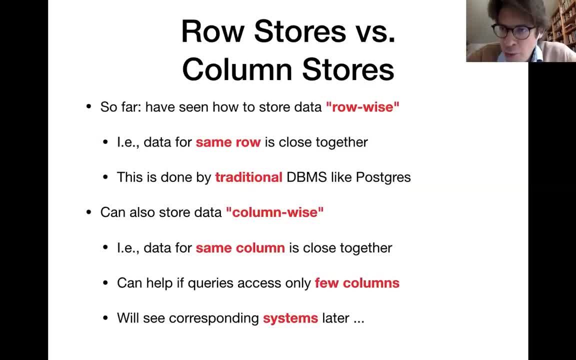 What we have been discussing so far essentially assumes that. you know, we assume that data which belongs to the same row is stored close together on a page, And that is the traditional way of storing data which is, for instance, used by Postgres. 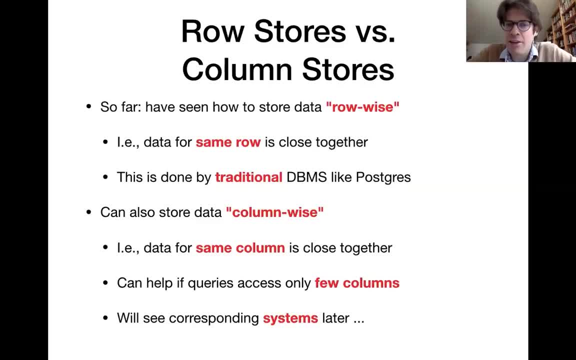 Since it stores data from the same row close together, it's also called the row store architecture. Nowadays there is another breed of database systems which stores data differently and rather tries to store data. which is stored data differently and rather tries to store data. 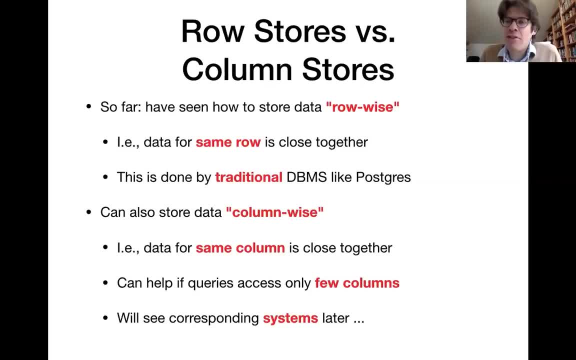 which is stored data differently and rather tries to store data which is stored data which is stored, data which is stored data from the same column close together. That can be a performance advantage in cases where you can tend to access only a few out of many columns of your tables. 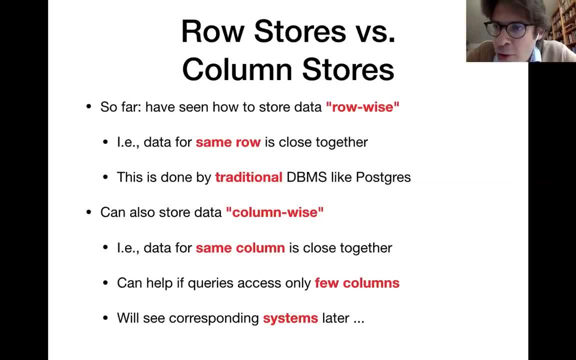 if you have this, then with the row store format, you would load entire data pages like one of those pages, a unit at which we retrieved data, for instance, from the hard disk, And if you load one of those pages with the row-wise format, it would contain data about all the different. 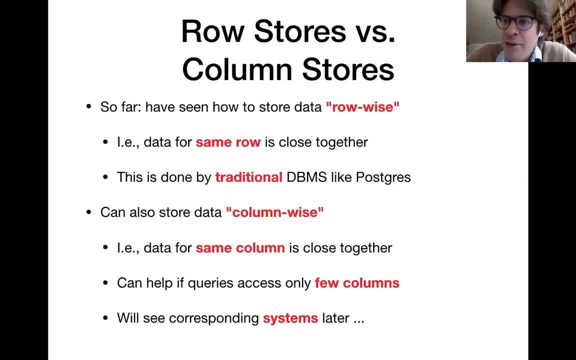 columns for specific rows, and if I'm not interested in many columns, it means I'm loading a lot of data that I actually cannot use, and in those cases a column store architecture might be more efficient. but that is a topic that we will discuss in more detail later, where you also see specific systems that use. 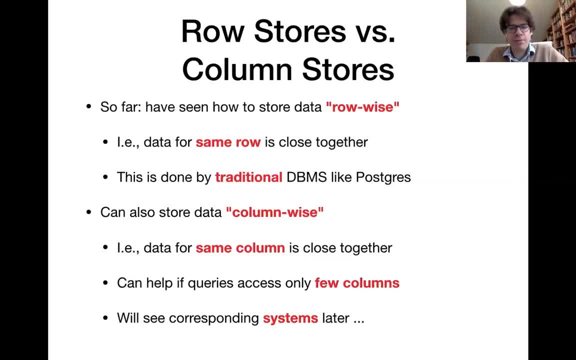 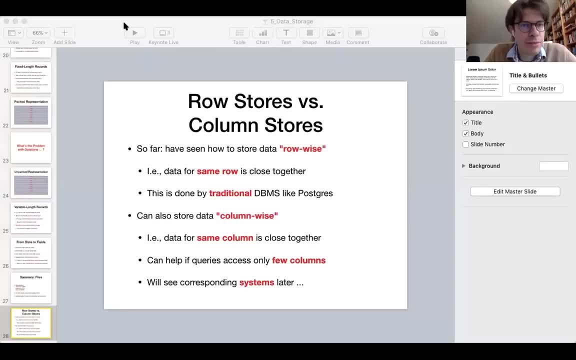 this a newer column store format. all right, now let me quickly change the slide deck here. we're gonna continue with the topic of how we store data, but we're gonna see more sophisticated base of storing the data that makes that make retrieval more efficient and with tomb son, welcomed today. 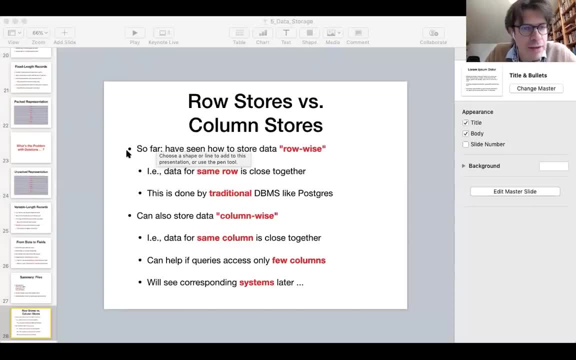 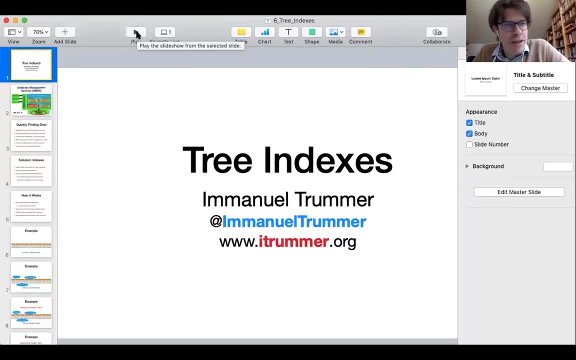 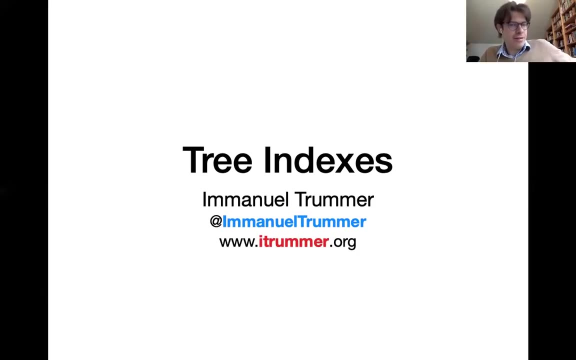 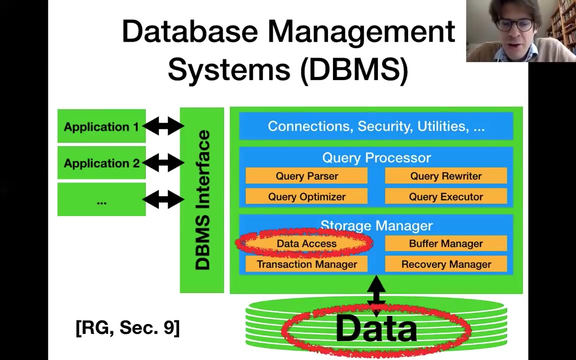 you, and those are news lights. I believe that we should all be able to see the tree in x's a slide. that, no, all right, okay. so in the following, we're going to discuss more about how we can store our data in order to make access as efficient as. 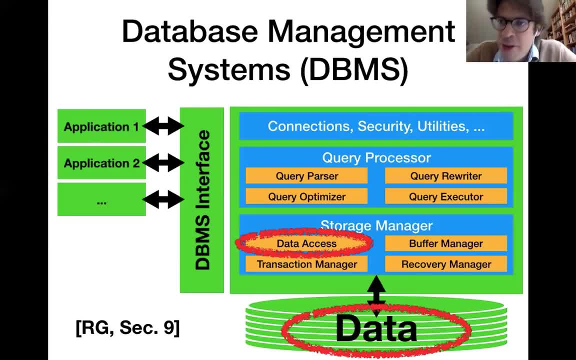 possible. So, within this big architecture of database management systems that I have initially introduced, this concerns the data itself, the way in which we store it, as well as this component that I have named data access within the storage manager, which contains the algorithms that 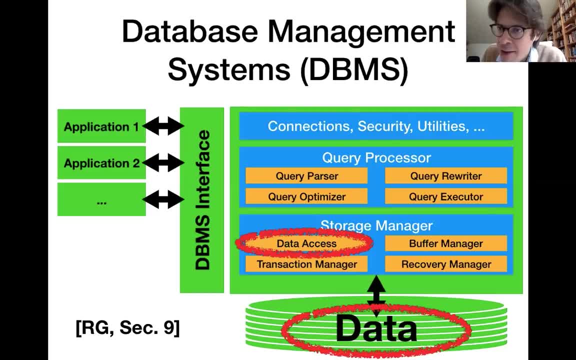 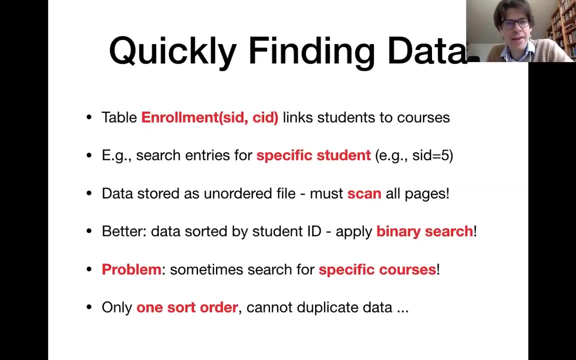 exploit the data structures for efficient access and that handle them. The relevant chapter in the Ramakrishnan and Gerke book, that is chapter nine, for what we discuss in this slide deck And the problem that we will be looking at in the following lectures, that is, the problem of quickly. 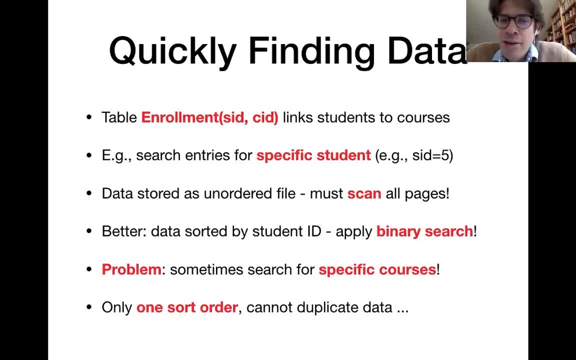 finding specific entries in your data set. Now, to make things a little bit more concrete, think, for instance, of the enrollment table that we have seen in our example database. Enrollment table contains information about the students and the courses that they're taking, So it essentially contains pairs of the student ID and the course ID. 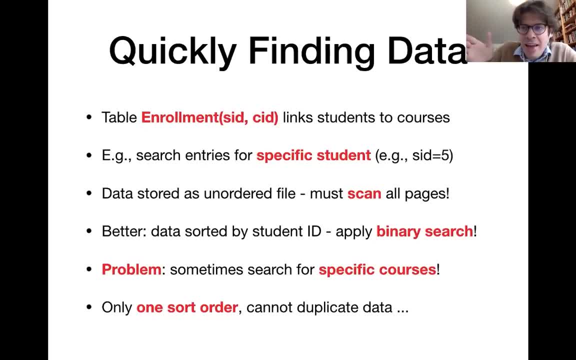 with the semantics, that the corresponding student is taking the corresponding course. And now let's imagine that we have searching for the enrollments for one specific student, for instance. Maybe he wants to find the enrollment information for the students of SID file. Now, if I store data using the format that I have introduced, 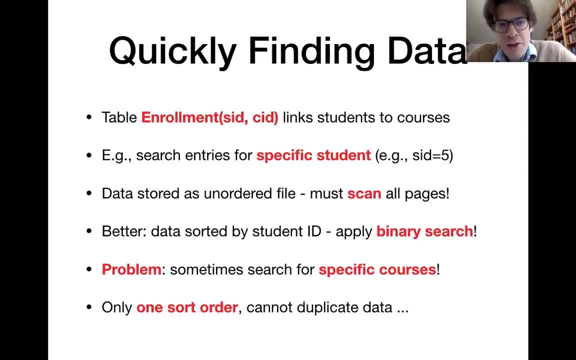 directly before Then. I could, for instance, store the data from the enrollment relation as a collection of data pages and I might either have them, as I think this, or as a directory. So in order to find the enrollment information for the same student, I would have to go through all of those pages and 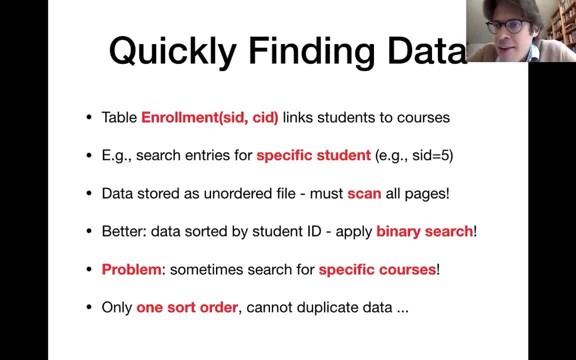 to look at all records on each of those pages in order to check whether the student ID equals to 5. And, as you can imagine, if I have a lot of students, then that is actually quite inefficient because I need to look at all data, but I'm only looking for a. 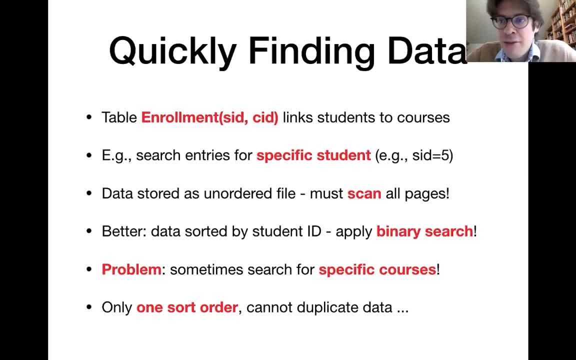 bunch of entries. typically A better version is already if I just the salt the data by the student ID. If I have sorted my data by the student ID, then it can apply something like binary search, for instance, in order to narrow it down quite quickly to those entries that I'm 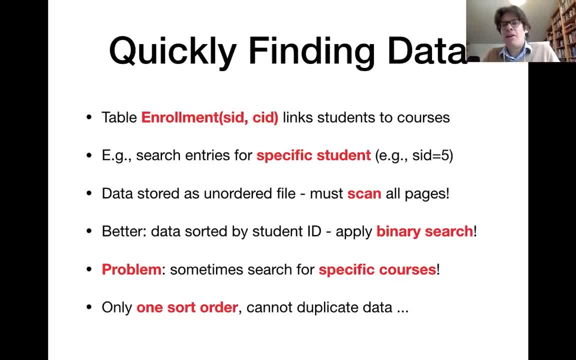 interested in. so that is already significantly better. But the problem is this: for one data set I have to choose the one specific way of ordering it. so here, for instance, if I choose to solve the enrollment relation by the student ID, then 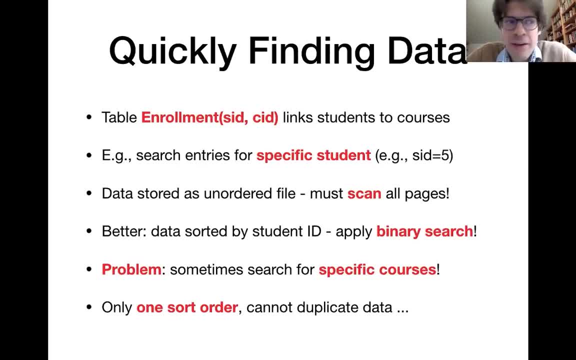 it will make it more efficient to find information about specific students. But if I'm now searching for information about specific courses, for instance inverse, then the student thought order doesn't help me at all and I have to choose one single thought. So, in order to make the student ID, I have to choose one single. 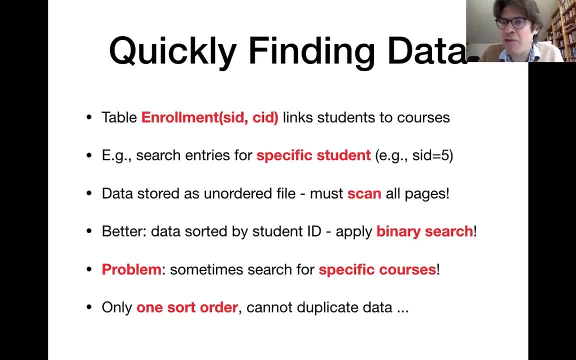 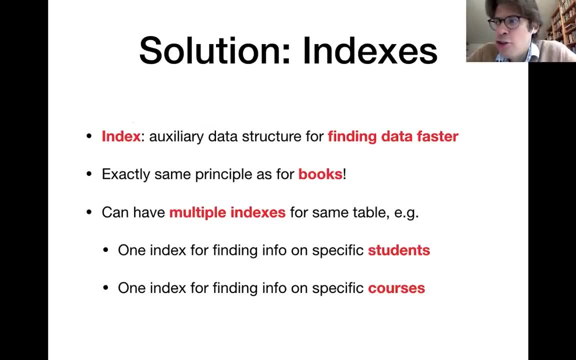 order. Multiple ways of accessing your data more efficient. We can use something called an index, which is essentially an auxiliary data structure used for finding data faster, and indexes are really exactly the same principle as indexes for books. I mean here, for instance, I have this New York tour guide and in the end, 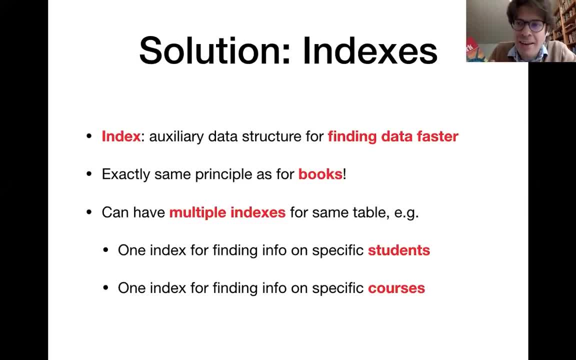 it has an index which contains the name of the student and the name of the student. It contains the names of different attractions, sorted in alphabetical order. For each of those attractions, it has a reference to the pages on which I find the associated data and. 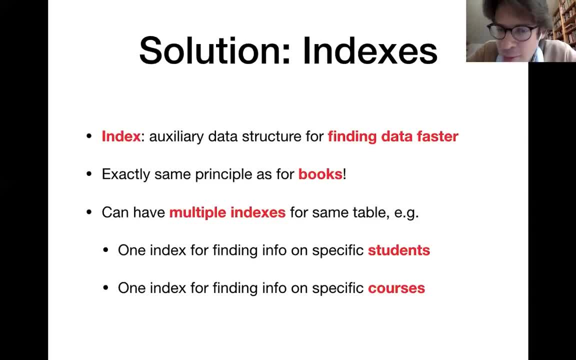 indexes, a database, a management systems. They do exactly the same thing And the nice thing about them is that I can have multiple indexes for the same tables or for the enrollment table. I could create one indexes for quick look up of specific students and another. 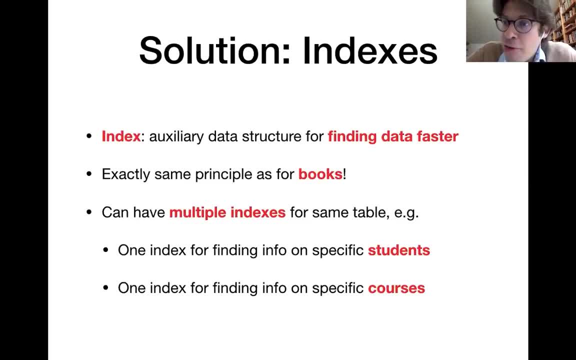 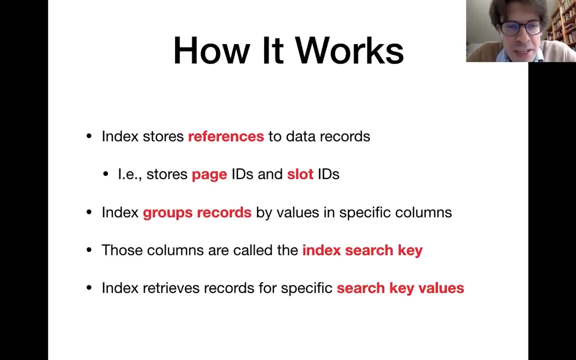 index for quick look up of specific courses. right, And that means I can make multiple ways of accessing data in the same table more efficient with that method. Now, in more detail, the index stores references to data records. As we have just seen, those data records, those references, have the 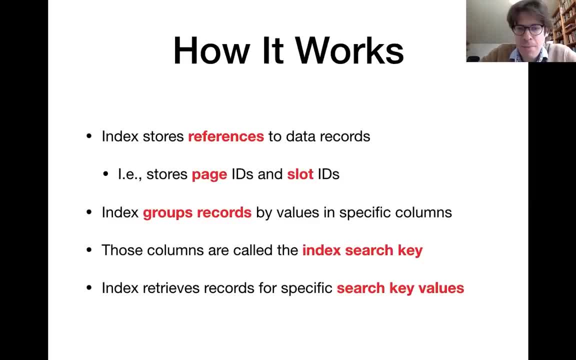 form of a page ID and a slot ID. Um, Now Indexes. they always refer to one specific table, These, the indexes that you see here in the lecture, And indexes are always specialized for one search key. So the search key that is essentially a subset of table columns. 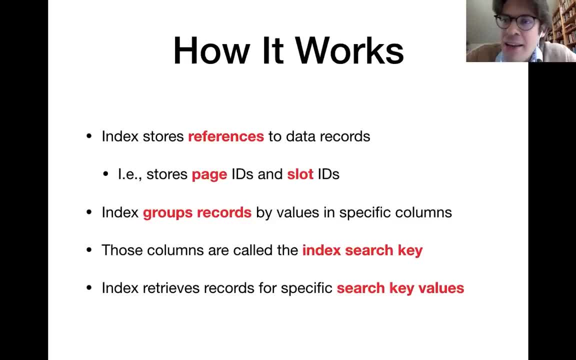 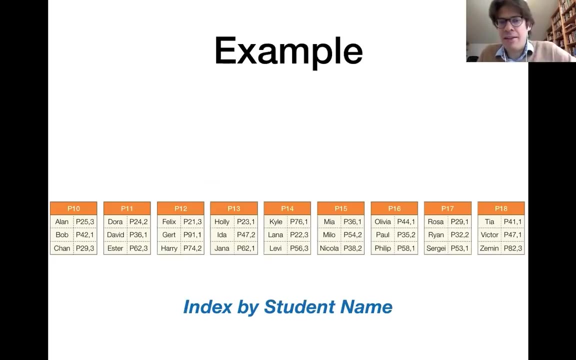 And then the index helps you to quickly retrieve entries that have specific values in those search key columns. You want to search according to a different columns? then you need a new index, basically right. Okay, So let's start with a simple indexing example. 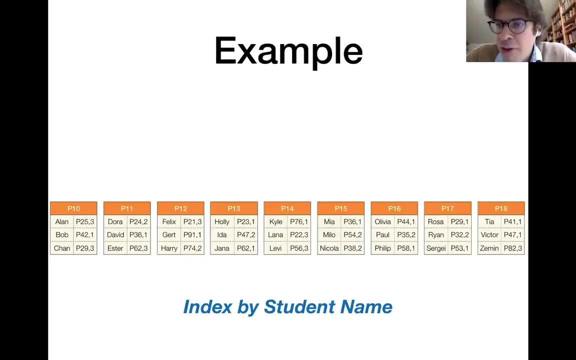 So let's say that I want to retrieve enrollment information for specific students. Then I can create one of those index structures in order to make access by student names more efficient. Now the data of the index itself, because it's also Data, So we again store it as a collection of pages. 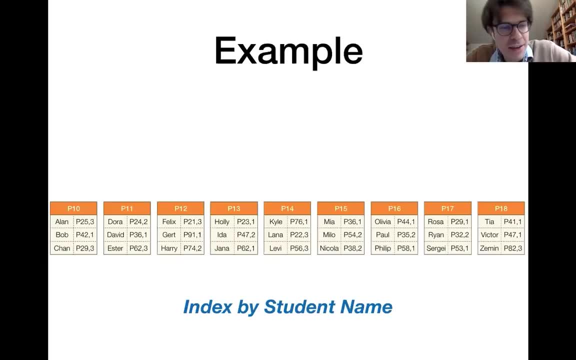 So the index is also stored as a file, And here in this simple example, you see that I have multiple pages that belong to the index and each of those pages has, on the left-hand side, the um, the value values from the search. 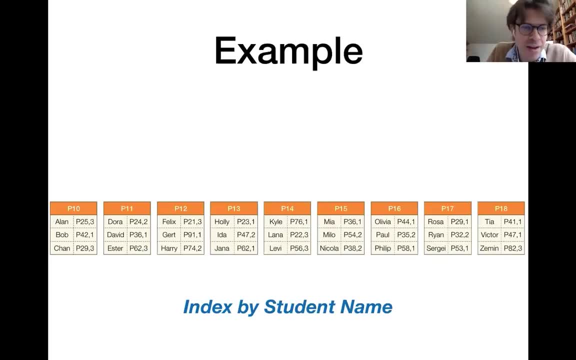 key, which in this case is the student name, And on the right-hand side you find the record IDs, meaning the page ID, followed by the slot ID. In order to keep the example simple, I have made those pages fairly small, So we have at most three entries per page. 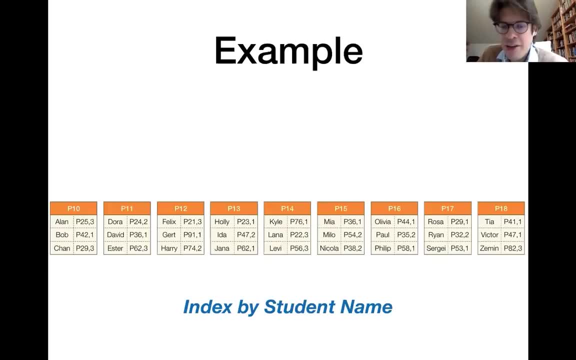 In reality, of course, you would have typically hundreds of entries per page. So here you have the index page idea for the pages that store the index. Okay, You have the index data and uh, as I have already discussed on the left column, you: 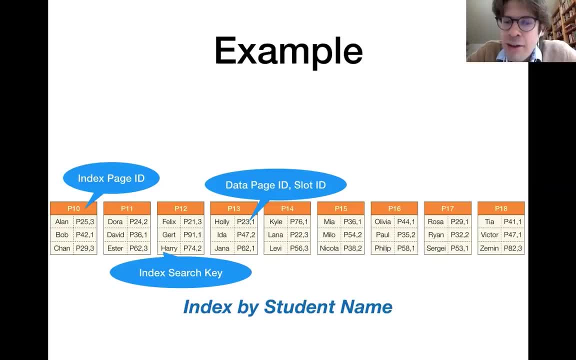 have the index search key on the right column. You have the associated record IDs And now if I search, for instance, uh, for a student named Alan, then I can use something like a binary search in the index. I can first look at page number 14 and see whether the entries on that page come before. 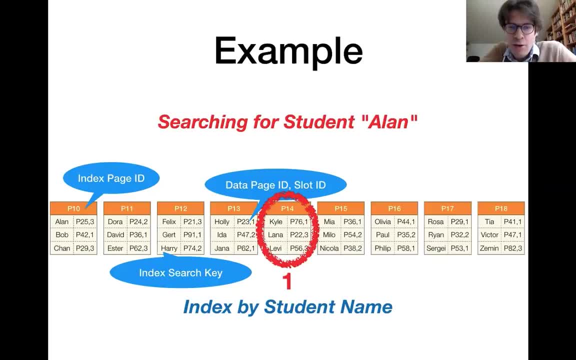 or after, And I can see that the entry that I'm looking for here, those student names. they are ordered in alphabetical order, So Alan comes before Kyle, so I have to go to the left side of that um of that page. 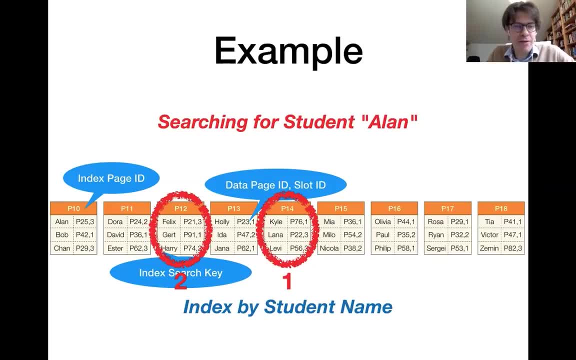 number P14.. All right, So that would be a P12.. And now I compare against. and Alan comes even before Felix, So I have to check out this one. And Alan also comes before Dora. So now I have found the last page, and here I had to access, uh, four pages in order to. 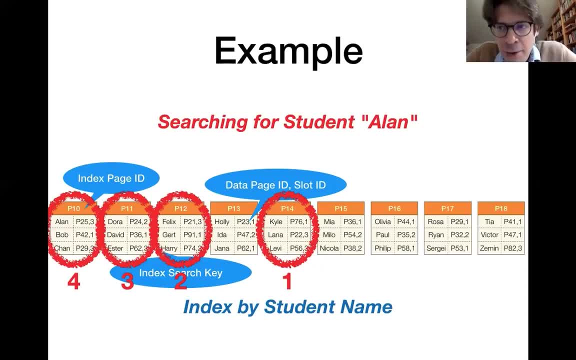 retrieve the data I'm looking for, And we have already very quickly discussed this, but let me remind you that, in the context of database management systems, um, often the cost for accessing data actually dominates entire processing costs. Uh, and that is why those index structures that we were talking about earlier, uh, are. 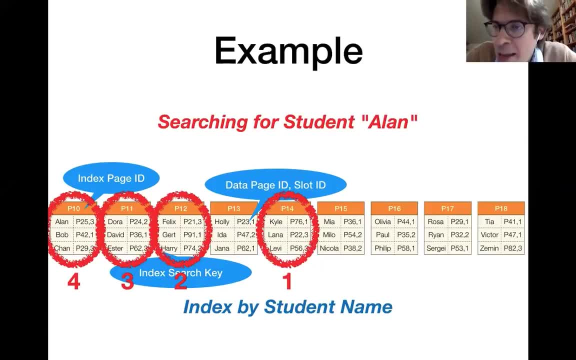 optimized for minimizing the number of pages that I need to load from hard disk in order to find the data that I am looking for. So according to that cost metric here we would have loaded four pages, So that means four cost units for the access. 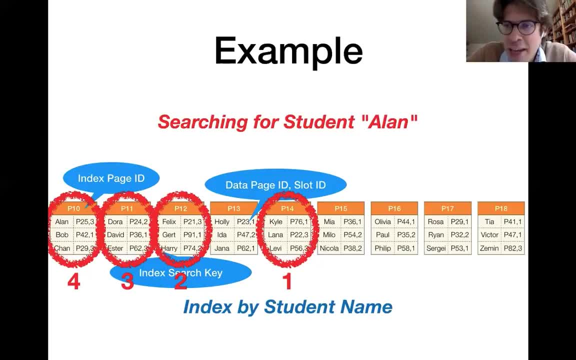 Then, finally, since the index only contains a reference to the actual data I'm looking for, I would still need to count one more um page access in order to load the data that is uh referred to for Alan, which I find at page number 25 in slot number three. 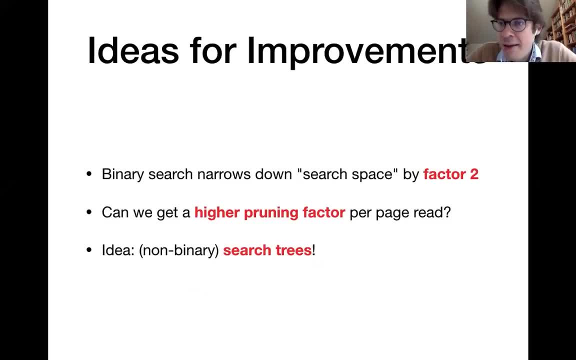 Now, that is one first simple indexing structure, but in the following we're going to improve on it. Now, the first thing that we want to improve is this: right now I have a flat index, a structure which sorts by the student name, and that means I can use binary search. 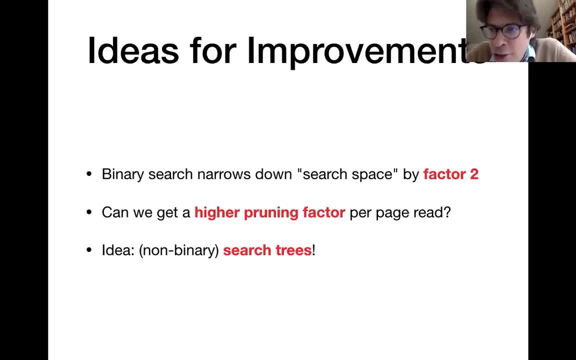 Uh, with binary search, whenever I load a page from hard disk, it means that I'm essentially narrowing down the search space by factor two. The index structures that are actually used in database management systems. they try to be more efficient per page access. 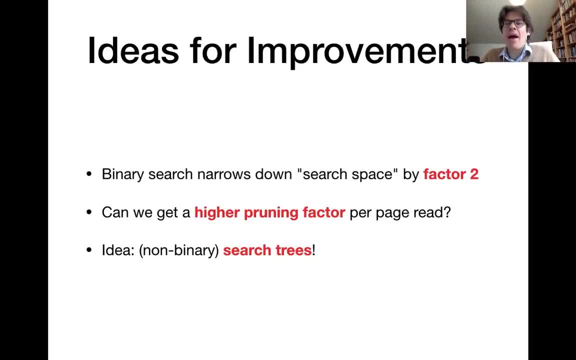 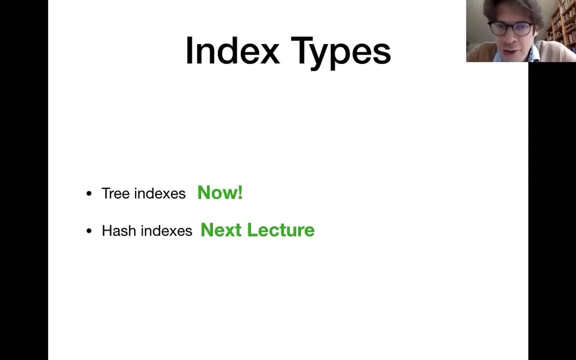 So they try to narrow down the search space, um, by a much higher factor than two for each page load operation. They can't do this, For instance, Using so-called uh index trees, tree indexes. they will be the focus of this and still the 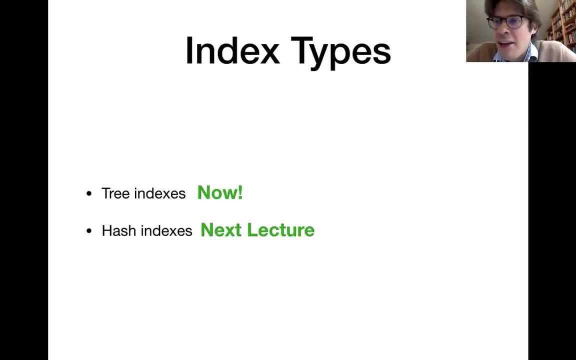 following lecture, but, uh, already as a little output. um, there's essentially two big branches of indexing pipes. One is organized as a search trees, One is organized as a hash tables, basically, and uh, we're going to first discuss the 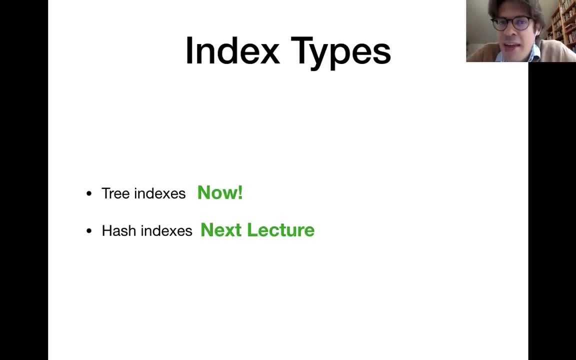 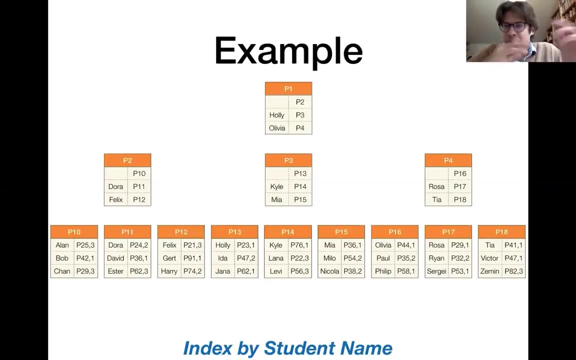 tree indexes. Later We're going to discuss about the hash indexes. This is how I can um use one of those tree indexes for this example here. As you see now we have a more pictures in the index um the index data that we have. 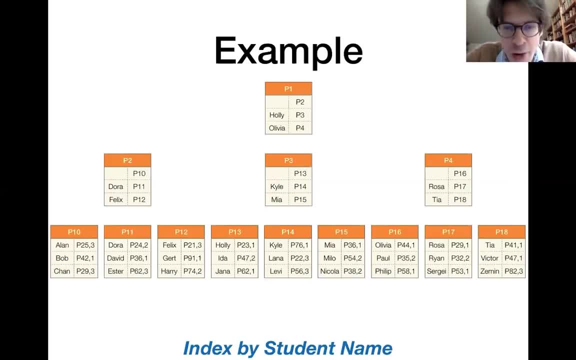 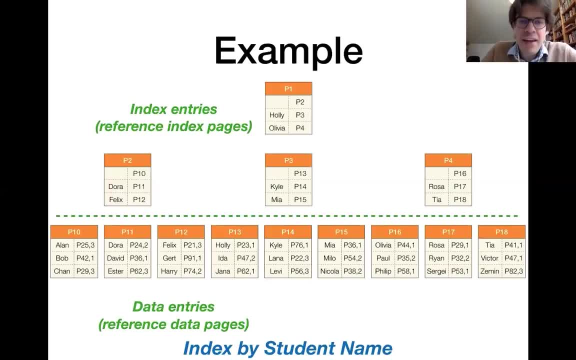 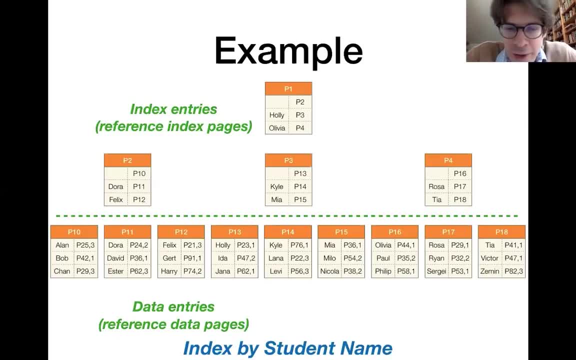 line, then you see some slight differences. So the entries on the lower part of the screen, those are the so-called data entries, because here each entry on a page references specific data. So in this case there's specific student names and next to it is references to. 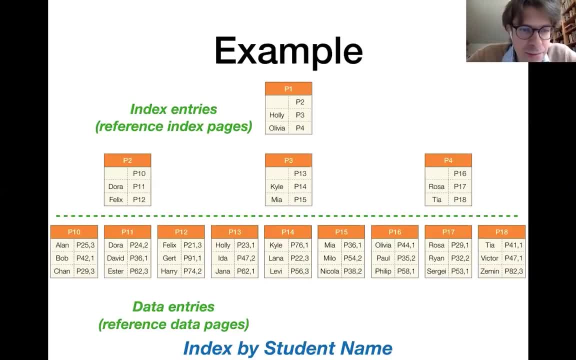 where you can find that data. If you look at the entries on the upper half of the screen, then they are organized a little bit differently. So those entries on the upper half of the screen, those are so-called index entries and they don't point to actual data, but they point to other. 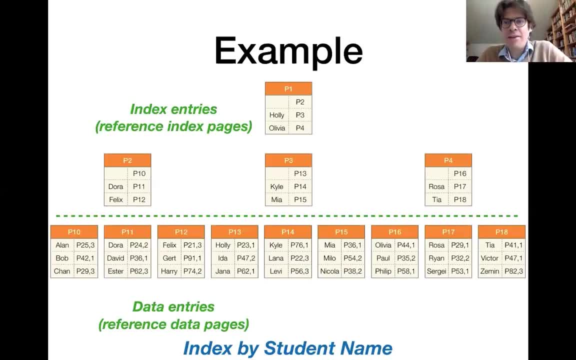 pages from the index itself. So here the semantics is this: On the columns on the left hand side, in those index entries we essentially have references to specific key ranges- search key ranges- and then on the right hand side you have references to associated indexing pages. 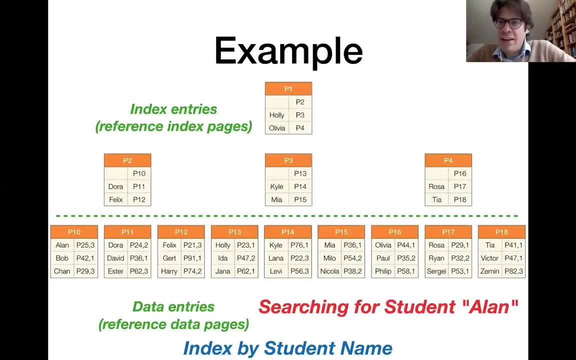 Now, in order to make things more concrete, let's have a look at a concrete example again. So we are searching for this- a student again- and in order to use one of those index trees, we always start at the root node, which is the node at the very top. So here I'm looking. 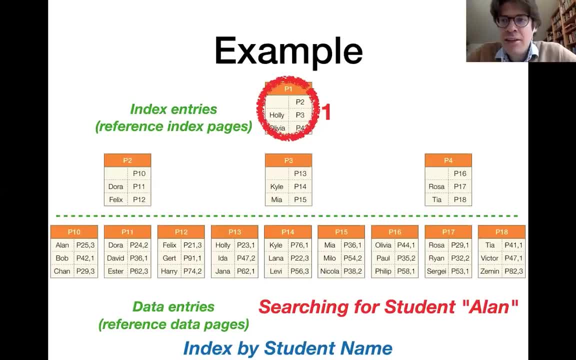 for the index tree and I'm looking for the index tree at the very top. So here I'm looking for the index tree and I'm looking for the index tree at the very top. So here I'm looking for student Alan, and student Alan would be ordered before Holly in alphabetical order. That is why I 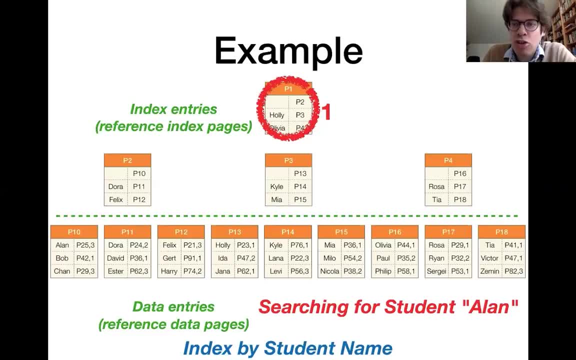 need to go to the corresponding page 2 of the index that is referred to. So now I'm looking at the page number 2 and again I'm comparing. I'm searching for Alan, So Alan comes also before Dora. So I want to look at the index, page 10. and now I'm at the right page and I 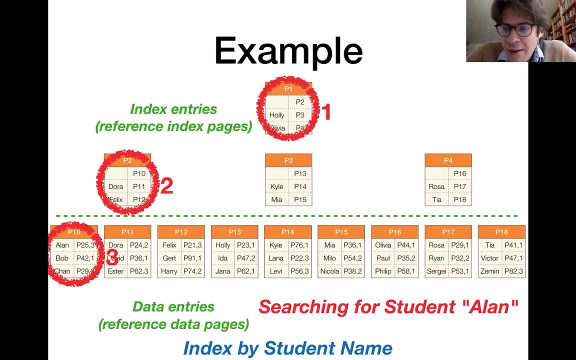 need to go to the corresponding page 2 and again I'm comparing, I'm searching for Alan. So here I'm finding an entry for Alan and because of that, and now that I find the corresponding enrollment information on page number 25 and slot number 3.. And here I have some discussion about like. 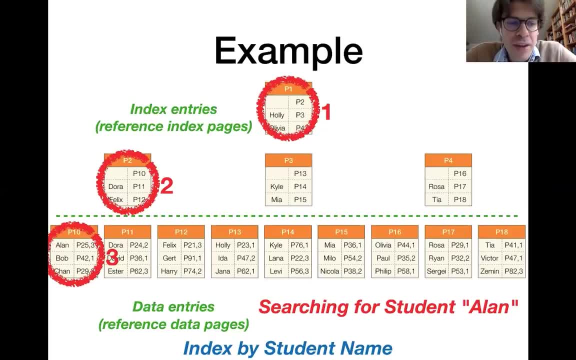 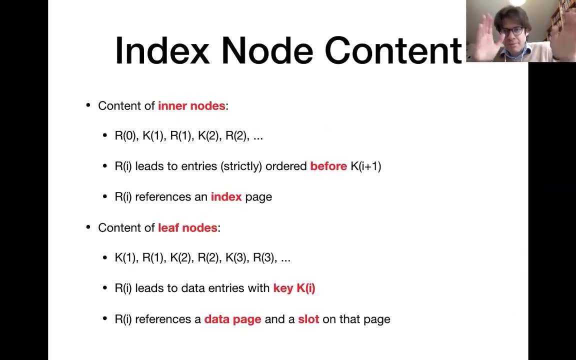 pointers, I assume. the question is whether those record IDs essentially correspond to pointers, and that is pretty much the case. So they give you one specific address where you can find data that you are looking for. All right, So here to make things a little bit more formal. 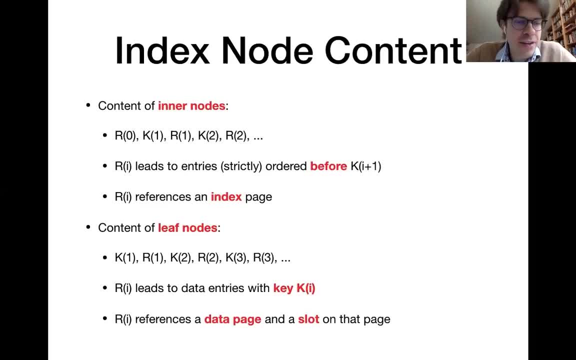 a description of the content that we have in those different types of nodes. Now, in the inner nodes of the index, we have those index entries and the content that they store. it's alternating between references to index pages and references to index pages, So the reference to index pages. 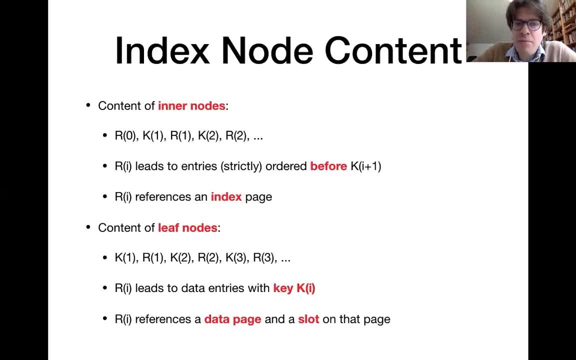 and the search keys. So we alternate between the two with the semantics that the references point to entries that are strictly ordered before the key that you find next, Right. So here, for instance, a reference one would point to two entries that come as strictly before search key. 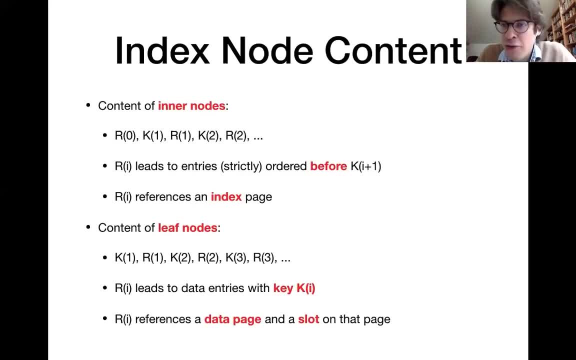 number two, Right. So if you're searching for something, then you just need to identify the corresponding key value range within one of those inner nodes in order to know which index node you need to look at next. The leaf nodes are structured a little bit differently. They have keys followed. 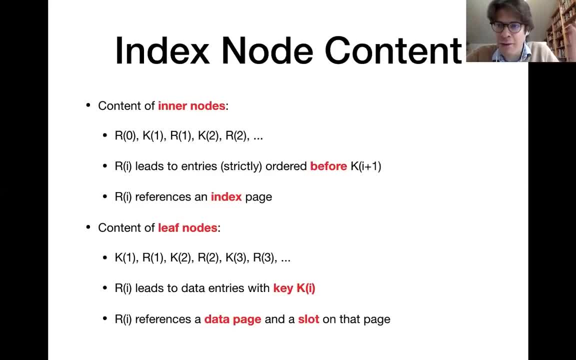 by references. So it doesn't start with a reference, It starts with a key, And for each of those they have a key, And then they have a reference, And then they have a key, And then they have a reference, And then they have a key, And then they have a reference, And then they have a key. 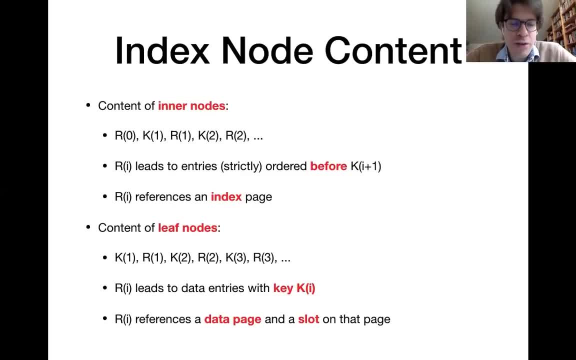 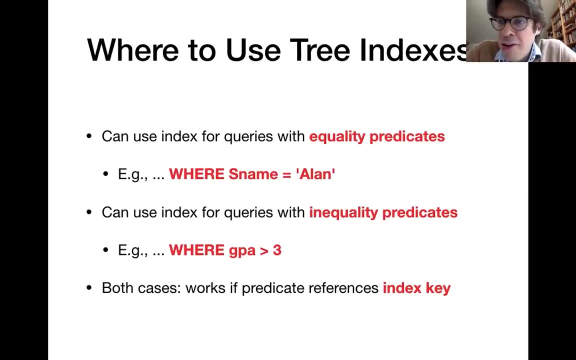 So those keys- the corresponding reference contains a link to the data that is associated with this search key. So we can use those indexes first of all in order to answer queries with equality predicates, And we have already seen that, for instance, if I'm looking for a row satisfying the 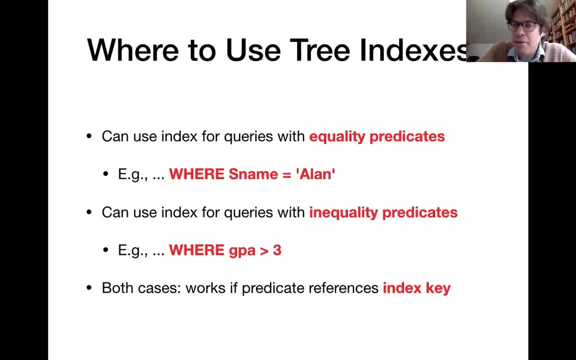 condition student name equals Alan, then I can use the index that we have just seen in order to efficiently answer them. What I can also do is to use them for inequality predicates, For instance, if I have an index by the GPA column. 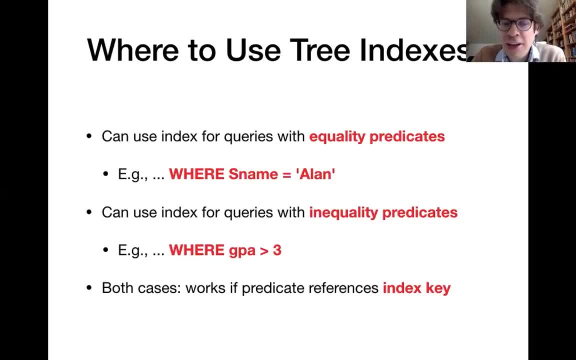 then I could use one of those indexes in order to quite efficiently retrieve those entries with a GPA greater than 3.. You're going to see in more detail how retrieval works in those cases in the following. Now, in any case, this works if the predicate 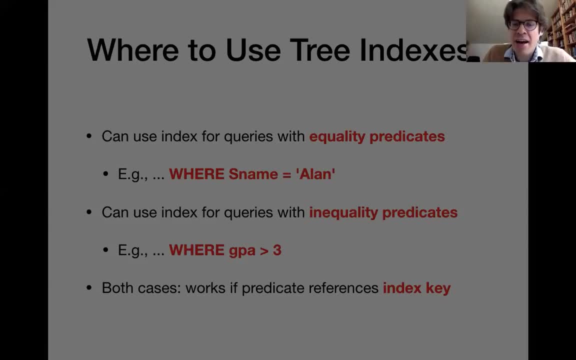 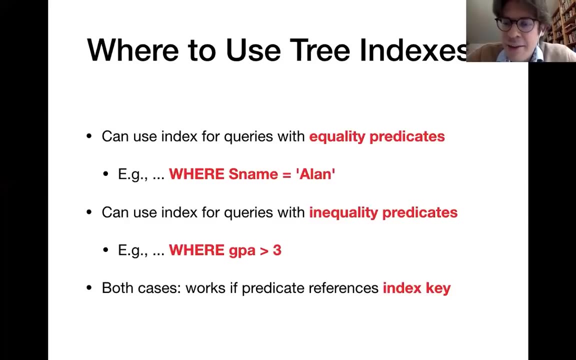 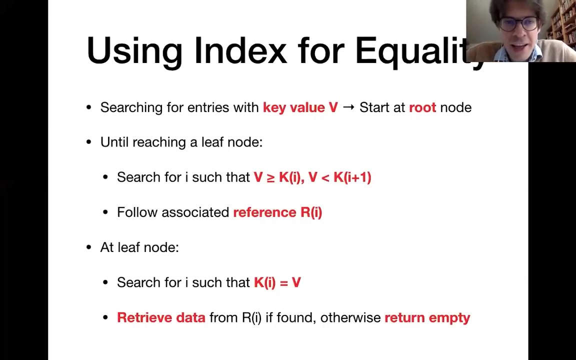 that you have in your query references the index search key. All right, So here to make things a little bit more concrete: how can we use this? This is the index for equality predicates. This is the algorithm that you would use for that. 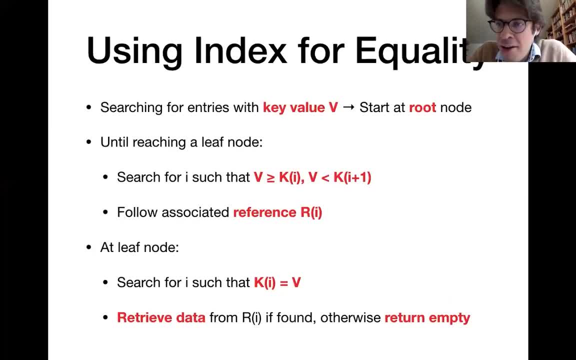 So whenever I have an equality predicate in my query and I want to use the index in order to find corresponding entries, then first of all I start at the root node of the index, which in those slides was on top, And until I reach one of the leaf nodes, 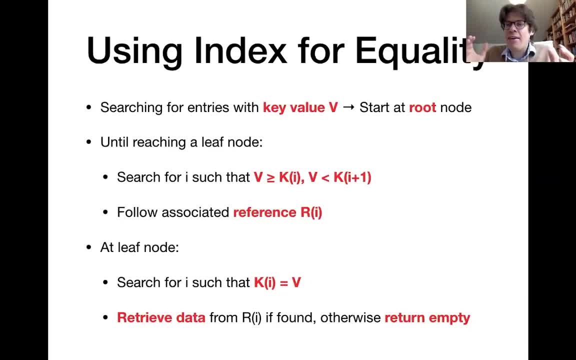 I essentially OK, OK For each node, identify the right key value range that the entry I'm looking for must be contained in. Then I follow the corresponding reference to the next index node, and so on until I reach one of the leaf nodes. 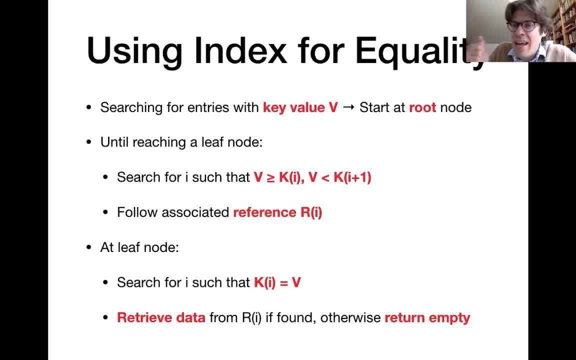 And at the leaf node I see better- an entry exists for the corresponding key And if I find such an entry, then I follow the record ID in order to retrieve the associated data. So, of course, whenever you use one of those indexes, 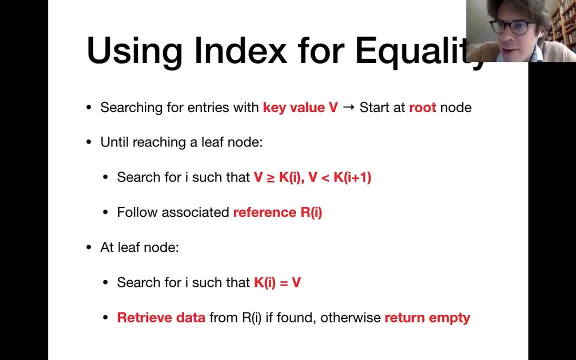 it is not guaranteed that you find any entry at all for the key that we are looking for. Perhaps we don't have any student named Alan Batchester right, But at least the index directs you towards the leaf page on which the entry would be located, if it exists. 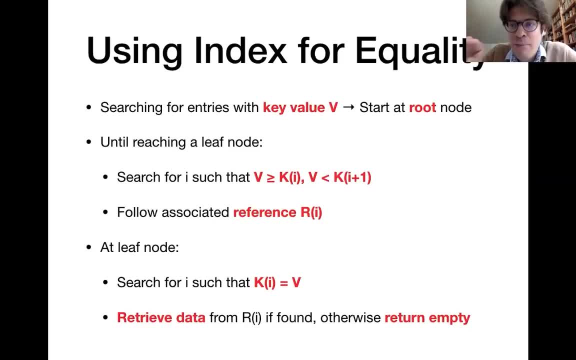 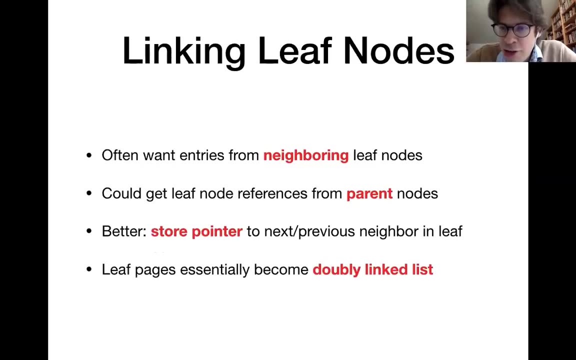 So after we have examined that leaf page in the index, we can be certain one way or another one, whether the entry is in the index or not. All right, Now there's a couple of optimizations of those index data structures that we will discuss in the following. 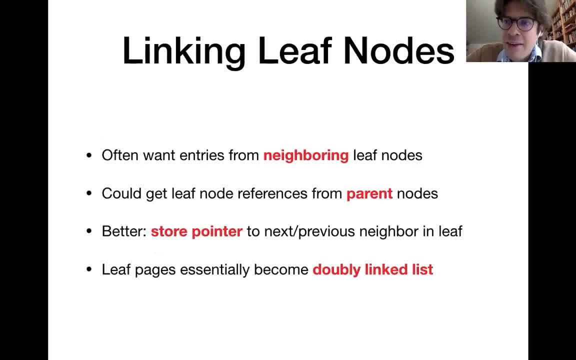 Going to quickly outline the first one, and then we will discuss more in the following. Now, often I might want to retrieve multiple um entries from an index, For instance if I have one of those inequality conditions. In that case it can be good for performance. 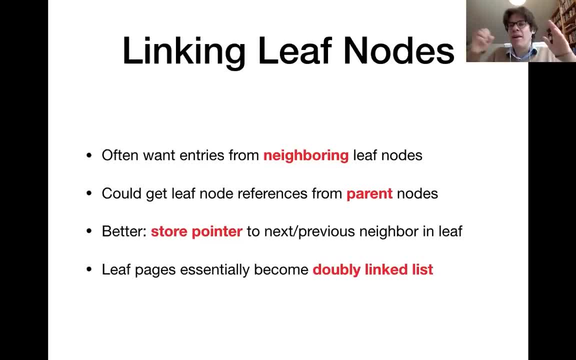 if the leaf nodes of my index are also linked to each other. So if I want to retrieve information in neighboring leaf nodes, I don't need to go over the parent nodes anymore, But instead I can leverage those links in order to go from one leaf node. 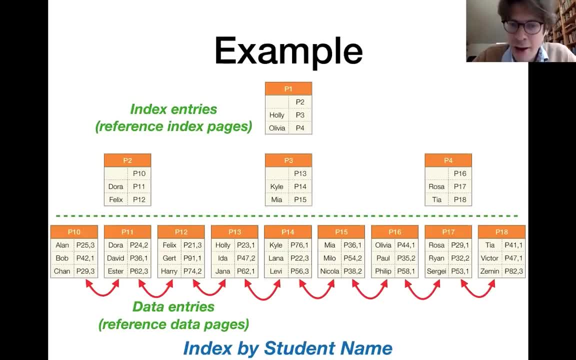 to another one, And this is how that would essentially look like. So you mentioned, for instance, that we want to find all students whose name starts with a letter between a D and a K. Then I could use this index in order to find the first student whose name starts. 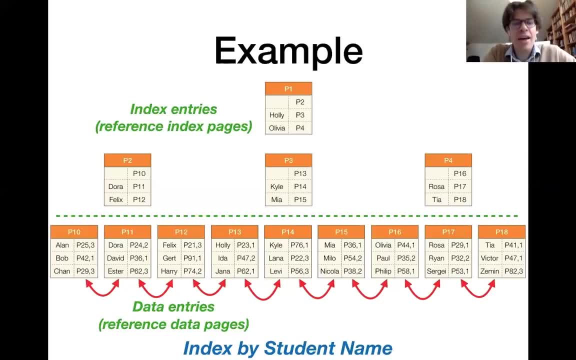 with a letter D, which is Dora, over here, And using those links between the leaf pages, I can just start From the Dora page, which is page number 11.. And then um, jump to page number 12,. 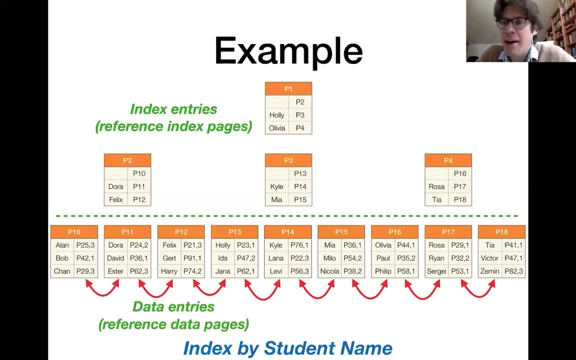 to page number 13,. to page number 14, until I find entries which start with a letter after K, And so I can quite efficiently use the index in order to retrieve those students whose name starts with a letter between D and K, And what enables me to do that is linking the leaf nodes. 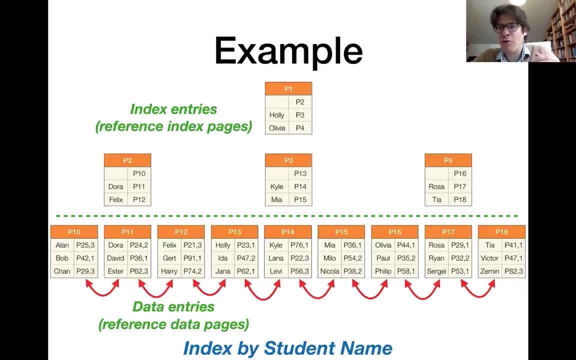 The leaf pages in my index by essentially storing the pointer to the next and the pointer to the previous leaf page in each of those leaf pages. So that was one optimization. We will see more optimization and different indexing variants next time. The homework, by the way, will be out this afternoon. 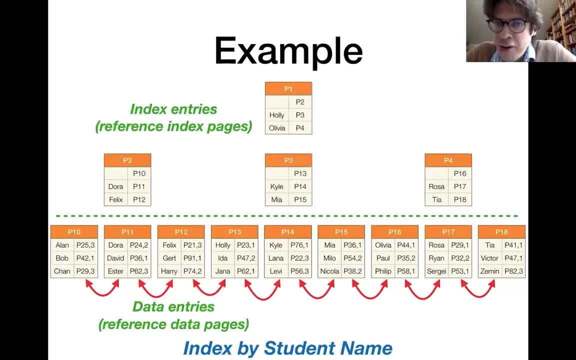 You will find it on CMS And I had questions about putting it on different platforms, So I will also put it on Piazza And you have one week for doing the homework. It focuses on SQL, as promised, And yes, Right. 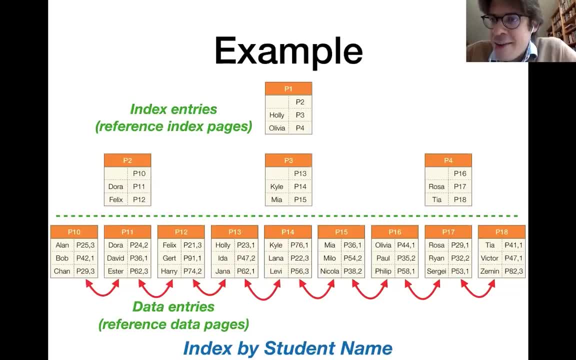 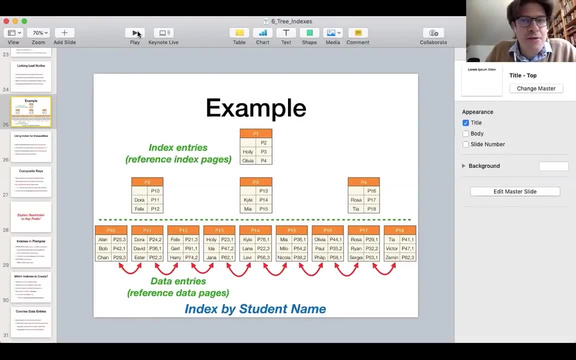 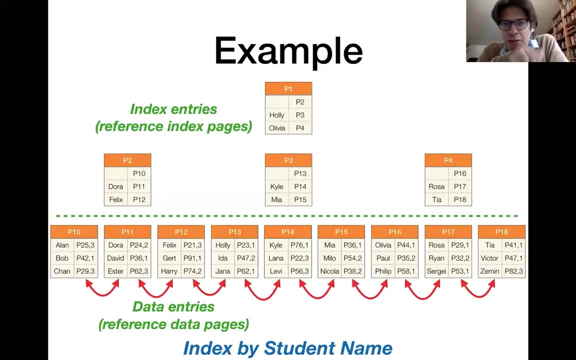 Good Then, have a nice day And see you on Wednesday. OK, So let's get started. Let's see what we have here. Let me quickly reorganize that a bit, OK, So the last time, the slide that we finished with: 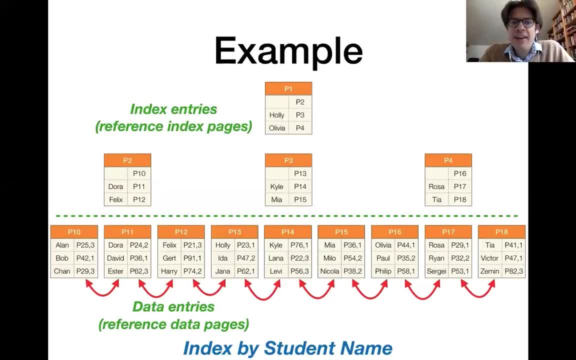 that is this slide over here, I believe, And what we see here, that is a tree index which indexes by student names. So if you have a table, for instance, like enrollment information, Entries that satisfy certain conditions, then an index is probably a good idea. 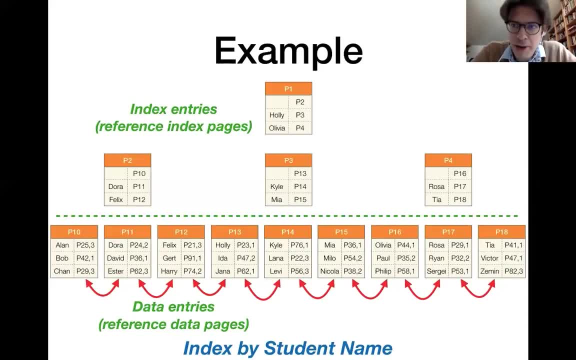 And in general, those indexes. as we have seen, they were pretty much like the indexes at the end of a book For a given search key. they provide you with references to the pages where you find the associated information. Now, last time we have been looking at those tree indexes. 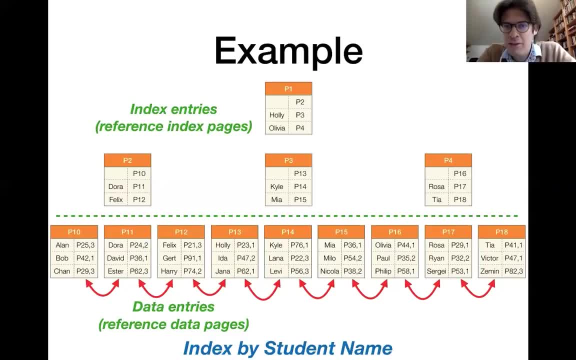 that you see here. So, in order to use this, we have to find the indexes, This tree index. here, for instance, in order to look up data associated with one specific student, we would start at the root node, which is page 1, P1, on top of the page. 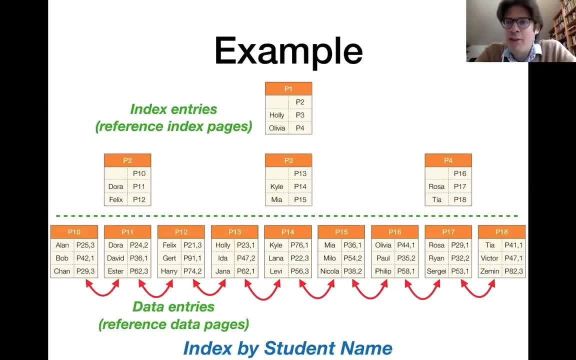 And if you're searching, for instance, for student Alan, then we would compare Alan against the keys that we see here, And we see that, in alphabetical order, Alan comes before Holly. So that is why I want to continue with page 2.. 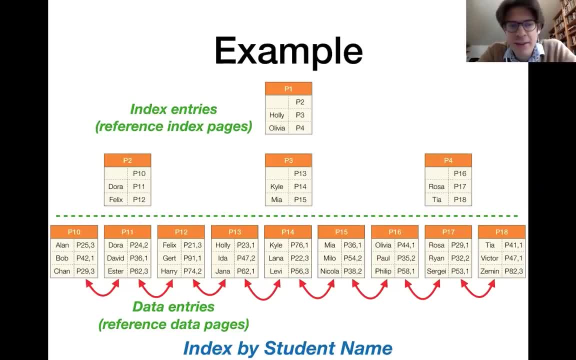 And on page 2. I'm comparing Alan against the students again, And it comes before Dora. So that's why I'm continuing with page 10.. And on page 10, indeed, I see the student named Alan, If I want to find, for instance, all students. 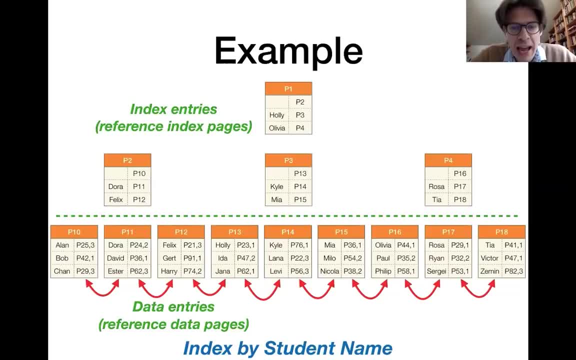 within a certain range of names, everything between Alan and Kyle, for instance- then I would start as if I wanted to find all the information about Alan, But then afterwards, after I have reached page 10, I would use those things between the leave pages. 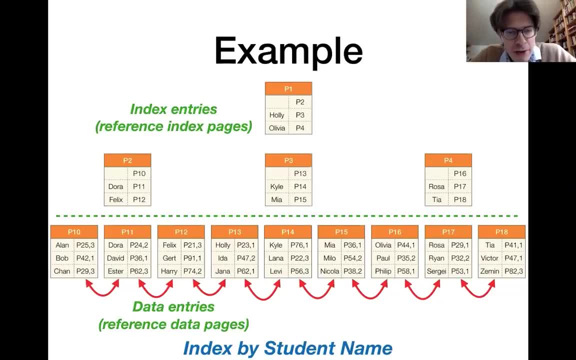 in order to continue to page 11,, page 12,, page 13,, page 14.. And here I find Kyle's and the names that come after Kyle in alphabetical order. So this is when my search stops. So this is how we can use those indexes. 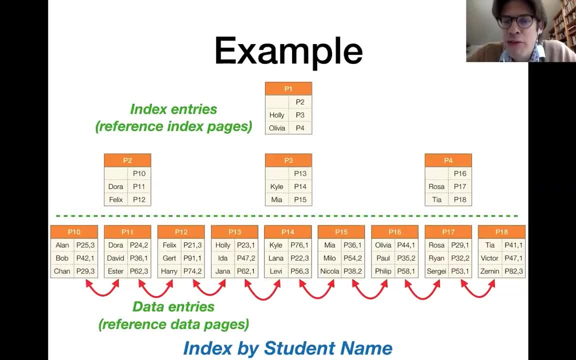 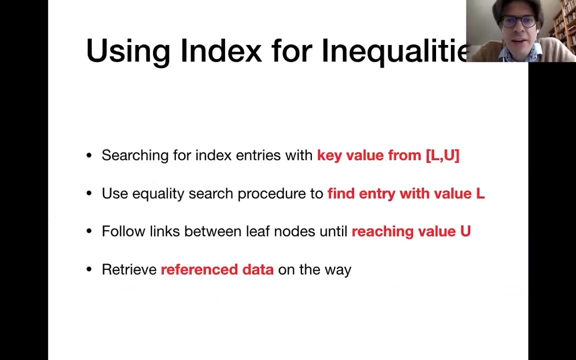 And you can have multiple indexes for the same table with different index search keys. One index for student names, but index, for instance, for course, information. all right now. this here summarizes more formally the treatment of inequality predicates, which I have just done. so if you are searching for search keys within certain bounds, L. 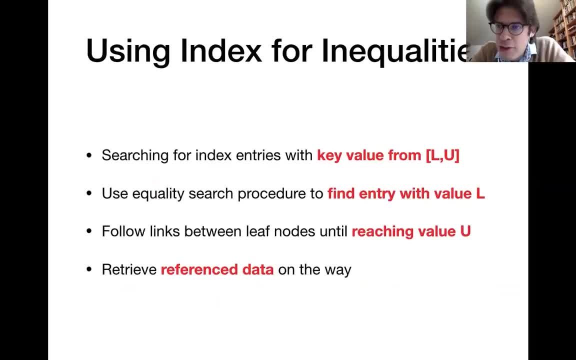 and U, then what we do with the index is that we first search for the first page, for the first leaf page from which we find entries for L, and then we use those things between the leaf pages in order to traverse the index and we keep reading until the entries the encounter come after U in the key order. all right, 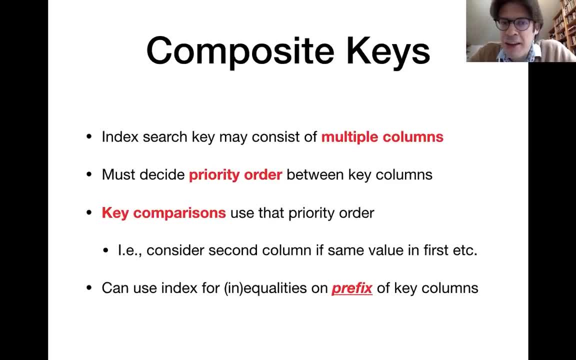 so this is ways we can use those indexes, and so far we have been discussing about search keys that correspond to L and U, and now let's talk a little bit more about search and the use of L and U and L and U and U, and we can use these in other ways with other groups, but 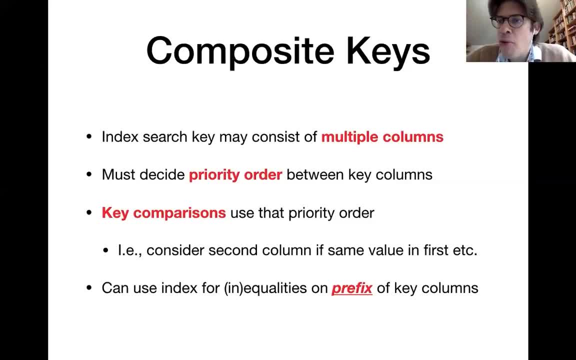 one thing as well that we can use for L and U and find objects. so search has to be used after all. okay, let's just say now, let's say we have our web shop and then we have a deep web shop, and if we look at our web shop we have a, basically. 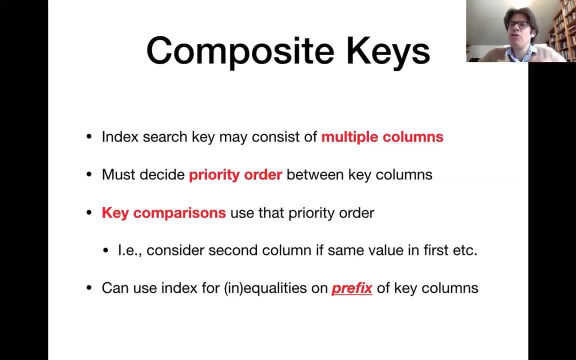 simple column of items and all right now, when we start searching for our web shop, we have a table with information that is in there, but sometimes we do not see any product. but we have already information about the product that is in there and that's want to start a targeted advertisement campaign. it might be useful to retrieve customers that are 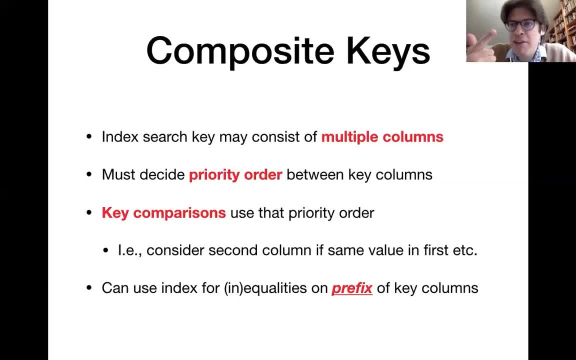 defined by a specific SIP and by a specific product that they bought last. So I want the combination of the two properties And, in those cases, an index which uses the combination of the SIP code and of the last product as a search key might be useful, And you can do this in. 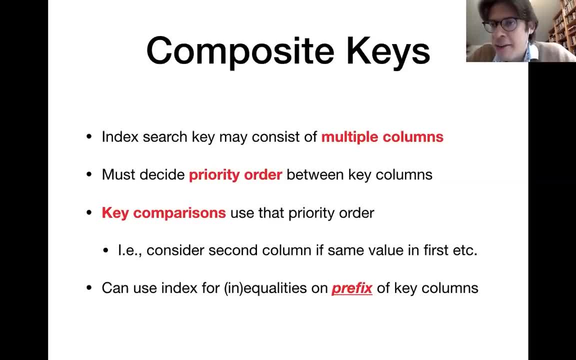 relational database management systems. You can define indexes that use a search key, a combination of columns from the same table. What you need to do in that case is to decide on some priority order between the different columns that appear in your key. You must decide whether it is first SIP code. 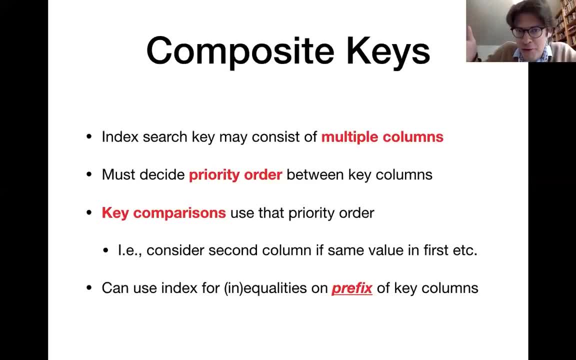 then product, or whether it's first product and then SIP code, for instance. Now, this order matters for all of these things, So you can define indexes that use a search key, a combination of columns from the same table and then SIP code for the key comparisons. Now, in order to use one of those, 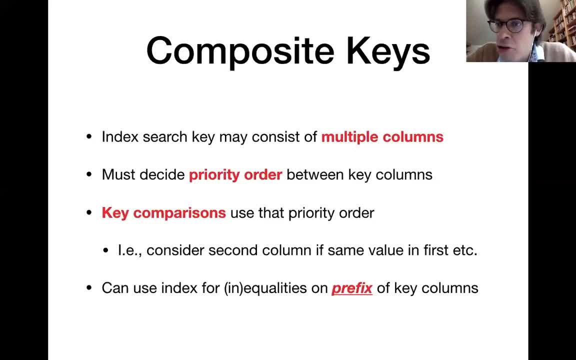 indexes. you have already seen that what you essentially need to do is that you go from one index node to another one And in each index node you must perform a couple of comparisons between different keys in order to establish which key comes first in the key sort order And the 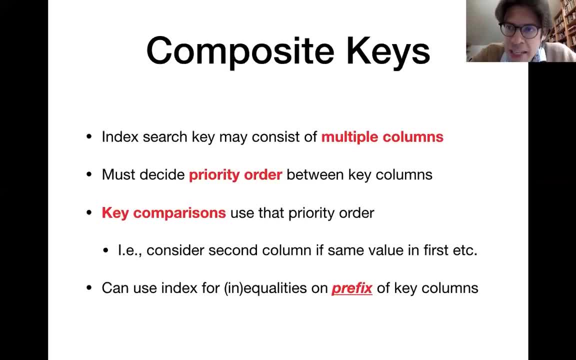 priority between different columns in your composite keys matters for how those comparisons are executed. For instance, if we decide to start the index key with the SIP code and then later comes the product, it would mean that then comparing those composite keys- when comparing two keys, I would 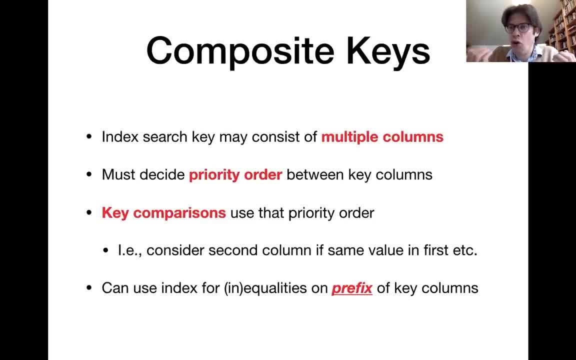 first look at their SIP codes And only if their SIP code is the same one then I'm going further to the product and see which one comes first according to the product. So during those comparisons I treat those component columns of your composite key in the order in which they appear in the key. 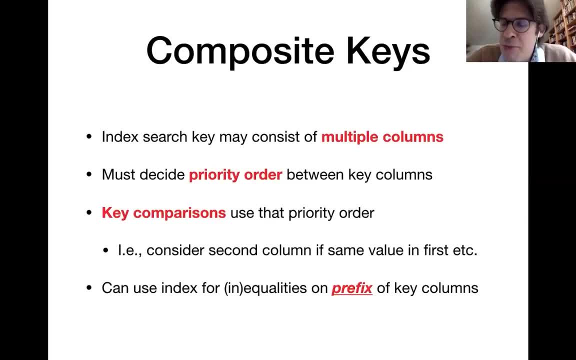 And because of that it means I can use those index data structures in order to retrieve entries that satisfy predicates which are either equalities or inequalities on all key columns or on some prefix. So if you have decided to first use the SIP code and then the product in your composite key, 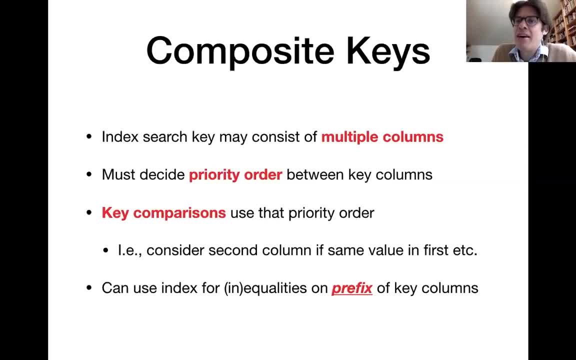 then you can use this index to answer queries that restrict only the SIP code, but you cannot use them in order to answer queries that only restrict the product, Or at least it's not recommended to try that. It would be inefficient. Can anyone tell me why we have this restriction to key prefixes? 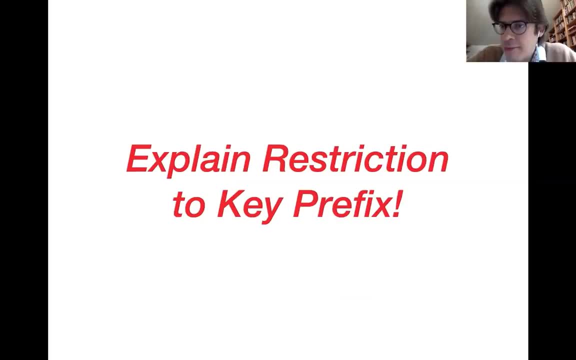 In your own words in the chat, Some intuition for why that is the case, Or you don't even need to put it into the chat, Just think about it a little bit for a minute. It's good to verify your understanding of indexing structures. So if you have a composite key, 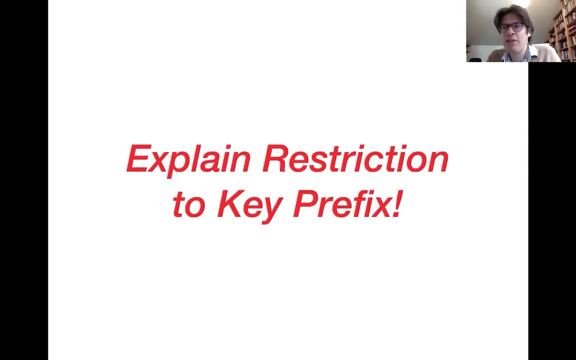 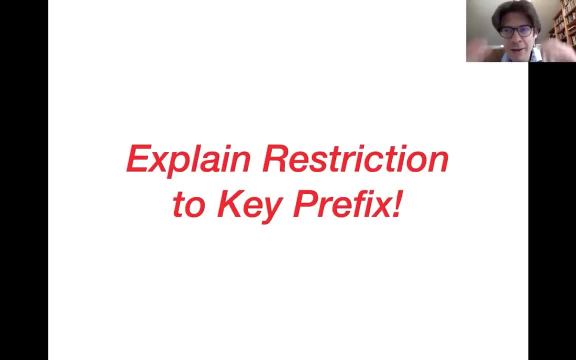 the SIP code, but not for single restrictions on the product. Can anyone have some intuition for why that might be the case? If you imagine what the index looks like, Particularly if you think about what you have in the leaf nodes of the index? 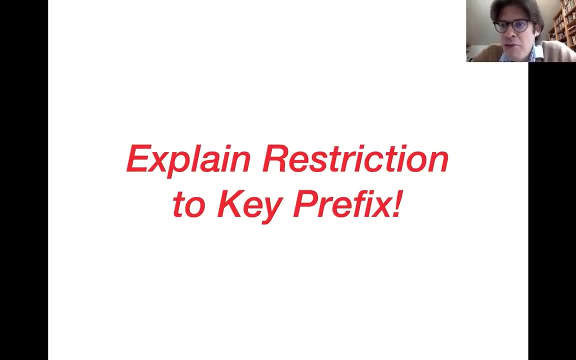 Ordering the SIP code before the product. Ordering the SIP code before the product means that the SIP code will be prioritized in the key comparisons. Give you a few seconds to marinate with it. Give you a few seconds to marinate with it. 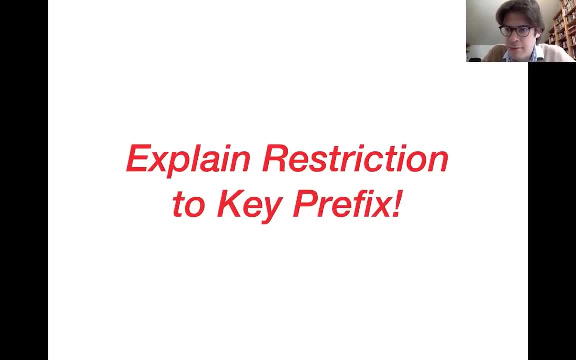 okay, yes, very good, and i think i see the right. yes, so here i basically i see the right references. okay, very good. um, you have to think about the, the source order. indeed, now, if you think about the order in which the entries appear only in the leaf nodes, for instance, if we prioritize the zip, 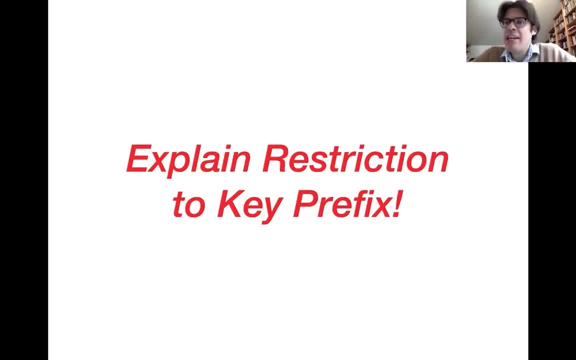 code in our comparisons as opposed to the product. it means that things with the same or similar zip codes will appear close together in the leaf nodes of the index and on the other side, if we prioritize the zip code in the comparisons, then things that have the same product- customers who 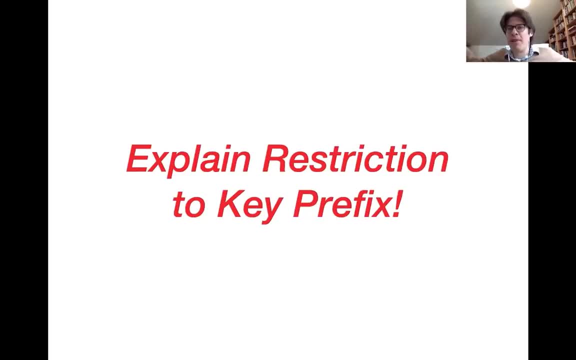 bought the same product, they might appear all over the place. basically, they are not necessarily close together. and those index structures, they are only efficient if they are used to retrieve data that appears close together in the index. so if you have prioritized the zip code in your comparisons, 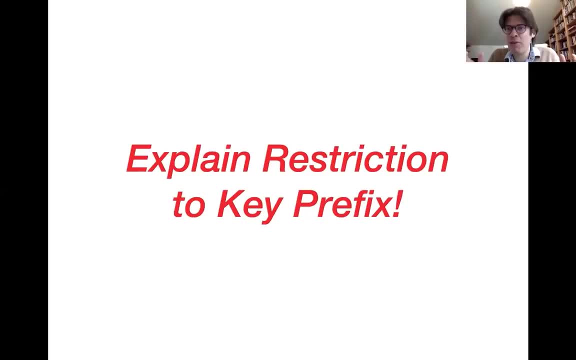 then customers with similar zip codes will appear close together in the index, and that is why you can retrieve them quite efficiently. on the other side, if you want to retrieve customers who bought the same product for any zip code, then those customers will be distributed over the whole range in your leaf nodes. so it is. 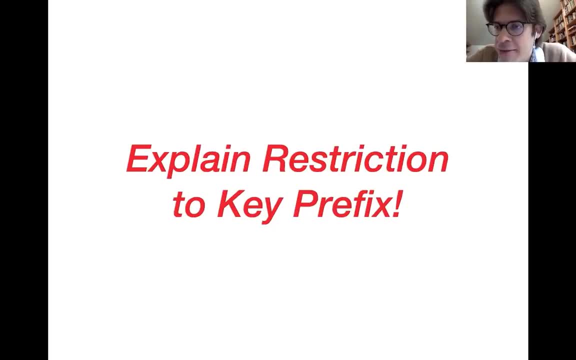 not particularly efficient to retrieve them with the index right. so maybe as a little homework it might make sense to imagine how that index with the composite key looks like and, for instance, make a little drawing. but here the core idea why we want to restrict ourselves to the prefix of the key. 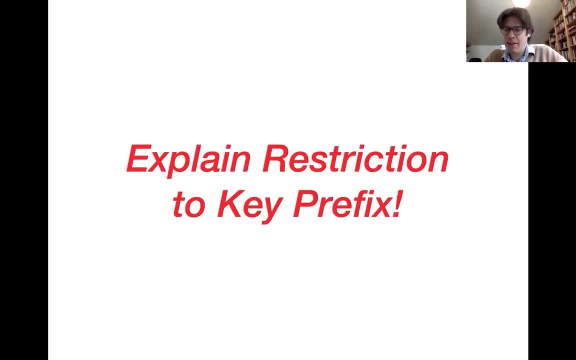 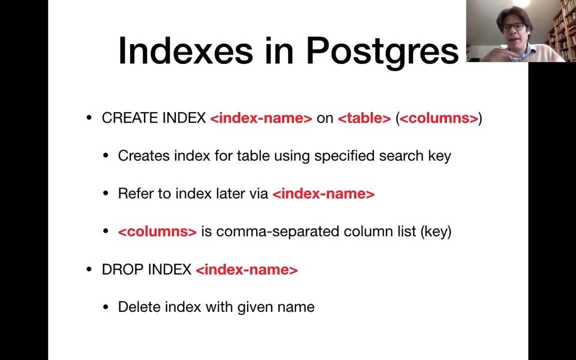 columns is right here and was in the chat. good, now let's have a look at Postgres. so far we have been discussing about indexes in a rather abstract manner. now let's see how they actually appear in a real database management system. now, in postgres, for instance, and in most other database systems too, you can decide which indexes 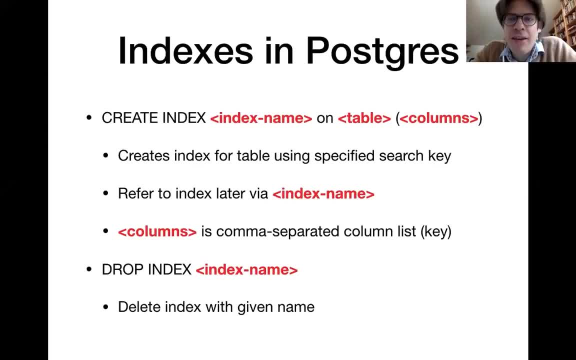 the database system should create. there are commands for that. they might look slightly differently in different database management systems. in postgres you simply write create index, then some index name on the table that is being indexed, and here between those parentheses you have a comma separated list of they grown will be a valid index. let's have an x and these indexes or 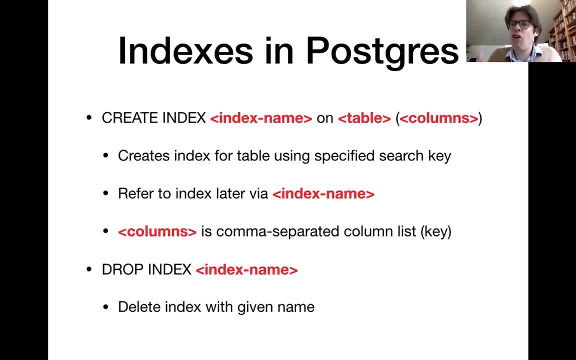 inner benches comes with a88 provides some kind of index specific within. in this case this brings to table columns, and those are the columns that the index should refer to. So it can be one column or it can be multiple columns. In that case it's a composite. 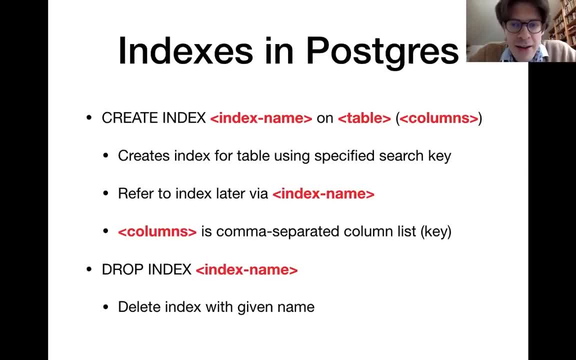 index Now here. yes, so here you have the syntax, and the reason that you can give a name to the index is that you can refer to that name later. For instance, maybe at some point you want to delete the index again, and then you can do. 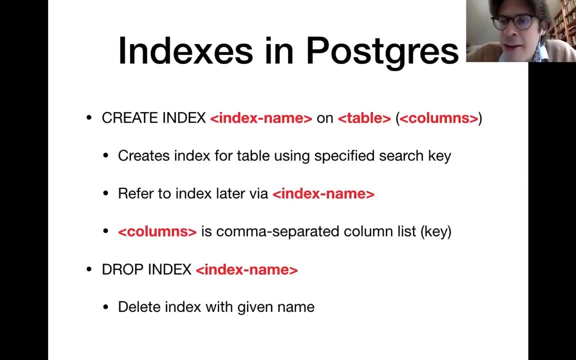 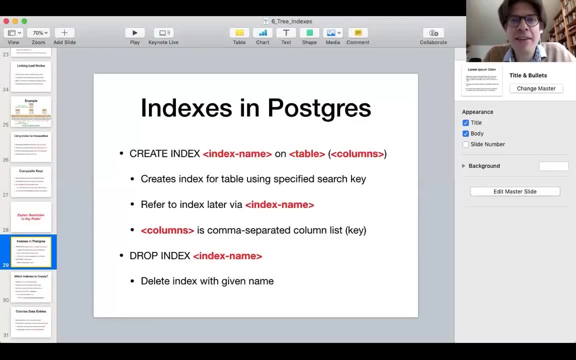 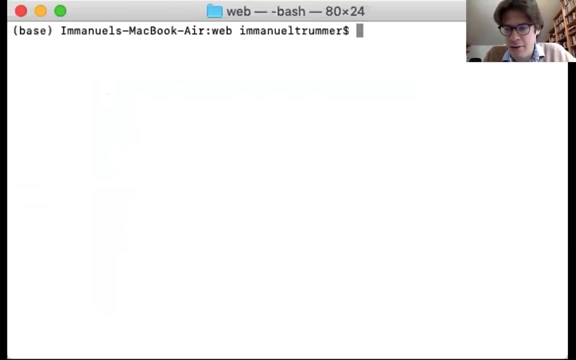 this with the command that you see below: Drop index, and then you'll write again the index name. I'm quickly going to demonstrate that in Postgres, just like you have seen in index creation once. Alright, now you should be able to see my terminal here. 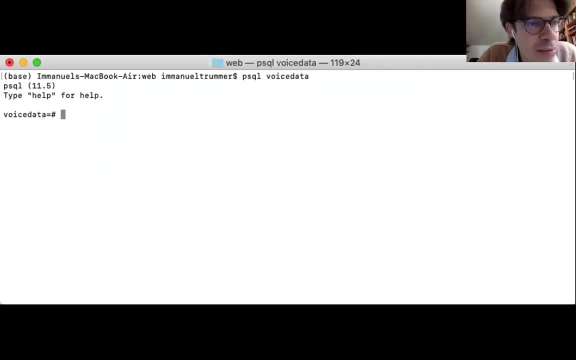 Let's actually look in logit. Where should I install this? By pumps and all kinds of things. but this is what I do work with. You can do that at least all about on the whole domain doomed with the data There. you can see that what I did with 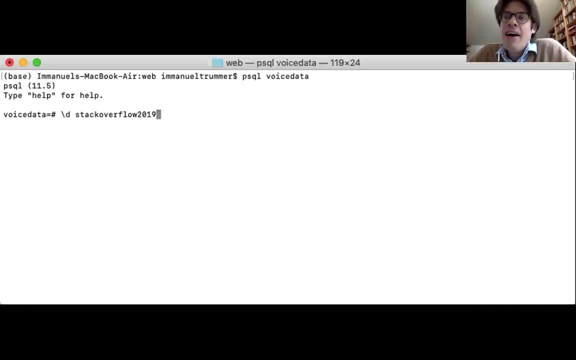 framework array, what I did with pipelines, and now we'll talk about mybecause dest kaye database. Sometimes it takes time to do that database All right, And what I have here, for instance, is OK. and here I have, by the way, an interesting question in the chat. The question is whether you have to explicitly tell the database management system. 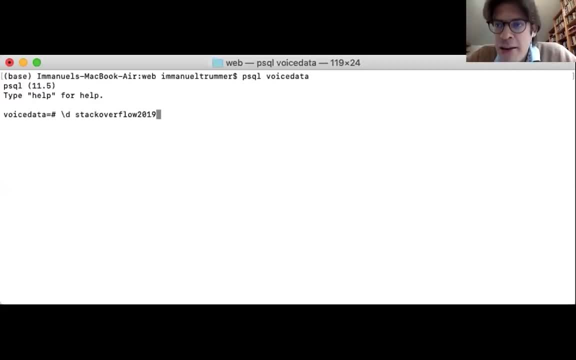 automatically. most of them allow you to control which indexes are created, because it's a decision that is difficult to make automatically. I'm going to say a little bit more on this in the following: in the following slide about the pros and cons of creating indexes and. 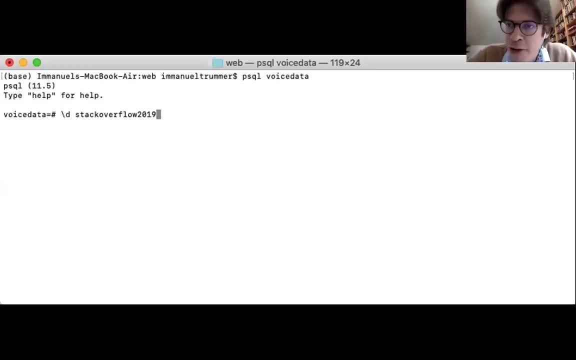 how to decide which ones to create. But for the moment, let's first of all look at a concrete example where we are creating indexes in a database. So what I have here in the database, that is the results of the stack overflow developer survey. you make a big survey among 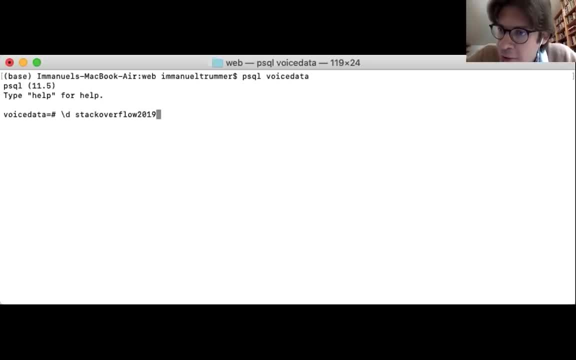 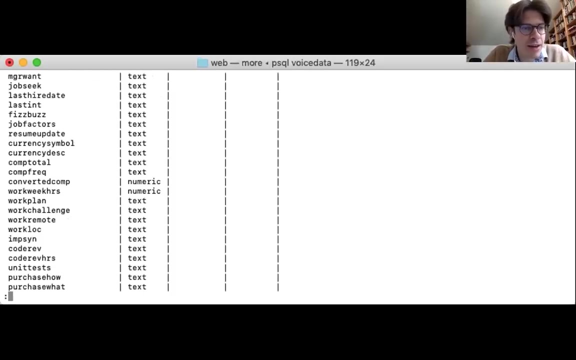 software developers every year and they publish the results And they ask questions about all kinds of details about their job and so on. And here I have the data from that survey And here you see it has many columns which correspond to different questions that were asked And the number of entries. 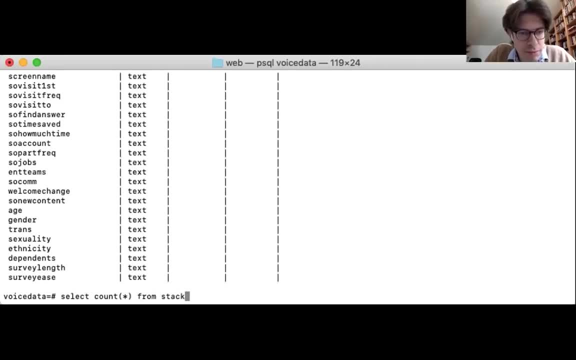 the number of entries here, that is about 90,000 respondents. So if, for as far as surveys go, this is actually pretty large, As far as data sets go in general, of course this is not that large, All right. 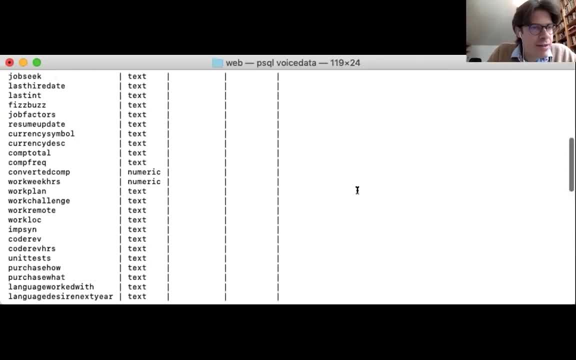 So, for instance, there's a column about the country that the developers come from. I could, for instance, want to count how many participants we had from different regions of the world, And in order to make that efficient, maybe I want to create an index on the country column. 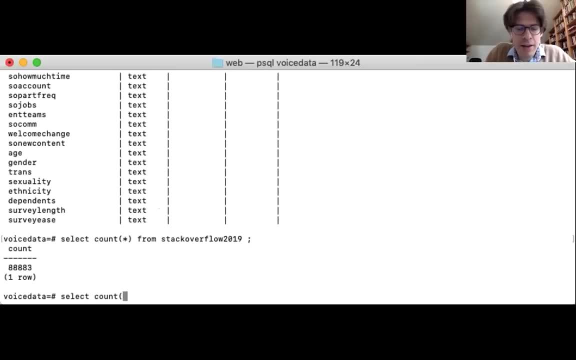 Let's maybe first try the query without the index, If we- Oh and, by the way, let's quickly enable timing of queries in order to be able to compare performance with and without indexes in the following. So we enable timing, And now let's. 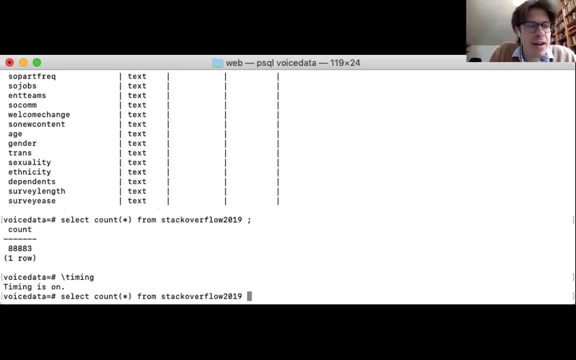 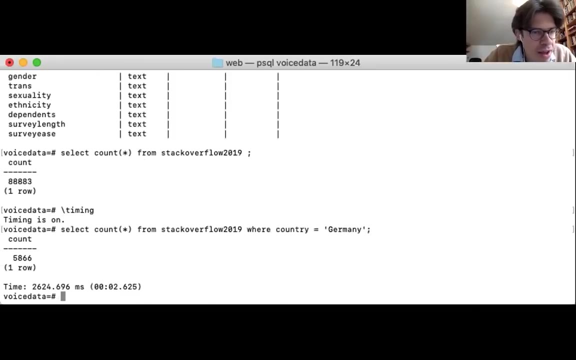 first of all count the number of participants, for instance from a country in Europe, Let's, for instance, say Germany: All right, Okay, All right, All right, All right, Okay, And that took a little bit And we have something like about 6,000 participants. I'm running. 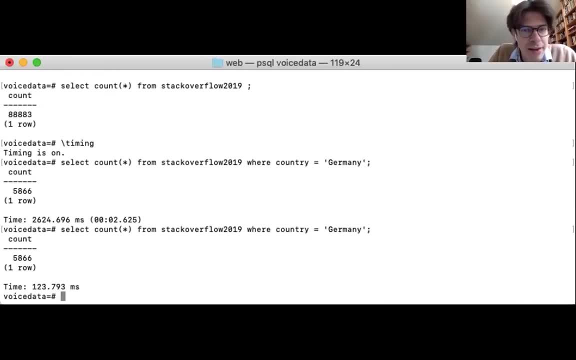 the query again, And now it actually gets already much faster. That is something that we discuss in more detail in the following lectures. Those database management systems: they're able to cache data that was recently accessed. So, as you see here, the query suddenly. 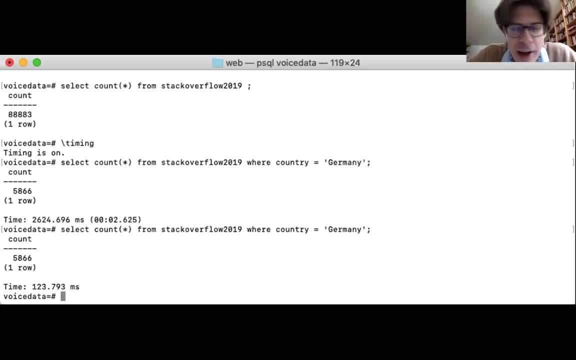 gets much faster. I wanted to get the Okay. The query is now now faster, more realistic time in order to make the following comparison more realistic. All right, Now let's see what happens if we create an index on the country column. 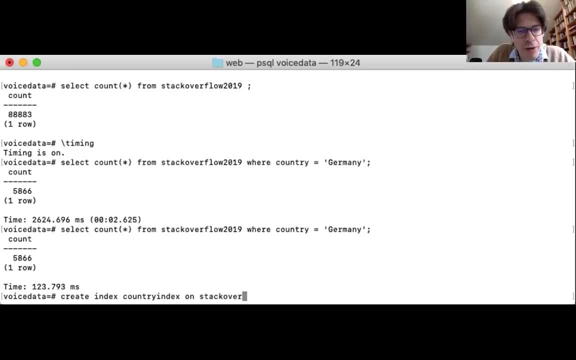 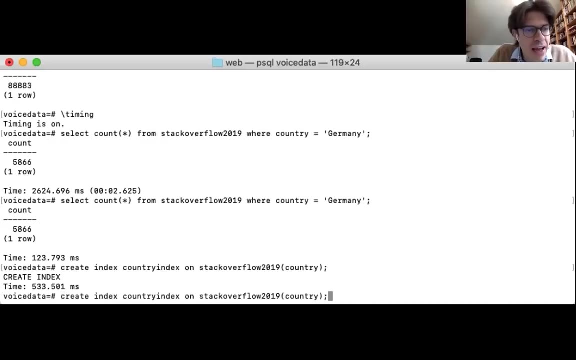 Create index- country index on the stack overflow table And the columns that we want. that is the country column. All right, So now we have created the index. It was actually pretty fast. And now let's run the same query from before. 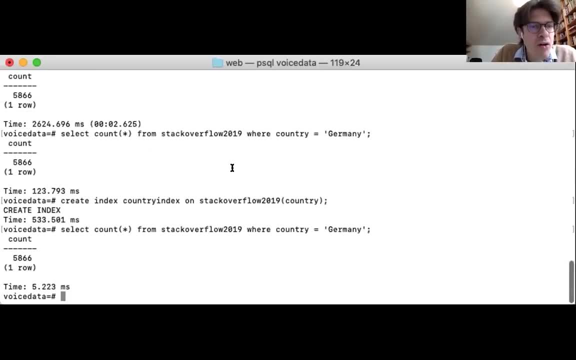 All, right Now. what you see here is the time for the query after we created the index, And, as you see here, it's about five milliseconds Now. without the index here we had something like 124 milliseconds. So this is, I mean, both are very small times, of course. So right now for data of this size. 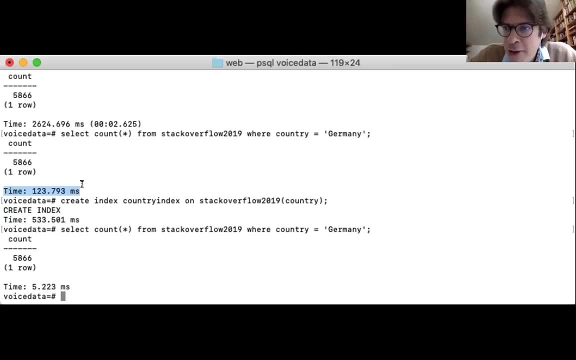 it doesn't matter so much, But you see that there's a difference of several orders of magnitude. If you mentioned that typically we would work with much larger datasets than that, then you can see. but having one of those indexes actually makes a big difference. 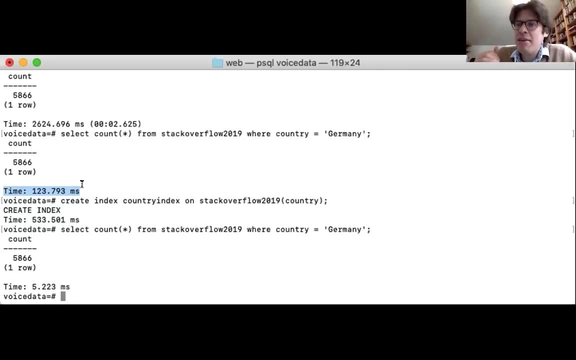 Because this country index now has allowed us to immediately retrieve references to those entries that are associated with country Germany, and that is much faster than having to go to all that, through all the pages of the table, in order to check whether there's any entries for German, for instance. now let's drop the index. 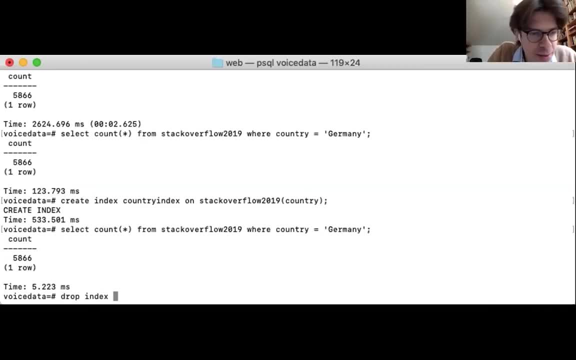 again, just to see whether it was all the coincidence, maybe that's one, the same query again. all right, so it's still getting a little bit faster, due to caching effects probably, but still it is the same order of magnitude as before. you are much faster than using the index and the command I used to get the time. 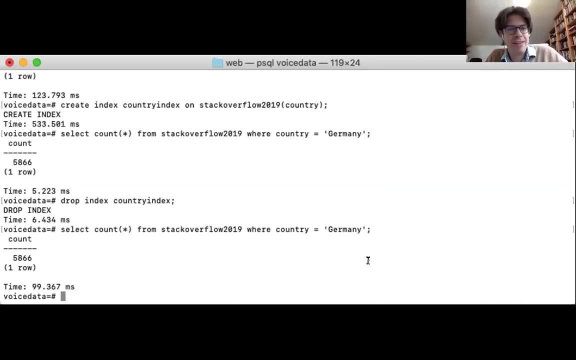 it is backslash timing, exactly. thanks, all right, mm-hmm. now perhaps one more example for a composite index, just that you have seen this as well. I guess I could, for instance, use the thing it was called employed or employment column, and here and first of all, showing you what distinct values appear in that. 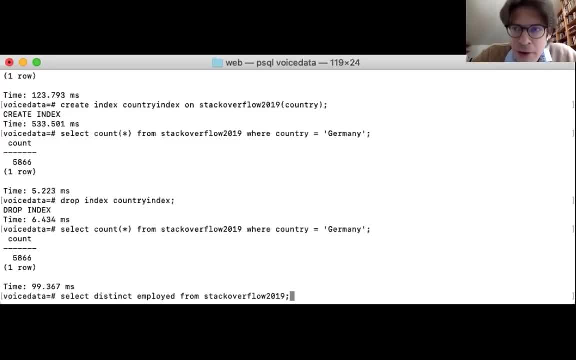 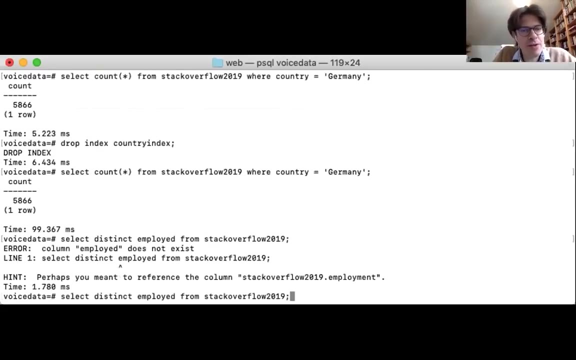 column. so this select distinct is, in my experience, pretty useful if you want to get a first impression of the data set. you want to find out which values appear in a certain column, which is what I'm doing here. make sure whether the column was called employed or employment. let's see. okay, it was actually called employment, and 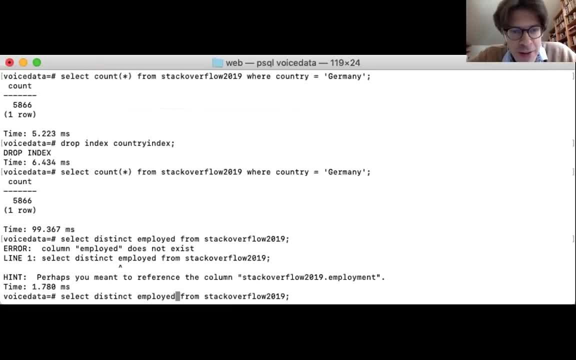 here you see a useful feature of Postgres. it actually it tries to correct the queries that you are entering by making suggestions. here we have referred to the column employed and it suggests that maybe I wanted to refer to the column employment instead, because it's a similar name and it is right. so that is. 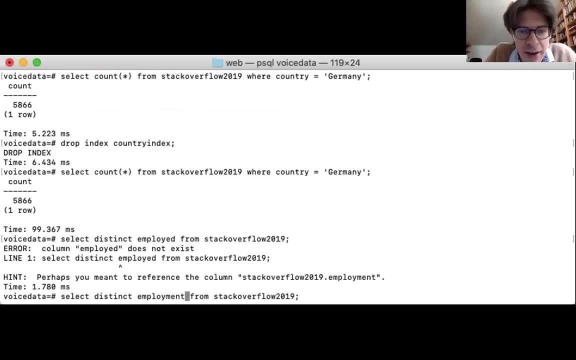 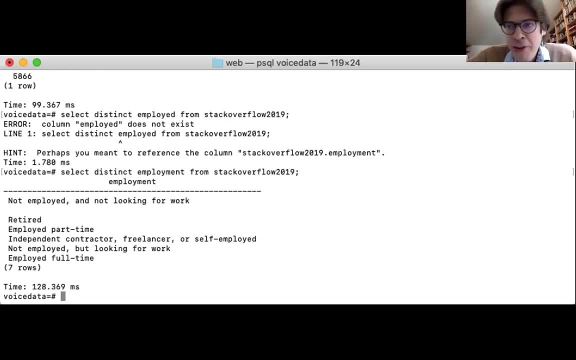 useful. let's look at the employment column instead. all right, so here there's a couple of different employment statuses, and perhaps, for instance, I want to count the number of retired employees in Germany or in France, or in the US. so let's actually create an index that allows me to quickly look up entries that satisfy a predicate. 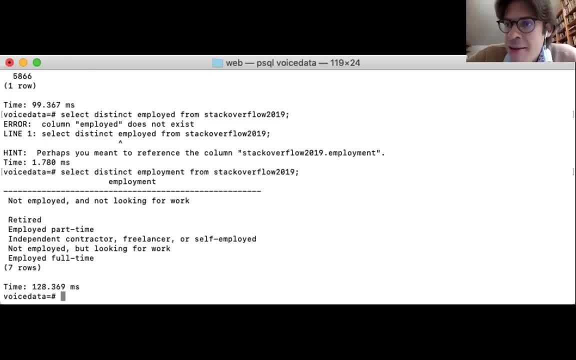 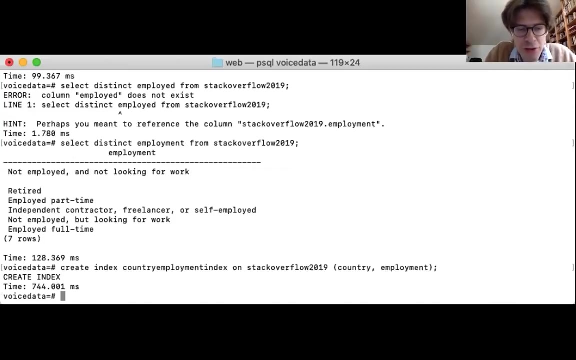 on the employment status and another predicate on the country. so let's create the country employment index on the stack overflow table, which uses the columns like country comma: employment. all right, okay. so now we have created this index, which is also quite quick to do, and now, for instance, we could select the number of retired employees in Germany. 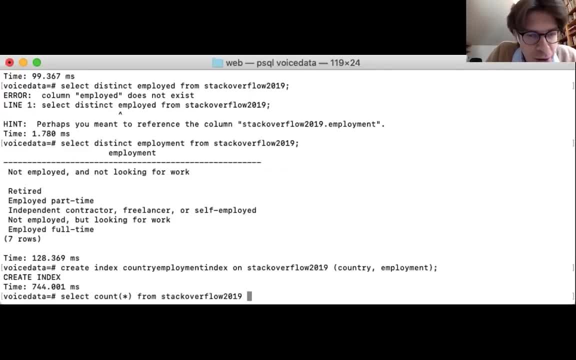 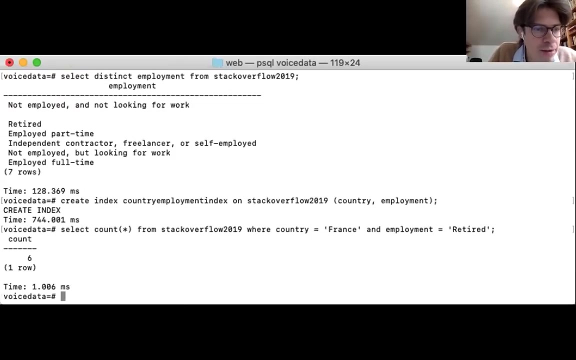 so let's say we've got one here and we can actually take a look at the number of developers where country equals Germany. let's actually take France for a change, and employment status is retired all right. so that takes one point zero zero six milliseconds. it's actually very fast. 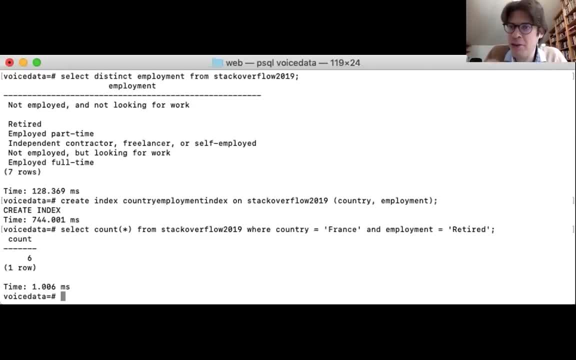 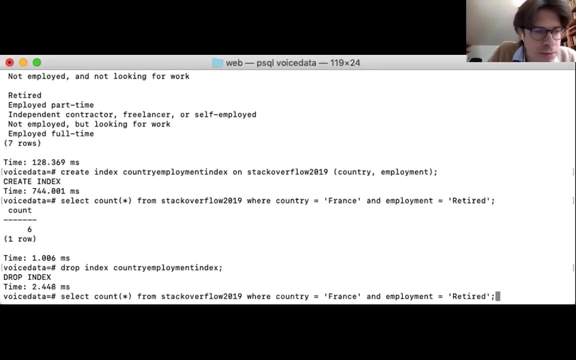 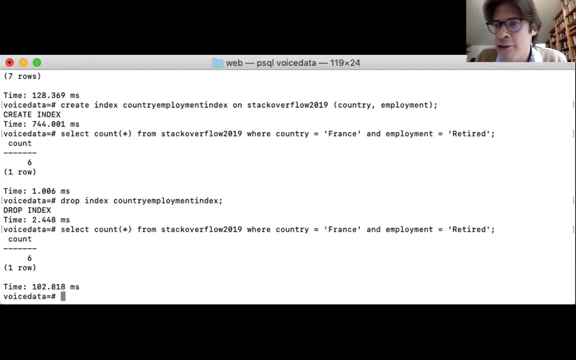 do? we only have six entries, because it's quite a specific combination of properties. let's actually drop the index in order to see what we get then. all right, and as you see, here again we have an execution time that is by orders of magnitude above the one without the index, even though for those small data sizes, of course, it doesn't. 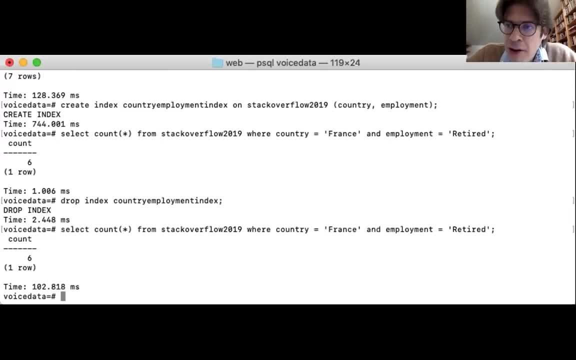 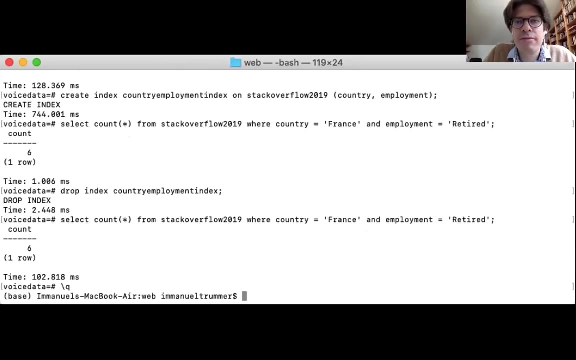 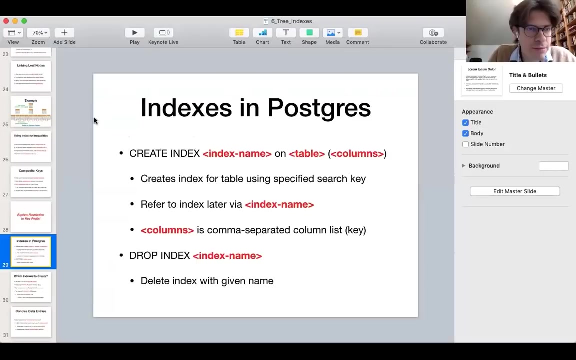 matter too much, but if you have a large database and your queries process slowly, then thinking about creating some indexes to support them is probably a good idea. okay, all right, let's go back to the slides. so this is the syntax in postgres and, as always, i encourage you to play with it a little bit. 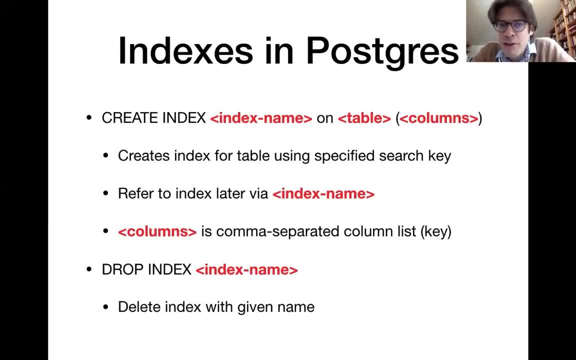 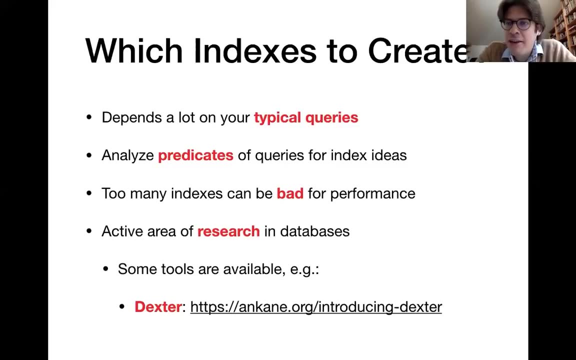 yourselves if you have already tried some data sets. in principle, those commands also work in the db fiddle. now one question that was already raised here is which indexes should we create generally, or whether the database management system can decide all by itself or by itself. so i'm going to 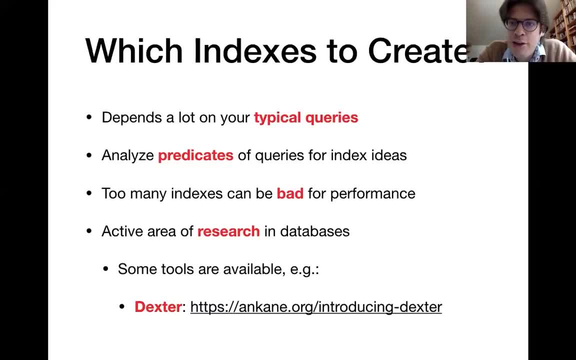 go back to the database management system, and i'm going to go back to the database management system and i'm going to go back to the database management system and i'm going to go back to the database management system by itself. which indexes to create? now, first of all, let's discuss a little bit about how you can. 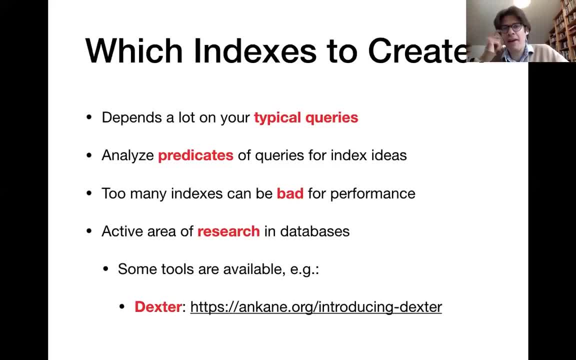 decide which indexes to create in a specific situation. and in order to decide which indexes to create, you generally have to look at the typical queries. in particular, you have to look at the predicate, meaning the where clause of those queries, which gives you some ideas for candidates that might make good indexes. 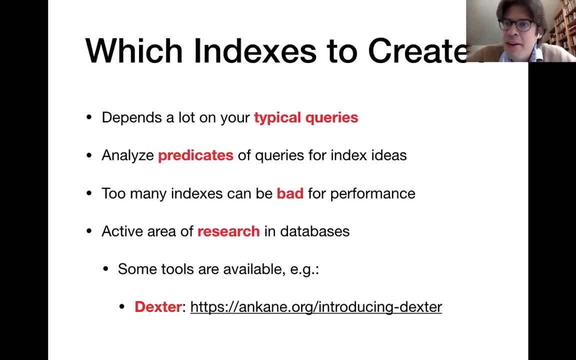 which perhaps may change a little bit now. in the examples that we've seen here, creating the index always reduces query execution time, so i don't want to mislead you into thinking that indexes are always a good thing to use for performance, because that is definitely not the 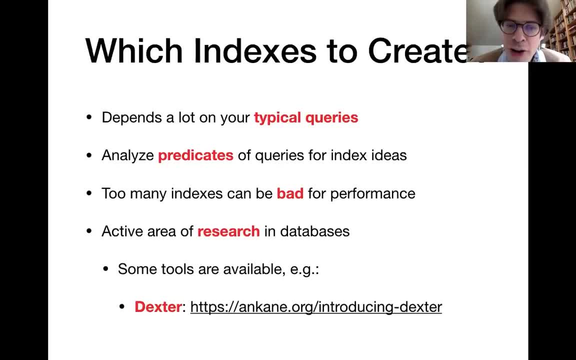 case now, first of all, indexes. they are, for instance, not useful if your predicates are not selective enough. so if your predicate actually is satisfied by your�� most of the entries in your table, you don't really need an index for that query. Another reason is that- and we will see this in more detail in the following- if your data often 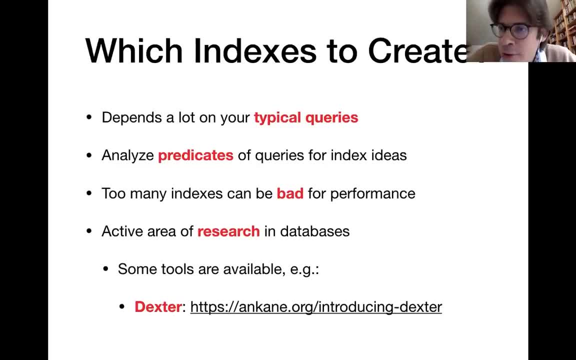 gets updated, it means that each associated index also needs to get updated, which also causes some overheads. So if you have too many indexes then it will be very expensive to update your data. We're going to discuss more about index updates in the following. 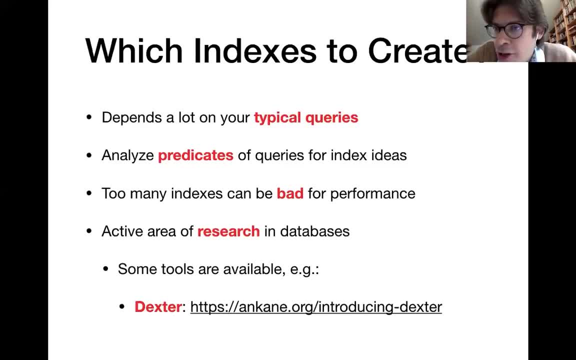 And then finally, of course, each index is a data structure again, so it needs some space. That means the more indexes you create, the more space you use up on hard disks, So at some point you probably run out of space. But a question about which indexes to create is really an 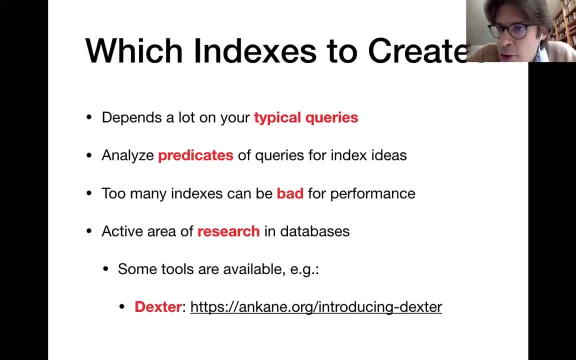 interesting one and it's a difficult one. So in the database research community you're already looking at that question- how to decide which are the ideal indexes to create- already since decades, basically, And research is still ongoing, so it is a tough problem. 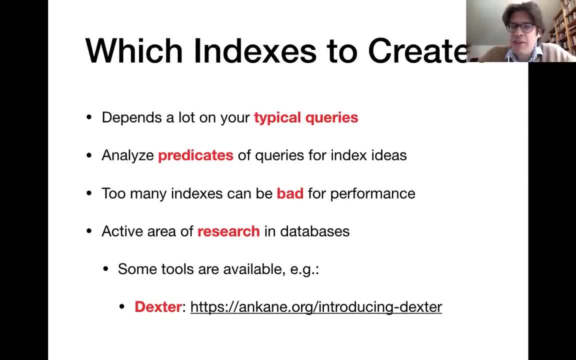 There are some tools available which allow you to do this. There's, for instance, the desktop tool for Postgres, which tries to figure out automatically what indexes you could create, And there are some database management systems that essentially automatically decide to create indexes, for instance the so-called monadb database management system. 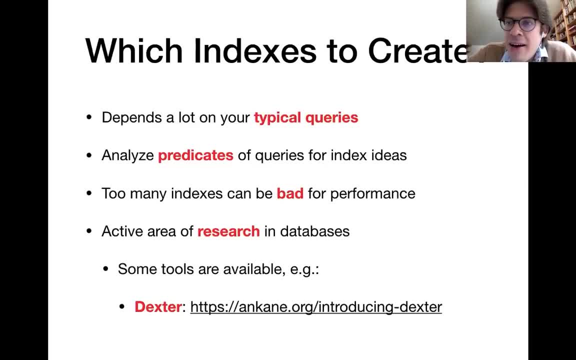 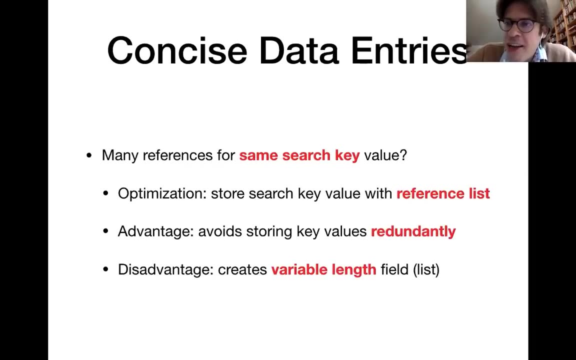 And those database management systems. they might create or drop indexes independently in the background, but in general it's very hard to decide what are good indexes to create All right Now. in the following, we're going to discuss about a couple of different optimizations. 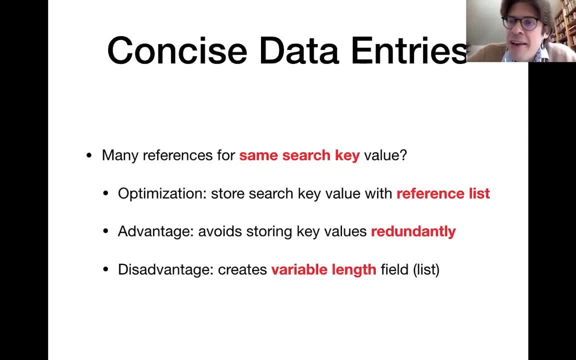 to indexes and also about how we can handle updates in the context of indexes. One thing that I believe was already pointed out by one of your peers in the last lecture is that sometimes you have the situation where your index stores duplicate keys. For instance, maybe for the enrollment table there's many entries for the same student. 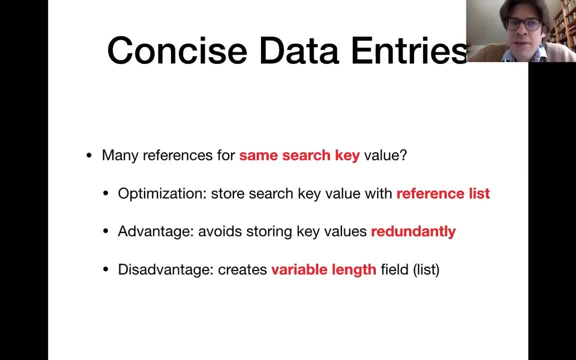 somebody who is enrolled in lots of courses, And then the question is: do we really want to store the name of that student repeatedly in our index, each time referencing the corresponding enrollment row? There is a more efficient alternative, which is simply that we store the name of the student once. 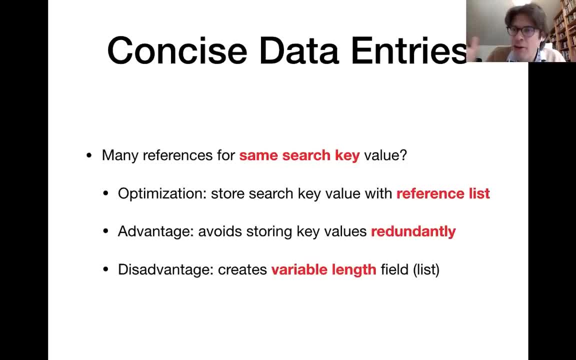 in a leaf node and then we store a list of associated references, So we just avoid repeating the duplicate key and index data structures. do that? There's a slight disadvantage to doing that, which refers back to the lecture on data layout, where we have seen how we decompose the space. 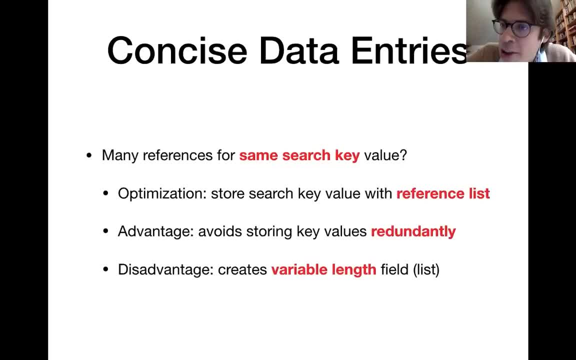 and one of those pages into smaller and smaller units, And we have seen that having, for instance, records of the same length often makes it easier to partition the space of a page. Now, if we say that we allow variable-length lists of references for one key, it means that we might. 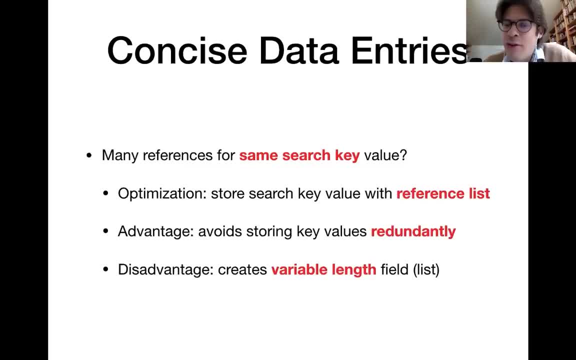 turn a fixed-length record into a variable-length record when we are talking about the entries in the index, And that makes a few things a little bit more difficult than handling all the bookkeeping associated to data layout. But that is a reasonable trade-off. 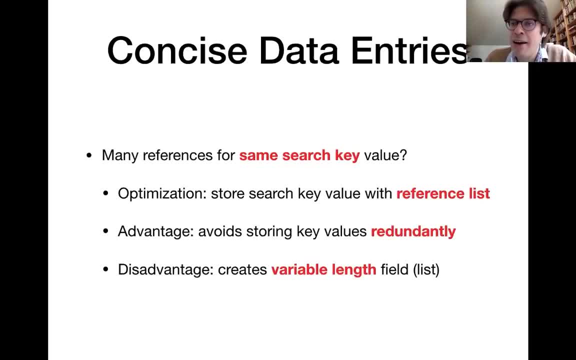 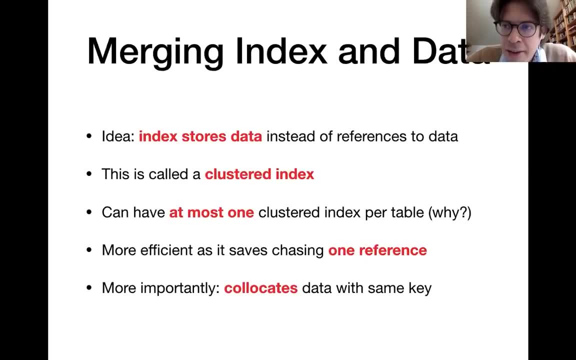 and in practice, you would typically avoid repeating the same key in your index. Another thing is this: Right now, the indexes that we have discussed, they store references to the actual data. In the leaf page of the index we have the so-called data entries, but often those 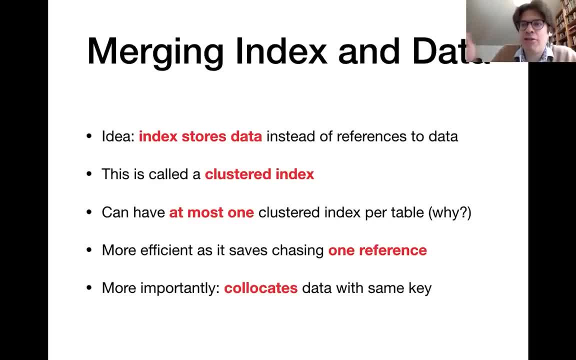 data entries correspond to references to the actual data. Instead of that, you could also just store directly the data that you're interested in in the leaf nodes, and if you do so, it's called a clustered index. Now, as long as you don't want to store your data, you can store it in the leaf. 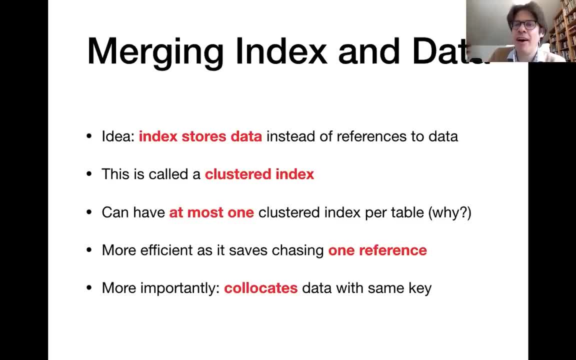 page of the index and if you store your data repeatedly, you can only have at most one of those clustered indexes per table. But that can actually be quite efficient because first of all with this clustered index you save one reference If you don't store the data in the leaf nodes. 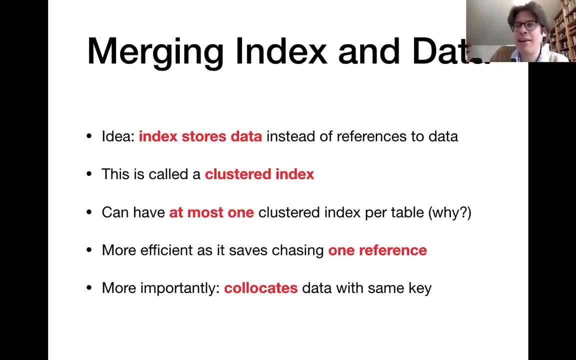 then you would have to follow up a reference to the data. If you store the data directly, then you can save the time for that. Secondly, if your index stores in the leaf pages references to the data, then in order to retrieve the data you have to follow all of those references. And even if those 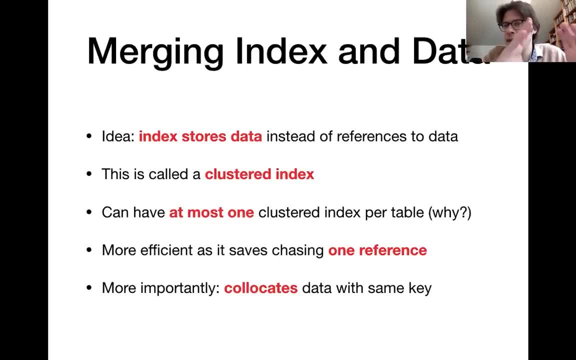 references are stored close together in the index leaf node. the associated data might actually be widely distributed in the data pages, And that means in order to collect, for instance, all the data for the same student, we might actually have to access lots of different locations in your 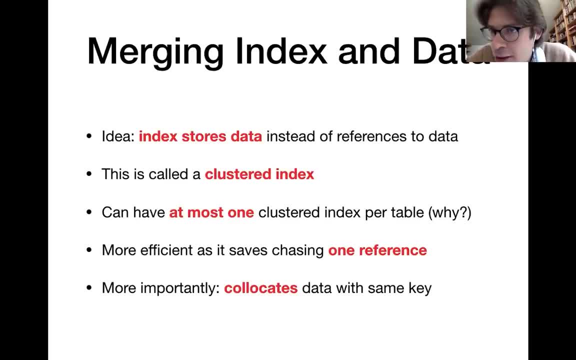 actual data set And that can be inefficient, As we have seen. for instance, if you store the data on hard disk, it means you have to move your read and write head quite a few times, which takes time. So if you store the data instead inside of the index, it means that you are guaranteed. 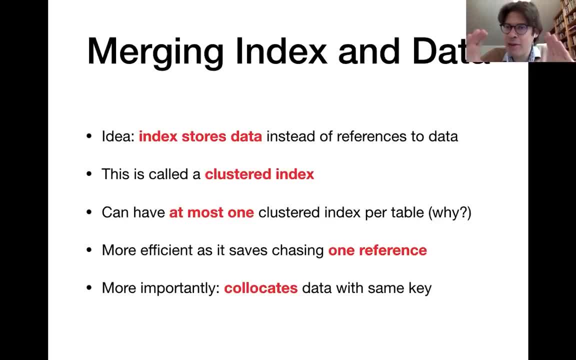 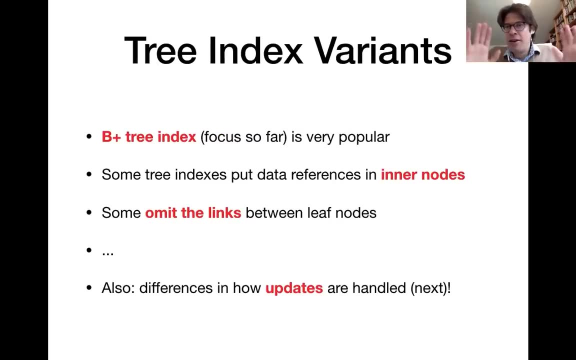 that all the data for the same student appears close together And that can be retrieved efficiently with one or at most a few page read operations. So that's why you might want to use clustered indexes, if you can. Now, this is just some overview of the indexes and the optimizations that we can apply to. 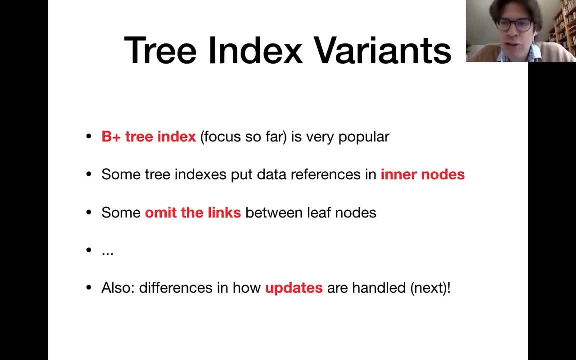 them. What we have seen so far pretty much corresponds to a very popular brand of index, which is the B plus tree. That is also the default index created by Postgres, which we have just done. There's several variants of that. for instance, there are a tree index variants that put a data entries, meaning references to. 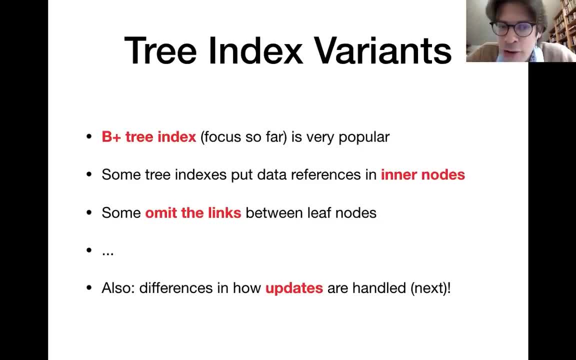 data or actual data in the inner nodes of your tree, as opposed to the leaf nodes only. There's some variants that omit, for instance, those useful links between the leaf nodes and the tree indexes. So if you have a tree index, which is a tree index. 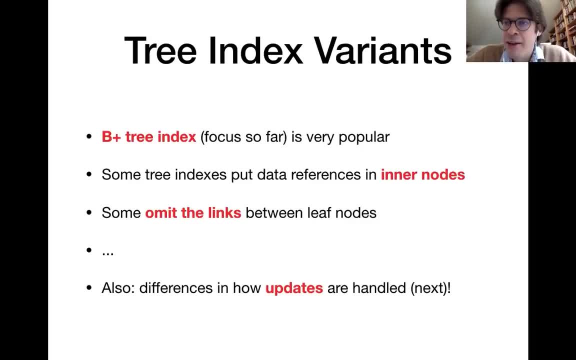 and so on and so forth. there's many variants of that, But in practice one of the most common indexes is this B plus tree, which essentially we have been discussing about so far. Now, one important topic in the context of indexes is data updates. The index indexes the data, so if the data changes, the index 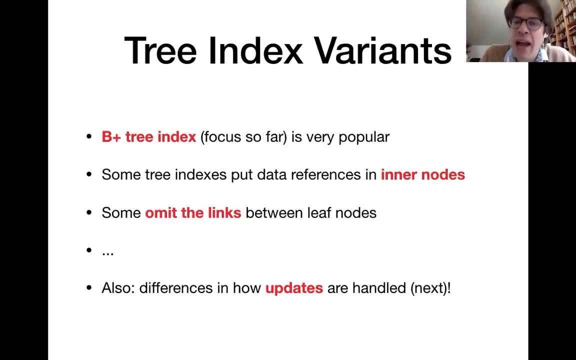 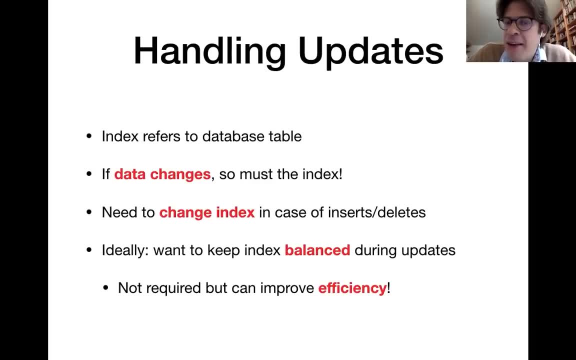 must change as well And there's different ways to handle data updates. Now, if you have a tree index, which is a tree index, which is a tree index, and you can have the index and the tree index which is a tree which is a tree index, now, generally you might have inserts or 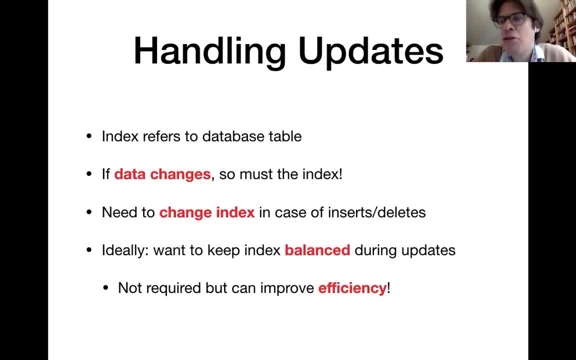 deletes to data or updates, which you can imagine as a combination of a delete and insert. even to practice, this typically implemented more efficiently. If your data keeps changing back and forth, then one thing that you might want is that you keep your index tree somewhat balanced throughout a 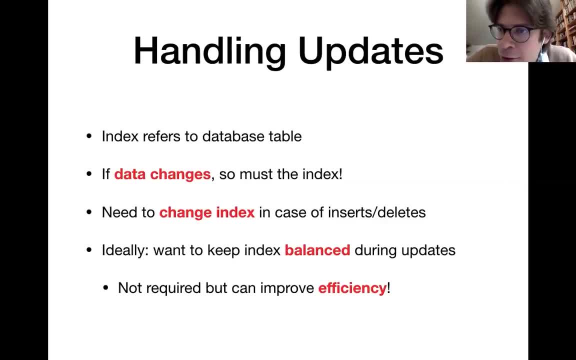 all those insertion and deletion operations, And you might already have seen that in the context of general search trees. Now, often with those search trees, it's a good idea to keep them somewhat balanced in order to maximize efficiency. Now, in the following, let's first of all see what happens. 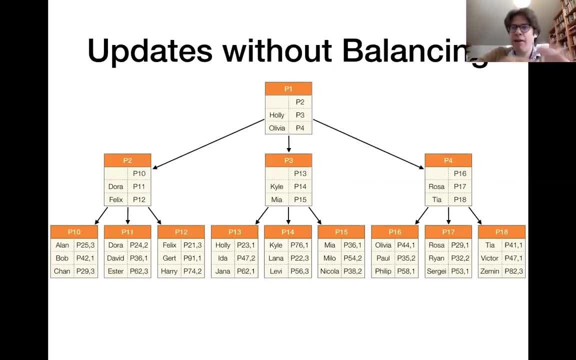 if we don't balance the tree after updates. Here we have the index tree for students again, and now we are inserting a new student called Bella, for instance. Now, if we start from the root and go down to the leaf nodes, page 10 is where the student Bella should be inserted. 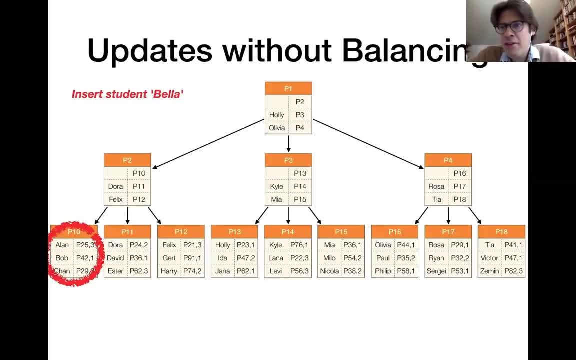 according to the alphabetical key order, But unfortunately you see that the page is full. We don't have any free space left. Now what we can do is that we create a new page- page 19,- and we insert the student name there. 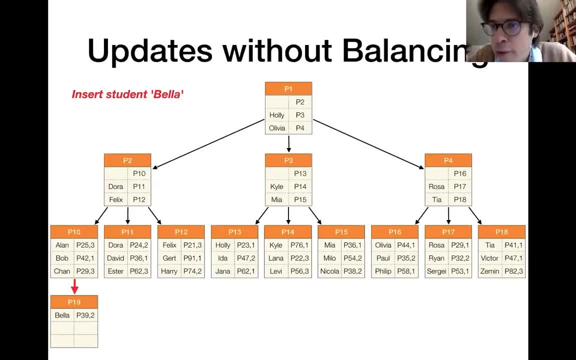 And that here is called an overflow page in this context, because it becomes necessary as the data in page 10 is overflowing, so to speak, And you also see this little arrow in red pointing from page 10 to page 19.. That essentially represents a little pointer reference. 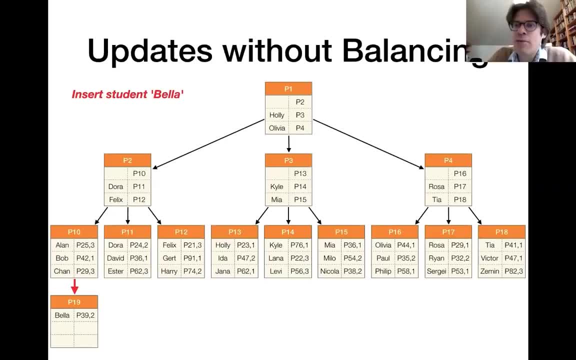 that we store as metadata on page 10, which points to the following page: page 19,. page 19,, page 19.. So that's the one thing that we keep going into is serving overflow pages, As long as there's no overflow page. 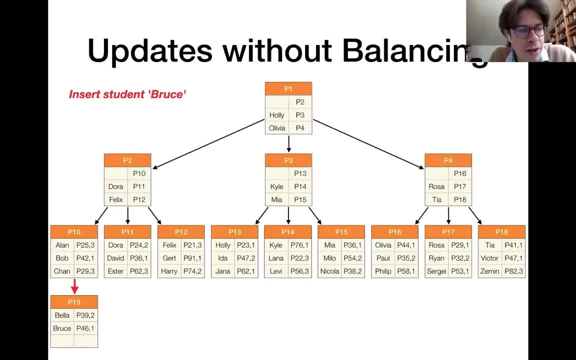 we simply set that pointer to null. essentially, Now we are inserting Bruce as well, and we still have space on page 19.. Now we insert Cara, And now we want to insert Connor, But here we are running out of space again. 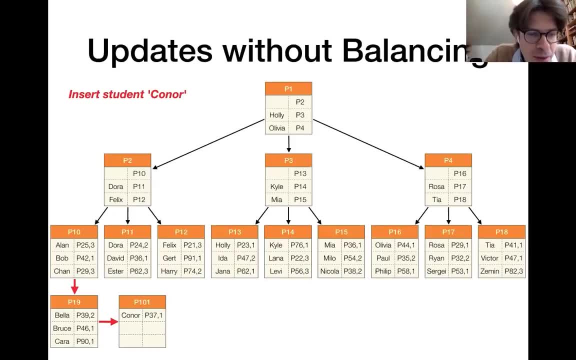 So we are creating again a new overflow page here, page 101.. And then the first overflow page has a pointer to the second overflow page. right and now, before we start deleting things, i want to point out that having those overflow pages might make retrieval inefficient, because if 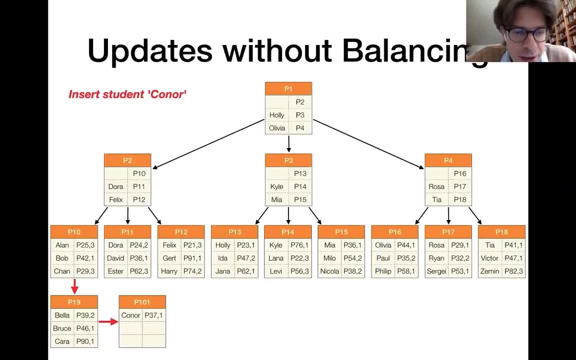 you're searching, for instance, for connor, then in order to get there, i would have to pass one, two, three, four, five pages, uh, while for most other entries i would only have to pass three pages in order to find them. so those overflow pages which make the tree imbalanced. 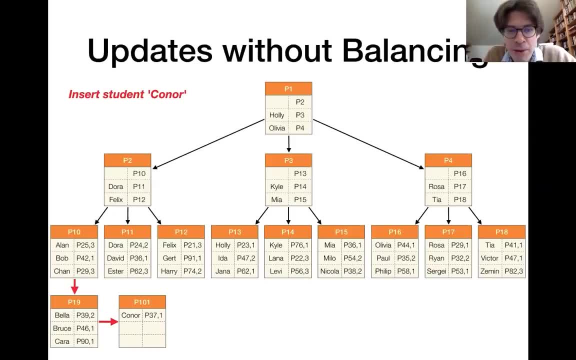 they are not good for retrieval performance. now let's also delete a few students. let's say, we are deleting rosa. um, let me quickly move the chat so i can see my slides. um, let me quickly move the chat so i can see my slides. um, we are deleting ryan, we are deleting sergey, and at this point you see another inefficiency. 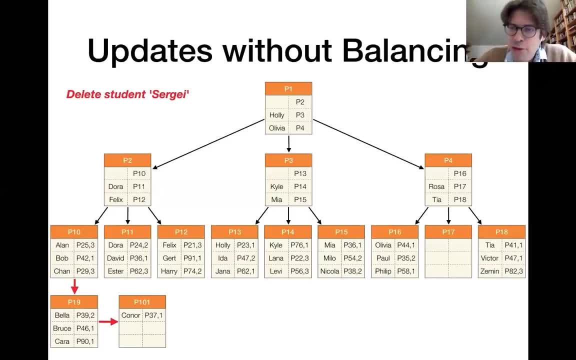 here because we don't rebalance the tree. if you look at page 17 that we have deleted the students, now it has become completely empty. so here we are using space. we are reserving space for that page 17, but we don't actually store any entries on it, so we are wasting space. 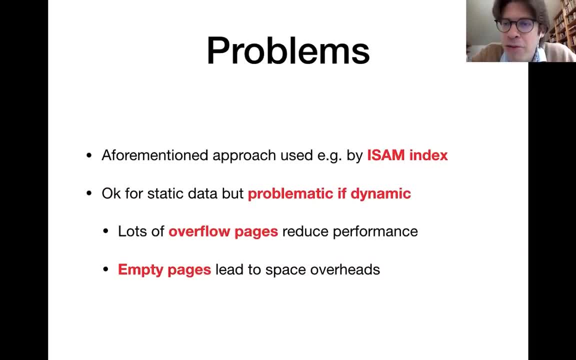 we are wasting space on it. so if we move these things, we are only losing space for the sample to be actually taken care of. so let's have a look at the problem now. those are the problems with those static index structures. it has been done. there have been index structures. 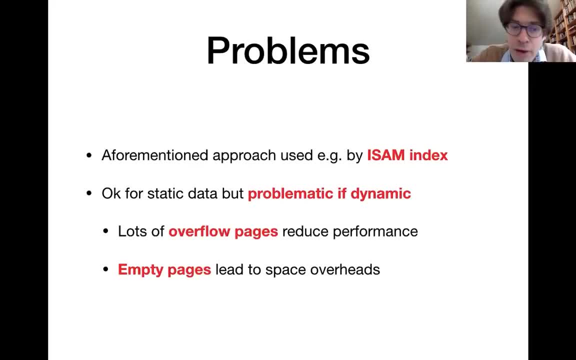 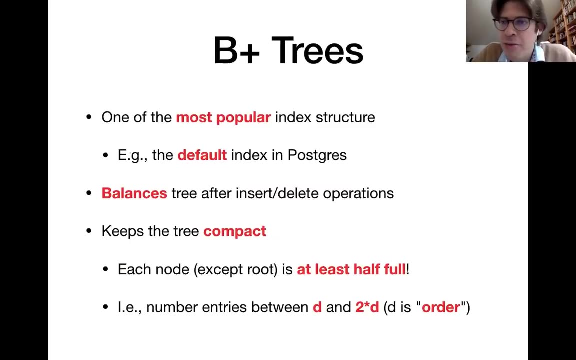 which do that, and, for instance, the isam index is an older one, and that is okay as long as your performance, and you might also have lots of empty pages, which means that you are wasting storage space. both are undesirable. that is why data structures such as the v plus tree, 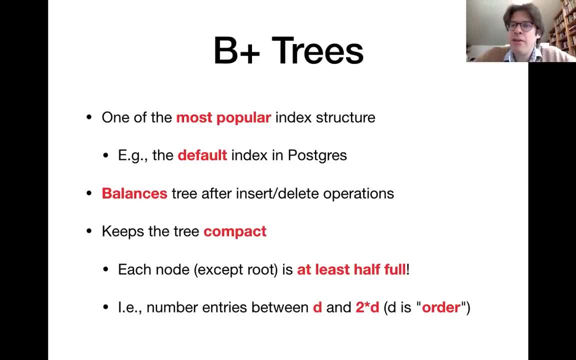 they're doing things a bit differently in order to cope with more dynamic workloads that keep updating your data. we have already seen that this is the default index structure in postgres. it is very popular and it balances the tree after insert or delete operations: the primary goal. 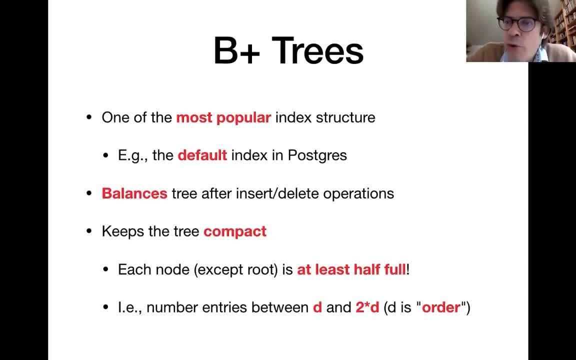 of b plus trees is always to keep this index tree somewhat compact, and that means you want to make sure that your nodes are at least half full. that was not the case for the previous index, where one of the pages became completely empty. a d plus tree would not allow that to happen, so 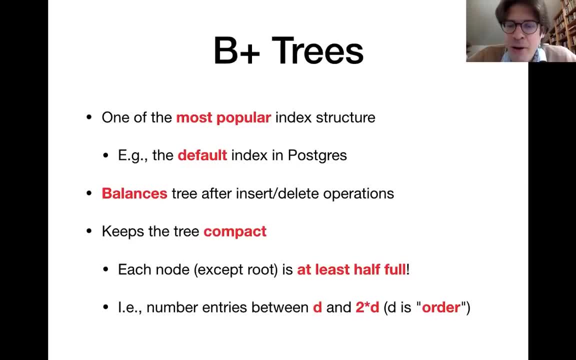 every node within the node in node a is usually half full, although that doesn't always change. we call also the number of um minimum entries per node the order of a tree, and it is often abbreviated with a little d in those textbooks. and so since we require nodes to be at least half full, 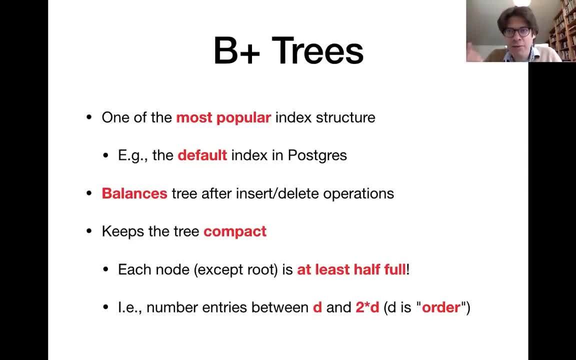 with the exception of the root node, by the way, because maybe you only store one single entry in your entire index. but uh, besides the root node, we require nodes to be half full, and that means entries that we have per node is between the order d, the minimum number of entries and two times d. 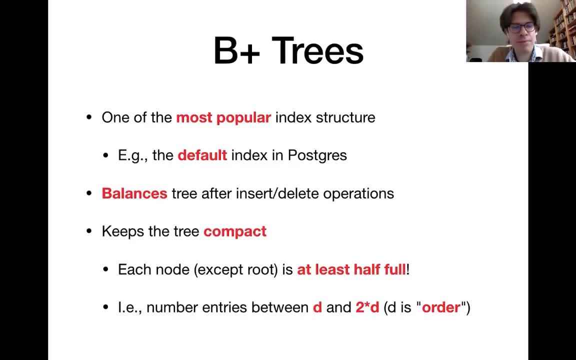 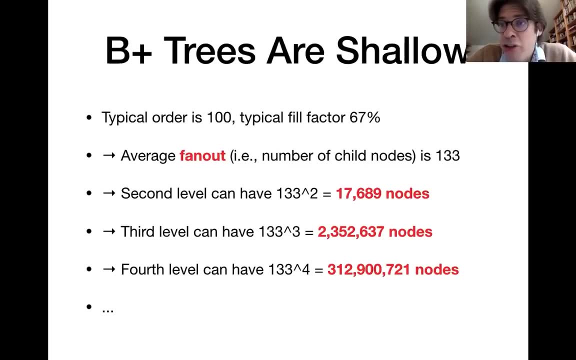 that is the maximum number of entries per page. now, in practice, um b plus trees are relatively shallow, even for large data sets. see a couple of deck of the envelope calculations in order to demonstrate that point. um a typical order is something like 100, so you would be able to fit between 100 and. 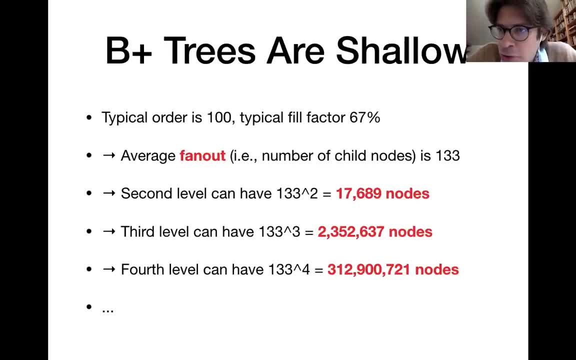 200 entries on each of those nodes. like, the number of entries per node is defined by the page size and by the size of the index entries. so typically the page size is a couple of a kilobytes, and then with typical entry sizes you end up with something. 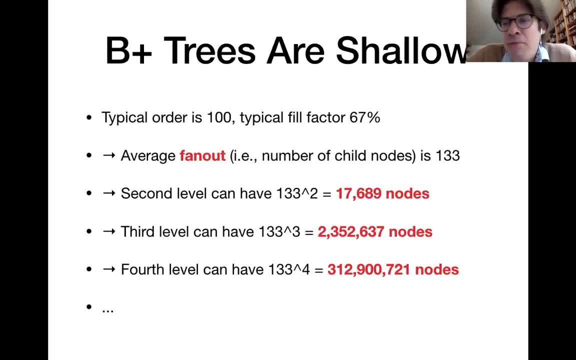 between 100 and 200 entries per node. now, in practice, um, you are a fill state somewhere in between the extremes. something like two thirds four is typical, and that means that the average fan out, meaning the number of child nodes for your index nodes, is about 133. so that means that the 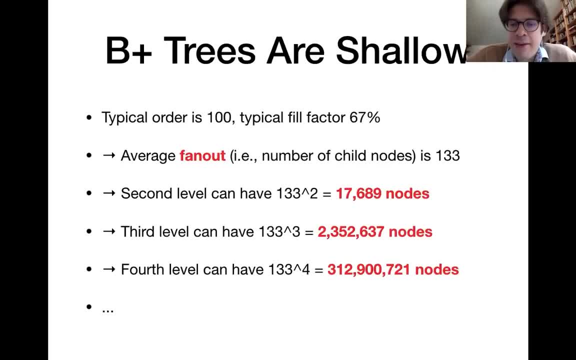 second level of your tree can already have something like nearly 20 000 nodes. the third level can have something over two minutes million nodes. then we have over 312 million nodes, and so on and so forth. so just for demonstrating that, even just with a handful of tree levels you can already index most, even the large data sets, 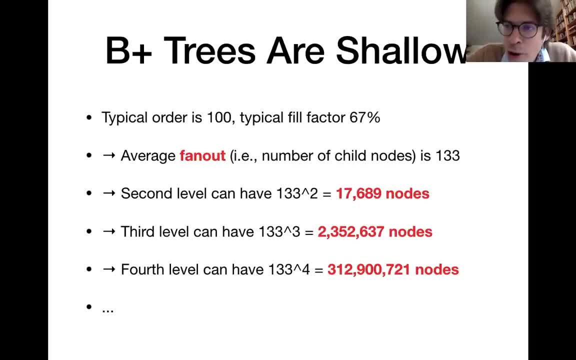 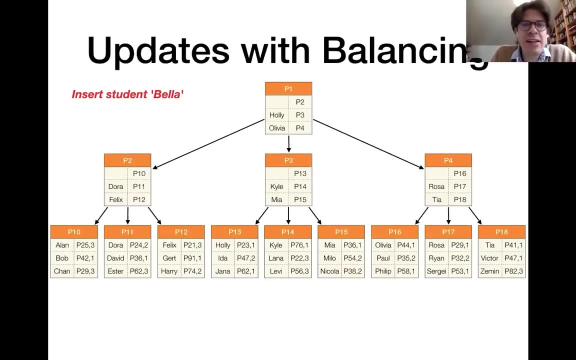 and that is one reason why those trees are so popular. um, it allows you to go to the data that you're looking for with only few node, with only few page accesses on the bay. let's see how those are going to be working with this, and then we can also check these. 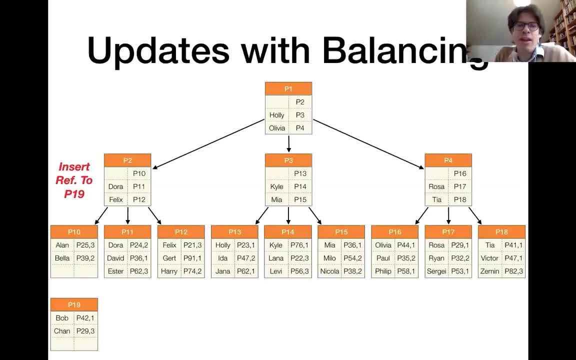 for instances. so, for instance, we have a hyphen here, so we can call it like that in case you are 这里, okay, or here to page number 19,. and then we would be done Easy. Here we are more ambitious and we actually want to insert a reference. 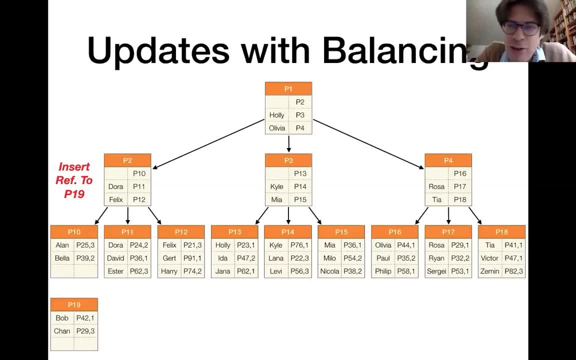 to page number 19 in the parent node to page number 10, which is the page number two. So I didn't want to insert the reference to page 19 here. If that works, then great, we are done and we have a balanced tree. 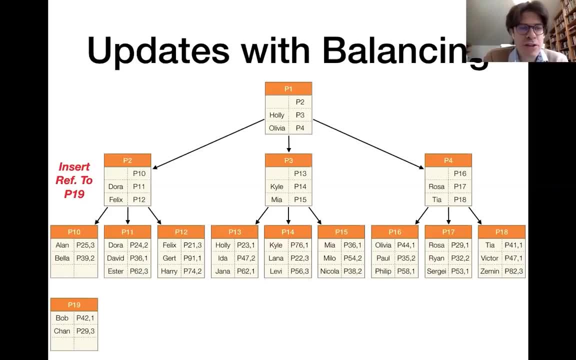 In this case, unfortunately, it doesn't work, because page two is also full. So we have to propagate the page, split up the tree and here we have to introduce one more page, which is page 20.. And so page two and page 20,. 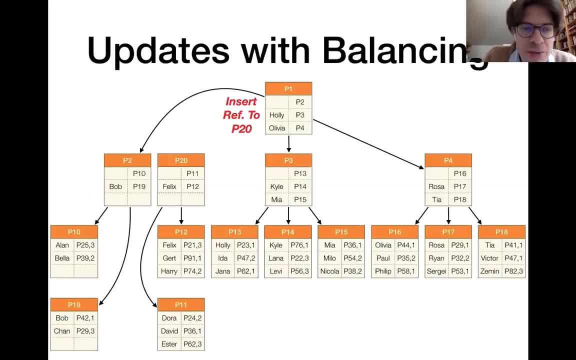 they now divide the entries among themselves that have been formally stored on page number two, together with the new reference to page 19.. So now we have another dangling page- page number 20, that no other page is referencing currently. So again we have to go to the next higher level in the tree. 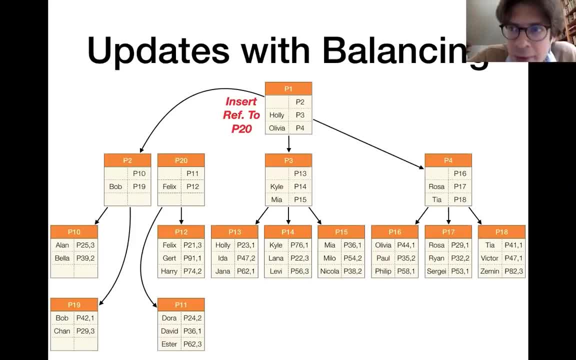 in order to insert a reference to page 20.. But again, the current root node, page number one, is full, So we want to insert the reference, but there's no space left, so we have to split the root node again. 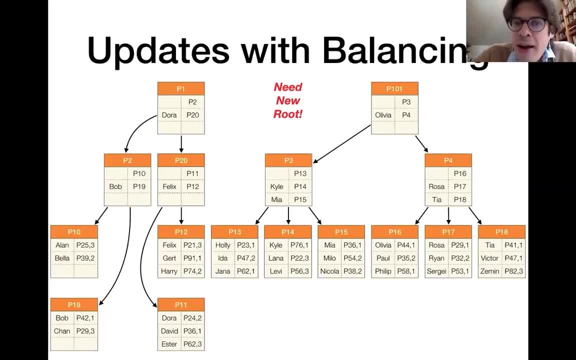 Now we have introduced one more node- page 20, and another a new reference to page 101.. And now our entire tree is actually split into two trees, which we don't want. So in order to connect to an actual tree, we need to introduce a new root node. 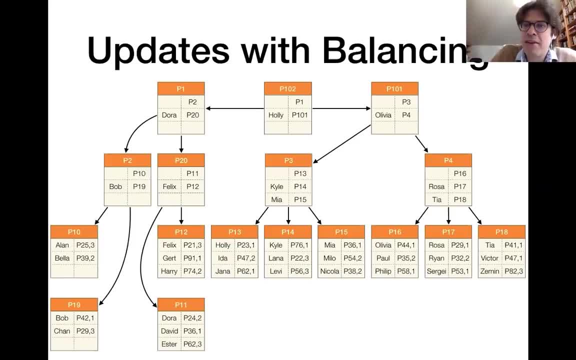 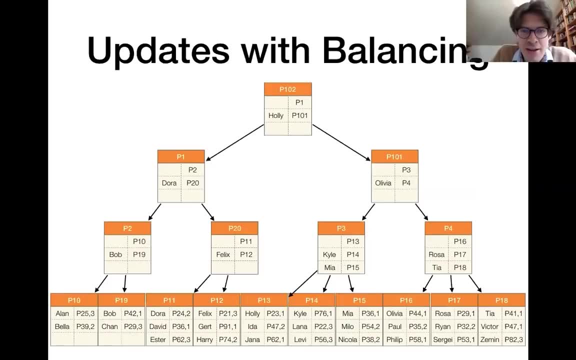 that references page one and page 101.. And we do that here with page 102.. Let me just rearrange the nodes a little bit to make it easier to recognize it as a tree, which is this. And now we ended up again. 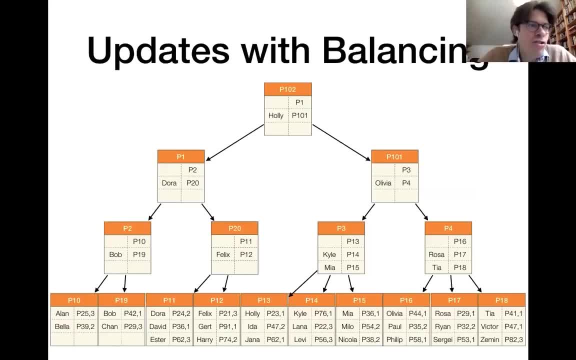 with a balanced search tree into which a student, Bella, has been inserted. As you see here as well, this tree has one, two, three, four levels, The original tree that we started with before inserting Bella. let me quickly go back to that one. 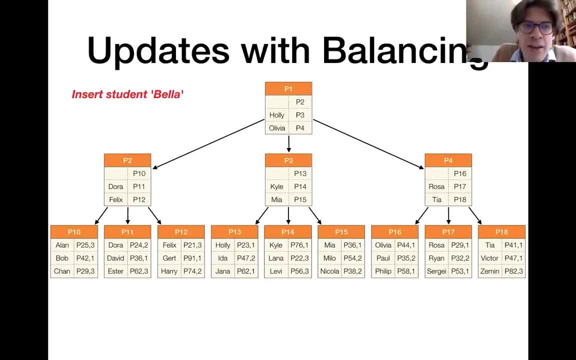 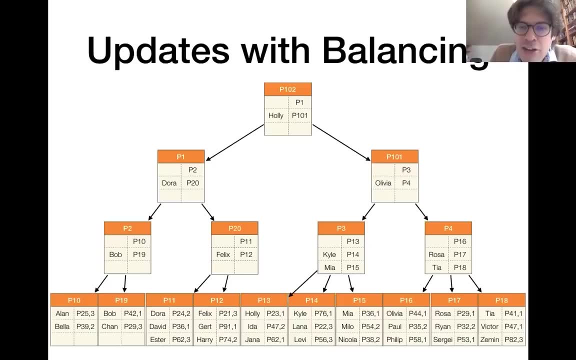 this one only had one, two, three levels. So because we inserted that new student, it actually caused several reorganization operations, And now we have a tree that has one more level, All right. So now let's see a deletion operation in order to see the inverse. 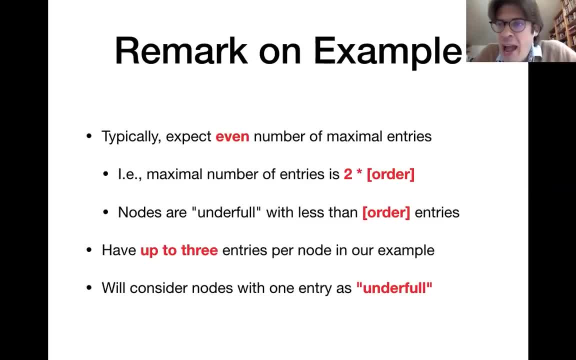 And before we do that, we should quickly, proactively discuss about one possible source of confusion. You might have noticed that in my example, each page has up to three entries. I'm doing this because this is what just fits best on my slides. 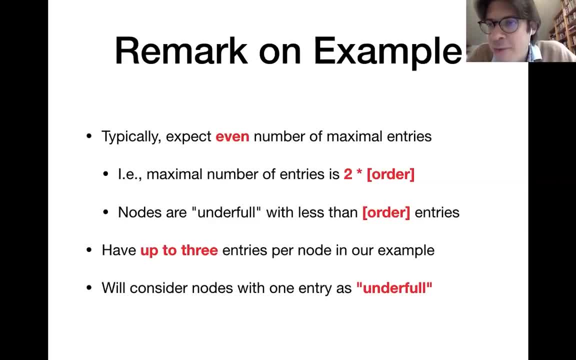 On the other side. we have seen that, according to the formulas we saw before, the number of entries per node is always between d, between the order d, and 2 times d, And that means that you would expect an even number of entries per node. 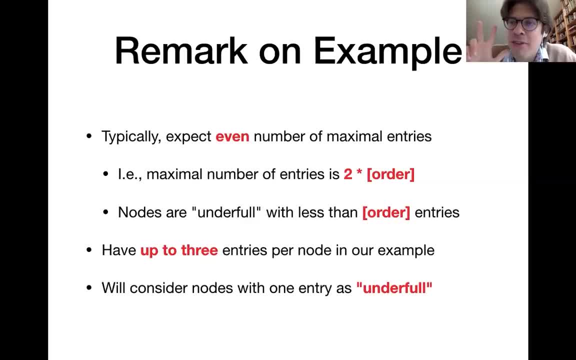 Now, in this example I'm not doing this. I'm working with at most three entries per node, but that is just motivated by the dimensions of the slides. Typically, we would say that a node is considered under full, below the field threshold that is required. 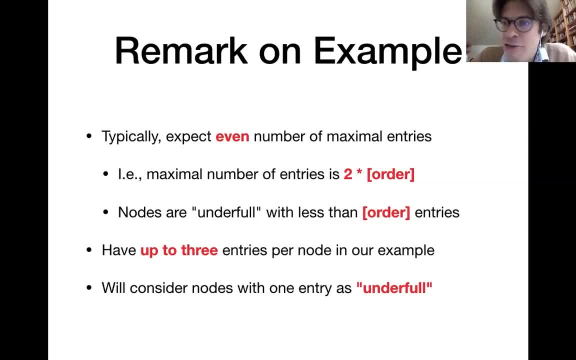 If it has less than d order entries, we would say that a node is considered under full. Here we have up to three entries per page, So half of that would be 1.5, which is not an integer. So for the example in the following: 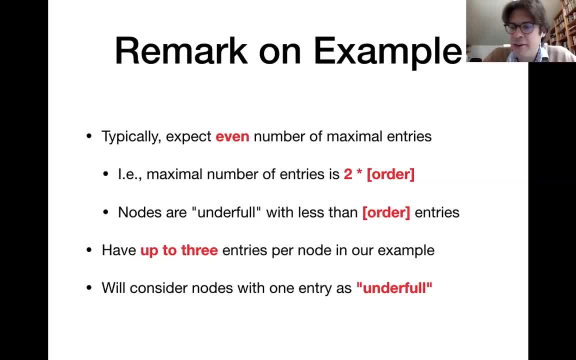 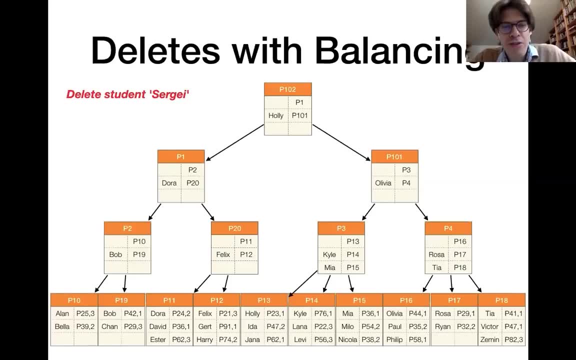 we will say that a node is under full if it has less than two entries on it. All right, so let's actually see what happens if we delete a couple of students here. So let's first of all delete Sergei, And now let's delete Ryan. 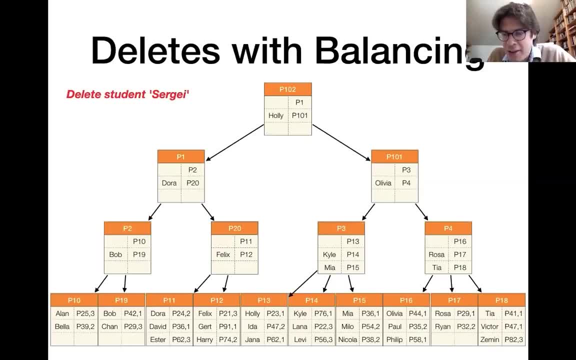 And so here we have deleted Sergei. and now next one, we are deleting Ryan in page 17.. And, as you see, page 17,. now Ryan vanishes, And at this point we have the problem that page 17 has become under full. 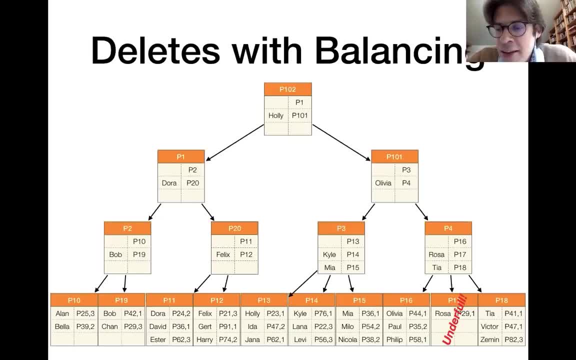 because we require at least two entries per node and here we do not have it. have them. so what we can do in this case here is if we look at the siblings of p17, particular p18, those nodes, they can spare some entries. they are comfortably above the minimum threshold of 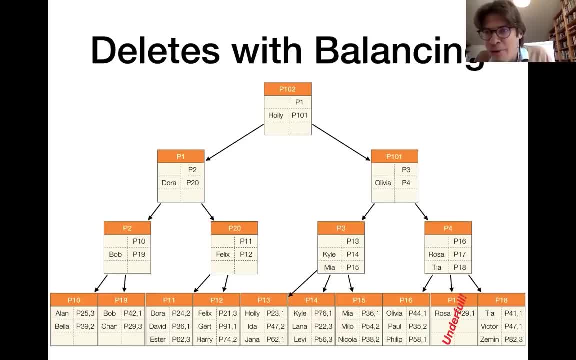 entries per node, so we can essentially shift a couple of entries from page 18 to page 17 over here. we also need to change corresponding references on page 4, and now we have come back to a tree that is balanced and they each node is at least half full. yeah, that was the 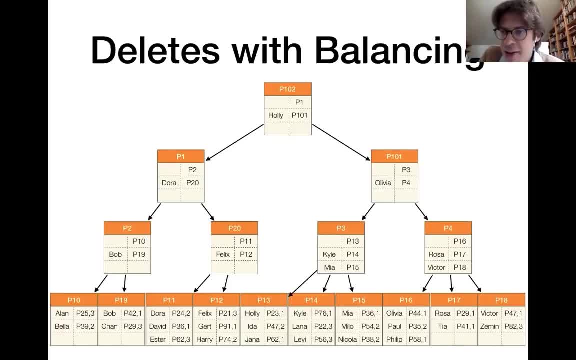 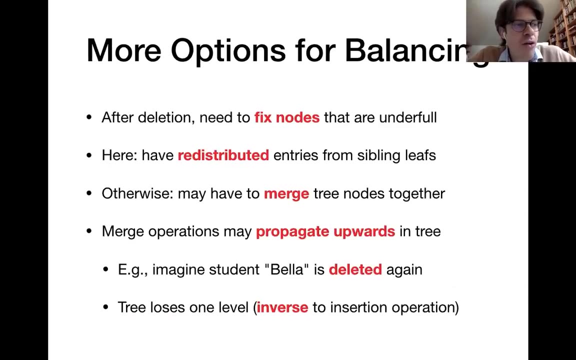 bad state with the under full note. and here we are gonna getting back to the good state by shifting entries from page 18 to page 17. all right, and now I'm gonna show you one more way to deal with imbalances caused by deletions. so 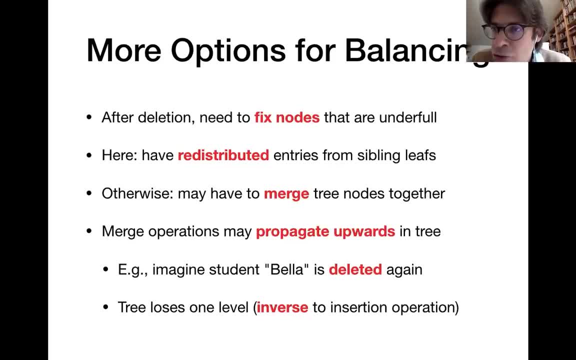 in the previous example we have essentially redistributed entries from the sibling to the node that was under full. another operation that we can do, which tends to be a bit more expensive, that is that the merge nodes in the tree together again and then, once we merge two nodes, then it means that the parent node will have one reference less. 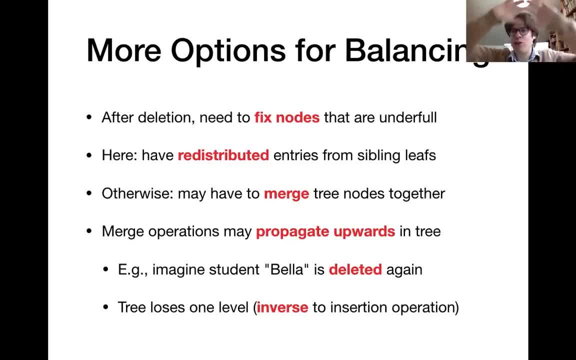 so potentially the parent node also becomes under full and has to be merged again. so similar to how those H splits can propagate up the tree, which we have seen for insertions- those are node mergers- can also propagate up the tree in case of deletions. so for instance here let's see, let's say 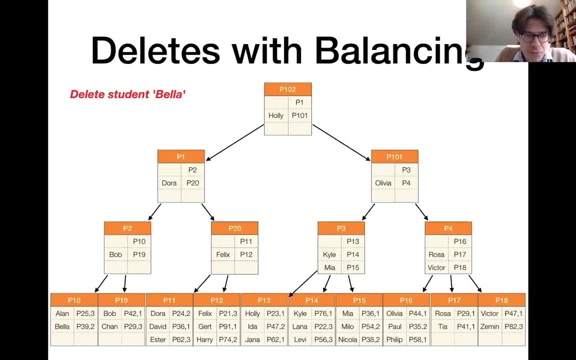 that we are deleting student Bella again, and here student Bella appears on page 10, on the left lower corner here. so now I'm deleting that from page number 10, and at this point page 10 has become under full. now the problem is, I cannot really redistribute entries from page 19, because then 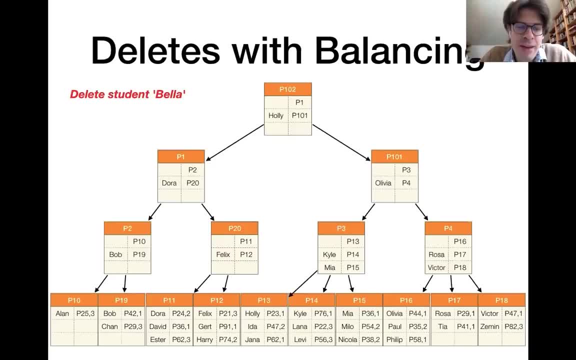 page 19 would become under full. I could think more about redistributing things, but at some point it it becomes too expensive. so instead of that I might rather want to merge the nodes. so if I do this, then so page number 10 has become under full. so if I merge together page 10 and page 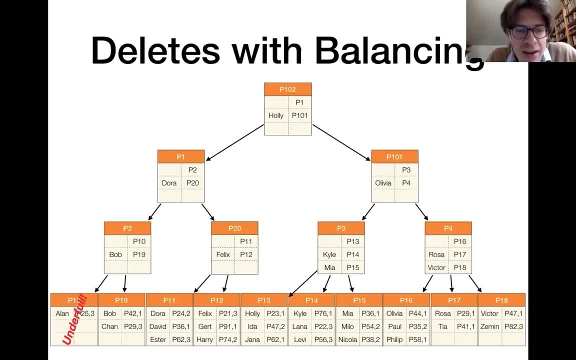 19. it means that page 2 has one entry less, so we might also want to merge it with page 20, but then page one has one entry less than before, so we might merge it with page 101 and so on, and then the root node has one entry less, so it becomes. 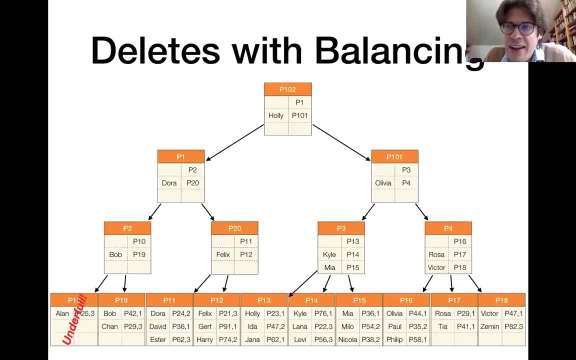 unnecessary, so to speak. so I leave it to you to trace the example back in more detail after the lecture. but what we are doing here is pretty much exactly the inverse of what we have been doing before. before we have been inserting student Bella. this is why we had to add one level to our tree now. 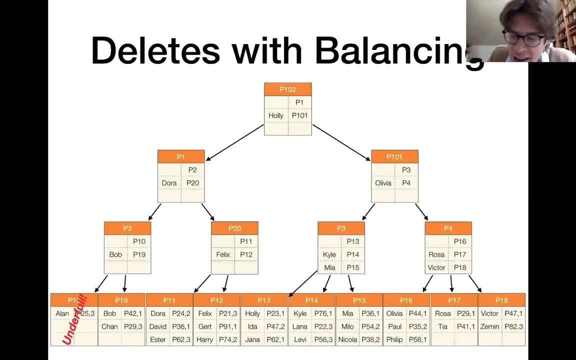 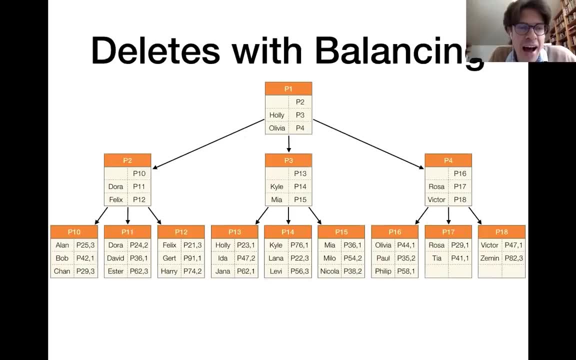 we are doing the inverse. we are merging together nodes again and in the end you will end up with a tree that has one level less. again it has three levels after deleting Bella. before it had four levels. here again, each of the nodes is at least half full and the tree is balanced. that's always the state that we want. 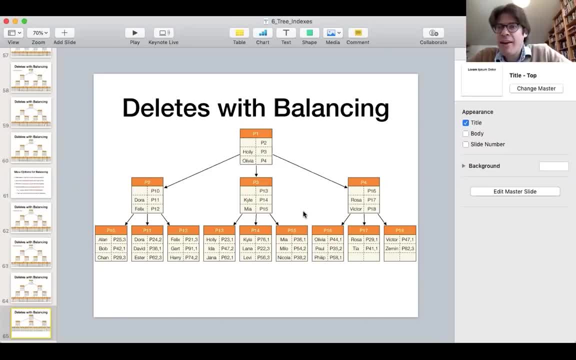 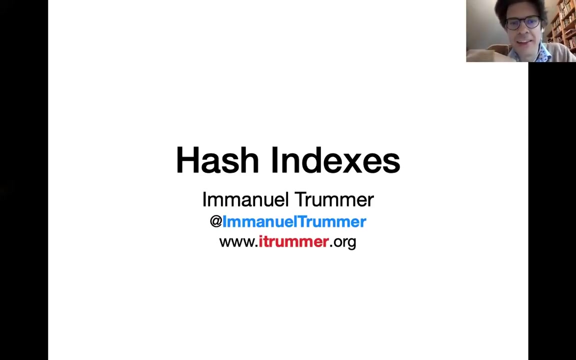 to come back to good, so great questions. that was a tree index data structures. next time we will start with an alternative, which is hash based indexing as structures that are based on a hash function. I wish you a nice day and I see you on Friday. all right, let's get started. so hello. 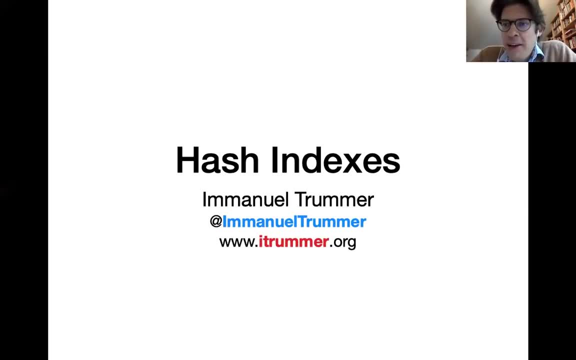 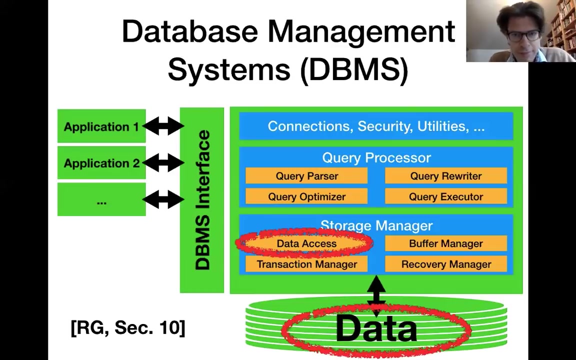 everyone, and today we are gonna probably finish our section on indexes. the last time we have been talking about a tree index structures essentially correspond to a search tree, and this time we're gonna talk about a different type of indexes, which is based on hash functions. that's my slide here, all right, so here we have again this. 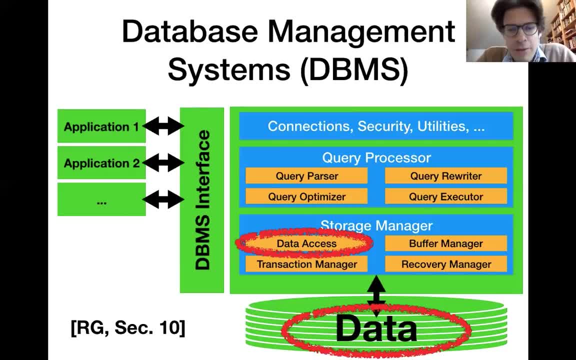 architecture of database management systems. so you're currently still discussing about how the data is generated and how it is used in the database management system. so we are currently still discussing about how the data is laid out in order to make it efficient to access, and we're also talking about the data access. 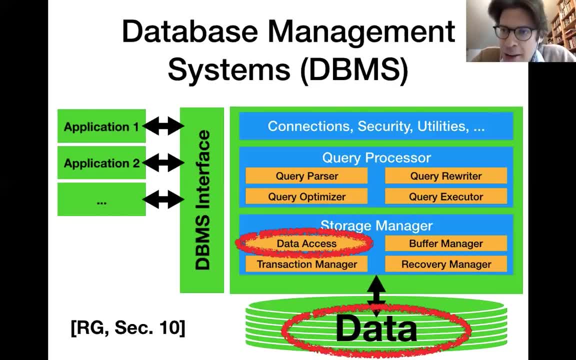 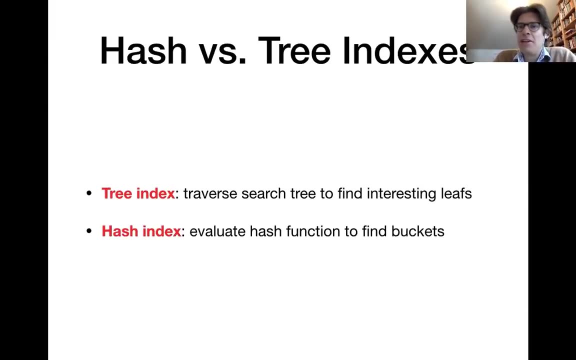 component in the storage manager for hash indexes, the relevant chapter in the Ramakrishnan Agarika book, that is the number 10, and so far we have been discussing about those tree indexes where you essentially traverse the tree from the root node to one of the leaf nodes in order to find 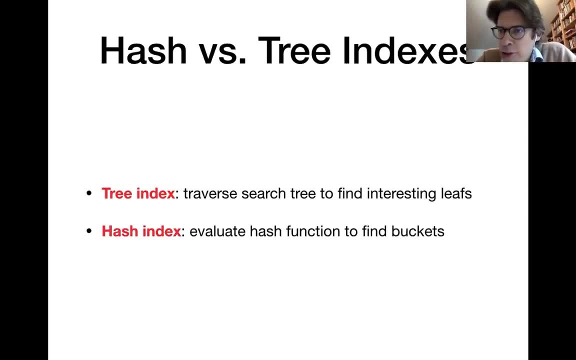 those tree extracts to the application, as in this case, bamboo tend to be used to track and wenn there is no restaurant drive, you can always connect to offering разб. you please log in and let've take a look on the one piece of this community. 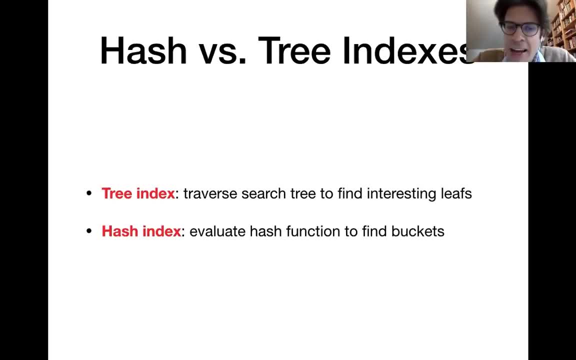 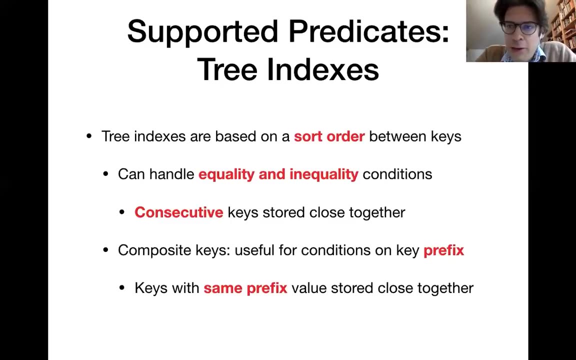 hotel. let's begin the video, and this is where we gonna cookент Now. let's first of all discuss a little bit about the types of predicates that those different indexes can support. Now, tree indexes are fundamentally based on a comparison between keys. So if you think, for instance, about the leaf nodes of an index tree, then the entries in the 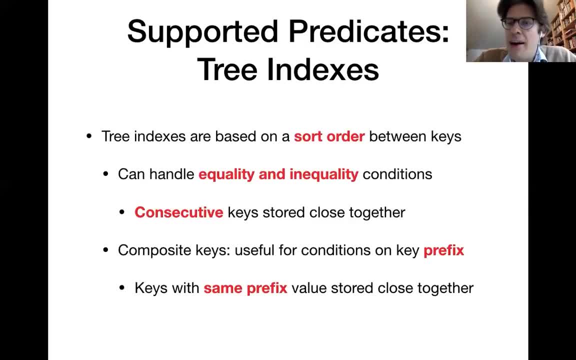 leaf nodes are sorted by the key. That means that keys like entries for the same key are stored close together. It also means that entries with similar keys are stored close together, and because of that I can exploit those tree indexes quite conveniently in order to treat. 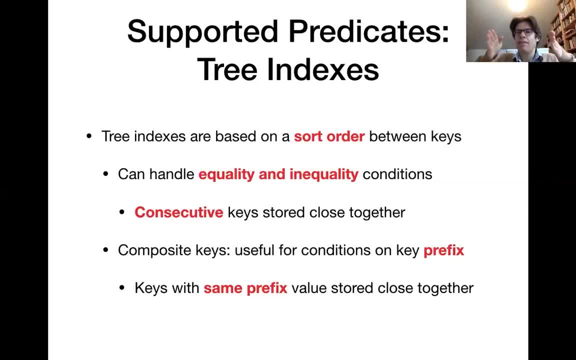 inequality conditions. Just need to scan some range in the leaf nodes and there I will find all the key, So I can see that the tree indexes are sorted by the key and the leaf nodes are sorted by the key. That means that the tree indexes are sorted by the key, So I can exploit those three. 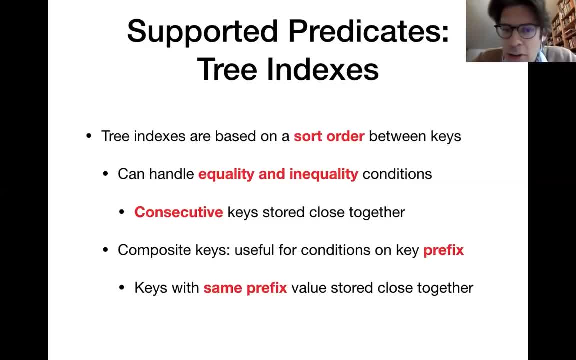 those entries with similar keys stored together. Also, we have seen that we can use tree indexes with composite keys and if I sort keys by composite, if the key is a composite of multiple columns, then it means that those entries which have the same or similar values in a prefix of the key columns they are. 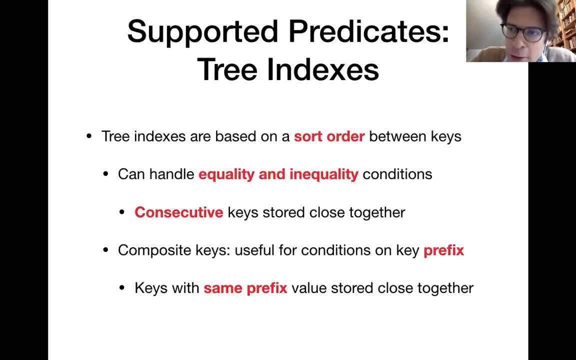 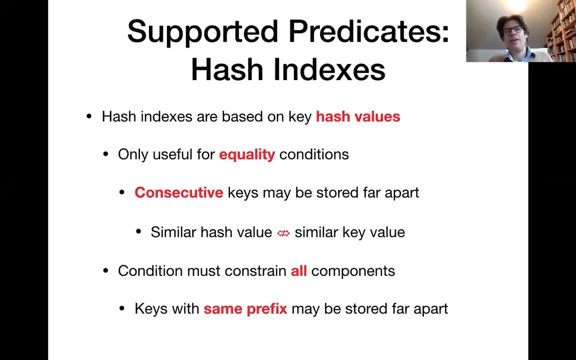 still stored close together, And that is why I can use those tree indexes also in order to treat predicates that refer to a prefix of the composite key columns. Now let's see how that works for hash indexes. Now, hash indexes are based on hash values. That makes the 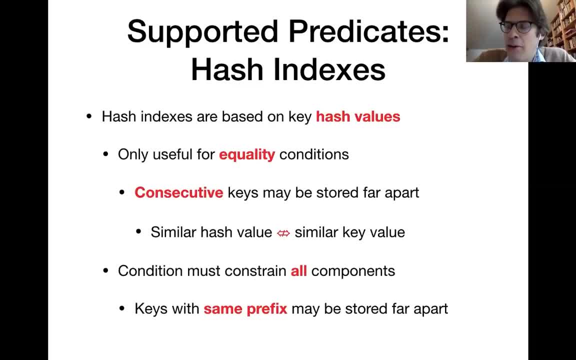 hash values useful for equality conditions, because if two entries have the same key, then the hash value is also exactly the same, and that means they will be stored in the same bucket. Now, on the other side, if two keys are similar, close together, it does definitely not mean that their hash values are close. 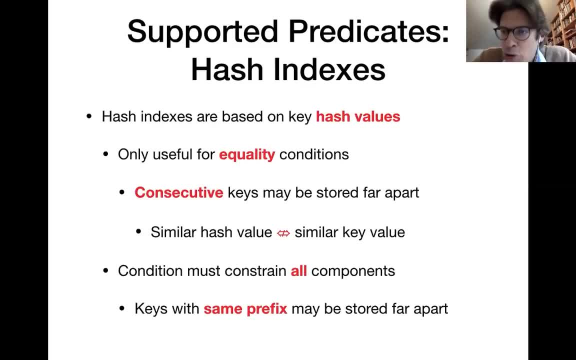 together in any way, And that means that they will probably be stored in different hash buckets even if they are not close together, Even if their key values are relatively close. And since similar keys are not stored close together, it makes it inefficient to try to use hash indexes. 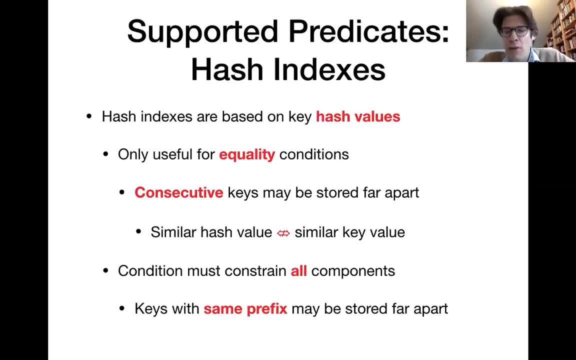 for inequality predicates. Also, if you have a composite keys, then if you have the same value in a key prefix, when comparing two entries it does not mean that they will be stored in the same hash bucket. Most likely they will be stored in different hash buckets. 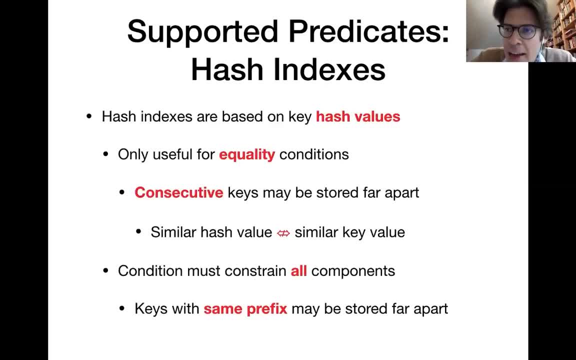 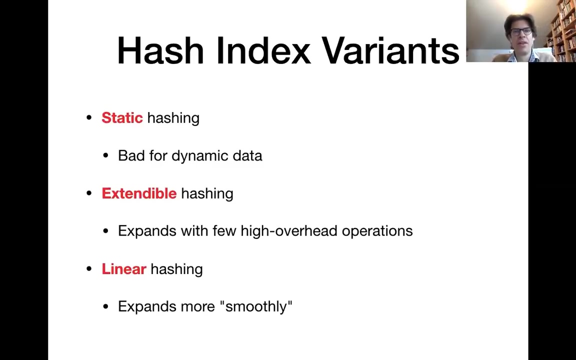 And this is why you typically want to use hash indexes only if you have conditions on all the columns of the composite key. So, in a way, hash indexes are a little bit more restrictive in terms of the predicates that you can use them for when comparing to tree indexes. Now in 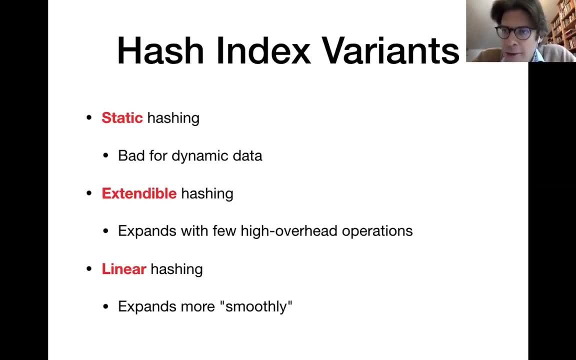 the following: we're going to see a couple of different hash indexes. We are going to see three different variants. This is a high level overview. in the following We're going to go into detail. We are going to start by looking at something. 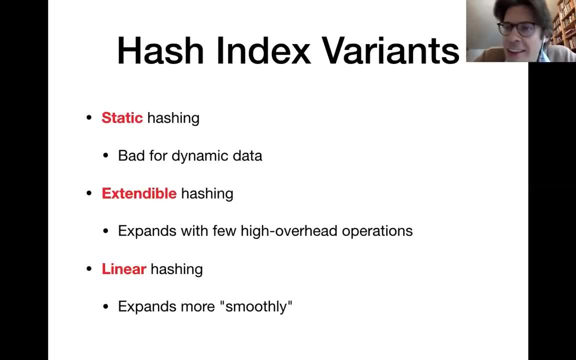 called static hashing And, as the name already indicates, it's not a good idea if you have very dynamic data with lots of insertions and deletions. In those cases, you probably want to use something like extendable hashing. Now this one. 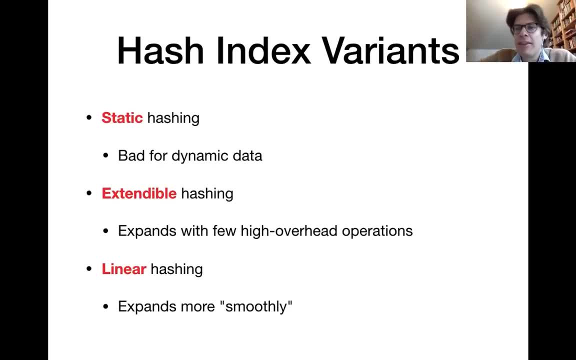 has one drawback, which is that if you keep inserting data, then every once in a while you need to perform one expensive operation in order to update the index, And we will see later precisely what that operation is. Then we have something called linear. 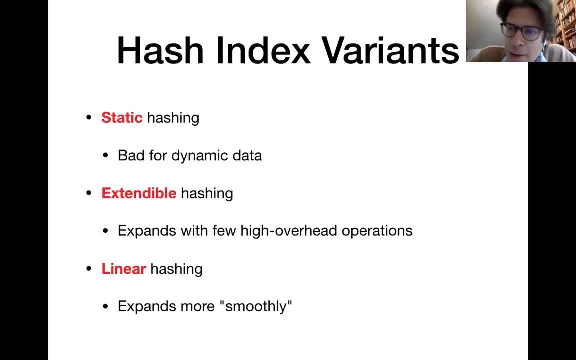 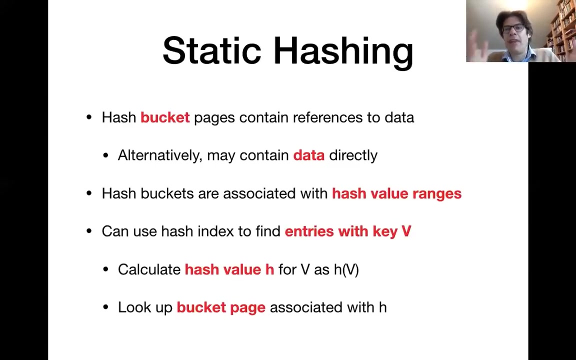 hashing, And this one has the advantage over extendable hashing that it extends the index very smoothly without costly operations. It has a couple of other drawbacks, But we're going to discuss them in detail in the following. So those are the hash indexing variants that we will look at in the following. Static hashing is perhaps. 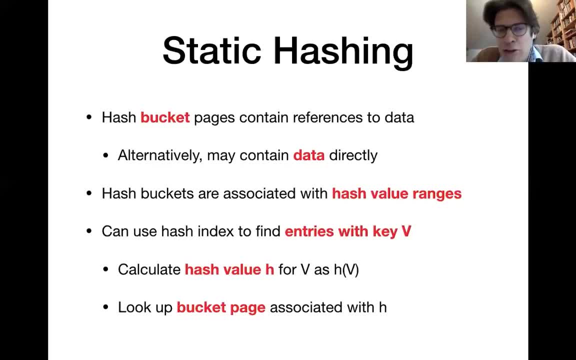 the simplest one among those variants. Essentially, you have pages associated with hash buckets and they store the references to the data. Or, what is also possible, like in the case of tree indexes, you might even store the data just directly. Now, the hash bucket pages. they are associated with specific value ranges. So the way you 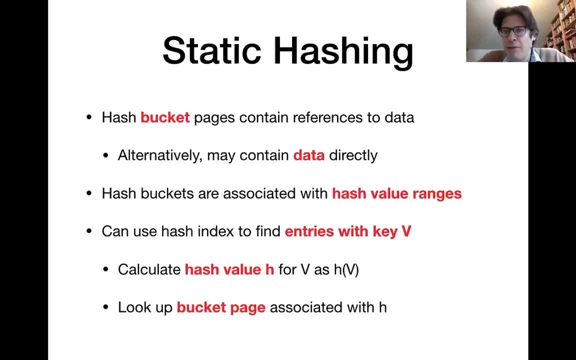 use. one of those indexes when looking for entries with a specific key value is that you first of all calculate the hash value for that key you're looking for And then you look up the bucket page which is associated with the hash value. This is a little illustration. 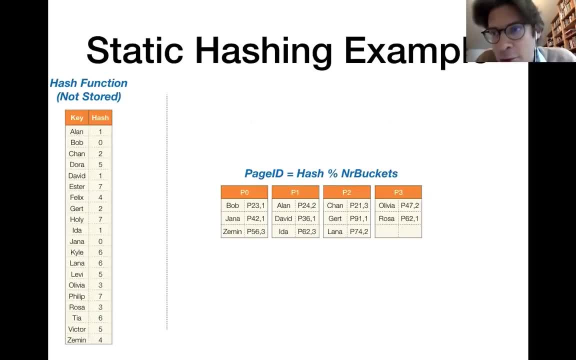 here. You can see, here you are storing entries about students And on the left hand side of the screen you have the hash function which associates specific student names with a hash value. just to make sure This hash function is not explicitly stored as a table, You only 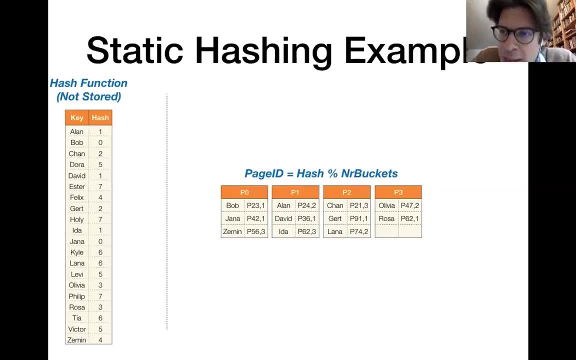 calculate it based on the bits that are directly available in the key. I'm just putting the hash functions here for convenience, But it is not actually stored anywhere in your database. Next slide, please. what is stored in your database? that are those pages that you see in the middle. 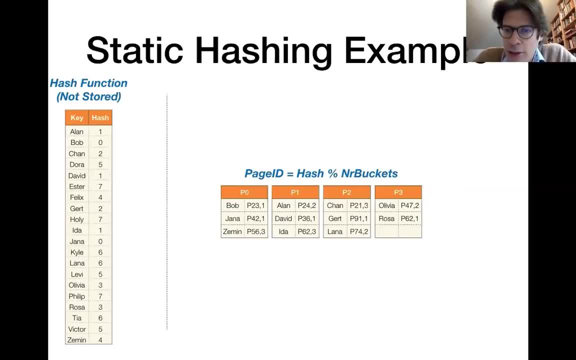 of the screen here, page 0 to page 3, and here we use the simple system that the page ID corresponds to the hash value modulo- that's what the percentage sign symbolizes, modulo the number of buckets. so for instance, if you want to store student Ellen, you look up in the hash function, okay, and then would have a 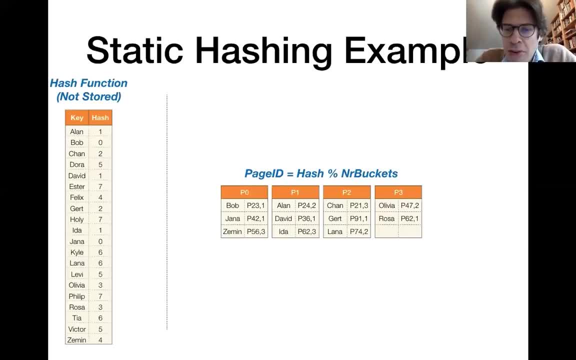 hash value of 1 and 1 modulo the number of buckets, which is 4 here, that would still be 1. so we will store Allen in page number 1, and this is indeed there you can find him. or Bob, for instance, has hash value of 0. so here we. 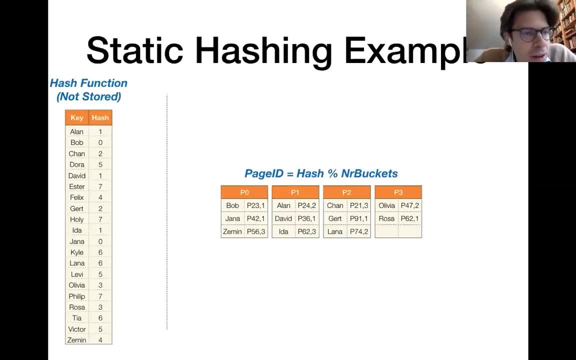 store it on at page number 0, that's maybe. have a look at one more. Dora has a hash value of value 5, and 5 modulo number of buckets, which is 4, is 1. this is why we would store her on page number 1, but we actually haven't stored her anyway. so 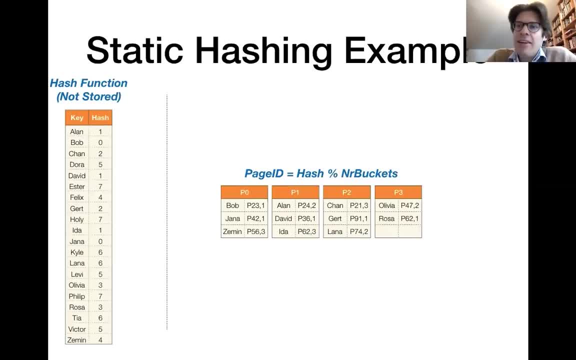 the hash function here. it gives you the hash values for all the students that we will consider in the following examples. here, in this example, we have only inserted a subset of students, so let's maybe see one more, okay, for instance, salmon. so this one has a hash value of 4 and 4 modulo 4 is a 0 again. this is why. 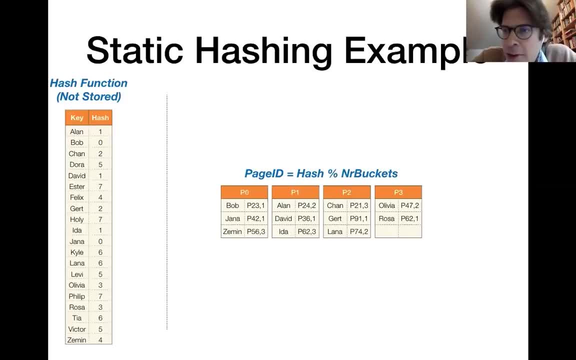 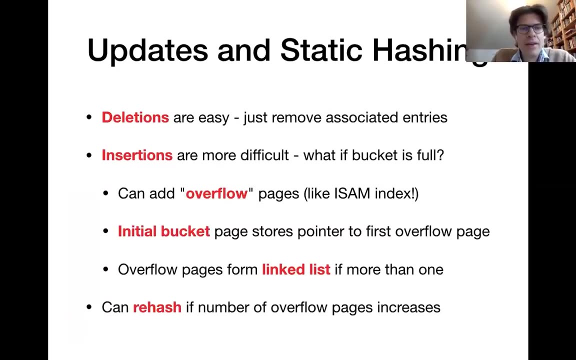 we store him on page 0, as you see here. so you, that is pretty intuitive- you calculate a hash value and then you look up the associated bucket page. there you find your entry, if it exists in the index at all. now let's see how those indexes change if we change the data, because the 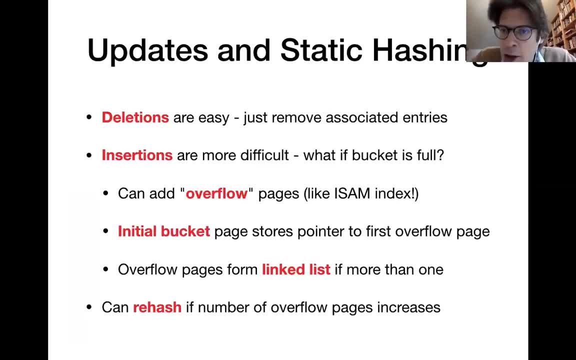 index always has to refer to the actual data. so if the data changes, then you must also change the index. now deletions are relatively easier. you just remove the associated entries from the associated hidges. that always works, and I think there might be a question and earth. 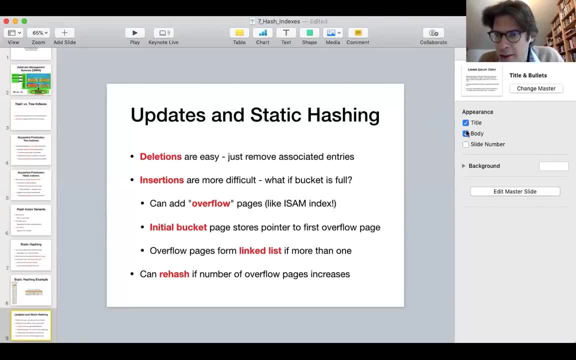 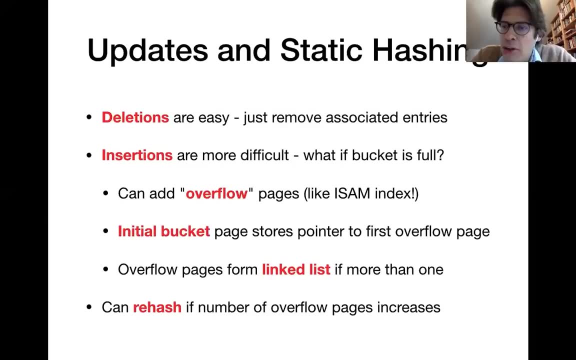 what our keys with the same prefix. so that question refers to the composite of keys. I imagine we have discussed about an example last time, for instance, where we have tools here with code prompted opt, and when we have done this you can see they are basically the same as at all on browser song. so both of us- you may not use code, even though we didn't understand each other. negative. then next step, when you just checking 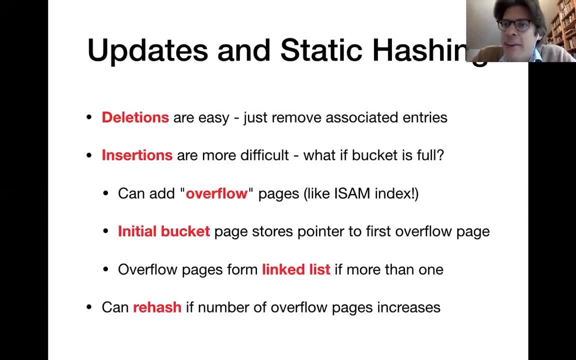 it's like pretty obvious things that adding in one index, one composite index that allows you to efficiently retrieve customers in specific zip codes that have bought one specific product. so you have essentially conditions on two columns and your index. I can use both columns as a search key. but if you have one of those composite search keys, then 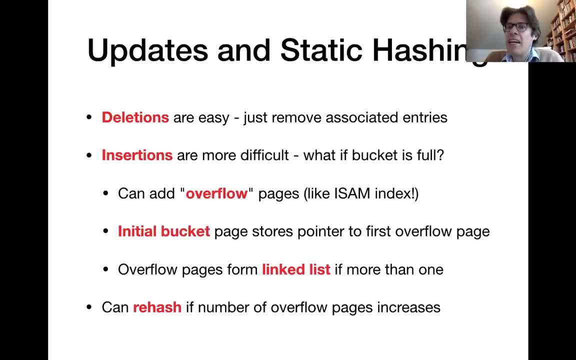 with tree indexes you have to choose an order between the different components of the composite index, and if you want to use the tree index, you can only do that if your predicates refer to a prefix of the composite key columns. so, for instance, if you have indexed first by zip code and second by a product, then 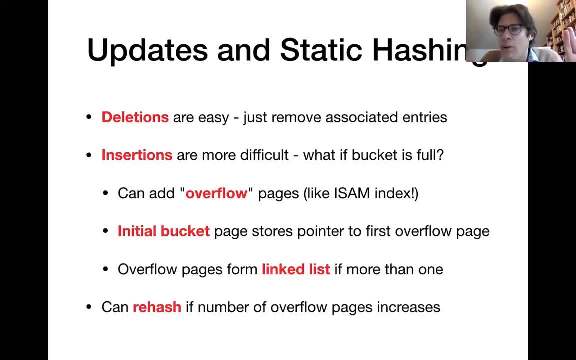 you can use that index in order to answer an equality on the zip code, but you cannot use that index to answer an equality on the product alone. you can only use it for predicates that restrict prefixes of the composite key. all right, sure, okay, and back to the hash indexes. 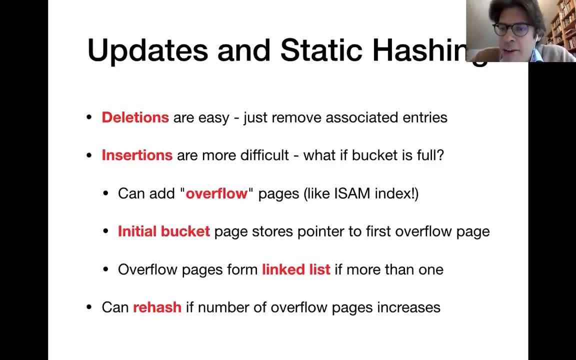 so we have discussed that. deletions are relatively easy to do, because I just removed the associated entry. insertions are a little bit more difficult because maybe that's page of which you would insert an entry is already full, so we have something which we call a page overflow. now, in those 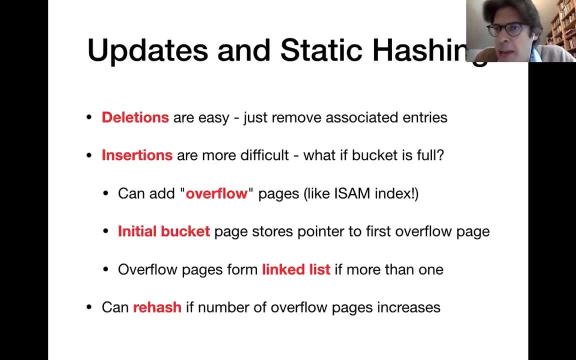 cases you somehow need to add additional pages to the index, clearly, and you can do this using so called overflow pages, which we have already seen in the case case of tree indexes. So this is a very similar principle. Now, so the initial bucket page essentially stores a pointer to the first overflow page on which you have stored entries. 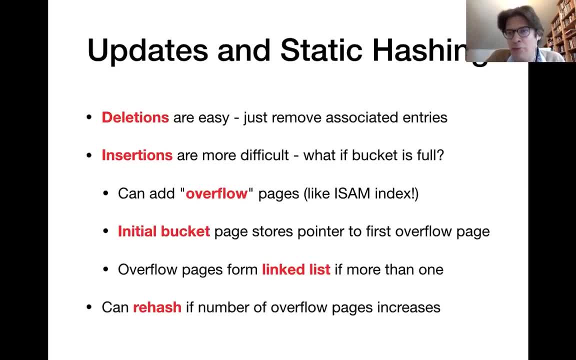 after insertion, And if you keep inserting entries, you might even need multiple overflow pages. So in that case the first overflow page would store a pointer to the second overflow page, the second overflow page stores a pointer to the third one, and so on. So you will get. 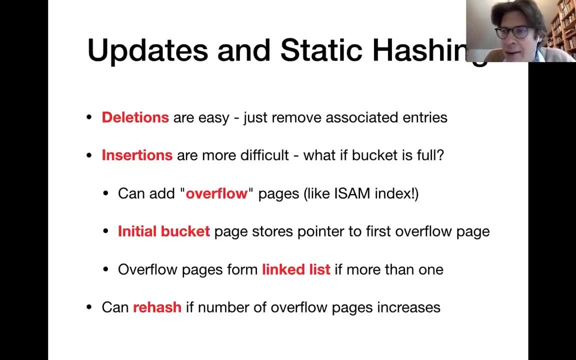 a linked list of overflow pages. in the end, At some point, that becomes inconvenient with so many overflow pages. So what you can do at this point is that you just essentially recreate the entire index from scratch. You rehash every entry that you have in your index. 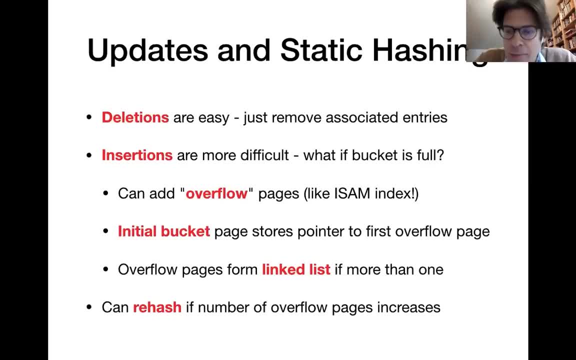 and then you can avoid overflow pages again, But that, of course, is an expensive thing of operation, and while you're reorganizing your index, your database may not be able to accept the new input, which is very inconvenient. All right, And here is one question very 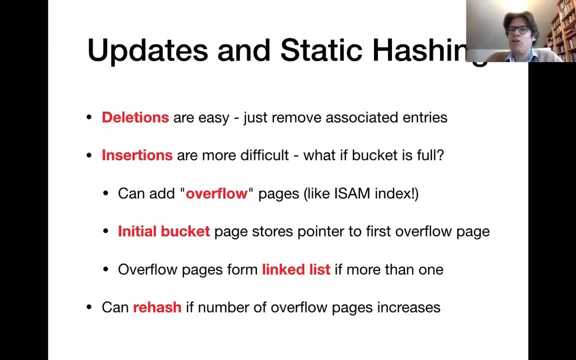 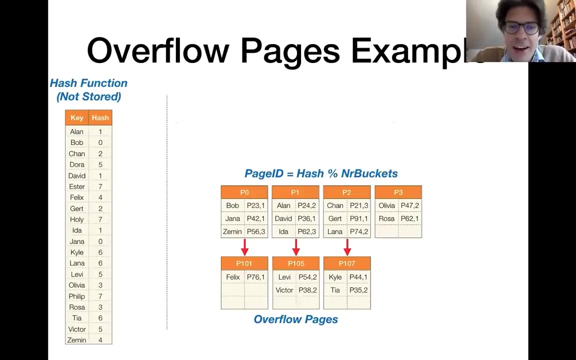 strictly speaking, The hash bucket, that is essentially some range of hash values, and then there is a page which is associated with that range of hash values. So they are linked very strictly speaking. there is a subtle difference. All right Now, this is an illustration. 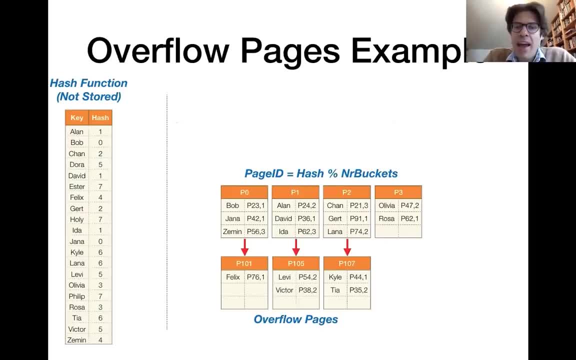 of those overflow pages Here. you see, we have expanded the index that we have seen in the last example. We have inserted more entries and obviously we didn't have enough space anymore for those entries. This is why we needed to add overflow pages. And you see, 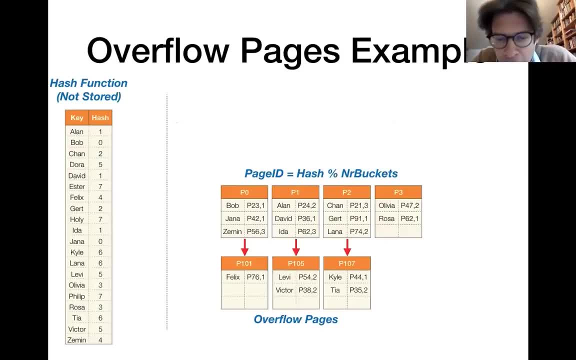 those overflow pages: P101,, P101,, P102,, P103,, P104,, P105,, P106,, P107,, P108,, P109,, P109, P1011,, which is P101,, P105, and P107. on the bottom of the screen, Those red arrows indicate 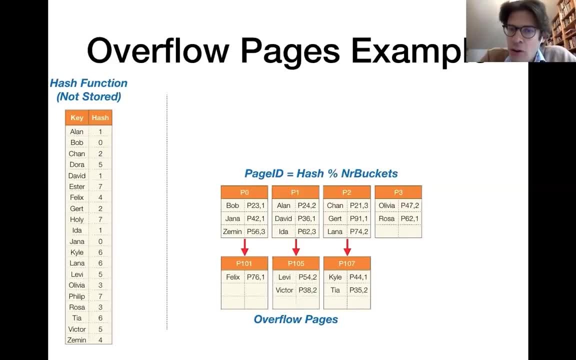 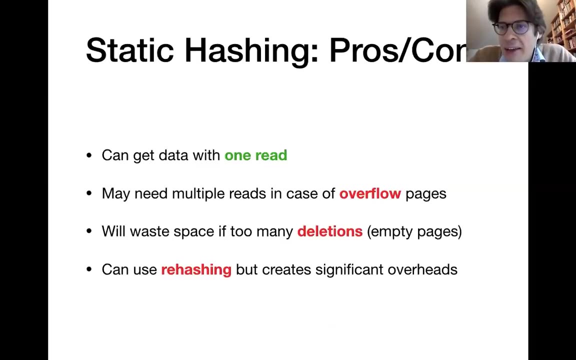 pointers that are actually stored on those original pages and they link to the first overflow page. If you would have multiple overflow pages then they would form a linked list for the same hash bucket. So if you analyze the pros and cons of those hash indexes, then 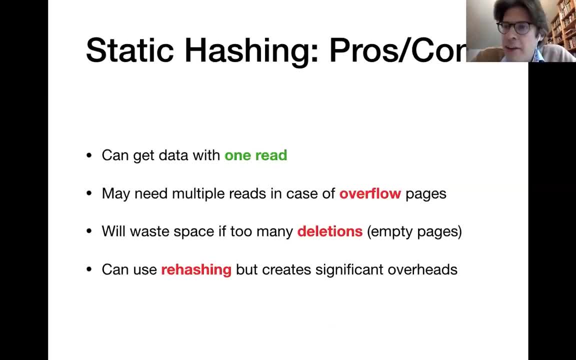 clearly what is going on. The first thing that is good is that you can data with one single page read, at least as long as you don't have overflow pages. If you remember, for the tree indexes, in order to find the entries that we were looking for, we typically had to look at multiple pages. 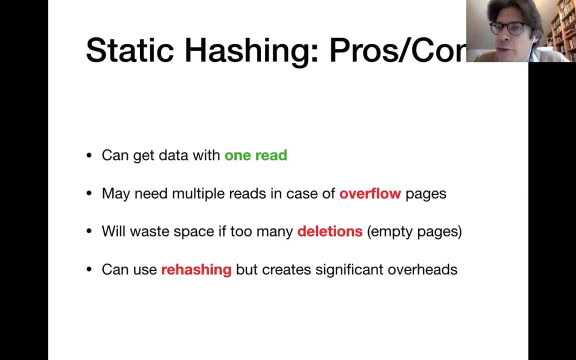 starting from the root node, then one node in each of those tree levels, So in a way those hash indexes. if you calculate the hash function, you know which page to look at, so that can be very efficient. On the other side, of course, with static caching, if you have overflow pages, then 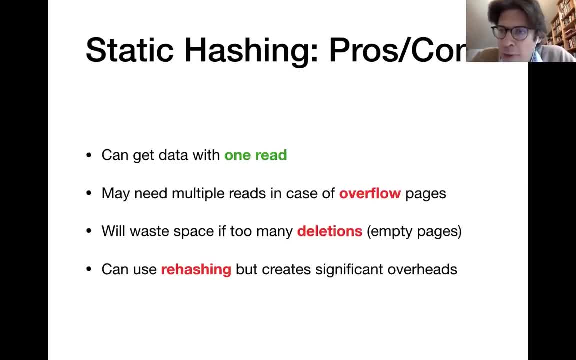 you might have to look on multiple overflow pages to find the entries that you're looking for or in order to conclude that the entry you're looking for is actually not present in the index. In any case, you would have to look at multiple pages, and that is bad. 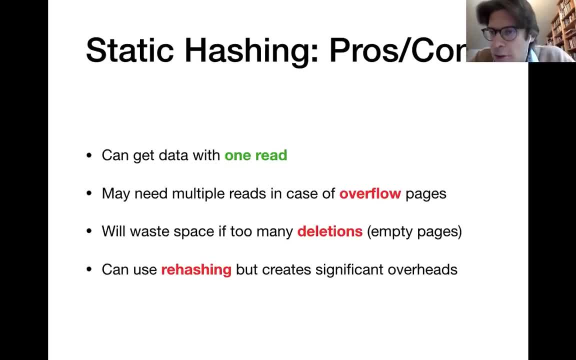 for performance. You also have said that deletions are easy because I can just take out the entries, But of course it means that at some point I might have to look at a number of pages, and there are lots of empty pages. That was already a problem that we quickly discussed in the 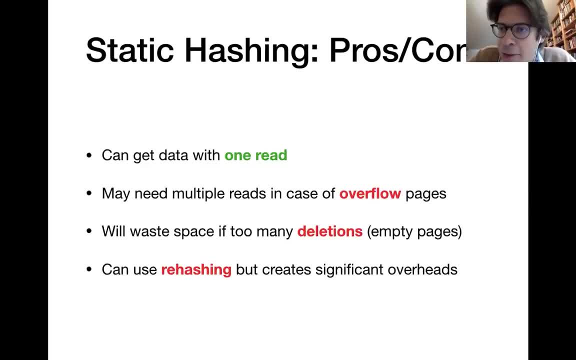 context of the static tree indexes that we have seen. So if you delete more and more data, at some point you will be wasting space, because you have lots of pages in your index that are either empty or near to empty. What you can always do is that you rehash everything. 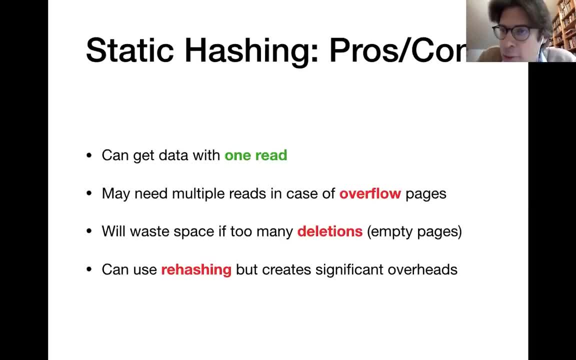 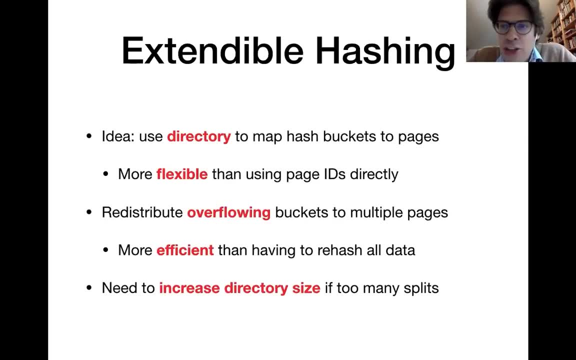 you recreate your index from scratch, but, as discussed, that is quite expensive. Now an alternative which works better for dynamic data is a so-called extendable hashing, And here the idea is that we introduce one new level of indirection, We introduce a directory. 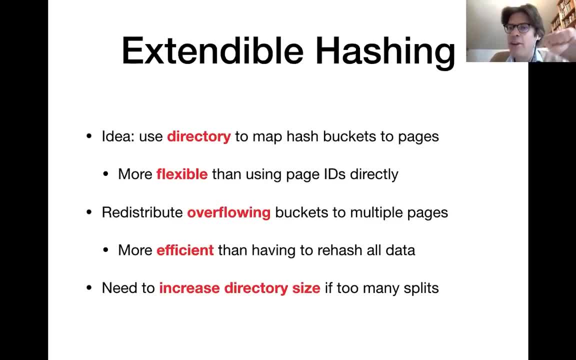 which links a specific hash bucket to specific pages. So instead of calculating the hash value and then directly looking up the corresponding page. So instead of calculating the hash value and then directly looking up the corresponding page. So instead of calculating the hash value and then directly looking up the corresponding page. 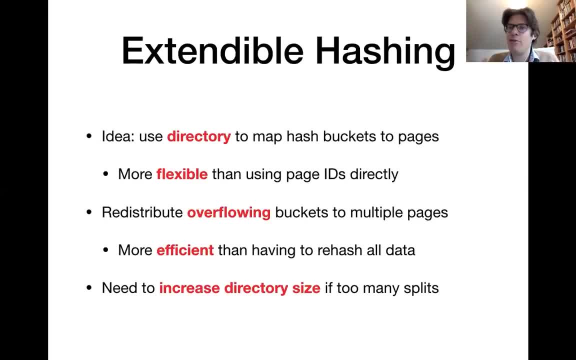 you would calculate the hash value, then you would look up in the directory which page is associated with that one, and then you would look up the corresponding page. Now, what it gives us this directory is essentially more flexibility about how I handle situations. 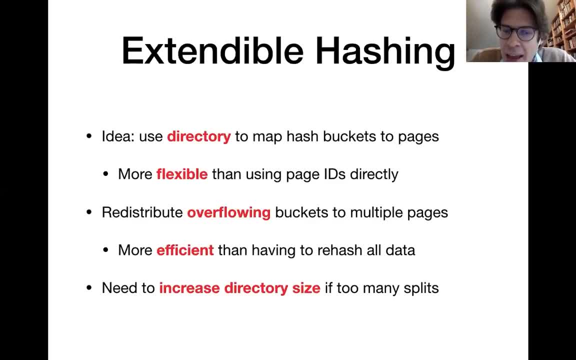 in which I need to add pages to the index. So, essentially, if I have one specific page that is overflowing, then I introduce a new page and I rehash the entries that were on the original page, together with the new entry that I'm currently inserting in order. 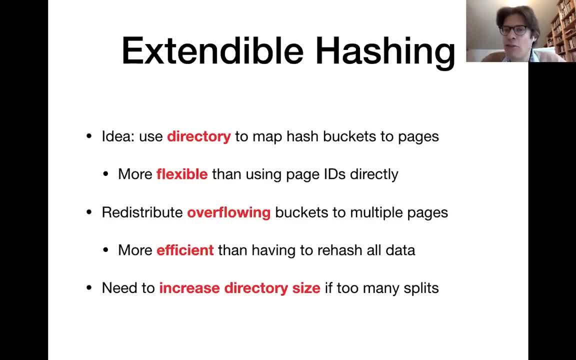 to balance those entries just across those two pages. As I'm adding more pages every once in a while, I need to increase the number of pages that I'm adding to the index. So I'm going to increase the number of pages that I'm adding to the index. So I'm going to increase the number of pages that. 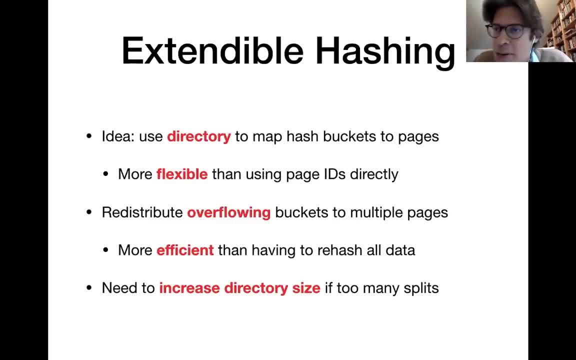 I'm adding to the index. So I'm going to increase the number of pages that I'm adding to the index, the size of the directory, and then it can be a little bit expensive, but in each case it is much cheaper than having to rehash, having to recreate the entire index from scratch. 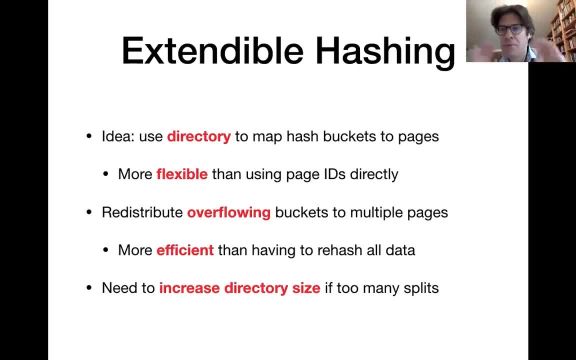 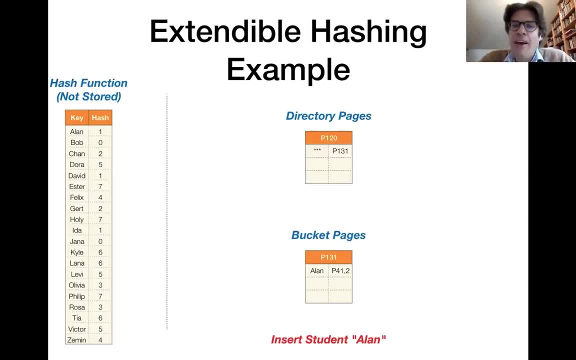 which is what static hashing has to do. Let's make things a little bit more concrete by an example. So in this example I have extendable hashing and on the top of the page you see the directory pages. right now that's only a single one page: 120.. And on the bottom of the screen you see the bucket pages. 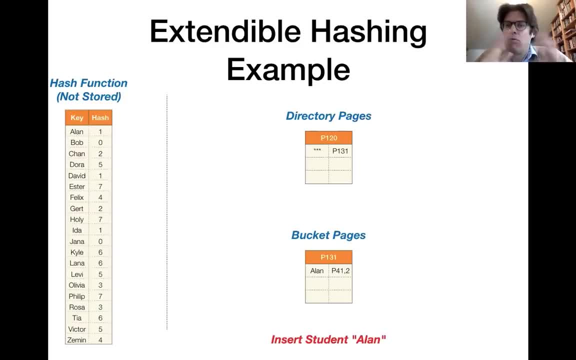 page 131.. Now, right now we only have one single page that stores a data entries, which is page 131.. So the directory only has one single entry. here on the left hand side, you essentially see the hash values that we are. 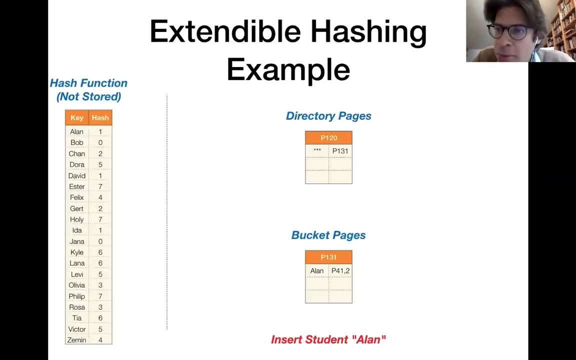 associating with a page- And in the right column you see the corresponding page that we are referencing- And to make the following easier to follow here: for the moment I have written the hash values in the hash function according to the normal system, But now let's actually switch and write those hash values in the binary system. 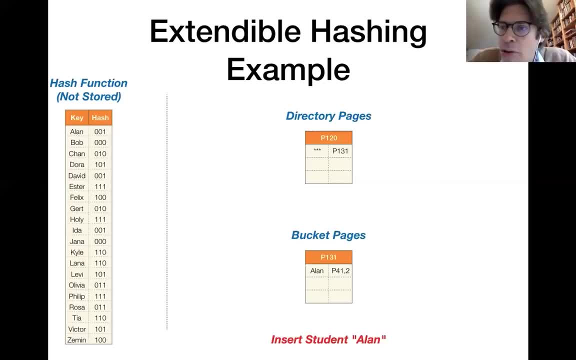 because it will make the following example, of course, more convenient to represent. So here we had the hash values between zero and seven. that is, that means I need three bits in order to represent that, And right now in the directory, you see on the left column, we have those three. 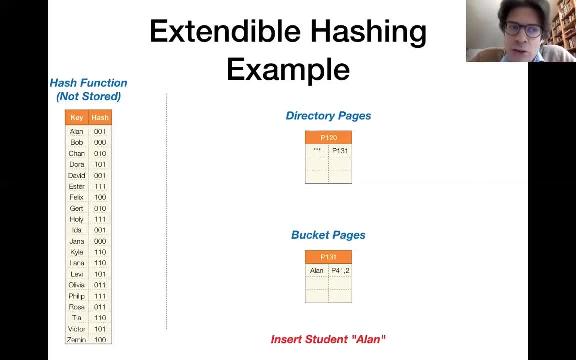 stars. And by that I mean that here we are associating all entries, independently of the values for those three bits of the hash function, with page number 131.. Now we have just inserted student Alan into the index which you see on the bottom of the page. Now let's insert a student Bob next. 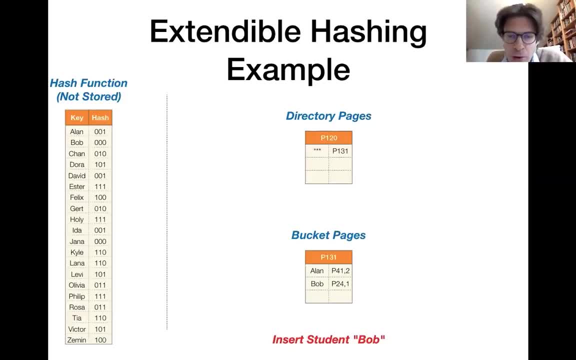 All right, so here nothing much happens. we insert Bob on page number 131, which is the page associated with all hash values as indicated by the directory star, star, star. So we can have any values for the hash bits. All right, now let's just insert the next student in alphabetical order, which is Chen, And again we can. 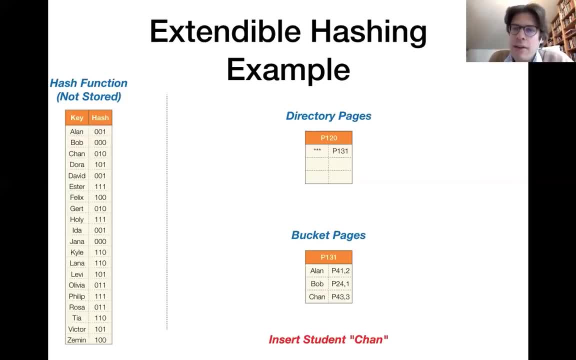 insert the student here on page 131.. Now it becomes interesting, because if you insert the next student, Dora, we don't have enough space anymore on page 131. That means we need to introduce a new page, but we don't want to introduce an overflow page. 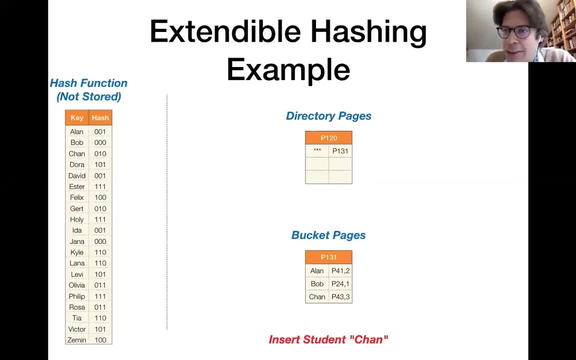 So we need to add an associated entry to the new page in the directory. So now let's do this. And here you see, on the bottom I've introduced a new page 133 and in the directory have introduced a new entry. so, and now we have. 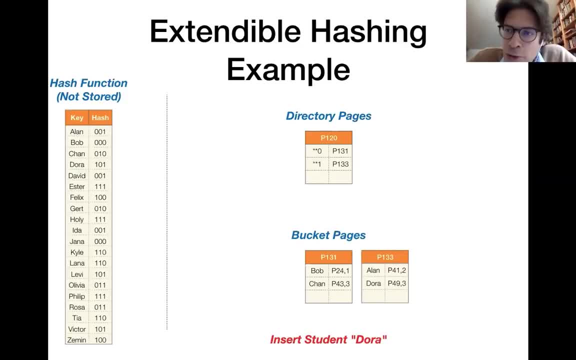 two entries, so you somehow, so we somehow, have to associate them with non-overlapping value ranges of the hash function. so here you say that page number 131 is associated with all entries whose hash value ends with a zero, and page 133 is associated with all entries whose hash value. 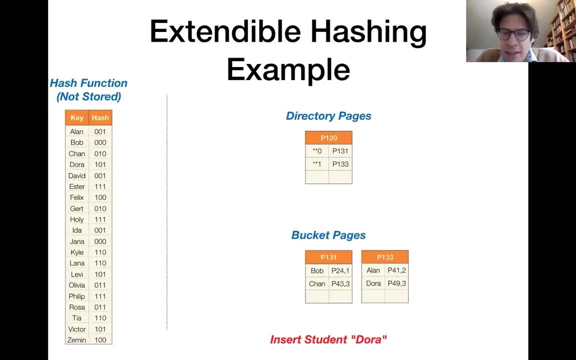 ends with a one, and here on those pages 131 and 133, i have distributed the entries accordingly. i needed to distribute the old entries on page 131 and the new entry, student dora, that i have just inserted. and you see, for instance, bob has a hash value of 000, so it ends with a zero and that means we put it on page 131. 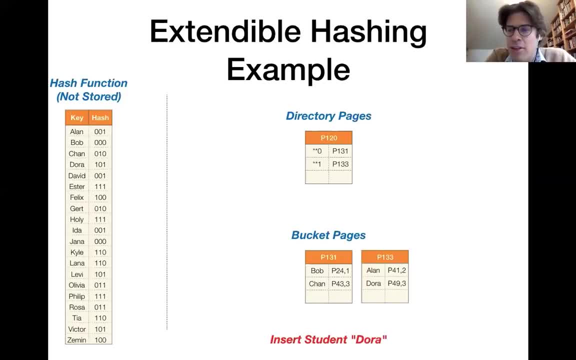 while alan has a hash value of 001, so we have to put it into page number 133, all right? so let's insert david and david has a hash value of 001, so it ends with a one and we should insert it according to the directory. 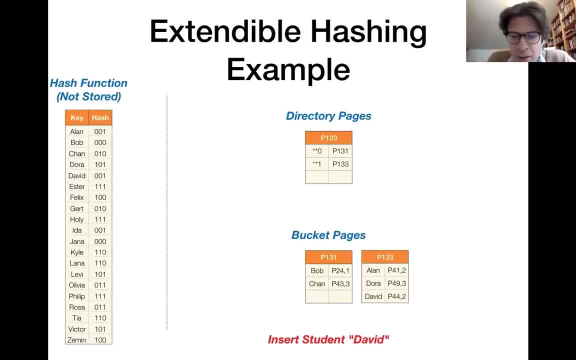 into page number 133. all right now. next student is would be esther. um, and if we insert esther, then something interesting happens, because esther, the hash value, ends with a one and it would need to go into 133, but that page is already full. so i have to add more pages. um, if i add more. 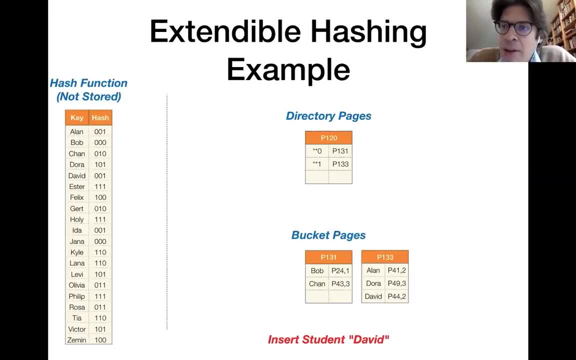 pages, i again need to assign them to non-overlapping value ranges in the directory. so far in the directory i have only considered uh one single bit, the last bit, and that was sufficient in order to distinguish two different uh pages. but now if i add a third page then like one bit is not. 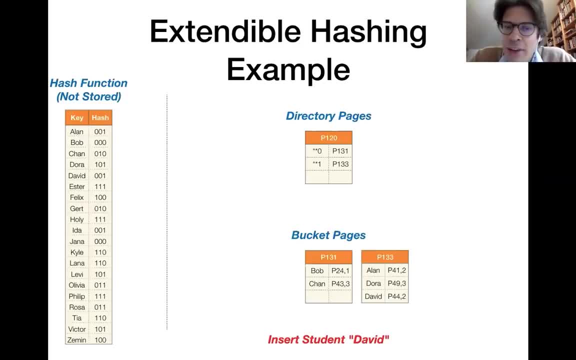 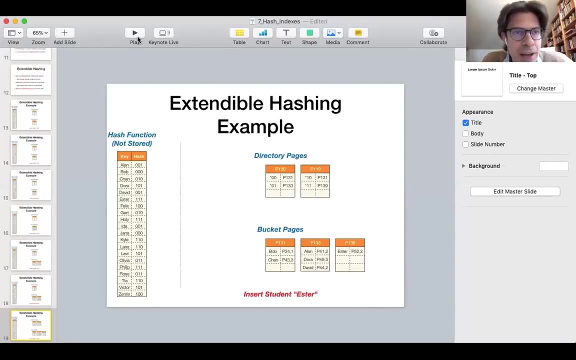 sufficient anymore to distinguish between three pages, so that is why the directory will need to consider two bits now. so let's do this, so we are adding a one new page. let me quickly move the chat so i can recognize the page number. and that page is 139, and in the directory we have 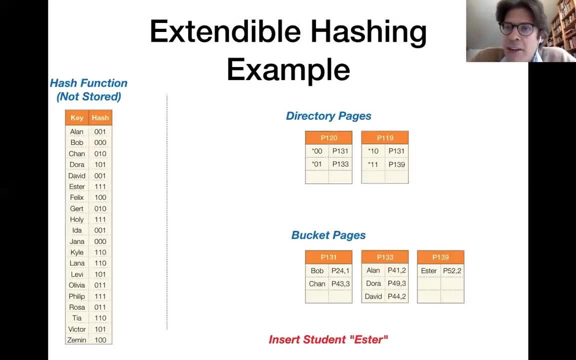 expanded the directory, because now we need to consider the last two bits instead of only the last bit, and, as you see, here i'm associating those different pages with non-overlapping value ranges. now one interesting thing here happened, so the new student that i wanted to insert, esther, would have to be inserted in page number 133. um, so this: 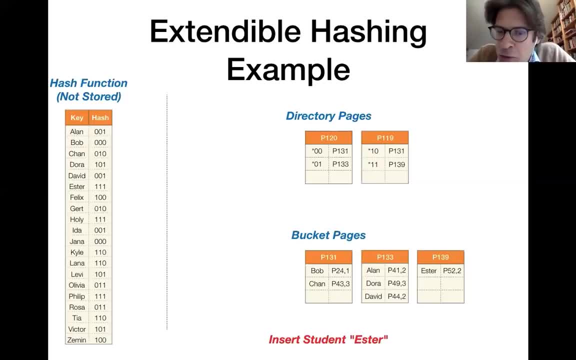 specific page was overflowing with entries and that's why i actually only wanted to to split that specific page. on the other side, page number 131, that one still has some space available and it is not overflowing. this is why we have not split page number 131 and if you look at the directory you see that essentially all the 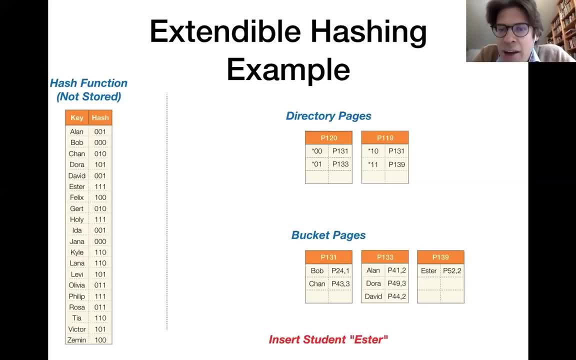 hash values ending with zero zero and all the hash values ending with one zero. they are both assigned to the same page, number 131.. eventually, once we add more entries, then we probably need to split 131 as well and then those entries in the directory change. but for the moment there's like: 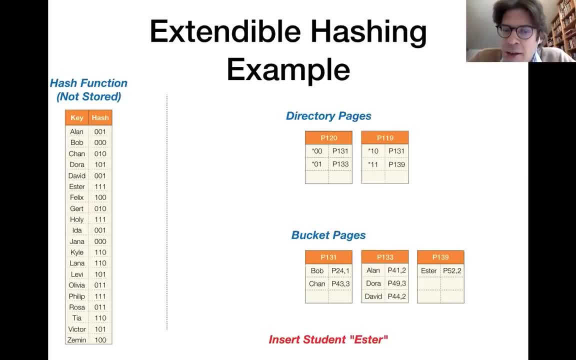 um. two entries in the directory that point to the same bucket page, all right, so let's insert a few more students. it's the same principle. now we've inserted felix and now we are inserting gert, and gert has a hash value zero, one zero. so that means it would have to be inserted into page number 131. 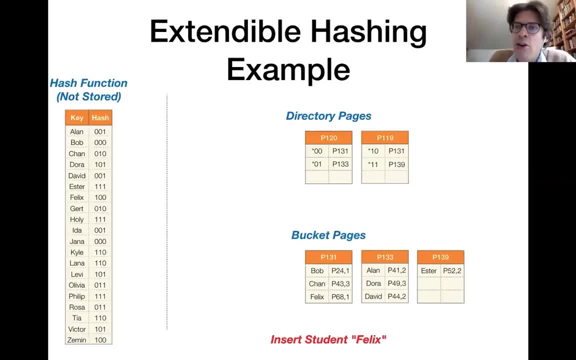 but now that page is also overflowing, so we need to split it into two pages and we are doing this by adding one more page in the bucket pages and redistributing the corresponding entries. and, as you see here, now we have updated the directory and, and page 131 only has one entry left, um. the other entries, um have moved to page 126. 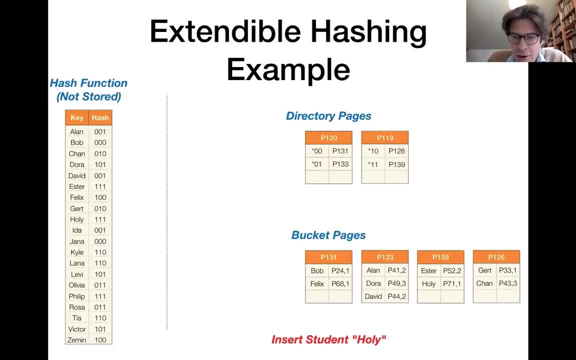 so, and now we can insert a little bit more, and at some point- um, we have too many bucket pages to index them with two bits alone, so at that point need to expand the directory further in order to consider all three bits of the hash function, and if that happens I also have to increase the size of the. 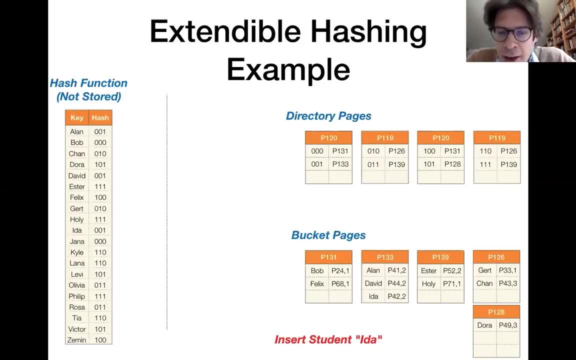 directory and as you see here now the directory considers all bits from the hash function. there is some pages that are linked to repeatedly in the directory, for instance page number 131 again, and there's other pages that are linked to only once, depending on how many insertions we had for the 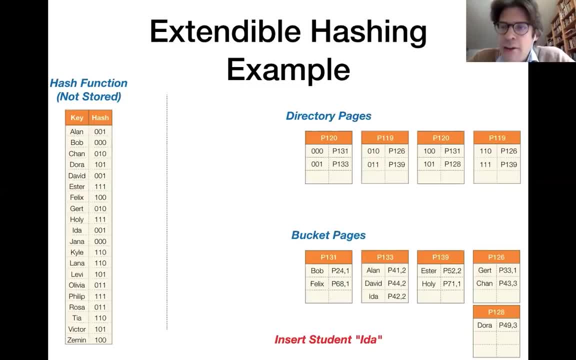 corresponding range of hash values. so this approach is pretty flexible. I encourage you to have another look at this example. but the main point really is that we have this directory which associates hash value ranges with specific pages, and having this directory gives us a lot of flexibility in order to only split those specific buckets that are. 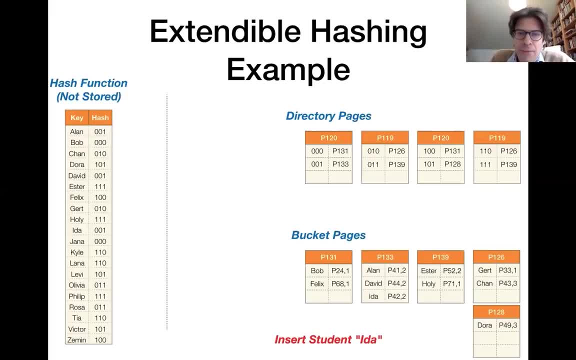 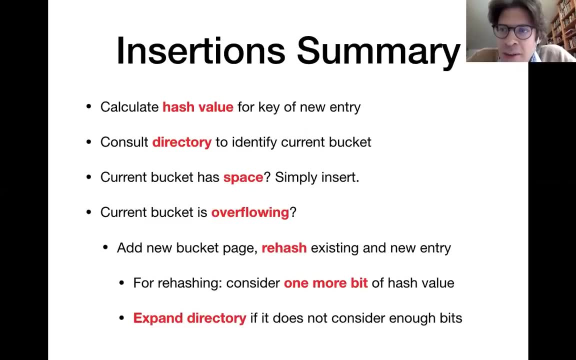 currently overflowing. now, here you have a little summary of this insertion algorithm that we have already executed so far. so the way it works is that you- you can see that we have already executed so far. so the way it works is that you- you can see that we have already executed so far. so the way it works is that you. 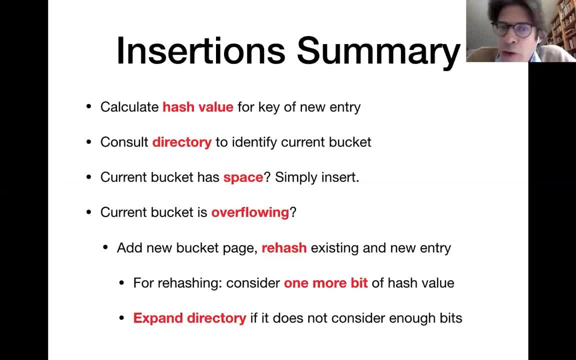 always start by first calculating the hash value for the new entry that you always start by first calculating the hash value for the new entry that you are currently trying to insert. then you look into the directory in order to identify the associated page and if that page still has some space, great we. 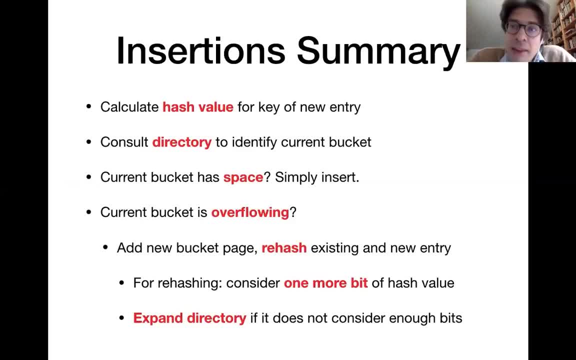 simply insert the new entry, no problem. if the page is currently overflowing, it cannot store the new entry anymore. then it becomes more interesting. then it becomes more interesting. we always have to at a new bucket page and we have to redistribute the entries on the page that is currently overflowing. 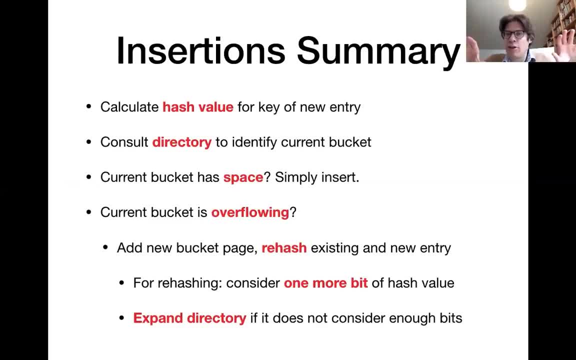 and the new entries on those two pages in order to redistribute them. between those two pages. I consider one orbit from the hash function and, if needed, I might have to expand the directory if currently- still Currently- the directory considers less bits than what I have used in order to redistribute. 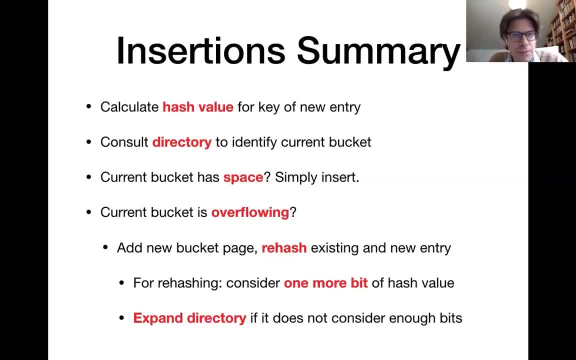 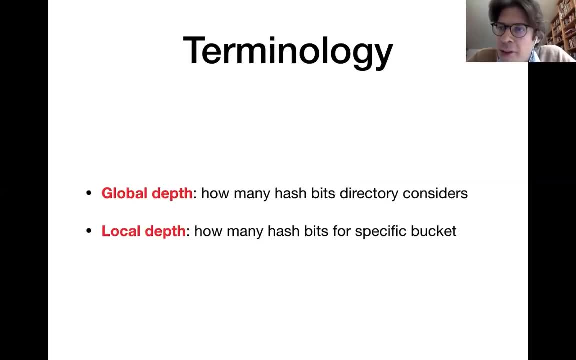 the entries after the insertion. There's some terminology that is often used in the context of those extendable hash indexes. You also find it in the book, So I wanted to quickly link this description to that terminology. So we always have discussed about the number of bits that are considered in specific cases. 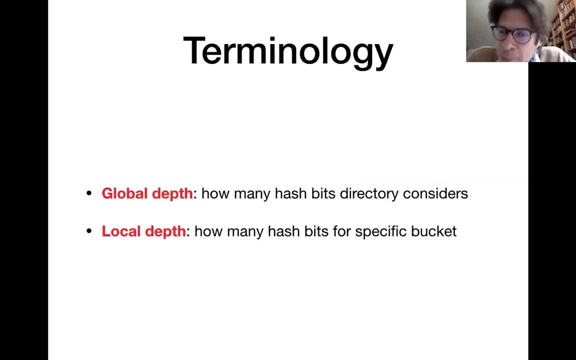 Often people say that global depth, this is the number of bits from the hash function that the directory currently considers, and the local depth for one of those hash bucket pages. that is the number of bits that you need to consider in order to be sure that. 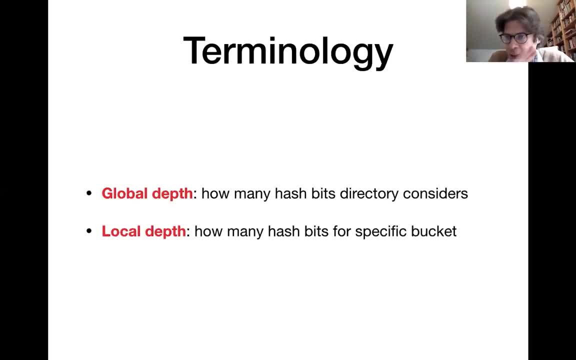 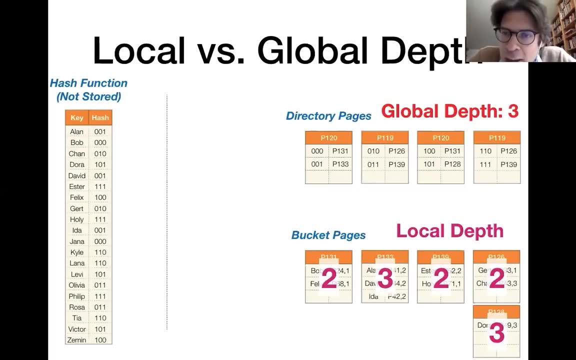 an entry is located on that page. So let's go. Let's quickly make that a little bit more concrete by the example. For instance, here: this is the state that we finished in and in the directory. you see that we have a global depth of three, because the directory is currently considering three. 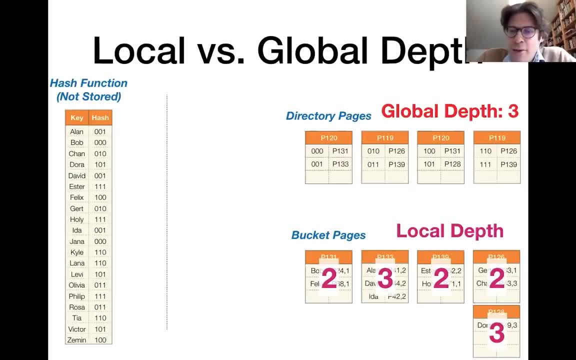 bits. On the other side you have different local depths for the different bucket pages. For instance, take page number 131.. So this page is referenced twice in the directory: On the first directory page and on the third directory page. I actually just spotted that. 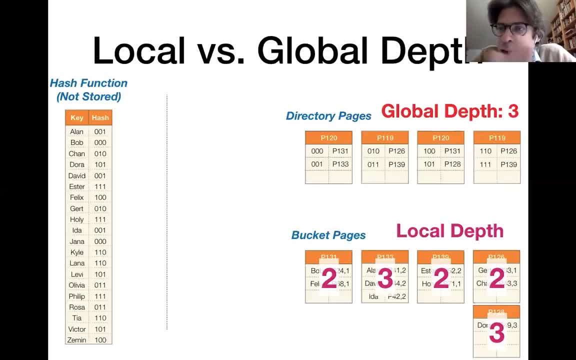 we have, like, multiple directory pages with the same page ID, which should not be So. you should have different pages. Of course that's a little typo, but we see that we have a page, number 131, linked to twice in the directory. 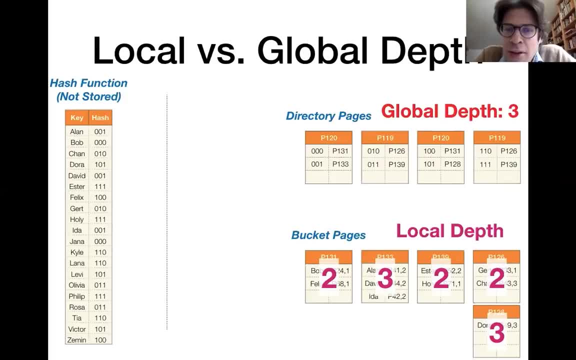 Once for the directory, Once for the hash values: zero, zero, zero and once for the hash values one, zero, zero. That means, whenever you know that the last two bits of the hash function are zero, zero, you can be sure that the corresponding entries are associated with page number 131. 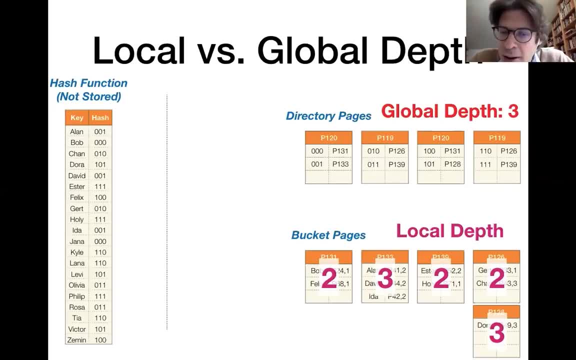 So, in order to know that page number 131 is interesting to you, you only need to consider two bits, and that is why the local depth for page number 131 is two. On the other side, if you're taking page 133,, for instance, then that page is only: 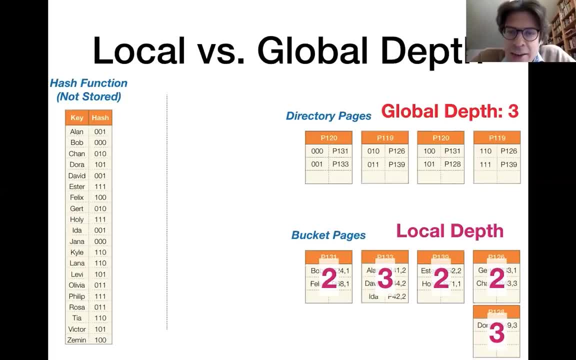 linked to once in the directory, And that means that, in order to be sure that this is the interesting page for the entries you're looking for, you have to consider all three bits from the hash function. That is why the local depth for page number 133 is three, because you have to consider 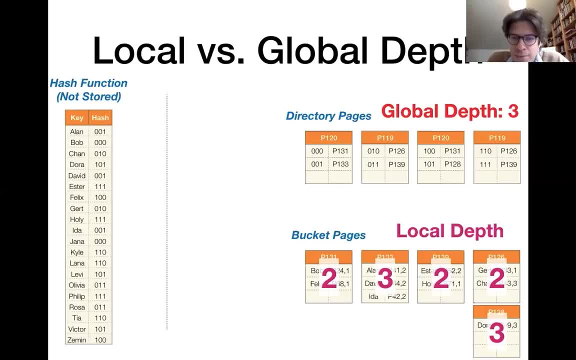 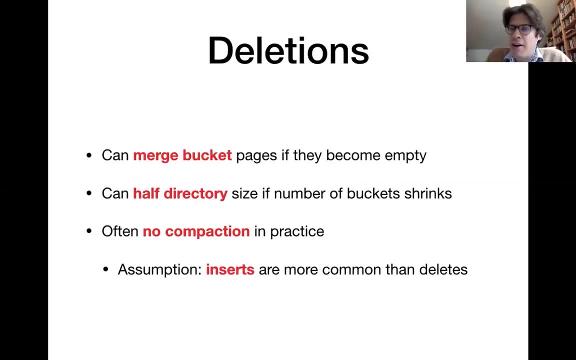 three bits in order to be sure. So that's why the local depth for page number 133 is three, because you have to consider all three bits in order to be sure. All right Now, this is how insertions are handled. and maybe one last word on global versus local. 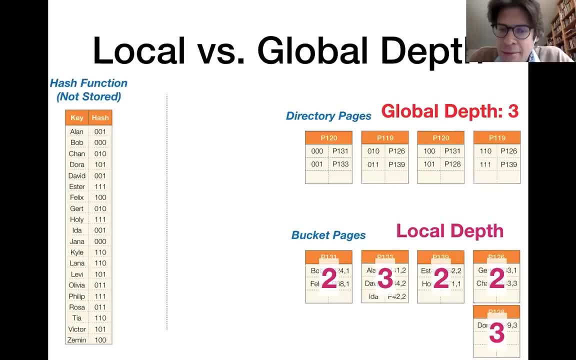 depth. You can say that the condition which causes you to expand the directory, that is always if the local depth becomes greater than the global depth. So the global depth of the directory must always be an upper bound on the local depth of all of your bucket pages. 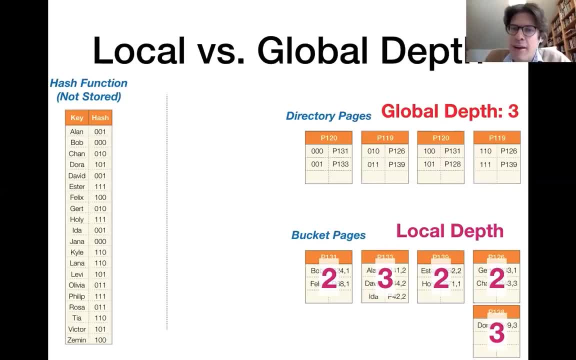 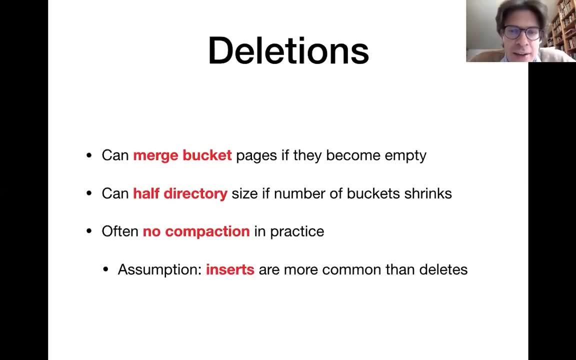 That is one way in which this terminology becomes useful. All right, So now we have discussed about insertions into those extendable hash indexes. Now, what about deletions? Clearly, if we have enough deletions, then we could merge together again some of those. 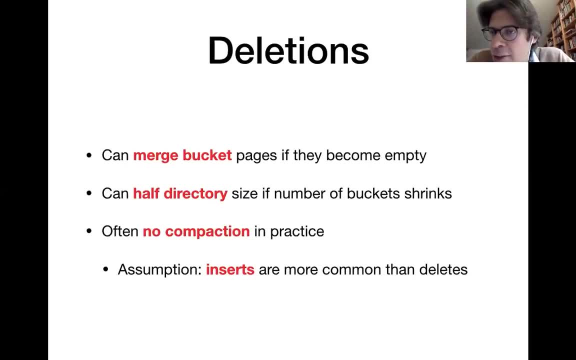 bucket pages. So if the number of entries on them is low enough in order to fit on one single page, At some point, if I keep merging pages and the number of pages therefore shrinks, I might even be able to reduce the size of the directory. 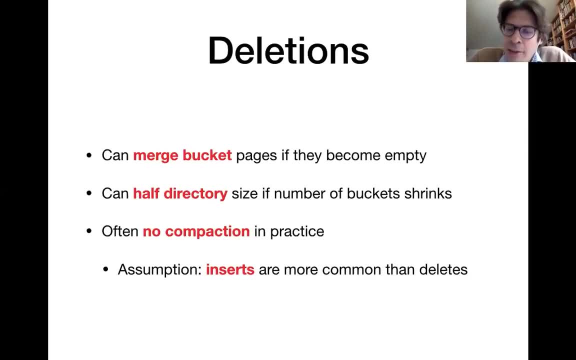 In practice, however, people often assume that insertions are more common than deletions, And so the implementations that we find in practice. they might often not do anything sophisticated in case of deletions, But handling insertions well, that is pretty important. 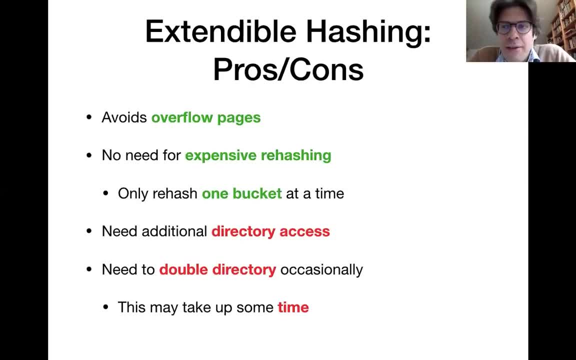 Now if we analyze the pros and cons of that index. So a first pro, of course, is that we avoid overflowed pages And on the other side we don't need any expensive rehashing. So when we redistribute, Okay, 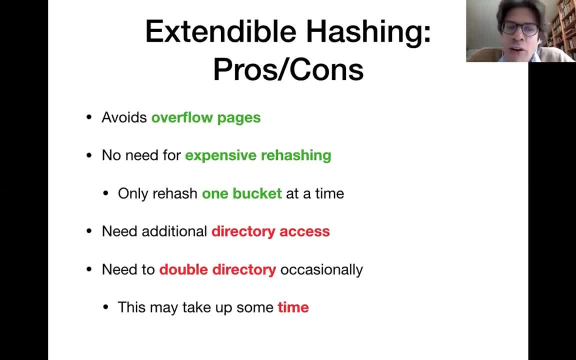 So when we redistribute entries, it's always only the entries on one of my pages, So that means quite reasonable overhead. On the other side of course, I'm introducing a directory, So I need one additional access in order to look up things in the directory. 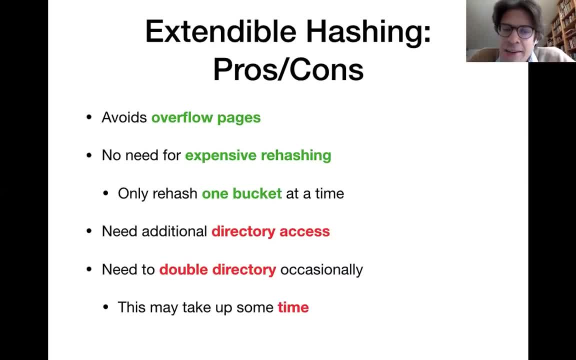 And every once in a while- and that is more important- I need to double the size of my directory If the local depth exceeds the global depth. Now doing this operation- double the size of the directory- that takes some time, which is inconvenient. 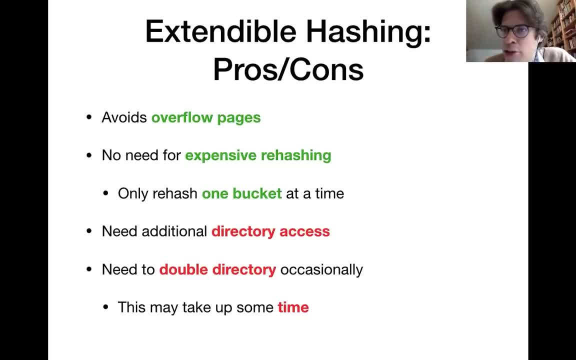 Of course it is much faster than having to recreate the entire index from scratch, which is what static hashing might do, But nevertheless it is a little bit inconvenient. So the idea of the next hash index method that we will consider is to avoid this occasional 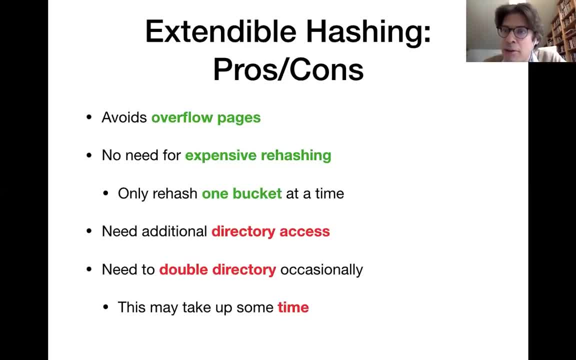 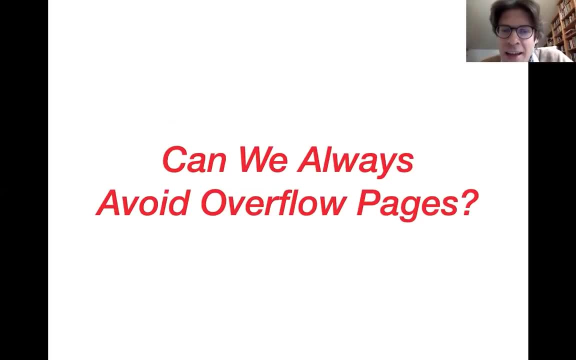 overhead of having to double the size of the directory. Maybe one last question before we switch to the next hashing index. On the last slide I wrote that we can avoid overflow pages at least often. The question is: can we always avoid overflow pages with that kind of index? 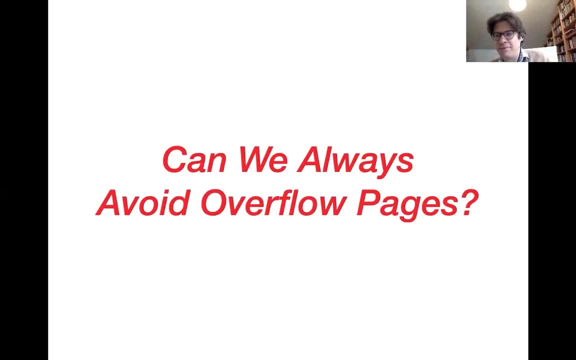 Or is there situations where we cannot avoid them, perhaps? Okay, Yes, Yes, That is the right answer here in the chat. Very good, Exactly So. the thing is that hash values are generally not unique, So you might have a hash condition that multiple entries map to the same hash value. 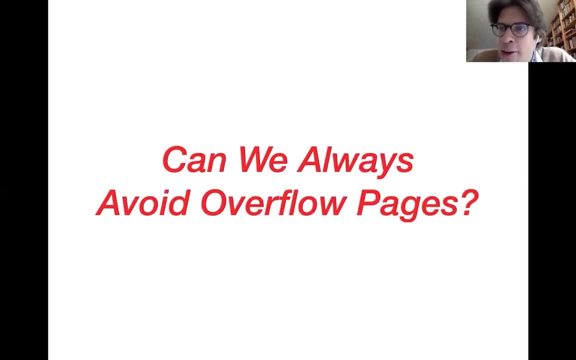 And in those cases there is no number of bits that you could consider in order to separate entries from each other, Then you might not have another choice than to use overflow pages. Of course, you might wonder: Maybe If I use a different hash function I wouldn't have that problem. 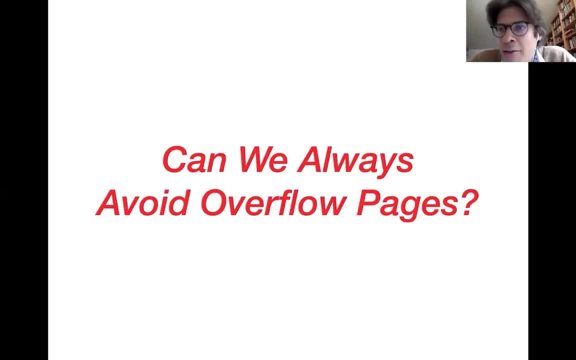 But in the end you might even have multiple entries for the same key. If you think about the enrollment table, you might have multiple entries for the same student, And if you have too many entries with exactly the same key, then even the best hash function. 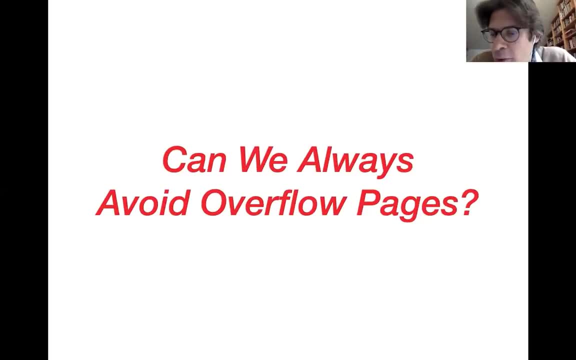 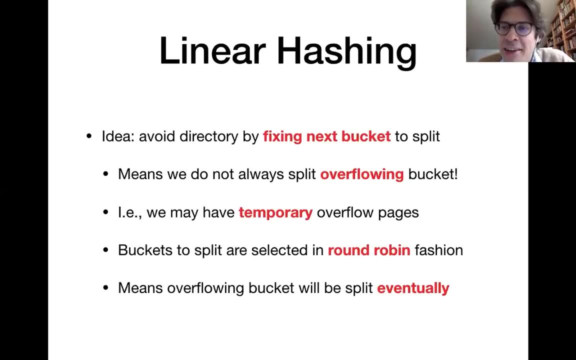 of course, will not help you anymore, And then you actually have to work with overflow pages. Very good, All right, Let's continue with so-called linear hashing. So that is the last hashing hash index method that we will see. So the idea here is that we essentially get rid of the directory again. 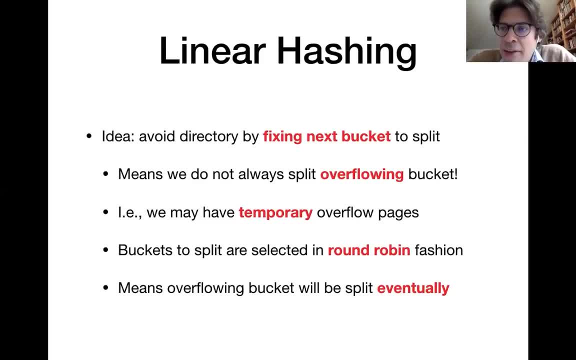 Now, in a way, it is the directory that gave us the flexibility to choose which specific pages, which specific buckets, we wanted to split after insertions. So let's go back to the previous slide. Let's go back to the previous slide, All right. 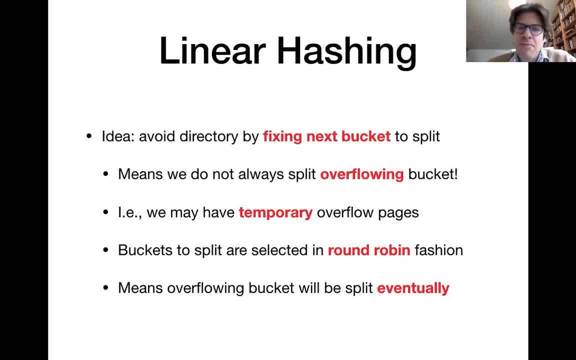 So if I get rid of the directory, then it means I also have to give up some flexibility in choosing which buckets I split next, Because I don't have a directory anymore to keep track of that. So what I do, therefore, is that we are selecting buckets to split according to a round robin. 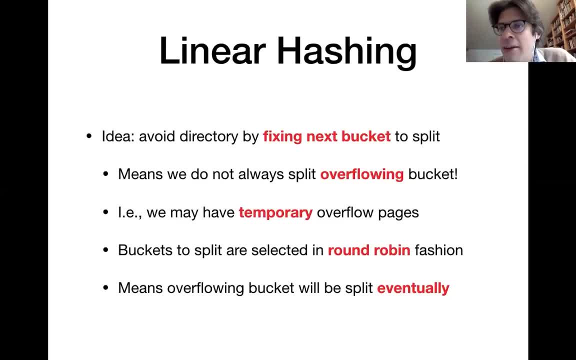 principle, And in particular That means not even be able to immediately split one of those buckets that are currently overflowing. So that can seem inefficient, and it sometimes is. You have bucket number five is overflowing, but the next bucket that you have to split is bucket number one. that might be currently almost. 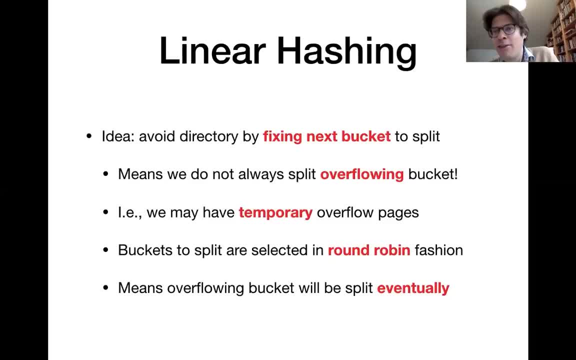 empty. So, nevertheless, since you are fixed to one specific order in which you need to split the buckets, it means that you would have to split bucket number one and you would have to introduce an overflow page for bucket number five, Of course, eventually, if you keep splitting, 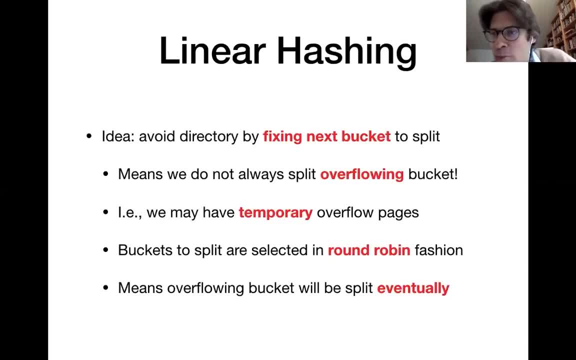 buckets, then after a while you will reach bucket number five and then you will probably be able to get rid of the associated overflow page. But at least temporarily you will have to allow for some overflow pages, but typically they don't persist for very long. 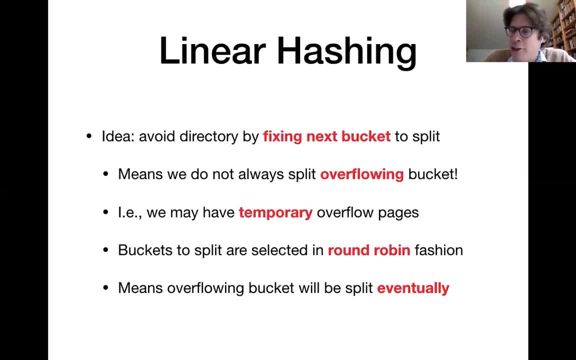 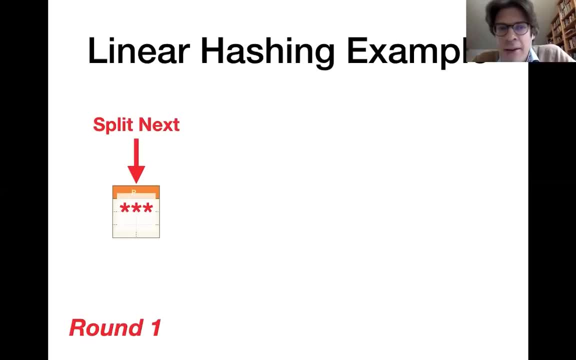 So that is the high level idea behind linear hashing. Now let's see a little illustration for how that works. So generally, splitting proceeds in so-called rounds, and on the left lower corner of the slide you see the round counter. A round essentially ends once you have. 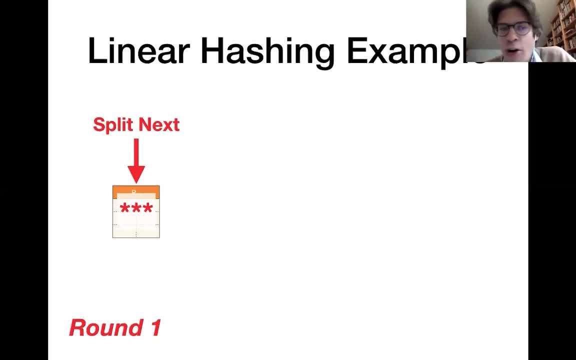 split all the buckets that existed at the beginning of the round And you see there's a big red pointer pointing to the bucket that will be split next, After a round is finished, you will reset that pointer to the first bucket again and then the next round starts. So right now we only have 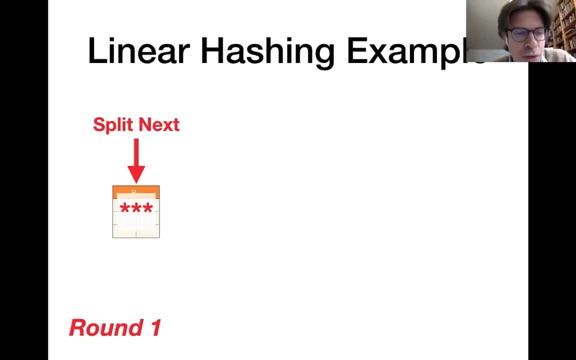 one single bucket that exists at the beginning of the round, and those three stars here mean again that this page here is supposed to contain all the entries, for any value, of those three hash bits. All right, so now let's assume that we have insertions and therefore we need to. 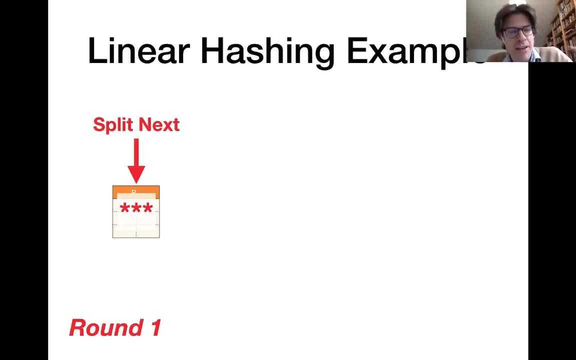 split this bucket over here. So now we are splitting this bucket, and we are splitting it into two buckets, one of them associated with hash values, where the last digit is zero, and one associated with hash values, where the last bit is one. And now, since we have 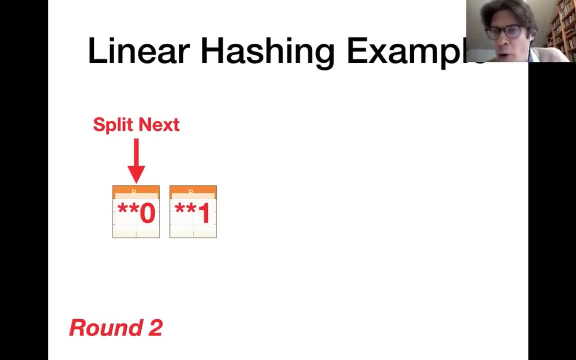 the only bucket that existed at the beginning of round one. we also immediately enter round number two, as you see in the counter here, and we are resetting the split. next pointer to the first entry, to the first of our buckets here. Okay, so now I assume that we have even more insertions. 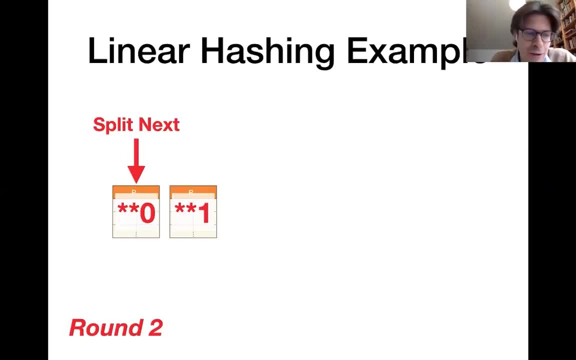 into our table and therefore into the associated index. So now we have again to split that bucket that our pointer is referencing. So now we have one bucket that is associated with hash values ending in zero-zero and one bucket that is associated with hash values ending in one-zero. All right, so we are still around at two. we are now pointing to the last. 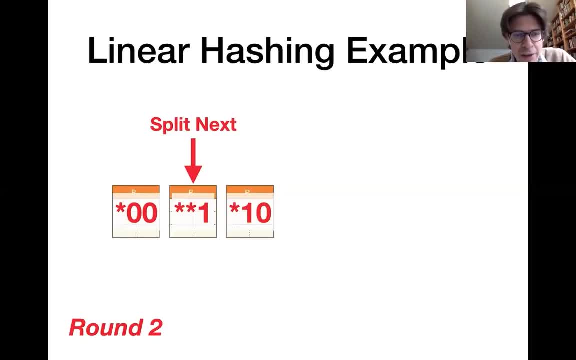 bucket that existed at the beginning of the round. here, after we split that one as well, we are resetting the counter again and we are entering round number three. So now we have four buckets that are associated with the four possible value combinations of the two last bits of the hash function. Okay, and now we can continue. 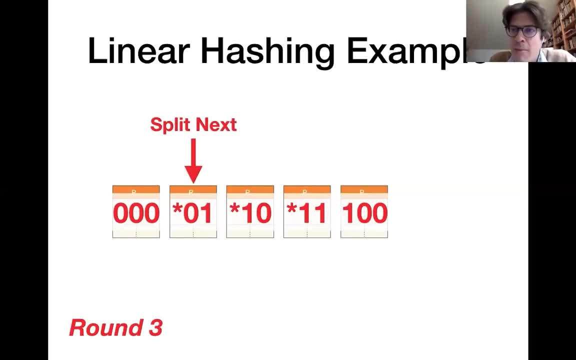 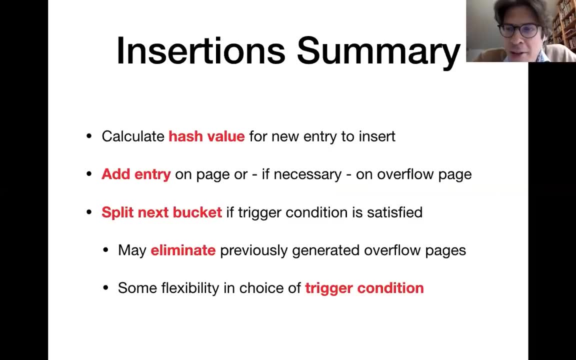 this and we can split the first bucket here and the second bucket here and so on, But the principle is the one that is summarized here. So if we want to insert something into one of those linear indexes, then first of all we calculate again the hash value for. 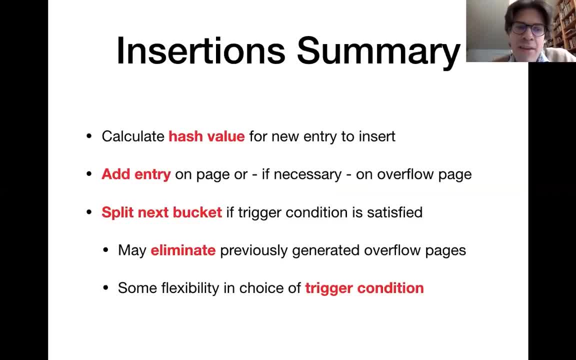 the new entry to insert, And then we add this entry on the associated page. or if that page is full, you might have to introduce an overflow page, Hoping, of course, that this overflow page will be eliminated relatively soon. Now, if some kind of trigger condition is satisfied, we 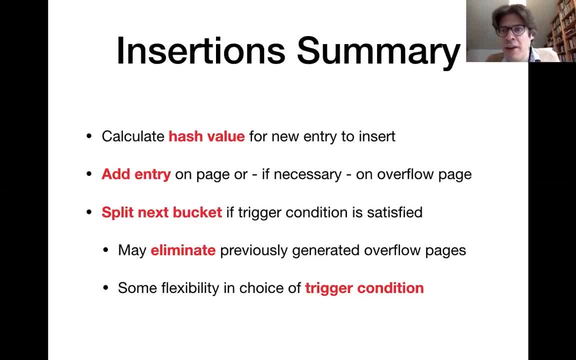 decide to split the next bucket. We have no choice about which bucket we can split. We can only split the bucket that our next split pointer is referencing, And there is some flexibility in how we can choose that trigger condition. For instance, we can say that the 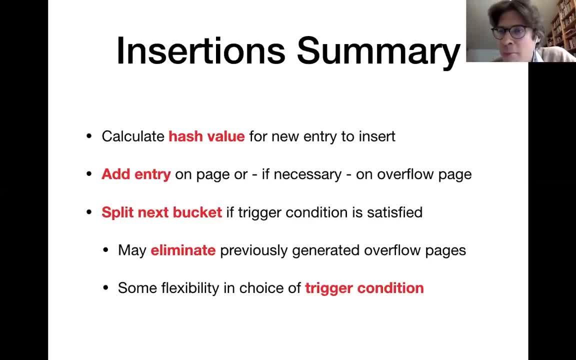 next split today lasts until sundown. So in this case we can say, in order to say that one next different switch is hidden to ensure that we had got no entry, the next switch is going to beimos, the second split folder, And in the second split we have one negative. 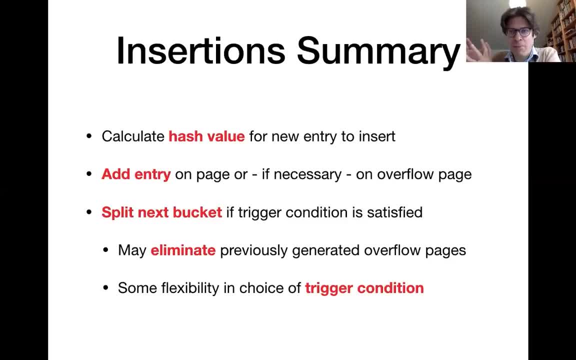 feature In the second split. we have no entry link and similarly there is no exit link, So the result is always like this and so on. Now again, we can give a short water trend if this is what we want. Thekor taking is actually one justice for this. in these cases, as in our, 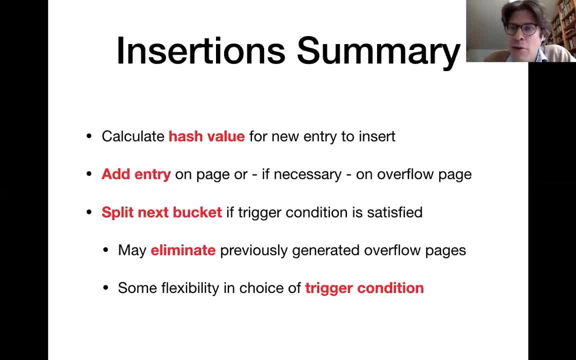 expression. Thisazing is satisfied, and the point is that it fills this vacancy quota again. just why, anatkρώош notice, is we tall? whether we want to talk about any other depends on which. if you continue splitting buckets, all right, so those splits will eventually eliminate overflow. 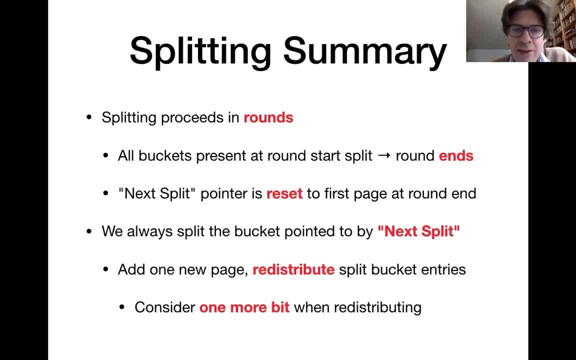 pages and, as we have discussed, the splitting generally proceeds in rounds. so if we have split all the buckets that existed at the beginning of a round, then the current round ends. and if the current round ends, then, as we have seen in that little illustration, we reset the power. 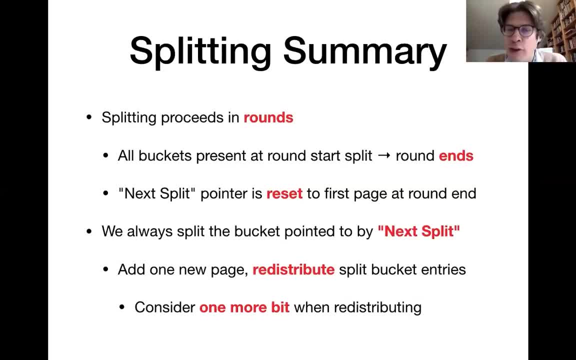 pointer to the next bucket to split, to the first of the current buckets. all right, and the bucket that we split next, that is always the one that we are pointing to. if we add a new page, then we generally redistribute the entries from the split bucket and we do so by considering one more bit from the associated hash function. 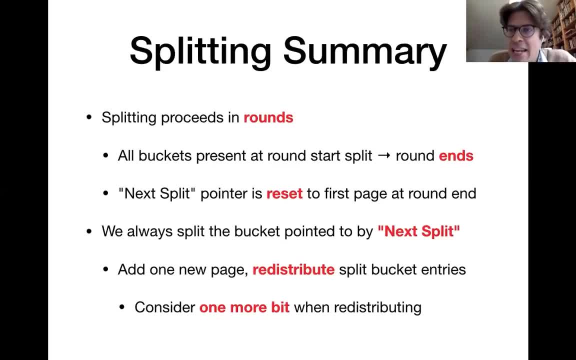 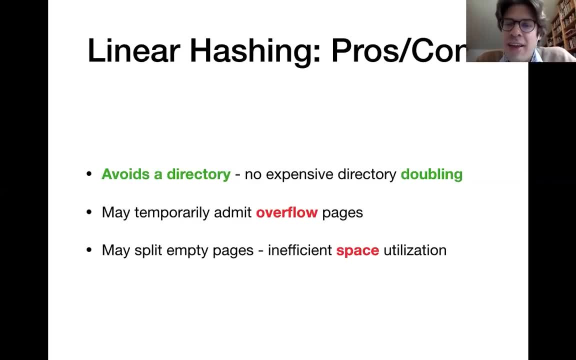 so that is the principle behind linear hashing and if you compare the pros and cons, then the nice thing about linear hashing is that it avoids the directory, so we don't have any expensive directory at doubling. it has to draw back, that it might temporarily admit overflow pages and it sometimes may split pages that are empty or near empty, which means 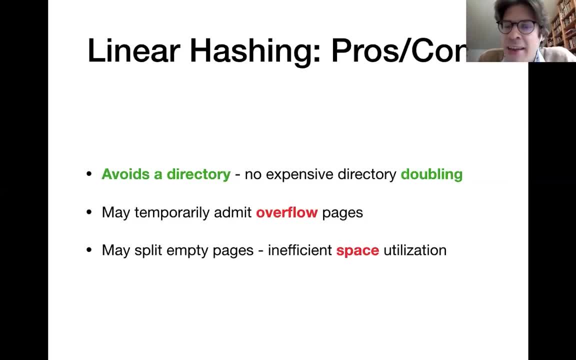 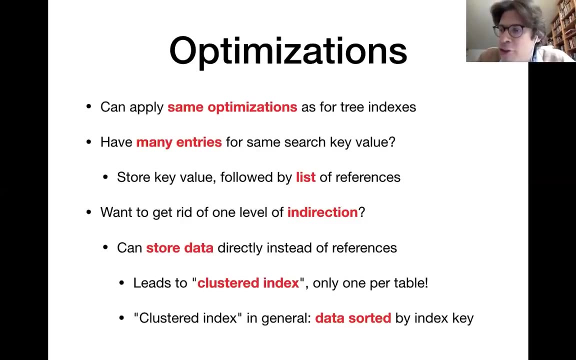 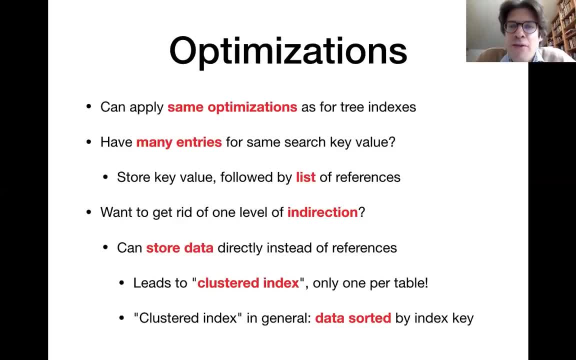 principle, we can use all of those optimizations for a hash indexes as well. for instance, if you have many entries for the same a search key value, then we can store that key value, ones followed by a list of references. so we have also that possibility for tree indexes. the advantage is that I store 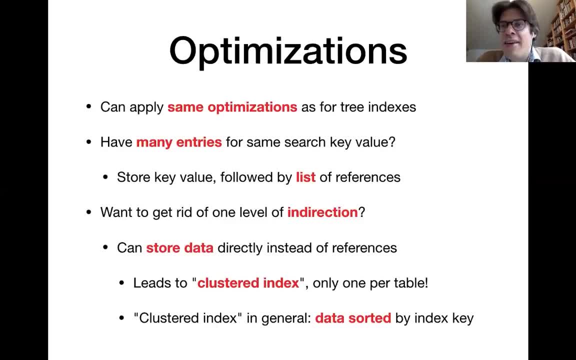 less redundant data. a disadvantage is that that I might transform a fixed length entry into a variable length entry, And it means I would have to store additional metadata on my page in order to save where this list starts and where this list ends, for instance. 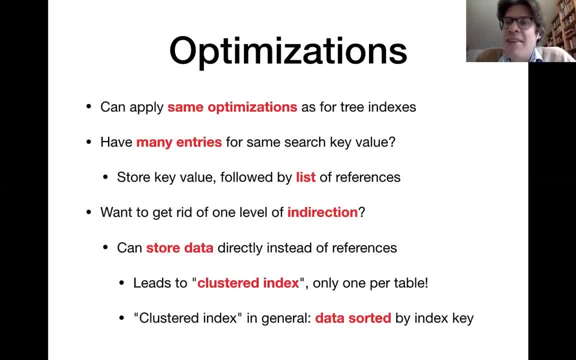 Also, so far, we have assumed that my data entries in the index, that they essentially store references to the actual data. but that is not necessary. I can, in principle, also store the actual data directly. Now this is what we also call a clustered index. 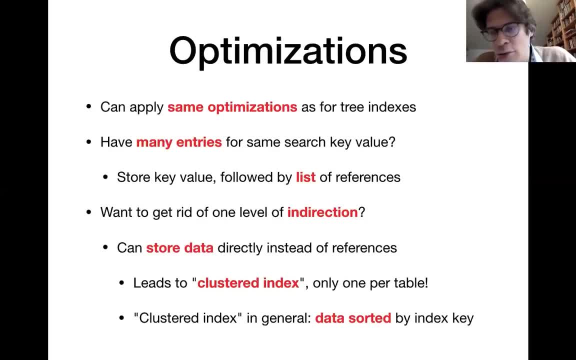 As long as you don't want to store duplicates of your data, which you generally avoid, it means that you can only have one of those indexes per table, because that index is essentially merged with the table data right. So that makes retrieval more efficient because you save one lookup and also you are guaranteed. 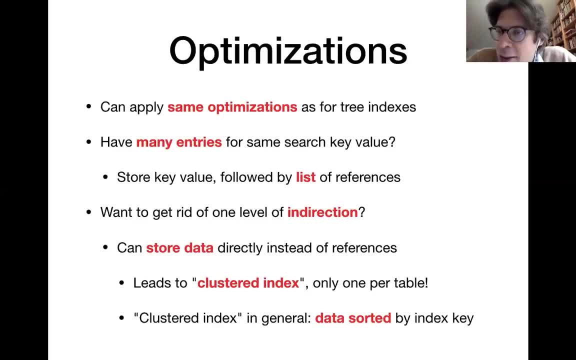 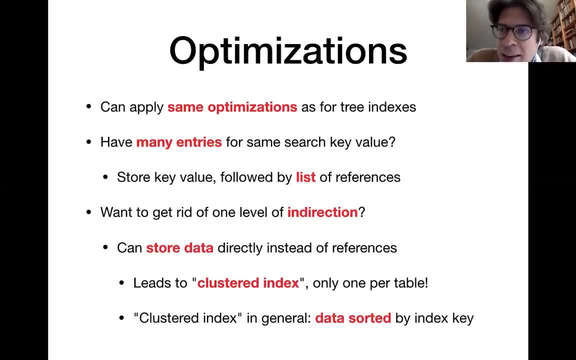 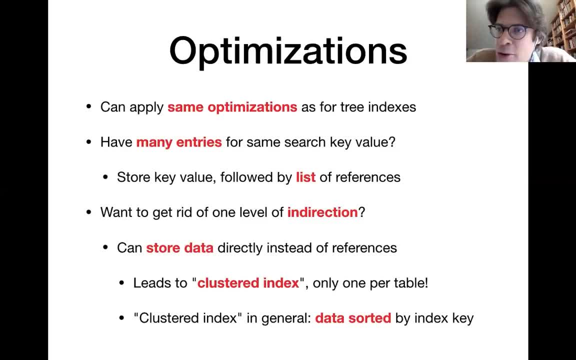 according to the index search key, because that means things that are stored close together in the index will also be stored together in the original data set and that makes it quite efficient to retrieve the associated data with a few page accesses. So if the order of the data is consistent, 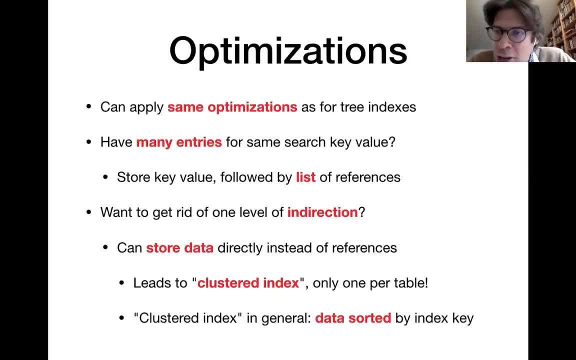 with the index search key, then that is also called clustered index in general, And to here retrieval is also more efficient in general than if that is not the case. So those are just a couple of optimizations in the context of hash indexes And they're essentially the same optimizations. 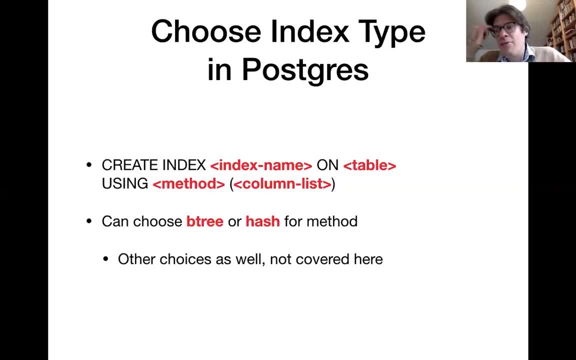 that you can apply for tree indexes. Now a little word on how we can use those Indexes in Postgres, and I'm going to show a quick example about that next time. So in Postgres you can choose the type of index. 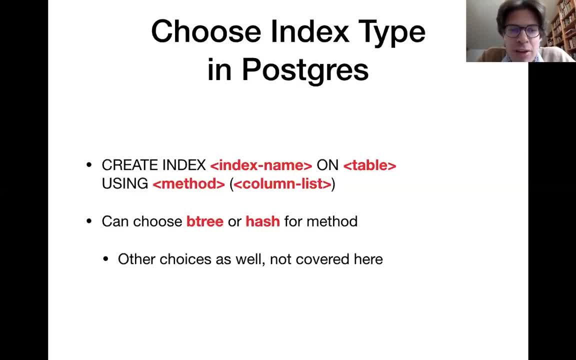 that is generated By default. it will generate B-trees, but you can specify explicitly which type of index you want it to generate. So if the syntax here create index, then the name of the index, then on the table that the index. 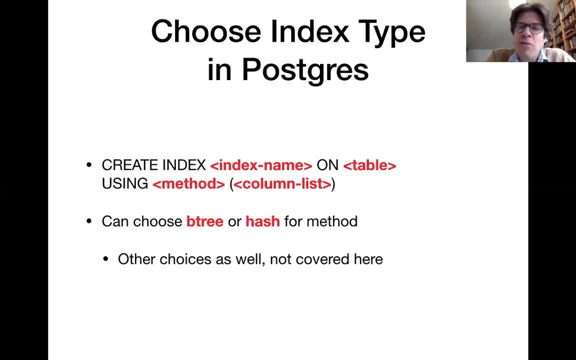 refers to, and if you insert here using method- the method can be, for instance, B-tree or hash or other methods that are discussed in the documentation- Then you can choose what type of index you generate. And again, here between parentheses, 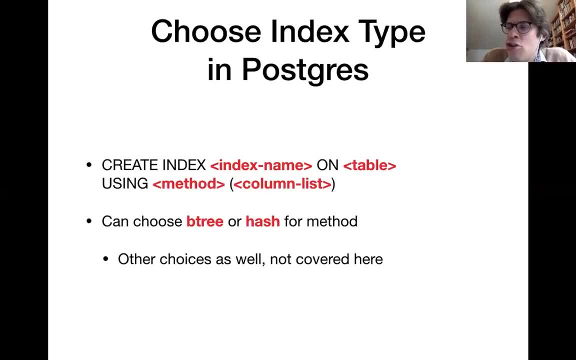 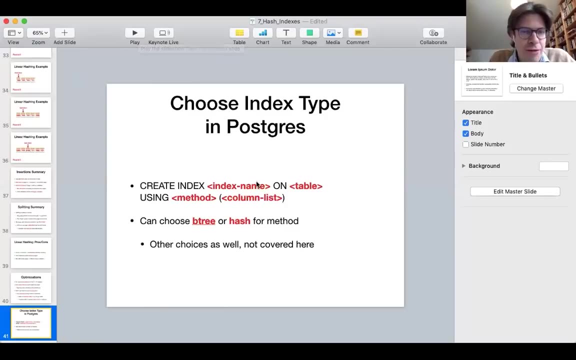 you can specify the columns that your index should refer to. So if you want a composite index, you can specify multiple columns here. All right, And now we have already reached the end of the lecture time, So I'm going to show you quickly how. 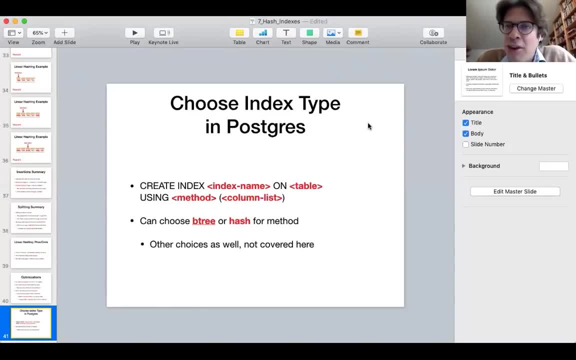 to use those indexes in Postgres next time. The next homework will focus on indexes, so I encourage you to revise the indexing material a little bit over the weekend And otherwise have a great day and see you next week, All right, 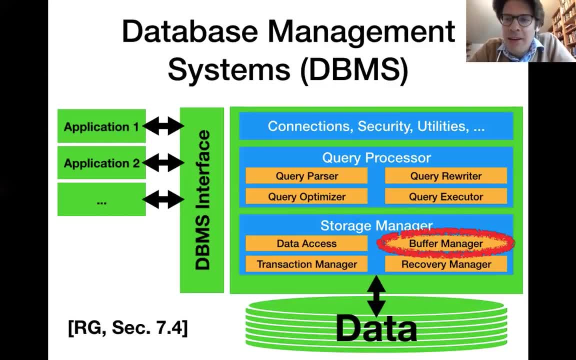 So the last time we have been discussing about index data structures, more generally, about how the data is set up on hard disk in order to make access efficient, In order to work with the data, we first of all have to bring it into mainnet. 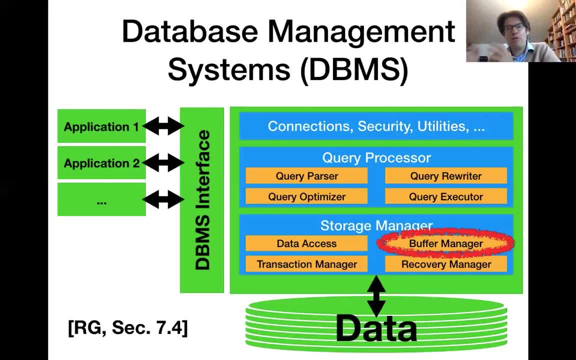 So we have to bring it into the main memory. More precisely, we have to bring it to the processor. But today we're going to talk about how we bring the data into main memory And there's one component in the database system, that is the buffer manager, which controls data movements. 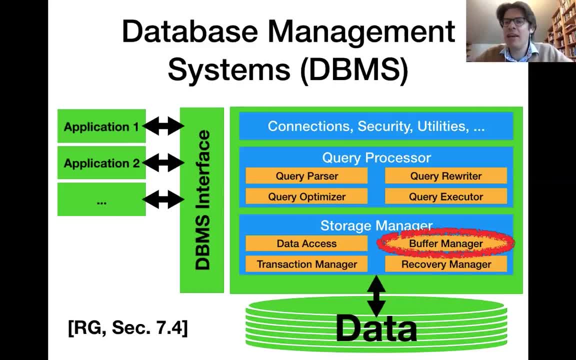 between hard disk and main memory And moving the data is necessary in order to compute with it. Now, the relevant chapter in the Ramakrishna Nagarka book, that is, is about 7.4.. We're going to first discuss about the buffer manager. 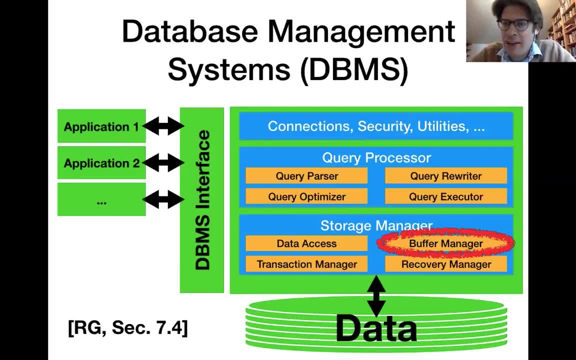 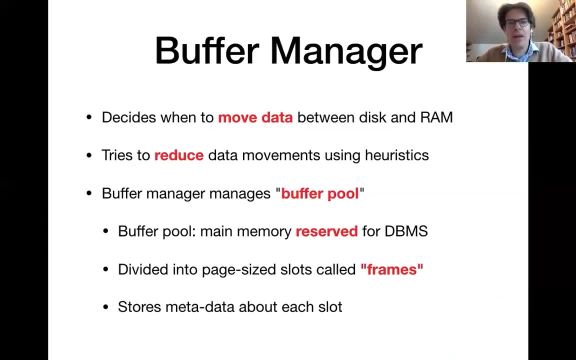 and then later today, if we still have enough time, we will start discussing about the query processor component. So let's first chat about the buffer manager. Now the buffer manager generally decides when to move data between hard disk and RAM. The buffer manager tries to be smart about that. 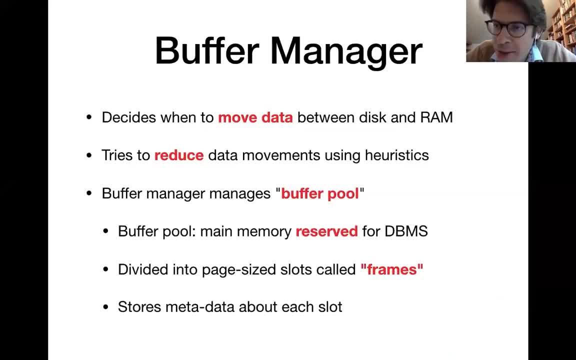 It tries to minimize the number of RAMs, It tries to minimize the number of data movements, And for that it uses a couple of heuristics. We will see one of them in order to try to estimate which pages are most valuable and should be continuously stored. 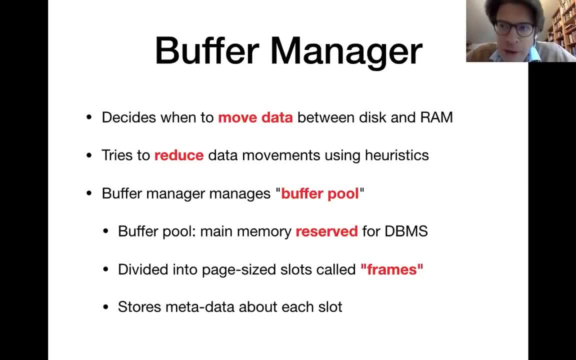 The name buffer manager connects to the term buffer pool And the buffer pool that is an area in main memory that is reserved for the database management system. So this buffer pool, it is essentially divided into so-called frames And those frames they essentially 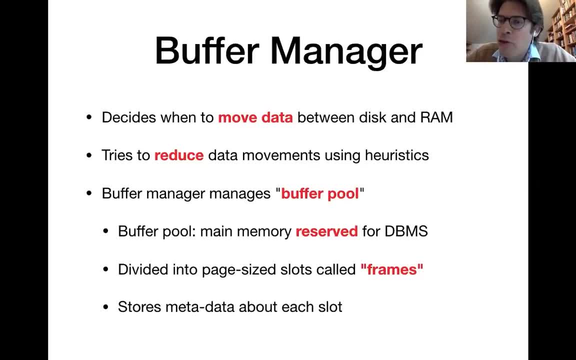 have enough space in order to store one of those pages And the page. that is generally the granularity at which we receive data from hard disk. So the buffer pool contains lots of slots, those frames where you can store pages, And it contains some metadata about each of those slots. 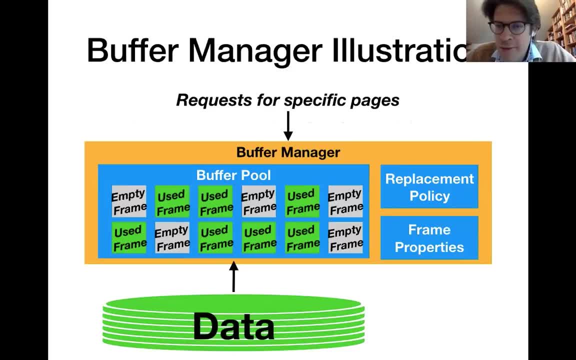 Now, here you see, an illustration of the buffer pool. So the buffer pool essentially gets requests from higher levels in the database management systems And those requests they are about specific pages. So once the buffer manager receives a request for a specific page, it needs to make. 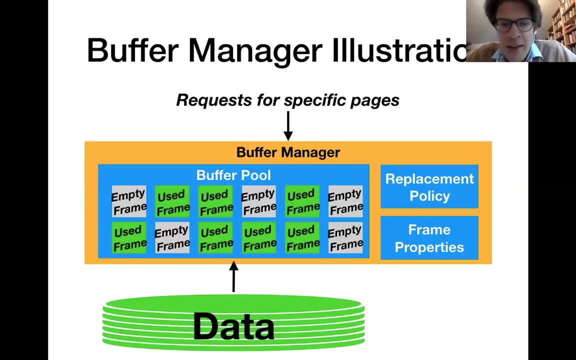 that page available in main memory. The buffer manager stores pages in the buffer pool that you see here. At any point, some of those slots, some of those frames might be empty, but others are used up by a page. So then getting requests, the buffer manager, 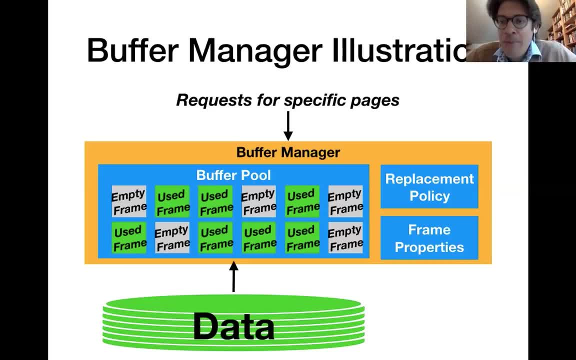 would first check whether the corresponding page happens to be already stored currently in the buffer pool And if not, it will fetch it from the hard disk here. Now the buffer manager stores some metadata about the content of those different frames And it also uses internally some heuristics. 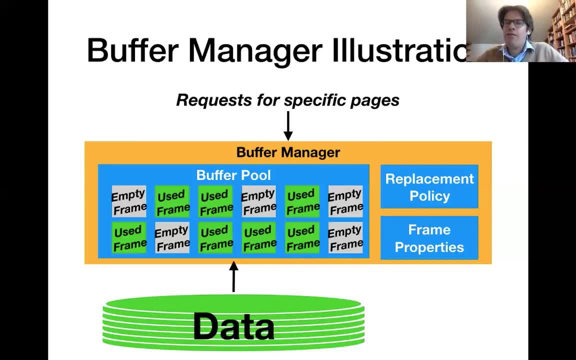 in order to decide, for instance, which pages in the buffer pool to erase in order to create space and which other pages to keep. So that is the replacement policy, And we are going to discuss about the metadata and about the replacement policy in the following. 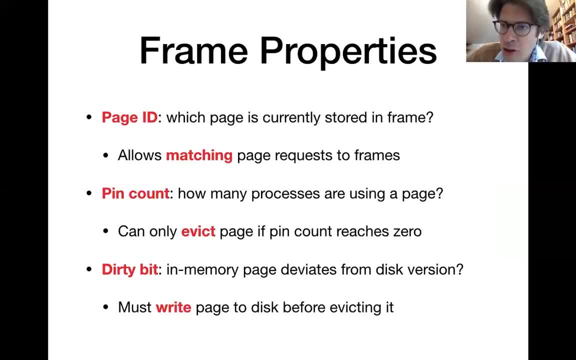 Now, those are the properties that we store about each of the frames. First of all, of course, we want to store the ID of the page that is currently stored in the frame, if any, Because that allows the buffer manager to match incoming requests for specific pages. 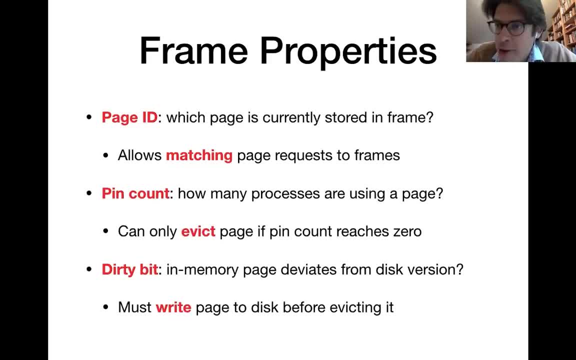 to frames in which the corresponding page is stored, if we are lucky. Also, we store for each of the frames a so-called pin count. The pin count essentially tells you how many processes, how many clients, so to speak, are currently using the content of that frame. 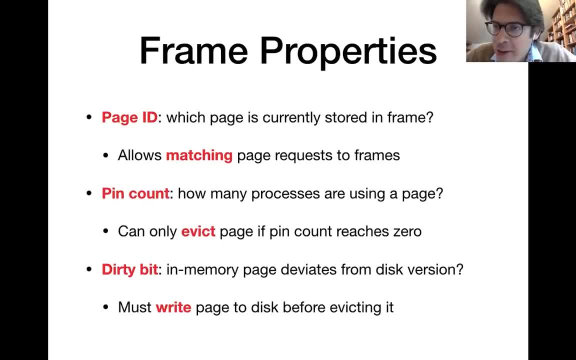 And if there is still people using the content of the current frame, then that prevents us from erasing it and replacing it. So the pin count serves as a kind of a safety guarantee that people don't suddenly have a page erased that they are currently working with. 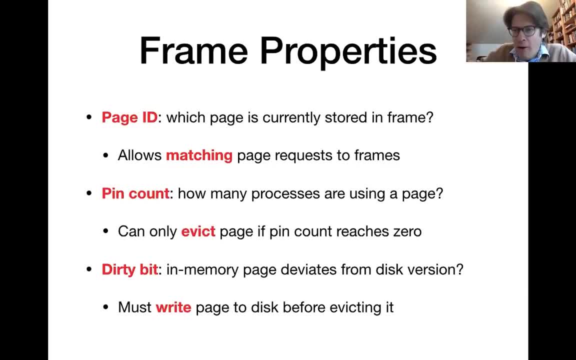 So we can only evict, meaning prune out from the buffer pool, those pages where the pin count has reached zero. Also, we store a so-called dirty bit for the frames, for the pages that are stored in those frames. So we store a so-called dirty bit for the frames, for the pages. 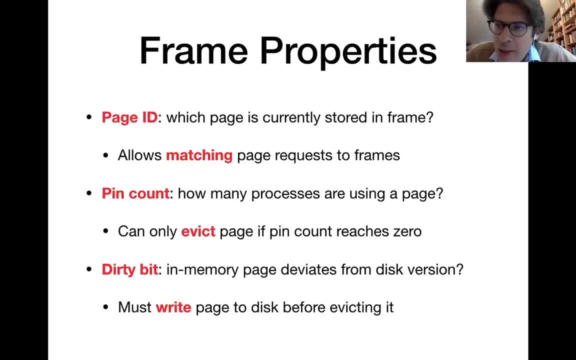 that are stored in those frames. So we store a so-called dirty bit for the frames, for the pages that are stored in those frames, And that dirty bit essentially tells you whether the in-memory page was changed since it was loaded from hard disk. And that is important because changes in main memory. 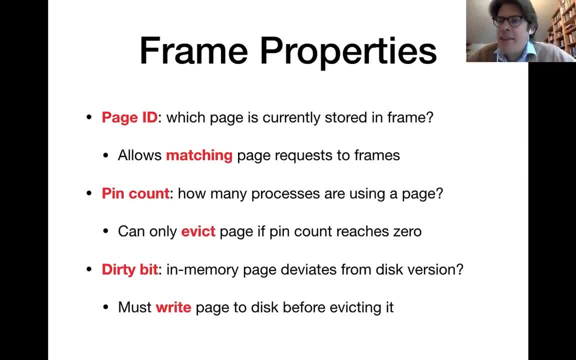 are generally volatile, which means that they don't persist if power suddenly switches off, for instance. or, of course, if you erase the corresponding page And the dirty bit essentially tells the database, tells the database management system, that there is some changes on a page which 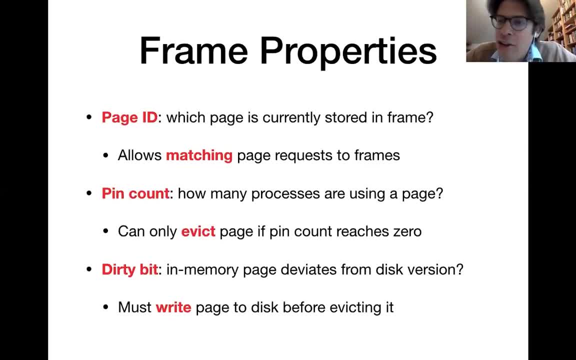 would be lost immediately. if the power suddenly switches off And it also tells us that if you want to erase the corresponding page, then, in order to make the changes persistent, we first have to copy the current page to hard disk in order to overwrite the original version of the disk. 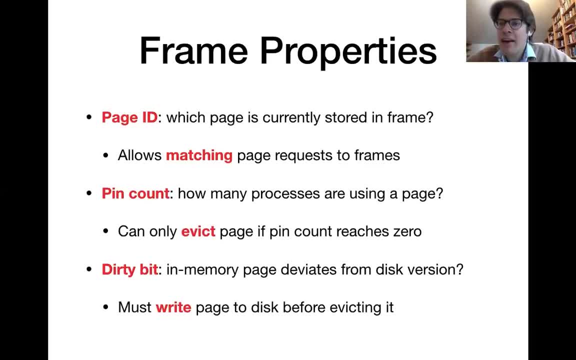 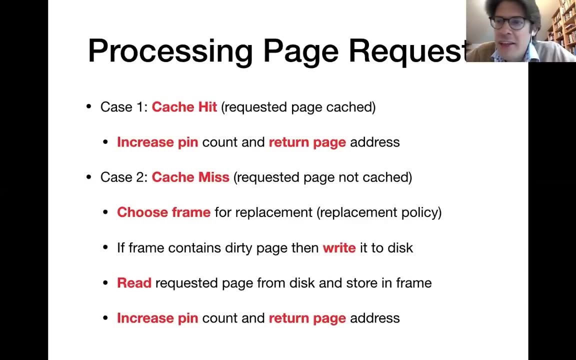 of the page usually Right. So the dirty bit tells us whether there's any changes that we need to back up before we can erase the corresponding page. Now, this is the algorithm that the buffer manager essentially executes Whenever we have a request for a specific page. 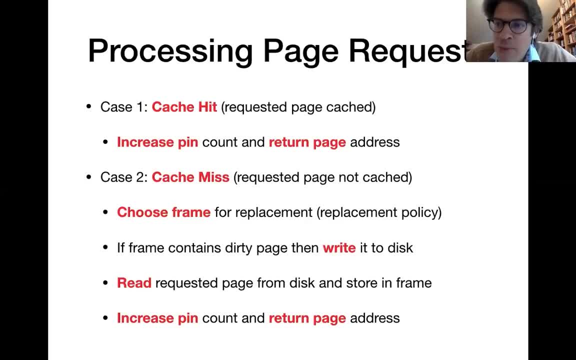 then the buffer manager first of all checks whether this page can be currently found in the buffer pool. In that case we call it OK, We call it a cache hit. This is case number one here, And in that case it is actually pretty short. 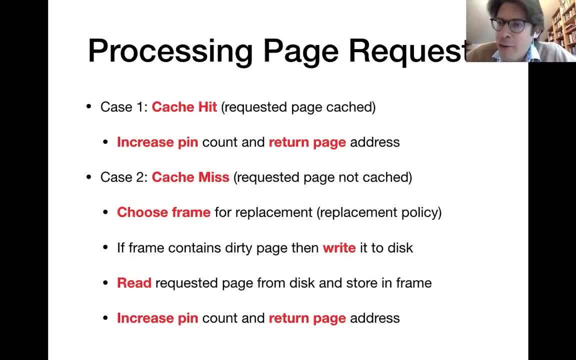 What we have to do. we just increase the pin count for that page, meaning there's like one more process interested in that page, And then we simply return the address of the page to the request store and then the buffer pool is done. 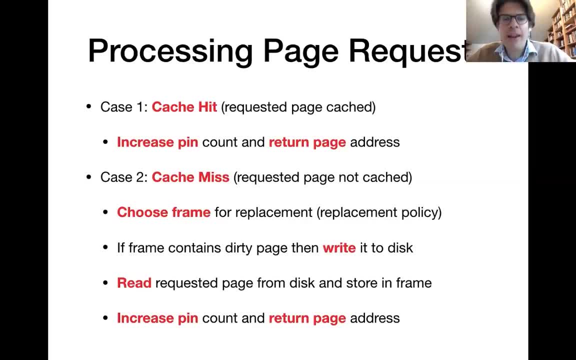 So that is the efficient case. Now, if you have a cache miss, which means that the requested page is not yet stored in the buffer pool, then things become more expensive. The first thing the buffer manager needs to do in this case is to choose. 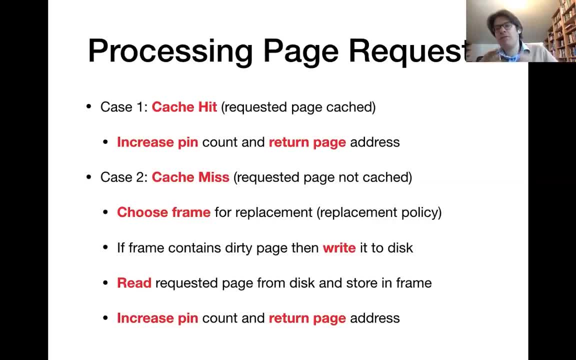 a frame for replacement. Of course, in principle, it could be that we have certain frames that are currently unused, that are empty, so we can simply copy a new page into them Now, when running your database management system, for example. 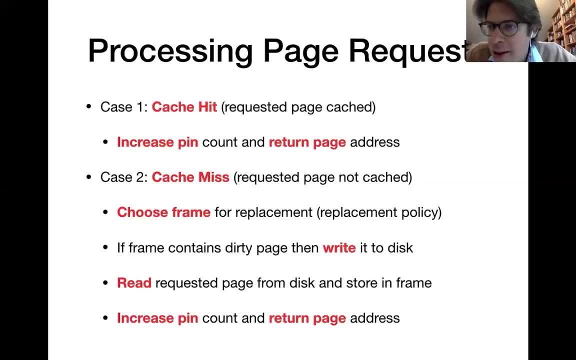 for a while, then that is atypical. Typically the entire buffer pool is taken up. So in choosing a frame for replacement, you're essentially saying that the current content of that frame seems uninteresting and it can probably be deleted. So that is an important decision for performance, which 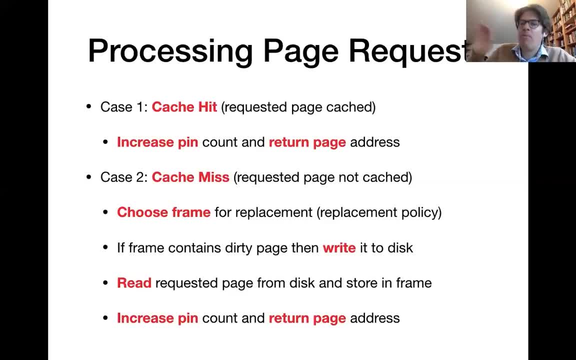 frame you want to replace, And we're going to discuss more about that on the coming slides. Now, after we have selected a frame for replacement, we have to check the dirty bit, Because it could be that the current content of that frame had some changes which haven't been persisted to hard disk yet. 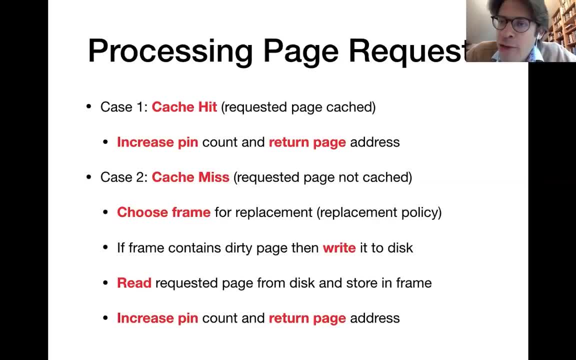 So if that dirty bit is set, then we first of all need to write the current frame content back to hard disk. There's one question in the chat about whether a frame can have more than one page. But those frames they are chosen in size. 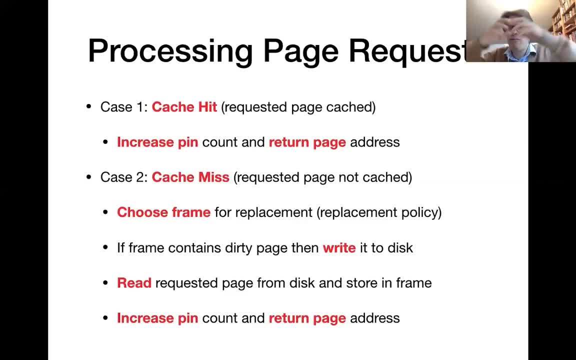 such that they store precisely one page. So you can have many frames, but each of those frames typically stores only one page. All right, And the address of the page that is returned? yes, that would be often the address of that corresponding memory. 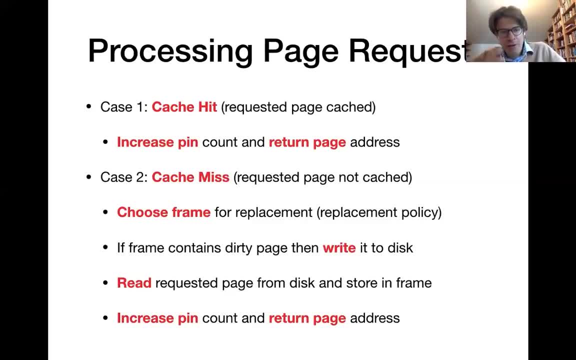 location. All right. So now we potentially had to write the page back to a hard disk in order to persist the latest changes. After we have done that, we read the requested page from hard disk and then we write it into the frame in the buffer pool. 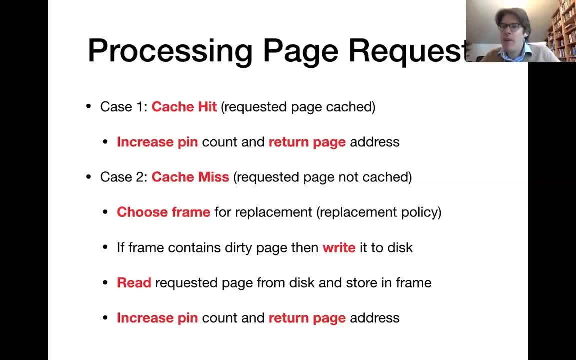 And still, we need to increase the pin count in order to make sure that this page is not suddenly evicted. And finally, again, we return the corresponding address. This is the algorithm. This is the function that the BufferManager executes At this point. you might be wondering whether we couldn't. 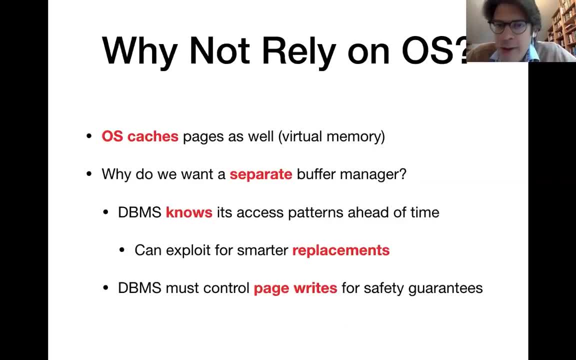 use functionality offered by the operating system. So if you have ever taken an operating systems course, then you will probably have talked a lot about caching. So there is some functionality in the operating system that does something a little bit similar. So the question is, why do we need a specialized component? 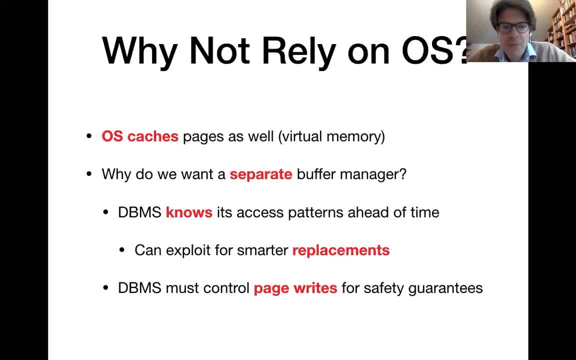 All right. So the question is: why do we need a specialized component for the database management system? And there's two principal reasons. The first reason is that the database management system has often very specific access patterns. So we'll see in the following that the generic strategies 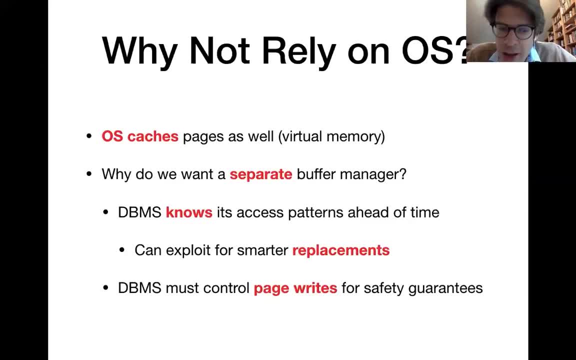 by the operating system often don't work so well for database management system. So a first reason is efficiency, And the second reason is that the database management system is very particular in its access pattern, So we probably want to implement a specialized buffer management strategy. 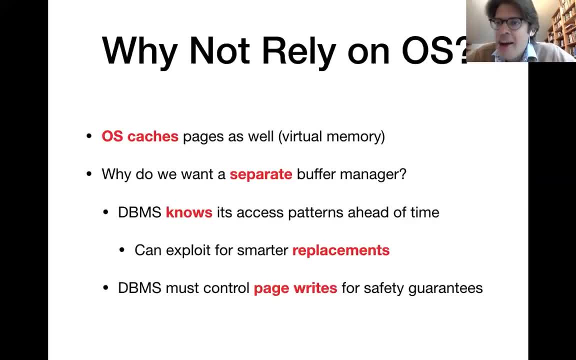 Another thing is that the database management system makes very strong guarantees to users about having data secure, even in case of a server crash. And in order to make those guarantees, which we'll discuss in much more detail later, the database management system needs very tight control over when pages are written back. 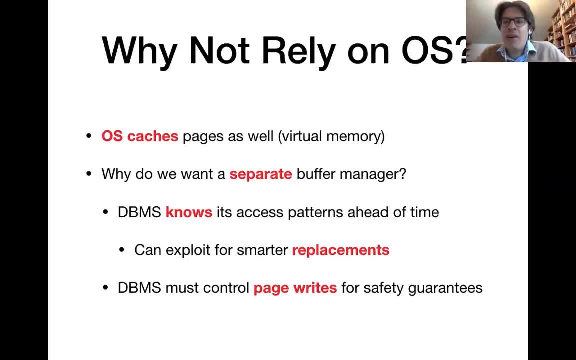 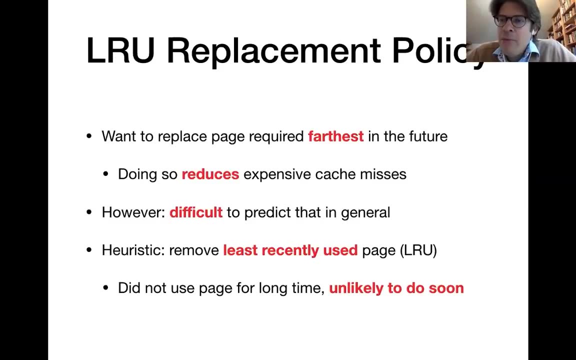 to hard disk or loaded from hard disk into main memory. So it needs very tight control over that in order to make those guarantees, And that is often not offered by those generic components Now, for instance, to make that a little bit more concrete. 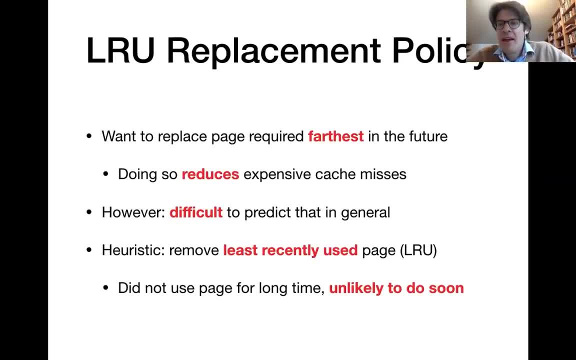 one very popular replacement policy. that's the following: one It's called the least recently used replacement policy. So, in general, what you ideally want from the buffer pool manager's perspective is to always replace those pages in the buffer pool which will not be required. 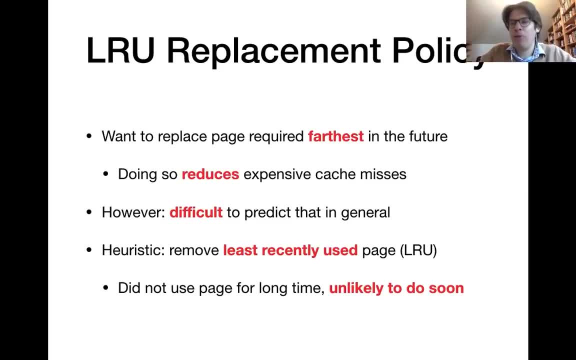 for the longest amount of time. So you want to drop those pages which will not be required for the longest amount of time. That, of course, is difficult. It's difficult to predict in general, So we typically use heuristics, for instance by saying: 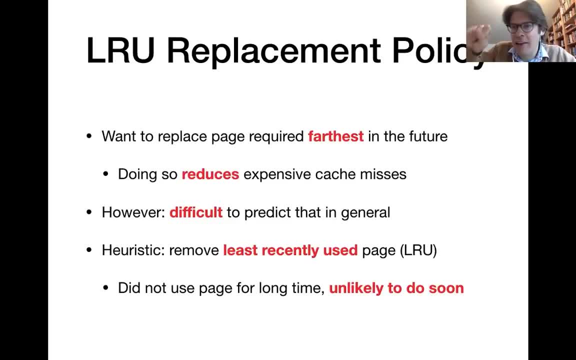 if I haven't accessed one page that is currently in my buffer pool for a long time, then I am unlikely to do so again anytime soon. That is the least recently used heuristic, And it essentially means that if I have to decide where to create space, for instance in the buffer pool, 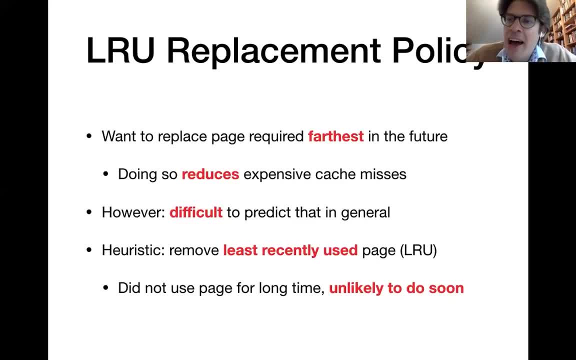 or somewhere in memory In general, then I'm always deciding to overwrite that page which hasn't been used for the longest amount of time. So that is the least recently used heuristic And it is a very popular replacement heuristic used, for instance, by operating systems. 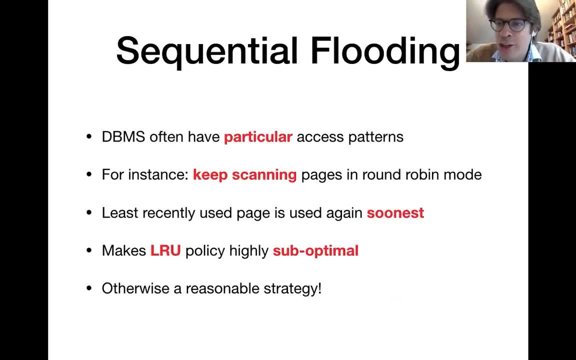 Now one case in which that one works badly, and unfortunately that case is quite common in the context of database management systems, That is, cases where repeatedly, as can the same pages. Now that might seem strange, because why would you read something again after you have just read it? 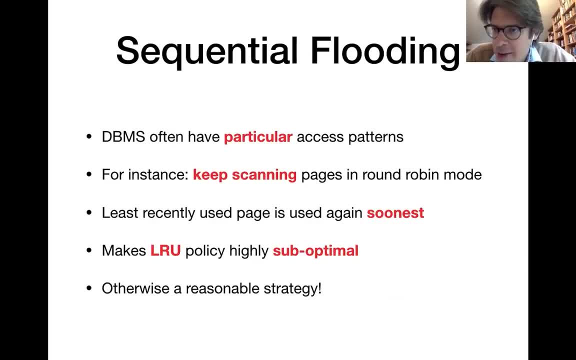 But there is common cases in a database management system where you want to do exactly that. For instance, if I am joining together the relation, the table with the students and the table with the enrollment information, So I'm searching for enrollments matching the students. 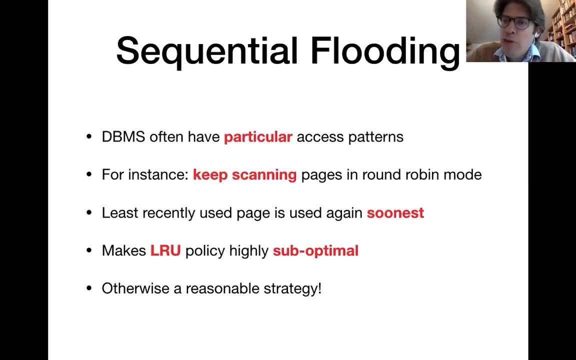 Then one popular way to proceed would be to first load one chunk from the students table into main memory and then iterate over all the pages of the enrollment table in order to find matching pairs. And once we have done that, then we load the next chunk of data from the students table. 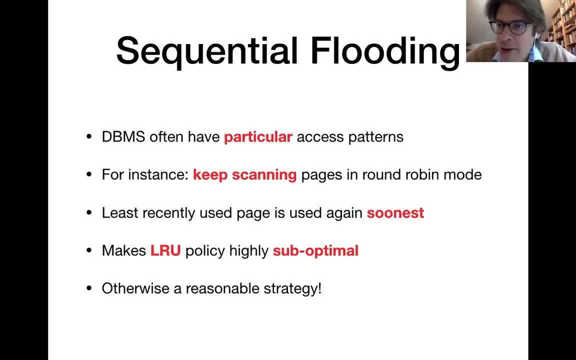 and again iterate over The pages in the enrollment table, And we take the third chunk from the students table and again iterate over the pages from the enrollment table. So this is a case where we will keep iterating over the pages in the enrollment table. 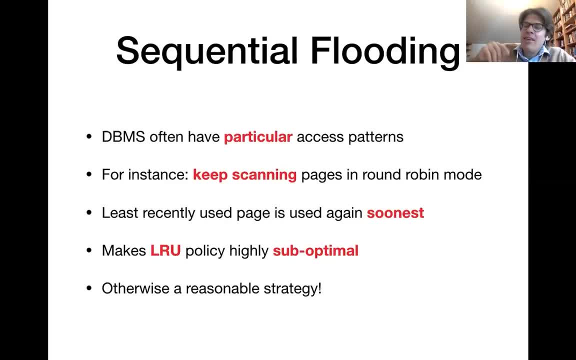 multiple times in a row And here, if we keep repeating, essentially in a cycle, over the pages in the enrollment table, it means that the page that I have not accessed for the longest amount of time is always the page that I will read next. 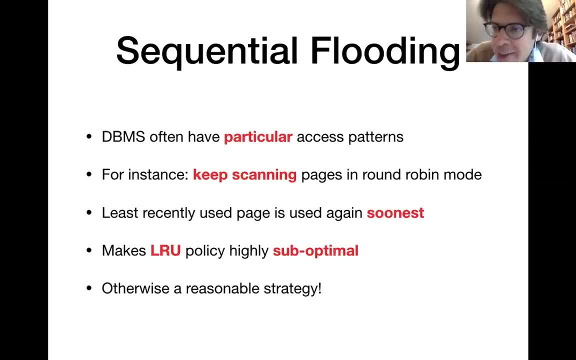 because I'm essentially doing a cycle in the enrollment table And because of that, always deleting the page that I haven't used for the longest amount of time is, of course, highly suboptimal. That is what the least recently used policy does. 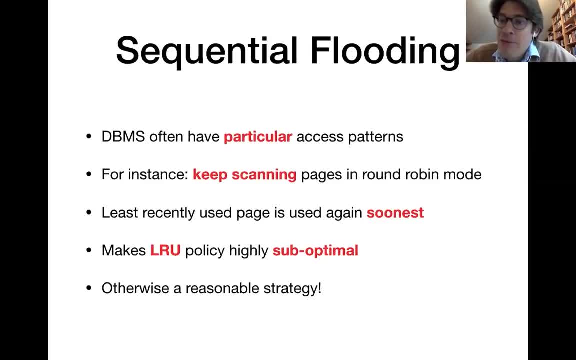 So this is just an example for a policy that seems perfectly reasonable in general, but that's sometimes works very badly in the context of database management systems. So this is a common access pattern for database management systems and to the interplay between that pattern. 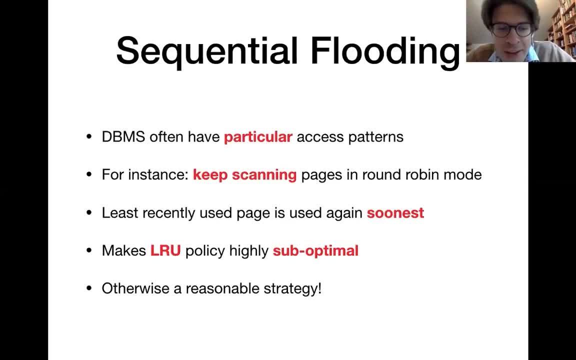 and this policy, the least recently used policy that is also called sequential flooding. OK, And here I have one more question in the chat. OK, What happens if the buffer gets full and no frames can be evicted? Will reads come directly from disk? 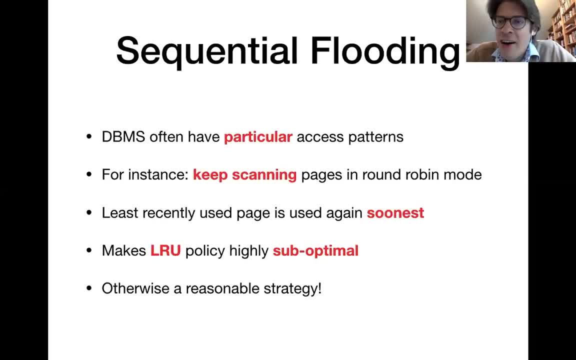 That is a great question. So there might be a situation where I have a pin count greater than zero on all my pages in the buffer pool and then I still have some requests coming in. Frankly, in those cases it depends on the implementation. 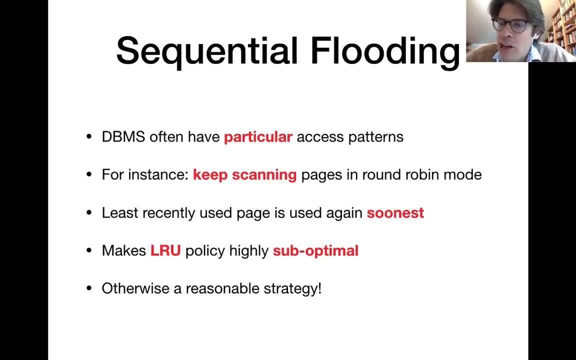 but often the database management system would just essentially reject any further work. OK, Thank you, Thank you. So a lot of times we don't even need to see the data work until the memory situation improves. So I mean, in the end, you always 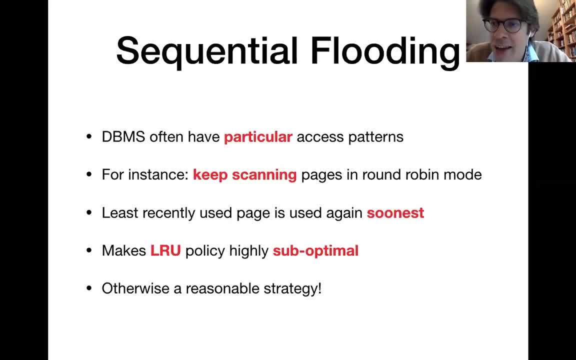 need a little bit of space in the memory to store those pages from hard disk, And if you currently don't have main memory then you probably want to first process the current tasks before you accept new tasks. So the database management system would often reject data requests. 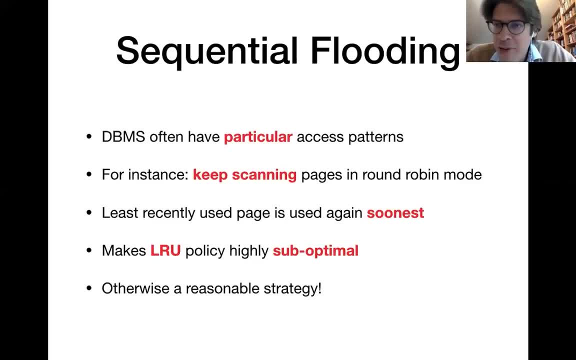 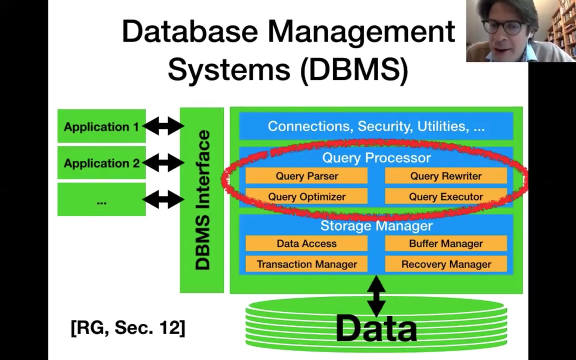 All right, Great question Here: with this example- sequential flooding- we essentially see why using generic buffer strategies for replacement does not work very well in the context of database management systems. All right, So that was a high level overview of the buffer manager. 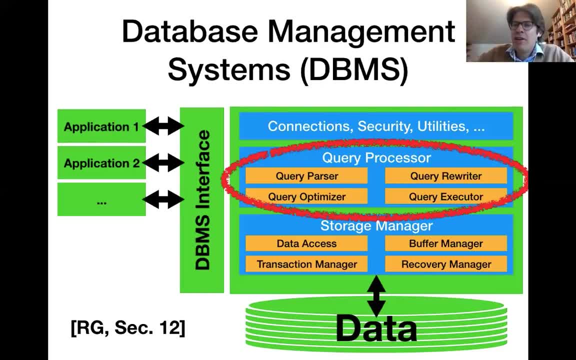 which is the component that connects the hard disk to main memory. Now, in the following, we're gonna start discussing in a lot of detail about the query processor in this and in the following lectures. This is the component here encircled in red. 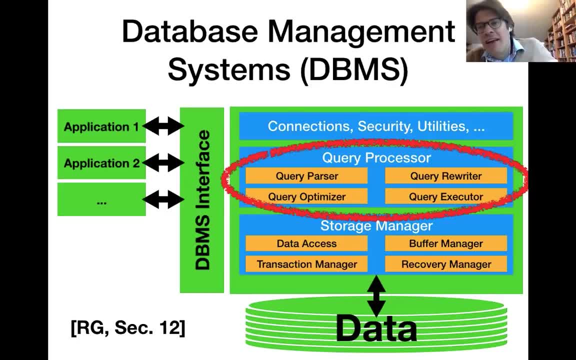 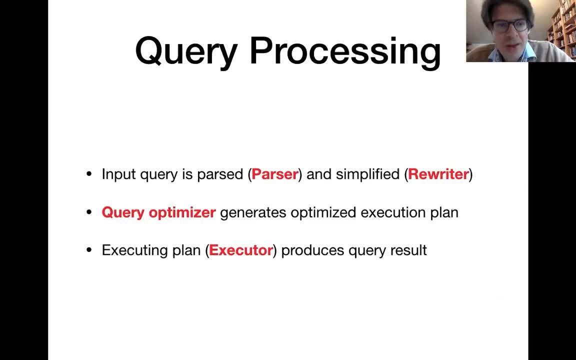 and the associated chapter in the Ramakrishnan and Gyalke book, that is, chapter number 12.. So, at a high level, this is what happens when a database management system is processing an input query. So first of all, your input query is parsed. 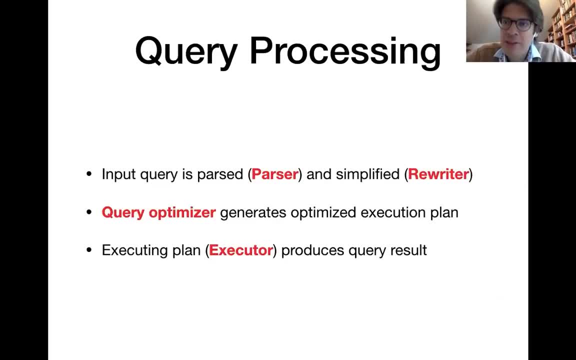 meaning it is internally translated into a tree representation, And then the database management system uses a couple of heuristics in order to simplify that query. This is what the rewriter component does. Now, the query optimizer is more sophisticated than a rewriter. 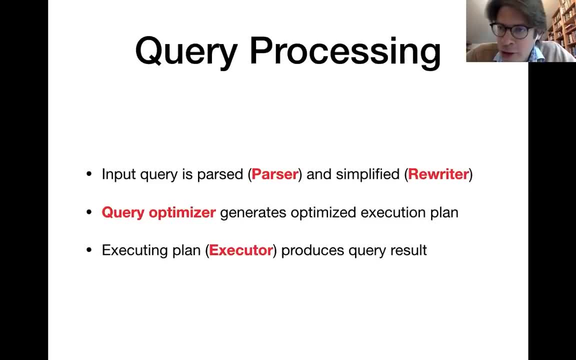 It also changes the query in order to make it more efficient, but it does so using much more sophisticated methods. In particular, it typically tries to predict the execution cost of different plan alternatives, and then it selects the cheapest one. We will discuss about this in much more detail later. 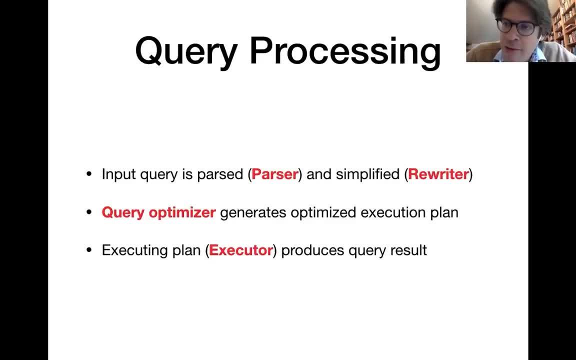 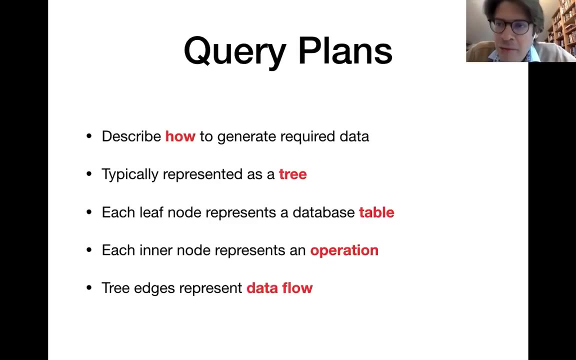 After we have selected a processing plan for the input query, we forward it to the execution engine, which executes it step by step in order to produce the final query result. Now those query plans that are processed by the execution engine. they essentially describe how data is generated. 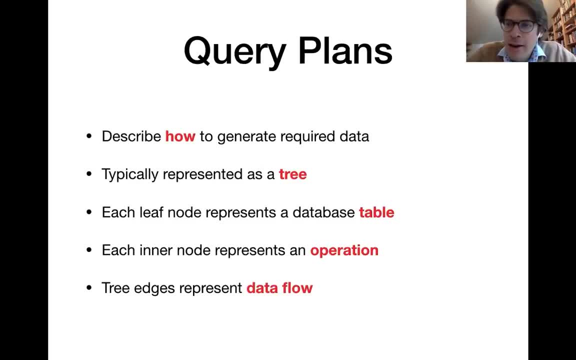 They describe that process step by step. We typically represent them as a tree where each leaf node of the tree corresponds to a data source, to a table. in our context, The inner nodes of the tree: they represent operations and the tree edges connecting different nodes. 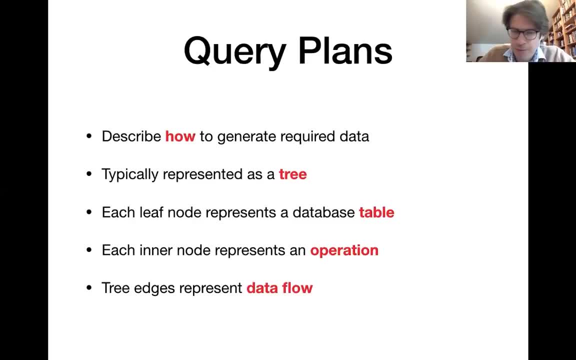 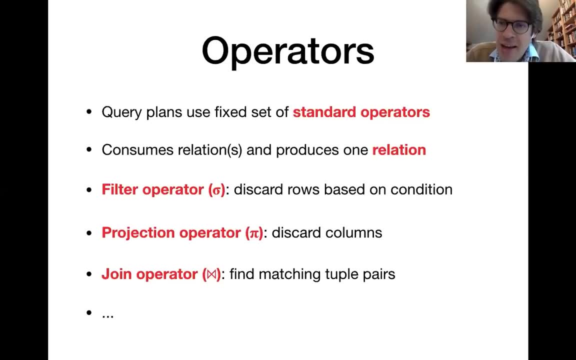 they essentially represent data flow. The inner nodes in the query tree correspond to operations and, in order to process data, database management systems use a fix, which is a set of standard operators. Each of those operators consumes one, or two in case of joins and some other relations. 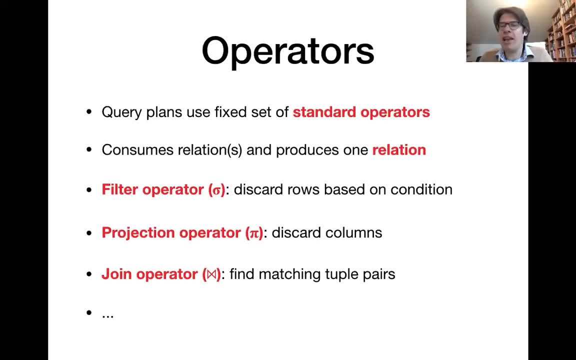 and the output produced by an operator is also a relation. So this is why you can compose those operators, because the inputs are relations and the outputs are also relations, aka tables. So that means we can flexibly compose those different operators together into a tree. 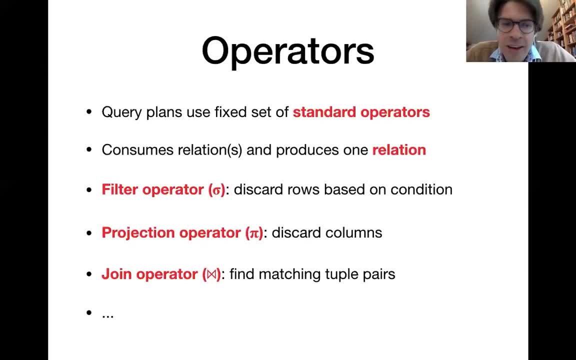 Now, a couple of standard operators that we will be discussing more about is, for instance, the so-called filter operator, which is typically abbreviated by the Greek letter sigma, and that one simply discards rows based on a condition, So it checks for each row. 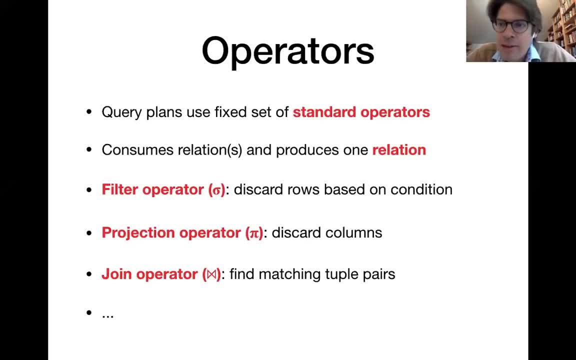 whether it satisfies a condition, and if so it keeps it, otherwise it discards it. Then we have the projection operator, and that one discards columns from a relation. and we have the join operator, which combines two relations by finding matching couple paths. 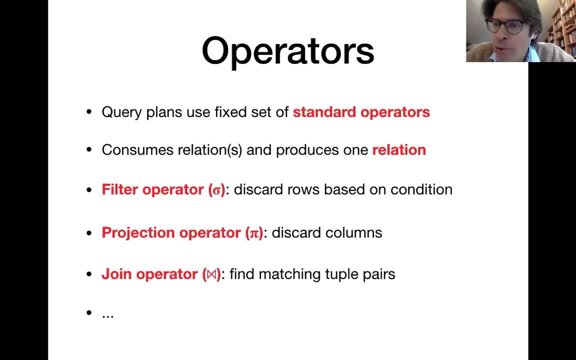 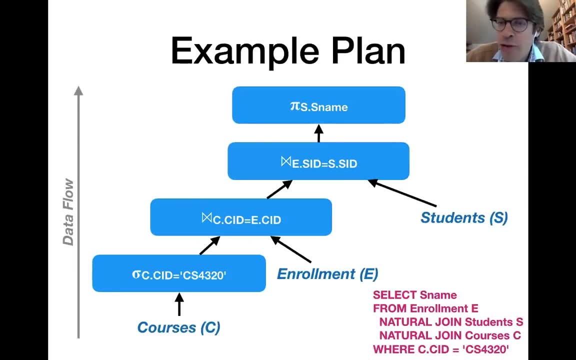 based on some condition and so on. So this is some of the operators that we will be considering And this is an example for one of those operators that, for one of those query plans represented as a tree On the right lower corner of the screen. 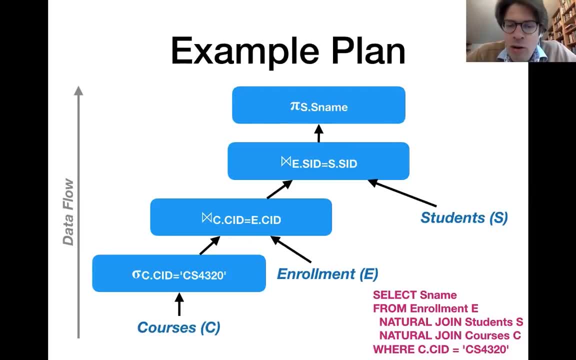 you have the associated query, which essentially combines students and courses over the enrollment information and restricts the focus to the CS4320 course. And finally, it only wants to retrieve the names of the students which are enrolled in that course. So the data flow always goes from the bottom of the screen. 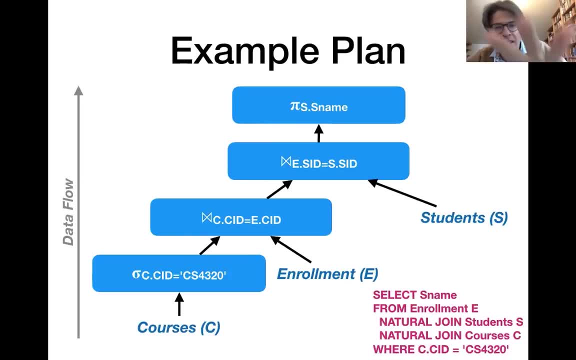 towards the top of the screen. So, in order to evaluate this plan, we would essentially start with the leaf nodes, which correspond to tables that are already available in my database management system. So here, for instance, we can start with the courses that are already available in my database management system. 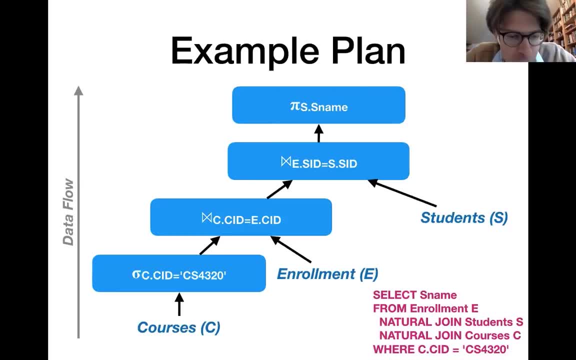 So let's look at the first table And the first operation that is written here, that is, this sigma operator with the condition written as subscript: ccid equals CS4320.. So we are restricting ourselves to the course with that course ID. 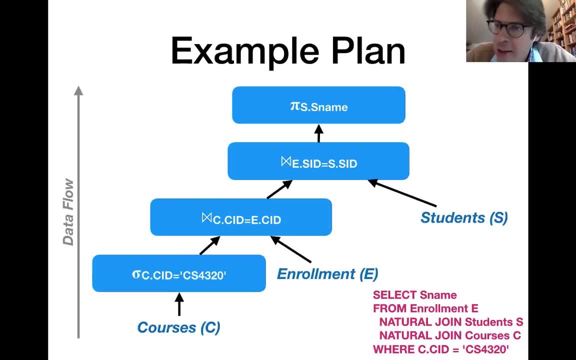 And, as we have seen before, this little sigma over there, it represents a filter operation. After this operator, we will discard all the rows which don't have the course ID 4320,. right Now, the output of the filter operation that is essentially coming out of the top. 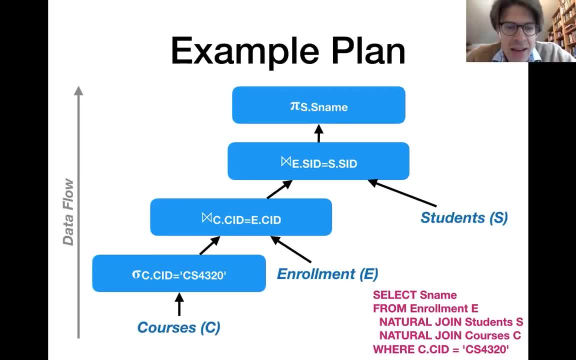 of that operator box in the plan and it is fed into a join operation together with the enrollment table. So this is a join operation. therefore it requires two inputs. And here we are joining those CS4320 course entries with the enrollment table. 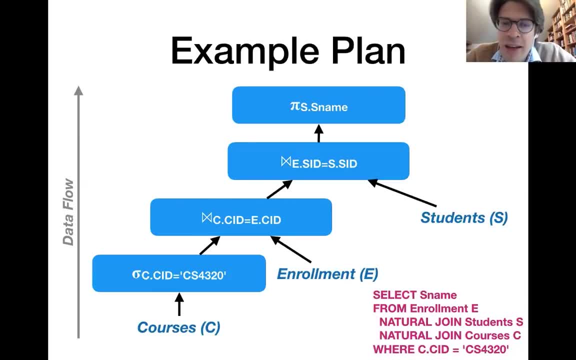 And the result of this join operator that will be the path of matching tables. So here, essentially, I am retrieving enrollment information for the CS4320 course. The next operation is also a join. again, Here I'm joining enrollments. 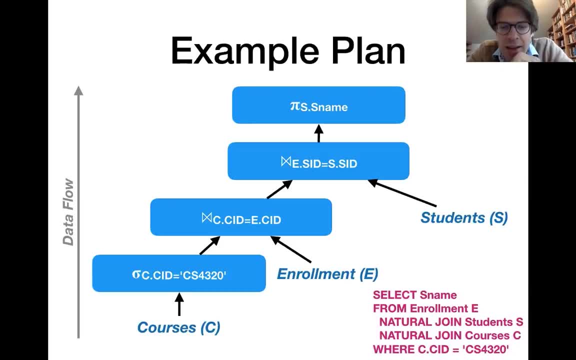 with the associated students And the input to that is the enrollment information for CS4320, as well as the information about all students And the output of that. join will be a path of students together with one CS4320 course they have enrolled in, basically. 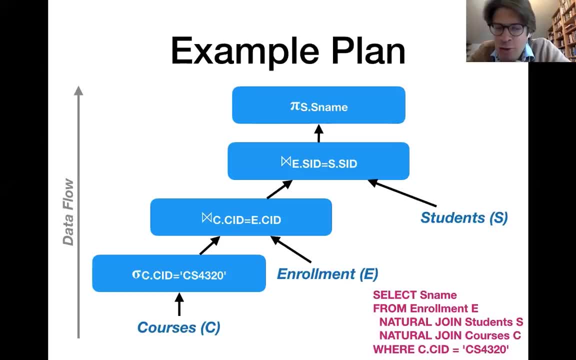 So what I'm ultimately interested in is only the names of the students who were enrolled in 4320, so the final operation, the root of this plan tree, that is, a projection operation with MSDSP. they are essentially discarding all columns except for the one that I have selected here. 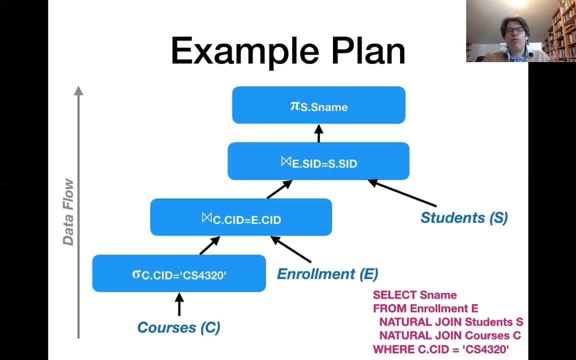 which is the student name, And therefore the output of that plan is the names of the students enrolled in 4320.. And that would be one out of many possibilities to answer the query below. There's different possibilities. For instance, we could change the order. 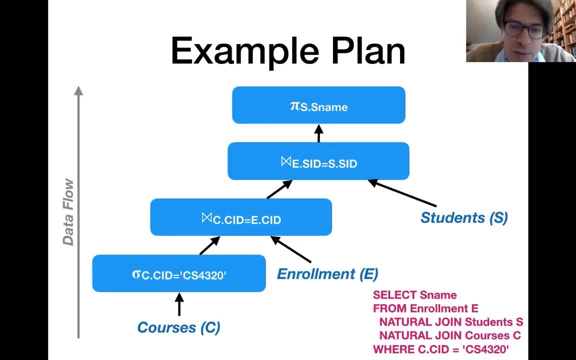 in which we apply the joins, or we could maybe do the projection, Or we could, for instance, do the filtering later in the plan tree. So there's different possibilities how I can process the query. All right, And there's some question in the chat. 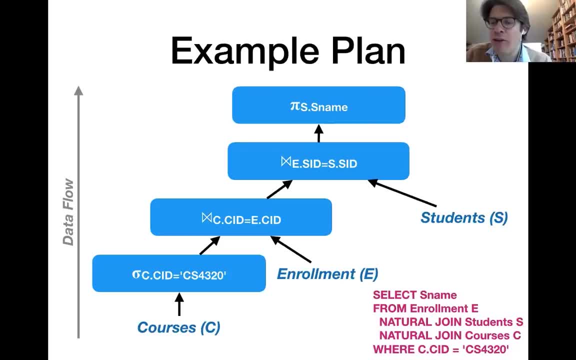 about whether there's operators for adding columns or rows as well. So of course your database management system internally has some operators in order to add rows. It also has operations that allow you to add columns to a table. But in the following we're going to first of all 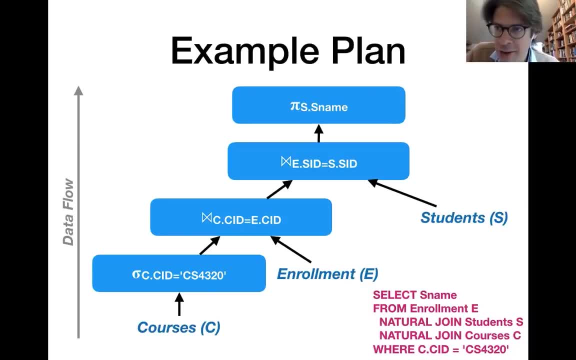 focus on processing queries which do not change the data. Later in the course, we will also discuss transactions which might actually update your data, And there's a couple of new issues that arise in this context, So we will discuss about that. For the moment, we only discuss about queries. 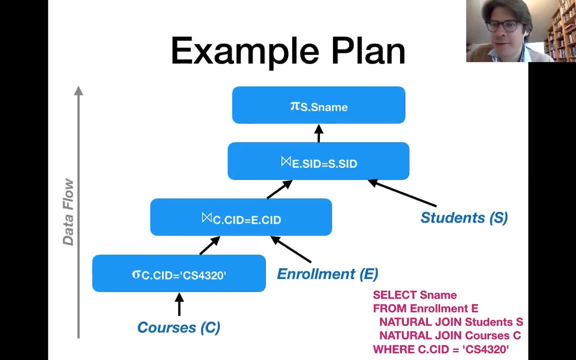 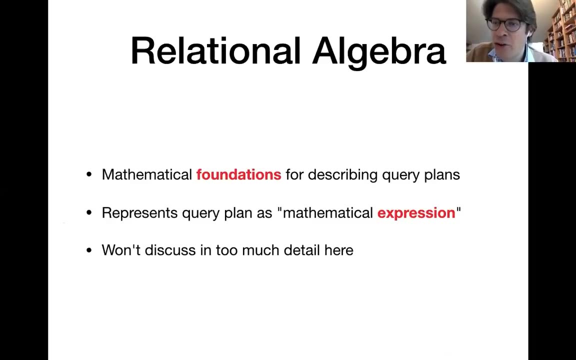 that analyze your data? Great question, All right. So this is an example query plan that I wanted to show you Now, the mathematical foundation for those query plans that is called relationship. It's called relational algebra. I'm not gonna discuss relational algebra in too much detail. 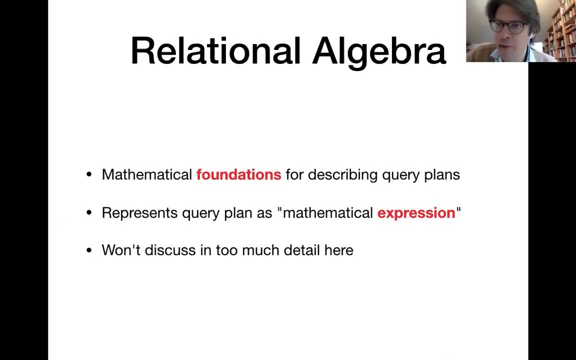 but I wanted to point out that connection. You can also find more details in the Ramakrishnan and Gacke book. So essentially relational algebra is a mathematical version of those query plans. It essentially represents a query plan as a mathematical expression. 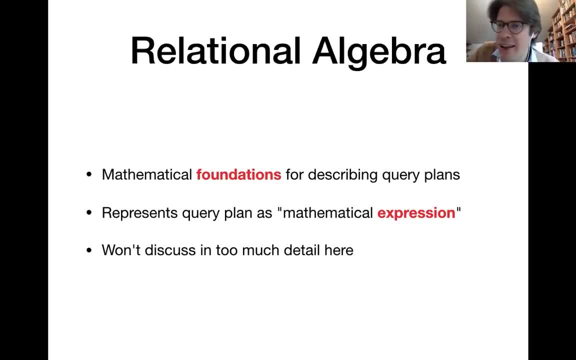 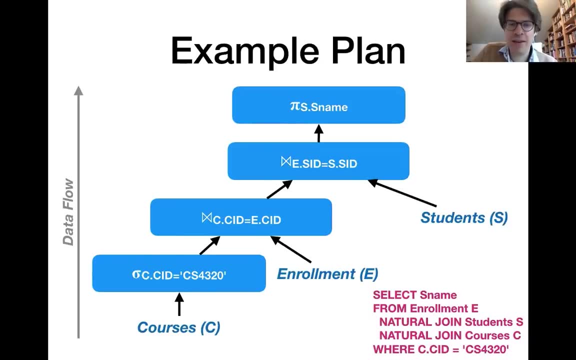 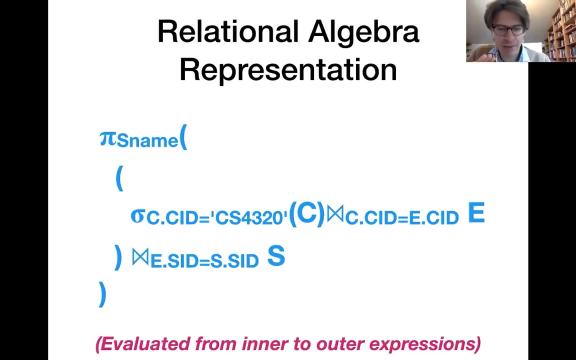 And just to show you how we would represent the plan, like the one we have seen before in a relational algebra. So this plan that we have just seen. if we want to represent this as a relational algebra expression, this is how it would approximately look like. 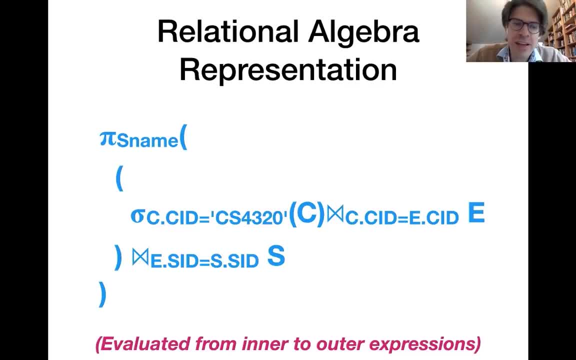 So those relational algebra expressions, as you see, they use the same symbols for the operators that we have also used in the plan tree. Yeah, in a way a more concise way of representing those plans as expression rather than as tree. 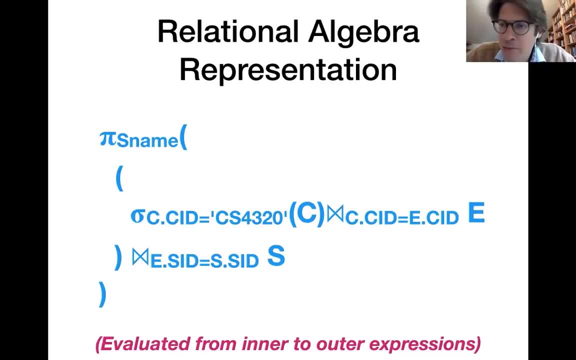 The semantics is that we start evaluating those expressions from the inside and then we work our way towards the outside. So here we would first start with one of the innermost expressions, which would be this filtering operation applied to C, which is the courses. 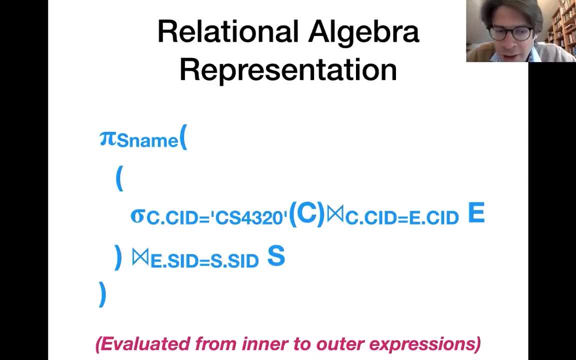 Then next would be, for instance, the next would be the join on the course ID, And then we would join the reside of that with the student ID And finally we would apply the projection. So it's the same thing but represented differently. 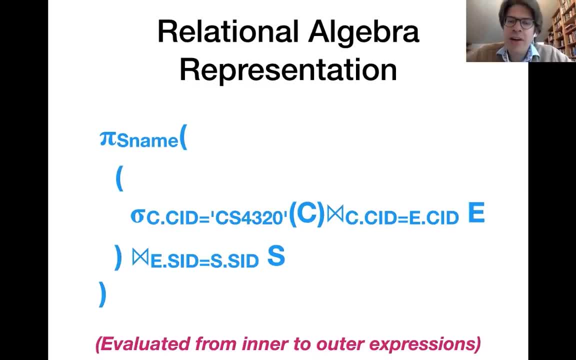 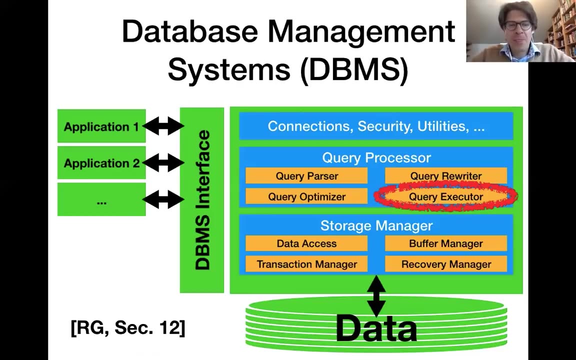 So I'm not gonna go too much into detail, but I wanted to show you one relational algebra expression at least and explain how that relates to query plans. All right Now. this was a high level overview of a query processing. Now, in the following, 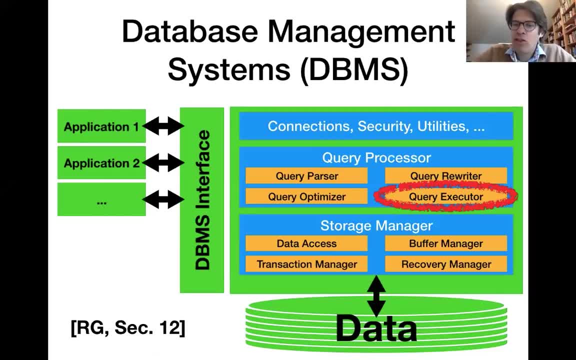 we're gonna discuss a little bit more about the different components of the query processor, and that will keep us busy for a couple of lectures. Now, in the following, we're gonna start talking about the execution engine. Now, in the following, we're gonna start talking about the execution engine. 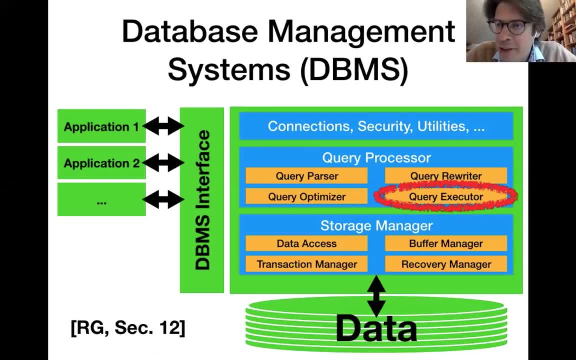 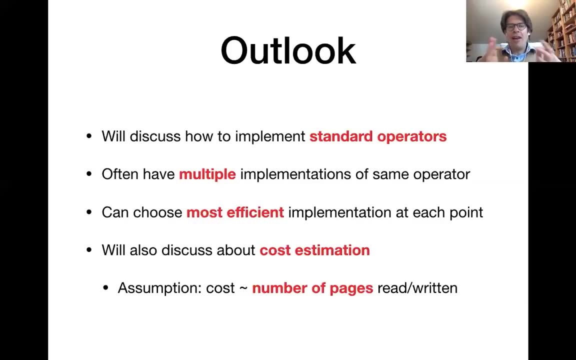 because in order to understand, for instance, how the query optimizer makes the choices and so on, you first need to understand how query plans are processed in the execution engine and what the performance trade-offs are. all right now, the first thing we will be discussing about is how we can. 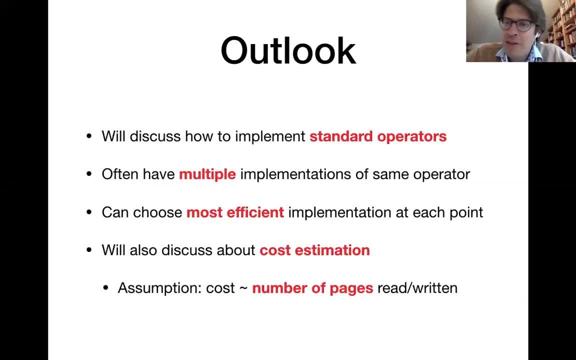 actually implement those standard operators that you have just seen. i told you that database management systems. they use a set of standard operators in those query plans and typically for each of those standard operators, like the join for instance- you would have not one implementation but many alternative implementations, and this is what allows the database management system. 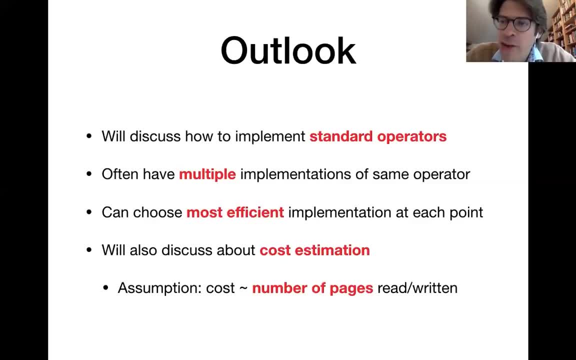 to choose in each situation, that implementation which is most efficient, right. so that is the reason why you want to have different implementations for each. you want to have different implementations for each case. you have an implementation that is just right for that specific case. so we will discuss about a couple of different algorithms. we will also discuss about how to 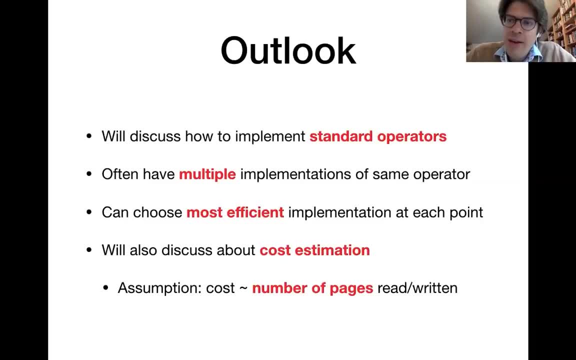 estimate the processing cost for those algorithms because some of those algorithms that we will be discussing, they might seem a little bit unusual at first and in order to understand why they are designed the way they are designed, we will discuss about how to estimate the processing cost for. 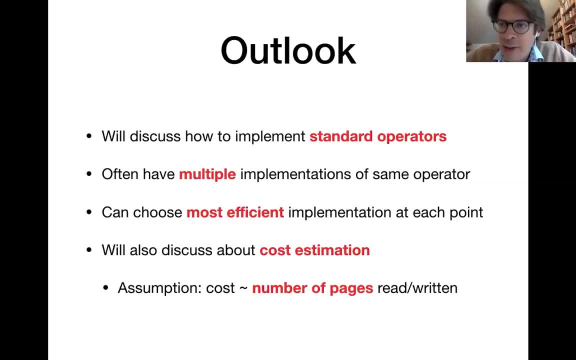 those operators, because otherwise those algorithms won't make sense. so we will discuss about the implementation and about a cost estimation. we will use a very simple cost model in the following. it is simply based on the number of pages that need to read from hard disk in order to execute. 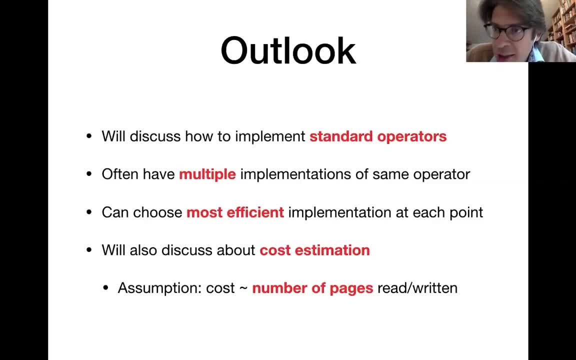 an operation. now, that is, of course, a simplifying, but it is a very simple model and it is a very simple model and it is a very simple model. any part of experiments that take place and that areいただ by existing, you don't. you don't get this idea or, you know, understand their. 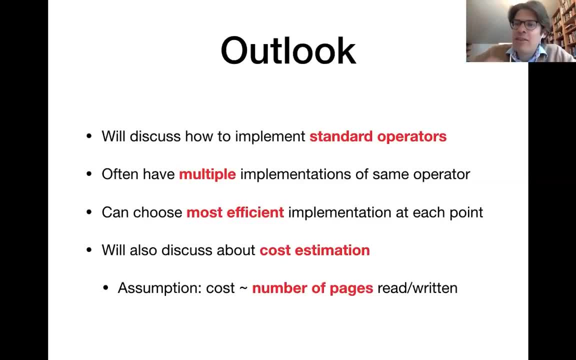 empathy. we will deal with, let's say, someuent also have some overheads, due to the actual processing, for instance, but data movement overheads often dominate total processing costs in those situations And that is why we will simplify by estimating cost as the number of pages that have been read or written to hard disk. 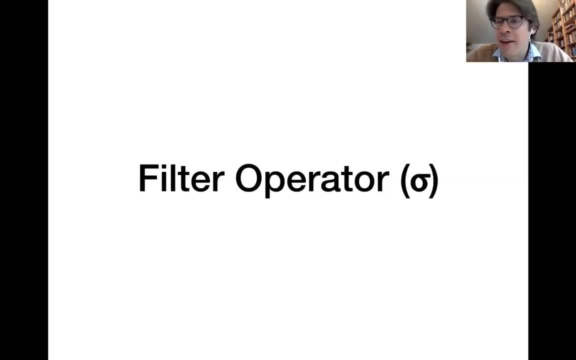 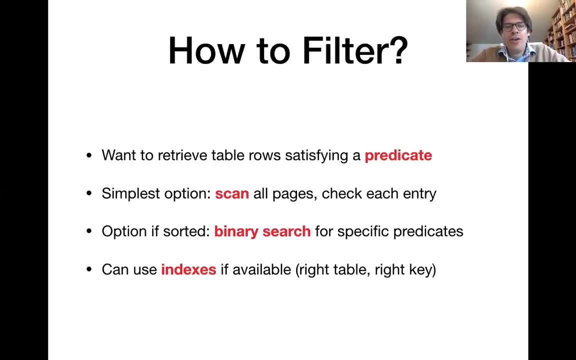 The first operator that we start discussing, that's the filter operator. The corresponding algorithms are simpler than, for instance, for the join algorithm, but we will see that there's already a lot of different ways of executing a filtering operation. So in general, when we filter, we want to retrieve rows that satisfy. 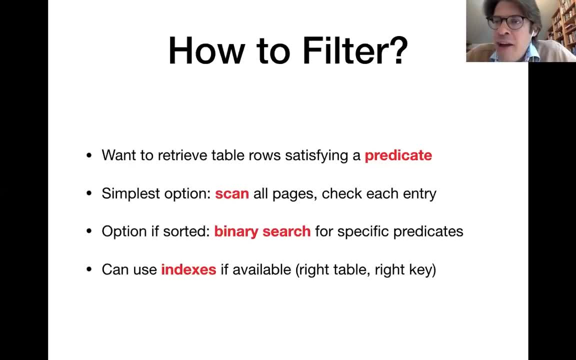 a certain predicate, And in theory there's different ways to go about that. The simplest possibility is that I just scan all pages of the corresponding table, And then I can just go back and do the same thing over and over and over again. And then I can just go back and do the same thing over and over again, And then I can just go back and do the same thing over and over again, And then I can just go back and do the same thing over and over again, And for all the entries. 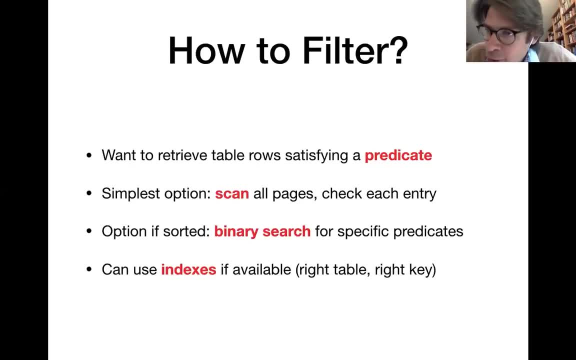 on each page, I check whether they satisfy the predicate or not. If they satisfy the predicate, then I add them to the output. That is the simplest alternative. Now, if I know, for instance, that my data is sorted according to a column that appears in the predicate that I'm interested in, 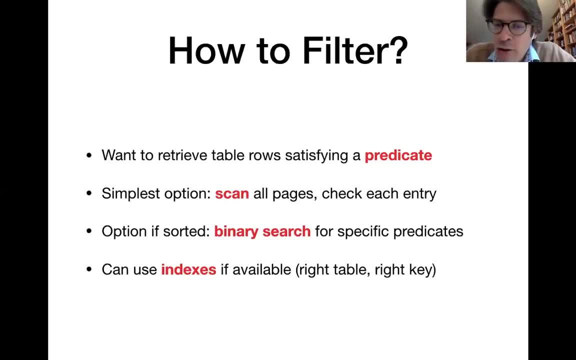 for instance, I'm searching for information on one specific course and my data is sorted by courses. Now, if that is the case, I can typically do something smarter And I can apply some kind of binary search. as we have already quickly discussed in the lecture on indexes, I can use some binary. 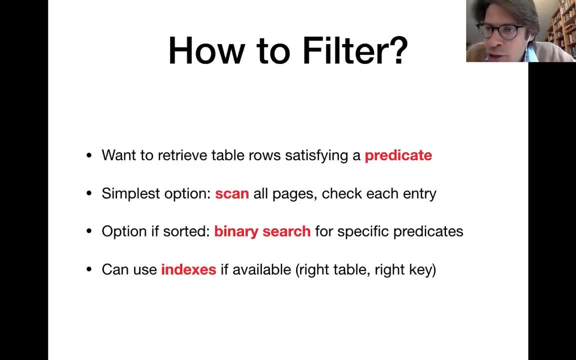 search in order to quickly identify the page on disk where the information, where the first entries for the course I'm looking for, are located. So that is often already more efficient And, of course, if indexes are available for the right table and for the right predicate and right type of index. 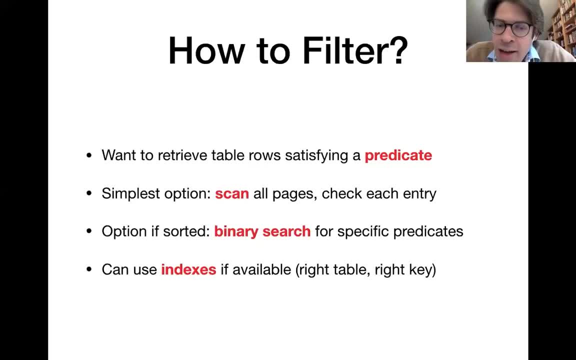 all of that. in those cases, I can use indexes in order to find the data faster, depending on the properties of the data and of the index. All right, So that is the high level outline In the following. we're going to make that more concrete and estimate processing costs. 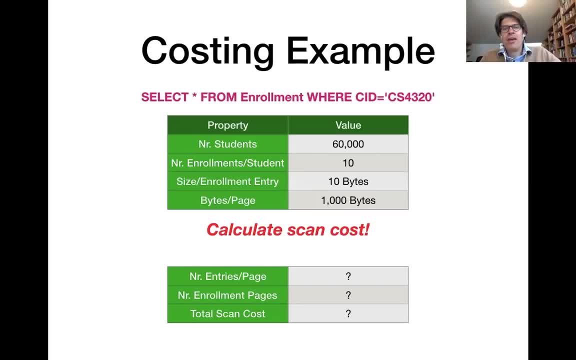 for those different alternatives. Now let's start with a simple or with an example here. So what we want to do is to retrieve enrollment information where the course ID equals 4320. again Now, in order to get a hang of a cost estimation, I give you a few minutes in order to try to figure. 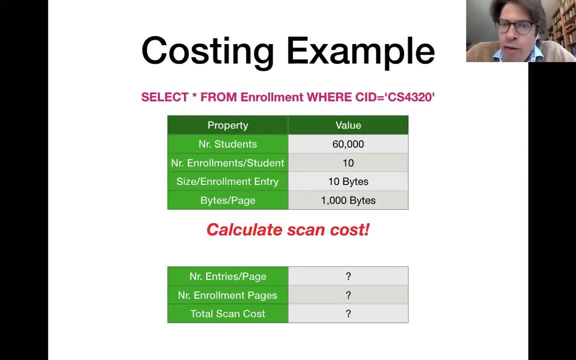 out how we can compute the cost for scanning the enrollment relations. So that would be the simplest way for executing this filter operation. Now, here on the upper half of the screen, you have a couple of numbers that are helpful in order to calculate that. For instance, 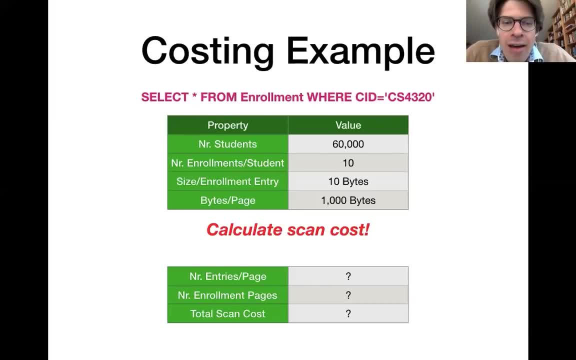 you have the number of students given, You have the number of enrollments per student, You have the size per enrollment entry And you have the number of students that are given, the number of bytes that we can use per page. Now take a minute to think about. 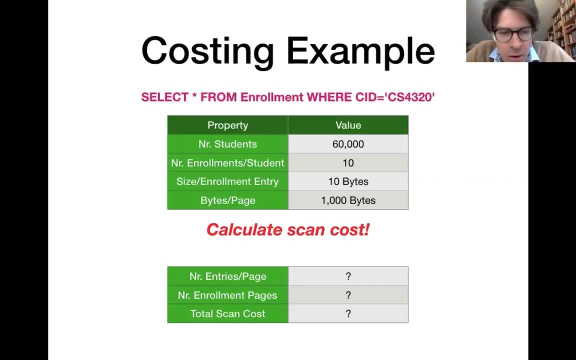 how you would fill in those fields on the bottom of the page. In the end, the goal is to estimate the scan cost, but in order to make it a bit easier, I have essentially given you a different intermediate numbers that you probably want to calculate in order to get there. First would calculate the number of 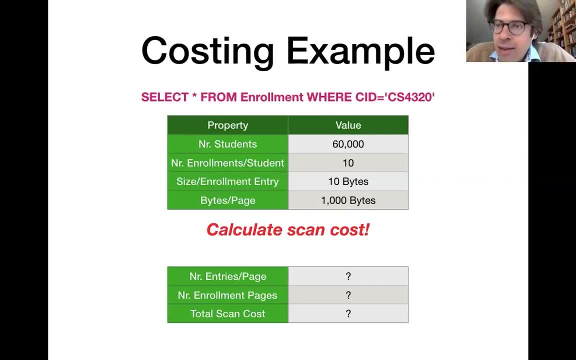 entries that you can fit on one page and derive from that the number of pages of the enrollment table, and from that you can quite easily derive the final cost. I give you a minute and if anyone has questions beside that, please write them in the chat. 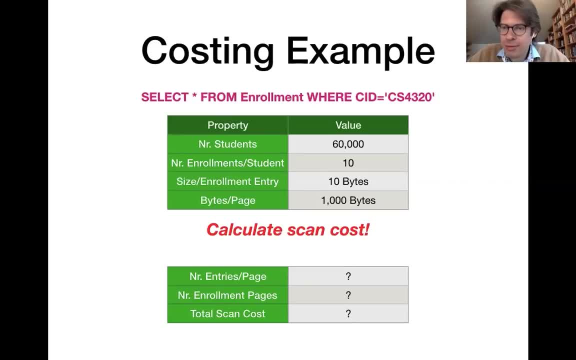 Thank you. So this cost estimation is something that the query optimizer would typically do in order to decide on the most efficient way for accessing a certain table. There doesn't seem to be any questions for the moment. All right, I think I can directly resolve it here. 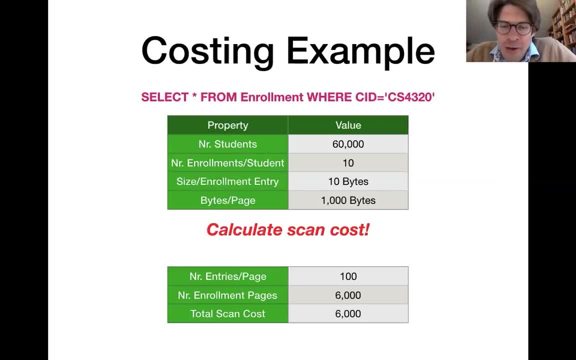 All right. so first of all, we typically want to estimate how many entries we can fit on a page in order to calculate cost, And this is something that we would typically want to estimate: how many entries we can fit on a page in order to calculate cost. 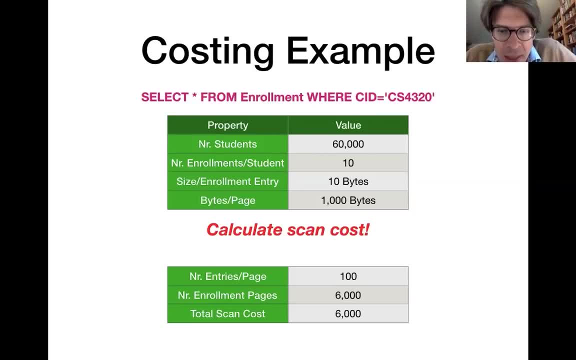 And that depends on the page size as well as on the entry size. Here we have a thousand bytes per page and each entry uses up 10 bytes, so we can fit a 100 entries on each page. And since I have 60,000 students and for each student I have 10 enrollments, that makes 600,000 enrollment entries. 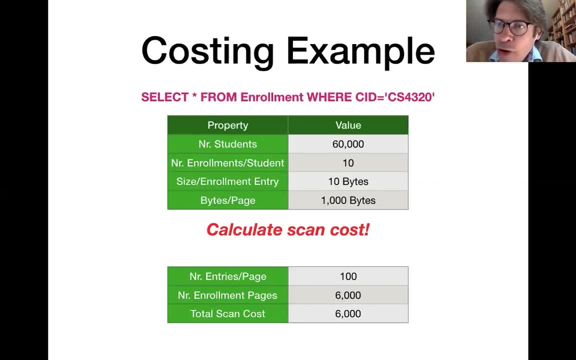 I can fit a hundred of them on one page. So if I divide one by the other, I will end up with 6,000 pages. And since I'm simply scanning all the pages and since I'm calculating cost as the number of pages accessed, 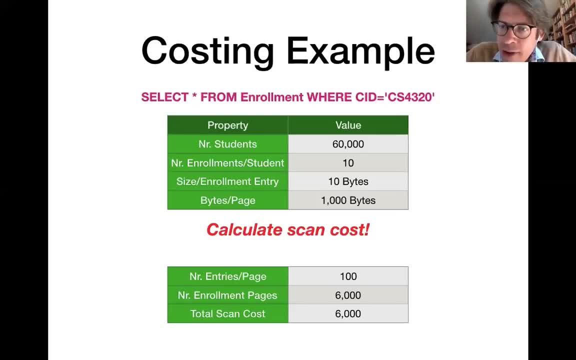 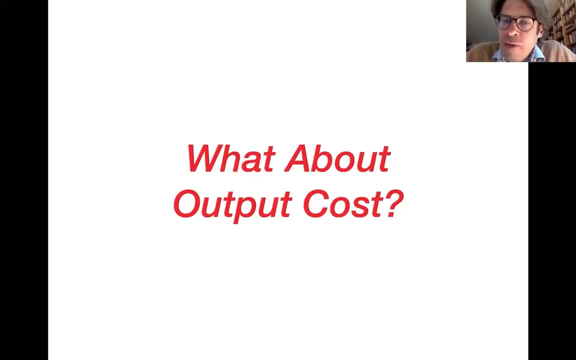 that means that here I have a cost of 6,000 page accesses. All right Now. perhaps some of you are wondering about the cost. All right Now. perhaps some of you are wondering about why we don't count any cost for, for instance, 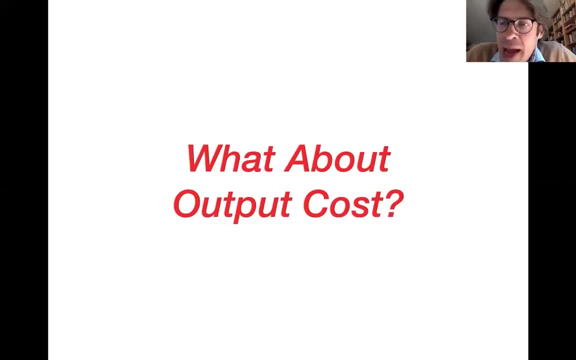 writing the output of the operation back to hard disk or anything like that. Does anyone have an idea why we are not considering the output cost? So then please put it into the chat. Yes, Okay, Some good propositions coming in here. Yes. 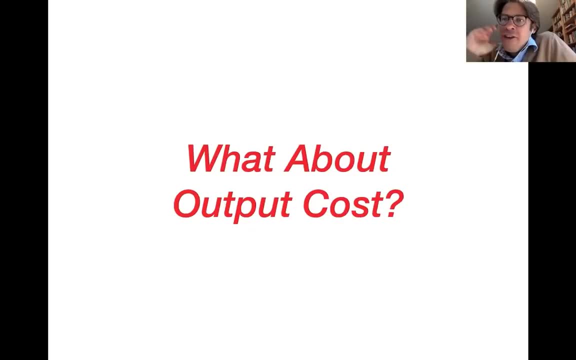 Okay, All of these are possibilities. Yes, Exactly So I mean, in a way, the output cost essentially okay. bottleneck is on the scanning. Yes, That is true as well. Yes, Okay. So all of those are great points. 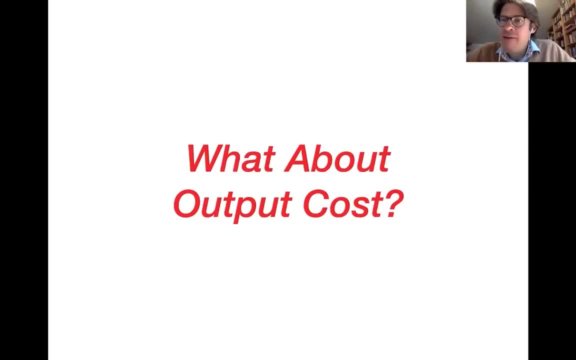 And also if you think about the way in which the cost information is typically used. typically, you calculate cost in order to choose between different operations for the same query. Why doesn't it make sense to consider the output cost in order to choose between different alternatives? 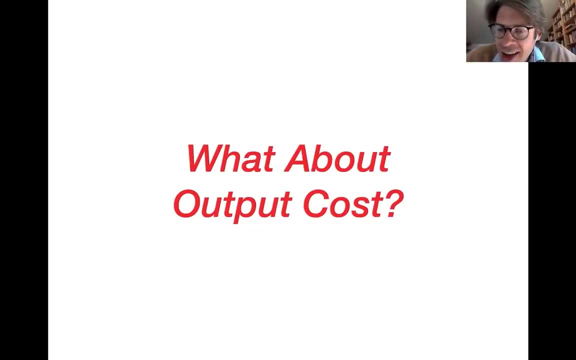 Exactly Yes, So in here. so all of those are great points. by the way, And I mean perhaps the main reason in practice why we don't consider the output cost when using cost to compare different alternatives is that, since all alternatives answer the 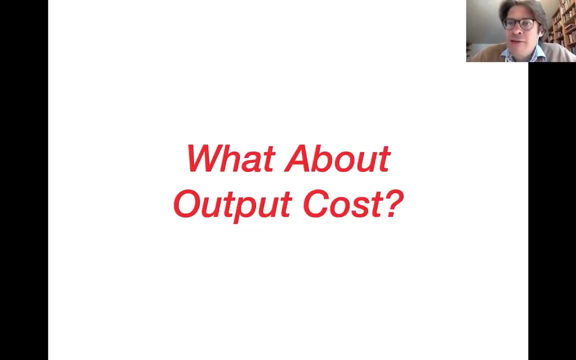 same query, all of them must produce the same output. that is why the cost for processing the output is essentially a constant. Okay, And so that is why, when calculating cost, we typically neglect any cost that is associated with the output that an operation is producing. 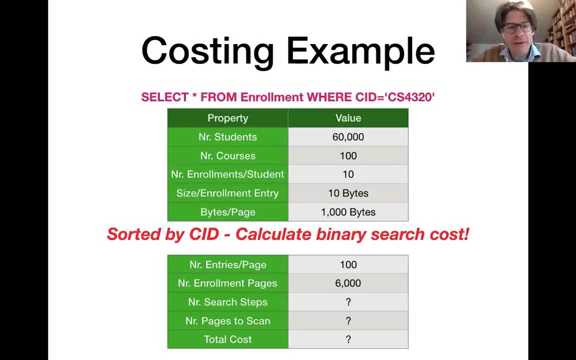 All right, Very good. Now let's consider cost for the second alternative that we have seen. We have the same query, but this time we assume that our data is sorted by the course ID, and that is helpful, because then we can do a binary analysis. 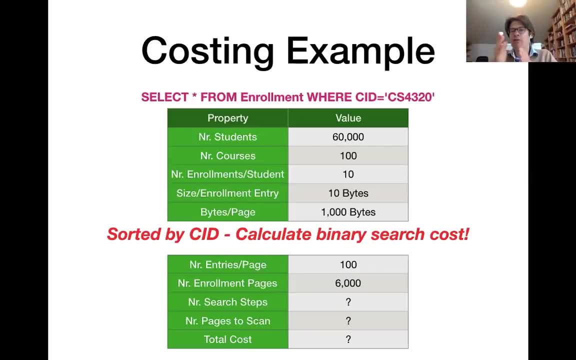 Okay, So we can do a binary search. So via binary search we would essentially search for the first page containing the CS4320 entries And then, starting from there, we would scan all data in order of pages until we find the first entries that are not for CS4320 anymore. 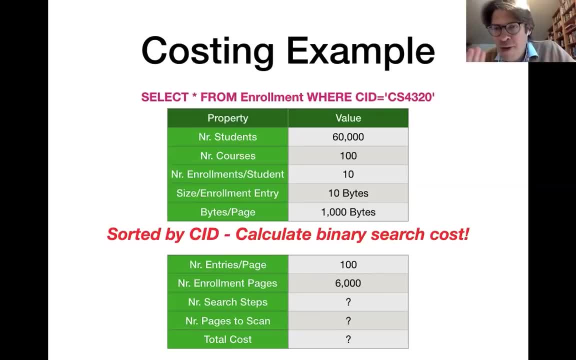 So again, I give you a minute before resolving the example. Here you have again the information. on the upper half of the screen We have the number of students, the number of courses- That information is new because now we need it- And the number of enrollments per student. 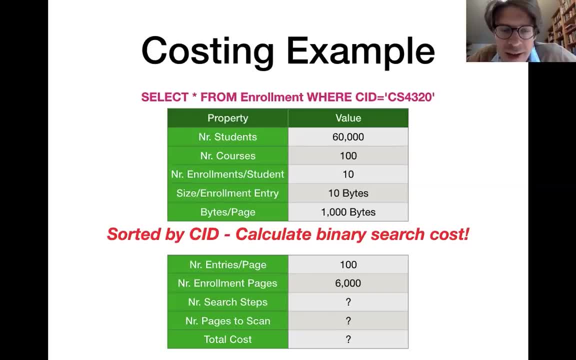 Again the size per entry and the number of bytes per page. All right, And here on the bottom We have already the number of entries that you can fit on the page. We have the number of enrollment pages Now I would recommend you to first calculate the number of search steps executed by binary. 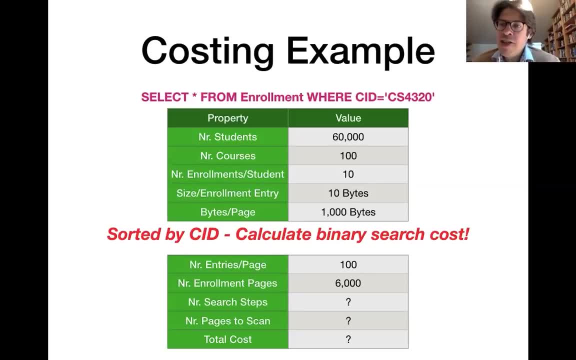 search, Then to calculate how many pages we scan, starting from the first page after binary search has been finished, And from that you can quite naturally derive the total cost. Give you a minute. If there are any questions, please put them into the chat. 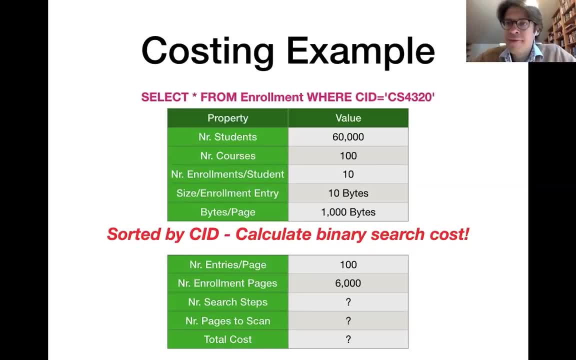 Thank you all, Thank you all very much, Thank you, Thank you, Thank you All right. so even if you didn't have yet time to do all the calculations, perhaps you had some time to think about how you would do those calculations. and let me resolve this. 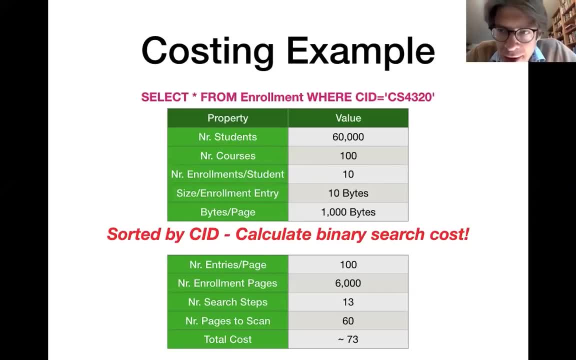 So, since we are executing a binary search, the number of search steps is given by the logarithm of the number of points. So in each search step you're looking at a page and you're deciding whether the entries you're looking for are located to the left or to the right of that page. basically, 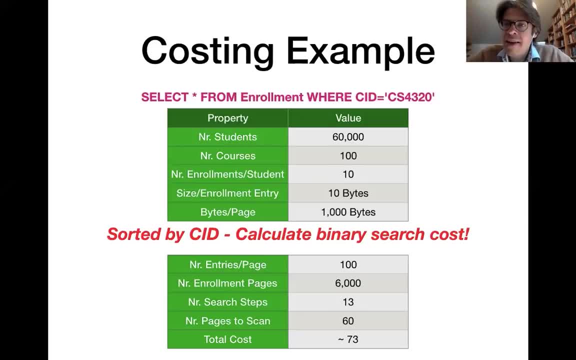 So in each search step we are essentially dividing the range of pages that we are interested in by a factor of two, And that means that if I want to find one page on 6,000 pages, then after 13 steps I will have definitely narrowed it down. 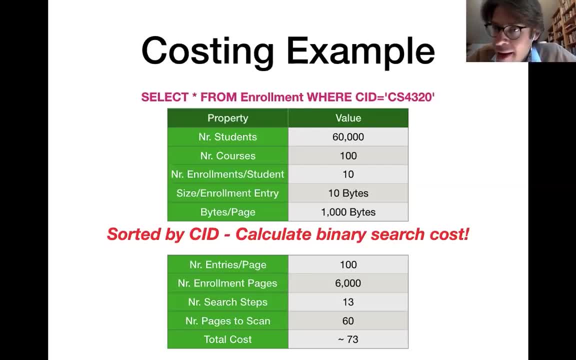 And that means that if I want to find one page on 6,000 pages, then after 13 steps I will have definitely narrowed it down to one single page, and then I know where I can start my scan. Now, the number of pages that we scan, that essentially depends on how many entries I have for the CS4320 course. 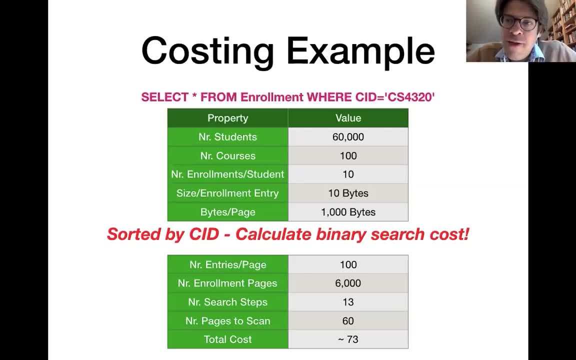 Now here, the information that I have given you is that we have 100 courses. so we can estimate that if we have 60,000 students, 10 enrollments per student makes 600,000 enrollment, And if I have 100 courses, then I can assume that in average, I have 6,000 enrollments for the CS4320 course. 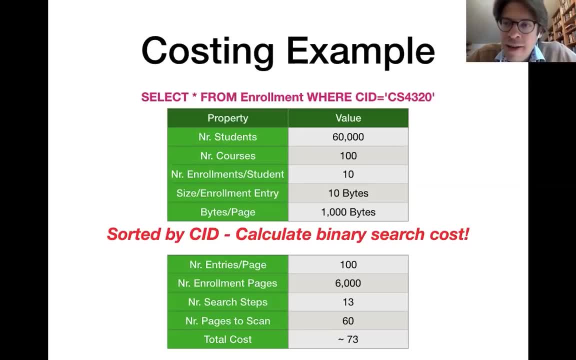 And since I can fit 100 entries on each page, 6,000 divided by 100 is 60 pages, so I assume that the result to this query contains 60 pages, And this is how many pages I need to scan after I have 100 entries. 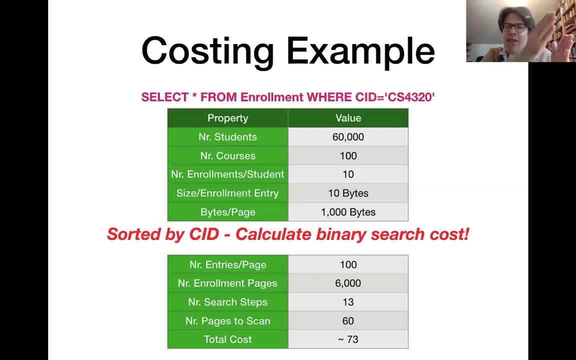 So I have found the first page from which to start the scan via binary search, And then, in order to get the total cost, you just have to count together the access cost for those two different phases of the algorithm. Then you end up with something which is already significantly cheaper than what we have seen previously. 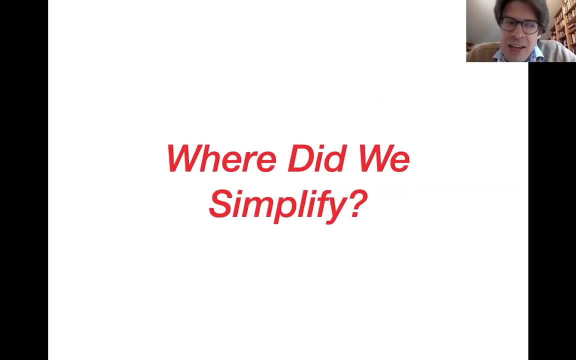 Now, one question to you would be where we have used the simplification. I think I'm just going to answer that question for you. For instance, one way in which we have used simplification here is that we have assumed that we have the same number of enrollments for each course. 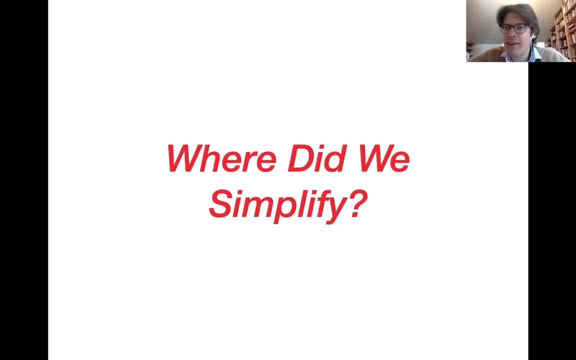 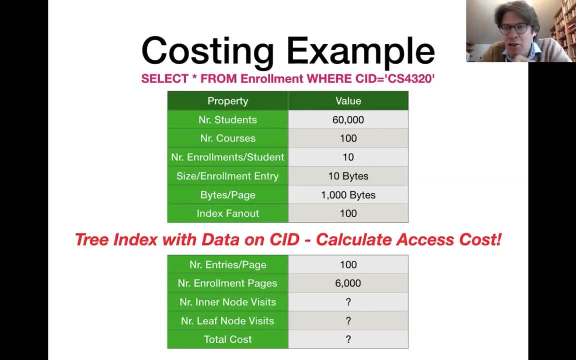 Because we simply said we have a total number of enrollments and we are dividing that by the number of courses to get an estimate for how many enrollments we have for each course the index has, and then I recommend you to estimate the total cost by. 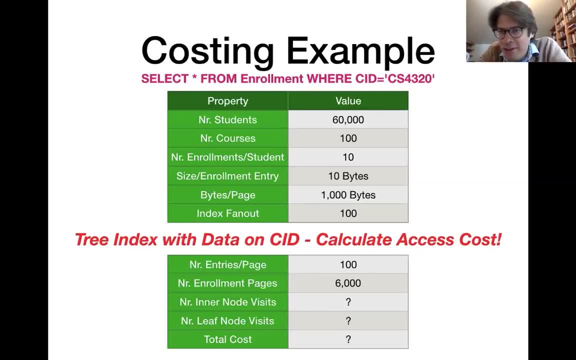 calculating the number of inner nodes that you visit in the index, the number of leaf nodes that you visit in the index, because each node corresponds to one page axis- and then finally, to calculate the total cost. all right, so we have reached the end of the lecture. I hope you're having a nice day and I see. 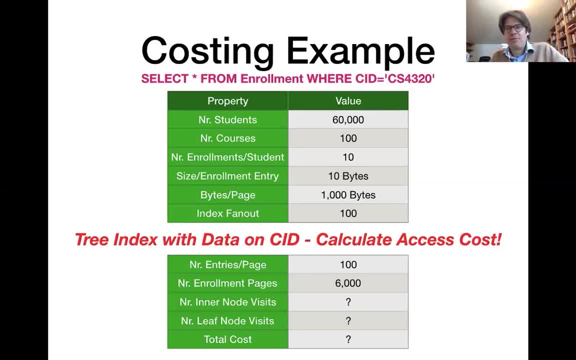 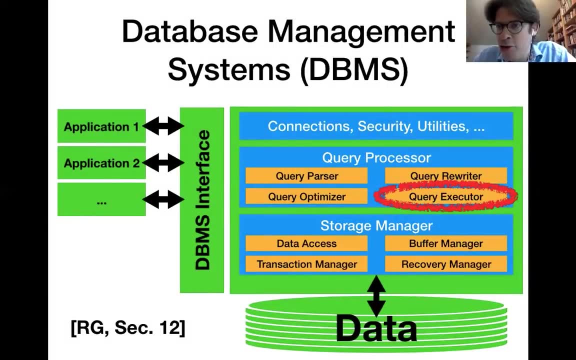 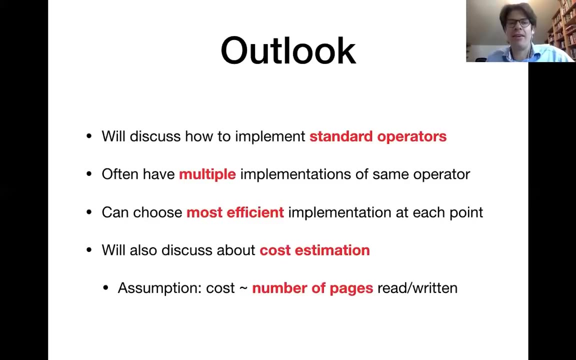 you again on Wednesday. so for the moment we are discussing about the query execution engine, the relevant chapter in the Ramakrishna Nagarka book, that is chapter 12, and we have started already last time discussing different operator implementations for the standard operators because database management systems. they execute your queries by a sequence. 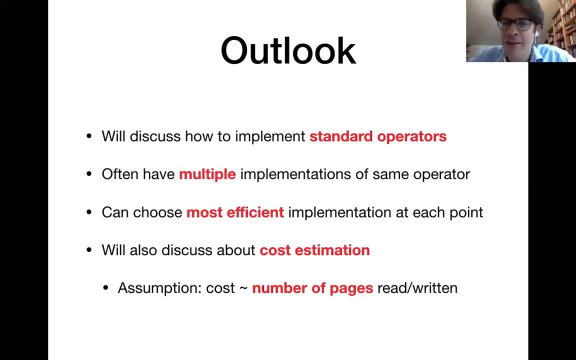 of steps where each of those steps is one of the standard operators, and for many of those standard operators, such as filtering something or joining two tables, you actually have many alternatives, implementations for the same operation, and that enables the database management system to always choose the most efficient one. now, in order to understand why those algorithms are defined the way, 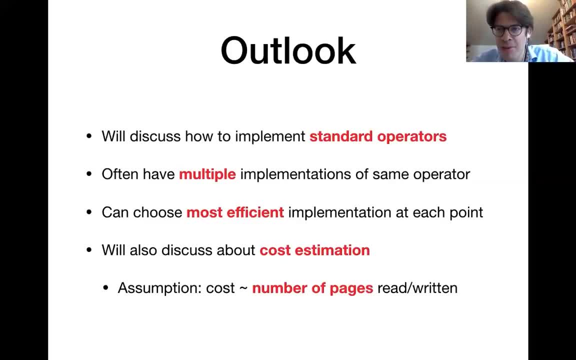 they are defined. we will discuss the algorithms and also we will think about how we can estimate the execution cost of those algorithms, because then the algorithmic improvements that we will see over time will actually make sense. all right, and as we have also discussed last time, we will generally measure cost. 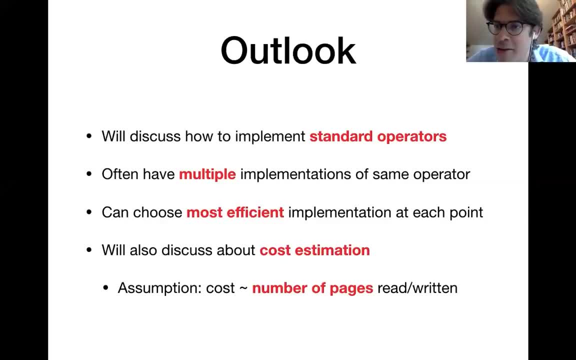 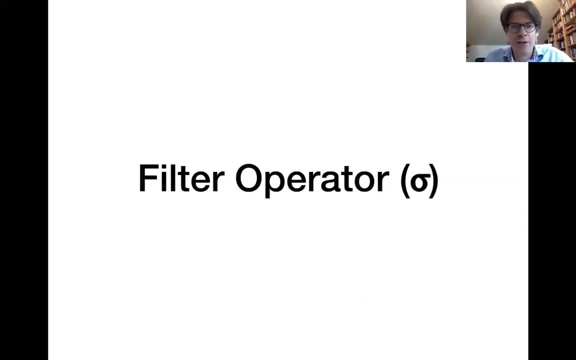 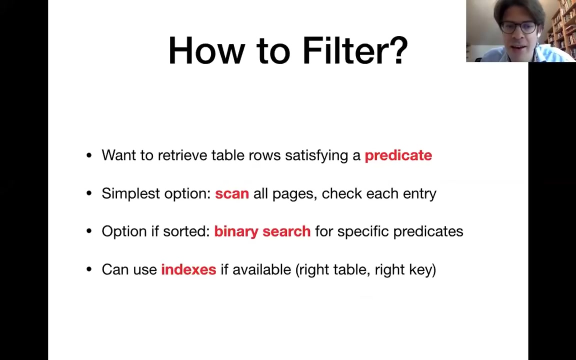 by the number of of pages that are written to and from hard disk. Alright, so those slides. we have already started discussing that last time. We have started discussing about the filter operator and we have seen that there's multiple possibilities to access the same table when trying to retrieve the 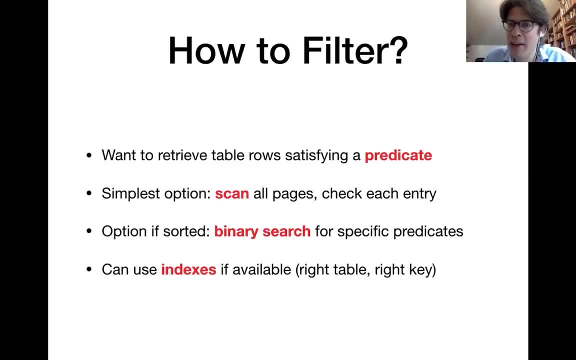 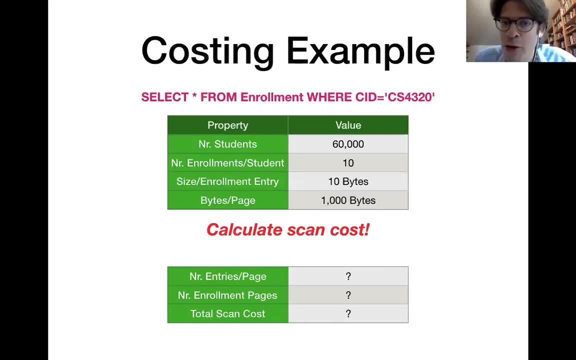 rows that satisfy a certain condition. We can scan, we can use binary search or we can use indexes, and the last time we have already looked at an example for how we can calculate the cost of a scan, which essentially just is the number of pages that we need to read from a relation. So here we have the numbers. 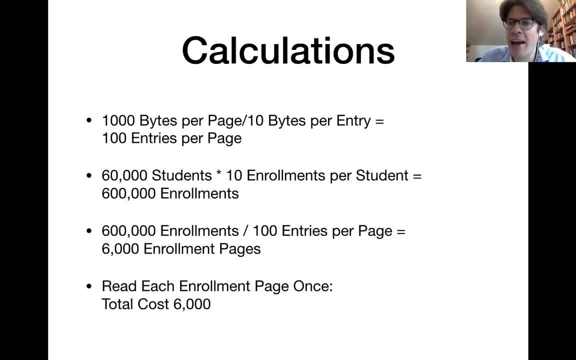 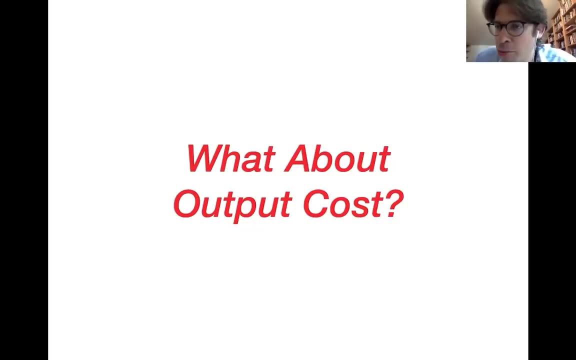 from the example, and on this slide you also have more details about how you can get to those numbers in the example. Alright, we have also discussed the number of pages that we need to read from a relation. So here we have also discussed that the cost for the output, for writing out the output of an operation, is 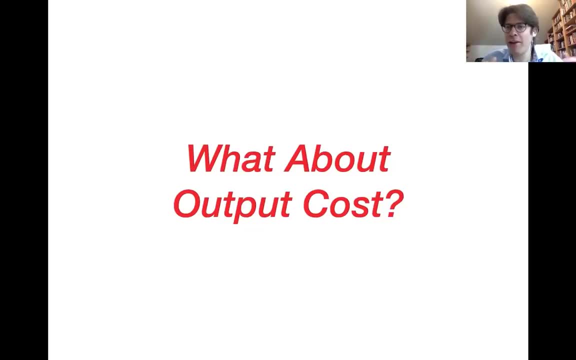 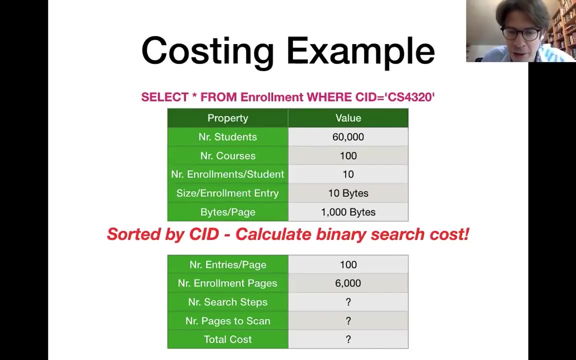 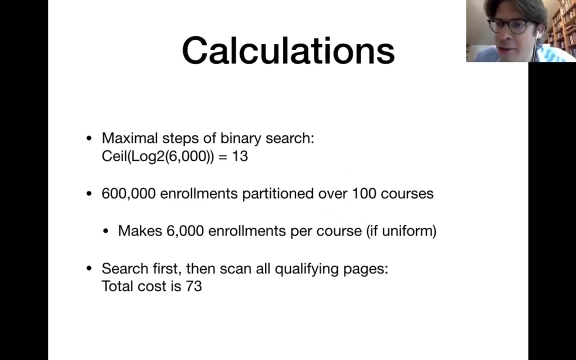 typically not counted, because that is the same for all alternative implementations of the same operation. We have also seen the example for binary search. Again, here you have the numbers, and here you have the steps that we did in order to get to those numbers. Alright, 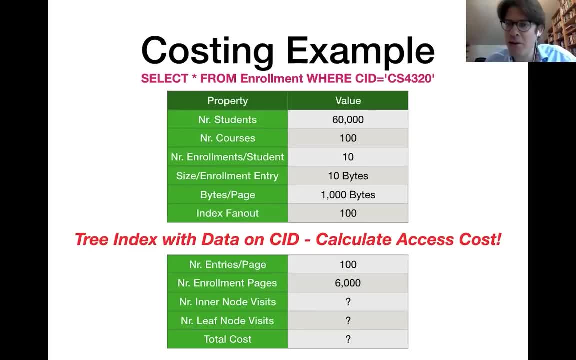 now, the next thing that I want to discuss about is indexing and how we can use indexes for evaluating filter conditions. So here we have always this query where we select enrollments for which the course ID equals CS4320 and on the upper half of the screen you have a couple of properties of the 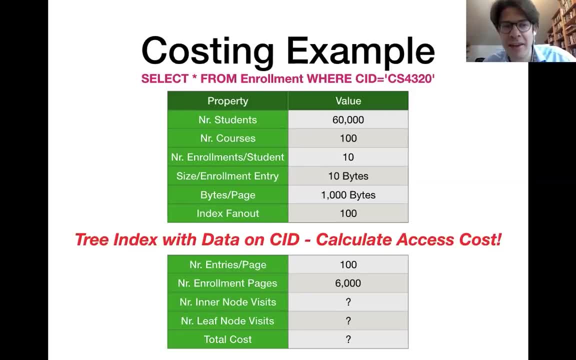 enrollment table and of the entire system. For instance, we know how many students and how many courses we have. We know that we have an average 10 enrollments per student and we have some information about the size of those different entries and about how many entries we can fit on one of those pages. 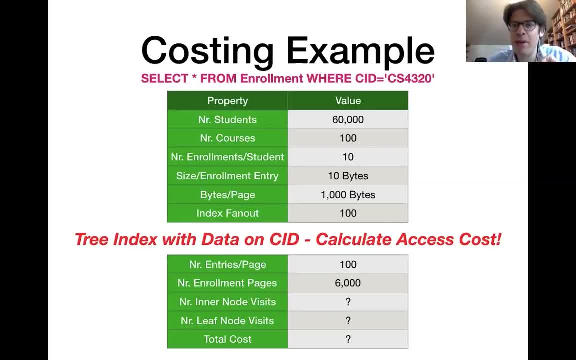 Now, here, since we deal with indexes, we also need some information about the index fan out, which means the number of child nodes for each index node, and here that is a hundred. So, given that the number of child nodes for each index node, and here that is a hundred, so, given that, 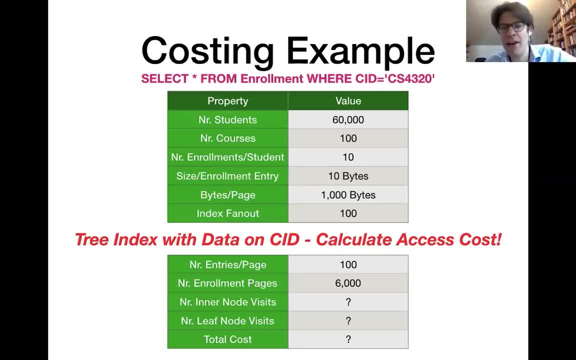 we have 100 entries per page. we have already calculated that before- and that the number of enrollment pages is a six thousand. think about how you would calculate the cost for using that index. So you have to think about how many inner nodes we have in the index that you need to visit, how many leaf nodes we 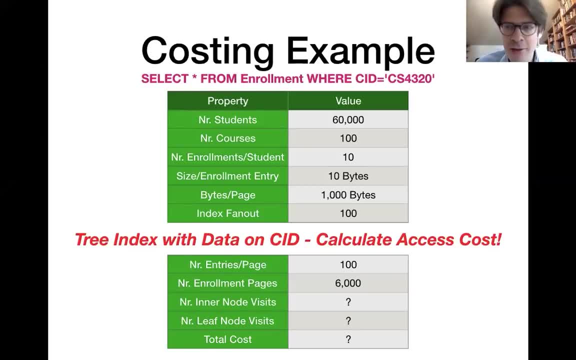 have and then what the total cost is. So here we assume that we are given a tree index and it's one of those tree indexes where the data is already integrated into the index itself, so you find directly the data in the index leaf nodes. I give you like a minute or so to think about how. 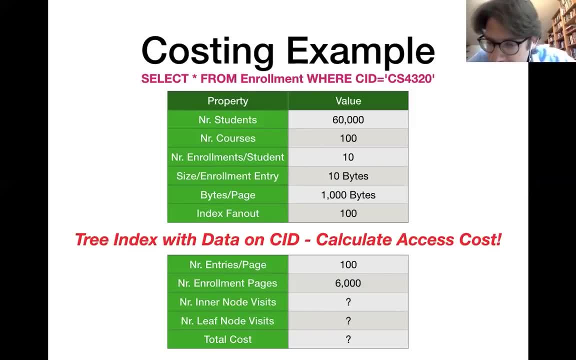 you would go about that? and the question on the index type in the hash. so this is a tree index, All right. So maybe you might not have had enough time for doing the calculations, but perhaps at least enough time to think about how you would go about doing the 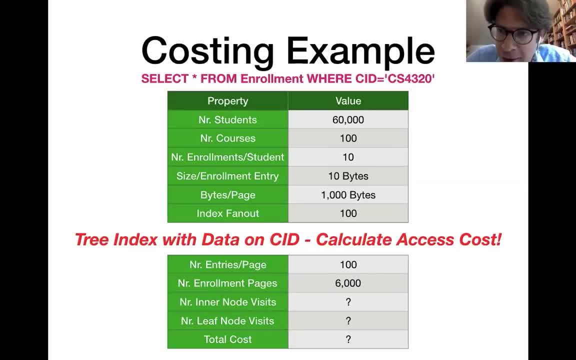 calculations. Yeah, I mean I haven't really think about it, But I do think it would be probably good to have enough time for doing the calculations, but perhaps at least enough time to think about how you would go about the numbers, about calculating this. 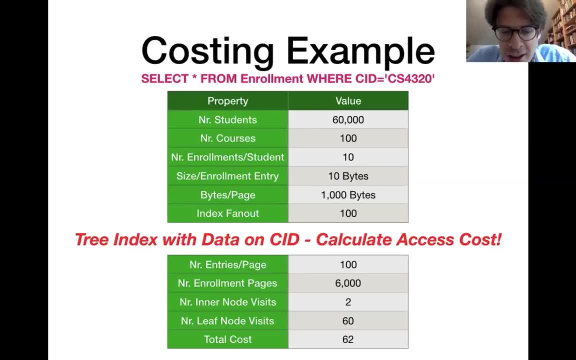 So this is the solution here: We have a fan out of 100.. That means the index root node has 100 child nodes And it has 100 square, meaning 10,000 grandchildren. So that means that we have only an index of height 3 in total. 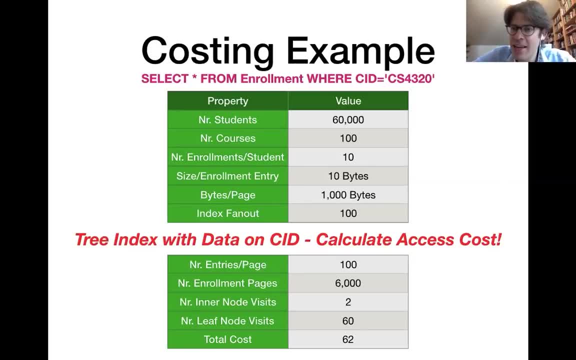 And that means we only have to step over two inner nodes in the index before we reach one of the leaf nodes, And then for the leaf nodes, we just have to scan them in order to retrieve all result tuples. And already in the previous calculations, 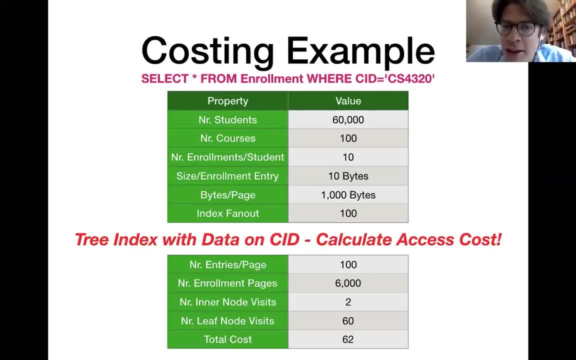 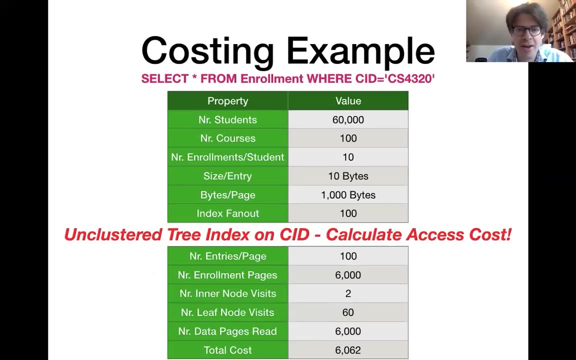 we have seen that the results to this query fit on 60 pages, So the total cost is 62 pages. You also have those detailed calculations. I'll just show you the evaluation summarized over here. All right Now. last example, on filtering. 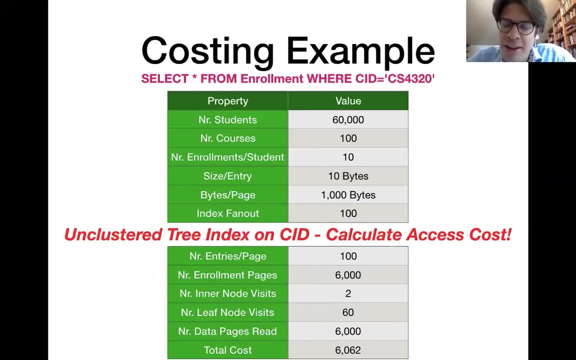 Let's assume that we don't have one of those indexes which integrate the data already, But let's assume that we have an unclustered index instead. So the entries in the index leaf nodes, they are not the actual data, but they point to the actual data. 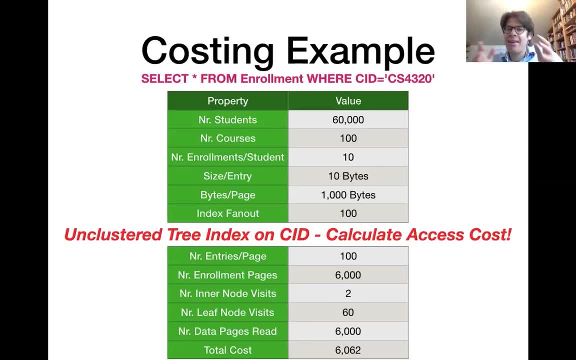 which means we have some additional overheads for accessing the actual data. So here, if you look at the lower half of the screen, you have the same number of inner nodes visited, the same number of leaf nodes read, But then additionally we still need to access the actual data. 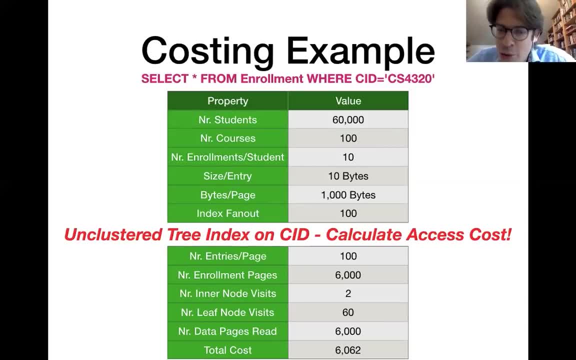 And assuming that those entries that we are looking for- we are looking for 6,000 entries in total- that they are located on different pages, it means that they have to read all those 6,000 entries. So we have 6,000 pages from hard disk. 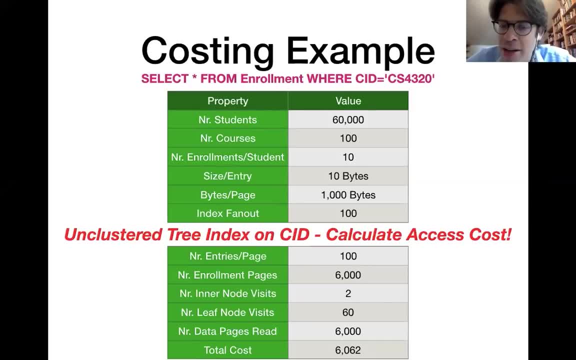 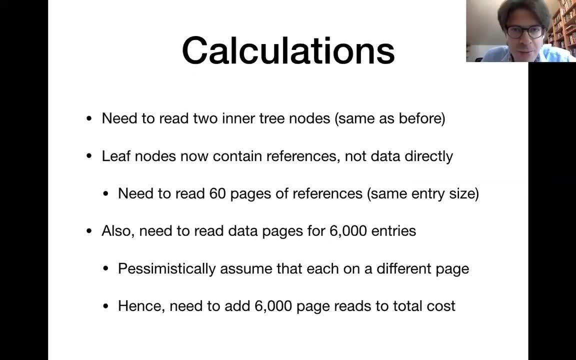 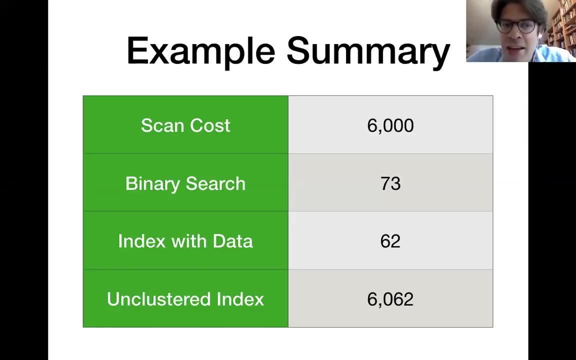 And that makes access with that index actually quite expensive. Here you have again a summary of those calculations. Now, altogether we have seen different ways of answering the same query. We have seen that scanning the entire table can be quite expensive. 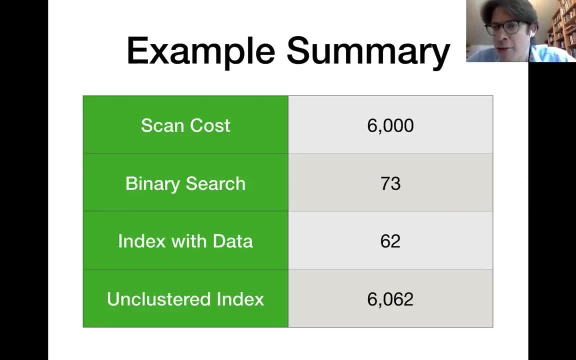 Using binary search is already much cheaper. It requires, of course, that your data is sorted Indexing. if the index is clustered and contains the data in the leaf nodes, that is actually quite cheap. typically, Using an unclustered index is typically more expensive. 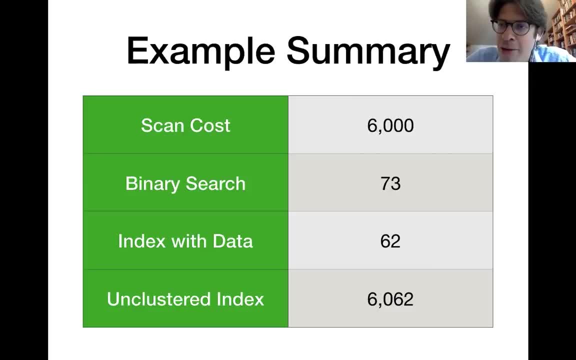 And often it is even more expensive than scanning an entire table, And in this case that actually happens. So using the unclustered index is a little bit more expensive, at least, than scanning the entire table. So even if you can use an index, you 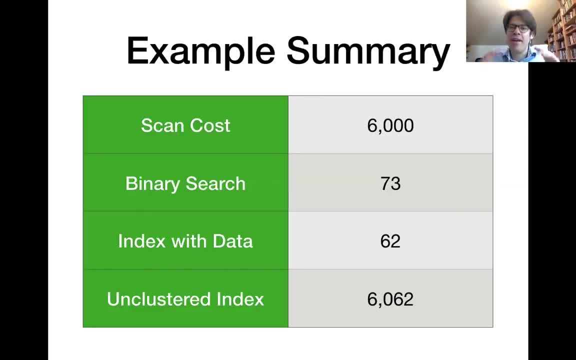 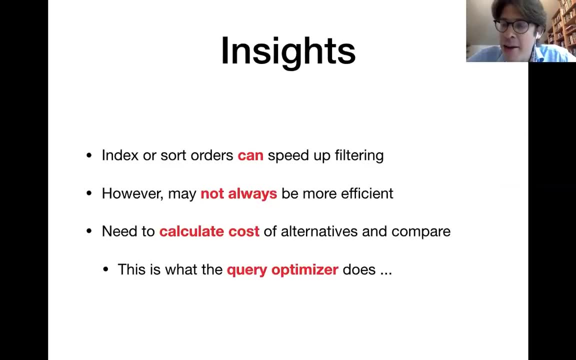 can easily do that, But it's not always a good idea to do that. You always have to calculate the cost of different options and then select the minimum one, All right. So typically it's not you doing this, but it is the query optimizer of the database system. 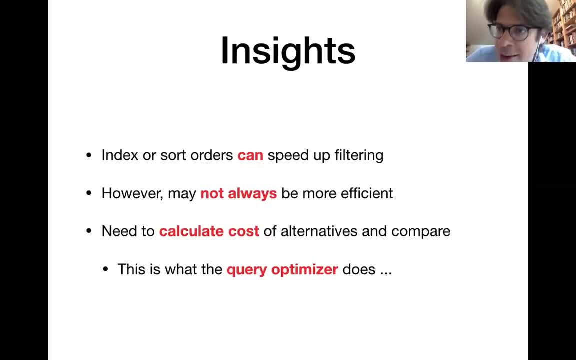 Once it receives your query, then it thinks about all the different ways in which it can answer it. It tries to estimate the cost of different possibilities and to compare them and then to select the minimum one. And if it doesn't get the minimum one, 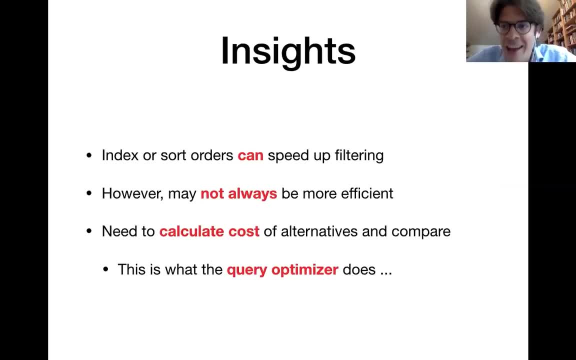 then it goes to the next step, And it goes to the next step, And if it doesn't get the minimum one, then it goes to the next step. So it's trying to say, OK, let's see if the amount of time it takes for the query optimization. 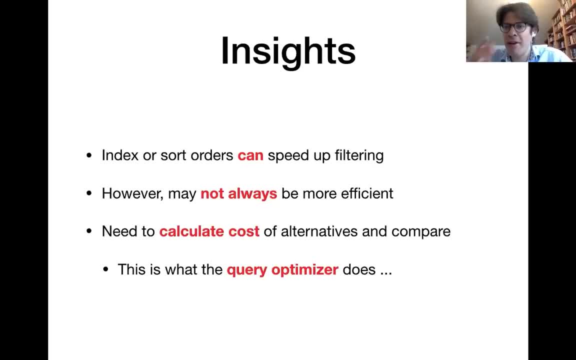 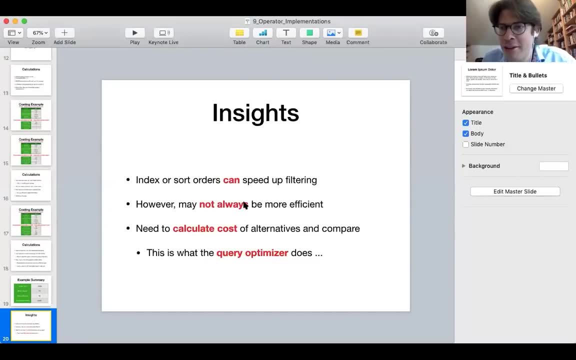 doesn't work out. And then, if you don't understand what's going on inside a database system, you will not be capable of fixing it. So it's good to know what is going on in the background. Now, in the following, I'm going to show you a little example. 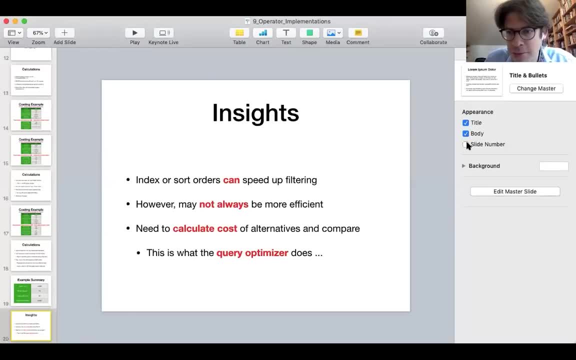 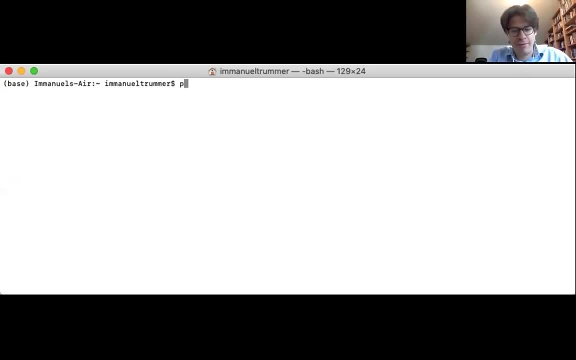 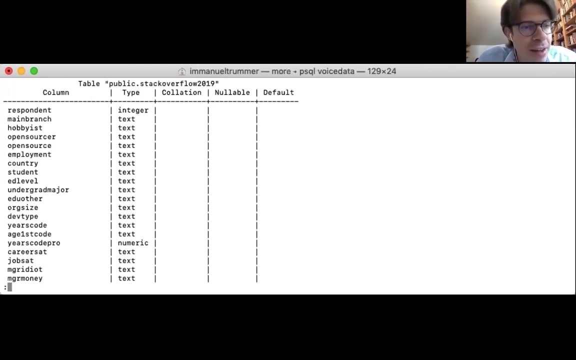 my terminal. all right, okay, and so here for this example, i'm gonna use again the stack overflow developer survey table, which contains results of this developer survey conducted by stack overflow. quickly going to show you some of the columns that the table contains, so each column corresponds to a different question. essentially, 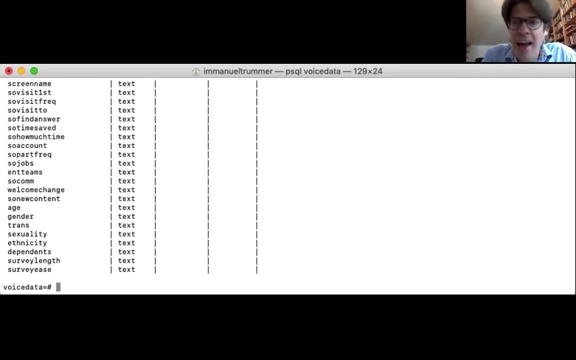 all right. and now, for instance, we had one column about the employment status, so perhaps at some point i want to filter the entries in the table according to the employment status and in order to make that faster i might want to create an index on that column. so 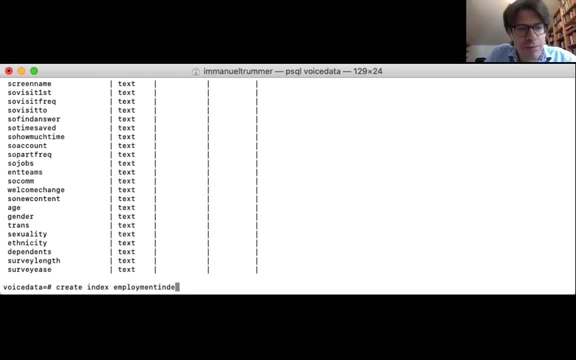 let's actually do that. here we are creating an index on the employment column of the stack overflow table. it takes a few seconds and now we have the index. i'm enabling timing, okay, and now, if i have a, for instance, a scalability option, yes, that's good. so what happens is the scrub. 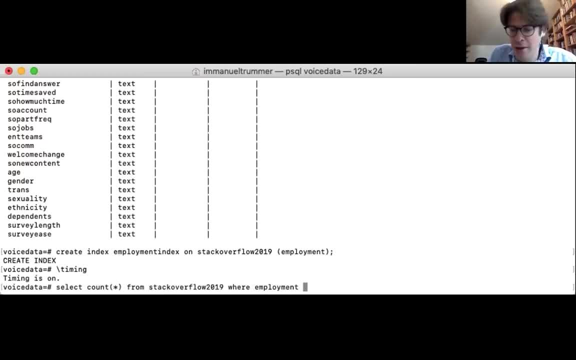 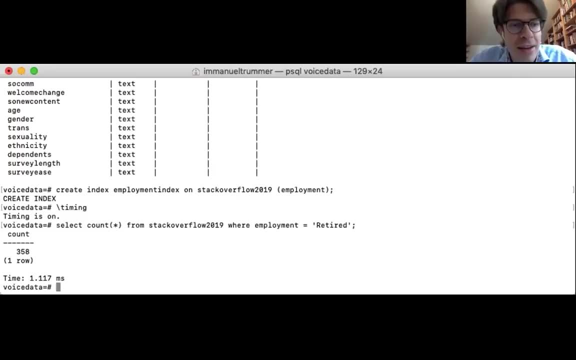 that i'm spraying on that column goes: the Following database is a list of credited rubric. oh yes, i have enjoyed that, or with after the check, but under that, anyway, that's the max. last thing and always remember is, let's say, weather, which means that the weather 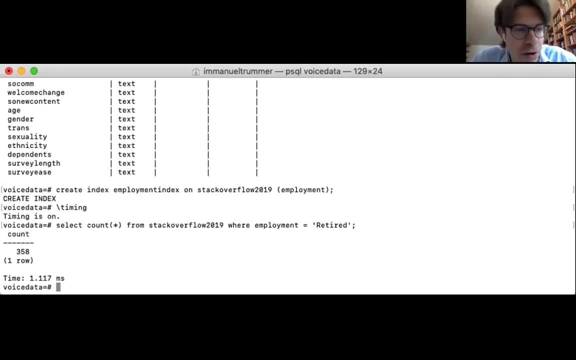 거울 is assumed to be expect to be stable when it's not, as i said, as i said in the previous conversation, so that information may be shaking a lot so it typically is hard to count in aah. So without indexing we had times of typically something around 100 milliseconds for queries on that table, So now it is much faster. 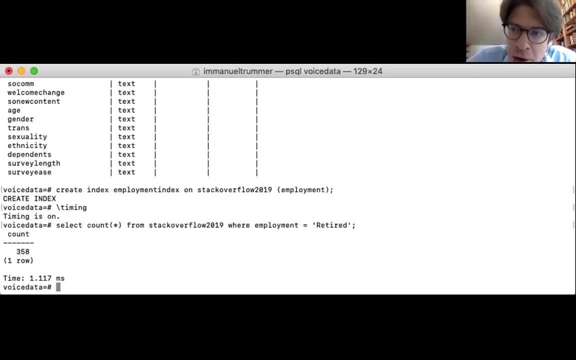 All right Now, if I want to know more precisely what's going on internally, whether the query optimizer decided to use the index or not, you might want to try out the explain command, and the explain command essentially tells you how the query optimizer plans to answer a given query. 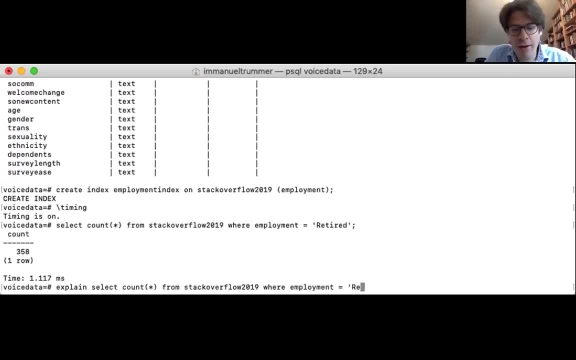 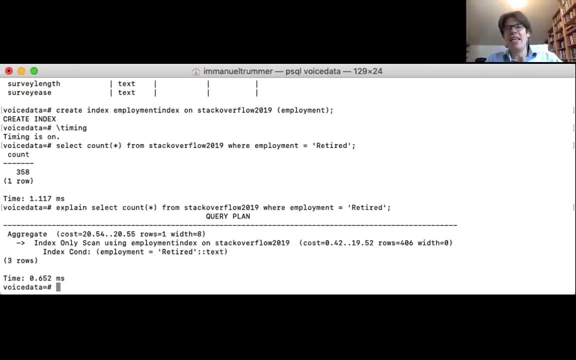 So if I enter the same query as before, All right. Then the explain command tells me essentially the different steps in the plan that the query optimizer intends to execute. Now what we have here. you see the keyword index in here. So it seems that the query optimizer decided indeed to use the index over here, with an index only scan. 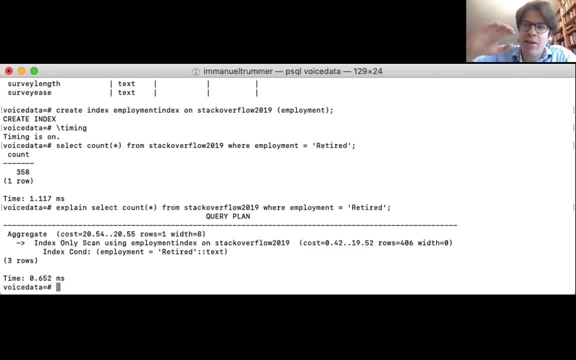 And the final operation in that plan, which always comes first when representing those query plans in this format. that is an aggregation, because I actually wanted to count those people. All right, So that is how the query would be executed. So, for instance, I mean, since here by default they have created a tree index, that can also use that index for inequality predicates. 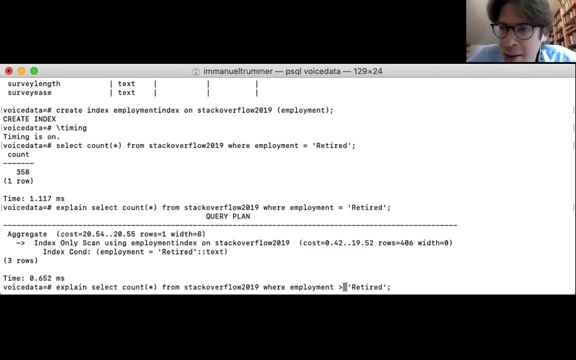 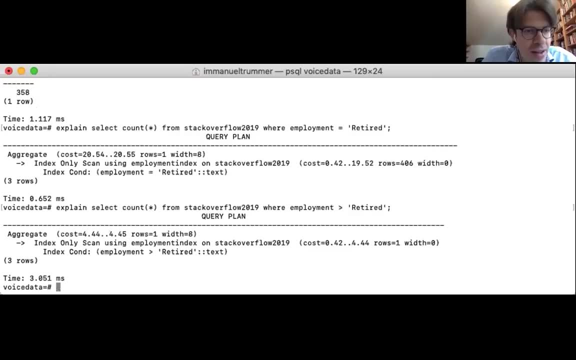 so if I, for instance, replace the equal sign here by an inequality, then what would happen here is that the query optimizer decides to use the index as well. now tell me in the chat what you think will happen now if I replace this inequality by an inequality into the other direction. do you think it will? 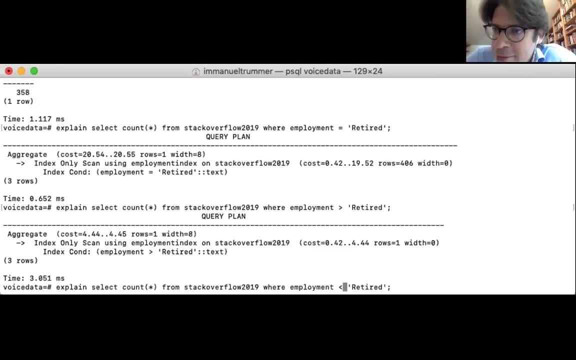 change anything? can it even change anything? anyone wants to make a guess I'm already asking about, then probably something is gonna change. let's actually do that all right, and here actually nothing is gonna change. okay, so it seems that if I replace this inequality by the other direction, then it is still the cheapest. 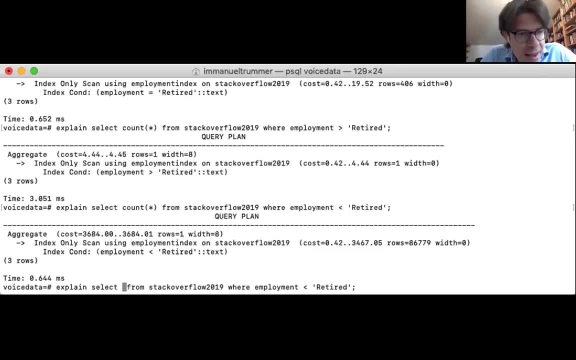 to use the inequality. but if I slightly change the query by adding, for instance, instead of counting the number of people we have a specific employment status, I am what I rather want: to select the specific respondent IDs of those people with a specific employment status. and if I do this over here, then you see the 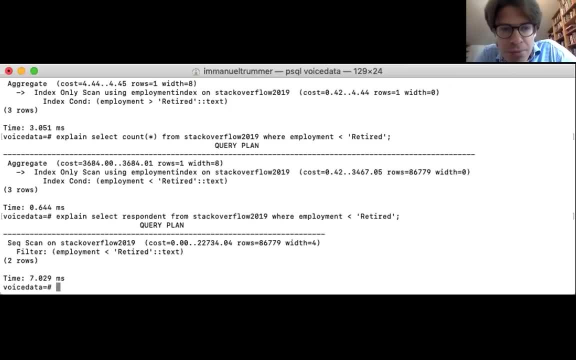 that the query optimizer has stopped using the index because it seems to think that not using the index is more efficient here. So the thing is this: the index that we are using here is, by default, an unclustered index, So it points to the data. 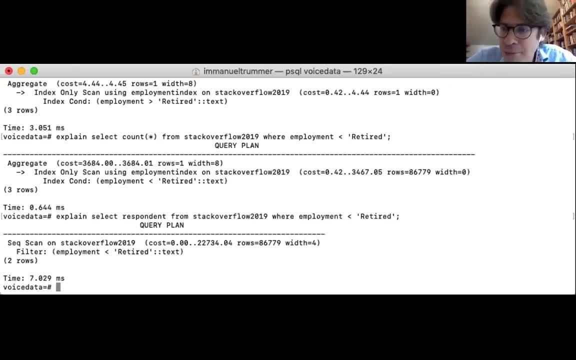 instead of containing the actual data. And as long as we use account aggregate, it means that we can only work with the index and count the number of entries that satisfy the predicate in the index, But as soon as I add different columns that are not directly a part of the index, search key. 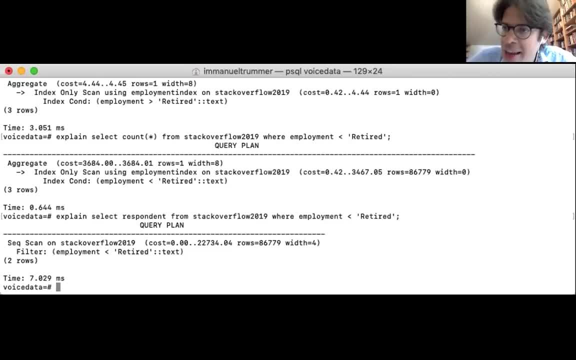 they actually need to go through the leaf nodes in the index and retrieve the associated data from the data table, And doing that can be quite inefficient, depending on how many entries you have to retrieve. So here, with this inequality, I'm actually not using the index. 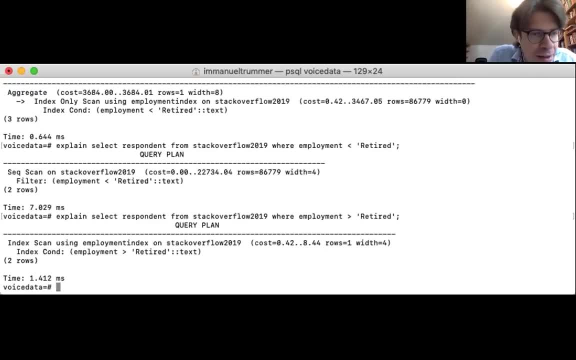 based on the query optimizer. If I replace it by this one, then it suddenly starts using the index again. But the thing is that here I am using inequalities with the constant and I also make sure that the turnover is a very stable term. 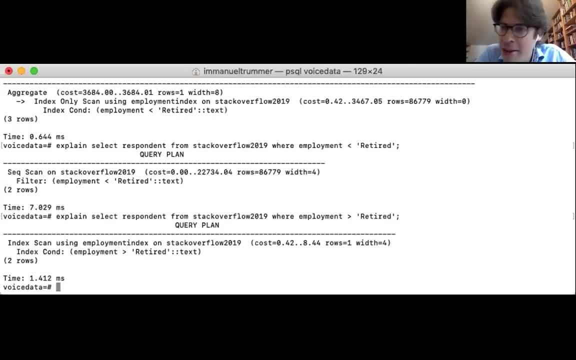 So, as I say, I'm not going to modify it too much. see the cost estimates for executing those different plans that you have between parentheses, the cost estimates and estimates about how many rows will satisfy the condition that you have in the query. So I mainly wanted to show you 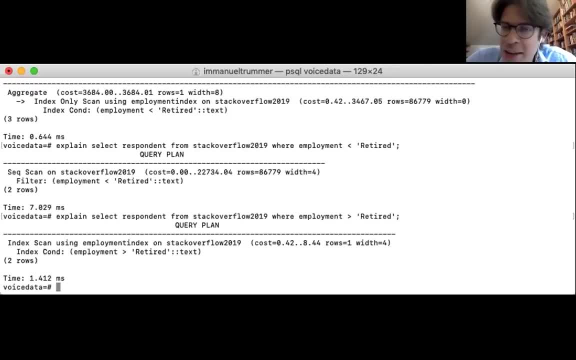 how you can get a sense for what's going on inside the database system, how the query optimizer decides to execute certain plans. You can get that with the EXPLAIN statement and, as you see here, for multiple queries that are somewhat similar because they use the same constant and the same table in the same 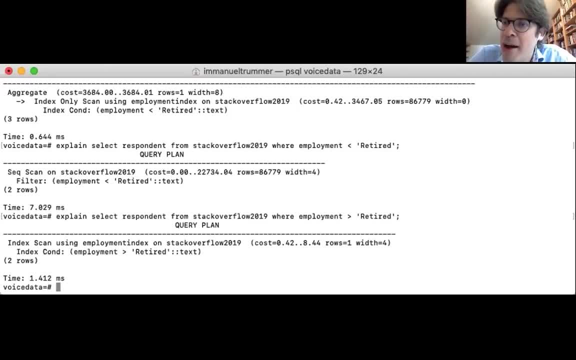 type of condition. still, for some of them the query optimizer will decide to use an index, while for others it will decide not to use the index and just to scan all the pages of the table instead. So the query optimizer essentially does this kind of reasoning that we are also doing by 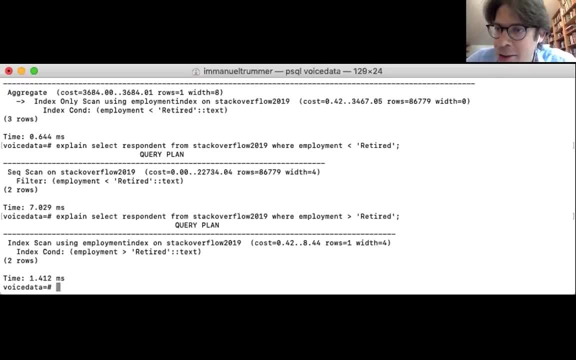 hand in order to understand how that is done. And here is a great question about whether we can force the query optimizer to use the index. Well, indirectly, yes, there's a couple of possibilities in Postgres to at least prevent the query optimizer from choosing certain operator implementations. So essentially you will. 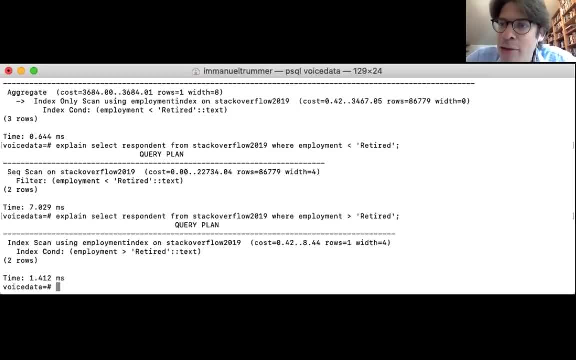 force the query optimizer to use the index. if you do this, disable all other alternatives. so in a way, yes, there's a way to force the query optimizer. there's other database systems that offer you more diverse possibilities to influence what the query optimizer is doing, but it is. 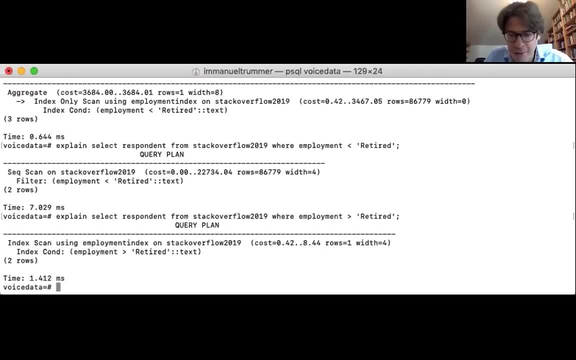 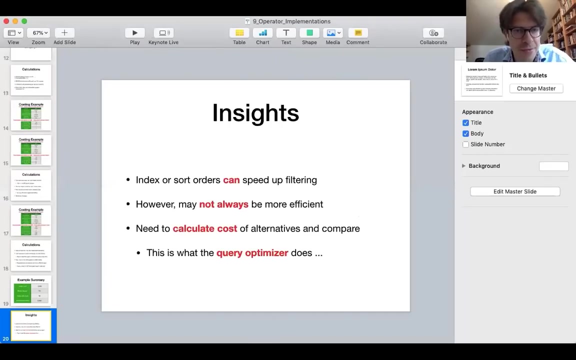 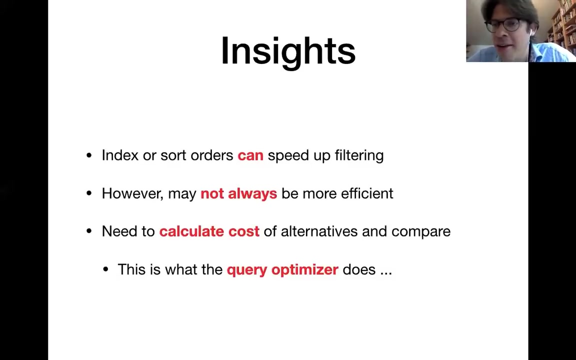 possible. all right, now let's go back to the slides. you so? now you should see the slides again, and on this one, I'm essentially making the point that we always need to calculate the cost of different alternatives in order to select the optimum, because it is a purely unclear what the best. 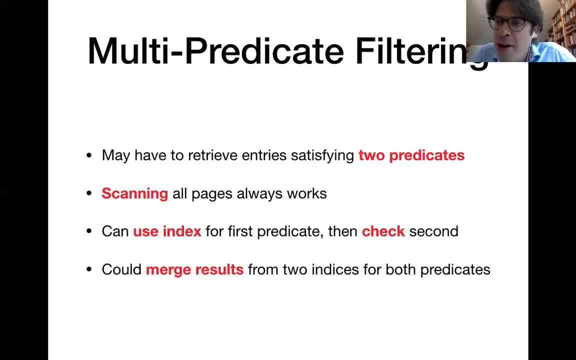 alternative is now. one last word on filtering. so far we have considered cases where we have only one single predicate to answer. that is a little bit easier in practice. you might sometimes have multiple predicates within the same filter operation, so in those cases what still always works, of course, is to just 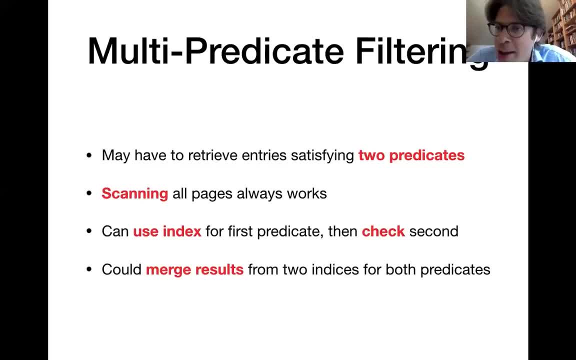 scan all the pages from the table and to evaluate those two predicates on each entry. you can also make a mix. you can, for instance, use the index in order to retrieve entries satisfying the first predicate and then you evaluate the second predicate on those entries that you just retrieved, or 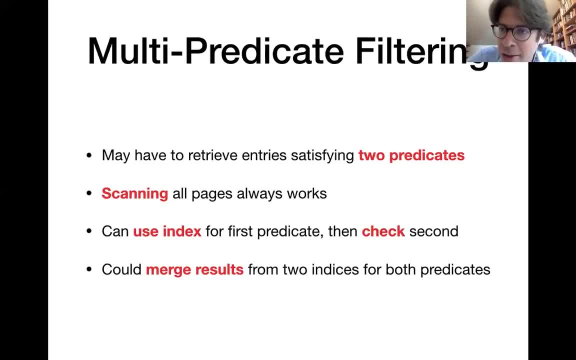 you could. even if we have two corresponding indexes for one index for each of the two predicates, then what you can do is you essentially retrieve the entries that match the first or second predicate from those two entries and then do the summary And in the end you merge them together and only keep the ones that appear in those indexes. 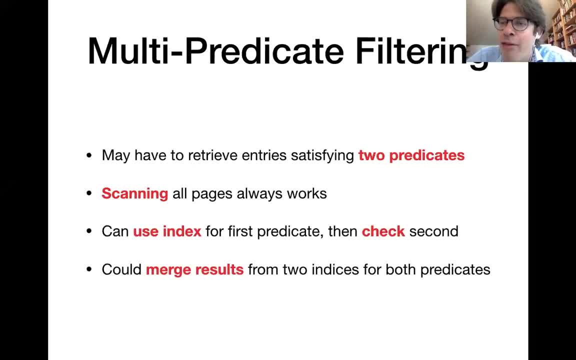 So once we have multiple predicates then you have one more possible Combinations. if you also have indexes, then predicates become really complex. then typically in practice The cheapest alternative is often to just scan the entire table and evaluate all of those predicates at once. But it depends on the particular 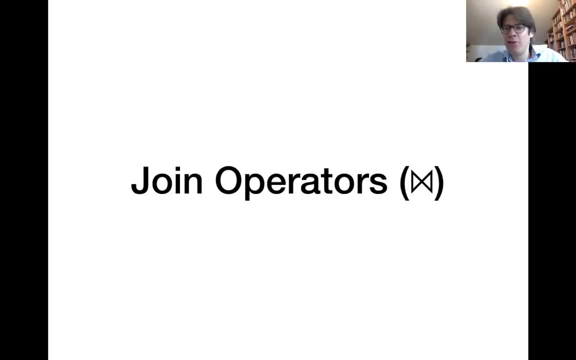 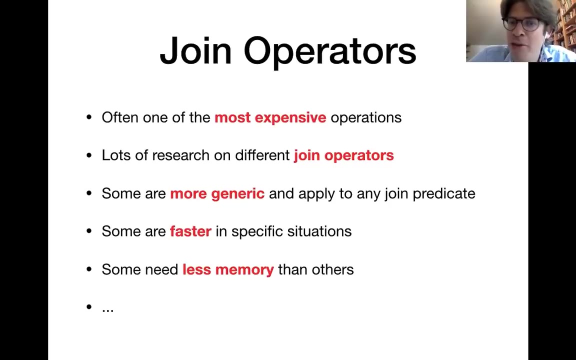 All Right, so those were a couple of different base to do the filtering. next We are going to discuss about join operators and we will actually discuss a lot about different join operator Implementations, because that is, in fact, is one of the most expensive operations in a query plan and that is why there has been lots of research on different join operator implementations and 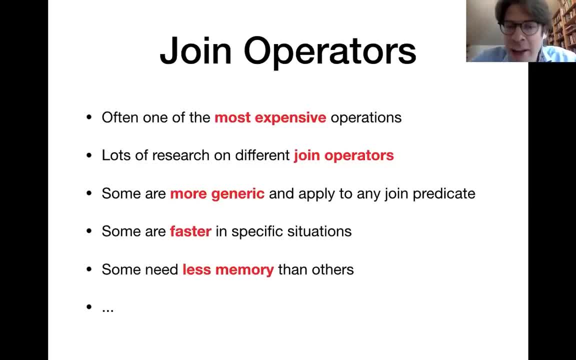 People have developed a whole variety of Alternatives. some of them are more generic and you can apply them for arbitrary join conditions. others have advantages because they are faster for certain types of joint predicates, and Some are great because they need particularly Little main memory while executing. so there's a lot of different pros and cons and your database management system. 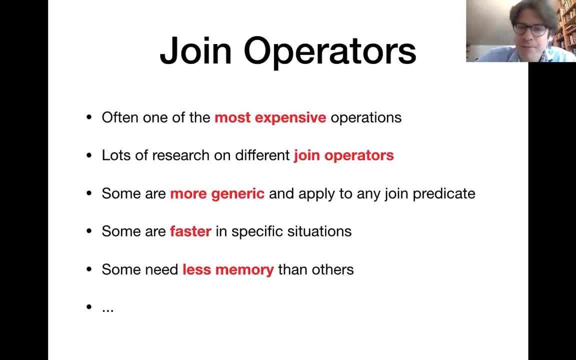 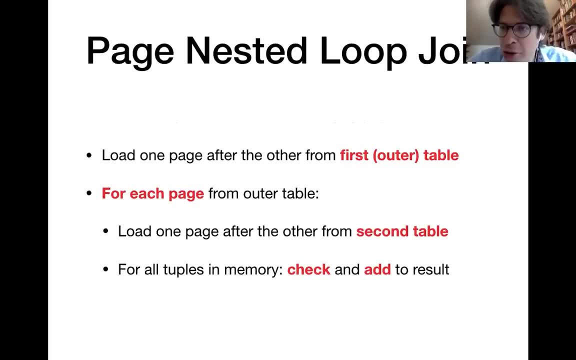 typically supports many different join operator implementations and Then it chooses the best one at runtime. So the simplest, the join operator that we will see in the following- that is the page nested- loop join, and the idea here is Very intuitive. So you want to join two tables. 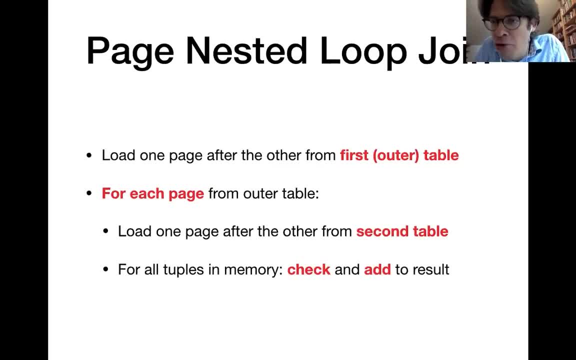 Let's say I want to join the student table with the enrollments, with the join condition that the student ID should be the same. Okay, so the way the page nested loop join works is simply this: I designate one of the two tables as the outer table. 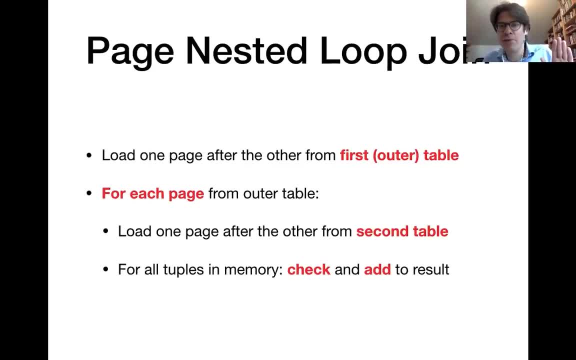 Let's say that is the Student table and the other table That's the so-called inner table. We will see why they are called that way in a second. Alright, so I would proceed by loading one page from the outer table, from the students, from hard disk into main memory and 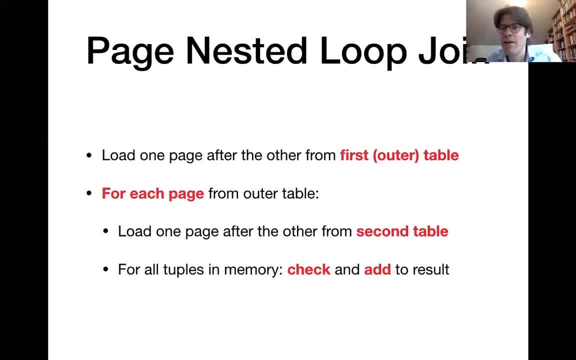 Then I would iterate over the pages in the inner table, Load to one into main memory after the other one. So the new page always overrides the previous page. and for all the tuples that I have in main memory, I will pairwise compare them, evaluate the joint condition and, if it evaluates to true, 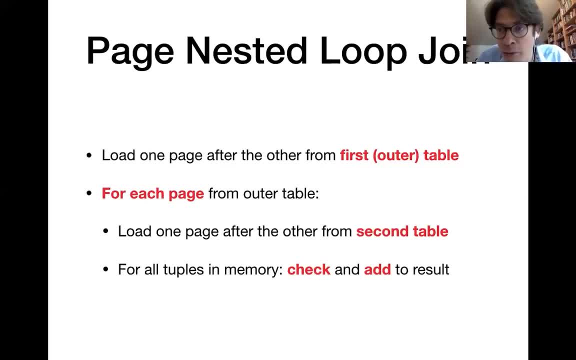 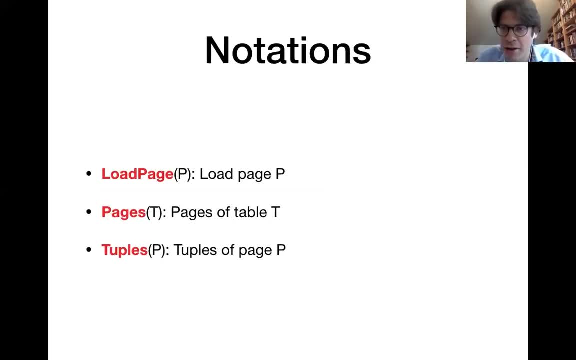 Then I add the corresponding tuple pair to the joint output. All right, so that is pretty Intuitive, but let's see some detailed code on this. So in the following pseudocode I use the notations that you see here. We have a command for loading pages from hard disk into main memory. 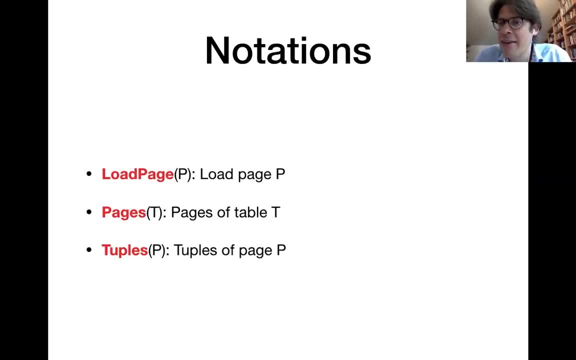 we have a command pages of T in order to get the set of pages associated with a table T, and The command tuples of P essentially retrieves the tuples which are stored on page P, Assuming that this page has previously been loaded from hard disk into main memory. So we assume 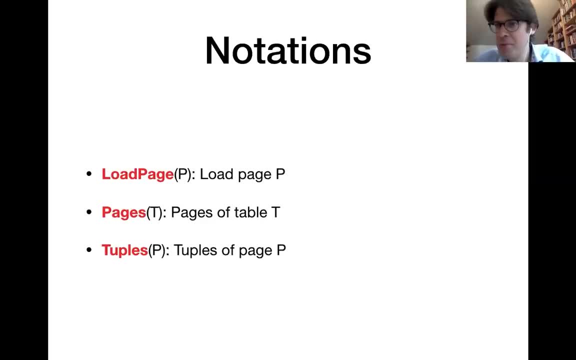 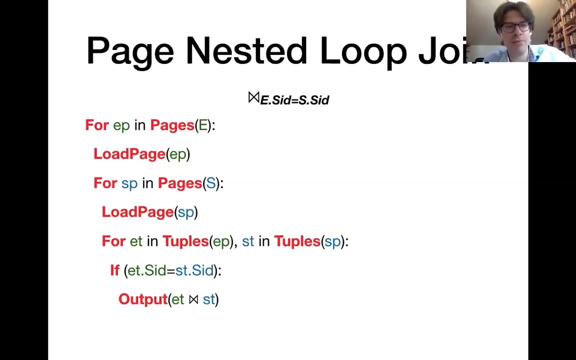 That at the beginning of execution of the join All the data is located on hard disk, because it doesn't entirely fit into main memory. Now let's say that we want to join the enrollment relation with the students relation. So in this example We actually made the enrollment relation the outer relation and the students relation the inner relation. 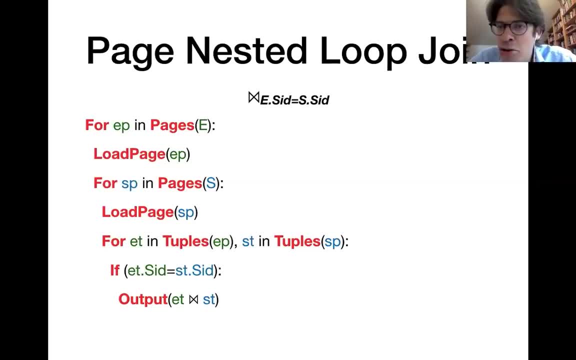 because, as you see, in a pseudocode and I have essentially two nested loops- and that is where the name from the algorithm comes from- and then The table that I'm iterating over in the outer loop that is called the outer table. So what I'm doing here is essentially I'm 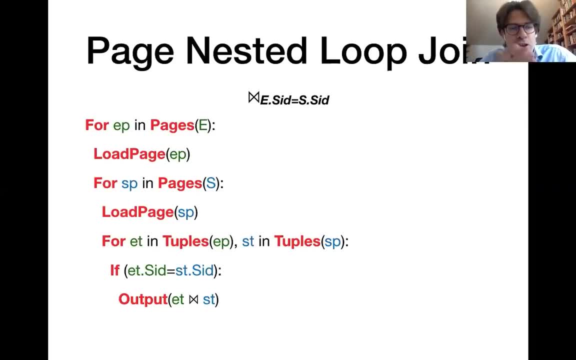 iterating over the pages of the enrollment table. for each of them, I'm loading the corresponding page into main memory. and Now I'm iterating over the pages from the students table And for each of them, in the inner loop, I'm also loading it from hard disk into main memory. and then, for all the tuples, 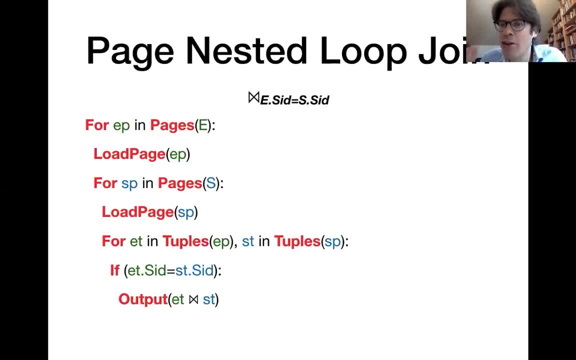 That are stored on the currently loaded enrollment page and on the currently loaded Students page. I'm matching them pairwise and I'm evaluating the join condition. Enrollment student ID equals student student ID for that tuple pair and if it is satisfied, and adding it to the join result. 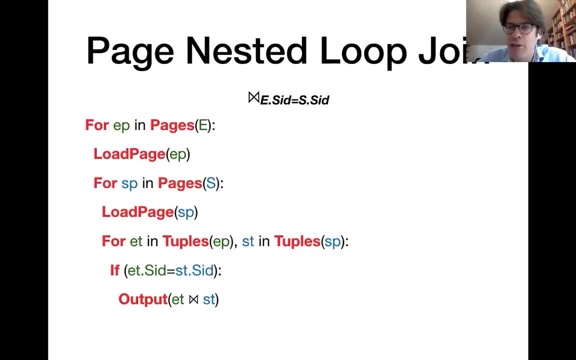 So that is the page nested loop join algorithm. Now in the following let's analyze a little bit how we would calculate the cost of this operation based on the number of pages in the enrollment and in the student relation. Now This load operation over here in the outer loop that is executed exactly once for each page in the 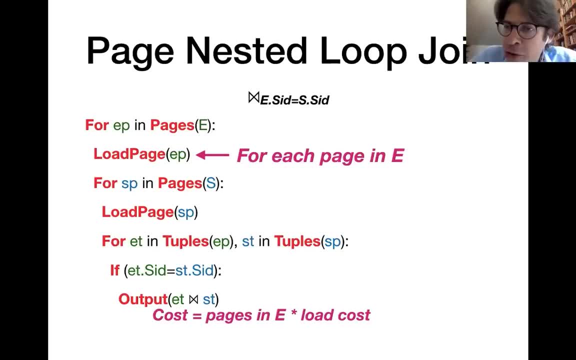 Enrollment table right because we iterate over all of them in. each one of them is loaded once. Now if you look at this load operation in the inner loop, that one is executed more frequently Because I hear we are in the inner loop. That means we are iterating once for each page in here in the outer loop. 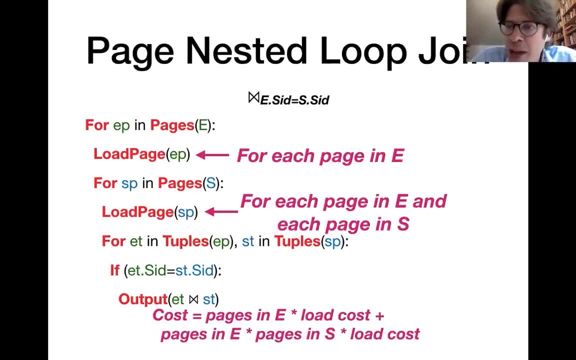 And in the inner loop We iterating over each page of the students table and therefore this command here will be invoked a number of times. that corresponds to the product of the number of Enrollment pages in the number of student pages right. So here on the bottom of the screen, you see that I'm calculating the cost, I'm adding up the different across components, So I 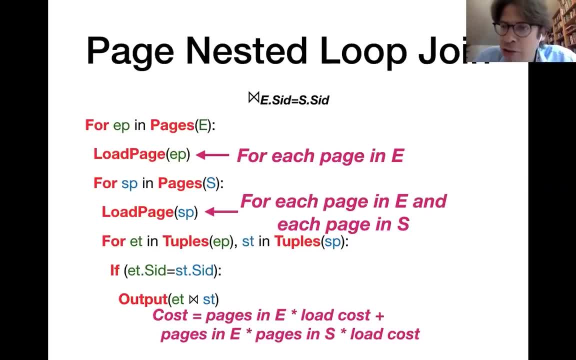 assume that I have some constant cost for loading pages from hard disk, and here I have counted the cost for executing that first loading command- e times pages in e times, and and Now I'm counting the cost for the second load command over here. But I also might 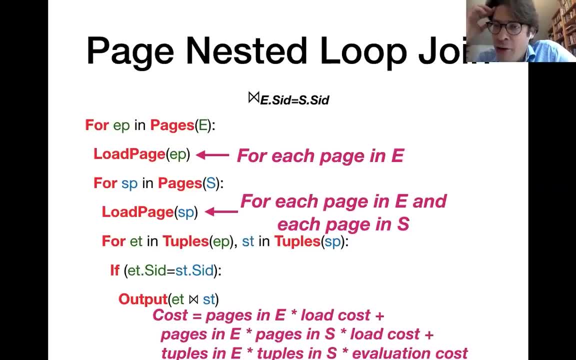 Sorry, but also might want to account. that is the cost for evaluating the join condition itself. so doing this doesn't require you to load data, but it has some computational cost. so here on the lowest row on the screen, I'm counting the predicate evaluation cost. 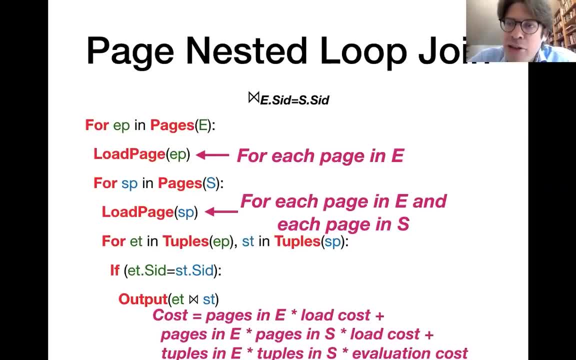 And query optimizers like the one from Postgres would take this loading cost and this evaluation cost into account. Now, here in this course, we use a highly simplified cost model. You're only looking at the number of data load operations. This is why, in the following, we will neglect: 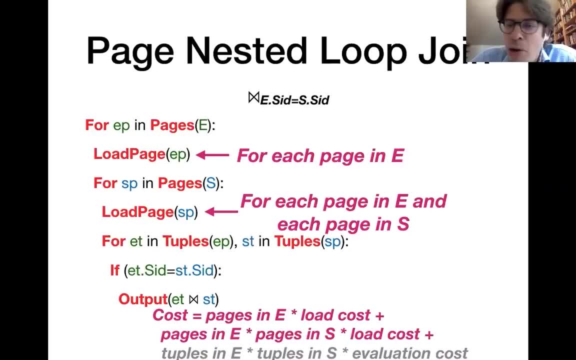 those cost components that relate only to computational cost. All right, So this is the cost of the page nested loop join algorithm And it essentially just iterates in two nested loops over the pages of the two input relations. Now we can also think about how much main memory that 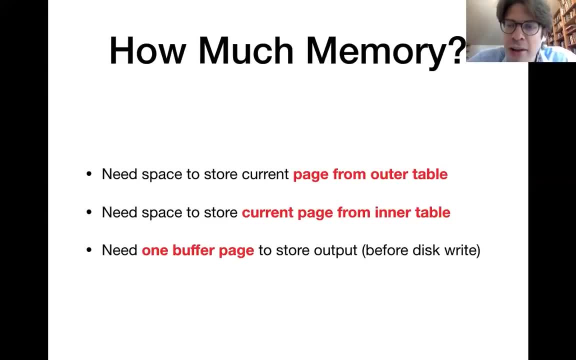 algorithm would need. So, first of all, we need enough space to store one page, the current page and the current page. And we need enough space to store one page, the current page and the current page. And we need enough space to store one page- the current page and the current. 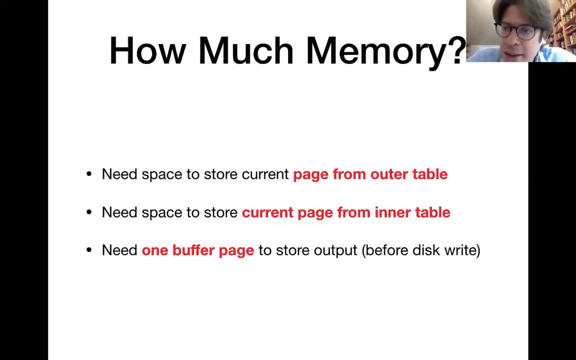 page from the outer table And on the other side we need the space to store the current page from the inner table And not directly shown in the pseudocode, but what you also want in practice, that is one buffer page in which you can store join result tuples. So in principle you could. 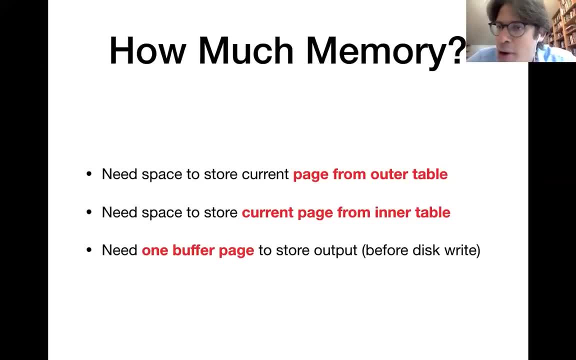 imagine like writing those join results directly to hard disk. But we know that data movements become much more efficient if we move the page from the outer table. So we need enough space to store those join results directly to the infections. So we have slightly 1.5. 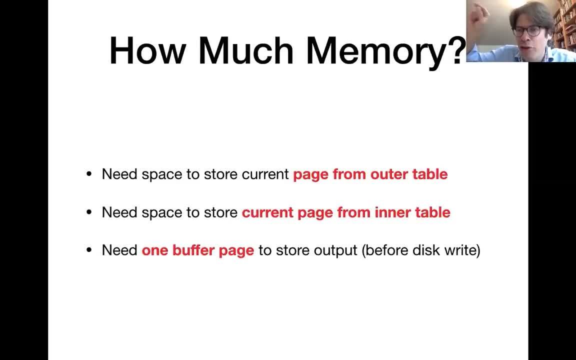 liquid programa. we would put a buffer page in the main memory, in the buffer pool, and be right tuples into that page whenever it is full. we copy its content to hard disk- again one operation- and erase the buffer against so we can insert more research. so all together what you 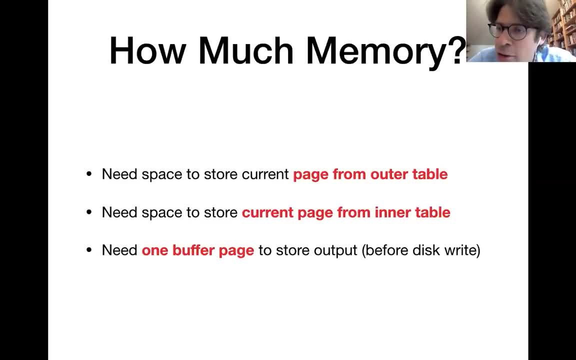 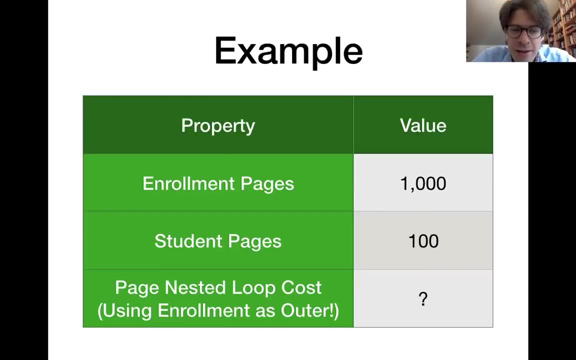 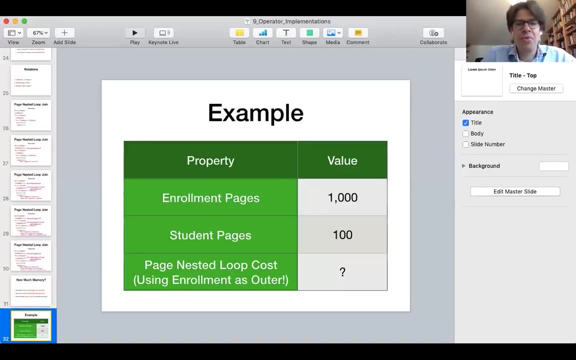 need are those three pages, which makes this argument. So, for example, we have one in Maru 보여, which makes this algorithm quite main memory efficient. Now, this is a little example here. Let's quickly move the chat a bit. So we have a thousand enrollment pages. 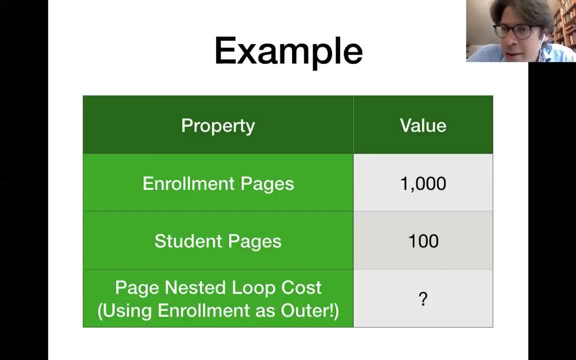 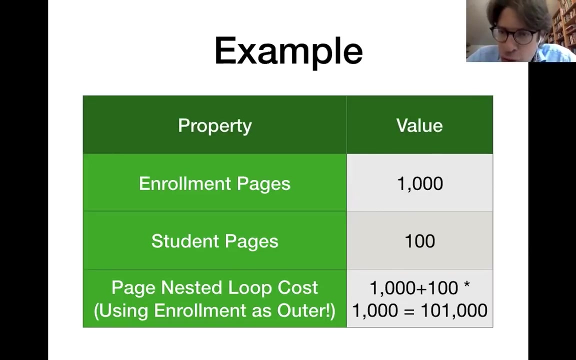 and a hundred student pages. So think a second about what the cost of the page nested group join would be in this situation. And we assume that the enrollment table is used as the outer table. Okay, All right, And here you have the solution. 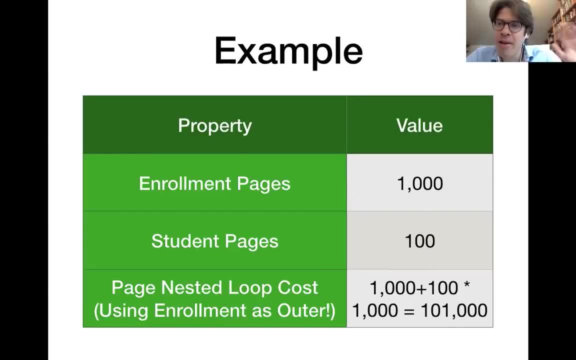 So if you simply if you apply the cost formulas from the last slides, then you essentially need to count the cost for reading the outer table pages once that is associated with the first load operations, And then you need to count the number of loads for the second load operation. 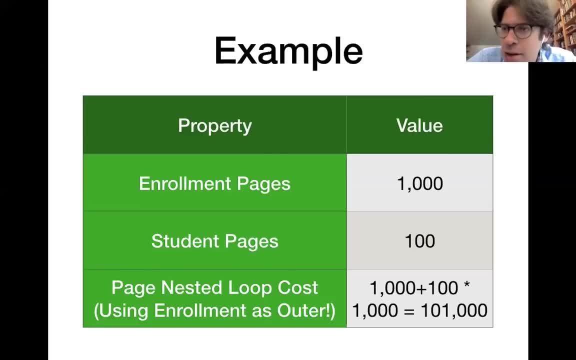 in the inner loop And essentially for each page in the outer table. you're reading all the pages of the inner table And that means there's a thousand times the 100 pages And in total you get a relatively high cost compared to the joint algorithms that we will see later. 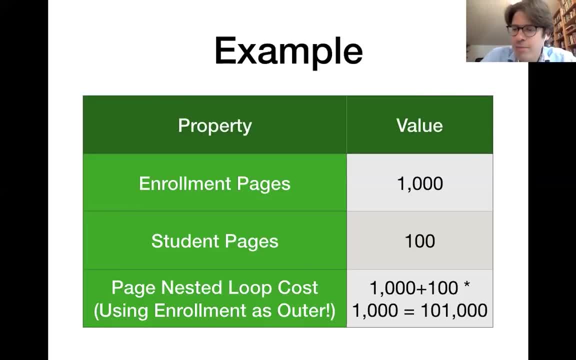 of about 101,000 pages. Does anyone see an easy improvement to this cost? Just a small one? Oh, yes, very good, Here it is immediately the right answer in the chat. Exactly, So what we can do is to simply swap the order. 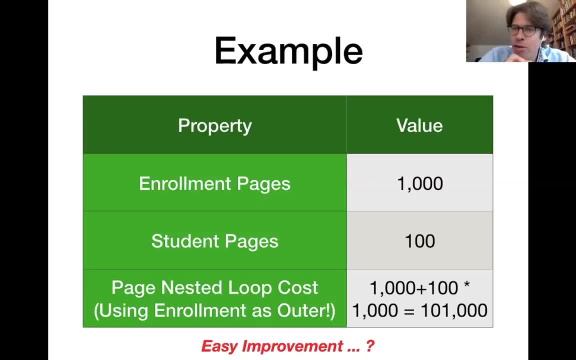 of the joint operands, because then I would replace this term 1000 here by the term 100, because if I use the student table as outer relation, then I only need to count the cost for reading the pages of that page And then I can choose to do this. 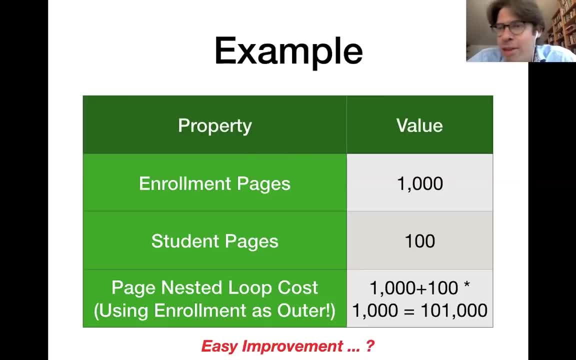 So I can just add a new item to my list by adding the new audience And then all I need to do is just go to the tab with that link and I can do a new order of that item so you can see the total number. 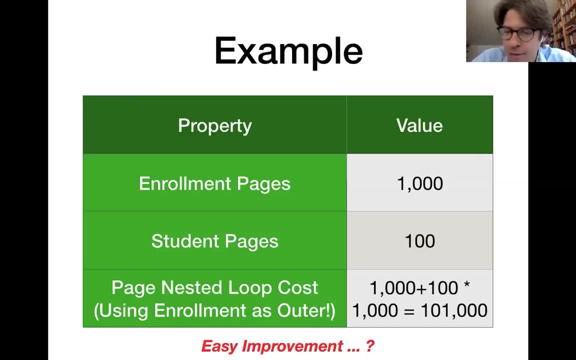 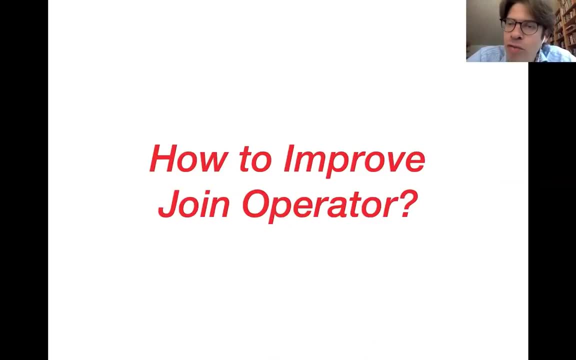 of the order functions. that I just did and let me just type it in here. Now let's go back into the graph, as I told you. so here in the graph, this is the order of the load operations, which is going to be the order of information. 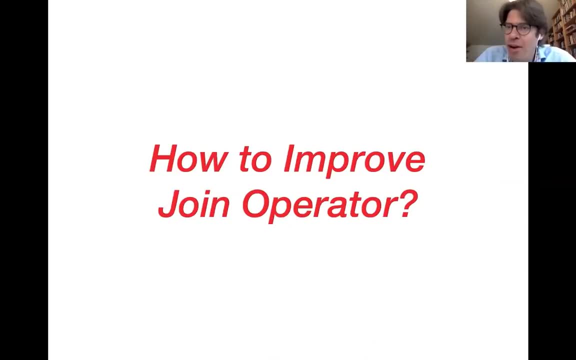 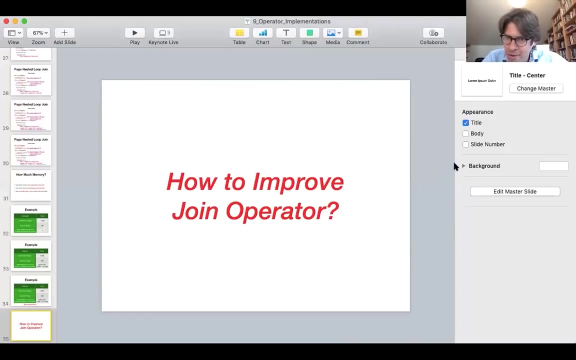 that I'm going to be using to make this work. So at this point you can see that that is one, two, three, four, six, seven about how we could improve this join operator further. okay, very good. and that refers exactly to: 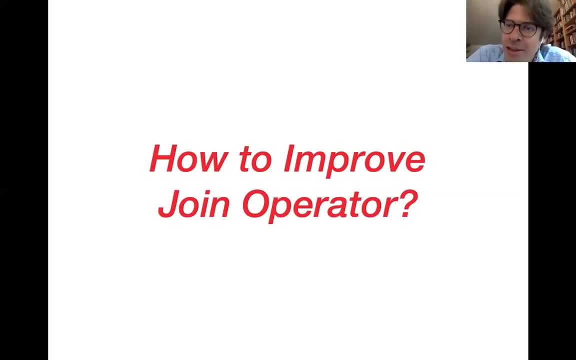 what we will see next. so here the suggestion is to essentially keep pages longer in main memory, because it is true that for some of those pages we will keep loading them and then erasing them, and then loading them and erasing them, so we actually load the same page many times from hard disk during one 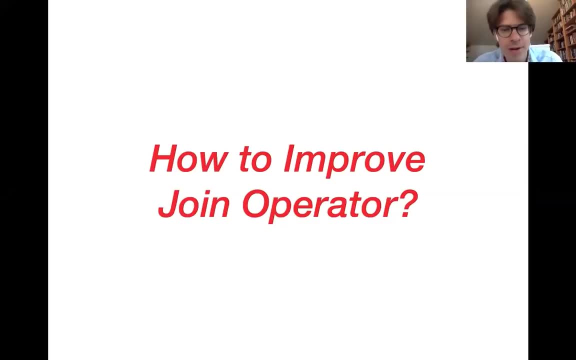 single join operation and intuitively that seems inefficient. all right, so let's see how we can improve over that join operator by keeping things longer in main memory. now that leads us to the next step, which is to keep pages longer in main memory leads to the so-called block nested loop join. 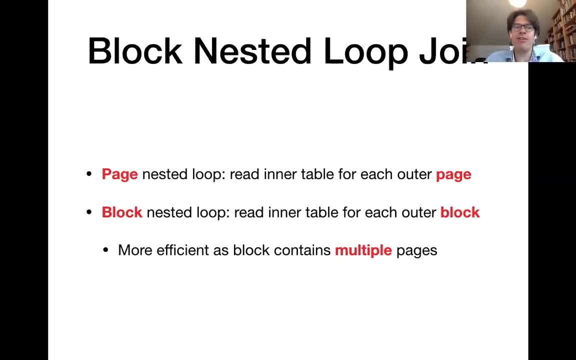 And the main improvement compared to the previous algorithm is essentially the following: In the previous algorithm we have read the inner table once for each page from the outer relation. Now, the block nested loop join instead reads the inner table once only for each block of pages from the outer relation. 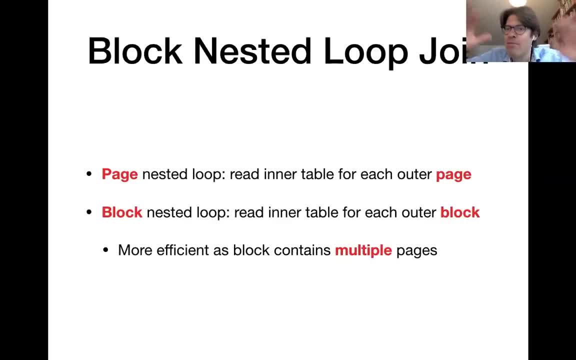 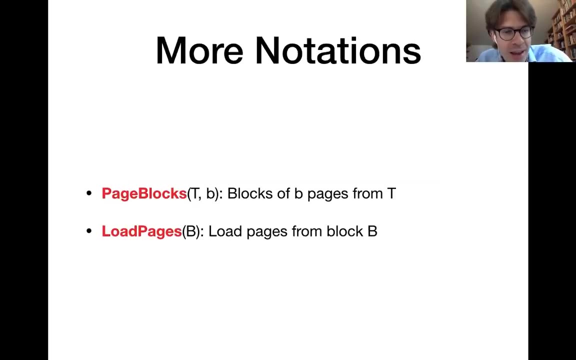 if it can fit that block of pages at the same time into main memory, And since one of those blocks contains multiple pages, doing this should be significantly more efficient than the page nested loop join that we have just seen. So let's see what that looks like and following. 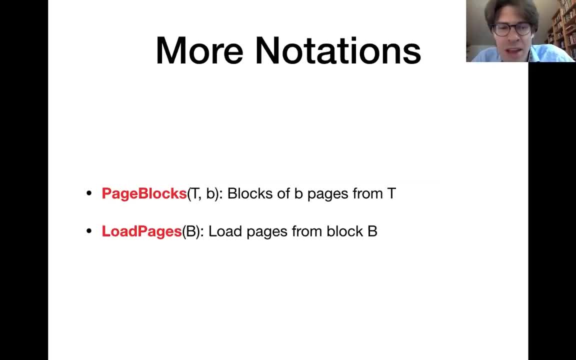 I'm gonna use those notations here in addition to the ones that we have seen previously. So here the notation page: blocks T, comma, B: that essentially is the set of blocks of pages from table T, where each block contains B pages, And also in order to mark the difference: 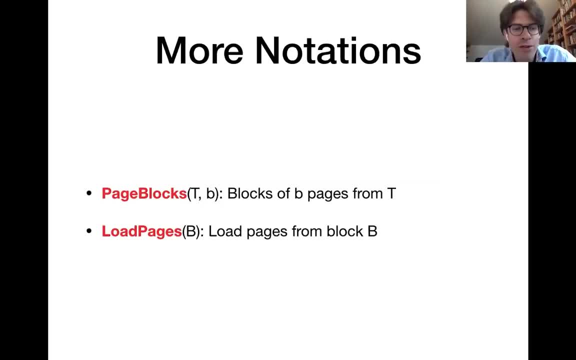 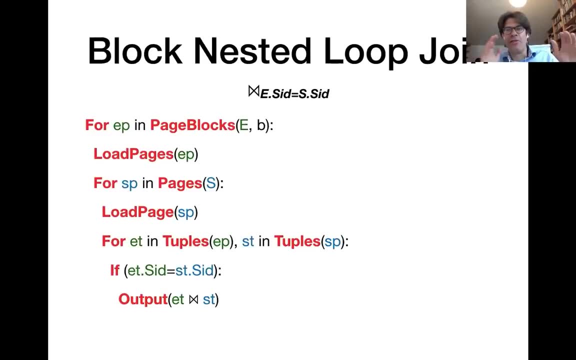 that I'm loading multiple pages instead of a single page. I'm also using load pages, the plural, for one block of pages. All right, so that is the block: nested loop join, And you immediately see that it is kind of similar to the previous page: nested loop join. 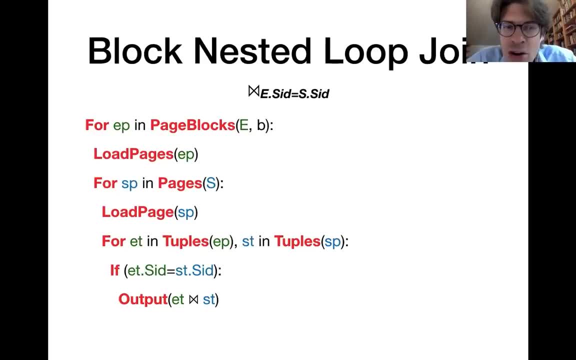 because here we also have two nested loops that iterate over both of B and C. So that's the input table. So we are joining the enrollment table with the students table. And now let's see what actually changed. And what changed is mainly what you have marked up in red here. 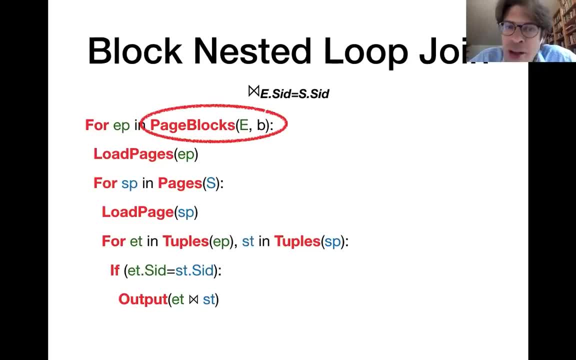 Essentially, instead of iterating over single pages in the outer loop, we iterated over entire blocks of pages in the outer loop And then, correspondingly, in the second line of the pseudocode, use the load pages command for this entire block of pages. 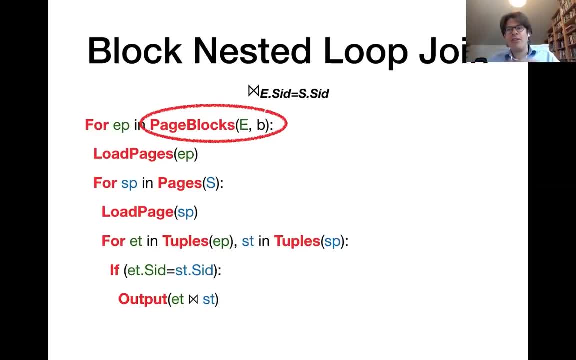 And then correspondingly, in the second line of the pseudocode, use the load pages command for this entire block of pages. All right, now let's analyze how that changes the cost function. So this command over here, actually nothing much changes. I still need to read the pages of the outer relation. 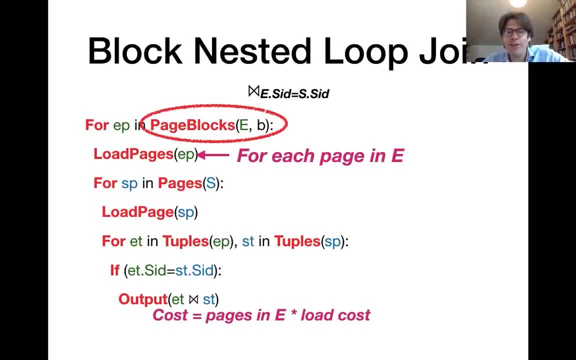 the outer table once And therefore I need to count the cost for pages in the enrollment table times, the loading cost, All right now where the whole thing helps. This is for the second instruction here, because previously I had to invoke this For each page in students and for each page in enrollment. 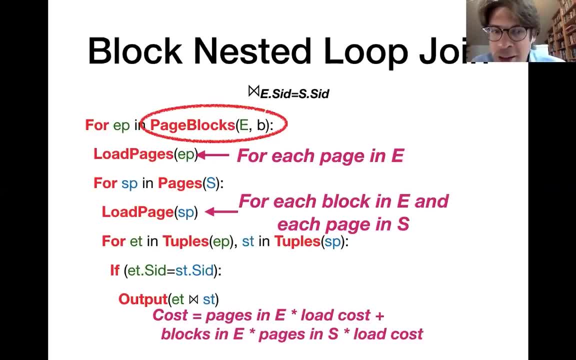 But now I have to only invoke that for each page in students and for each block of pages in the enrollment, And since the number of page blocks is smaller than the number of pages, I'm therefore saving a lot of processing costs, depending on the block size. 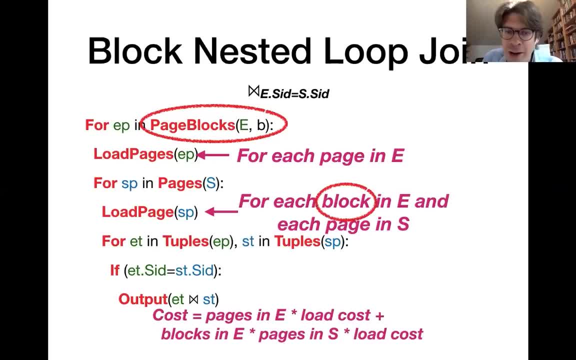 All right. so this is the entire cost function, And essentially the only thing that changes is that here we are multiplying by the number of blocks instead of the number of pages. All right, and this is why that factor also appears in the cost function below. 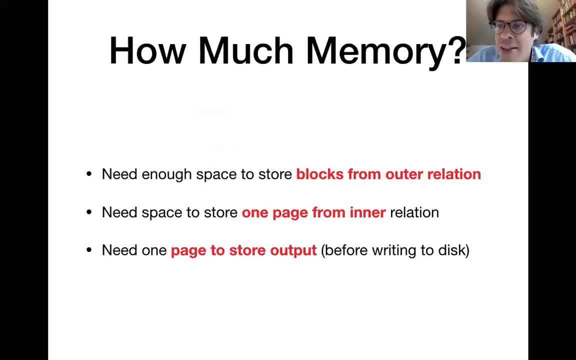 So the trade-off here is that the page nested loop join needs extremely small amounts of main memory. It has a very small memory footprint, which is an advantage. But the block nested loop join is faster And in exchange for that it consumes a little bit more main memory. 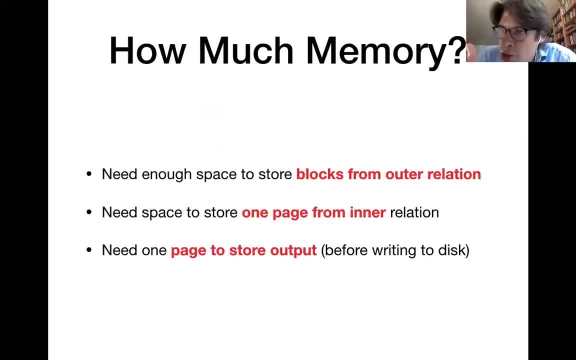 We still need one output buffer page, like before. We also need one page to store the current page from the inner table. On the other side, we need enough main memory to store an entire block of pages from the outer table. So this is what takes most of the main memory. 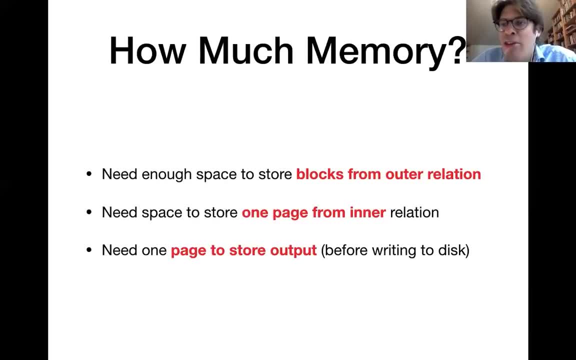 when executing this join And you have a bit of a choice there, because you can choose how large those page blocks should be. If you make them larger, you need more main memory, But on the other side you might reduce the number of iterations. 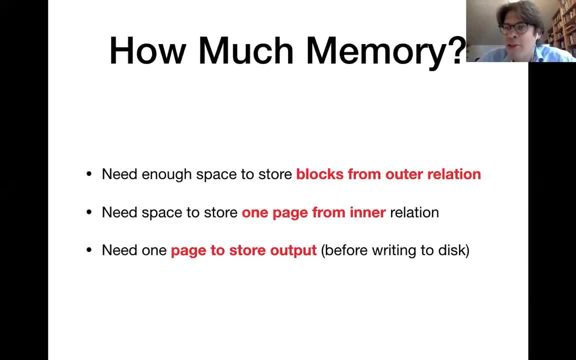 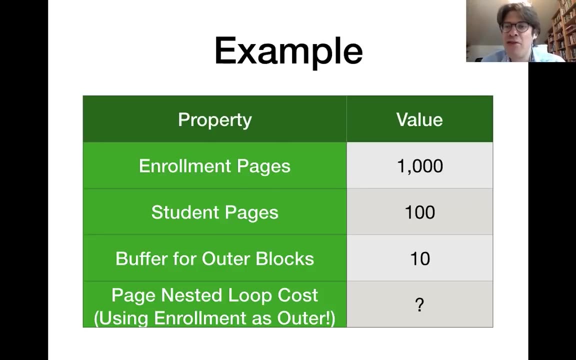 of the inner loop of the algorithm. So there you can trade between times and between processing memory. So let's make a little example. Let's essentially make the same example as before, but this time we assume that we use a block nested loop: join. 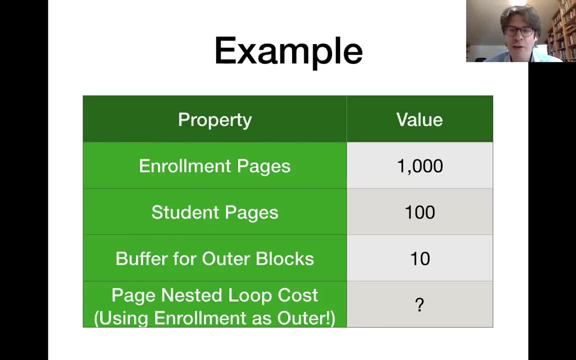 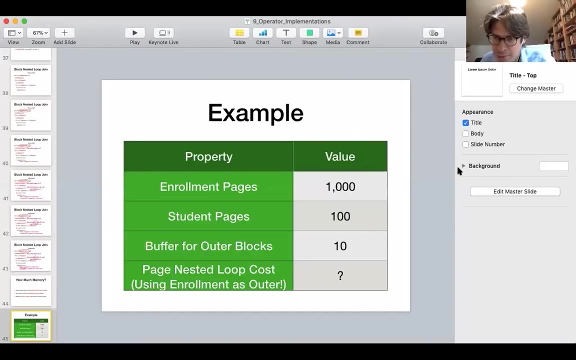 So here we have a buffer size of 10 for storing all the blocks. I'll give you a second to think about how you would go about calculating the cost here, But I'm looking at the chat to see whether there's any questions. Okay, 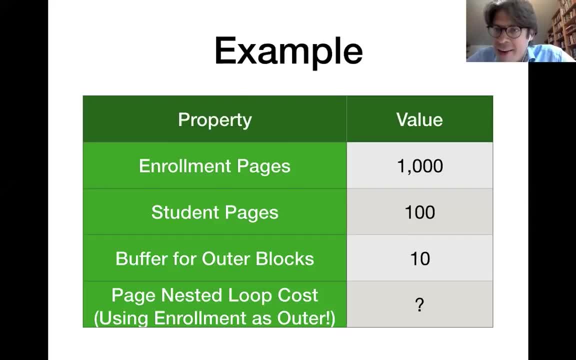 All right, Yes, And here there is a question about why we do not count the cost of writing something to hard disk. So that's a great question. So the only thing that would be written to hard disk? potentially that would be the result of the join. 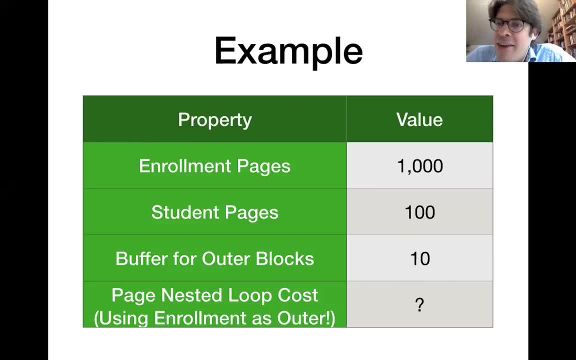 And we have this convention that when calculating the cost for those operations, we do not consider the cost of writing out the result of the operation. We don't write out the count, the cost for writing out the final result of the operation. And the reason for that is simply that 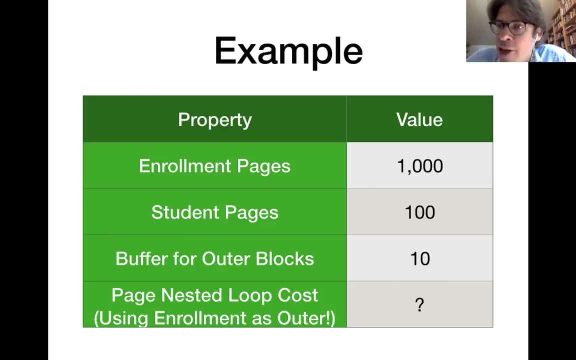 when calculating cost, we always want to compare multiple alternative operations And since all of them are generating the same result, their cost for writing out the result will be the same. So that is why we do not count it, because it would be constant for all the different alternatives anyway. 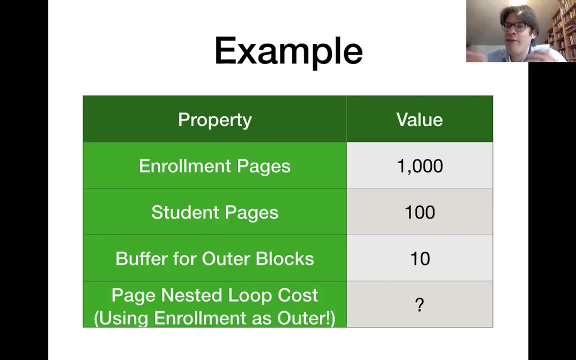 And our main goal with those cost calculations is always to compare different operations, different implementations for the same operator. So in practice of course you might have some cost associated with that, even if you are not considering it by convention, Of course. 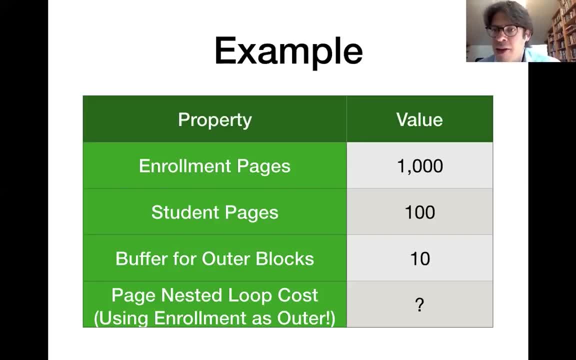 it depends also on the context of the operator. For instance, maybe you only want to count the number of uh join results, but you don't actually want to produce the join results. In those cases the output of the join would never be directly written to hard disk. 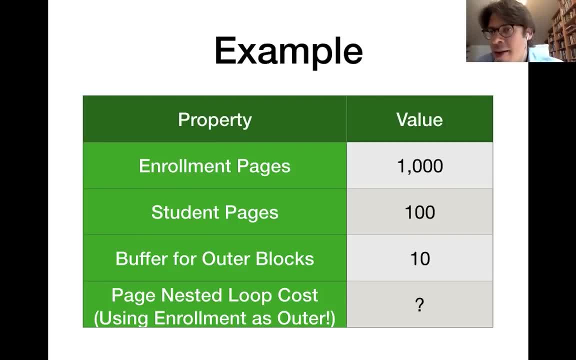 but it would only be counted. In that case you wouldn't have any output cost. So it depends a little bit on what next steps we want to take based on the join output, And here we don't consider the output cost at all. 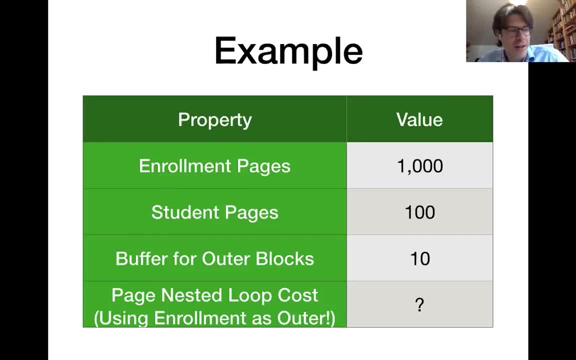 All right, So let's have a look at the solution to the example. So, um, what we have here is that, essentially, we still need to read the enrollment pages. So here we still consider enrollment as an outer table for consistency. Uh. 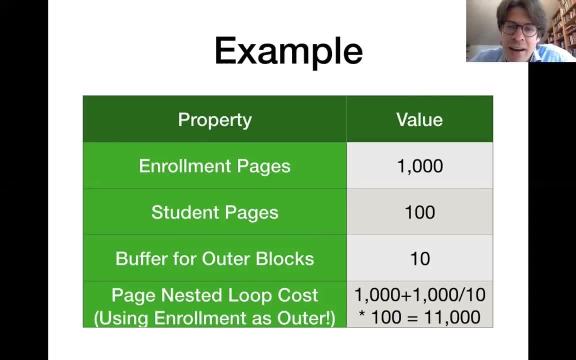 but then the number of times that we read the uh student pages is reduced. We have a blocks of size 10 and we have um. we have a thousand um pages. So we divide the 1000 by 10,. 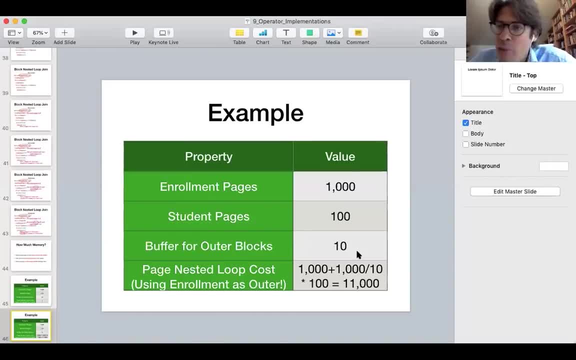 and then we uh multiply it by the number of pages in the student's table, which is a hundred. So here we have reduced cost compared to the page nested loop. join uh from something over a hundred thousand to 11,000. 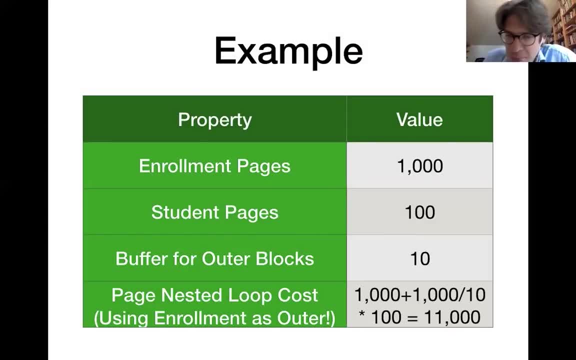 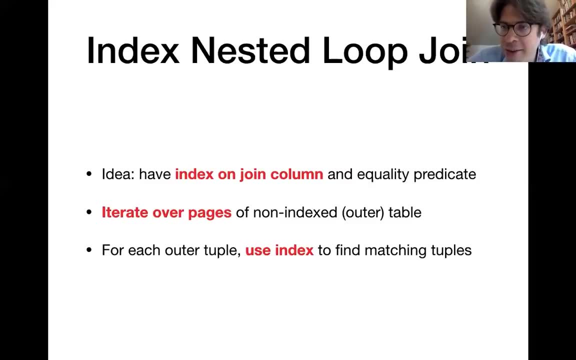 So roughly by factor 10.. All right, Now one final nested loop join variants that I want to discuss today. That is, the index nested loop. And, uh, we have already seen that indexes can be useful in order to um, in order to execute filter operations. 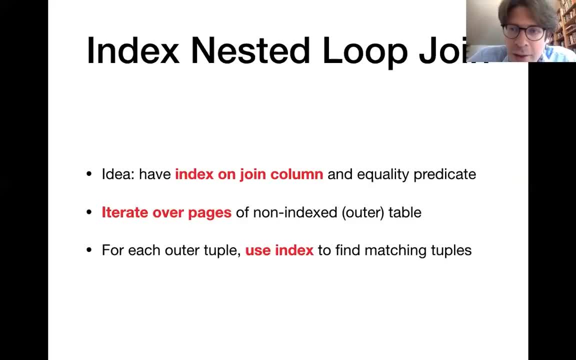 You can also use them in the context of joints And the main idea here is that I have, uh, an index on the joint columns for one of the two columns, Uh for one of the two tables that I'm joining, And I assume that the joint condition is an equality predicate. 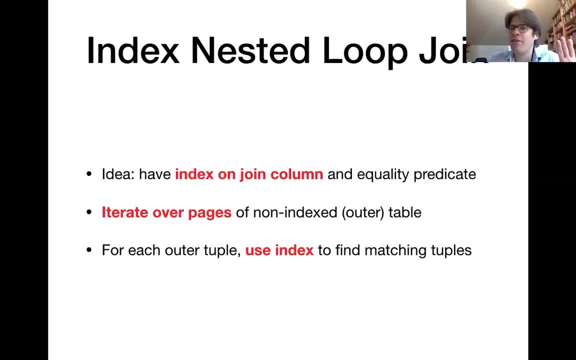 which is the case in our example where we have an enrollment table and the students table and we want to find uh pass of couples that match on the student ID. So student ID from enrollment equal to student ID from the students table. 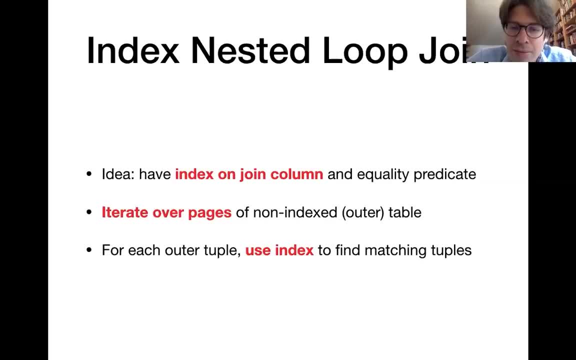 So therefore it is an equality joint predicate. And now if I have an index, for instance the student ID, I can exploit that one during the join, And the main idea to do that is that I'm simply iterating over the pages of the non-index. 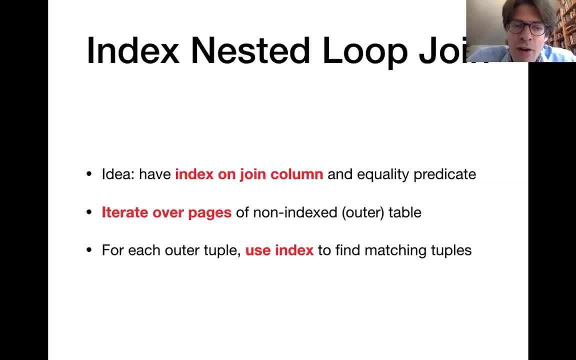 the outer table And then, for each entry on one of those pages, I use the index in order to retrieve the matching tuples from the other table. In order to make this work, I first of all need a joint with an equality joint condition. 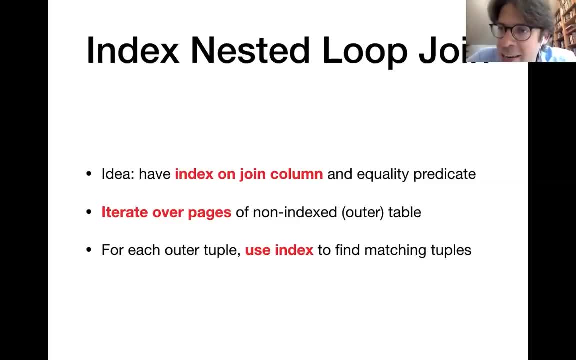 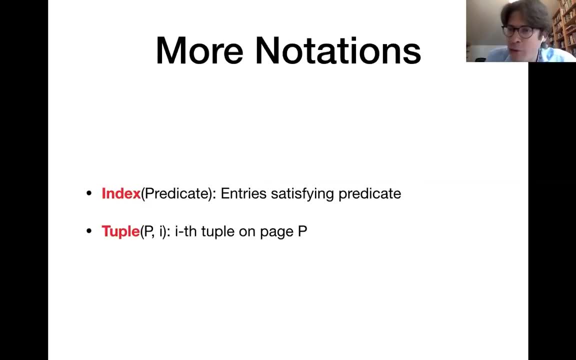 And also I need to have an index on the correct table and the correct column. Let's see in more detail how that works like, And here, in addition to the notations from before, I'm also using the notation index of predicate. 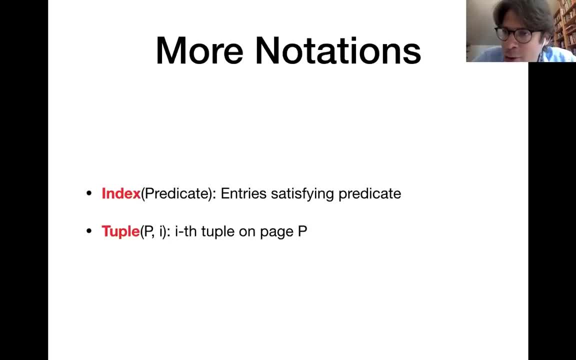 which essentially symbolizes an index. look up in order to retrieve all the entries satisfying the predicate in parentheses. And uh. here I'm also using the notation tuple P, comma I, uh, in order to designate the tuple number I on page number P. 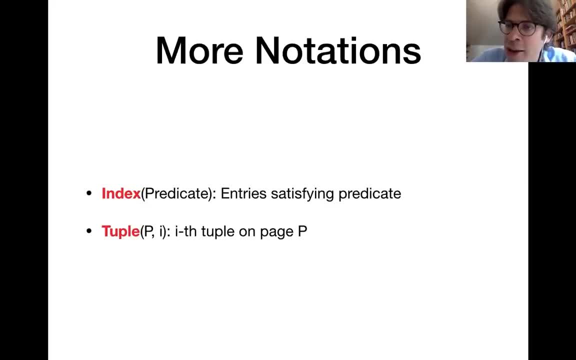 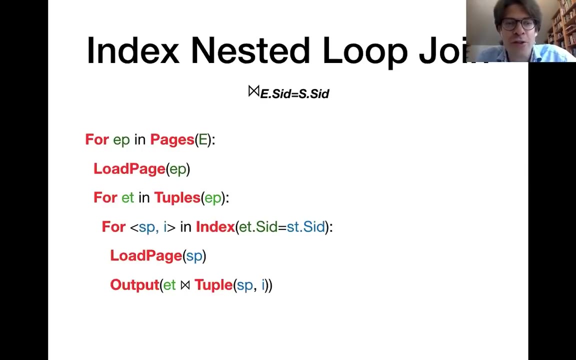 because, while I'm getting back from the index, that will be those record IDs which, as we have seen before, always consists of a page ID together with the corresponding slot number. Now, this is how the algorithm looks like. So again, we are iterating over the pages of the enrollment table in the outer loop. 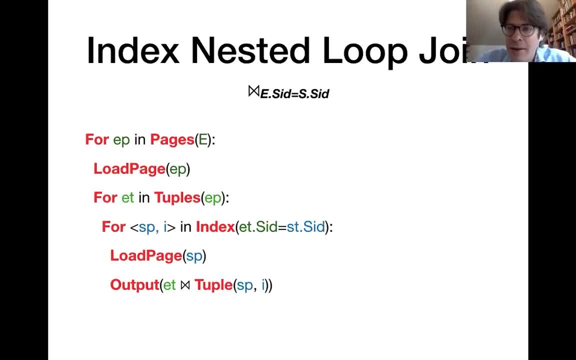 and we load each of those pages. Then, for each tuple on the currently loaded page, we consult the index in order to retrieve matching tuples from the other table. So in this case, more concretely, we have one enrollment, tuple um. 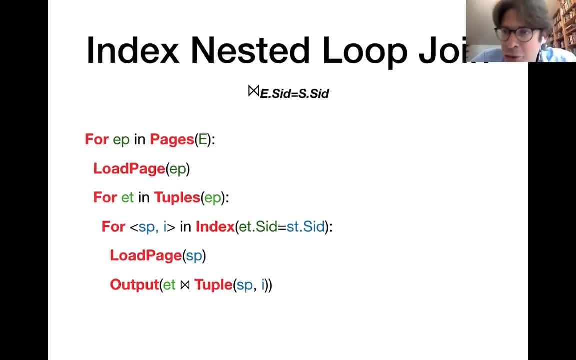 and that enrollment tuple contains a course ID and a student ID And uh, I can use the index in order to uh retrieve the entries in the student table with the corresponding student ID. So, and once I have found that, I load the corresponding page and then I add the tuple combination to the output. 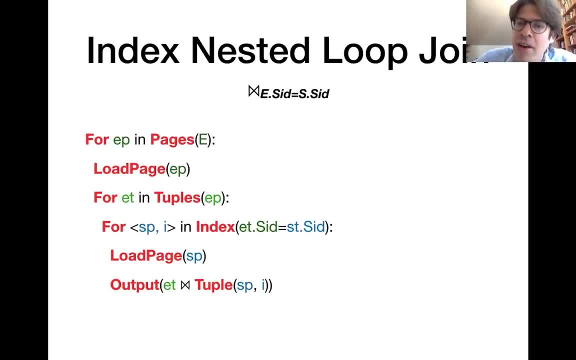 In the previous joins we always had this if condition because I had to verify whether the join predicate holds. Now, if I'm using the index here, then, uh, I am essentially guaranteed that this join condition is satisfied, So I don't even need to check anymore. 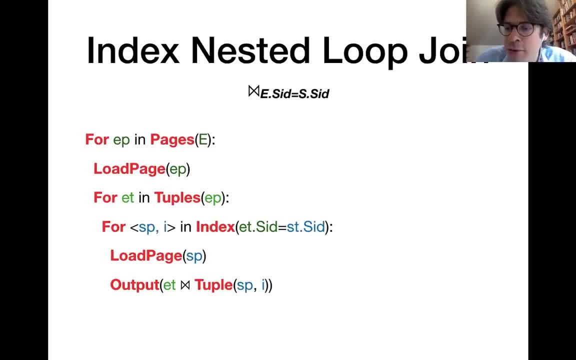 Just add the tuple combination to the join result. All right, And uh, if I count the the cost uh for that uh index over here, then uh, of course, here again I'm loading each page from the enrollment table once. 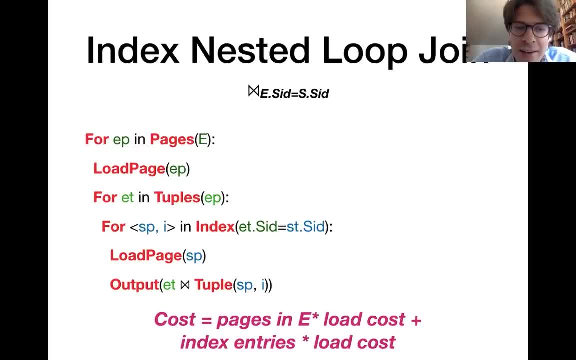 And uh, also, for each uh indexed entry that uh my index is returning to me, I need to load the corresponding page Now, uh, the cost of that depends a little bit on where uh those index. 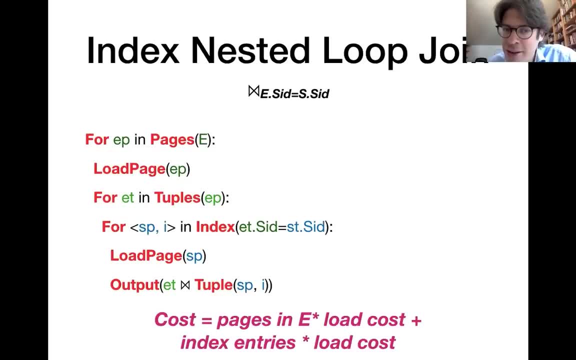 those index entries are distributed on hard disk. If you're very lucky, then those entries are clustered together, or uh, at least approximately. And uh, that means that, uh, since we are using the buffer manager, um, we can essentially 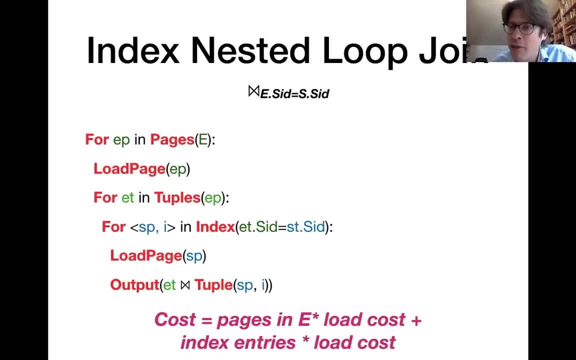 uh reuse previously loaded pages quite a lot of times, But, in order to simplify the cost analysis, we typically make the assumption that uh each page that we are uh retrieving for an index results tuple, each of those pages is located somewhere else and we have to load it for the first time. 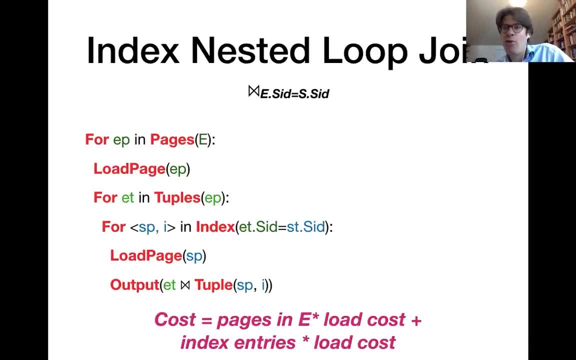 So, uh, this is why, typically, we would just count the page loading cost times, the number of entries returned by the index, in order to get the access cost associated with the second load page command in the pseudocode. Of course, all of those cost formulas make simplifying assumptions, as you see. 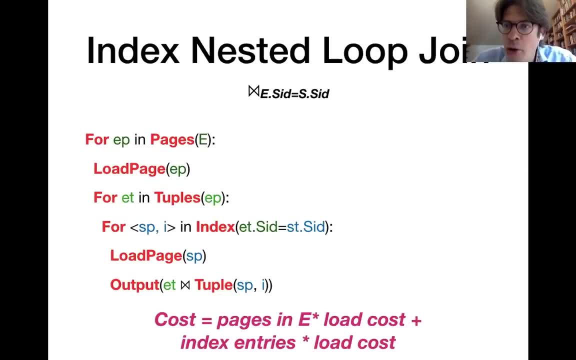 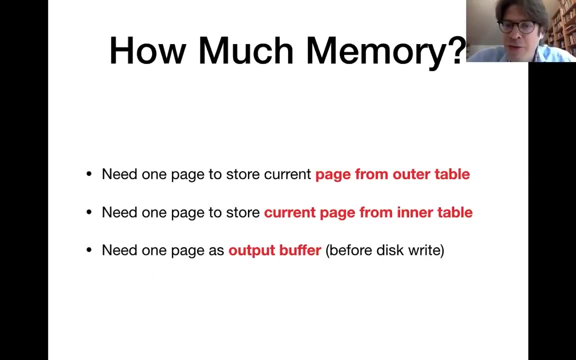 But uh nevertheless, um, they often allow you to at least make some rough estimates in order to uh determine that one option is significantly better or significantly worse compared to a different option. Now, in terms of uh main memory consumption, 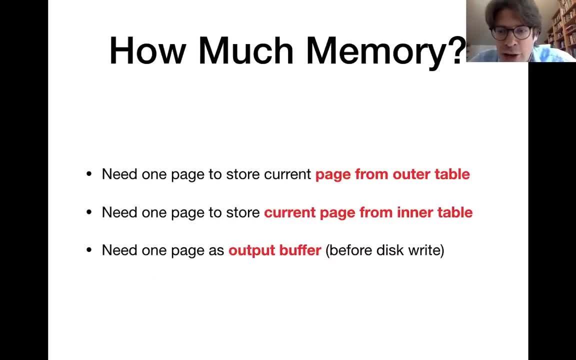 that algorithm is also, uh, quite reasonable, but we just need one page to store the current page from the outer table and then one page to store the current page from, uh, the inner table, And uh, furthermore, we need our 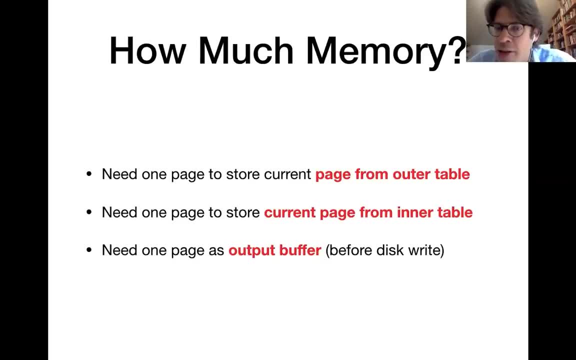 uh, typical output buffer page. So altogether three pages should be sufficient Here. of course I'm not uh counting any storage for the index. The index would be typically uh stored on hard disk, All right. 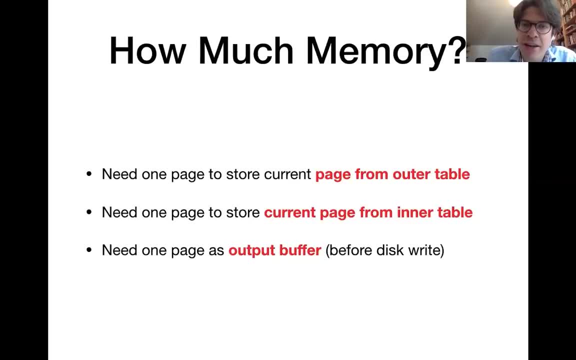 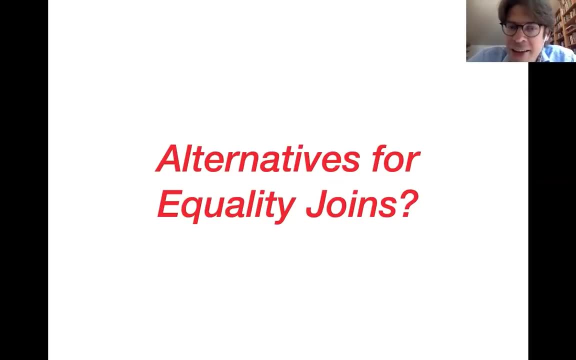 So, um, those are the joint algorithms that I wanted to uh discuss today. Um, perhaps you can read, uh, uh, perhaps you can already think a little bit about other things that we could exploit in order to make joins with equality conditions. 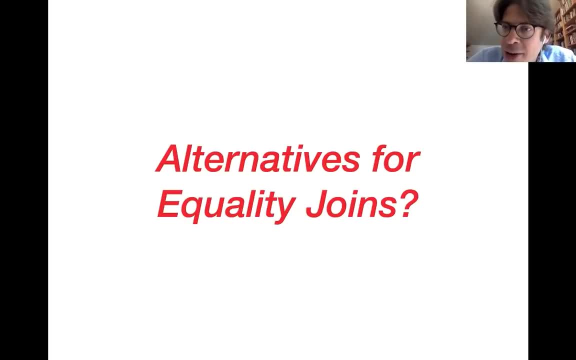 uh more efficient. or you can just uh look at the next slides uh, which are already online. Um, in the next lecture, we're gonna discuss about a couple of more sophisticated joint algorithms that uh specifically apply for equality joint predicates. 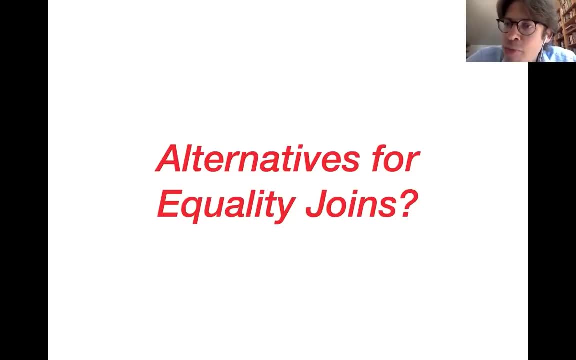 Um, but uh, we're not going to go over all of those, uh, but we're going to talk about, uh, the very basic ones that we've covered, which are the nested loop joins. They are very vers-, those nested loop joins. 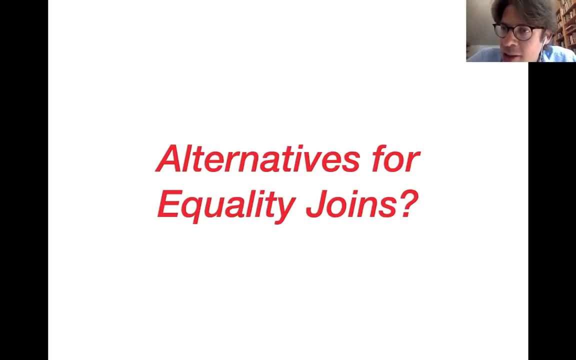 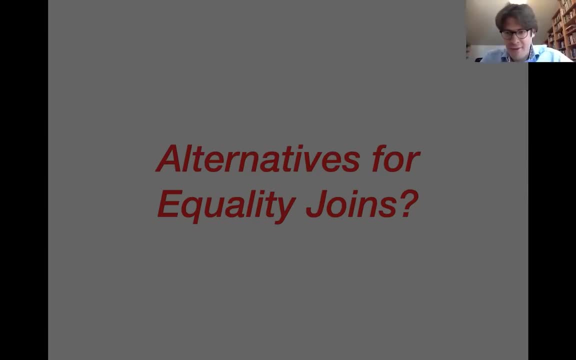 in general, they are quite uh versatile and they are uh heavily used in uh database management systems also, for instance in Postgres. All right, You see there's like one question in the chat. 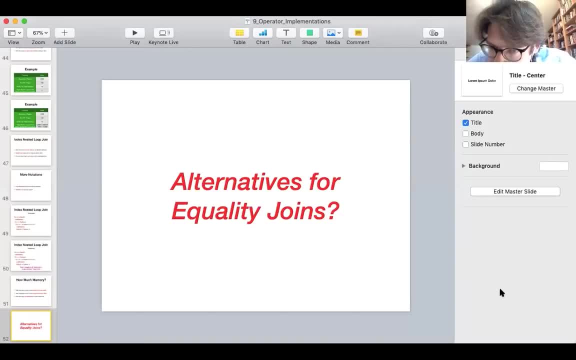 I'm going to answer this one and then uh. all right. So here the question is whether the data is useful in the database. Uh is whether there's other joint predicates than equality joint predicates. that's a well justified question, thank you. so in practice, by far the most common joint condition is indeed equality. 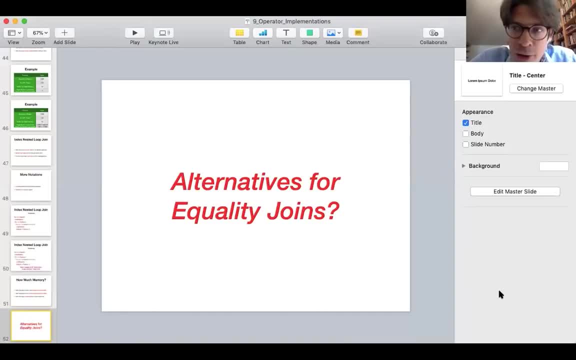 joint conditions and in most of the examples that we have seen here, if not all, we have used the joint conditions and equality joint conditions. now, in principle, you can also use different joint conditions. you can essentially use arbitrary joint conditions and, even if that happens less frequently in practice, every once in a while you have a join with non-equality joint conditions. 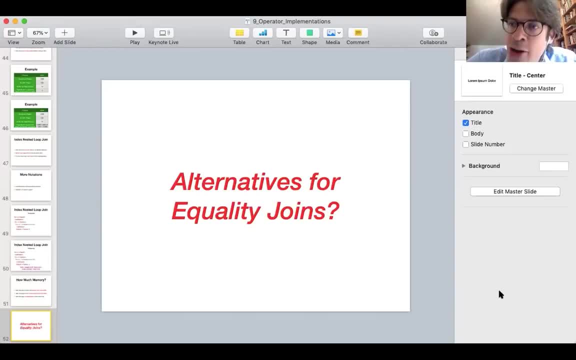 that is why it is very important for database management system to support some join operators which can deal with non-equality joint conditions and, for instance, the page nested loop or the block nested loop join. they have that property that they can deal with arbitrary joint conditions. okay, good, have a nice day and then i see you again on friday. 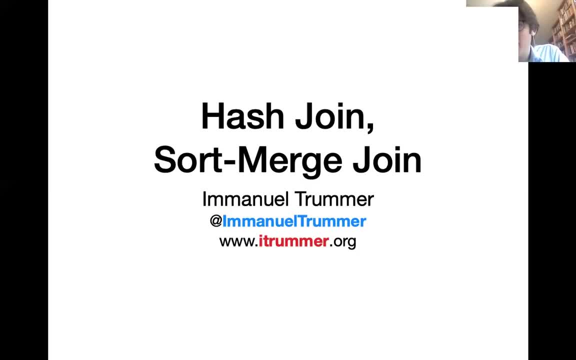 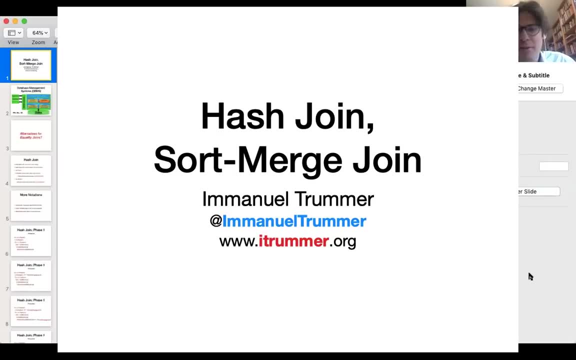 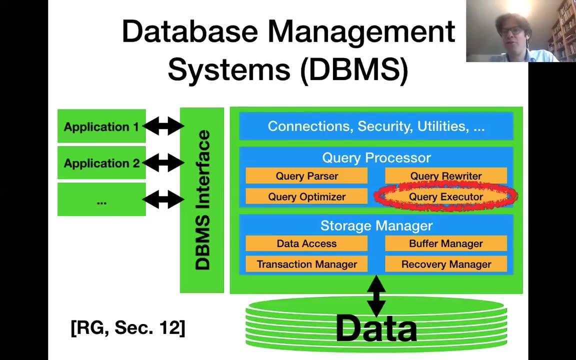 all right, let's get started. and uh, currently we are discussing about- and again, i clicking to make sure that my slides advance, all right, so currently we are discussing about the engine and, more precisely, discussing about how the standard operators for data processing are implemented, and the relevant chapter is still Ramakrishnan. 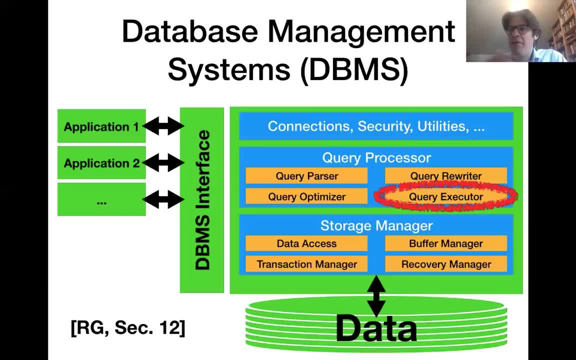 and Gerke, chapter number 12.. So we have discussed about a couple of operators for filtering and for joins in the last lecture For joins, we have been discussing about those nested loop join variants which typically have two nested for loops that iterate over the two input relations, and then they try to 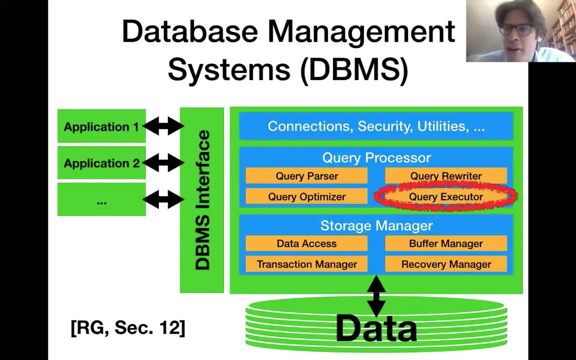 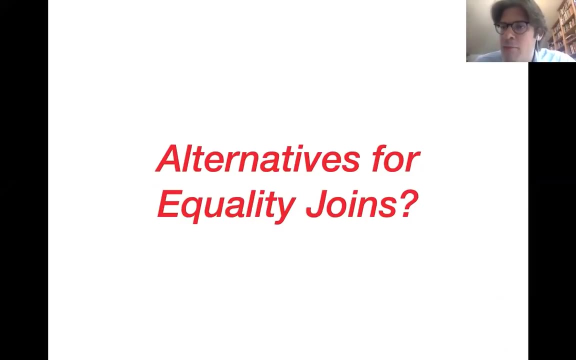 find matching tuples. Now in this lecture we're going to discuss about two more join operator implementations. They are very, very popular in practice and are, for instance, also implemented in the Postgres database system. Now, those join operators: they apply in cases where our join condition is an equality between a 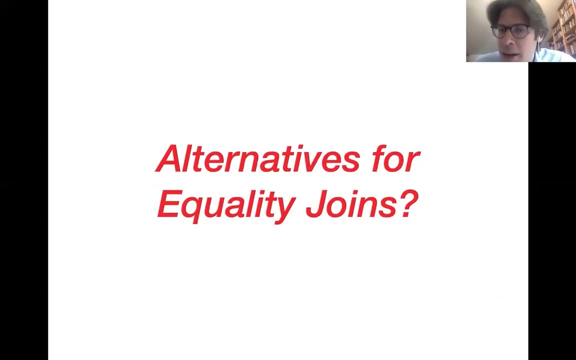 constant and a non-constant. So in this case we are talking about the, for instance, also implemented in the Postgres database system. They are very, very popular in practice and are perhaps the most typical case in practice. Now it's time I asked you to. 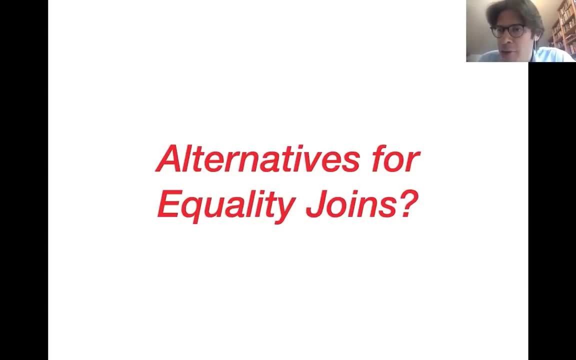 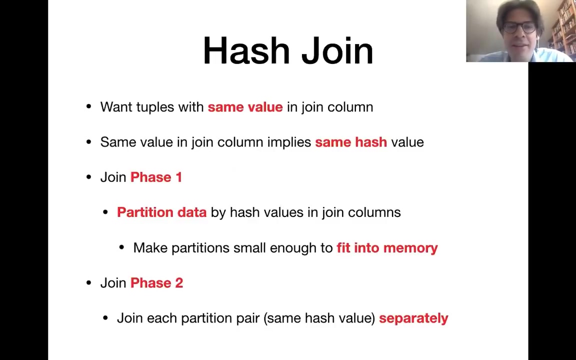 think a little bit about what we could exploit in order to make joins more efficient in those cases, and the first possibility that we can exploit is to use hashing. Now, the first new join that we will discuss today, that is the hash join, which uses a hash function in order to speed up the 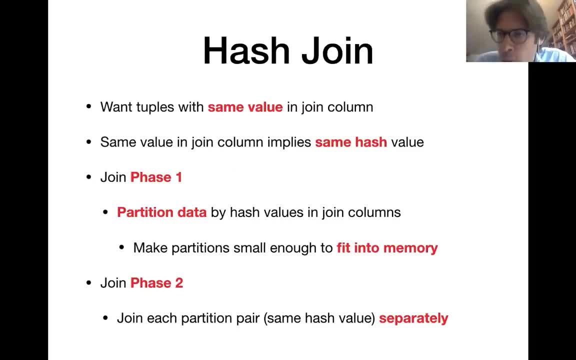 join. So we are now focusing on equality join conditions. that means we want tuple pairs which have the same value in the join column and, of course, if they have the same value in a joined column, it means they also have the same hash value in a join column for an arbitrary hash function. So we exploit this as 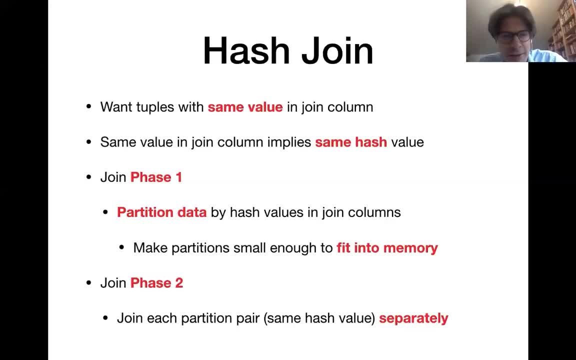 follows now. the hash joint has two phases. in the first phase we essentially partition all the input, both input tables, using the hash function. So first of all we essentially make one pass over both input tables, then we apply the hash function in order to partition that data into buckets. 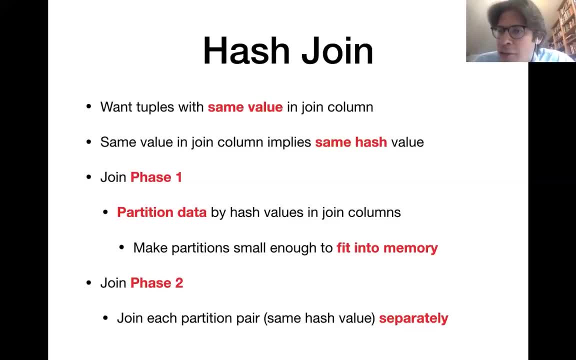 that are associated with a specific hash function- values, And we try to partition the data into sufficiently small partitions such that one of those partitions fits into main memory. That's what we need, Because in the second phase of the join we will go over those hash value buckets one by one. 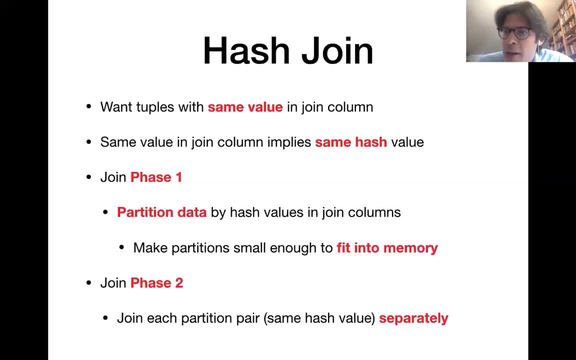 And for each bucket, we will load one of them entirely into main memory in order to join the corresponding tuples separately. We can do that Because, since we are looking for tuples with the same value in the join column, they must be located in the same hash bucket. 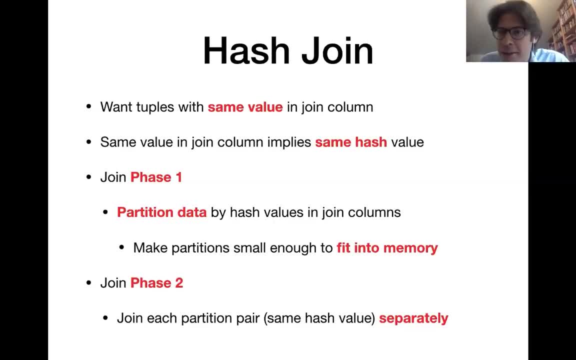 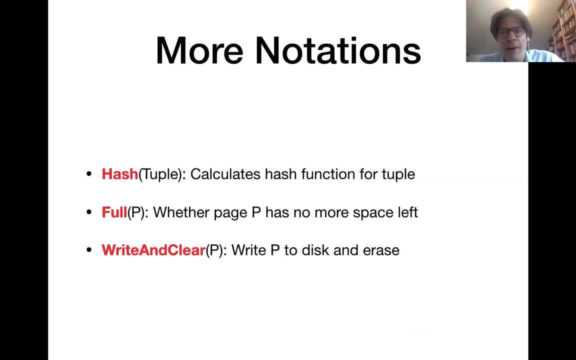 This is what the join exploits. Now, that is the high level overview. Now let's see some pseudo code. for that, I introduced some new annotations. First of all, quite intuitive, the hash function, which calculates the hash function for a tuple in the join column. of course, 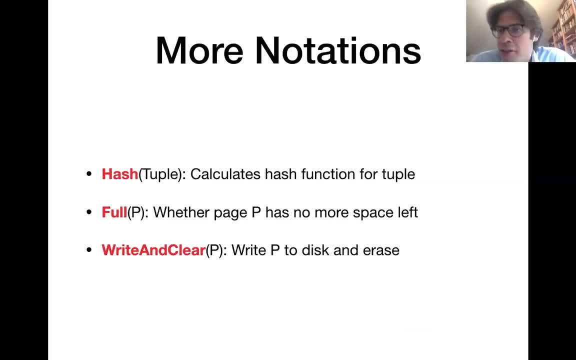 Then I introduced the full predicate, which essentially tests whether one page is completely full and has no more space left for insertions, And then I introduced the write and clear function over here. So that is used for the output buffers And it essentially does two things. 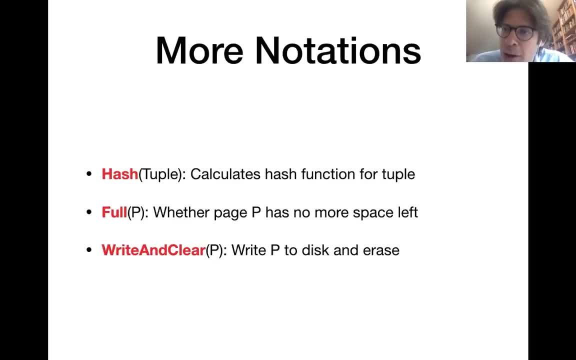 First of all, it copies the current content of the output buffer to hard disk, And then it clears, it erases the content of the in-memory buffer Such that it can consume new entries. All right, and with those notations and the ones that I had introduced the last time, 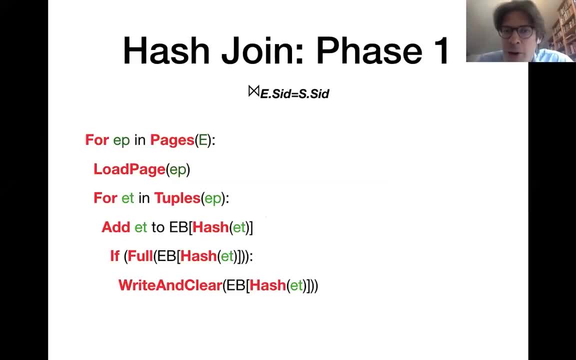 this is the pseudo code for executing phase one. in this example, join between the enrollments and the students, And we want to find a pass of tuples where the student ID is the same. So here, first of all, we are going over the pages. 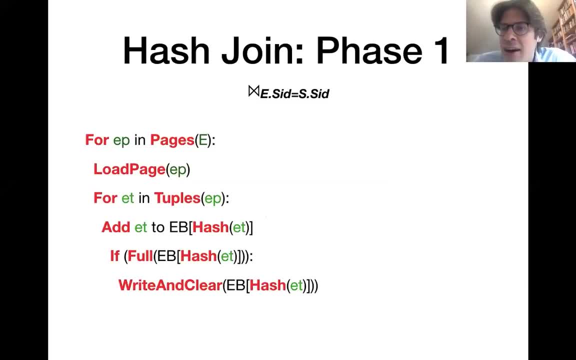 of the enrollment table. We are sorting, we are partitioning those tuples using the hash function. So here we go over the pages of the enrollment relation here, For each page we load it from hard disk, of course, And then we iterate over the tuples on that page. 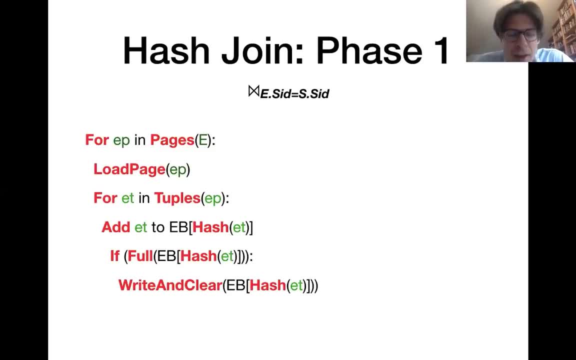 which we have just loaded, For each tuple, we are adding it, We are essentially copying it to the output buffer that is associated with the associated, you know, selected- hash value, And if the output buffer becomes full, then we clear it and write the content to hard disk. 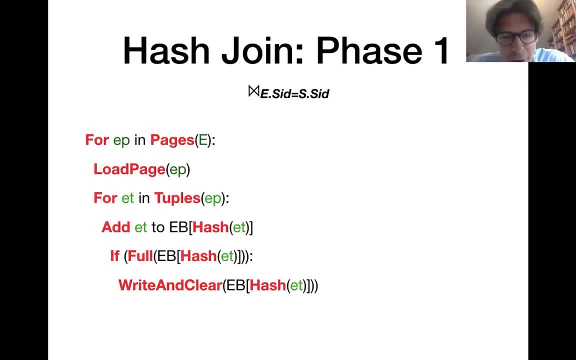 First write the content to hard disk, then we clear it, of course. All right. So this is the first phase of the join, in which we partition tuples by the hash function And we apply it here to the enrollment table. You will see the student table in a second. 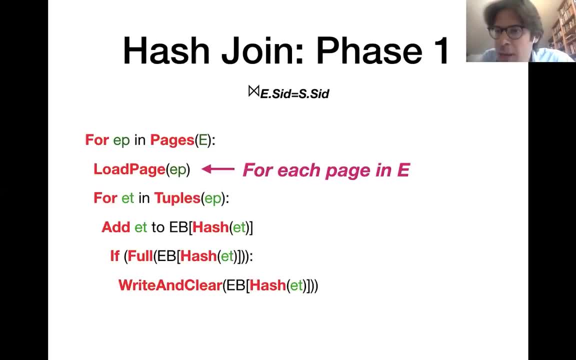 Quickly reasoning. we have to talk about the cost. So this load page command that is involved once for each page in the enrollment table, And the other one here, the write and clear command, also writes one page to hard disk. So that also costs us something. 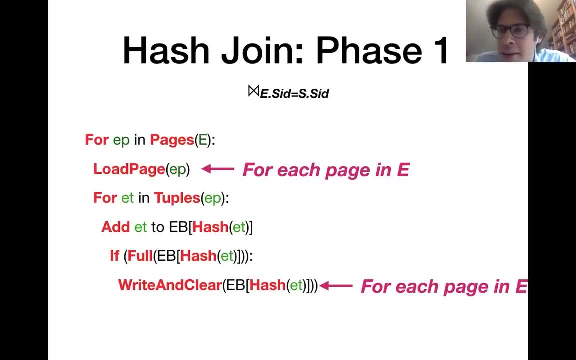 And since we just partition the data, the size of the input is the same as the size of the output, which means that this one, the second one, the third one, the fourth one, the fifth one, the sixth one, the sixth one. 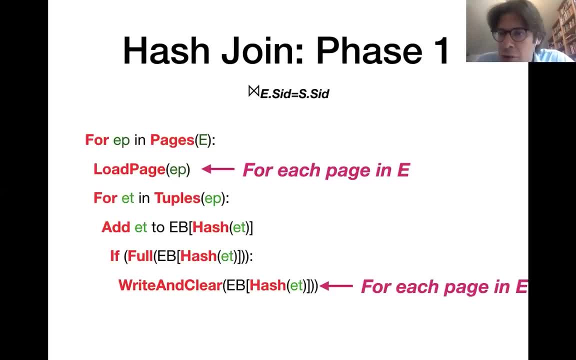 we call them to the measurement table And this second call is also executed once for each page in the input table. All right, So we have said that we measure costs only by the number of pages that have been read or written to and from hard disk, right? 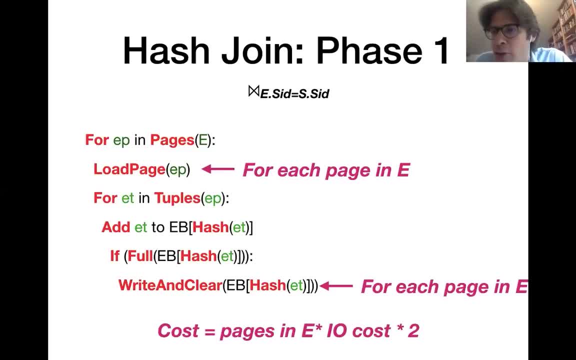 So in this case the cost is simply two times the number of pages in the table that we are partitioning. Now, here I'm partitioning the enrollment table. I also need to partition the other one, that is, the student table. that is the correct slide. so here I'm simply doing the same thing. 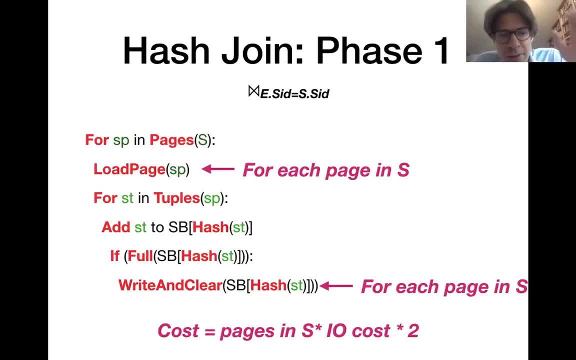 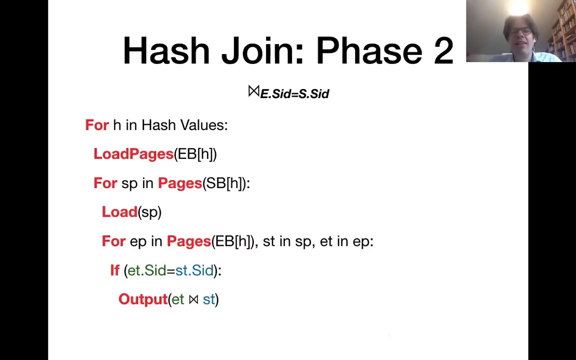 that I did before, but for the student table, to rating over the pages, partitioning them by the hash function and writing those output buffers to hard disk whenever they become full. all right, so now I have partitioned both my input tables by their hash function in the joint columns now in the second. 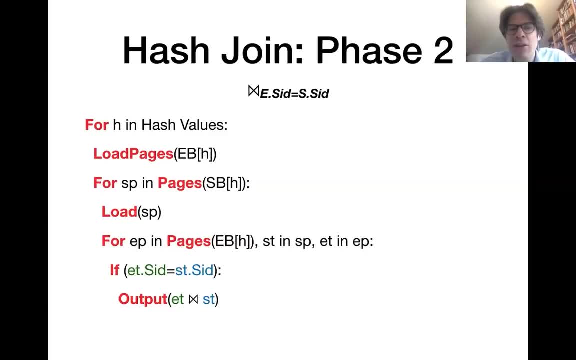 phase I'm treating each hash bucket one by one. so I am iterating over the possible hash buckets and for each of them I am loading entirely the associated tuples from one of the two input relations. so here I have decided to entirely load the pages for the current hash bucket for the enrollment at table. 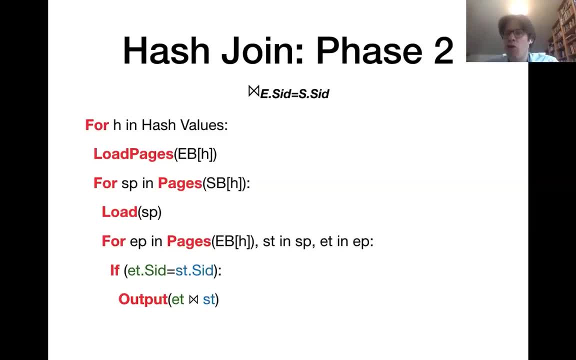 and after I have loaded the complete hash bucket for one of the input relations in domain memory, then I'm simply iterating over the pages from the other table, one by one. I'm iterating over the pages from the studio Jaum Management麽 table And I only need to consider those pages from the same, from the corresponding hash bucket. 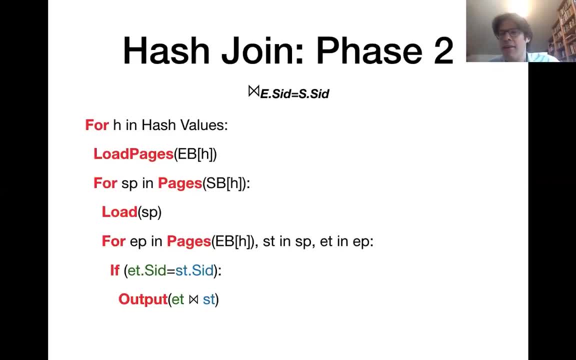 that is associated with the current hash value. And then, for all the tuples that I have in my memory, I compare them and I evaluate the join condition. I still have to do that, because just because two tuples belong into the same hash bucket, it does not yet mean that they have the 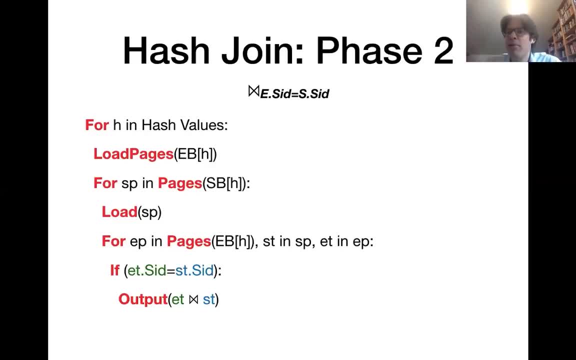 same value in the join quality, because typically multiple values get hashed to the same value. All right, And then I simply output the tuple pairs that match together. Okay, And here there's a great question in the chat. Okay, And there's also a great answer in. 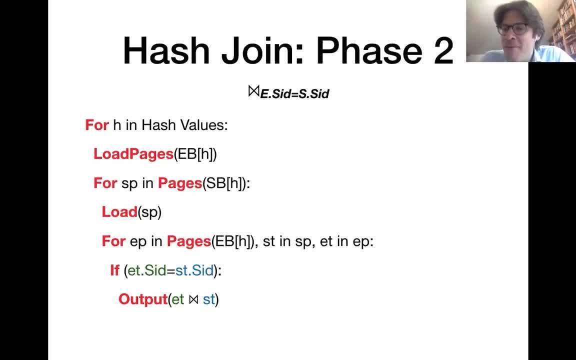 the chat. Okay, I quickly addressed that. So the question was: we have said that we typically don't count the cost for writing out the output of an operation, because it doesn't really help us to compare different implementations for the same operation, because the output is always the same. 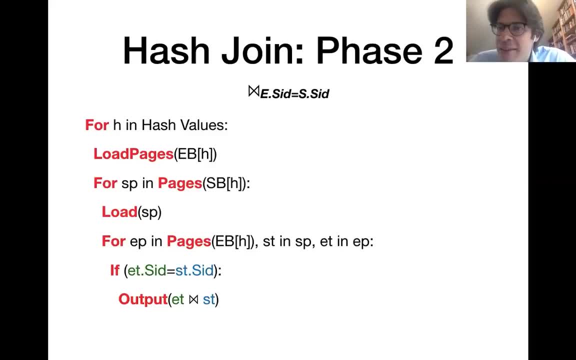 Now, in this case we have counted cost for writing something back to hard disk. Now the difference here is that what we are writing out is not the final result of the join, but it is just an intermediate result. So if you compare the hash join, for instance, 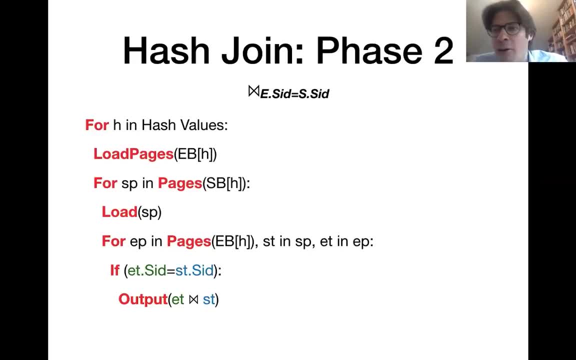 against the blockness, the loop join, that one doesn't write out some intermediate result which partitions the data according to hash value. So that's why, when comparing this join operator to other join operators, we want to count the cost for writing out those intermediate results. 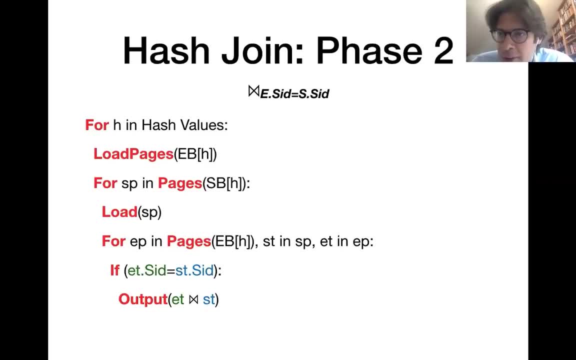 but we do not want to count the cost for writing out the final result. Great question, All right. So in the second phase of the join we join each hash bucket separately And afterwards we produce the complete join design. And if you look at the cost, 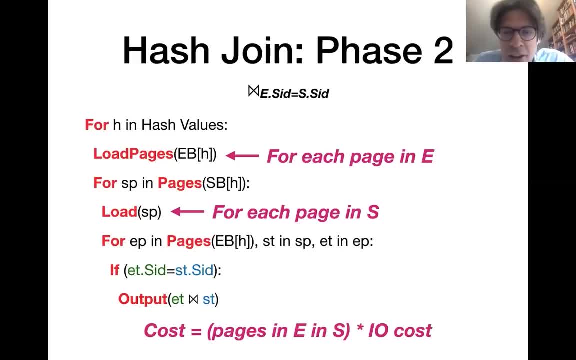 then the first command that is executed for each page in the enrollment table and the inner one is executed for each page in the student table. So maybe it makes sense to have a second look to verify why that is the case. But of course each page of the student table. 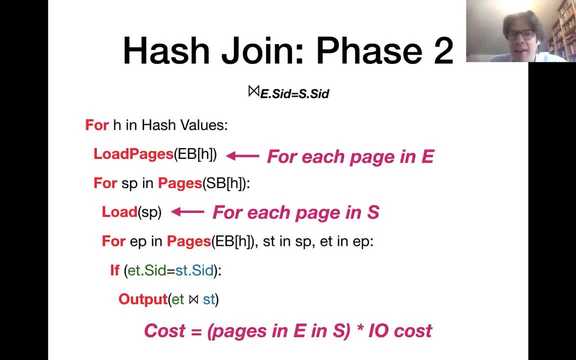 can only be in one of those hash buckets. So if I count together all the times that this command is invoked, then still I come back to the number of pages in the student table. All right, And this is why the total cost of this 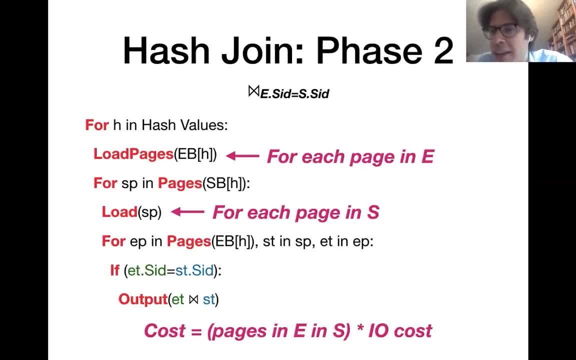 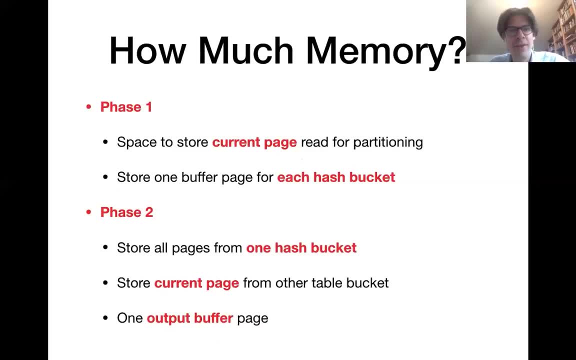 is essentially the number of pages in both the input tables, And I don't count the cost for writing out the result of that. Now let's quickly think about how much main memory we need for that. So we will be discussing a lot about main memory consumption today. 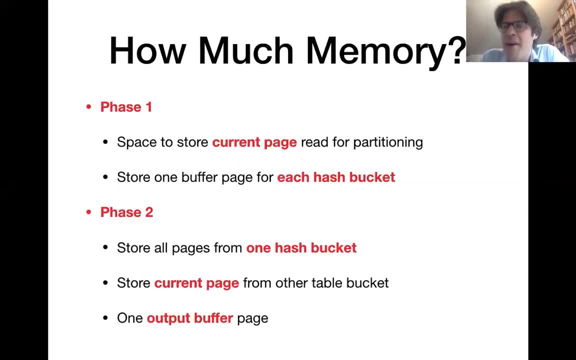 because, together with runtime, that is a very important metric in the context of large-scale data processing. So for this join operator, in the first phase of the join, we first of all need to reserve one page in my buffer pool which, as a little reminder, 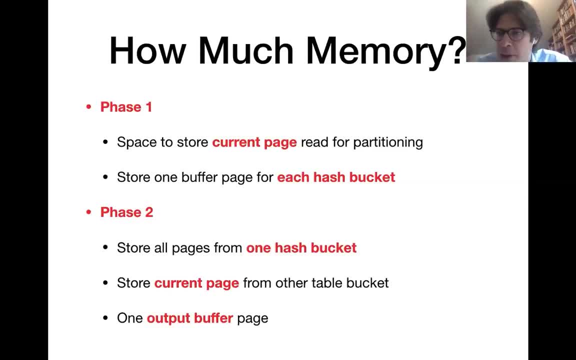 is the part of main memory, which is the main memory of the data, is the part of main memory, which is the main memory of the data. So I need one page in main memory reserved for the database management system. So I need one page in memory. 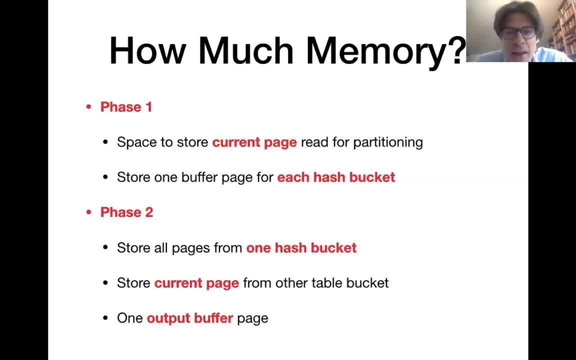 to store the current page for partitioning, And then I want one output buffer for each of the hash buckets. So, as we will discuss in more detail later, the more hash buckets I want, the more pages in main memory do I need to reserve for this first phase. 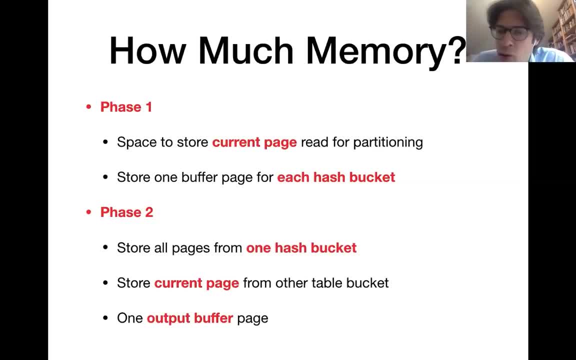 In the second phase I want to store all pages from one hash bucket from one of the relations. So in order to minimize main memory consumption I typically want to choose the smaller table for that And also I need to count one page for the current page from the other table. 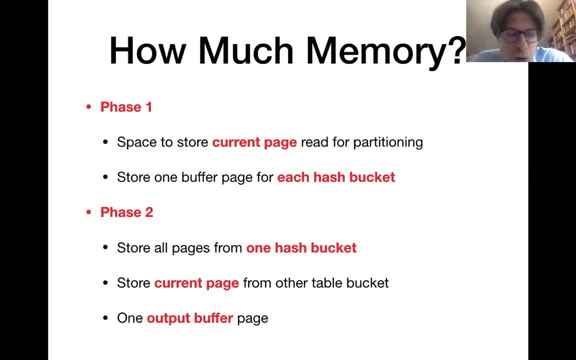 And then I still need one output buffer. So here are the number of hash buckets plus two. basically, That's how many main memory pages I need. Now there's a couple of questions that I would like to ask you, So the first one is: 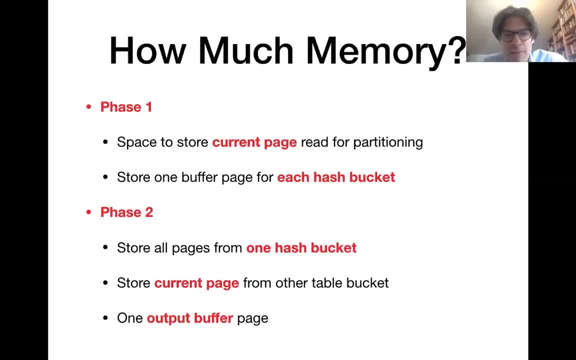 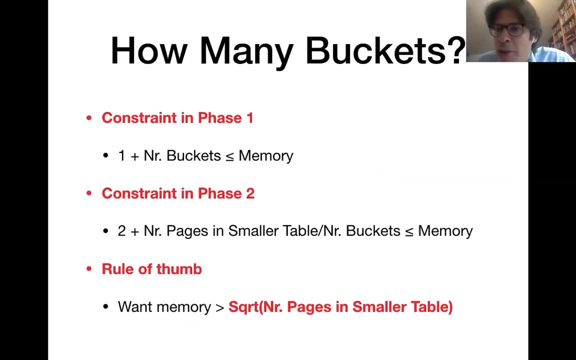 how many hash buckets do I need? And then the second one is: how many hash buckets do I need? And then the third one is: what are the constraints in terms of how much main memory I want? at least, let's say So first of all. 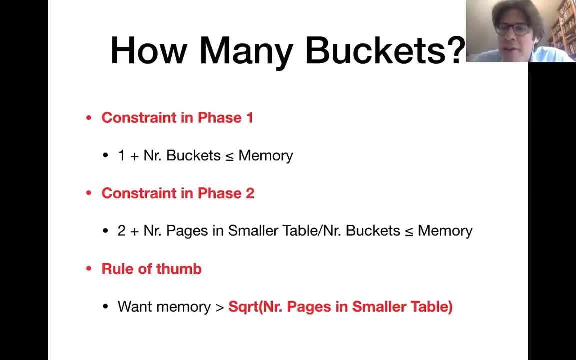 in the first phase, I essentially want one more page than the number of hash buckets. Also, in the second phase, in order to be able to load one partition entirely into main memory, I want to make sure that those partitions are small enough in order to fit into main memory. 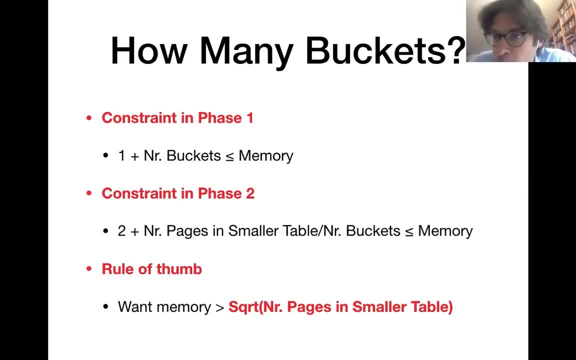 Now, if I assume a perfectly uniform distribution of data over hash buckets, then I can say that the size per hash bucket is simply the number of pages, let's say in the smaller table, divided by the number of hash buckets. That is the expected size. 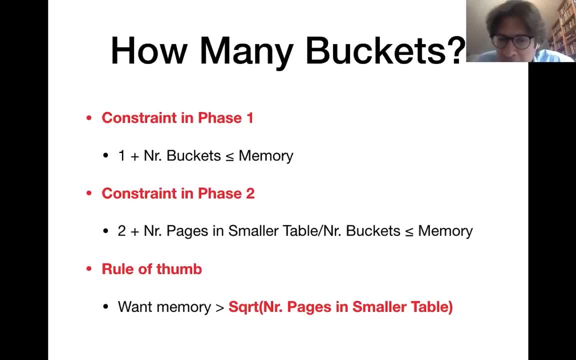 of one of those hash buckets And therefore, in the second phase, one of those hash buckets plus the input buffer and output buffer plus two, is small or equal to the amount of main memory that I have And as you can verify by some calculations. 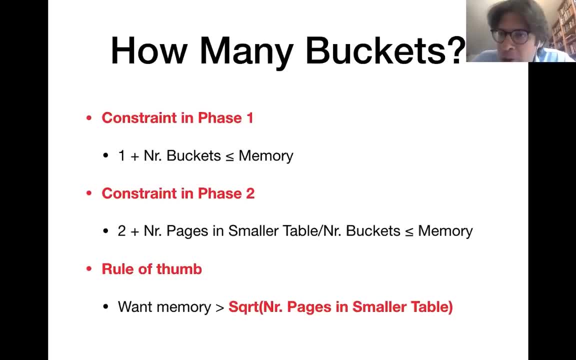 that I won't do here, but there is a rule of thumb that makes sure that those two conditions are satisfied, and this is that we want. the amount of main memory available is a little bit greater than the square root of the number of pages in the smaller relation. 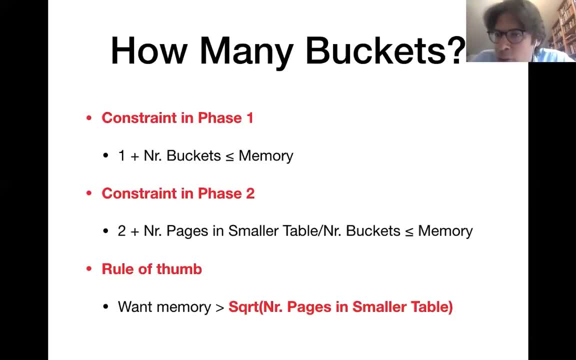 So if you have a number of hash buckets that corresponds to the square root of pages, then you expect the size of each hash bucket is a total number of pages divided by the square root, and that again is the square root of the pages, Then both of those conditions- 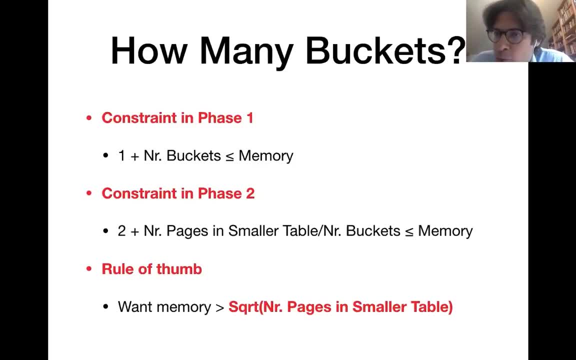 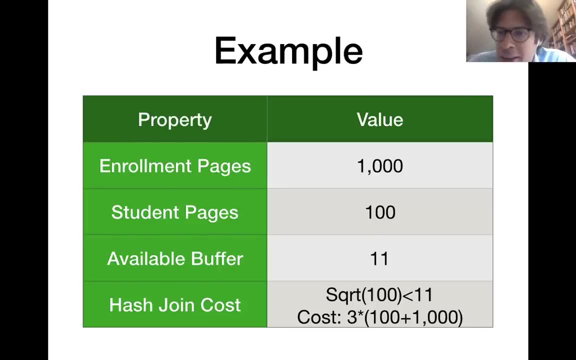 they approximately check out. So that is the rule of thumb: how much main memory you need for the hash join. This is a little example here, the same example that we have been using for the nested loop joins. And here we are joining the enrollment. 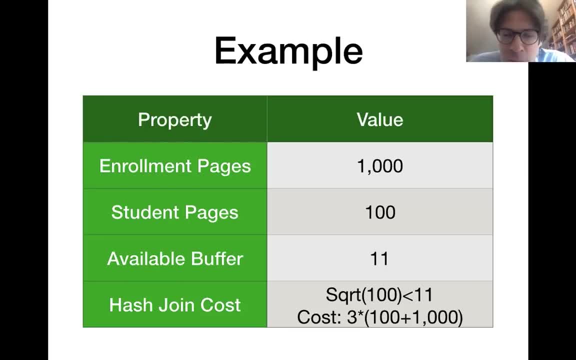 and the students tables with 1000 enrollment pages and 100 student pages, And let's say that we have 100 other pages available. So the smaller input table is the students here and it has 100 pages. So the square root of that. 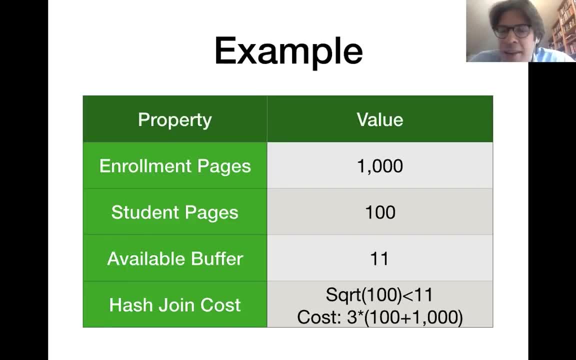 is 10,, which is a little bit smaller than the amount of main memory that we have available. so it seems okay. And then the cost of this join. that is simply three times the size of both inputs combined I have in the first phase. 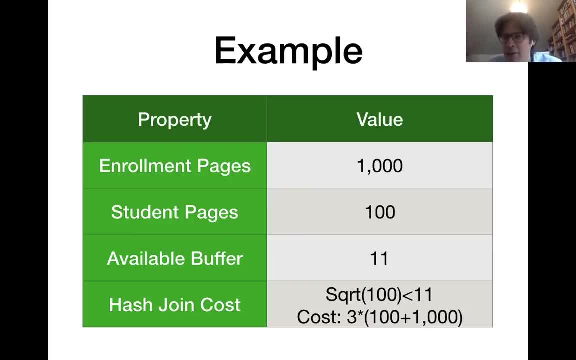 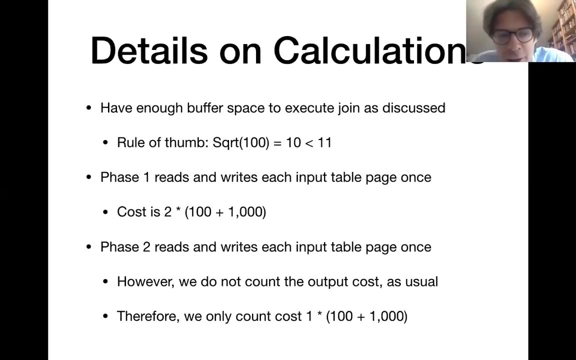 of the join. I am reading everything once and writing everything once In the second phase of the join. I am just reading everything once and even if I would write out something, then I wouldn't count that cost because it is the final join result. You see the calculations. 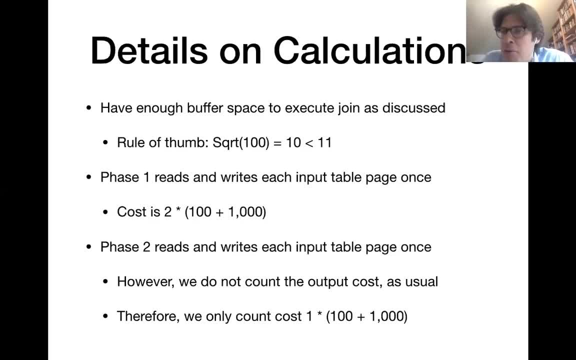 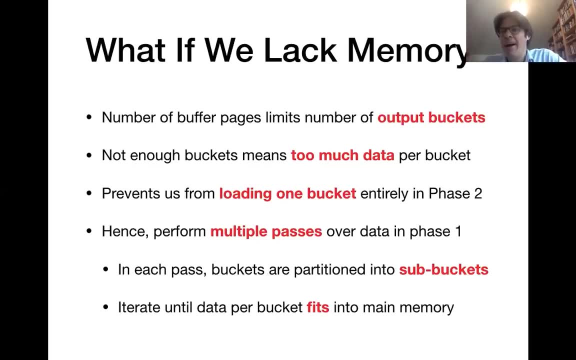 in a little bit more detail, but we are just applying the formulas that we have seen on the previous slides. Now I have described the rule of thumb for the main memory you typically want for this join in order to execute it If you have less main memory. 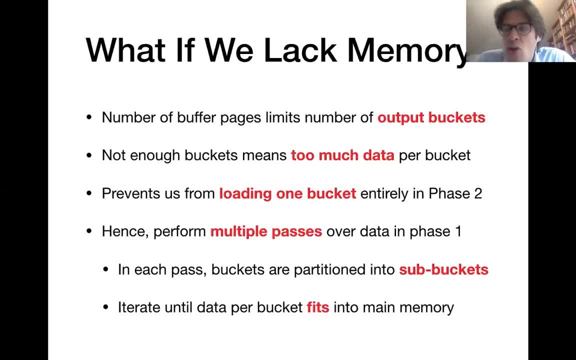 than that. you can, of course, always use a different join operator which might be less memory hungry, or there is also ways to adapt this join operator to deal with smaller amounts of a main memory. Now, if we have not enough main memory, the problem is this: 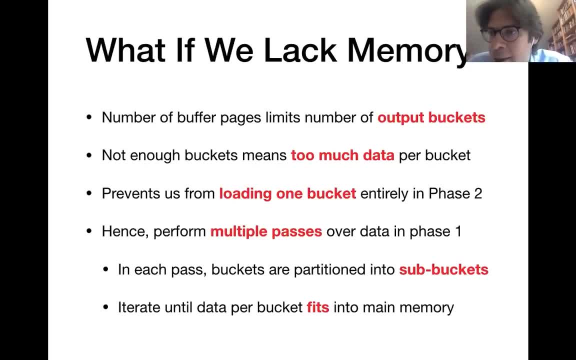 I will have a buffer in main memory for each of my hash buckets. So if I have less main memory, I will have less hash buckets, and that means that each hash bucket contains more data. That creates a problem in the second phase because I cannot fit. 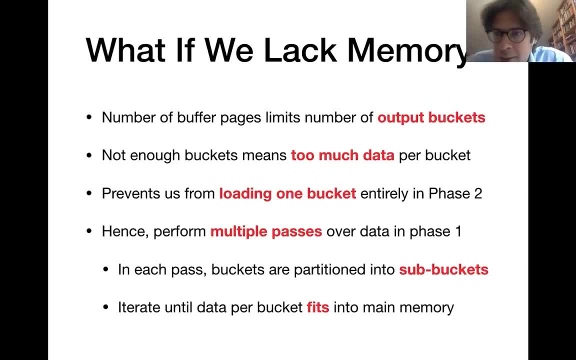 one entire hash bucket into main memory anymore, because they become too large Now. what I can do in those cases is that I don't execute one partitioning pass or partitioning passes. So in each of those follow up passes I divide data in one bucket. 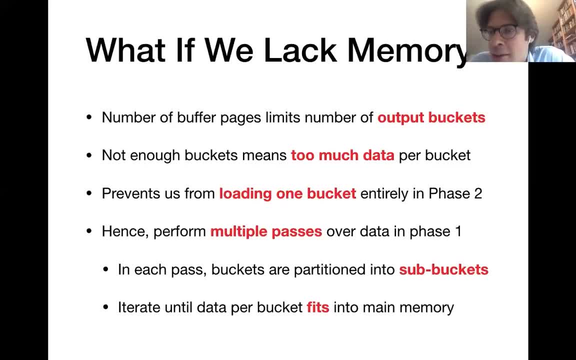 into sub buckets, so to speak, which of course means that I need a different hash function. So instead of partitioning everything in one pass over the data, I would partition things into more and more fine grained buckets by iterating over the data multiple times in the first join phase. 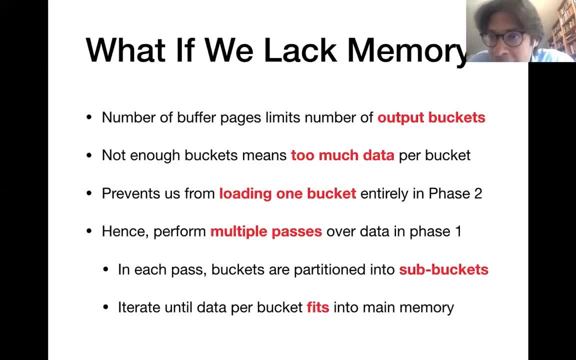 or say that in the second phase I have reduced the size of those hash buckets enough, such I can fit one of them entirely into main memory. So that is a possibility. but of course the join becomes less efficient because I need to make multiple passes over the data. 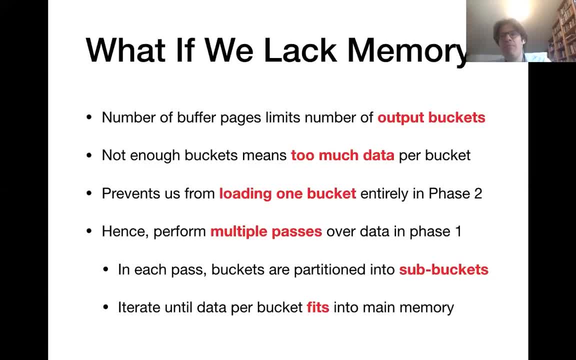 so I need to read and write it multiple times. So at some point it might become interesting to use one of the other join operators instead. And that is a great question here. What is the basically? by how much is it recommended that we decrease the size of those buckets? 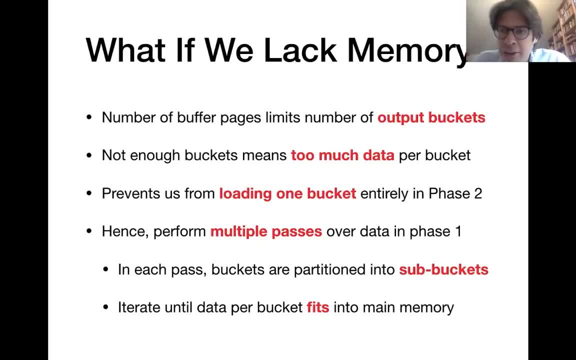 in each pass over the data? Well, that's a great question. You essentially want to maximize the effects of those passes over the data. You want to partition data as quickly as possible. So that means that in each pass over the data you probably 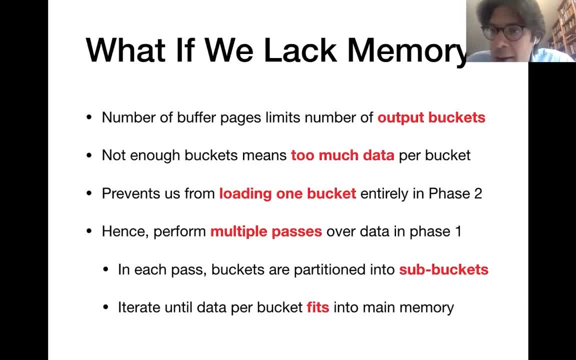 want to divide everything into the number of sub-buckets you can. If you have b-buffer pages available, that always means you need one input buffer and that leaves you with b-1 output buffers. So this is the number of sub-partitions that you probably. 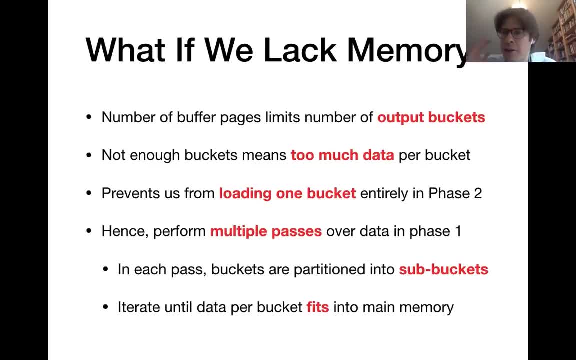 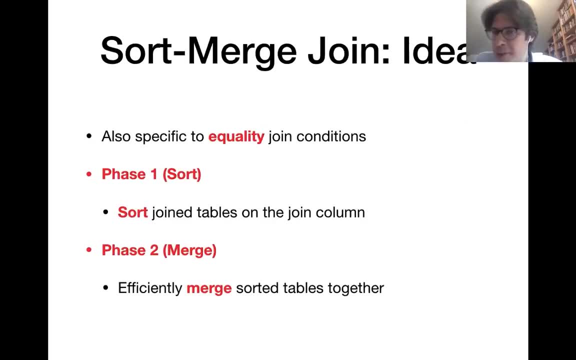 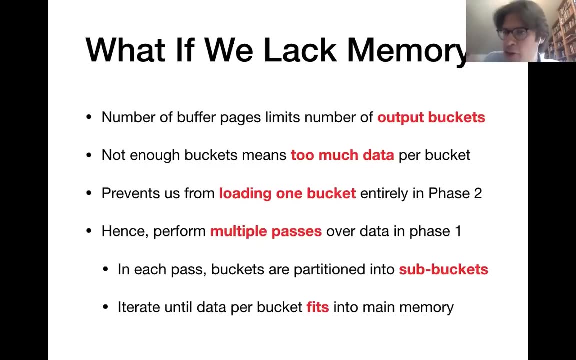 want to create, So as much partitioning as possible per iteration. All right, So that was the hash join, One of the most popular join algorithms And heavily used in database management systems. Now, in the following, I'm going to introduce one more. 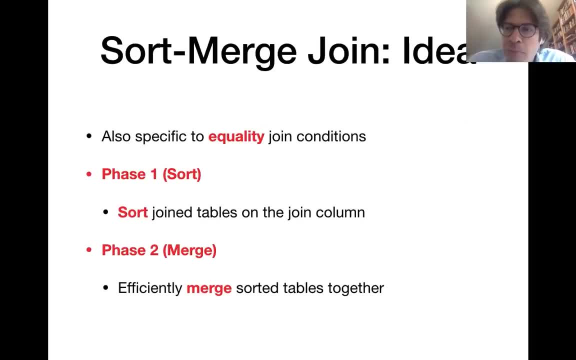 join the sort merge join, which also applies to cases where I have an equality join condition. That is also a very popular join operator. Also, this join algorithm executes two passes over the data. In the first pass over the data we sort the two input. 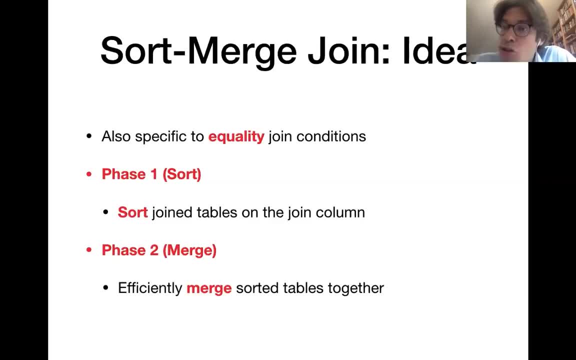 tables according to their value in the join column And then in the second phase we use those sorted tables in order to merge them together and quickly identify tuple pairs that have the same value in a join column. So that is now much faster because I have 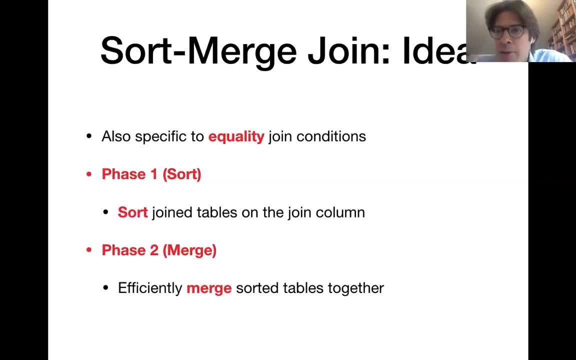 previously sorted the two input tables And, by the way, in some cases I might already have a table sorted beforehand. And then, of course, the sort merge, join becomes particularly interesting, because you might be able to omit one of those sort operations in the first phase In the following: 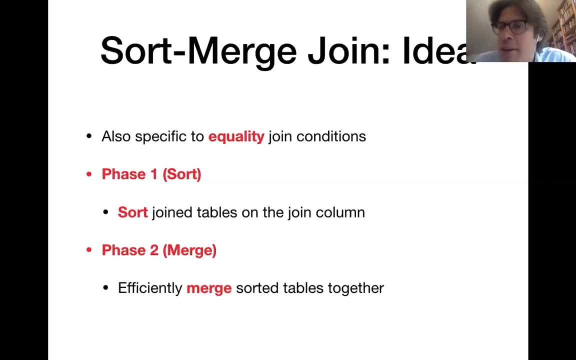 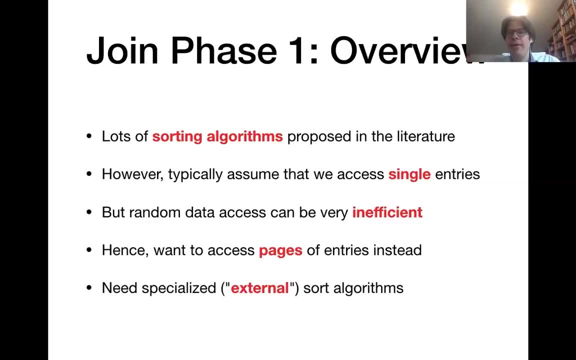 we're going to assume that both of the input tables need to be sorted first. Now you probably have heard a lot about sorting algorithms already. There's many sorting algorithms available. The problem is that most of them assume that we can access single entries in the data. that 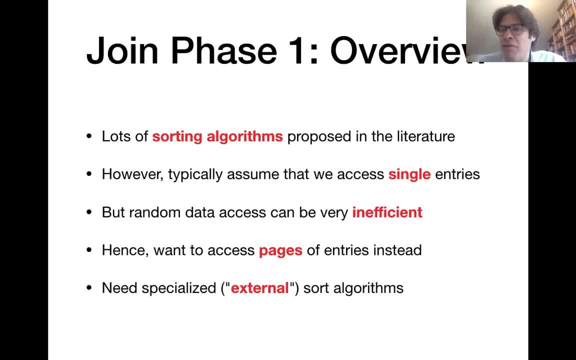 I am sorting Now. if I would do this with data that is located on hard disk, it would actually be very inefficient to jump back and forth between different single entries in that data because, as we have seen those storage media they often have some overhead for accessing. 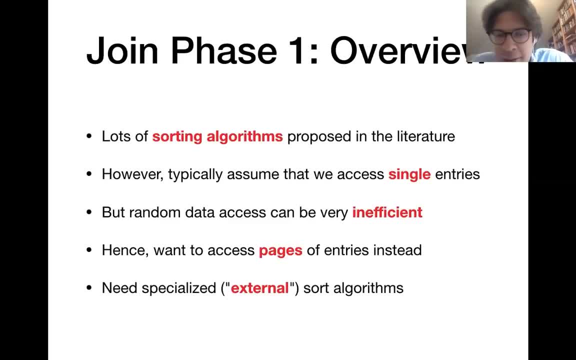 specific locations, for instance on hard disk, So random data access is efficient. This is why we rather want to access data in chunks, in pages of entries instead. And in order to make that efficient, you want some specialized join algorithm which takes that restriction into account, And those are called. 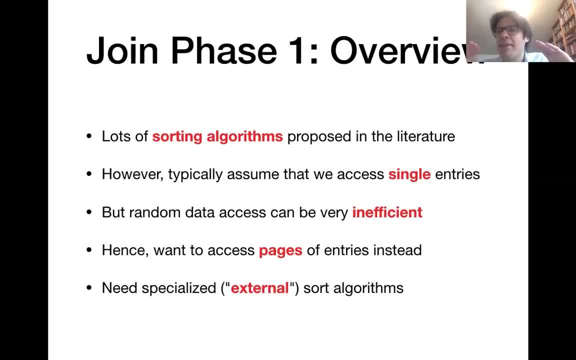 the external sort algorithms because they assume that the data to sort is not stored in main memory but somewhere outside of main memory, meaning for instance on hard disk or on some flash device or on tape. So there's in each case on some medium that doesn't make random access. 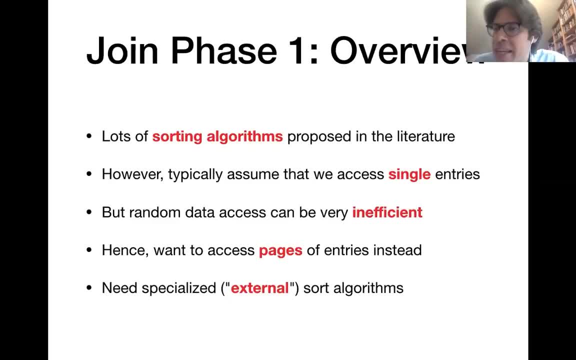 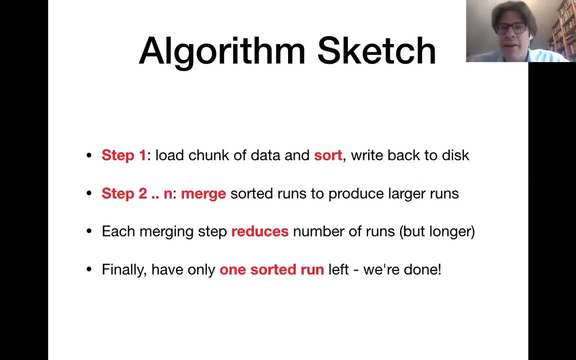 very efficient. In the following, we're going to see a sorting algorithm which takes that into account. Now this sorting algorithm proceeds in multiple steps. In each step, we iterate over the data and read the data once and write the data once. Now, each of those steps: 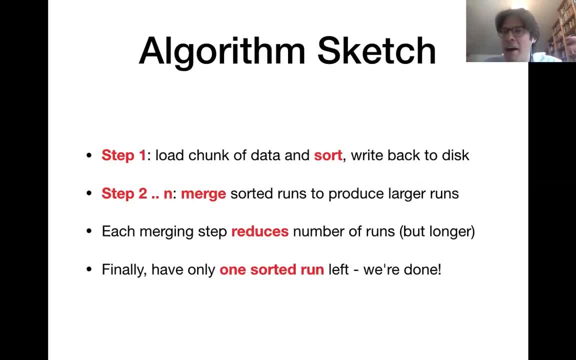 sorts the data more until finally all the data is sorted. In the first step we simply do the following, Assuming that we have a certain number of main memory pages available: we just fill all of our main memory with data from hard disk and then we sort it in. 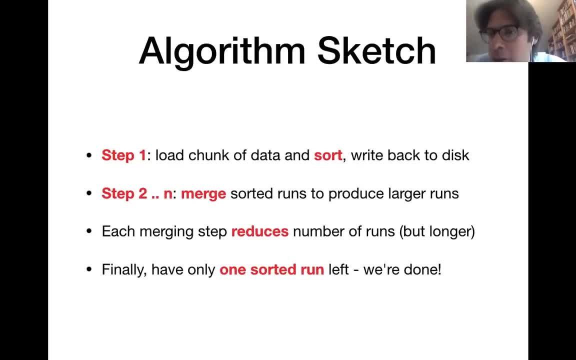 memory and then we write the sorted version back to hard disk, potentially overriding the original unsorted data. So after this first step we have multiple sorted chunks of data. We also call those sorted chunks of data runs sorted runs. In the following steps we are always merging. 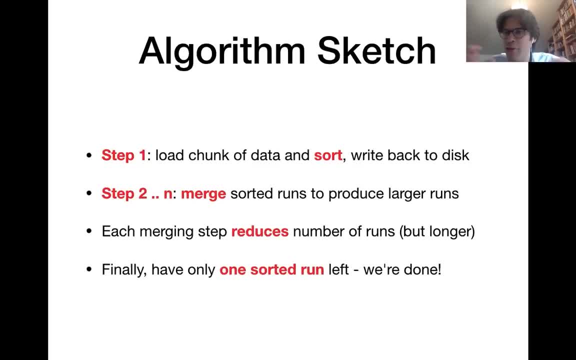 together multiple of those sorted chunks in order to generate larger sorted chunks. We only can merge a limited number of chunks of runs in each step, So that means we might have to execute multiple steps until we have merged together all the data and at that point we get one completely. 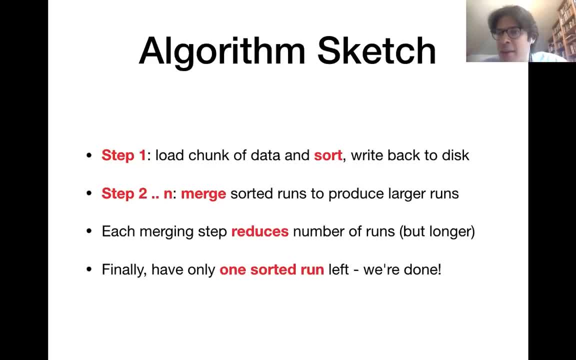 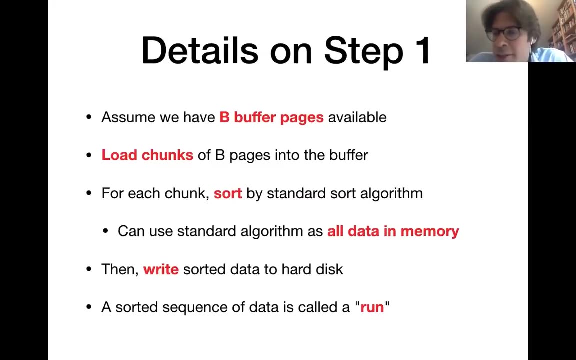 sorted data And after we have achieved one big sorted run, then we are done and the data is completely sorted. So let's see the first step in a little bit more detail. So we have B buffer pages available. we typically use the constant B in the 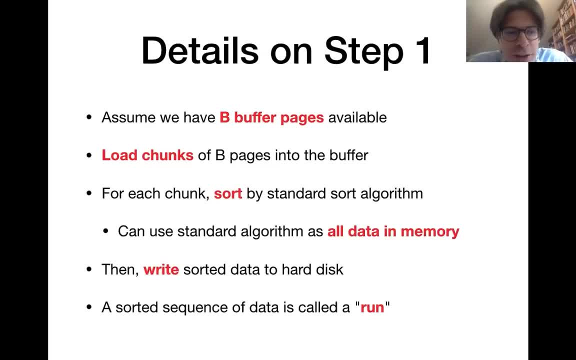 following: to designate the amount of buffer pages. So we load chunks of size B into our buffer and then we sort the chunk. We have some standard sorting algorithm because now we have the data in main memory And after we have done that we write the sorted data. 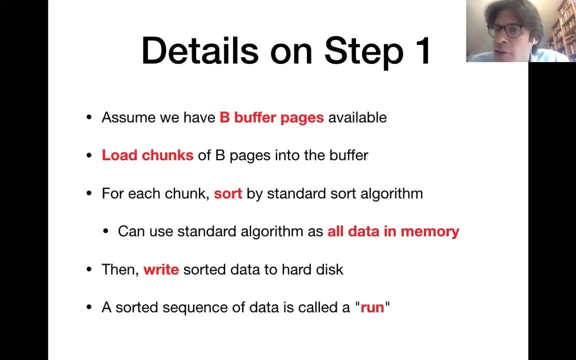 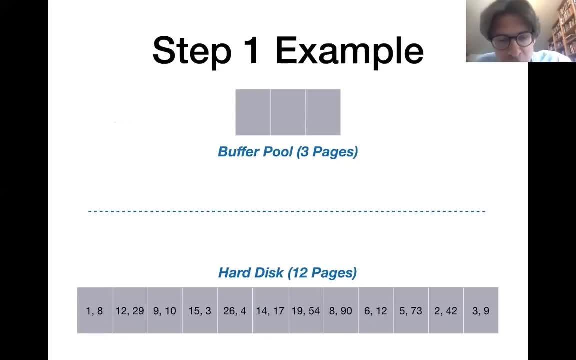 back to hard disk where it forms one of those sorted lines. Let's see this by an example. So here I assume I have the hard disk content in the lower part of the screen and in the upper part of the screen I have the buffer pool And, as you see, 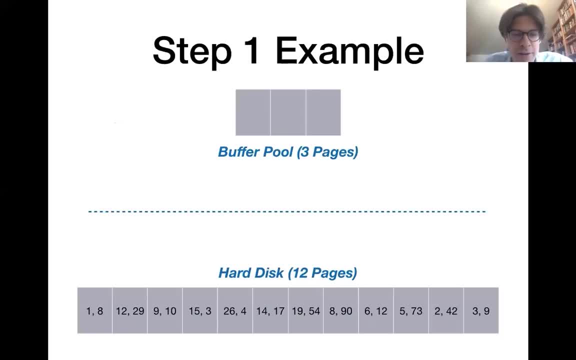 which is typical. the buffer pool is, of course, smaller than the hard disk. Now, in this first step of the sorting algorithm, I am first of all focusing on the first few pages of my hard disk content, which represents one of the two input tables to the join. 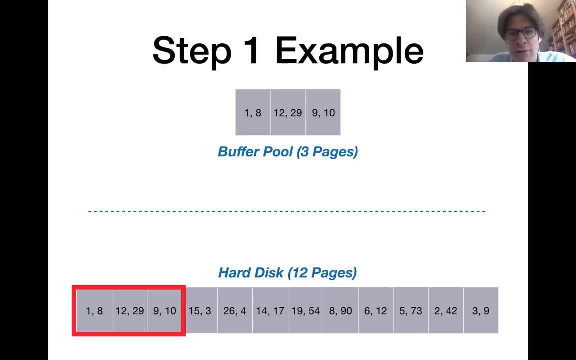 And I am loading that data into my buffer. Here the data is unsorted, as you see, So let's sort it by a standard sort algorithm in the buffer. And now I have sorted data in the buffer, I am writing it back to hard disk. 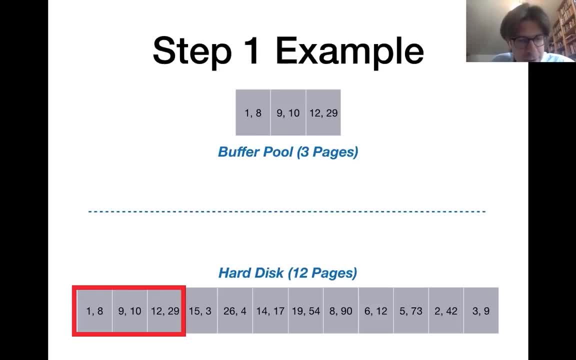 overriding the previously unsorted data. Alright, Now I have written it back to hard disk. Now we load the next chunk of data into our buffer, We sort it in our buffer and we write it back to hard disk again. Alright, So this is my. 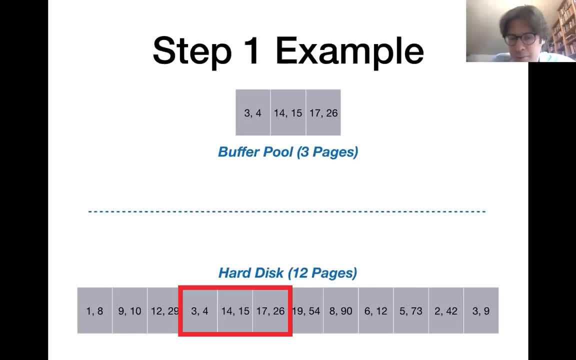 second sorted one on hard disk. Now I am loading the next chunk of data. Again, I am sorting it, I am writing it back to hard disk. I am doing the same thing for the last chunk of data: Sorting, writing, and now on my hard disk. 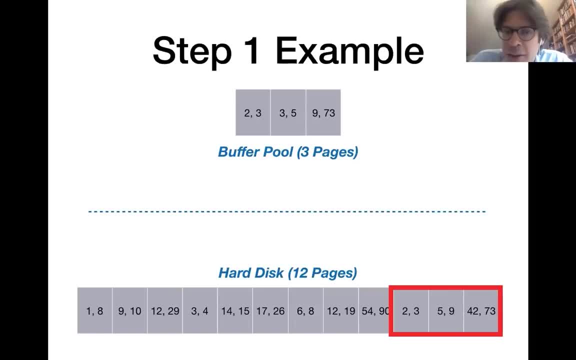 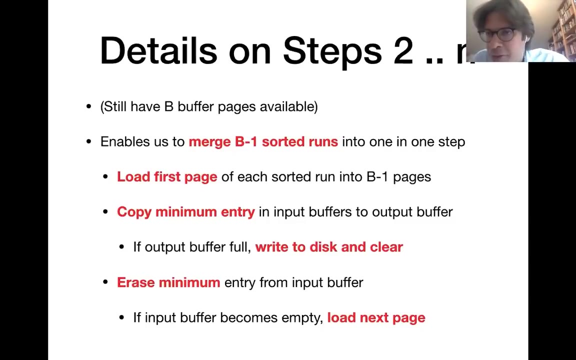 I have four sorted chunks of data, and each of those chunks has length- three, of course, because this is the maximum number of pages that I could fit into my main memory. Alright, Okay, So this is the first step. It produces a certain number of sorted runs. 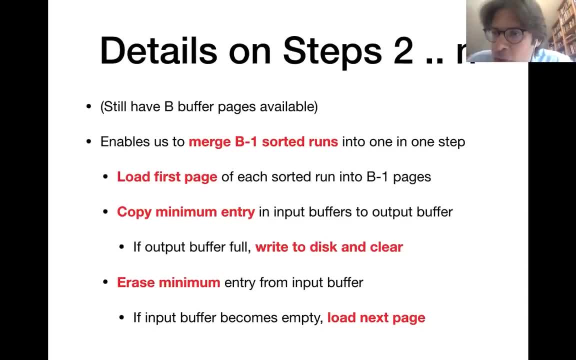 Now, in the following steps, I am merging those runs together in order to produce larger sorted runs. Now, I can only merge a fixed number of runs in one step. More precisely, if I have bbuffer pages, I can merge b-1 sorted runs, and it will become clear in a second why that is. 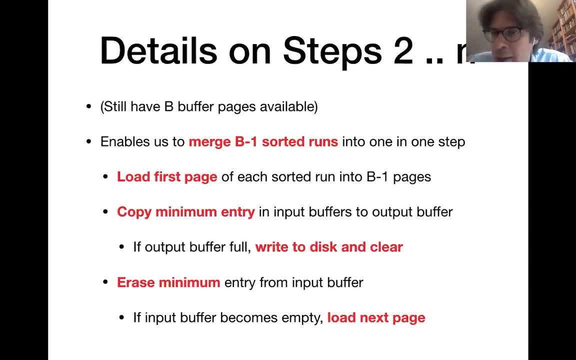 So for each of those sorted runs I need to reserve one input buffer in my buffer pool. So that means if I want to sort together, merge together b-1 runs, I need to reserve b-1 pages And among all the data that I have in 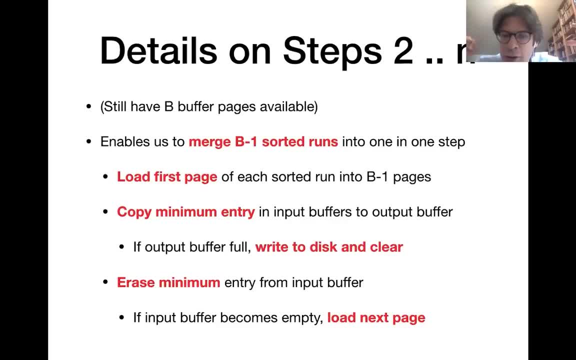 main memory. I am identifying the minimum entry null and I am copying that one into an output buffer and erase it from the corresponding input buffer. So the output buffer. this is where I am setting up my last buffer space page, because I need to write things into the output buffer. 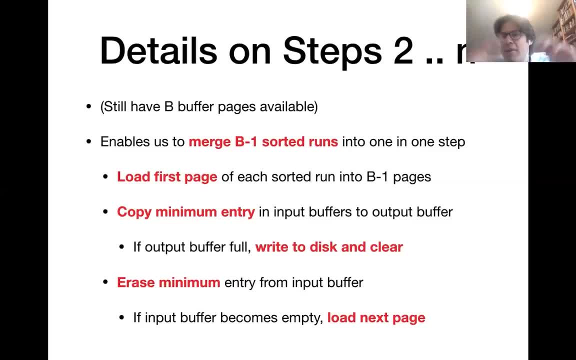 before. I am writing them to hard disk. Now. whenever the output buffer becomes full, then I am writing it back to hard disk and I clear the contents. Whenever my input buffer becomes empty, then I am loading the next page from the corresponding sorted run. So each input. 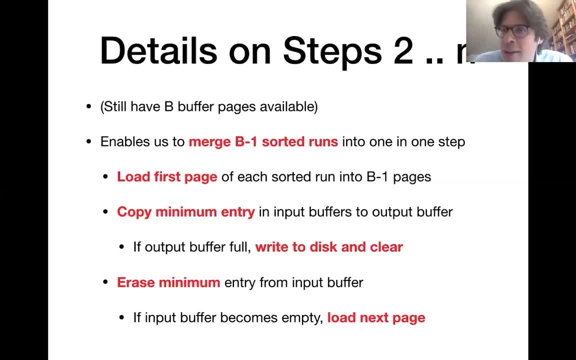 buffer is associated with a different sorted run, and so if one of the input buffers becomes empty, then we load the next page from that same sorted run into the input buffer, And since those runs are sorted, I know that I am receiving the entries for each run. 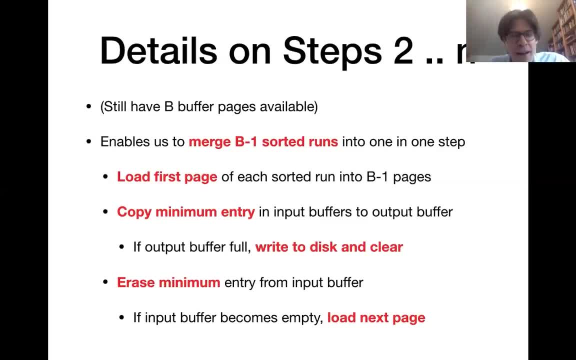 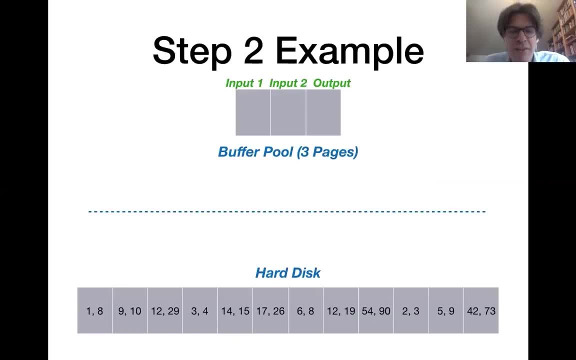 in increasing order. Alright, Let's see this by a little example again. So here I assume that we have previously executed the first step of the sorting algorithm. So we have 4 sorted chunks of size 3 and now I am merging them together. 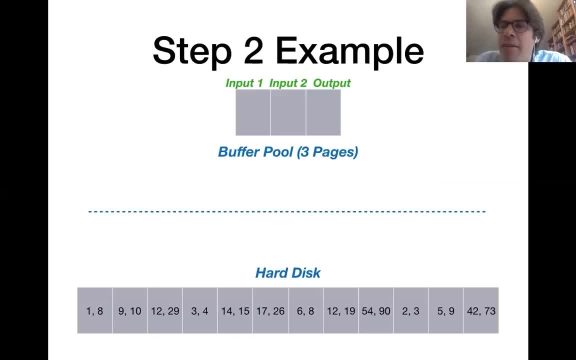 So here I have: b equals 3. that means I can together merge b minus 1, meaning 2 sorted runs in each step And here in the buffer pool. you see I have already written the function. for each of the spaces in green We have one input. 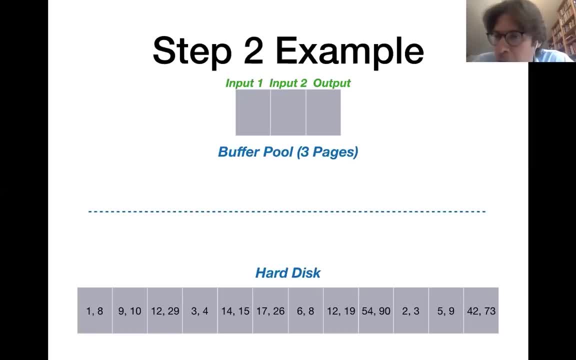 buffer for the first run, one input buffer for the second run and we have one output buffer. So we start by loading the first page from the first two sorted runs, and the first sorted one begins at the leftmost page and ends at the third page from the left and 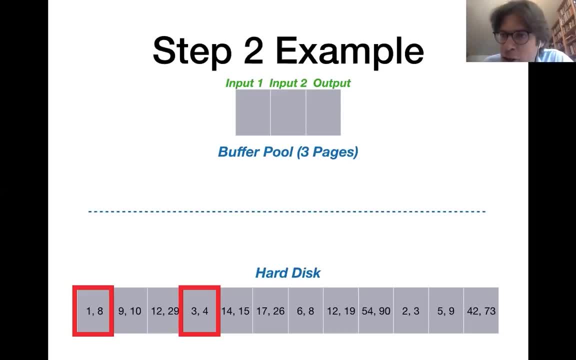 the next one starts from the fourth page from the left and goes until the sixth page from the left. So those are the first pages of the two sorted runs, and now I am loading them into the corresponding input buffers. Now I identify the smallest entry in: 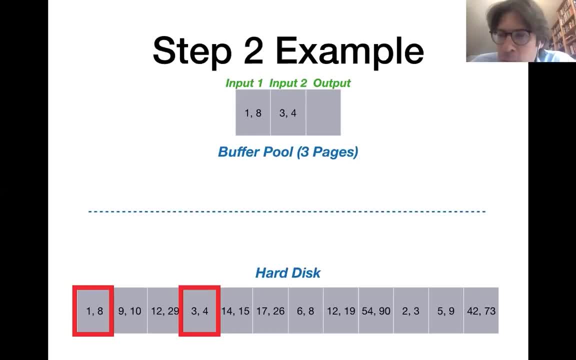 my buffer pool and that would currently be 1.. So I am copying that entry to the output buffer and I am erasing it from the corresponding input buffer. Now the next smallest entry, that would be entry number 3 over here. So I am. 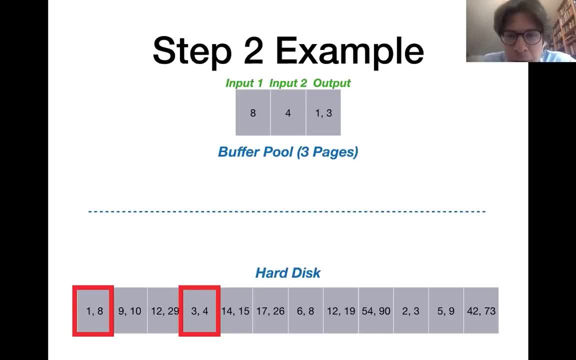 copying that to the output buffer and erase it from the corresponding buffer. Now, at this point my output buffer has become full, So here I assume that I can only fit two entries on each of those pages. So since the output buffer is full before 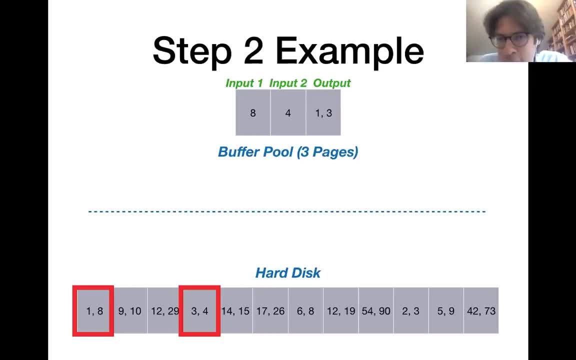 I can continue. I first of all need to save its content to hard disk and I need to erase it so it can accept more entries. Of course, in principle I could also write the output buffer to hard disk before it is completely full, but you don't. 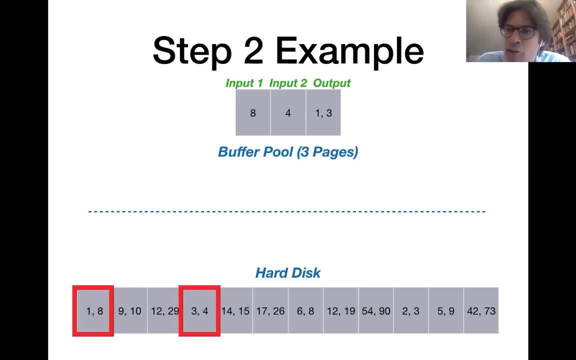 want to do this because each time that you are writing something to hard disk, you have pain with overheads. So I only want to write the output buffer content to hard disk when it is absolutely necessary, And in this case it is. So let's write the. 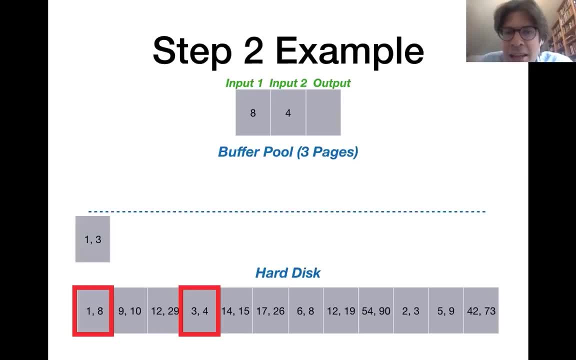 output buffer to hard disk and now we can clear it so it can receive more entries, And at this point the smallest entry in main memory, that is four. so I'm copying that into the output buffer. and at this point the input buffer number two has become empty. So now I'm advancing. 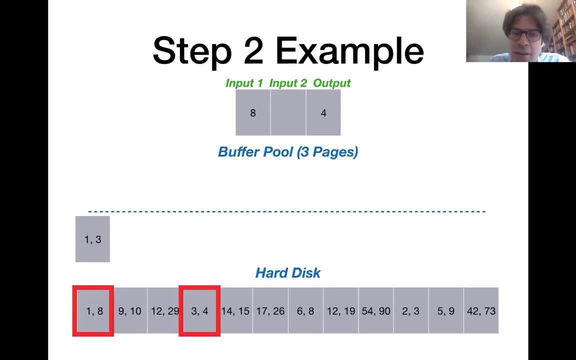 the corresponding focus page in the second sorted one to the next page and I'm loading the content into my buffer. Now, among the remaining entries, the eight is the minimum, so I'm copying that one from the input into the output buffer and erase it in the input buffer. 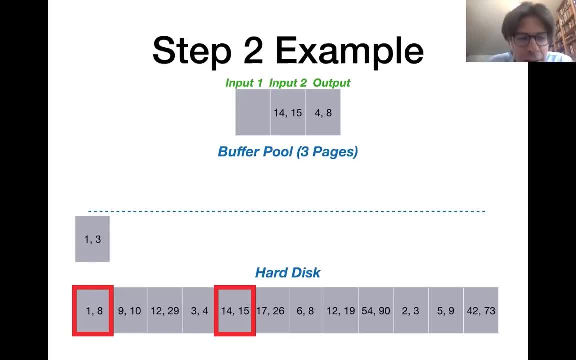 Here again, my output buffer has become full, so I'm copying that to hard disk and erase the output buffer in memory. At the same time, my input buffer number one has also become empty, so I'm loading the next page from the first sorted one, and at this point, 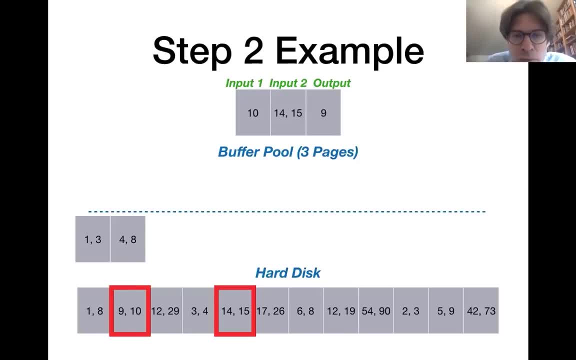 the smallest number in main memory, that is nine, so I'm copying that to the output buffer. Next one would be ten, and here my output buffer is full, so I'm writing it to hard disk. Also, my input buffer had become empty and rewinding to show that to you. 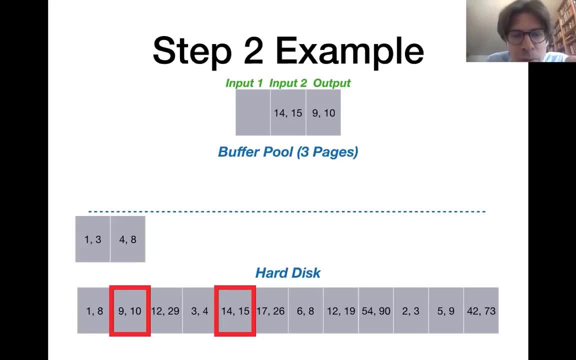 so input buffer number one is also empty. so I'm copying the output buffer to hard disk. at the same time I'm loading the next page from the first. sorted one, Alright, and now the smallest number would be twelve, again then fourteen, and at this point you probably 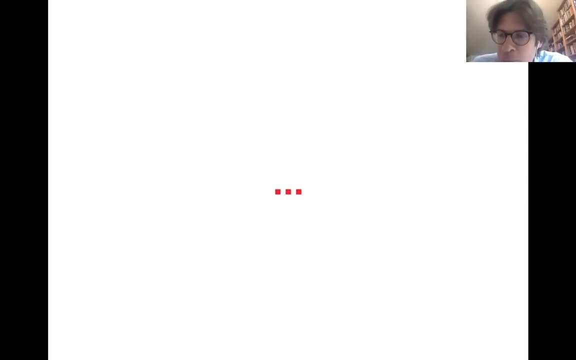 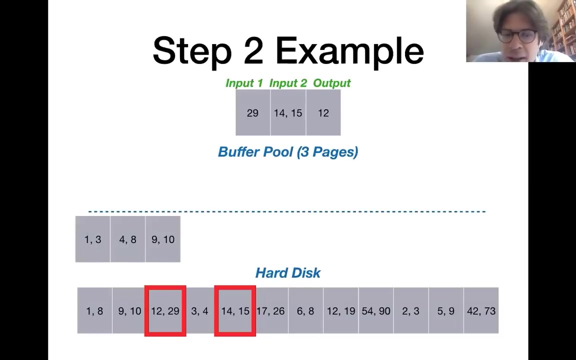 see where this is going. so I'm not going to complete the example, but if you do, then we have completely merged the two- first sorted ones from the input and then we are merging them into one sorted one that has now twice the size of the input sorted. 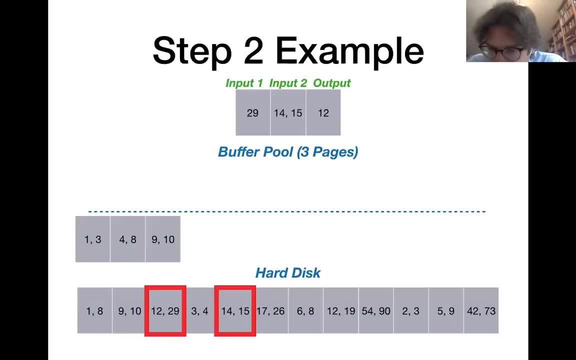 ones, Alright, and there's a couple of questions, Alright, and a couple of answers. yes, we are merging the two sorted ones, so the output that I'm generating here, that will become a full merged, sorted one, which contains all the elements from the first two sorted ones and combines. 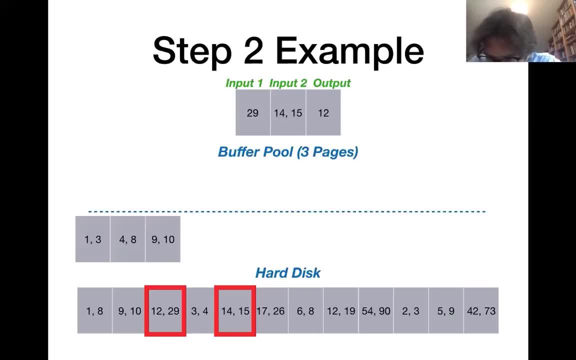 them into one sorted one, Okay, and there is a question about why not put the first page of the third sorted one instead of iterating through a run. Does it matter? Okay, and that is a great question. in fact, it does matter because you essentially rely in the algorithm. 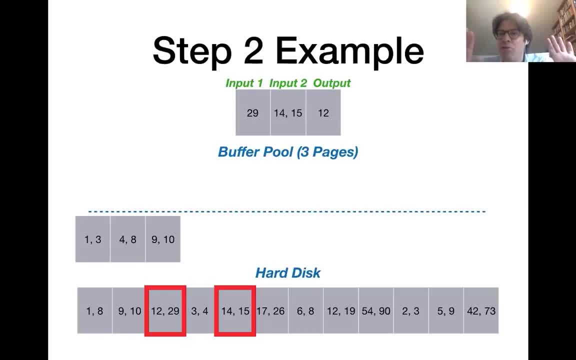 on receiving tuples in the input buffers in increasing order. So if you switch from a page from one sorted one to a page from a different sorted one, then the entries on that other page might be larger or smaller than the ones that you have been treating before. 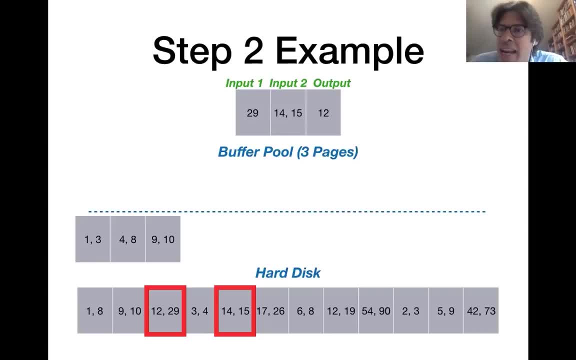 But this algorithm here essentially assumes that at any point in time it always has the minimum entry in main memory that hasn't been written out to hard disk yet. And in order to make that assumption it requires that for each of the input buffers I'm receiving, 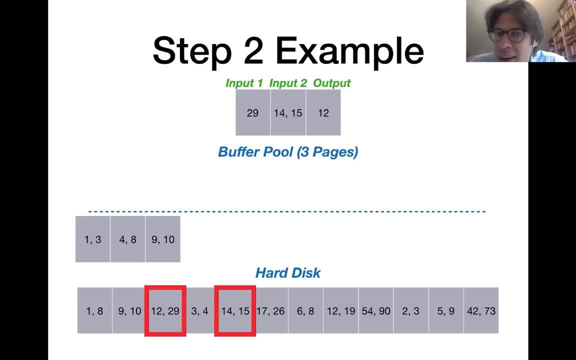 the sorted ones the entries from the corresponding one in ascending order. So it would be a violation of the assumptions that the algorithm is based upon if in one of those input buffers I would first have a larger number and then later would have a smaller number again. 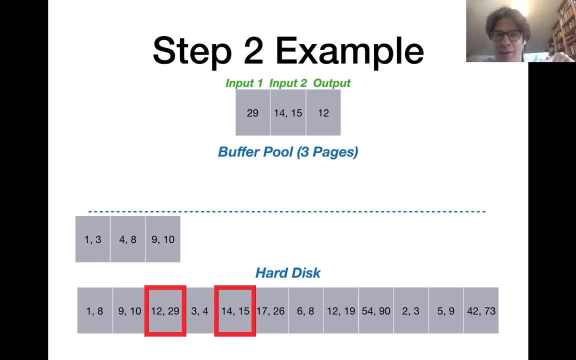 because at this point the algorithm has already written the output buffer to hard disk and it would assume that it doesn't have to go back and change anything anymore. So we can only merge together sorted ones, And in this case, since we have a four sorted ones, 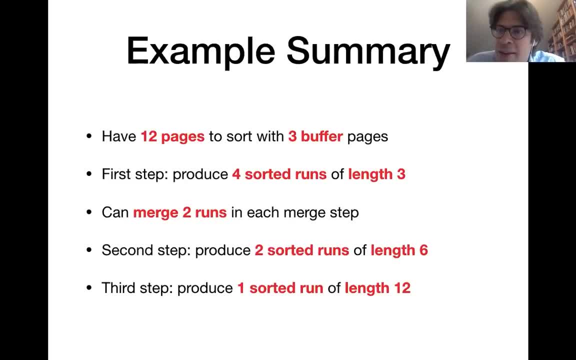 initially it would mean that we need actually two passes over the data until we have merged everything. So, as a summary, we have twelve pages and we have, but we need to sort and we have three buffer pages. The first step produces four sorted ones of length three, and then I can. 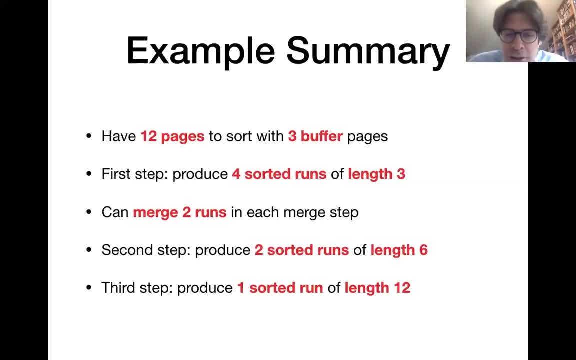 merge together two ones in each of those merge steps. So the second step which I have shown you, at least the beginning of it, it takes two sorted ones of length three and produces one sorted one of length. So the second step, takes runs of length three and produces runs of length. 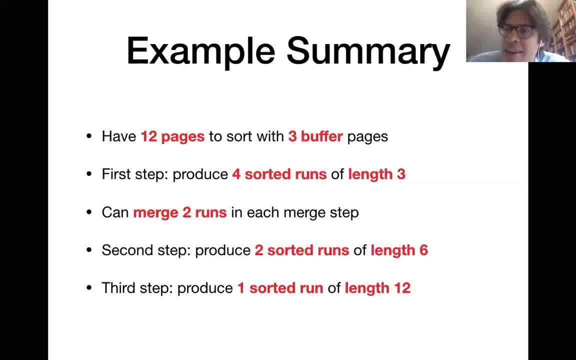 six. And the third and final step takes two runs of length six as input and produces one run of length twelve as output, and that integrates all of the data that we wanted to sort. So after this third step, over here we are done, And yes, there. 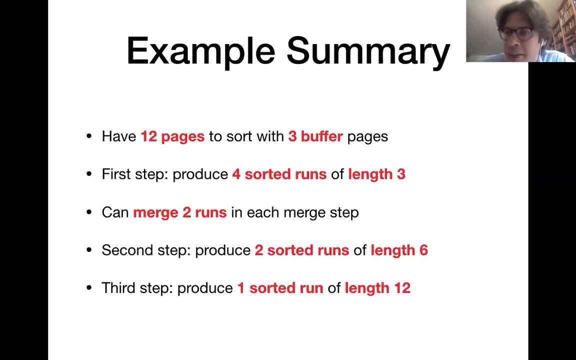 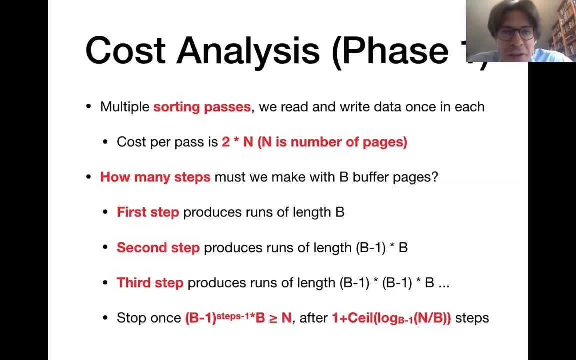 is some connections to bottom-up merge sort, indeed All right. So if we analyze the cost of that phase, we have to execute multiple sorting passes and in each of those passes we read and write the data once. So if n is the number of pages to 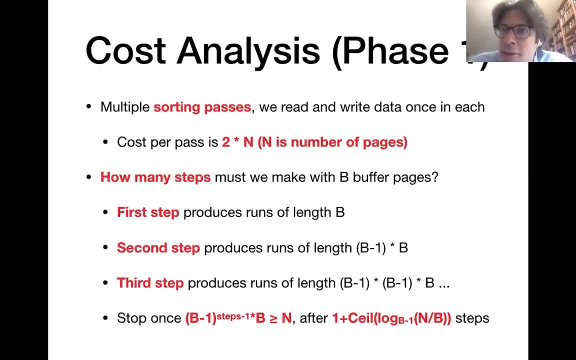 sort, then the cost per pass is two times n reading and writing. Now the interesting question is: how many passes do I need to make until all the data is sorted And we can think about the length of the sorted runs that I am producing? because if that length reaches the 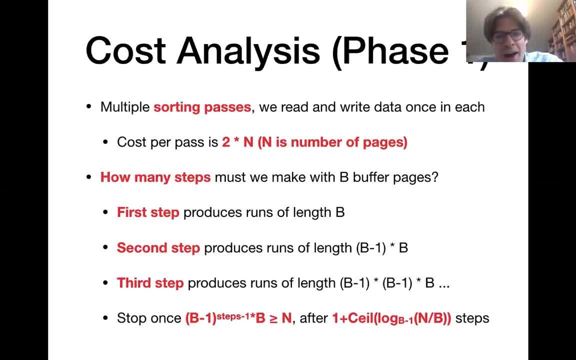 entire data set. I know that I am done Now. after the first step we have sorted runs of length b, which is the number of buffer pages. In the second step I am merging b-1 sorted runs together, so the length of the output run multiplies b. 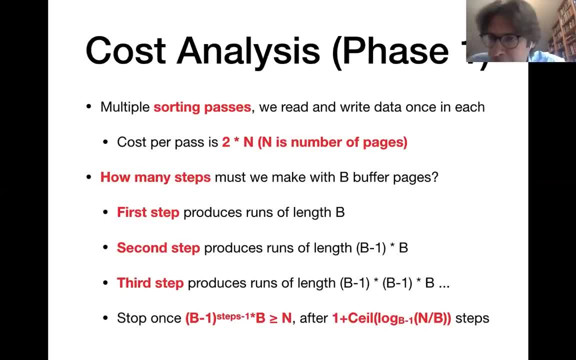 by b-1.. In the third step, in the following ones, I am also merging together b-1 sorted runs, so the length always multiplies by that factor and therefore once the length of those runs, as a function of the number of steps executed, has reached or exceeded, 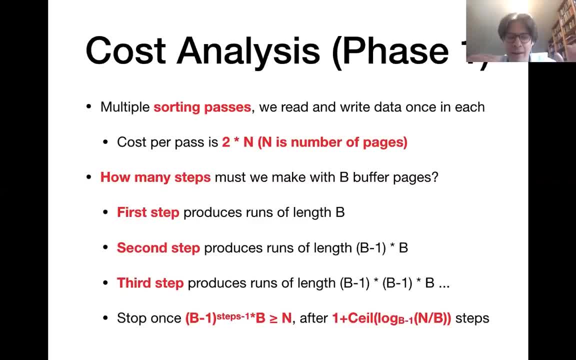 the total number of pages, then I know that I am done. So you have the formula here on the bottom of the slide, and if you resolve that towards the number of steps by taking the logarithm on both sides, then you end up with a formula that depends logarithmically. 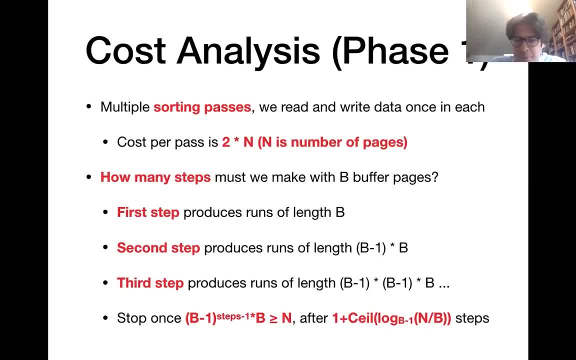 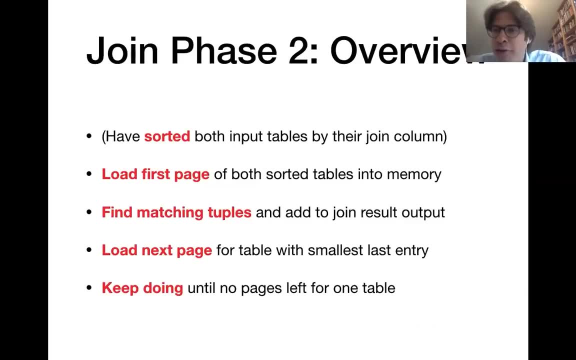 on the number of pages. Alright, So that is the first phase of the sort merge join, where I am sorting the input relations. and now I assume that I have both input tables sorted by their values in the join column, So after that it becomes quite efficient to 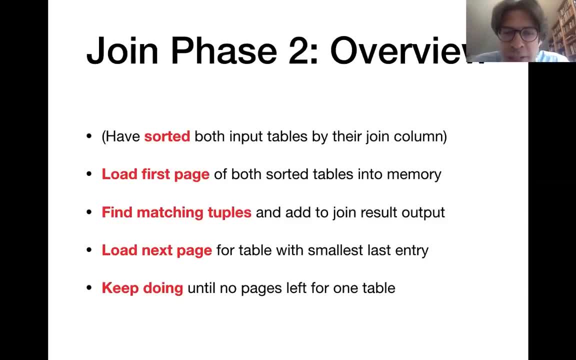 merge them together in order to produce the join result. So we proceed by first loading the first page of those both sorted tables into main memory, and then I compare the tuples that I have in main memory in order to find matching tuples, and once I have done that, for all the tuples. 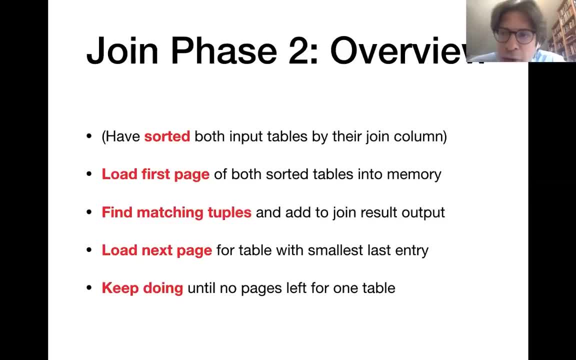 in main memory. I am loading the next page for one of the two sorted input tables and I am always loading the next page for that table where the last entry is the smallest, because maybe the next page from that page still needs to be matched against some currently loaded tuple from the 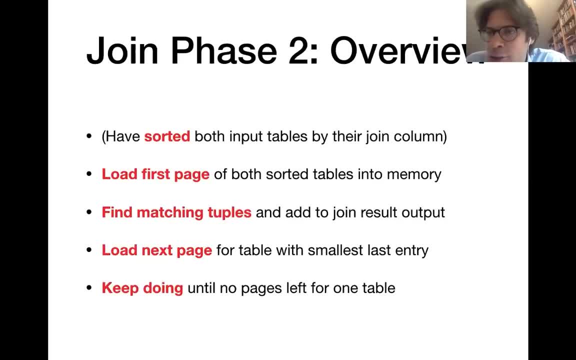 other table. Alright, And I keep doing this essentially until, for one of the two input tables, I have no pages left at this point in order to have produced a complete join result and I can terminate. And here again, the algorithm is crucially based on the assumption that my 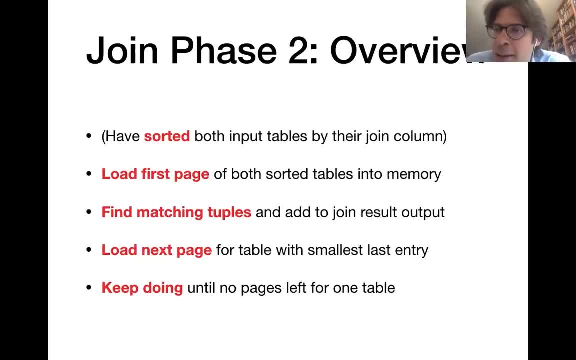 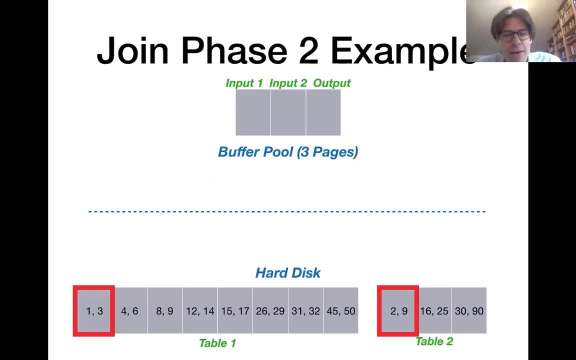 both input tables are sorted once this phase starts, because otherwise I would miss potential join results. Now here a little example about how I am doing this. now on hard disk I have data for two tables, where the first table is a little bit larger and, as you see, here we have already. 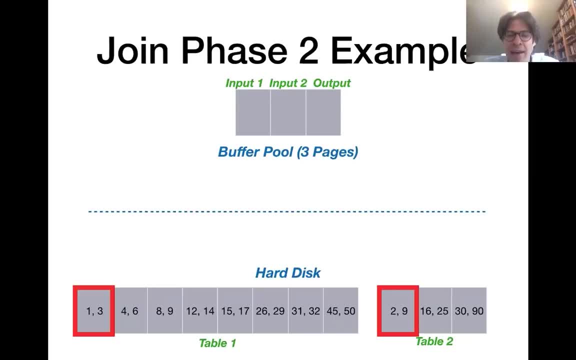 executed the first phase on both input tables. that is why those tables are sorted and I still have three buffer pages. and for this second join phase I also need an input and an output. two input buffers here and one output buffer, and I start by loading the first. 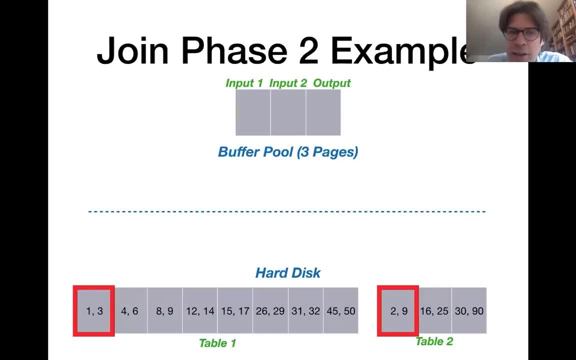 page of each input table into the associated input buffer. So I am doing this over here and now I am trying to identify matching tuples here. Now, in this case, they don't seem to be any matching tuples, so I am first of all excluding that it can be any matching tuple. 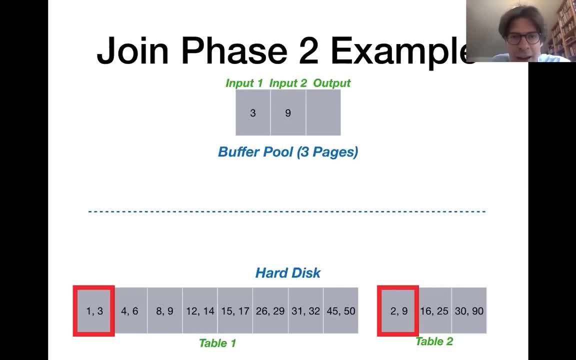 with the minimum here, then I am deleting the minimum that I now have in main memory. no matches so far, also no matches for the three, so I am deleting it At this point. I have run out of input for the first table, so I am loading data for the next page and again. 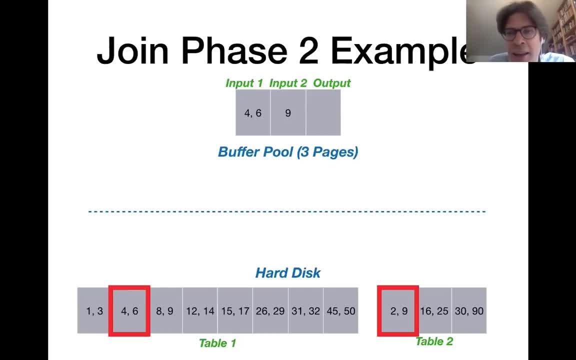 I am looking at tuples in increasing order. so four- no, there is no matches for four. six- no, there is no matches for six either. Alright, at this point, my input buffer one has also become empty again, and so I load the next page. so I am analyzing. 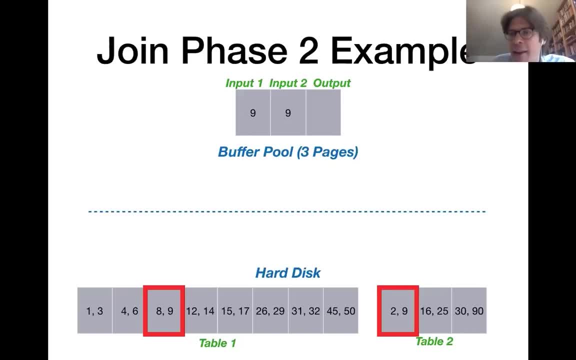 eight, no matches for eight, nine. and now I have a first match because here I have a tuple with value nine. so assume that this value is the value in the join column, so the tuples with value nine match together. so I am copying that to the join output and 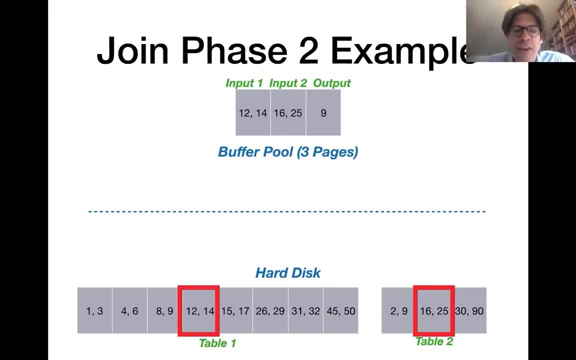 here I am loading the next page from both of the input tables and again I am going over it. fourteen no matches. should load the next page from the first table. fifteen no matches. sixteen no matches. seventeen no matches. I should load the next page and here: twenty five. 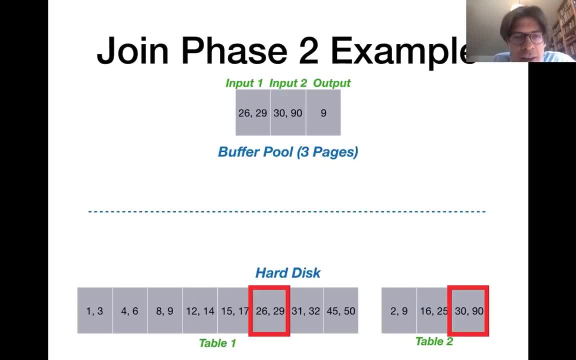 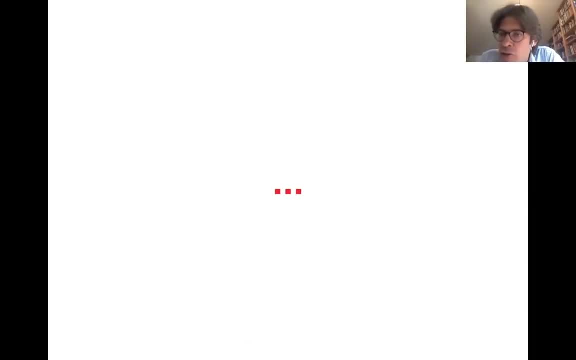 no matches, I should load the next page. twenty six, no matches. again twenty nine, nothing, and so on. so this is the principle: how I merge together two sorted tables using their value in the join column in order to produce the join result. alright, one special case that I have not shown in the example: 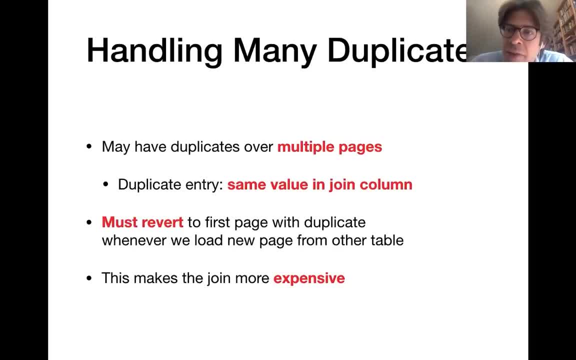 but that I quickly want to discuss is the case where we have the same value, essentially tuples that have the same value in the join column, and there is many of them in one table, so they extend across multiple pages of that table. now, if you have that, if your first table contains- 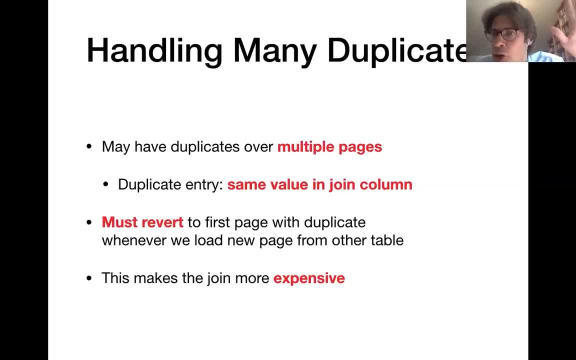 many tuples with the same value in the join column spread out over multiple pages, because there is too many to fit on one single page. whenever you load a new page from the second table, in order to be sure that you find all matches for the tuples on that page, you actually have to. 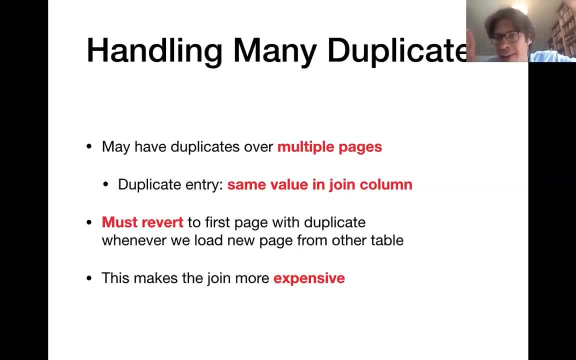 go back in the first table, to the first page, on which you find entries with the current value in the join column. so whenever you load a new page in the second table you will have to go back a few pages and consider all the pages in the first table which have the same value. 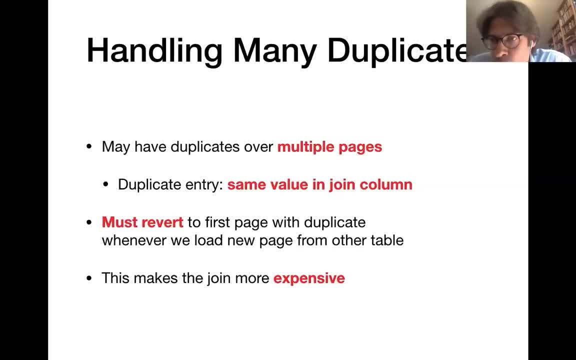 in the join column. this case is rather atypical still. I mean the implementations of sort merge joins consider it. but if that case happens then of course efficiency decreases because you have to read pages multiple times. so that makes the join more expensive. now in the following cost: 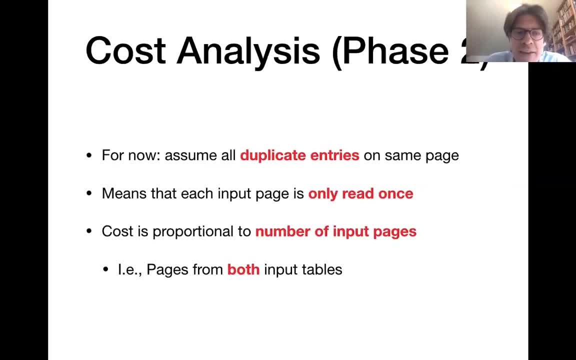 analysis, we will actually assume that this case does not happen. so we assume that each of those pages is read only once, and then the cost of this merge phase is essentially proportional to the number of pages in both input tables and, as before, they're not counting the cost for. 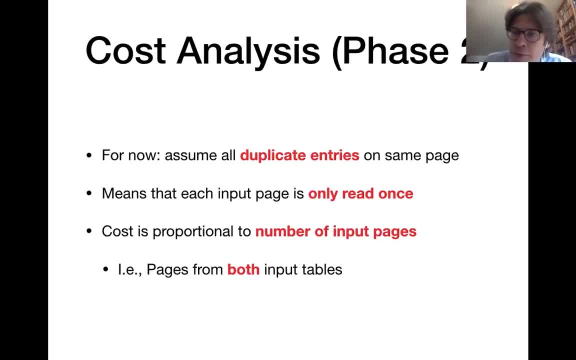 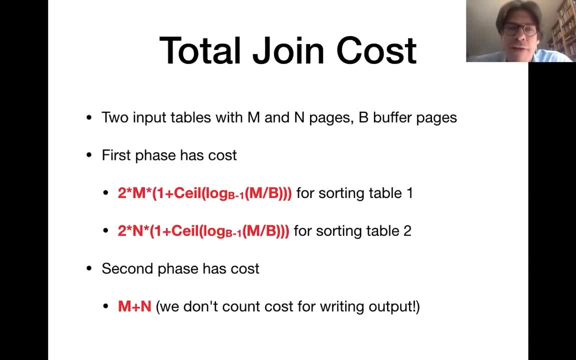 writing out the result of that join and this is the overview of the total join cost. we have two input tables with m and n pages and b buffer pages. then in order to calculate the cost for the first phase, we have to calculate cost for sorting the two input. 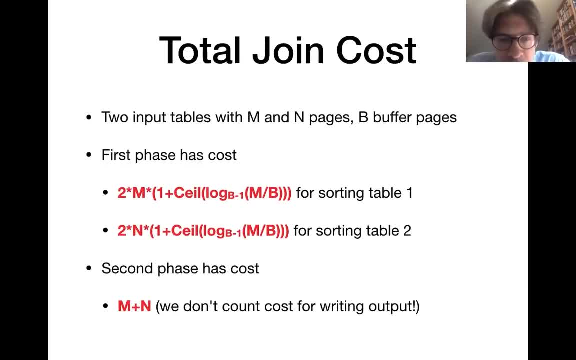 tables. so we just use the cost formula from the previous slide and we use it once with m and once with n pages. so here in the second formula, by the way, i see that argument of the logarithm that should be n divided by b instead of m. 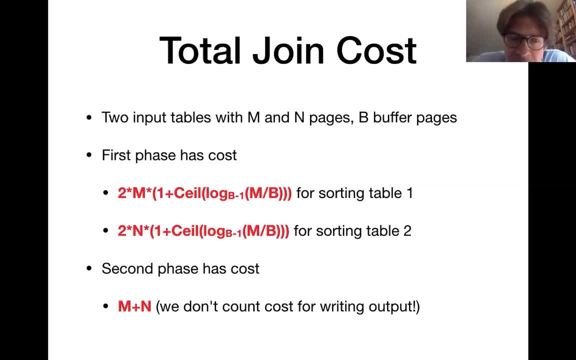 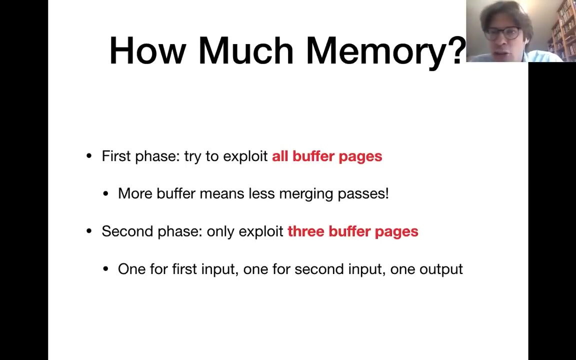 divided by b, for the second phase, the cost is essentially the size of our two input relations, m plus n, and so in total we have the sum of all of those components as total cost for the join. now the question is: how much main memory are we using in order to 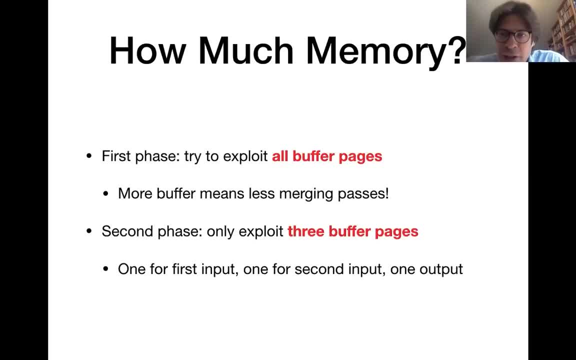 execute the join now. in the first phase we are essentially trying to exploit all buffer pages. essentially, the more buffer pages we have, the more sorted ones we can merge together in one step and that means we reduce the number of steps if we can exploit more main memory. 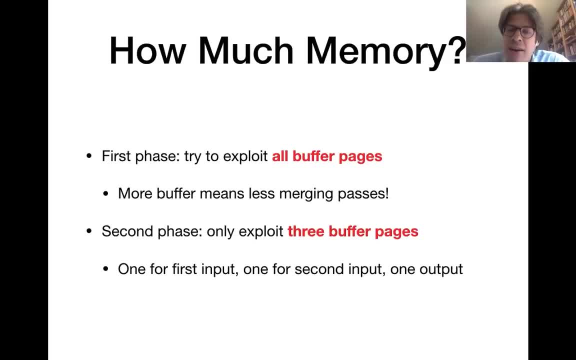 in the second phase, however, we only exploit three buffer pages: one for the first input, one for the second input and one for the output. now, this already tells you that maybe something can be improved, because here in the first phase we are exploiting all main memory, but in the 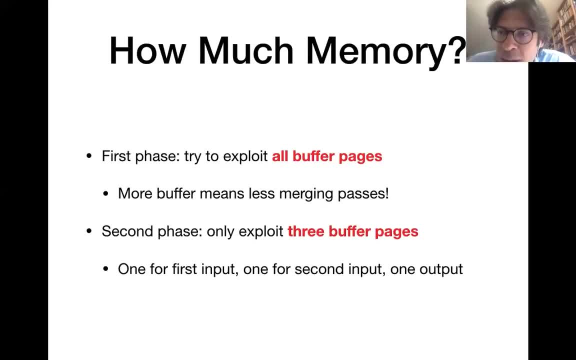 second phase, we only exploit a part of a main memory and in the context of data processing you can often speed up things if you are willing to use more main memory. so this is somehow strange and it already gives us the feeling, perhaps, that maybe there is something. 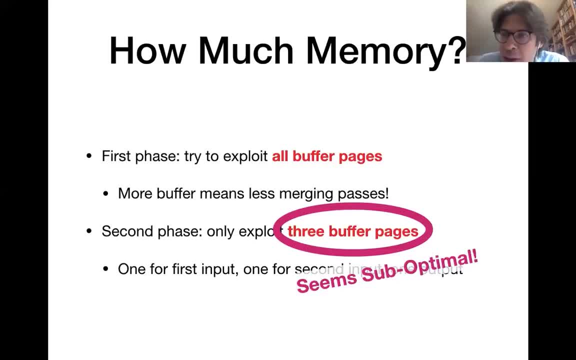 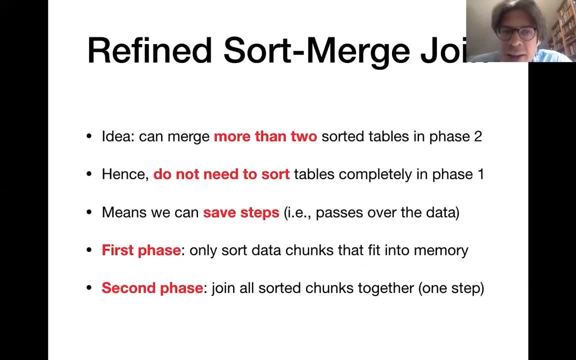 that we can improve with this join operator. there is indeed something called the refined sort merge join which exploits that we actually have more main memory than we are using with this first version of the join operator, and the high level idea of that join algorithm is that we can actually 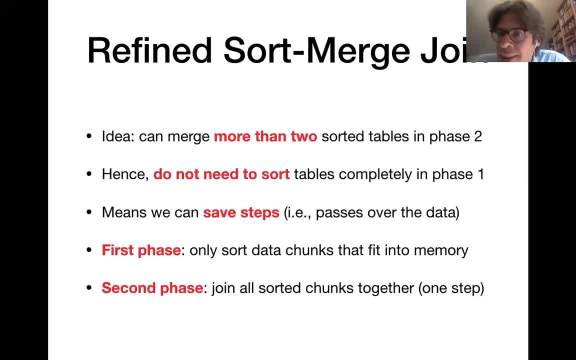 merge together more than two sorted tables in the second phase of the join because we have more main memory available. so we can exploit that by not completely sorting the tables in the first phase of the join. so far we assume that those two input tables, they are completely sorted. 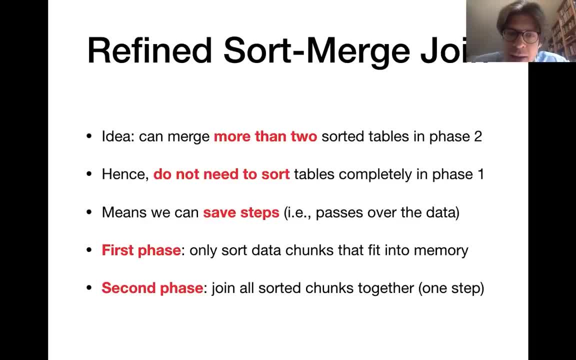 before the second phase of the join starts. but that is not really necessary now if you don't need to sort the two tables completely. it means that we save a couple of passes over our data and that means we are saving quite a few input like page read and write operations. 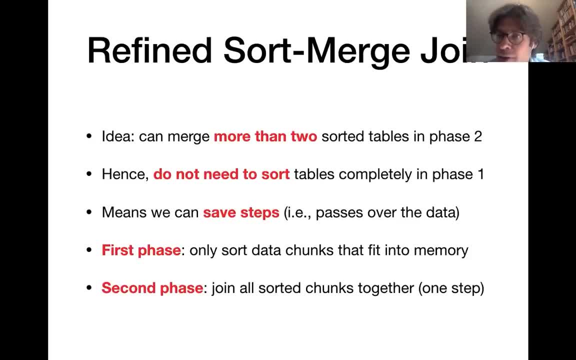 so what we do with the refined sort merge join if we have enough data? in the first phase we only sort data chunks that fit into main memory. so essentially we are only executing the first step of the first sorting phase, so we just load chunks of data into main memory. 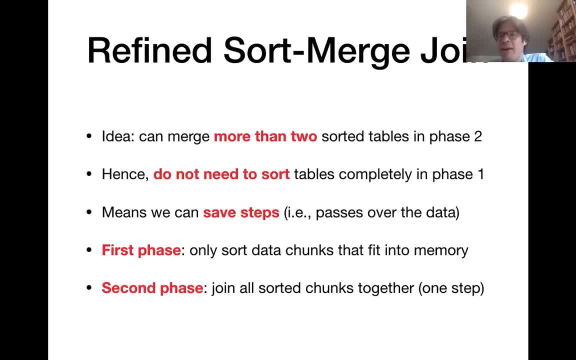 we sort them, write them back to disk. we do this for the entire table and afterwards we are done so. at this point we have not completely sorted the table, but we have produced sorted runs of a length that is proportional to our main memory. and now in the second phase, 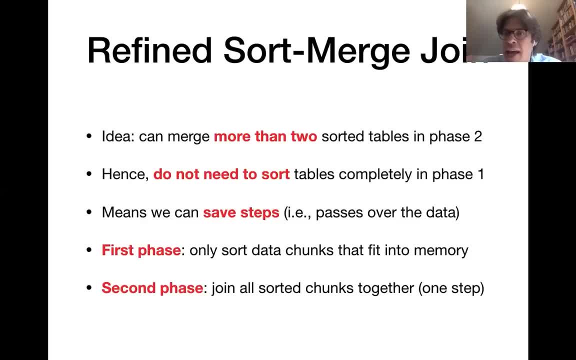 instead of at the same time joining together two sorted tables, we essentially join together a number of sorted table fragments. a number of sorted runs from both input tables. that is proportional to the amount of main memory that I have available. so when merging together those multiple sorted table parts, 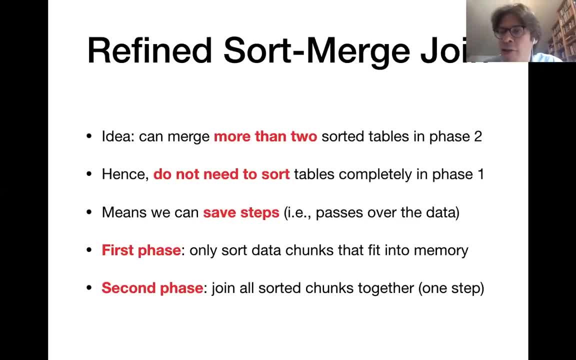 I am reserving one input buffer for each of those sorted table parts and if I do this, if when having like the first page from each of those sorted table parts in main memory, then I can also efficiently identify the next matching tuple, so I can do the. 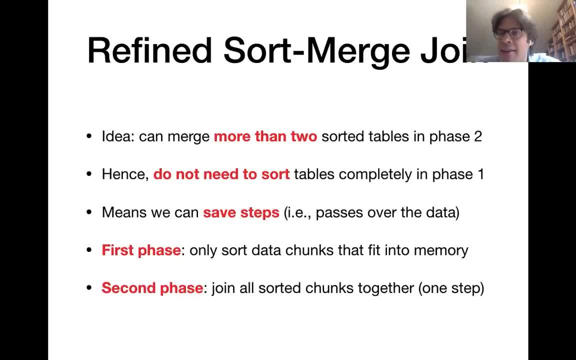 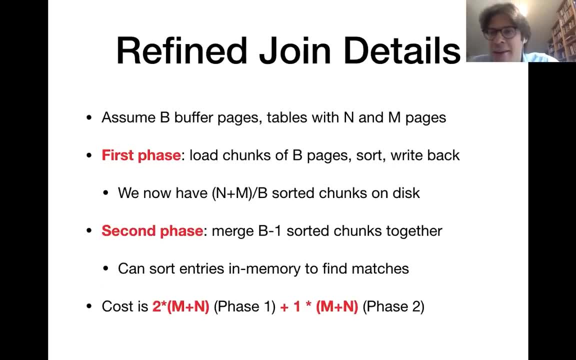 entire join in one pass over the data. so here a little bit more detail and we're gonna discuss that in a little bit more detail next time. so we generally assume that we have b buffer pages. we have input tables with n and m pages in the first phase. 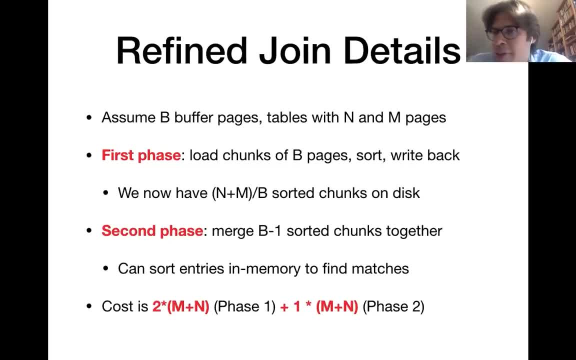 we load those chunks of maximum size, what fits into my main memory b pages, we sort them, write them back to disk and afterwards, when taking together both input tables with n and m pages, I will have a number of sorted table chunks. that is proportional to n plus m divided by 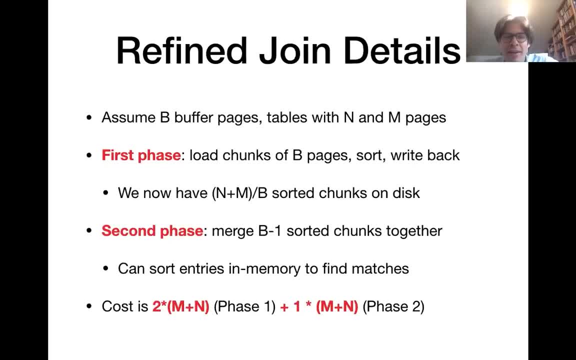 the buffer size. then in the second phase I will merge together b minus one sorted table chunks together, because I need for each one my input buffer and one output buffer, and if I can do this in one pass then my total cost will be in total two times. 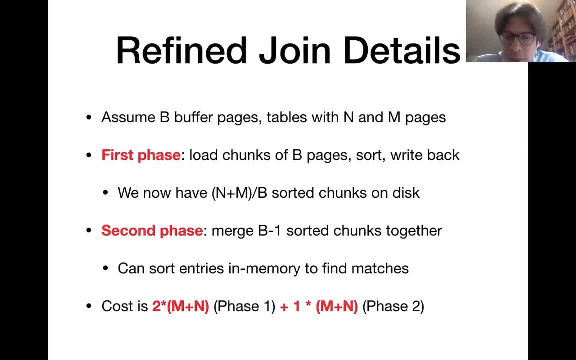 n plus n for the first phase, reading and writing once and one times. n plus n for the second phase, which is only reading the data once. alright, so I'm gonna stop here. we are gonna discuss the refined version of the sort merge join in a little bit more detail. 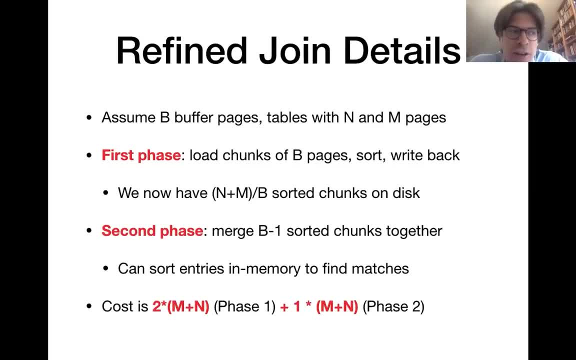 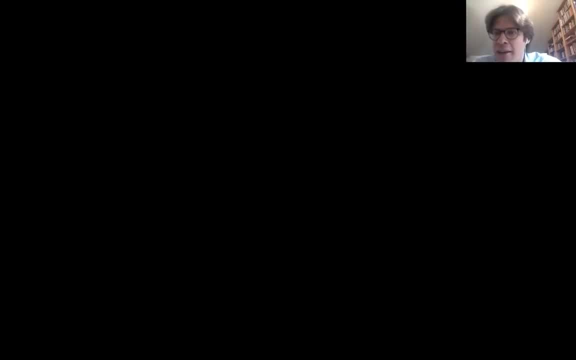 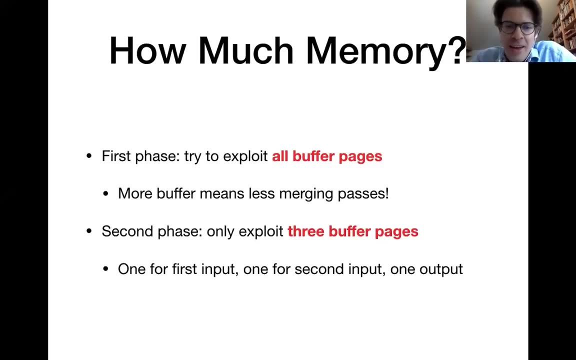 next time. this is the last join operator implementation that we will see and finally we will compare those different operator implementations together. have a nice weekend and see you again on Monday. so in the first phase of the sort merge join, we are essentially exploiting all the buffer pages. 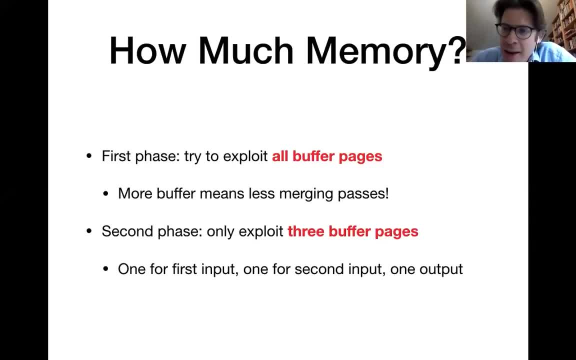 in order to do the external sort algorithm that we have seen in the second phase, we only exploit three buffer pages: one in order to read one page from the first input table, one to read one page from the second input table and one output buffer. and we have already 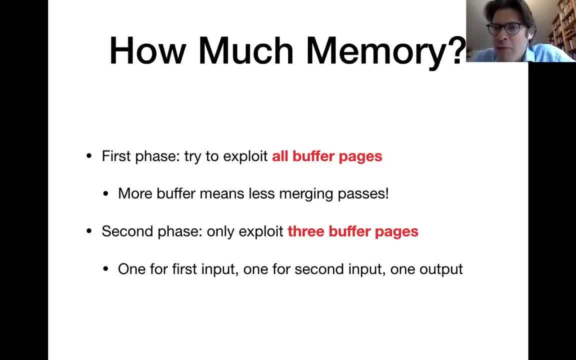 said last time that there is some kind of imbalance because we use a lot of main memory in the first phase but we don't use so much main memory in the second phase and that often means that we can make the algorithm faster if we exploit all the 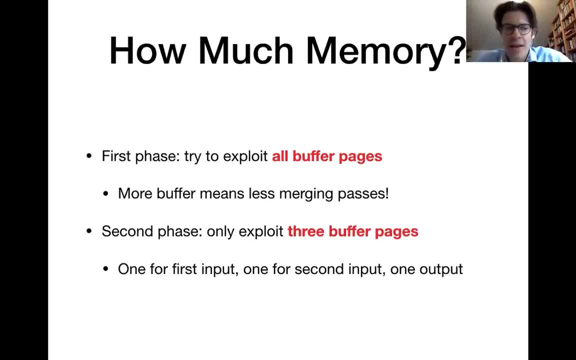 main memory that we have in both phases. so the last time I've already quickly mentioned that this is possible. there is something called the refined sort, merge, join, and here the idea is that I can merge together more than two sorted tables in the second phase. I just need to make sure that. 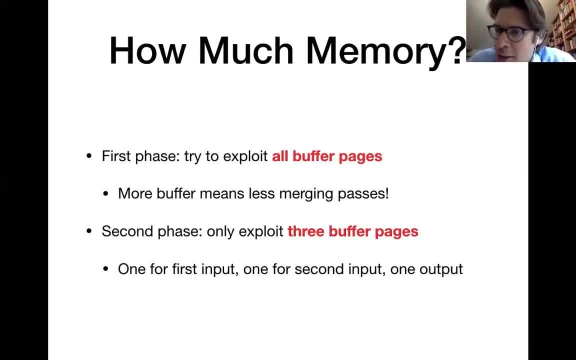 I have one input buffer for each of the tables that I'm merging together, but if I have more than two input buffers available, I can merge together more than two tables at once, and this refined algorithm exploits that. the main idea is that in the first phase I don't sort the input tables. 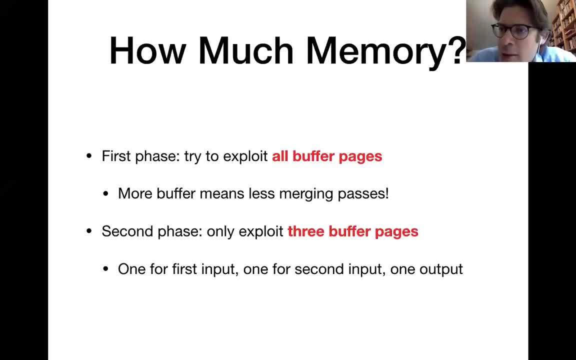 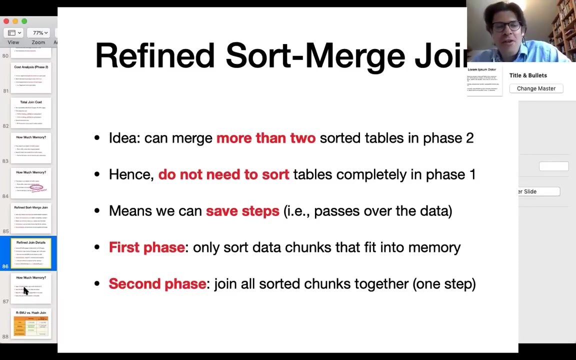 completely, but I only sort them partially. now that produces a set of sorted table chunks basically, so it is more than two, and then in the second phase I'm merging together all those sorted table chunks in one pass. so in the first phase of the refined join I'm loading. 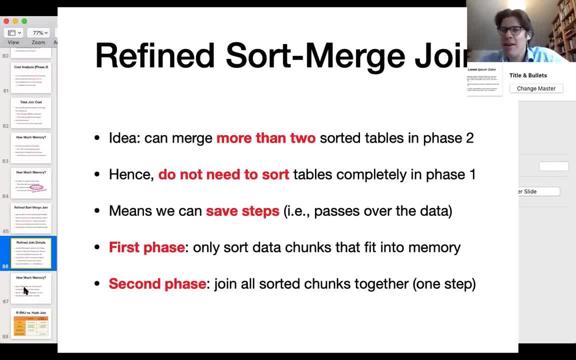 the pages of data into my main memory and then I'm sorting them and then I'm writing the sorted version back to hard disk. so if I have n pages in one table and m pages in the other table and b buffer pages, then the number of sorted chunks that I will 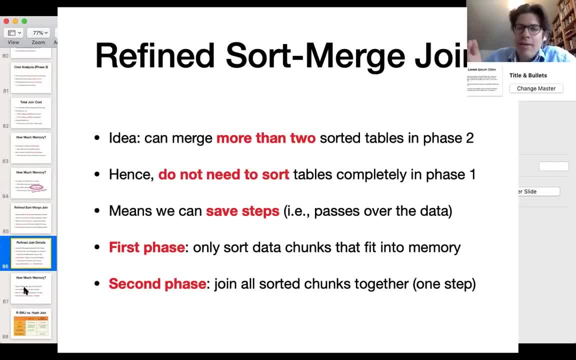 have stored on my hard disk will be m plus m divided by b afterwards. now, in the second phase, I'm merging all of those sorted chunks together in one step, and in order to do that, I just need to make sure that I can reserve one input buffer. 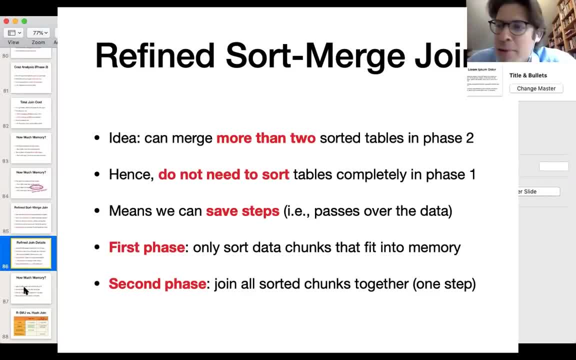 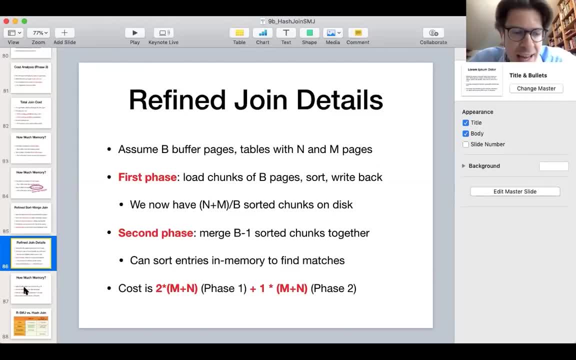 page for each of those sorted table chunks. and if I can do all of this, then the cost of this refined sort merge algorithm is, first of all, two times the sizes of both output tables in the first phase. because here I am reading all the data once and I'm 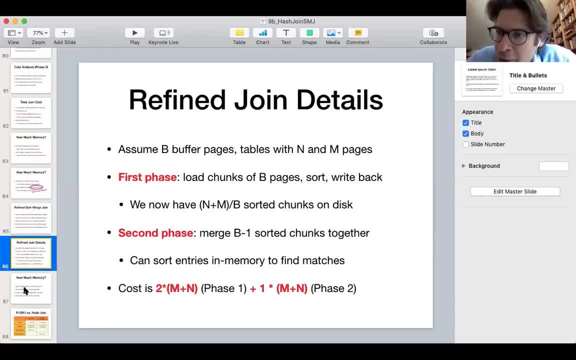 writing all the data once and in the second phase, since we don't count the cost for the output, I'm just reading all the data once in order to merge it. alright, so this is the refined sort: merge at join. in order to make it work, I need: 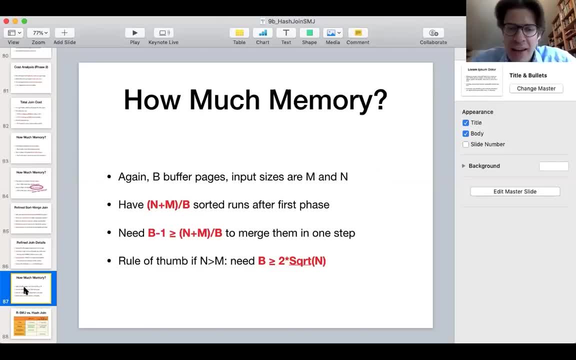 enough main memory. so now we can think about how much main memory we need in order to make that work. so, in general, if I execute the first phase, where I sort as much data as I can possibly fit into main memory, then the number of sorted chunks after the first phase- 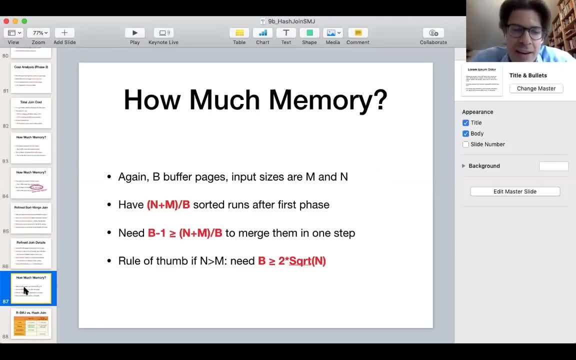 is m plus m table sizes divided by b. and now the constraint for the second phase is that I need to be able to reserve one input buffer for each of those sorted chunks that I want to merge together. so I still need to reserve one output buffer, and that is why. 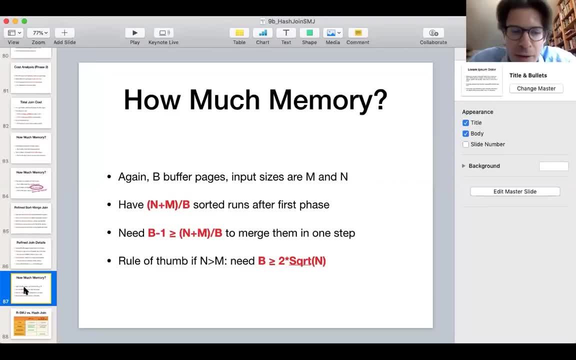 I am subtracting one from b- the number of buffer pages- and then I get the amount of buffer space that I have available as input buffers. so I have b minus one input buffers and that must be greater or equal to the number of sorted chunks that I want to merge together. 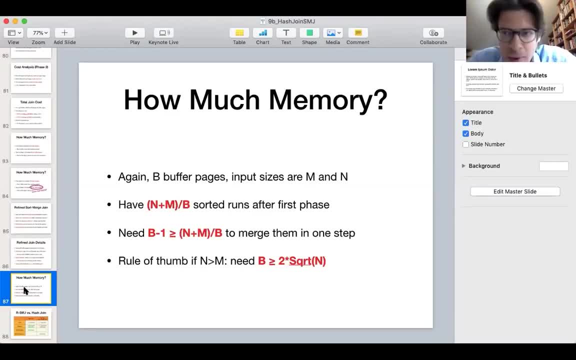 in one step and that, as we have just calculated, is the two table sizes divided by the buffer size. so I need this constraint to hold: b minus one must be greater or equal to m plus m divided by b. and, as a rule of thumb, in order to 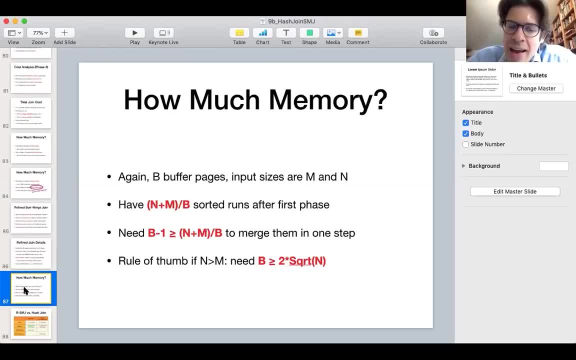 satisfy this constraint. I should have something like the square root of the larger table as a main memory times two. furthermore, if I have that, then those constraints are satisfied. so this is the refined version of the sort merge join. it is the most popular variant of the sort merge join. 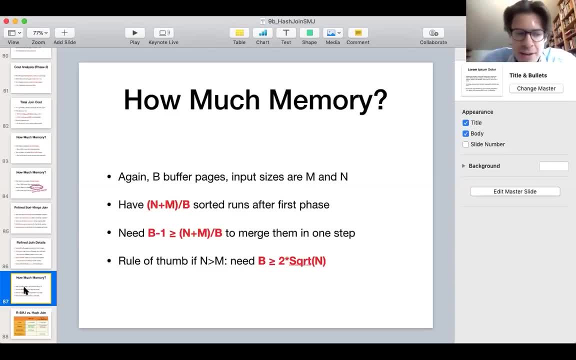 because it only goes over the data twice, once in each phase, and in terms of cost it is actually quite similar to the hash join algorithm. so this is why people often compare the pros and cons of the hash join algorithm and of the sort merge join algorithm, because both of them are also. 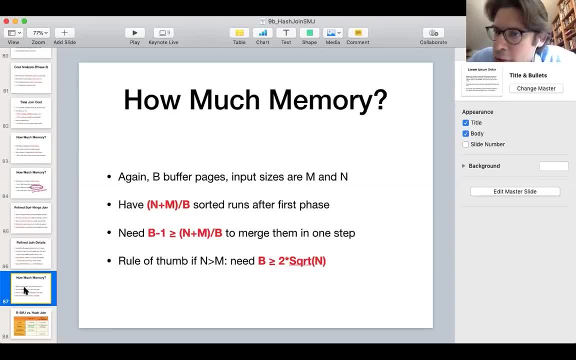 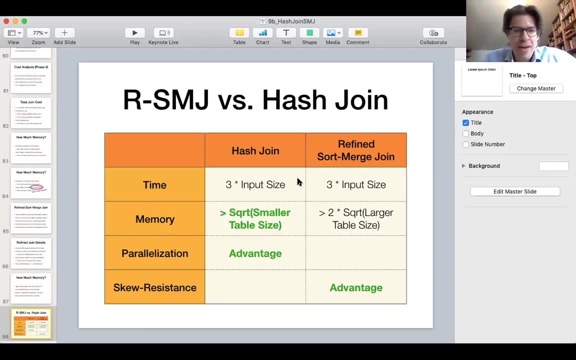 applicable specifically for equality join conditions. now, this is an overview. here we have the hash join and the refined sort merge join, which both have a time complexity that is proportional, that is linear in the input data size, measured by the number of pages. so time wise they can be. 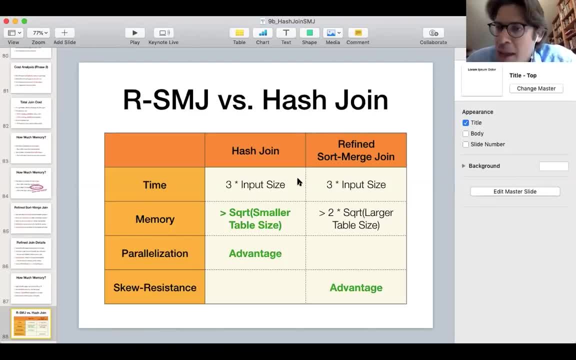 near equivalent. then, comparing the main memory consumption, we find that the refined sort- merge, join- takes a little bit more main memory, because here you're taking the square root of the larger table, while for the hash join you're taking the square root of the smaller table size. 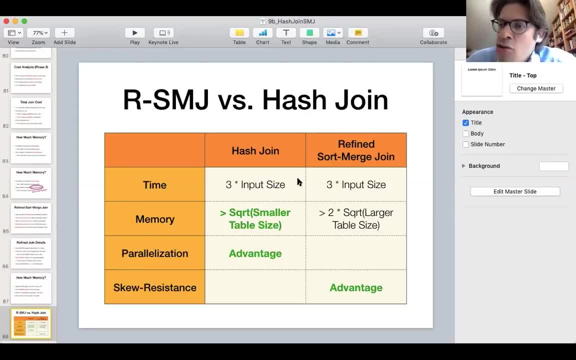 because you can choose for which of the two input tables you're loading the corresponding hash buckets into main memory at once. so slight advantage for the hash join here. and when it comes to parallelization, then the hash join is actually also a good idea. you can very easily calculate those hash. 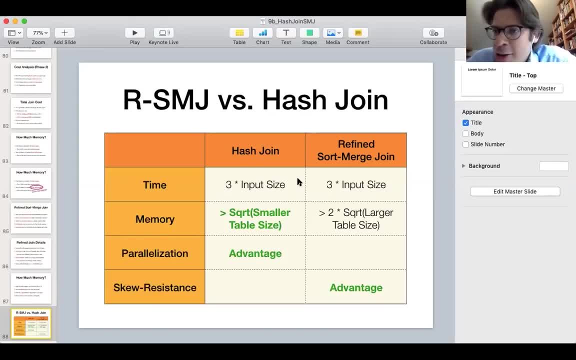 functions in parallel. in the first phase and then in the second phase you can just assign different hash buckets to different processes. so that is quite convenient. having said that, the refined sort merge join can also be parallelized, but it is particularly convenient for the hash join. now, when it comes to 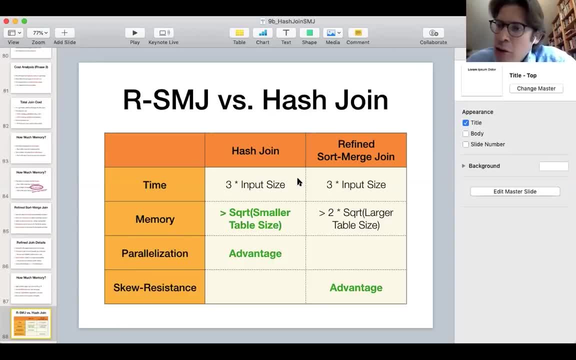 skew resistance. and that means how well does the join algorithm work if i have, for instance, lots of duplicates in my data? in that case the hash join algorithm might not be the preferred choice, because if we have lots of duplicates, then all of them will have the same hash function. 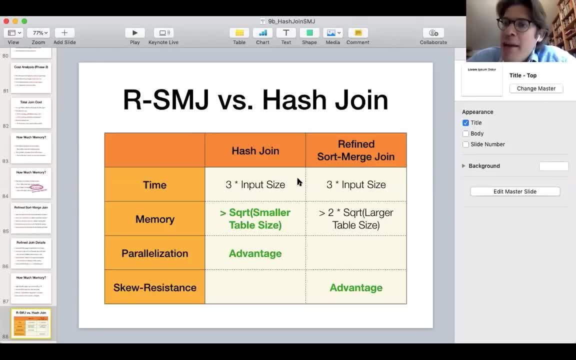 value and that means all of them will belong into the same hash bucket and that means that it becomes very difficult to fit things into main memory. so if you have a lot of duplicates, then the hash join algorithm might not be the optimal choice. on the other side, for the 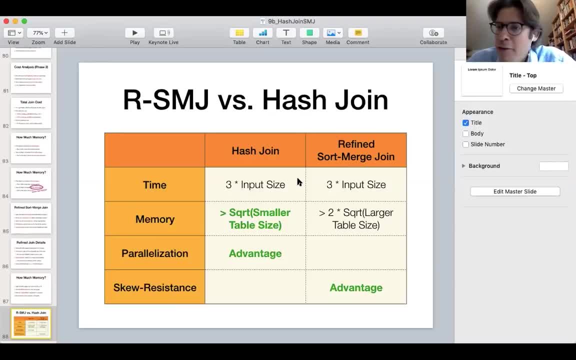 sort merge join that one can deal relatively well with skew. you just have lots of duplicates that appear one after the other in the sort order. so if you have lots of skew then perhaps the refined sort merge join algorithm is a good choice. another point that is not mentioned here in the slides: 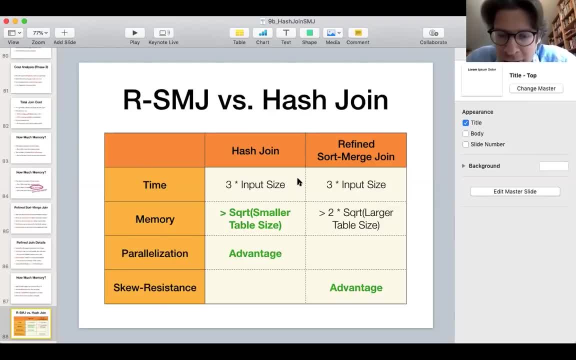 we will come back to that point later, but i already wanted to mention it here. one advantage of the refined sort merge join is that the output of this join is automatically sorted and there are certain operations that become cheaper if you have sorted data. we will see some of. 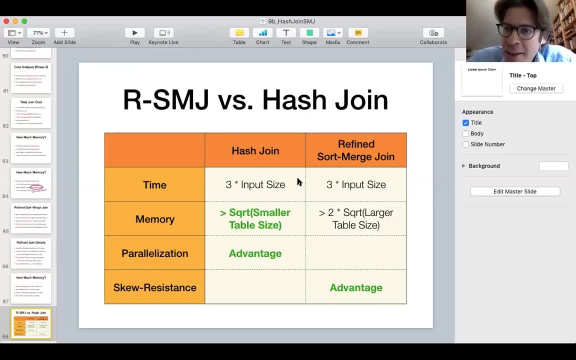 those operations in the following slides. so in some cases, even if using the sort, the refined sort, merge, join alone is not what you want to do, maybe you still go for it because it makes the following operations cheaper. that's something that we will come back to later. 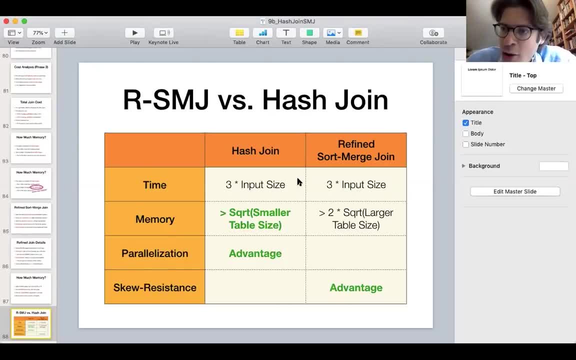 alright, and this concludes our section on join algorithms. we have seen various join operator implementations. some of them are applicable specifically for equality join conditions, which is perhaps the most common case in practice. others are more flexible and can be applied for arbitrary join conditions. they have different pros. 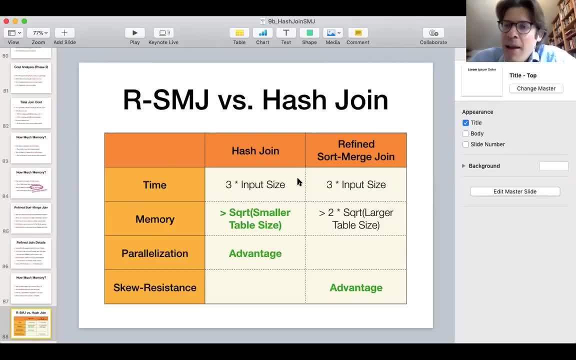 and cons in terms of time, complexity, as well as in terms of main memory consumption, and the hash join and the refined sort merge join. this is some of the most commonly used join algorithms in practice. alright, now we are going to see a couple of other operators in the following and: 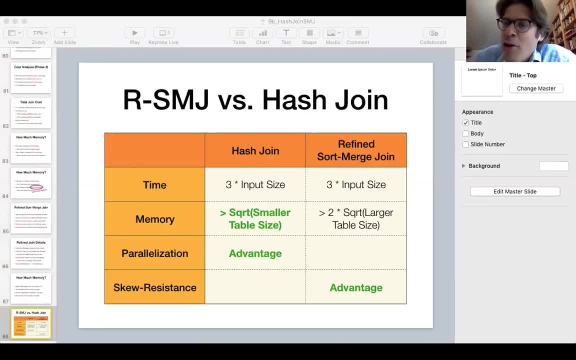 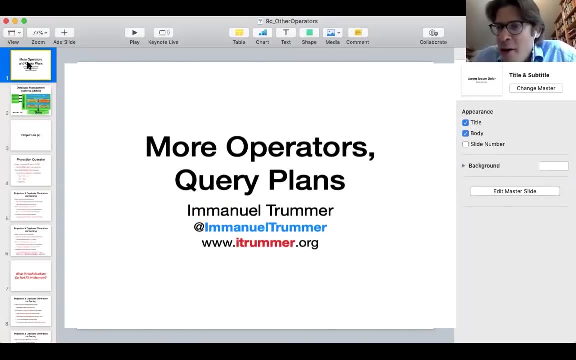 in the end we will also start discussing about how we can compose those operators into query plans. I quickly switched the slide deck and please let me know if there is any problems seeing those slides. now, in the following we are going to discuss about a couple of other operators. 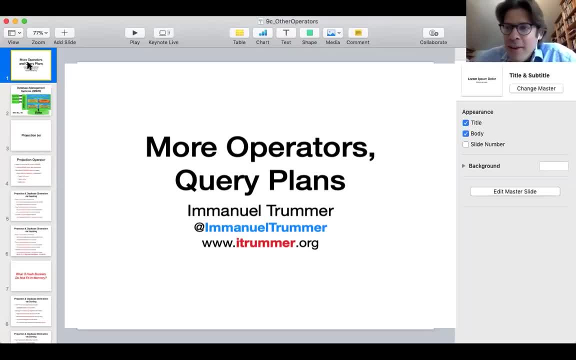 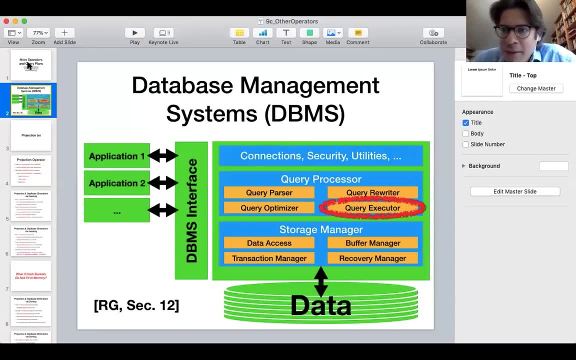 and finally we will start discussing about query plans. so here that is always the architecture slide at the beginning, but nothing has changed compared to the last slide deck. we are still discussing about the query executor, which executes those query plans, and the relevant chapter in the Ramakrishnan and. 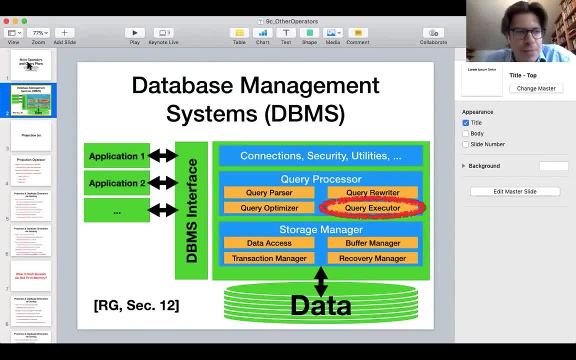 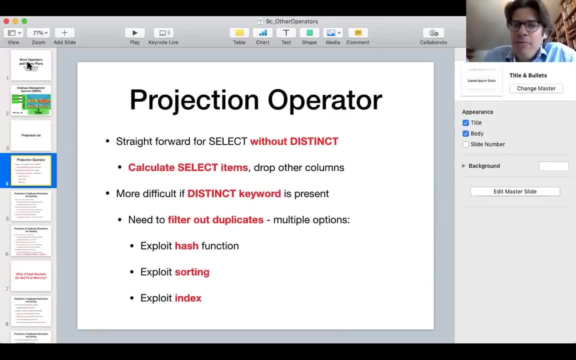 Gerke book, that is still chapter number 12. now, first of all, we are going to discuss about the projection operator. now, the projection operator simply means dropping away those columns that are not mentioned in the select clause and that can be quite straightforward to implement where it gets, however complicated. 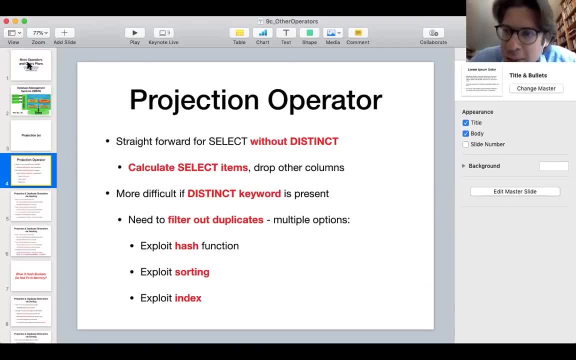 is if you use a select distinct as opposed to a simple select. if you write select distinct, it always means that the system should eliminate duplicate results, and then you have to implement this in a naive way. it would require pairwise comparisons between different records in the data set in order. 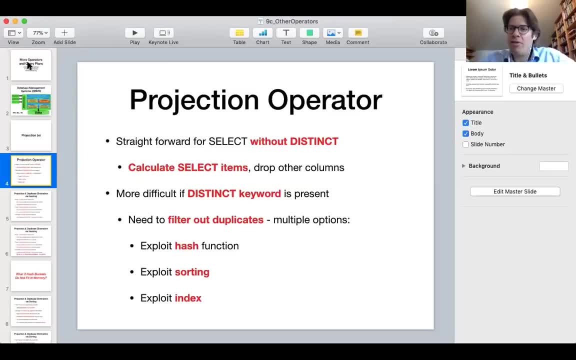 to identify those duplicates. so, in order to avoid all those pairwise comparisons, which would be inefficient, there is a couple of ways of doing things in a smarter way. first of all, you can exploit hashing, which essentially allows you to restrict comparisons to tuples that appear in the same 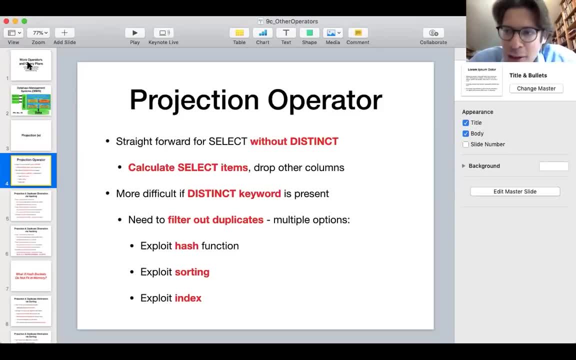 hash bucket, or you can use sorting, which means you can restrict comparisons to tuples that appear close together in the sort order, or you can exploit indexes if available, and since an index might already give you a sort order, it means that you can exploit the sort order without having to do the 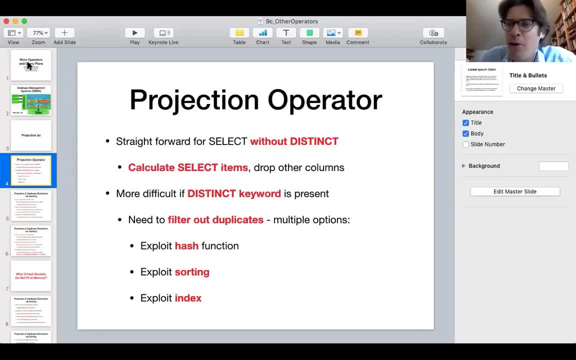 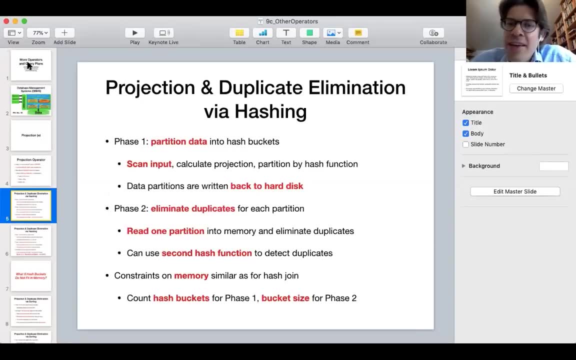 actual sorting. now. in the following we are going to discuss about those possibilities in a little bit more detail now. first of all we are going to see how we can do the projection and duplicate elimination using hashing. so this algorithm again executes two phases. in the first phase we are 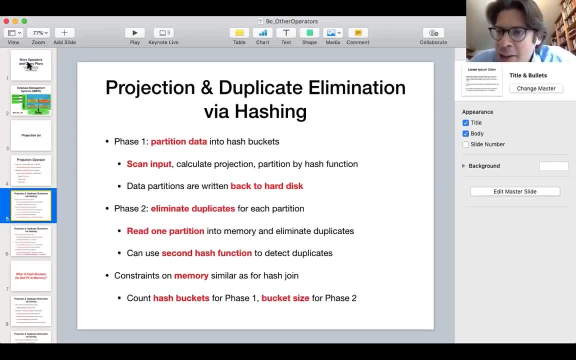 partitioning the data using hash function. in the second phase we eliminate duplicates for each of the hash buckets. now in a little bit more detail. in the first phase we would just read the input data one page after the other one, and for each record in the input data we would 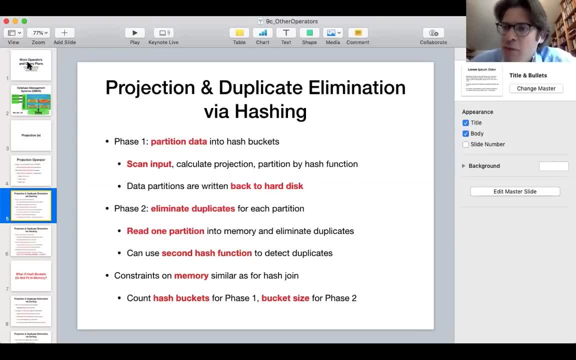 immediately calculate the projection, which essentially means that we are throwing away columns that don't appear in the select clause. then we partition the data using the hash function. so again we have like one output buffer associated with each hash bucket and then, based on the hash value, we are 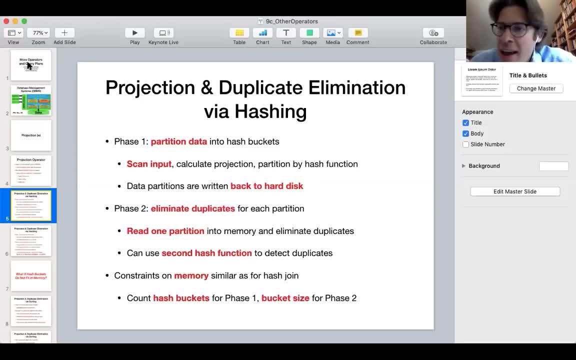 writing the tuples into the corresponding hash bucket, and whenever one of those output buffers becomes full, then we write the content back to hard disk. so this is what you have already seen when we were partitioning inputs in the context of the hash join. so the principle is exactly. 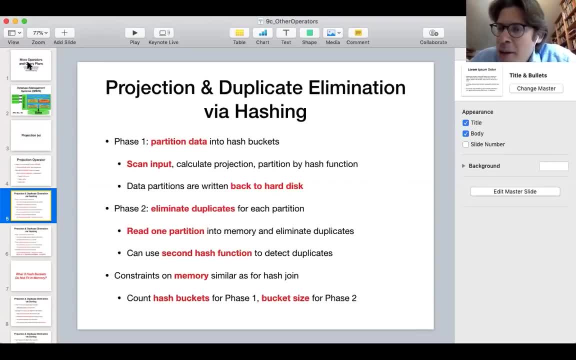 the same, except that we are dropping columns that don't appear in the select clause when loading data. in the second phase we load the data for one of those hash buckets into main memory and for the data that we have currently loaded we eliminate the duplicates now in our cost model. 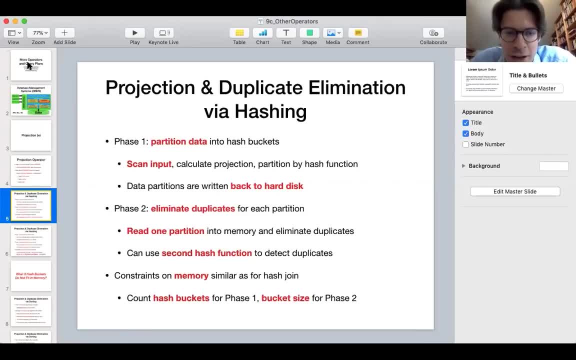 we only count a cost related to loading data from hard disk, so essentially those comparisons for in memory data are for free, according to the simple model. in practice, people often try to make even the in memory comparisons more efficient by using, for instance, a second hash function that you 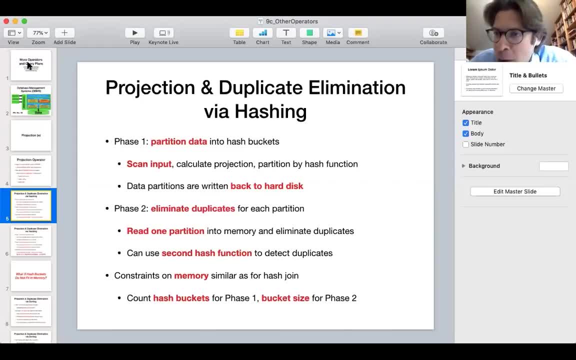 apply to the tuples that appear in each of those hash buckets in order to quickly find potential matches, potential duplicates, to eliminate the constraints for main memory. they are similar as for the hash join. in the first phase, you need to be able to reserve one output buffer for each hash bucket and 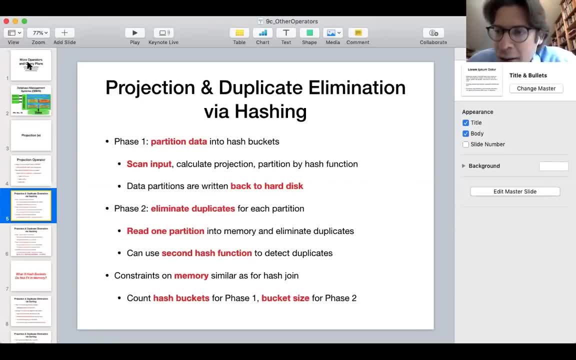 in the second phase you need to be able to load into main memory one entire hash bucket, so that applies a couple of constraints on memory size. the reasoning is the same as for the hash join, and if you do that in two phases then the cost is at most. 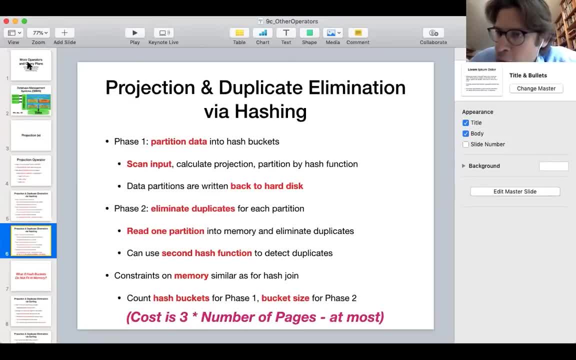 three times the number of pages, because in the first phase we are reading data once and we are writing data once. now the data that we write might actually be a little bit less than the data that we have read because, first of all, we are dropping unnecessary columns that don't appear. 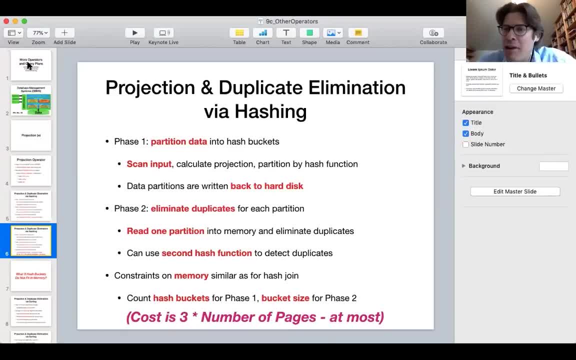 in the projection and also if we happen to already detect some duplicates, then we can already eliminate that data. so the data that we write to hard disk after the first phase might actually be smaller than the data that we have read from hard disk at the beginning of. 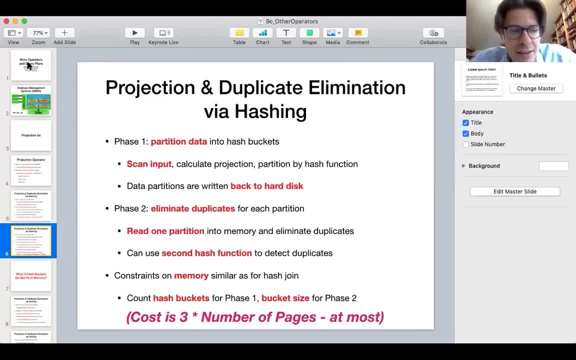 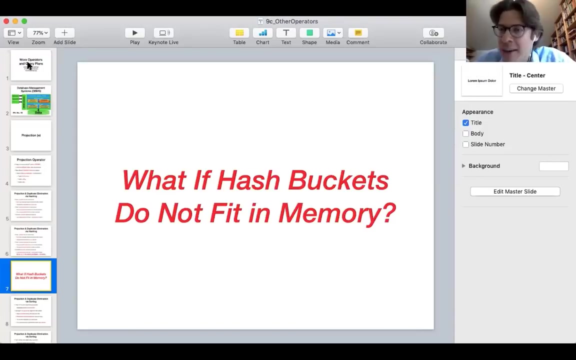 the phase. so this is the cost, assuming that you can do the whole duplicate elimination by two passes over the data. now imagine for a second that in the second phase we are unable to load one entire hash bucket into main memory. does anyone have an idea about what we could? 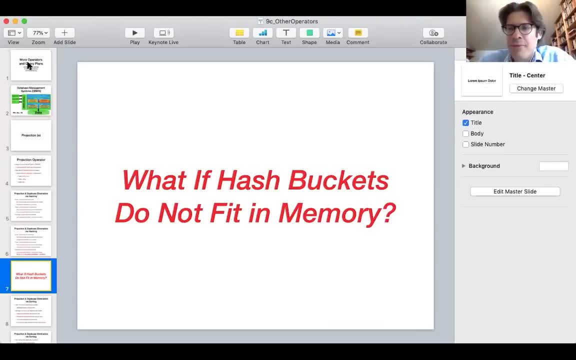 do in order to deal with that situation. we had already discussed a similar case in the context of the hash join. we also sometimes had cases where it is not possible to fit one entire hash bucket into main memory. so what can we do in order to reduce the size of those hash? 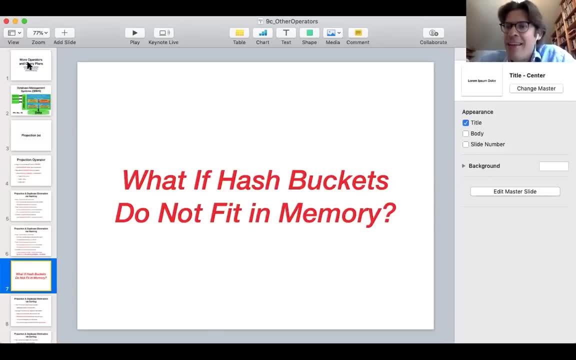 buckets further. yes, exactly, yes, very good. so here i see the right answer in the chat. exactly, so we can just split those buckets further into sub buckets and in order to do that, we can just pass over the data multiple times in the first pass. we are partitioning data into large buckets. 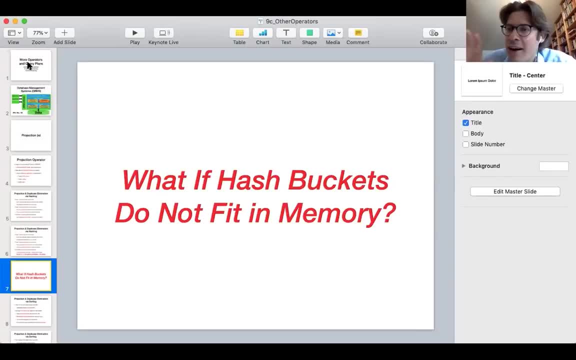 then in the second pass, we partition each of those buckets into smaller sub buckets and so on. we can iterate that until one of those hash buckets fits entirely into main memory. of course, in order to be able to do that, we must assume that we don't have too many. 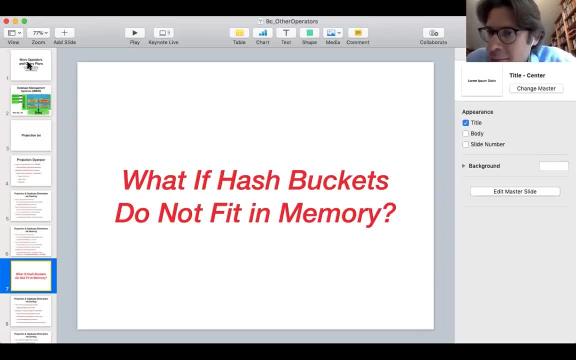 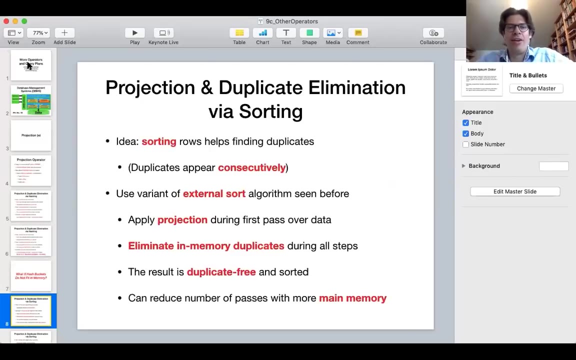 duplicates in our data set in, because if you have too many duplicates, then all of them will end in the same hash bucket and that can be problematic. okay, so now the second possibility to speed up duplicate elimination, that is via sorting. so here the main idea is that duplicates 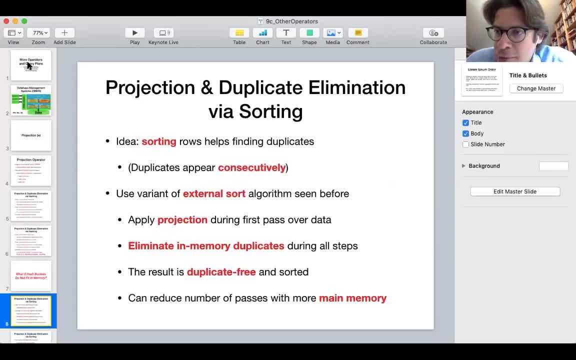 must appear close together in a sort order. so also by sorting things we can reduce the number of required comparisons, because now we only need to compare things that appear close together in the sort order, and in order to do that I can use a variant of the external sort algorithm. 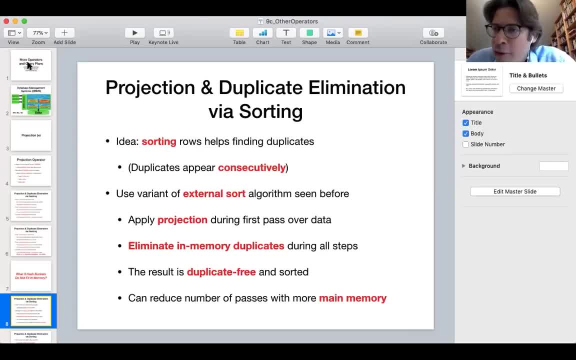 that we have seen before. so in the first pass over the data, I am again applying directly the projections, which means that I'm throwing away columns that don't appear in my select statement whenever I do one of the sorting steps, whether that is the initial step or whether that is some of the merging steps. 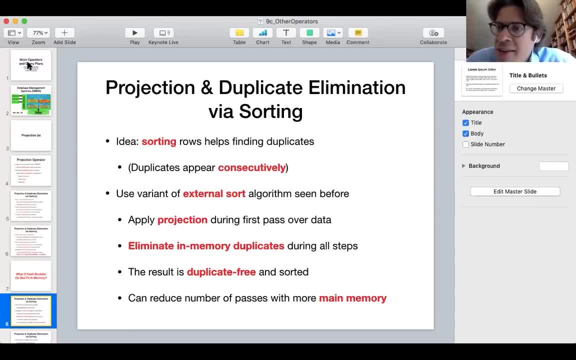 always, I eliminate duplicates immediately once I discover them, and the result of this variant of external sorting is, first of all, sorted and, more importantly, it will be duplicate free. so this is very similar to this external sort algorithm that we have seen in the context of the sort 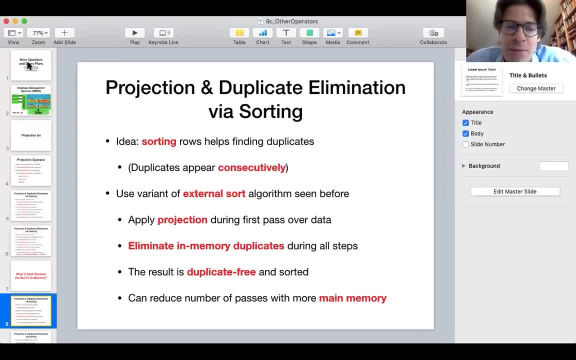 merge, join, just that. here I am eliminating unnecessary columns and I am eliminating duplicates as soon as possible. the amount of main memory is not fixed, but the more main memory you have, the faster it gets, because you have to make less passes over the data and then the cost is at most. 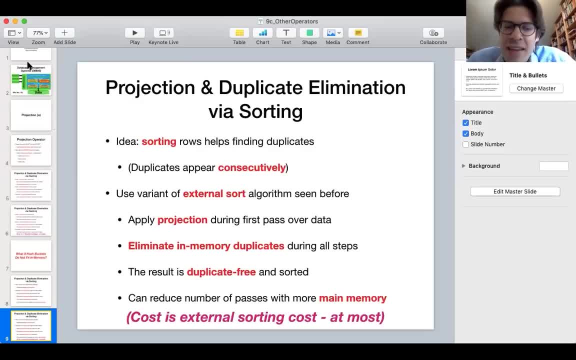 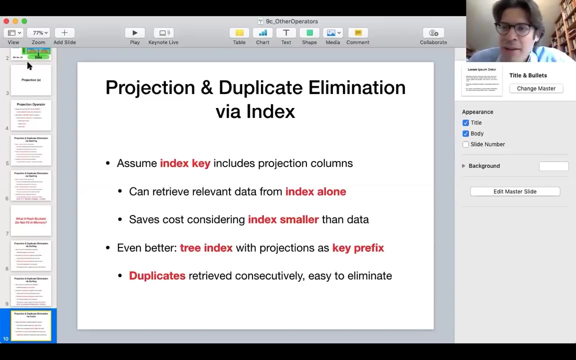 the one of external sorting, because the data that you are sorting here it might actually decrease over time once you drop columns or once you eliminate duplicates alright, so that is a possibility to do duplicate elimination via sorting. if you have an index already available, you might be able to save. 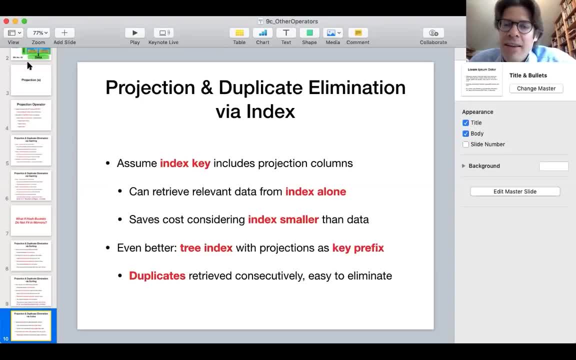 the sorting step. the only thing you need is that the index key includes the projection columns, so, first of all, we can use the index in order to retrieve all the relevant data without having to look at the actual table data, and since those indexes are typically much smaller. 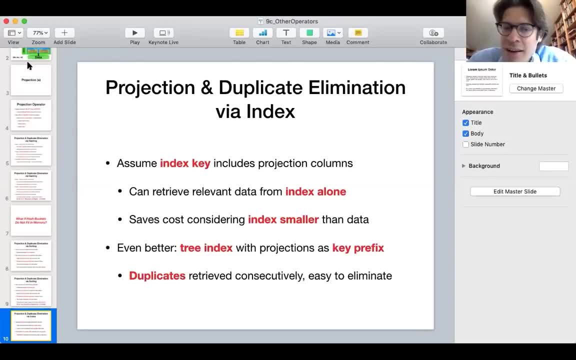 in terms of data size compared to the actual table. that saves some cost. what's even better is if you have one of those indexes that return the data in sorted order- particular tree indexes that we have seen- and if the columns that you are projecting on form at least a prefix. 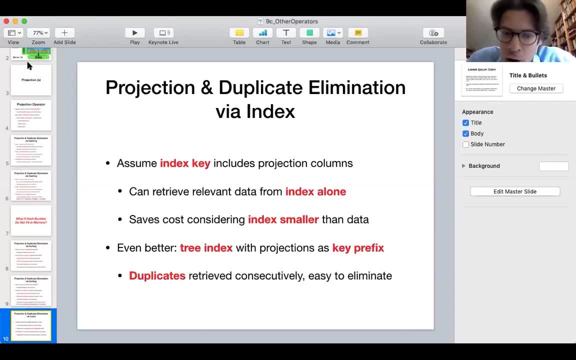 of the index key. that means that you can retrieve the tuples in sorted order from the index and that makes it very easy to eliminate duplicates. so if you have an index available, that might make it much faster to execute one of those select distinct classes and the cost here. 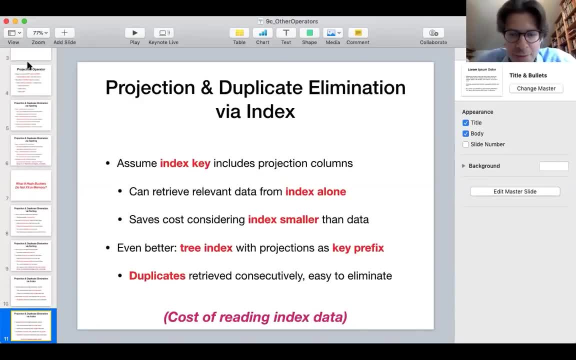 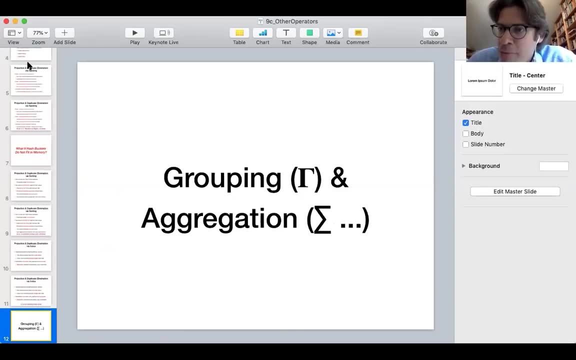 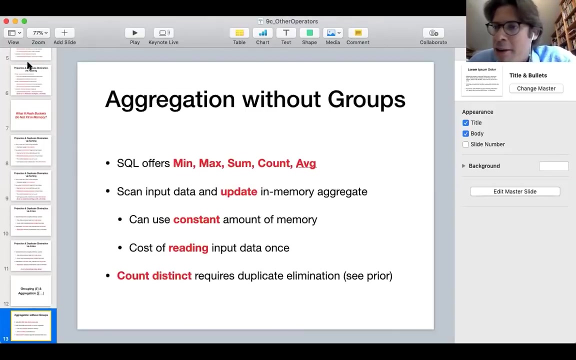 is generally the cost of accessing the index. now that was the projection of the table. next we're going to discuss about the grouping and aggregation. now aggregation without grouping is relatively easy to do. you might still remember that sql offers those aggregation functions you see. here you can calculate minima, maxima. 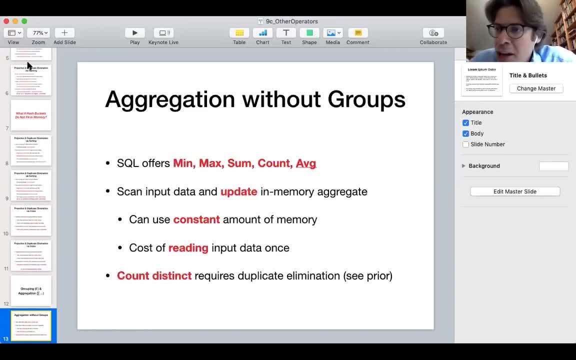 sums, counts and averages and typically, if you don't have any groups, you can scan the input data and you have some fixed counter in main memory that you keep updating whenever you read new records from the data. that works with a constant amount of main memory and once you have scanned, 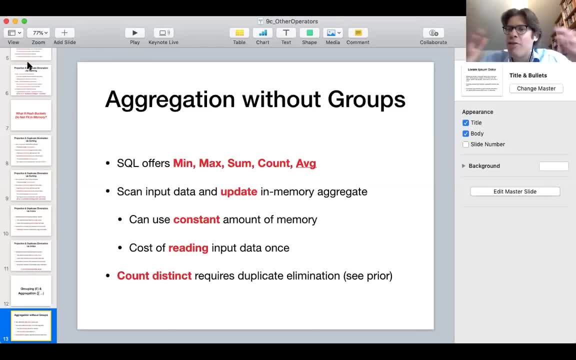 all the data, then you have the final aggregation value in memory, so, for instance, the minimum seen so far in main memory, and you keep scanning the tuples from the table and update the minimum whenever you encounter a new minimum. the only aggregation that can become a little bit more expensive. 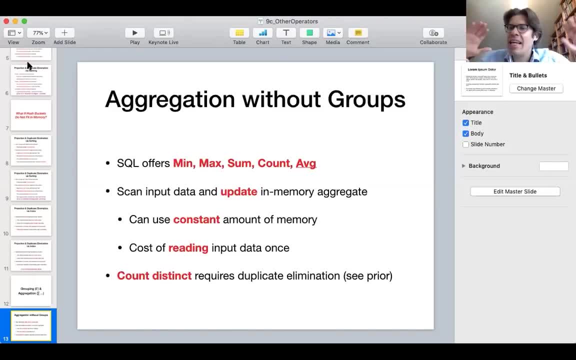 even without grouping, that is count, because inside the count operation we can also have distinct keywords. so we ask the database system to specifically count distinct elements, and if you do this, then again we need a method for duplicate elimination and in order to do this we can use the methods. 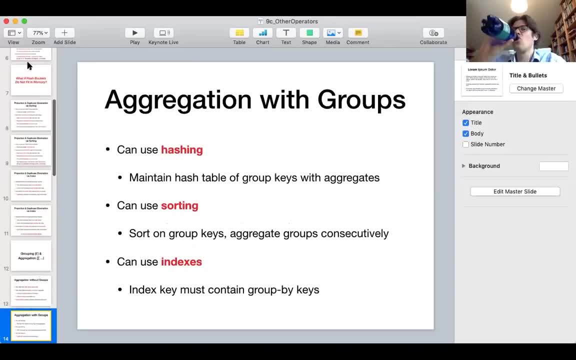 that we have seen for the projection on the previous slides. so the distinct elements are restricted to the count. alright, there is a question about how minimum and maximum relates to deletions. so in general, we will discuss more in coming lectures about how we can update data. for the moment, we assume 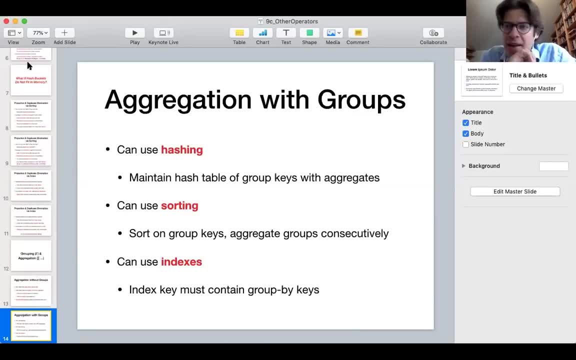 that the data remains the same as the previous ones. so the question is: how do we do this? if we have an aggregation together with grouping, then we have to do a little bit more. we have again those possibilities to use hashing, sorting or existing indexes, if they are available. 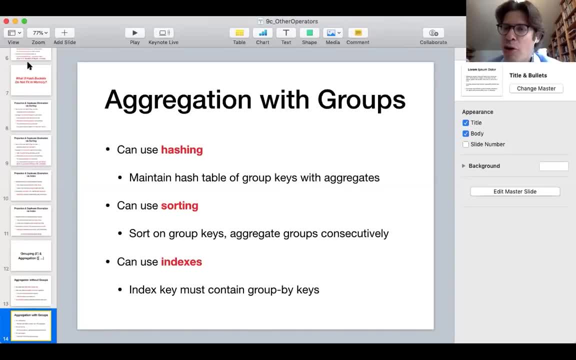 so if we decide to use hashing, for instance, then we would maintain aggregates. so we go over the data and for each new tuple we determine the corresponding hash bucket in our in-memory hash table and there we update the counters that are associated with the corresponding group key. 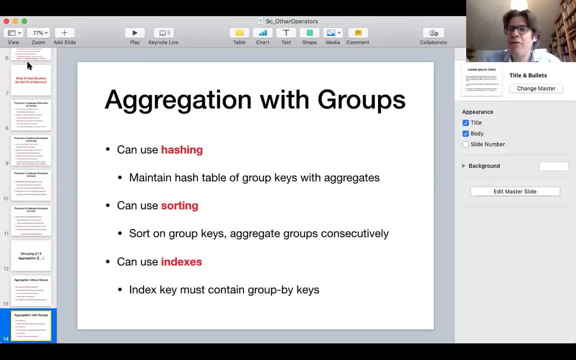 we can also use sorting, because, after you sorted your data by the group keys, it means that the members of the same group appear consecutively and because of that you can essentially calculate the aggregation value for each group, one after the other one. so here we sort by the group keys. 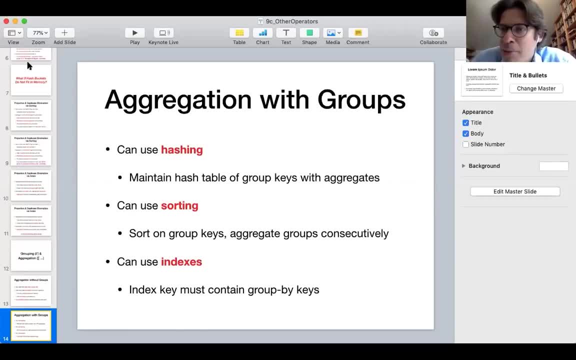 and then we can calculate those aggregates consecutively for each separate group. and finally, if you have indexes, that might also help you to speed up things here- we want the indexes to contain the group by keys, and then you can again treat each group separately with entries which have specific values. 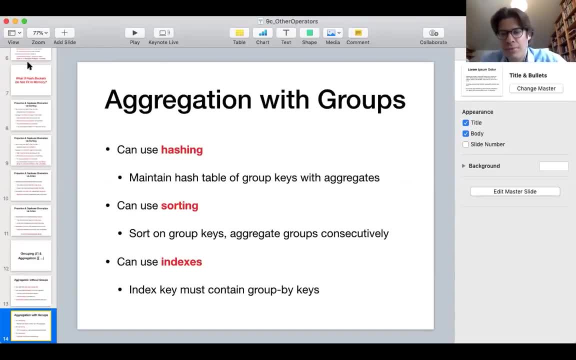 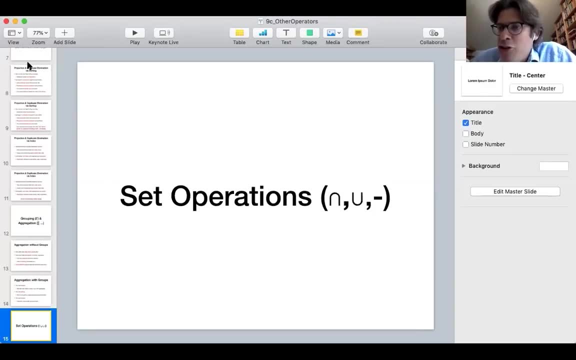 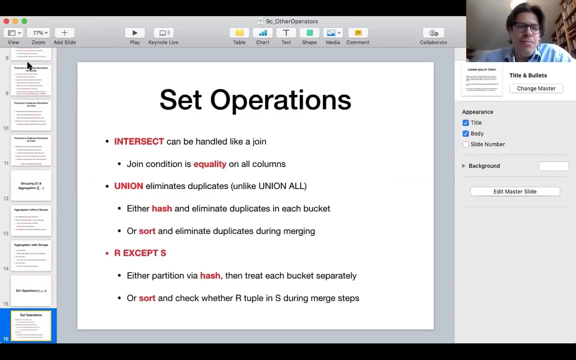 in the group by columns. so last we will discuss about the set operations, union and intersection, and set minus operations. so here the principles are similar to the ones that we have already seen before. for instance, the intersection can essentially be handled by some kind of join, the only thing that you need. 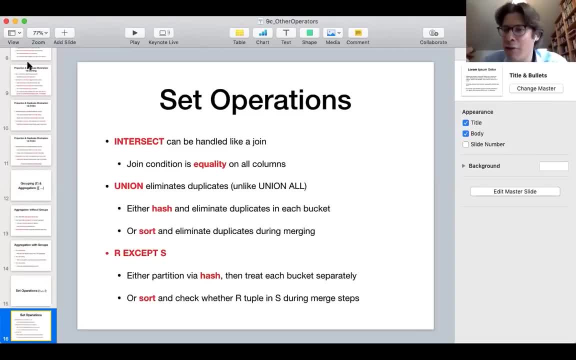 is a join condition which essentially makes all the columns equal, and then the result of that join will give you the intersection result for union. the union operation eliminates duplicates by default, so you can use similar techniques to before in order to detect those duplicates. either way, we can use a hash function. 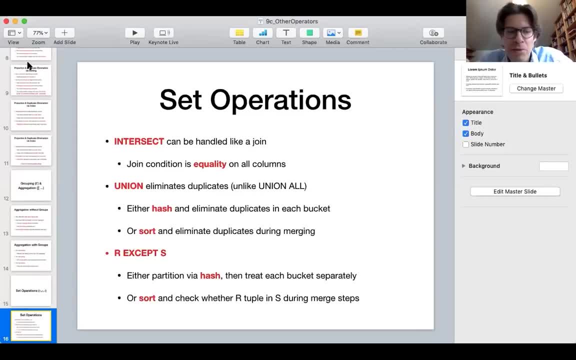 to eliminate duplicates in each hash bucket separately, or we use the sort function and then we know that duplicates will appear close together, so that also makes it easier to eliminate them during merging. if I have the except operation, which means that I am subtracting one set from another one, 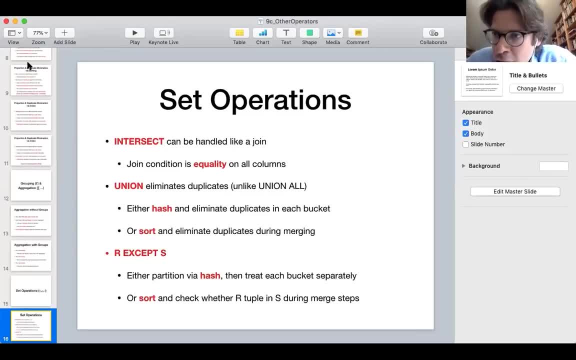 then I can also reduce comparisons if I first partition the two relations r and s into hash buckets and then treat each hash bucket separately, or I can again sort them such that the same entries appear close together and then I can just check whether tuples in r also appear. 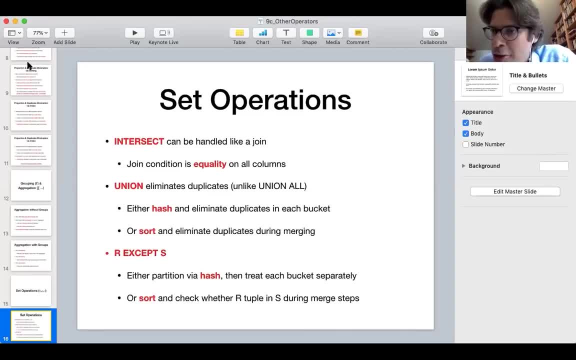 in s. so in general, as you notice, for many of those operations I am using kind of the same ideas in order to speed them up. whenever I have something that would require pairwise comparisons, I am typically using either hashing or sorting in order to reduce the number of comparisons required. 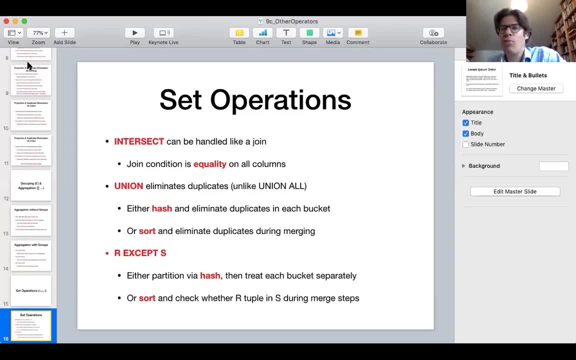 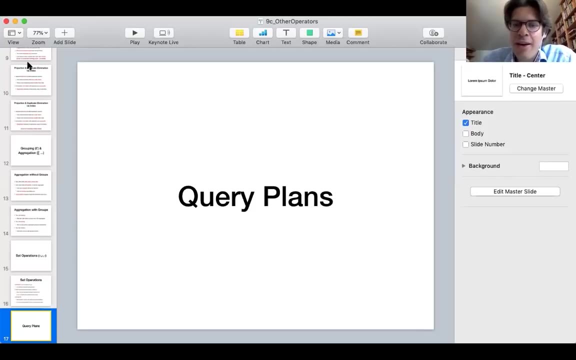 or if I have a suitable index, I can often use that one as well. so there is a couple of ideas about how to speed up data processing that transcend all those different operators. alright, so now we have seen all the implementations of those separate standard operators now in the following: 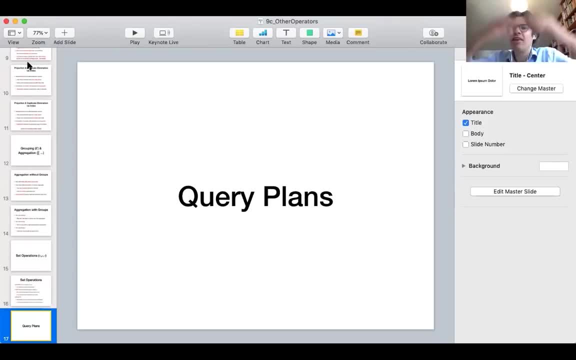 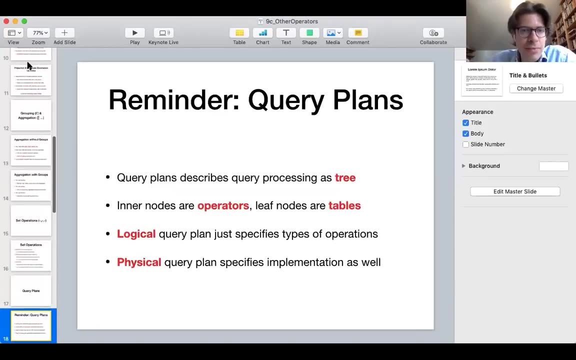 we are going to discuss more about how we can compose multiple operators into one common plan, because that is what is typically required in order to answer your queries. now, as a little reminder, query plans are typically represented as trees and the inner nodes in those trees they correspond to. 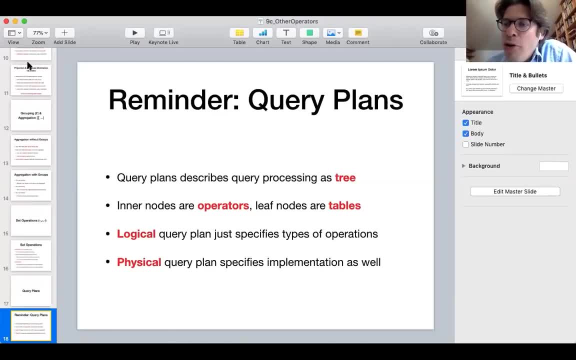 tables. now the logical query plan specifies just which operation types have to be applied, in which order. the physical query plan is more detailed and additionally specifies how those operators are implemented. and now you see why that is important, because we have seen all those different operator implementations and choosing the right one. 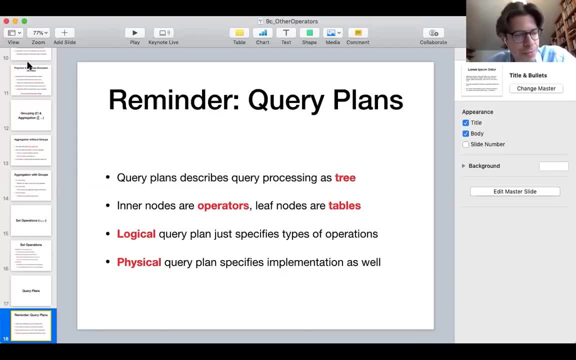 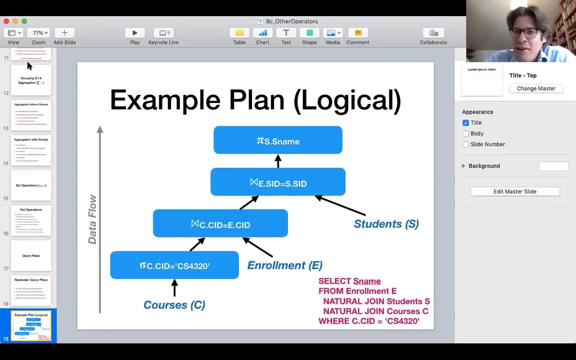 can actually make a big difference for performance. now this is an example logical query plan over here in order to answer the query that you see on the right lower corner of this slide. so here we are, selecting the names of students from a join between students enrollment information. 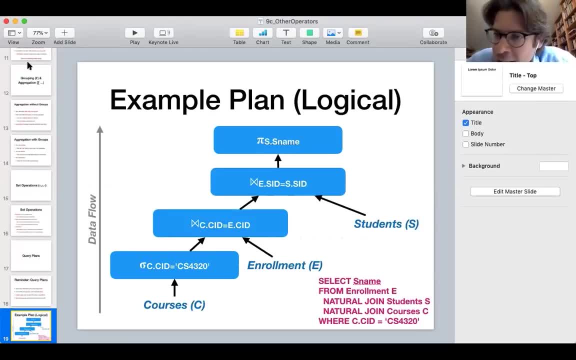 and courses, matching up students with the courses that they are taking. and additionally, we are narrowing things down to the courses, to one course specifically, which is CS 4320. now those query plans are evaluated bottom up. so here I am, starting, for instance, by reading the courses. 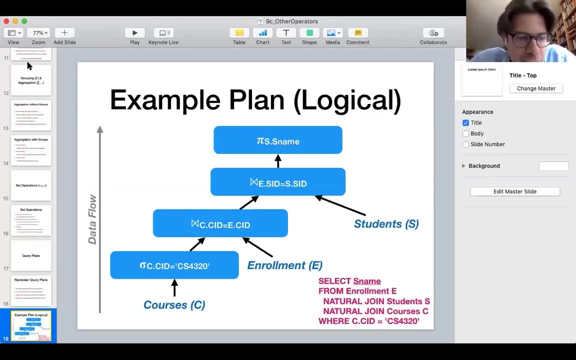 a table. then I am applying the filter condition, and the filter condition is represented by this little sigma together with the corresponding condition. then I am feeding the result of the filter into a join together with the enrollment table and we join using the course ID and the result of that join. 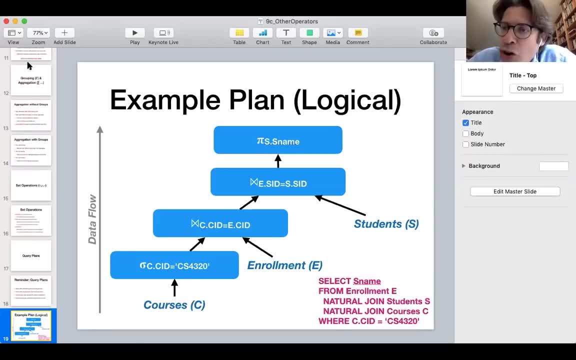 is fed into the next join together with the students table. and here I am joining on the student ID. finally, I have a projection operation where I am eliminating the columns, except for the student name column. so the data flow in this plan goes from the bottom to the top. 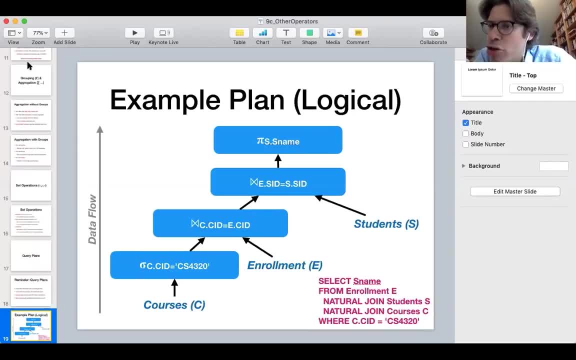 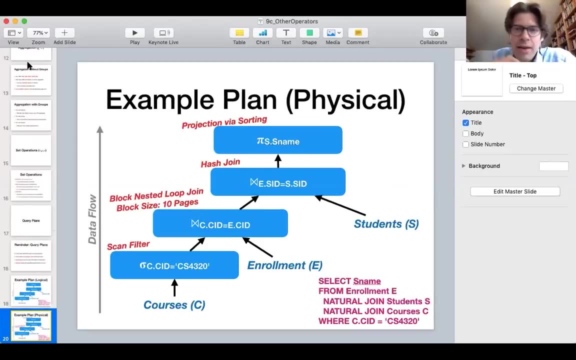 because it only specifies that we have to do a join, for instance, but it doesn't yet specify how to execute this join. now, this is the physical plan version, which provides more details, and here you see that I have written the way in which those operations are implemented. 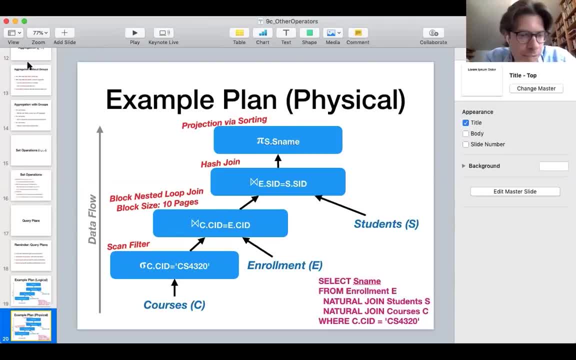 next to each of those nodes. so here, for instance, the initial filter, that is just a scan filter, so I am not using indexes or anything fancy, I am just scanning the pages, one after the other one, and I am evaluating the filter condition. the join here, the first one. 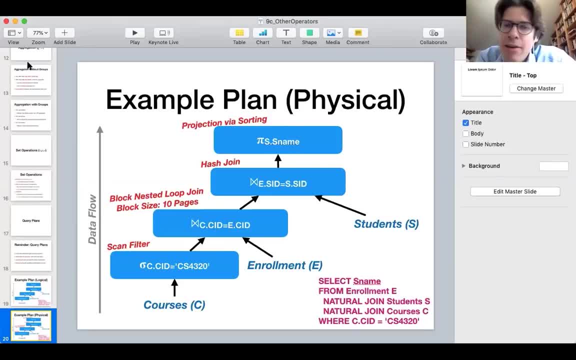 is implemented as a blockness, a loop join, and the physical plan also specifies details such as: how many buffer pages do you want to reserve in order to store blocks from the outer relation? and when writing those query plans, then by convention the left input operation is always. 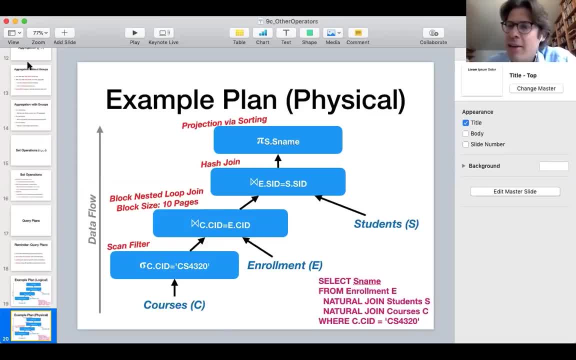 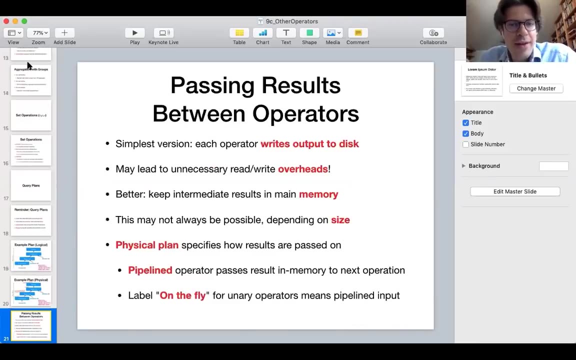 the outer relation, which is important, for instance, for the cost of those join operations. now, the second join will be the hash join that we have seen and then, finally, I am doing a projection now, when composing those operators, it is important how I am passing on data from one operator. 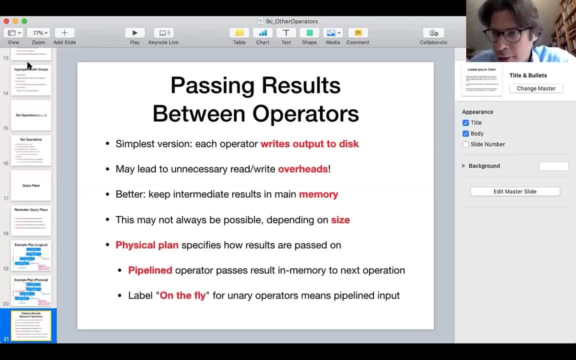 to the next one, and in this naive implementation I could say that each operator simply writes the result of the operation back to hard disk and then the next operator in the plan can read that result from hard disk again. now, the problem with that is, of course, that it is less efficient than possible. 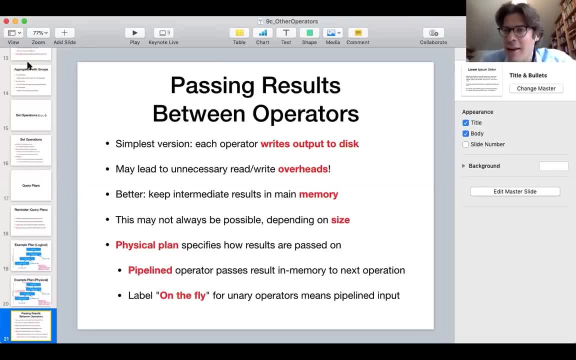 because I keep writing things to hard disk and then reading the same things from hard disk again. so, in order to make things more efficient, people typically try to keep the intermediate results in memory if possible, in order to avoid writing and reading them. whether that is possible or not depends on 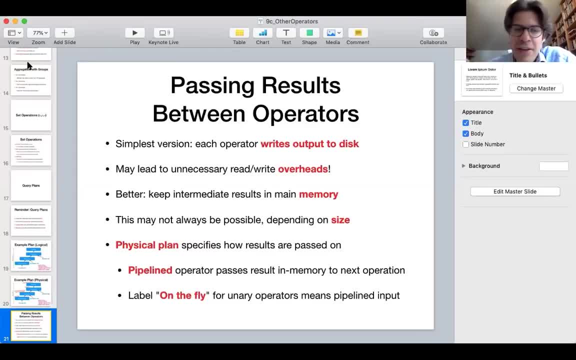 the operators involved and on the sizes of those intermediate results. so the physical plans additionally specify how those results are passed on between different operators. now there is the keyword pipelining, which you might already have come across. so in this context, pipelining means that one operator passes. 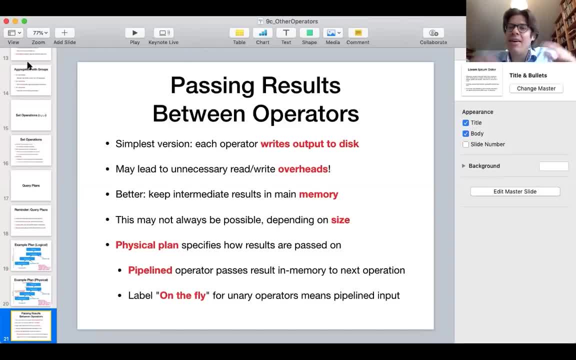 results, or besides pieces, in to the next operator in main memory. so we avoid writing results to hard disk and then reading them again, which is also called materialization. and another label that goes together with pipelining, that is the label on the fly, which is typically used. 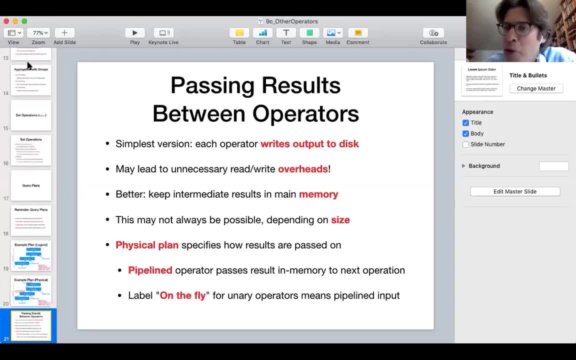 for unary operators, meaning operators that have only one single input, like a filter or like a projection, and for those operators it means that the input comes directly from main memory and doesn't have to be read from hard disk, which means that those operators in our simple model are essentially 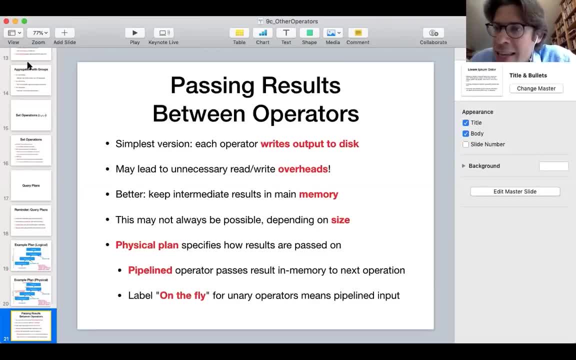 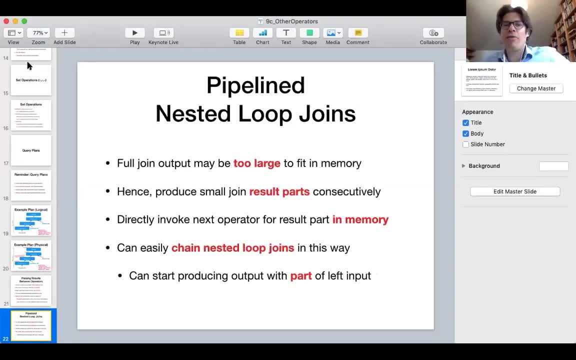 for free, at least when it comes to the input. they might still have to write their output somewhere. okay, now, one way is to use pipelining, in which pipelining is often used, so i'm mentioning that, since it is a very common pattern. that is, if you pipeline multiple. 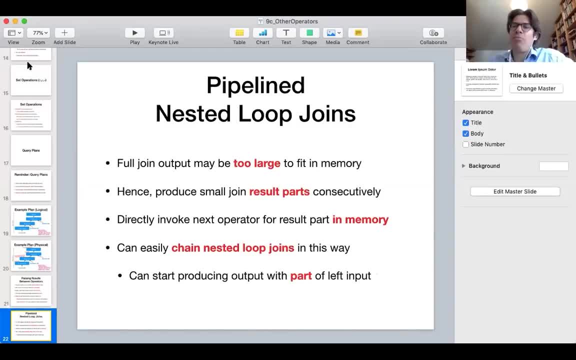 nested loop joints together in a chain, basically. so you often have the problem that the full output of a join operation might be too large to fit into main memory entirely. so the idea here is that instead of producing the whole join result at once, i can just keep the 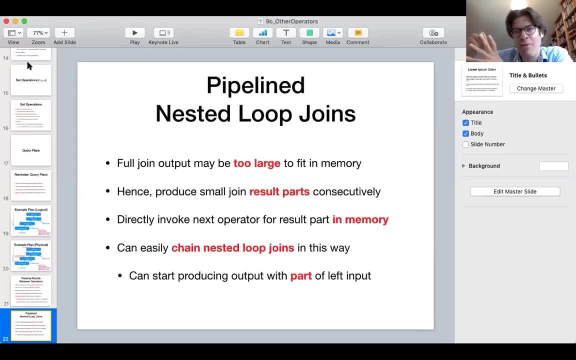 main memory and then immediately invoke the next operator on that in memory result part and nested loop joints. they work very well with that because, if you think back of how the algorithm works, they always get this chunk of data from the outer table and then they match that up with the pages. 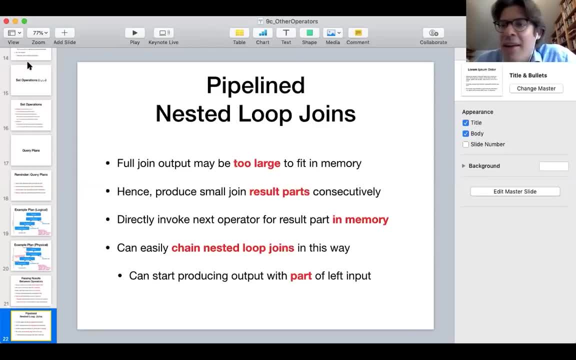 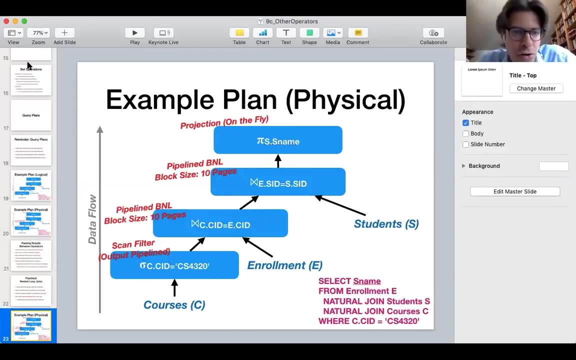 in the inner table. that means they can already get started quickly if they only are given one block, one part of the outer table. they don't need to wait until they have seen the entire table. and here, for instance in the example, we could also use a two pipeline. 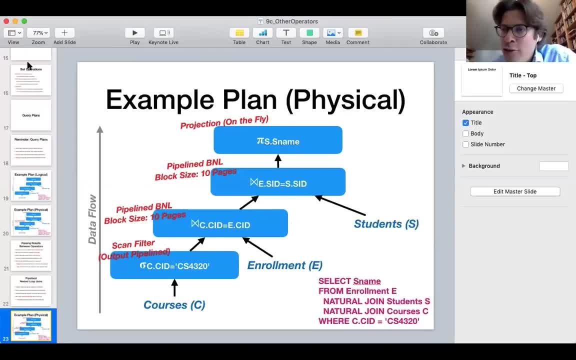 block nested loop joints. essentially, the first one produces always some part of the join result that is kept in memory, and then the second one processes the current part of the join result and produces again a part of the second join result. so this is the physical plan now marked. 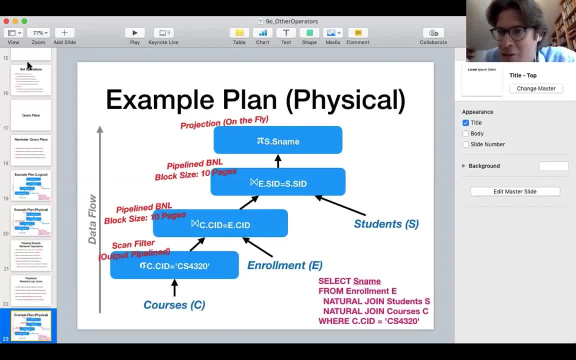 up with some labels that indicate how data is passed along between those different operators, and i'm gonna go over it in a little bit more detail. so again we start by the filter operation, and here we are, scanning all the pages from the courses, relations, and here the output. 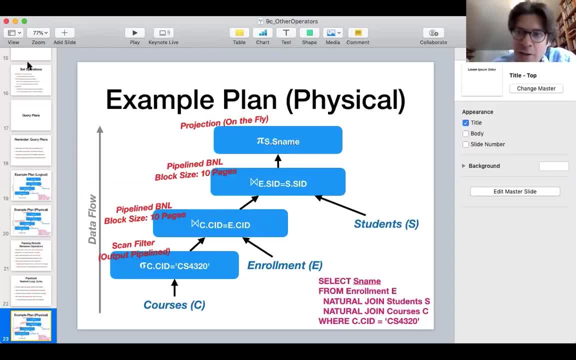 of the filter operation is pipelined to the next operation, which is a join, which means that we don't write it back to hard disk. and now there's a second join operation. it has a buffer of size: 10 pages for the outer, meaning for the left table. 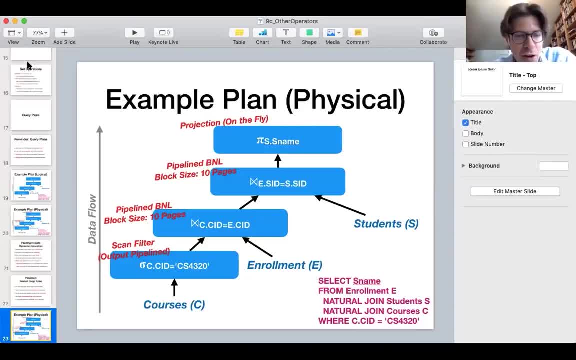 for the left input. so that means that this filter operator, the, keep scanning course pages and filtering them until the filter result has filled up the entire buffer of 10 pages for the following join. and if that has happened, then the following join proceeds in order to fill: 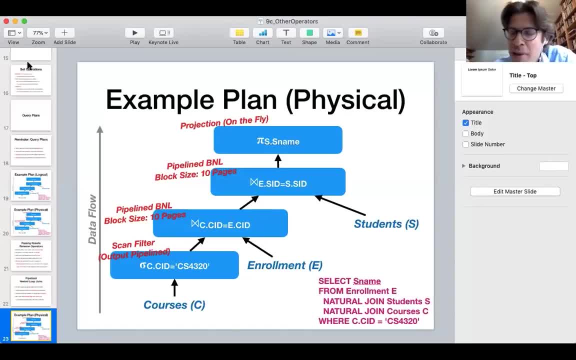 up the input buffer of the next join, which also has 10 pages, and once that has happened, the next join also processes the input in the input buffer and matches up the input in the left, in the left, on the left side, with the pages of the students. 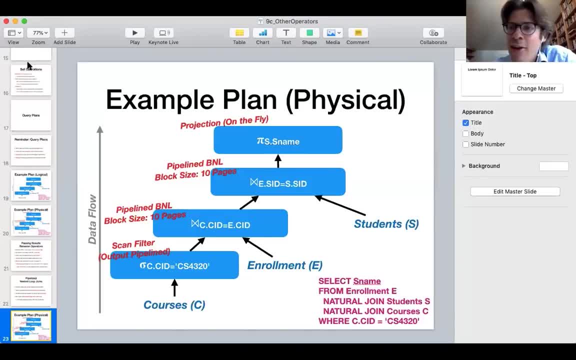 relation and pipelines it directly to the coming projection, and here we use the keyword on the fly for the projection, meaning that the input to the projection is in main memory and does not have to be read from hard disk. so here i'm optimizing performance by avoiding writing data. 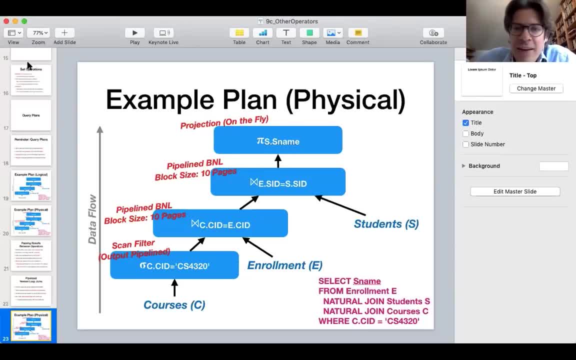 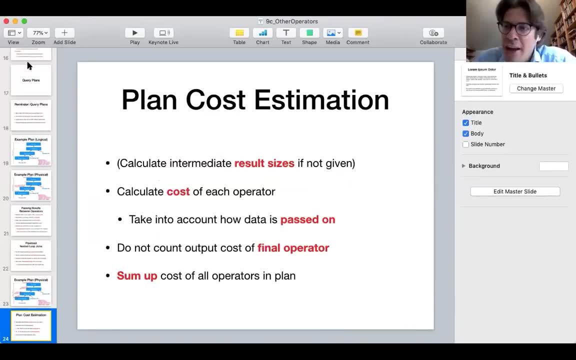 to hard disk and in the following as a little exercise. we're gonna make more exercises on that, but i wanted to encourage you to apply this principle here in order to estimate the processing cost of the plan that we have seen on the previous slide. so i will show it. 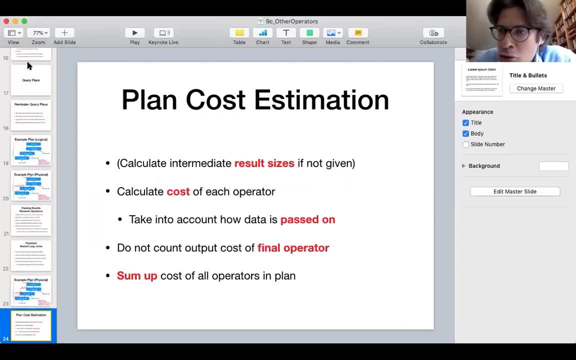 again in a second. so what you essentially need to do? so you generally need to estimate the sizes of each intermediate, precise if they are not already given. in this simple example, i'm gonna give you the intermediate beside sizes. then you have to estimate the cost of each operator, taking into 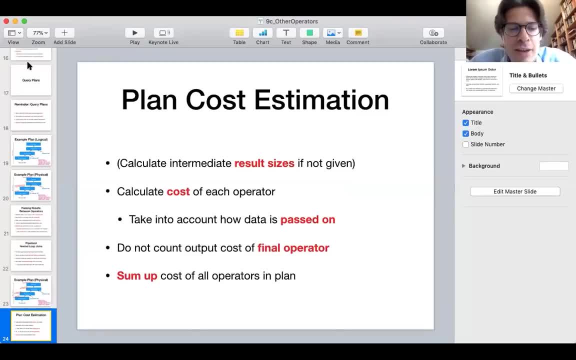 account how the data is passed on between different operators. don't forget, do not count the final output of the entire plan. you might very well have to count cost for writing out intermediate besides, but not for the final result. and finally you just sum up the cost of. 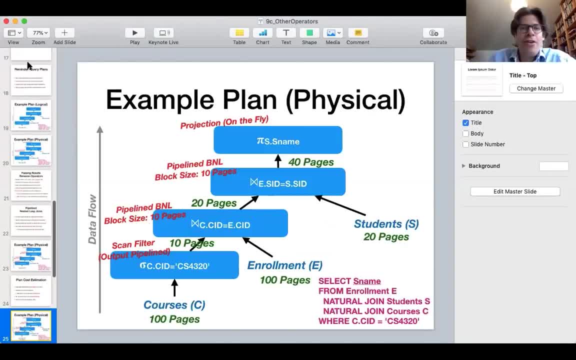 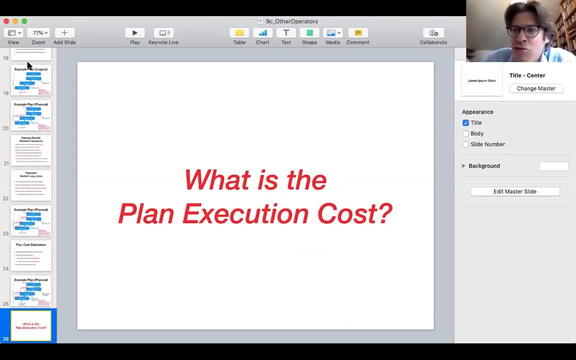 all operations in that query plan. so here i have the same plan together with intermediate, besides sizes in green and also sizes for the base table. so now have a look at this plan and try to estimate the execution cost, or think at least about how you would estimate the execution. 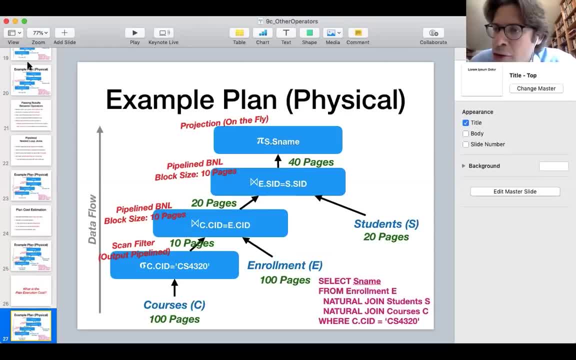 cost. i'm gonna give you just a few, one, two minutes- and while you're looking into this i can also answer questions in the chat, if there is any, and afterwards i'm gonna show you the solution and those set operations. okay, very good question. somebody's asking. 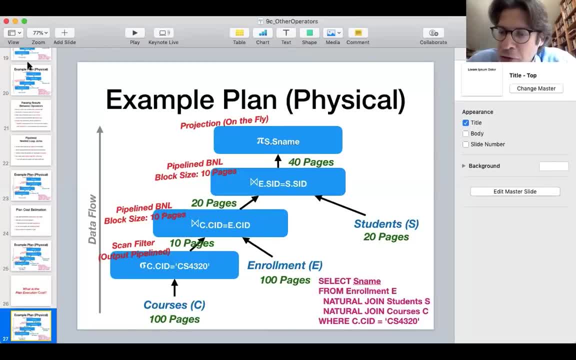 what the constraints are on the inputs for those set operations like union and intersection, and indeed you need that those inputs are compatible, meaning that they have the same number of columns and that they have the same column types. please feel free to post the questions in the chat. 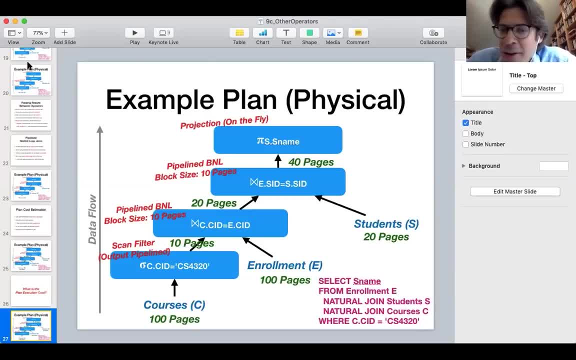 and otherwise i'm going to give you and otherwise i'm going to give you a few minutes. if you have any other questions- and yes, the column names can be different, but as long as they have the same type and there's the same number of them, you can use one of those- 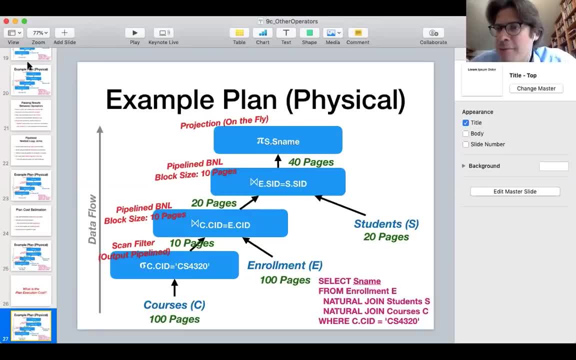 union or intersection operations. So when trying to estimate the cost of those plans, here we have already the intermediate side sizes. So essentially we have to go over the different operators in the plan and try to estimate the processing cost for each of them using the cost formulas that we have seen so far. 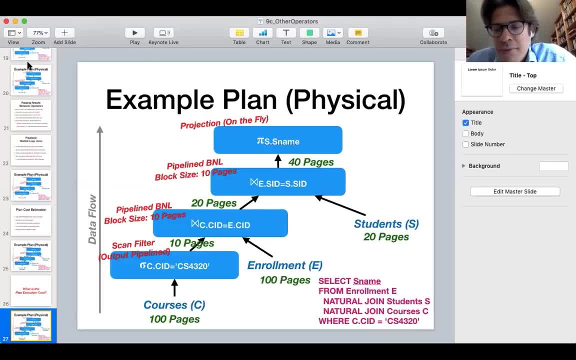 Thank you, Thank you, Okay, So let's see. all right, now we are running out of time, so i'm gonna give you the solution here. all right, so let's first of all start with the first operation, which is this filter, and here we have a simple filter. we don't use any indexes or anything, so here they're just scanning the. 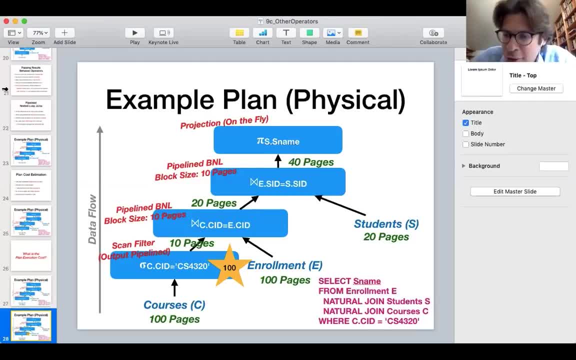 input pages one by one, and therefore the cost of this filter operation is simply the number of input pages which is given here, which is 100 now after the filter. you see that the amount of data reduces after the filter we have to join, and here photos join. the input buffer can contain: 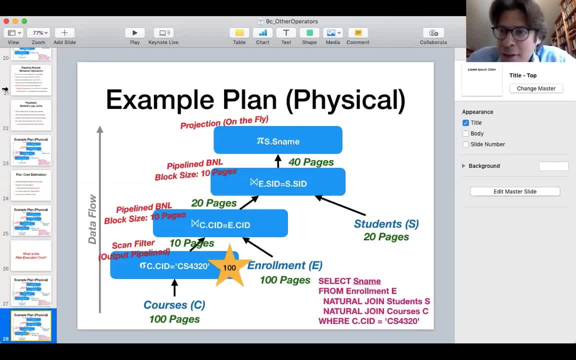 10 pages. so this is exactly the full filtered beside and for each block from the outer table. so whenever we fill the input buffer, we have to reach the pages of the inner table, which is the enrollment table one, simply due to the definition of how the block nested group join works. so since 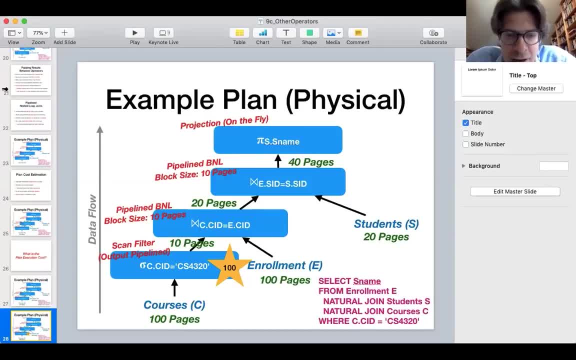 we fill the input buffer once. in total, it means that we have to reach the pages of the from the inner relation, from the inner table once, and that means that our cost is simply 100.. so typically, when starting a block, nested loop, join and having data on hard disk initially, then 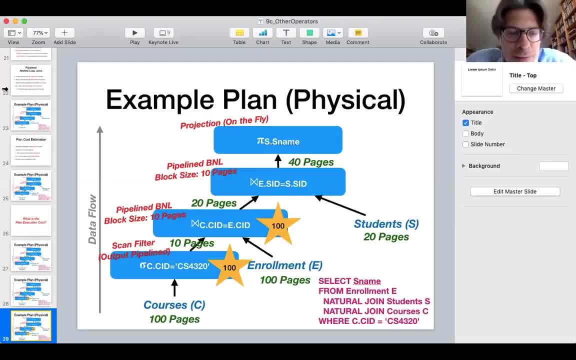 you'd also have to count the cost for reading the outer table. but here, in this case, the filter operation pipelines the reside into the join input buffer and therefore we don't need to read any data from hard disk for that, and this is why we don't need to add anything, we simply have the. 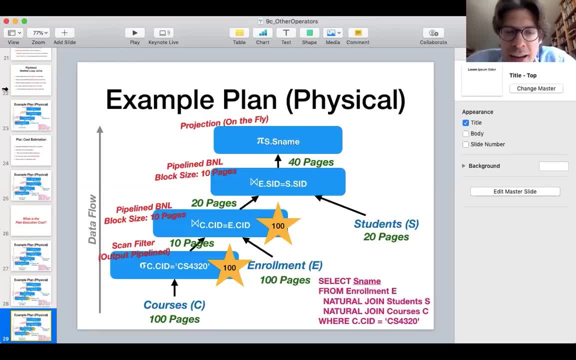 cost of reading the enrollment table once now. the next joint also has an input buffer size of 10 pages, but the total reside of the previous join because now it has more columns it is actually 20 pages and with 20 pages we can fill the input buffer to the following joint twice. 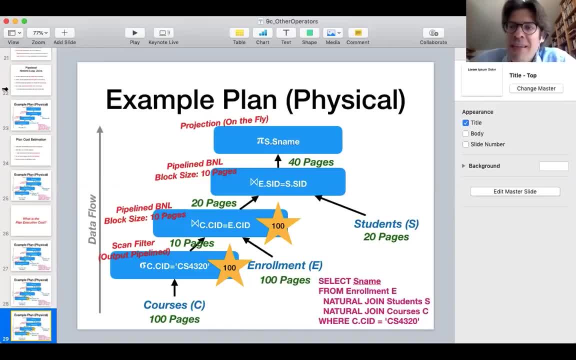 and that means we have to read the pages from the inner table twice as well. and here we have the students table with 20 pages. if you read that twice, it will give me a cost of two times 20 makes 40 pages. and now the question is: how much does the final projection operation cost? and in this, 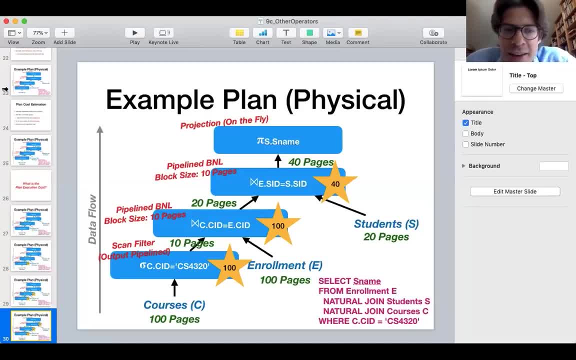 case uh, since we are immediately pipelining the output from the join into the projection, the projection is executed on the fly, it doesn't need to read any data and the output of the projection is the final query resides. we don't count the cost for the output either, and that? 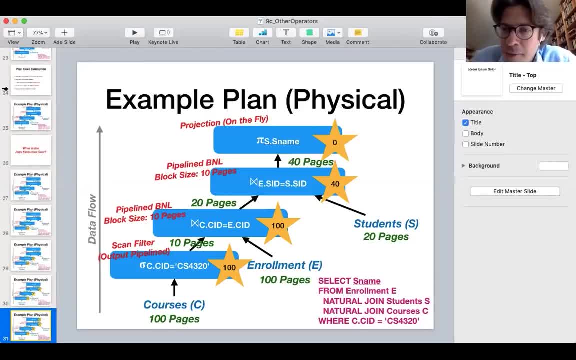 is why this projection operation has simply cost zero. in order to get to the cost for the entire plan, I'm simply summing up the cost for those different operations. if I sum that up here, then it gives me a cost of 240, and that is the cost of this. 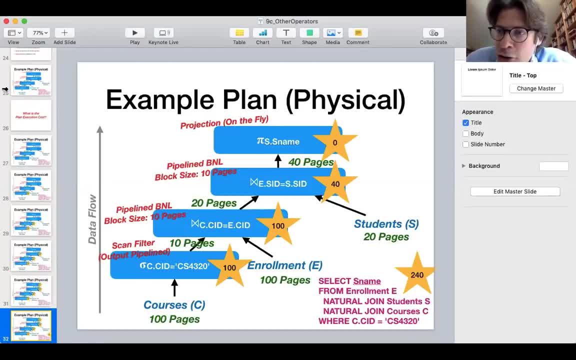 simple example- plan, so I encourage you to have another look at this example. we're going to make more example for plan cost estimation in the following. also tomorrow we will release the next homework, which will focus on indexing, so I also encourage you to have another look at indexing and 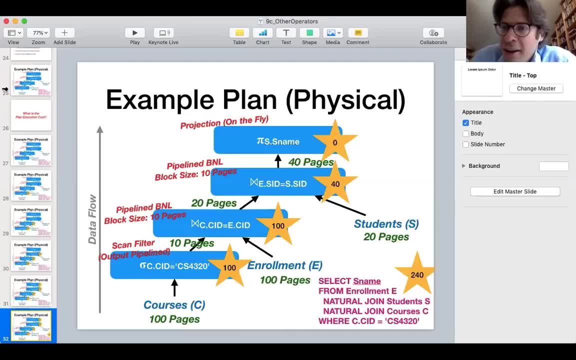 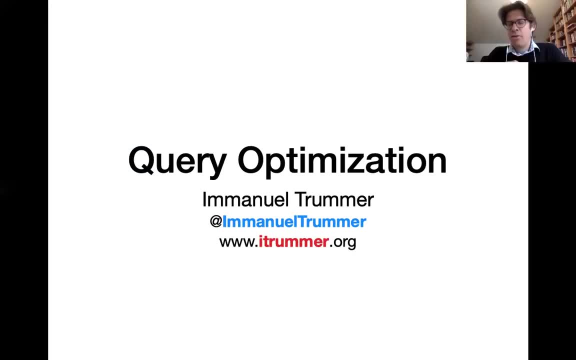 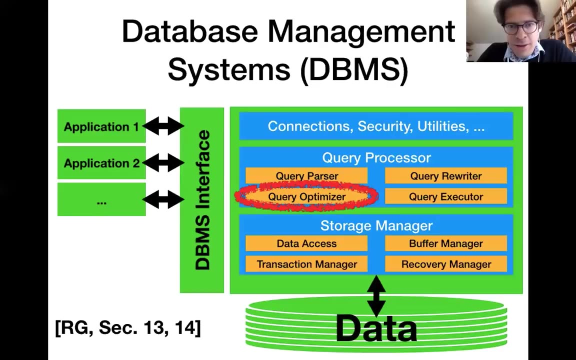 if you haven't done that already, and apart from that, I wish you a nice day and I see you again on Wednesday. all right, let's get started. um, please let me know if the slides work. so I'm now switching to the architecture slide and hopefully you see the overview picture with the query optimization. 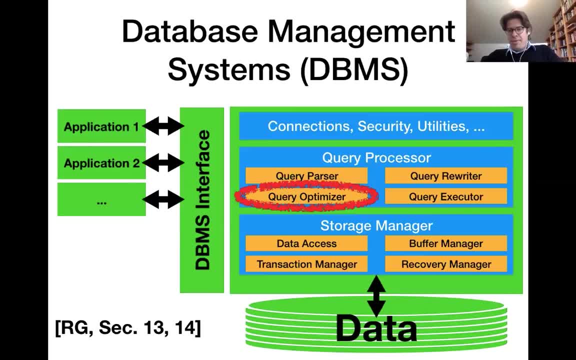 component and circles. all right, okay, seems to work good. so the last time we have been discussing about how we execute query plans and how we implement the different operators in those query plans. today we are going to discuss about how the database management system selects the optimal plan for an incoming query and the component in the database systems which does that. that is the 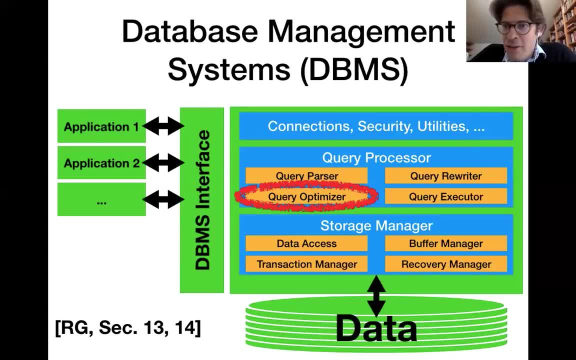 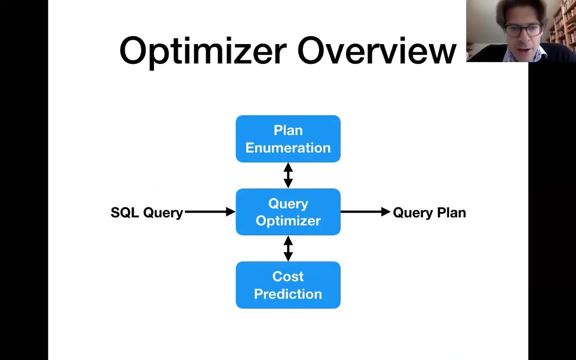 query optimizer, which you see here, and the relevant chapters in Ramakrishna and Gake. those are chapters 13 and 14.. so this is a high level overview of how one of those very optimizers works. so you have an SQL query incoming which describes the data that the user wants to generate, and then the query optimizer. 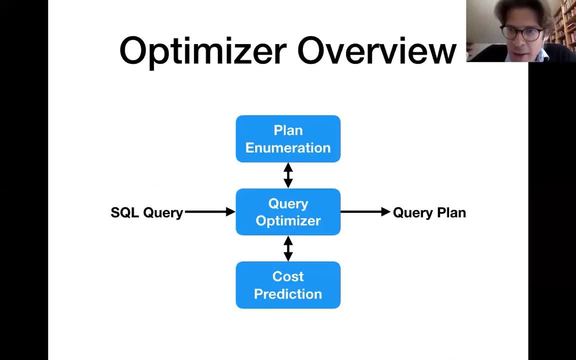 selects the optimal, the most efficient processing plan, which is then forwarded to the execution engine that we have been discussing over the past lectures. so the job of the query optimizer is to make all of those decisions like: in which order do we do that, which operator implementations do we use, and in order to do that it? first of all, 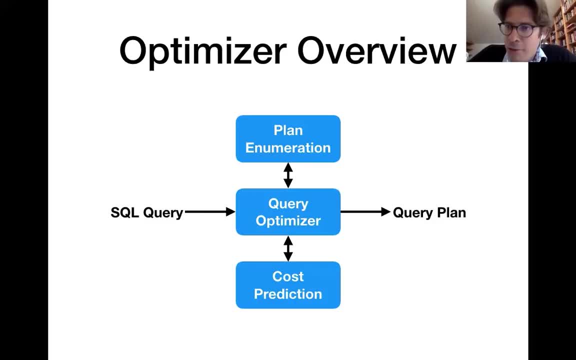 needs to be able to consider different candidate plans for a given query, so it has a component internally which allows it to enumerate candidate plans for the given query, and it also needs to be able to compare those candidates in order to select the best one. and in order to do that, it has a cost model in order to 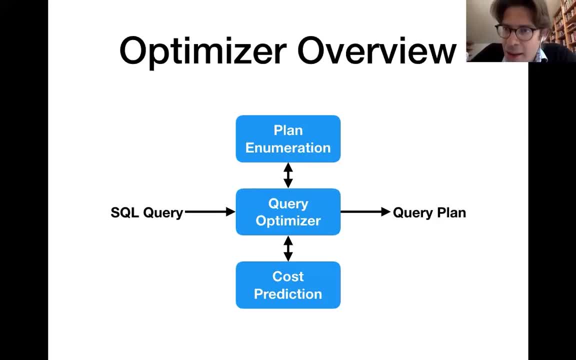 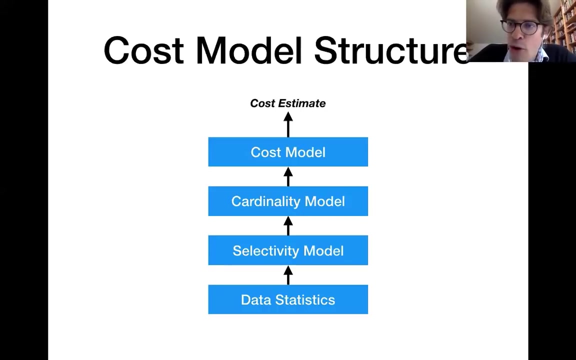 predict the execution cost for one of those plan candidates and then it tries to select the one where the expected execution, the predicted execution cost, is minimal. that is the high-level overview of the query optimizer, and in the following we're going to first of all discuss about how the cost estimation works. now, this is the high-level overview of how 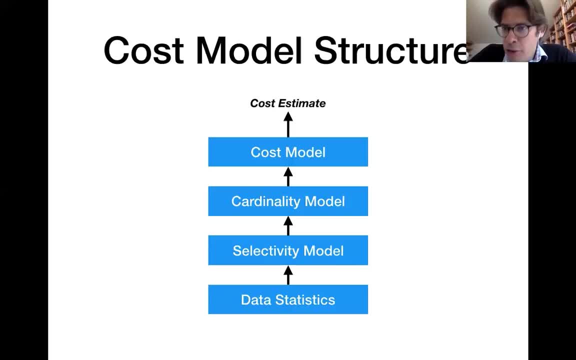 cost estimation works. so, first of all, cost estimation is typically based on data statistics. so the database system will store statistics like: what is the number of distinct values in a column, what is the range of values? and those statistics are necessary in order to estimate the credit plan execution costs. now those data statistics. they are first of all. 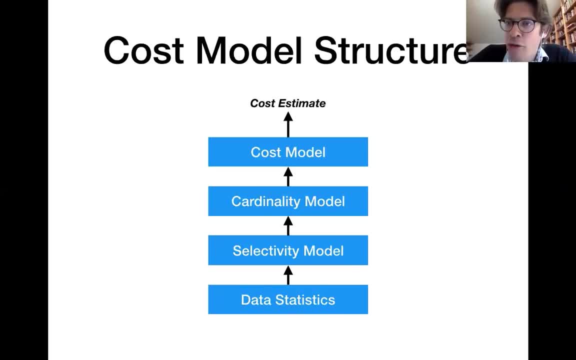 used to estimate the selectivity of predicates that appear in the query, and then they are used to estimate the activity of predicates that appear in the query. now those predicates, which filter rows. they essentially get assigned to a probability that they are satisfied for a randomly selected row. so we basically 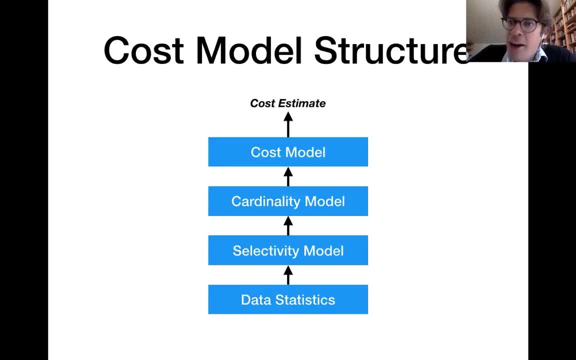 want to know how restrictive are the predicates that appear in the query and, based on that, we try to estimate the sizes of all intermediate results that get generated when executing a certain plan because, for instance, depending on the order in which you join different tables, you might end up 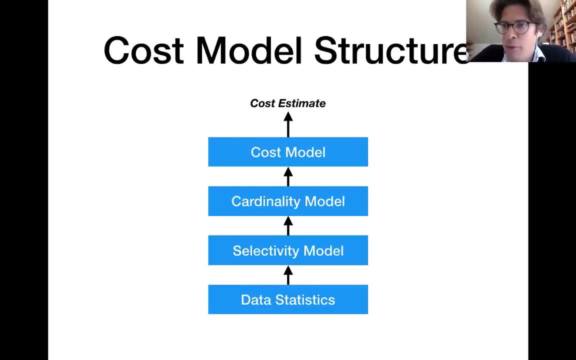 generating different intermediate results, and some of them can be quite large so they're expensive to process. you want to avoid that, while others are fairly small, which is better, and with the cardinality model we try to distinguish between those cases. finally, given the size estimates for all relevant intermediate results, we are trying to 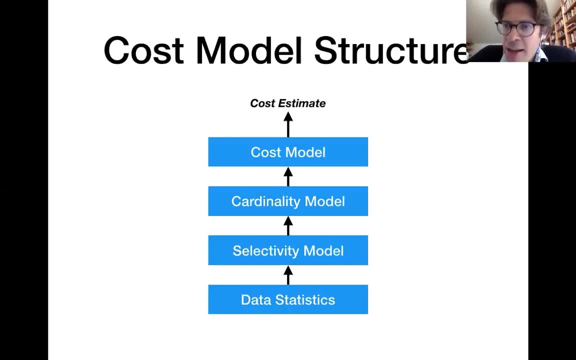 predict the cost of the plan, and we do this in a similar way to what we have already seen so far. we have seen a simple cost model to estimate the cost of single operators, and last time you also have seen how we can estimate the cost of an entire query plan with multiple operations, and the query optimizer uses a slightly large number of containers. 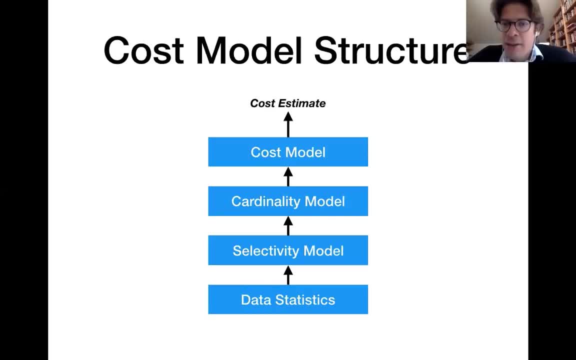 The query operator uses a slightly larger number of containers, more sophisticated version of that, And that is used in order to assign a candidate plan to an estimated execution cost. So let's discuss in a little bit more detail about those different steps of cost estimation, starting with the data statistics. Now, which statistic precisely we are? 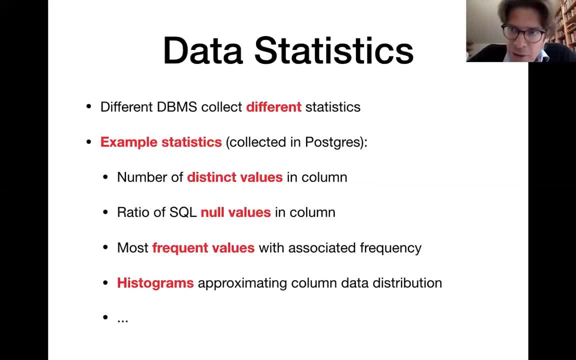 using. that depends on the database management system. Different systems store different statistics. For instance, in Postgres we have statistics for each column, such as the number of distinct values, the number of null values. Often database management systems store the most frequent values for each column, the heavy hitters, so to speak, And they often use histograms. 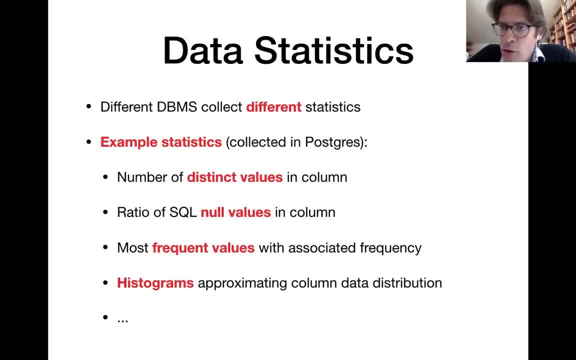 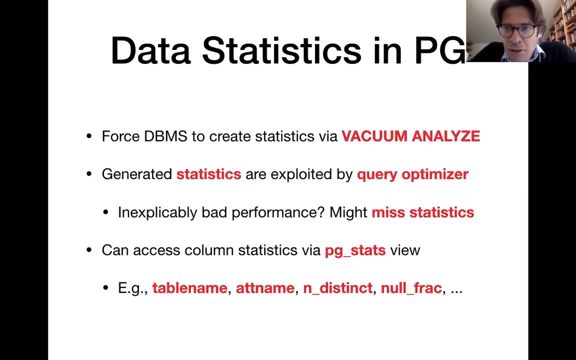 in order to get some coarse-grained impression of the distribution of your data And that is used in order to estimate predicate selectivity, For instance in Postgres. more specifically, those statistics, you force the database management system to create them by running the vacuum analyze command. Sometimes the database system might also decide itself. 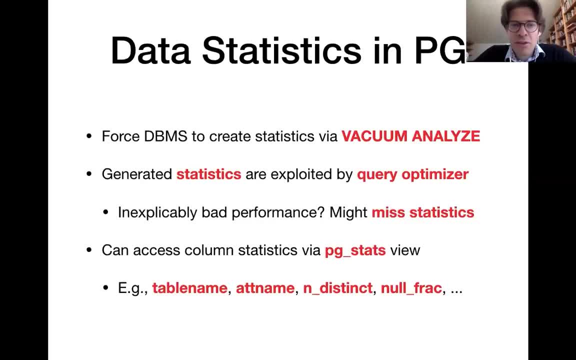 to create those statistics, but you can force that with this command And those statistics are used to form the base for query optimization. So one hint from the practice. if you observe that you have strangely bad performance in query processing, then every once in a while the problem. 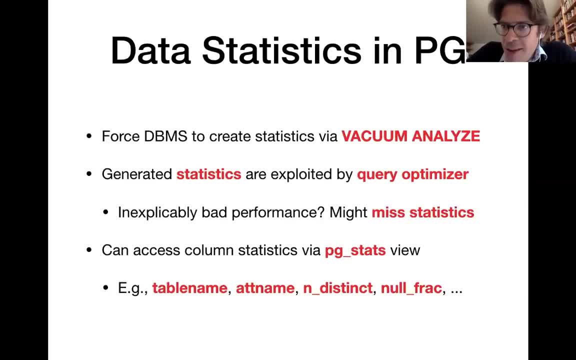 will be solved if you just run vacuum analyze, because the problem is that the query optimizer doesn't have accurate statistics and so doesn't choose good query plans. So that is good practice. to run this command, You can also directly inspect the statistics that are created by the Postgres optimizer. There's the so-called 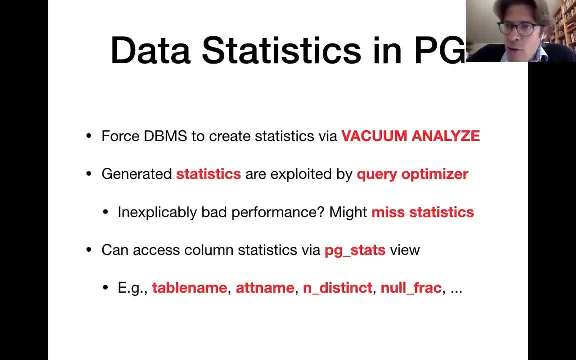 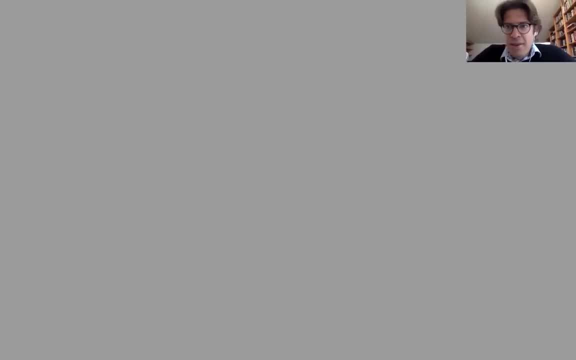 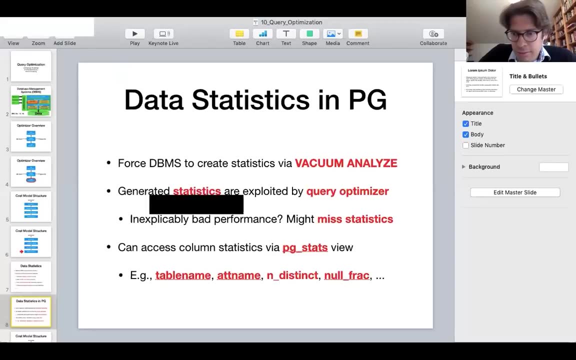 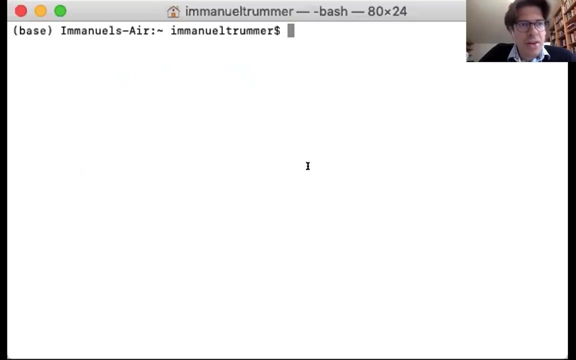 PG stats view, which contains all that information, And I'm very quickly going to demonstrate how you can access that. I'm quickly going to switch to sharing my terminal, So let's see what I can do. Okay, So let me just go right to the database. 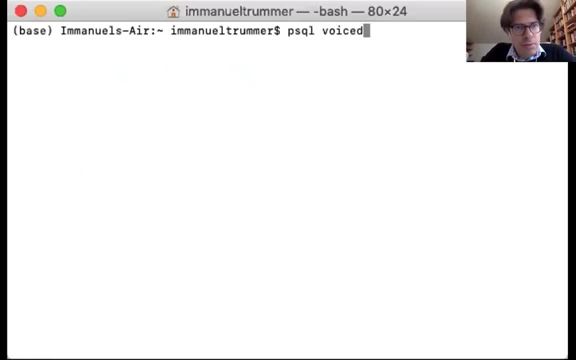 All right, You should now be able to see my terminal window In the database- and I'm going to use this one here- And once we're all in the database, you can see that it is a very normal parameter. So, it's a very normal parameter. 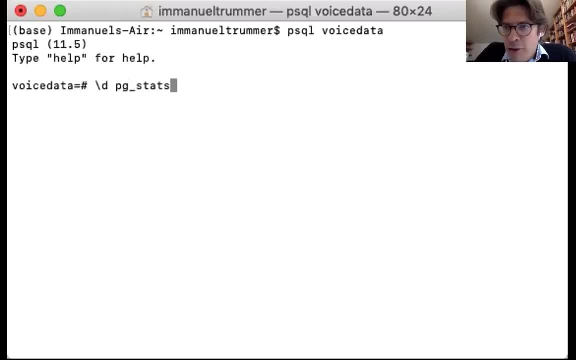 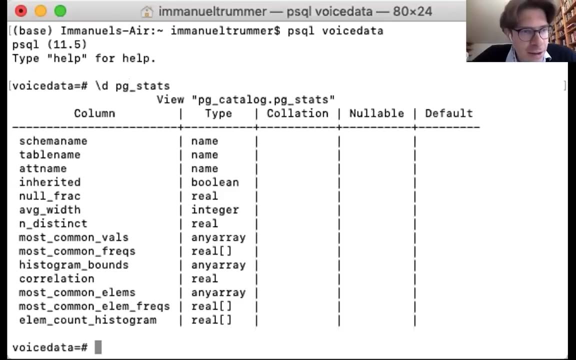 the data structure, the relation containing those statistics, that is, the PG stats data structure. here you see the different columns. I'm not going to discuss all of them in detail, but you see, for instance, they call them null track, which would indicate the ratio of a null value in a given column. all right, 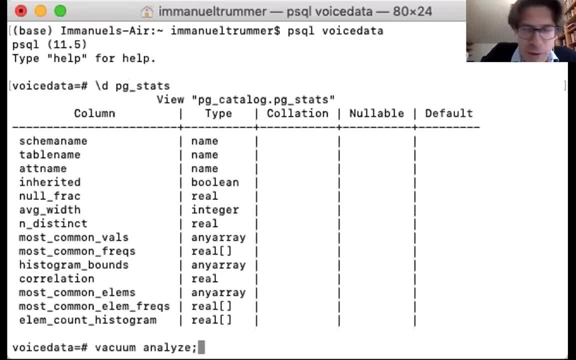 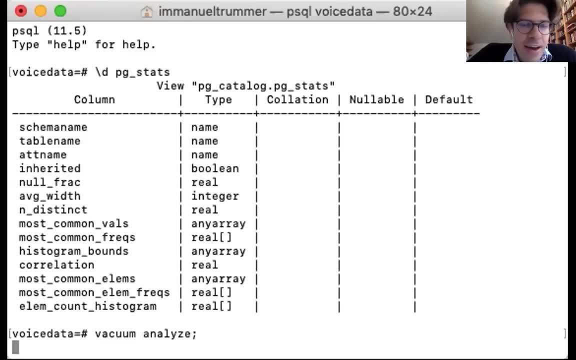 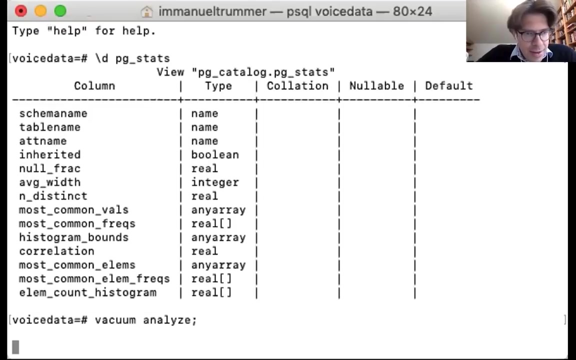 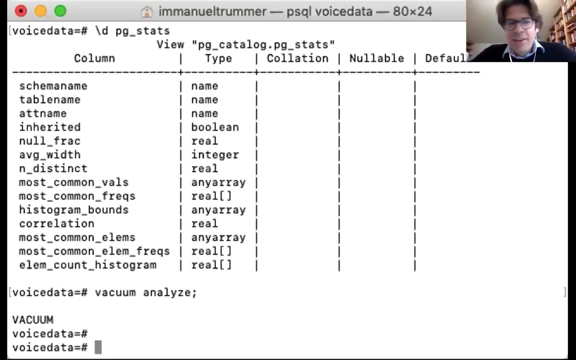 and just to be sure, we are running the vacuum analyze command. in the last couple of times, we have already been using the table containing the results of the stack overflow developer survey, so let's quickly examine the statistics. once this command here finishes, I'm actually sure that the statistics are up-to-date. okay, finished, all right. 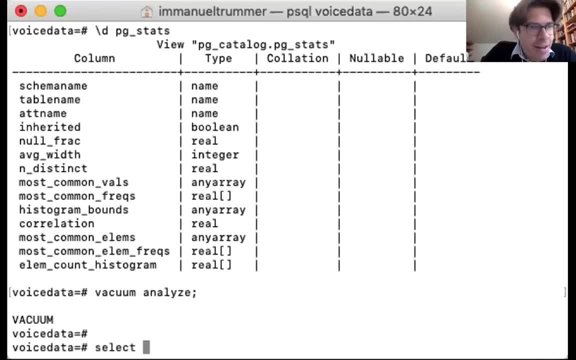 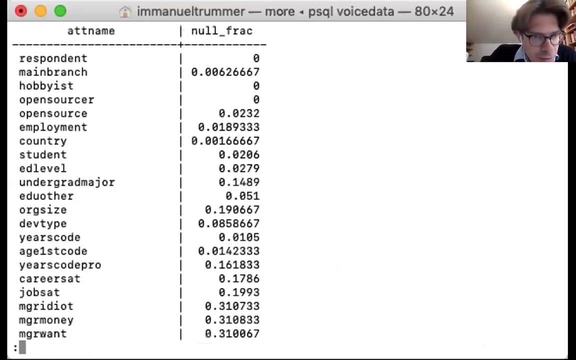 and now let's, for instance, say that we want to analyze, for each attribute, for each column, the fraction of a null values, and the table that we interested in, that is the stack overflow 2019 table. all right, and as you see here, now we see there are statistics about how, which. 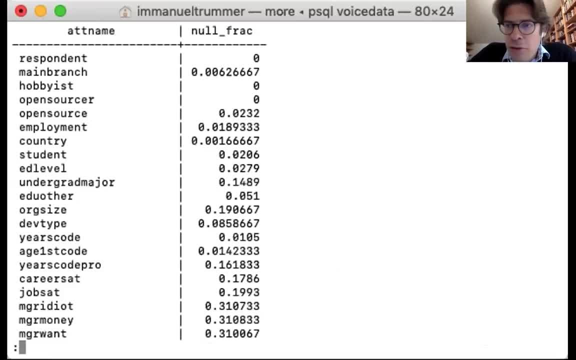 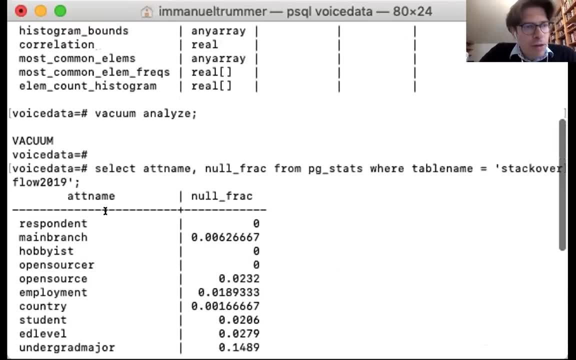 percentage of the rows contain null values for the corresponding row. all right here, of course, the respondent column, for instance, that one is the ID column. so here we do not have any null values because that is a primary key, that is, this allowed it for some of the other columns. we actually have a. 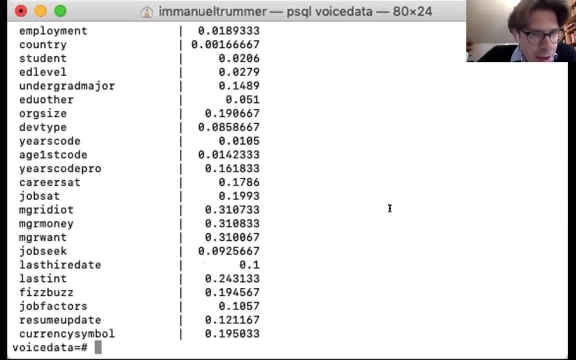 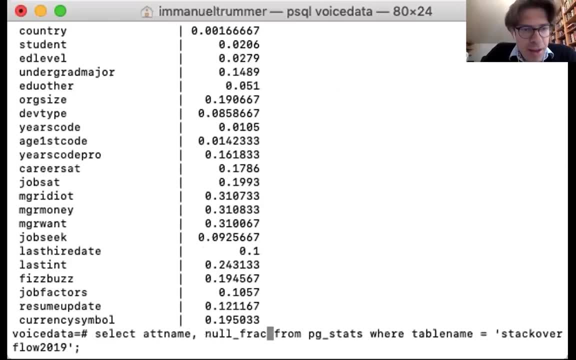 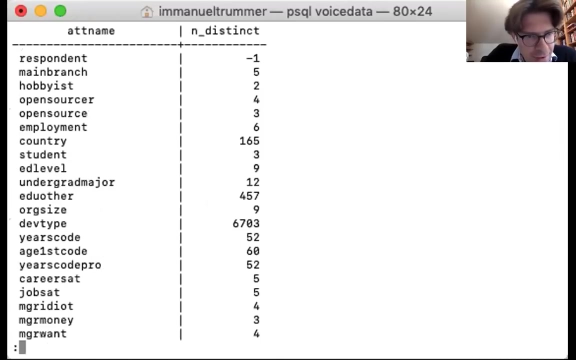 relatively high percentage of null values, values um, and here you see the estimated percentage. that's baby. we've got one more statistic two, all right, so here we have the number of distinct values. uh, some of them are positive. if it is positive, it is directly the number of distinct values. some of those values here are also: 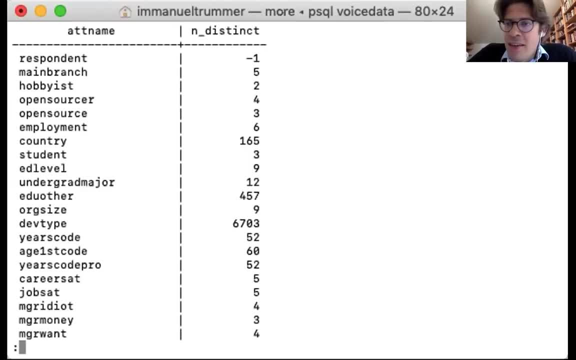 negative, and that means that we are essentially talking about the percentage. so if the number is negative, then basically that is the number of distinct values divided by the number of rows. so um. here, for instance, in the very first attribute, the respondent attribute, that is the primary key. so here we have um, a distinct value, um ratio of 100. so that means that every 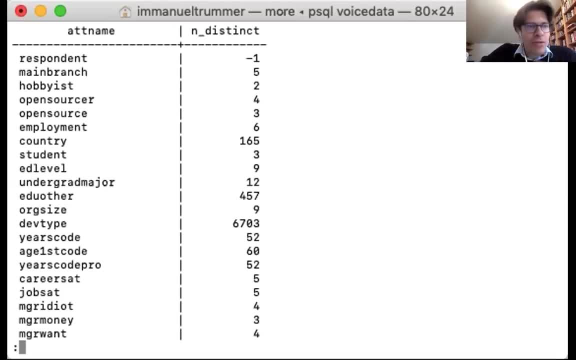 row contains a distinct value by. for some of the other columns we have a relatively low number of distinct values and there's many more statistics contained in this piggy stats um view. so if you're interested, i encourage you to explore that further. but just to give. 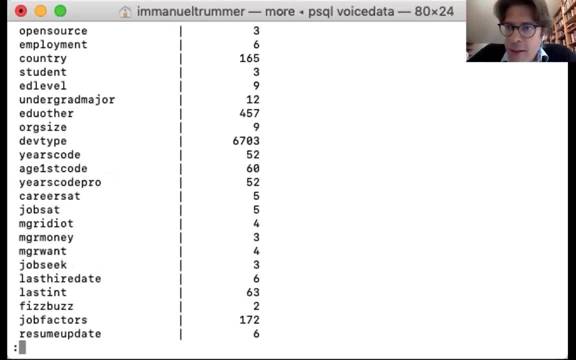 you a little bit of an expression for the types of statistics that, uh, an optimizer stores. and here we have the question in the chat about whether minus one means 100, a unique, and yes, exactly yes, and that's already answered. great, so that is exactly the case. so 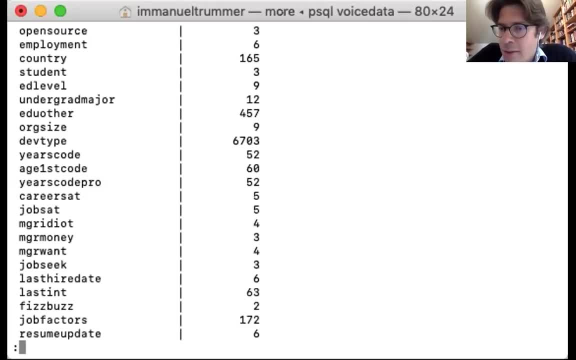 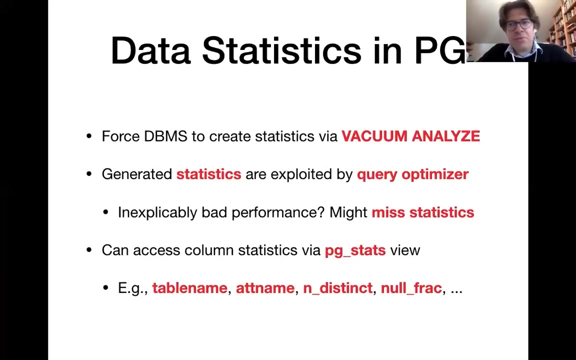 minus one means 100 distinct values. all right, good. and those statistics are used by the optimizer in order to decide which query plans to use. let me get back to my slide deck. all right, so those statistics are used by the optimizer in order to decide which query plans to use. let me get back to my slide deck. 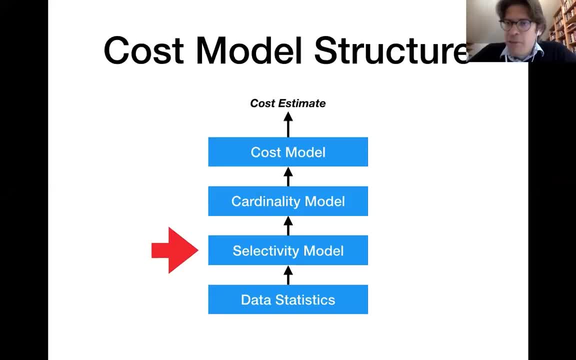 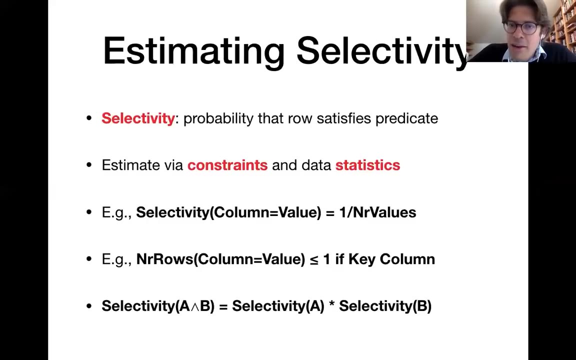 from the input to the selectivity model, where we estimate, for each predicate in the query, the probability that it is satisfied for a random row. now, generally, the selectivity is defined as the probability that the random row satisfies a predicate. in order to do that, we can generally use 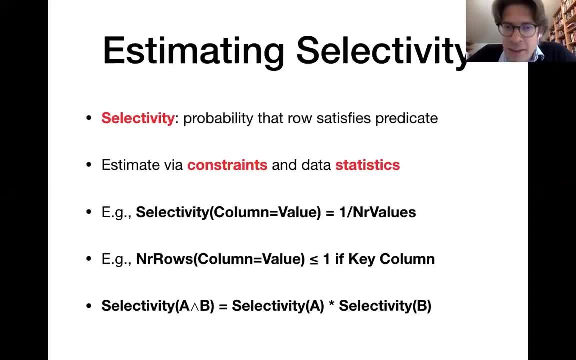 constraints on my database and those data statistics. now we have already discussed about the data statistics constraints. we have also discussed, but already a couple of lectures ago. those are things like knowing that a certain column contains a primary, like a certain column forms the primary key, or that there's a foreign key constraint between other columns, for instance. 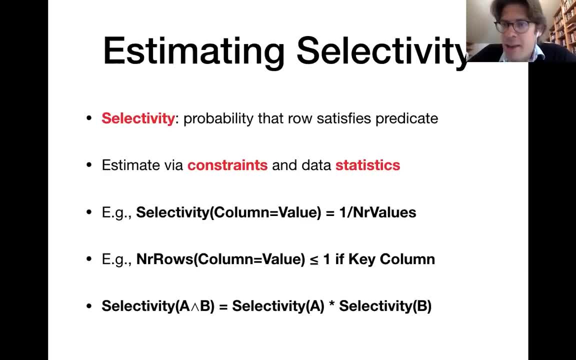 if you know that a certain column is the primary key, then automatically you can infer that it will contain unique values, and the query optimizer makes this kind of reasoning. now, for instance, we could say that if we know how many distinct values we have in a certain column, 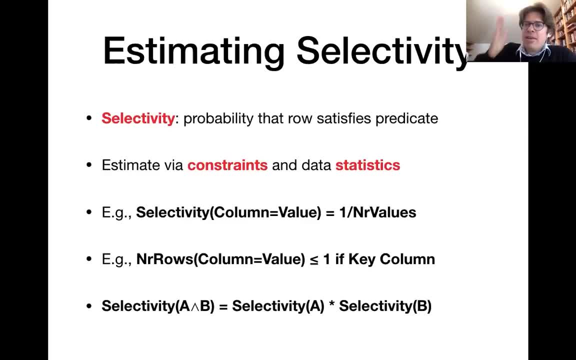 and then we have a predicate of the form: a column equals value. then under certain assumptions, we can say that the selectivity of the predicate is expected to be one divided by the number of values. or, for instance, if we know that we are talking about a primary key column, then 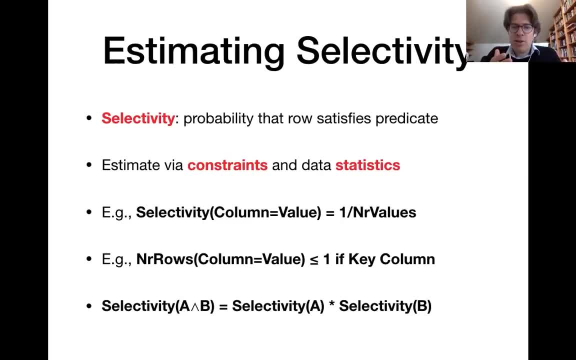 we know that if i fix the value in that column to one specific value, the result must contain at most one single rule, and in practice i often have composite predicates. so here for instance, if i calculate the selectivity of a conjunction between two predicates, a and b, then on a certain 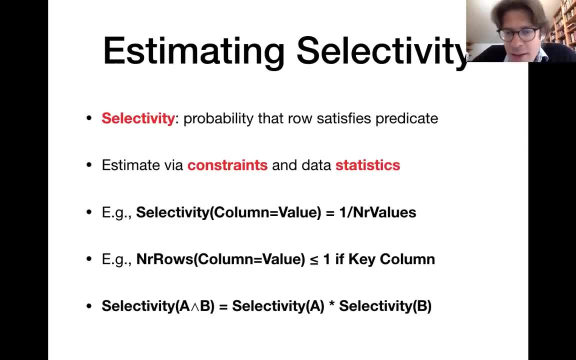 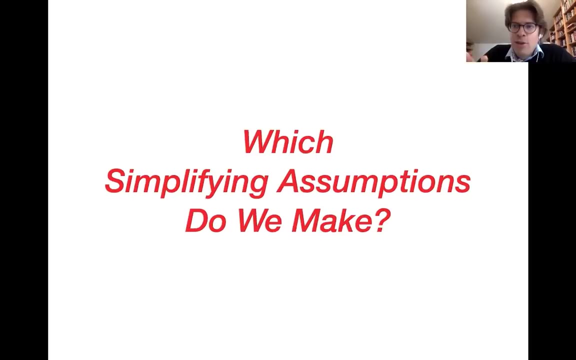 assumptions. i can say the selectivity of a and b equals the selectivity of a times the selectivity of b. so i can decompose the selectivity estimation for the composite predicate to into selectivity estimation for the component. now i have already mentioned assumptions a couple of times, so can anyone tell me in the chat? 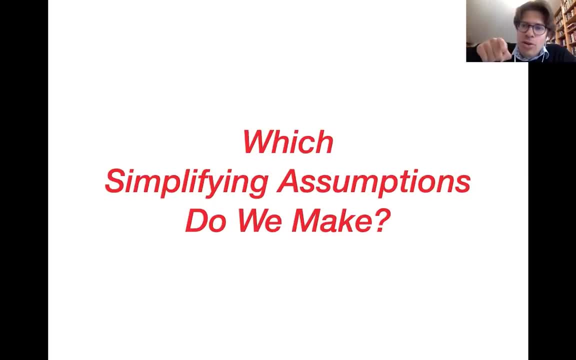 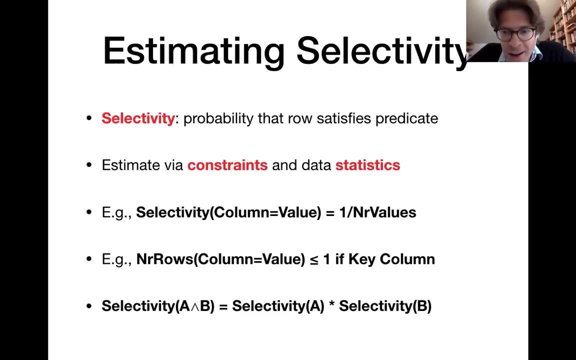 which assumptions we seem to be making in order to come to those formulas here. independence, very good, here we have independence in the chat, and that is indeed the assumption that we are making for the last, for the last formula. here we assume that those two predicates a and b 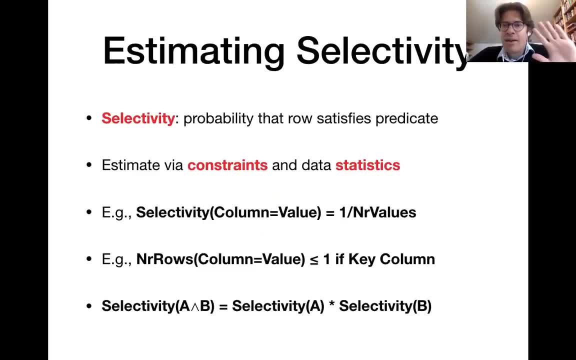 are independent, and this is why the selectivity of the composite predicate is the product of the two predicate, the selectivities. does anyone have a different assumptions here? okay, very good, and here is: the values are equally distributed. very good, and that is indeed the assumption that we are making in order to get to the first formula. we assume that whenever i fix 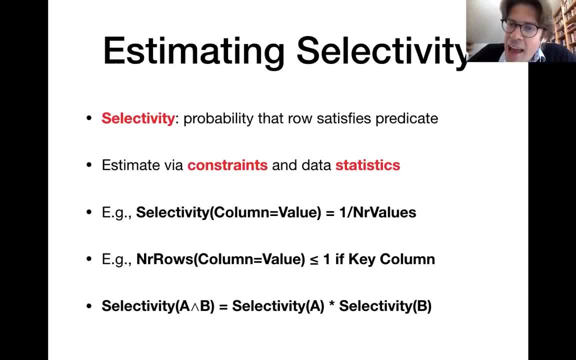 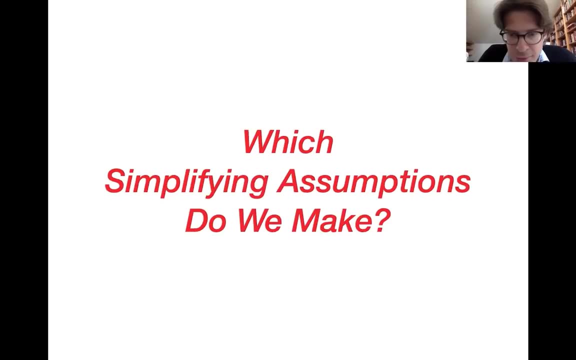 the column to any specific value, then we have the same selectivity. so implicitly i'm assuming that all of those values are equally frequent. so i assume that data is uniformly distributed across different values in that column. now here there's the summary, and indeed those were the two. 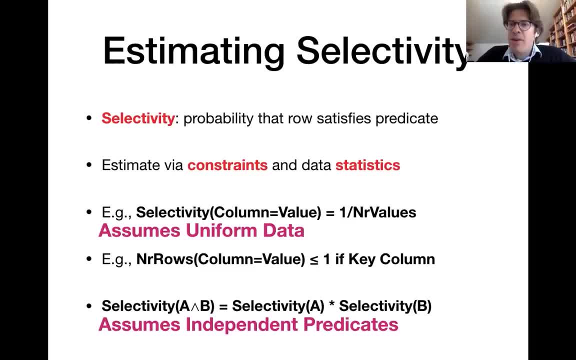 assumptions that i was aiming for now. by the way, for the case with the constraint, if you know that a certain column is a key column, then uh, in order to get to this, uh inequality here, we don't need to make any further assumptions. so that definitely holds. but for the other selectivity estimation formulas, we 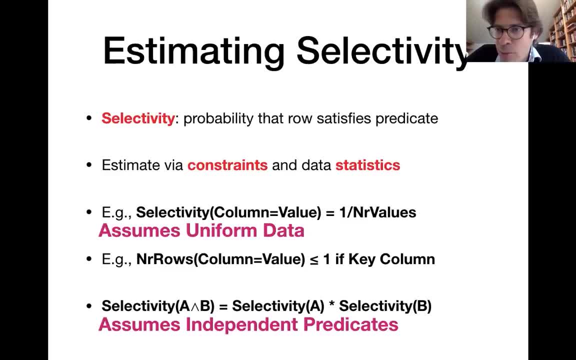 made indeed, a couple of strong assumptions and in practice, those assumptions, of course, they don't always hold, and that is also one of the main reasons why query optimization can go wrong. some of those assumptions are not satisfied. nevertheless, in many cases those assumptions are not too far from. 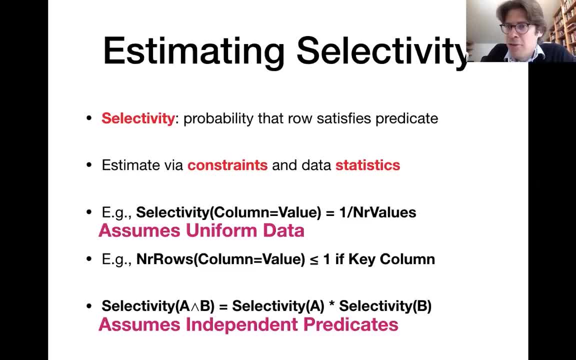 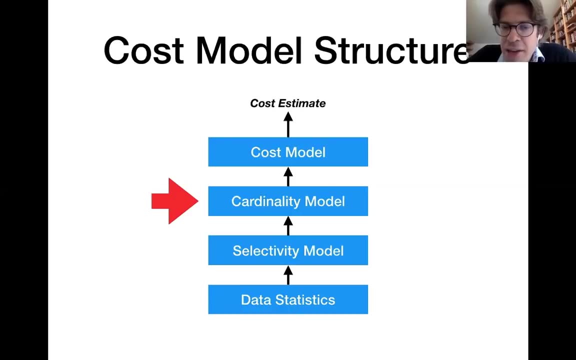 the truth. so this is why those assumptions are used in practice. for instance, the postgres optimizer will at least make the independence assumption typically and thereby assign each of the predicates to a selectivity estimate. now the next step is to use those selectivity estimates in order to estimate the cardinality. 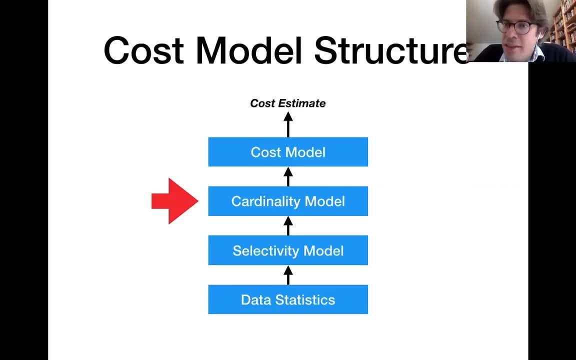 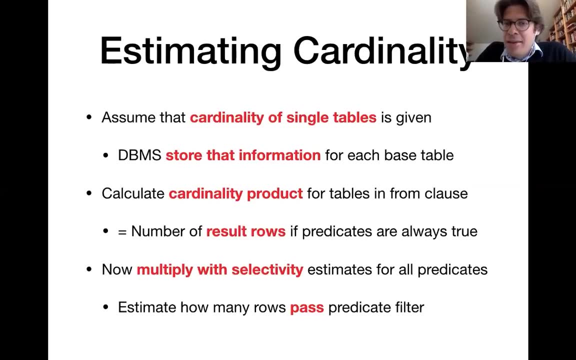 meaning the number of rows in certain intermediate resides, all right. so we generally assume that the cardinality of a single tables is given because that is information that a database management system needs to store anyway. so we have the number of rows in each of the base tables and if i want to, 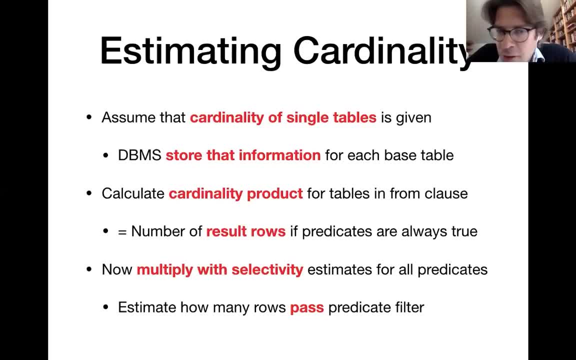 calculate the cardinality estimate for a certain intermediate result, then first of all i can consider all the tables which are involved in that reside. if the reside is expressed as a query, then it would be all the tables that appear in that queries from clause. so i'm taking all those tables in a front clause and then i form the product of their 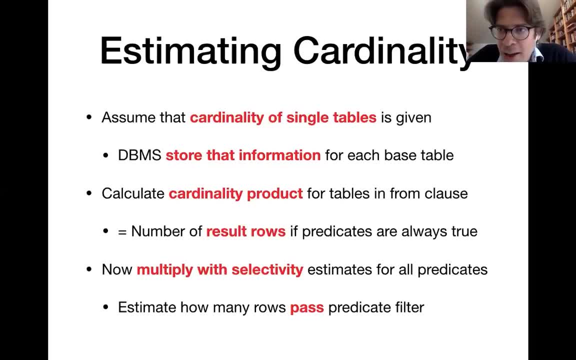 cardinality values. so that reside basically is the result of the table at the front of the table, and that would be the cardinality if all the predicates involved had the selectivity of 1, meaning that they are always satisfied. So that is of course by 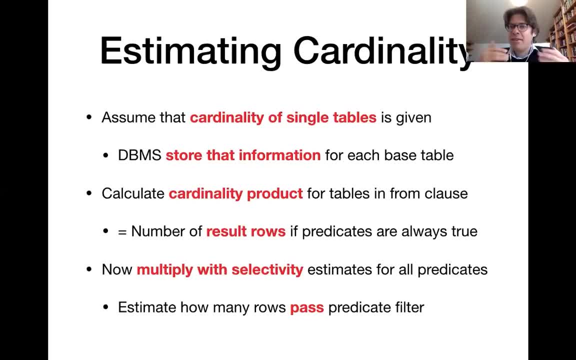 far an overestimation. So we need to take into account the more realistic estimate of the predicate selectivity. So after we have multiplied all the table cardinality values, then we multiply that with all the predicate selectivity values of all involved predicates and to then all the cardinality values times all the. 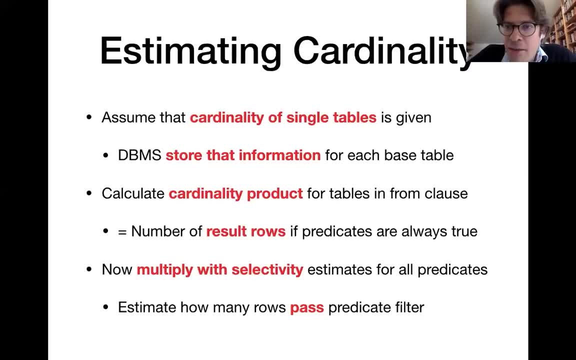 selectivity values. that gives me a rough estimate for the size of one of those results. Ok, and that's interesting. There's a question about the seminar yesterday which focused on approximate processing. That's actually an interesting connection there, because indeed in approximate, 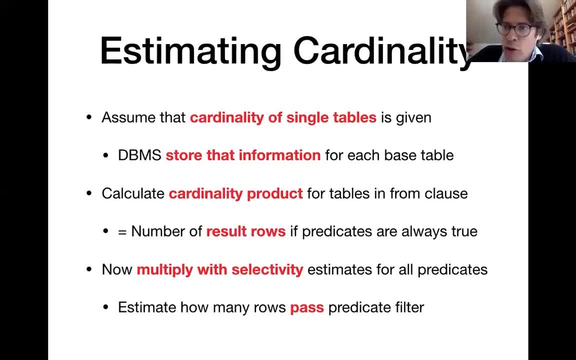 Zoe Proизστice processing. we work with some coarse-grained data statistics. There, the goal is to produce an approximate query result, But it is true that we use somewhat similar data structures in order to get some approximation for the sizes of intermediate results. 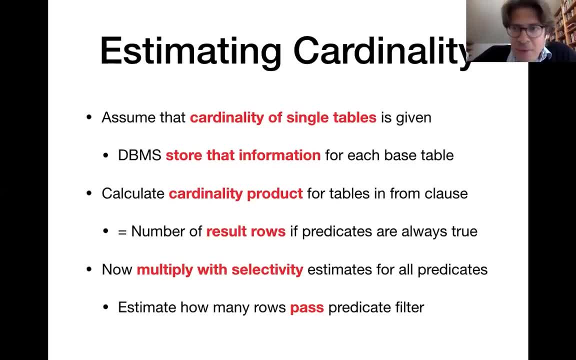 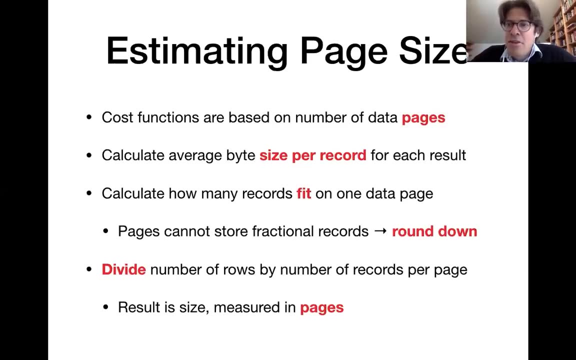 So there is some connection between those two. OK, All right. So now we have estimated the sizes of intermediate results in terms of the number of rows. Now we still need to estimate the size in terms of the number of pages Because, for instance, in our simplifying cost model, 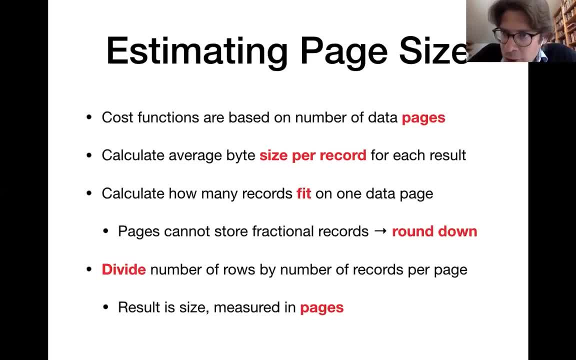 we have calculated the cost of an operation by looking at the number of pages that it needs to read and write from hard disk And also those optimizers like the one from the Postgres database system. they also calculate cost based on the number of pages. 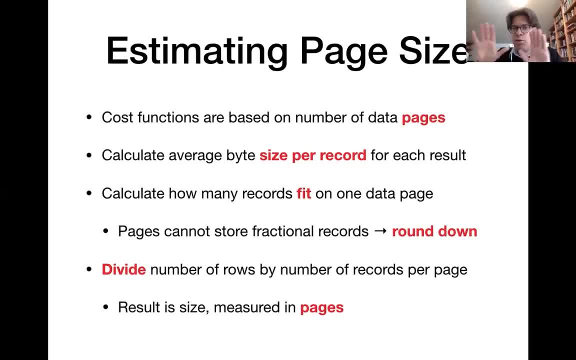 All right. So in order to get from the cardinality to the number of pages, we first of all need to reason about how many rows fit on each of those pages. Afterwards, it becomes relatively natural to calculate the number of pages In order to estimate how many entries I can have. how many? 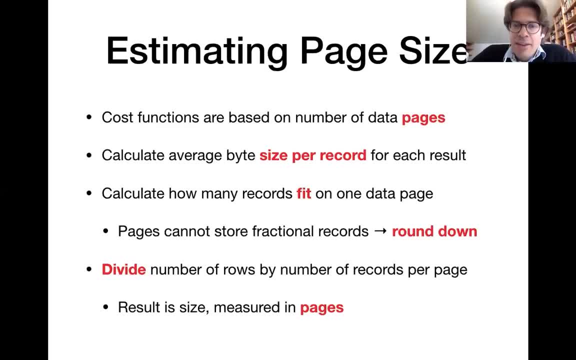 rows I can have on each of the pages. I essentially think about the number of bytes required for each record, And then I pretty much just divide the space on the page by that rounding down if necessary, because pages cannot store a fractional tuples. 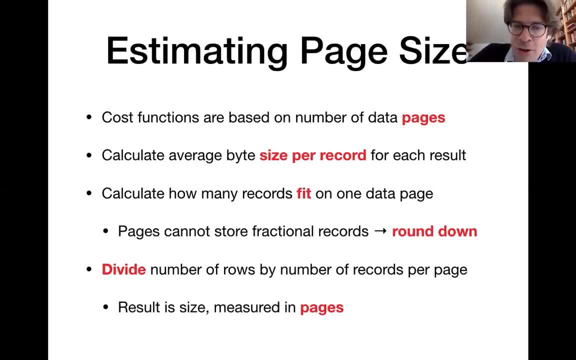 That is a question that I'm often getting here. So yes, So one page can only store entire tuples, All right, And after that I can use the number of rows estimated before and combined with the number of rows per page, And then I get the page estimates. 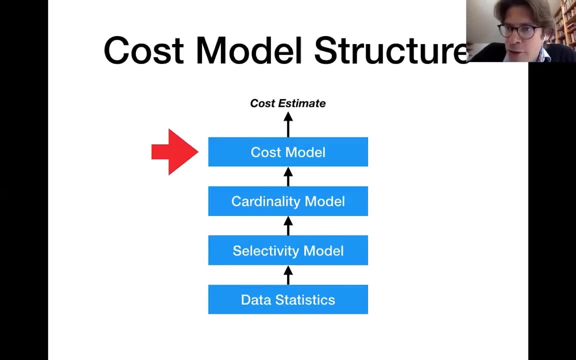 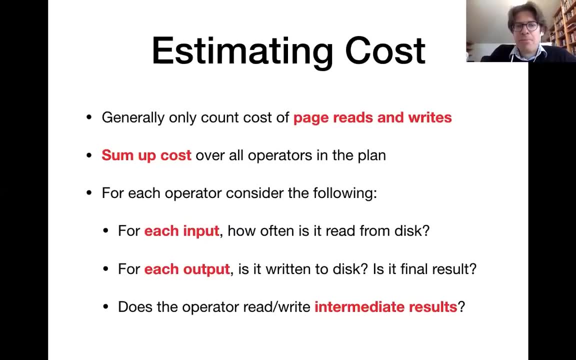 All right. Finally, now I have all the information that I need in order to estimate the cost of different operations in my query plan. Now, here we have this very simple model where we only count the number of reads and writes for this course. 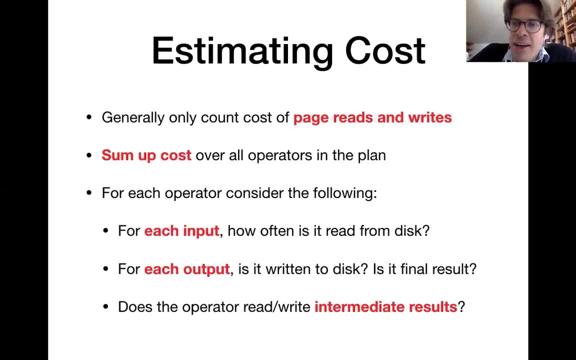 So the Postgres optimizer, for instance, would additionally consider some functions of the computation cost, But nevertheless it would also consider the number of page reads and writes, And often that is in practice a significant, if not the most significant, cost component. 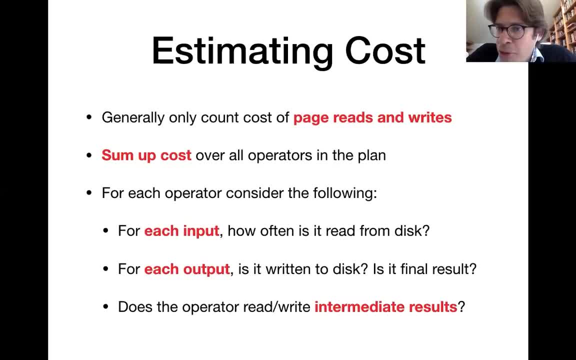 Now we essentially just sum up the cost of all operations in the query plan And for each of those operators. for each of those operations in the plan you need to consider first of all for each of the inputs: are those inputs read from hard disk? 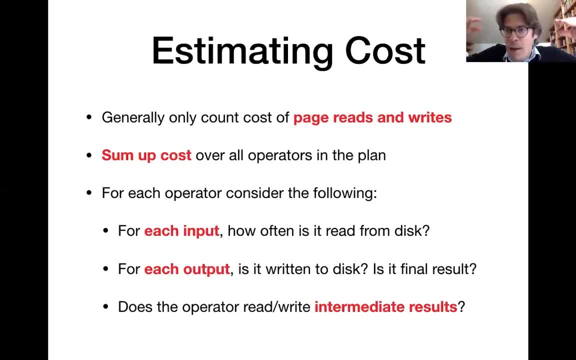 or are they already in memory once the operation starts? Because we have seen that operators can sometimes pass on the result of an operation to the next operator without ever writing it down. So we need to consider whether we are writing it to hard disk, And that makes things cheaper, of course. 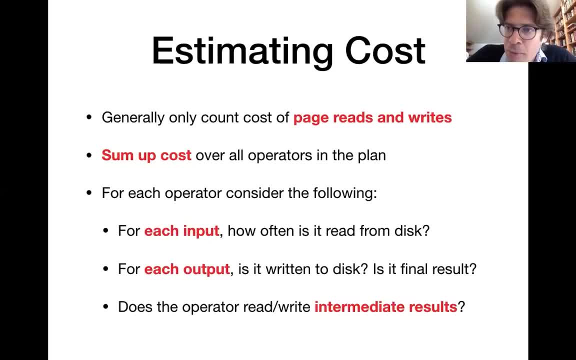 So, for each input to an operation, think about how often we need to read it from a hard disk, if at all, And for each output, we need to consider whether we write it to hard disk or not, except for the very final output of the query plan. 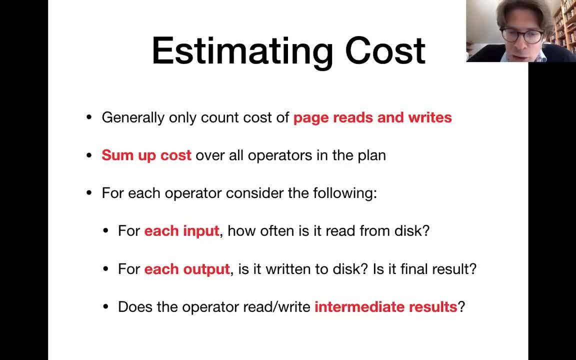 because that by convention we generally don't consider in our cost calculations. Looking at the input to the operation and at the output might not be sufficient because some of the operators that we have seen they might internally write intermediate results to hard disk. 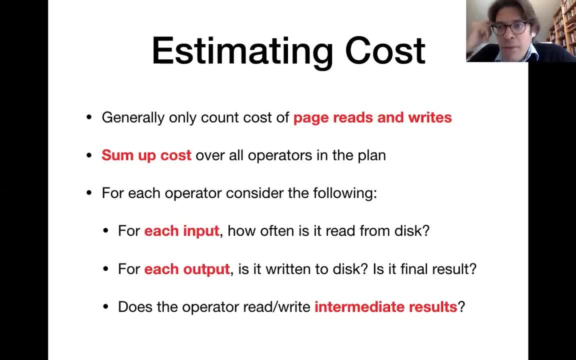 and read them again. If you, for instance, think about the sort operator it might make multiple passes over the data and write out intermediate results, And so looking just at the output of that operator and at the input of that operator might not be sufficient. 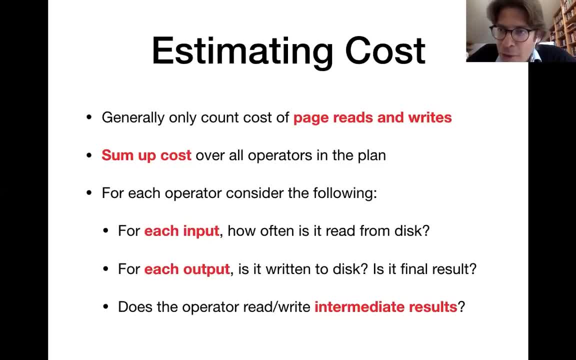 you also need to think about how often it internally writes data to disk and reads data from hard disk. All right, And in the end you sum all the, basically the cost of all data movements. You sum them up in order to get to a total cost. 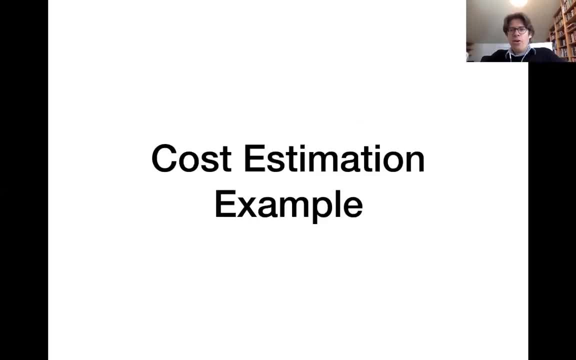 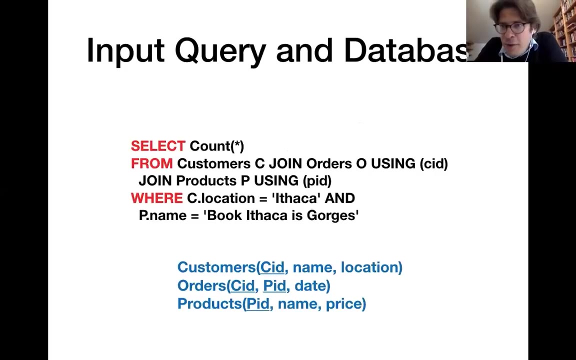 for the entire query plan, All right. Now in the following I'm going to make a little example for a cost estimation, just that. we have seen the entire process from start to finish. a little bit All right. So this example will focus on the query that you see here. 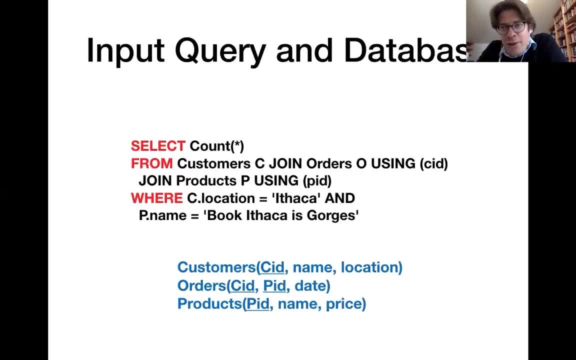 Let's say we have a little online shop, a bookseller, for instance, And we want to know how many customers in Ithaca have ordered a book called Ithaca is Gorgeous, All right. So we want to count those customers and orders. 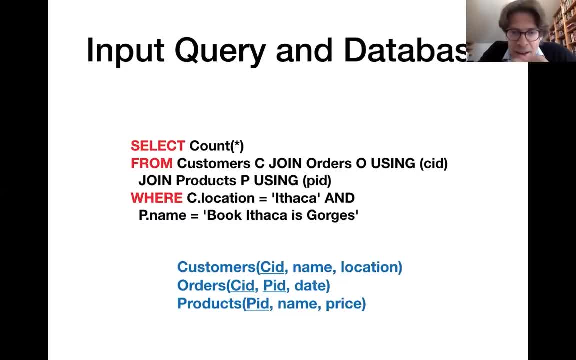 And in order to do that, we have this query here. Here it operates on the database that you see below, on the lower half of the slide, We have a customers table with the customer ID. That is the key, And it has a name and location for the customer. 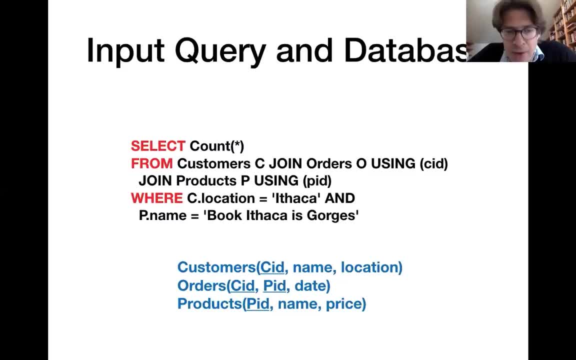 So we want to restrict that location to Ithaca in the query. Then we have the orders which connect the customer's CID to products- PIDs and with a specific date when the product is ordered, And All right. Finally, I have the products with the product ID which: 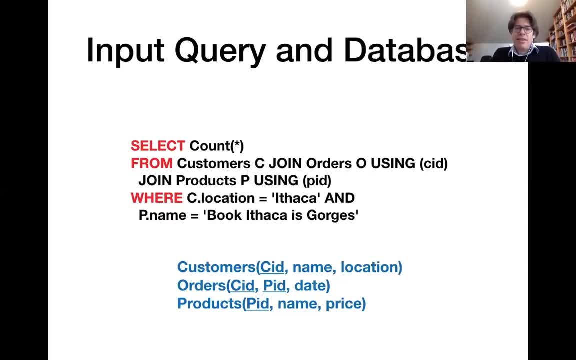 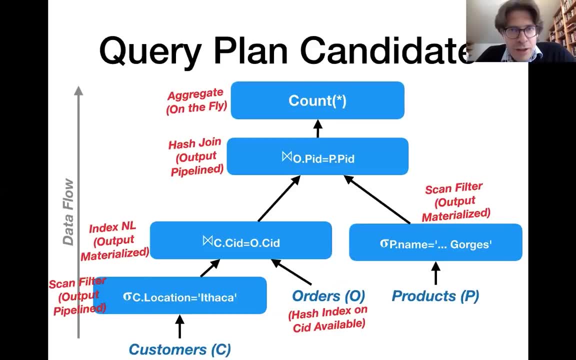 is key: the name and the price for the product. All right. So the first step here is that I need some kind of candidate plan for which I'm doing this estimation. So in the following we're going to analyze the candidate plan. 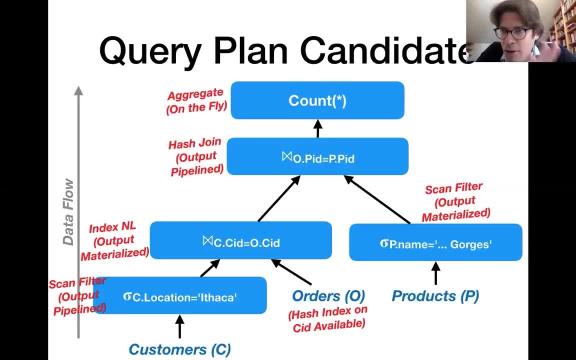 that you see here. So the data always flows from the bottom Here. we wants you to ask these questions, And then, then hab, we're going to solve the platform here, And at this point we just need to add these up. 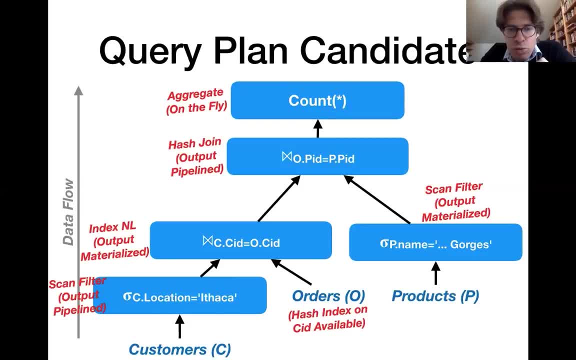 Let's say 10.. This is the capital set. Let's add an item to the system platform here. So we have to enter our global data nested loop join. So this index nested loop join here joins with the orders table and in order to 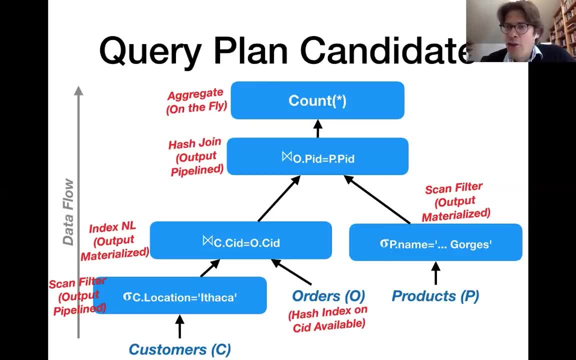 do that it uses a hash index on the custom ID attribute of the orders table. Now the result forms one of the two inputs of the next join. The other input is the filtered products relation, where I am filtering two products with a certain name and the result of that and the former result. 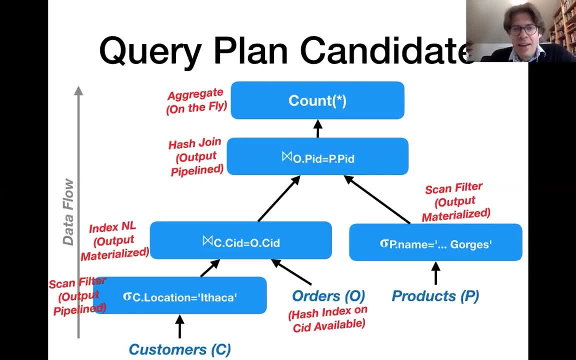 forms the input to a hash join and this hash join pipelines the output to account operator, which is executed on the fly, meaning that it doesn't need to read its input from hard disk, it just gets its input directly in memory. and the final join, by the way, joins 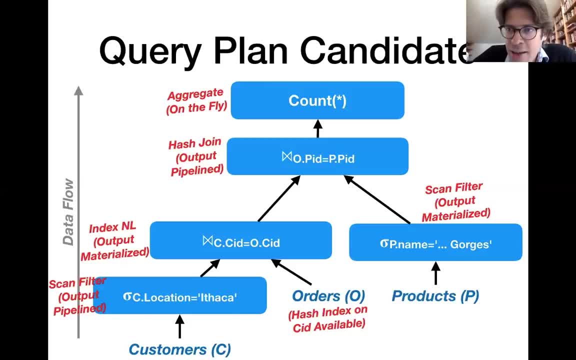 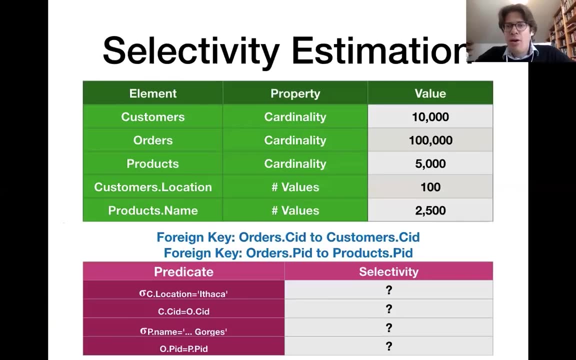 on the like product ID column. so we want to find matching entries with the same product ID. That is the Ferris Plan that you will go over in the following. Now the first step is to estimate the selectivity of a predicate. Now, here on the upper half of the screen, we have some information. 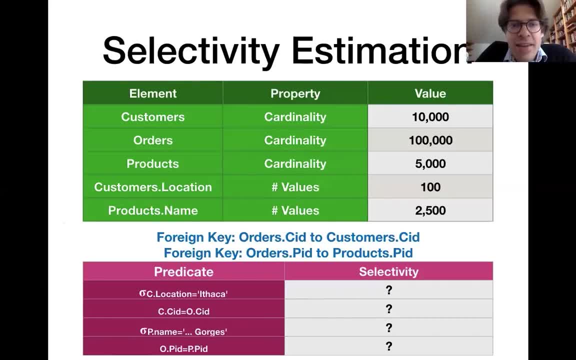 about the product ID column and we want to find matching entries with the same product ID column. So we want to find matching entries with the same product ID column. So we want to find matching entries about the data, some data statistics. You have the number of rows in the different tables. 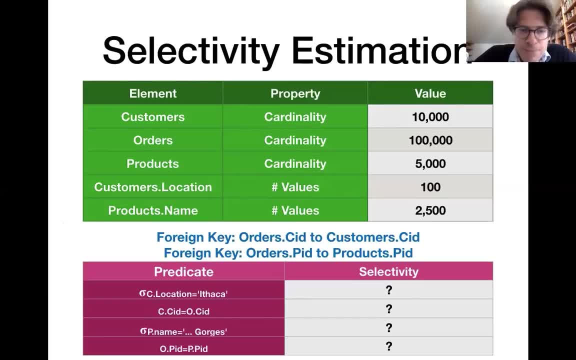 You have the number of distinct values in certain columns, In the middle of the screen you have constraints, like foreign key constraints, in this case. more specifically, And on the bottom you have the different predicates that appear in the query, And now I'm gonna give you a minute in order to think about. 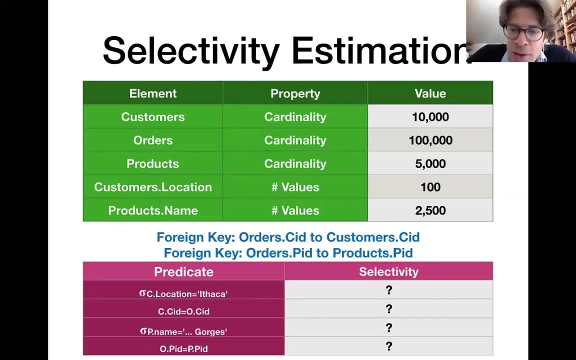 how you would estimate the selectivity of those predicates. And while you're doing that, I am gonna look at the chat for questions before we will resolve that here. So that is the first step. we are trying to estimate for each predicate which percentage of rows. 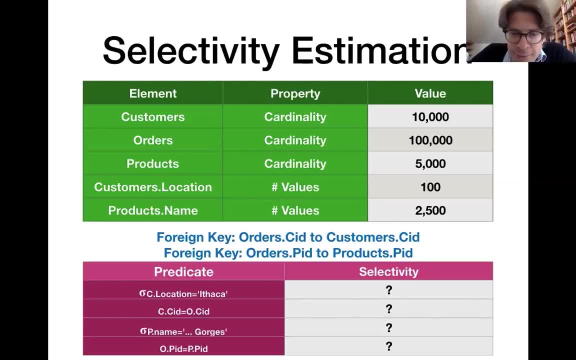 satisfies that predicate, that is the selectivity And, as we have seen before, you can make those simplifying assumptions, such as uniform data distribution or independent predicates. So we have the first step in order to estimate the selected predictability of those predicates. 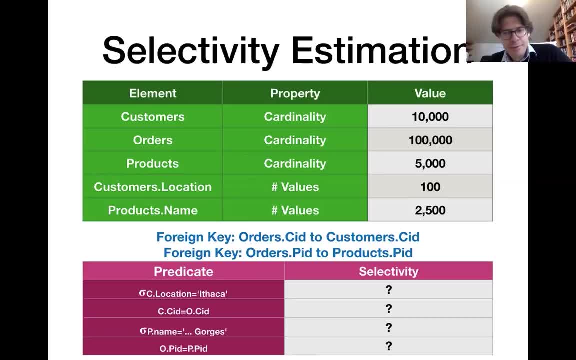 And once you have that, you can start to work with the table. And then the second step is to calculate the set of variables of the set of variables, And the third step is to calculate the set of variables for the set of variables. And this is just to give you a sense of where we are going. 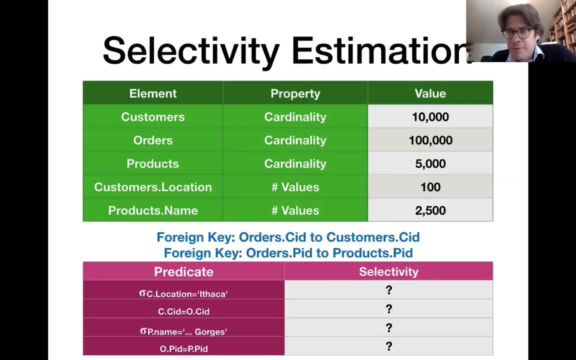 So we are gonna start with the set of variables. The set of variables is called a set of variables, So we're gonna use those. all right, i think let's continue here. i think it might have been at least enough time to think a little bit about how you would approach this problem, but perhaps not doing all the precise. 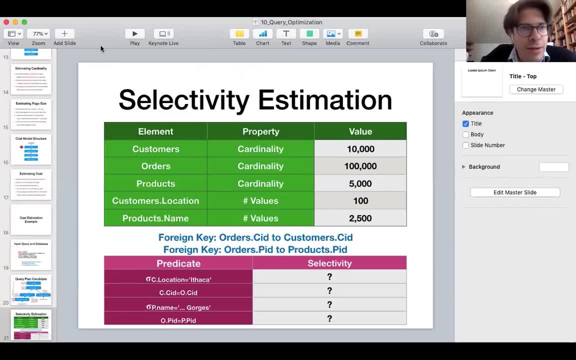 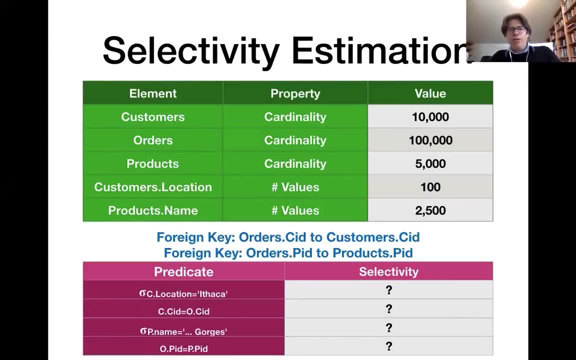 numbers that we quickly missed the chat, so i see the first slide all right. so that would be some estimates of all those predicates. for instance, we know that there's a hundred different locations according to the statistics in the green table and therefore, if i restrict to one of those locations, then using the formula that we have seen. 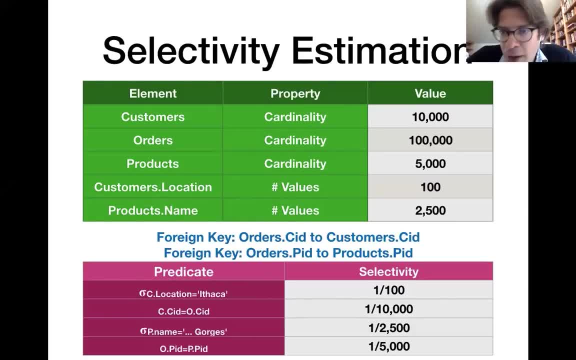 but before we can estimate the selectivity of one divided by a hundred. and here if we have uh like the joint, basically the joint condition between the customers and the orders, where their customer id must be the same, so, um, there's a foreign key constraint uh, from the orders to the customers, that means for each order. 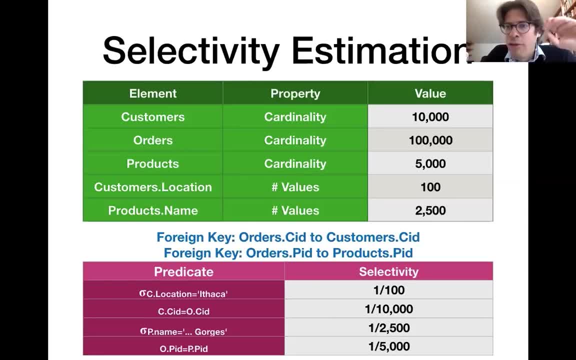 i will have one specific customer associated with the order. so that means, um, if i multiply the cardinality of the customers and of the orders table, uh, then i would pair up each order with a 10 000 customers, which is way too much. so. in order to bring that down to a more realistic 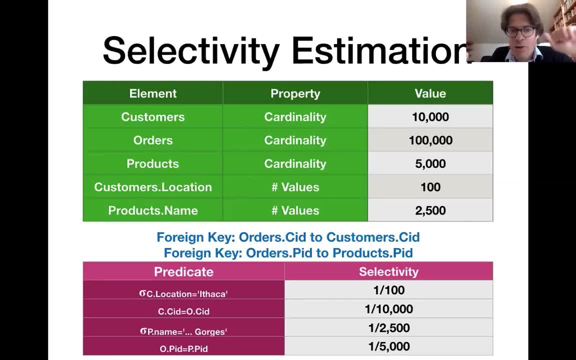 number, i want to divide that by 10 000, because each order is not associated with all customers, with all 10 000 customers, but only with one customer. in order to express that, i divide one by ten thousand. now, similarly, if i divide one by ten thousand, i divide one by ten thousand. 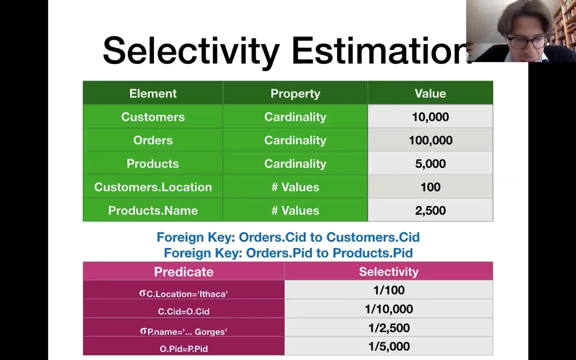 by fifteen thousand, i will have one column that is likely be the of the go and two in order to be the of the go and have five or six customers即 orang segments normally. and so if i tie up four columns, i add in four and they begin to create the cost of that. 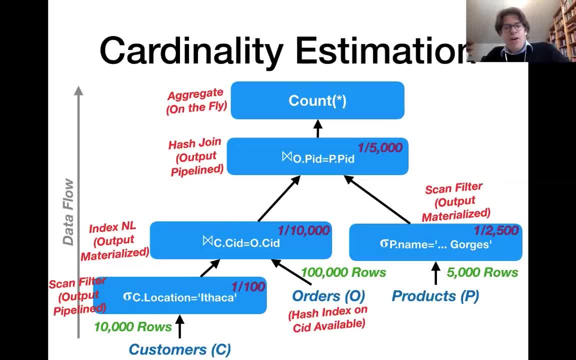 property and the traditionally counter being the common, common strength, that this is fell down. i twist, they divide by three and then i will also divide and multiply the cost away by three and then, if we let it go on a left to right hand side movement, it'll break down. 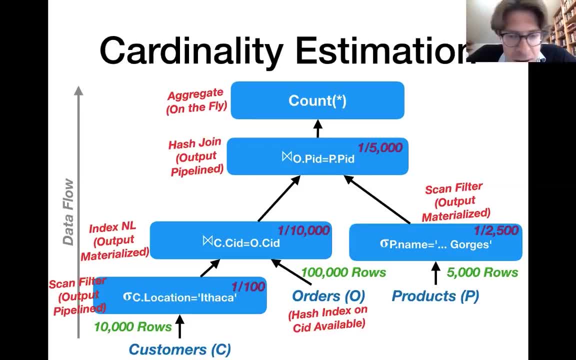 operator in purple and we are given the number of rows in the base table. so I'm here. for instance, if you have 10,000 rows in the customer table and the selectivity of the first predicate, as we have estimated, you see, here the estimate is 1 divided by 100. so if I multiply that together then I simply end up with. 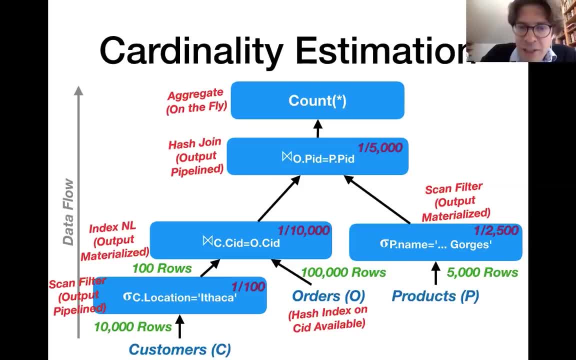 an estimate of a hundred rows for the output of that filter operation. and if I have the join here, then in order to estimate the size of the next join here between customers and orders, then I just multiply the input sizes. that would be a hundred times a hundred thousand, which is the number of orders, and then divided. 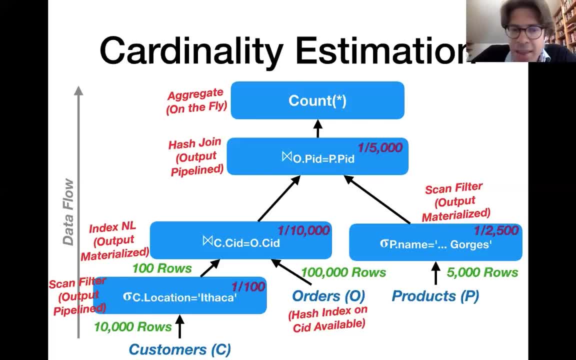 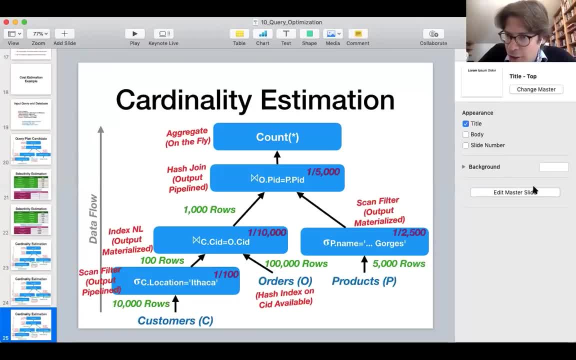 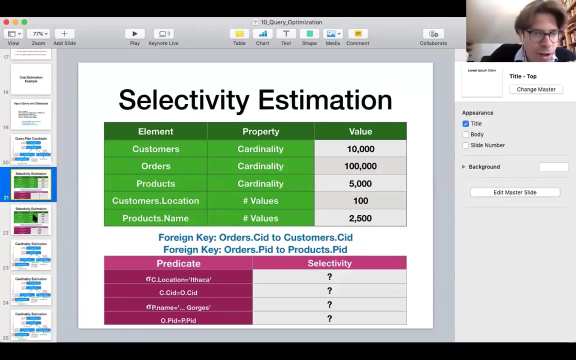 rows and quickly see where there are some questions in the chat. okay, there are some questions about how we get- I don't understand how we get- 1 divided by 100 and 1 divided by 5,000 and 1 divided by a thousand. okay, so, um, so that would be 1 divided by 100, 1 divided by 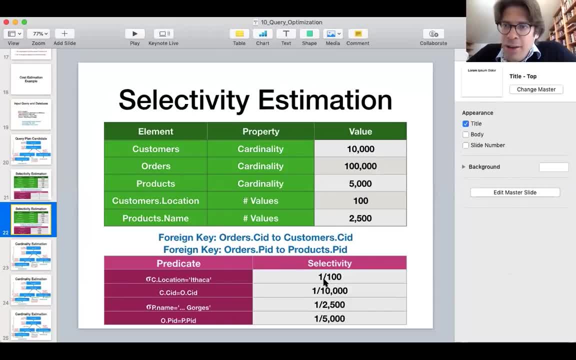 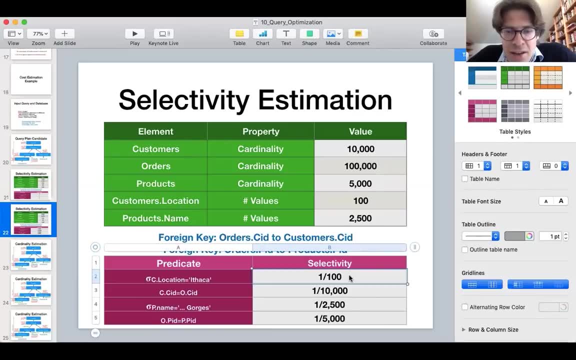 tens of so um in general, in order to get to those estimates, for instance here the estimate one divided by a hundred, we assume that those are uniformly distribute it. that means that we have a hundred different values for the location called and we filter to any single one of them Because we assume that each location 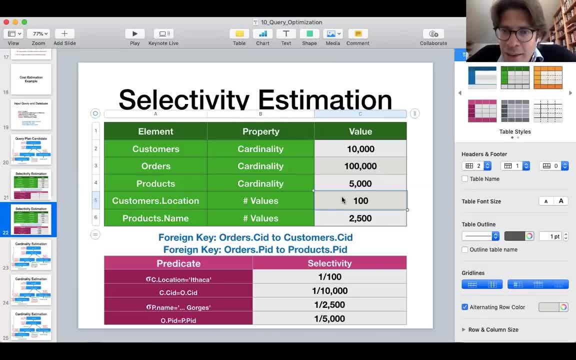 appears with equal frequency. we estimate that the selectivity is one divided by a hundred, because only every hundredth row will be for one specific location, And the principles for estimating this, for instance for the joint condition, is that if we pair up random combinations of customers and orders, then the 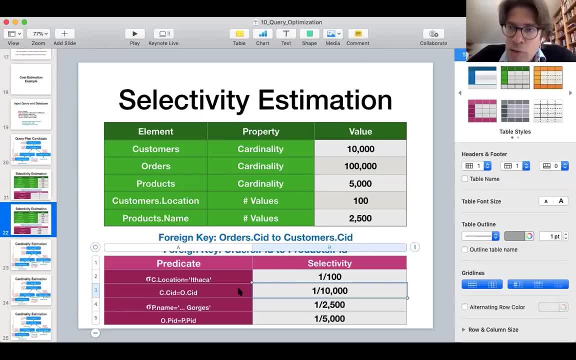 probability that the order refers to the right customer. that should be one divided by the number of customers, And here we have 10,000 customers. This is why we are dividing one by 10,000. All right, Basically for the joint condition, the selectivity is the probability that a randomly selected 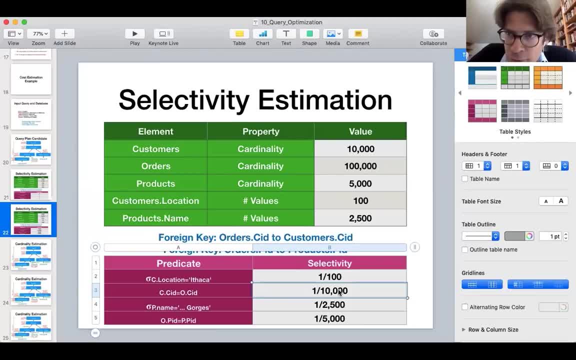 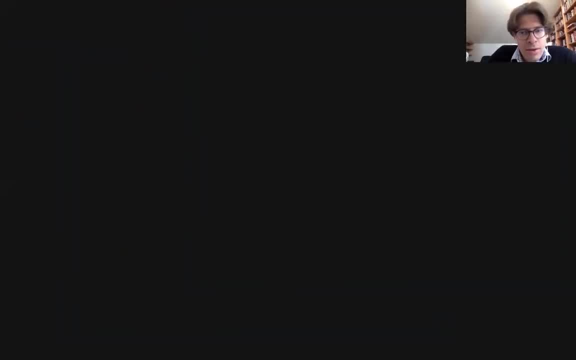 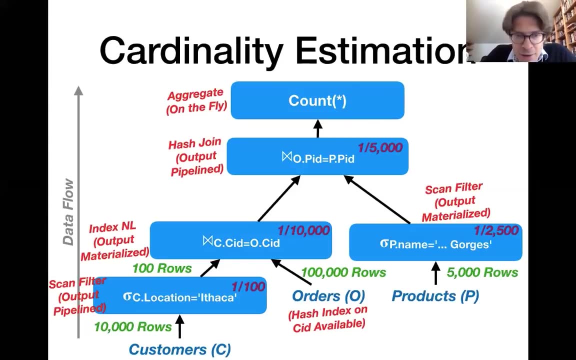 order and a randomly selected customer match, meaning that they have the same customer ID. All right, So now we have used those selectivities in order to estimate the sizes of different intermediate results. So we have the number of inputs, the number of outputs, the number of inputs and the 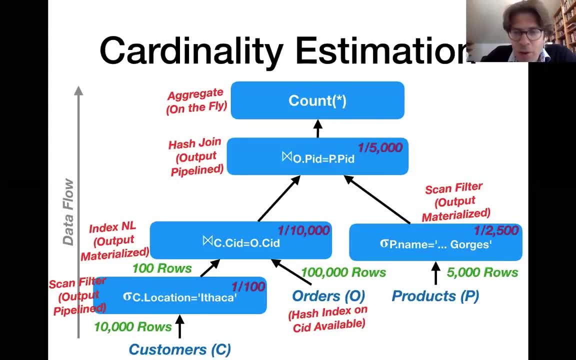 number of inputs, And then we multiply the results here. So we are multiplying here. for the latest result, we are multiplying 100 by 100,000, and then by one divided by 10,000, which is the selectivity, And that gives us 1,000 rows. 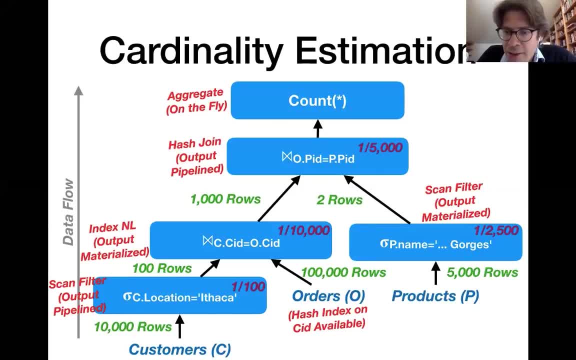 Now, here on the other side, when applying the selectivity and the number of input rows, then we end up with two rows And here, if we multiply the two together, then we get the number of inputs And then we add the input. 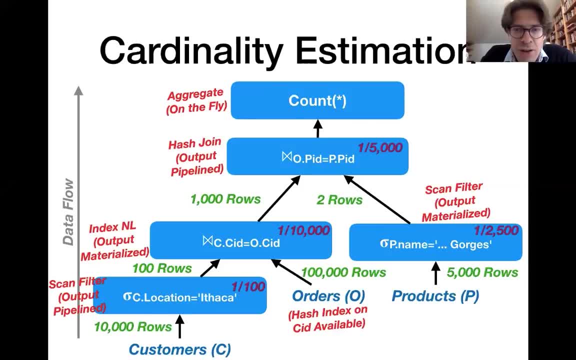 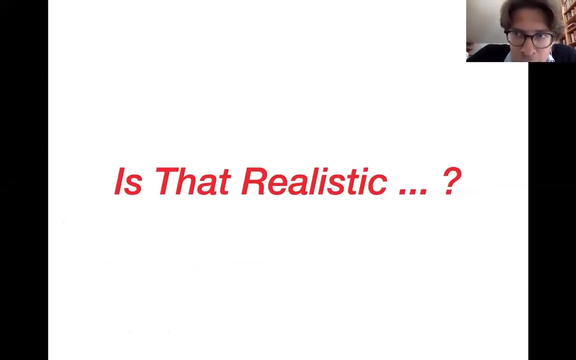 for the next joint and multiply by the joint selectivity, by the joint predicate selectivity, then we end up with an estimate of two divided by five rows. So a little bit less than half a row expected. Okay. So little question those size estimates that we have been calculating so far. 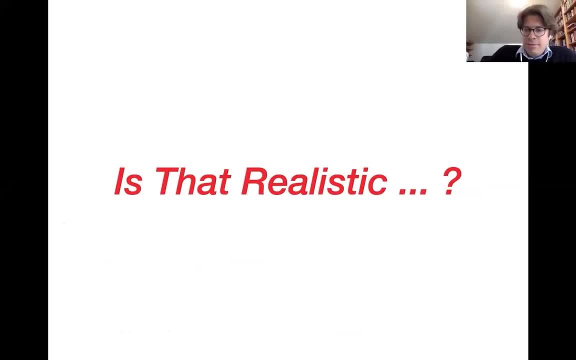 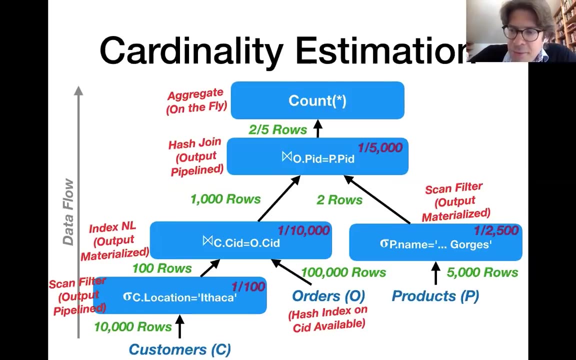 do you consider them realistic Or is there maybe something wrong with them? Does anyone feel that those estimates might not reflect the accurate sizes for some reason? Do you believe that in the end, when asking this query, we really would get probably no single result? 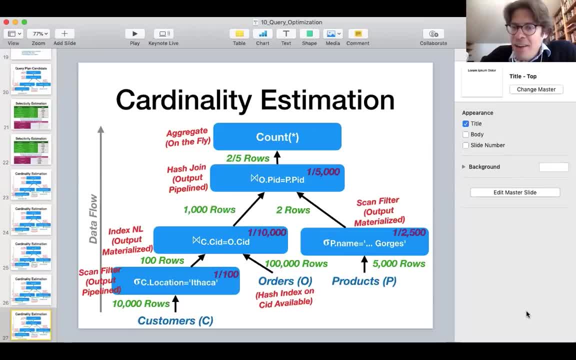 Okay, very good point here in the chat Somebody: oh yes, very good, very good, Okay. so people are generally attacking our simplifying assumptions. Very good, and that is exactly. yes, Yeah, okay, very good here. 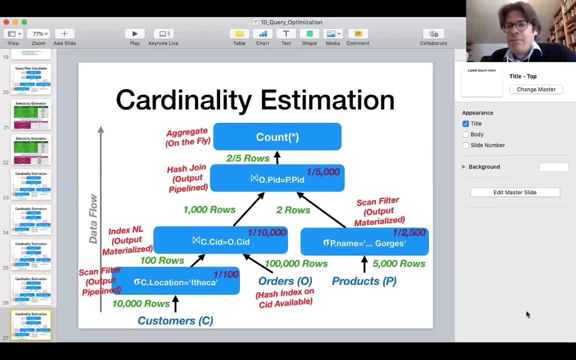 More propositions coming in, Exactly. So there's our simplifying assumptions, and people are already criticizing the uniform distribution. It might in reality not really be uniform, right? I mean, maybe for instance there's like different locations. If there's another location in New York City, for instance, 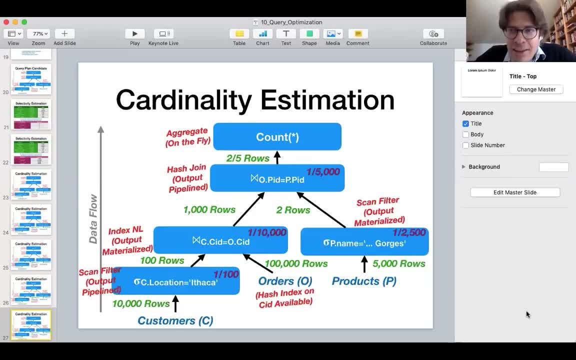 it might have a slightly higher frequency than Ithaca in our data set, depending on like which customer base you're serving. Yes, so uniform distribution, that is a stretch. What else? Yeah, you think about how different predicates connect together. 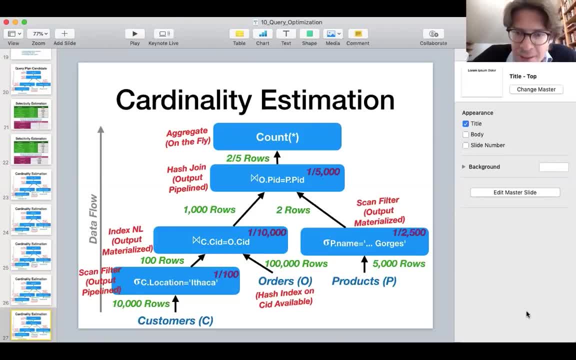 Yes, exactly, There could be some dependency between those predicates. I mean, this book here is obviously it is quite focused on Ithaca, it seems. So I would assume that, you know, there's like I don't know. I don't think that it's gonna be quite as good as. 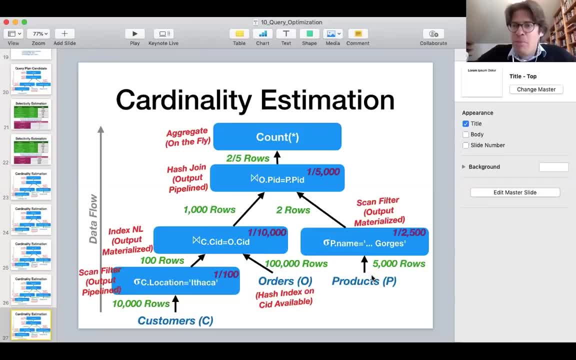 that for people living in Ithaca there's a much higher probability to buy that specific book. So this is not independently random distributed, but probably most of the people buying the book they will also be from Ithaca, or a large percentage of them will also be from Ithaca. 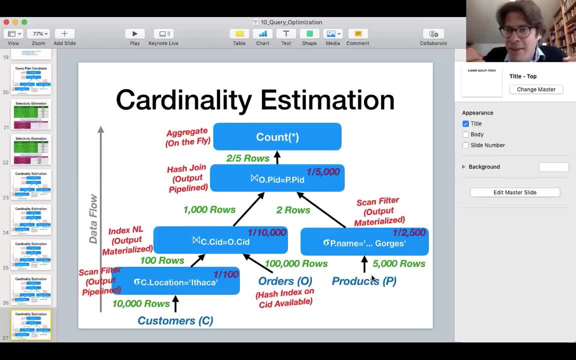 And that means that probably those two predicates together they're less selective than this analysis makes us think. So probably in the end, since there's this dependency between those two predicates, I would end up having more result rows than I'm expecting in this analysis. 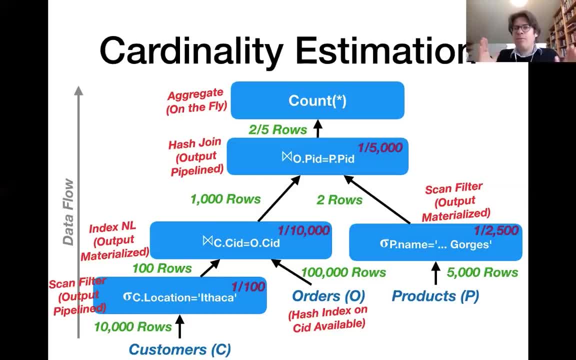 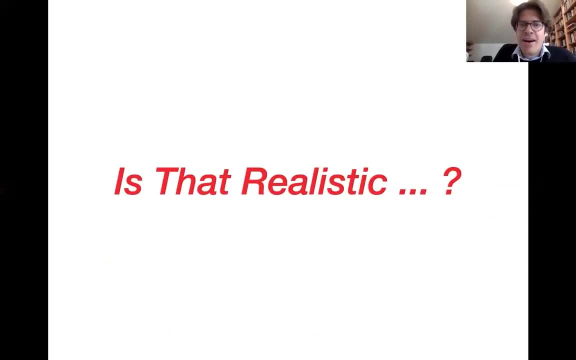 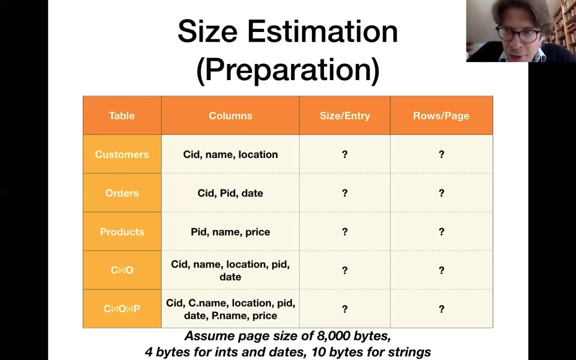 All right, very good, And the reason is that you're making those simplifying assumptions which are not always justified in practice. All right, so it is not realistic In reality. there's a couple of problems with that. Nevertheless, let's continue. 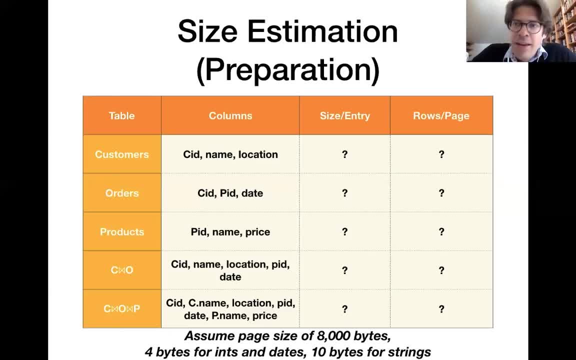 with those simplifying assumptions. So I mean, in reality, those simplifying assumptions. they don't always hold, but often they at least allow us to get some rough estimate of the quality of a given pair of bands. So, even though it's not completely realistic, 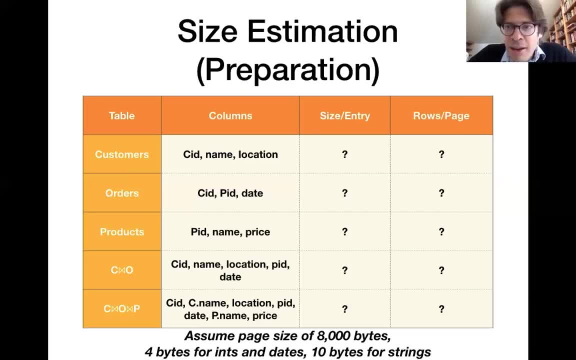 let's continue with it, And the next step here would be to use those row counts, those estimated row counts, in order to estimate the number of pages. And in order to do that, you first of all should figure out how many rows you can fit on each of those pages. 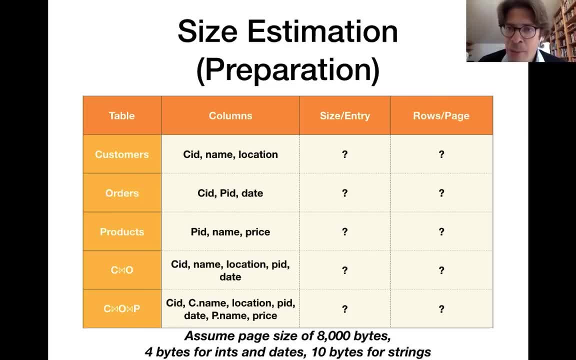 For that you need to know how much bytes are used up by one specific row. So, assuming that we have a page size of 8,000 bytes and assuming that we use up four bytes for integers and dates and 10 bytes for strings, 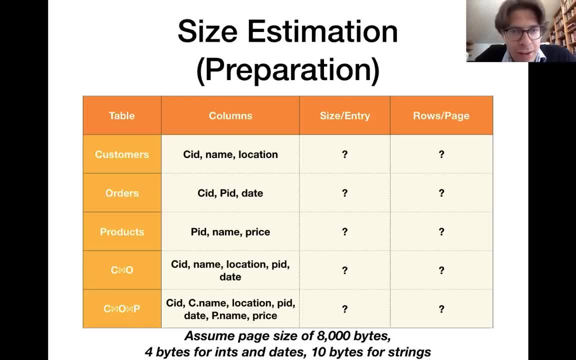 So, in order to so looking at, for instance, the first, you would be taking the ethics table with the columns custom ID, name, word, location. what would be the number of bytes per entry here? the number of bytes per row? 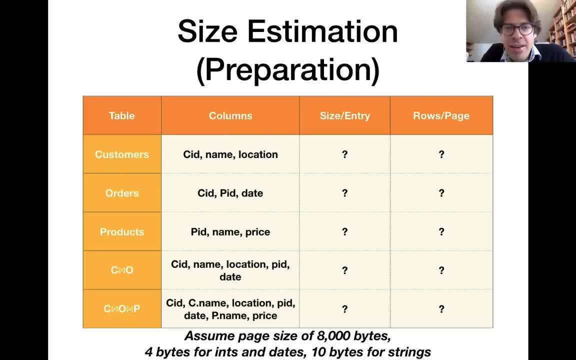 Counting it together into: yeah, basically you have four bytes for the customer ID, 10 bytes for the names field, because that is a string and is also a string. so we end up with 24 bytes per row And if we have that, then we can simply: 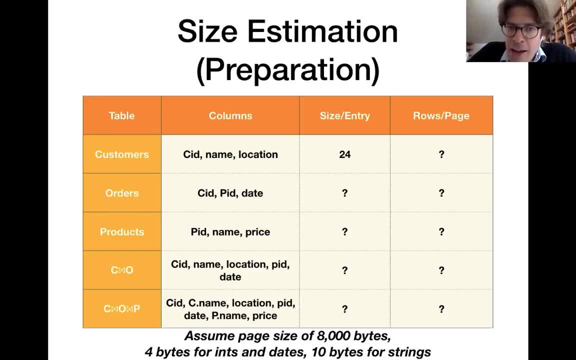 divide 8,000, the number of bytes per page by 24, the number of bytes per row And to round down, then we get this number of rows over here. So if we make the calculations- and I encourage you to do that in order to get the hang of it- 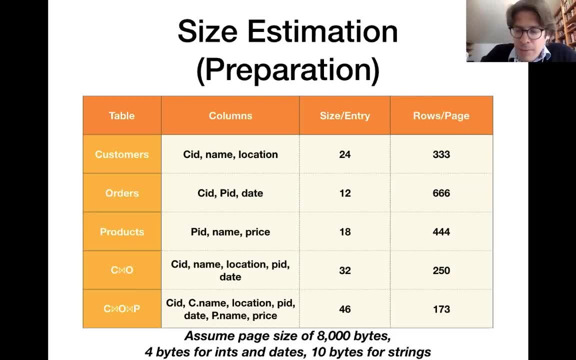 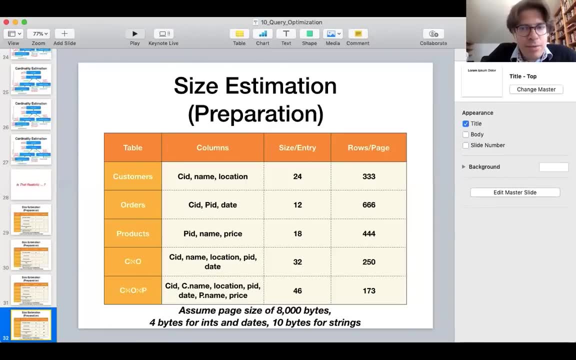 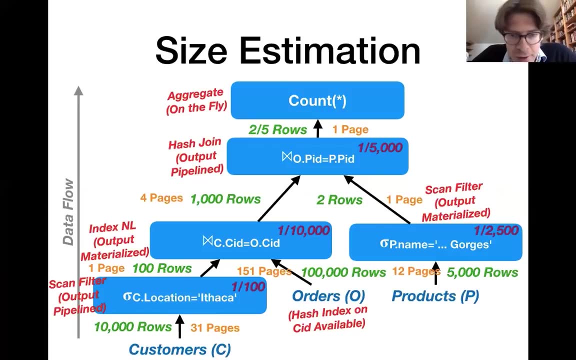 then we end up with those numbers over here. All right, quickly move the chat, All right. so here I have already done the calculations. You see the size estimations in orange here, associated with the corresponding row counts for the different intermediate results. 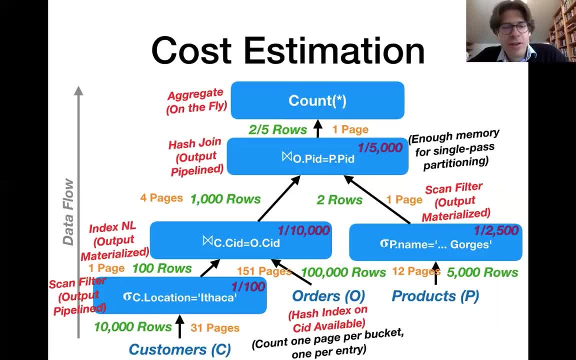 Now the next step. So here is the question. the next step is to calculate the number of rows over here, And the number of rows over here would be to do the cost estimations. So here we're, going through the different operators in the plan in order to do the cost estimations. 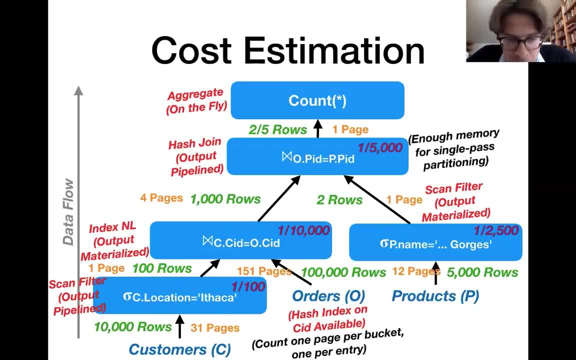 Starting, for instance, with the filter on the customer table. So if I have 31 pages as input, so here for this operator, I assume that initially all data is located in a data set on hard disk, so therefore I need to read those 31 pages. the output is pipeline. 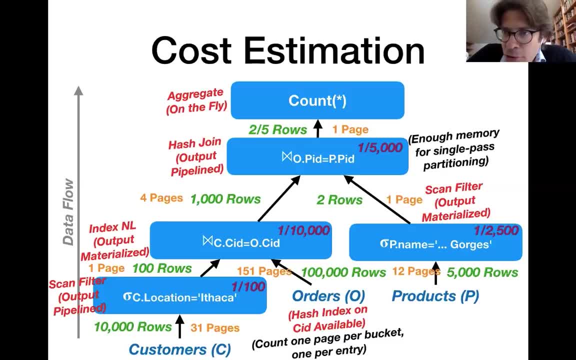 that is good, so I don't have to count cost for writing the output to hard disk and I simply end up with a cost of 31 pages for reading that, all right now. the next one is the index and nested loop. join between the customers and the. 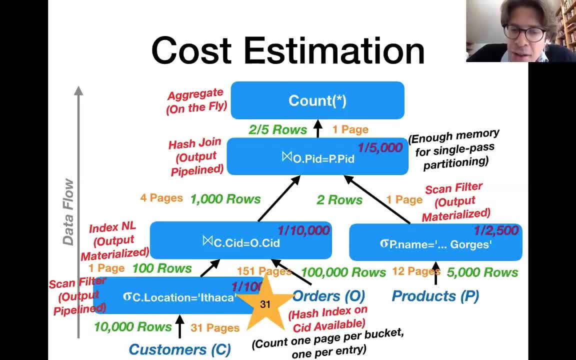 orders. I assume that I have a hash index available on the customer ID and now, in order to estimate the cost of those index accesses, I need to make some additional assumptions here. so here I assume, to simplify things, that this is a hash index which doesn't have any overflow pages, at least at the moment. 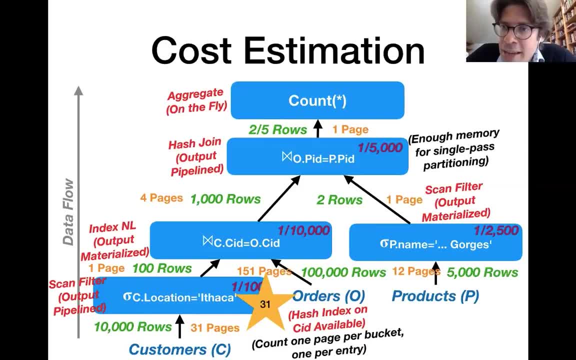 and then I simply estimate the index access cost as a hash index which doesn't have any overflow pages, at least at the moment. and then I simply estimate the index access cost as a having to read one page from hard disk in order to look up entries in the. 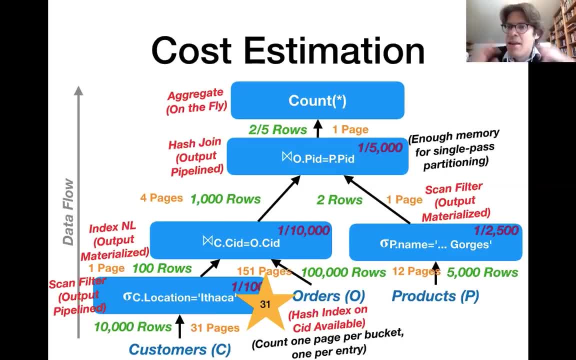 associated hash bucket. and then if the index contains references to the data but not the actual data, then I still need to count one page access for loading specific entries, then following the references that are contained in the index. so I am making pessimistic assumptions because I assume that those 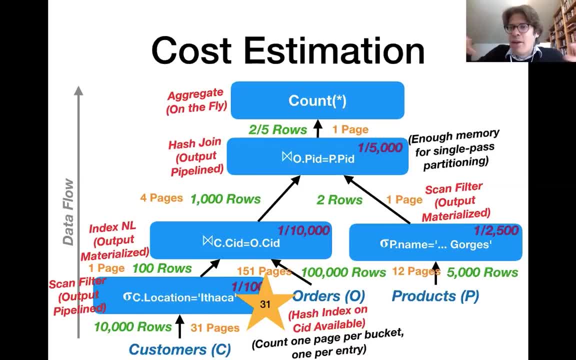 different entries that are contained in the index are the ones that are not? are the index references that they are located on different pages? I need to count one separate page access in order to retrieve each of them. so, assuming the index is unclustered and, in this case, over here, 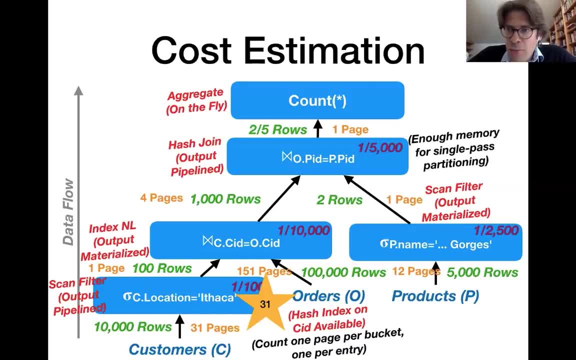 my input to the index nested loopchart. on the one side I have a hundred rows. that is on the non indexed, that's for the non indexed tables. so for each of those hundred rows I need to first of all look up the course corresponding hash bucket and that gives me one page access and 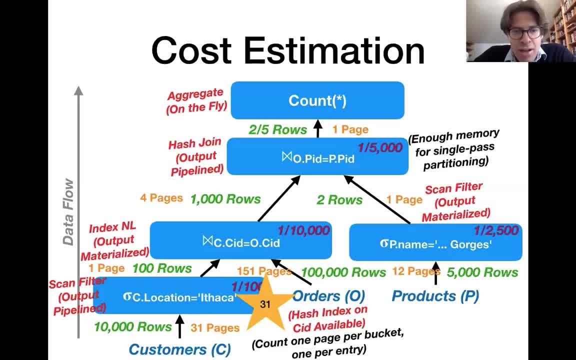 Now I see that in average I have something like at 10 orders for each of the customers. That means because here you see, the input to the Inexhaustible joint is 100 customers and after joining with orders I get a thousand customer order combinations. on average I have 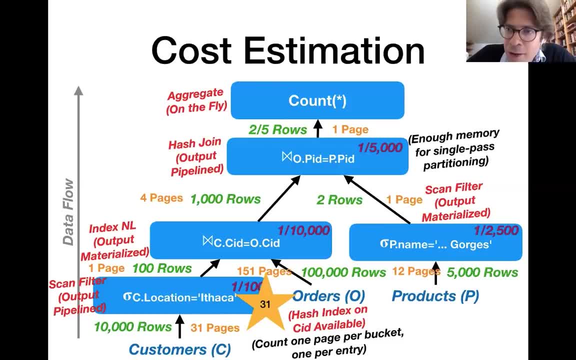 10 orders per customer and that means that after looking up the hash bucket page, I still need to load entries from 10 pages for each of those orders for the current customer and that means that per customer I have essentially a cost of 11 of 11 pages and 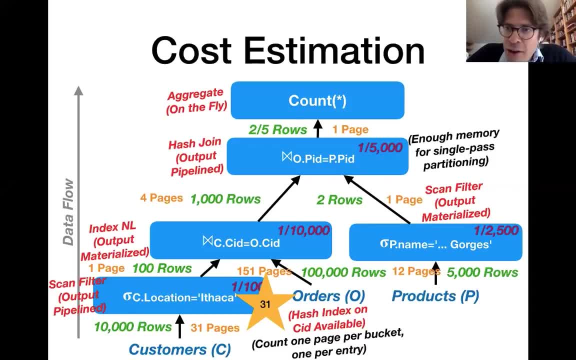 Additionally, here the output of the joint is materialized. I also need to count the cost for writing out this output and all Things considered I'm getting a hundred customers. times cost 11 per Customer plus four pages that need to write out to hard disk. So that is the entire cost of this joint operation. 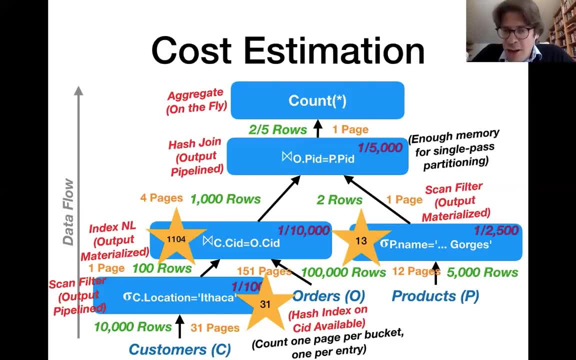 All right now, in order to analyze The cost here of the filter on products that works as before. here I'm reading the 12 pages and I'm writing out one page and for the hash join: as you see, here We are assuming that we only need one single path for the partitioning, because we have 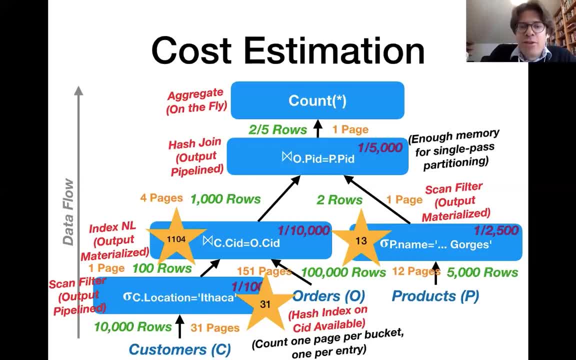 enough main memory available. so because of that, the cost of the hash join is simply three times the input size, and Here there would be three times The four pages plus one page makes 15 pages. the nice thing is that I don't need to write out the output and 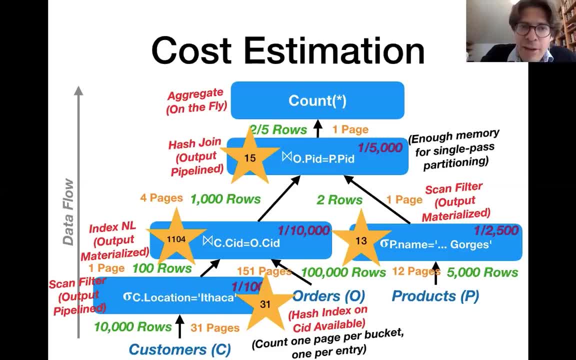 Also for the following count operation. assume that this is executed on the fly, So you have a cost of zero, also because we don't count any cost for writing out the final result of the query plan. So here we have. I counted the cost of each single operator. 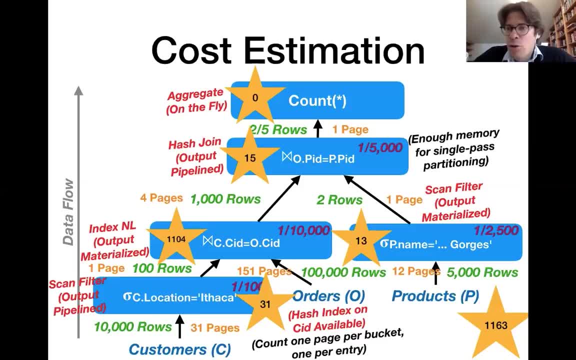 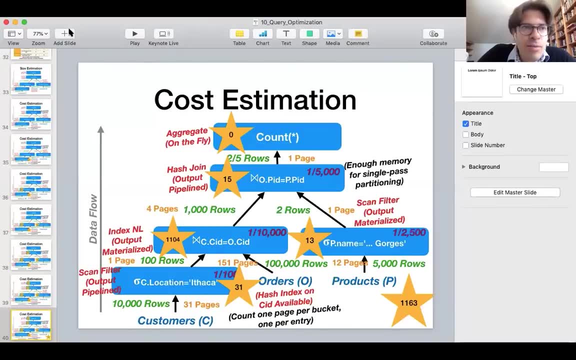 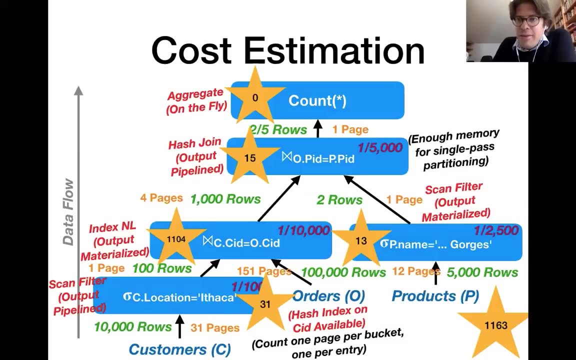 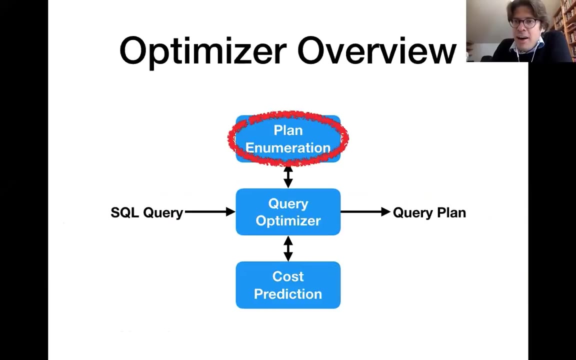 and if I count all the Count, all of this together, then I end up with the total cost of the plan, which is a little bit over 1100 pages. All right, so That was the first part of the session on a query optimization. so In the next lecture we're gonna continue talking about carry optimization. 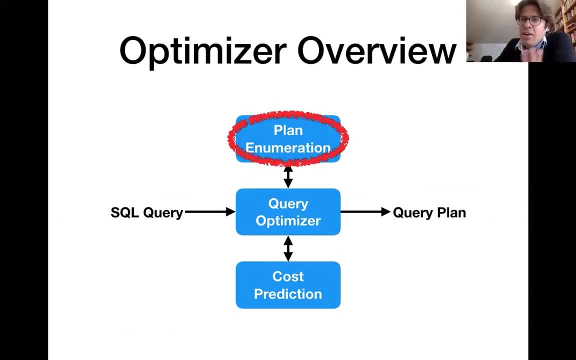 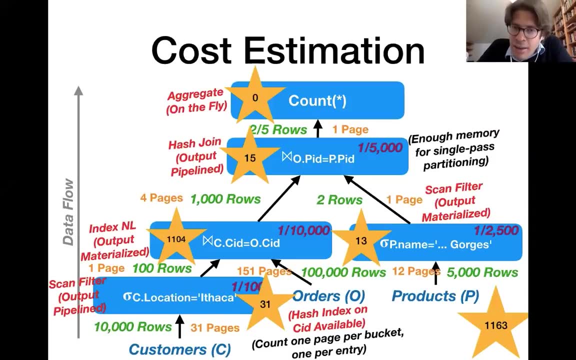 But now we will. in the next lecture we will discuss about the plan enumeration step, So I recommend you to go again over this example in a little bit of detail. So this is really an end-to-end example. We start with the data statistics, We end up with cost estimates for the plan. 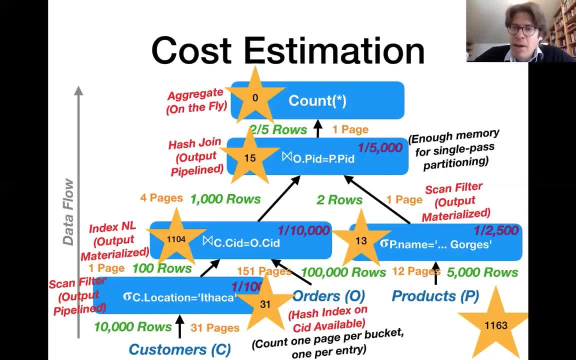 You might also want to vary the example a little bit, and we also see a couple of other examples in this direction, but I definitely recommend you to go over this Example in detail again. alright, so Here let me quickly see whether there are some quick questions I can answer in the chat and 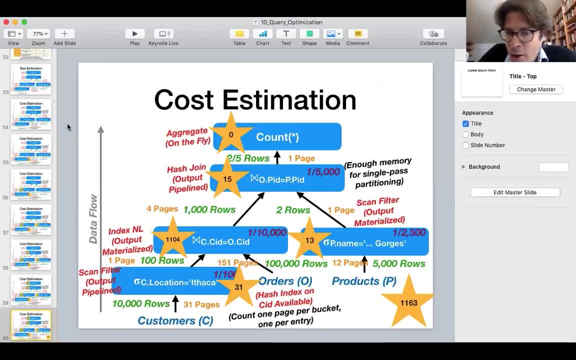 then you're gonna Gonna stop. So here I see, for instance, one question about how we get to the 15 pages for the hash join, and We have seen a cost formula for hash join: We just multiply the combined input size by three, because in the partitioning path 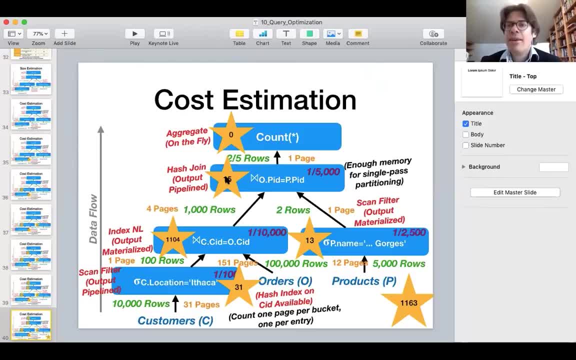 We are reading things once and writing things once, and then in the actual joint pass in phase two, We are reading things once again. So here I have four pages on the left, one page on the right. That means five pages in total, and I multiplied it by three gives me 15 pages. 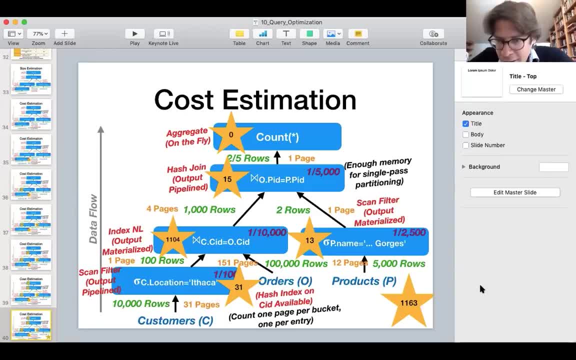 And Okay, basically There's like questions about Multiple items here for the cost estimation. So in order to get to most of those a page, the sizes, We simply look up how many rows we estimate here and then about like how many rows we can fit per page. 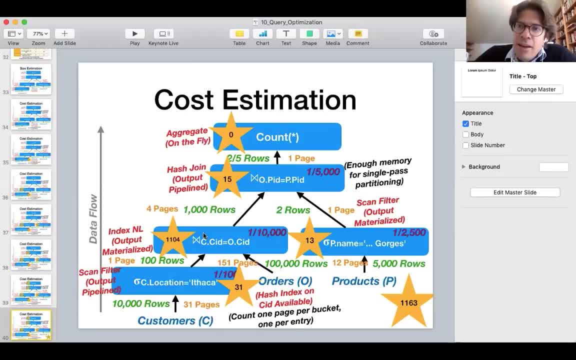 For the corresponding result. so we had this a step, that we calculated estimates for the byte size per row and for the number of rows that fit on one page. So I'm applying that here in order to get from the row estimate to the page estimates And in order to calculate this. 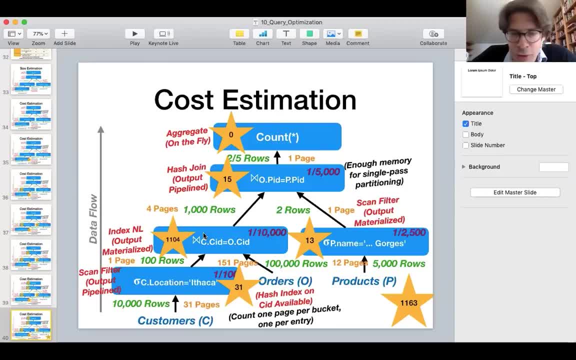 1104 pages for the index, a cost for the index nested loop joint here. I essentially assume That for each of the customers I will have an average ten orders and I'm using a hash index in order to retrieve them, which which means a cost of one page. 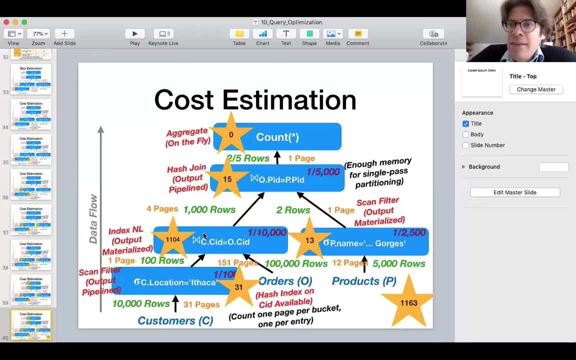 in order to read the references in the hash bucket, and then cost of 10 pages in order to read the actual data which we assume is located on different pages. So it gives me a cost of 11 per customer. I have 100 of them. 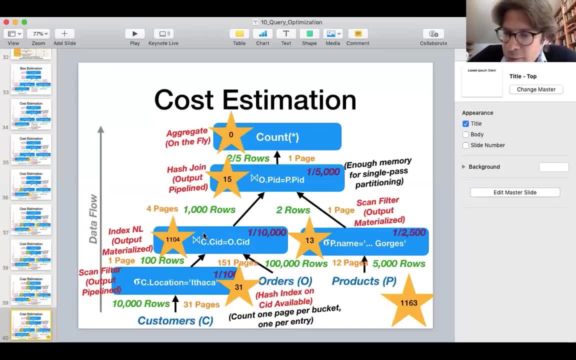 and then I need to count the cost for writing out the joint recital. That is how I get to this cost down. All right, so we are at the end. I wish all of you a nice day, and then I see you again on Friday. 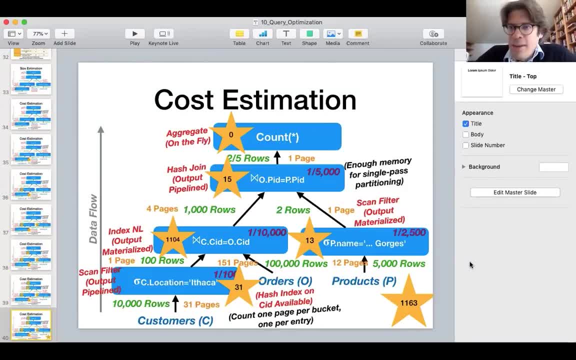 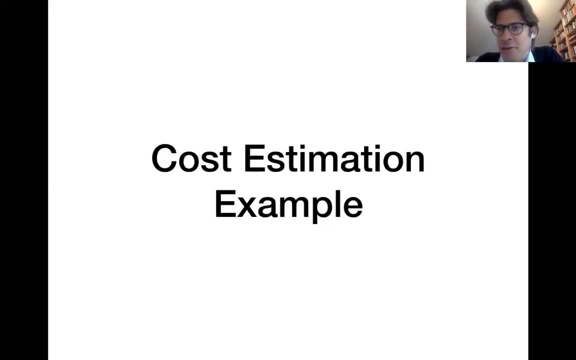 where we continue with a query optimization. Have a nice day. All right, let's get started. So the last time we have been discussing about a query optimization and we will continue discussing about a query optimization today, then we might still have enough time to start a new topic. 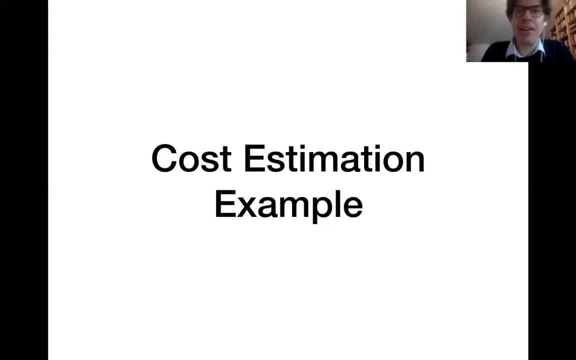 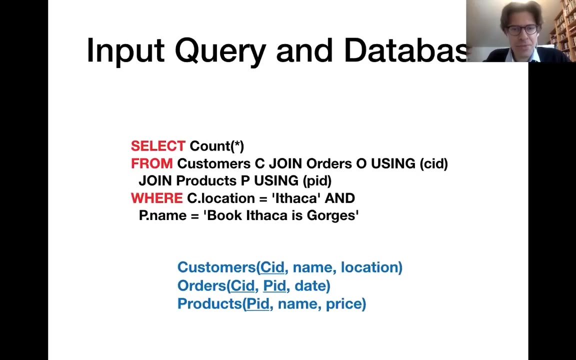 So the last time we have stopped with this example over here we have seen an example for how the query optimizer estimates or predicts the execution cost of a plan before the actual execution. Now here we had the example query on the example database. We want to find out how many people in Ithaca 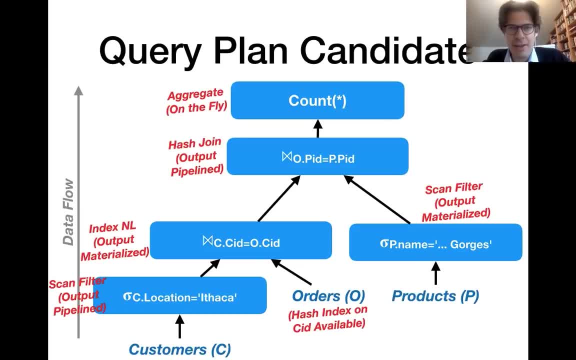 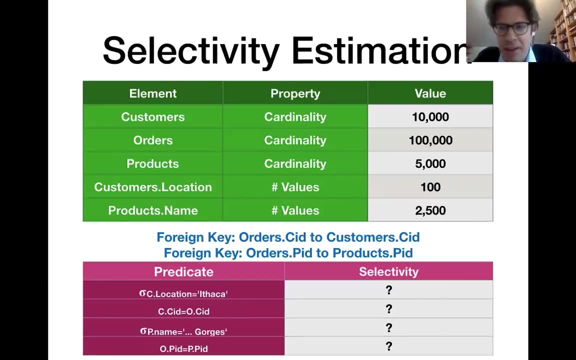 bought books about Ithaca, and this is the example plan for which we did the estimation. So the first step that we always make is to try to estimate the selectivity of the predicates that appear in the query, meaning the ratio of rows that satisfy the predicate. 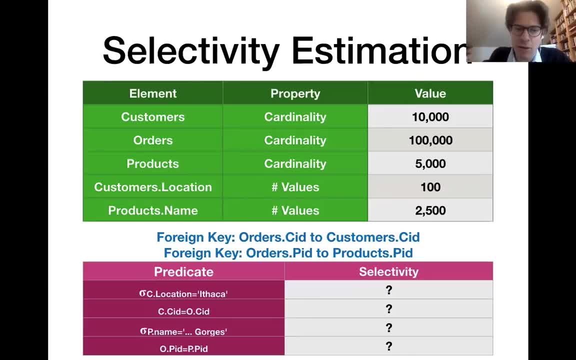 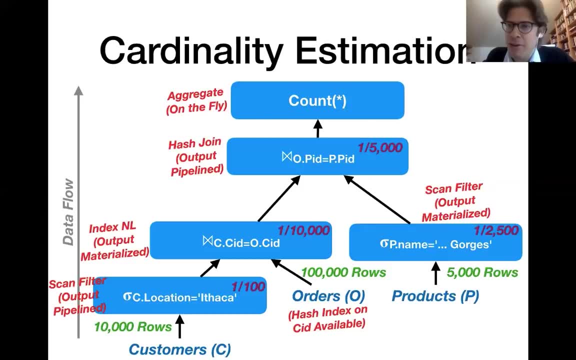 and we have done that here, based on statistics and on constraints, and come up with those estimates over here. Now the next step is to estimate the sizes of intermediate results, based on the cardinality of the base tables here and based on the predicate selectivity values. 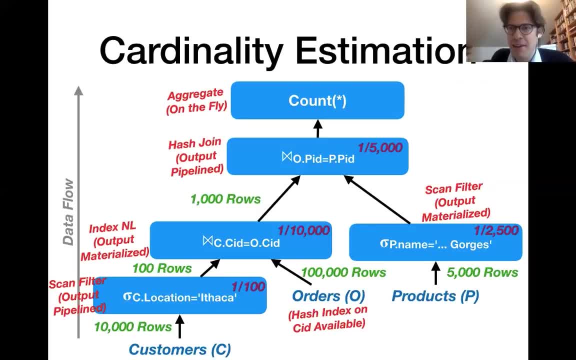 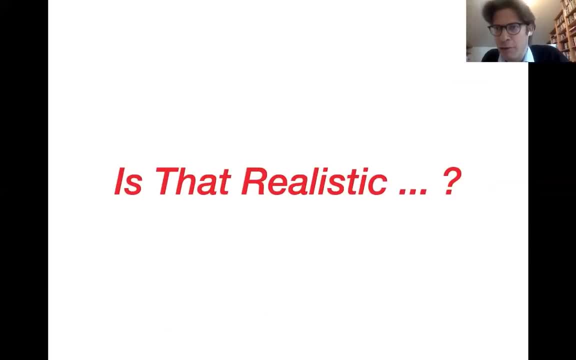 All right. so here we have estimated the sizes of those intermediate results in the plan And we have concluded that our estimates might not be entirely realistic because they don't take into account correlations between different predicates. But that is a simplification that query optimizers. 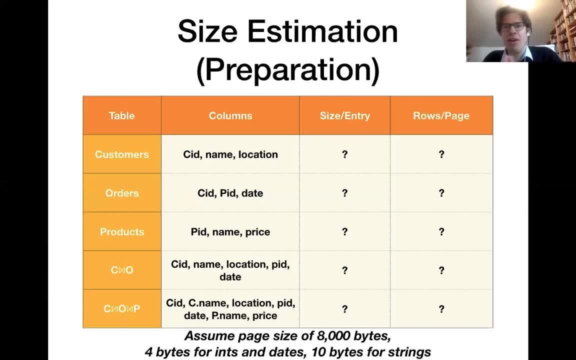 typically make, And with that simplification now we have estimated the sizes of entries for different relations, We always add up the byte size of the different fields in a record And then we think about how many rows you can fit on one page with that size. 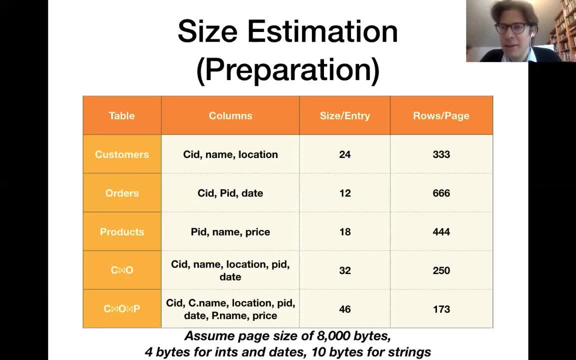 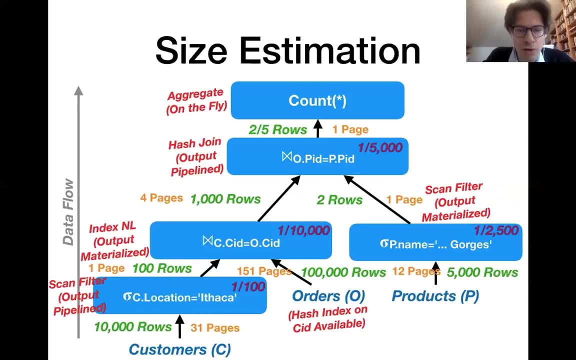 And if it doesn't give you an integer- the division- then you always have to round down because pages cannot store. So we have to do additional tasking to make sure that they're all aligned. We have to run the next part and we 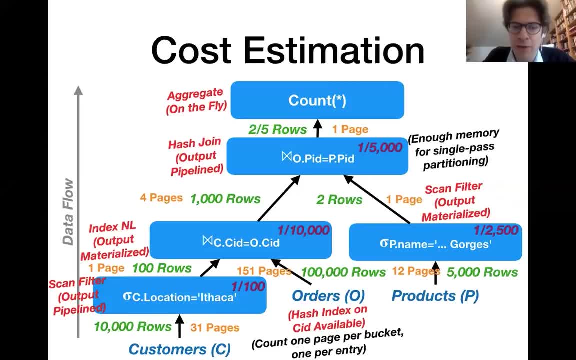 have to pay attention to the cost of the search results in order to be able to estimate the cost of the different operations. All right now, with that, we have inserted those estimates into the plan here in order to estimate the cost of the different operations, which. 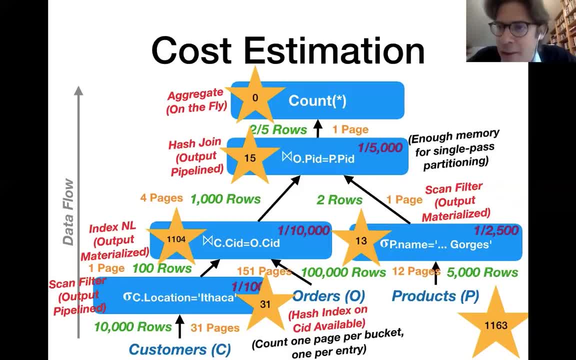 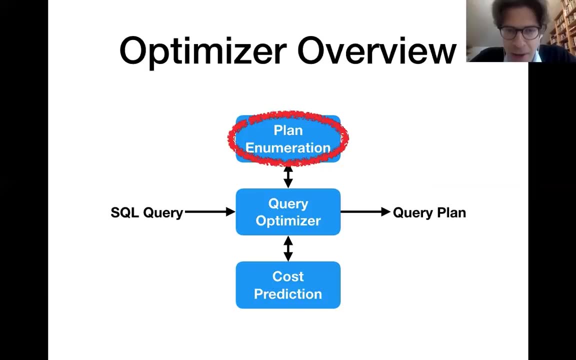 we also have done estimates- plan execution costs- and then, based on those estimates, they select the plan that they think will work best in practice. So we have been discussing about the cost prediction component of the query optimizer last time. Next we will discuss about how the query optimizer enumerates. 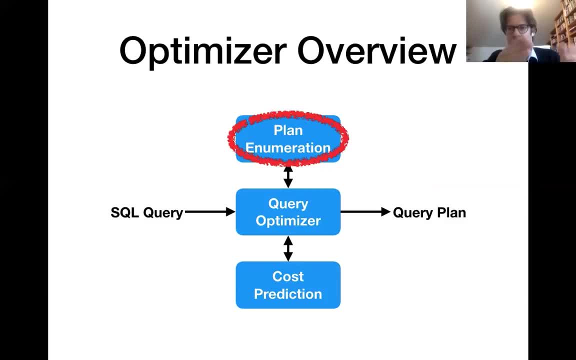 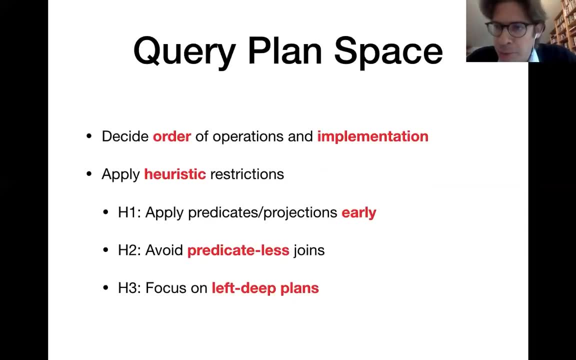 a different candidate plans. that is done in this plan enumeration component. Now the plan space for query optimization generally includes decisions about the ordering of operations. Also, we have a choice between different operator implementations. so the query optimizer makes both types of decisions and that gives you a pretty large 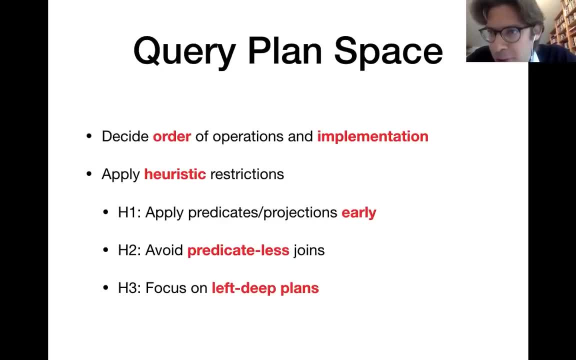 search space And, of course, query optimization happens at runtime, directly after a new query comes in. So you want to make sure that query optimization does not take too long, And that is why people typically try to restrict this huge plan space by using some heuristics in order to 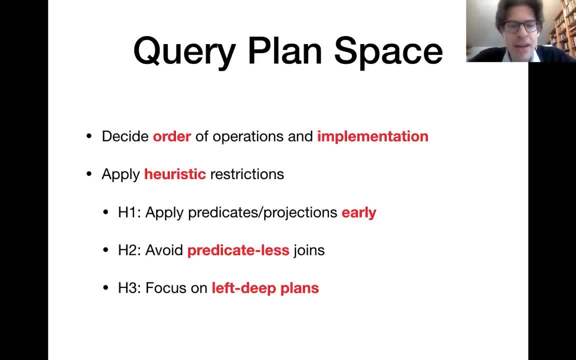 make query optimization faster, And in the following I'm going to discuss some of the most common heuristics that query optimizers make here. Those are the three heuristics that you see here. First of all, we try to apply predicates and projections early. We want to avoid certain 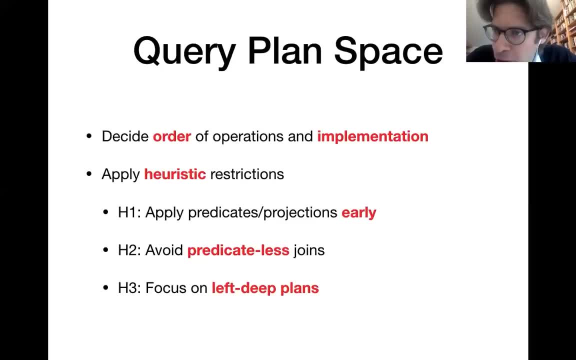 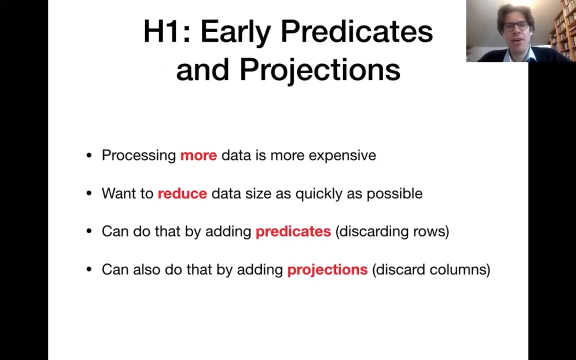 joins which cannot exploit a join predicate, And we typically focus on so-called lefty query plans. I'm going to discuss those three different heuristics in more detail in the following. So, first of all, in general, when processing data, it's typically more expensive to process. 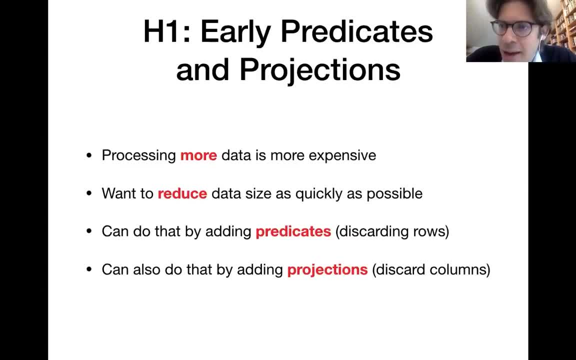 more data, And that is why we want to reduce data sizes as quickly as possible during data processing, And you can essentially do this in two ways: Either you throw away rows or you throw away columns. Both reduces the data size, And that means that you want to typically apply. 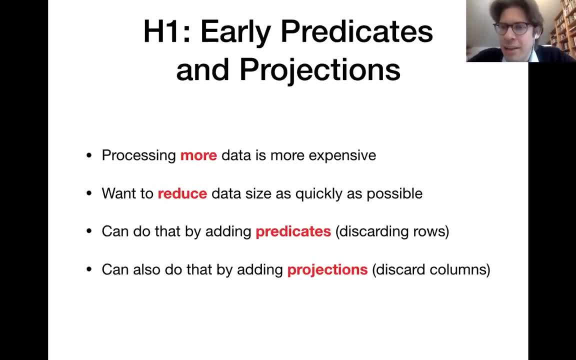 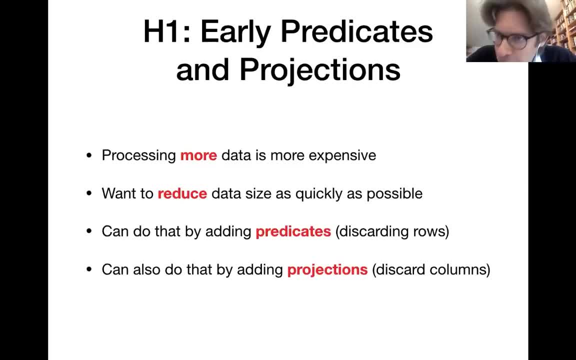 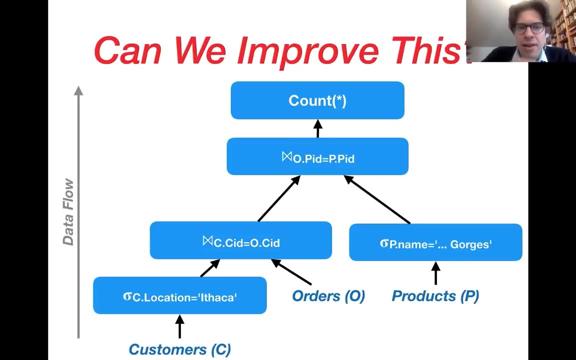 intermediate result And also for projections. you want to apply them as early as possible, meaning you want to project out a column If you are sure that it is not used any more in the future, during the same query plan. For instance, considering this plan from before, can anyone use the preceding term for the query? 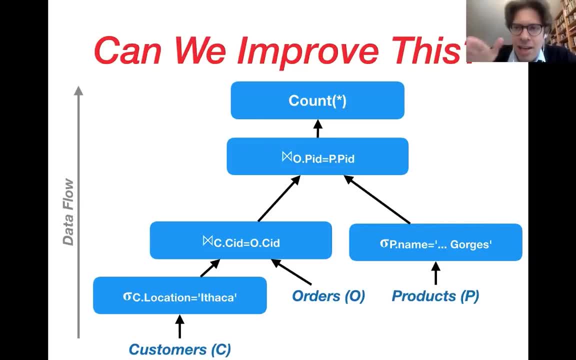 plan. see and tell me in the chat possible improvements of that plan, any suggestions for possible improvements, if you think about the heuristic that we have just seen. okay, very good, all right, so people are thinking about the projection and that is, in this case, the right track. so, yes, we. 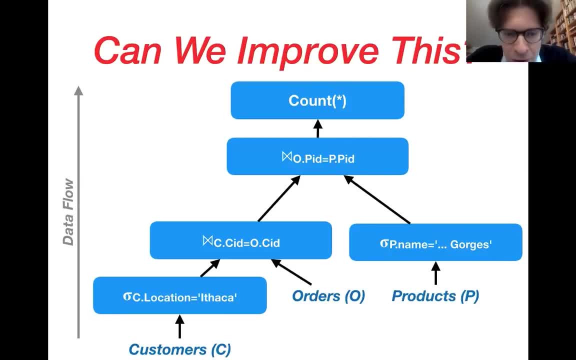 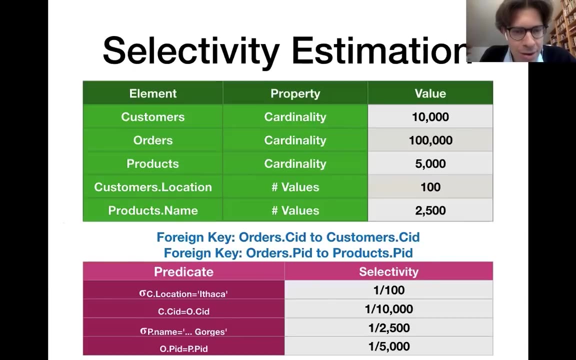 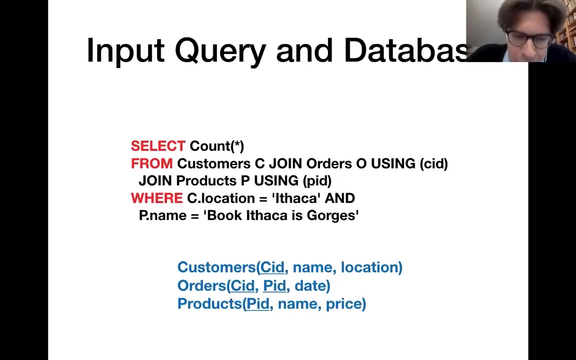 can try to get rid of more columns during processing and perhaps I should show you quickly the database that this query refers to again. we had that a couple of slides ago. so here we have the customer relation with the customer agent, the customer name and the location. we have the orders relation with the customer ID, product ID. 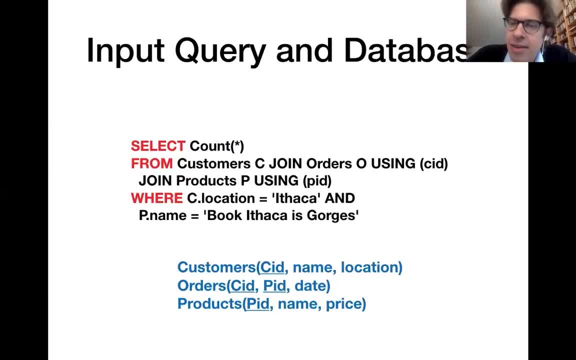 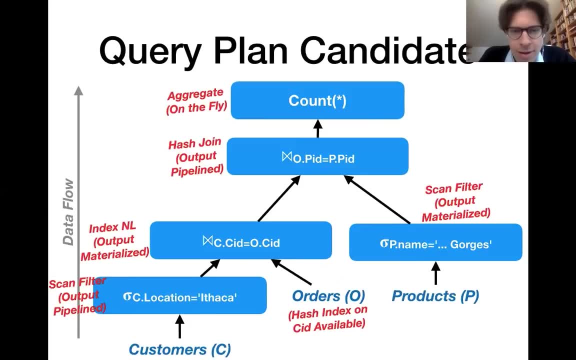 and the date, and we have products with the product ID name and the price. so each of those tables has three columns and if you look at the very plan over here- so that is the same query plan as we see later- then it turns out that we can probably 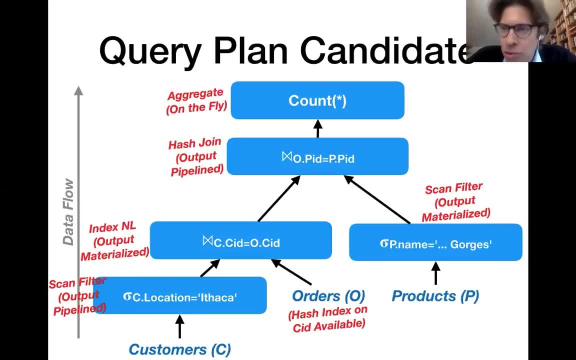 get rid of some of those columns during processing, without, without any drawback, basically. so, for instance, if you think about the orders column in the, or like about the date column in the orders table, for instance, that one is not used anymore, so it doesn't appear in any predicates, it doesn't appear in any aggregates, so you could immediately 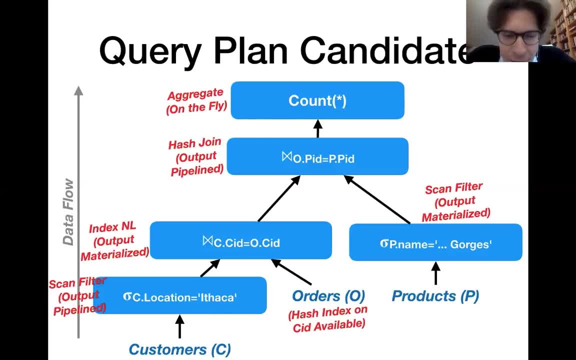 project out that column- the date column, for instance, and also after applying filters, for instance after applying the filter on the customer location and restricting it to either cut. after that we don't really need the location column anymore, so we could also throw that one away later. and that reduces the size of my entries so I can fit more entries onto a single page. that means I 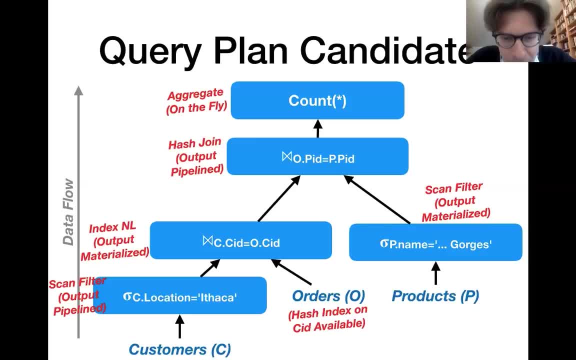 need less pagers overall, alright, All right. I need to be careful when projecting out columns. I don't want to project out any columns that I still need later, because later in the plan I have a predicate that refers to that column or an aggregate that refers to the column. 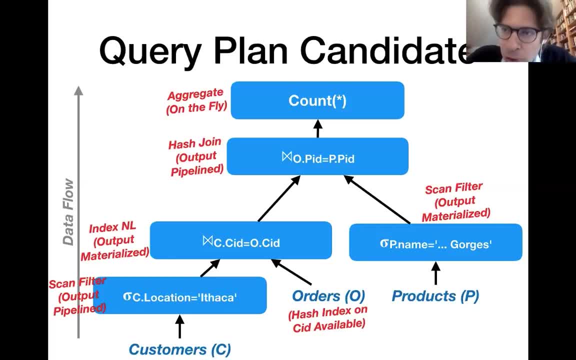 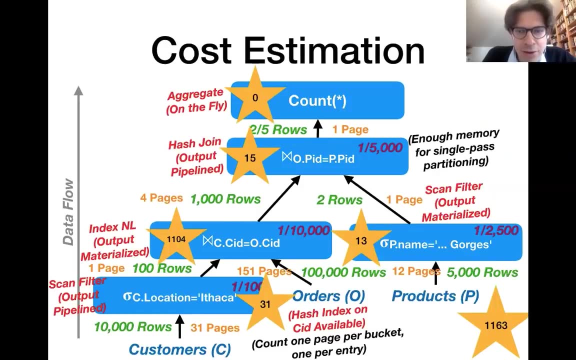 or perhaps it appears in some joint condition. all of those would be possible, But if none of those apply, then I can typically project out the column, and I should do that in order to reduce the data sizes. All right, Let me jump back to the example. 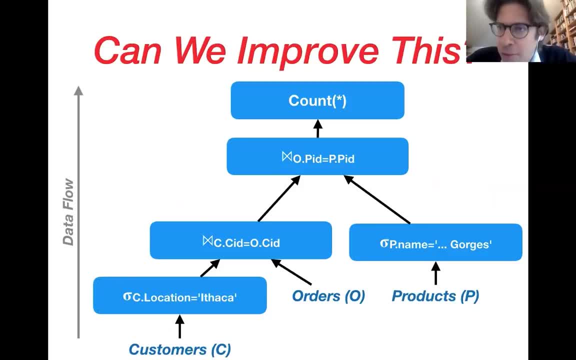 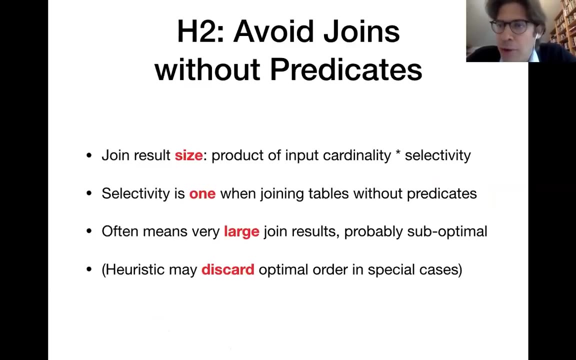 All right, And here we are. So this is how we can improve this example further. We can project out columns early once they become useless. Very good, All right Now. another heuristic that is commonly used is avoiding joins without join predicates. 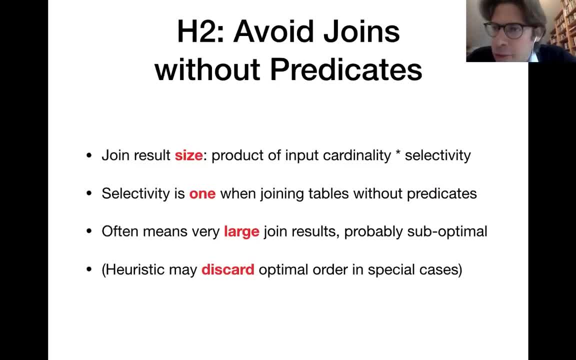 Now, if you need to join a set of tables, then in principle, you have a lot of choices about the order in which you do those different joins, And that means, in particular, you may also decide to join together two tables that are not directly connected by any predicates. 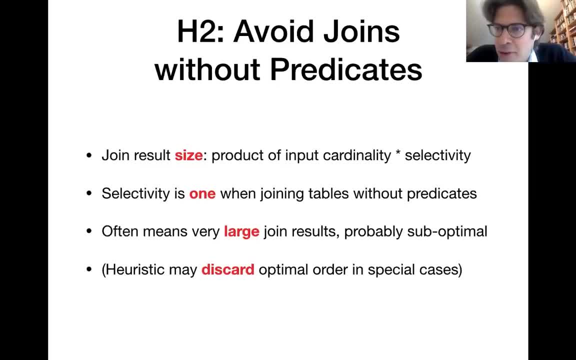 Well, the size of a join result is always the product of the input cardinality values, the number of rows in the two input tables multiplied by the selectivity of the join predicate. And if no join predicate is directly applicable, it means that you have a selectivity of one. 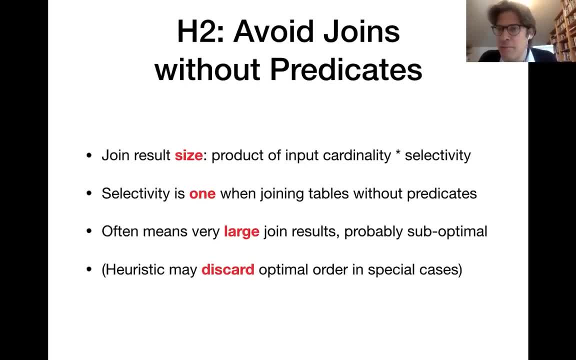 which means that every possible row combination from the input satisfy the empty join condition And therefore you typically get a very large join result and people want to avoid that. This is why typically we do not consider any plans that contain joins with empty join conditions. 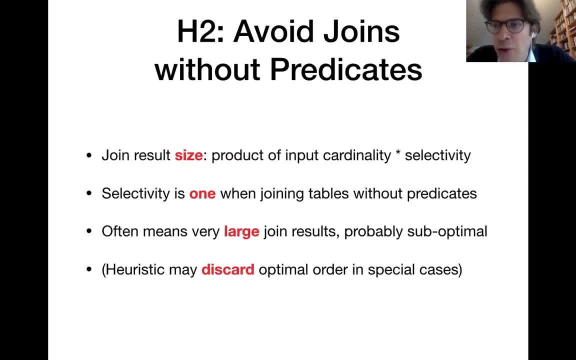 There are some special cases where actually using one of those joints would be optimal. they are rare. that is why this heuristic is used quite frequently in practice, for instance by the postgres optimizer and, typically, you, the plans which pass this heuristic filter. they typically tend to contain: 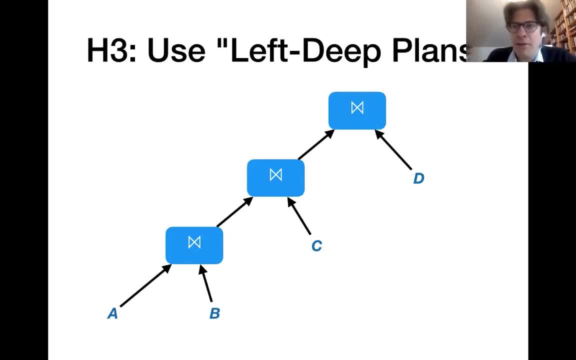 the optimal plan. finally, often- not always, but often- people focus on left deep query plans and a left deep query plan that is illustrated here. you see where the name derives from, because here we are gonna, we're going in deep towards the left, in this plant tree, in this representation. so essentially a 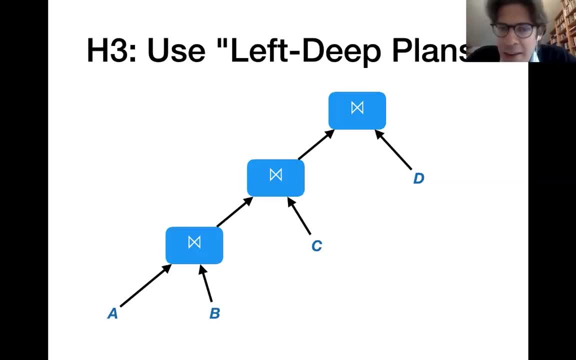 different way of formulating what a left deep plant is would be to say that the right operand of each join in the plan is a base table. so in principle you could also you could join things together and then join a second set of table together and then join those two table sets. 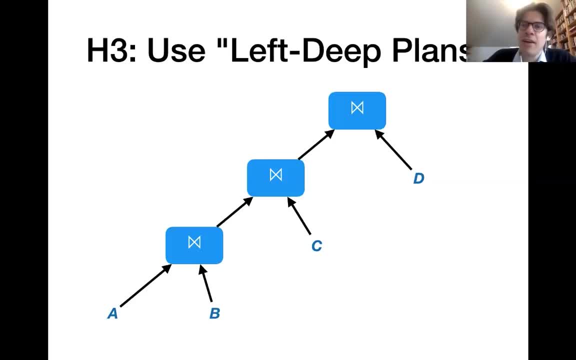 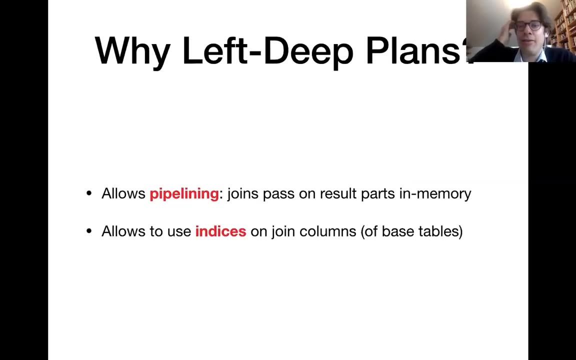 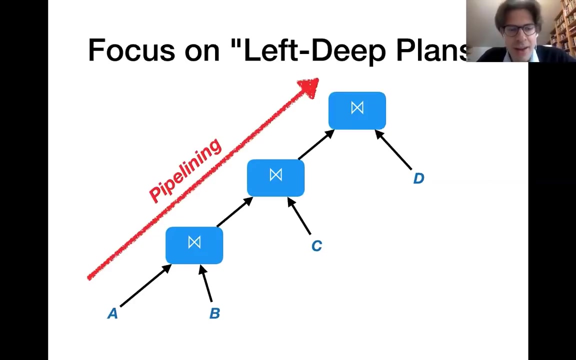 together, that would not be a left deep plan. but if the right operand of each join is a base table, then it is left deep, a query plan. and the motivation for focusing on that specific class of plans, that is a first of all, that it allows easy pipelining, because here, if the if you use, for instance, nested loop, 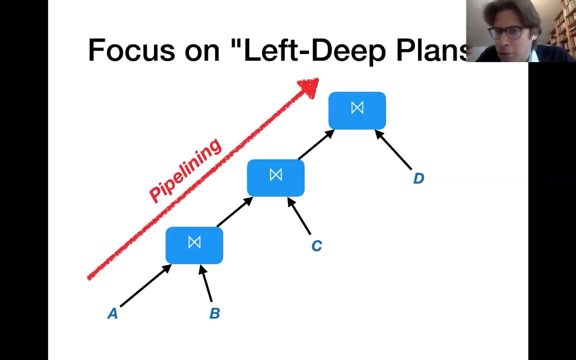 joins, then those joins they can start processing if they're only given some part of the left input which they can read from main memory, and then they produce a part of the output also in main memory, and then they produce a part of the output also in main memory, and then they 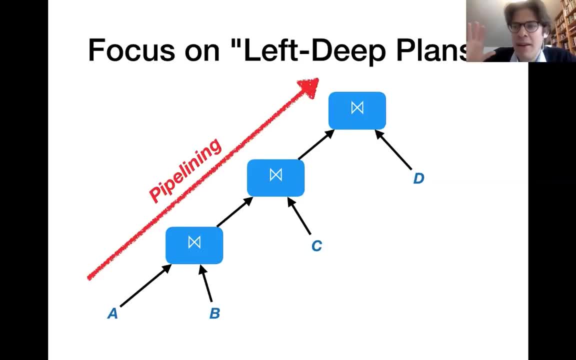 produce a part of the output also in main memory and then they write it into the in-memory input buffer of the next join. so you have a pipeline of multiple joins where you avoid writing intermediate results to hard disk between different join operations and with this lefty plan. 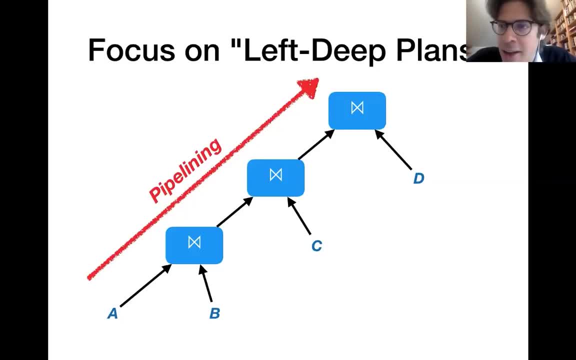 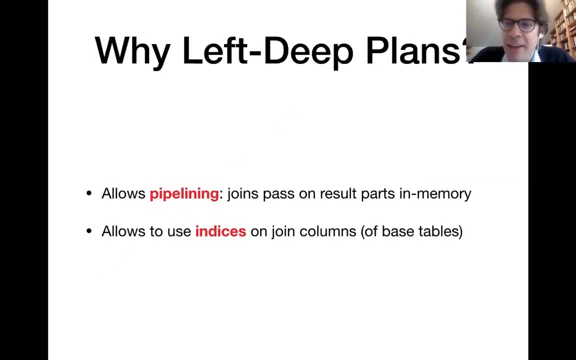 doing that becomes very efficient. the other motivation for using those lefty plans is that also if you have, for instance, created index data structures on columns from the base tables, then you can- as long as you have at least one base table in your joints, you can potentially exploit those. 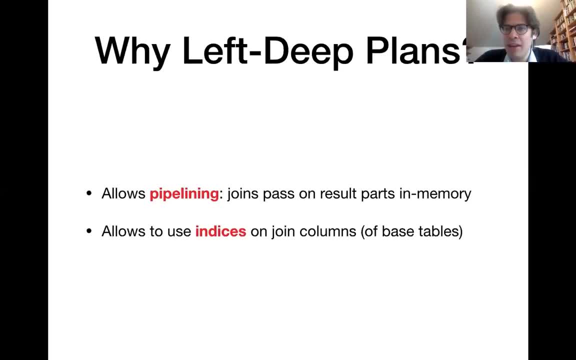 previously generated indexes, if those indexes refer to the joint column and if you have an equality join condition. so for those reasons lefty plans tend to work well. there is a significant less lefty query plans than general query plans, so that also is a heuristic that is frequently used in practice, but not by the Postgres optimizer for 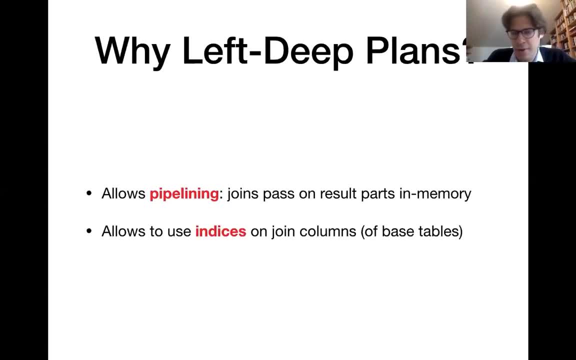 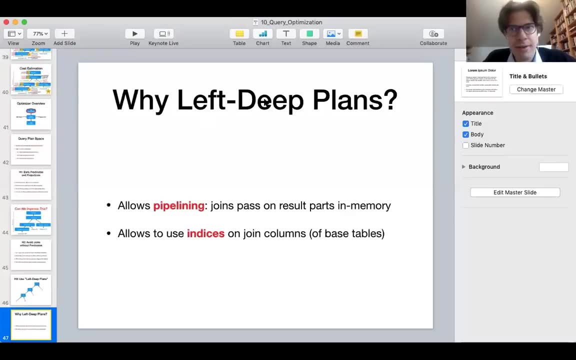 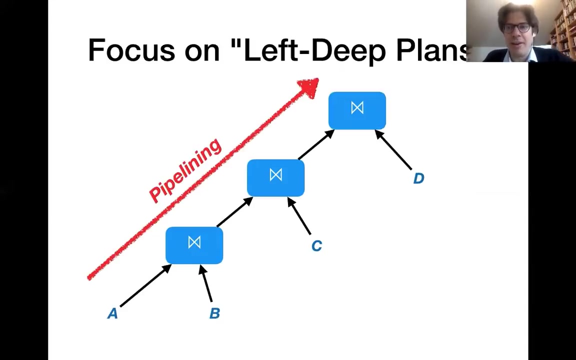 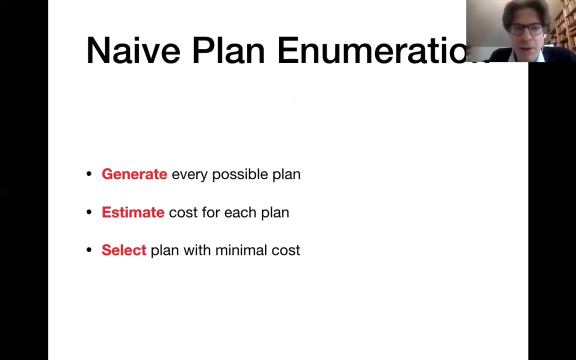 instance- and now I need to advance my slides here. all right, graphical, oh, that's again all right. so this is the reason why people tend to go for lefty- that we want to consider for a given input query, And now we still need to somehow enumerate. 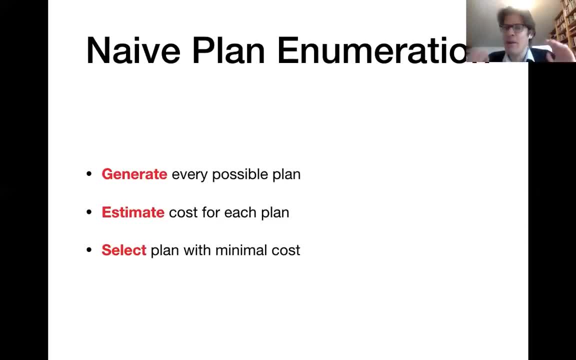 those potential plan candidates and estimate the cost for each of them and then finally select the plan with minimum cost. So at least that would be the naive way of doing things: simply generating all possible plans, then evaluating them according to our cost model and then selecting the minimum one. 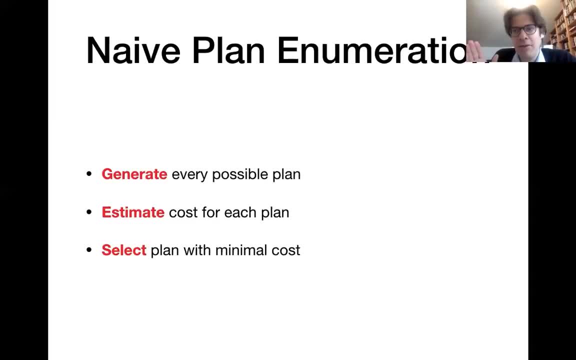 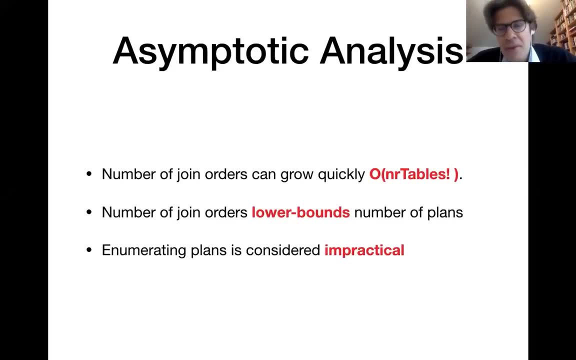 But doing that can actually be quite expensive and there's better way of doing this, as we will see in the following. Now the thing is this: I mean, if you focus on a left deep query plans, then essentially the structure of the plan tree, 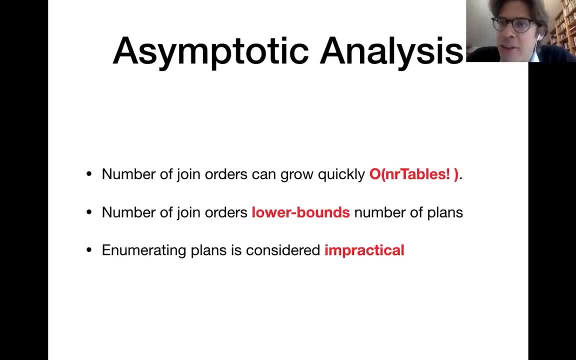 is fixed pretty much, but you still have the choice about the order in which different tables appear in that plan. So, And in the worst case, the number of possible orderings between N tables, that would be N factorial, because you have N choices for the first table. 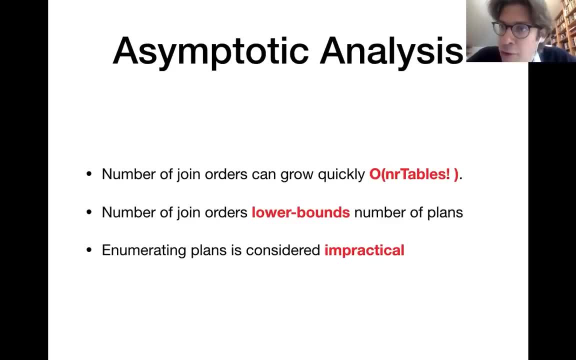 and N, minus one choices for the second table and minus two choices for the third table, and so on, And all those choices they multiply together in order to find the total number of possibilities, And that grows very quickly in the number of input tables. 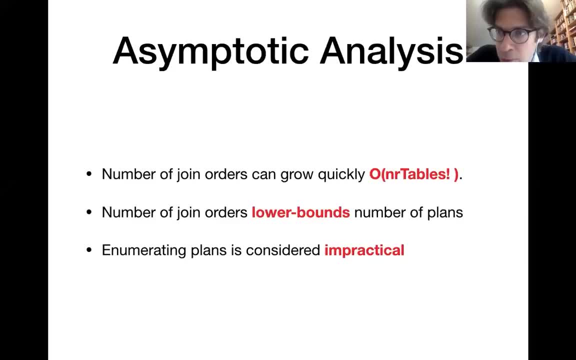 So this complexity is considered highly impractical. If you would try writing a query optimizer which does that, then for most the queries in practice that would not work very well and query optimization would probably take longer than the actual query execution Because that is also on the number of join orderings. 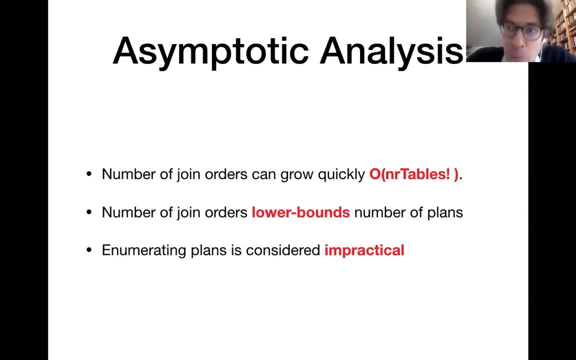 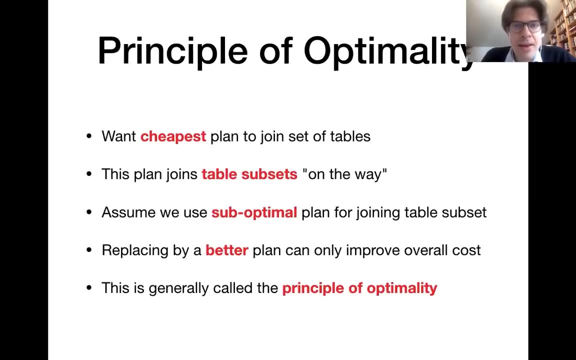 But, as we have discussed, the query optimizer makes more decisions than that. For instance, it also chooses the operator, implementations and all those choices together they form a really large plan space and you don't want to enumerate all possibilities Now. this is why people in practice exploit. 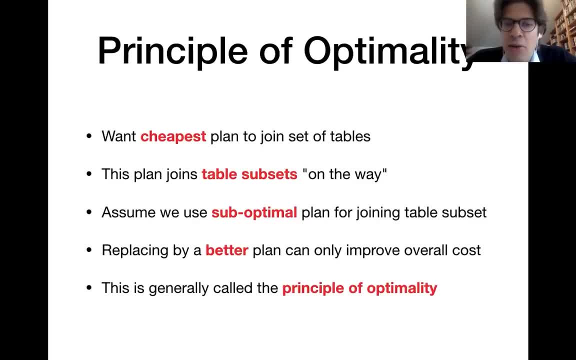 some formal properties of the query optimization problem. In particular, what is useful is the so-called principle of optimality, And that generally means that we can get an optimal solution to a problem by combining optimal solutions to sub-problems And in the context of query optimization. 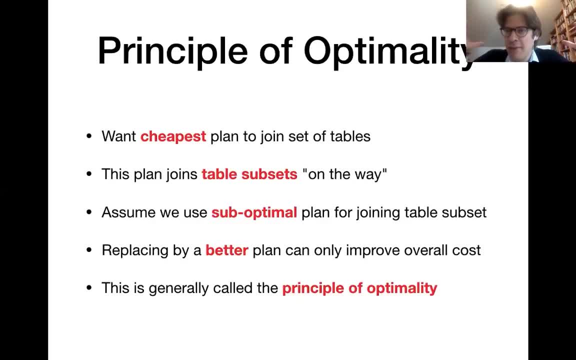 the entire problem is joining a set of table efficiently, and the sub-problem would be joining a subset of tables efficiently, And the principle of optimality, as I discuss in a little bit more detail next, will essentially tell us that by combining optimal plans, 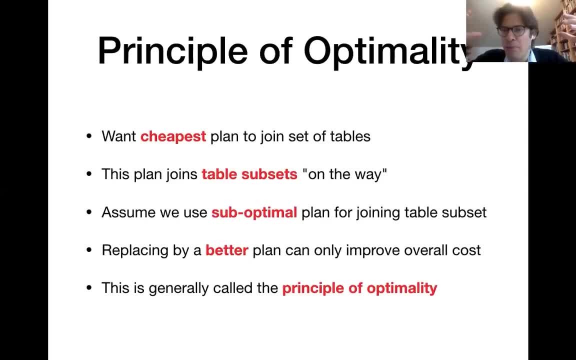 for joining table subsets, we can obtain an optimal solution. So we can obtain an optimal plan for joining the entire set of tables. So in a little bit more detail I'm discussing that now here on that slide. So I mean we generally want to find the cheapest plan. 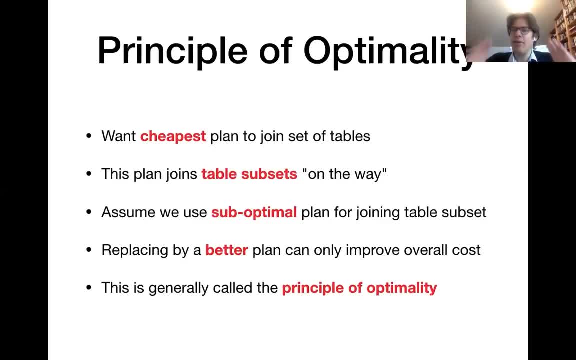 for joining a set of tables, And that means that in order to get there, we have to first join table subsets, on the way to the full join, so to speak. And if you think about it, you could find that even if you had a set of tables- and you had a set of tables- 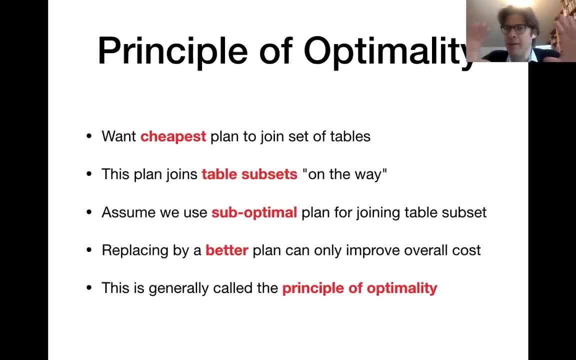 you could find a set of tables and you could find a set of tables. If you have a plan which first joins a table subset and then it joins more tables until it has joined all the tables, then there's no possible motivation to use any suboptimal plan for joining one of those table subsets. 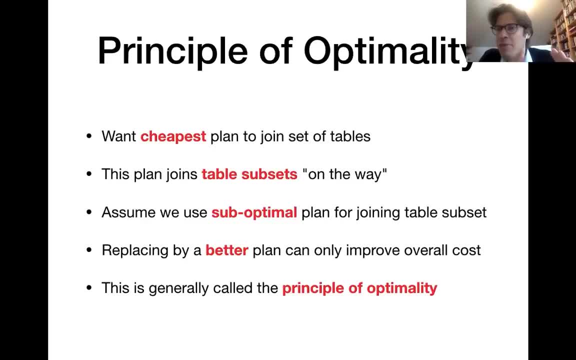 I mean whenever one part of your plan which joins a table subset is suboptimal, you could improve it, meaning to reduce the execution cost, Then there's no way why you would not want to do it. The quality, the execution cost of the overall plan can only improve, meaning decrease as well, by replacing some plan part by a better plan. 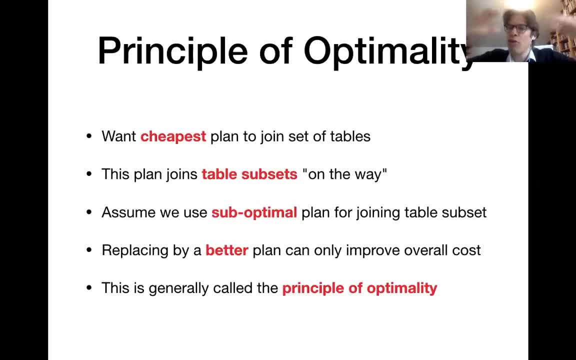 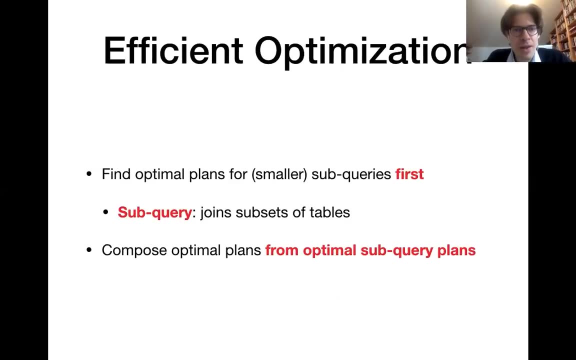 And that is why we can get an optimal solution to the overall problem by composing optimal solutions to subproblems. And this is why the query optimizer typically exploits in order to avoid enumerating all possible plans. All right, So what we generally will do- and I'm going to show illustration on the next slide- that is that we try to find optimal plans for joining subsets of tables first. 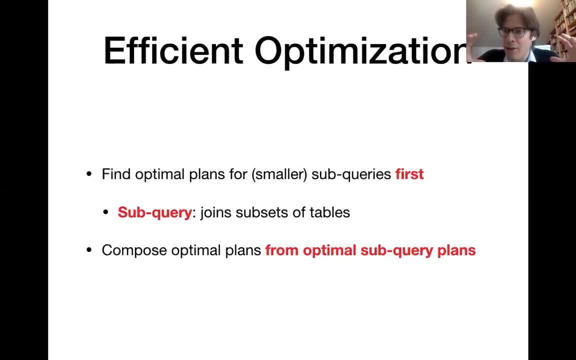 Those like those like the task of joining one of those table subsets that is also called a subquery in the following. All right, And then, after we have created plans for joining those table subsets, We will compose them into larger and larger plans for joining more tables. 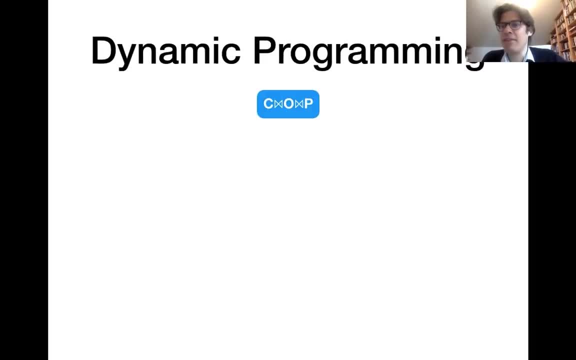 So I'm going to illustrate that process in the following. It is a dynamic programming approach And we start with a set of tables that we want to join, For instance, in our example query. that would be the customers, the orders and the products. 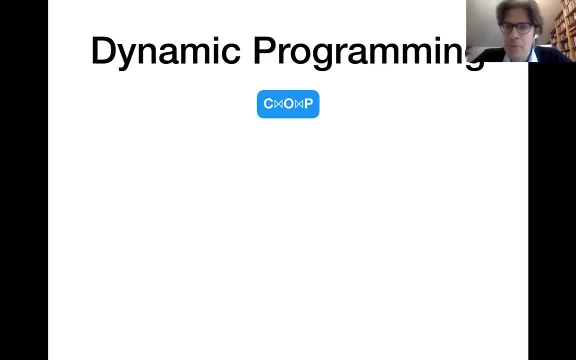 Here you have COP. We want to join that, And in order to join that we first of all have to join the subquery. We want to join two of those tables together, So we can reduce this problem of joining three tables into one of the problems of joining two tables. 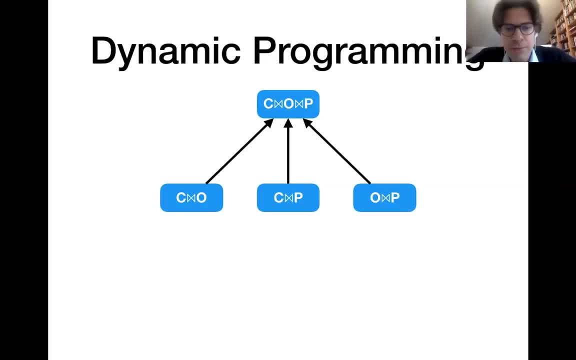 And here there is three possibilities- And also in order to join those two tables, then we essentially decompose the problem of joining two tables into the problem of joining those tables And finding some optimal actions. And then we have access paths for those different tables, meaning deciding whether I want to use an index or whether I do not want to use an index. 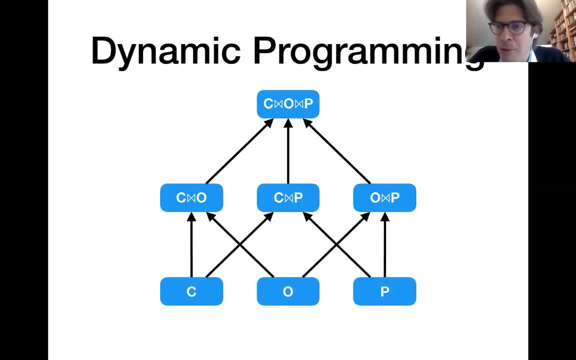 And if I decompose the problem in that way, it motivates the algorithm, the query optimization dynamic programming algorithm that is, for instance, used in the Postgres database system, And this algorithm essentially proceeds in multiple phases. In the first phase, it would consider the optimal way of accessing different tables. 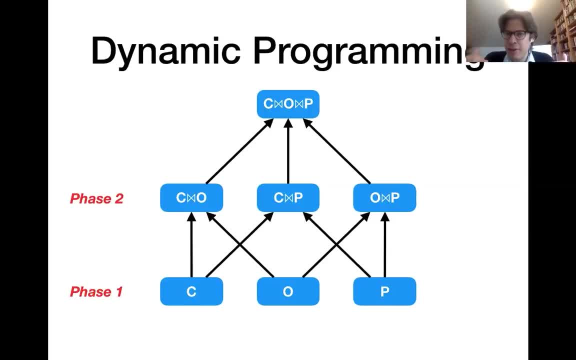 Then in the second phase it would exploit those optimal single table access plans and find optimal ways of joining table paths. So in the actual plan, at execution time we will only make one of those three possible joins. Either we join C with O or C with P or O with P. 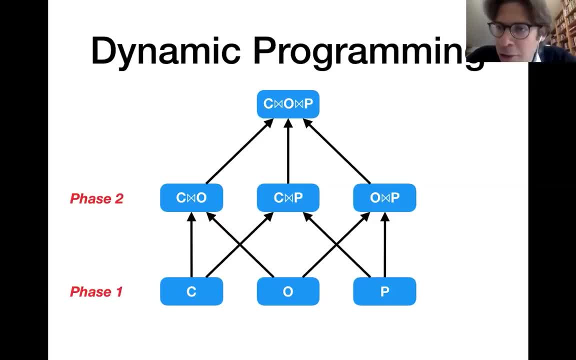 We will only make one of those joins. But here the algorithm needs to consider all three possibilities And for each of those table paths it will calculate the optimal way of generating it by exploiting the previous results, And then finally it will compose the optimal plan for joining all three tables by reusing the optimal plans for joining table paths. 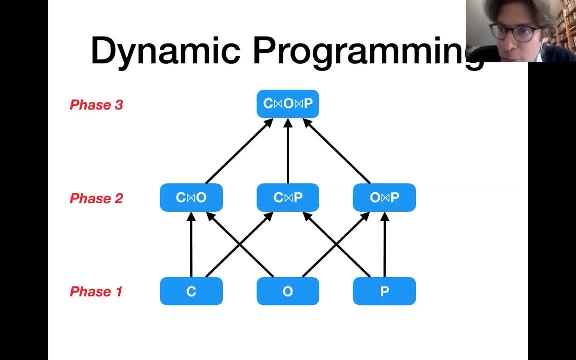 For joining table subsets that it has calculated before. So this is how the algorithm proceeds: It executes multiple phases And in each phase it considers larger table subsets. So in phase number I it will generate optimal plans for joining sets with I tables inside them. 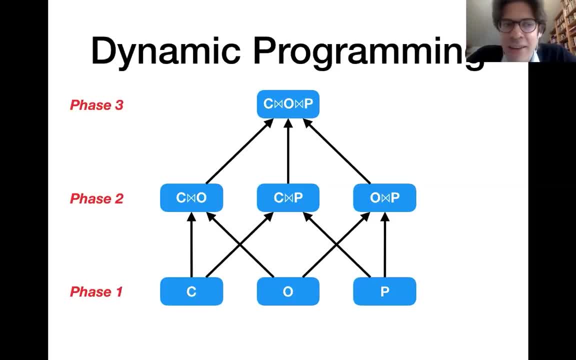 And in order to do that, it will reuse sets for I For joining less than I tables that were generated in previous phases. So that is, on a high level, how query optimization considers different plan candidates And, in order to decide which of them are optimal, it uses cost models such as the ones that we have seen before. 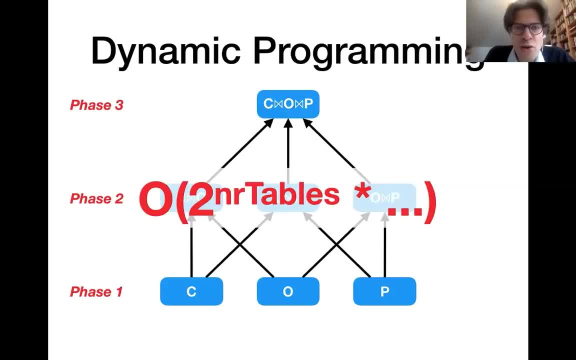 Now, this was a high level overview about query optimization. Oh and yes. Last remark: here We have seen that the complexity for joining N tables is N factorial, And we said that this is impractical. So it is interesting to think about by how much this algorithm reduces those optimization overheads. 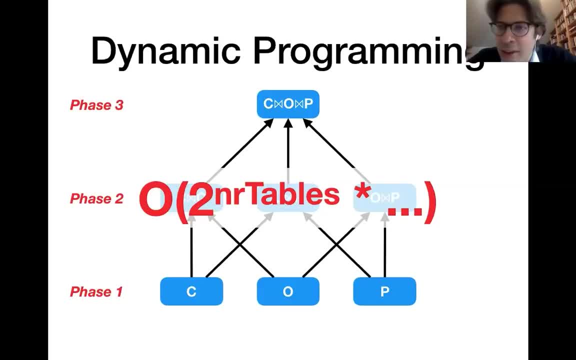 And I'm not going to go into detail here. But if you make the calculations, then, since this algorithm considers all possible table subsets, its complexity is determined mainly by a factor where we essentially account the number of table subsets, And that is not higher than 2, to the power number of tables. 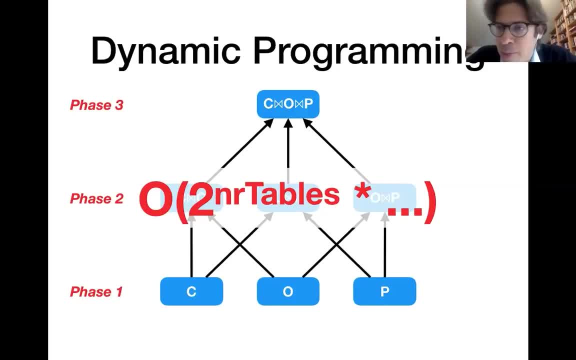 That is the possible number of table subsets, Okay, And this complexity is already significantly better than number of tables factorial, Which we had before for the naive enumeration. So this is why this algorithm is typically used in practice for most queries. Often query optimizers actually have kind of a backup plan. 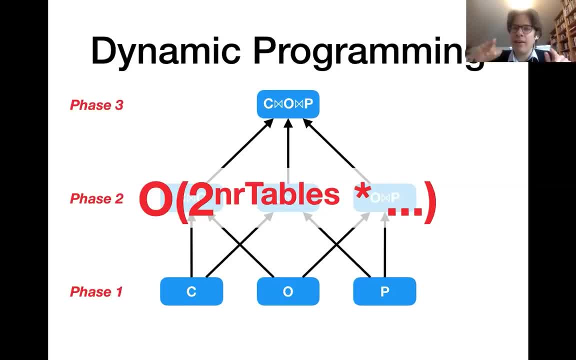 If some really large query comes in, then using this algorithm can still be too inefficient Because, as you see, the complexity might grow quickly as a function of the number of tables. still, And this is why optimizers like Postgres, for instance, 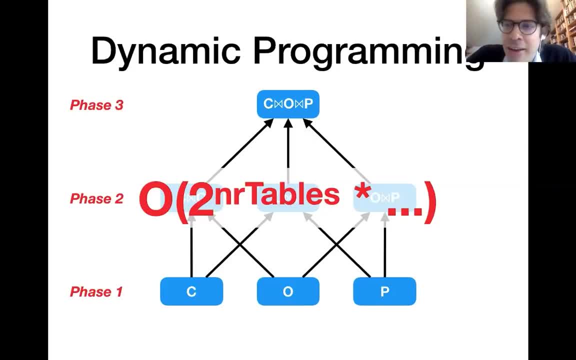 they have a backup optimizer that is using simple randomized algorithms, like a genetic algorithm, for instance, And that optimizer is invoked if the query size exceeds a certain threshold. So by default, for instance in Postgres, it switches to the backup optimizer if you have more than 12 tables. 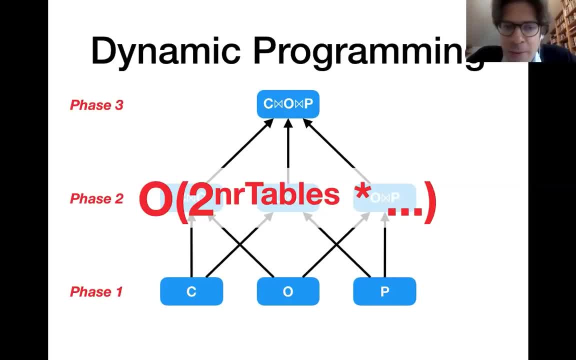 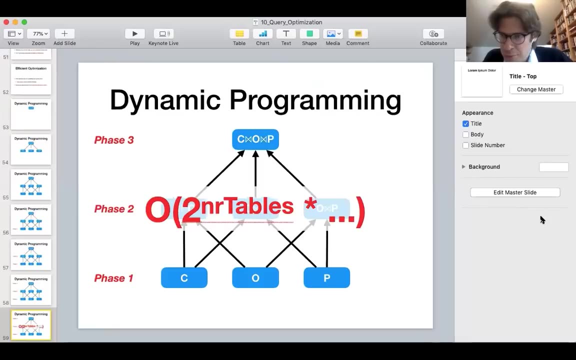 So in the following, I'm going to show you a little bit more about how to see in Postgres what is going on inside the optimizer, And I'm also going to check the chat for whether there are questions. Okay, And that is an interesting question. 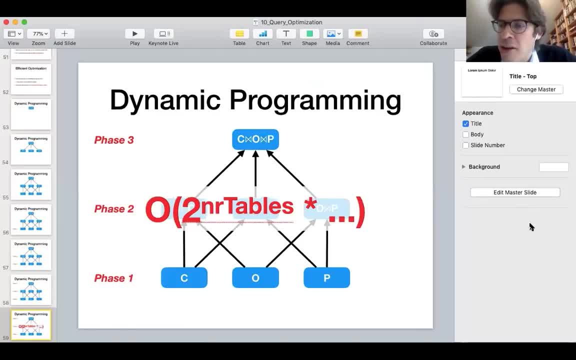 The question is about how the optimizer knows the cardinality of join results without executing the plans. So it does that by using the model that we have seen before, That we are estimating the selectivity of predicates that appear in the query. So it does not assume that everything is a Cartesian product. 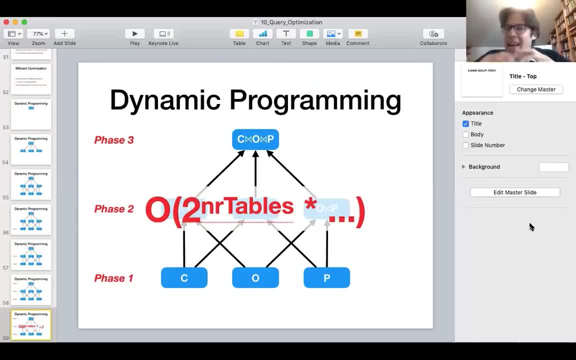 But instead it assumes that you can estimate the selectivity of the different predicates using those simplifying models that we have seen before, based on data statistics and based on constraints such as foreign key constraints. All right, If there are any more questions about query optimization. 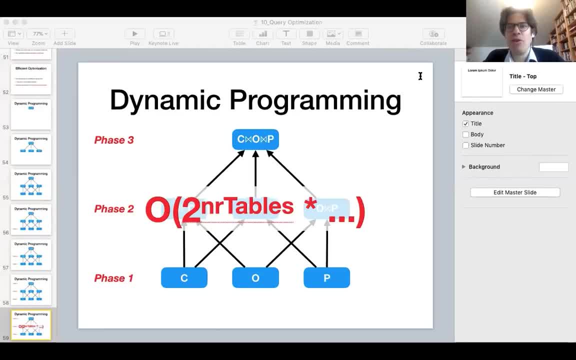 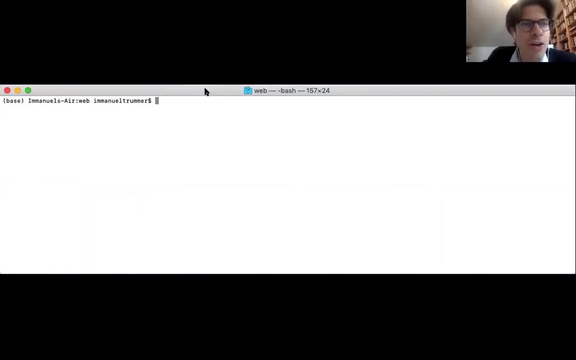 please feel free to put them into the chat. I'm going to give a little demo about the Postgres optimizer And I'm going to have a look here on the chat in case any questions pop up. All right, You should now be able to see my terminal here. 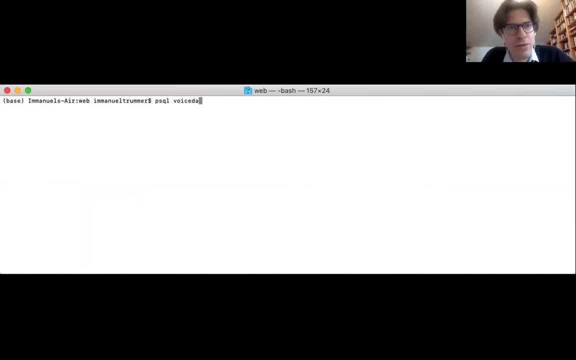 Can everyone see the terminal? If not, then please complain. now. All right, And here I'm using again the database that I have already used in the past. couple of examples: It contains information about the Stack Overflow Developer Survey from 2019,. 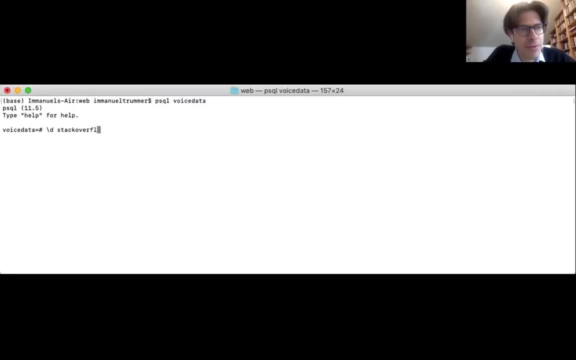 which is stored in this table. here, As you see, there's lots of information about those developers. All right, So in the following I'm going to run a couple of simple queries And by the way, before I start with that, here you see that this command, backslash D, also shows you. 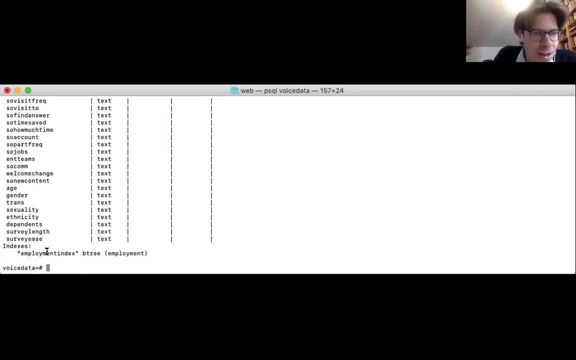 the indexes that you have created. So here I still see the index that you've created during one of our previous examples on indexing. All right, So let's for instance say that I want to narrow down which factors contribute to the salary. 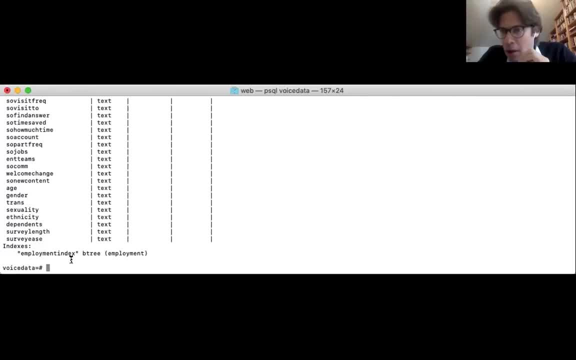 So perhaps I want to compare different developers, perhaps from the same country, to make it more comparable, because different countries have different salary levels been calculated in different ways. They've been calculated in US dollars. So I want to compare developers from different from the same country in terms of their salary. 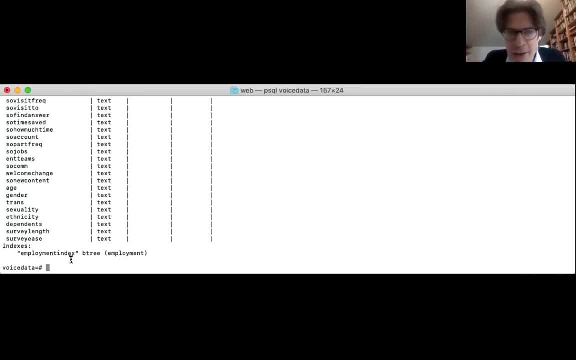 So I could do something like a self-join, meaning I join the Developer Survey table with another copy of the Developer Survey table And I join them together on the country, meaning I want to retrieve pairs of developers from the same country. So let's actually do that here. 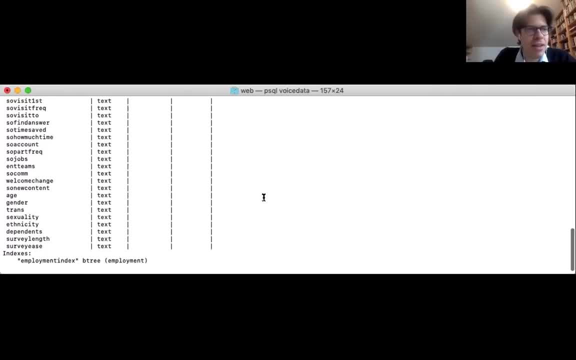 Let's say that we want to be interested in the converted compensation column which we have over here, So that column represents the salary, the yearly salary, calculated in like transformed into US dollar amounts. All right, So here, for instance, If I call the first copy of the StackOverflow table as one, then I could retrieve the associated salary. 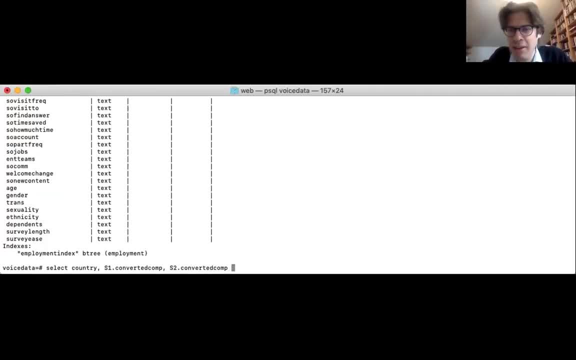 and also the compensation from the second copy. Here, that is the first copy, That is the second copy, And I want to make sure that we have the same country. Actually, I want to make this non-ambiguous. Even here the system might recognize that it doesn't matter because from both copies. 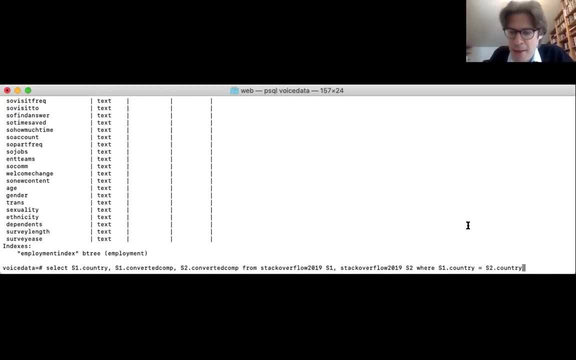 I need to have the same value for the country, All right, So let's do that And execute this query, by the way, is probably not very efficient. I'm not sure whether that finishes quickly, But probably I would want to use a limit clause or something like that in order to reduce the output size. 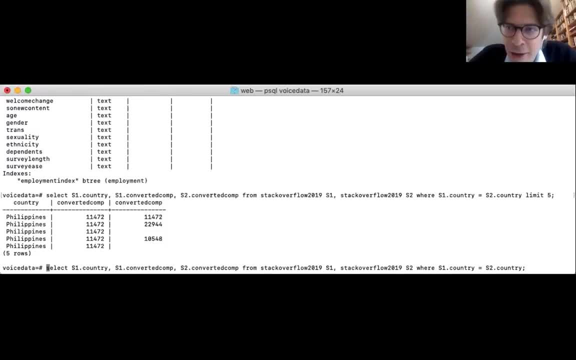 All right. But so the query works And I'm less interested in the result of this query, but more interested in how that query is executed. So in order to find out how Postgres intends to execute a query, we can use the Postgres explain command. 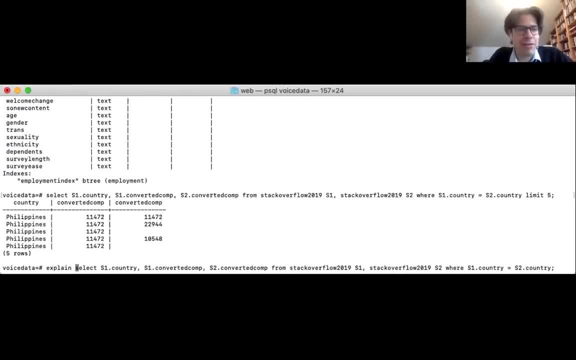 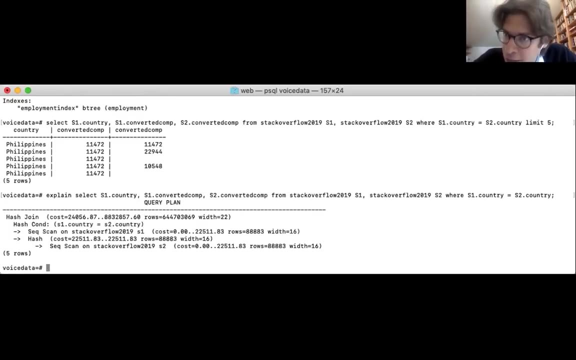 So you just prefix the query with explain, And now the database system will show you the plan according to which it intends to execute the query. So what we have here is a plan which uses a hash join. We have seen the hash join In one of the previous lectures. it's a very popular join for cases with an equality join condition. 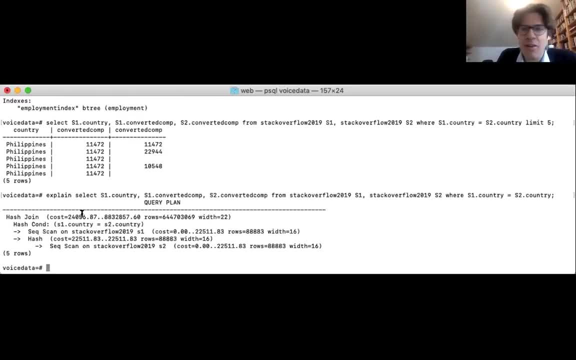 And here, in this query plan, you see all the different steps that the database system plans to execute once we actually submit the query. So it starts with a sequential scan over the stack overflow table And then it builds a hash table, which is here: 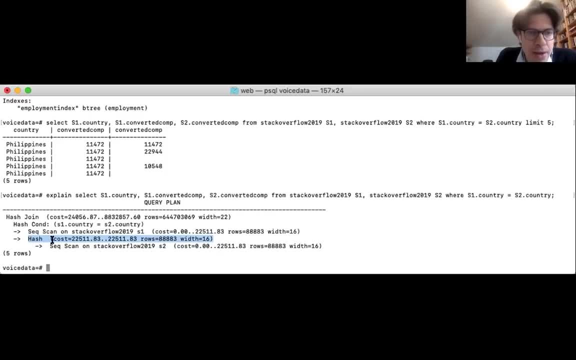 The penultimate row, You see that for each row it generates a multiple estimate. For instance, before we had a question about what the optimizer assumes about a cardinality, And here you see the estimate that the query optimizer generates for the cardinality of the output of the corresponding step. 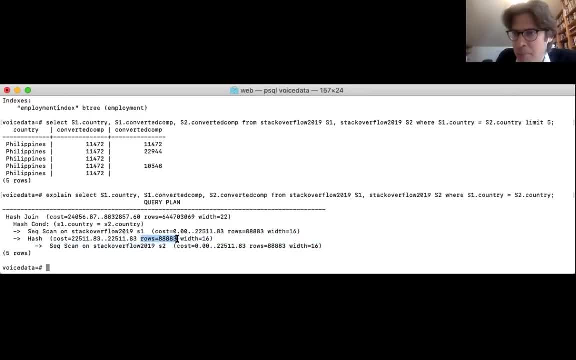 So I assume you probably see what I'm marking up here in the terminal, And if not, I'm talking about the penultimate row in this plan, which starts with the hash, And here we have 888,883 rows And we also have this width estimate which essentially estimates how many bytes we have in each of those rows. 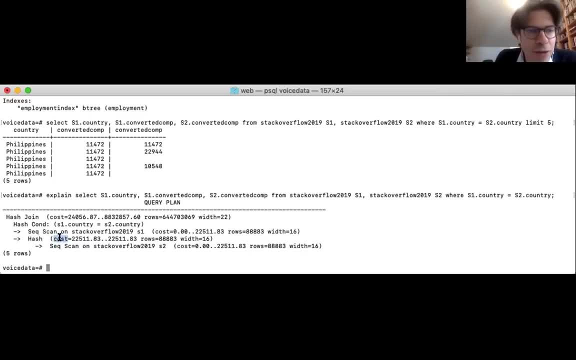 And we have a cost estimate, which is derived from the others, which tells you the estimated execution cost. There's two bounds for the cost. The first bound, that is a startup cost, meaning that is the cost for preparatory. This is the cost of the preparations. 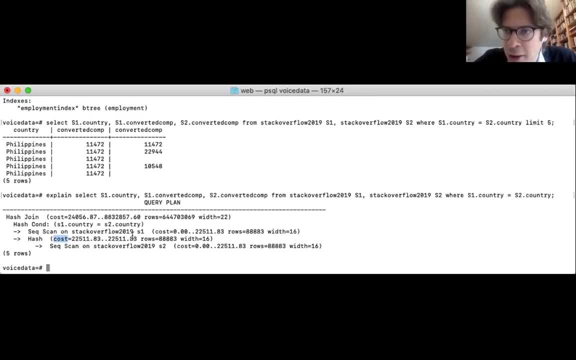 Something like creating a hash table, for instance, is counted as preparation. So this is something that needs to happen Before you can have the first join result tuple. So especially if you are interested not in retrieving the full result but only a part of the result, using, for instance, a limit clause- 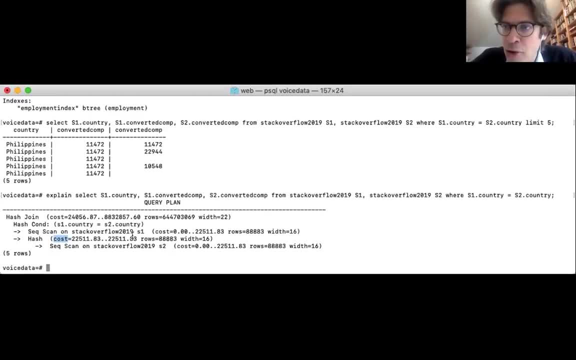 then the first cost component becomes particularly important, because this is the time you have to wait before anything interesting happens. So here we're building the hash table, And then we execute the hash join using the hash join condition. s1.country equals s2.country. 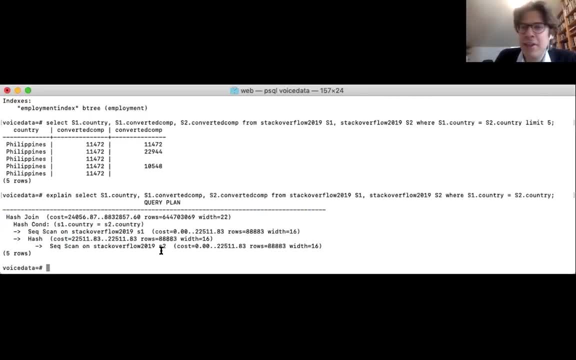 And finally we get a query result. During one of the previous lectures we had a question about whether we can force the database management system to execute queries in a certain way, And I believe I quickly mentioned already that you can at least indirectly force the database system to use certain methods. 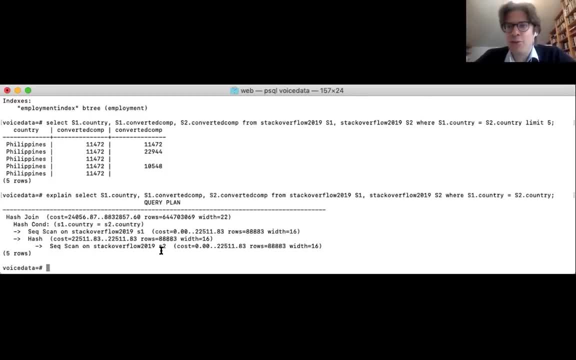 So I can say here that in this case we are currently using a hash join. So perhaps out of curiosity I could see what happens if I disable the hash join. So the database system will not use the hash join anymore, And I can do that with the command that you see here. 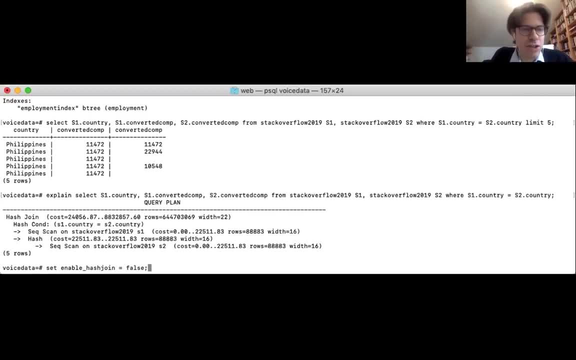 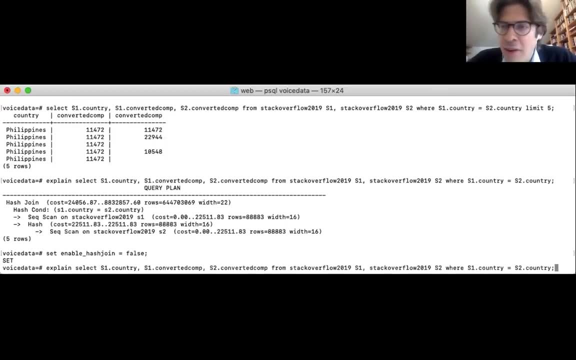 I disable the hash join And if I want to know how the database management system executes my query, executes the query after that. Does anyone have a guess for which join operator we might be using now, If you think back about the join operators that we have seen? 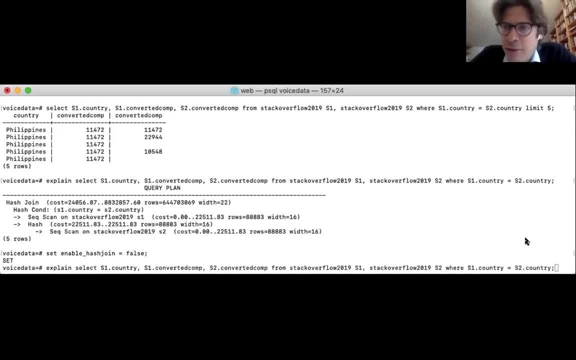 if you consider the type of join condition that we are currently facing, okay, and one possibility would be a block nested loop. that would definitely be possible. Yes, I agree, And perhaps when taking into account that we have an equality join condition, 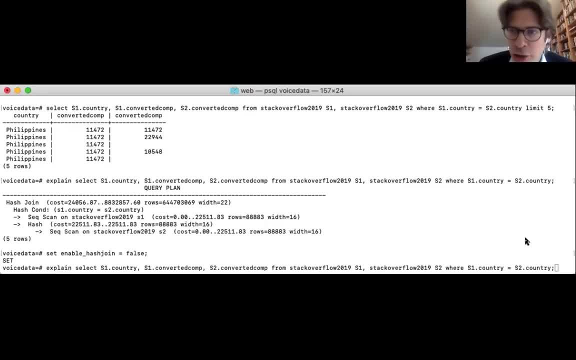 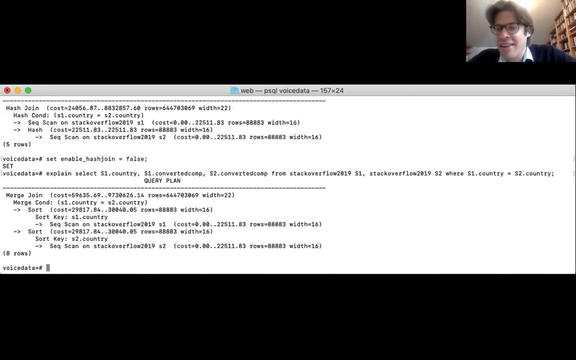 there's another specialized join specifically for the join condition. Very good, yes, very good. Yeah. I see the proposition salt merge join And that seems like a good guess. Let's see what the query optimizer is really using And, as you see, indeed it is using the salt merge join. 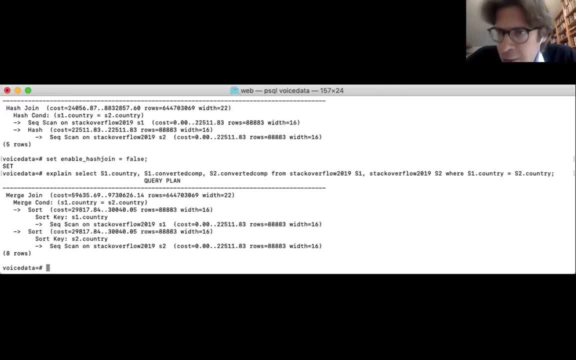 now that the hash join is disabled. So typically if you have equality join conditions, then either salt merge join or hash join probably is most efficient. The advantage of all those block and generally nested loop variants is that they are quite flexible when it comes to. 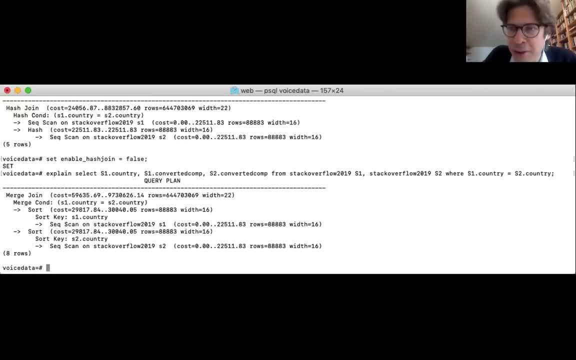 the join condition. So let's actually see what happens if I disable the merge salt merge join as well, And perhaps quickly, I should say a few words about the plan that we have just seen. So here we execute a salt merge join. 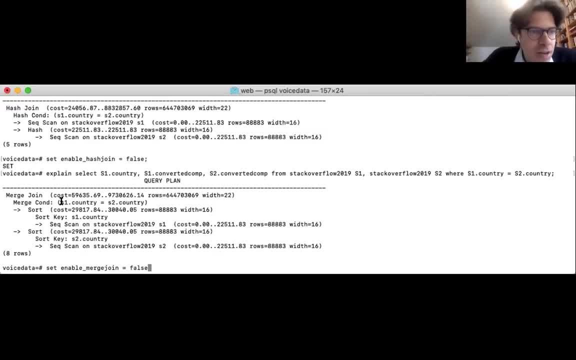 So that means we first of all want to sort the two input tables And as you see here, they're pretty good. The plan shows two salt operations on the input, with the country key over here, And then finally we have the merge join happening. 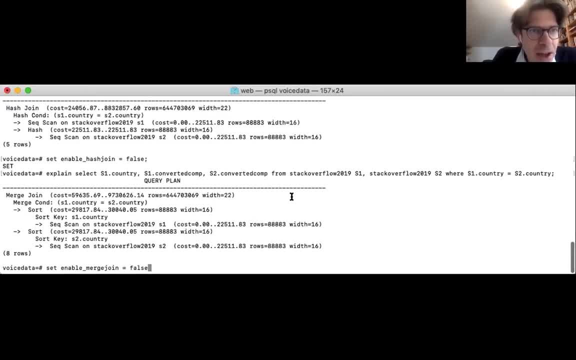 on the sorted inputs And if we compare the cost estimates to the ones from before for the hash join, you see that the total cost- that is the second bound here- was something like eight 1,833,00 rounded. And for the second case, 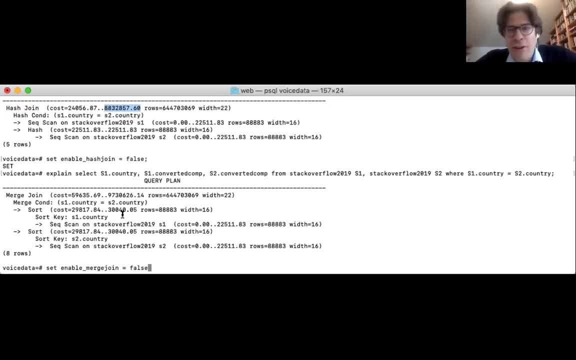 we have 9,731,000 rounded. So here it seems they're close in terms of estimated cost. But the first alternative, the hash join, is at least estimated a little bit cheaper still. That's why the query optimizer prefers the first version. 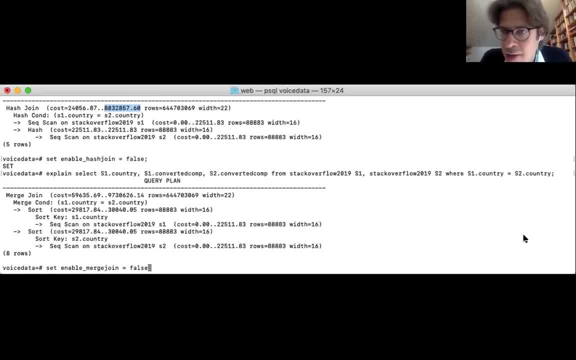 and here we have an excellent question in the chat, very good. so the question is: here we have a query where I'm referencing the same table twice and I'm using the same table for both join inputs and here the join condition is simply equality within one, within one join column. so it absolutely would make. 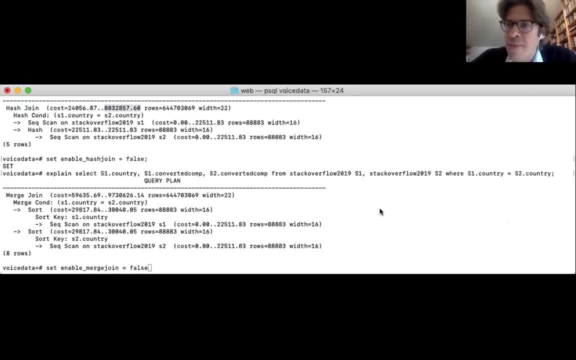 sense intuitively, to essentially sort this table once, then write the sorted version to hard disk and then to use that sorted version order to make the join right. so there is a couple of points, a couple of possible reasons why this might not be happening, but it is a great point and I mean that seems like 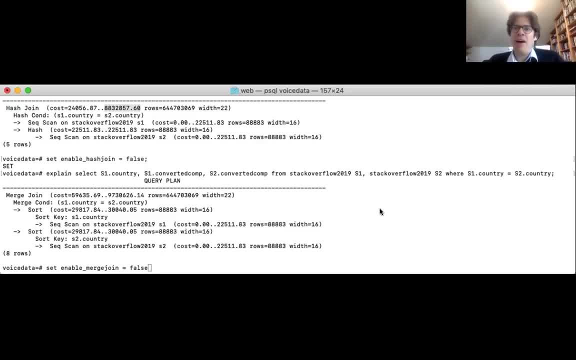 something that might be very efficient. so I mean one a point is that probably in this case there's a certain cost associated with materializing the sorted relation on a hard disk. so here, overall, this is not yet a very large data set, so I could imagine that we are able to fit the sorted version into main. 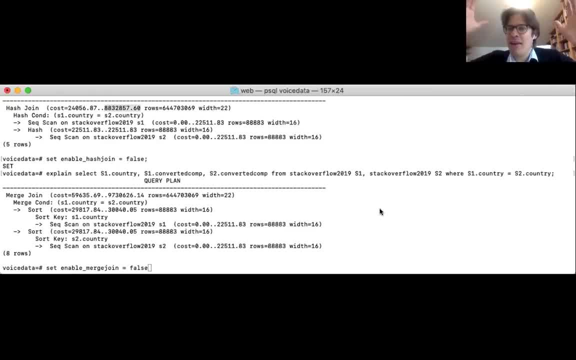 memory. so instead of sorting it and then putting it back to hard disk and then using it for both of the, for both of the, the joint operands, it essentially sorts it in main memory. so you could imagine that even if you sorted in memory, then you could reuse the sorted version for. 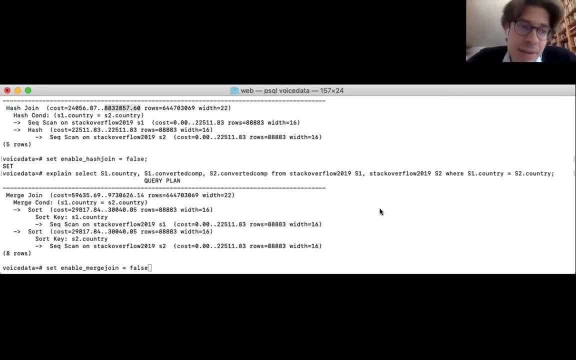 both join inputs. I think that, yeah, I mean that totally makes sense. so here that it would, one would have to analyze why precisely that is not happening. I would assume that the it would be possible to actually sort the sorted version in the memory, but that is not the case. so if I do, 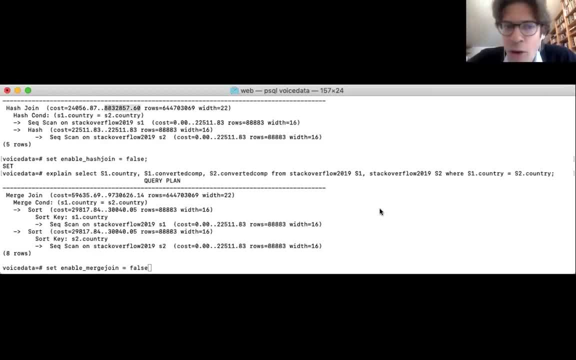 I would have to analyze why precisely that is not happening. I would assume that that here that is simply a limitation of the execution engine that it can efficiently exploit, having, like the sorted version in main memory and using it for the to join operands. yeah, but this is a great question and I agree it. 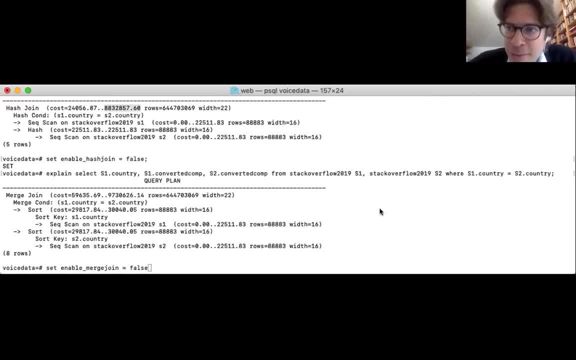 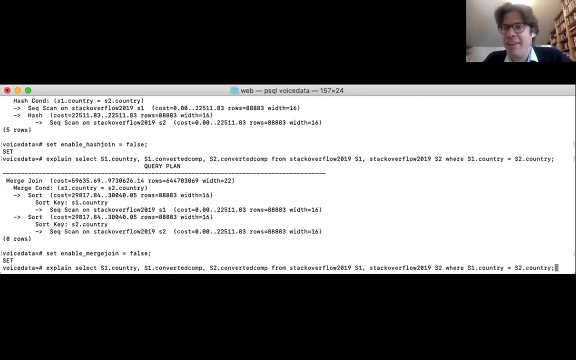 seems like there is some potential for optimizations. very good, all right. nevertheless, let's see what happens if you also disable the sort merge join. and does anyone have a guess for what join operator might be used now? yes, and now the proposition is: practice the dupe join because, thank you, there's. 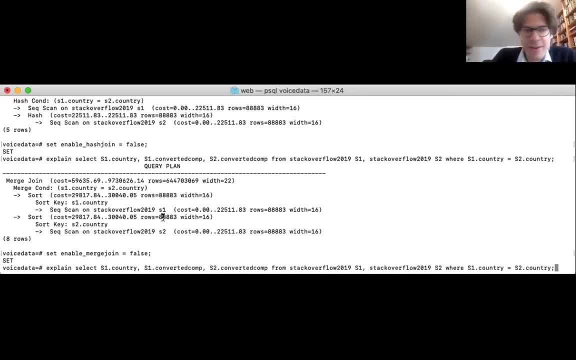 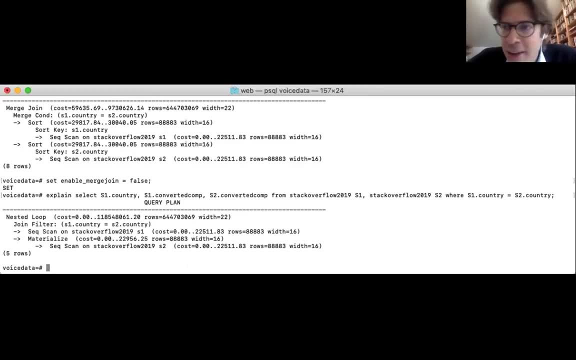 not so much left, at least among the ones that we have discussed so far. so let's see what the query optimizer says. all right, and indeed now we are down to the nested dupe join, so that's the one that we are using here. all right, so here the 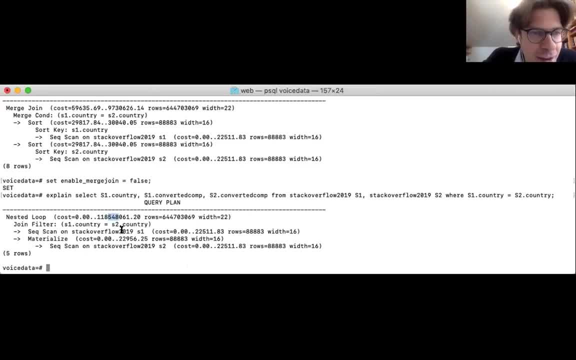 cost is already. the estimated cost is now significantly higher than before, significantly higher than before. so that's the one that we are using here, something around a hundred and nineteen a million. and, by the way, those cost estimates you don't directly map to execution time, so it's a rather abstract. 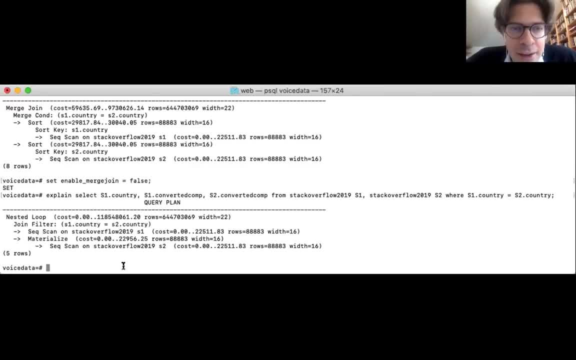 measure of cost, but still the understanding is that the lower the cost, the lower the execution time tends to be. so it's not they. it's not directly possible to calculate to transform this cost estimate into expected execution time, but somehow better plans have lower cost estimates, all right. so now actually let's enable those. 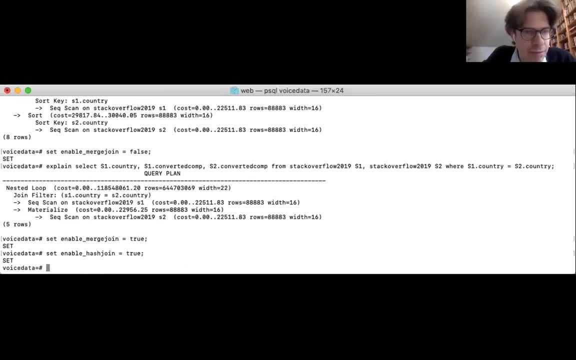 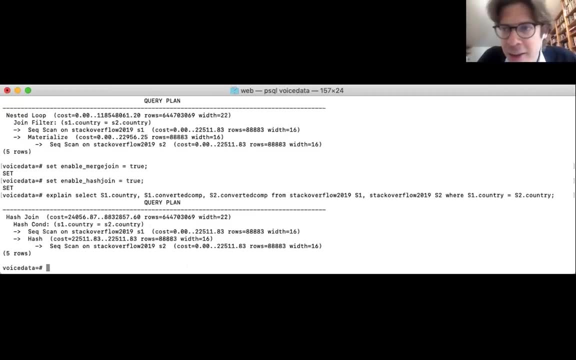 those join algorithms again. now we try it again. then we have the hash join if the optimizer has the free choice. perhaps a wonderful variation of that query here. so we assume that the full reside is a little bit too large, so maybe I just want to get a quick. 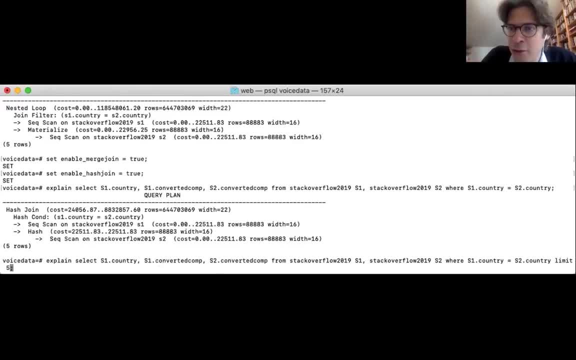 impression for what the reside looks like. so I'm adding the limit goals. does anyone have a guess for which join operator the optimizer might select in this case? we know that without the limit closet this elect the hash join. perhaps it just selects the same one, but doesn't once you reason why we might. 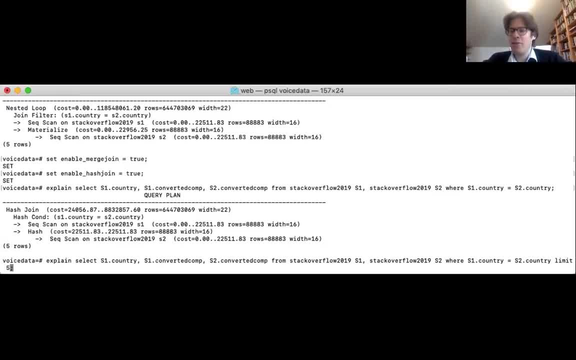 select a different one now. okay, very, very good. ok, yes, very good. so here I see a proposition that perhaps now we want to find only five join resides tuples finally. so It seems possible intuitively to generate those five tuples relatively quickly and It might be disproportional to spend to invest a lot of time into pre-processing. 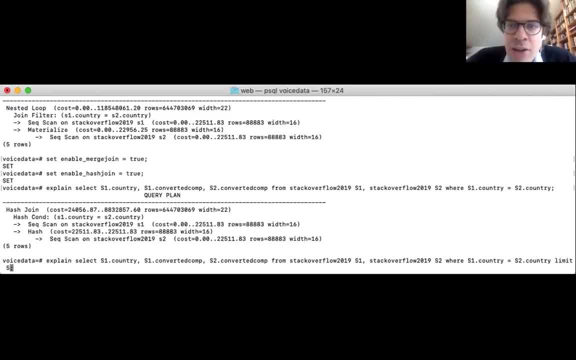 something like creating a big hash table or something like Sorting the entire relation. that might pay off later when doing the actual join and generating the full join result. But if you only want to get the five join result tuples, I probably want to use something with very little pre-processing over it. 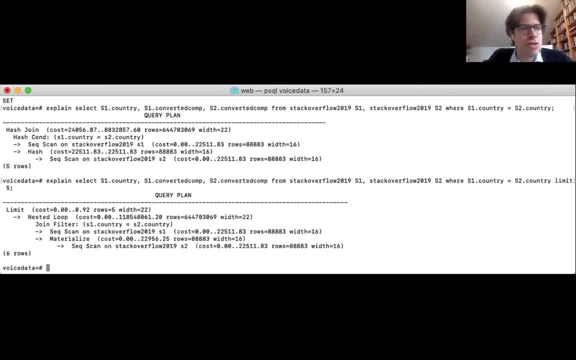 So let's see what the query optimizer actually chooses. and indeed, now that we use the limit clause, It suddenly switches back to the nested loop join, because that one can directly start producing recite tuples without investing time into creating a hash table or sorting things Alright. so this gives you a little impression for how the 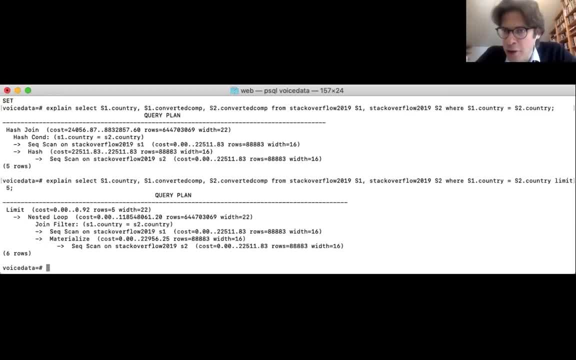 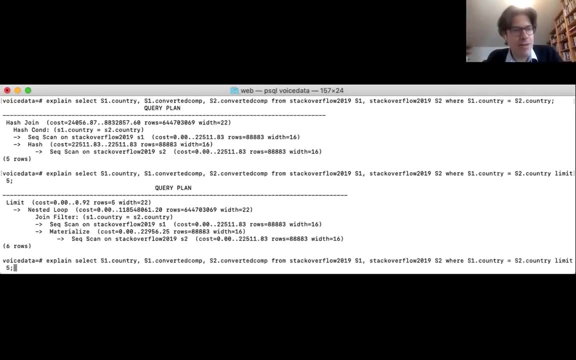 Query optimizer works internally. I encourage you to play with it a little bit. You already had- you probably have written a couple of queries already, So maybe you're interested in seeing which kind of plans the query optimizer Executes internally. and, by the way, one other command that I wanted to show you. we have to explain command. 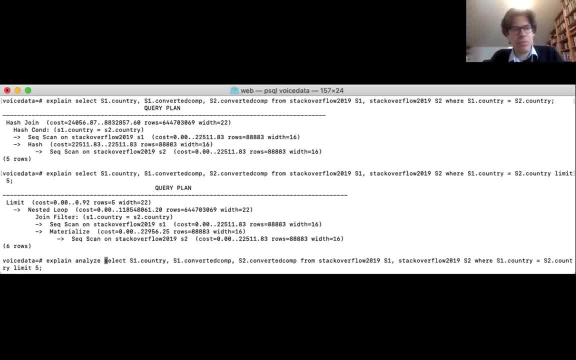 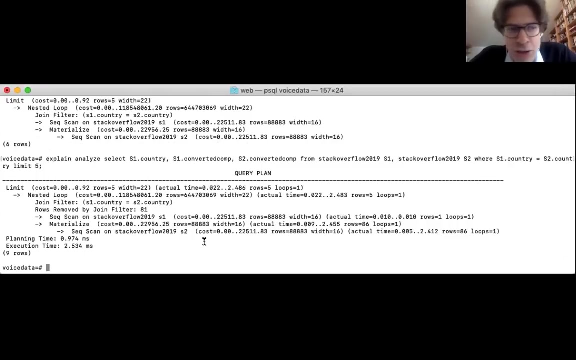 You also have to explain analyze command, And what happens here is that a query optimizer will show you the plan That it executes. it will execute the plan and it will collect statistics and compare those statistics with the original Estimates. so if I, for instance, Do this over here, then you see now at the bottom and getting planning time, which is typically short. 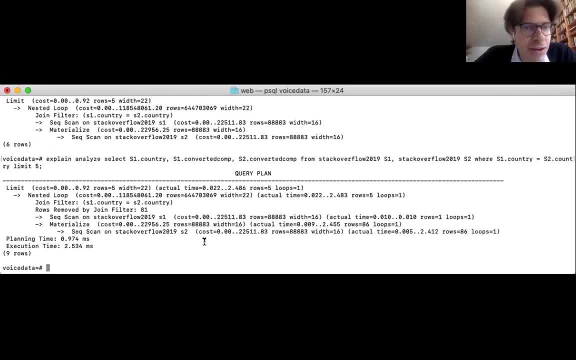 The execution time, which in this case is also a very short, and you still see the query plan on top for each of those steps. in the query plan you see Cost, cardinality and size estimates, and behind that you see actual time rows and loops, Which essentially means here we see how much time it actually. 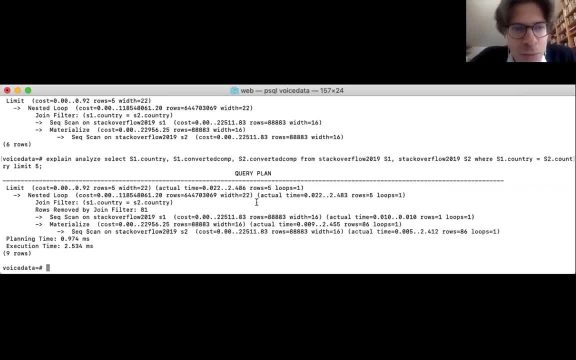 Used for processing and how large the output size actually was. And here, when comparing those two, For instance, They can be. yeah, do you see that the, for instance, like the number of rows, the estimate and the actual number of rows are often significantly Different? not at the very end, though. 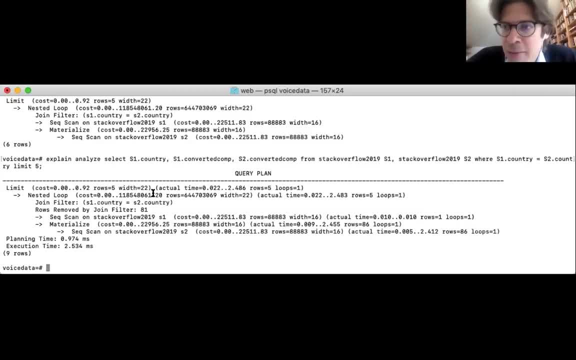 So if you compare that then typically you will see some differences, which means that the estimates by the optimizer- They are not ideal. always make sure to run that vacuum analyze before, during that in this database I already did. but If you run vacuum analyzed and those estimates come closer to reality and still there will be a difference. 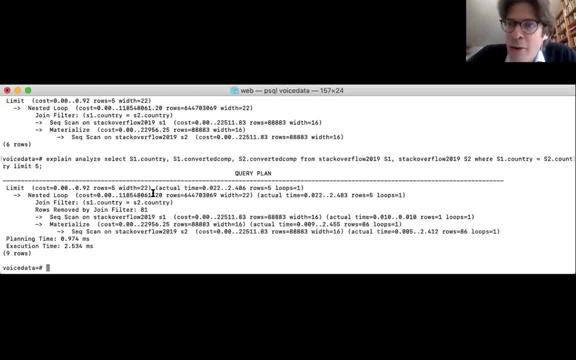 But often in practice, that difference is small enough in order to select at least reasonable query plans. All right, so this was a little Impression for how you can get some insights into how the query optimizer works in practice. All right, let's get started and 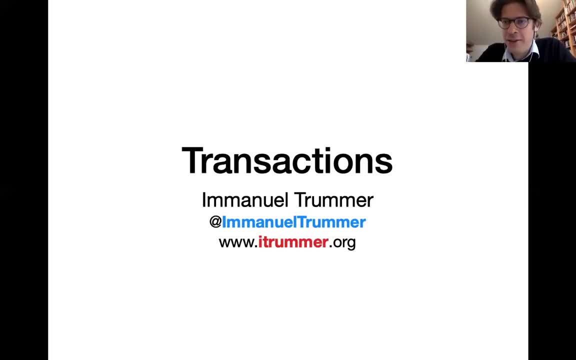 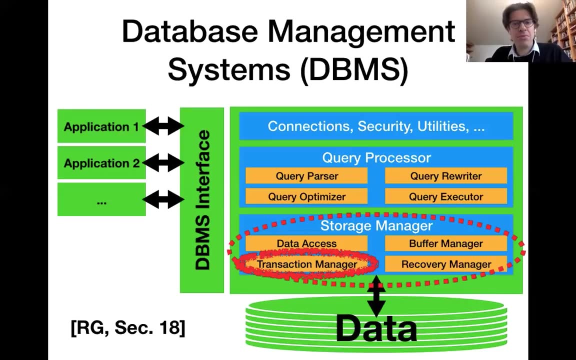 Today we are going to talk about Transactions. have already very quickly introduced a topic in the previous lecture. now we're gonna see the details. So We are going to define what a transaction is in a moment and know already that the components in the database system That are important for transaction processing. 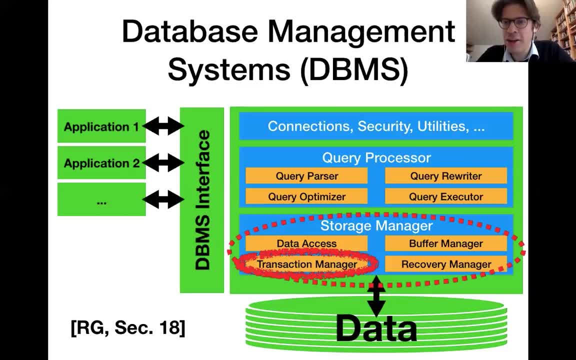 They are mostly located in the storage manager, and here in particular we are focusing on the so-called transaction manager component, but in they all of the other components in a storage manager. they contribute towards making enabling database systems to give all the Guarantees about transactions that we will discuss in more detail in the following. now the relevant chapter in Ramakrishna and Galka: 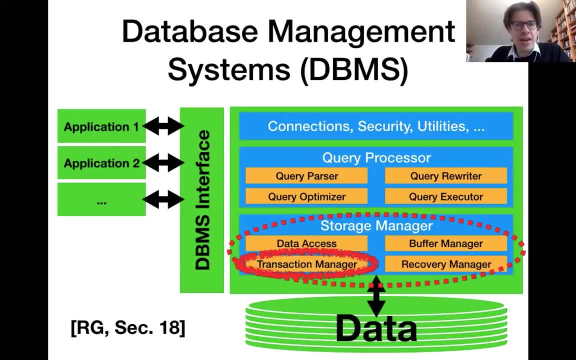 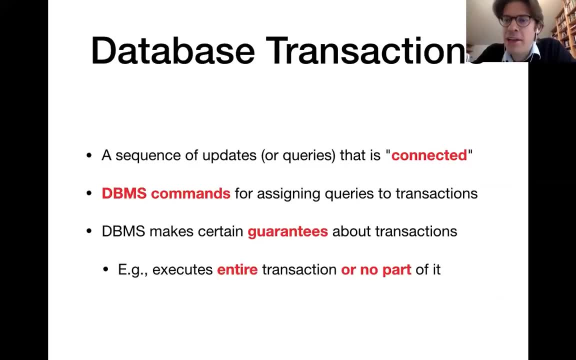 that is chapter number 18, and First of all you're gonna define what a transaction is. So a transaction is generally a sequence of updates and queries that is somewhat semantically Connected and you can tell the database management system that they are connected. You will see corresponding commands, for instance in Postgres and later and once the database system knows. 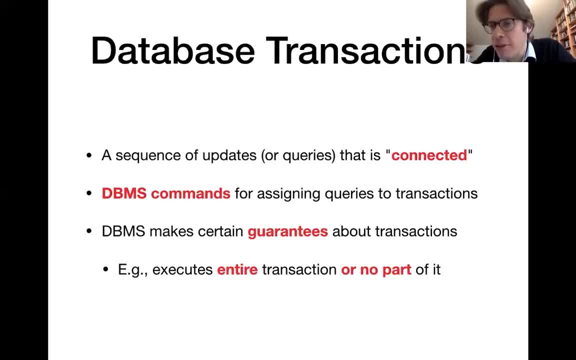 That certain steps belong to the same transaction, then it ensures a certain guarantees. for instance, It makes sure that either all of the steps associated with a transaction are executed or that, no, none of those steps is Executed, so you cannot have situations which only part of your transaction was executed but the other part was not executed. 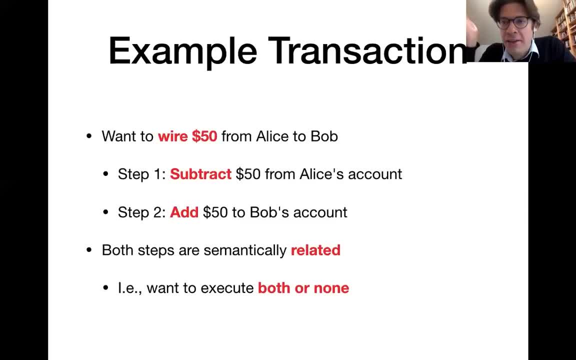 So one example domain which you definitely need transactions, that is banking, and let's start with a very simple example for transaction. Let's simply say we want to transfer $50 from the account of Alice to the account of Bob. So that means we essentially have two writing steps, two updates to the 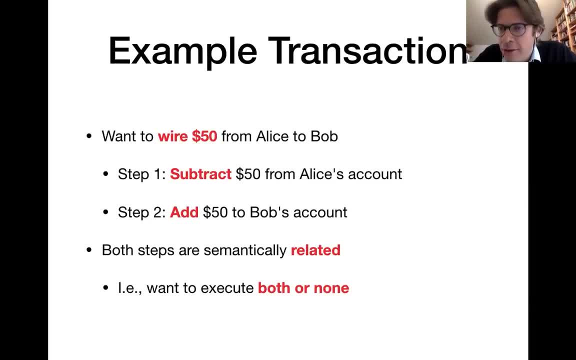 database. First of all we need to subtract $50 from the account of Alice and then we need to add $50 to the account of Bob, and both of those steps are semantically related. so obviously you do not want to execute only one of those two steps, because otherwise, either Bob has not as much money as one should. 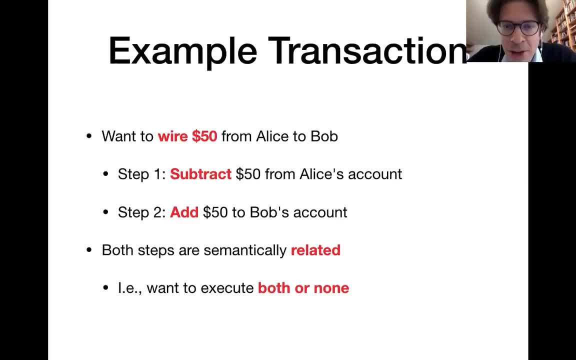 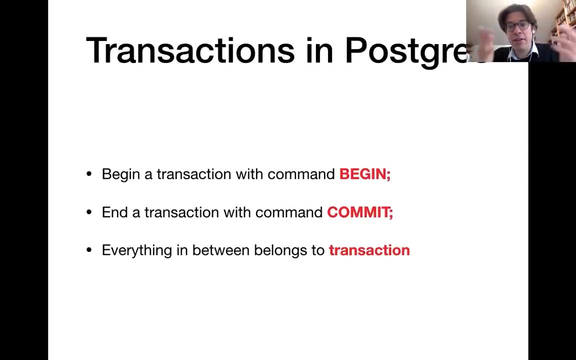 expect or otherwise. both people have more money than they should. So those two steps are semantically linked and you would typically represent them as one transaction to the database system. Now, for instance, in Postgres, In Postgres you can start a transaction with the begin command. then all of the following commands will be considered as: 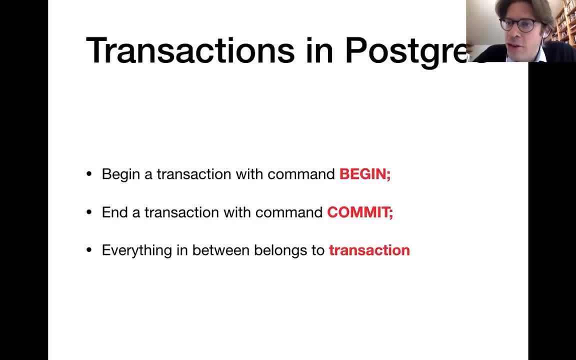 part of that transaction and then, once you have finished all the steps from your transaction, then you can write the commit command. then the database management system knows that this transaction has been finished. it now should be executed. So everything between begin and end is part of the same. 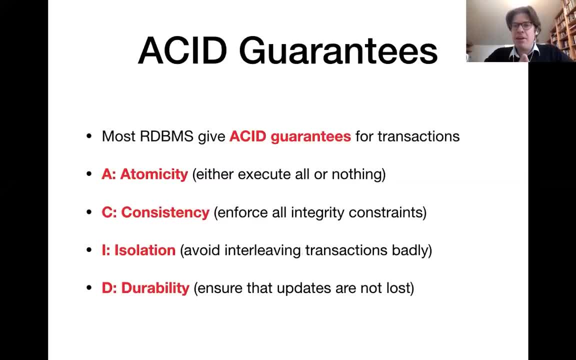 transaction Database management systems. they make the so-called ACID guarantees when it comes to transaction processing, and this acronym abbreviates four important properties In the context of transaction processing. The A, for instance, stands for atomicity, and that means we either execute all of the steps in a 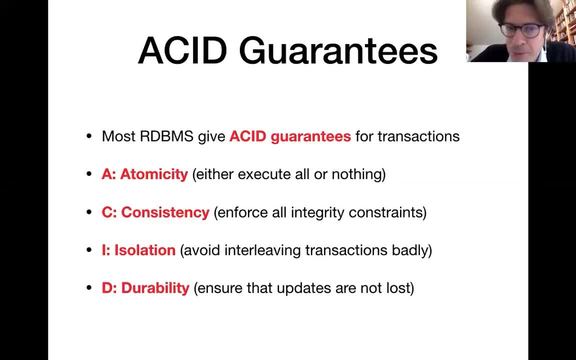 transaction or we execute none of them. There's C for consistency, and here that essentially means that the transaction leaves the database in a consistent state. So all of the constraints on your data will be satisfied, otherwise the transaction is aborted. Now, typically, you have multiple users executing transactions concurrently on. 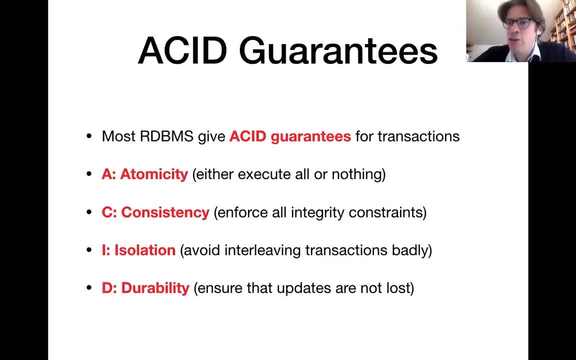 the same database, and then it becomes important to shield one user from the actions of another user, and this is what we mean by isolation, So we make sure that those transactions from different users don't interleave in a bad manner. Finally, we have durability, and that means that once a database system is 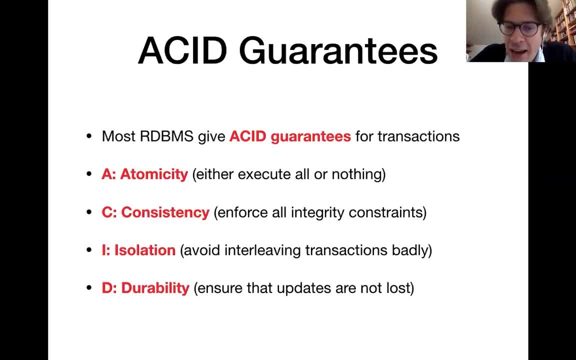 executed, it is guaranteed that the updates by the transaction are never lost, and that includes situations where, for instance, your server suddenly crashes, maybe there's a power outage or something like that, but the database makes sure that it can recover all the updates by a transaction. So this was a short overview, and on the following we're going to see those important properties. 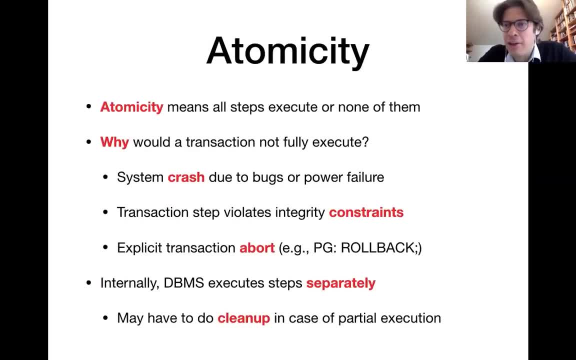 in a little bit more detail, starting with atomicity. and, as I have said before, atomicity generally means that we execute either all of the steps in a transaction or we execute none of them. Now, first of all, why would a transaction not fully execute? There's various reasons, actually. 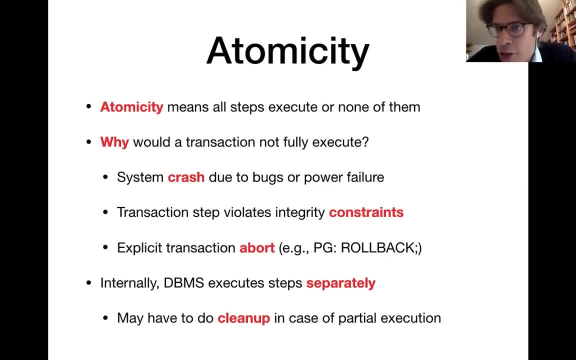 One reason, for instance, is that the system suddenly crashes while it is in the process of executing a transaction. So the reason is that the system suddenly crashes while it is in the process of executing a transaction. So the reason is that the system suddenly crashes while it is in the process of executing a transaction. 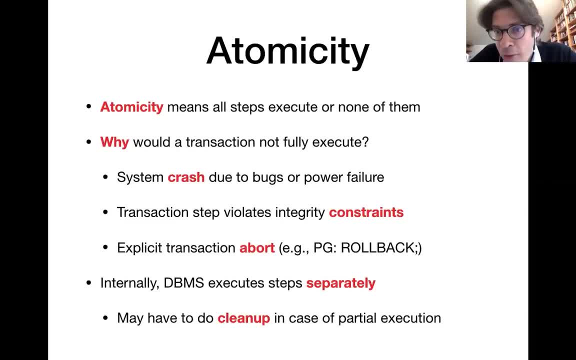 So the reason is that the system suddenly crashes while it is in the process of executing a transaction. Maybe, for instance, there's a software bug, or maybe there's a power failure. Another possibility is that a transaction does not execute because it tries to make an update. 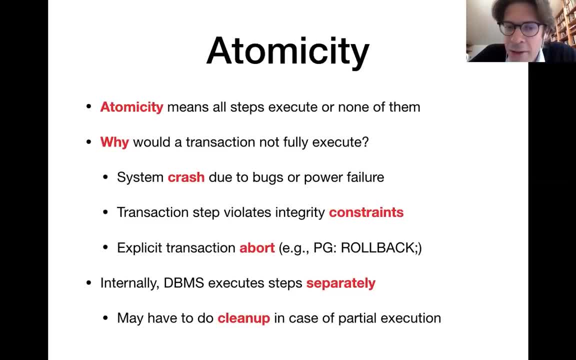 that violates some of the integrity constraints. For instance, it violates a foreign key constraint connecting two tables. Also, you have an explicit command to abort the transactions. For instance, people might use that with a condition around it. So, for instance, if certain conditions are not satisfied, then a transaction is aborted in. 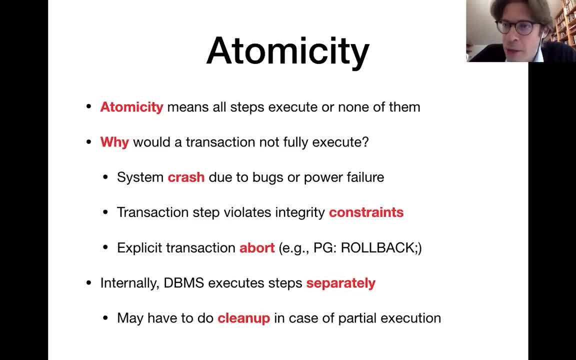 Postgres The corresponding command is called a rollback. Now internally, the database management systems. of course they don't execute the entire transaction in one atomic step, but they execute one step after the other one. So that means if there's really a problem in the transaction. 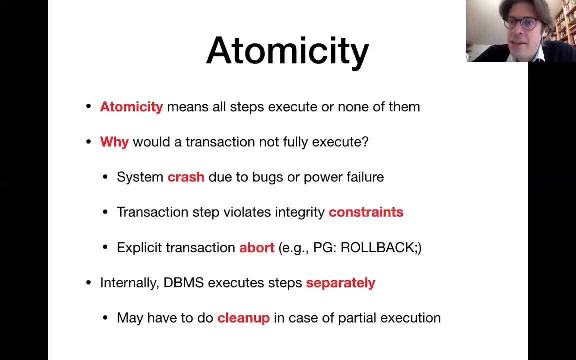 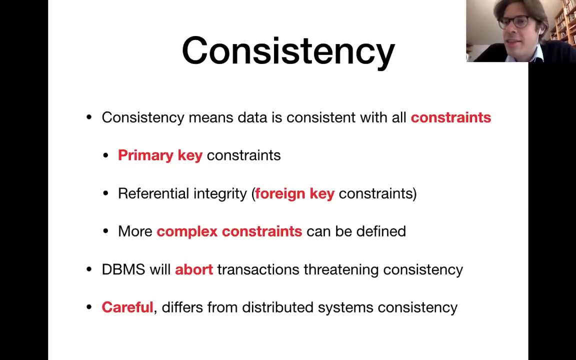 then suddenly it's interrupted. Then internally the database management system actually has to execute a couple of clean-up steps in order to make sure that no partial effects of the transaction are represented in the database. Consistency is about guaranteeing that all integrity constraints on the database are satisfied. 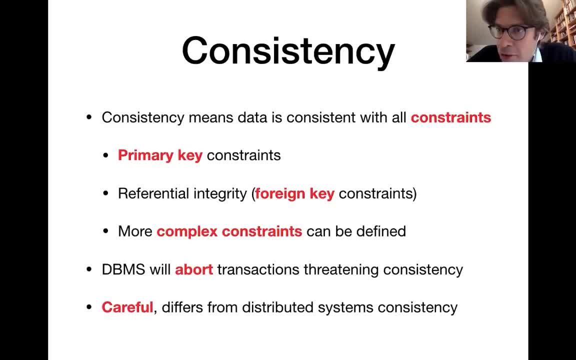 So those constraints include, for instance, primary key constraints, So transactions cannot insert any duplicate values in terms of the primary key columns. We have a foreign key constraints which connect different tables together, And you can also define a more complex constraints And, in general, if a transaction tries to make an update that threatens to violate. 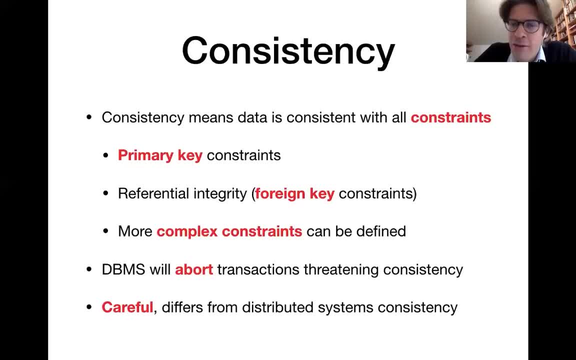 some of those constraints, then a database management system will abort the transaction And there's a little caveat that comes with this term. There's also consistency in the context of distributed systems. You might already have taken corresponding courses, So please be aware that the consistency in the database sense is a little bit different. 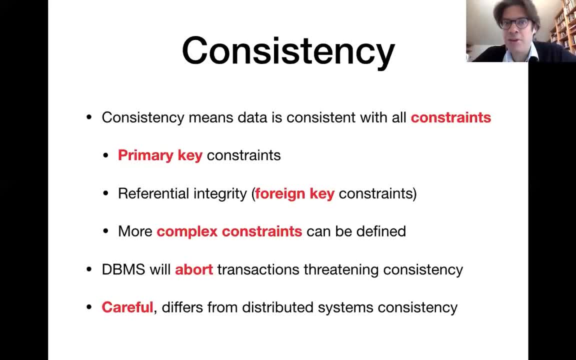 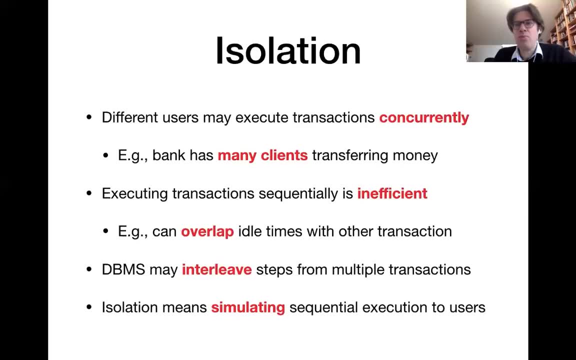 from the consistency in the distributed system sense. So here consistency means that all the constraints in the database are satisfied. Now isolation means that we shield users from the action of other users, which is important because different users typically execute transactions concurrently. For instance, if you have a banking application, then you would typically have many clients. 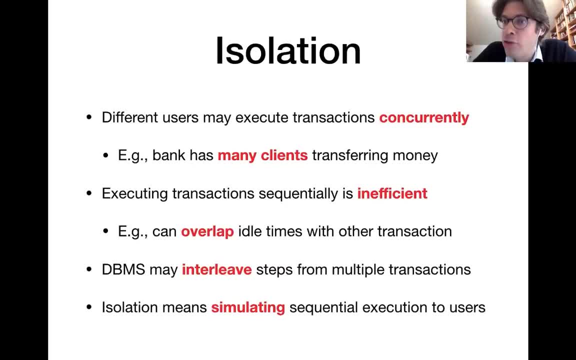 that are trying to transfer money or do other things with their accounts concurrently, So the database system needs to be able to handle that. Now we could, of course, imagine maybe we just keep things simple and we just execute one transaction after the other one. The reason why we're not doing this is performance. 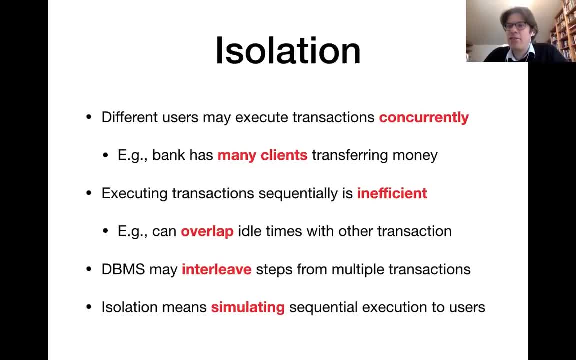 For instance, imagine that one transaction is currently waiting to load data from hard disk. So in general that only takes maybe a couple of milliseconds, But in the context of data processing that is actually a long time. So instead of waiting until the data has loaded from hard disk and keeping the processor idle, 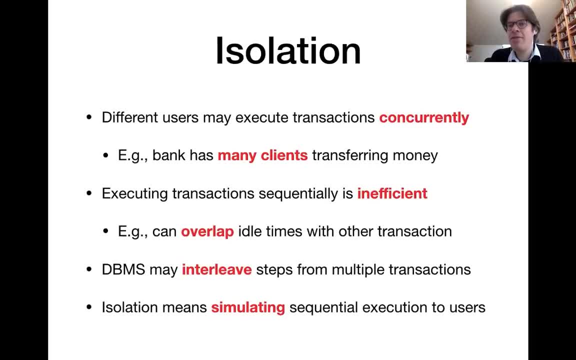 until then, what we could do is that instead, we fit in between a step from a different transaction which executes on data that is currently already in main memory, So the access will be very fast, And doing that can often increase efficiency, so that that motivates us to try to overlap operations from different transactions instead of executing 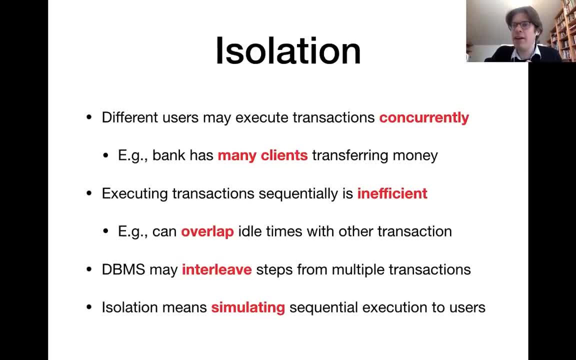 them serially, meaning executing one transaction after the other one. Now, even if we internally interleave the steps of multiple transactions, we don't want users to become aware of that, Because, as a user, if you're writing a transaction, things become very, very complex. if you need to. 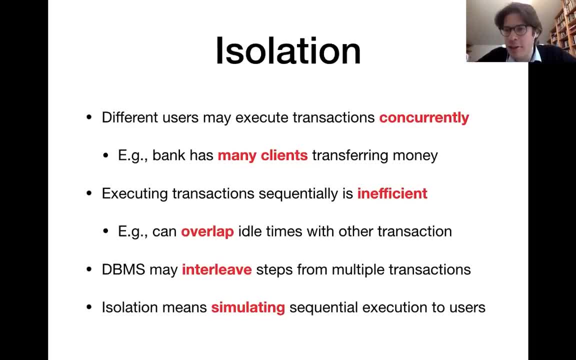 take into account that other users might change the data that you are working on while your transaction is executing. That would become very complex code. So, in order to keep things simple, we want to simulate to users that their transaction executes as the only one in the system currently. 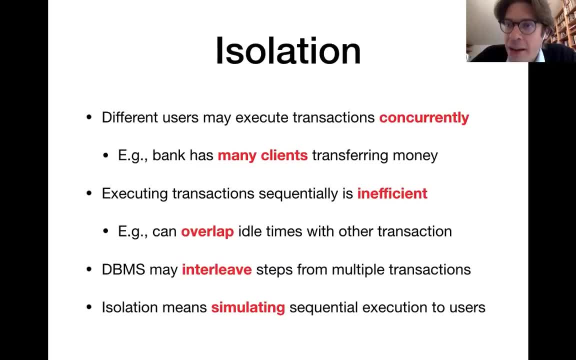 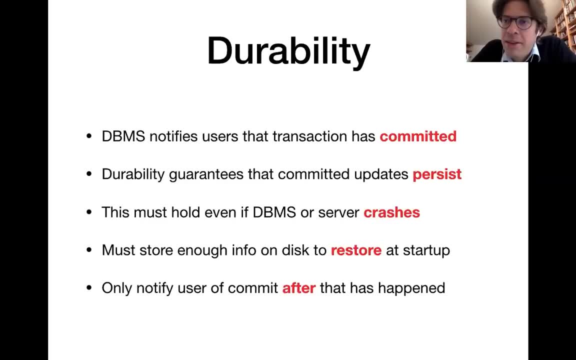 And that guarantee is called isolation. Finally, we have durability, And that means essentially after the database system has told you that your transaction has committed, meaning the execution has finished and everything related to this transaction has been done. At that point, the database system guarantees you that the updates of the transaction will. 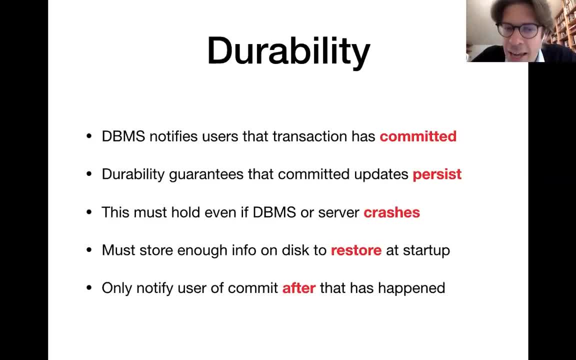 be persistent in the database state And that holds even if we have those crashes, For instance due to power failure. No matter, the database system must guarantee that it can recover all the effects of the transaction before it tells you that a transaction has committed. 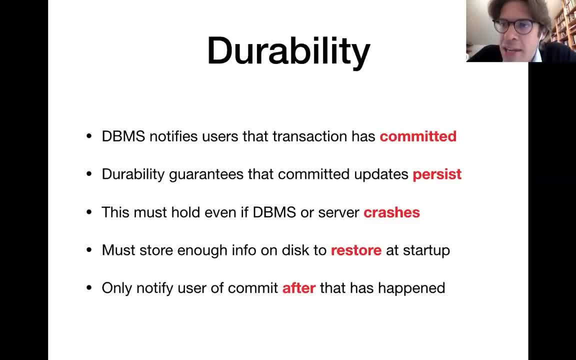 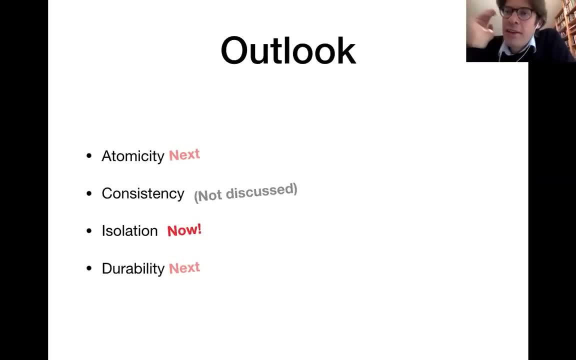 So this guarantee is about keeping your data safe, All right. So those are the four guarantees that database systems typically use And we're going to discuss what we make when it comes to transaction processing- the ACID acronym In the following. we're going to discuss those properties in more detail. 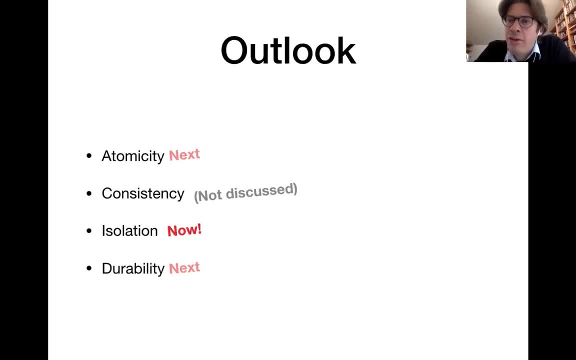 Except for consistency. Consistency is fairly natural to implement. That just means that the database system checks all the constraints and aborts transactions if they don't satisfy them. So we're not going to discuss that in more detail, but we are going to discuss about. 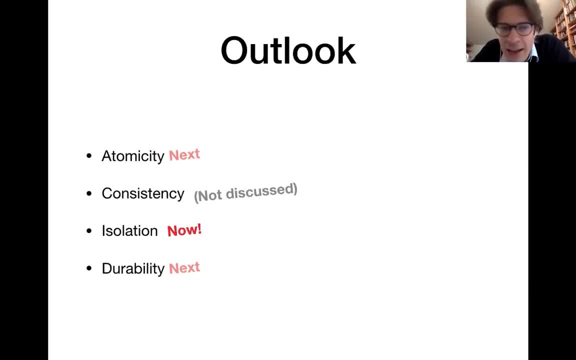 isolation. now in the coming slide deck And in the later lectures we will discuss about atomicity and durability. So in the following we're going to first of all discuss about the isolation guarantee, where we shield users from the actions of other users. 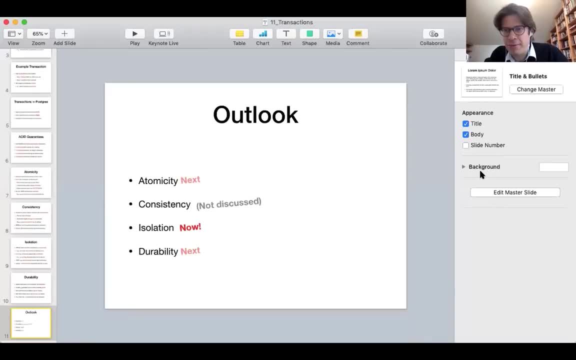 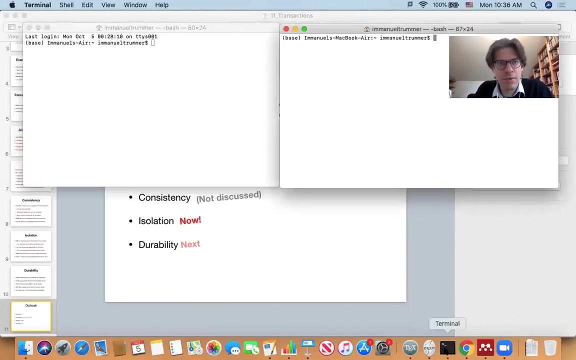 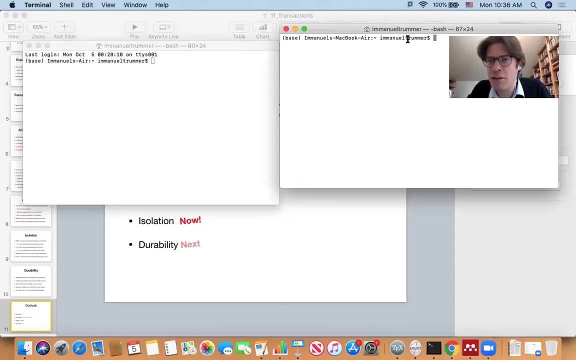 All right, And I have a little demo For you. So For the, For the, For showing the effects of isolation. Prepare that All right. Okay, So now you should be able to see my screen: The, The. 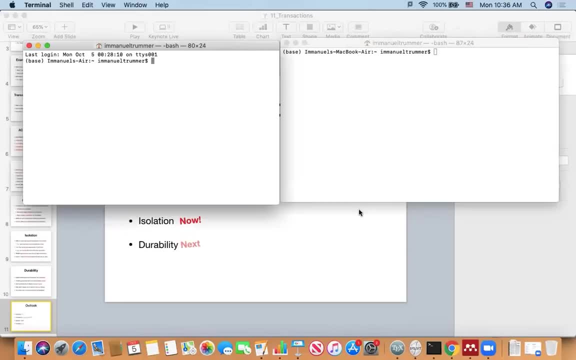 The, The, All All right. So now I want to give you a little demonstration for the effects of isolation. So if you have installed Postgres on your machine, then you can also try the demo yourself. So generally we need to log into the database simulating two different users. 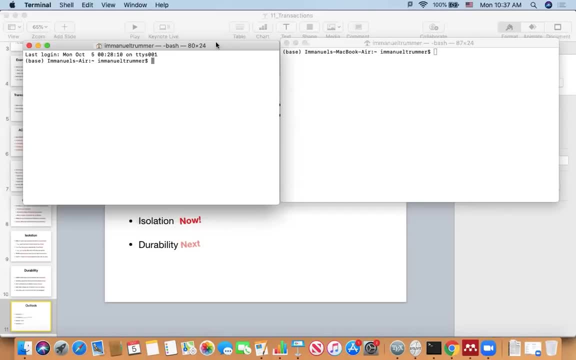 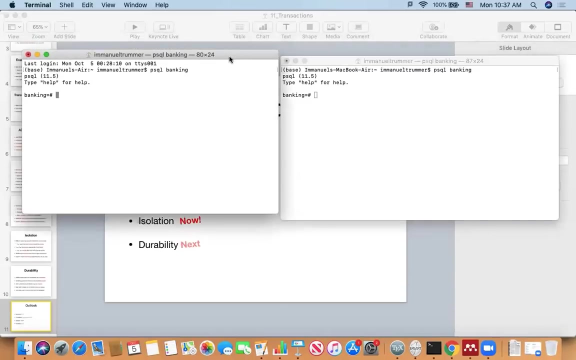 So here I have opened two different terminals And now I have already created a database called banking. So this is what we will use for this example. All right, So now I'm logging into the database in both of those terminals. All right, And you see that work. So now we are connected twice to the same database. 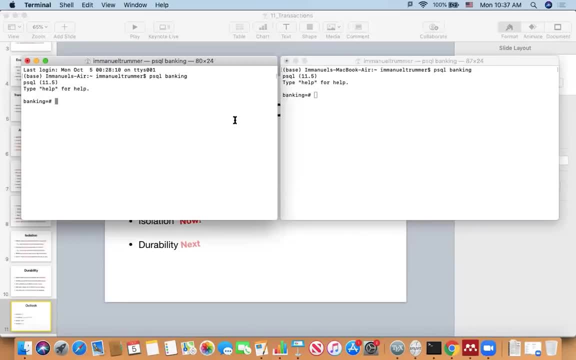 All right. So for this example, let's create a simple table representing the account balance of different users. So we have A name and we have an amount of type- integer- All right. And now this table has been created. So I see it here. 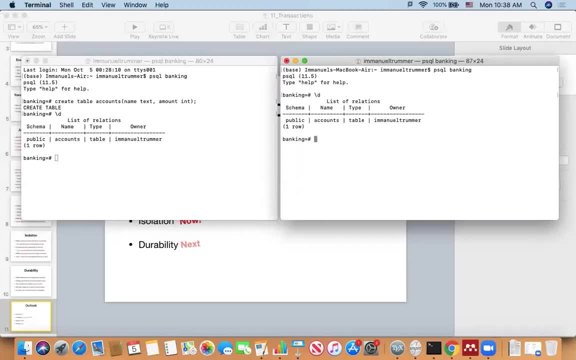 And of course you also see it here, because here we are connecting to the same database. Now let's insert a couple of example values into that database. Let's say that Bob Oops. Let's say that Bob pays $100. And let's also give $100 to Alice. 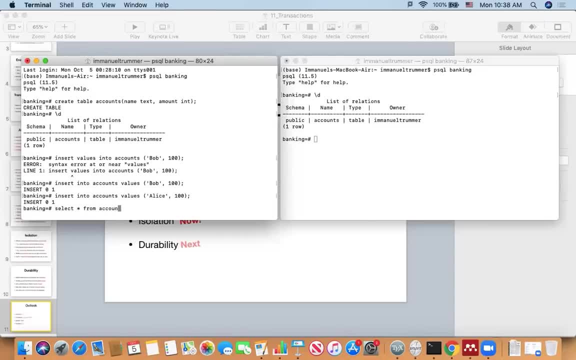 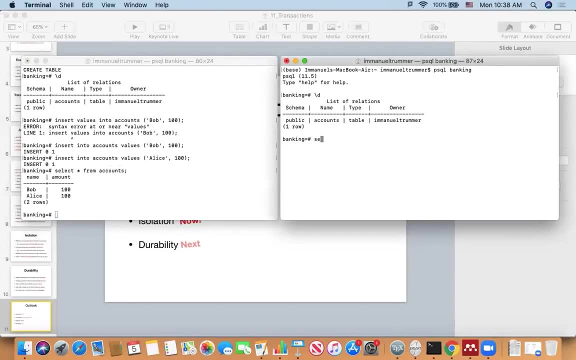 All right. So if you show the content of the table, then now both of them have $100. And here it's going to be the same thing, All right, Okay. So now, in the following, we are going to start a transaction. 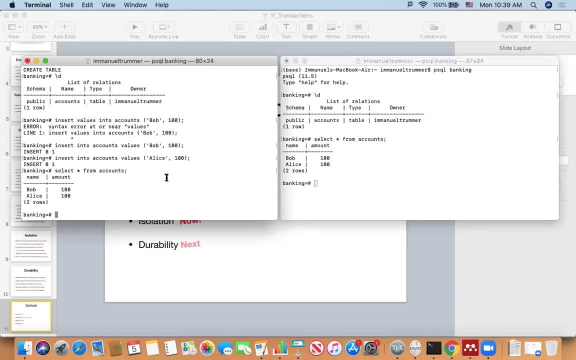 And we're going to transfer $50 from Bob to Alice. So first of all we are starting the transaction. So here we are, marking to the database system the point where the transaction begins, And the following commands will be considered as part of that transaction: 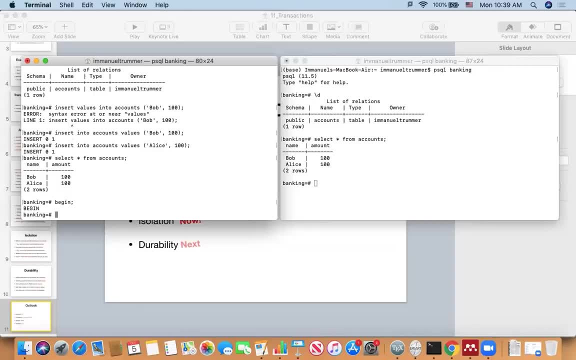 All right. So now the database system has Notified us that the transaction has started And, as first part of that transaction, We reduce the amount of dollars on the account of Bob. We set amount equal to amount minus $50.. Where the name equals to Bob. 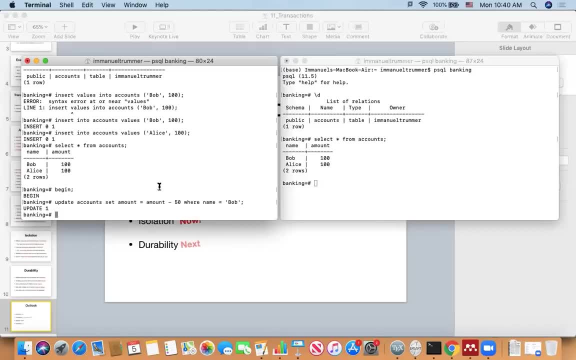 All right, And now here in the left terminal on the screen, let's call that user number one. So user number one has now executed the first change on the database and reduce the dollar amount of Bob by $50.. So if user one runs the corresponding query showing the content of the table, 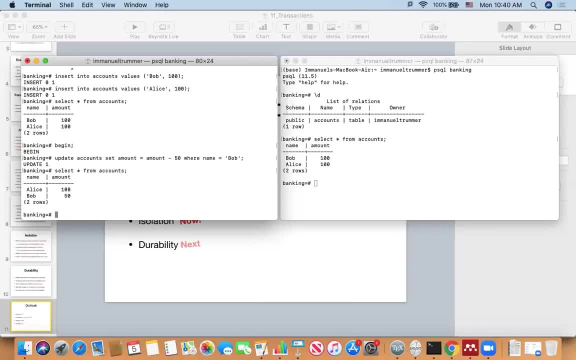 Then that change is already reflected. Well, you see here The dollar amount of Bob has been reduced by $50.. Now, on the other side, if I go to the other user, to user number two here in the right hand terminal on the screen, 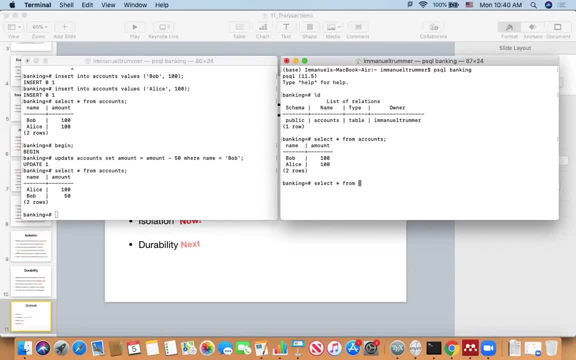 If that user currently runs, select the content from the accounts table. Then, as you see here, nothing has changed, And this is isolation in action. So on the left hand side, we have already started changing the database And we can see here: 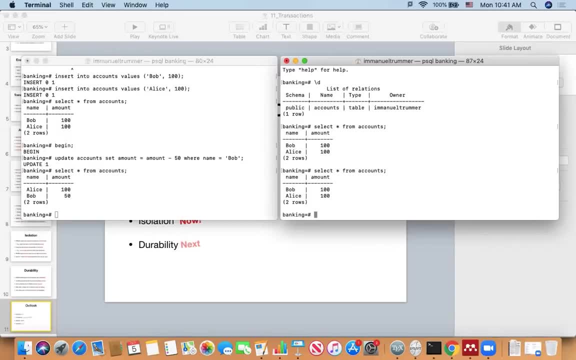 Those changes ourselves, But on the right hand side, a different user doesn't currently see those changes at all. Let's continue. So user number one now adds the $50 to the amount to the account of Alice. All right, And again, if you see what happened here, we see that Alice now has $50 more than before. 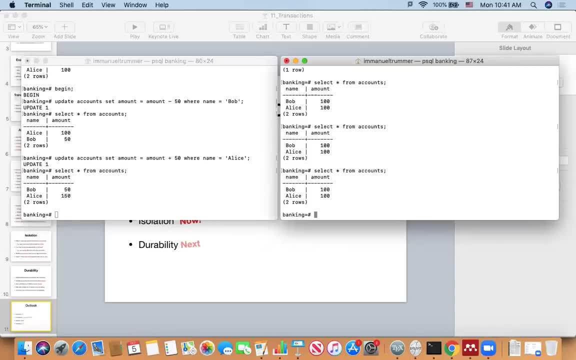 Again on the other side for the user number two. nothing has changed so far. Both of them still have $100.. I mean that makes sense already at this point. It could be that perhaps the transaction of user number one aborts for some reason. 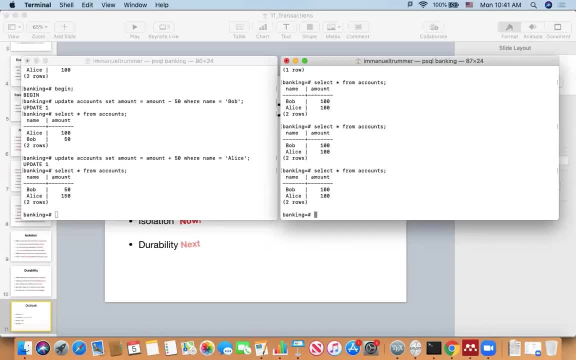 And then none of those updates should actually happen. So in order to Make those updates take effect for all the other users in the database, in order to publish those changes, so to speak, The command that user number one has to run, that is a commit. 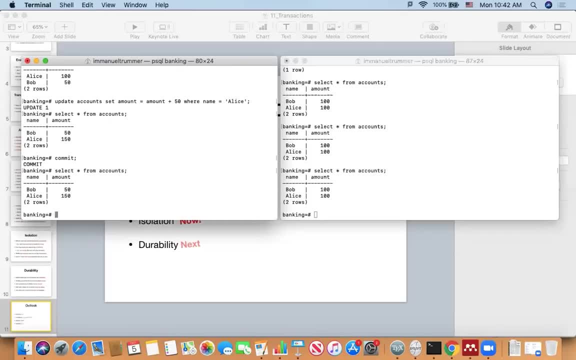 And now the transaction has committed, So user number one, of course, can still see those changes. But what has changed is that user number two now can also see those changes. And what you have seen here is an example of isolation, Because as long as the transaction of user number one was not committed, only user number one was able to see the changes. 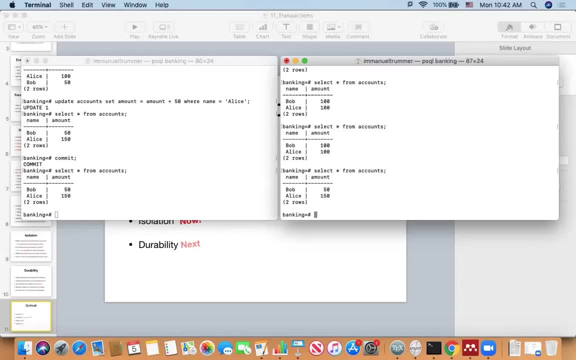 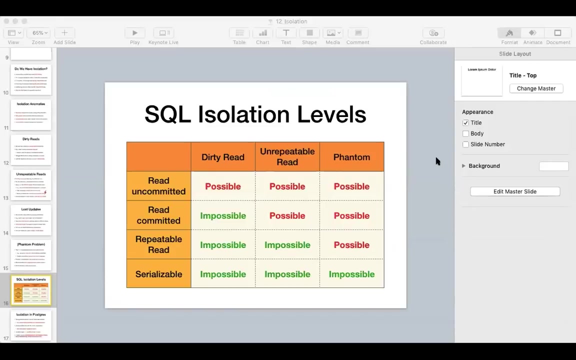 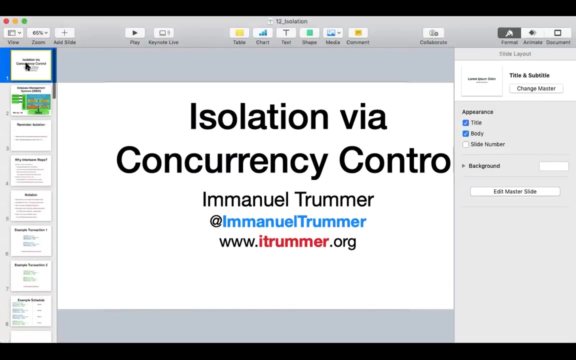 But user number two did not see the changes yet. All right, So this is one simple example where we use isolation in the Postgres database system. Now let me quickly switch to my slides. OK, And that's already done. Yes, Yeah. 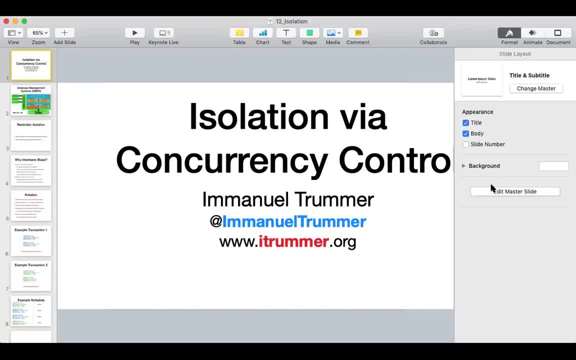 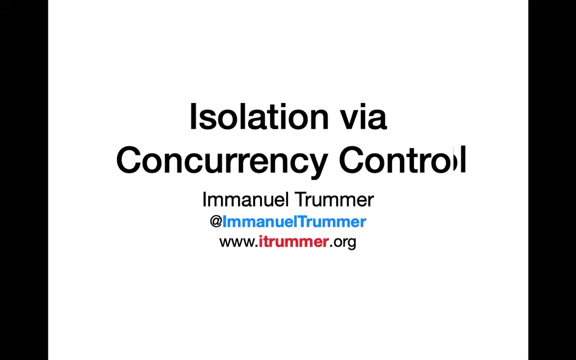 some questions in the chat about how we can actually achieve those guarantees. We are going to discuss about that in a minute. So the operations and different transactions in general don't have to be competitive. All right, So in the following we're going to discuss in more detail about: 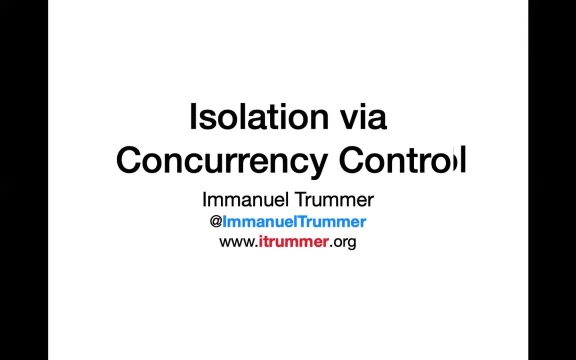 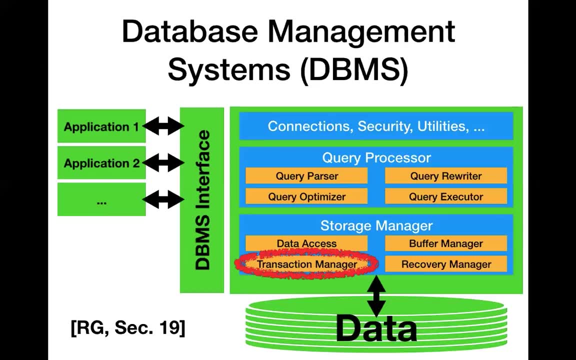 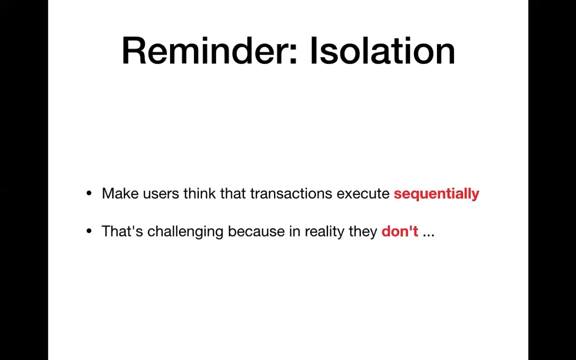 isolation and about algorithms by which we can achieve isolation. Now, here we are again talking about the transaction manager, specifically for isolation, the most relevant chapter in Ramakrishna and Agarka, that is, chapter number 19. And, as I have already explained, isolation is 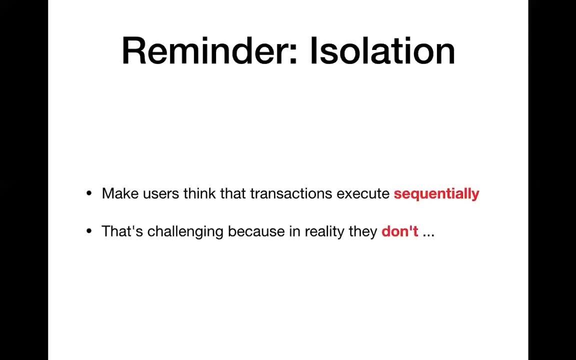 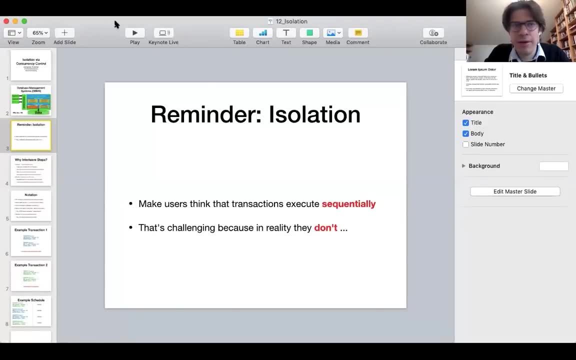 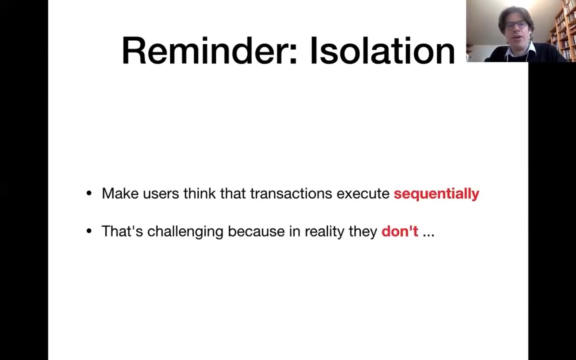 generally about simulating sequential execution to the users. So we are going to talk about this in detail. But first let's discuss in a little bit more detail about why we don't want to execute one transaction after another one, And again we'll talk about the reason why we don't want to execute one. 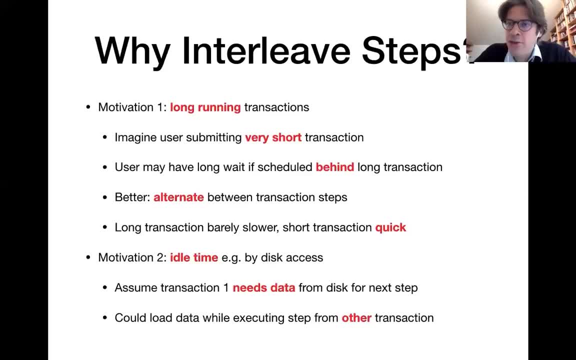 transaction after another one. so we can see that it's not necessarily the case that we cannot execute just one transaction after another one, And there is at least two motivations, The first one being very long running transactions. I mean transactions like transferring a certain dollar amount from one account to another. 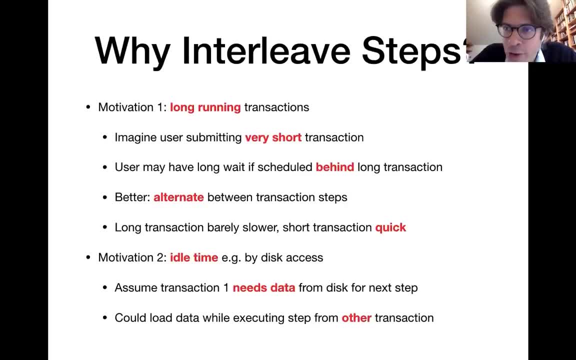 one. they are typically very fast to execute. But you could also imagine having some transactions that do very complex analysis on your database and executing those transactions can actually take a long time. And if you imagine that we are executing all transactions one after the other one, 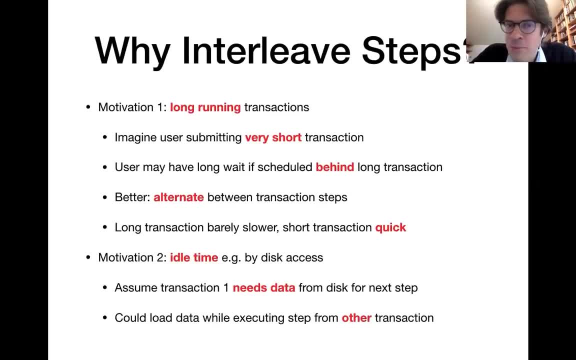 serially, then if you, as a user, submit one of those very short running transactions, however, your transactions get scheduled after one of those very long running transactions. In that case, you, as a user, would have to wait for a long time until your transaction. 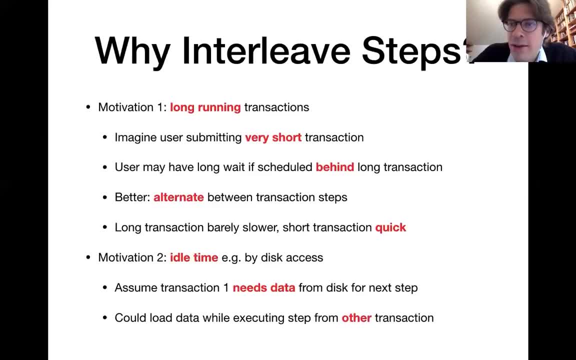 processes, even though your transaction is actually very short and inactive, expensive. so what is better here is to rather alternate between steps from different transactions, which means that the long transaction might be a tiny little bit slower because we interleave a couple of steps from the short running. 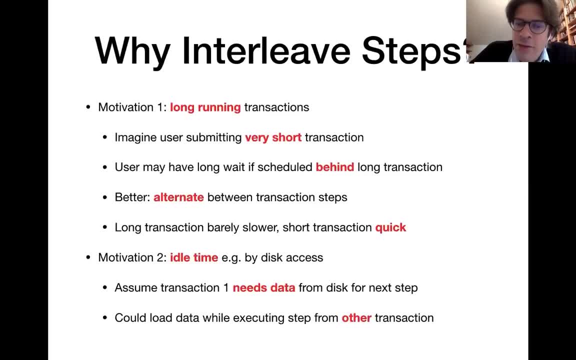 transaction. but the short running transaction will be as quick as one should expect, and that is why doing like interleaving steps from different transactions seems like a good idea in this scenario. also, every once in a while, transactions might have to wait for data before executing next step instance, if 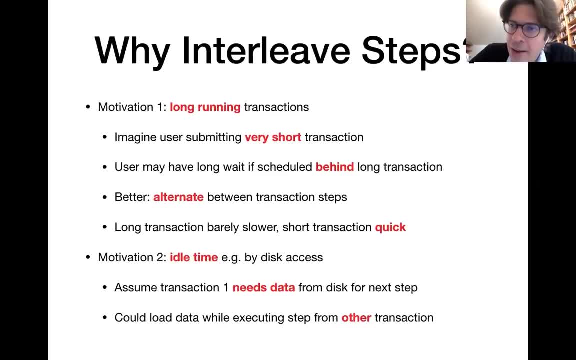 your data is mainly located on hard disk, then you might have to wait until we wait until we load that data from hard disk into main memory. and when waiting for data, then of course there's the choice that we just keep idle until the data is loaded, and then we wait for the next step, and then we wait for the next. 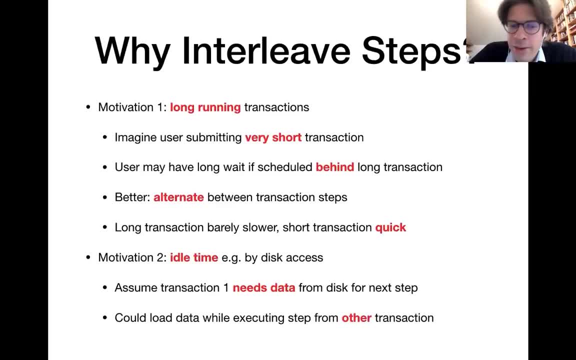 data arrives. but that wastes time. so it is better to rather schedule a step by a different transaction which can already proceed, because the data it needs is already in main memory, and then, once that step from the other transaction finishes, maybe at that point data has been loaded, so the 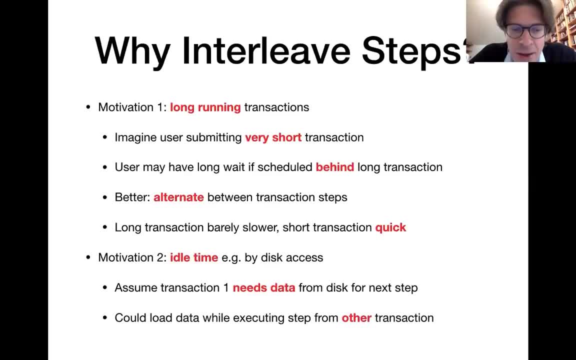 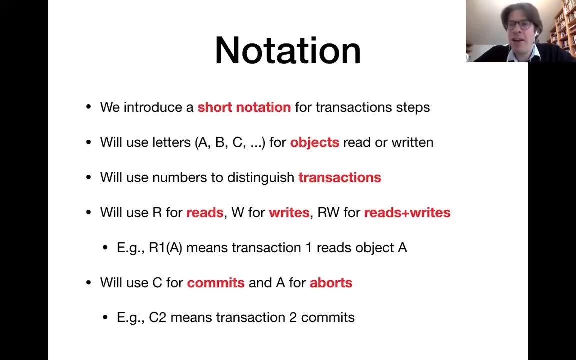 first transaction can make progress again. so for at least those two reasons that people are interested in interleaving steps from different transactions. now, in the following, we're gonna discuss a lot about how we can interleave steps from different transactions to make sure that nothing bad happens, and in order to keep the examples we will see concise, we will use the 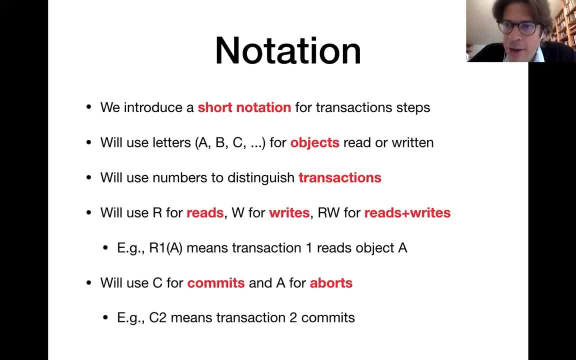 short notation that is introduced on this slide. so this is important. you need to memorize to chalk notation because we will keep using it in all of the following examples. all right, so generally in that chart notation we describe, read and write operations by transactions on database objects. so for the database objects we typically use letters like A, B, C. 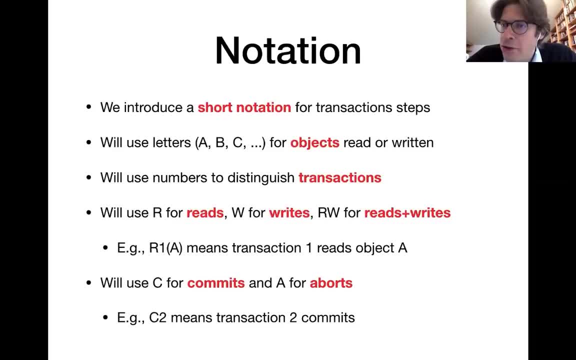 a see, and in order to distinguish different transactions, we use a number, so that is typically represented as t1, t2 and so on. in order to represent operations by those transactions, we use r to abbreviate reads, w for abbreviating writes and rw for abbreviating a. 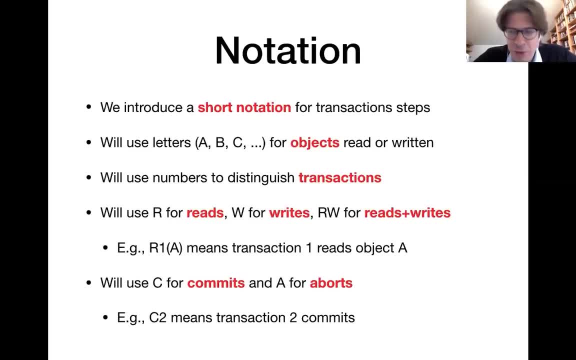 combination of a read and a write. so for instance, if you write r1 of a, that means the transaction number one reads object a. you also use a c for commits and a for aborts. so if you write, for instance, c2, it means that transaction number two wants to commit. 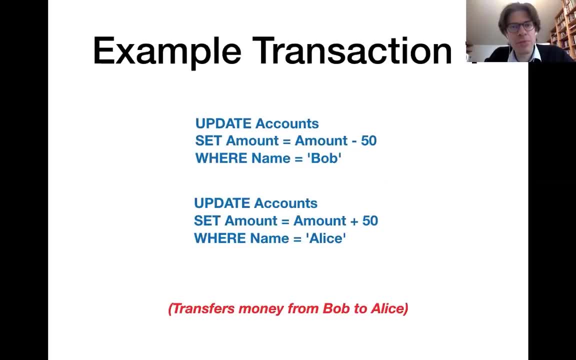 now let's make you a little example with transactions, again from the banking domain, and here we have pretty much the transaction that we have seen in our little demo. here we are transferring 50 dollars from the account of bob to the account of alice and, as we have seen, this requires two steps. 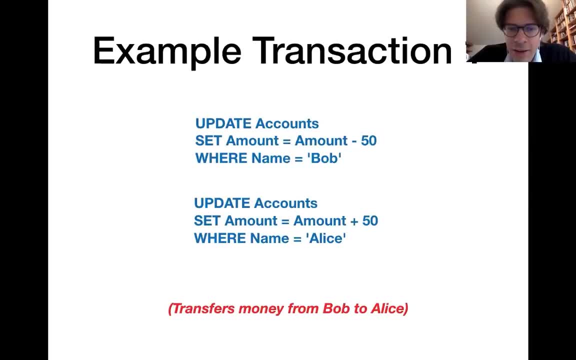 where we update the amounts in both of those accounts. now let's use a second transaction which, for instance, adds the yearly interest rate. so here let's say that we're adding 10 percent and we need to add that for both of those accounts. so in principle you could do this by one single. 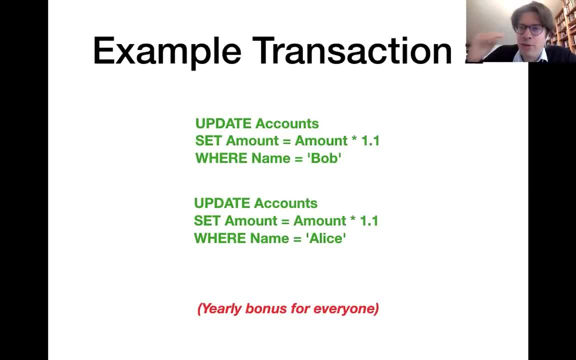 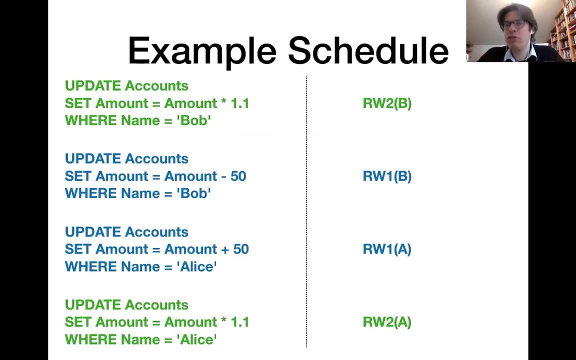 query, of course, but here, for the sake of the example, let's say that we do this for different accounts separately, all right, and if those two transactions execute at the same time, there's different possibilities about how we're going to do this. so let's say that we do this for the 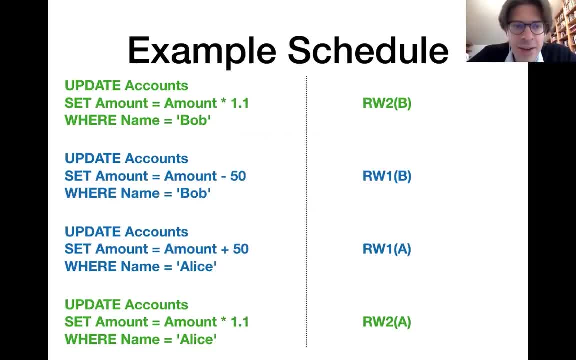 same time. now we can interleave the steps of those transactions. so here there's a first possibility. we could for instance start with the first operation of the second transaction and then do the first transaction and finally do the second operation of the second transaction- again second transaction. 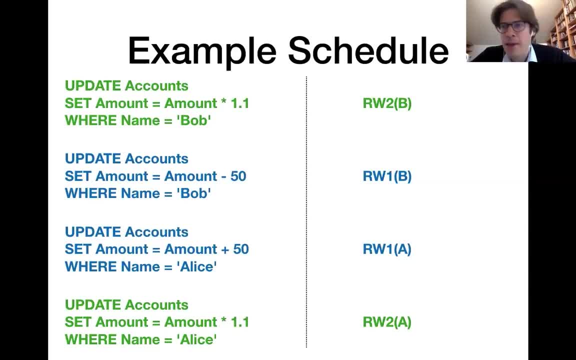 in green, first transaction in blue. now here on the left hand side you see the more verbose queries. on the right hand side you see the shorthand annotation. so here, for instance at the beginning, we are updating the account of bob, which means that we first of all read: 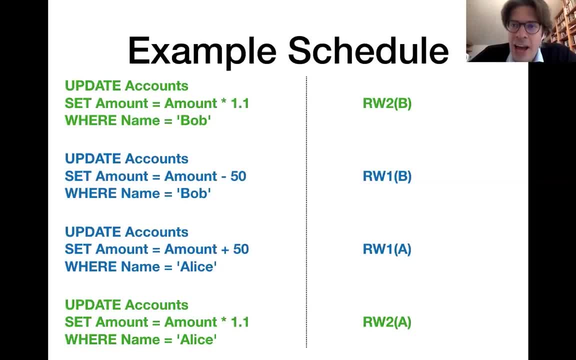 the current amount and then we write an updated account after adding 10 percent and that is represented by this rw for read. write two is the transaction id and b is the database object that we are writing on. so in this case, the database objects we are talking. 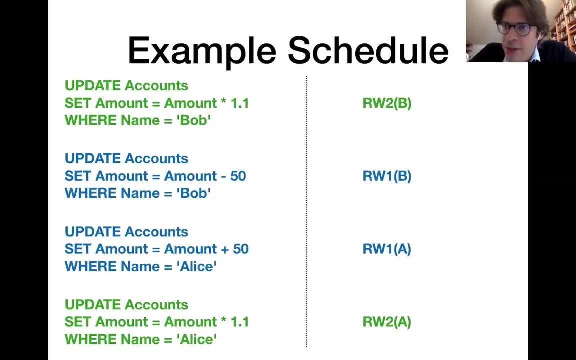 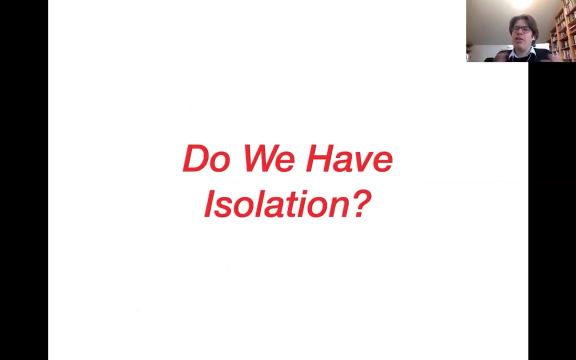 about. those are specific rows in the table, and here by b we mean the row that is associated with bob and by a we mean the row that is associated with else. all right, so this is one possibility of interleaving the operations of different transactions. now, first of all, if we do this, if we interleave the operations in that way, do we have isolation? so 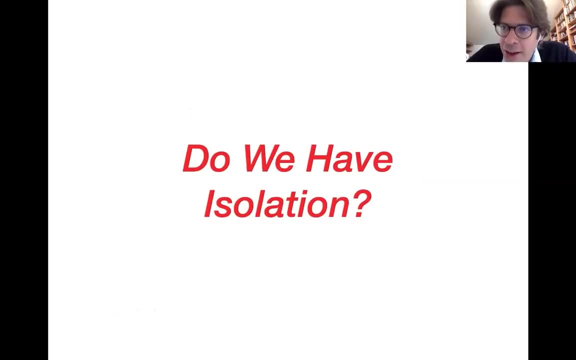 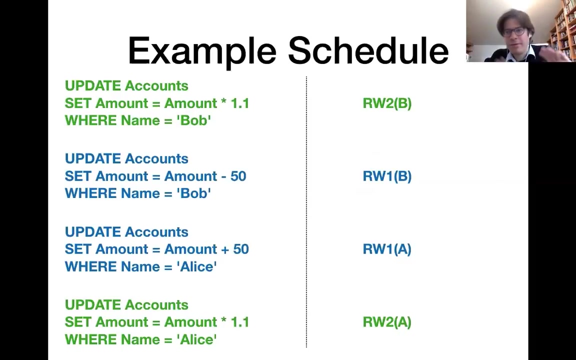 will what we get be consistent with executing one transaction after another one, or is that perhaps something that? do we see any effects that we would not see when executing one transaction after the other one? if anyone has an idea, okay, somebody mentions data dependency issues. yes, yes, can anyone, uh, perhaps make a guess about, um, what changes compared to executing? 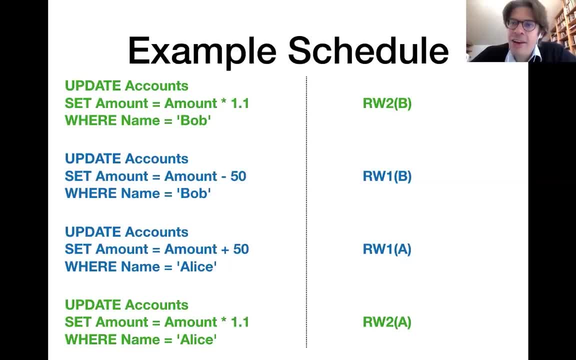 one transaction after another one, if you think, for instance, about the final state of the database. okay, okay, very good, all right. yes, very good. and here i see the suggestion that the amounts in the account might be higher than they should be. yes, okay, very good, all right. so this is the exactly. this is the right. 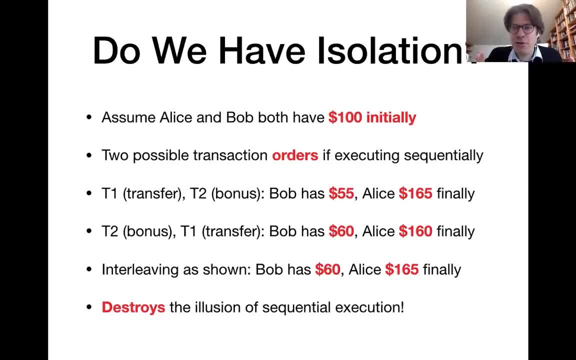 direction. so, um, if we play through in more detail, so if we execute one transaction after the other one, there's really only two possibilities here, because you only have two transactions. so either we execute the first transaction first and then the second transaction, or we execute the transaction. 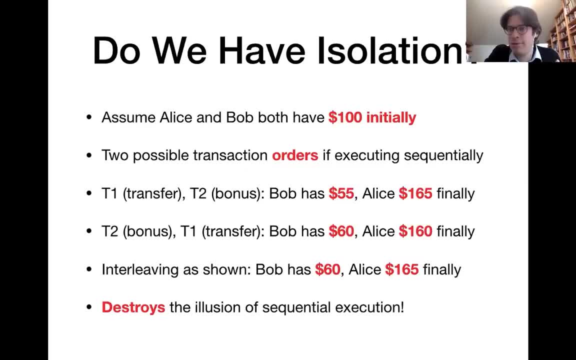 or we execute the second transaction, transaction number two first and then transaction number one, And here we have tried that, both possibilities. So if you first execute the transfer and then the bonus, After doing that Bob should have a $55, because the transfer was from Bob to. 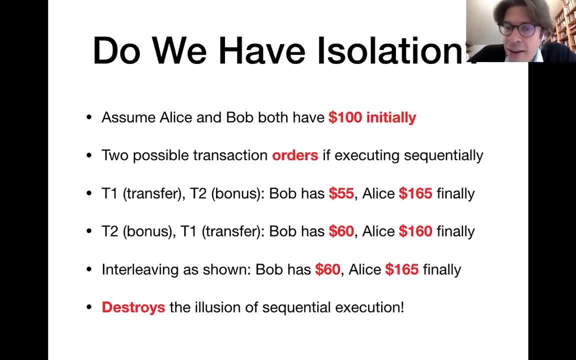 Alice. initially We assume that both of them have, for instance, $100. And if you first transfer $50 from Bob to Alice, then Bob has $50 left, And if we add 10% afterwards, then Bob has $55.. 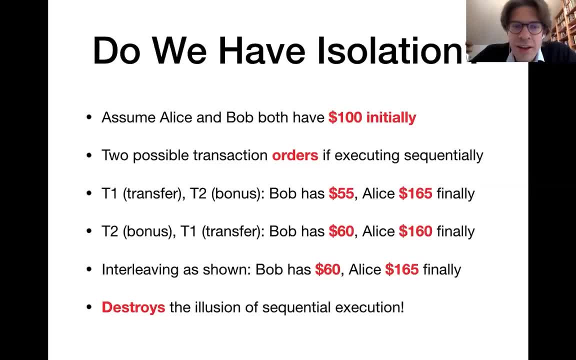 Alice on the other side, since we do the transfer first she has $150 and then 10% bonus makes $160.. So if we first execute a transfer, then the bonus, then this is the amount of dollars that we should find in the end. Now on the other side, if you first execute the bonus transaction and afterwards 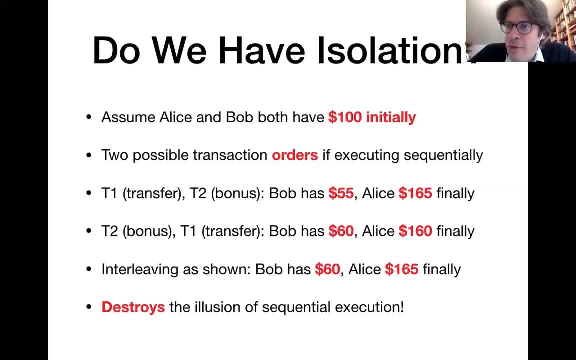 the transfer. Now, if both of them have $100, then after the bonus both of them have $110 because we're adding 10%, And after that we are transferring $50 from Bob to Alice. So Bob is left with $160, but Alice will receive $160.. So those are the two possibilities. There's no more. 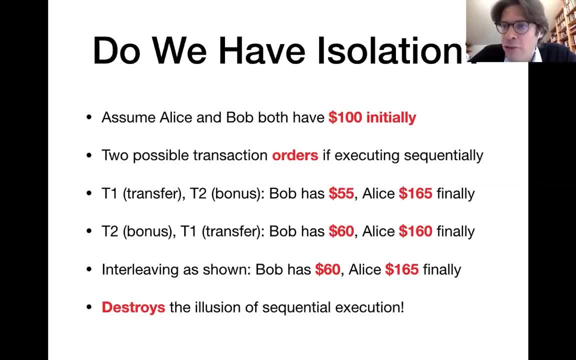 possibilities. with two transactions, I only have the choice between which one of them I execute first And, as we see both of those possibilities, they lead to a different final state in the database compared to the schedule that we have seen. Let me quickly remind you how that looks. 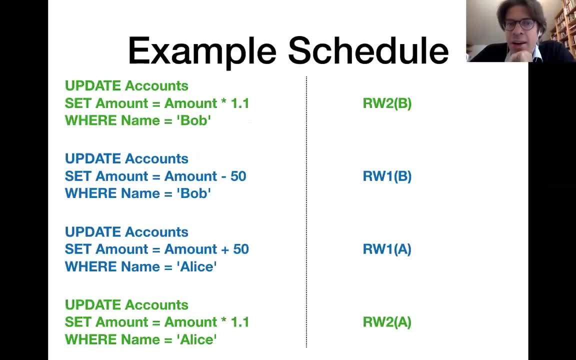 like So here. first of all we are adding the bonus for Bob. So if Bob has initially $100, then Bob will afterwards have $110. Now we are reducing the account of Bob by $50.. So from $110 to $60. While for Alice we increased from $100 to $150. And now we are adding still a bonus for. 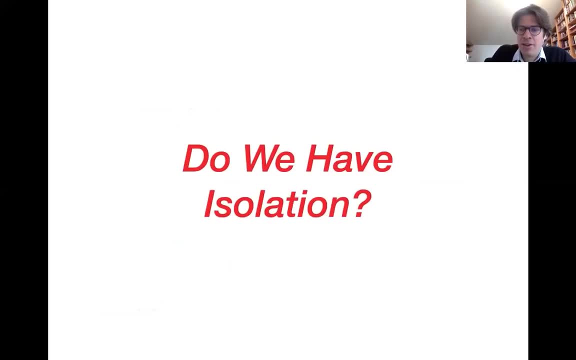 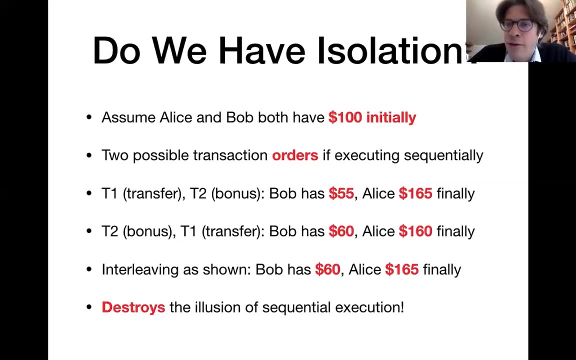 Alice, which means that we have $165 for Alice. So in the end we end up with $60 for Bob and $165 for Alice, And this final state is not achievable with any of the serial executions. Of course, in a certain way you say both of them. 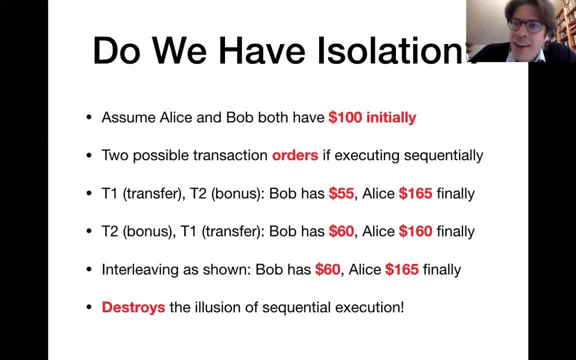 actually have more money than they should have. So from their perspective it's a good outcome. But the bank of course controls the database server And from the bank's perspective it's not a good outcome. All right, And in any case, having this essentially destroys the 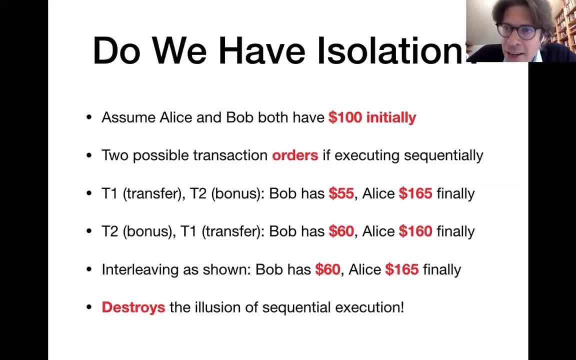 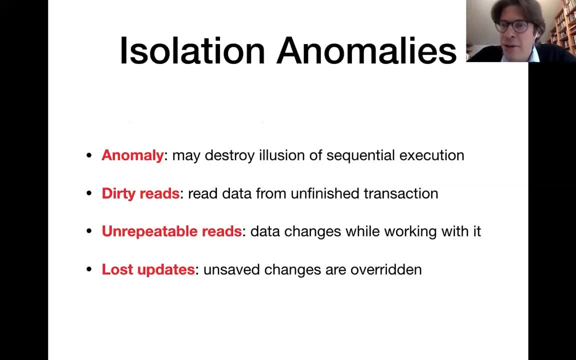 illusion that your transactions execute serially that we want to give to the users. All right Now, generally, whenever we destroy the illusion of serial execution towards the users, we call that an isolation anomaly, And in a forum we're going to see a couple of different types of 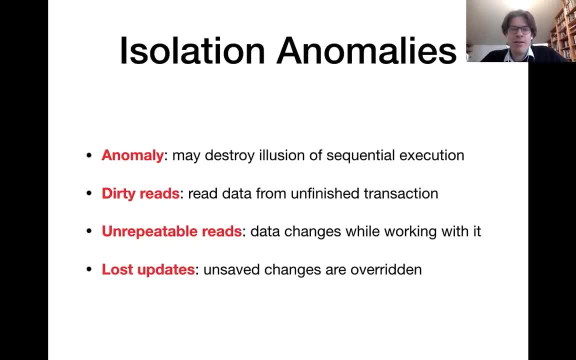 isolation anomalies And, in particular, we're going to have a closer look at dirty reads, unrepeatable reads and lost updates. So dirty reads- short description- essentially means you read data from a transaction that has only partially finished. Unrepeatable reads means we're reading data once. 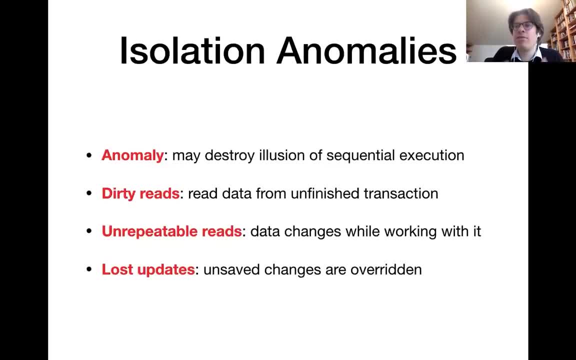 and then another transaction comes and changes that data And once we read the data a second time in the same transaction, suddenly it has changed And that also destroys the illusion of the system being the only one executing the system at the same time Also lost updates means. 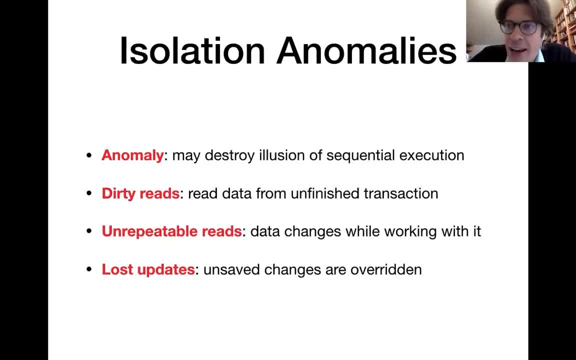 that different transactions essentially override the changes of other uncommitted transactions in a bad way. So all of those things can lead to problems and destroy the illusion of executing alone in the database Following. we're going to discuss those different anomalies in a little bit. 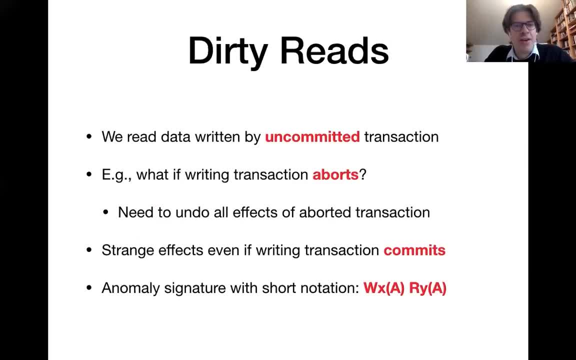 more detail, All right. So first of all, we are going to discuss a little bit more about dirty reads, And that generally means that we read data from an uncommitted transaction. So if we read data from another transaction, it means that we might be influenced in what we do next. 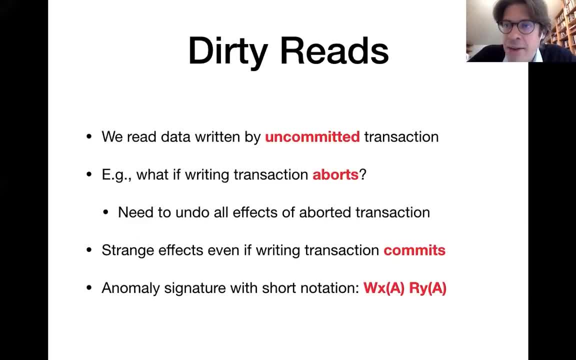 by the values that we have read And if you read data from uncommitted transactions, it's actually very risky because we never know whether that other transaction might actually finally commit or whether it might finally abort, Because if the transaction aborts, then I have 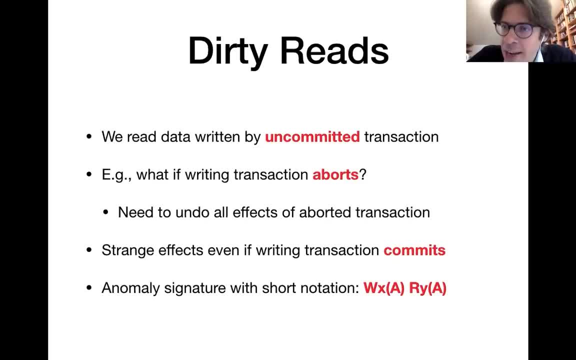 read values and acted upon them which are actually invalid, because the database should in the end look as if aborted transactions have never happened. So if I read values from those uncommitted transactions and get influenced by those values, it might indirectly reflect the result of the changes caused by those transactions that might later abort, which is 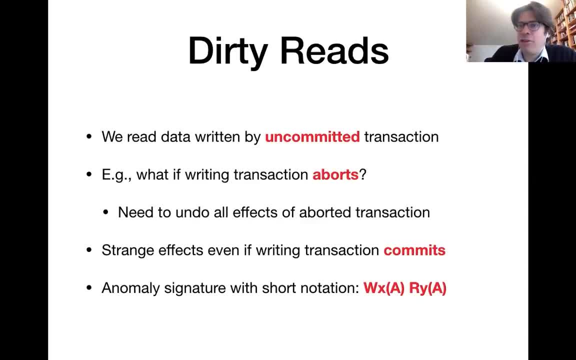 invalid, Even if I read data from another transaction that might finally commit. that still might lead to a strange effect. So generally, dirty reads is something to avoid And in the demo that we have seen before, for instance, you've seen that when user number one was updating the database, 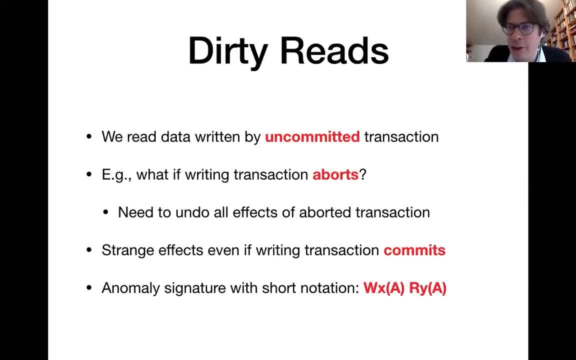 number two did still not see those updates before the transaction has committed. So this is what we are trying to do there. The database system is trying to avoid dirty reads. So user number two cannot yet see the uncommitted changes from user number one. 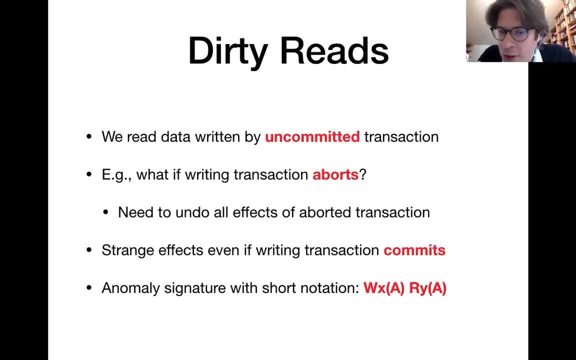 And once we think about the shorthand notation that we have introduced, then the general signature, so to speak, from those dirty reads that is right by some. first transaction X on object A, followed by a read by another transaction, but on the same object, without. 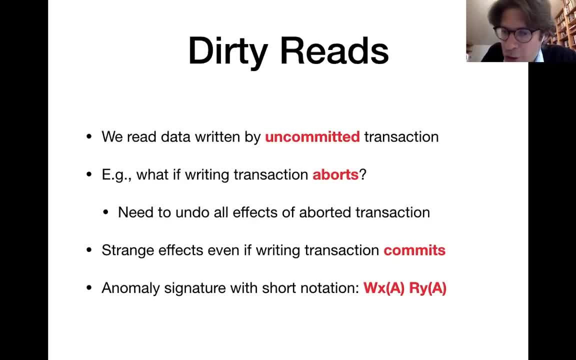 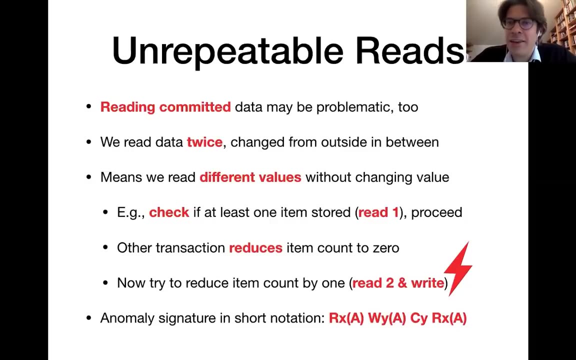 any commit between those two operations. So the first transaction, X, has not yet committed and still transaction Y is already reading its values. Unrepeatable reads. It means essentially that the data you are working on keeps changing without you being the one changing it. 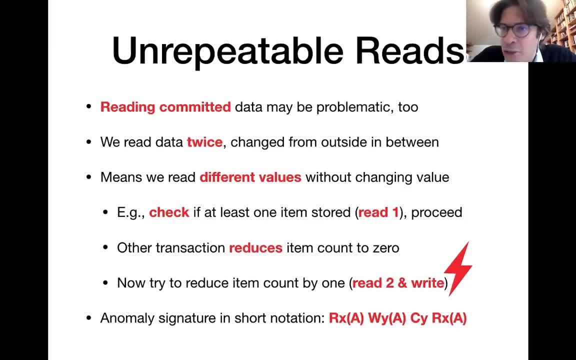 So that is very clearly destroying the illusion of being the only one executing transactions at the same time. So, in general, an unrepeatable read means that you read the same data twice without changing it, but still suddenly the data changes, Which means there must be a change. 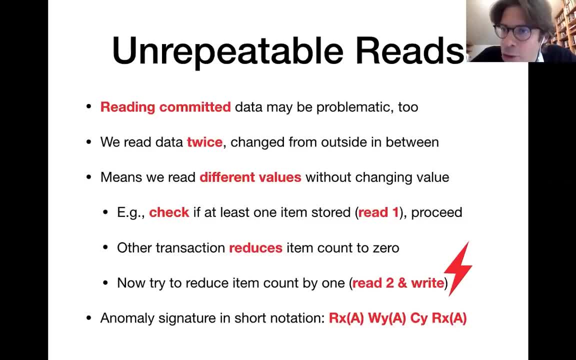 There must be somebody else changing the same data concurrently with me, For instance, one situation which that can cause a problem. Let's say that we are talking about the database of an online shop And that database essentially takes in orders from customers. So before accepting an order, it needs to check whether it still has enough items in. 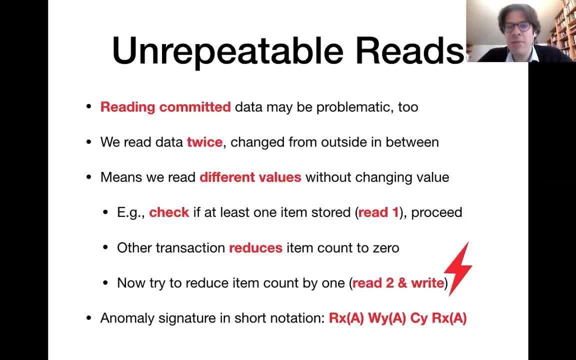 store in order to satisfy the order. So we could imagine that it still has enough items in store in order to satisfy the order. So we could imagine that it still has enough items in store in order to satisfy the order. And now, if we wanted to discuss a transaction, that we check the number of items once and 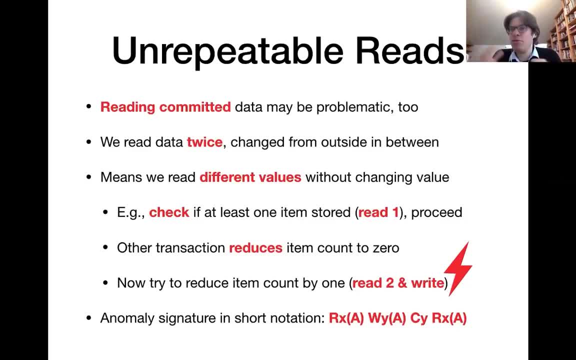 we see, Oh, we still have an item left, And then we do something else. But in the meantime a different transaction, perhaps a different order, comes in and reduces the item count that I'm currently working with. And now, once I try to finish the order and want to reduce the item count further, maybe, 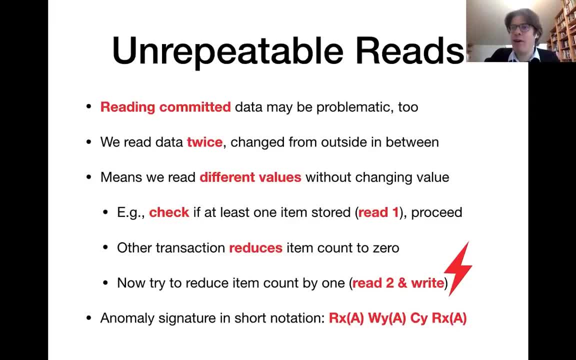 transaction has already reduced it to zero. so now i'm trying to subtract one and make it negative, which probably is not permitted by the database. so, um, at that point i am creating a problems and i might end up with an inconsistent database. so, um, that is one situation in which those 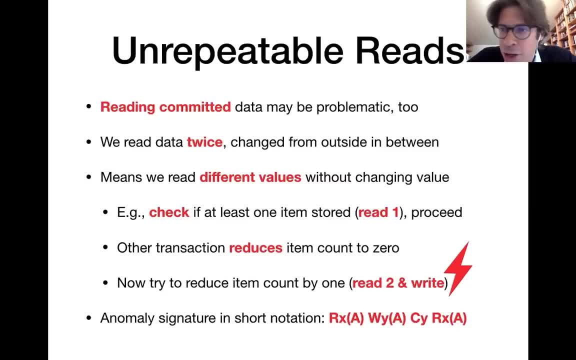 unrepeatable reads can create problems, but that's just one example and the general signature of those unrepeatable reads is that one transaction, x, reads an object a. then another transaction comes along and changes the value of object a and commits. so even if i don't have a dirty reach then 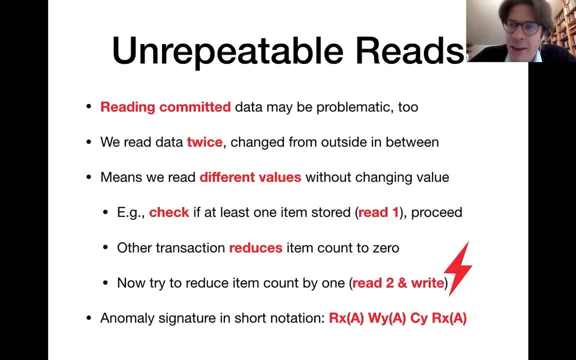 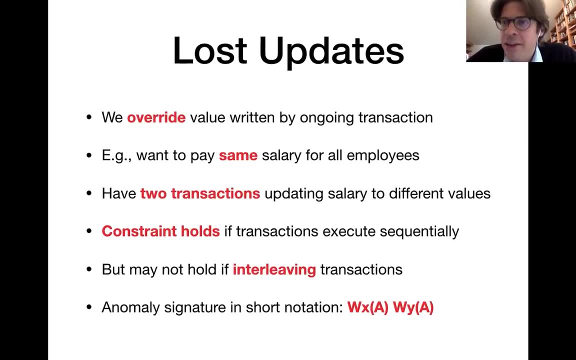 that value has changed and now the first transaction, x, again reads the same object and now suddenly finds that it has changed. so that is another anomaly that we want to avoid. um, one more is a lost updates and that essentially means that different transactions override each other's values while they are executing, and that can create problems, because 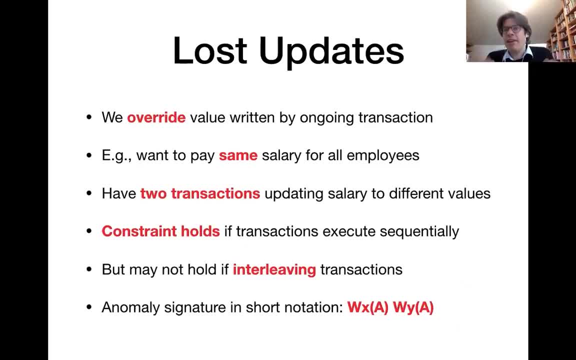 it can lead to an inconsistent database state. for instance, let's say that you want to keep the salary of all employees in a certain department the same, for fairness. so you have multiple transactions that update the salary, and if two of those transactions interleave their operations, it might be possible. 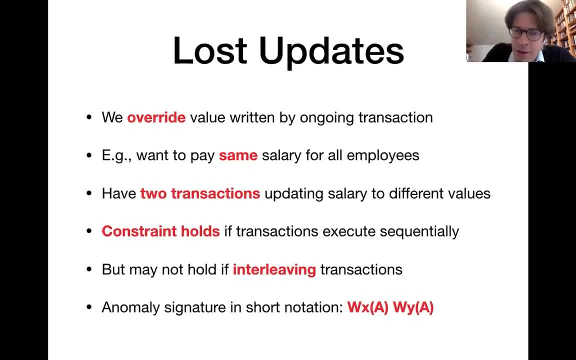 that some of the employees get salary one, while some other employees get salary two, which is something that you want to avoid, and you could avoid that if executing transactions one after the other one, because then it would be guaranteed that all employees always get assigned to the same. 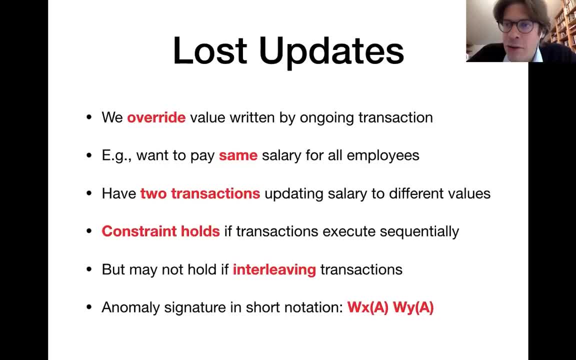 salary. and that problem is generally called the lost update problem, because the updates from some transactions- they might get overridden by other transactions and without a committing before, and the signature of that anomaly is the one that you see here. that's simply like one transaction, x writes a value to an object a and then before that transaction. 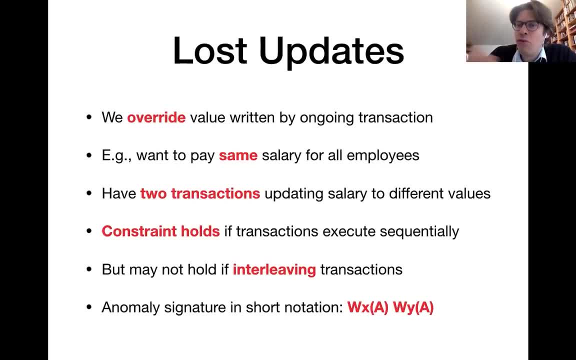 commits another transaction, y comes along and simply overrides the value of that value, the value on the same object. that is the last update problem. uh, one more problem, one more anomaly that we will discuss um a little bit more about later in the course. that is the so-called 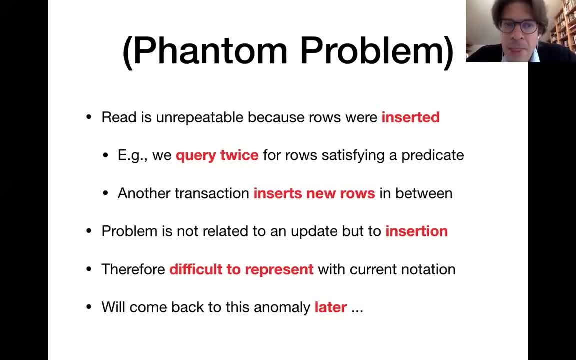 tantrum problem, so i'm already mentioning it here anyway. um, that is kind of like an extension of the unrepeatable read, but in the context of insertions, another something such as, for instance, retrieving all the students whose name starts with a certain letter- all right, and doing that twice. 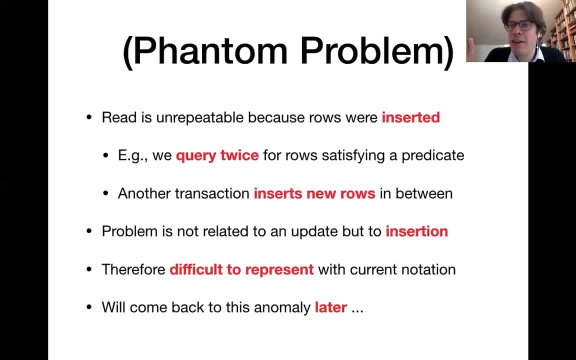 within the same transaction. now it might happen that when running the query the second time, suddenly more students appear in the recycling. that can happen if a different transaction has inserted students and the Using of these formulas. that is called the hythm problem, and that is actually a problem. 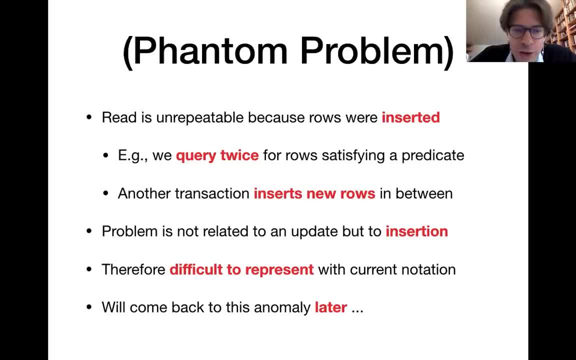 In the case of the, the theorem part of the solution, from the elements of the problem. Then there are a bunch of other problems need to be fixed to do that. So the problem is the replenishment of data between the first query and the second query. 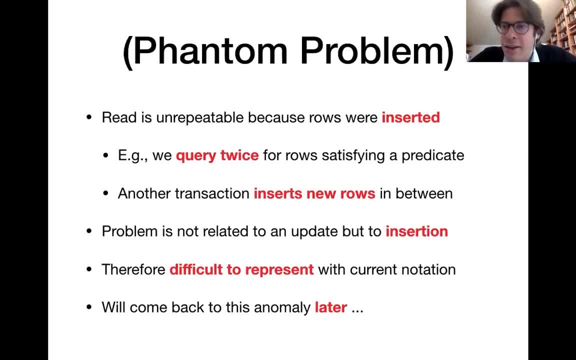 objects A, B and C and so on. Here, what we're doing is that we're essentially inserting new objects after a query has executed the first time and before it executes the second time, And for that reason we're going to discuss that in more detail later- and we are 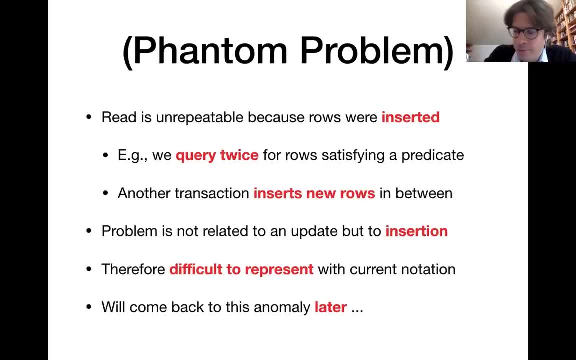 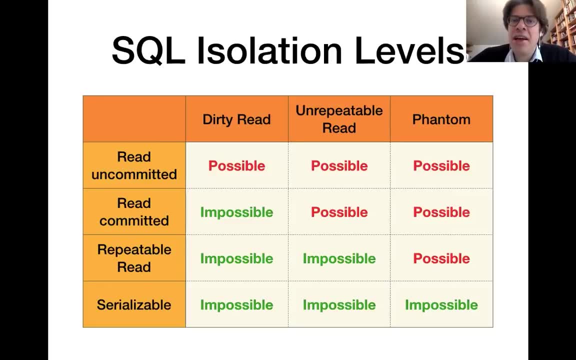 going to first focus on the first three anomalies. All right Now. in the SQL standard you actually have different isolation levels, So that means that for certain applications it might be acceptable to have some of those anomalies, but not others. Isolation can be very expensive performance wise, So that means that sometimes 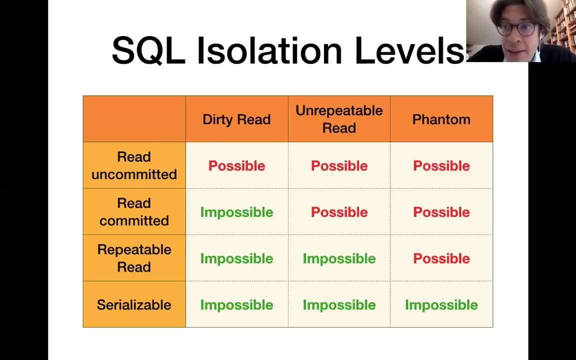 you might be willing to accept even some slightly strange behavior of your database If, in exchange, your database can process transactions much faster. And this is why SQL gives you the choice between different isolation levels. So here on the left column you have the different isolation levels, read uncommitted, which allows essentially anything. 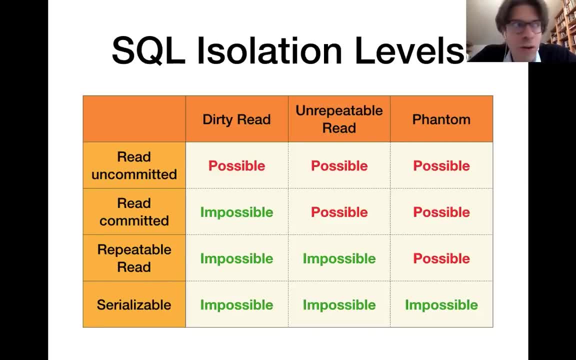 Read committed, which already avoids a dirty read because we are only allowed to read data from committed transactions. Repeatable reads, which avoids the repeat, unrepeatable read anomaly. And finally, to analyze the book, which means that here we have a nearly perfect illusion of isolation. 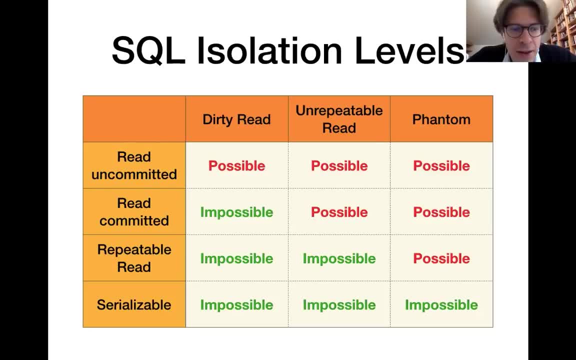 So here on the column on the left you see the different isolation levels and the top row is associated with those different anomalies And you see for each isolation level whether the corresponding anomaly is greater or less than or equal to, greater than or equal to. 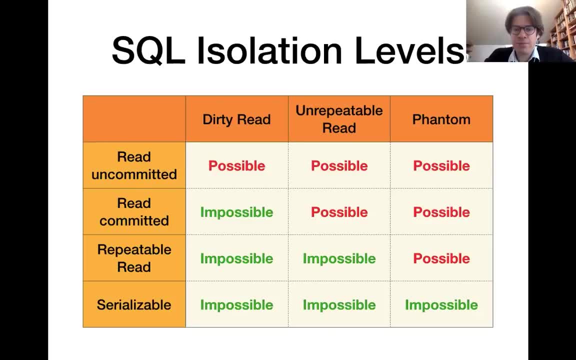 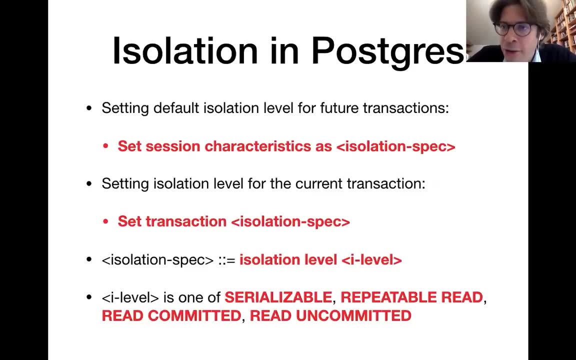 greater than, or greater than or equal to. So that's one of the reasons we're going to have. this may appear or not. this is how we can change those things in Postgres. in Postgres, you can, for instance, set the default isolation level with the set. 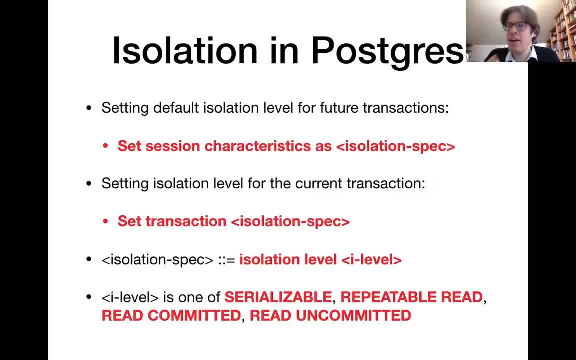 session characteristics commands. you can also set specific isolation levels for specific transactions, because perhaps you have some transactions that are more critical than other transactions, so you can set higher isolation levels for a more critical transactions. you can use that by writing something like set transaction isolation level serializable, for instance, and then this current: 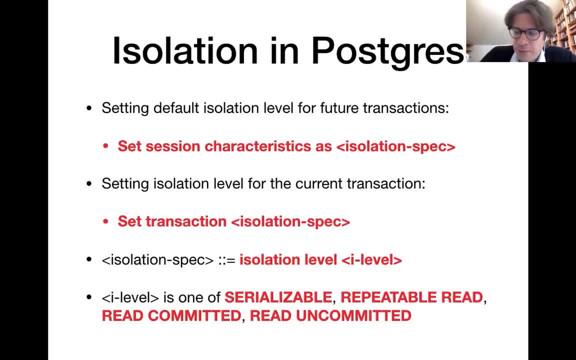 transaction would be assigned to that isolation level. one thing to know is that many people think by default, the database system might support the highest isolation level, but that is often not the case and that can sometimes lead to problems. so, for instance, in Postgres, the default would be a recommitted. so one of the 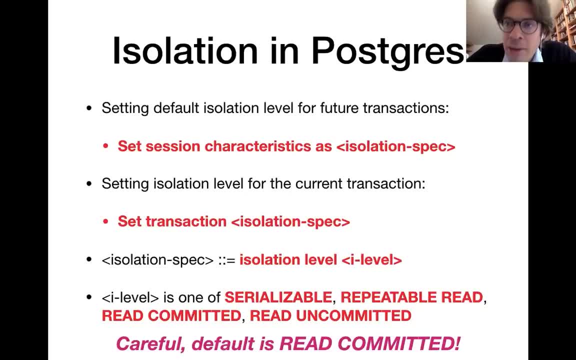 little bit weaker isolation levels actually, so some of those anomalies might appear. you can manually set that isolation level higher and, depending on what kind of application you're working on, I would recommend you to do that. so make sure when using a database system that you're well aware of, which. 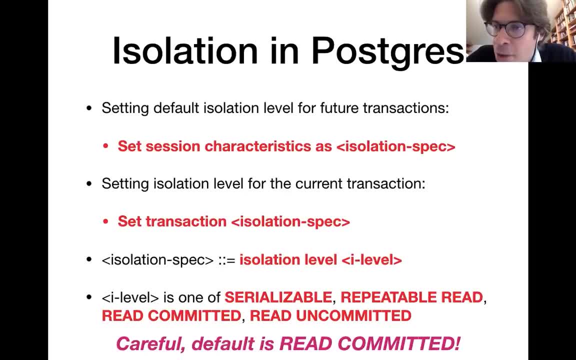 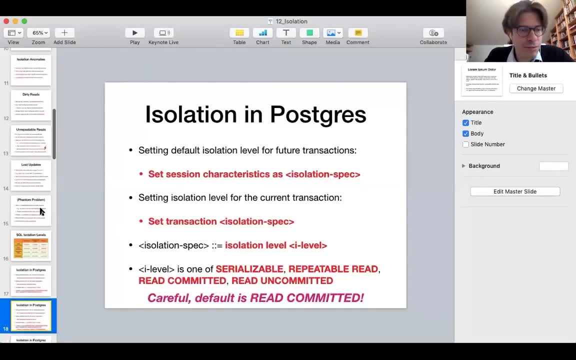 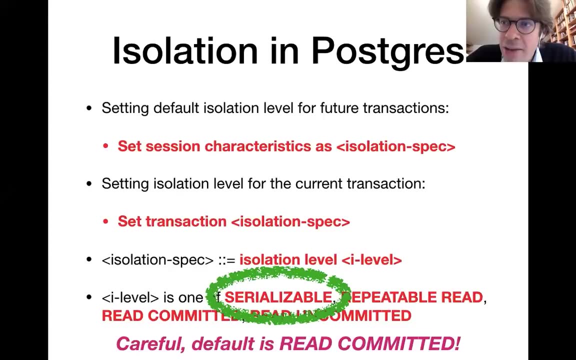 isolation level you need and which isolation level your database system is currently. he's all right now. in a following, we are going to discuss more in particular, about the serializable isolation level, and we're going to discuss about the protocols by which we can guarantee that you won't have too much time to start with that. 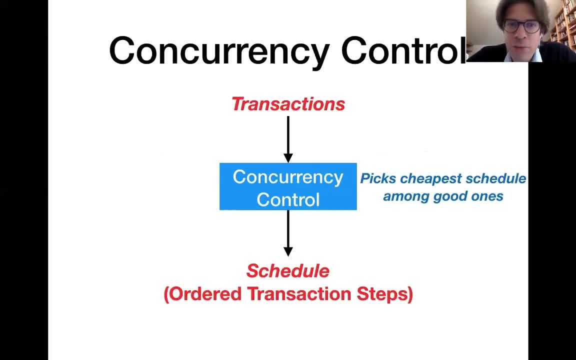 anymore today, but I already give you a little teaser or a sneak peek on what we will be doing. we will generally talk more about concurrency control, which is the process by which we achieve isolation, basically. so how that looks like is that you typically have three components: A main, 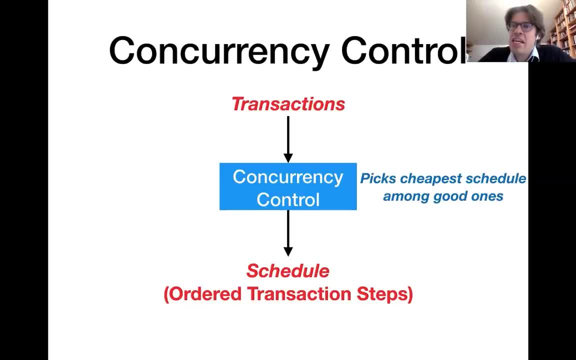 database system that it performs concurrency control. so the input to that component are the transactions and the output of that component is a schedule, meaning in order between steps of different transactions that might interleave the steps of different transactions, and then the goal of concurrency control is to select the 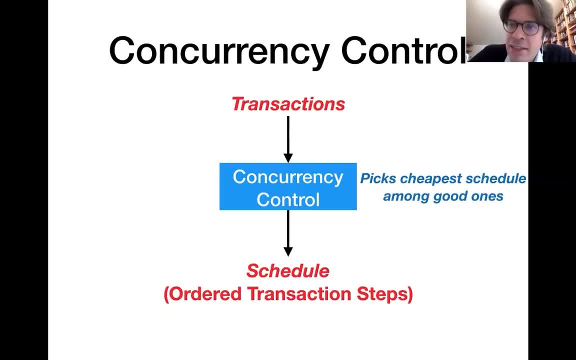 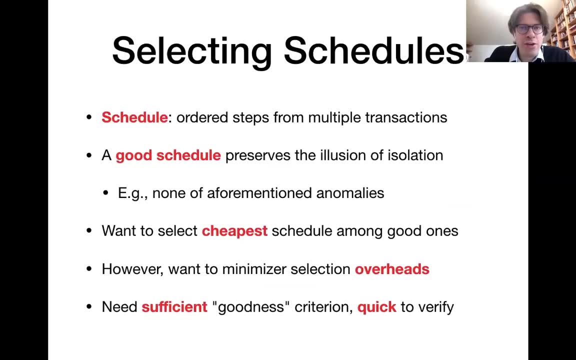 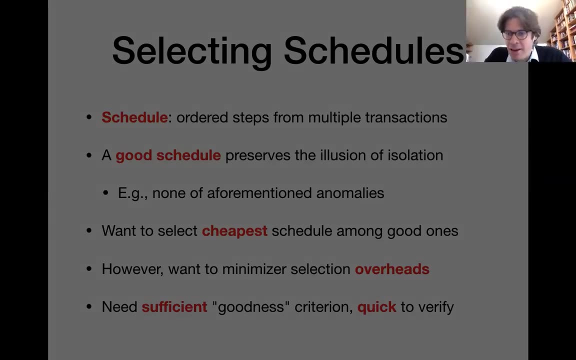 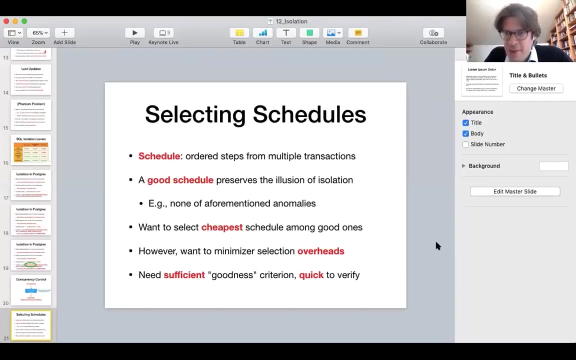 schedule that is cheapest to execute while still avoiding all of those anomalies that we have seen before. Alright, so we're gonna discuss more about this the next time. Let me quickly see. I think there are some questions in the chat. Okay, very good question. So the question is: why would I ever want to use a weaker? 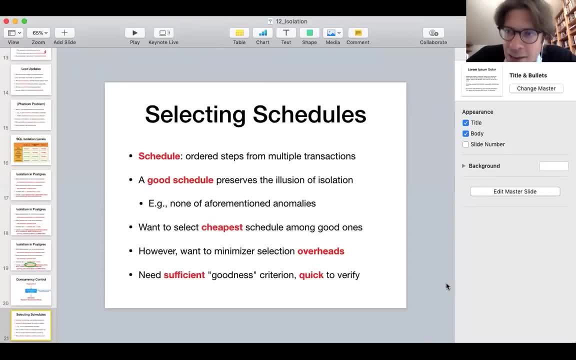 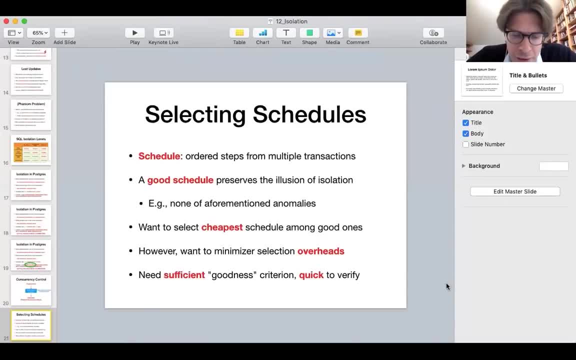 and what transactions you're executing on it. For instance, if you have something like: for instance, you have an online shop which has some kind of a visit counter for the website, which is also maintained in the database. Now, if the number of visits is a little bit off to what you would actually expect, it might. 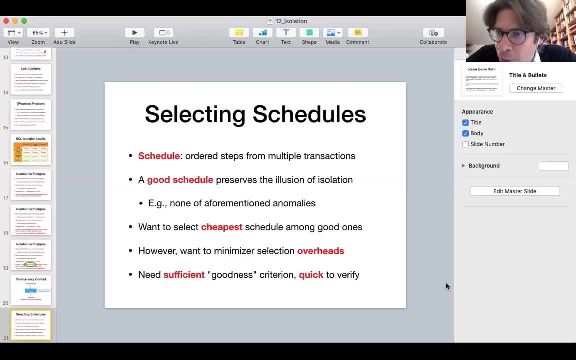 not be the end of the world. I mean, if you can get significantly better performance in your visit, count of the website might be a little bit off. you would probably accept it. Now, on the other side, when it comes to things like orders, when it comes to updating your 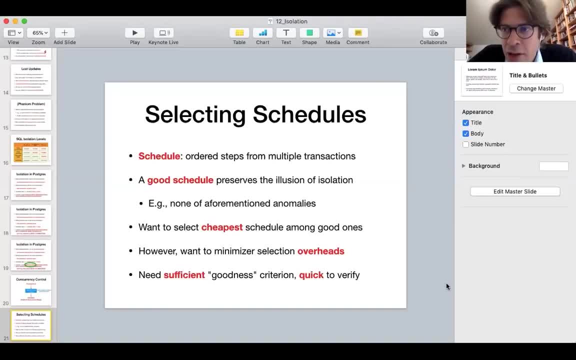 inventory list, then those are things that are highly critical, that you want to avoid any strange behavior. So that is why SQL allows you to set the isolation level for specific transactions, so you can distinguish the ones that are more important from the ones where a little bit of strange behavior might be acceptable. 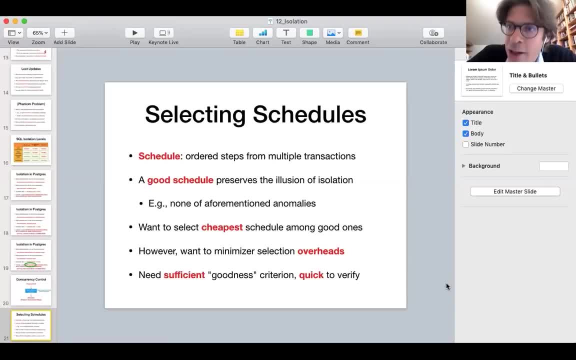 So it depends entirely on your application, but there is situations in which you probably want to accept a lower isolation level than serializable. Is there, at this point, any other questions on transactions? All right, okay, and there's one question about the difference between dirty and 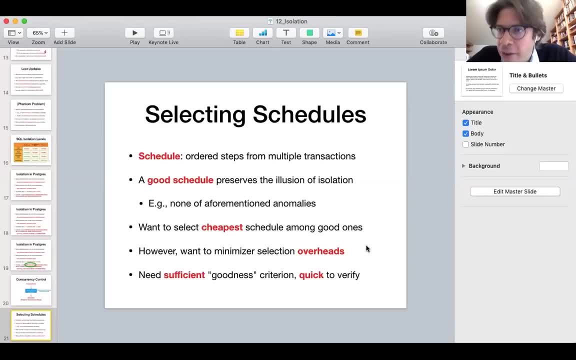 unrepeatable read, and that is a very justified question because it's a very common question, because there's some similarity between those two. I mean, in both cases we are reading something that we shouldn't really read. Now the thing is this: for dirty read, it means specifically, we are reading values from an uncommitted 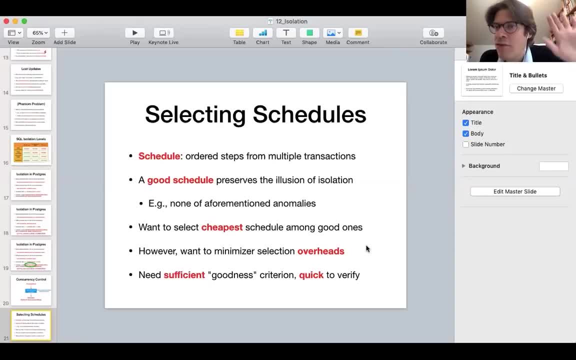 transaction. That means between. another transaction writes a value and I'm reading the value. there's no commit by the other transaction in between. Now for an unrepeatable read. the second read might actually be a dirty read because it's a very common thing. So we are reading the same value from another transaction, so we 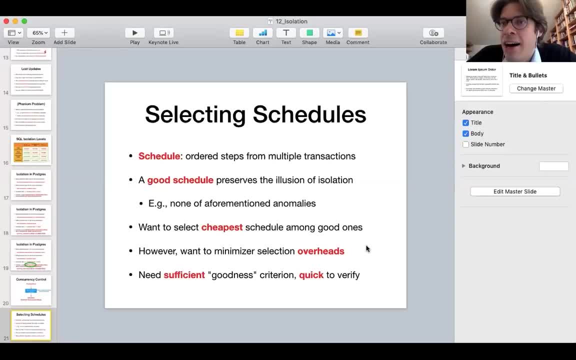 can definitely read some values from the transaction that has actually committed. So that means the transaction I'm reading from cannot abort anymore. but nevertheless it is an anomaly, because I have already read the same value before in the same transaction and now I see that those two values differ. So the 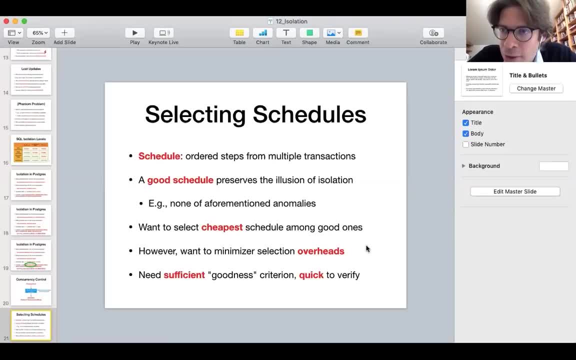 difference between the two is really on whether I'm reading committed or I might read a committed value which, however, differs from another committed value that I have read previously in the same transaction, And there's some question about whether people could maybe exploit those lower isolation levels in order to increase the visitor count. 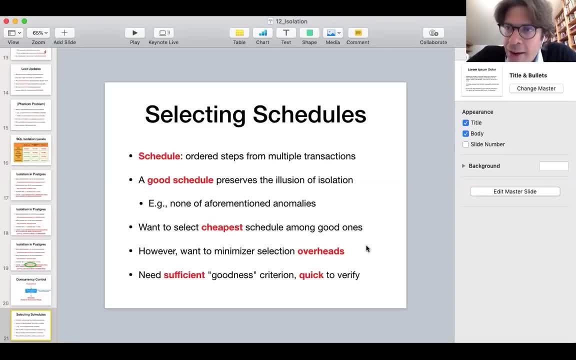 That depends a lot on how your data looks like and how your transactions look like. I mean, in general, the visitor count. I use that as an example for something where you might be willing to accept the values that deviate from the real values. 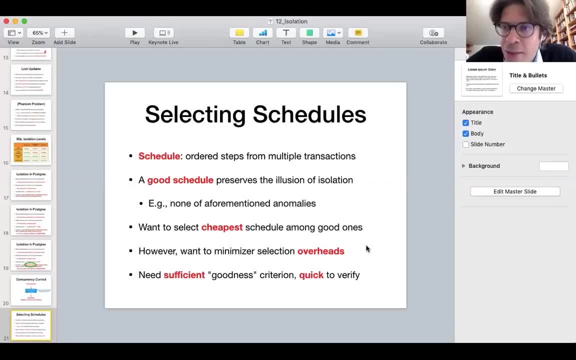 Perhaps in practice, if you see that your visit count seems to deviate by a lot from what you are actually expecting, then you might decide to also make that transaction serializable, the one that is updating the visitor count, But probably it's a piece of your database. 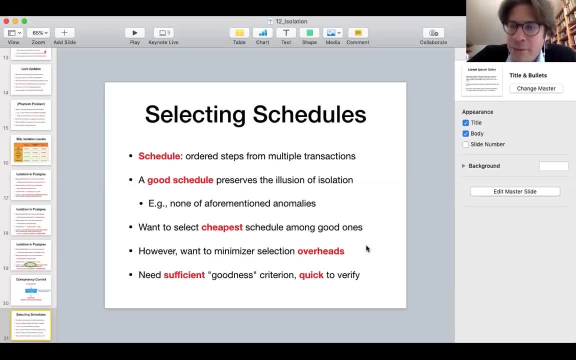 That is less critical than others. All right, good. So that was an introduction to transactions and we have started discussing about isolation. In the following lectures, we will discuss in more detail about isolation and about methods by which we can achieve isolation. Have a nice day and I see you again on Wednesday. 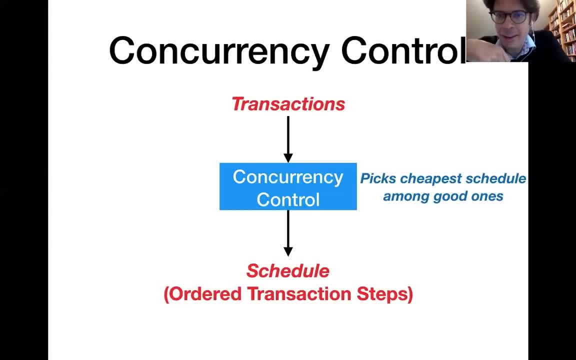 All right, let's get started. So The last time we have been discussing about transactions, which is the sequence of updates and queries that are semantically connected, And we have seen a few guarantees that the database system makes when executing those transactions. 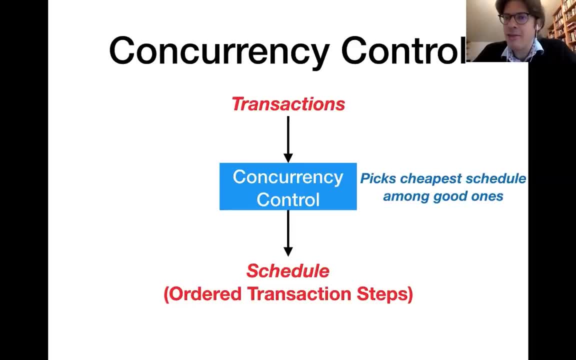 And one of those guarantees is that we isolate different users from each other which might be executing transactions concurrently on the same data, And if you are not careful, then this might lead to strange behavior from the user's perspective. So isolation is the guarantee that users will not be aware that multiple transactions are executing concurrently. 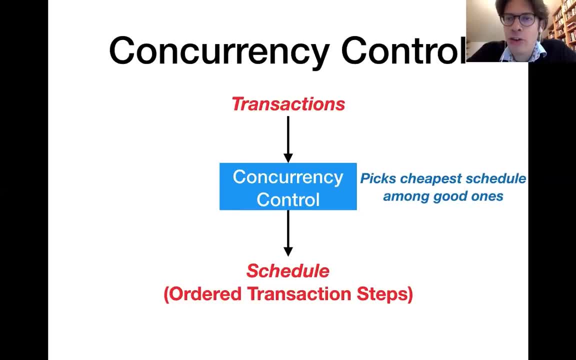 And the process by which we achieve that. that is called a concurrency control. Here you see the overview of what concurrency control achieves. The input is a set of transactions, Each transaction With a couple of Steps, And the output is basically a schedule which describes in which order the steps of different transactions are executed. 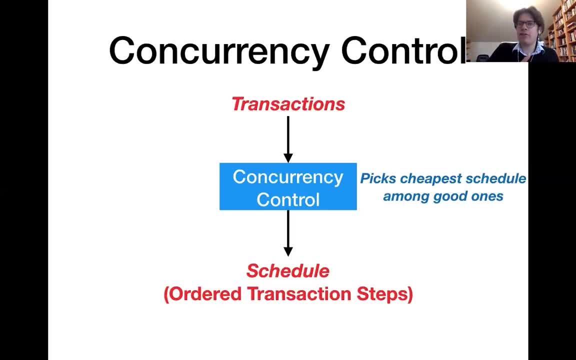 Now, that would be pretty simple as long as they execute one transaction after the other one, But for performance reasons, we don't want to do that. We want to interleave the steps of different transactions, And that means that we have to be careful when selecting a schedule. 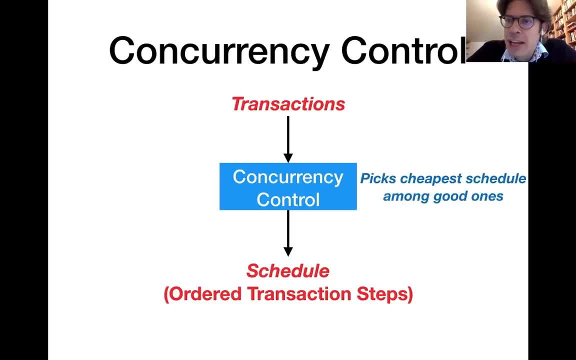 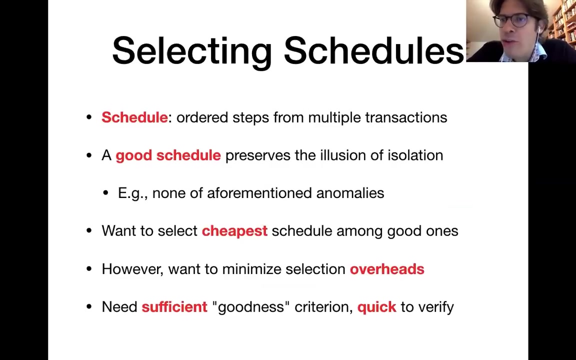 So the goal of concurrency control is to select a schedule which provides isolation while at the same time, being as efficient as possible. And all of this happens at runtime, So concurrency control also needs to be very efficient. So, first of all, in the following, we're going to discuss about how we select the schedule that we want to execute. 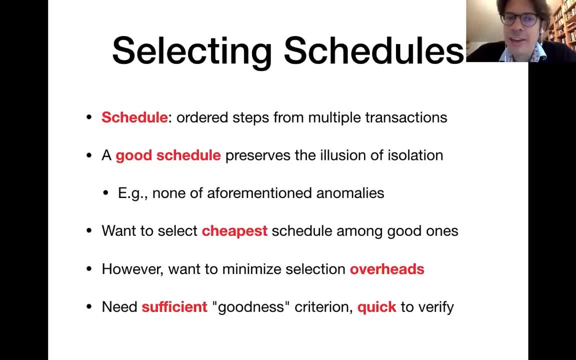 Now the schedule, as I have mentioned, that is, ordered steps, where each step is a read or write operation from multiple transactions, And a good schedule will provide isolation So users don't observe any of those anomalies that we have discussed last time. 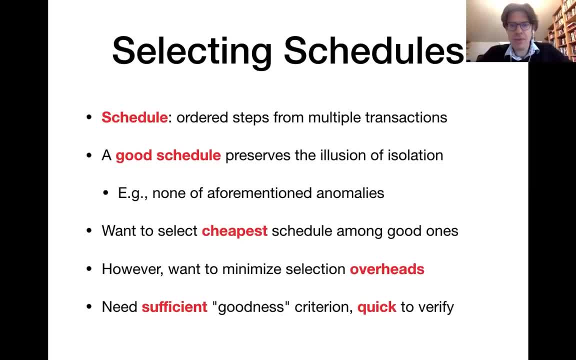 At the same time, a good schedule is cheap to execute. So we want to select ideally the cheapest schedule. So we want to select ideally the cheapest schedule Among the ones that avoid the relevant anomalies. On the other side, we want to reduce the overhead of concurrency control itself. 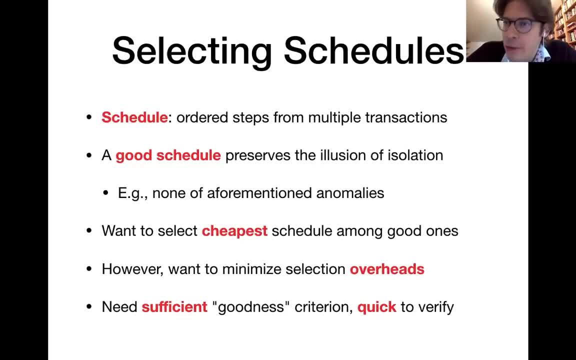 So that means we might make some kind of compromise. For instance, we might not consider all possible schedules when selecting the one for execution, But only a subset if doing so reduces the overheads of concurrency control. So in the following we're going to discuss about how we select the schedule that we want to execute. For instance, we might not consider all possible schedules when selecting the one for execution. We're going to discuss about how we select the schedule that we want to execute. We're going to discuss about how we select the schedule that we want to execute. 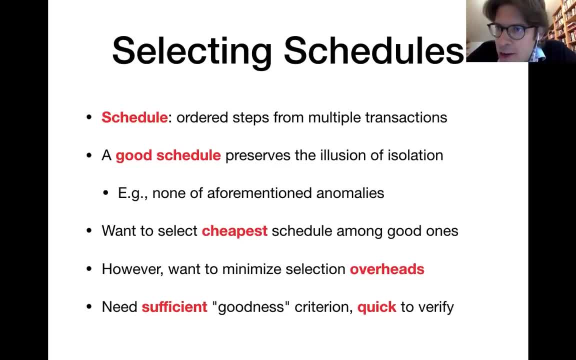 We're going to discuss about a couple of alternative criteria according to which we can select the schedules to execute. What we will finally come to is something like a sufficient goodness criterion for schedules that is quick to verify. So sufficient means that if this criterion is satisfied, 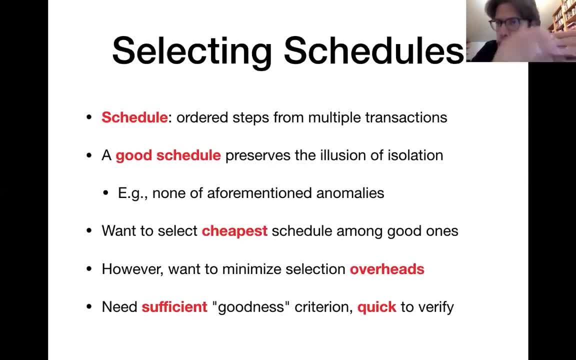 the schedule is guaranteed to be good to avoid the anomalies that we want to avoid. On the other side, there might be some good schedules that we are overlooking according to the criterion, because it is only a sufficient criterion and not a necessary criterion. So here we make a compromise, but in exchange we get a criterion that is: 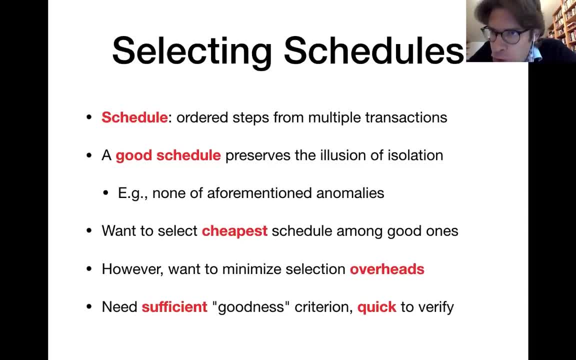 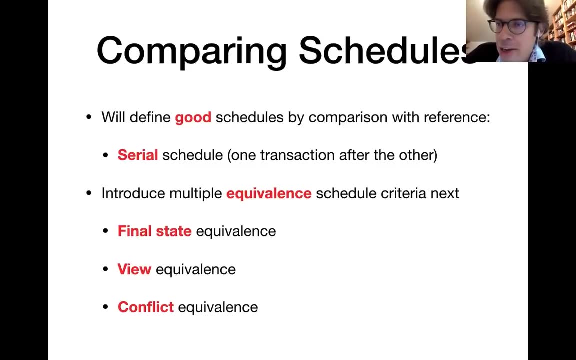 pretty quick to verify. so the overhead of concurrency control are known In the following when I discuss about a few different alternatives. So what is a good schedule? a good schedule generally avoids the anomalies which destroy the illusion of being the only user executing transactions at the same time. So we define good schedules by comparing. 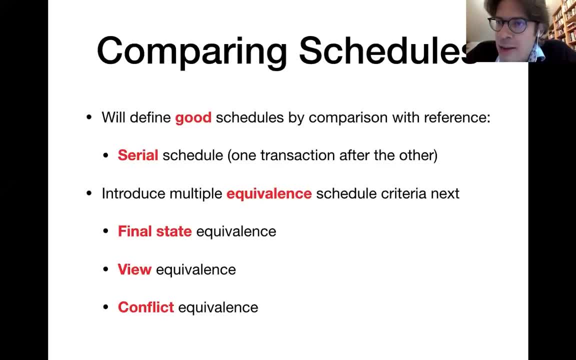 to a gold standard, which is essentially a serial schedule. So the user should feel as if transactions are executing serially, meaning one after the other one, while in reality we interleave the steps of different transactions. But if we compare a candidate's schedule to some serial schedule and we find that they 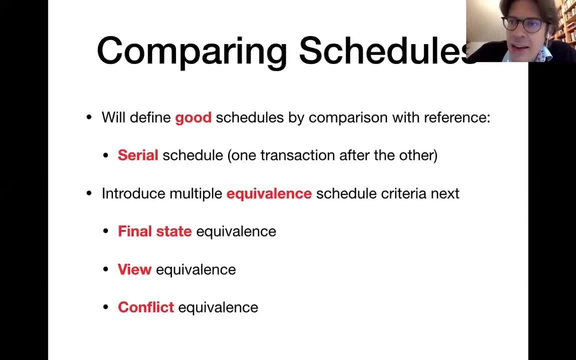 are equivalent, then we can conclude that a candidate's schedule is also good when it comes to isolation, because it looks like one of those serial schedules. So in the following we're gonna see a couple of criteria that allow us to compare different schedules against each other. We will see final state. 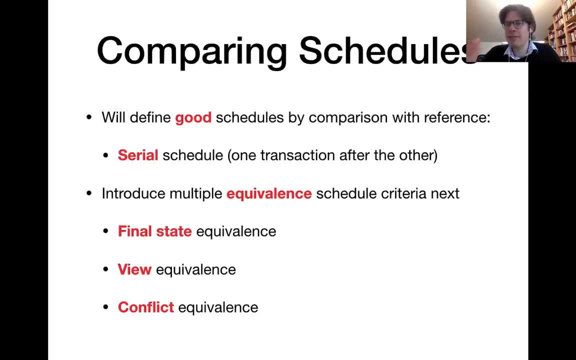 equivalence, where we compare essentially based on the final state that you have in your database after executing the two schedules. Then we compare according to view equivalence and that means when comparing two schedules, our users essentially see exactly the same things in the same order for both of those schedules, And conflict equivalence means that if you 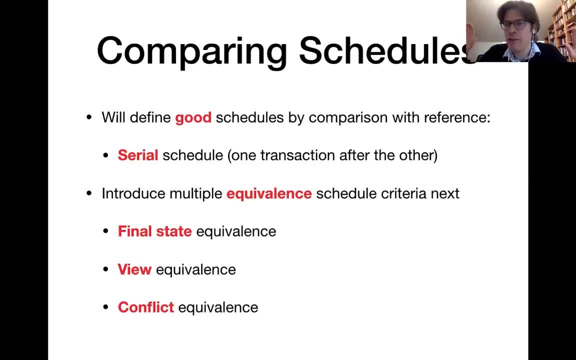 have pairs of steps in one of those schedules which conflicted with each other because, for instance, both steps, they change the value of the same object in the database- Then we essentially have those operations appear in the same order when comparing the two schedules. So in the following we're gonna see a couple of criteria that allow us to compare. 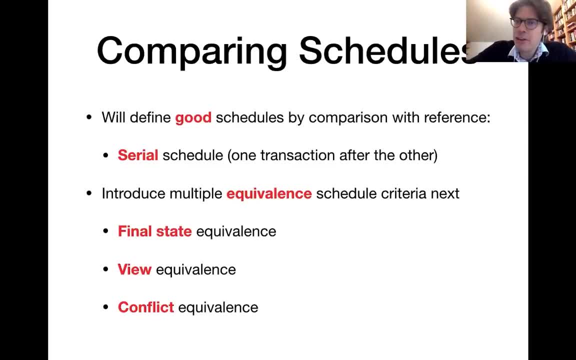 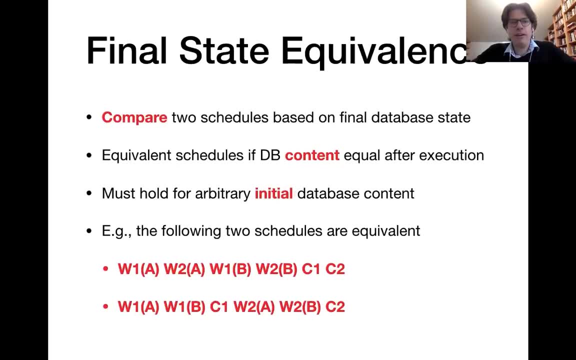 comparing those two different schedules. So this is an overview. Now we're gonna discuss those criteria in more detail, Starting with final state equivalence. So here we say that two schedules are equivalent if the final state of your database is the same after executing them, starting from an arbitrary starting. 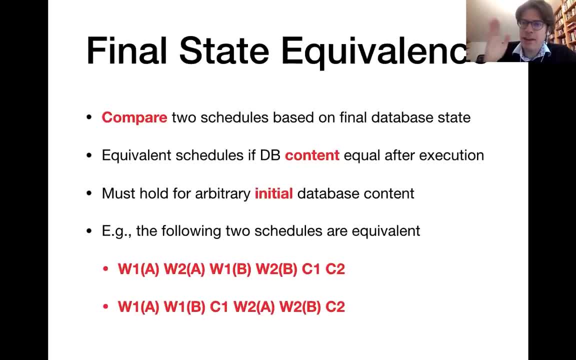 state All right. so, for instance, if If you look at those two example schedules here- and I'm gonna seize the opportunity to quickly remind you of the short notation for schedules that we have introduced last time- So here you have, those Ws. 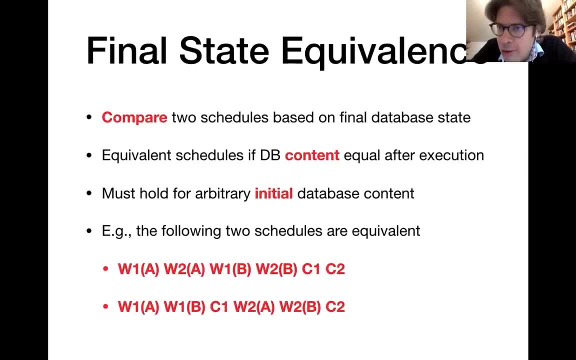 which always means a write operation. So we changed the value of an object in the database. Then you have those Rs. Actually, here you don't have Rs, but in general for the schedules that we will see on the next slides, you have Rs. 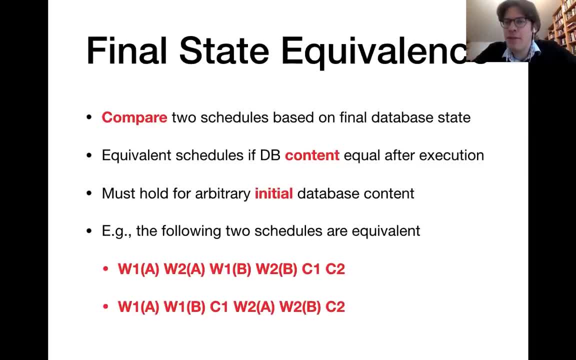 And in that case it's a read operation. They will read the value of an object in the database. With this notation you always have, for instance, the type of operation, which here is a write operations- W, followed by the idea of the transaction executing that step. 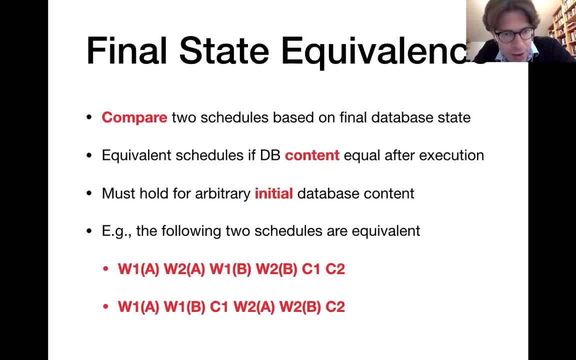 So we always use numbers for transactions. So here you are starting with a write operation by transaction one, And then, between parentheses, you always have the object in the database that the write operation refers to. So here we have object A, generically, And in reality concretely. that could for instance, 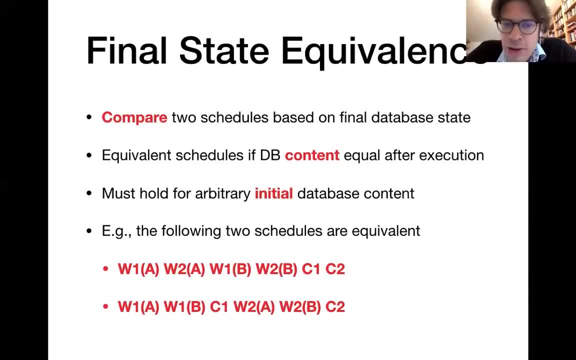 correspond to one row in your database. For instance, initially we had an example where we transferred money from the account of Alice to the account of Bob. Then you have to change values for those two database transactions. Okay, And here we have the question whether one query 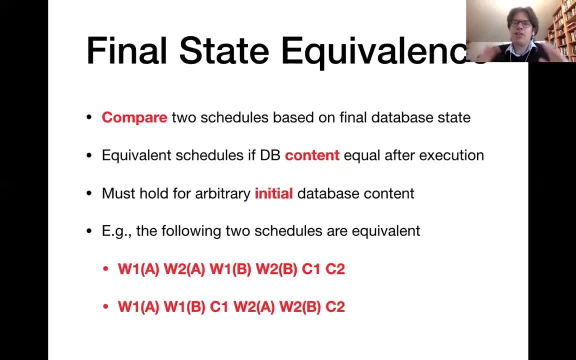 ever can have multiple transactions. So just to make sure queries are included as part of a transaction. So basically, one query would be a part of a transaction and update operations as well. All right, You also have the Cs here in this example schedule. 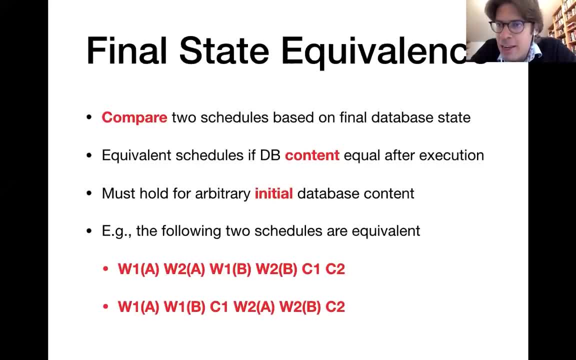 The C always means a commit operation And after the C you have the number of the transaction committing. So if a transaction commits, it always means that the transaction essentially is finished and wants to get executed. All right, Now here, when comparing those two examples, schedules: 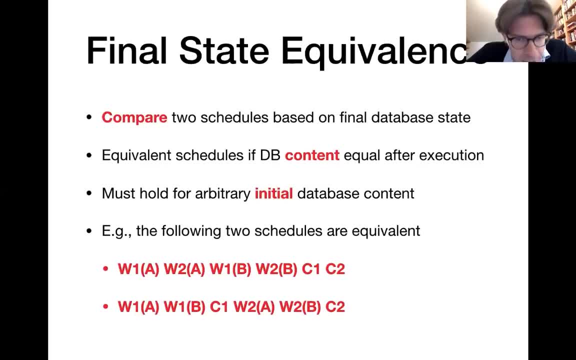 in the first schedule transaction one executes first and writes values to A And Okay. so here actually in the first schedule we have first the write operation by transaction one to object A. Then we have a write operation by transaction two to object A. 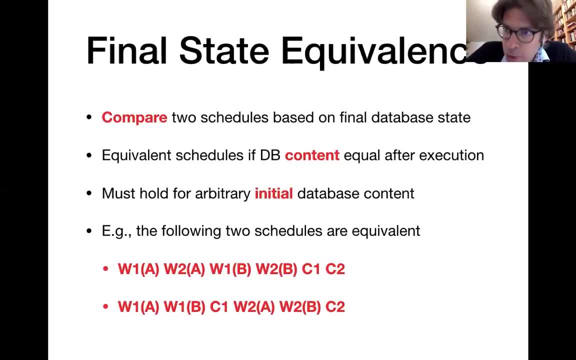 So the final value for A will be written by transaction number two. Then we have a write operation by transaction one to object B, followed by a write by transaction two to object B. So also for B the final value will be written by transaction two. 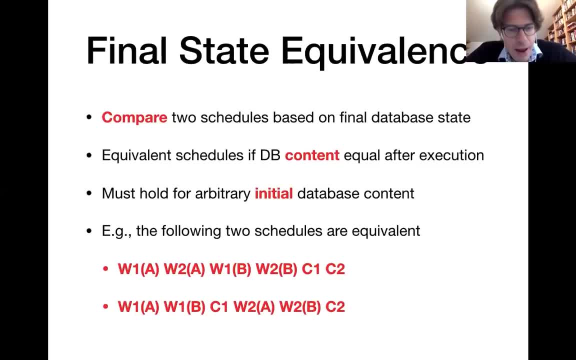 And finally both of those transactions commit. Now the second schedule over here first writes a value for object A via transaction one, Then transaction one writes also the value for B and commits After that. transaction two writes the value for A and the value for B. 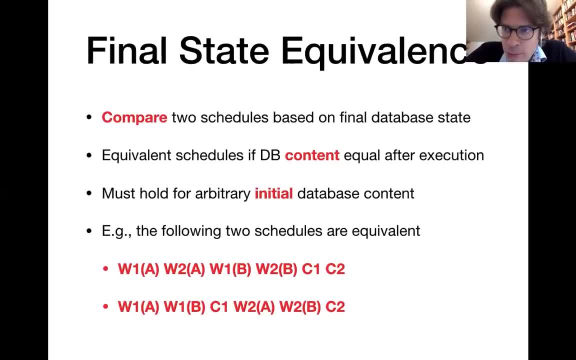 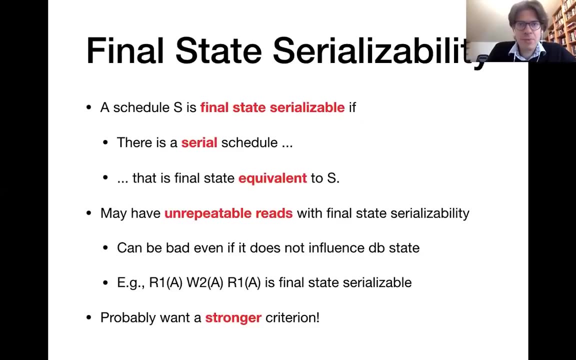 So when comparing those schedules, then in both of them transaction number two writes the final values for object A and B, And that is why those two schedules are final state equivalent. If we say that a schedule is final state serializable, it means that there is some serial schedule. 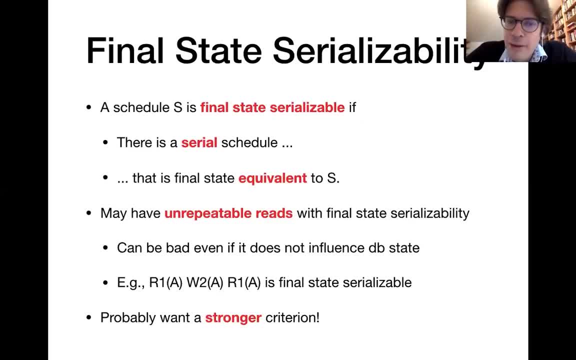 which contains the same transactions. That is a final state equivalent to that schedule that we are analyzing. And this other schedule that we are comparing against must be a serial schedule executing transactions one after the other one. So a schedule is final state, serializable. 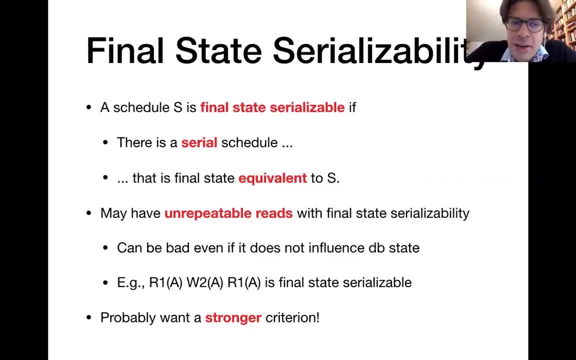 if you can find a final state equivalent serial schedule. Now, final state equivalents can be efficiently verified, which is good, but on the other side, it is not sufficiently strong as a criterion in order to avoid all those strange anomalies that we have discussed in the previous lecture. 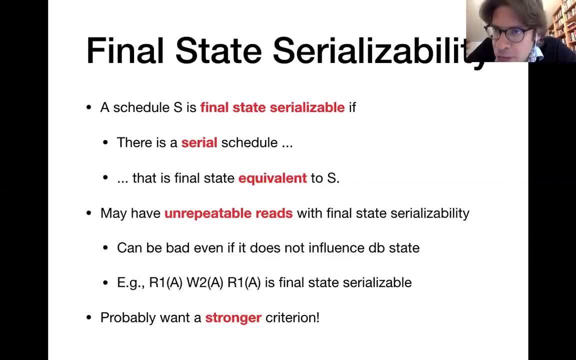 For instance- we have heard about this anomaly- unrepeatable reads, where I read one value once and then later I read it a second time And the value has been changed in the meantime by another transaction. So that is bad And even if a schedule is final state, serializable. 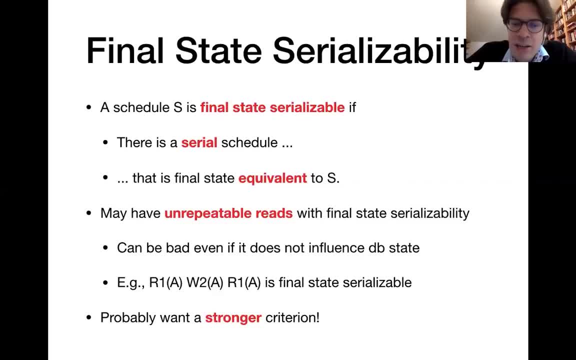 it could still have those unrepeatable read anomalies. So for instance, if you look at this schedule over here, we have first a read by transaction one of object A, then a write by transaction two to object A and finally another read by a transaction one of object A. 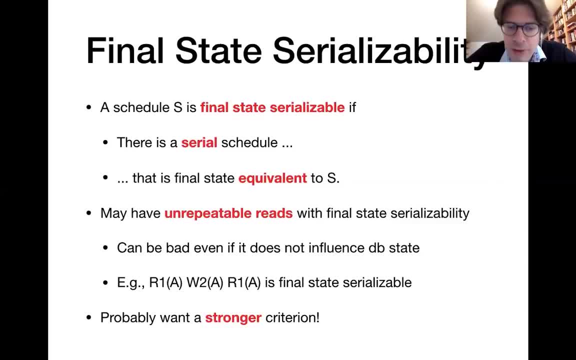 So here you have an unrepeatable read, because the second transaction might have changed the value of A in the meantime. On the other side, the schedule is final state serializable because transaction number two writes the final value for A in any case. All right. 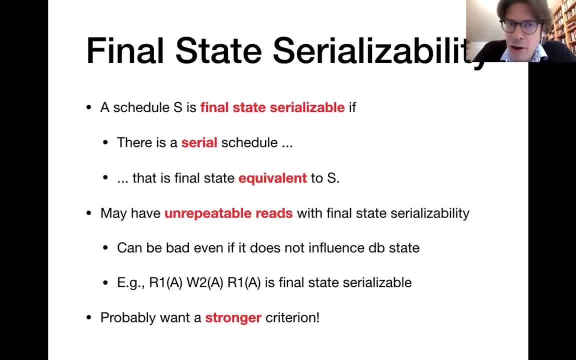 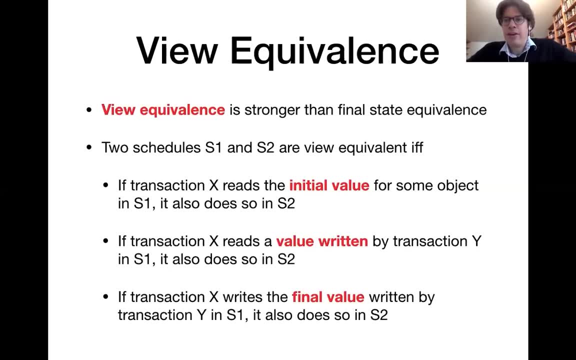 So probably we want a stronger criterion than final state serializability. That leads to a view equivalence And there we compare two schedules based on what the user sees in each order, And we have a whole bunch of conditions such that two schedules, S1 and S2, are a view equivalent. 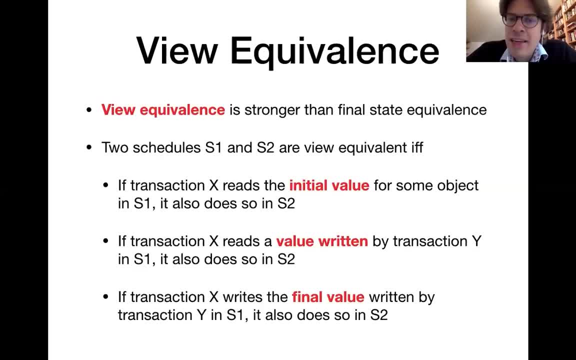 First of all, if some transaction reads the initial value, before scheduled execution starts, of some object in one schedule, then it must also do so in the other schedule. Also, if a transaction reads the value of an object that was written by another transaction before, then it must also do so in the other schedule. 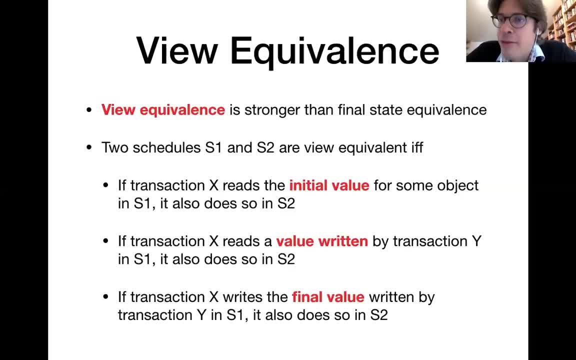 And then, finally, if some transaction writes the final value of an object in the first schedule, it must also do so in the second schedule. So we require all three conditions in order to say that those two schedules are view equivalent. Now you see, here we have some conditions that 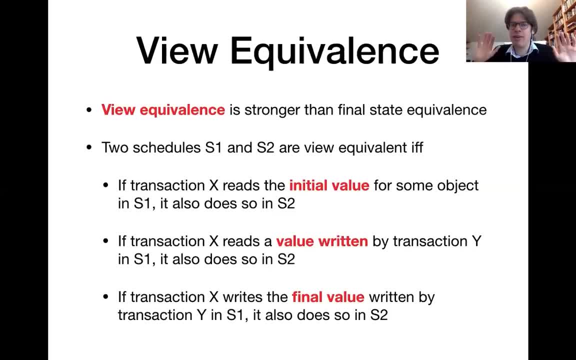 relate to the final state of the database, because if the final value was written by a transaction in one schedule, it must also have been written by that transaction in the other schedule. But we additionally have some conditions which refer to what the user sees or what the transaction. 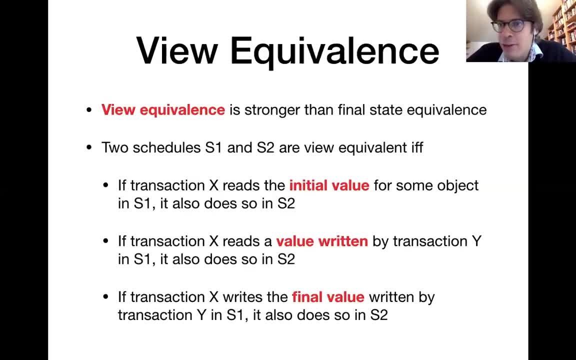 sees The transaction has seen the initial value in one schedule, it must also see it in the other schedule. and if transaction has seen the value written by another transaction in the first schedule, then it must also do so in the second schedule, In the second one. and that is where the name view serializable comes from. 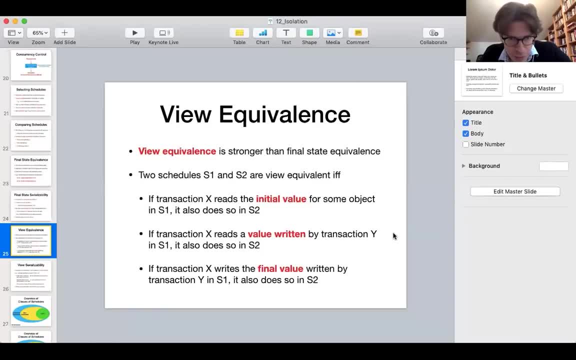 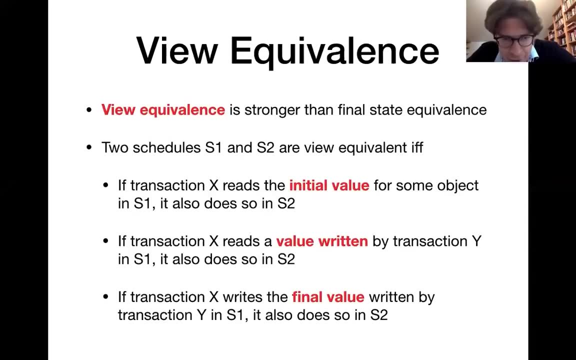 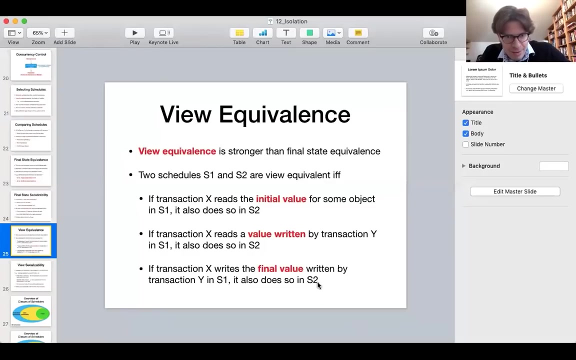 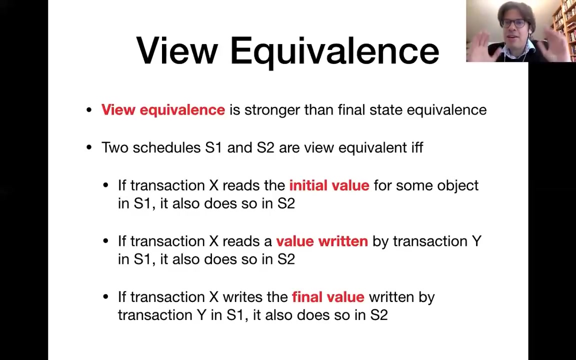 And here, all right. and there's a question in the chat that refers to a little typo here. So the last point actually should be that if a transaction x writes the final value in s1, it also does so in s2.. Can, yeah, so that is a little typo. Thank you, All right. so here the last condition, basically. 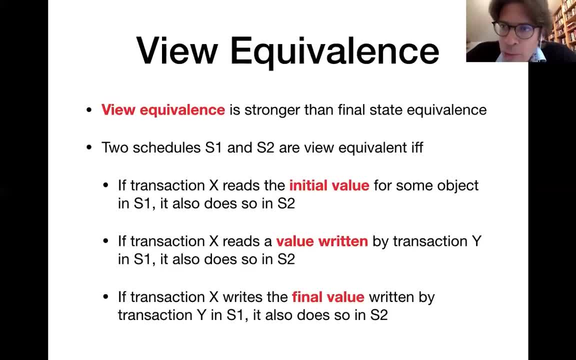 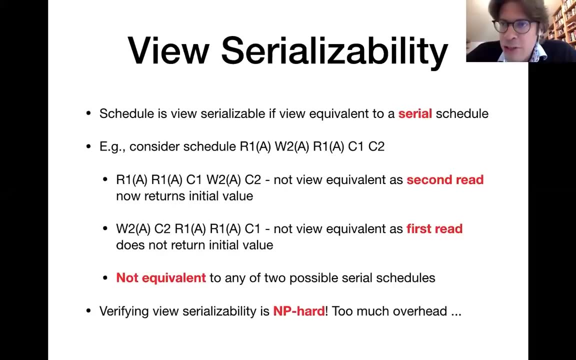 means that the final value of those objects should not change when comparing the two schedules. So that is basically referring back to final state serializability. All right, and then view serializability again means that we find a serial schedule which is view equivalent to the schedule that we are analyzing. 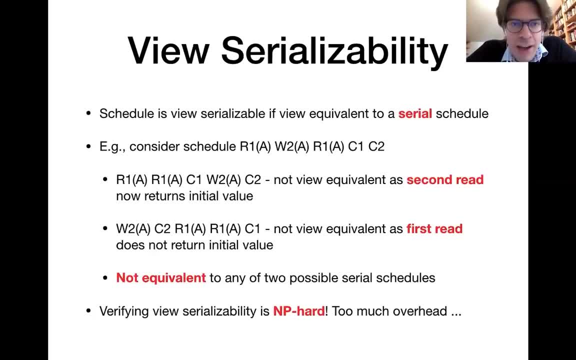 So for instance, here's an example where we are trying to determine whether a specific schedule is a view serializable. So in our case we see the schedule that we are analyzing here. First we are reading the value of object A by transaction one. Then we are writing. then transaction two writes the value. 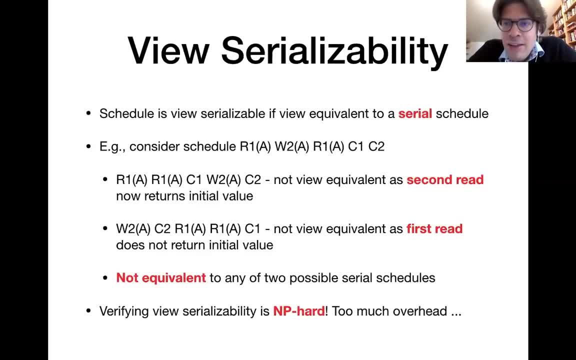 for object A And then transaction. one reads the value for A again. So this is the schedule that we have already seen before and here we have potentially an unrepeatable read. So we expect that the schedule is not a view serializable. So then we see that we are seeing a serialization After each transaction. when we have an evaluation, we see that there is no value in s1 ascoming s2.. After each transaction, we see that there is nothing, So there are no values in s1.. So this is the schedule that we are analyzing. 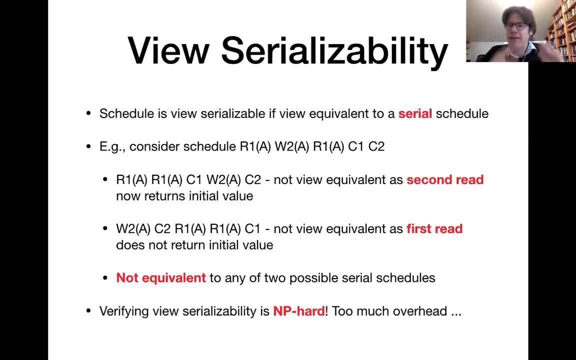 So, for instance, we see that we see a value in s1 as an option, which is view equivalent to the schedule is not view serializable, but let's make sure. So, since we have two transactions that appear in this schedule, there's exactly two possible. 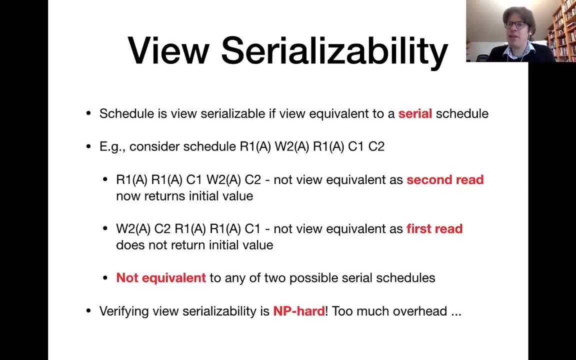 serial schedules that we can compare against. Either we first execute the first transaction and then the second transaction, or we first execute the second transaction and then the first transaction. Now, here we have both possibilities. So either we could have the first transaction execute first. 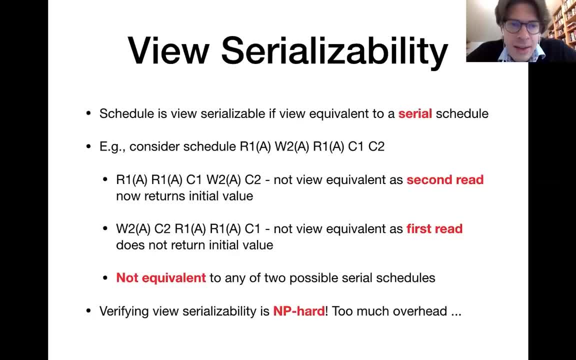 and followed by the second transaction. But this schedule, the serial schedule, is not view equivalent to the schedule that we are analyzing because the second read of object A in one schedule it reads the value of written by the second transaction. In the other schedule it reads the initial value. 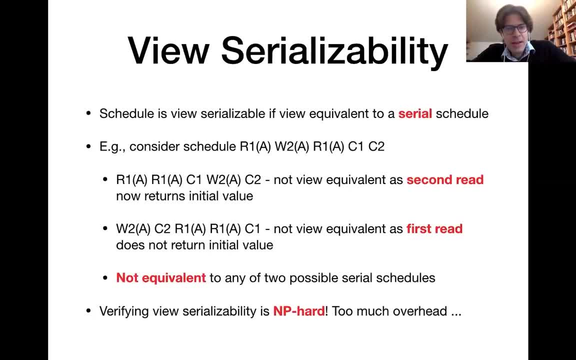 So that violates one of the three conditions. In the other case, where we execute the second transaction first, we have that both reads of A by the first transaction. They read the value written by the second transaction, but none of them reads the initial value. 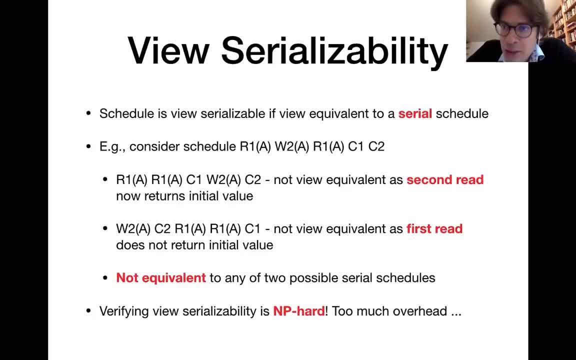 And in the schedule that we are comparing against one of those two read operations reads the initial value of object A, And because we cannot find any serial schedule that is view equivalent of the schedule that we are analyzing, therefore the schedule is not view serializable. 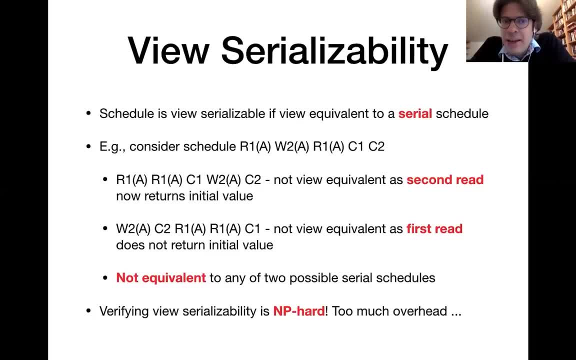 View serializability seems like a nice criterion. It is pretty strong, So it avoids those anomalies that we have seen. The only problem with that criterion is that it is not is that it is NP-hard in general to verify whether a schedule is view serializable. 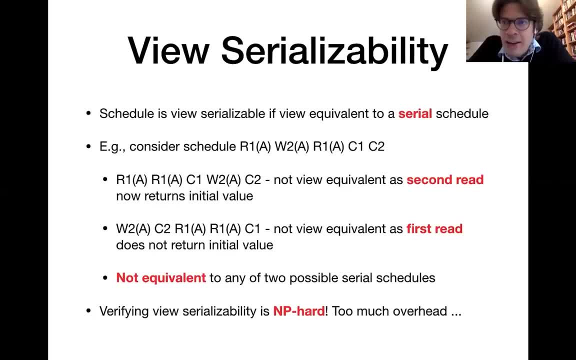 And NP-hard generally means that we don't know and don't believe that there exist any efficient algorithms in order to solve that problem And selecting a schedule. that is something that the concurrency control component needs to do at runtime very quickly once transactions are being submitted. 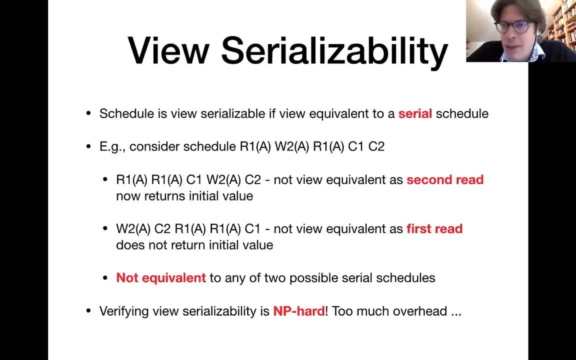 So we most definitely don't want to have a schedule that is not view serializable. So we most definitely don't want to have a schedule. that is something that the concurrency control component needs to do at runtime very quickly, once transactions are being submitted, to solve any NP-hard problems at runtime. 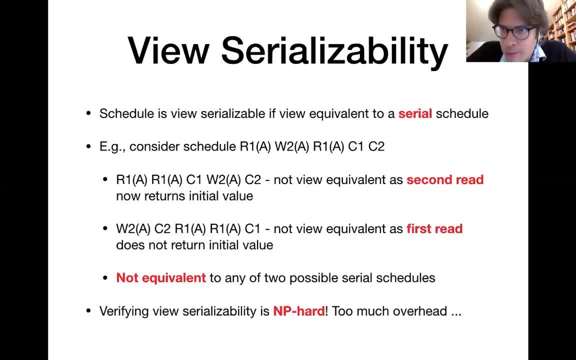 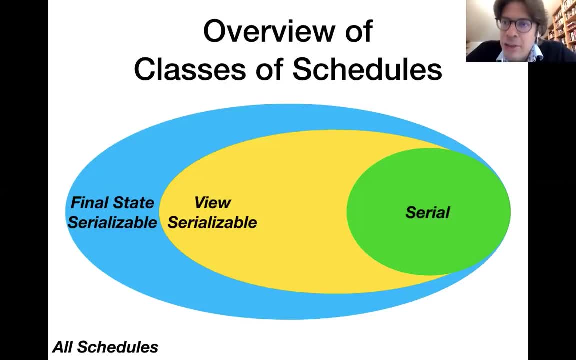 because that would slow down the entire database system. So this is an overview of what we have seen so far. This is an illustration of the different classes of schedules that we have been discussing about, as well as how those different classes of schedules relate to each other. 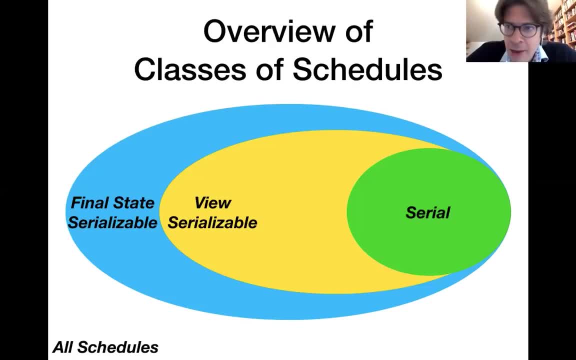 You see that we have inclusions. among them, We have a, first of all, a set of all possible schedules which contain the same transactions. Then you have the subset of schedules that are final state serializable. Then you have the even smaller subset of schedules that are view serializable And finally you 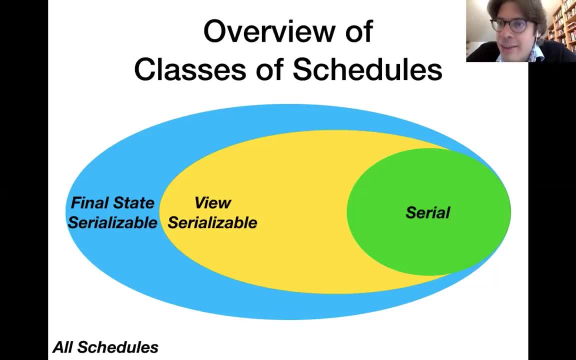 have the small set of schedules that are indeed serial. So all of those inclusions are proper. so you can always find the schedules that are included in the larger class but not in the smaller class. Now, having discussed all of those different classes of schedules, our final goal is to select the class of schedules. 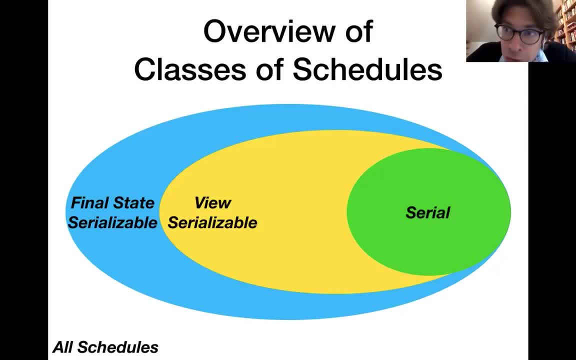 that we want to aim for in concurrency control. Now, serial schedules are easy to verify but they are very slow to execute. We have seen a couple of motivations for why we want to avoid the serialized schedules. Now, serialized schedules are easy to verify but they are very slow to execute. We have seen a couple of motivations for why we want to avoid the serialized schedules. 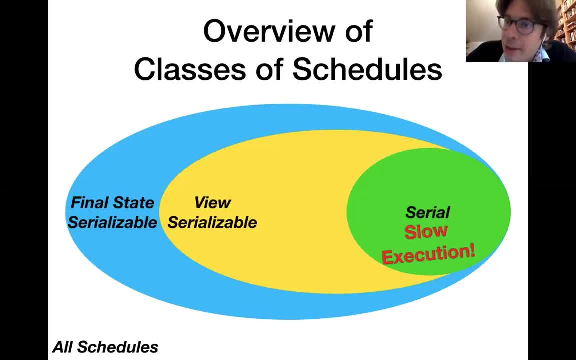 Serial schedules that execute one transactions after the other one last time We have seen view serializable schedules, but the problem with them is that they make concurrency control very slow because we would have to solve NP-hard problems. We have seen final state serializable schedules, but here the 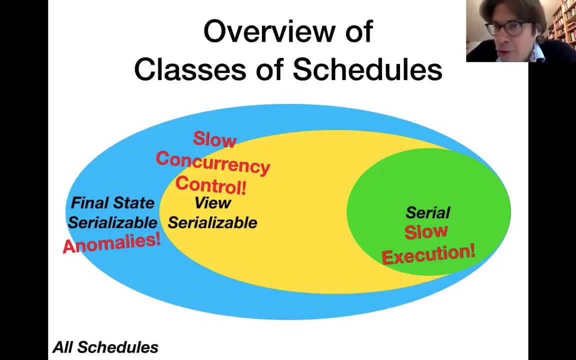 problem is that we might have anomalies. so we destroy the illusion of isolation And then we have the set of all schedules and there we have a pre-ிn Avi- not exactly the same problem. So in a way none of those classes of schedules seems to be a good choice for aiming as a goal in concurrency control. 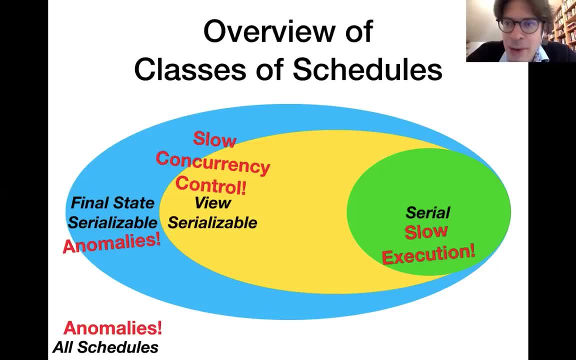 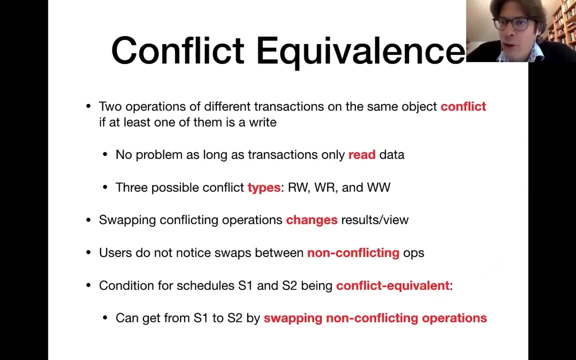 So we need something else, and in the following, we're going to discuss an alternative class of schedules that is a much better compromise between those different quality criteria. All right, now, the class of schedules that that we will be aiming for is a conflict- serializable schedules- and so, first of 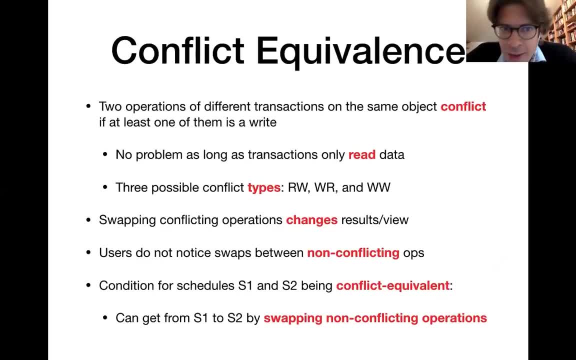 all, we introduce a conflict equivalence and to say that two schedules are conflict equivalent if they have the same conflicts appearing in them. now what is a conflict? so a conflict arises between two steps of like, two different transactions if they operate on the same object and one of those operations is a. 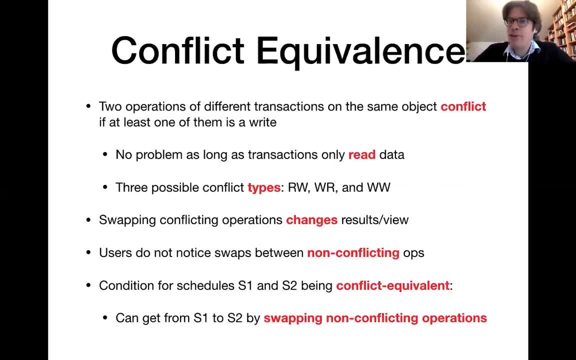 right operation. that is important because as long as transactions are just reading data, everything is fine and nothing bad can happen. but as soon as transactions not changing the data, this is where we need to be careful that we don't interleave transactions in a bad manner. so for a conflict we must have two operations by different. 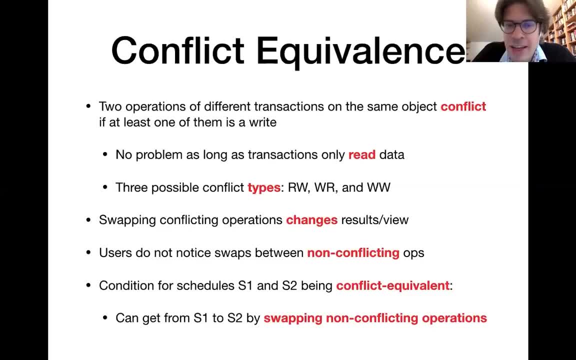 transactions where one of those operations is right operation, that Racing esos concept. importantly, Si possibilities, we could either have first read by the first transaction followed by a write on the same object by the second transaction, or we could have first write by the first transaction followed by a. 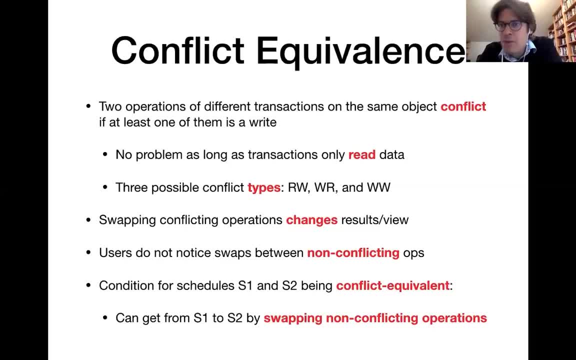 read of the transactions. so we simply have the transaction read at any angle to see if we made a difference in the Experience control. big chunks increase in by the second transaction. Or we could have two writes by two different transactions on the same object. Those are the possibilities Whenever I change. 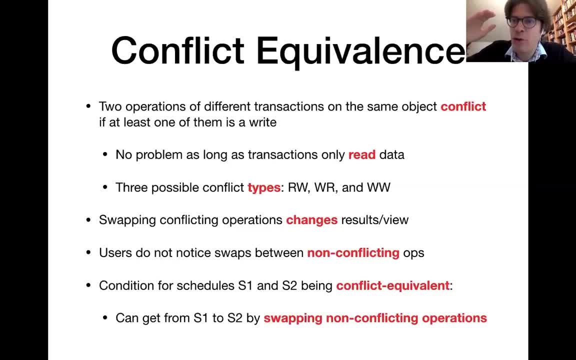 the order of some of those conflicting operations, so I change the order in the schedule. whenever I do that, I have a risk of creating differences either in terms of the final state of the database or in terms of what the users see in which order. On the other side, as long as I only change the 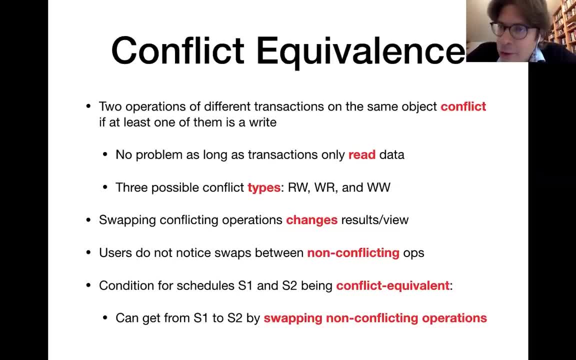 ordering between non-conflicting operations, I cannot have any of those bad effects. The final state will be the same and also users will see the same things in the same order. So I can say that two schedules are different, Conflict equivalent. if I get from one schedule to the other one by only 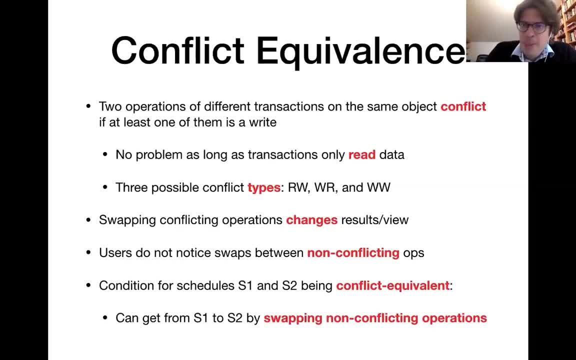 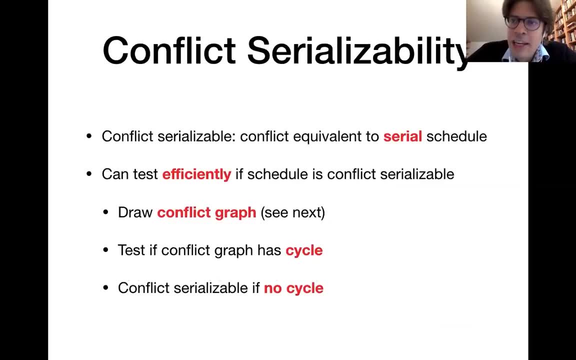 swapping non-conflicting operations And in line with that, we have conflict serializability. The schedule is set to be conflict serializable if there is a serial schedule and I can make sure that the serial schedule is conflict equivalent to the schedule that I am analyzing Now for a given set of. 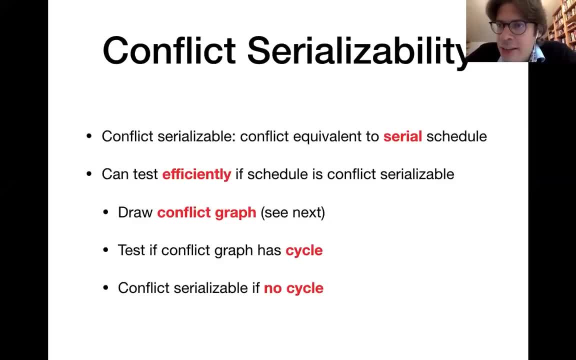 transactions, I have to make sure that the serial schedule is conflict equivalent to the schedule that I am analyzing Now for a given set of transactions. of course, there's many different serial schedules, So I don't want to try out all of them and compare them in terms of conflict. 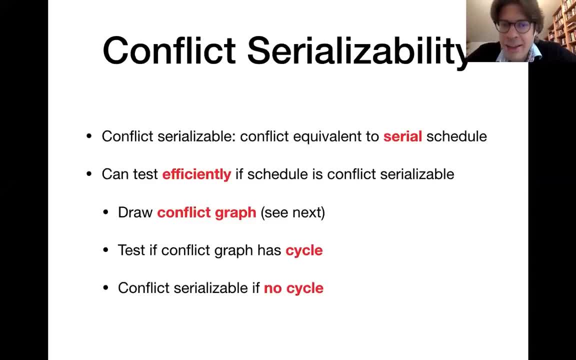 serializability in conflict of conflict equivalence. Instead, I want a more efficient method to test whether a given schedule is conflict serializable, And we can do that by the method that I'm going to describe in the following. It involves drawing a so-called conflict serialization. 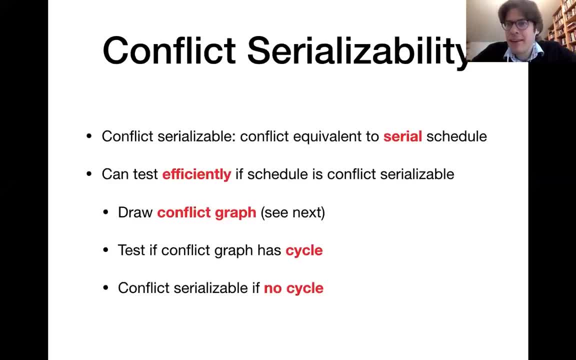 We will see in a second how to define that conflict graph for a given schedule. But it comes in the end down to testing whether this conflict graph has a cycle, And the schedule is only conflict serializable if this graph has no schedule, and that is something. it has no cycle and that is something that we can. 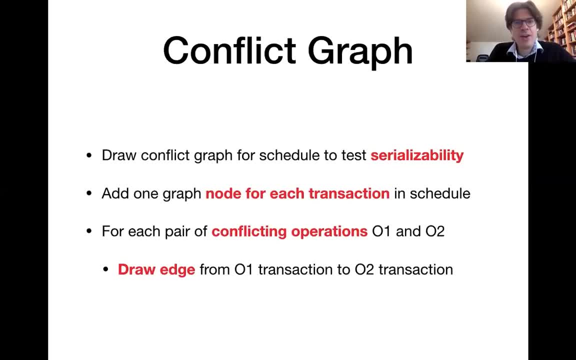 test very efficiently. All right, So this is the definition of the conflict graph. So if we want to find out whether one schedule is conflict serializable, then you're drawing this conflict graph for it And in the conflict graph you're introducing one. 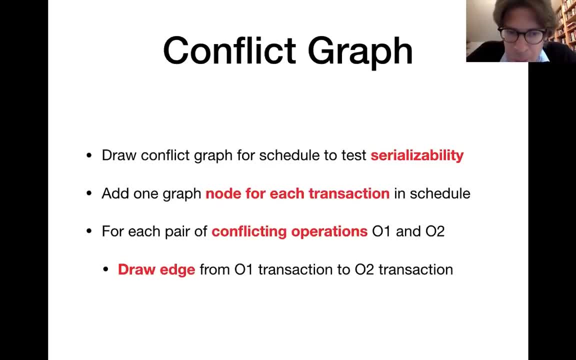 node for each of those transactions in the schedule And then for each pair of conflicting operations by two different transactions: operation 01 and operation 02.. We draw an edge from the transaction to which 01 belongs to the transaction to which 02 belongs. So this edge in the conflict graph basically indicates a conflicting operation. 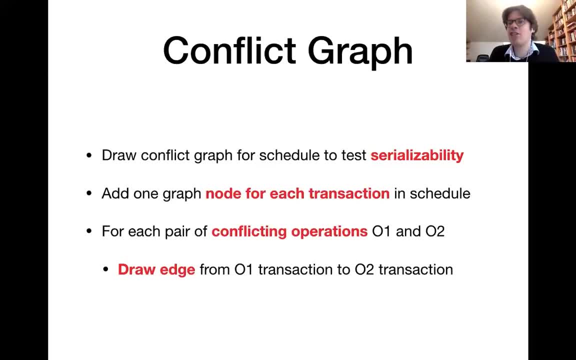 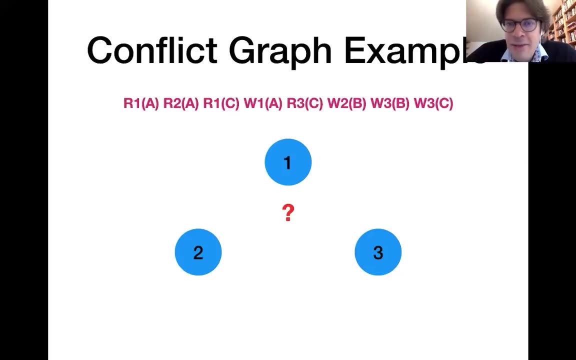 between those two transactions. We draw that edge from the earlier transaction, from the transaction with the earlier operation to the transaction with the later operation. Let's make a little example. So here we have a schedule, given on top in purple. It involves: 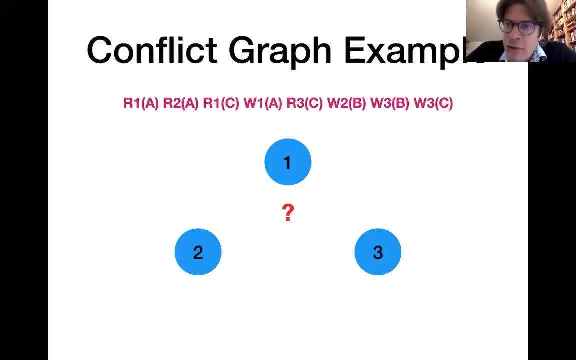 a three transactions. So definitely the conflict graph must have three nodes. Now can anyone tell me which conflict edges I should draw in my conflict graph over here? Or at least can anyone identify, for instance, one pair? Can anyone tell me which conflict edges I should draw in my conflict graph over here? 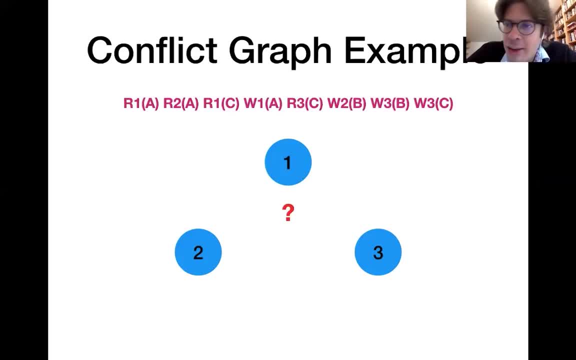 Or at least can anyone tell me which conflict edges I should draw in my conflict graph over here And tell me what edge I need to draw in the conflict graph because of it In the chat, please? Okay, there's a couple of things coming in, Okay, good, So in general, two operations conflict. 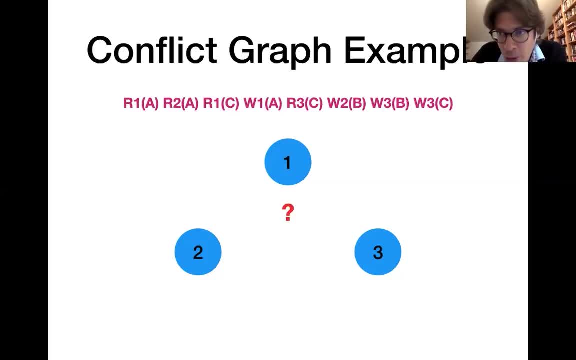 Okay, good. So in general, two operations conflict, I think are going to give the result that if they belong to different transactions, they operate on the same object and at least one of those operations is a right operation. So here, for instance, we have the proposition r1 followed by w3. 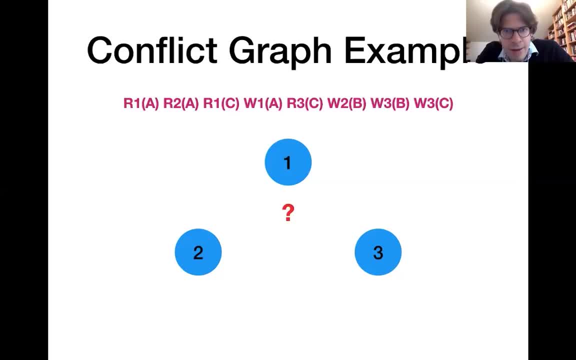 So let's see here r1, we have it here, Then w3, we have that at the very end. exactly the same object. we have different transactions and one of them is the right operation, and that means that we want to draw a line from the first transaction to the third transaction. 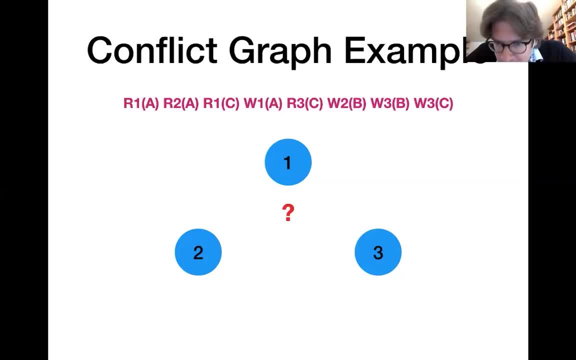 all right, w2 b and w3 b. all right, okay, exactly. so here we have two conflicting operations following each other immediately, um one right to be by transaction two and one right to be by transaction three. transaction two goes first, so we want an edge from transaction two to 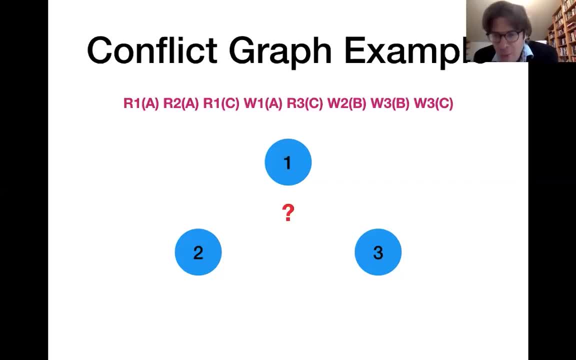 transaction three. now we have another one, w1a to r2a. all right, where do we have w1a? okay, um, so r2a goes first, right? so, um, we first have the read of a by transaction two and later we have the right to a by transaction one. so we 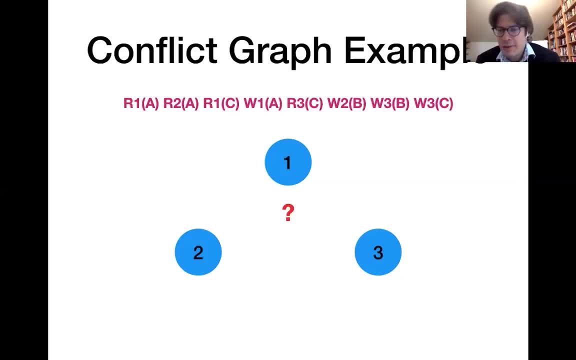 would want to draw a line from two to one. so this is the principle: compare passive operations in the schedule and see whether they conflict and then draw the corresponding edges in the conflict graph. so we have collected all of them here. now i'm drawing the edges. i believe we covered all of them very good. 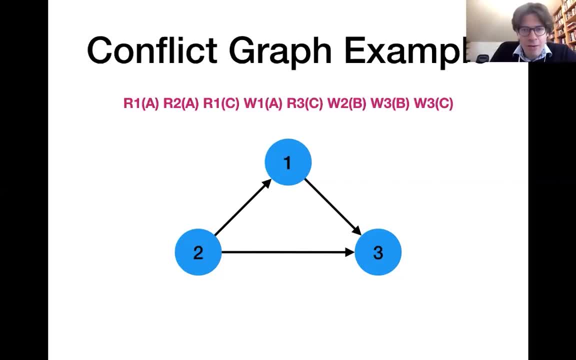 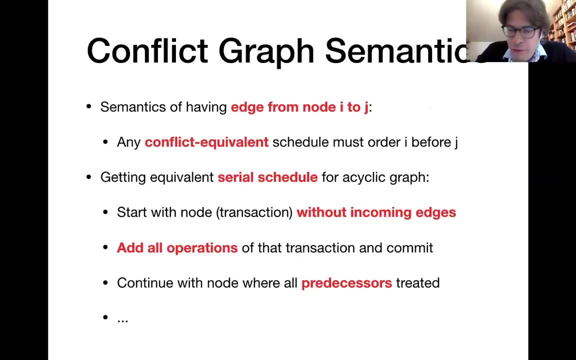 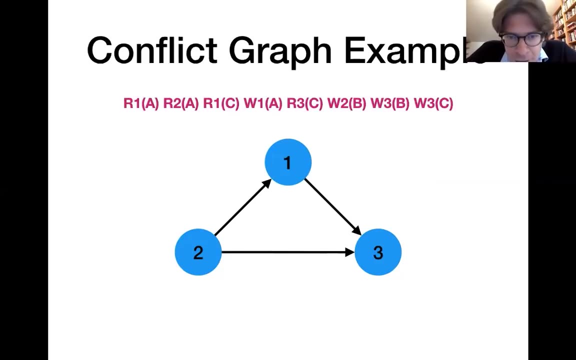 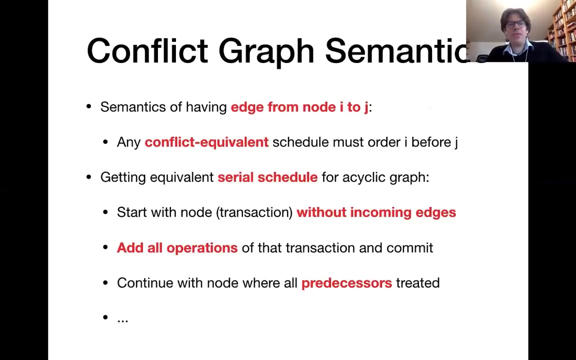 all right, so that is the conflict graph. and finally, um, i would have to check whether that conflict graph has a cycle or not, and this is the number of the actual contracts we have and case we don't have a cycle. so this one is a conflict serializable. all right, so. 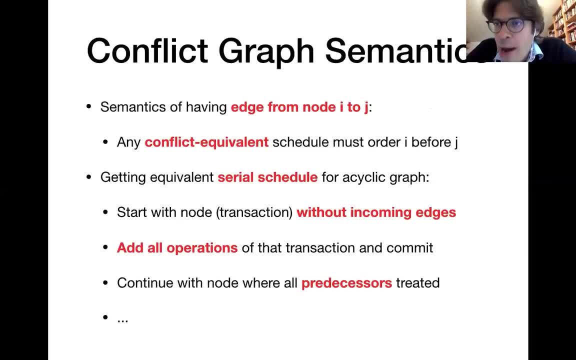 perhaps to illustrate that point a little bit more, why is it that you're looking for cycles? so if you have an edge from some node I to a node J, representing two different transactions, then it's actually means that any conflict equivalent serial schedule must order transaction I before transaction J. 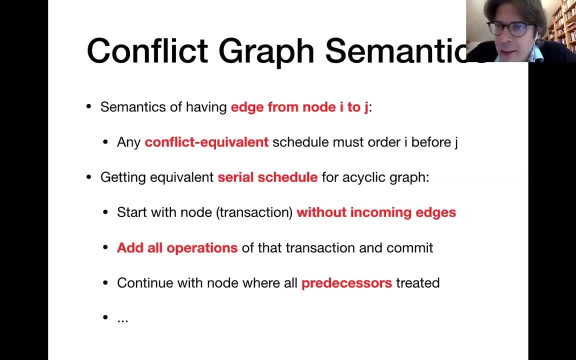 in order to avoid swapping the order of those conflicting operations and, because of that semantics, the way in which I can transform one schedule that is conflict serializable into the conflict equivalent serial schedule, it's by essentially doing a topological sort in the conflict graph. so essentially I start first of all with 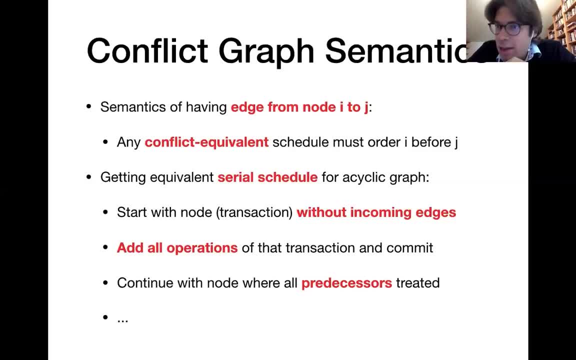 the transaction whose node has no incoming edges. then I take all the operations of the transaction and write them into my new conflict, the equivalent serial schedule. then I continue finding one node where all incoming edges belong to transactions that have already been treated, and I continue doing this until finally I know that I have treated all. 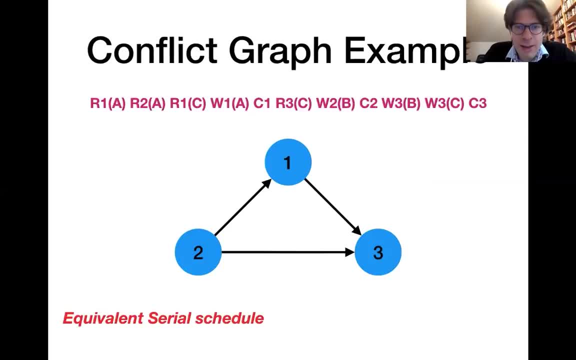 the transactions in the current schedule. for instance, in this example over here, we would first start with a transaction 2, because node 2 has no incoming edges, so I can order the order of each transaction in that node and then run the Melanome C operations of that transaction first. 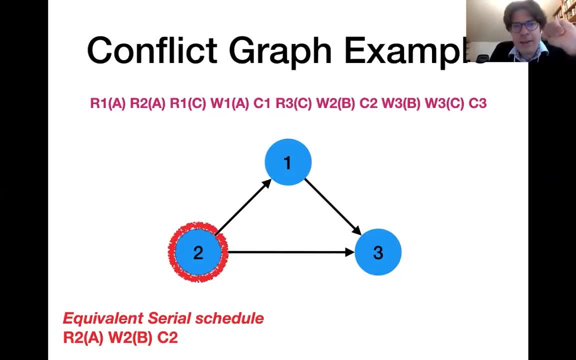 Now node one next doesn't have any incoming access from nodes that haven't been treated yet, So I'm gonna put transaction one next. And now, finally, I can put the operations of transaction three, And now I have a serial schedule that is conflict equivalent to the original schedule. 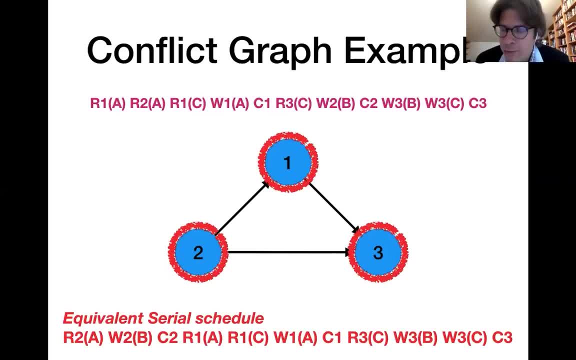 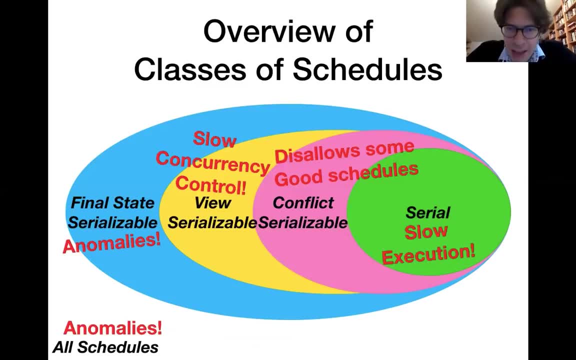 And can do that quite easily using the conflict graph. All right, so this is where we stand. now We have found one new class of schedules that are conflict serializable. There's one little drawback to them: They are a little bit too restrictive. 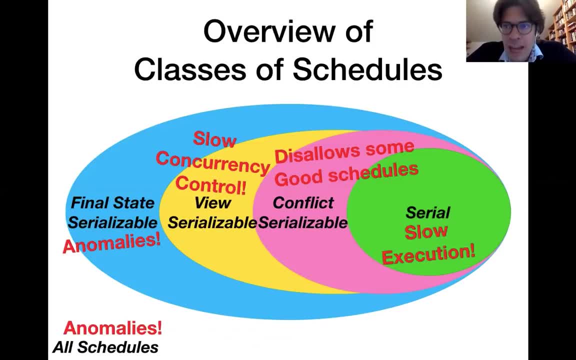 meaning there's some good view, serializable schedules that don't create anomalies, but they would not be allowed according to the conflict serializability criterion. But what we get in exchange is a criterion that is very efficient to verify using this conflict graph that we have seen. 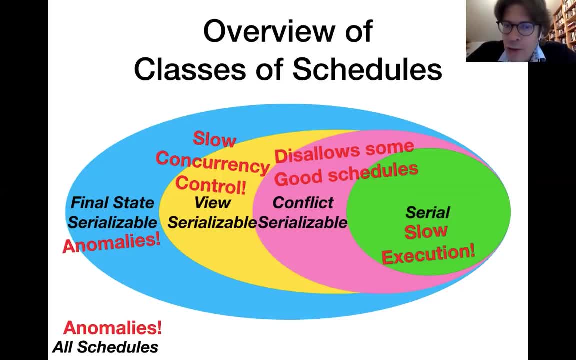 And that is why we will be aiming for creating conflict serializable schedules via concurrency control in the following. It is a compromise between different criteria. All right, Good, Any questions on this at this point? All right, Otherwise, just put them into the chat. 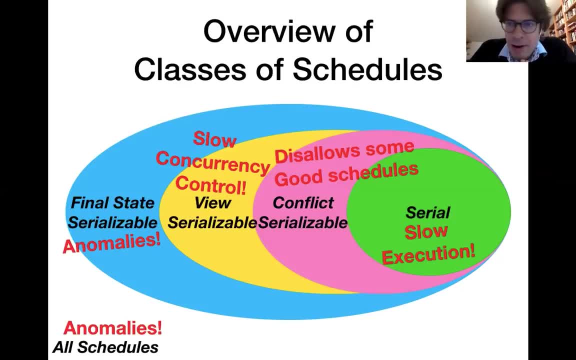 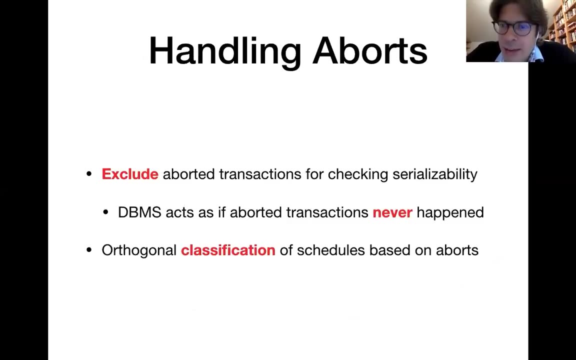 All right. So so far we have been classifying the schedules into this hierarchy, but we haven't really talked about the boards yet. So then, testing, for instance, whether a schedule is conflict serializable would first of all take out the operations. 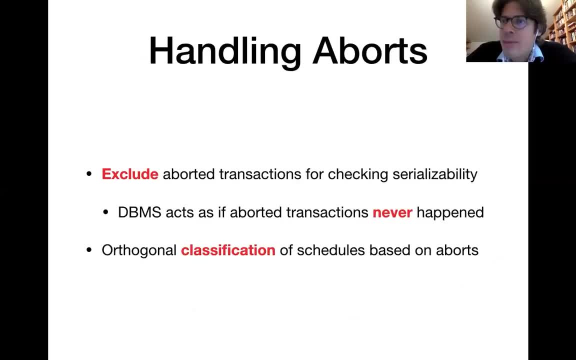 by all transactions that are finally aborting, Because the database management system essentially guarantees that transactions that have been aborted, that everything looks like they never happened in the end. So when testing all those previous criteria, you're not at all considering transactions, but you're at least considering the transactions. 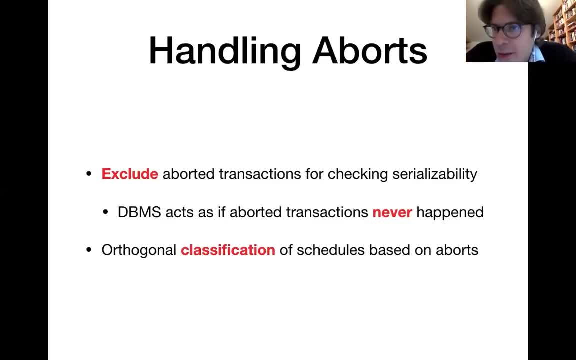 that have been aborted. On the other side, aborting transactions is something that is actually quite common in practice, So you also want to take it into account when choosing a schedule. So in the following we're gonna see another classification of schedules. 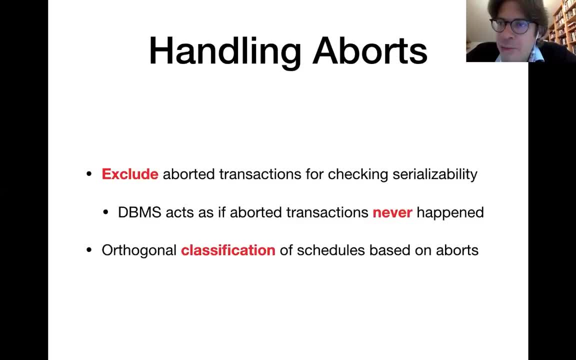 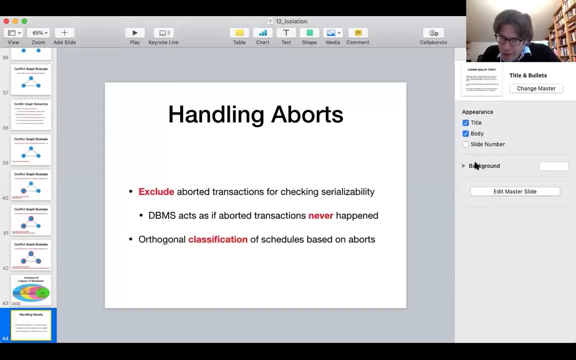 which is orthogonal to the previous one And it deals primarily with transaction aborts. And here there's a question. I think that still refers to conflict graph: If we have a cycle, is it considered as a programmer's fault or will it be randomly selected? 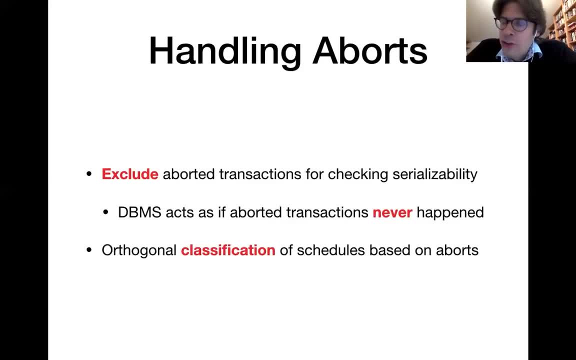 when one starts executing. So if there's a cycle in the conflict graph, it means that the selected schedule is not conflict-serializable. So typically the concurrency control component would aim to select only schedules that are conflict-serializable. 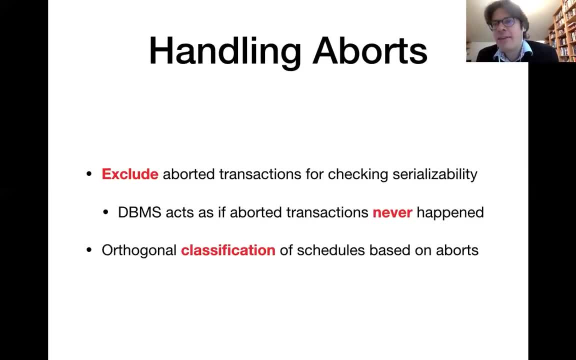 So if there's really a cycle in the conflict graph, that is something that should not happen when you use a concurrency control method that aims for conflict-serializable schedules. So the goal of concurrency control is to avoid any cycles in the conflict graph and to select schedules which don't have them. 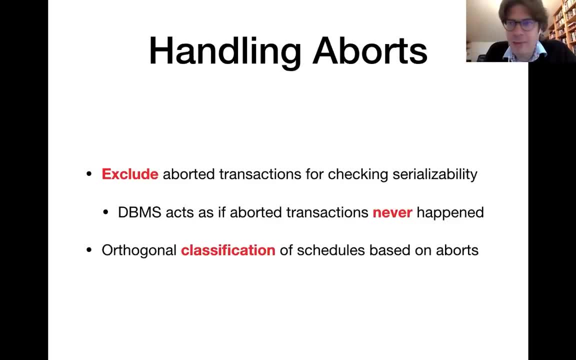 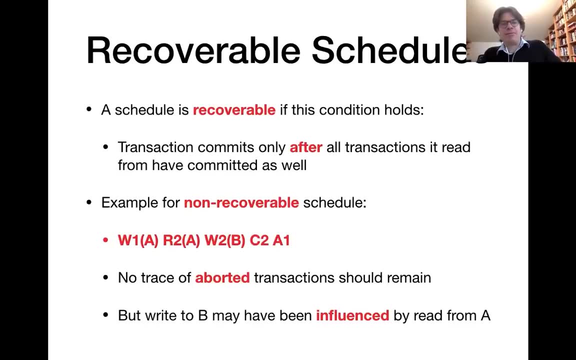 So yeah, if that happens it would be the fault of the programmer of the database management system. Okay, All right. So first of all we will discuss about recoverable schedules. Recoverable schedules, it's kind of you know. 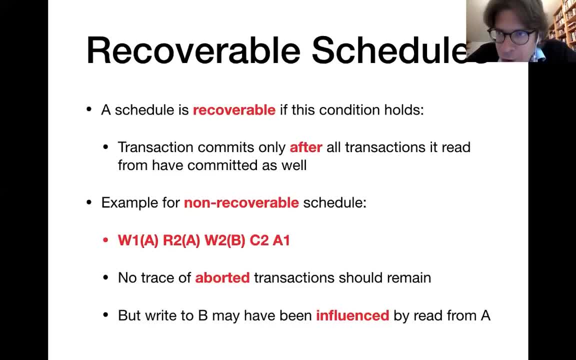 coverable schedules. it's a very basic criterion, saying basically that your schedule should leave the database in a consistent state. it's a very basic requirement if you look, for instance, at the schedule marked in red over here. so what we are doing here is we first have a write to object, a by transaction one. 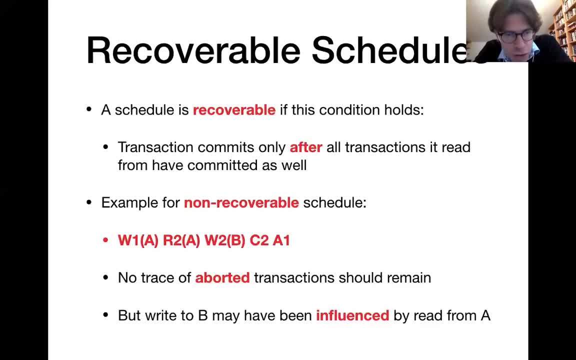 followed by a read of object a by transaction two and a write by transaction two on object B. and now a transaction two commits, but a bit after that transaction one aborts and that creates a huge problem for the database system, because the database wants to guarantee that committed transactions. 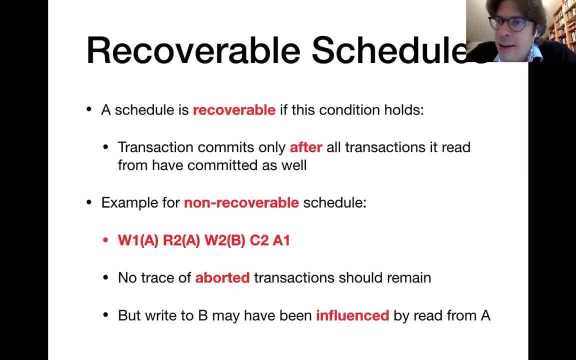 are never undone. on the other side side, it wants to guarantee that aborted transactions have no effect whatsoever on your database, and the problem is this: that transaction number two has read the value of object a. that was written by the first transaction, which means that transaction two might have been. 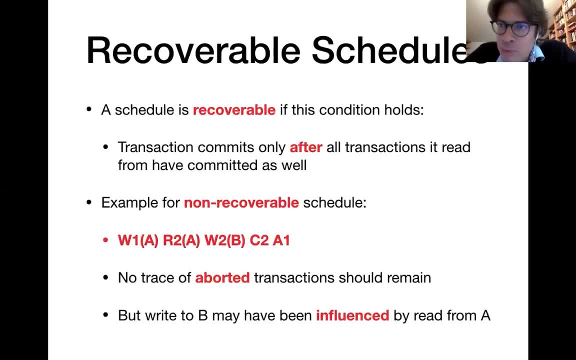 influenced in what it writes to object B by what it has read from object a and that means that logically, if transaction one had never happened, then transaction two might have written a different value to object B. now that creates a problem on one side. we want to guarantee that transaction two. 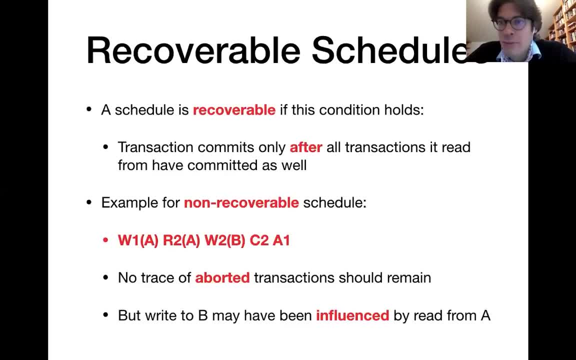 will never be undone, but it was influenced by transaction one and we want to guarantee that transaction one has no effect whatsoever on our database date. so this is a situation you totally want to avoid, because here in the database system essentially tries to guarantee two things that conflict of each other. we call such schedules non-recoverable and essentially such reports will be ever removed after it break down the anxiety pattern, which is obviously a��. 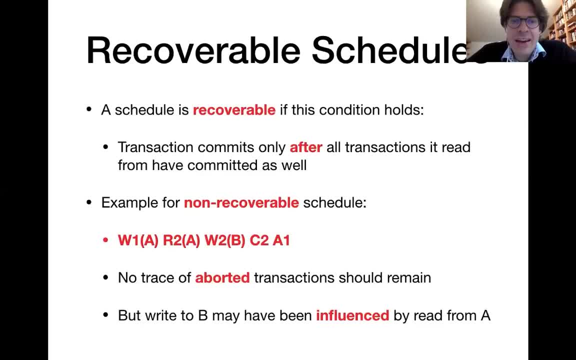 US also also thinks change is done. we call such schedules non recoverable and And essentially, in order to avoid such bad schedules, what we need to do is that we delay the commit of a transaction until we can be sure that all other transactions it has been influenced by have also committed. 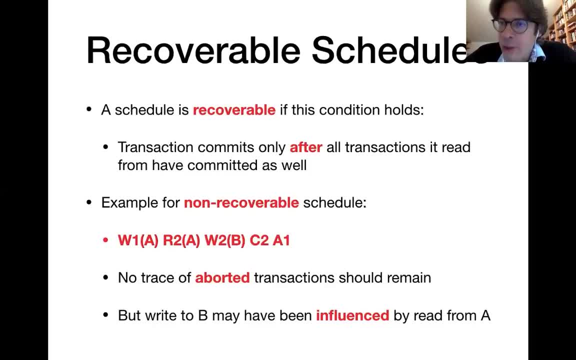 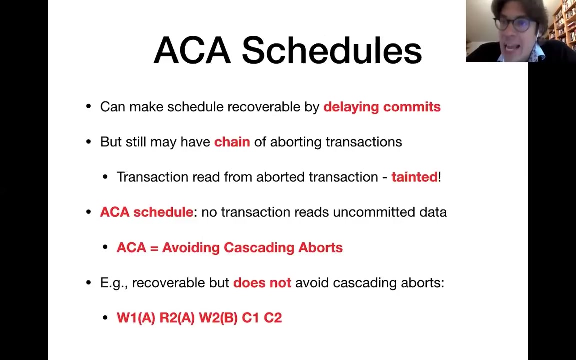 So, essentially, we want to make sure that a transaction only commits after all the transactions it has read from have committed, And if I have that, then I have a recoverable schedule. Now, recoverable schedules, that is something that you want in any case. 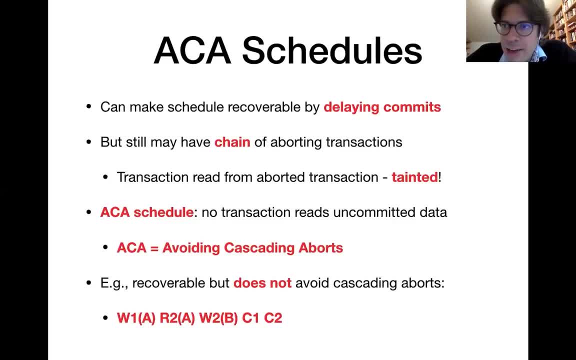 But aborts can even create problems if a schedule is recoverable, For instance, if you look at the schedule here below, here we have again It is, and maybe I should compare to the previous one. So here we have again a write to object A by transaction one and then a read of A by transaction two, followed by a write by a transaction two to object B. 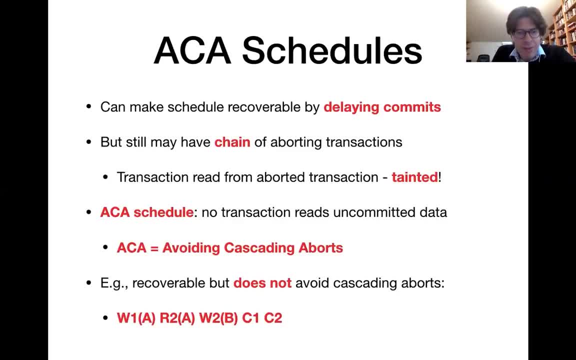 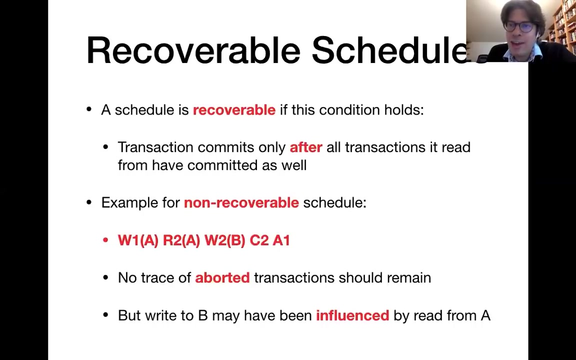 Now what we have done here is that we wait with the commit of transaction two until transaction And then we can see that the transaction one which has influenced transaction two has also committed. So if you compare that to the previous schedule here, the problem is that transaction two already committed before it knew that transaction one commits two. 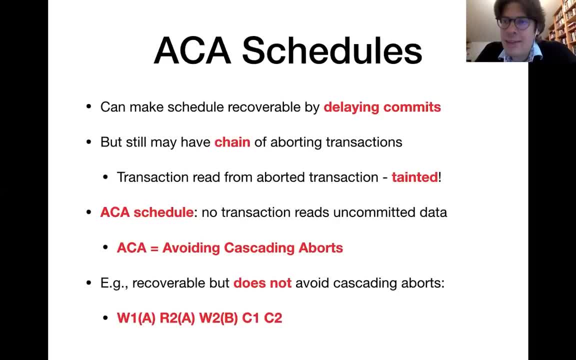 Right. So here we have essentially delayed the commit by a transaction two until we can be sure that transaction one committed. That makes it recoverable, which is good. But on the other side, if at this point transaction number one decided to abort, then you would also have to abort transaction two, because it has been tainted by reading a value of object A that has been written by transaction one. 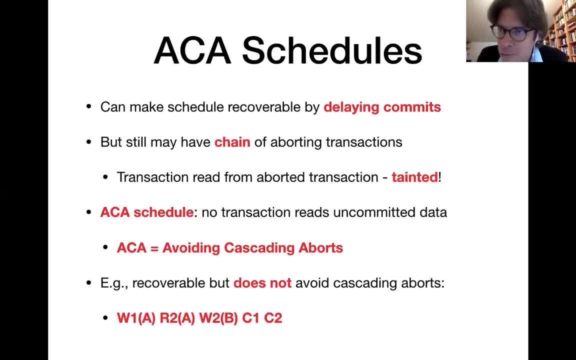 So that means that we have essentially cascading aborts, because One transaction, two and one abort, Now The transaction number one committed. So that means that we have essentially cascading aborts, because one transaction, two and one abort transaction aborts and that causes another transaction which has read from it to also 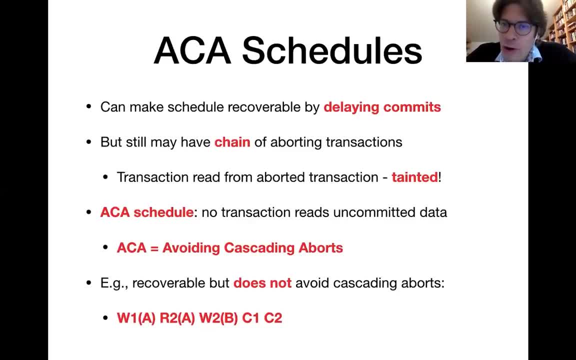 abort. That is something that we want to avoid for performance reasons, because if you have, like, a long chain of transactions where the first one aborts and that causes all the other ones to abort too, that creates huge overheads to the database system. 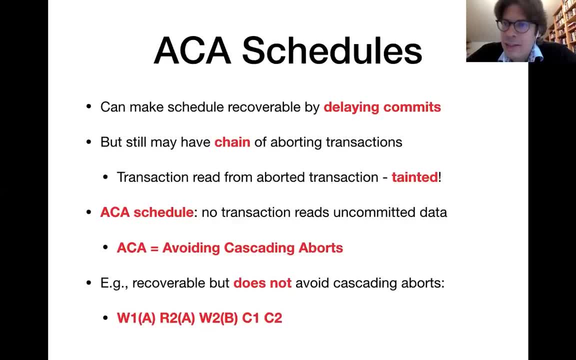 So that's why we're interested in creating schedules that avoid cascading aborts, also called ACA schedules, And in order to get there, the only thing we have to make sure of is that a transaction does not read uncommitted data. If we read uncommitted data, we might have a cascading abort. 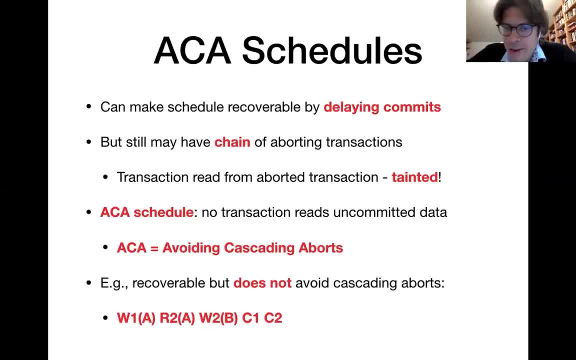 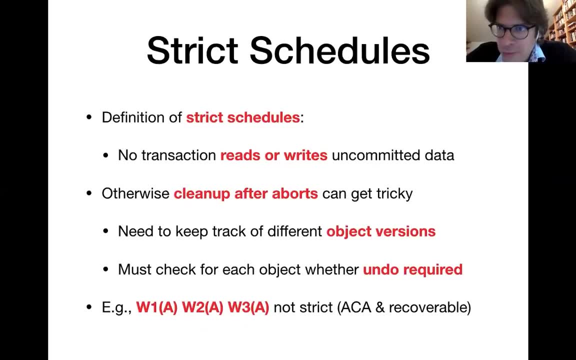 If we don't read uncommitted data, we avoid that possibility. So avoiding cascading aborts is good. There's still a couple of things. There's a couple of issues that can arise in the case of aborts if multiple transactions have written to the same object. 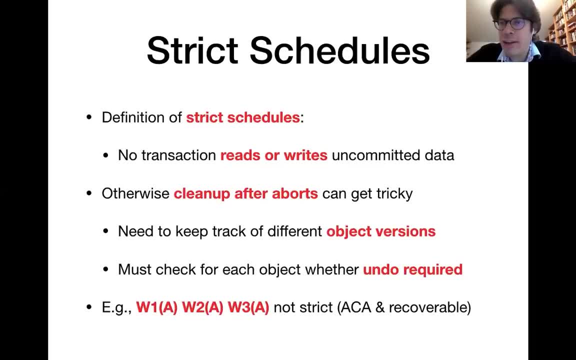 So, first of all, if multiple uncommitted transactions have written to the same object, it means that I need to keep track of which transaction has written which value, because if some subset of those transactions abort, I need to know which is the right value to assign to that. 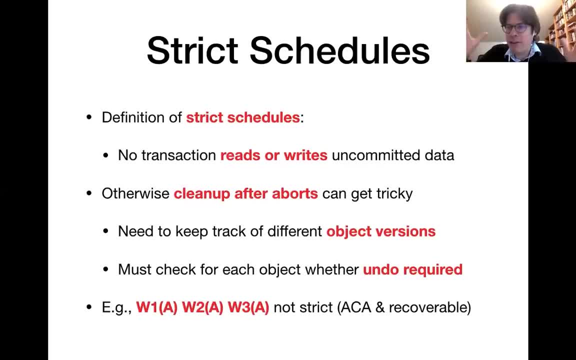 object. Also then, For instance, Aborting one transaction and undoing values for an object, reverting them back to the original value, I need to verify whether the current value of the object is actually invalid and whether I really need to undo it. 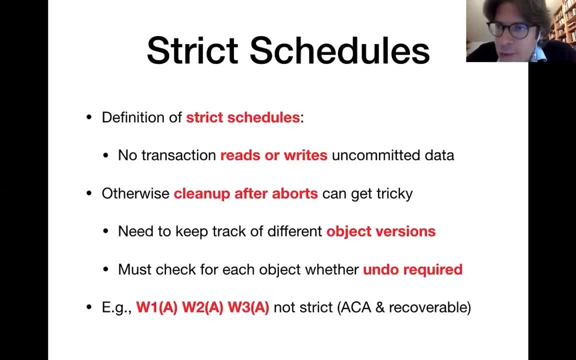 So generally having multiple transactions write to the same object where all those transactions have not yet committed, that can create some complications. Okay, So I'm going to show you how to do that. So I'm going to show you how to do that in the cleanup. 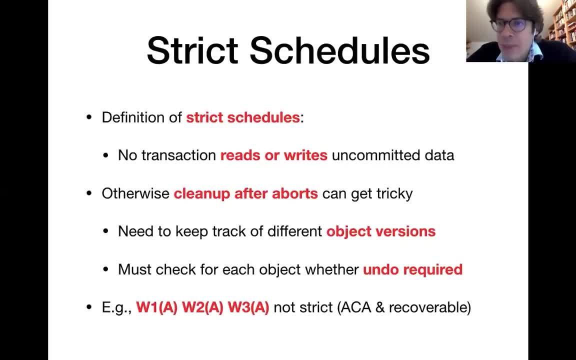 And that is why people in practice often try to avoid such schedules and go for strict schedules instead. Strict schedules generally means that no transactions reads or overwrites uncommitted data, So once one transaction has written a value to an object, then this value will not be. 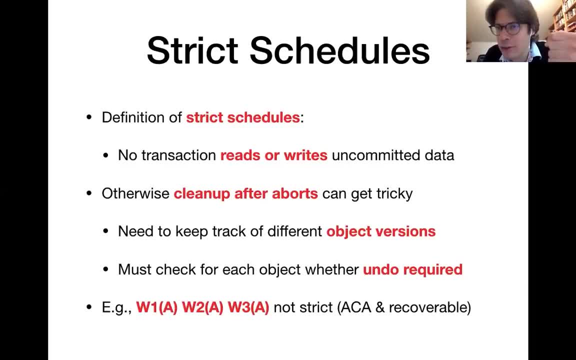 read and it will not be overwritten. And that's why people in practice often try to avoid such schedules and go for strict schedules until that transaction which has written the last value has committed All right. So for instance, here at the bottom of the slide, you have another example schedule where 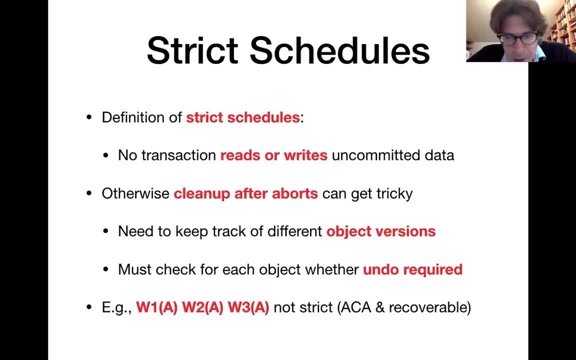 three transactions. write to object A. Now this schedule, first of all, is a recoverable. We actually don't see any commits at all in this schedule. It avoids any commits. Okay, So it avoids cascading aborts, because we don't see any reads of uncommitted data here in. 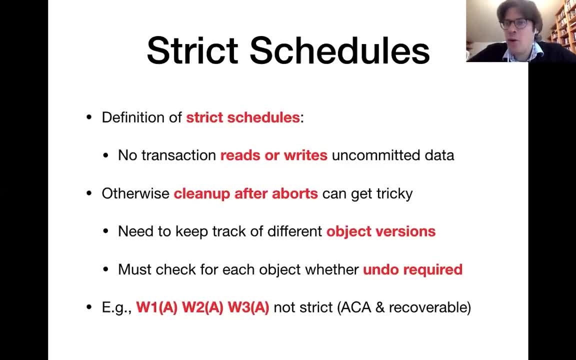 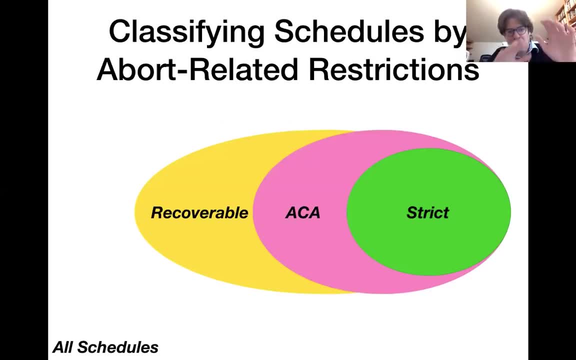 this schedule, but it is not strict because different transactions override each other's values before any of them commit All right. So altogether we have now seen another hierarchy of schedules. We have the set of all schedules. a subset of that is the recoverable schedules. 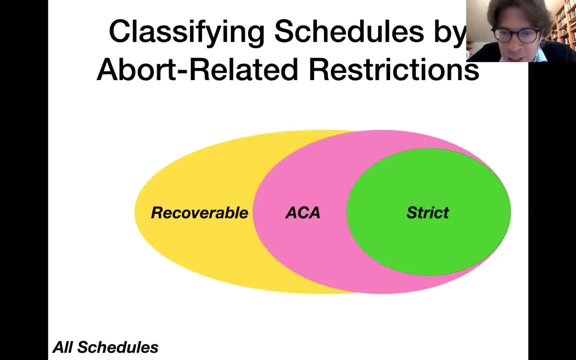 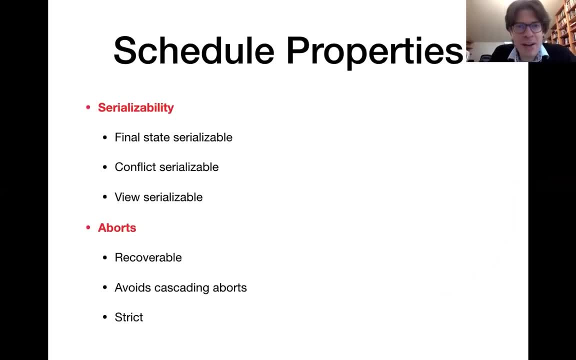 Then we have the ACA schedules that avoid cascading aborts. Then we have the sterile schedules that avoid cascading aborts. Then, finally, we have the strict schedules. So, in summary, now we have seen two ways of classifying schedules. First of all, based on serializability. 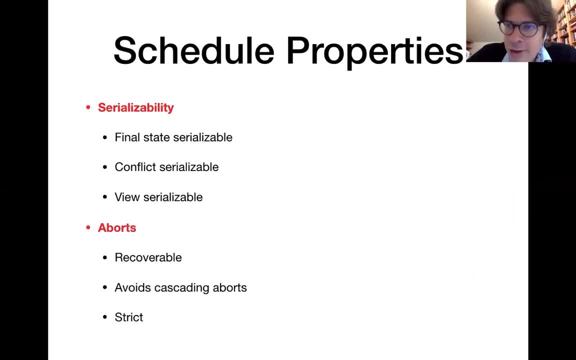 Then we have seen find-in-state serializable, conflict-serializable and new serializable, And then we have classified them based on aborting behavior. And then we have seen recoverable schedules- schedules that avoid cascading aborts- And then we have seen recoverable schedules that avoid cascading aborts. 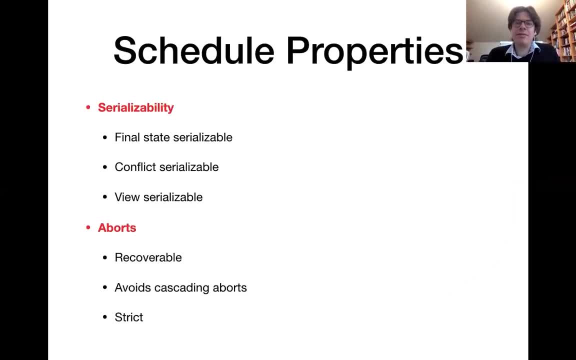 the strict schedules And which of those schedules you're going for. it depends on many factors for serializability. In the following we will be aiming for conflict serializable schedules because it's a good compromise between the quality of the schedules and the overheads of concurrency control For abort behavior. 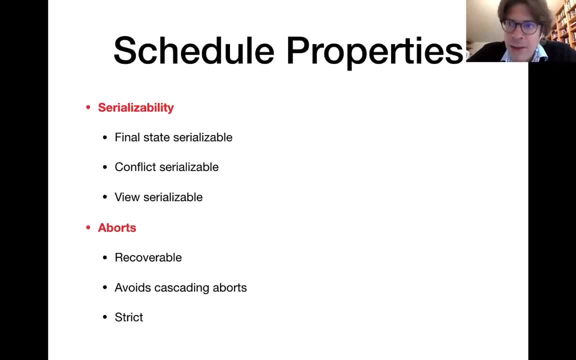 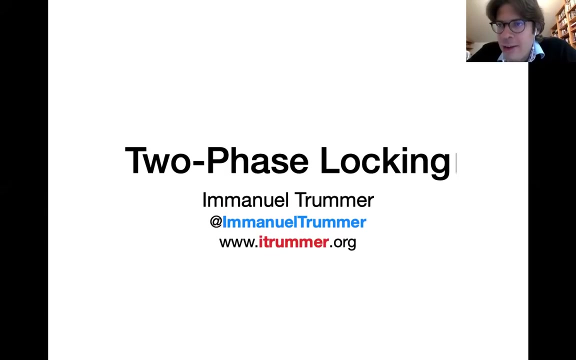 we will definitely go for recoverable schedules, but then, depending on the variant of concurrency control that we are discussing, we might sometimes consider only recoverable schedules, sometimes ACA schedules and sometimes strict schedules- Whatever provides the best performance in certain circumstances. So we will start now to discuss about mechanisms for concurrency. 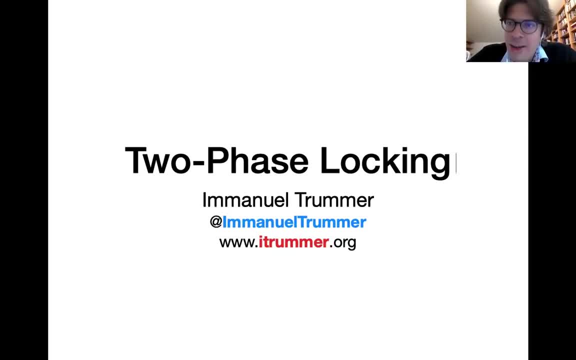 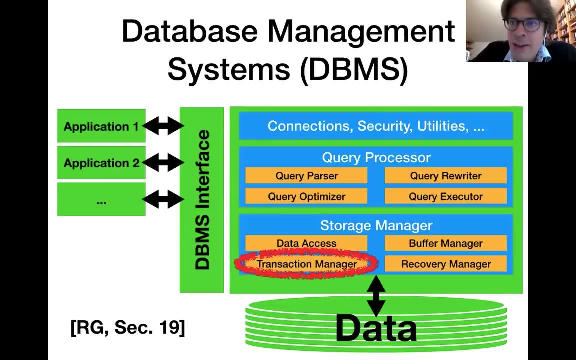 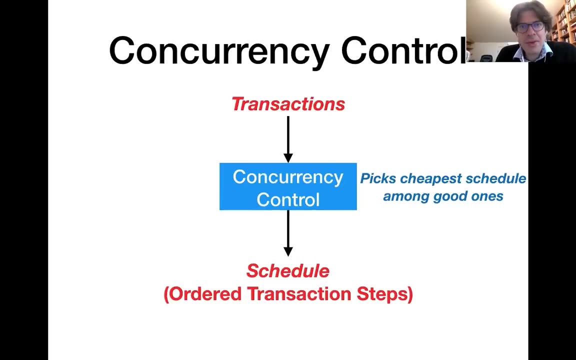 control and one of the most popular mechanisms, that is, two-phase locking. Here we are discussing about the transaction manager component of the database system, the relevant chapter in Ramakrishna and in Gerke, that is chapter number 19.. So, generally, what we are discussing about now is the algorithms that run inside of 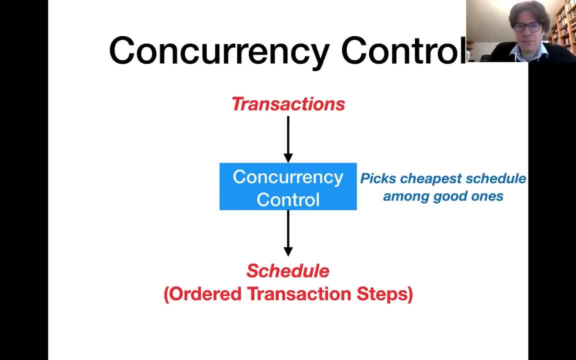 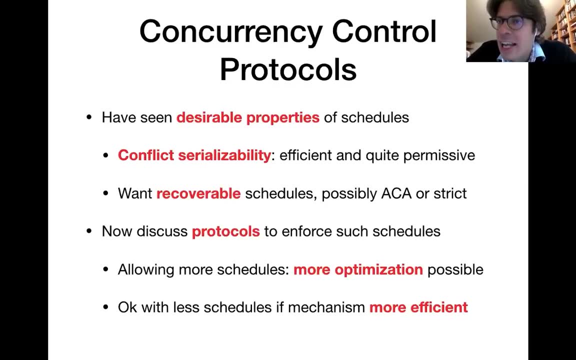 that concurrency control component. So what we have seen in the previous slide deck was generally a classification of schedules. So we have seen that we probably want to aim for conflict serializable schedules. We want recoverable schedules and, depending on the situation, sometimes we want ACA schedules and sometimes we want strict schedules. So now we're gonna. 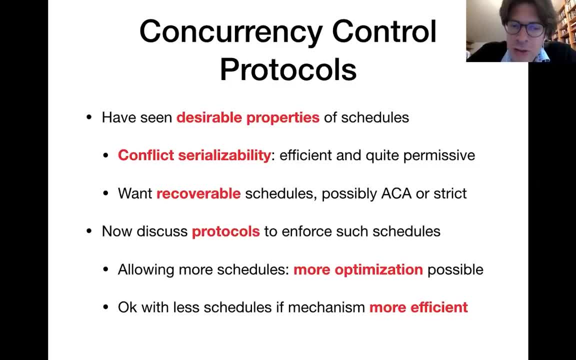 discuss about protocols which generate those schedules. There's always trade-offs. Ideally, we want a mechanism that allows many possible schedules to consider, because then we can select the most efficient one for execution. On the other side, we want a mechanism that is very cheap to execute, So we might be. 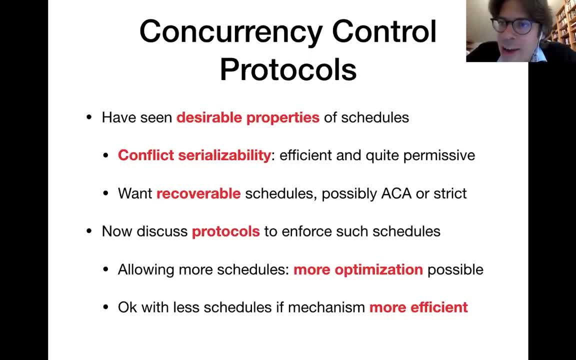 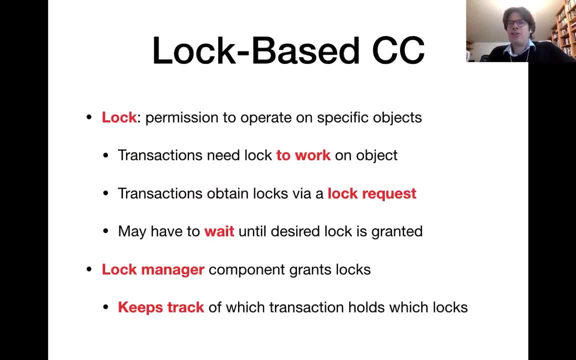 willing to accept considering less schedules if in exchange it reduces the cost of concurrency control. So in the next lecture mainly we will be discussing about a locking based concurrency control model. Now we're going to discuss more detail in the next lecture, but already I'll tell. 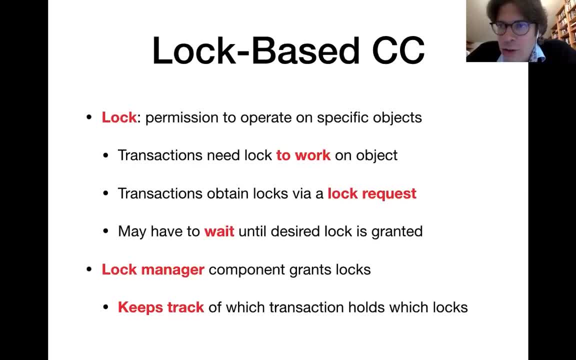 you a few basics. So generally, those concurrency control mechanisms will be based on locks, which essentially represent a permission to operate on a specific object, And the mechanisms that we will see essentially force transactions. the first acquire a lock on an object before they can work with it. 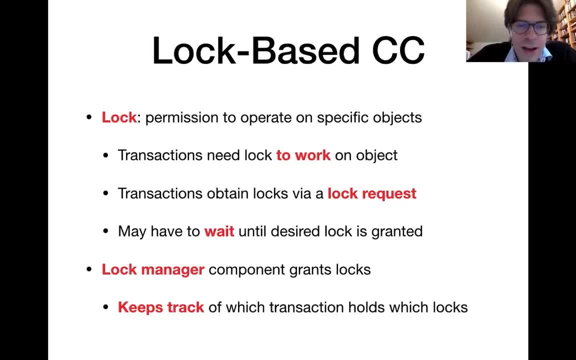 They submit those and lock requests to the lock manager and then they wait until the lock request is granted And only then do they proceed. The lock manager generally keeps track of which locks has been assigned to which transactions and it also keeps track of which transaction is interested in what. 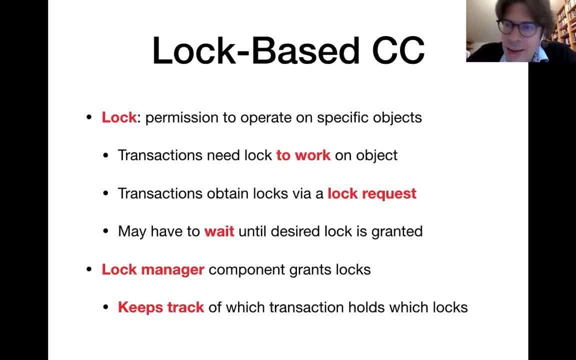 lock and it accused them. and then it grants transactions to the lock manager with locks and make sure that no two transactions have conflicting locks on the same object in the database. That is the high level principle. In the next lecture we are gonna discuss more details. 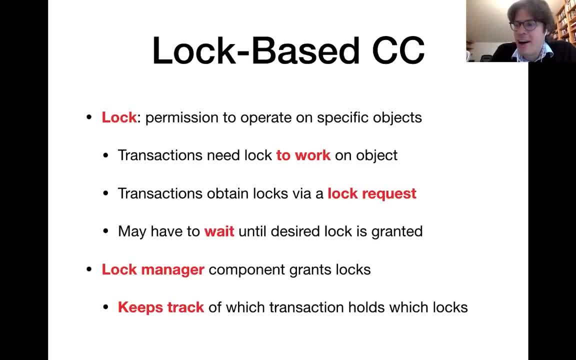 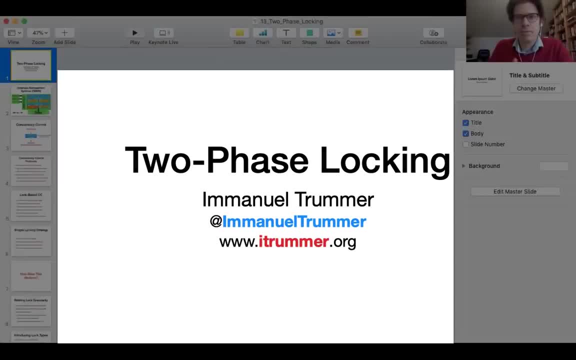 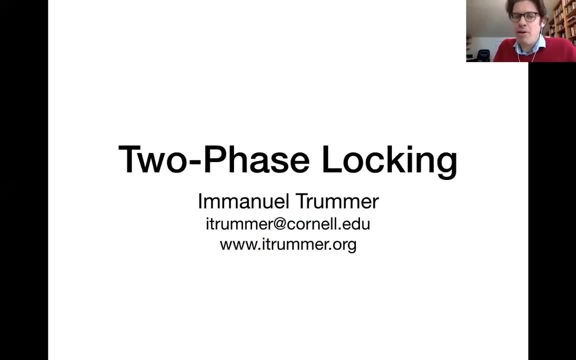 for one very popular concurrency control mechanism. Have a nice day, and then I see you on Friday. All right, let's get started. So today we are still gonna talk about isolation and concurrency control, And we are gonna see a specific algorithm in order to do concurrency control. 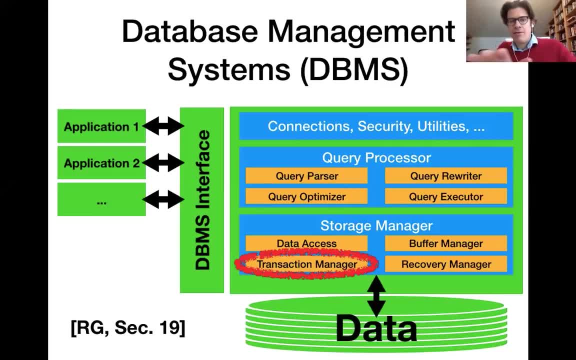 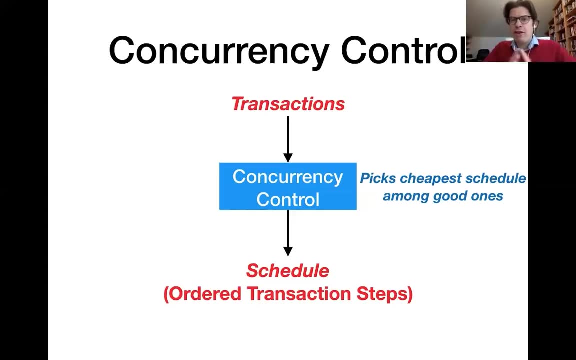 That algorithm is called two-phase locking. We are still discussing about the transaction manager in the database system and the relevant chapter for what we discuss here, that is, chapter 19 in the Ramakrishnan and Gerke book. So generally, we are currently discussing. 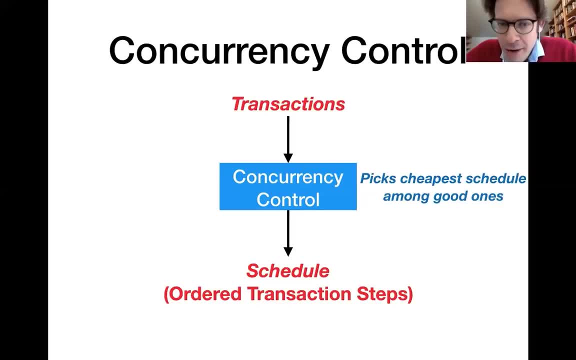 about concurrency control And, as a little reminder, concurrency control essentially takes as input a set of transactions which want to execute a read and write operations on the database. The output of concurrency control, that is a schedule which orders the steps, the read and write operations. 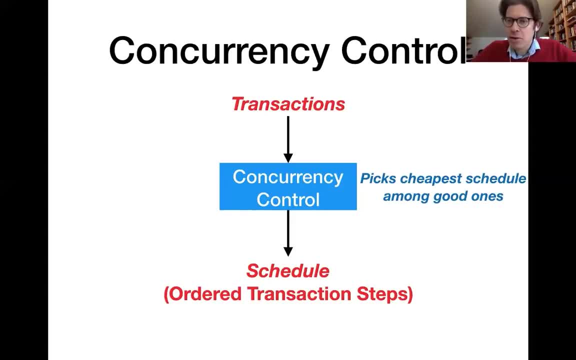 from different transactions, And it may do so in a way such that it interleaves the steps from different transactions. So we do not execute one transaction after the other one, but you might execute a few steps from transaction number one, then a step from transaction number two. 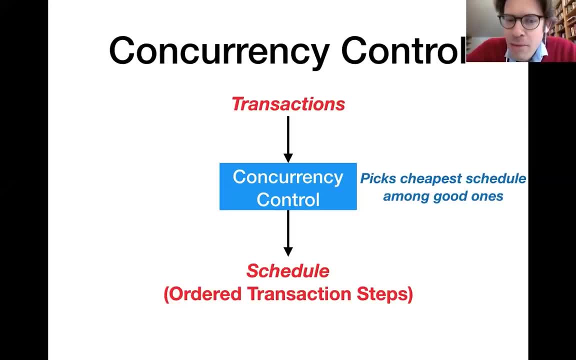 and then again some steps from transaction number one. But if you do this you have to be very careful, because otherwise it creates strange effects for the user and inconsistent data and concurrency control- that this does not happen. So we want to find algorithms that can actually do. 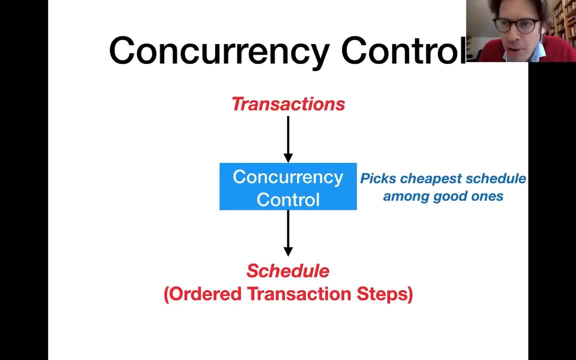 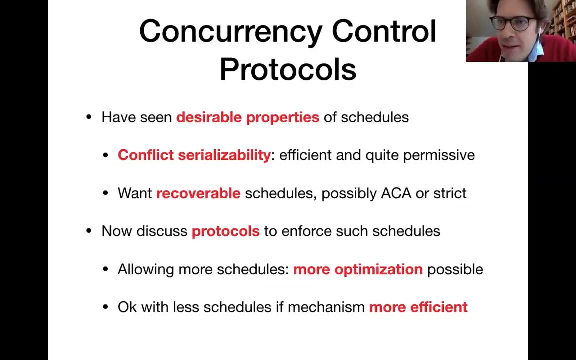 concurrency control and we're going to discuss about one of the most popular ones today. So far, we have been mostly discussing about what properties we want in one of those schedules. In particular, we have seen that conflict serializability is kind of a good compromise, because if your schedule is, 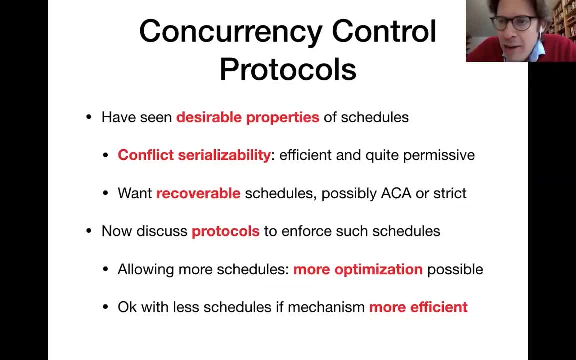 conflict serializable. it means that those strange effects due to interleaving multiple transactions, they cannot occur. So to the users it looks as if everything executes serially, one transaction after the other one. On the other side, conflict serializability has a nice property that we can quite. 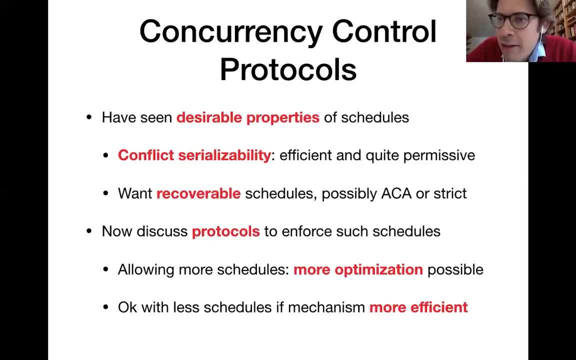 efficiently verify for a given schedule whether it is conflict serializable. And efficiency is very important, since concurrency control happens at runtime. So we do not want concurrency control to become the bottleneck. So we want conflict serializable schedules. We also want recoverable schedules And, as we have seen last time, that means essentially 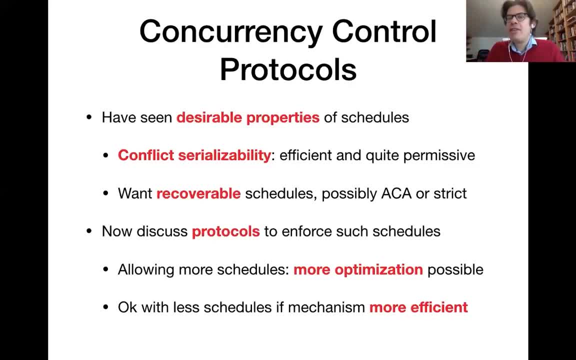 that one transaction does not commit until all the other transactions that it has read values from have committed before, Because otherwise you might end up with a database in an inconsistent state from which it is impossible to recover. So we want recoverable schedules And we have seen a couple of other. 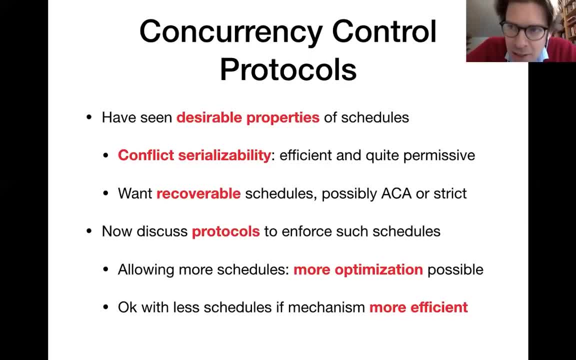 properties- avoiding cascading aborts and strict schedules- And, depending on the scenarios, we might also want some of those properties. Now, in the following we're going to discuss about protocols, about algorithms that allow us to enforce schedules with those desired properties And, generally, ideally, we want. 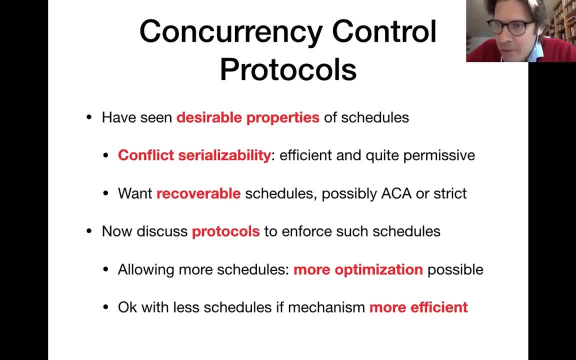 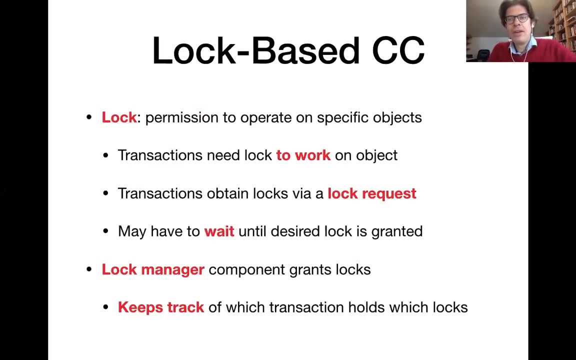 mechanisms that allow as many schedules as possible that have those properties that we're interested in, Because if you can consider more candidate schedules, then we have better chances of finding one that is particularly efficient to execute and therefore want to be able to consider as many schedules as possible. 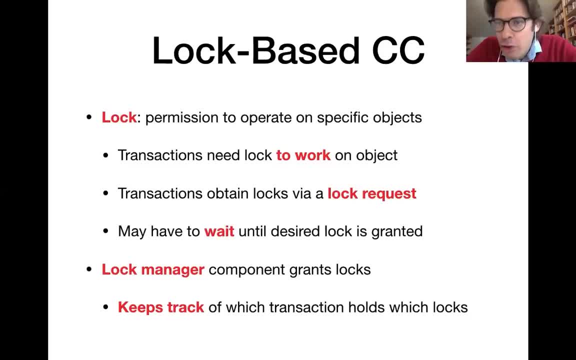 Now a very popular variant of concurrency control is based on locks. Lock generally means the permission to operate on a specific object in your database And, before a transaction, can do anything with a database object, which could for instance be one row in one specific table Before a. 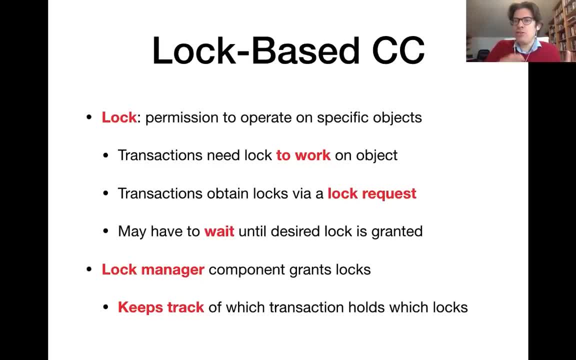 transaction can do anything with it, be it a read operation or write operation, it first must acquire a lock. So in order to acquire a lock, a transaction submits a lock request for the specific object and that request should be included in the to the lock manager, which is a component that generally administers the different. 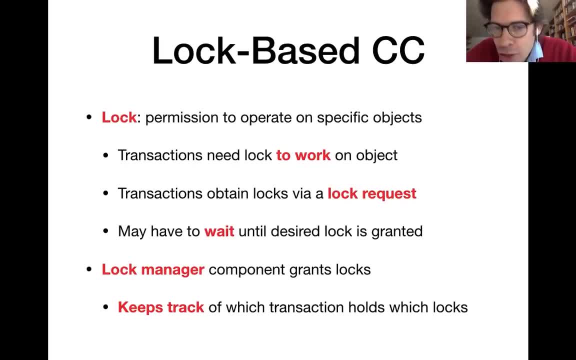 blocks and keeps track of which transaction has acquired which lock. Now, if a transaction requests the lock, that block might not be immediately available because maybe currently another transaction has the lock on the corresponding object and we have to wait until the other transactions gives back the lock to the lock manager and then the lock manager can. 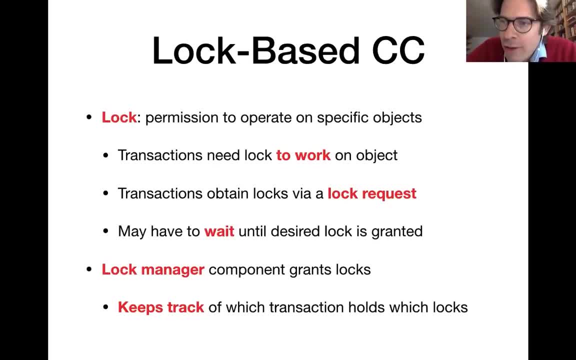 distribute that block again to the waiting transaction. So the transaction might have to wait a little bit until it obtains the lock. Once it has the lock, then it can start working on the object. Now this is the high level outline of locking based concurrency control. 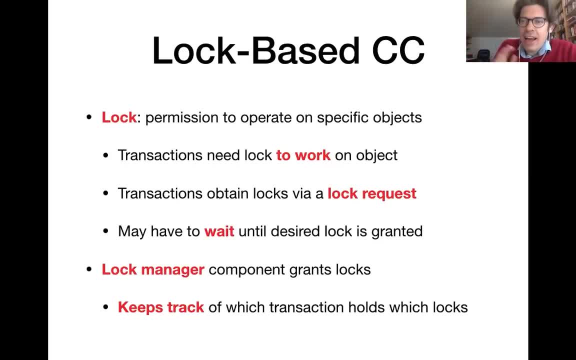 but there is many variants and in the following we're going to see a couple of them. Let's start with something very, very simple. Let's say that we just make one of the following variants and we're going to see a couple of them. 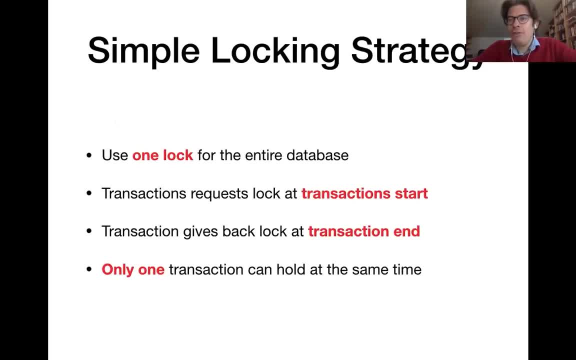 Let's say that we just make one of the following variants, and we're going to see a couple of them. Let's say that we just make one big lock for the entire database. So if a transaction wants to do anything with the database, it first has to request the lock. 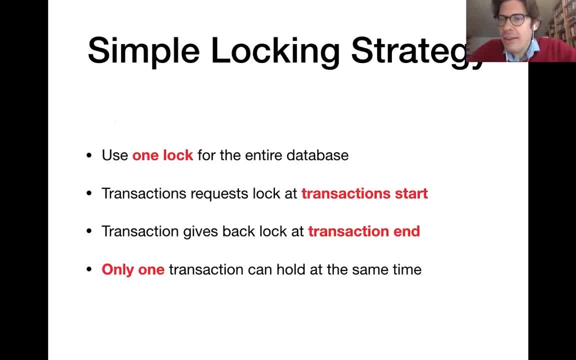 on that database and wait until it gets it. Then it performs its operations and at the end the transaction gives back the lock on the database to the lock manager. So that means that essentially only one transaction can hold this lock on the database at the same time. 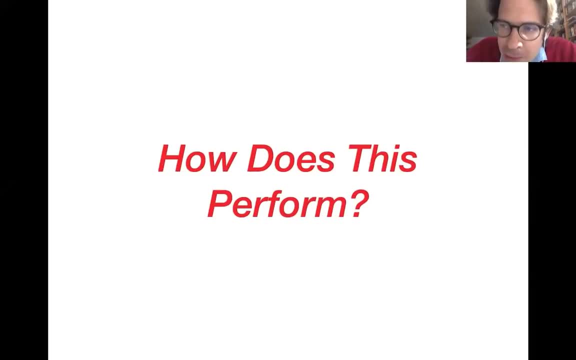 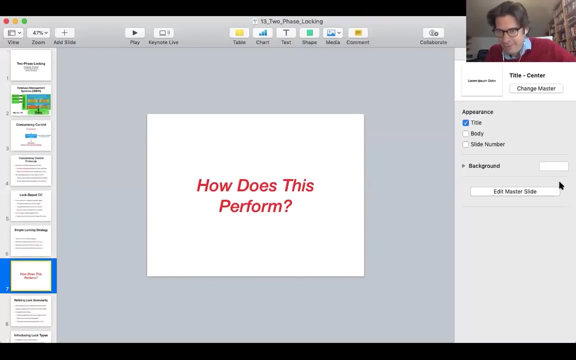 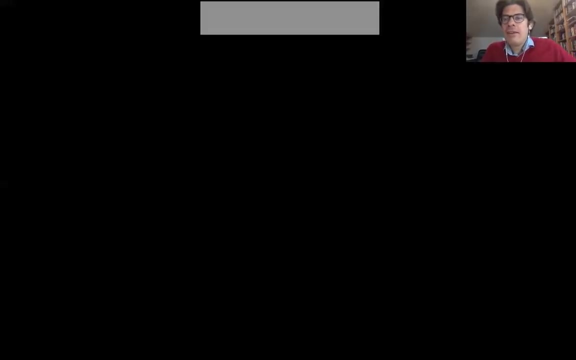 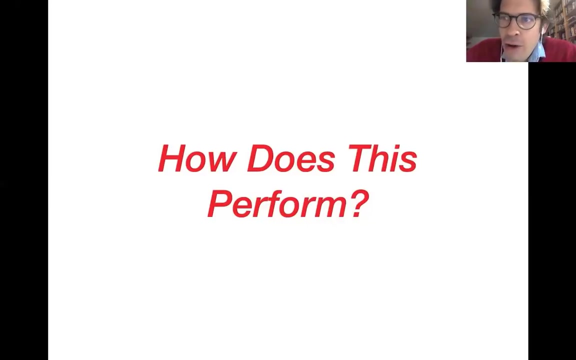 Does anyone have a quick comment about how you expect this scheme to perform In the chat? Yes, very good. Okay, very good. I see multiple comments and all of them are correct. So, yes, in the chat. Indeed, If we make one big lock for the entire database, then you're often unnecessarily blocking. 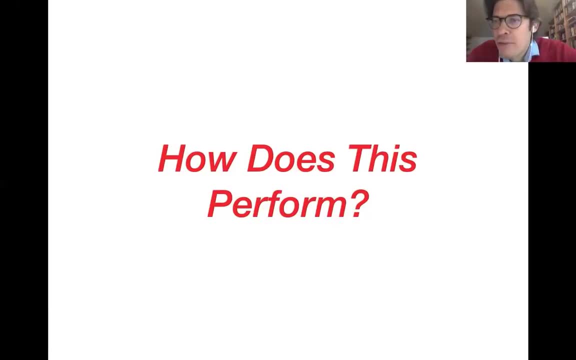 transactions from proceeding because different transactions might be able to work with different parts of the database at the same time. And if you really only have one big lock for the entire database, what happens? it means essentially only one transaction can execute at the same time. 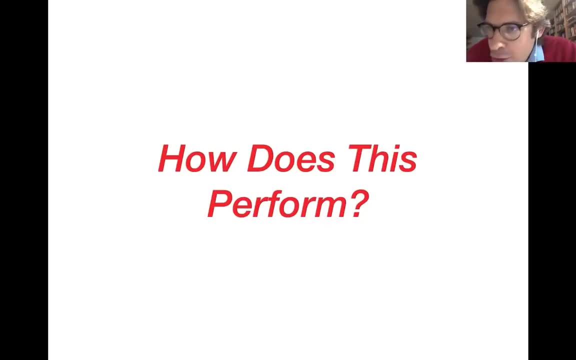 It acquires the lock at the beginning, it gives it back at the end. So that means what I'm essentially. I'm executing transactions serially, one transaction after the other one, And the whole point of concurrency control and preparing transaction schedules was that 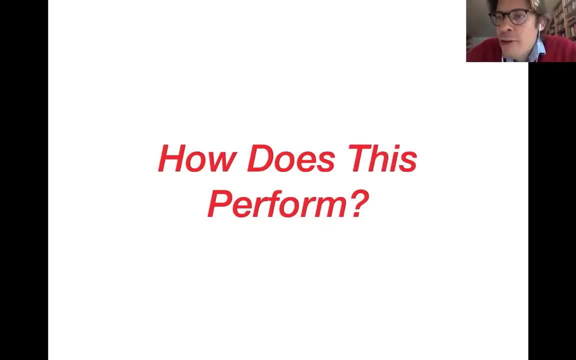 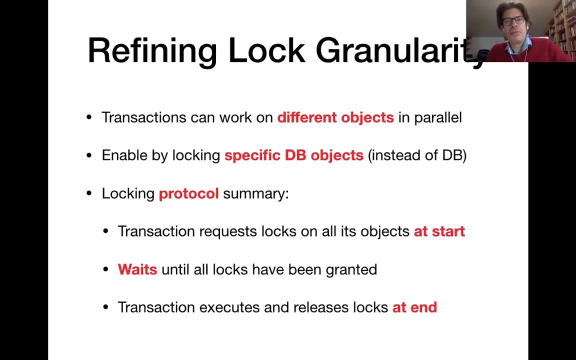 we want to get better performance than when executing transactions serially, So this is probably not what we want. Let's refine Now. a first refinement uses the observation that there's many objects in the database and what are the chances that two transactions want to access exactly the same object? So we should: 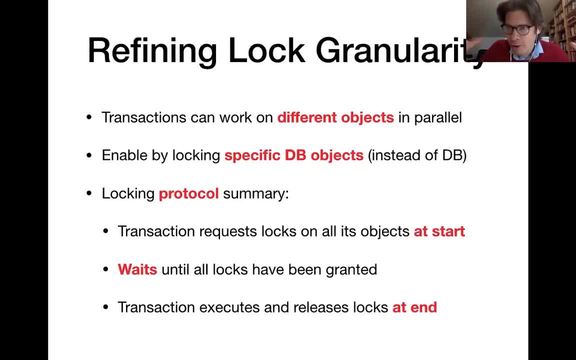 refine our logs to refer not to the entire database as a whole, but rather to specific objects in the database, So those objects could have different granularities. It depends on the implementation. For instance, we could say that one row in the table is an object. 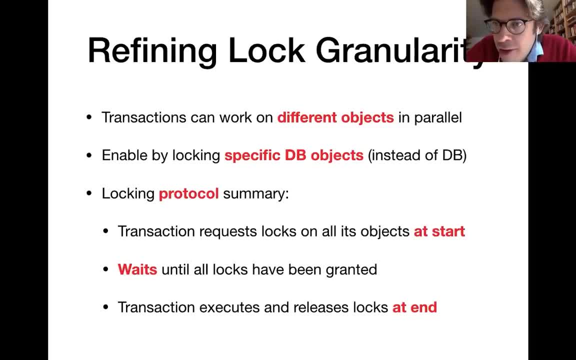 And if we have that, then transactions: they first of all decide which objects they are interested in, then they request the logs for all those objects and wait until they get them, Then it executes and finally the transactions gives back all the logs at the end of execution. So this: 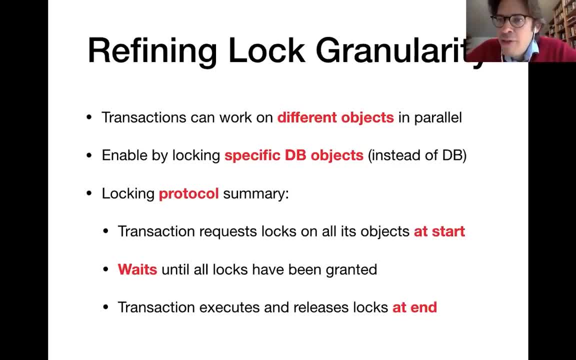 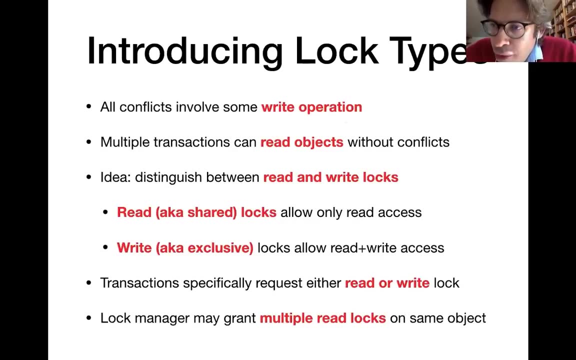 already works better than before, because now different transactions can be executed, proceed in parallel on multiple parts of your database. Now another refinement is the following: So we have seen, when discussing about conflict serializability, that conflicting operations: they always involve at least one write operation. 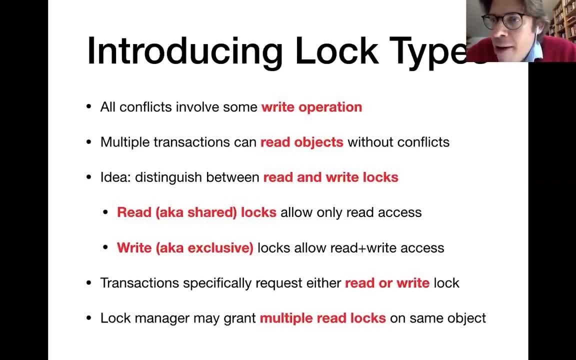 on the same object On the other side. as long as I only have read operations, I could actually allow many transactions to proceed in parallel. The problematic operation is really the write operation And in order to increase the number of transactions that can execute at the same time, I could start to distinguish between read blocks and 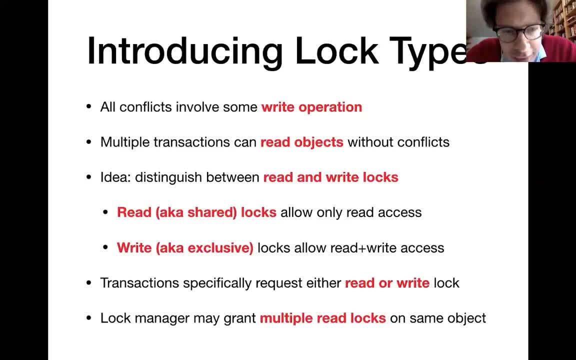 write blocks. So a read block- those are also called shared blocks- allows you to only read the values of an object but not to change them. A write block, also called an exclusive block, allows a transaction to read and to write the corresponding object. And if I have 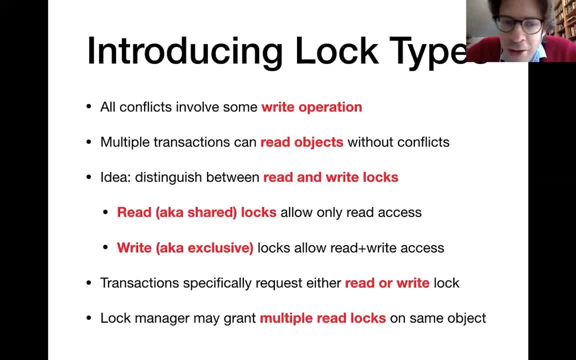 those different block types. I can exploit them because as long as transactions only want read blocks, I might be able. I can grant multiple blocks on the same object to different transactions. All right now, all of the transactions essentially have to decide whether they want to read an object. 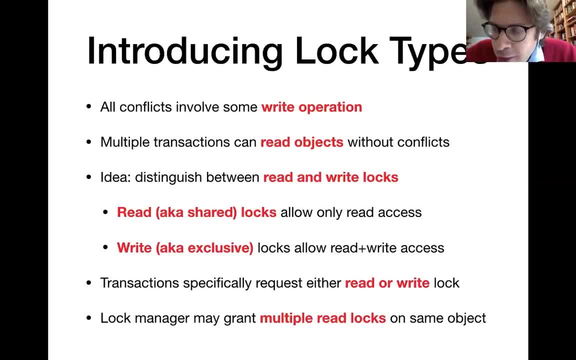 only, or whether they want to read and possibly write an object, Then you have to request the corresponding log type for the corresponding object. All right, and again. the effect of that is that we can possibly allow more transactions to execute in parallel on our database. 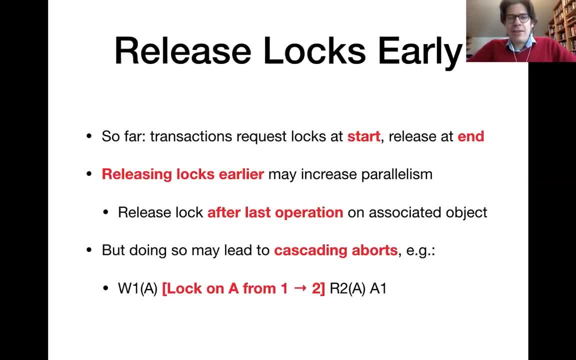 All right now. so far we have assumed that transactions request and wait for all the locks at the beginning of execution and then they hold those locks until the very end of the execution. At the beginning of execution, a transaction requests all the locks. at the end of 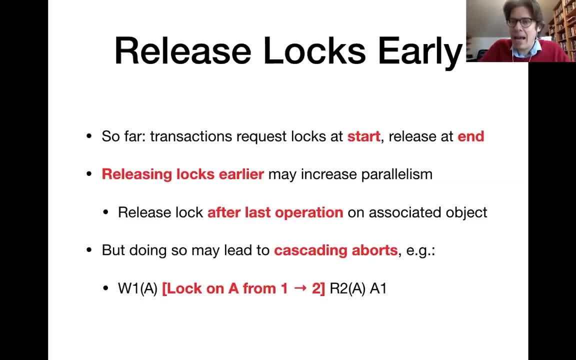 execution the transaction gives back all the locks. Now sometimes it might not be pleasant necessary to hold the lock on an object until the very end of execution. If a transaction is done working on an object, it seems reasonable that the transaction already gives back the lock on that object so that another 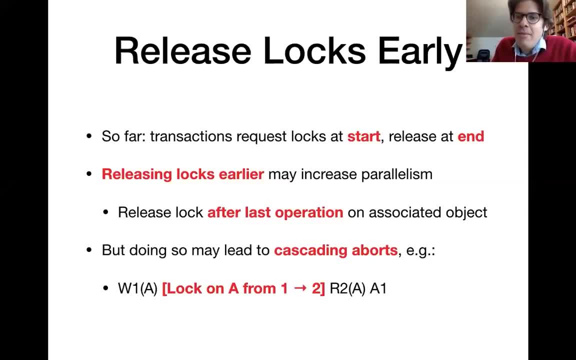 transaction can start working on that object before the first transaction is finished. Now this refinement can be a good idea, but it doesn't have to be. It can be a good idea because it might again allow more transactions to proceed in parallel On the other side. if you allow this, then you might have 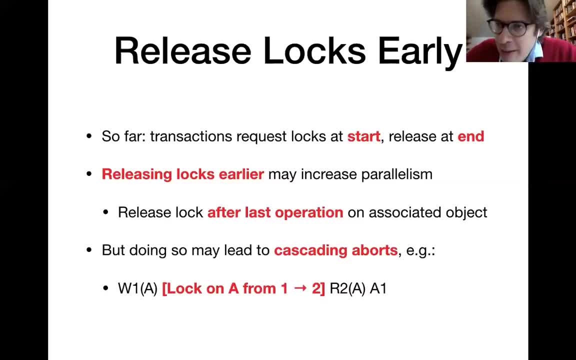 cascading aborts. And, as a little reminder, what is a cascading abort? So if a transaction aborts, it generally means that all direct and indirect effects of this transaction should completely vanish from the database. So it should look as if the transaction. 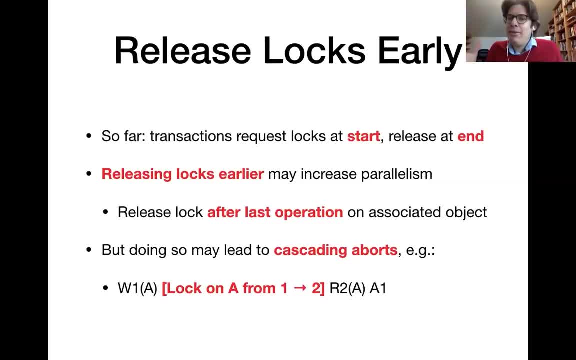 had never happened. And if a transaction writes a value to an object and that value is read by a different transaction, the value could have influenced what the different transaction is doing. That means if the first transaction aborts, it has indirectly influenced the behavior of another transaction. So if you abort, 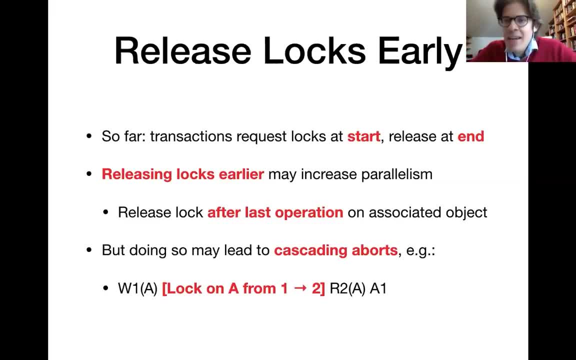 the first transaction, you also have to implicitly abort the other transaction that has been influenced by it. That is a cascading abort. And if you allow transactions to hand back locks after, before they finish executing, before they have to decide whether they commit or whether they 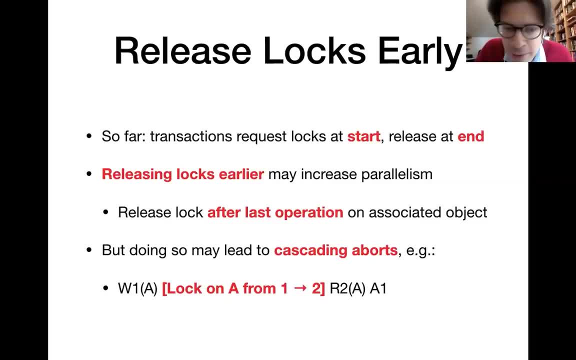 abort, then what you see in this example here can happen. So here we have a write operation by transaction 1 on object A, And now let's say transaction 1 is done with object A, so it could already hand back the lock on A right. So the 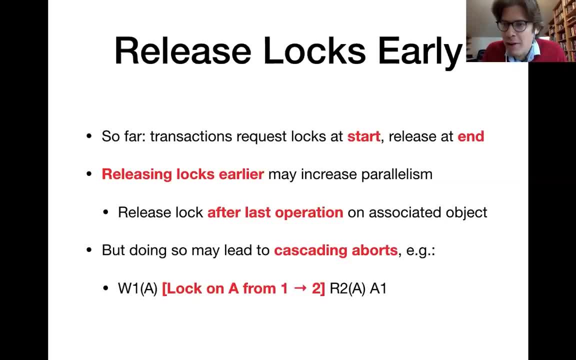 lock manager accepts the lock from transaction 1 again, and then it immediately hands it out to transaction number 2, which is requesting the lock on A because it wants to read the value of that object. So this is what you see here. basically, the lock changes hands from transaction 1 to transaction 2.. And now 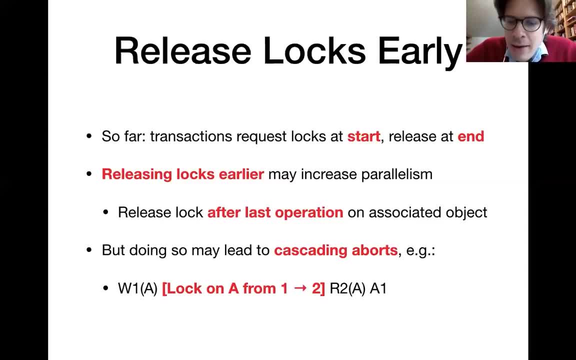 unfortunately, transaction number 1 decides to abort, And in that case we would also implicitly have to abort transaction number 2, because something that this transaction did could have been influenced by the value that it read from. A value has been written by the aborted transaction. So if we allow transactions, 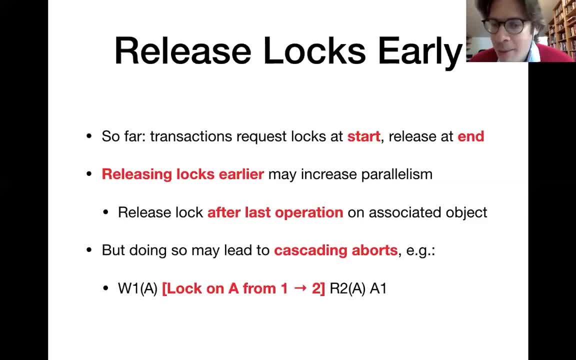 to hand back logs early. it means that we must accept cascading aborts, and then it becomes a design decision. There's a performance trade-off here and, depending on the scenario, one possibility might work better or the other. Now you might already guess the next refinement. So here we have relaxed the requirement. 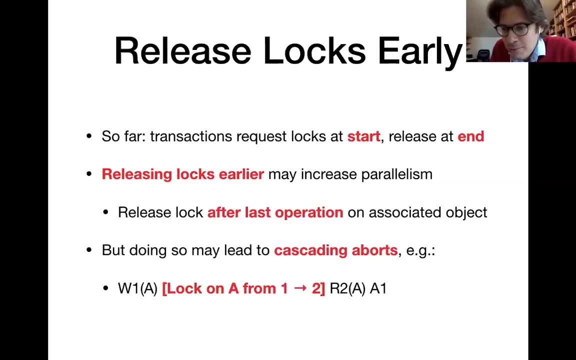 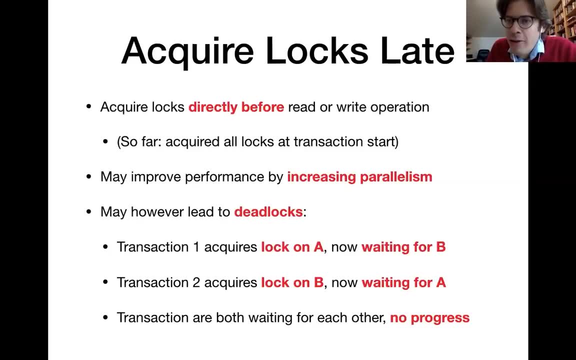 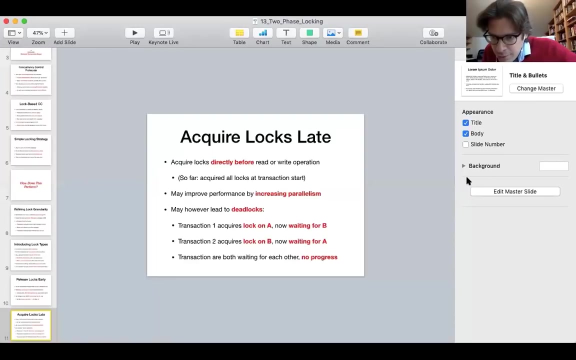 that transactions hold their logs until the very end of execution. And now the next refinement is that we allow transactions to acquire logs not at the very beginning of execution, but sometime during their execution. Quickly checking the chat here: All right, and here there's an. 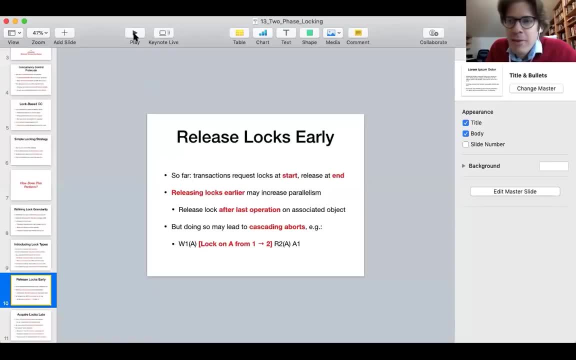 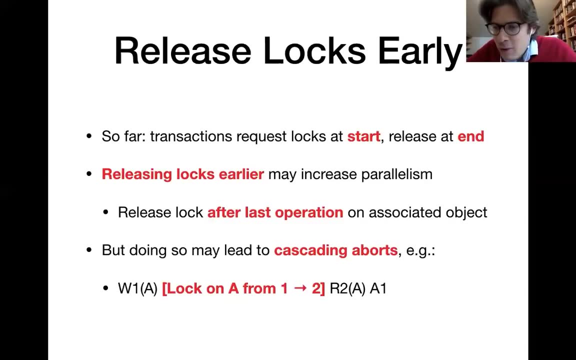 question about the last example. I'm gonna answer that before continuing. So here the question is if R2 had read a different object, whether it could have been influenced by A or not. It could not have been influenced by A, So we assume that the database system knows all the values in the database that transactions. 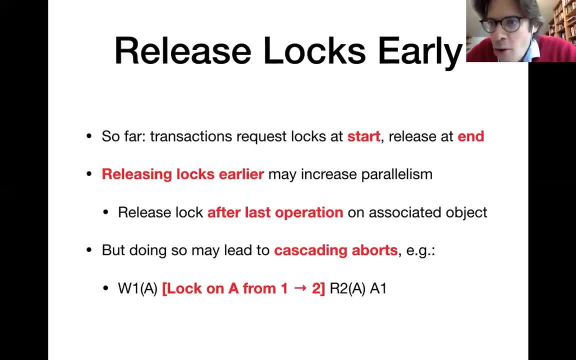 read or write. So if the database system doesn't know about any read or operation on A, then the transaction hasn't read the value of A and cannot have been influenced by it. And at least in the short example it seems that transaction one is only writing to object. 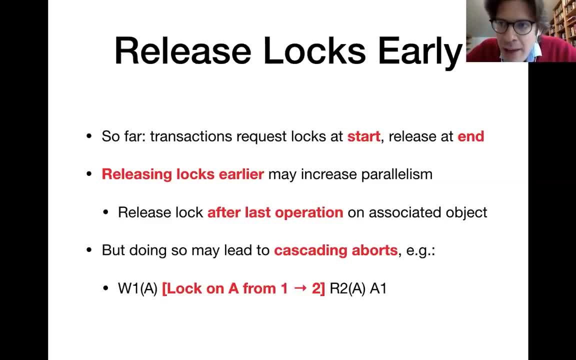 A. So unless transaction two is reading the value of A, it cannot be influenced by transaction number one. So here we only talk about influence, because one transaction reads a value written by another transaction. So in this case, if transaction two had read a different object than A, we wouldn't have 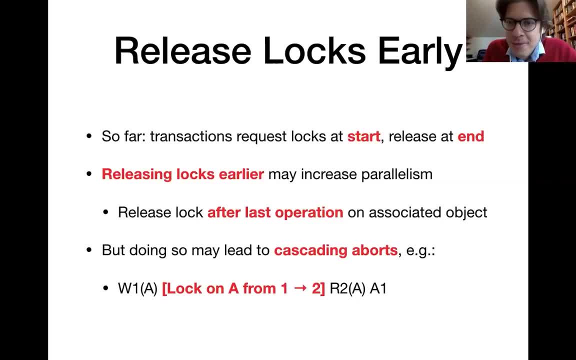 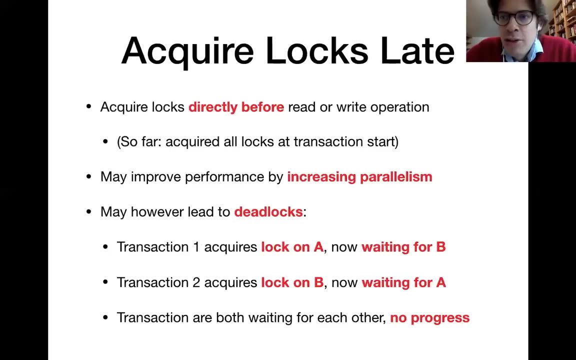 a cascade in the bottom? Great question. Let me quickly move the chat to the side. Okay, Here we have refined and allowed transactions to release logs earlier. Now we're going to allow them to acquire logs later. So essentially we have so far. 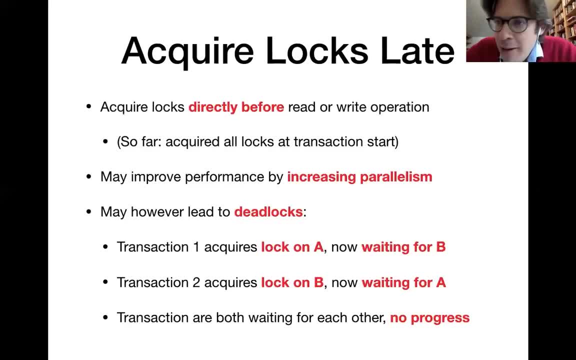 So basically we have required a transaction get all the read and write logs before transaction processing starts. But strictly speaking that's not always necessary, because maybe a transaction wants to start working with object A and it can already do this as soon as it has the log on object. 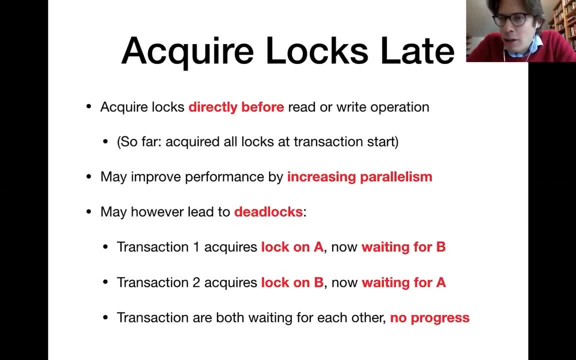 A. Afterwards it will continue working with object B, so it can delay acquiring the log for object B until it is done with object A. And, as always, if we reduce the time that logs are held by a transaction, it allows more transactions to proceed in parallel. 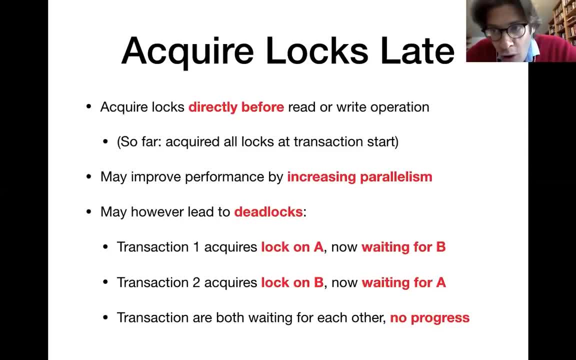 That's always the advantage. One drawback about acquiring logs late is what you see in this example. here It's called a deadlock- You might already have heard about it- And it essentially means that transactions are mutually waiting for each other and nobody can make progress. 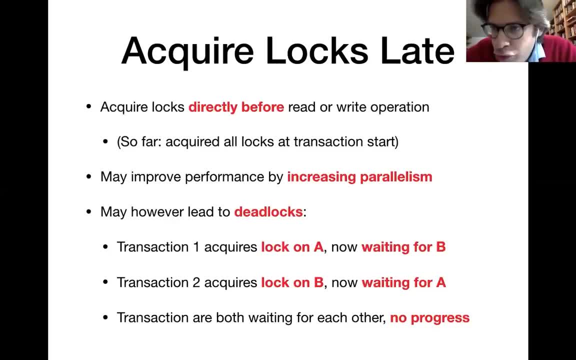 So here, for instance, a simple example: We have two transactions. In general a deadlock might involve more than two transactions, but in this example it's only two. And here transaction number one acquires a log on A and at the same time transaction. 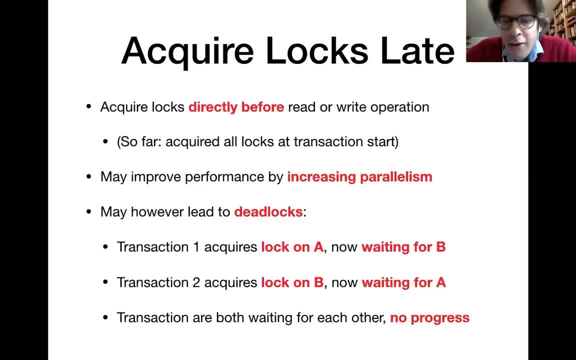 two acquires a log on B. Now transaction one has a log on A. transaction two has a log on B. Now transaction one wants to do something with object B, so it is now requesting the log for object B. This log is currently held. 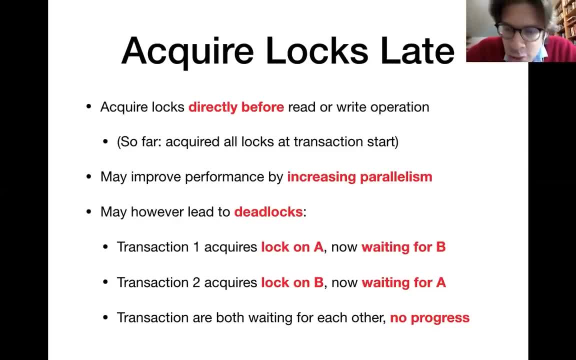 By transaction two. At the same time, transaction two is requesting the log for object A, which is currently held by transaction number one. So those two transactions each have one log that the other one needs to make progress, and that means that none of them can make progress because they will wait indefinitely. 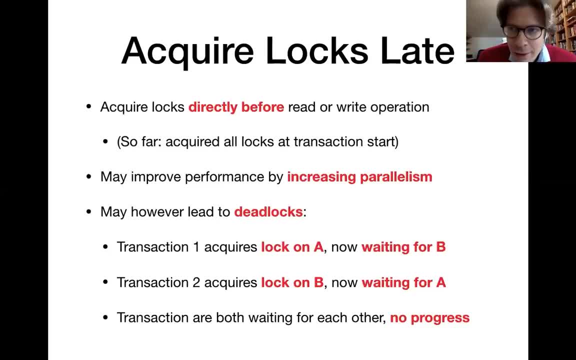 And what happens in reality is that the database system detects the situation and resolves the deadlock by aborting one of the participating transactions, so at least the other ones can make progress. We're going to discuss much more about deadlock handling in the following lecture. 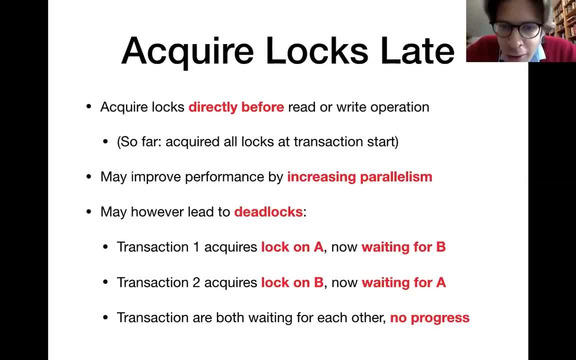 But just so you know, there's again a performance trade-off here. If we allow the transactions to acquire logs late, we might increase the number of transactions that can proceed in parallel. On the other side we might have deadlocks and that can have a bad impact on performance. 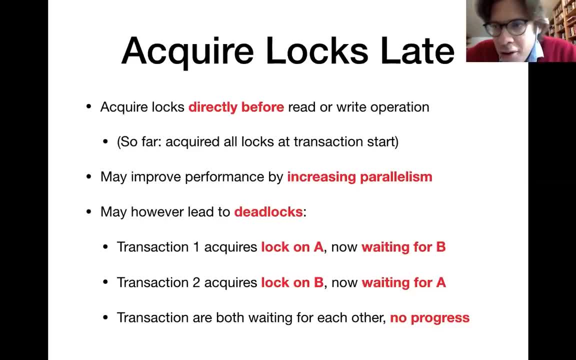 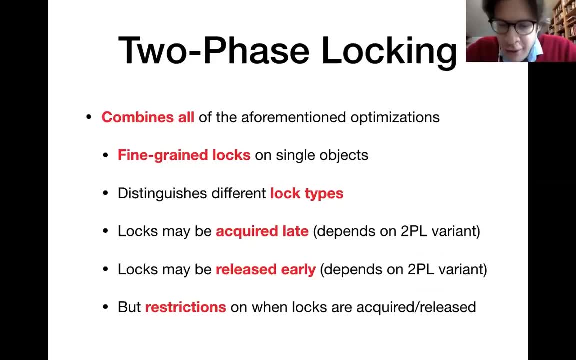 So, depending on the scenario, This is either a good idea or not a good idea for performance. Now, the title of this lecture is two-phase locking, which is one very popular locking protocol which essentially combines all of the advantages that we have seen so far. 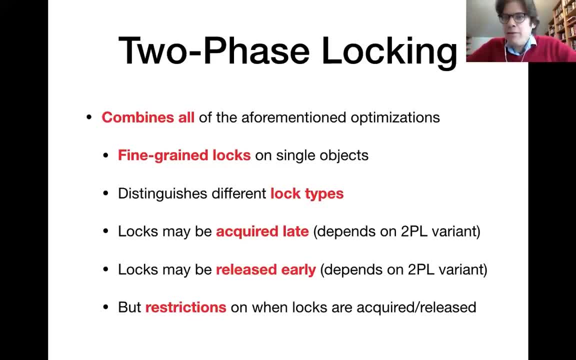 Namely. first of all, it allows for fine-grained logs. We don't have one big log for the entire database, but specific logs for database objects. It distinguishes different log types: Shared, meaning read logs. Exclusive meaning write logs. 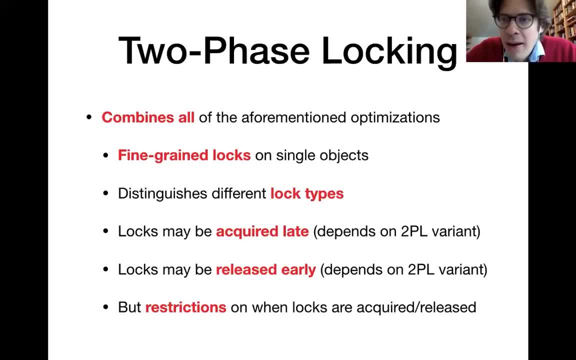 Depending on the variant of two-phase locking it might acquire to, it might allow transactions to acquire logs late. Also, depending on the variant, it might allow transactions to release logs early. There is, however, some restrictions in general about when transactions might acquire and. 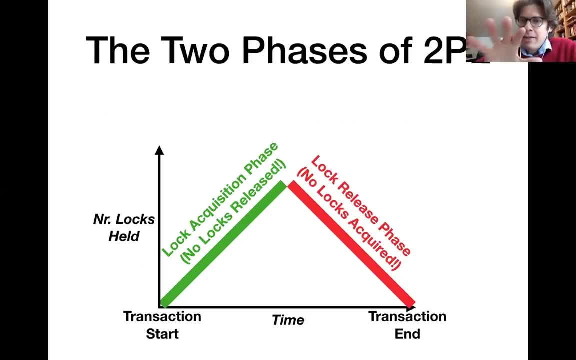 might release logs. This is an illustration Of those restrictions. as the name two-phase locking suggests, you must have two phases when it comes to locking. In the first phase, the transaction can only acquire logs on objects, but not release any. 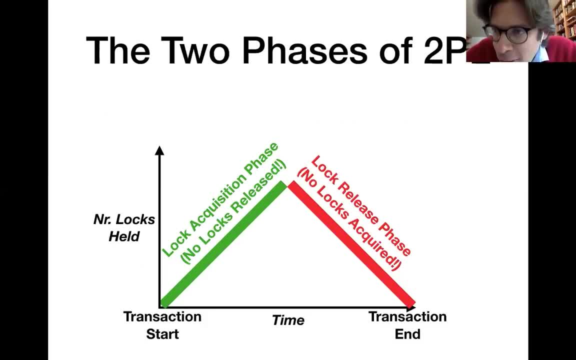 In the second phase, a transaction can release logs on objects but it cannot acquire any. So if you look at the number of logs acji, As you can see, the number of logs held per transaction over the along time larger than the approximate execution time of the transaction. 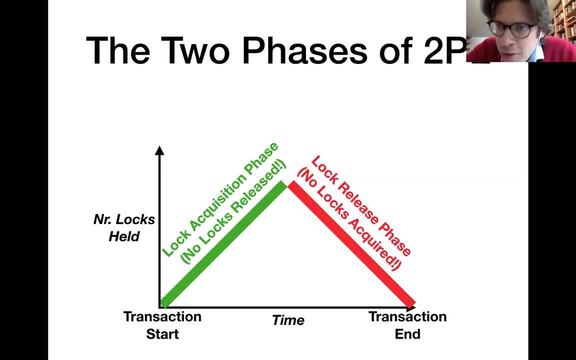 For the transaction, the exit second phase terminology in the transaction, into the transaction description of the transaction And, as you can see, the number placed on the blossom. And of course the number of logs held over the transaction. locks hold can only decrease. So those are the two phases of two-phase locking. 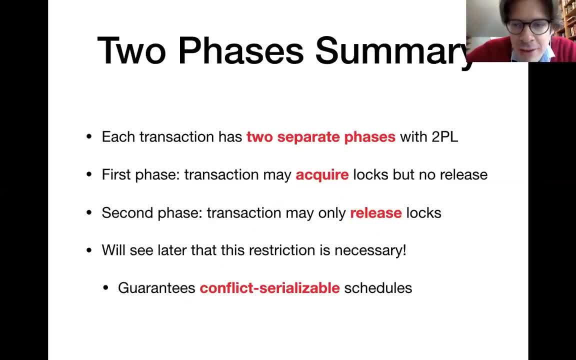 You have a summary of what I have just said. We have the phase in which we can acquire locks and we have the phase in which we can only release locks, And that becomes very important, as we will see later when we try to prove that this 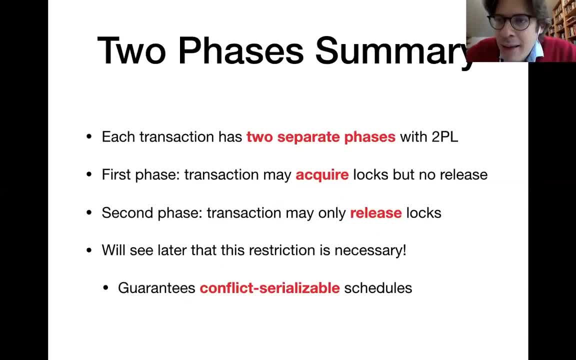 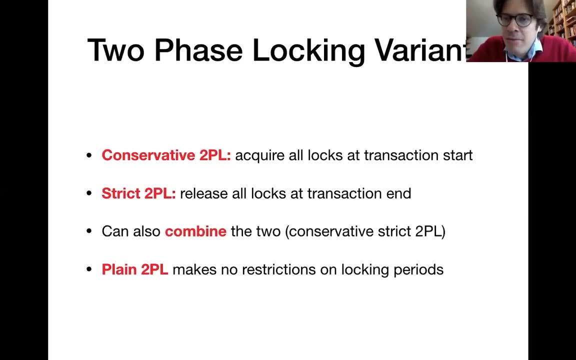 protocol guarantees that generated schedules are conflict-serializable. For that proof, we need that two-phase property. There's a couple of different variants of two-phase locking. First of all, we have conservative two-phase locking, which means that we do not allow transactions to acquire locks late. We 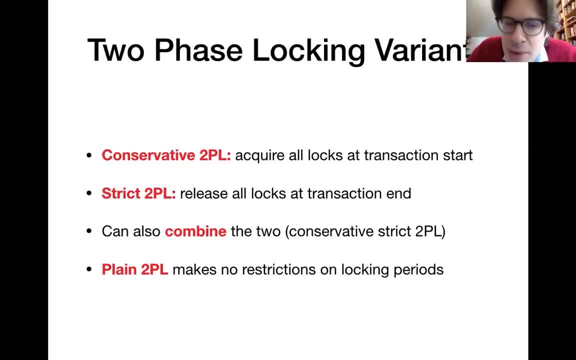 require them to get all their locks at the beginning of execution. Also, there is strict two-phase locking, which means that we do not allow transactions to release locks early. They have to keep them until the end of execution. So you can also combine those two and then you get. 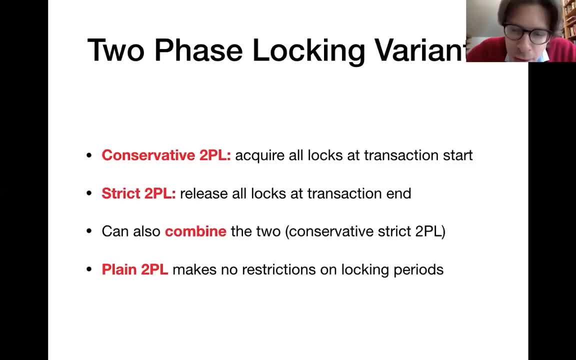 conservative strict two-phase locking and the plain two-phase locking makes no restrictions whatsoever. So we can illustrate those different variants using the same graph as we did in the previous slide. As we have seen before, we see how the number of locks of a transaction evolves over time. 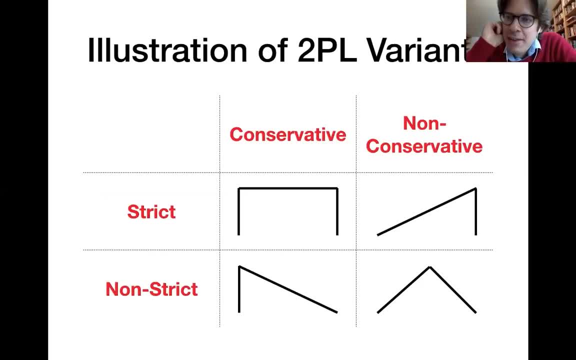 And as you see here for the conservative two-phase locking variants, at the very beginning of execution we always have a spike in the number of locks held. This is because we require conservative two-phase locking requires transactions to obtain all of their locks at once at the 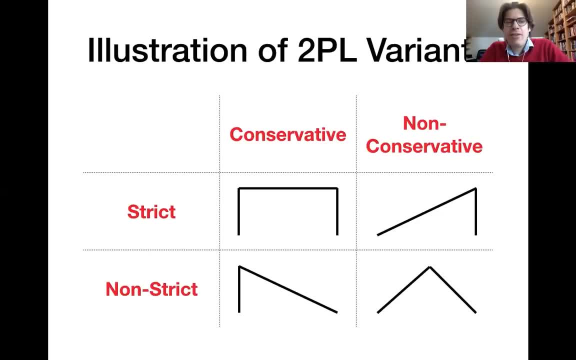 beginning of transaction execution. On the other side you have the strict variants until you have the sudden drop at the end of the transaction. This is because strict two-phase locking requires transactions to hold on to their locks until the end of execution and they release all of those locks at once. 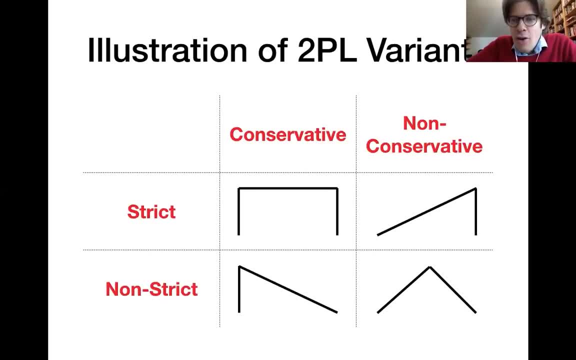 Now, if you look at the non-conservative, non-strict, two-phase locking, that's the plot that you have seen previously. here we can have some kind of ramp up. Here we can have some kind of ramp up. Here we can have some kind of ramp up. 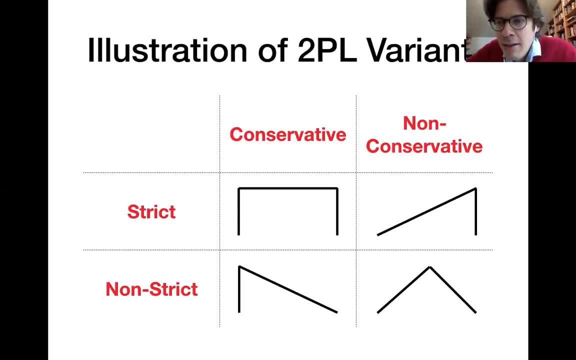 In the first phase and then some decrease in the second phase. Of course this figure here is simplifying. If you would draw that plot for an actual transaction execution you would get something much more messy. But the general tendencies that you see here, they do apply. 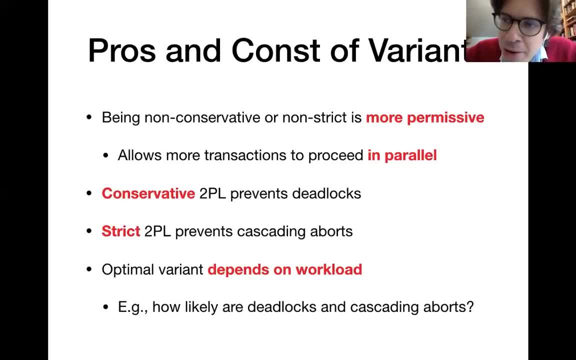 So all of those variants of two-phase locking are used and depending on the scenario- it depends on the scenario- which one of them performs best- There's a couple of pros and cons. There's a couple of pros and cons about those different variants that I'm summarizing here. 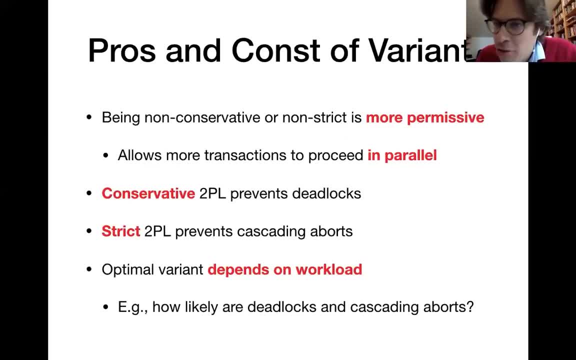 So generally, if you are non-conservative and non-strict, you're more permissive, which can be good for performance because it allows more transactions to interleave their steps and to essentially execute in parallel. The nice thing about conservative two-phase locking is that we prevent deadlocks, which 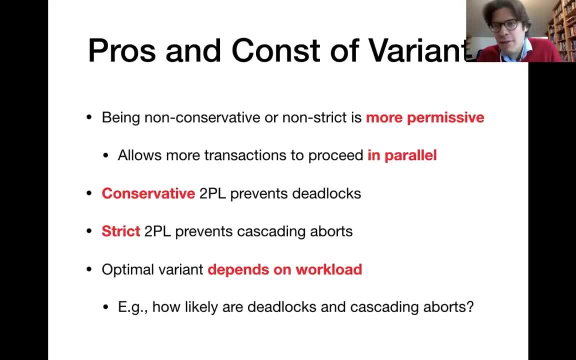 can be bad for performance because you might have to abort transactions and restart them. On the other side, if we go for strict two-phase locking, then we avoid cascading abort. So, especially in scenarios where it is quite likely that transactions abort, In those scenarios it can be helpful to have something which essentially localizes the 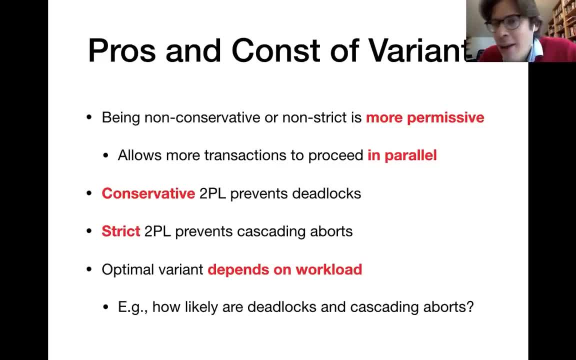 abort and avoids the chains of transactions that all have to abort because some initial transaction that they have directly or indirectly read from had to be aborted. So in general, you cannot say that one of them is better than the other one. It always depends on the specific workload which of them works best. 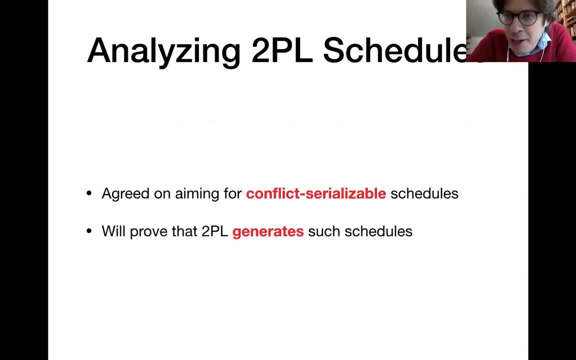 All right. So now we have seen two-phase locking, We need to convince ourselves that using it is really a good idea. Ultimately, what we want are conflict-serializable schedules. We have justified why we want conflict-serializable schedules in the last lecture. 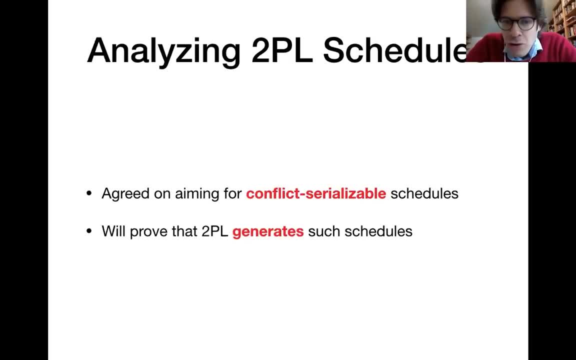 Now we have seen a concurrency control protocol, which seems to make sense, But at this point, how can we be sure that two-phase locking indeed leads to conflict-serializable schedules? How can we exclude that users see any of the anomalies that we have discussed in previous? 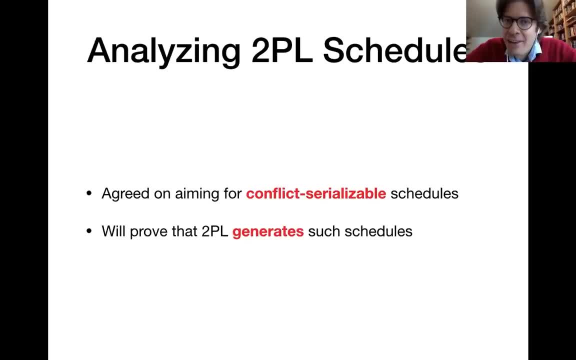 lectures In the following: we're going to analyze two-phase locking formally And we will prove that two-phase locking can only generate conflict. Okay, So we're going to use two-phase locking to prove that conflict-serializable schedules. Is there any questions on two-phase locking before I proceed with that proof? 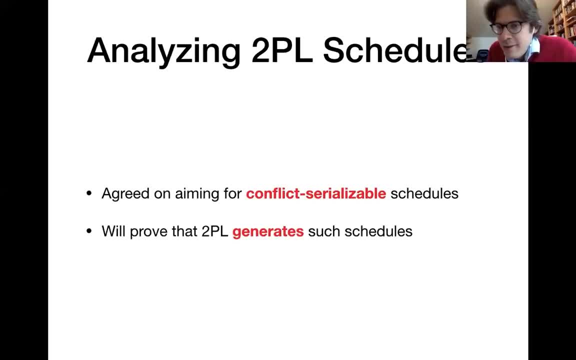 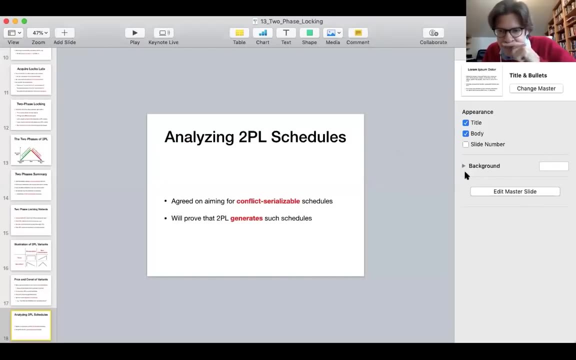 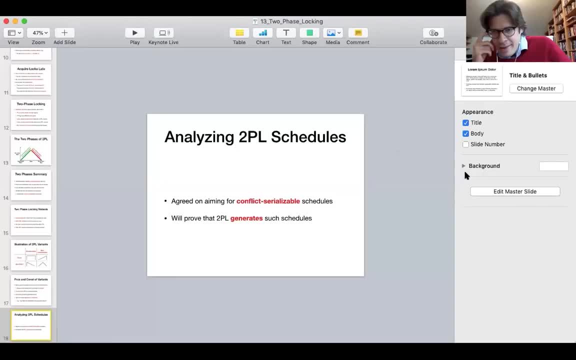 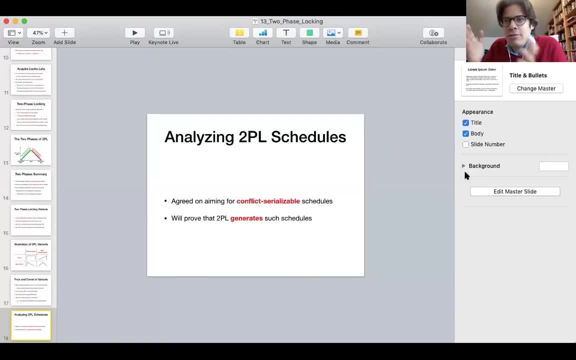 schedule that is serial, meaning it executes one transaction Okay, the other one, and we find that our current schedule is conflict equivalent to the serial schedule and two schedules are conflict equivalent if you can get from one schedule to the other one. we're only swapping operations that do not. 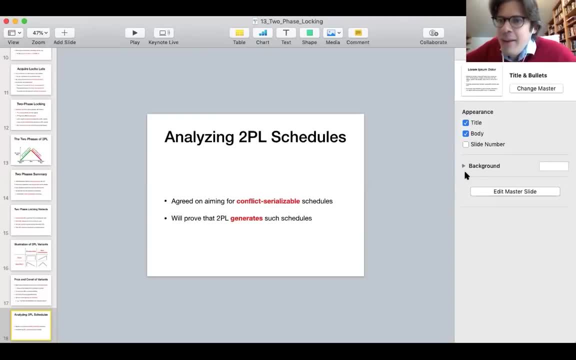 conflict and two operations conflict if they execute on the same object, if they belong to different transactions and if one of those two operations, at least one, is the right operation and the point of plain two-phase locking, we could say yes. so conservative two-phase locking has this advantage that it avoids step locks and strict two-phase. 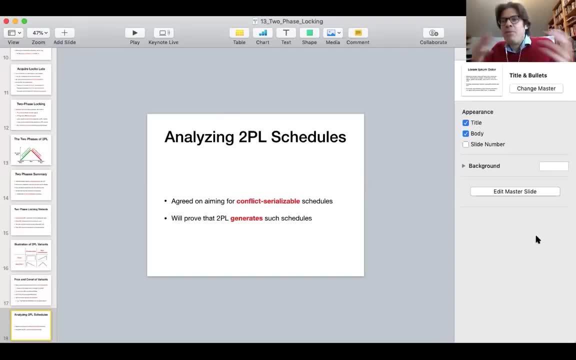 locking has the advantage that it avoids cascading a board. so what is the point of plain two-phase locking before any of those extensions? The thing is that plain two-phase locking allows transactions to acquire locks late and to release them hardly, meaning that the total time that a transaction holds a lock decreases in average, and 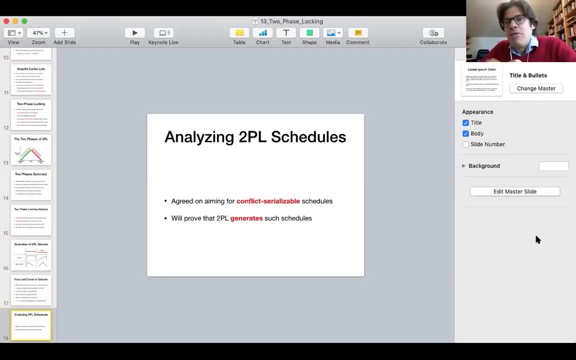 if a transaction holds a lock on an object, it prevents other transactions from accessing the same object. so the longer a transaction holds locks, the the longer it makes other transactions wait, And that is bad for performance. So if you reduce the time that a transaction is holding a lock, 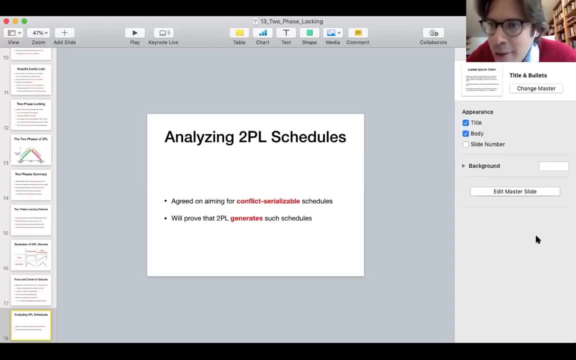 you reduce the lock waiting time for other transactions. That means that you generally reduce idle time and your transactions in the system can process faster. So if deadlocks and cascading of vaults are unlikely to happen, then you probably get the best performance with plain two-phase locking. 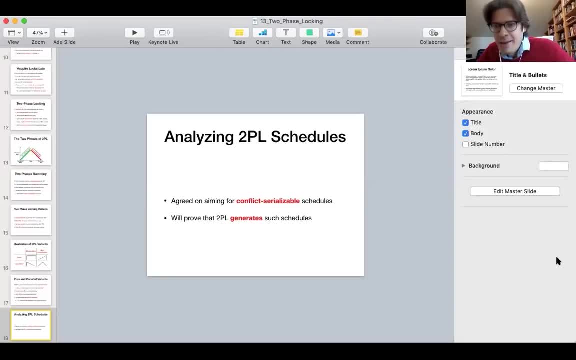 And yeah, it's a justified question. I mean, it sounds scary- Deadlocks and cascading of vaults- So one might think, why would people allow that to happen? But it really depends on the probability that it happens. If a deadlock is so unlikely that you would only have one deadlock per day, and you process millions of transactions, then probably you would still. but same for cascading of vaults. If transactions essentially never abort, then cascading of vaults are also extremely unlikely. So probably if you have only one cascading of vault per day or per year. 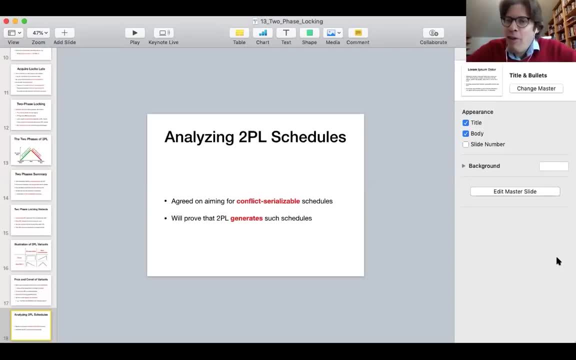 then you probably want to reap the performance benefits offered by reducing lock waiting times. So in the end it's a trade-off. You cannot say a purely which variant. which variant is best. It depends a lot on the properties of the workloads. 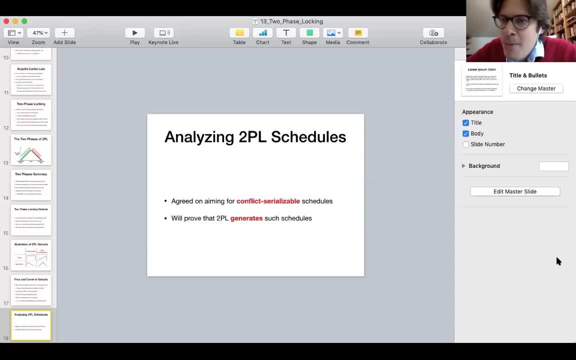 And this is why different variants are implemented in practice. And yeah, so in the end, if you're really serious about performance tuning, then you might even try for a specific workload which of those variants works best, But clearly you cannot say which one of them is the best. 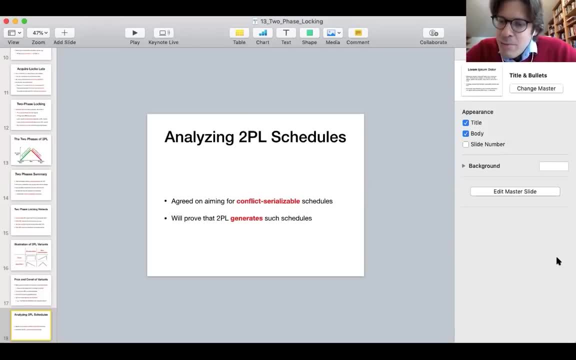 So the question is: what does it look like? what does it look like? And plain 2PL. why is it better than a transaction that simply grabs a lot before it needs an object and releases it directly after one? That's a great question. 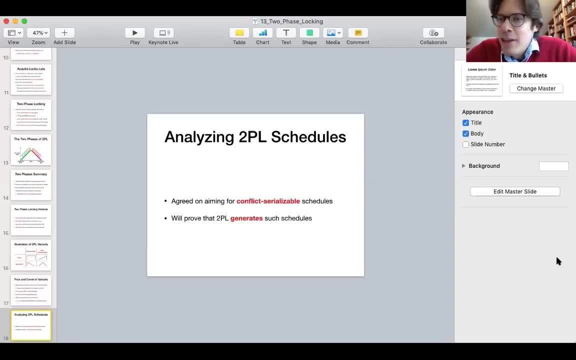 What is suggested here, basically, is something which doesn't necessarily follow the two phases of acquiring locks and releasing locks. So one could think, yes, why not? A transaction needs access to object A, so it acquires a lock on A, does what it needs to do with A. 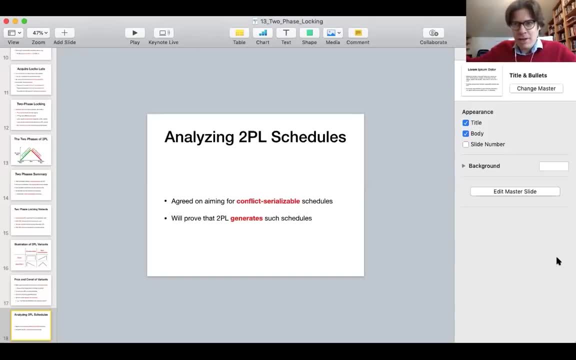 a and then releases the lock on a, and then it needs to do something with object b, so it acquires the lock on b, operates on b and releases the lock on b, and so on. in that way, i'm reducing the time during which locks are held. however, i'm not following those two phases of a two-phase. 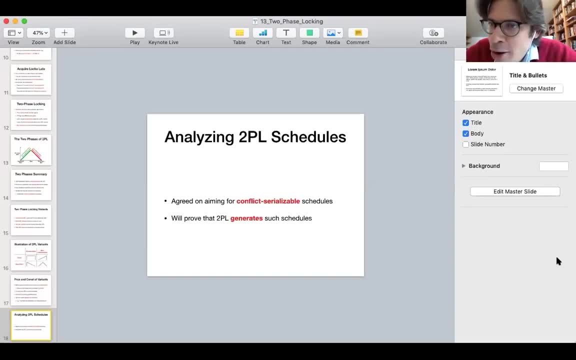 locking, because the transaction would first release the lock on a and then again acquire a lock on b, and at this point it is probably not clear why that is a problem. but during the proof that we are about to do, we will actually see why we need those two phases in order to guarantee. 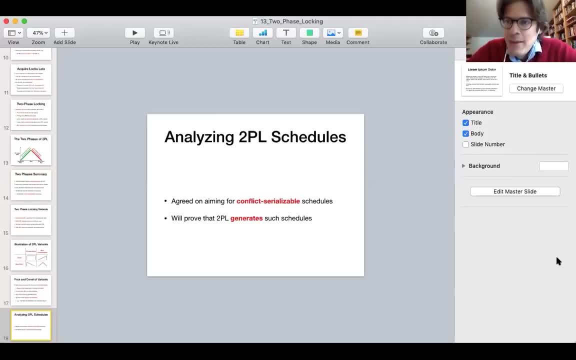 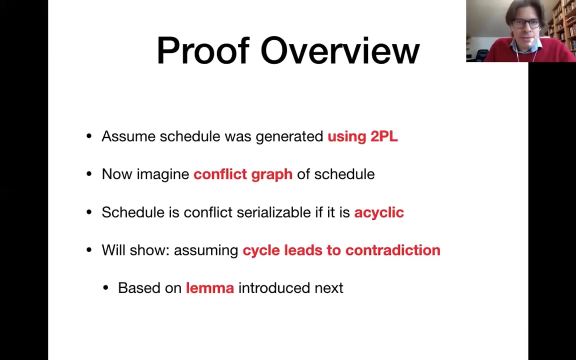 that two-phase locking generates conflict serializable schedule. so this is a great question. let's table it for the moment, but it will become clear during the proof. okay, great questions, all right, i think let's proceed with the proof. okay, so this is an overview of the proof that we will do in the following. so we will essentially 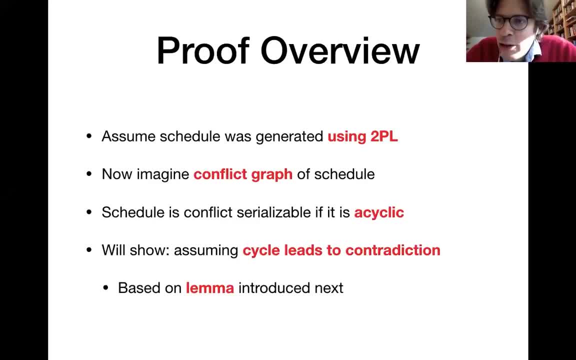 um analyze schedules that were generated using a two-phase locking concurrency control protocol, and now we assume essentially, could it be- that one of those generated schedules has a cycle in the conflict graph? because if it has a cycle in the conflict graph it means that it is not conflict serializable, as we have seen before. 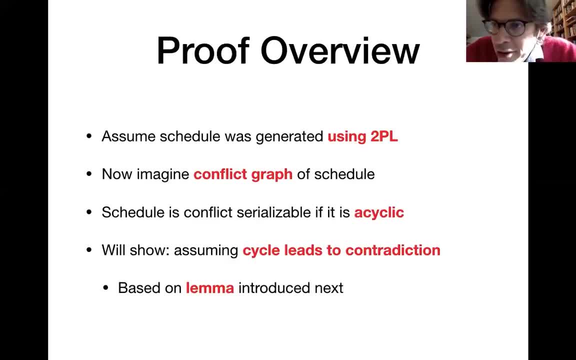 now in the following. we will essentially prove that if a scheduleологic was generated using two-phase locking, it cannot have a cycle in the conflict graph and therefore it must be conflict-serializable. In order to conduct this proof, as a help, as a lemma, we will prove the following. We will prove this. 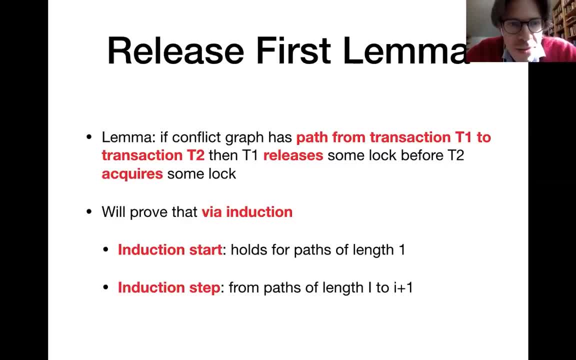 what I call the Release-first lemma, which essentially says that if in the conflict graph I have a path from transaction one to transaction two, then I must have that. transaction one releases a lock on some objects before transaction two acquires a lock on some objects. So very important, we don't even 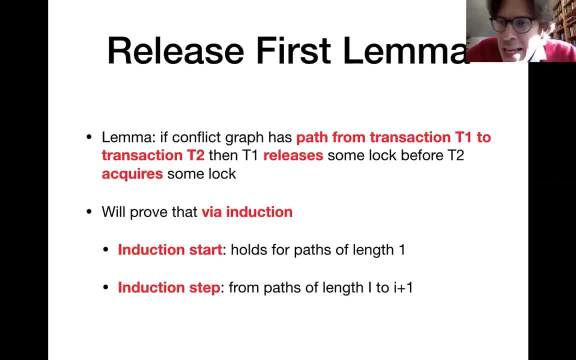 require the release transaction 1 and 2 are releasing and acquiring locks on the same object. it could be different objects, But if there's a pass from one transaction to the other one in the conflict graph then the first one must release a lock on. 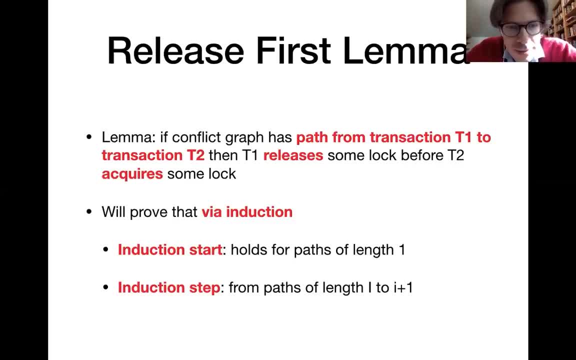 some object before the second one acquires some lock. This lemma will be proven via induction, And induction generally means that you first prove something about a trivial case and then you make the induction step, where you essentially reduce larger instances to smaller instances. Now, in this specific 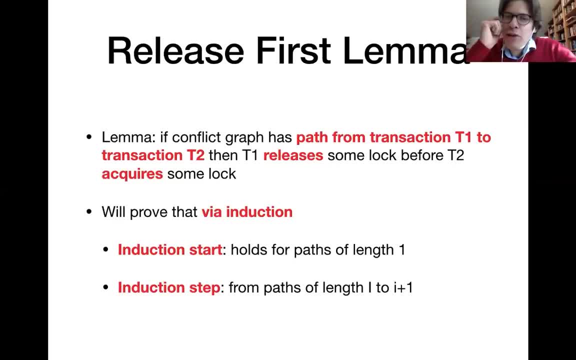 case, what we will do is: we will first of all prove: does this lemma holds for paths of length one? so basically, we have just one step from one transaction to another one in the conflict graph and in the induction step to proof that if the lemma holds, 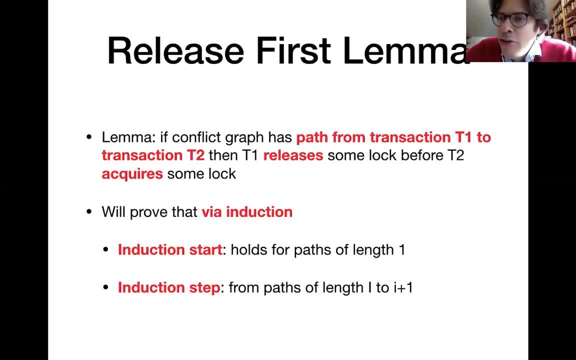 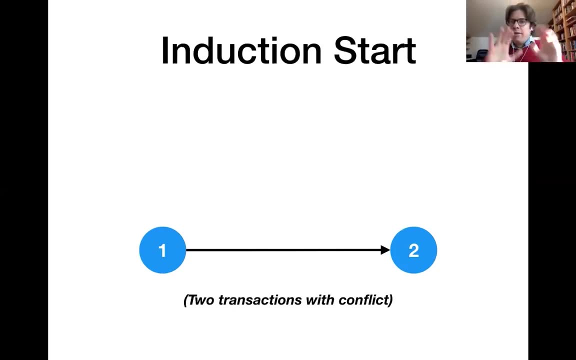 for paths up to length i, then it will also hold for paths of length i plus one. So we always extend the coverage of the lemma in terms of path length. This is the induction start. So we have two transactions, one and two. 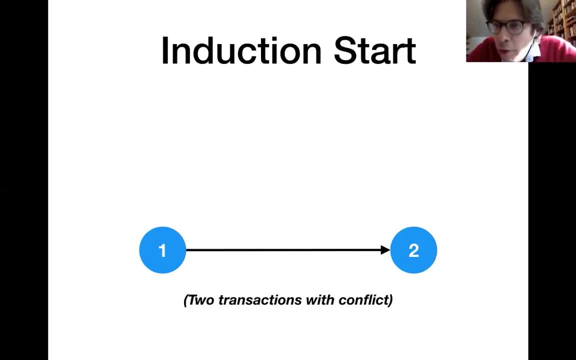 and they have an edge connecting them in a conflict graph of the schedule. That means they have a conflict And a conflict generally means that both of them work on the same object and at least one of them is writing to the object. So we essentially have three possibilities: Either transaction one is reading object a. 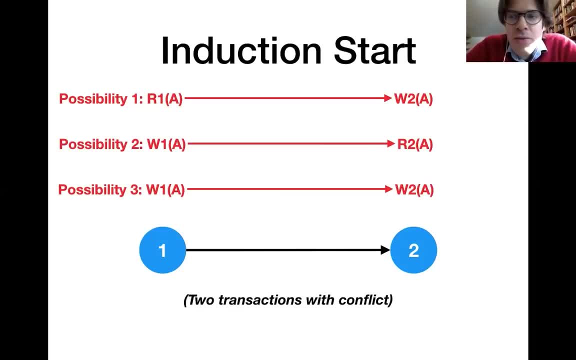 and then transaction two is overriding it. or transaction one is writing to object a and then transaction two is reading it, Or both of the transactions are writing to object a. So the second transaction is essentially overriding the value of the first transaction for a. 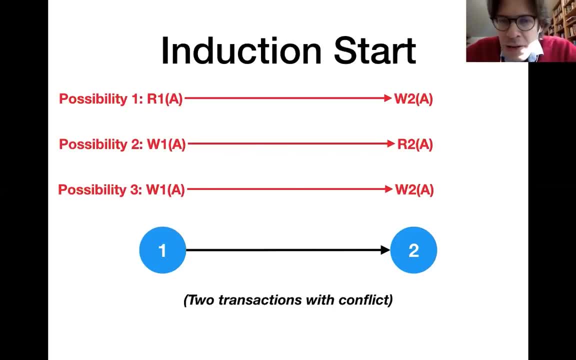 Now, in all of those cases, what I need to have is that transaction one releases the object on a before, transaction two acquires the log on a Now. transactions generally need logs in order to operate on objects, And here, for instance, for possibility one. 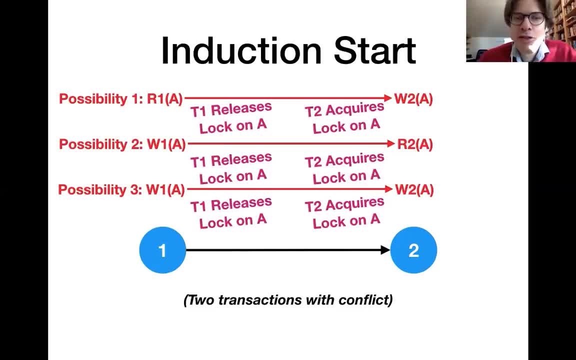 it seems that transaction one had at least the read log on object a, so it can read the value. Transaction two needs a write log, an exclusive log, in order to write something to object a. Now an exclusive log and the read log. they are mutually exclusive. So in order to grant an exclusive log, 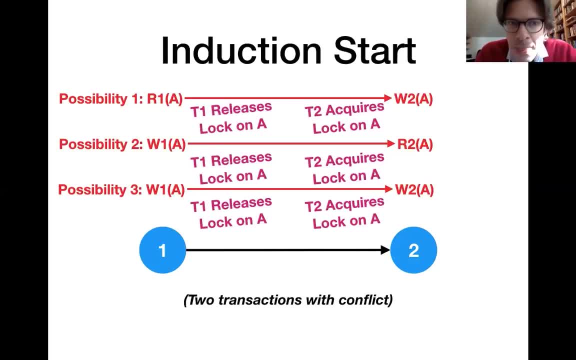 an exclusive log on object a to transaction two, the log manager first needs to get back the read log for object a from transaction number one. So here, definitely, in order to make this possible, in order to enable possibility one, the log, some log on object a needs to get released by transaction one and a log on object a. 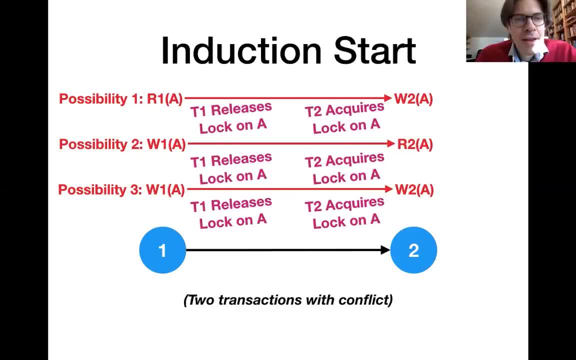 needs to be acquired by transaction two. Now the principle is similar for possibility two, also for possibility three. So here basically, transaction one needs first to hold an exclusive log on object a, and it needs to release that exclusive log so that transaction two can acquire another exclusive log on object a. So here again you have. 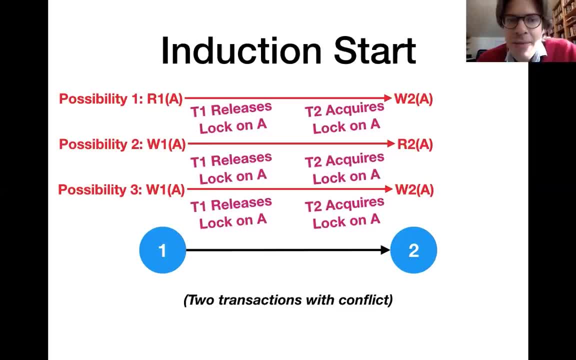 what we wanted to prove In all of those cases, because there's a conflict between them. we must have that transaction one releases a log on some object before transaction two acquires a log on some object. So this is what we want to prove. We have proven it for pairs of length one. 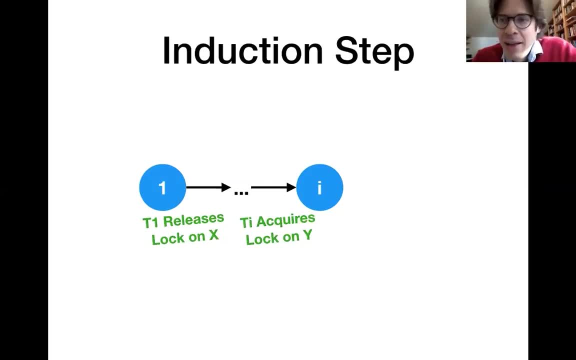 Now let's say that we have proven things for a pair's length of up to i, and now we want to prove that this implies that it can be proved for a five pay range and the%, And we also want to prove that this implies that it. 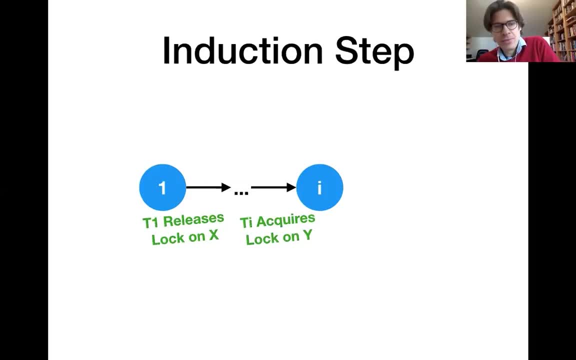 also holds for paths that are one step longer. So here we want to extend for paths with i nodes to paths with i plus one nodes. All right. So first of all we have, we assume that we have already proven via induction that if I have a path of a length of with 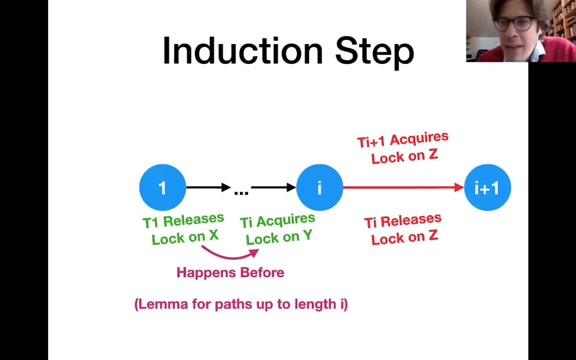 up to. i nodes that the first transaction in that path releases a lock on some object before the last transaction on that path acquires a lock on some object. It doesn't have to be the same object. So we have proven this. We assume that we have proven this via induction. 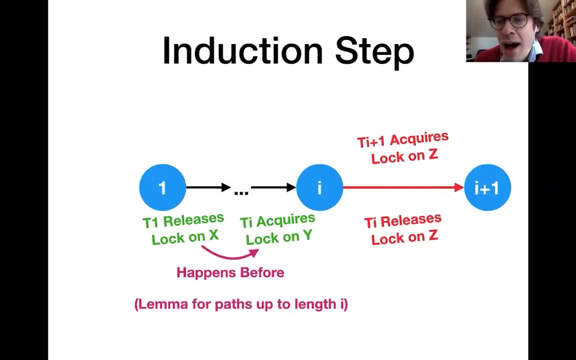 Now looking at the connection between transaction i and i plus one. using the same reasoning as on the previous slide, we also know that since there is a conflict between them, transaction i must release a lock on some object set before transaction i plus one acquires a lock on. 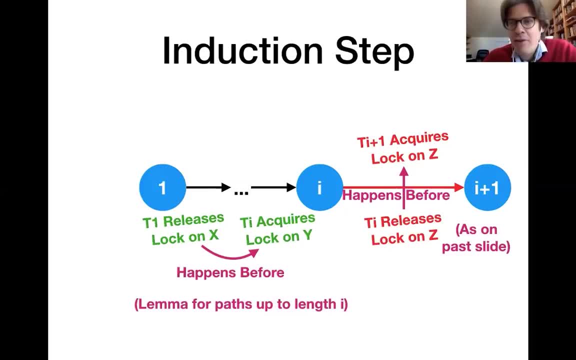 set. So this is even more specific than on the other side of the screen, because as long as we only consider one step and there's a conflict between them, we can never know that the other side of the screen is the same. we know that the conflict must concern the same object. 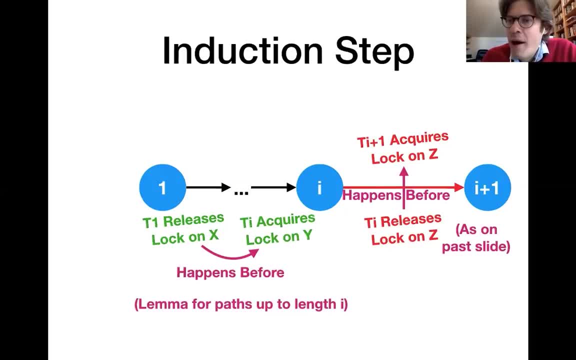 So the locks get released and acquired for the same object. All right, so now those things. so I'm already close to proving the lemma. I want to prove that transaction one releases a lock on some object before transaction I plus one acquires a lock on some object. 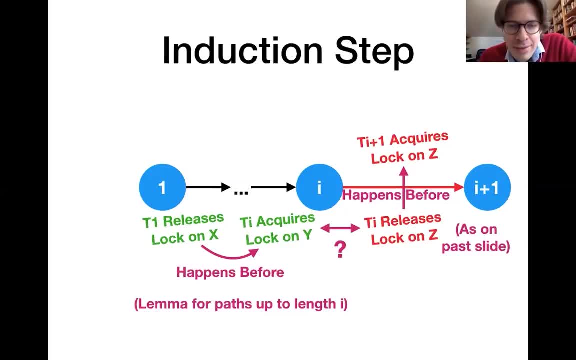 The question is just this: If I compare the acquire lock- acquireage I'd like- the operation by which transaction I acquires a lock and the operation by which transaction I releases a lock, which one of them happens first? We have had the question about why we need those two. 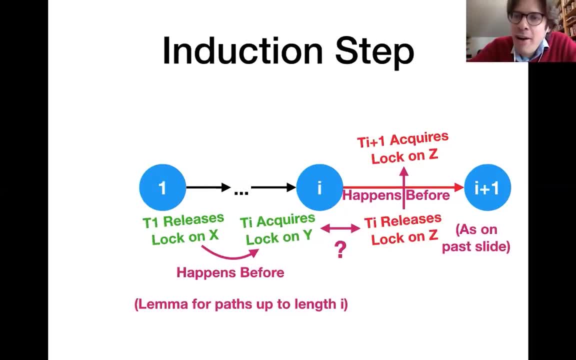 faces Of a two-phase locking, And this is exactly the point at which we need them due to the properties to do the constraints of two-phase locking. And now that I have those two faces where first I only acquire locks and then only release locks, 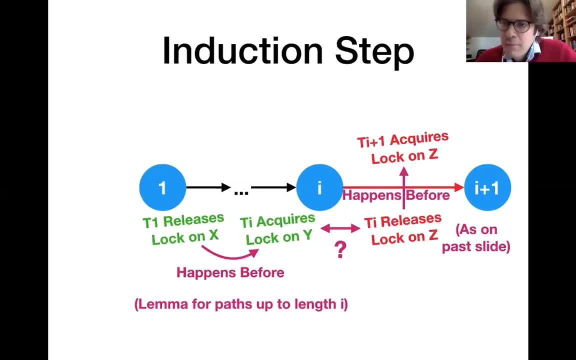 And that means, when considering this transaction, I, if I have, I acquire stock on while and I release a slot on set due to the constraints of two phase locking, and know which of them must happen first because transaction always acquire locks first before they release. 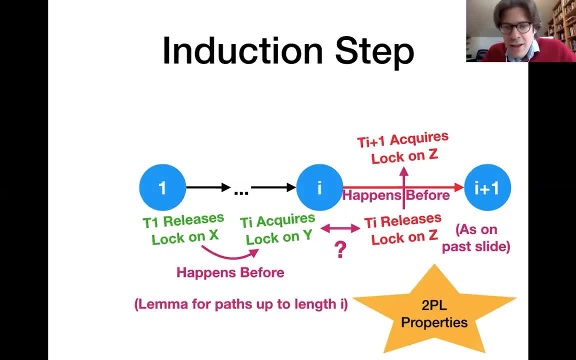 locks later, And that means due to the properties of two-phase locking and all that, we must acquire the lock on, why before we released the lock on set, Now I have here happens before. chain of events, and taken together That means again that transaction one on that pass releases a. 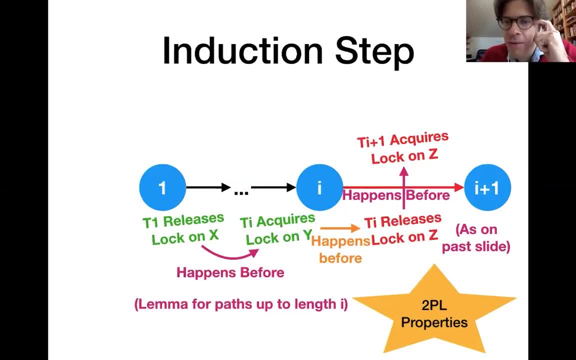 lock on X before Transaction, I, plus one on that pass, acquires a lock on set. And this is- this concludes the induction step. So by applying this recursively I can essentially expand the lemma to pass off infinite lengths And therefore I know that if I have a pass in the conflict graph. 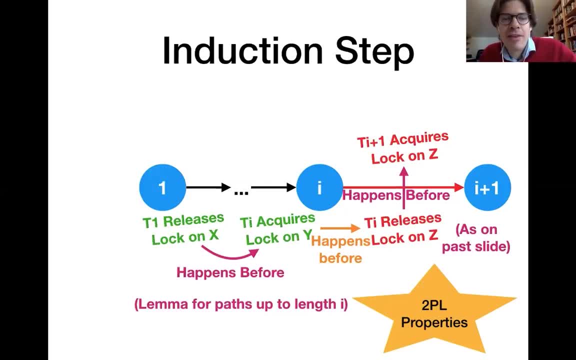 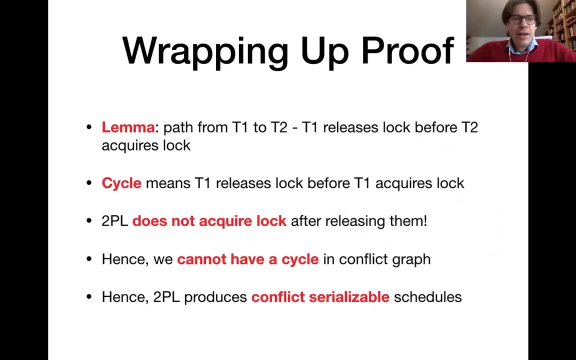 from one transaction to the other one, that first transaction must release a lock before the last transaction acquires a lock. Now, how does this help me with the proof? Now, if I have this lemma- and I assume that I have a cycle in the conflict graph- then due to this lemma, it essentially 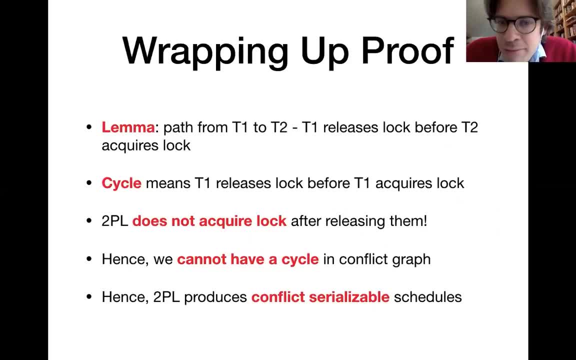 says that some transaction in that cycle releases a lock before that same transaction acquires a lock right. So we have a pass from T1 to T2, means, according to lemma, T1 releases lock before T2 acquires lock. Now I have a pass from a transaction to itself, a cycle, basically. 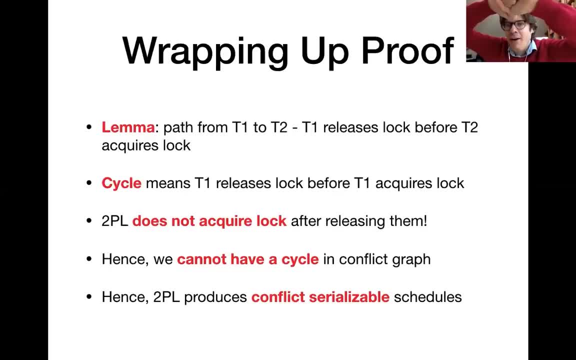 That means that T1 releases a lock before T1 acquires a lock. And now again we use the properties of two-phase locking because that is not possible. Transaction cannot acquire a lock after it has released the first lock on any object. 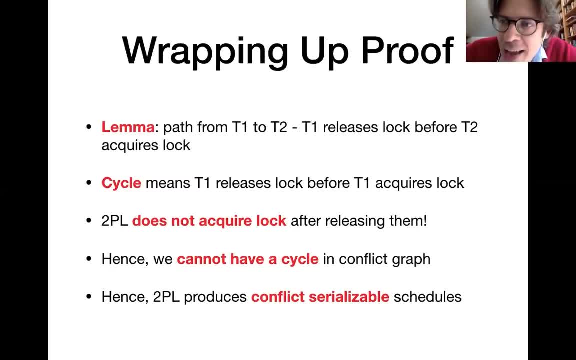 And because of that I can conclude that I cannot have any cycles in a conflict graph as long as I use two-phase locking in order to generate them. Had I not used the constraints of two-phase locking, then it could very well be a cycle in the conflict graph that I'm generating, and 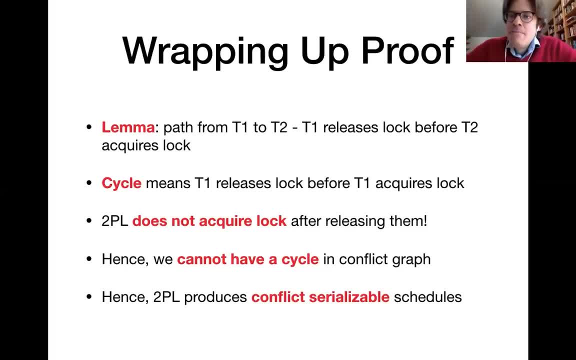 that means that I don't get a conflict-serializable schedule. But since I made those restrictions of two-phase locking, because of that I can be sure that all the schedules that I'm generating are conflict-serializable. All right, so now we have shown that using two-phase locking, we 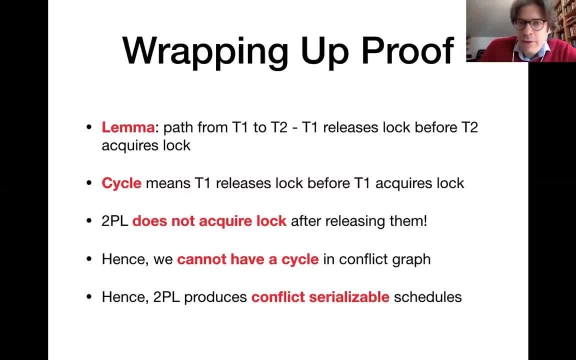 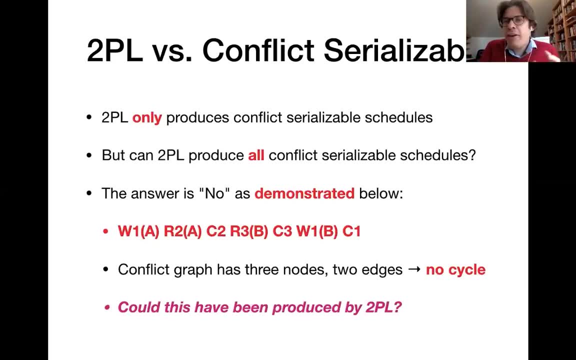 generate only conflict-serializable schedules. Now the last interesting question, perhaps, when comparing two-phase locking to conflict-serializability here, is: what about the other way around? Could two-phase locking, at least in principle, generate all schedules? 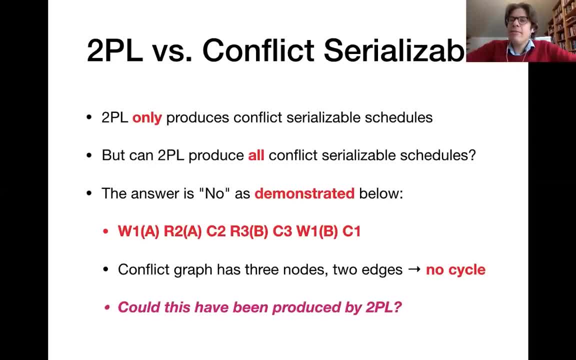 that are conflict-serializable And, as we see, we have two-phase locking And, as we see here using an example, that is not the case. In fact, I wanted to ask you whether that can be the case, based on the. 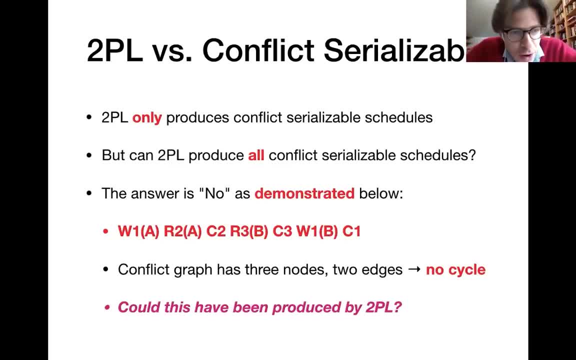 example that you see here. All right, I already gave you that, Okay, and it is also said on the slide. So we could not in general generate all the conflict-serializable schedules using two-phase locking, If you consider, for instance, 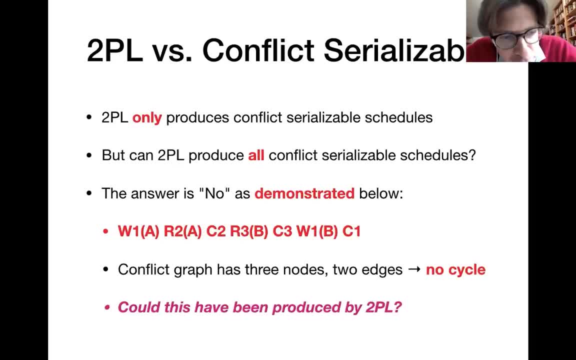 this example here, this example schedule: transaction one writes something to object A. transaction two reads from object A and commits. transaction three reads object B and commits. transaction one writes again to object B and then commits. So if you would draw the conflict graph, we have three nodes and we 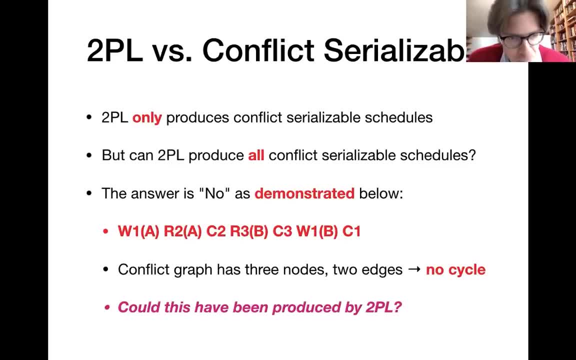 have two actors and we have a node. So we have a node cycle here. We have only this conflict on object A between transaction one and transaction two, and then we have the conflict on B from transaction three to transaction one. So this is conflict-serializable. but the question is, could this? 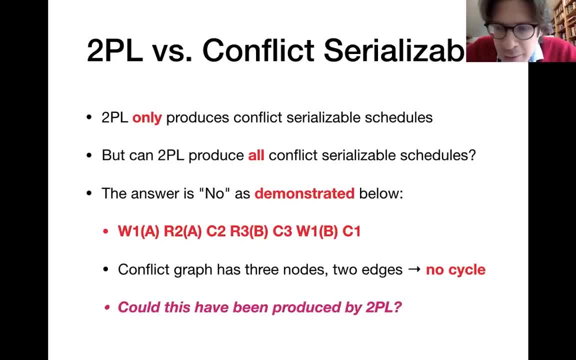 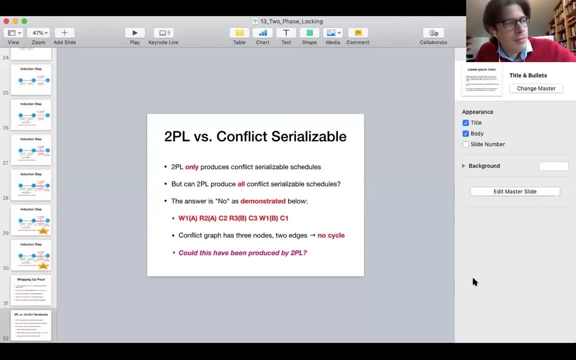 have been generated using two-phase locking, If you have a second to think about it and put a proposition into the chat. If you think about where logs are requested and granted, could we have factors? If you think about which logs transaction one, for instance, is a? 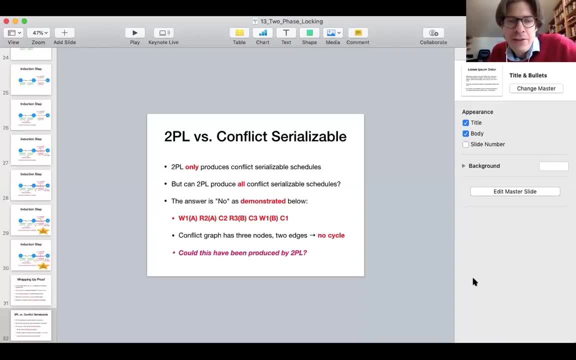 cost. and then if you think about why they're not being counted, they're not being generated, And if you look at where the destructs in the transaction one come, you'll say that they are, they help us, And then you could think of other ways to compute them. The last one is that the one call is considered from the other end. So if you're doing, let's say, for example, a transaction one, for instance a cost, and then we replace it with the transaction two, then we are on the point of analysis of the commonользability. 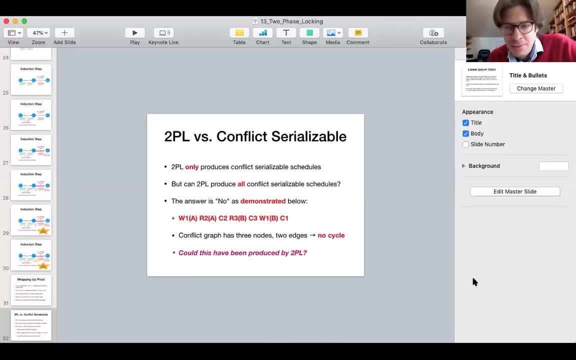 So, for example, this is a cost and it's a transaction. two, and at the end it's a cost of the common operation: acquiring and releasing. okay, some first propositions here. okay, very good, yes, very good. okay, so, very good, okay, so I have the correct solution by multiple. 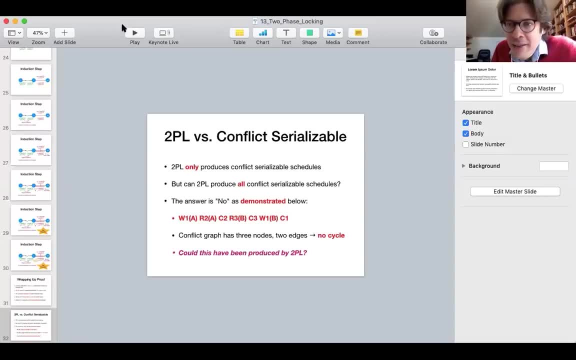 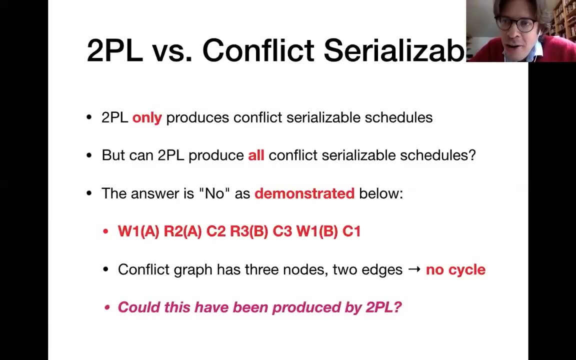 people very good, okay, all right, let's discuss it. I quickly in more detail, alright, so if you think about the lock requests, then, like about Ben transactions, acquire locks and release locks, and we focus on transaction one, alright, so the very first operation, the schedule is a right operation by 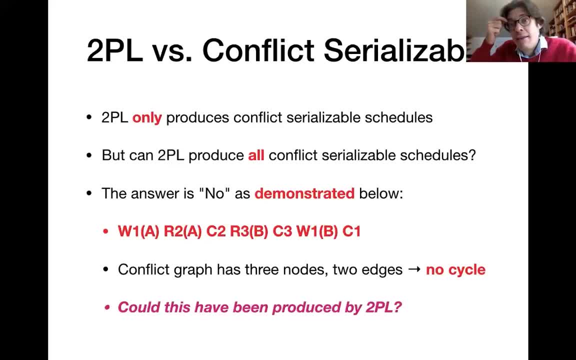 transaction one on object a, and that means that transaction one theory must have the right lock for object a, otherwise it couldn't write to it now. if immediately after that, transaction two seems to be reading from object a, that means transaction one must have given up the right lock on a, because otherwise 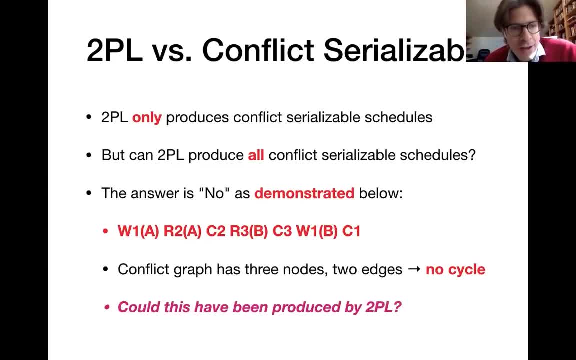 the read would not be permitted by a different transaction. so clearly, between the first step in the schedule, in the second step transaction one must have given up the lock on a. now things continue here. we have to commit, okay, and of course we know the physical number of the right locks you have to commit. 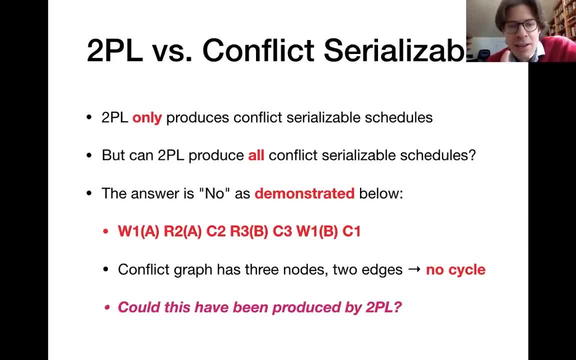 there is a right lock on a. so if, because it's a three-time decision, we not be able to have a spirit lock on object a, it must be 100, okay. so transaction three is reading object B. so clearly, at this point transactions we must have read lock on object B and then commit and now transaction one write to object b. that means that at this point transaction one would need to have a right lock on object B. now the question is: could it have had that right lock on object B? now the question is, could it have had that? 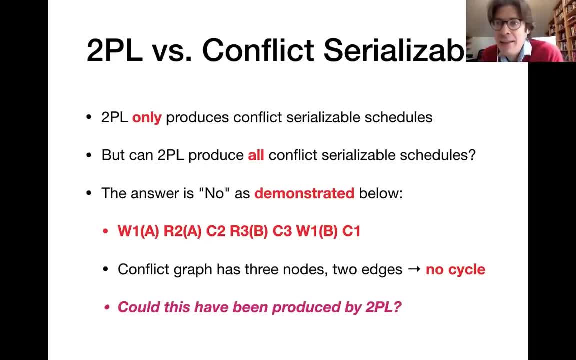 locked maybe since transaction start? the answer is no, since just before that transaction three has read from object b. so obviously transaction three had a read lock on b at that point. so transaction one must have acquired the lock on b? um directly before the write operation, but on the other side it has released the lock on a after the first step in order to make it. 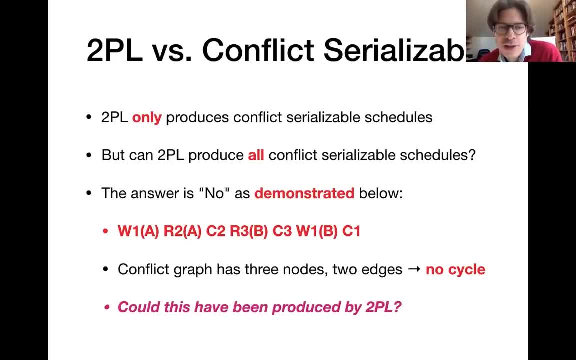 accessible transaction two. so what we would have here is that the first transaction first releases a lock- before it the lock on a- before it acquires another lock, which is the lock on b, and since too fast locking does not allow transactions to acquire locks after they have released any, 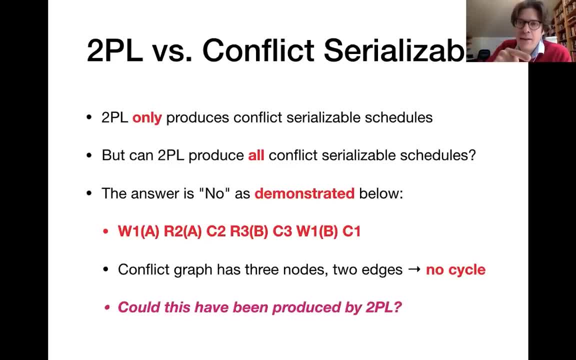 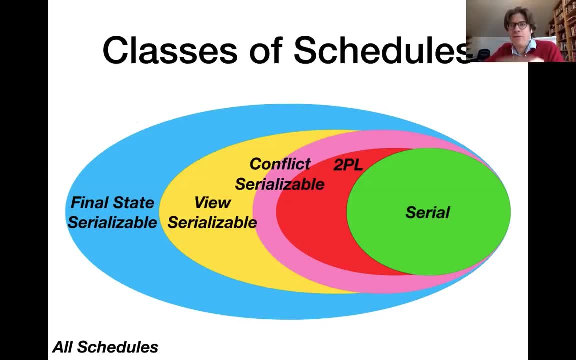 means that this schedule here, despite being contractualizable, it could not have been generated by two-phase locking. that essentially answers the question. now we have the full overview picture here. so we've discussed about all those different classes of schedules. um, we have, uh, all schedules contained within them are the final state. 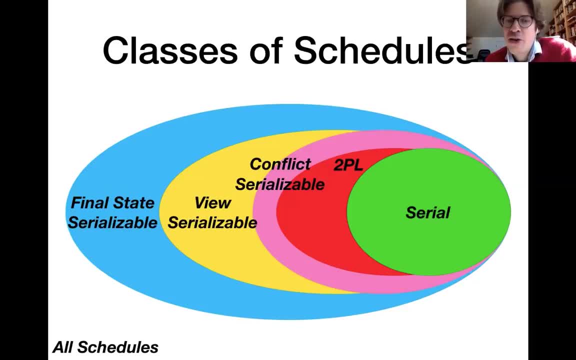 serializable schedules, then the view serializable schedules, then the conflict serializable schedules, and now we know that two-phase locking essentially is a subset, like the schedules that could have been generated using two-phase locking. they are a subset of the conflict serializable schedules and a small subset of that again would 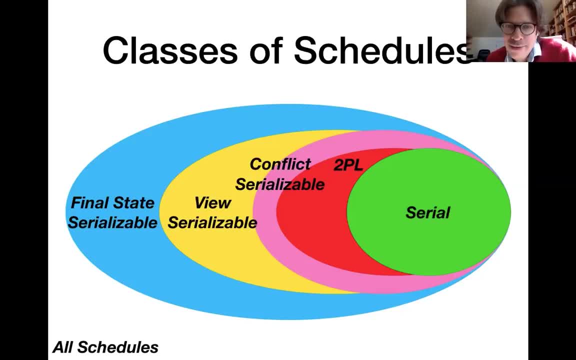 be the actually serial schedules. so this is basically what we can hope for. we guarantee that two-phase locking generates conflict serializable schedules. so we i have no strange anomalies. ideally, we, of course, would like two-phase locking to be able to consider all two conflict serializable schedules. that is not the case, but nevertheless, two-phase locking is one of the most. 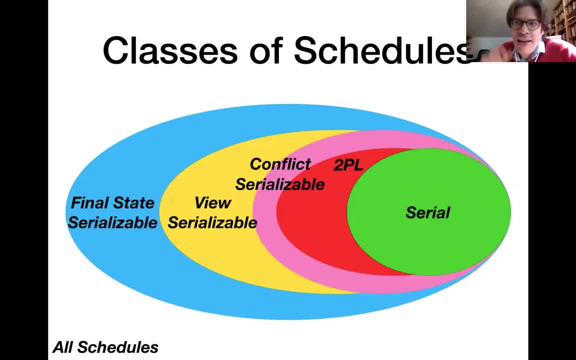 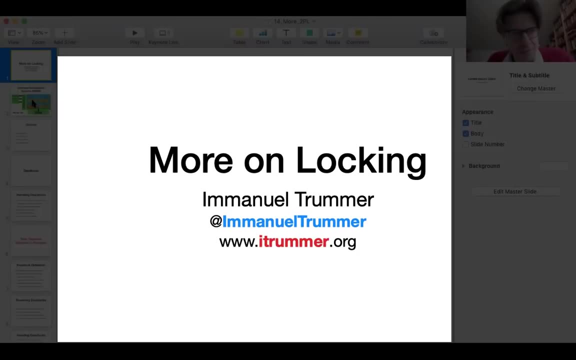 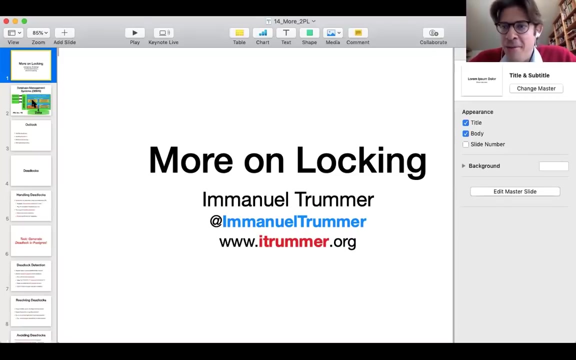 popular locking protocols used in practice. in the next lecture we're going to discuss about a couple of extension before we also discuss about different concurrency control methods. wish you a nice weekend and then i see you again next week, okay, good, so let's uh get started. sorry for the delay. um, today we are gonna talk more about locking, two-phase locking, that's. one of the most popular locking protocols- and we have seen the basics of proof- is talking last time. in this lecture we're going to discuss about a couple of special cases and scenarios. um, we are still discussing about the transaction manager. the data is still just coming. we see there is a flying 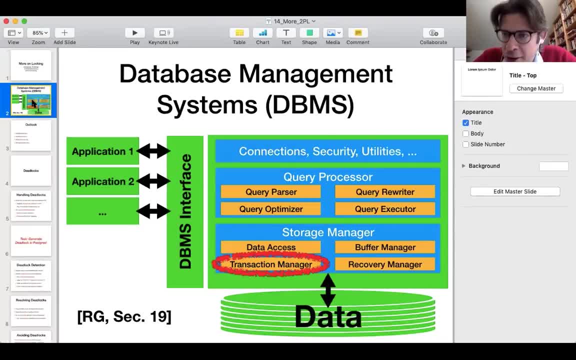 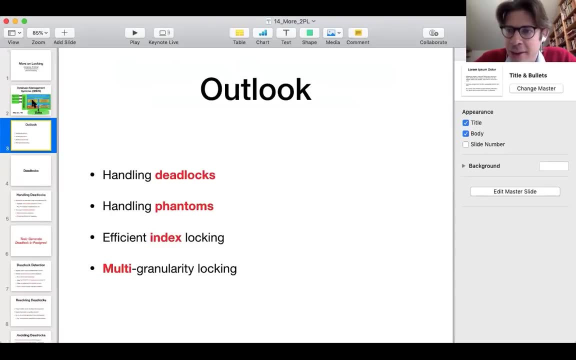 program. we are still discussing about the transaction manager database system and the relevant chapter in Ramakrishna and Gerke, that is, chapter number 19.. Now in this lecture we're going to discuss about a couple of special scenarios. We're going to discuss about what happens if we have a deadlock. We're going to discuss about an anomaly called 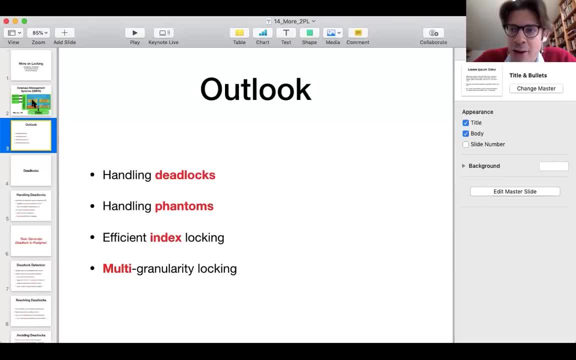 phantoms. I have already mentioned that anomaly quickly at the beginning, but I have told you that we will postpone the discussion until later. We're also going to discuss about locking specifically in index data structures and in the end we're going to discuss about multi-granularity locking. 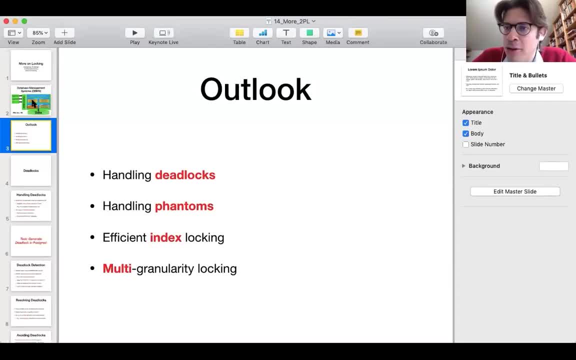 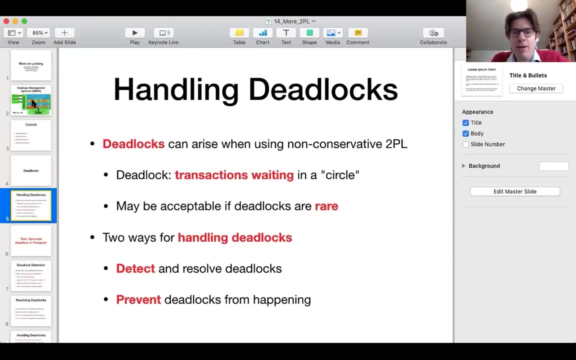 which essentially means that we can acquire locks on different type of objects, such as tables, as well as a single pages from a table. All right, we're going to start a discussion with deadlocks and, as a little reminder, a deadlock is something which arises if multiple transactions are mutually waiting for each other. 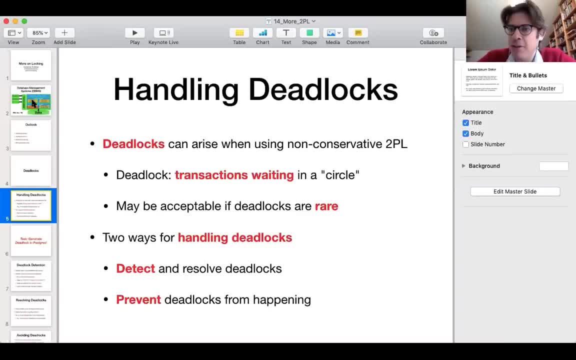 in a cycle. Why are they waiting for each other? Because each transaction is waiting to obtain a lock from the next transaction in this waits for cycle. This can happen only if you use non-conservative two-phase locking. We have discussed multiple locking variants last time. 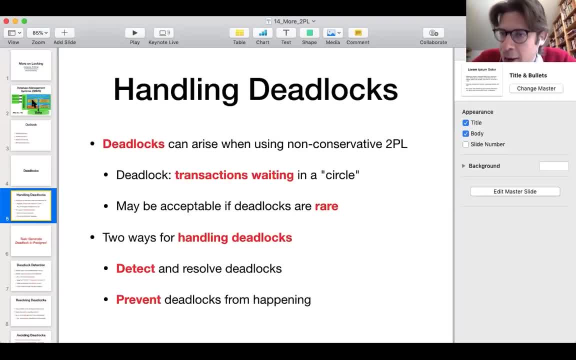 and some of them have a deadlock and some of them have a deadlock. So we're going to start with deadlock. So we have the nice property that they avoid a deadlock. and I believe one of your peers asked the question: if we have a mechanism that avoids deadlocks, why would we ever use something else? 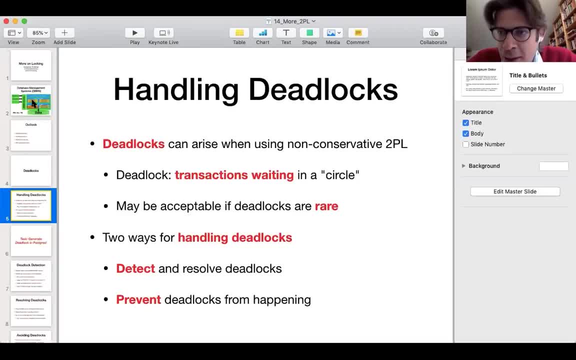 That's a good question. Now, it is true that the deadlocks can lead to problems, and we are about to discuss more about how to address those problems. On the other side, if you choose to accept deadlocks, you often get something nice in return. 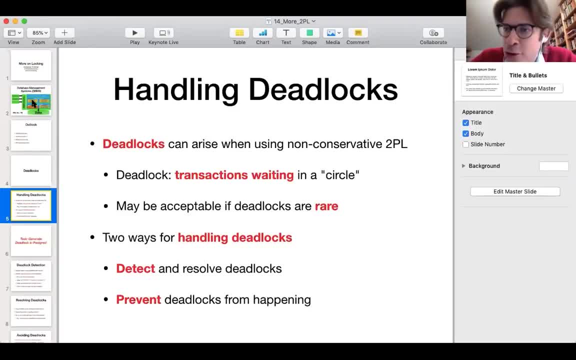 For instance, when comparing conservative and non-conservative two-phase locking, it turns out that a non-conservative two-phase locking allows potentially more transactions to proceed in parallel, and that can increase performance. So there's a trade-off and it depends on the scenario which one of them works best. Now, in the following we're gonna discuss: 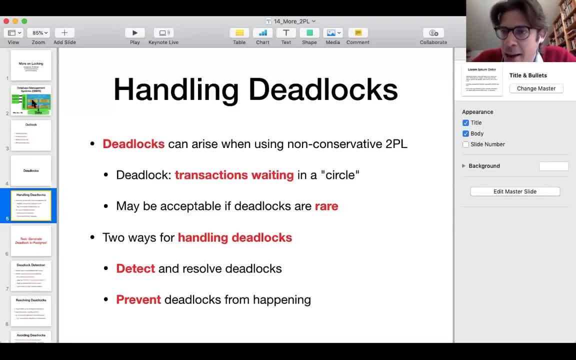 more about how deadlocks are handled, and there is essentially two ways that deadlocks are handled. There are two possibilities. Either you can essentially passively wait for deadlocks to happen. You try to detect them and to resolve them if you encounter them. The other possibility: 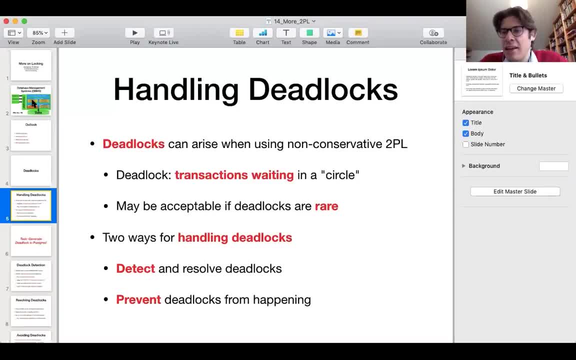 is that you are proactively preventing deadlocks from happening in the first place. One version of that, so to speak, is to use a concurrency control protocol where this is guaranteed not to happen, but in the following way. We're going to see a few alternative methods Now before we continue. first of all, we have been 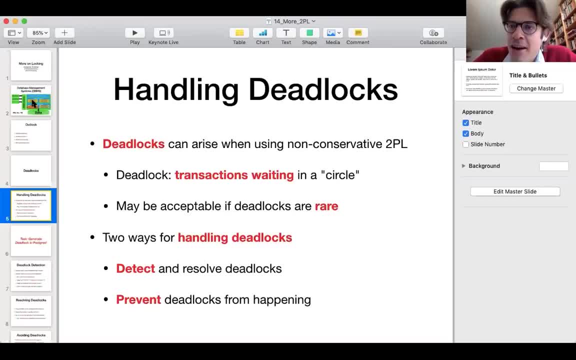 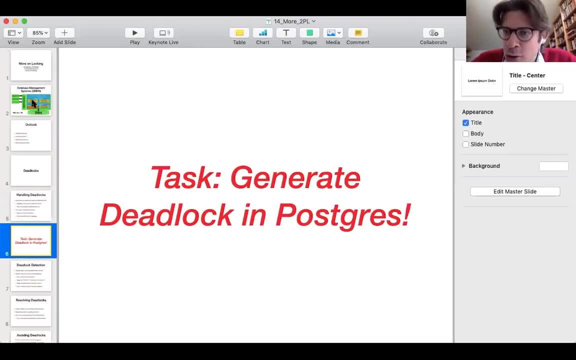 discussing a lot about deadlocks, but maybe many of you haven't experienced a deadlock in practice yet, So I want to encourage you, if you have Postgres installed, to try to generate a deadlock. You don't need to worry, nothing bad is going to happen. The database system will resolve it. but 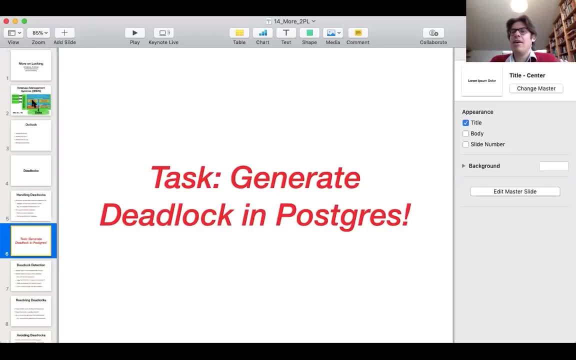 we have seen last time that we can simulate multiple clients connecting to the same database in Postgres simply by opening up two terminals, for instance, and having that try to generate a deadlock in the next couple of minutes. using two transactions is enough. If you don't have Postgres installed, then think about how you would generate a deadlock in Postgres. 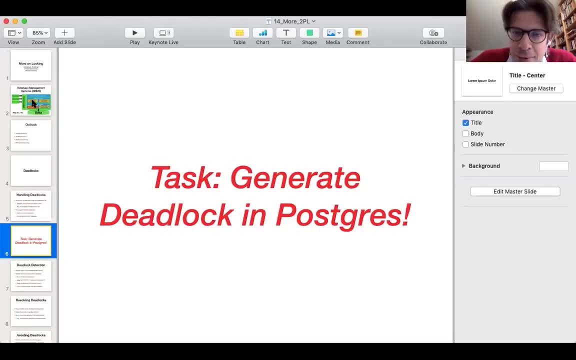 with at most two transactions. Now I give you a little bit- one to a minute of time. You can try to do it or you can just think about how you would do it. If you have any questions about two-phase locking, which is the basis for what we are discussing today, 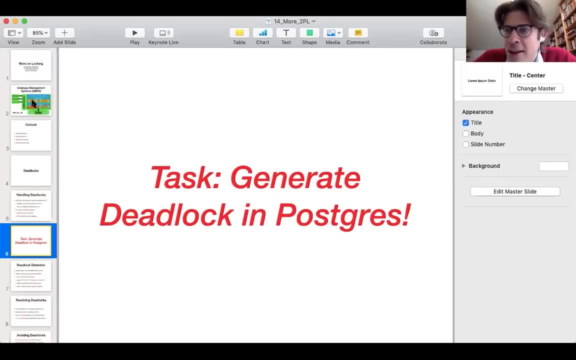 please feel free to ask them in the chat, and after that I'm going to show you on my computer how to realize one of these deadlocks. Please feel free to ask them in the chat, and after that I'm going to show you on my computer how to realize one of these deadlocks. 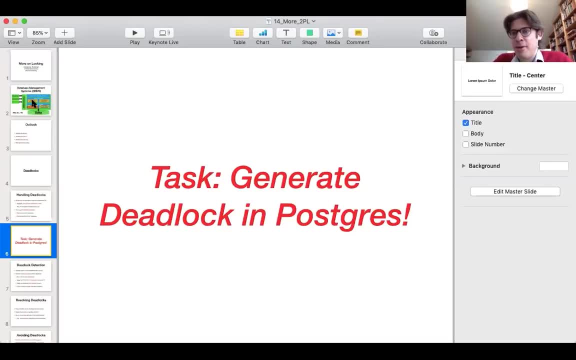 Please feel free to ask them in the chat, and after that I'm going to show you on my computer how to realize one of these deadlocks. Any questions on two-phase locking in the meantime? None, None, No questions on two-phase locking, it seems. 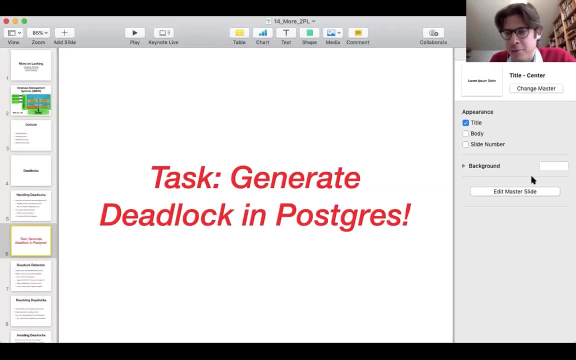 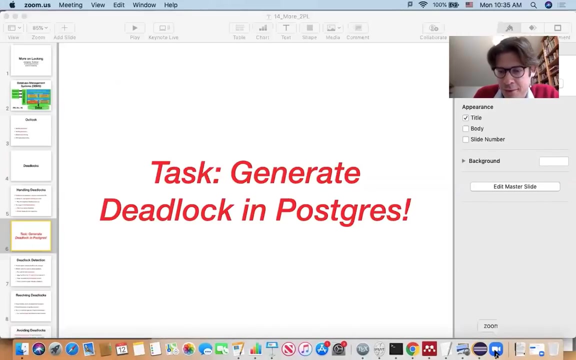 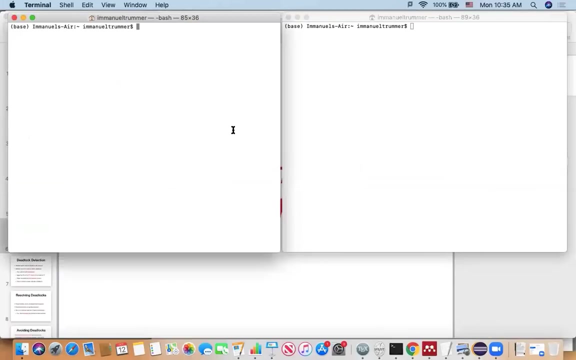 All right, Let's try it together. I'm going to share my entire screen, You know, By closing the chat. All right, So let's see how we generate a deadlock. So last time We have created a little banking database which contained information about the accounts. 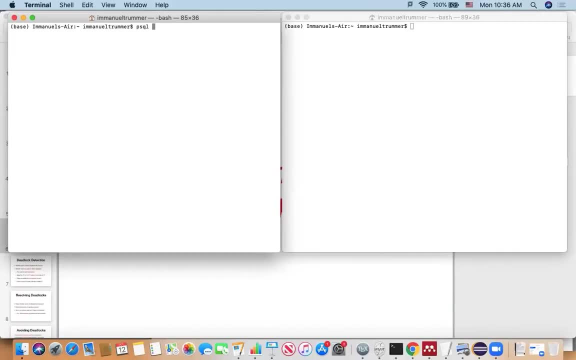 of different customers, together with an amount. Let me log into that banking database here with both terminals. I'm simulating two clients And, as a reminder, we had this accounts table with two columns. The first one is the name of a customer. 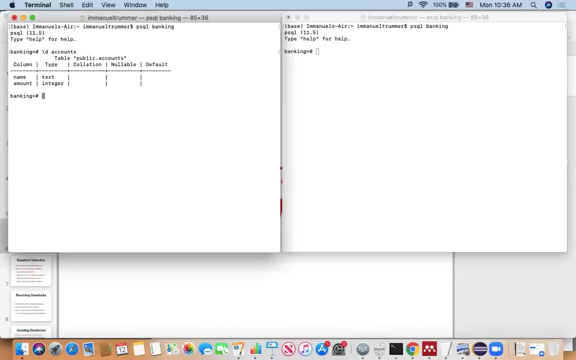 The second one Is the amount on that account. All right, And as you might remember from last time, we are starting transactions with the begin keyword. So here we have started a transaction And we're also going to start a transaction for the other customer. 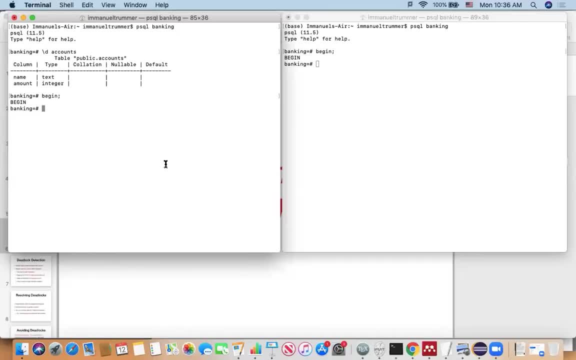 Now in Postgres, locks are associated with rows in a table. In this case, here We have one row For each customer account. So if I want to perform an operation on one of those rows, Then first of all the transaction needs to acquire a lock from the lock manager. 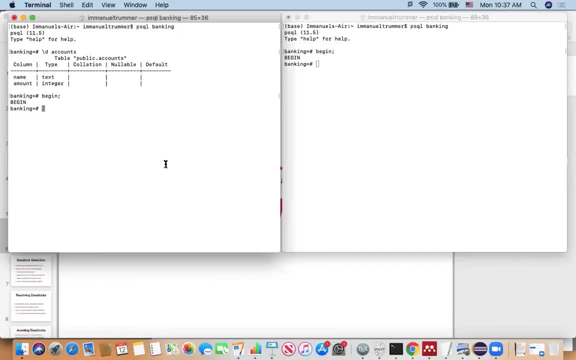 So let's, for instance, say That here we are trying to add $5 to each account. Maybe that's the yearly interest or some other bonus. So let's start with Alice over here And let's say that We update the accounts and we set the amount to the amount, plus $5 where name equals to. 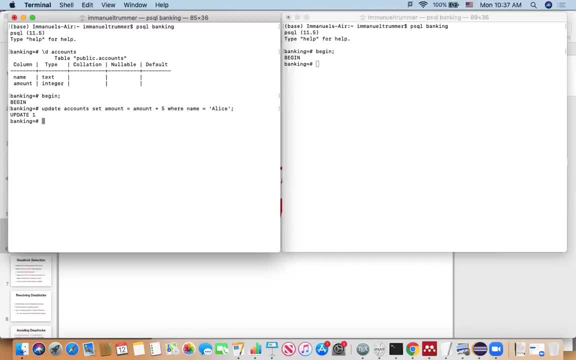 Alice. All right, So we do this operation. It works, Not a problem. So in order to make this happen, the transaction must have acquired the lock for the corresponding row for Alice from the lock manager in the database. Now, on the other side, 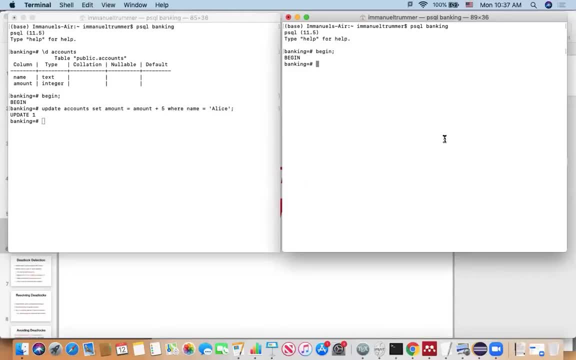 Let's say We actually Added the same thing. We are adding a bonus twice, So here We also update the accounts. We set the amount to $5 more. Here, However, we start not with Alice, But with Bob. 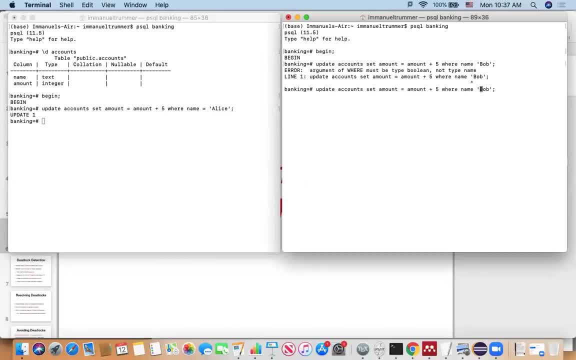 All right, Oops, And here I forgot the equality Sign. And now, since I made a mistake, I actually need to. I forgot the equality Sign. First of all, Let me start this again. All right, Okay, And. 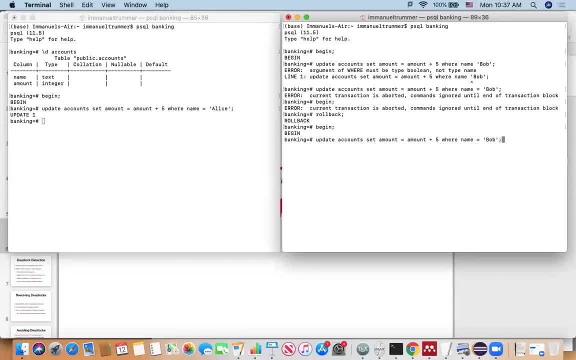 Now We have Made it, We have increased In this transaction. We have Added $5. To the account Of Bob. All right, And In order to make that happen, We have Added $5. To the account. 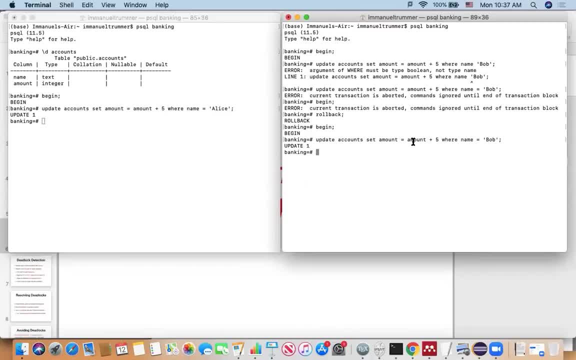 Of Bob. All right, And In order to make that happen, We have Added $5. To the account Of Bob. And in order to make that happen, This transaction Over here Must have Acquired A lock. 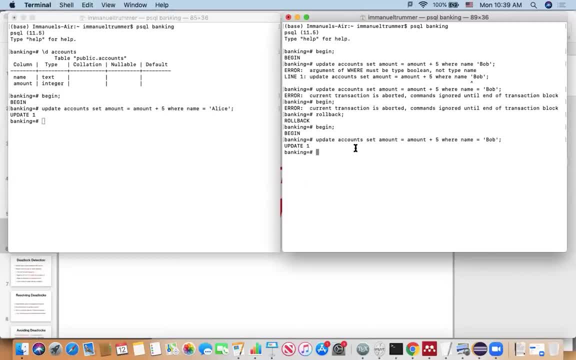 For the role That represents the account Of Bob. So now The Transaction In the left terminal Holds A lock On the Alice role And the transaction In the Right Screen Holds A lock. 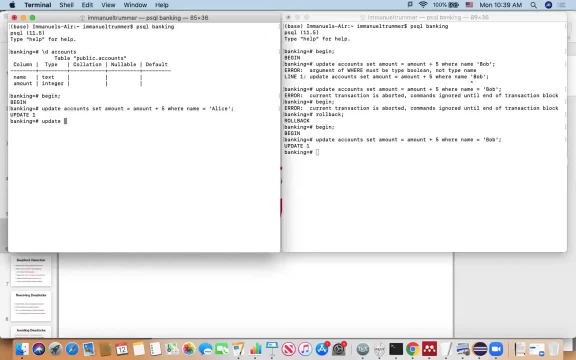 On the Bob Roll. So I have to speed it up a bit, Because otherwise You might Have to Do Something Here. It's not going to work, So Let's Say That Now, Here. 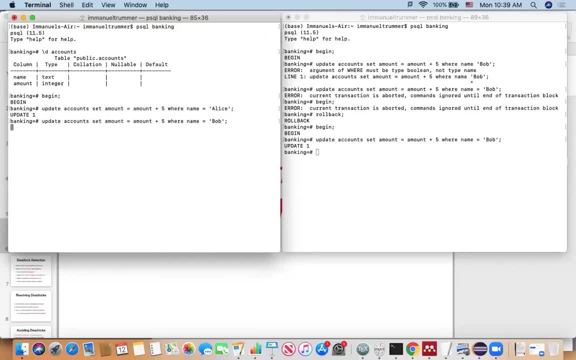 In the Left Terminal. Now I want to Increase The amount For Bob. All right, And What happens Here? You See That With The previous Command, The, and it doesn't immediately execute the command. the reason is that here i want to access the row of. 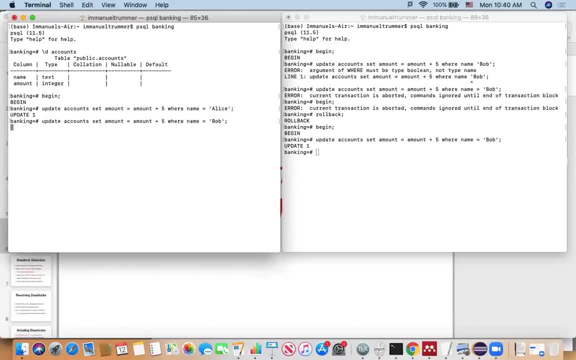 bob. so in order to do that, the transaction first of all needs the lock on the bob row, and that block is currently not available because the transaction on the right hand side of the screen is still running and that transaction is currently holding on to the lock on the bob row. so now i 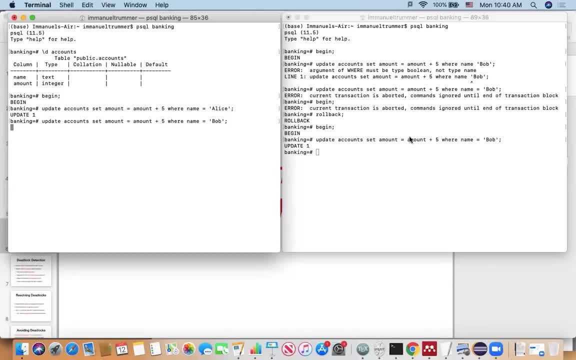 have two like one transaction waiting for another one. the transaction on the left terminal is waiting for the transaction in the right terminal. in order to create a deadlock, i need to close the cycle and make the transaction on the right hand side wait for the one on the left hand side, as 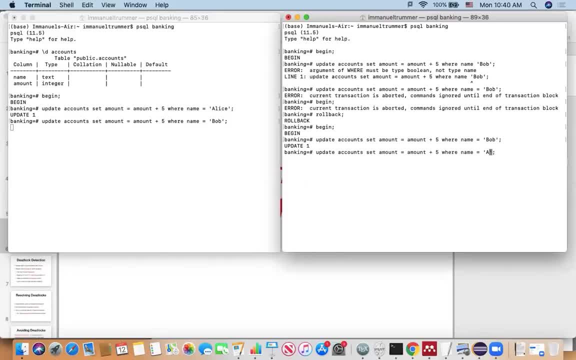 well, so let's actually accomplish this by trying to update the account of alice here on the right hand side. in order to do that, the transaction would need the lock for the alice row, but that block is currently held by the transaction on the left hand side, and so by doing this, we should create a deadlock. all right, and as you see here, 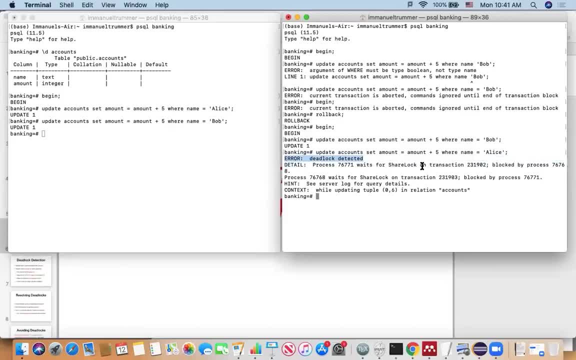 this is what happens. we get the error deadlock detected. so here we have a deadlock. indeed, any transactions in the database system detects that and it resolves the deadlock by aborting one of those transactions. and, as you can see here, the transaction on the right hand side is aborted. on the other side, the transaction on the 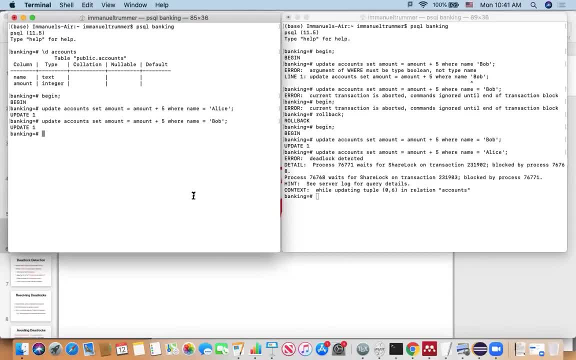 left hand side of the screen. this one has finally produced the output saying yes, we have updated the account of bob because, as the transaction on the right hand side has aborted, it also must release all of its locks so they become available. and finally, the transaction on the left hand side. 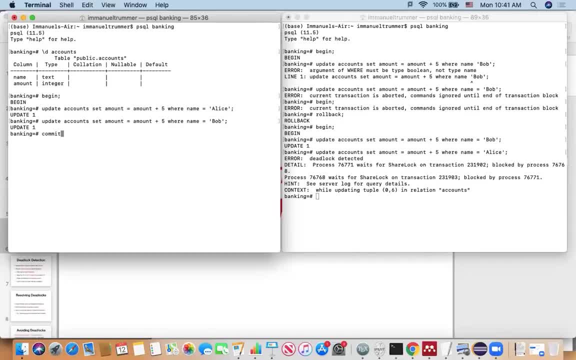 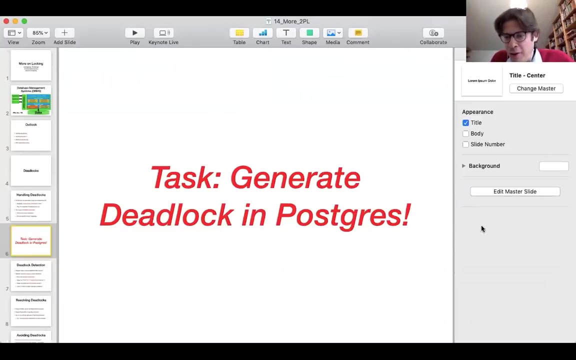 can acquire the lock for bob. and now we have done that and we have successfully updated the database, and here we have created a deadlock. it was resolved by aborting one of the transactions, all right. all right, let me quickly check where there's questions in the chat. 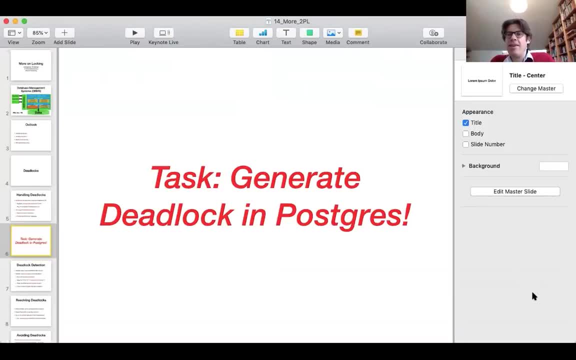 all right, and here a great question about how we make sure that locks are released, for instance, on the pop row. so, um, in general, those locks are released automatically in the background once the transaction finishes. it depends actually on the specific variant of two-phase locking when blocks are released precisely. uh often in practice we use uh two-phase locking. 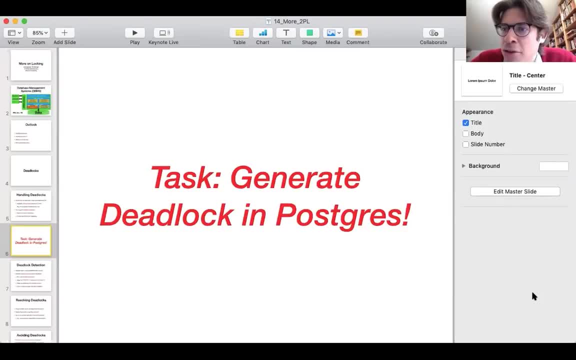 and we use the two-phase locking as a way to make sure that the two-phase locking is actually a strict two-phase docking, and then the locks are released once the transaction has finished executing at the very end. and okay, that's another great question. so, in this a case, how many updates have actually? 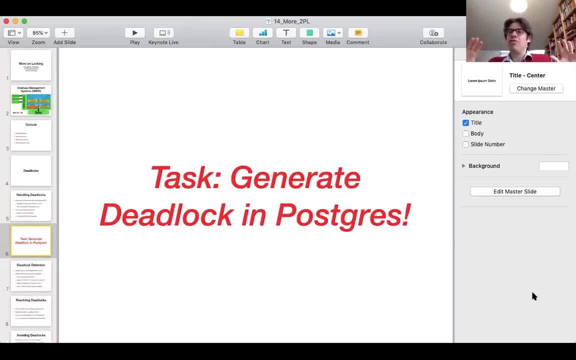 executed. okay, great question, all right. so we had two transactions that were in a deadlock with each other, so they were mutually waiting for each other and nobody was able to make the progress. now the database system typically resolves those stat logs by porting only one of those transactions that are waiting for each other, so we want to avoid aborting transactions, if you. 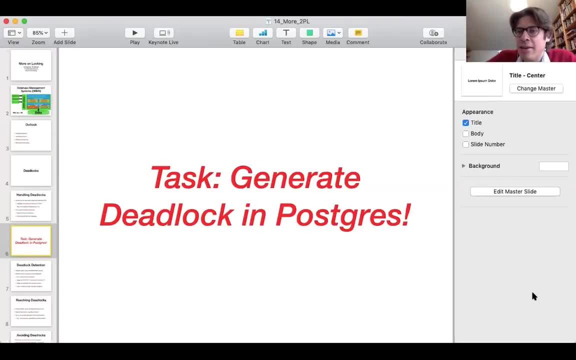 don't have to so. in order to break the cycle, it is typically sufficient to abort only one transaction within that cycle and in this case, a postgres decided to abort the transaction on the right hand side of the screen which had, which was trying to do, two updates, but those updates they have not happened because the 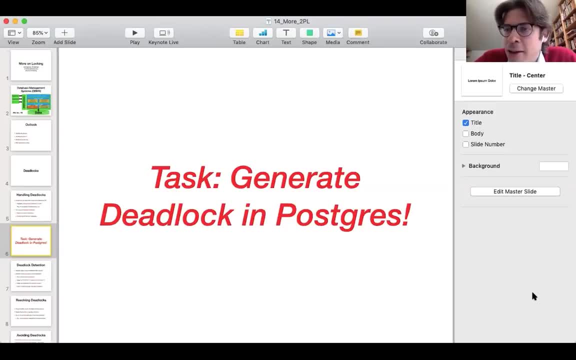 transactions was aborted and all its effects were rolled back. the transaction on the left screen was able to proceed after aborting the other transaction because by aborting the other transaction its locks become available. so the transaction on the left hand side has succeeded and has executed it actually and eventually gets back to the working state. stared. uh, just two updates, very good questions, all right. so now you should see my slides again, then actually check with. uh, okay, this, you're getting a little error message. okay, so let's continue without presentation mode, all right. so now we have seen how to reset and how they are automatically resolved. now a�rian wird die ein Hoover seg胡 ignoriert. 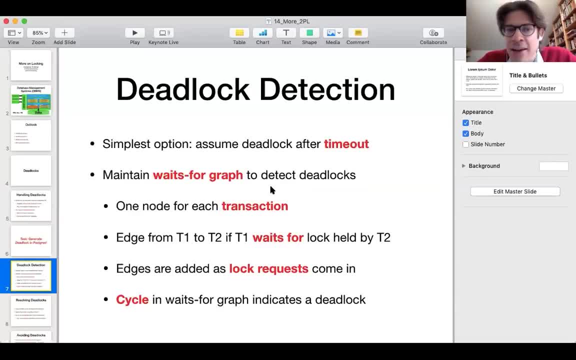 und teria eine, die gzek Bayerum 추 CF d markeden. nun am, in vorwürfe von rails können wir auf den nlaceoring gestehen, aber Here is an annual war profilenfülliges Ge mistress. what Postgres is doing internally is a deadlock detection. So typically, we try to detect deadlocks. 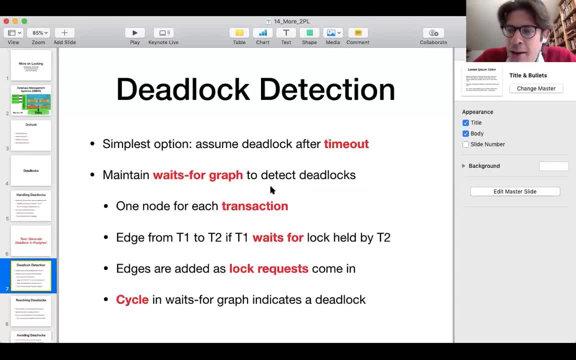 by creating a so-called Waits For graph. The Waits For graph is sometimes confused with the conflict graph, because in both cases the nodes are transactions, But the semantics of the edges differs, because in the Waits For graph you have an edge from one node to another one if the first 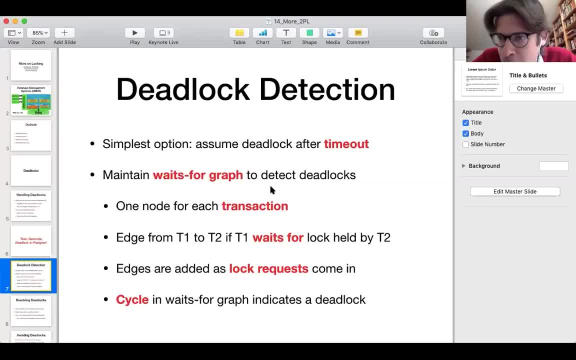 transaction is waiting for a lock by the second transaction. So the lock manager keeps track of this Waits For graph. whenever a transaction requests a lock, then that is not immediately available. Then we draw a cycle and then we draw an edge within the conflict graph and periodically. 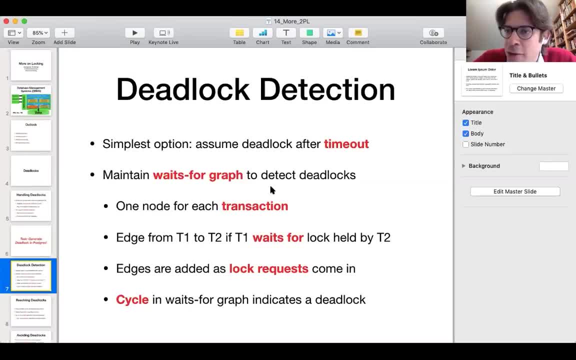 we check for a cycle. So if we have cycles in the Waits For graph, if you have a cycle, it means we have a deadlock and we need to take care of that. That is one of the standard methods to detect the deadlocks, Perhaps one of the simplest methods. 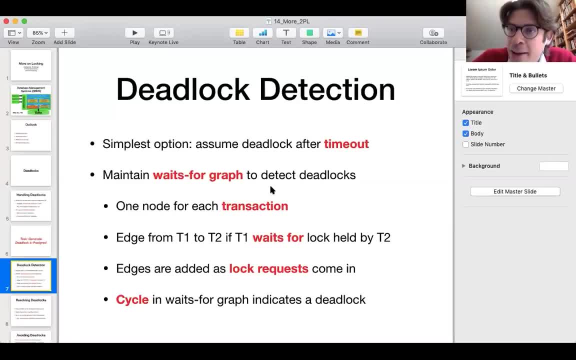 is to simply say that we assume there has been a deadlock if a transaction cannot make any progress within a given amount of time. However, of course, here it becomes difficult to choose an appropriate timeout. Maybe the transaction can't make progress within a given amount of time, However, of course, here becomes difficult to choose an appropriate timeout. maybe the transaction may have to wait for the deadlock. 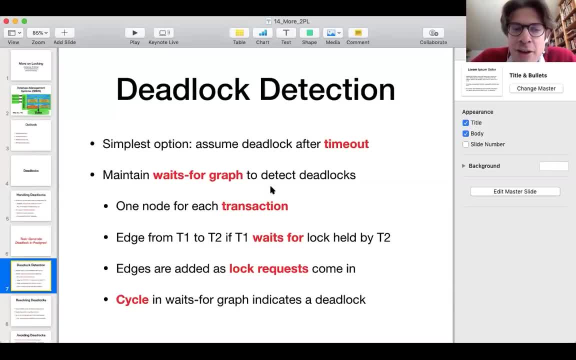 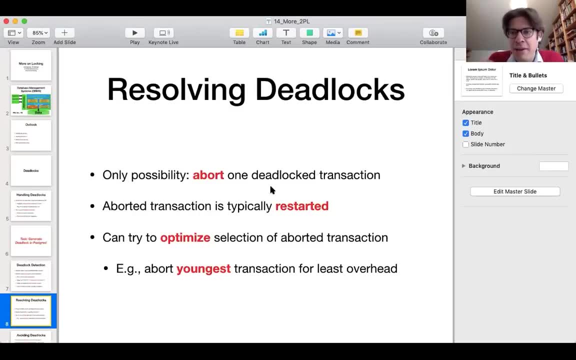 is not deadlocked, but just a little bit slow for the moment. So the method with the waits for graph is more reliable. If we have detected a deadlock, the database system tries to abort one of the transactions within the cycle. You have already seen this in practice here in Postgres. 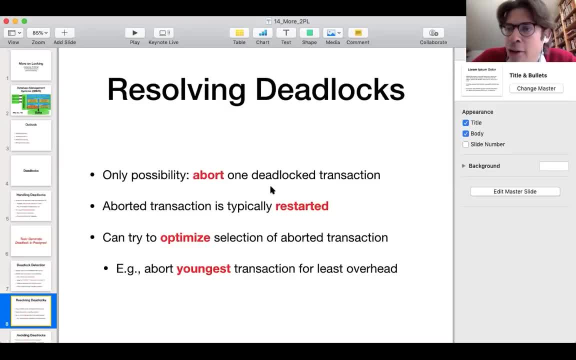 We automatically had one of the deadlock transactions aborted. Now, depending on the settings, the aborted transaction might be restarted. Here that was not the case. You can also try to optimize the selection of which transaction to abort, because if you have a cycle, 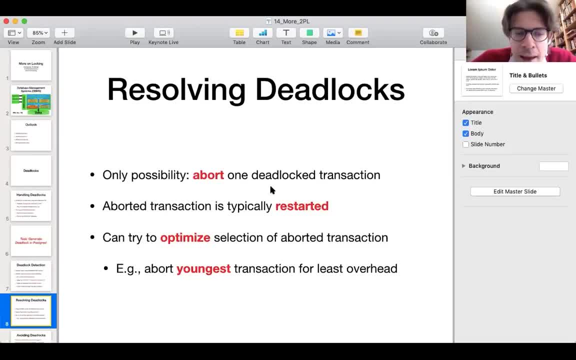 you might have multiple possibilities to break the cycle And there's a couple of heuristics the database systems use. For instance, you might say that the youngest transaction that has started most recently It has done perhaps the least amount of work. So by aborting that transaction we 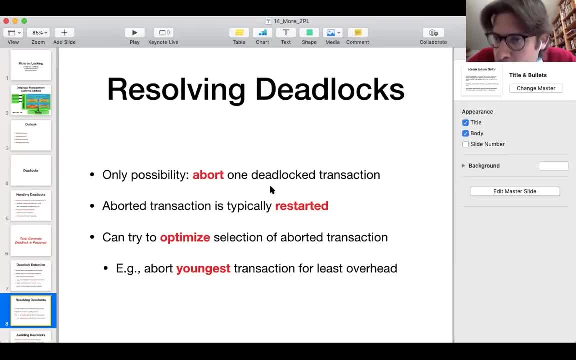 lose the fewest number of operations, which might be good for performance. So here the high-level idea is: we detect, we look out for deadlocks and if we encounter them, we resolve them by aborting transactions. The other possibility is that we proactively avoid a deadlock. 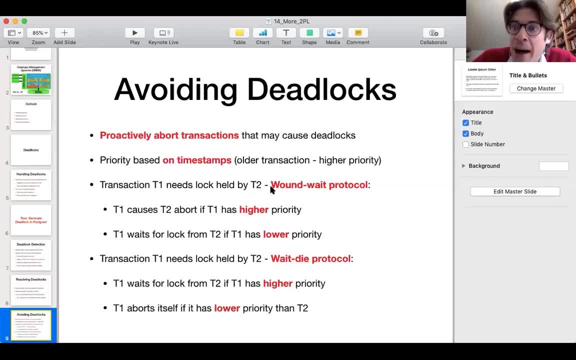 And we proactively abort transactions that might cause a deadlock. So that is a little bit more careful, because I am aborting transactions even if I don't have a deadlock yet. On the other side it can save overheads for deadlock detection, for instance. 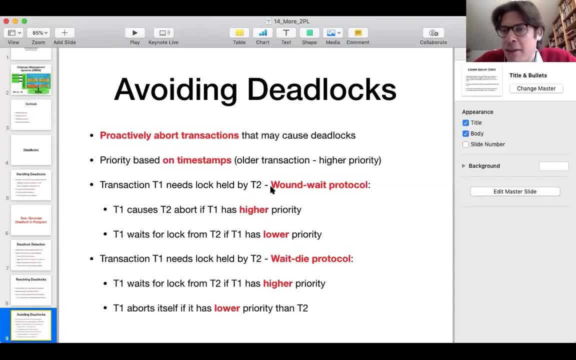 So again, you cannot say which of those methods is better. It always depends on the particularities of the scenario. Now, the strategies that we will see for avoiding deadlocks are based on transaction timestamps, So if transactions come into the system, they get assigned a timestamp. 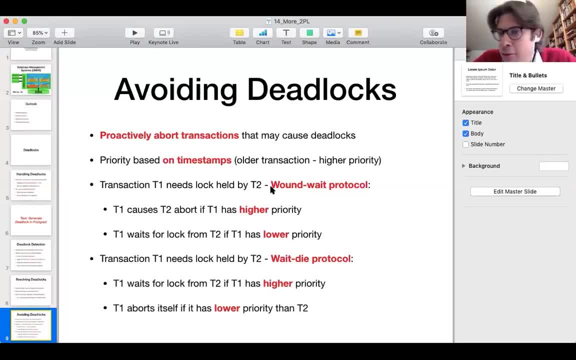 And we say that older transactions that run for longer they have higher priority. Now in the following, we're going to see two very popular deadlock avoidance protocols. The first one is called Wound Wait and the second one is called Wait, Die. 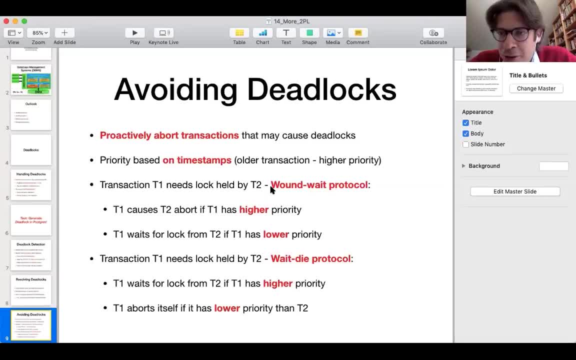 Now, in this naming of the protocols, the first part of the protocol name essentially tells you what happens if a higher priority transaction wants a lock held by a lower priority transaction. The second part of it tells you what happens if a lower priority transaction is waiting for a lock. 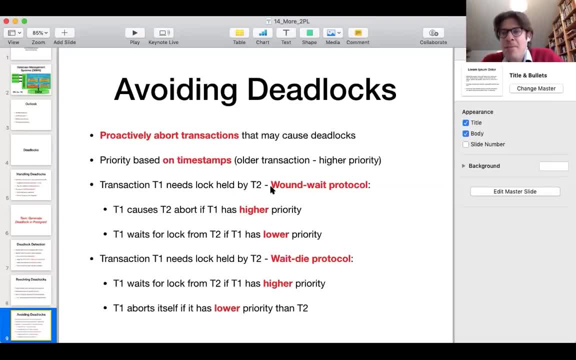 by a higher priority transaction, all right. So, for instance, in the first case- wound weight- we have a transaction T1 that needs a lock, which is helped by T2. Then T1,, so to speak, wounds or aborts the second transaction, if T1 has a higher priority. 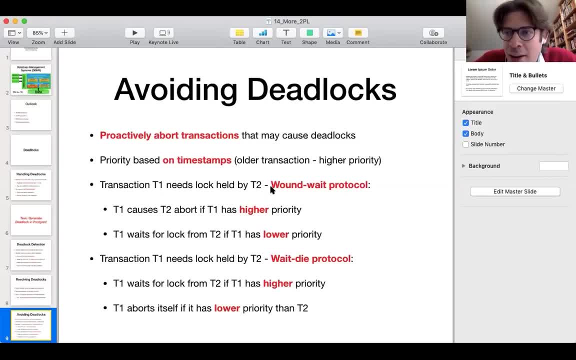 than the transaction which is currently holding the lock. So the higher priority transaction essentially goes ahead and grabs the lock and aborts the other transactions in the process. In the second case, if a lower priority transaction wants a lock that is currently held by a higher priority transaction, 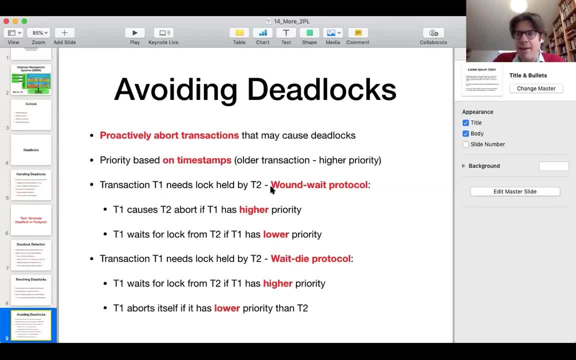 then the lower priority transaction politely waits until the lock becomes available. So the wait-die protocol works differently. So here, if a higher priority transaction wants a lock held by a lower priority transaction, then the higher priority transaction is allowed to wait until the lock becomes available. 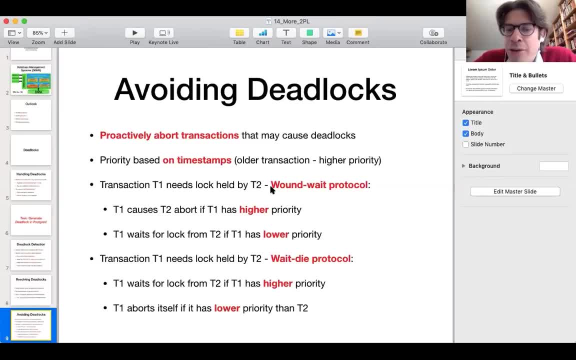 On the other side, if a lower priority transaction wants a lock held by a higher priority transaction, then the lower priority transaction is proactively aborted. So it's not allowed to wait until the lock becomes available. So those are the two possibilities And we're gonna see in more detail in the following. 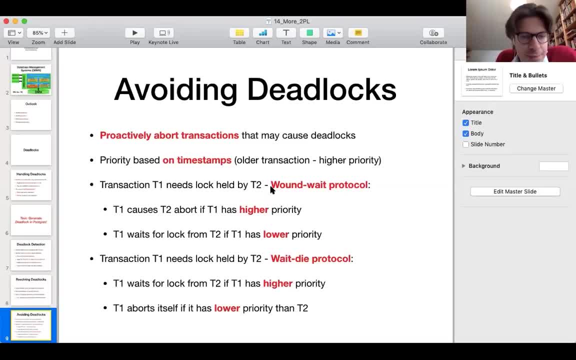 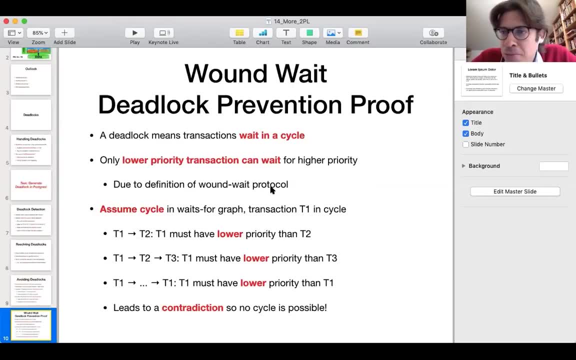 how they make sure that no deadlocks can happen. Here we start by analyzing the wound weight protocol and we justify why we cannot wait. We cannot get any deadlocks when applying this protocol. A deadlock always means that transactions are mutually waiting for each other in a cycle. 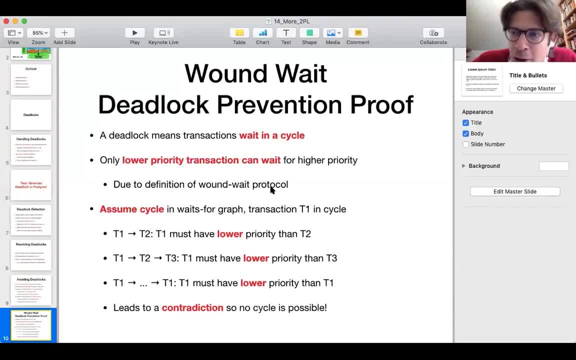 And, as I mentioned in those protocol names, the first part always says what happens if a higher priority transaction wants the lock of a lower priority transaction. The second part says what happens if a lower priority wants a lock from a higher priority transaction And we assume that the timestamps that those priorities 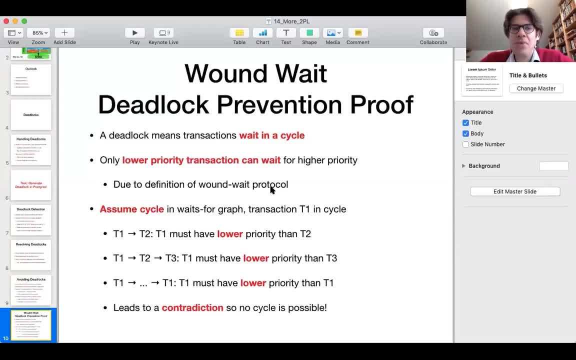 are based upon are unique. All right, So, which means that if you compare two transactions, then one of them would be higher priority, The other one will be lower priority, So there's only two possible comparisons. All right, So with the wound weight protocol. It only has one weight in the name. That means that transactions can only wait in one order of priority, so to speak. We have the weight as the second component, so only lower priority transactions can wait for higher priority transactions, but not the other way around. 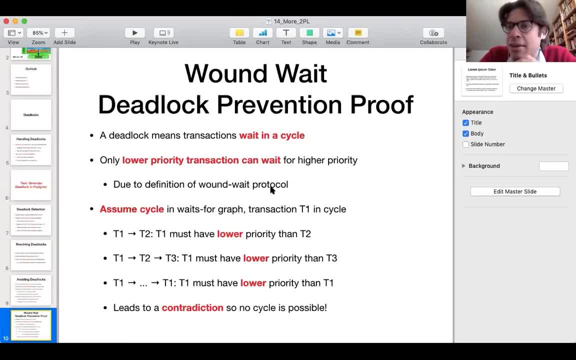 All right. And if we now assume that we had a cycle in the weights-for graph, each edge means that one transaction is waiting for the other one, So you always must have a lower priority transaction connected and waiting for a higher priority transaction. So if you have a path in the weights-for graph with the wound weight protocol, it means that 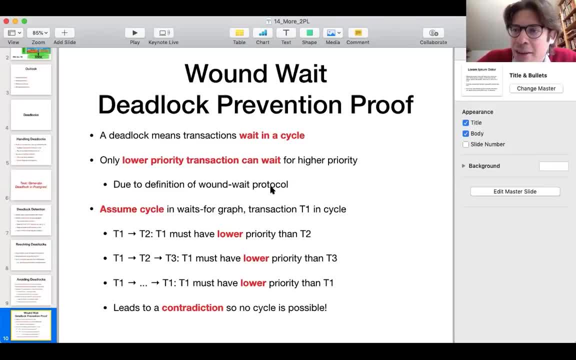 the first transaction in that path has a strictly lower priority transaction And that means if you have a cycle closing the path, then there must be a transaction that has a lower priority than itself, And that cannot be. This is why you cannot get any dead dogs when applying the wound weight protocol. 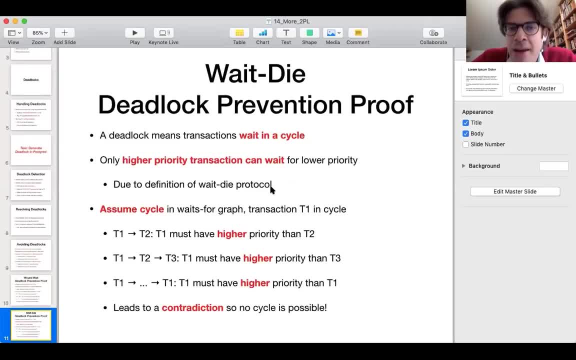 The reasoning for the weight die protocol is similar. Here it's the inverse. You also have only one weight action And this appears as the first component. That means that higher priority transactions can wait for lower priority transactions, And that means again that if you have a path from one transaction to another one in 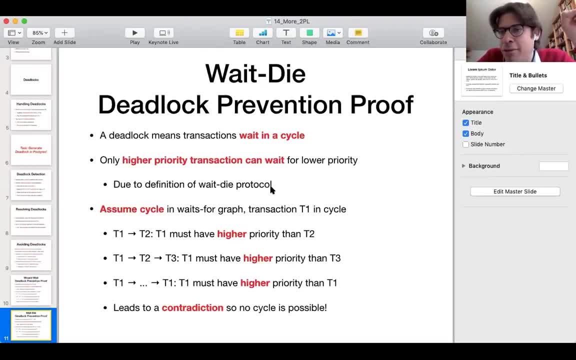 the weights-for graph, then the first transaction on that path must have a strictly higher priority than the last transaction on that path. Now we are closing the path into a cycle. That means that there must be a transaction which has a higher priority than itself. 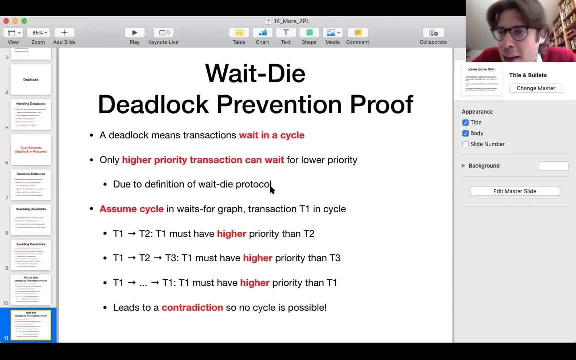 And that obviously cannot be again. So we have shown again that we cannot have a cycle in the weights-for graph with the weight die protocol. So those are those dead log avoidance strategies which allow you to skip tracing the weights-for graph, because you know that if you apply those protocols you are safe from dead logs. 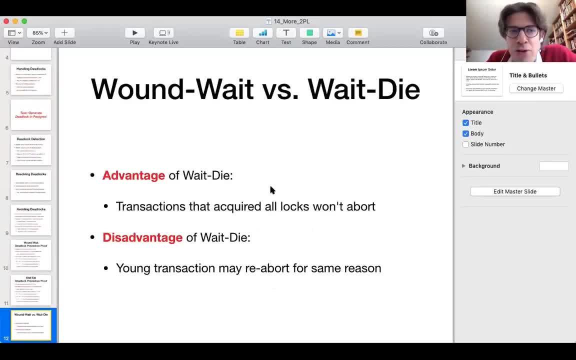 So if we compare those two different protocols, we'll know that the dead log avoidance is safe. So if we compare those two different protocols, we'll know that the dead log avoidance is safe. All right, All right. And for next, V8 and V8-die. it again depends a lot on the scenario which of them works. 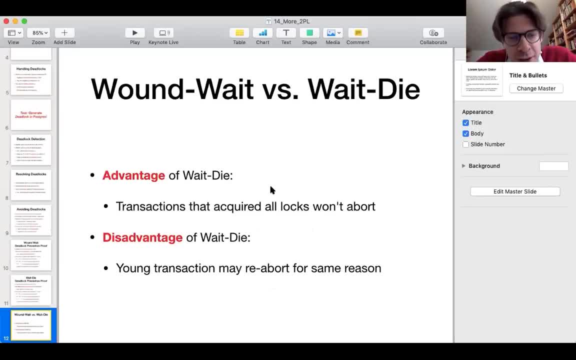 best Advantages that are often cited for the V8-die protocol, for instance, include that a transaction which has all the logs that it needs in order to proceed with execution, it will never get aborted. You don't have any wound operations where another transaction gets aborted because the 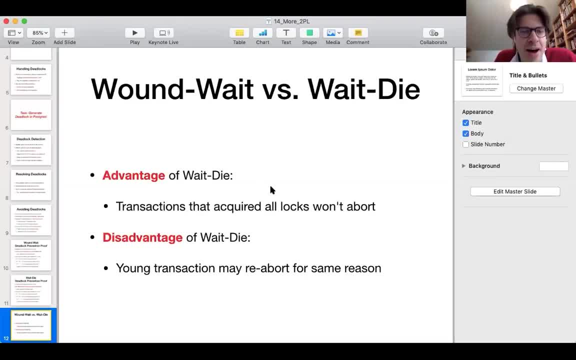 first transaction won't work. All right, Thanks, Thanks, Thanks, Thanks, Thanks to acquire a lock. A disadvantage of they die is that you might have young, low priority transactions that try to acquire the same locks multiple times once they get restarted and they get. 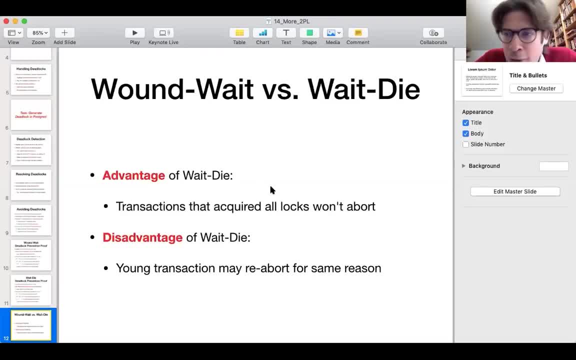 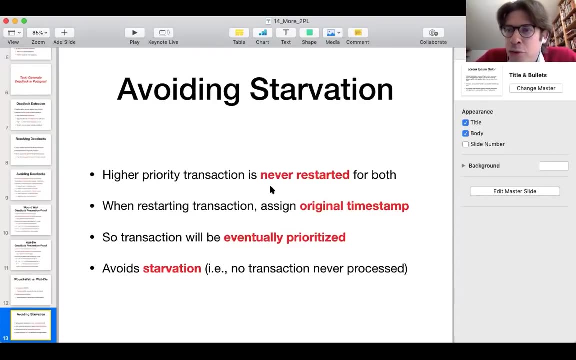 aborted multiple times for the same reasons, which is inefficient. but again, which of those protocols works best? that really depends on the particularities of the scenario. One little detail you have to consider when implementing this: you want to avoid starvation, so you want to enable each transaction to eventually proceed, which might mean that we 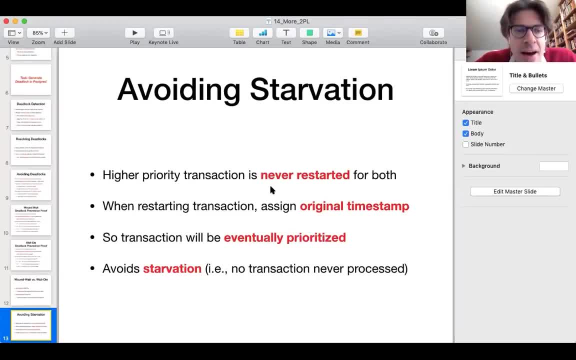 restart it after it was aborted. Both of those deadlock avoidance protocols have the property that the higher priority transactions. they are never aborted and restarted. So in order to make sure that a transaction eventually processes, we have to make sure that it gets a higher and higher priority as time progresses. So if we restart a transaction, 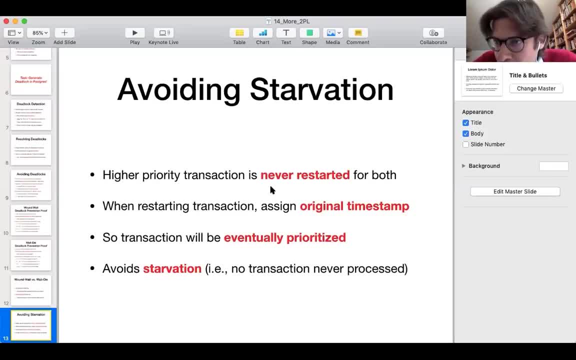 we don't want to give it a new, younger timestamp, because that would mean it has lower priority. Instead, we want to restart it with the same timestamp that it had when it originally entered the system. That means that over time the priority of a transaction will grow and eventually it must get processed. 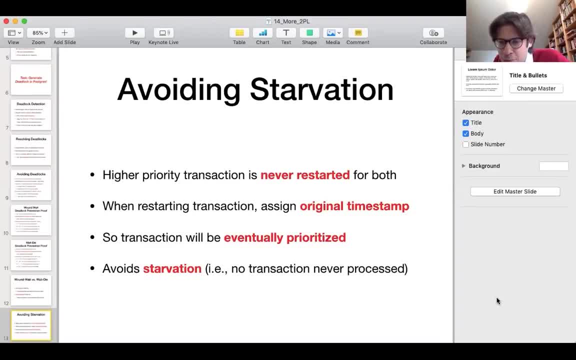 And there's a question on the wound weight protocol: How can T2 abort if T1 has higher priority? And that requires a lot of time. So the point in time at which transactions are requesting locks might not necessarily be aligned with the time at which those transactions start. 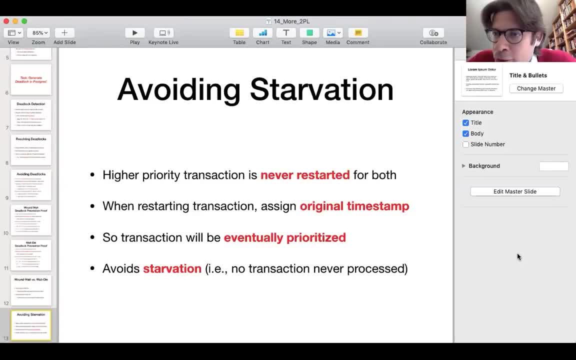 If transactions acquire all their locks at the very beginning of transaction start, then we have conservative two-phase docking and in that case deadlocks cannot occur from the the from the beginning. So here we have a non conservative two phase docking. So transactions might, even if one transaction- 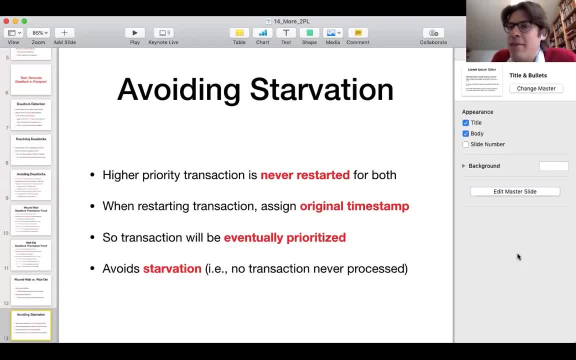 starts after another one, it might still be the first one to acquire the lock on one specific object, because they don't need to acquire all their locks at the beginning of transaction execution. All right, So this is deadlock avoidance protocols And in general, you have always those two possibilities: either you. 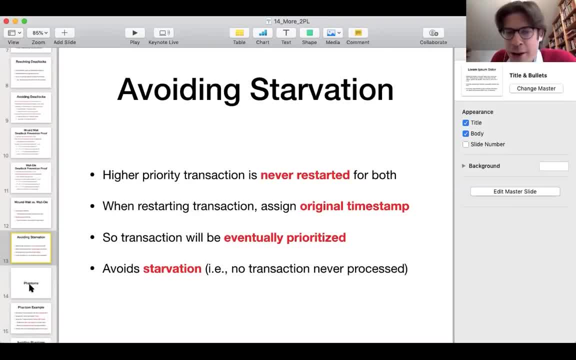 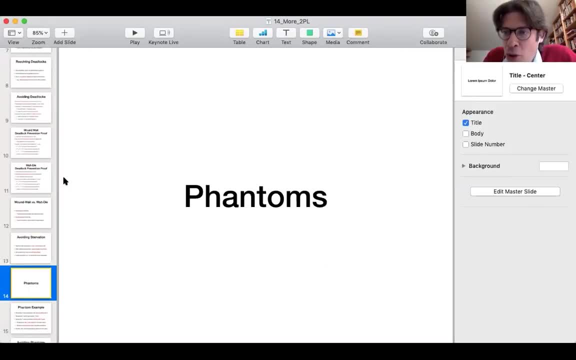 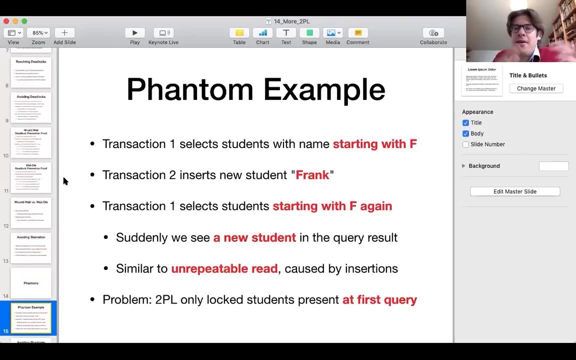 detect that box and react, or you avoid them by using one of those protocols. Now, next, we're going to discuss about an anomaly that I had quickly mentioned at the beginning, which are those so called phantoms. A phantom arises, for instance, in the following: 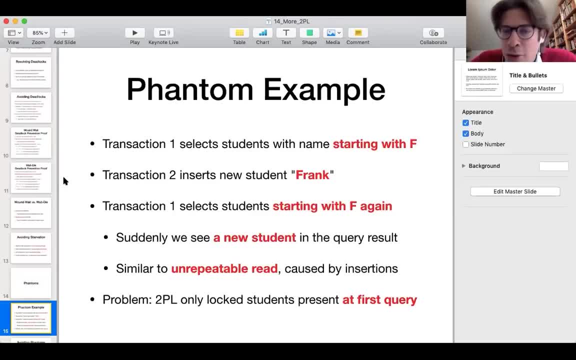 example. So let's say that a transaction selects all the students with a name starting with F. Now transaction two inserts a new student called Frank, And after that, transaction one again selects all the students starting with F. Now, from the perspective of that first transaction, it's: 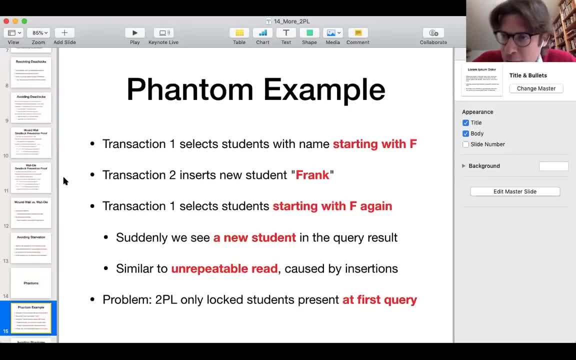 supposed to be the first transaction. Now, from the perspective of that second transaction, it's supposed to be the first transaction, But the phantom suddenly sees a new student named Frank appearing in the result set. So this is kind of a variant of the unrepeatable read, Just that in this case. 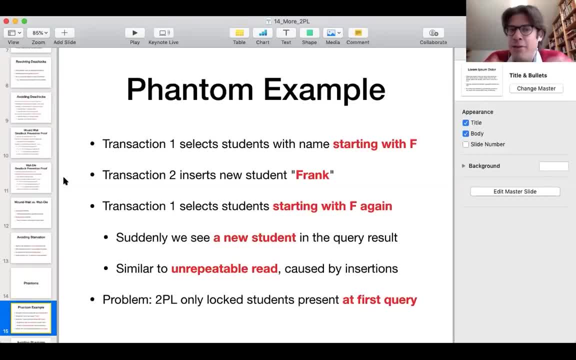 it connects to an insertion. The phantom is characterized by the fact that somebody inserted a new object in the database And it suddenly appears, if you run query, a query with the same predicates at 12.. All right, Now, if you use naive two phase locking, then you are. 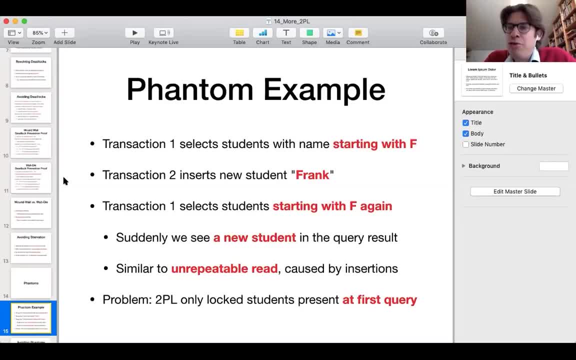 not safe from the problem Because two phase locking a purely only locks the objects that are currently in the database. So if somebody had tried to change one of the existing students that start with F, then two phase docking would have prevented that from happening. On the other side it 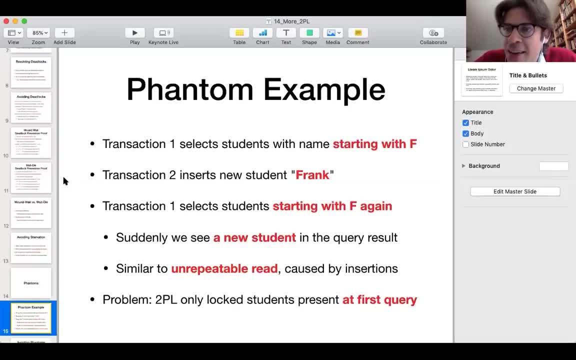 didn't prevent us from inserting a new object. So we are inserting a new student into the database because the lock for that object did not exist. then we acquired the locks at the first query of the first transaction. Now, what we want to do here is essentially to lock all the 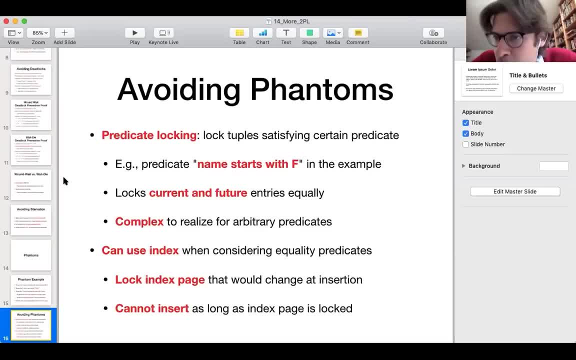 tuppers or the students in database that satisfy a certain predicate. Here the predicate is: name starts with F. So we don't only want to lock all the rows with the property which are currently in the database. Instead, we want to also lock all future entries with that property. So we 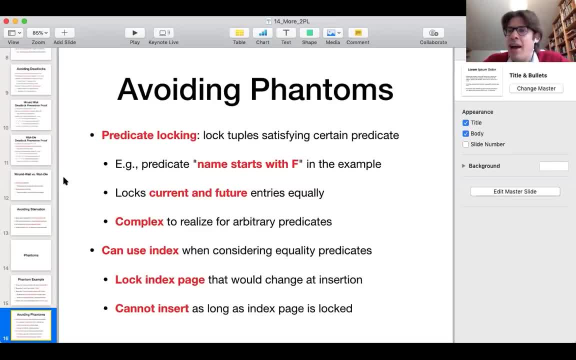 essentially proactively want to lock entries which have that property name, starting with F, but are currently not yet in the database. That is generally called predicate locking, because we don't lock a specific object but we lock everything that satisfies a certain predicate. predicate docking can be. 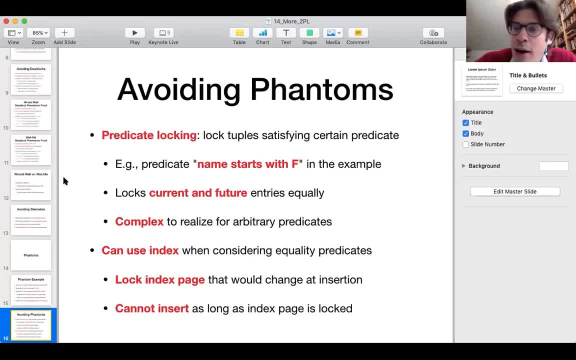 extremely complex, depending on which class of predicates you are considering. considering arbitrary predicates that can get extremely expensive, almost impossible to implement. So typically people focus on a reasonably simple cases. Now, if you have a student who has a predicate, that is not a range. 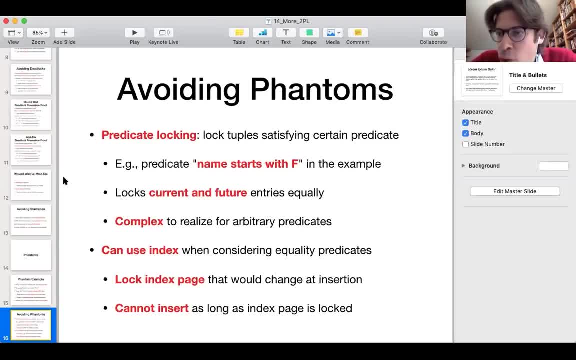 then you have to have a predicate, that is, a range predicate. Now, one common case is that the focus, for instance, on equality or on range predicates named starting with F. that would essentially be an example of a range predicate, And in those 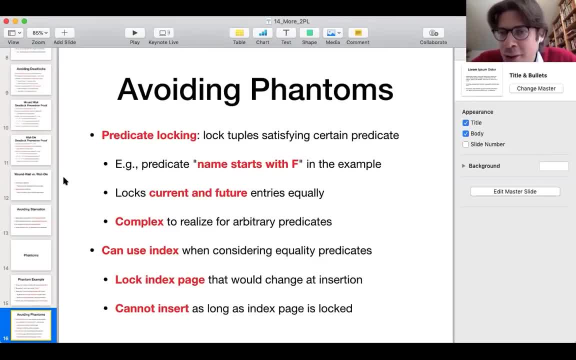 cases, if we have an index on the corresponding table, we have the students, for instance. if we had an index with the student name as an index search key, Then we know that after each insertion we need to update the index as well. So an efficient way in which people often 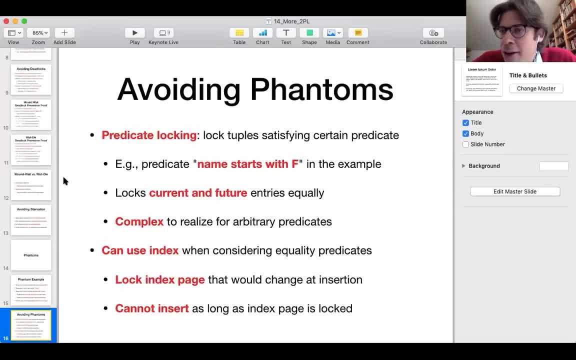 realize predicate locking is by not directly locking the table but rather locking an index which refers to the table and has the right index search key. So if we identify for the index the index leaf page, for instance, on which students with F would have to be inserted, if we lock 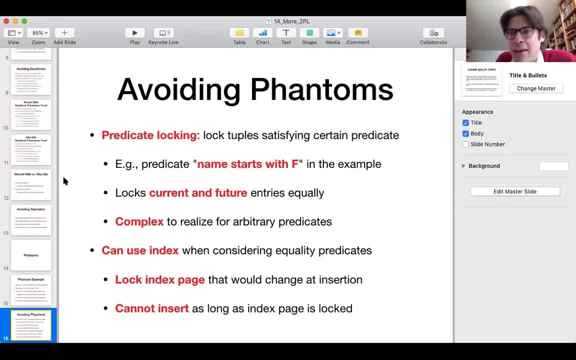 that page. it is as good as if we had locked the original data, because the second transaction cannot proceed with inserting students with F unless it also is able to acquire the lock of the associated index. And if the first transaction holds the lock on that index, it implicitly means that the second 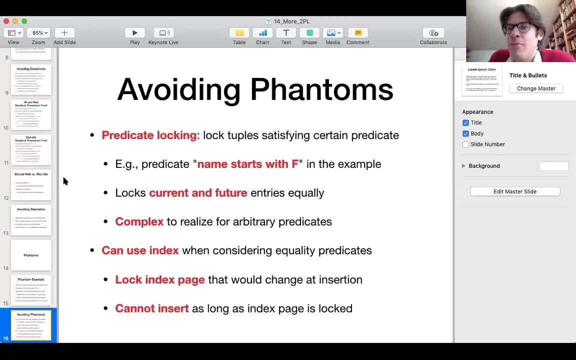 transaction cannot proceed inserting students with F Because it has to wait until the associated lock on the index becomes available again. And that is a great question. The question is, at which point in time does predicate locking actually acquire the locks? And if we use an index for predicate locking then we would acquire 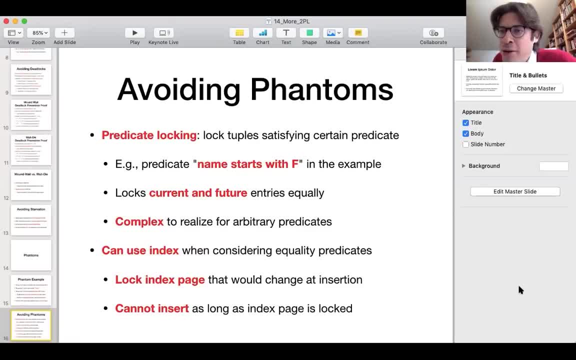 the lock on the index as soon as transaction number one. but I checked for students with starting with F for the first time. So essentially if we have predicate locking then we prevent insertions from happening. So we will not insert the corresponding objects into the database at all. And one. 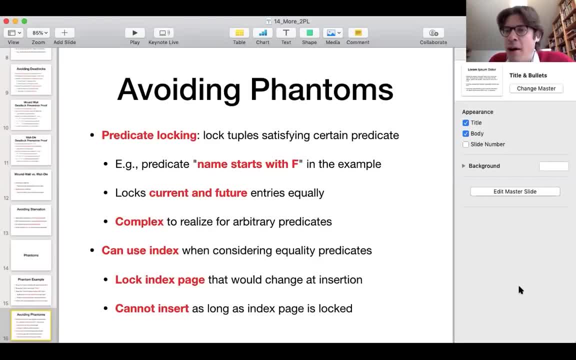 common way is to do this with indexing, and then you acquire a lock on the corresponding index pages. Now, in order to realize predicate locking, we can use indexes More generally. we all often have indexes associated with tables, and the question is: how do we? 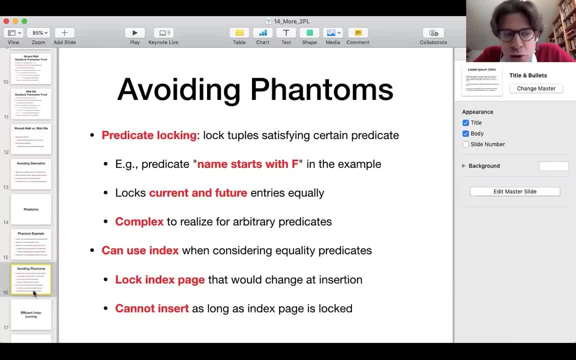 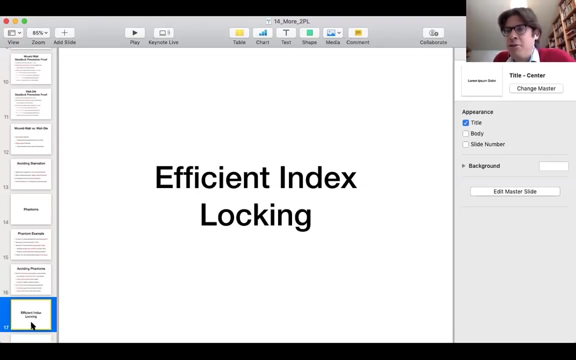 treat indexes in the locking protocol. So in the following we're going to discuss about efficient locking for indexes, which helps us when implementing predicate locking with indexes, but which also helps us in general in order to process data faster, which has some indexes created over it. All right, So first of all, a little question. So in the end, an index. 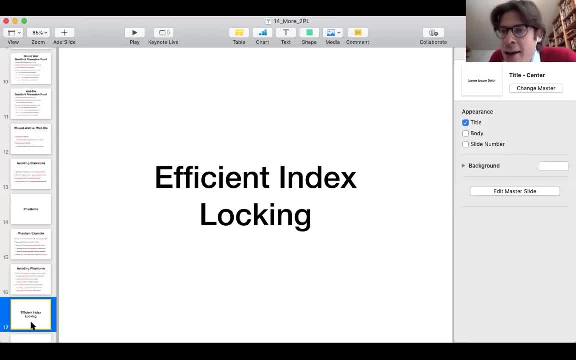 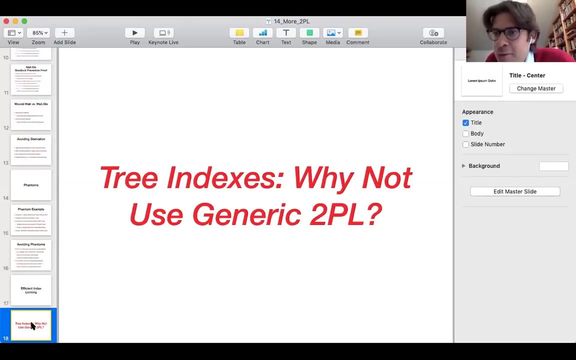 it's just a collection of data pages And we have seen two-phase locking which works for data in general. So in principle, we could use two-phase locking as usual and apply it in order to lock different data, different pages in my indexes. The question is: why is doing that not efficient? Can anyone write? 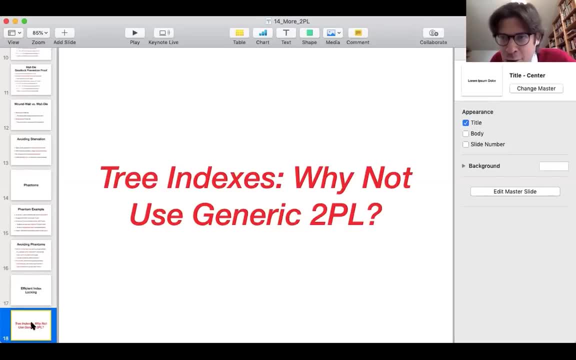 into the chat the reason why you do not want to use generic two-phase locking on index data structures. OK, So do the powerNav goes to that expression in mind. outstanding: If you think about specific access patterns for indexes, is there anything that comes to mind? 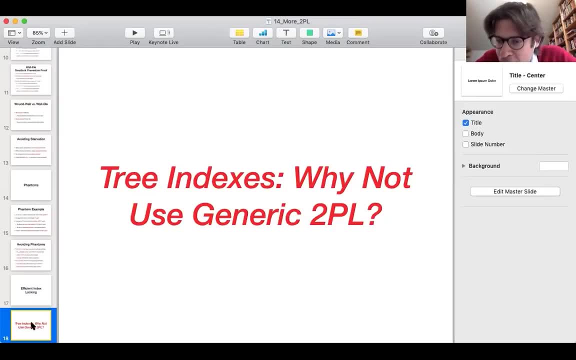 exactly so. the high-level point here is that if we use generic two-phase locking in order to lock pages of an index, then things become more sequential indexes. they used a frequent view and even more, even worse, if you think about the different pages in an index that are used. every single index. 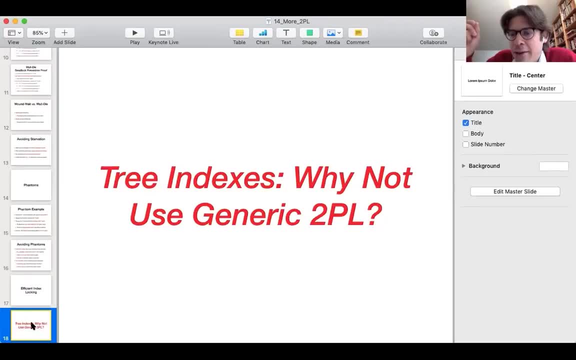 search starts with the root node of the index, so the root page of the index they receive a lot of traffic in. essentially, if we give to some transaction a lock on the root node of the index and a transaction, you hold this log until the very end of transaction execution. 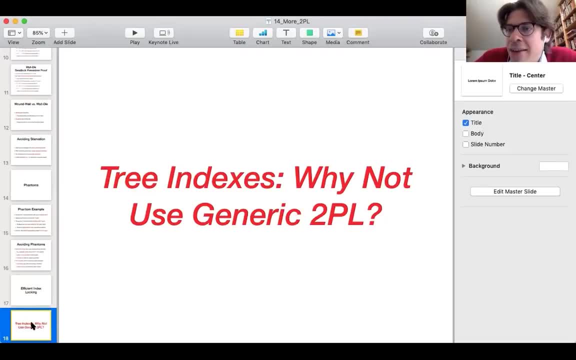 then none of the other transactions can get any locks on the same index and tú, they are trying to update the table that the index refers to. it means that none of the other transactions can make progress. so the problem is really that. the problem is really that we need to, that all the transactions need to pass. 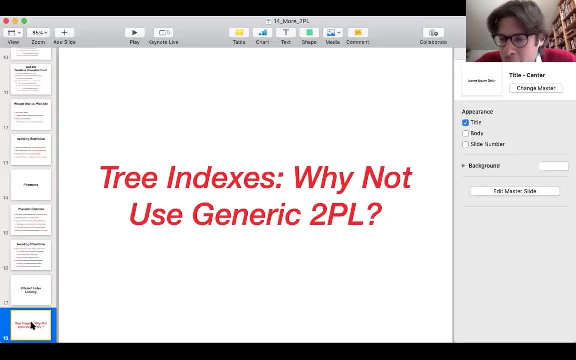 through the same index page when starting their searches. and here one question is about which pages in an index transactions locker in the first place, and when doing it naively, then the transactions would need to lock all the index pages from the root node to one of the leaf virus churches. because if you 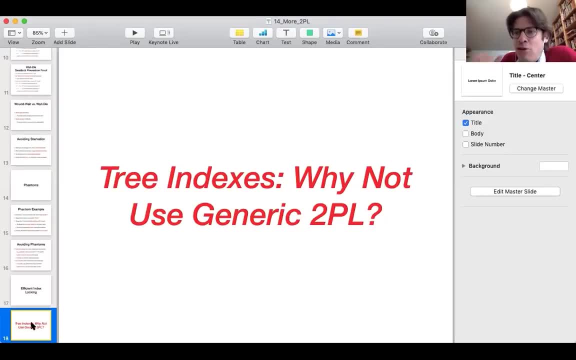 make a change in one of the leaf notes, there's always a chance that it propagates up the different levels of the tree until the near-nBI unit. they have seen a of examples for index updates in the indexing lecture and in some of those examples we had updates, insertions or deletions in one of the index leaf nodes. 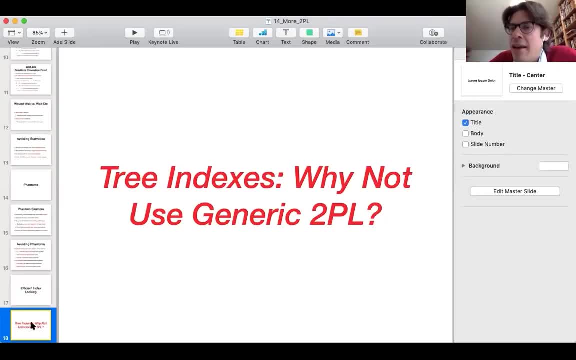 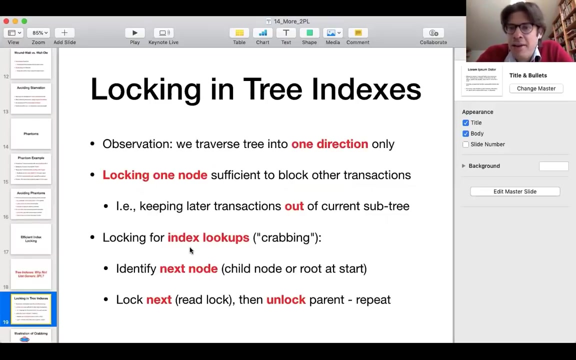 that propagated up to the very root of the index tree, and that is why, in principle, when doing it naively, then transactions would need to acquire locks on the entire path from the root to one of the leaf nodes, and that is very inefficient. but the great question: Good, now in order to lock indexes more. 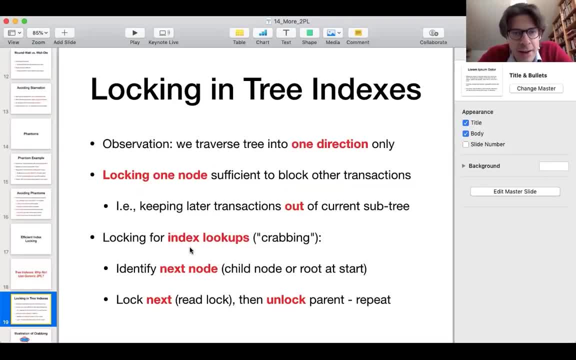 efficiently. we can explore a couple of particularities of indexes. so, first of all, we traverse indexes only in one direction. so at least as long as we're only searching, we're starting from the root. then we always step to one of the leaf node, the tight nodes, until we finally reach one of the leaf nodes. 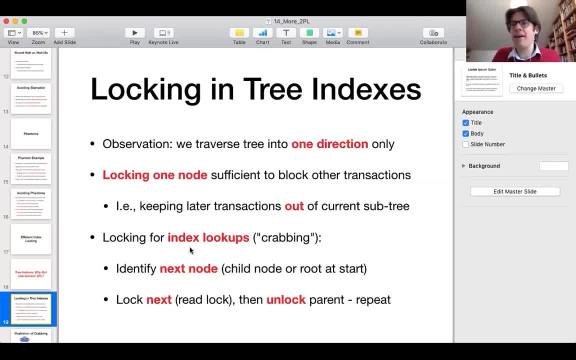 So, since we know that all the transactions traverse the index from top to bottom, it means that, in principle, in order to block other transactions from acquiring locks in the same sub-tree that you are currently working in as a transaction, it is enough to just 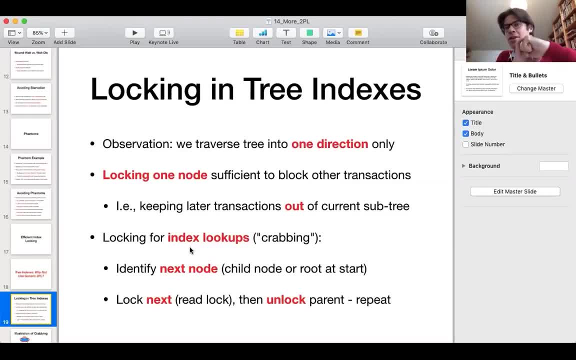 hold one lock on your current node and that will block all the other transactions from passing you over and entering the sub-tree that you are currently interested in. So this insight is extremely important because it essentially means that we can, specifically for indexes, sometimes release locks early, and that allows other transactions to proceed. 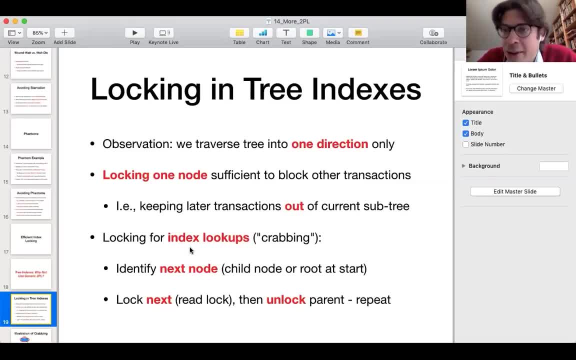 in parallel. The technique is called crabbing because it is supposed to resemble a little bit the movements of a crab, and what you do essentially is that you, at each step, identify the next child node in the index that is relevant, starting with the root node, as usual. 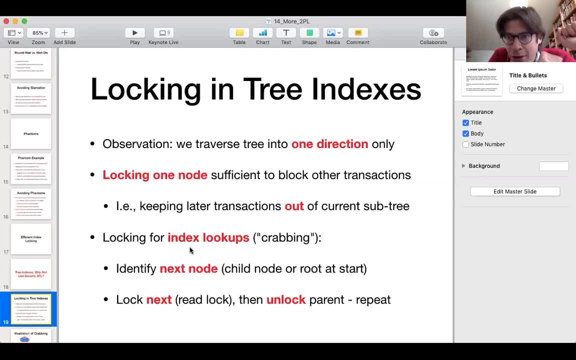 Then you lock the next child node. After you have the lock, you unlock the parent And then you repeat until you have reached one of the leaf nodes. So that is the method that we will use for index lookups which do not change the tree. 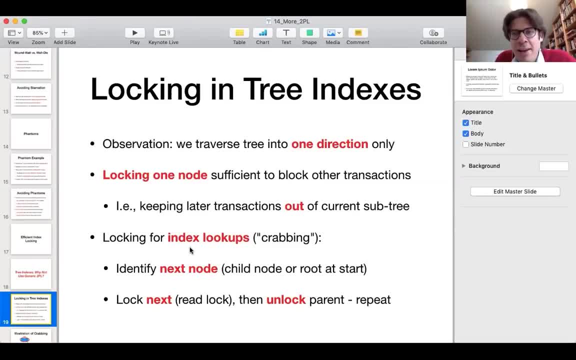 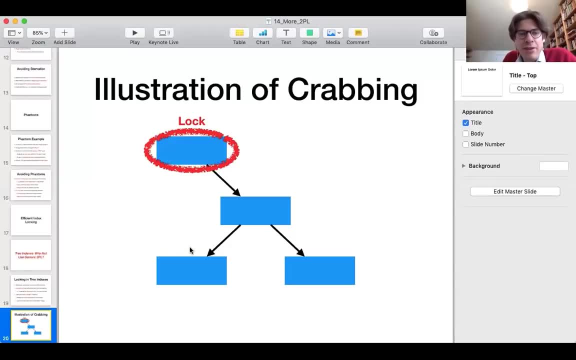 They only need to read it. Let's quickly illustrate how that looks. So here those blue nodes represent the path of an index tree, And here we start from the root. here We lock the root node And then we check which of the child nodes is most relevant. 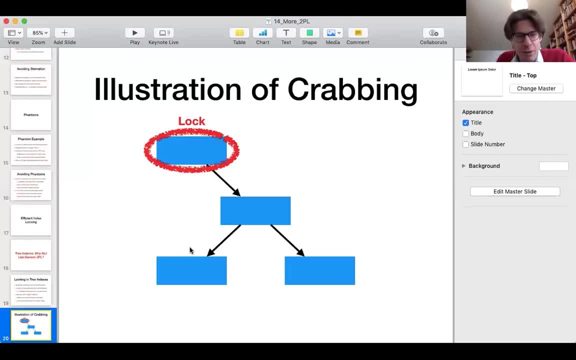 So here I'm only drawing part of the index, so that's why you only see one leaf node. We are locking that one And after we have the lock now we release the lock on the parent. Now we do the same thing. 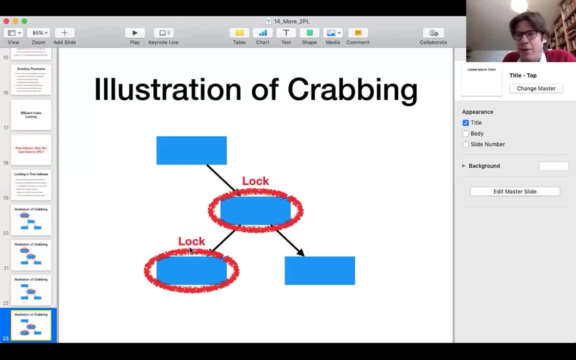 We identify the relevant child node, we lock it. After we have the lock, we release the lock on the parent node. That is crabbing, All right. So this works As long as we are only looking up things with the index. 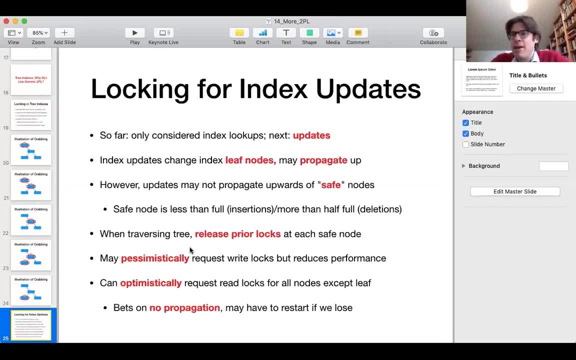 But what about index updates? I have already just mentioned that in the extreme case, some of those updates could propagate from one of the leaf nodes up to the very top of the index tree. At least we can guarantee in certain cases that an update cannot propagate beyond the 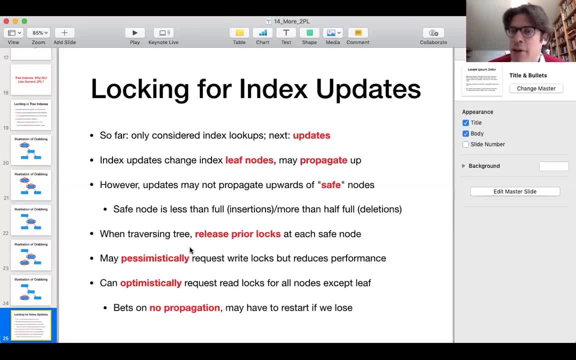 current node. This is what we call a safe node in the index, For instance for insertions. if I insert things into one of the leaf pages and it becomes overly full, then I would have to split the leaf page. And because I'm splitting the leaf page, it means I need to insert one more entry into. 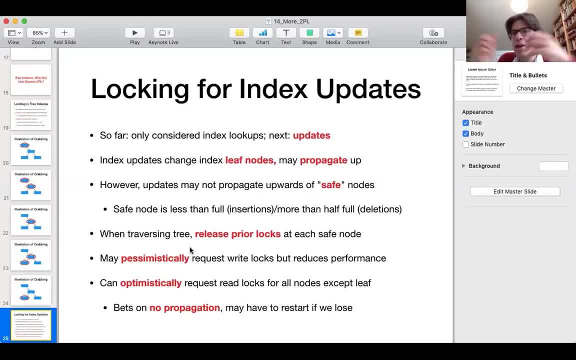 the parent And potentially the parent also becomes overly full and I need to split that one, which means I might have to add one more entry. If I do that, then I would have to split that one. If I do that, then I would have to add one more entry into the parent of the parent and 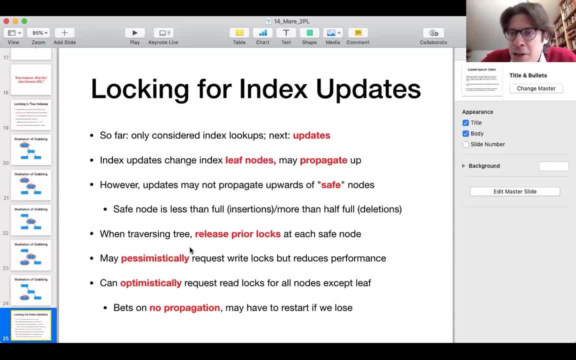 that might split them as well, and so on and so forth. Now a precondition for one of those splits propagating up the tree is that I have too many entries in one of those nodes. So if, in going down from the root to one of the leaf nodes, I suddenly encounter a node, 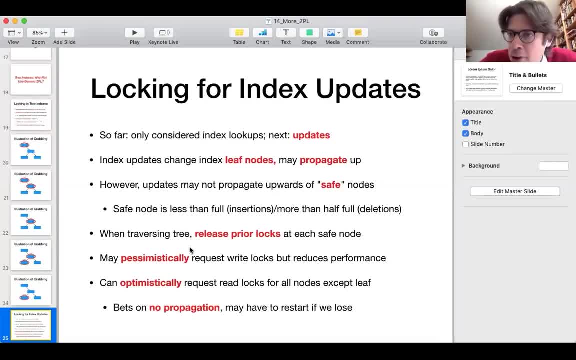 in the index that is not entirely full, then I know that even if I have a split below that node, That split will not propagate beyond the current node because it has still some slots available so it will not run out of space. So that would be a safe node in case of insertions. 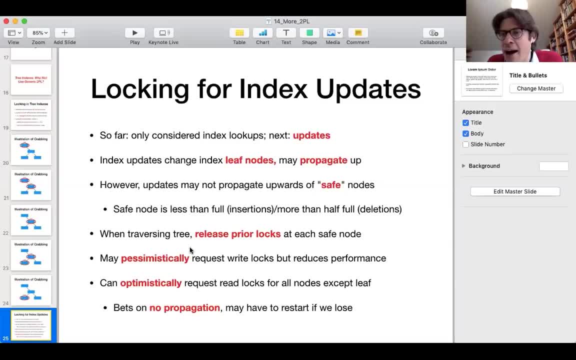 In case of deletions, it's the other way around. Here in deletions, I am deleting an entry on a leaf page. It becomes under full. That's why I need to merge it with one of its siblings, And because I'm merging the two now, I also need to delete one entry in the parent. So that's why I need to merge it with one of its siblings, And because I'm merging the two now, I also need to delete one entry in the parent. And because I'm merging the two now, I also need to delete one entry in the parent. 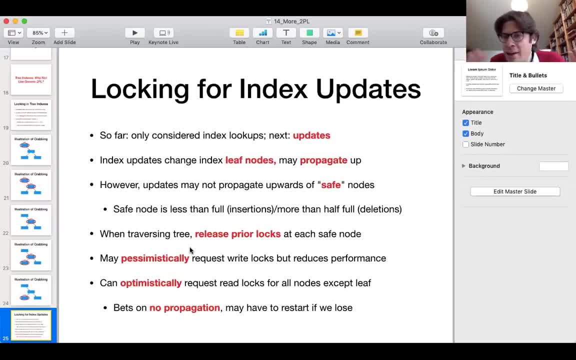 Which might mean that the parent also becomes under full. so I have to merge the parent again and so on. In case of deletions, I know that one of those merge operations cannot propagate above the current node if the current node has a little bit more entries than necessary. 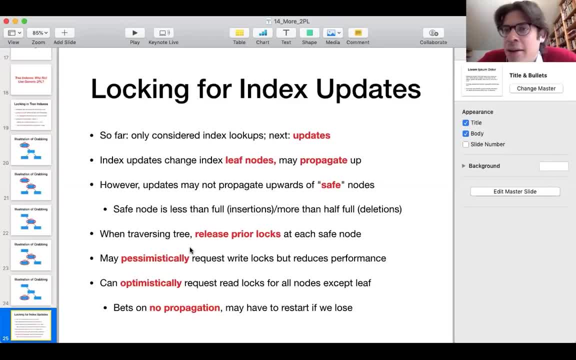 So I know that even if I delete one of them, it cannot lead to a merge for the current node. So one first strategy is that at least I take this into account Instead of holding all the logs from the root to one of the leaf nodes when going down. 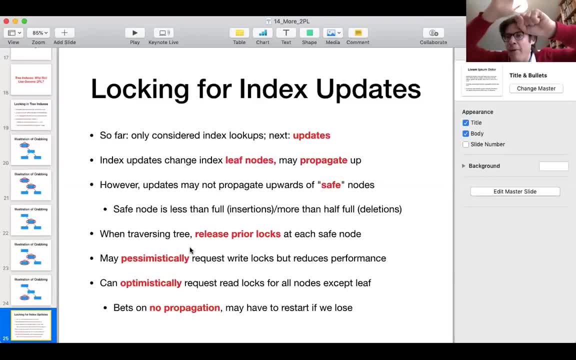 I quickly release logs above from safe nodes. So if I know that the current node is safe and updates cannot propagate beyond it, then it can release the nodes on its, the logs on its ancestors. All right, So that I can do. Now the question is which type of log I want to acquire. 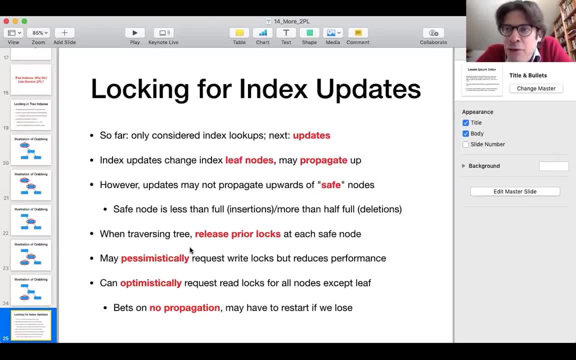 Now when, being very pessimistic, I would have to assume that updates always propagate up to the current safe node. That means that I probably want write logs up to the current safe node. Now write logs, AKA exclusive logs. they will prevent other transactions even from reading. 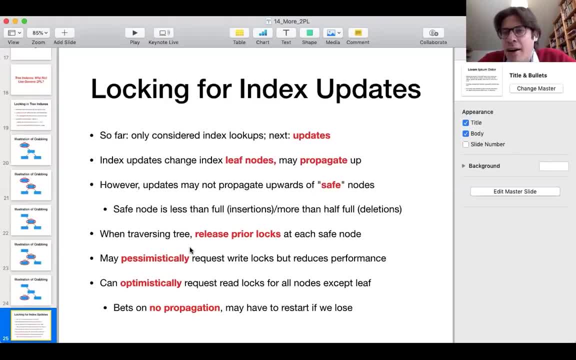 the associated data. So they are bad. They are bad for concurrency performance. So what I could also do is that I'm being optimistic and I assume that updates do not propagate up to the current safe nodes. That means that essentially I'm only acquiring a write log on the leaf page. 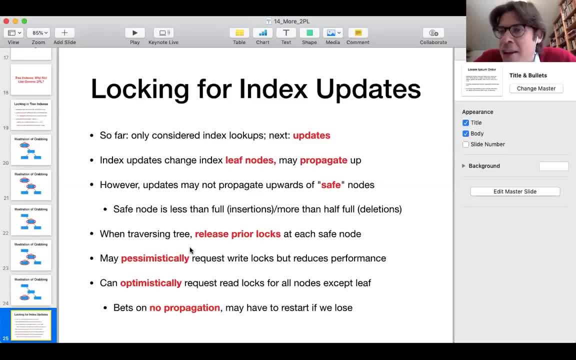 And I essentially am betting that no updates propagate beyond the leaf node. Now, if I win that bet, it means that I get better performance than I would have gotten with the pessimistic approach. If I lose the bet, it means that I might have to abort and restart. 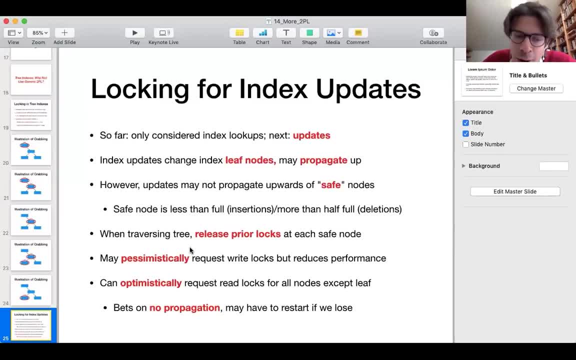 And this time I'm more pessimistically- acquiring all the logs. So again here, you cannot say which one is better. It always depends on the particularities of the scenario. All right, So that was indexed, So let's move on. 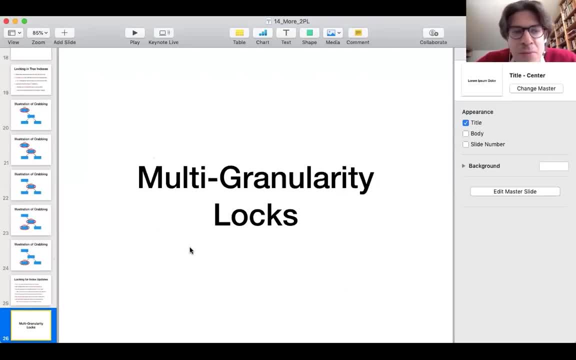 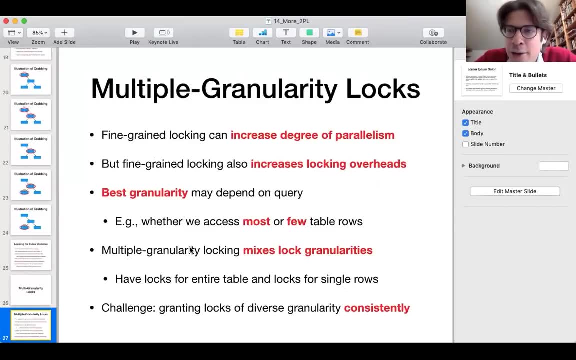 Index locking. We will not be able to discuss multigranularity locking in all detail. Just already, as a little teaser, I want to tell you that multigranularity locking essentially allows us to define logs at different granularities. For instance, we could have logs on entire tables together with logs on specific rows. 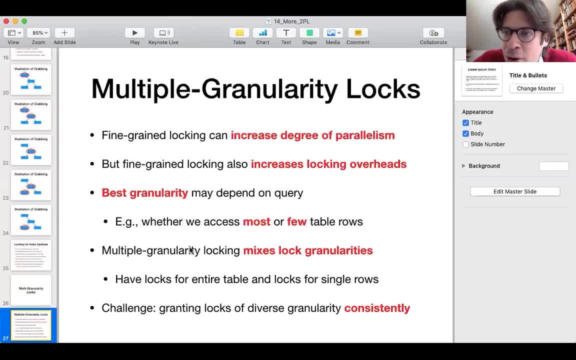 in specific tables And the next time we're going to discuss about how we can make sure that we grant the multigranularity locks in a consistent manner, All right, And if we have multiple? yes, there's a question in the chat. 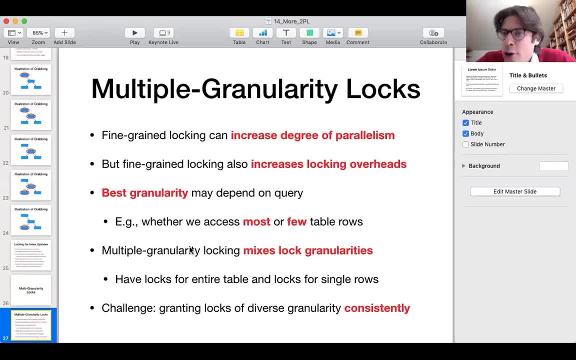 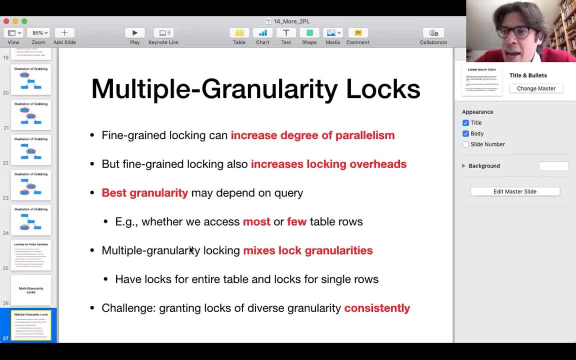 Right, So we need, you can- essentially you can- allow multiple transactions to read in parallel as long as none of them is changing the entries. And there's also a question about why we actually need read logs if we don't want to change, or if you don't expect that we need to change nodes above the current leaf node. 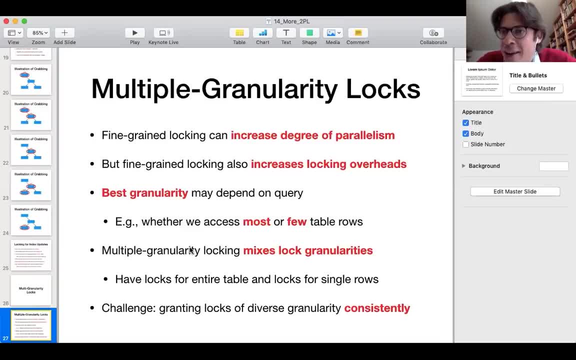 The thing is that, even if we don't want to change nodes above the current leaf node, even if we don't want to change the data in those nodes, we have to make sure that none of the concurrent transactions is changing those nodes above the node that you're currently. 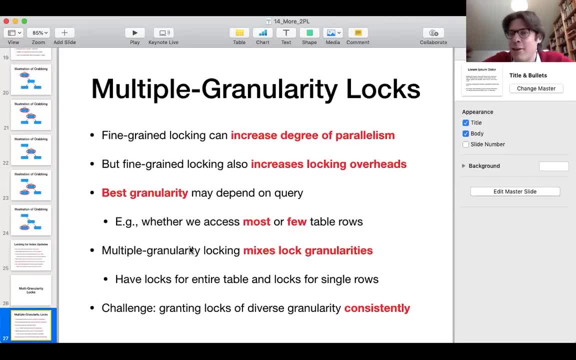 working on, Because those nodes they contain the references to the leaf node that you're currently working on, for instance, And if somebody suddenly changes those other nodes then I might end up with inconsistent data. So getting those read logs is just about preventing other transactions from happening. 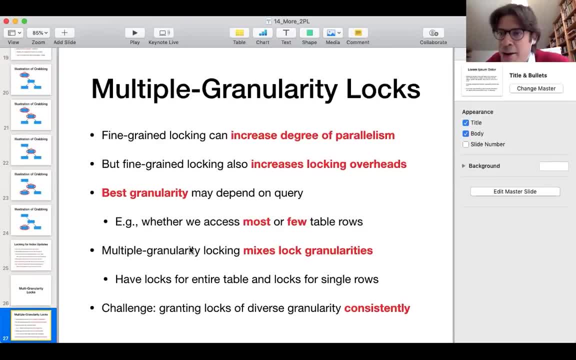 So that's the first step. All right, So we have a couple of questions. One is from preceding in parallel. Alright, Good, So we are at the end of the time slot. I wish you a nice day and then I see you again later this week. 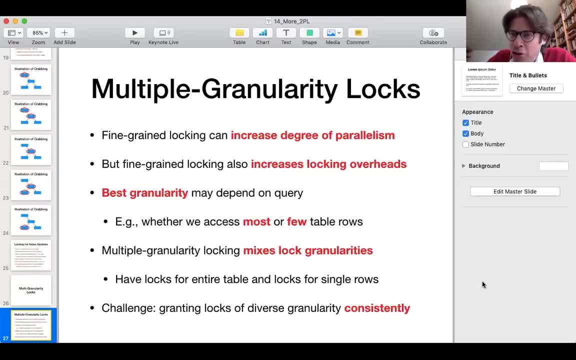 We will also have our third homework coming out tomorrow, And that homework focuses on joint processing, So this might be a good opportunity to review again the corresponding material, in case you haven't done so yet. Have a nice day, and then see you later this week. 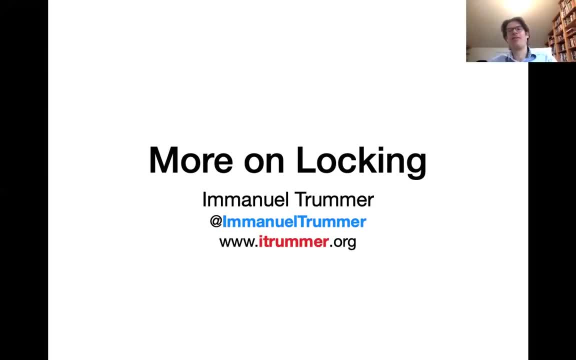 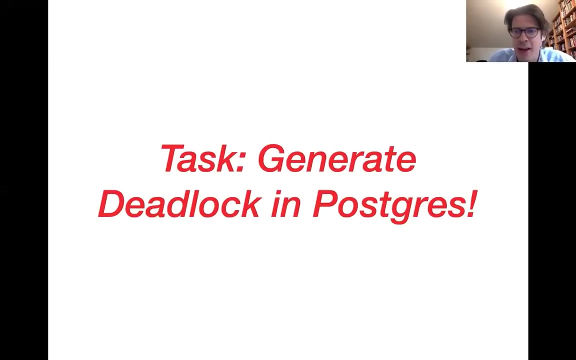 Okay, awesome, good, all right. So today we are going to discuss more about concurrency control. The last time we have been discussing about a couple of specialized topics around locking, We have discussed, for instance, about deadlocks, So here we had discussed about how to detect them or how to avoid them. 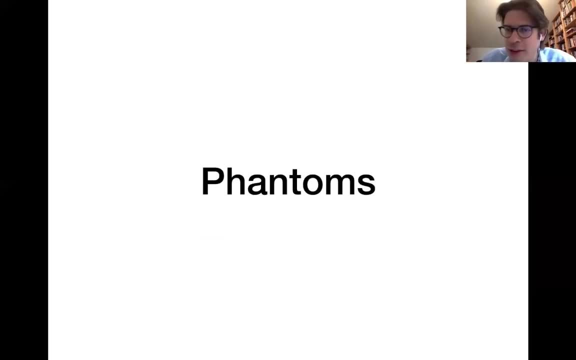 Then we have discussed about phantoms, which is this additional anomaly where I am retrieving a set of objects from the database based on predicates And when running the query twice, then I get suddenly different results because other transactions inserted something. We have discussed how we can avoid that using indexes. 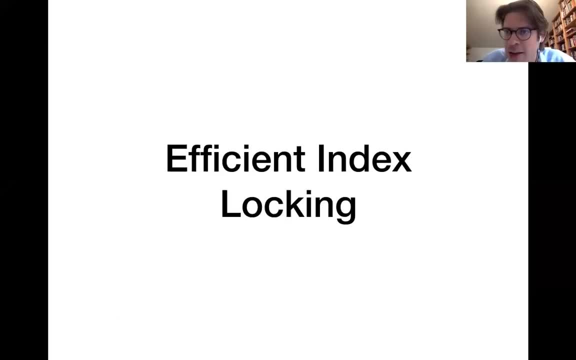 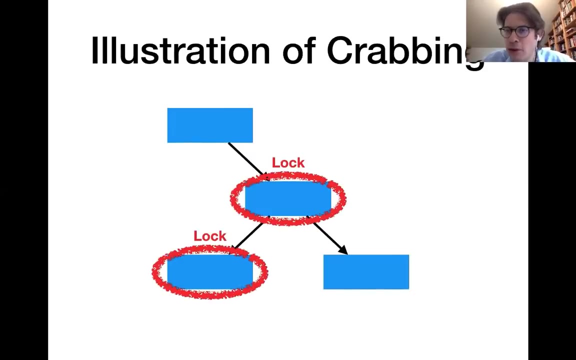 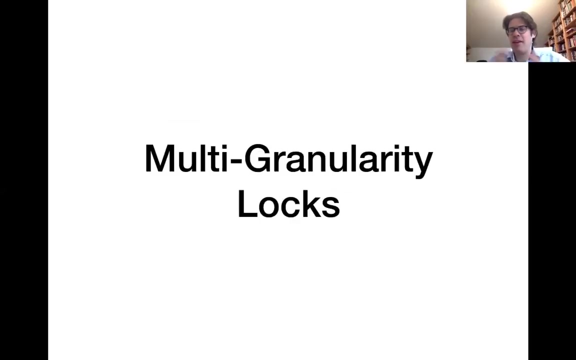 And we have discussed about locking in tree indexes, where you can use the generic locking protocols, but that is inefficient, So instead you want to use a specialized locking protocol At the same time when accessing an index. Now the final topic around locking that we will be discussing this is multi-granularity. 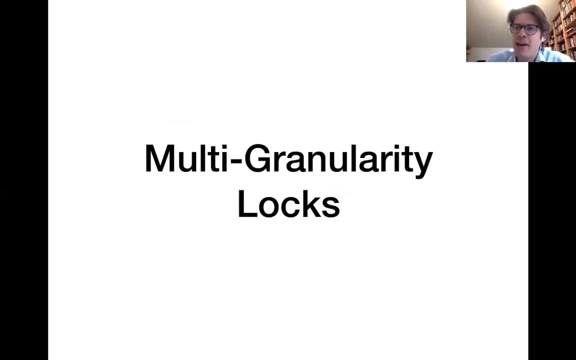 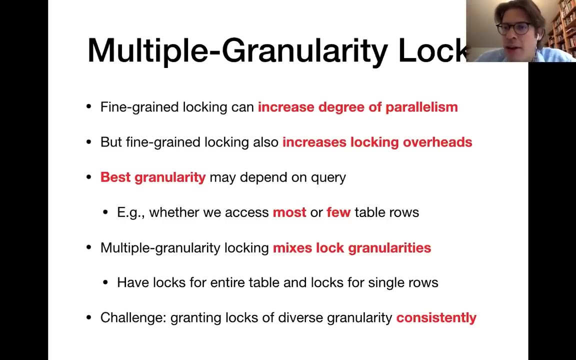 locking. After that, we're going to switch to discuss about a concurrency control methods that are not based on locking. First of all, let's discuss about multi-granularity locks. Okay, Okay, And the motivation for multi-granularity lock is that there is a trade off about the granularity. 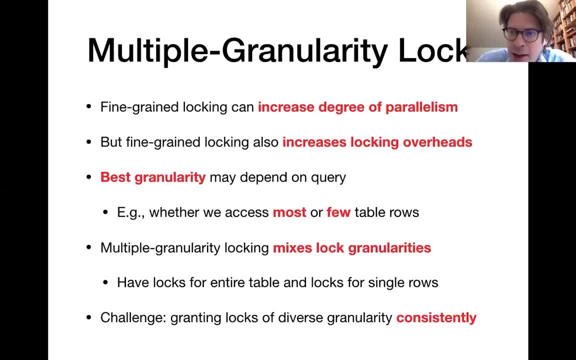 of locks. At the very very beginning, when we started discussing about locking based concurrency control, we had an example protocol that was very simple and it just locked the entire database, So only one transaction was able to operate at the same time. Later we have discussed that. 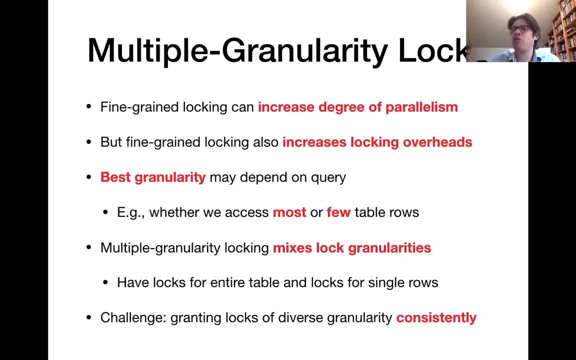 Okay, So we have a very simple example. We have a very simple example. We have a very simple example of how to use multi-granularity locks. So this is a very simple example. You can use multi-granularity locks on a single table or on single rows. 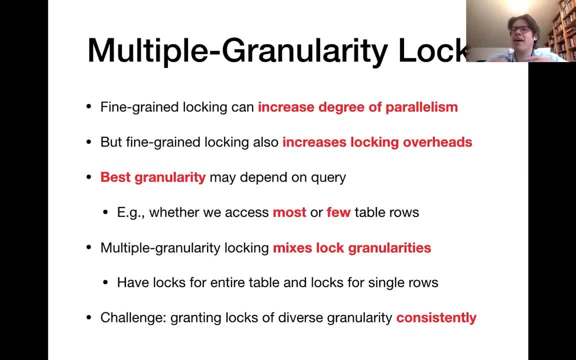 And single tables provides you with a higher number of transactions that can execute at the same time, So it's probably good for performance. The drawback of that on the other side is that if you have very fine grained locks, then transactions typically need to a lot of those fine grained locks in order to do. 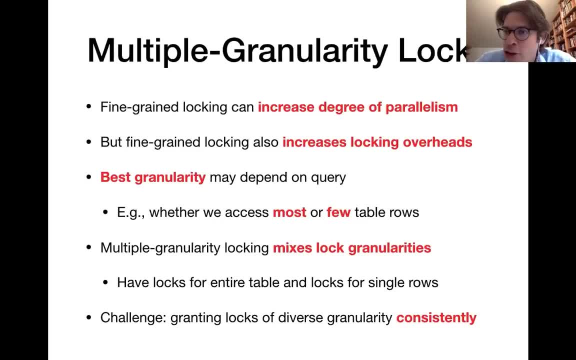 what they want to do. And each lock request and lock management also means a certain overhead in the lock manager And if the lock manager has to manage lots of very small locks on many objects in the database then that might actually become a performance bottleneck. 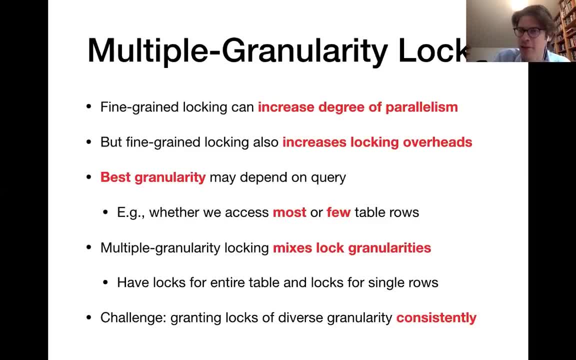 So there's some motivation for granting fine grained locks. There's also some motivation for granting more coarse grained locks, And it is difficult to say which of those works best in general. So with multi-granularity locking we don't have to make that choice because we can dynamically. 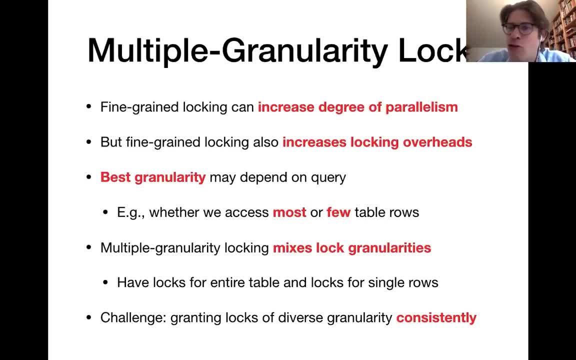 choose between obtaining locks at different granularities. So if a transaction wants to read most of the rows in a table, it may just get one lock on the entire table. But if a transaction only wants to access one specific row, then it may just get one. 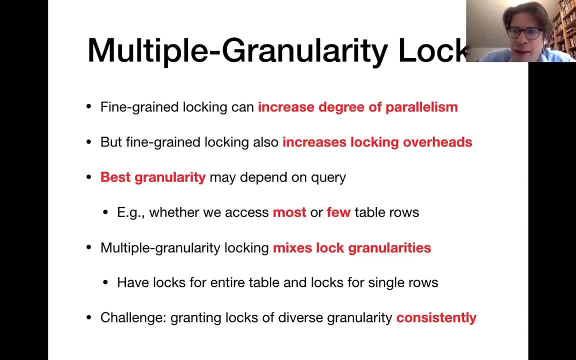 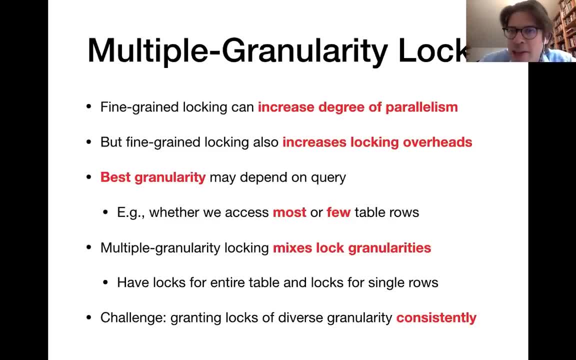 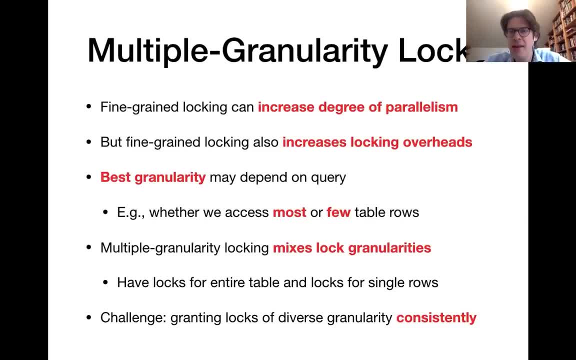 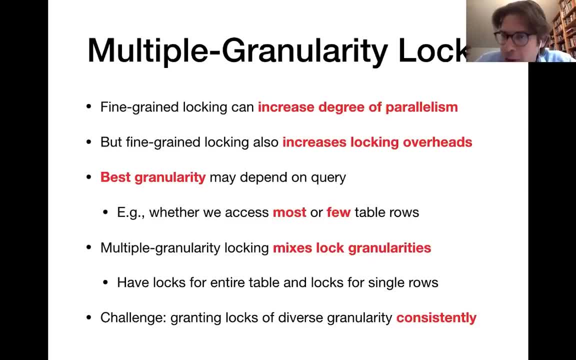 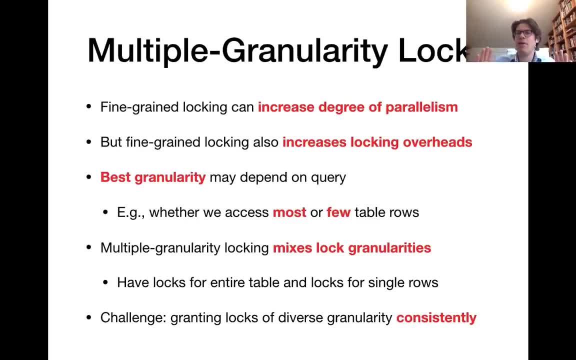 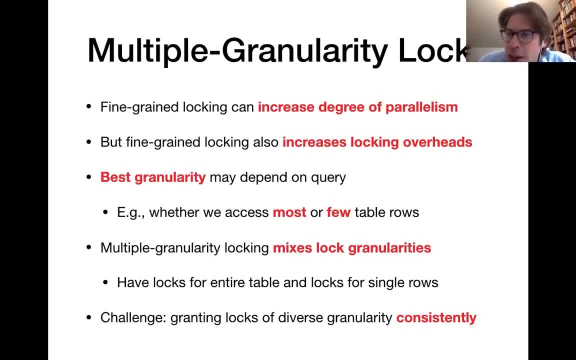 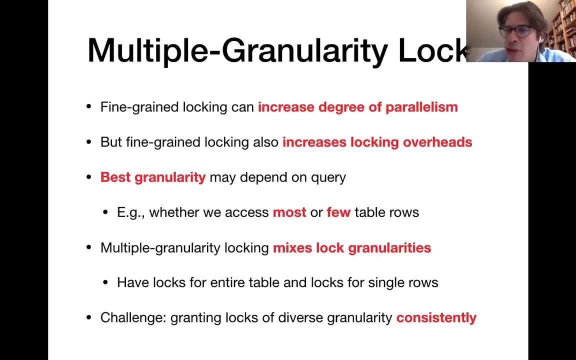 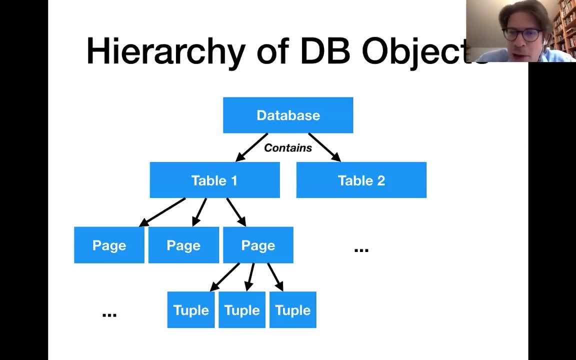 So in general we assume that we have a hierarchy of database objects. So here there would be at the root of that hierarchy the entire database, And then it splits up into single tables And for each table it splits up into pages. 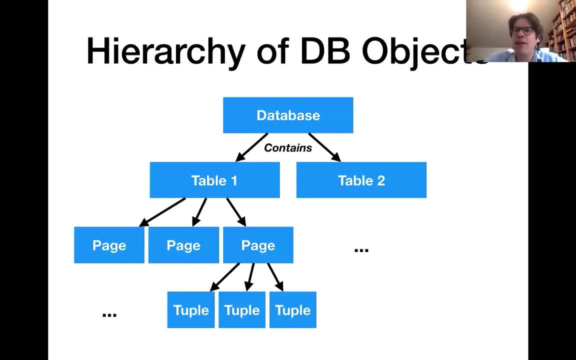 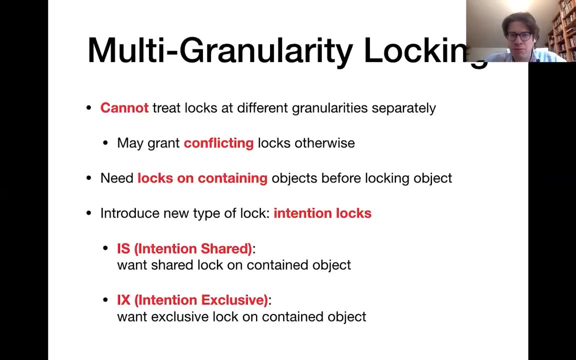 And each page splits up into different tuples again. So that is the hierarchy of database objects And with multigranularity locking we can obtain logs at different layers of this hierarchy. Now the way in which we make sure that we don't grant any conflicting logs: 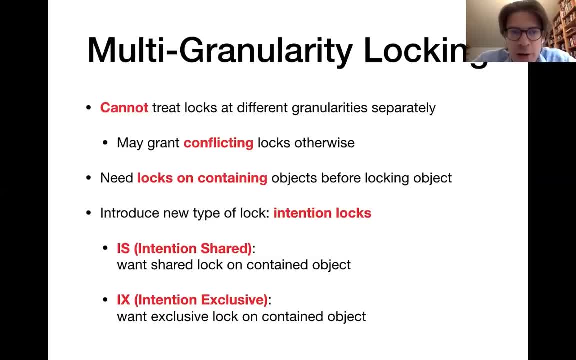 is by introducing new types of logs. Those are those intention logs. We have two types. We have the intention-sharing, We have the intent-sharing And we have the shared log And we have the intent-exclusive log And what that means essentially. 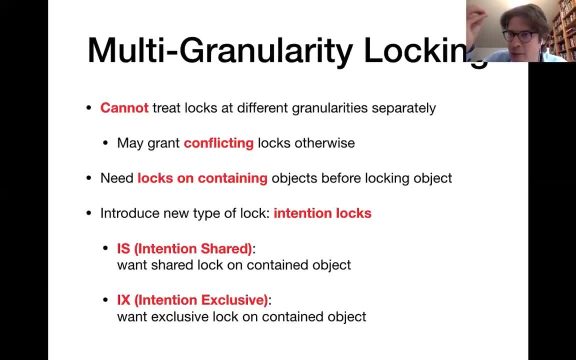 if you acquire an intention-shared log on some object in that object hierarchy that we have just seen, it essentially means that you intend to acquire a shared lock on one of the contained objects. So if you have an intention-shared log on a table, intent to acquire a shared block on one of the pages in that table or on one of the tuples on 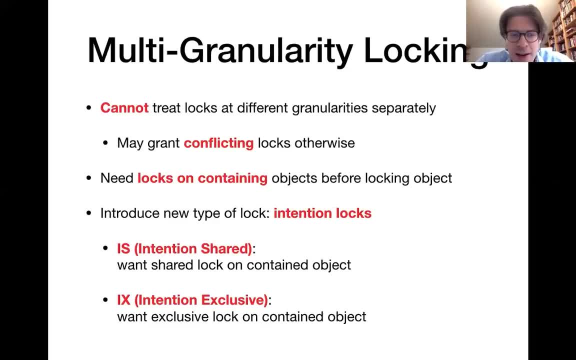 one page of that table, And similarly for the intention exclusive blocks. if you acquire an intention exclusive block on a table, for instance, it means that you intend to acquire an exclusive meaning, a right block, for instance some tuple or for instance some page within that table. 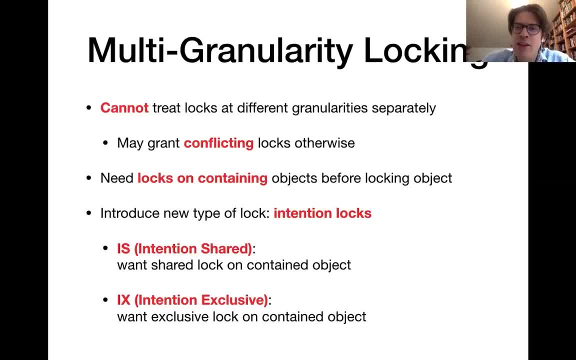 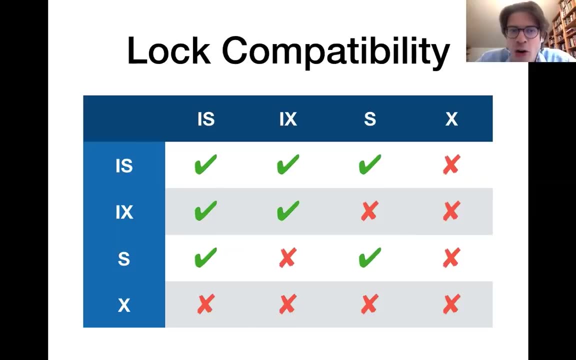 And we will see in the following why using those blocks prevents bad things from happening when granting blocks of multiple granularities. Now, this is an overview of which of those blocks are compatible. We have started out with only two types of blocks: the shared blocks. 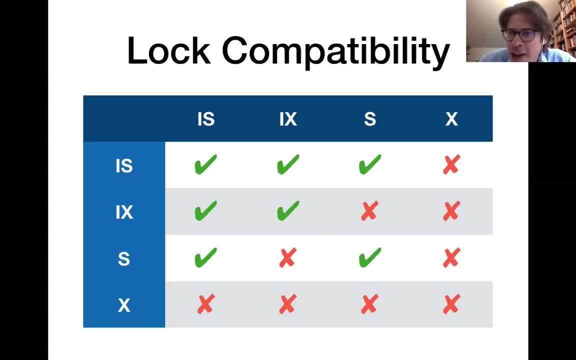 meaning blocks for reading data, and exclusive blocks meaning blocks for writing data. For shared blocks, we can grant the same shared block on the same object to multiple transactions For exclusive blocks. that is not possible. Now we've introduced two more types of blocks, so 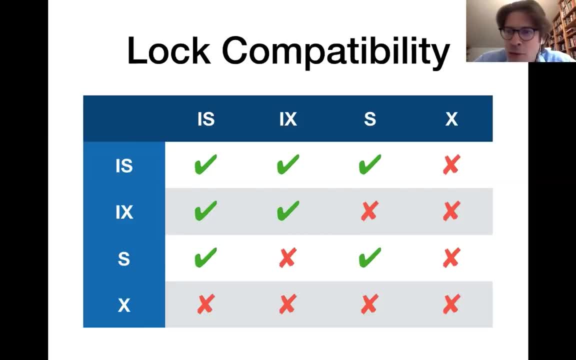 it gets a little bit more complex to keep track of which combinations of blocks are allowed and which combinations are not allowed. Here you see the full overview. I guess many of those combinations are intuitive, So if you have a combination of blocks you can grant the same. 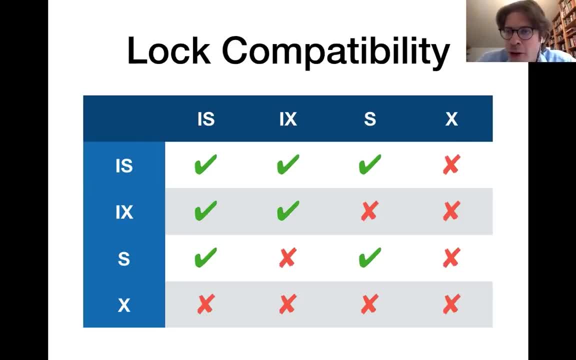 shared block to multiple transactions depending on the position of a block. So you always see the green check mark if the combination of blocks is allowed, meaning if block manager could grant those two different blocks to different transactions on the same object. Now, for instance, 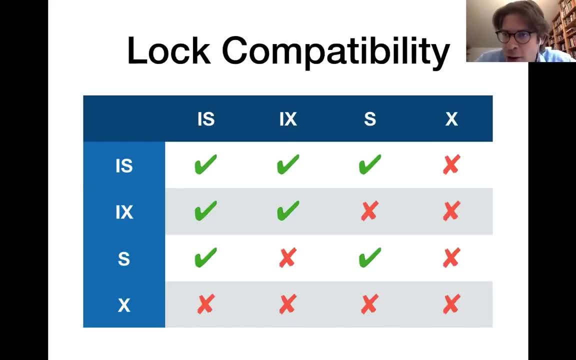 clearly, we can grant the same shared block on the same object to different transactions. That's why we have a tick at the corresponding position. One question that I often get about this matrix is, for instance: why is it that intention-shared and intention-exclusive logs should be compatible? 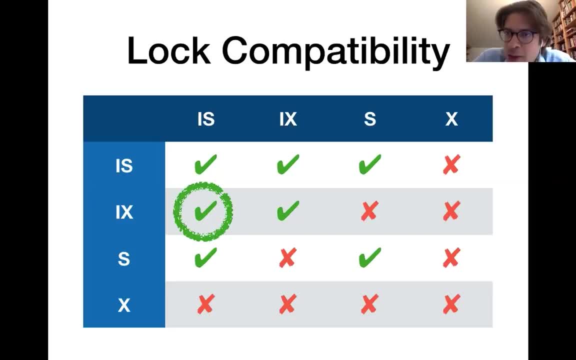 Because, as we know, shared logs and exclusive logs are not compatible. So why is this version of the logs more permissive? And so let's perhaps quickly discuss that point. So, for intention-, exclusive logs- it essentially means that you want to acquire an exclusive log on some contained. 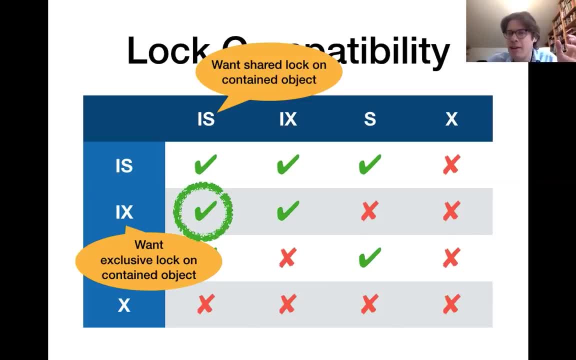 object. So if you get this on a table, it means you might want to get an exclusive log on a row. On the other side, the intention-shared log means that you want to acquire a shared log on a contained object, So that could be also a row. But the point is that 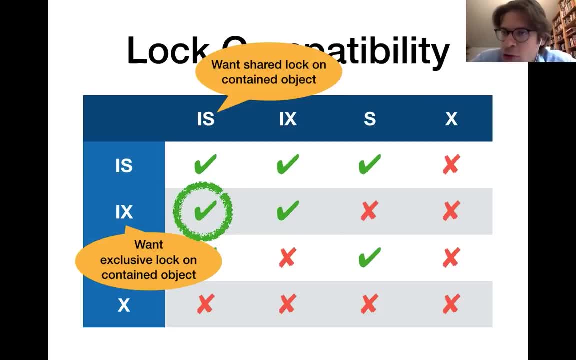 if you grant an intention-shared log on one table to a first transaction and an intention-exclusive log to a transaction on a table to a second transaction, at this point things could still go well, because maybe the first transaction is interested in a different row than the second transaction. So we don't know at this point whether 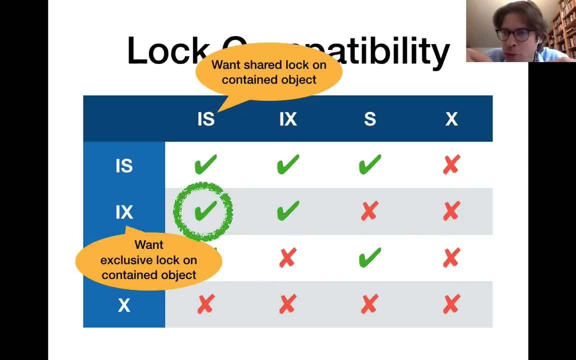 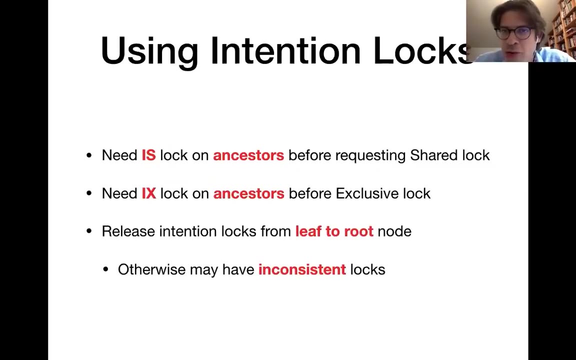 two transactions are really interested in the same contained objects or in different ones. And as long as they're interested in different contained objects, like different rows contained in a table, everything is fine, All right And the general rules to use those intention-logs is before you can request a. 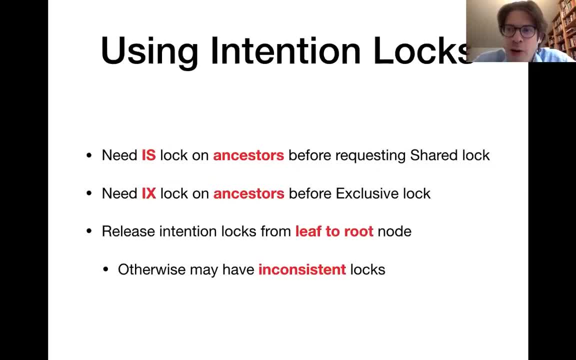 shared log on an object, you first must have obtained intention-shared logs on all the ancestors of that object in the object hierarchy. So if you want to acquire a shared log on a row in a row, you first need to acquire intention-shared logs on the containing page, on the containing. 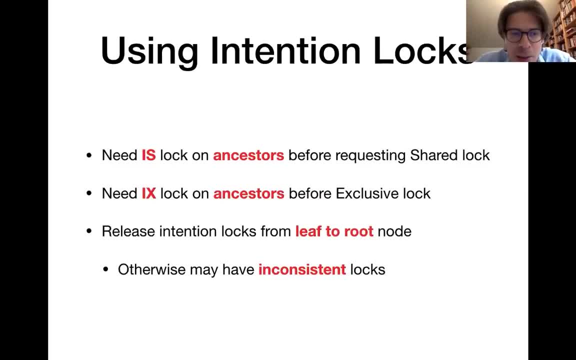 table and potentially on the containing database. Similarly for intention-exclusive logs. if you want to acquire an exclusive log on a row, for instance, you first need to acquire intention-exclusive logs on the containing page, table and so on. All right, So you need to acquire. 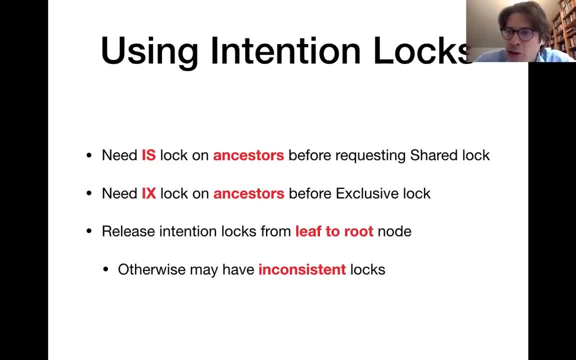 those intention logs before you can request an intention-shared log on a row, for instance, So before you can acquire logs that you actually want. One little detail about the point where you release those logs. again, It is important that you release those intention-logs, not starting. 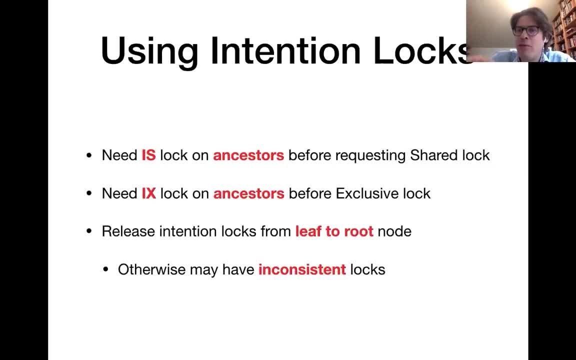 from the root of the object hierarchy, but rather starting from the leaves of that object hierarchy and release them in this order. Otherwise, there's a small time frame in which inconsistent logs could be granted. if you do it, if you release those logs the other way around- And now let's make it a. 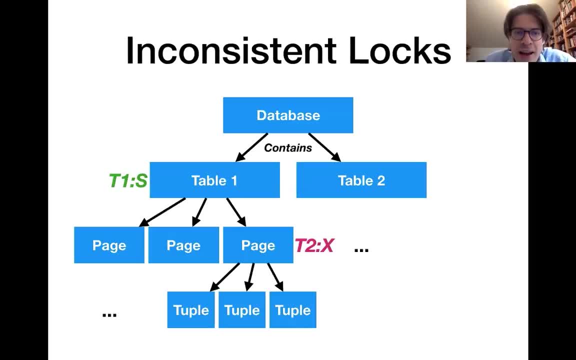 little bit more concrete why those intention-logs can help. For instance, imagine this situation here: Transaction number one, drawn in green, wants a shared log on table one On the other side. transaction two, here, drawn in pink, wants an exclusive log on one specific page in that table. 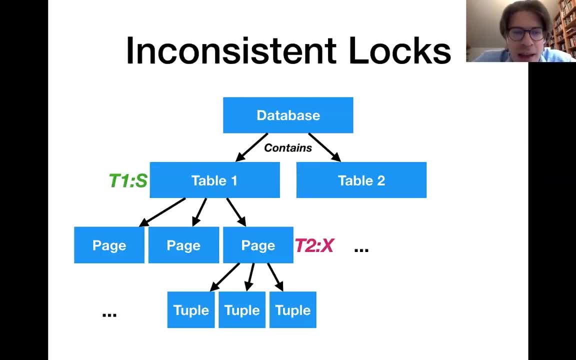 And clearly those two logs are the same. So if you want to acquire an exclusive log on a row, you can see that these two are mutually exclusive. So if we use the system with the intention-logs, then here you see the intention-logs that would be acquired. So here at the beginning. 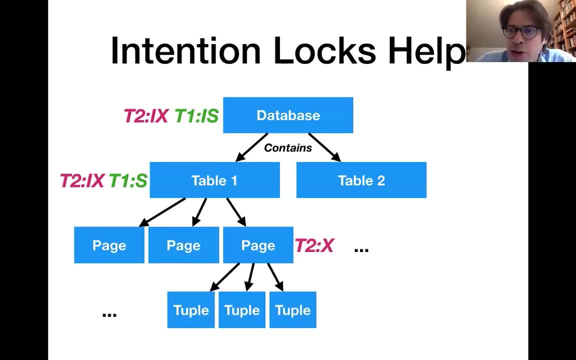 those transactions acquire intention-logs on the entire database, one intention-shared and one intention-exclusive. But those two logs are compatible because- at this point we don't know- transactions are maybe interested in completely different objects that have nothing to do with each other, except that they are both located in the same. 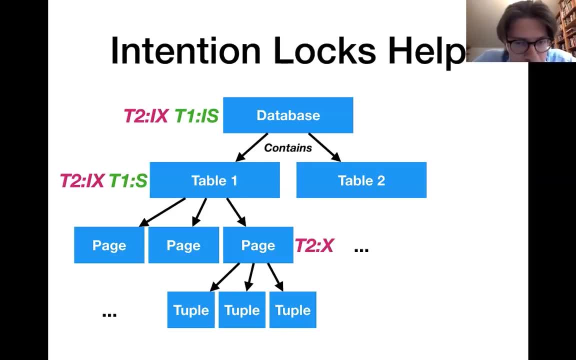 database. Now we continue to table 1 and for table 1, transaction 2 wants an intention exclusive lock via transaction 1 has already arrived at its goal and wants to acquire the shared lock directly And at this point the intention exclusive conflicts with the shared lock. This is why the 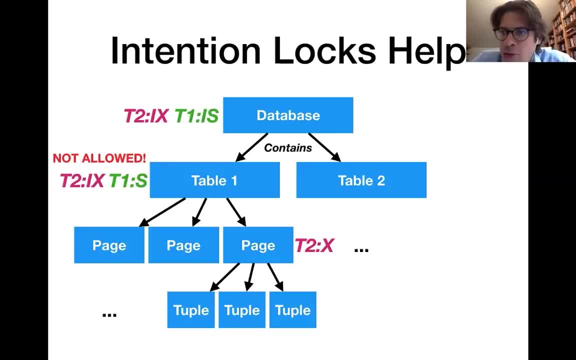 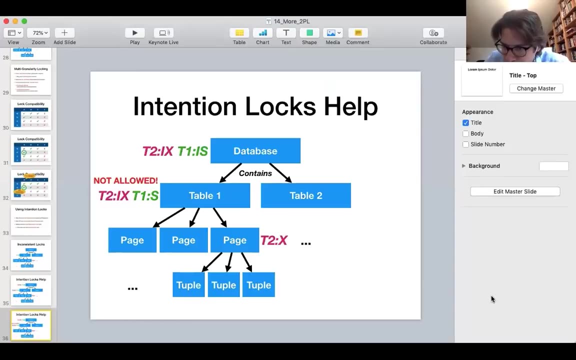 situation that we grant inconsistent locks to those transactions cannot happen because they're using intention locks. I believe there might be some questions in the chat. Let me quickly check that out And those intent. OK, this is a great question. The question is essentially: 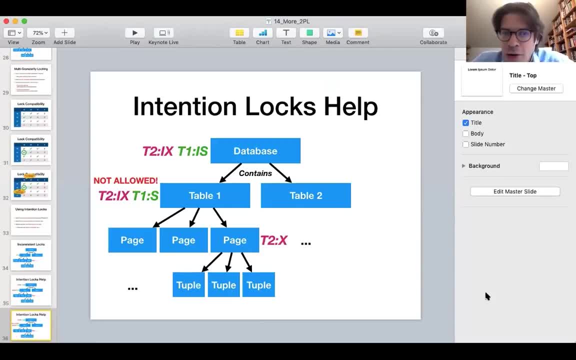 about, like how long we hold those intention locks. And the thing is that I mean, for instance, in this example here, if let's say that the first or let's say that the second transaction goes first and maybe succeeds in obtaining the 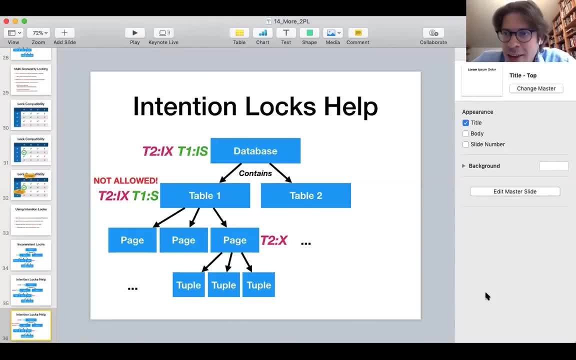 exclusive lock for the page that it is interested in, And now it would decide to release those lock intention exclusive logs on the ancestors. Now, at that point a transaction number one drawn in green, might actually proceed and acquire the intention shared log on the database and the 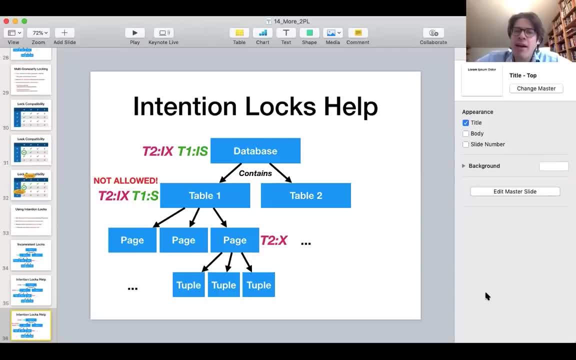 shared log on the table, But that would be inconsistent with the log that transaction two has acquired. So it is very important that we do not release those logs on the ancestors, because otherwise we might grant inconsistent logs. Great question. Now let me quickly change my set of slides If there's any follow-up questions or any. 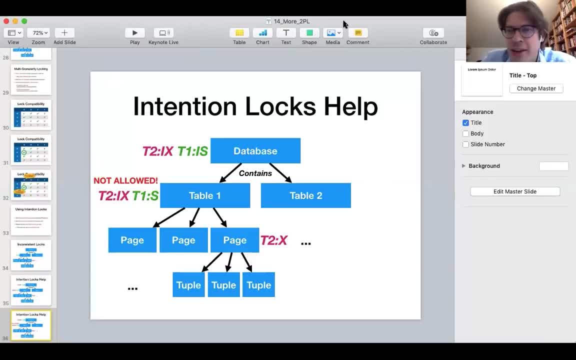 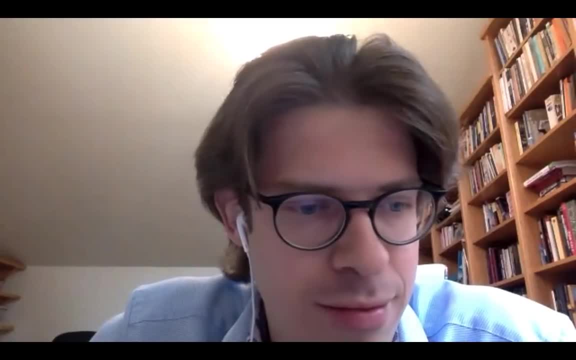 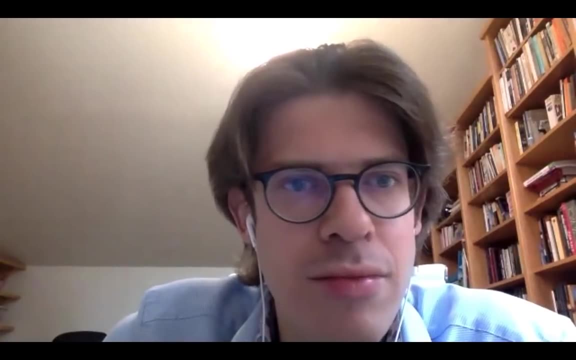 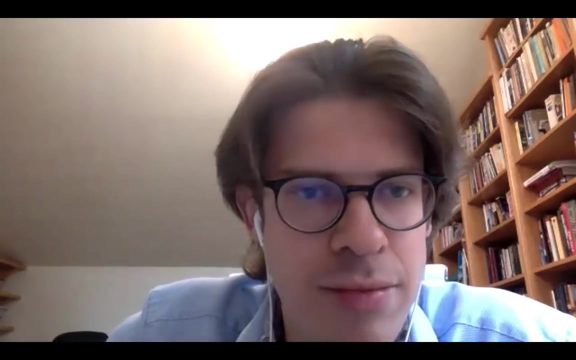 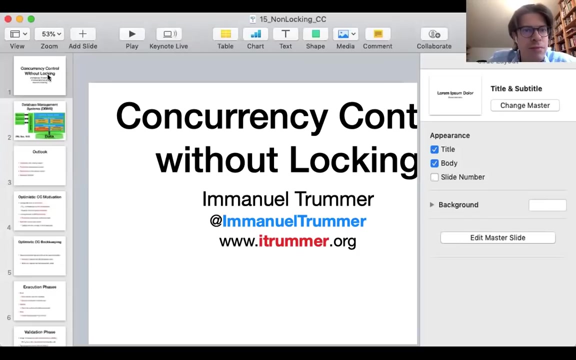 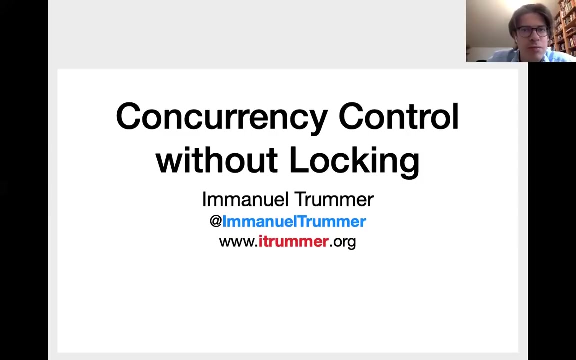 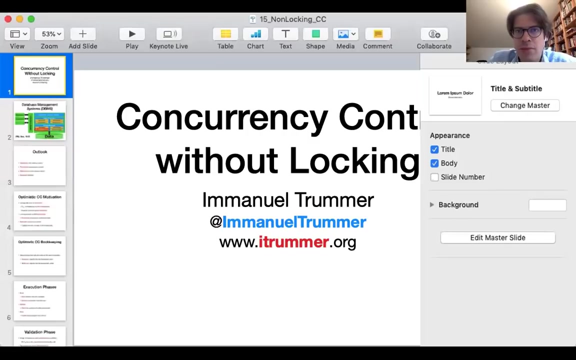 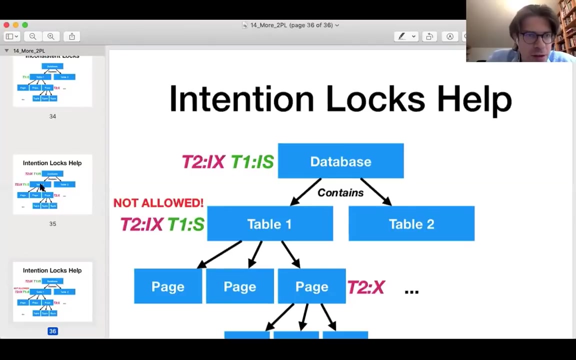 other questions, then please don't hesitate to put them into the chat. Thank you very much. And there was one more question about, like, the benefits of intention shared and intention exclusive logs. Perhaps we can even quickly go back to that one, to this example over here. 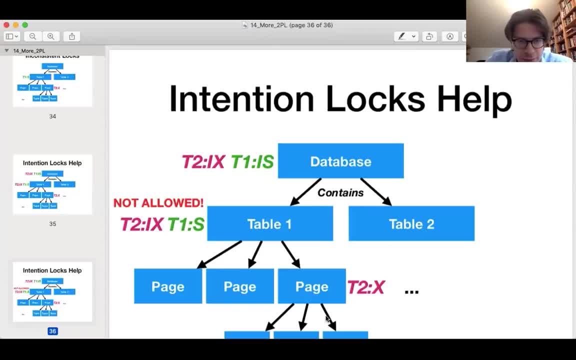 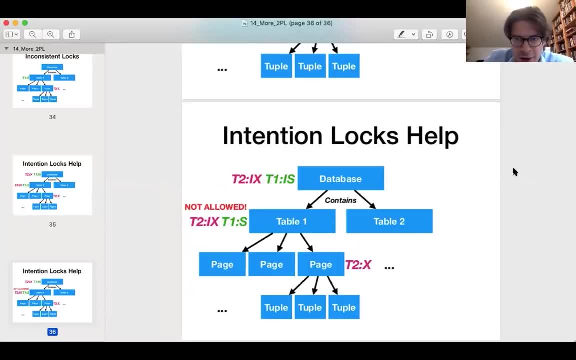 All right. So now you should see the example again. And here, essentially, if you would not use any intention shared or intention exclusive logs, then the database might grant inconsistent logs at different layers of that hierarchy. Here, for instance, there's transaction two wants an exclusive log on one specific page. 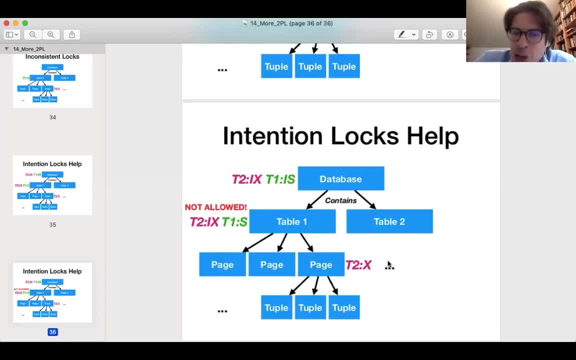 which is contained in table one, And transaction one wants a shared log on table one And logically, if some transaction has a shared log on the entire table, then the transaction one wants it implicitly means that it has a shared log on each page in the table. So that would. 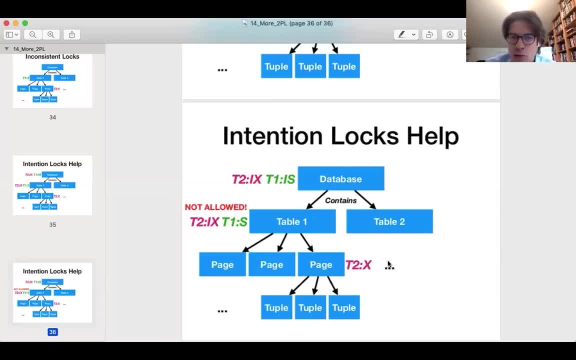 be inconsistent with granting an exclusive log to transaction two, And I mean an alternative to intention logs would be, for instance, that transaction one, before acquiring the shared log on table one, first checks all the pages and all the tuples of the table in order to see whether maybe some other transaction has acquired a shared. 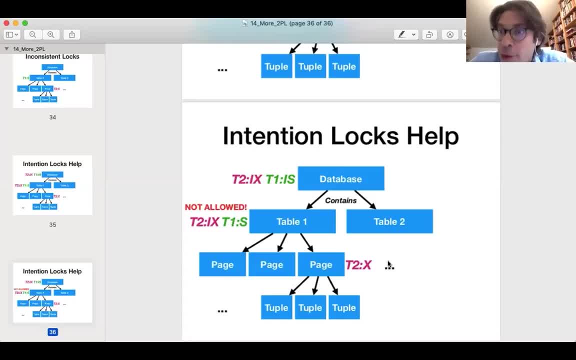 log. So that would be a conflicting log on some element within the table, But doing that, of course, is very inefficient. So the whole reason for multi-granularity logging is that we want to improve efficiency, And because of that it is much better if the second transaction 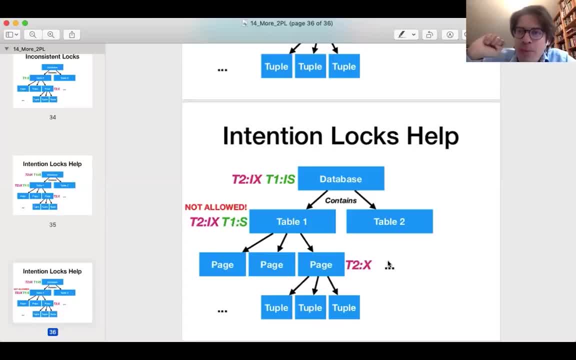 marks up not only the specific object, the specific node in the object hierarchy that it is interested in, but also all the ancestor nodes on the page. So that's a very interesting example, Thank you. Next slide, Thank you. So here I am, uh marking up the path from the root to the logged node in order to indicate. 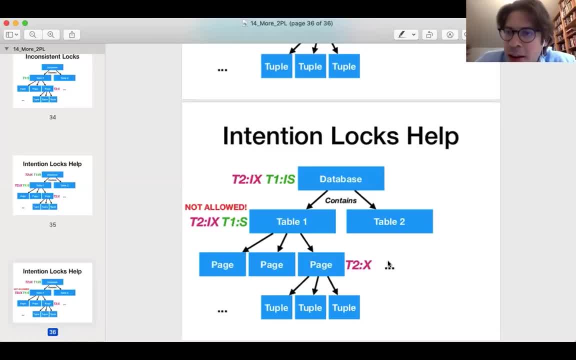 that there is some object within the table and within the database where we have an exclusive log. So marking up the path from the root to those objects in the object hierarchy is a means of avoiding over avoiding checking overheads when granting logs to coming transactions. 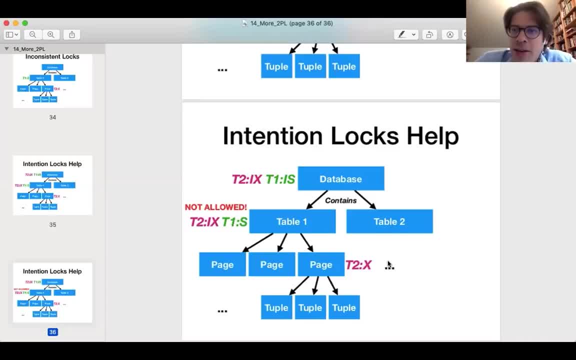 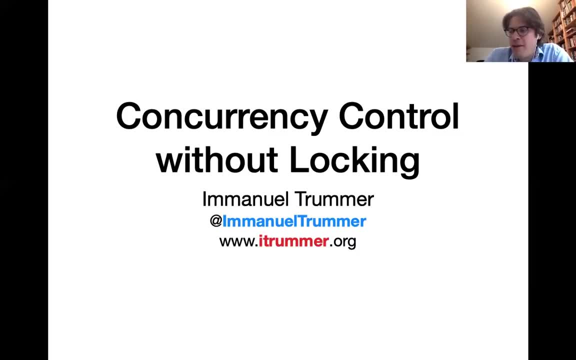 So there would be different ways of doing it, Thank you, Thank you. I would love to see ways of solving that, but via those intention logs it's pretty efficient. So far we have been discussing a lot about locking based concurrency control. Now, in the following, we're gonna discuss: 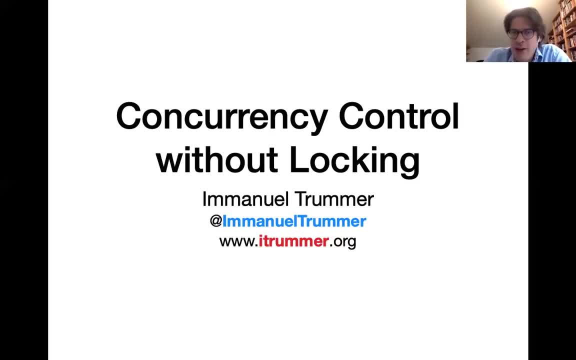 about the alternative methods to do a concurrency control without locking. Now it may seem a little bit imbalanced the amount of time that we dedicate to talking about locking based concurrency control and the amount of time that we'll be talking about all other concurrency control methods. 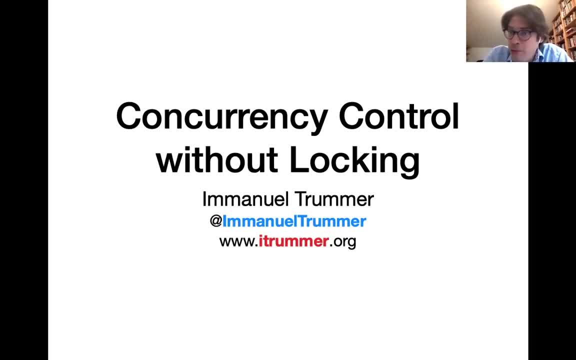 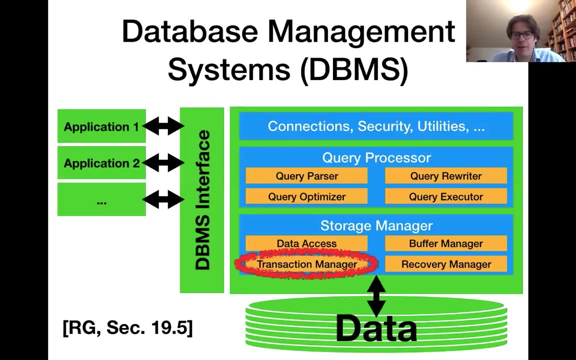 but in practice locking is perhaps the most popular concurrency control method. This is why we spend more time discussing about that. But there is various alternatives and in the following we're gonna see a little overview of those alternatives. So within this course overview slide we are still talking about the transaction manager And the relevant 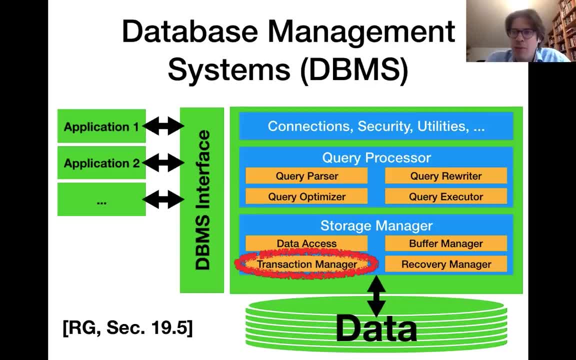 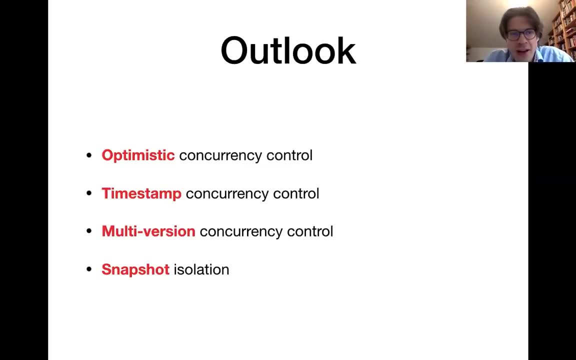 test in Ramakrishna and Gyarke is specifically chapter 19.5 for those concurrency control methods which are not based on locking. On the following we're gonna discuss about those four concurrency control methods: Optimistic concurrency control. timestamp concurrency control methods. 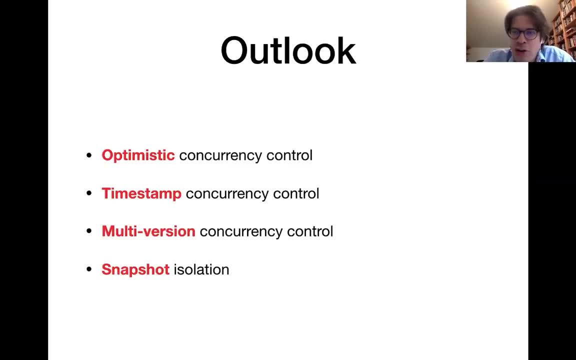 optimist, concurrency control, timestamp concurrency control methods, anticipatory concurrency control methods, multiversion concurrency control and snapshot isolation And many of those concurrency control protocols. they have some common ideas to them. For instance, many of them they use timestamps in one way or in another one. 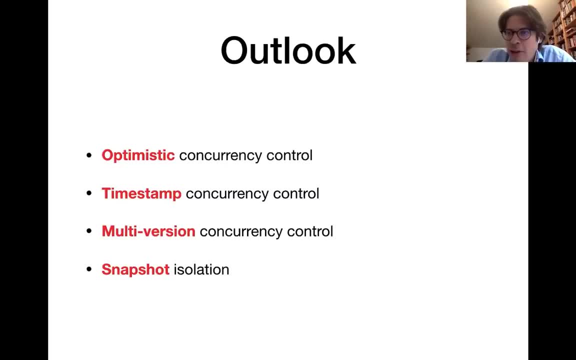 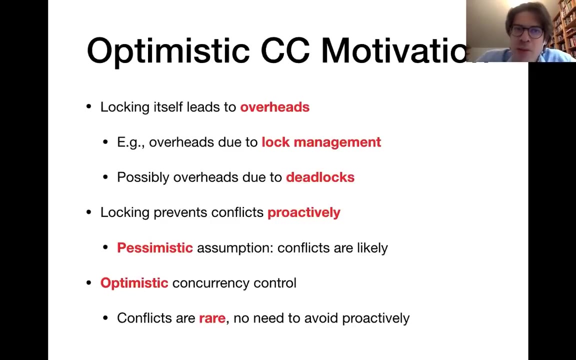 but in general they are different And you might find that for specific databases and workloads, one of those works better than the others, And it is difficult to say a theory which one it is Now. first of all, let's talk a bit about optimistic concurrency control. 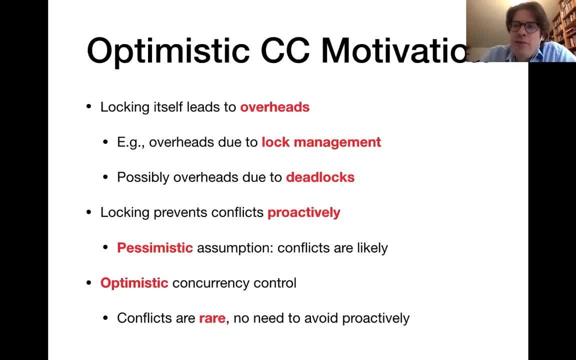 Now, in a way, locking-based concurrency control is rather pessimistic, because before doing anything, transactions always have to acquire those locks in order to avoid any conflict before they actually happen. Now that means that we have to pay with overhats for lock management. 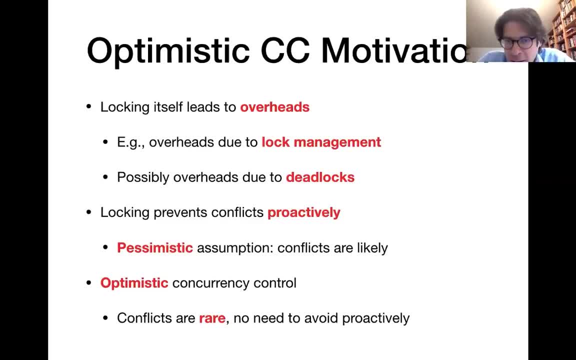 and, depending on the locking variant, you might also have things such as step locks, for instance. we are avoiding conflict between transactions, but it comes at a cost, And so, in a way, it is a pessimistic strategy that assumes that those conflicts between transactions are somewhat likely. 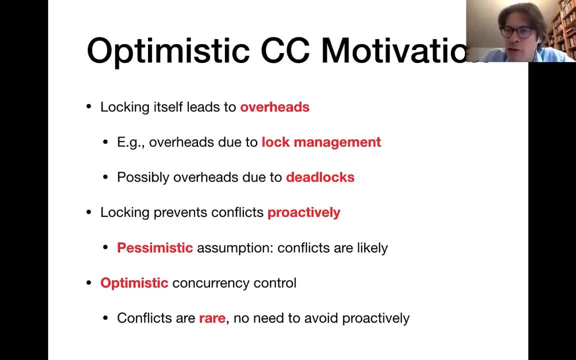 for transactions. they'll probably sooner or later trying to prevent them with payment کو. So transactions will probably sooner or later trying to prevent them with payment کو to write to the same object, or one transaction tries to read an object written by another transaction. Now the premise of optimistic concurrency control is kind of the opposite. 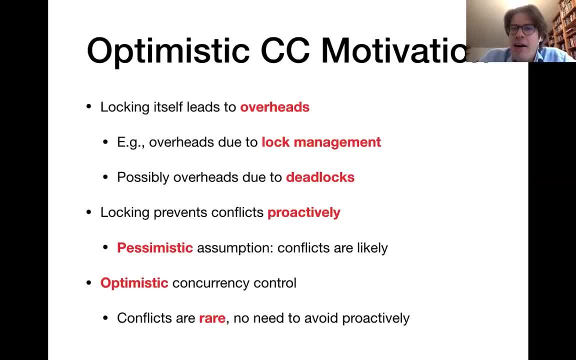 It's saying that those conflicts, they are rather unlikely. So let's maybe just proceed and do things and just assume that nothing bad will happen. Then at the very end, we will verify whether our assumption was actually justified. If it was not justified, we have to pay the overhead. 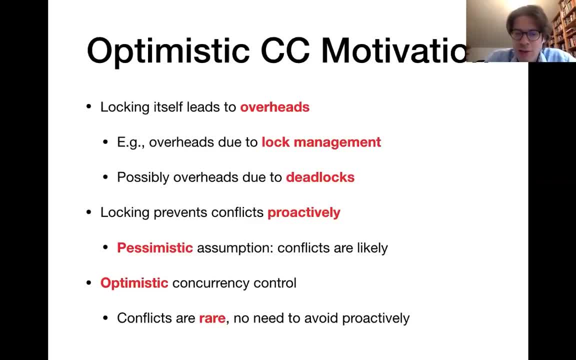 of, for instance, aborting and restarting the current transaction. So with optimistic concurrency control, we essentially trade blocking overheads for potentially higher overheads due to abort. We will discuss about the pros and cons in a little bit, So let's first get some overview. 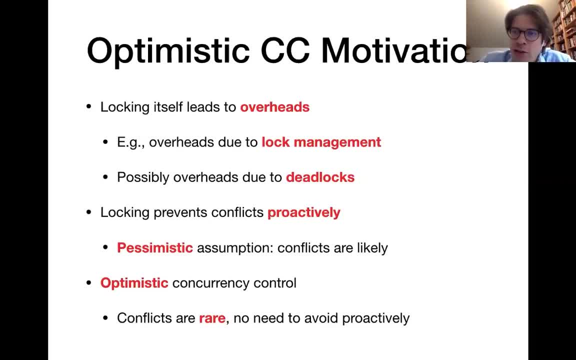 of the current transaction. So let's first get some overview of the current transaction. So let's first get some overview of the current transaction. So let's first get some overview of how optimistic currency control can work. In order to make it work, we first of all need to do some bookkeeping. 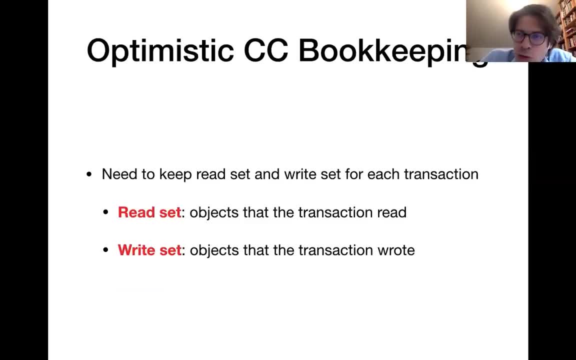 In order to make it work, we first of all need to do some bookkeeping. For each transaction, we need to keep track of the objects that the transaction has read and the objects that the transaction has written. This is what we call the read-set and the write-set in the following. 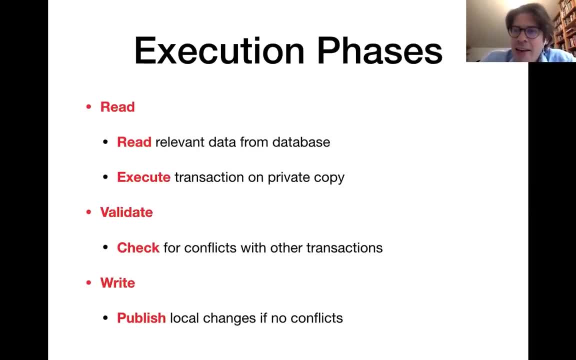 And based on those read and write-set, we can validate whether any bad conflicts happened or not. Now in more detail, the execution of a transaction consists of three phases: First, the read phase, then the validation phase and finally the write phase. What happens in the 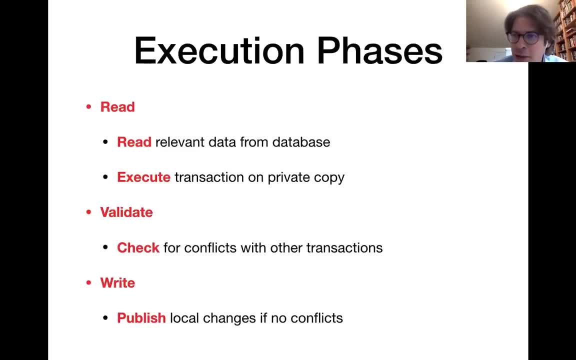 read phase is this: The transaction first of all identifies the objects that it is interested in in the database and then it essentially copies those objects into some private transaction specific memory location. so it gets its private copy of the relevant objects in the database. 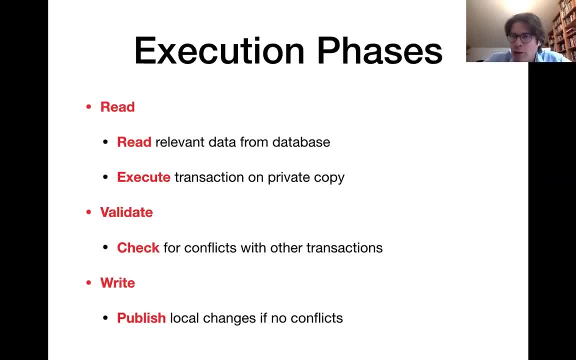 And then it also executes the entire transaction on this private copy of the relevant data. There is sometimes confusion about this phase, in my experience, because the official name of that phase is a little bit misleading, because it's the read phase, while it's the read phase, And that is where the third phase comes into play, And there is quite a few. 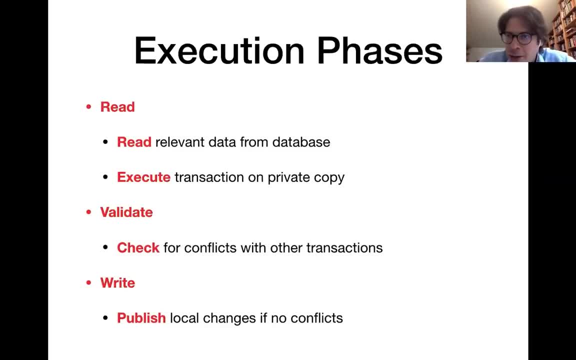 in reality, we're not only reading data, but we are also kind of executing the transaction on the private copy of the database. So read face. that is the official name. that is why I'm using it here, but I noticed that people tend to get confused about that. this is why I want to 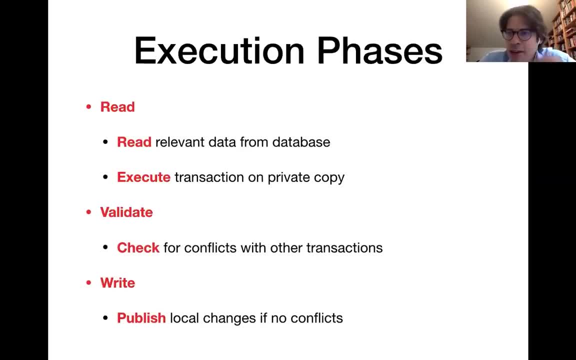 proactively avoid that confusion. So read face means reading the data, but also executing the transaction on a private copy. Now, before we can actually publish the things that have changed in the private copy of the data, we first have to validate in order to ensure that no conflicts. 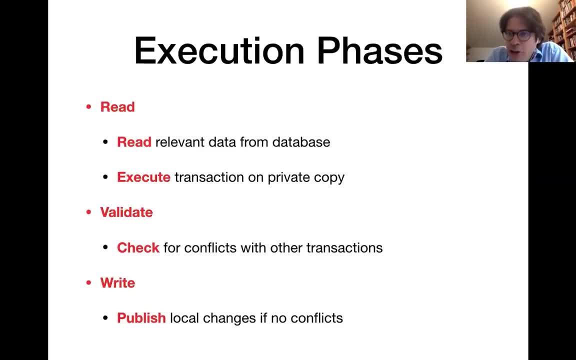 have happened During the validation phase. I'm essentially checking whether any other transactions have accessed the same objects that the first transaction being validated was working on and the other transactions have not been validated. So in this case I'm basically checking the if those changes to those other objects or those accesses to other objects. 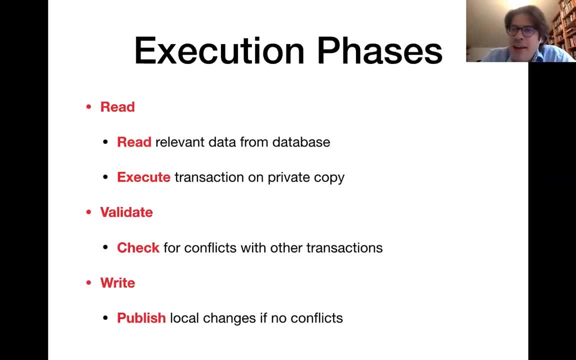 conflict with what my current transaction has done, then I actually have to abort and later restart the current transaction. So this is where optimistic concurrency control is optimistic because it assumes that in almost all cases this validation will check out okay and there haven't been any conflicts in the meantime. Now, if the validation succeeds, then we proceed to. 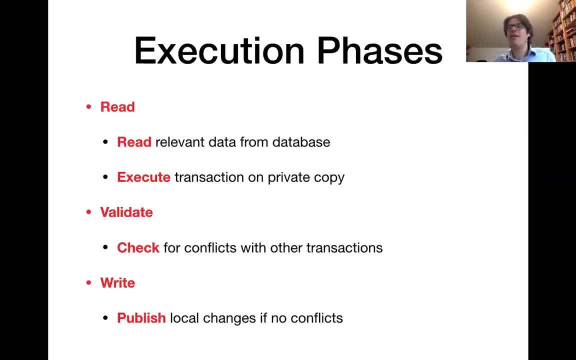 the final phase, which is the write phase, and here we essentially publishing the changes from the private transaction specific copy of the relevant data to the public overall database. So we are writing those private copy changes to the public database where other transactions can see it as well. Well, 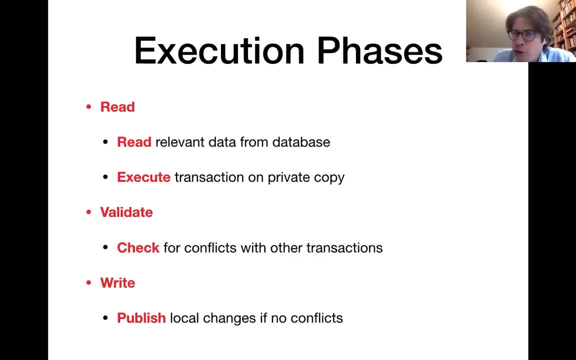 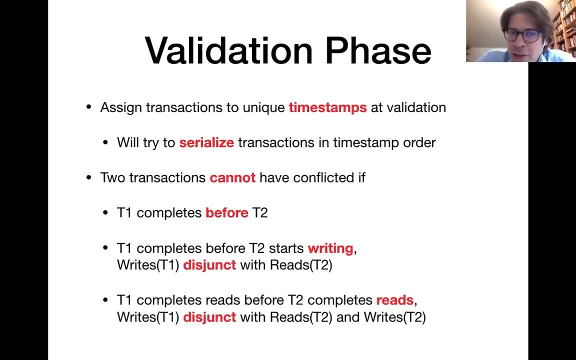 that is the end of the presentation. Thank you very much for your attention. Now we're back to the high-level overview of how optimistic concurrency control works. Let's discuss about the validation phase in a little bit more detail, because that is the key to concurrency: the control- 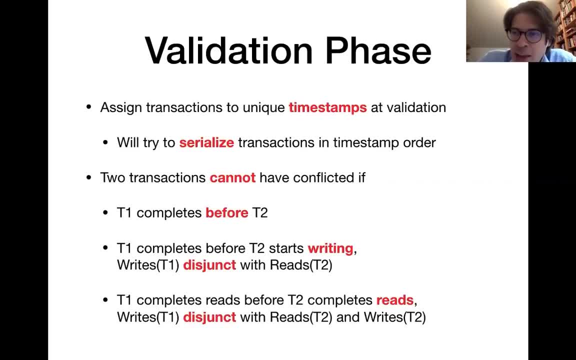 It generally works by assigning unique timestamps to transactions at validation time. So essentially our goal is to create, like serialization order of theSay tuning of a transaction to the server, at that搞던 token, to track Settings and verified items, order of the transactions that is consistent with those timestamps. 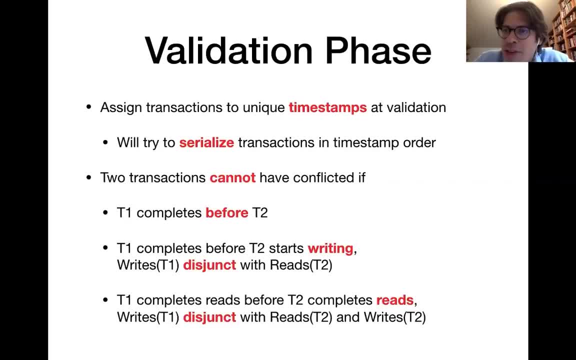 So in the end the database should look as if those transactions had executed in timestamp order And also what other transactions see. which transactions sees the changes from which other transaction. that also should be consistent with those timestamps. During the validation we essentially check a sufficient condition in order to make sure. 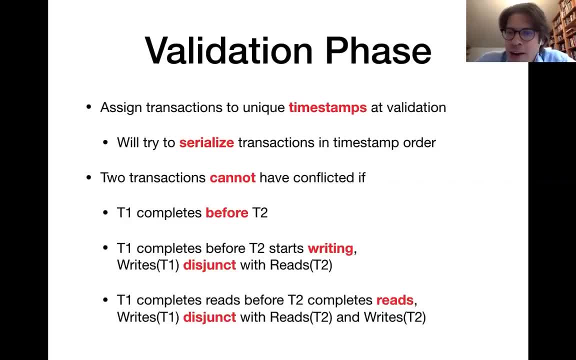 that no bad conflicts between transactions have appeared. Now we can be sure that there was no bad conflict between two transactions, for instance if the first transaction has entirely completed before the second transaction. In that case clearly there cannot have been any conflict. 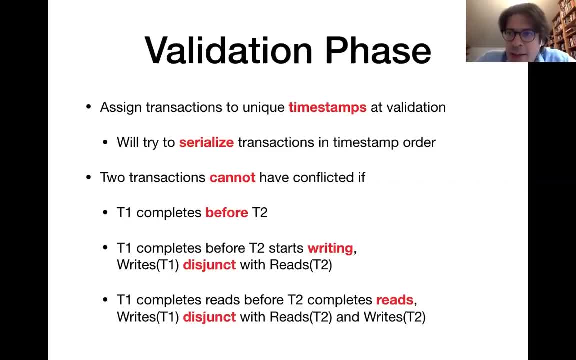 Also, we might refine that and say we also can be sure that there is no bad conflict if the first transaction completes before the second transaction starts writing. Also, in this case what could happen is that the first transaction writes values to objects that are read by the second transaction. 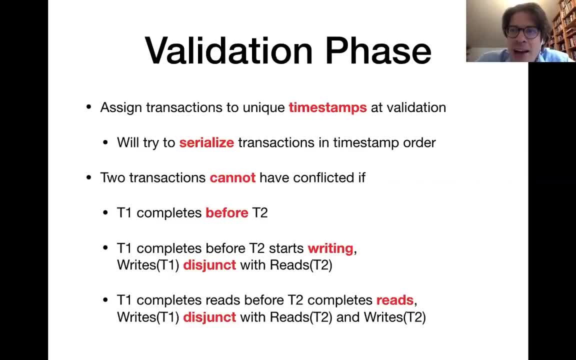 So here there could be some kind of a ban That influence linking the two transactions. But we can be sure that this does not happen if the write set of the first transaction, the object that the transaction has written to and changed, is disjunct with the set of. 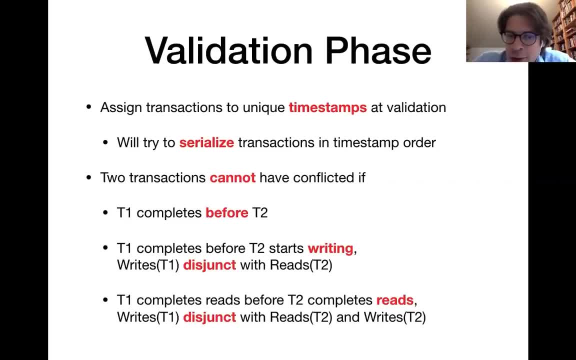 objects that the second transaction has read: So if that holds, then we can be sure that the first transaction hasn't influenced the second transaction. So here both of them cannot have conflict. Okay, So we have conflicted in a bad way. 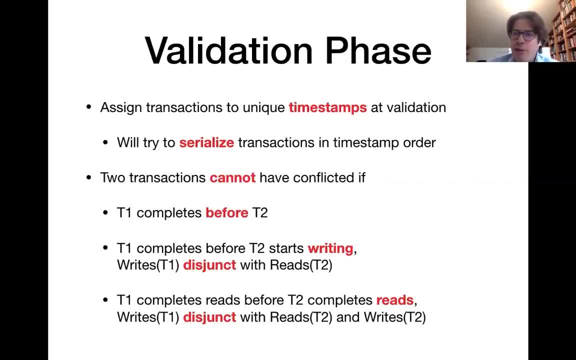 And as an extension of that, perhaps the first transaction completes before the first transaction completes its read phase, before the second transaction completes its read phase. That means that we could, for instance, have overlapping writes in addition to first transaction writing objects read by the second transaction. 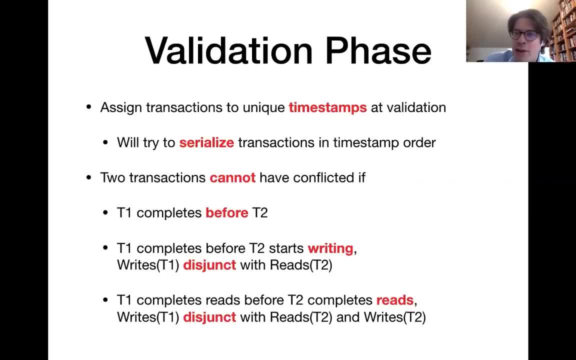 So, as an extension, We also want to ensure that the write set of the first transaction- the objects it has changed- is disjunct from the write set of the second transaction. In that case they cannot override each other's changes in a bad way. 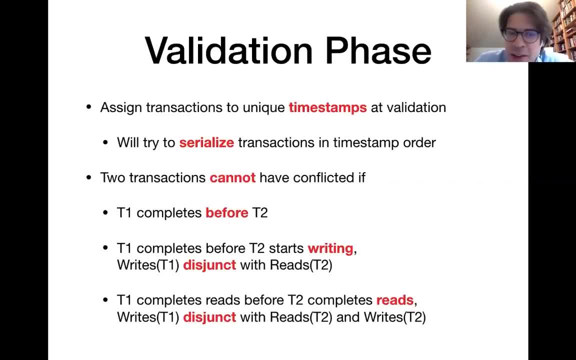 And we can also be sure that no bad conflicts have happened. So those three conditions is what we can verify in the validation phase and if one of them holds, then we can be sure that they have been no conflict. Okay, Those conditions. they are perhaps overly conservative in some cases. 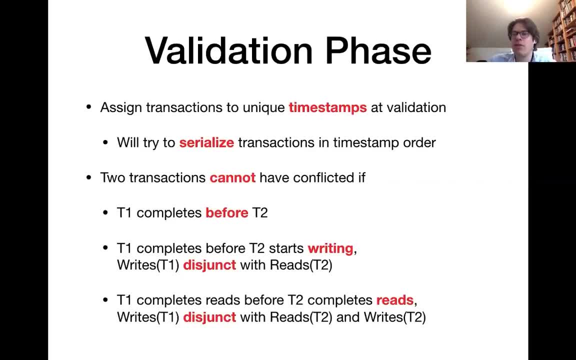 None of those conditions might be satisfied, but still everything would be okay In those cases. well, there's some trade-off between bookkeeping and between the probability that we have to abort the transaction even if there's no real reason for it. 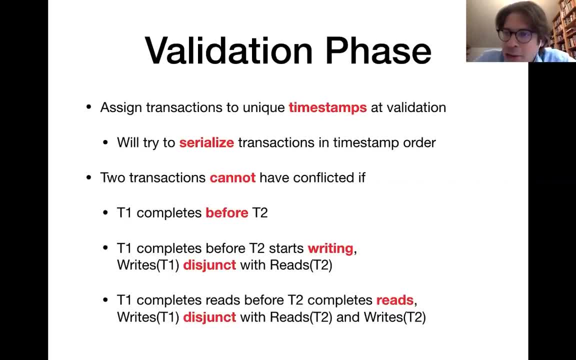 So typically this provides nice trade-off between those conflicting conditions. Okay, Thank you. Thank you All right. Excellent. Thank you very much, Dort. All right, I think it was such an interesting talk and you've had a great couple of questions. 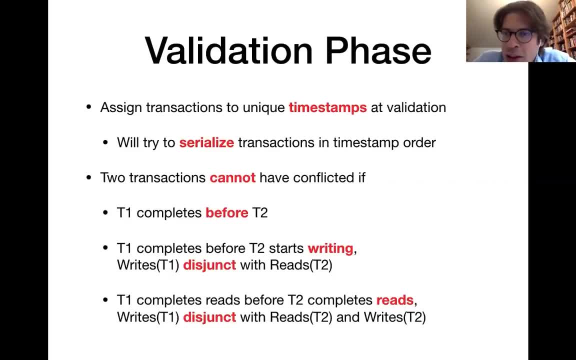 It really goes hand-in-hand with everything that was going to be done last time. You have done an excellent job, So thank you to everyone here, especially the international community, for yoursomething complicated questions that were dressed so nicely on this whole concept of the contribution of faith among the best practices. 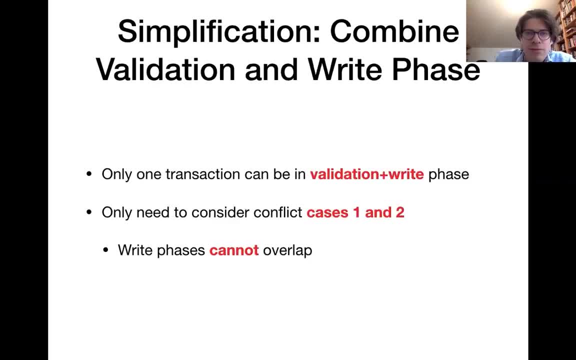 That's too good to hear. the write phase. One simplification that people often make in implementations in practice is that we combine the validation and write phase essentially into one single phase. Then we need to make sure that only one transaction can be in this combined validation and write phase at the same time, So while one 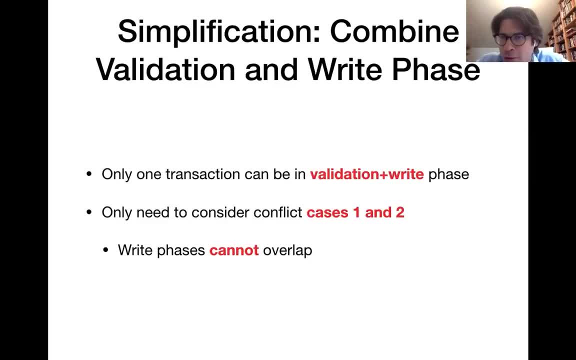 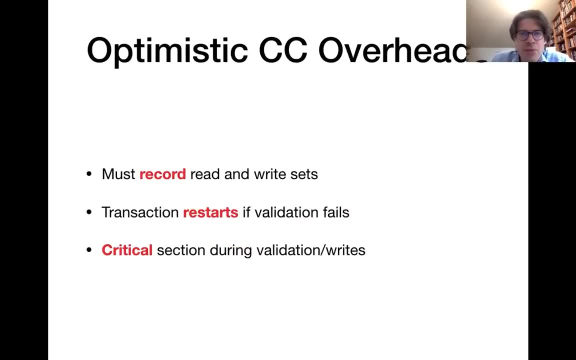 transaction validates and writes, other transactions are blocked from access to the public database. If you do that, the conditions simplify. You only need to consider the first two of them. This is simplification often encountered in practice. All right, of course there are some. 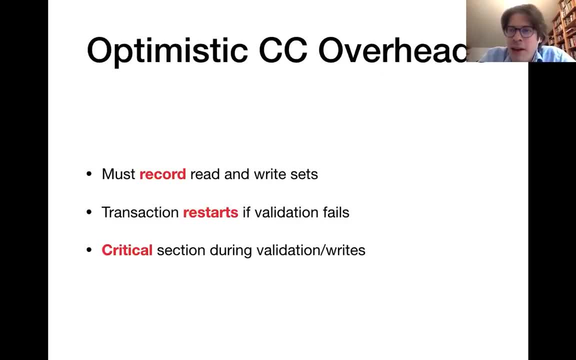 overheads. I'm saving the overheads for locking, but now I need to keep track of the read set and the write set And, of course, if my validation phase does not check out, then I have to restart it. first abort and then restart. 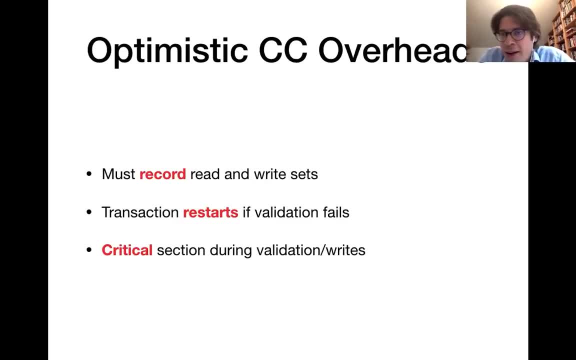 the current transaction And if conflicts are quite frequent, that is a high source of overhead. Also, depending on implementation, there might be a critical section where I reduce concurrency because only one transaction can operate at the same time if it is in this combined validation and write phase. 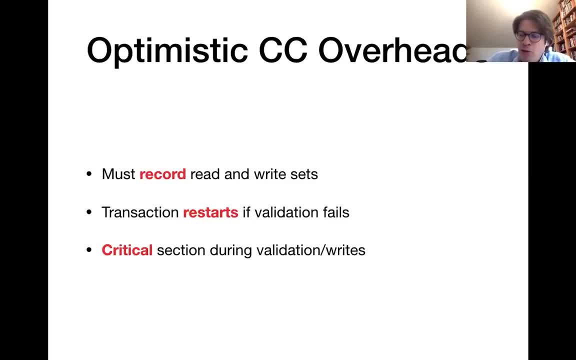 for instance. So the second point is the criticality of this configuration. So if I have two reality-based transactions, I can have two reality-based transactions and other. So there's pros and cons. probably want to use optimistic concurrency control in scenarios where conflicts are rather infrequent. 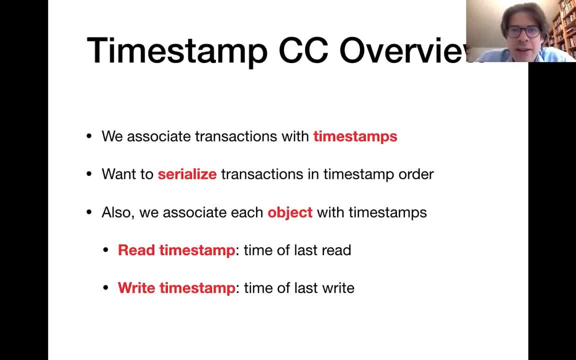 Another non-locking based concurrency control is a timestamp based locking. So here we associate again each transaction in the system with a timestamp and our goal is to serialize those transactions in the order of those timestamps. So the database should look as if those transactions had executed in the order of those timestamps. 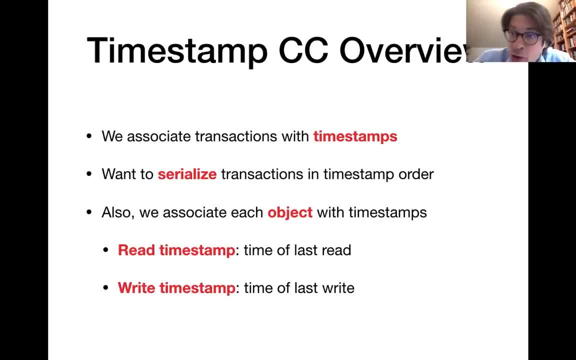 Now we not only associate transactions with timestamps, we also associate objects in the database with timestamps. Each object is associated with a read timestamp, which essentially is the timestamp of the last read operation on it, And with a write timestamp. So essentially those read and write timestamps for objects are set based on the timestamps. 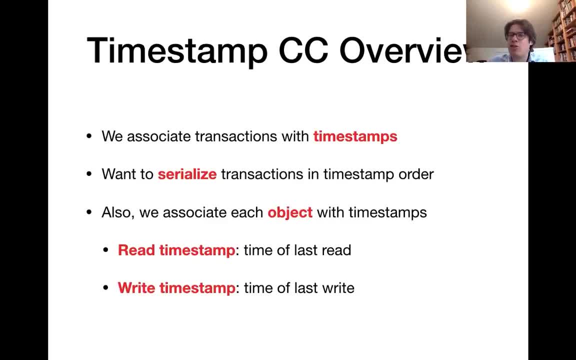 of those transactions. So if a transaction with a certain timestamp reads an object, then the read timestamp of the object is updated to the timestamp of the transaction Because, logically, essentially each transaction executed instantaneously at its time. And this is why we update read and write timestamps from the transaction timestamps. 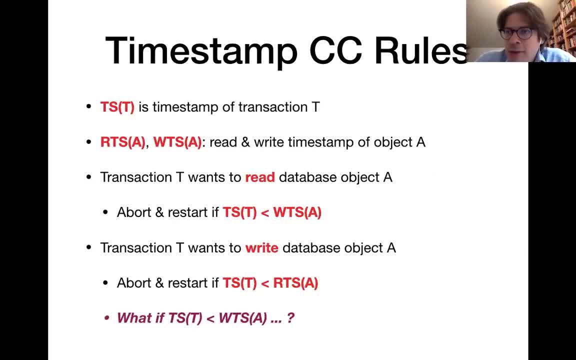 Now we have to essentially check a couple of conditions. whenever a transaction wants to read and write objects in the database, Those conditions essentially tell us whether, if we proceed with an operation, whether we're still consistent. So if we do that, we have to check the read and write timestamps whether we're still. 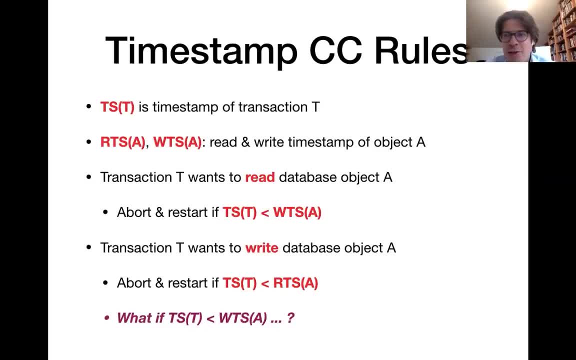 consistent with the timestamp order of the transactions. Now here I outline those rules that we have to verify. And if a transaction tries to do an operation that would violate one of those rules, then this transaction is reported aborted and restarted later. So here we use TSFT. 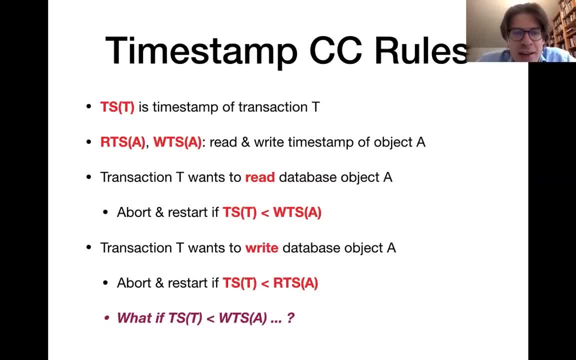 The transaction and RTS of A and WTS of A. those are read and write timestamps of the object A. And now if a transaction wants to read some database, object A, we have to abort and restart the transaction if it's a timestamp is smaller than the write timestamp of the 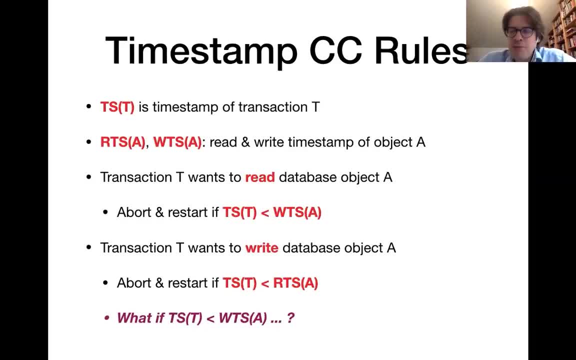 object that it is trying to read: Okay. So logically, this makes sense because of the following: So if a transaction has a certain timestamp, it means that everything should be as if the transaction had executed at that time. And if the transaction had really executed at a specific time, then the version of an 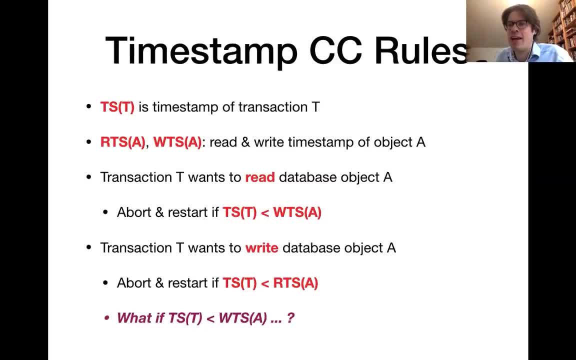 object that it reads must have been written by a transaction that executed before Now. In this case, we see that the object A has been updated by a transaction with a higher timestamp than the transaction that is trying to read. That means if we would allow the transaction to proceed and to reach the current value. 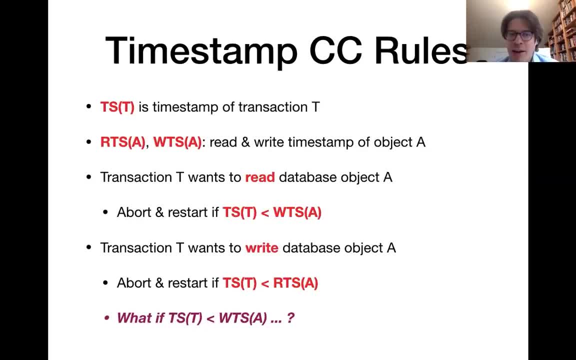 of A, we would be inconsistent with the timestamp order, because the transaction should have read an earlier value of object A, written by a transaction with a smaller timestamp, And because of that, Um, If we have this condition here, it means that we have to abort the transaction trying to 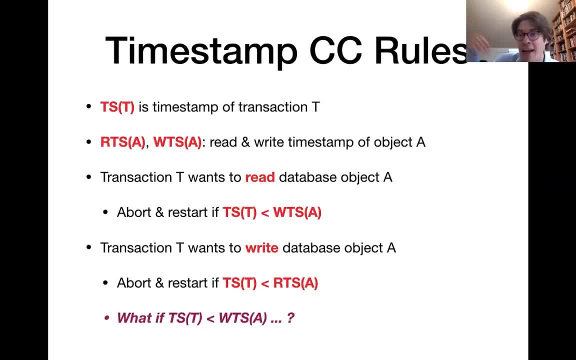 do the read and restart it with a higher timestamp. All right. Now on the other side, what happens if a transaction tries to write an object in the database? So logically, if a transaction executes at a certain time and writes a value for an object, 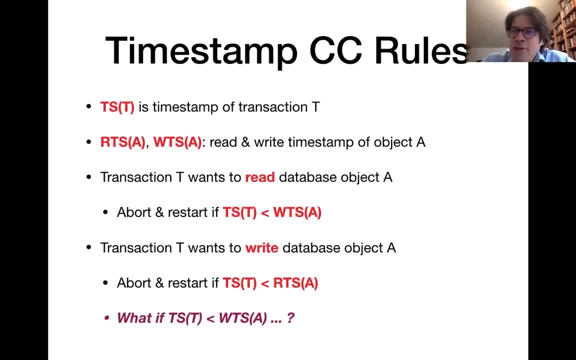 A, Then all transactions that are executing later than the current transaction should read the value written by the current transaction, because then logically it is as if everything had executed in the transaction timestamp order. Now, if we see that the timestamp of the transaction trying to do the write is actually smaller, 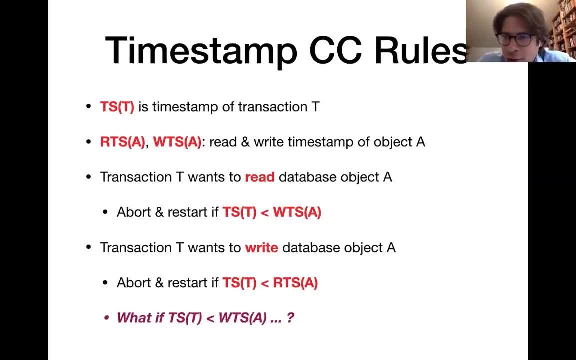 than the read timestamp of that object we are trying to write to Um. Then we see that another transaction with a higher timestamp has already read the current value of object A And that means that allowing the transaction to proceed with the write operation would mean that we are becoming inconsistent with the timestamp order because had the transaction 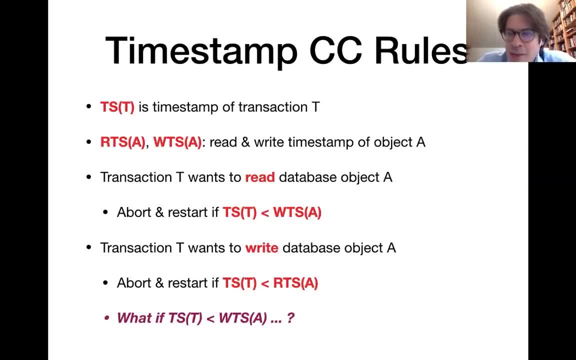 really executed at time t, it would have written the value read by the later transaction, But that has not happened, All right. So one interesting case that we might also think about is what about multiple writes on the same object, And, for instance, we could think about aborting and restarting a transaction if the transaction 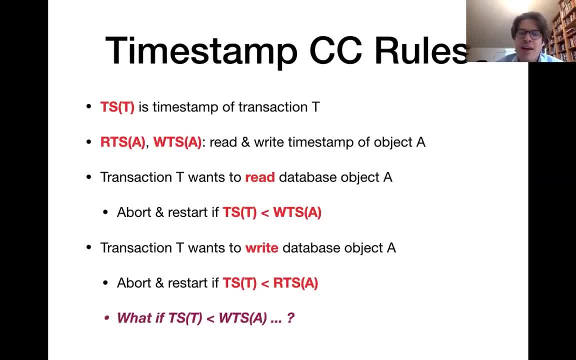 timestamp is smaller than the current write timestamp of that object. So Because, logically, if transactions had really executed in timestamp order, then the final write to object A would have been executed by the later transaction. But here we are essentially trying to override the later value with an earlier value. 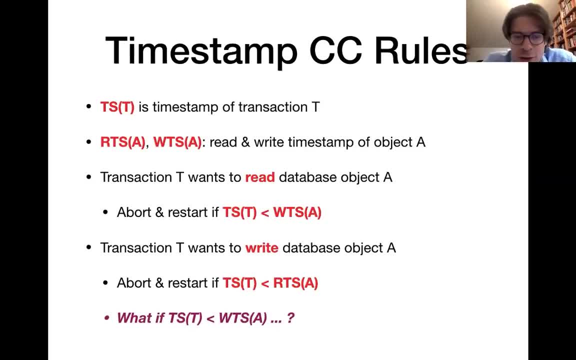 So a naive way of doing this is to just say okay, in those cases the abort and restart the transaction. So a randomหนle would have been executed in that order and we can show that the current write, current timestamp ordering does not succeed. if we would try to restart the 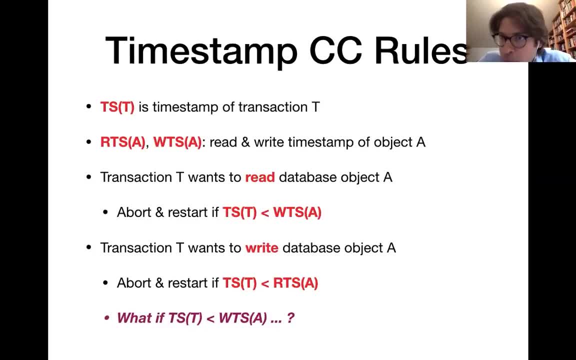 transaction with the original timestamp, we would run into the same problem again. So that's a great point, But what we are doing instead is that we are restarting the transaction now with a higher timestamp, and this is why things change. So, in theory, even with the higher timestamp, we might again have to abort. 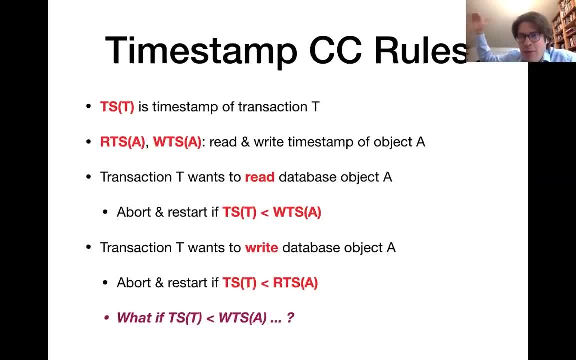 and restart the transaction a couple of times. but at least now we have the chance, with the higher timestamp, that the thing which led to the abort before won't happen again. Great question, And here: okay, that is the question about the case at the bottom of the slide here. 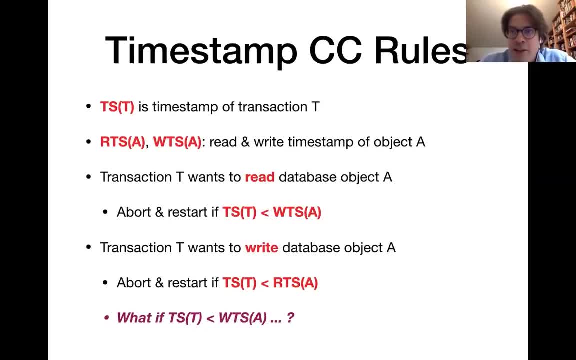 So I already said that one possibility to deal with this case would be to abort and restart the transaction. But since I marked this up and formulated it so tentatively, you can imagine that it might be a different way of doing things, And that is the so-called 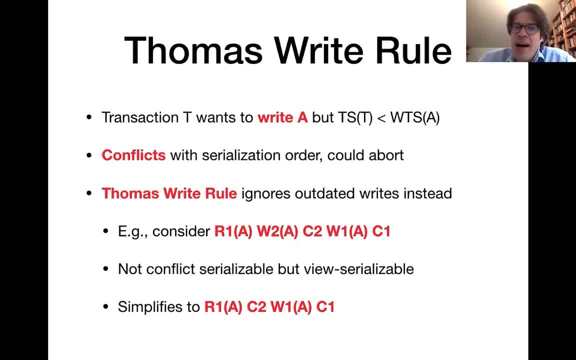 Thomas' right rule. This rule applies in the case that we have just seen, where the timestamp of the transaction trying to do a write is smaller than the current write timestamp of that object, which conflicts with the serialization order. so clearly we cannot allow the transaction to proceed with the write But on the 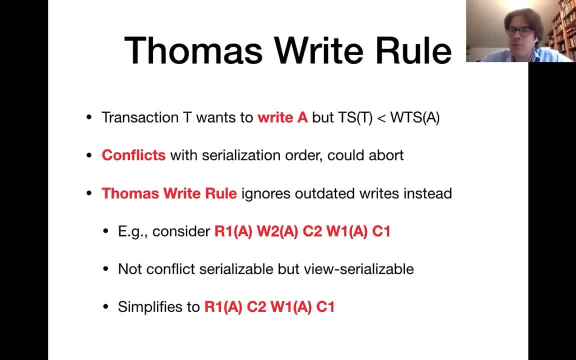 other side. we don't really have to abort the transaction either because we can just say this transaction would have written some value to object A. Analyzing the read timestamp we can see that the value of object A written by the transaction would never have been read, So essentially we can just act as if that. 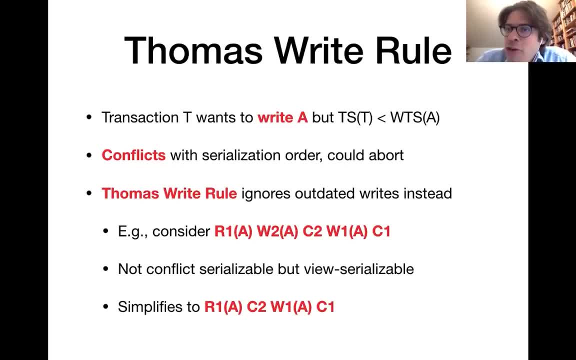 write operation had never happened. So we don't necessarily have to abort the transaction trying to do the write. And that is what the Thomas' write rule is. So essentially it states that we can ignore outdated writes and don't even need to abort. 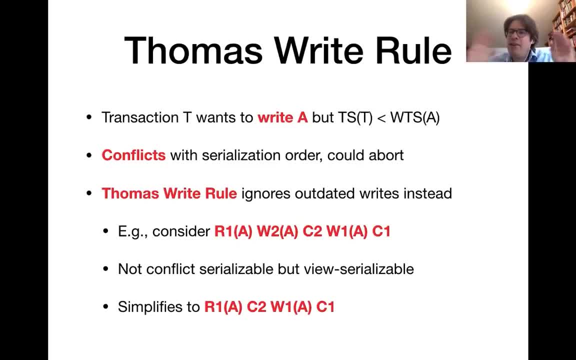 the transaction causing it. So essentially what it does, if you consider it from the perspective of the schedules that it allows. if you look, for instance, at this first schedule here, marked up in red, every read to object A by transaction A. 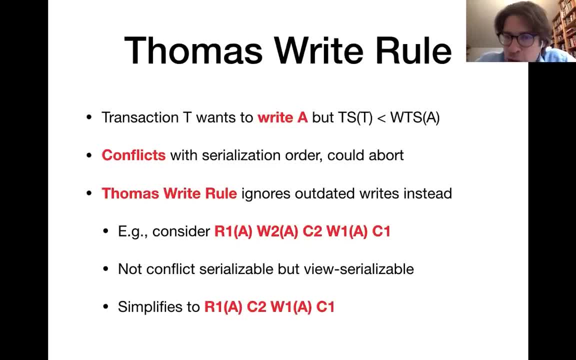 So essentially it states that we can ignore outdated writes and don't even need to abort the transaction. So for example, if the first schedule is read by transaction A, by transaction one, followed by a write by transaction two on the same object, then transaction two commits And now I have still a write of transaction. 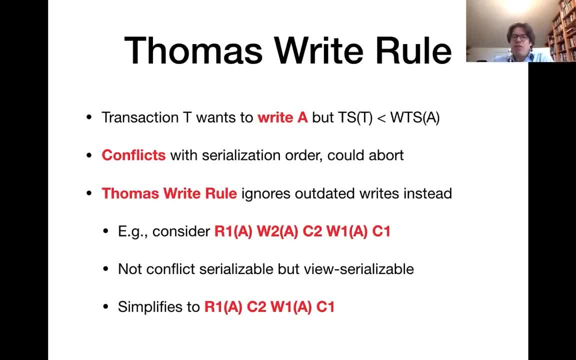 one on object A. Now, first of all, this schedule is not conflict-serializable, because here, if you see it, we have a conflict on object A, between transaction one and two, so the corresponding graphic would have an edge from transaction one. 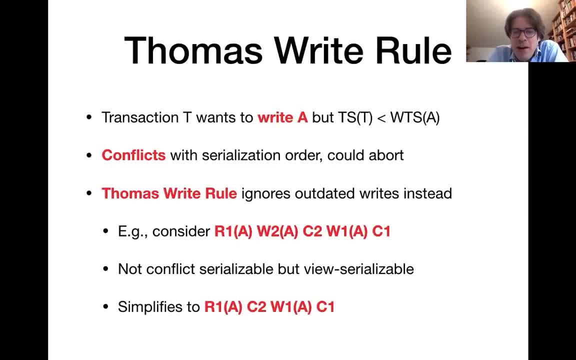 one to transaction two due to the read followed by the write, and also we would have an edge from transaction two to transaction one because of the write, followed by the final write by transaction one. So we have a cycle and that means this schedule is non-conflict serializable. 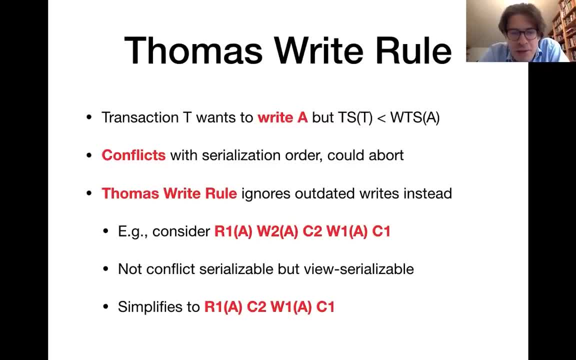 But on the other side it would be view serializable, because here the final value of object a is written by transaction one and transaction one also reads the original value of object a. So this write by transaction two to object a is kind of pointless. It is not read. 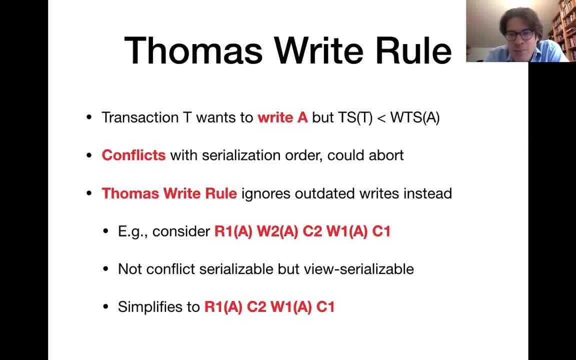 by anyone and it is changed again later by the first transaction. So actually we could kind of act as if that write to object a had never happened, And at the bottom you see the corresponding schedule. So here we just remove this write operation which doesn't. 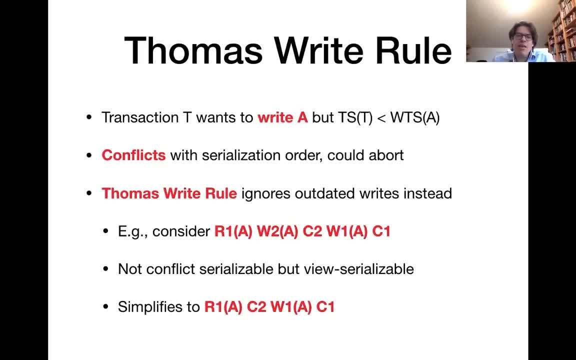 really have any effect whatsoever, And here we end up with a schedule that is serial. So actually we could move the commit by transaction two even before to make that more clear. But clearly a transaction two doesn't have any operations anymore. Here you only have a read by transaction. 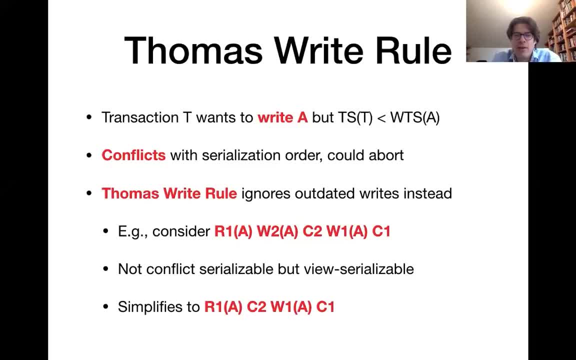 one followed by a read by transaction two. So we have a read by transaction one followed by a write of transaction one And those two schedules are view equivalent And the Thomas write rule essentially allows us to capture such cases to avoid abortions and restarts in cases. 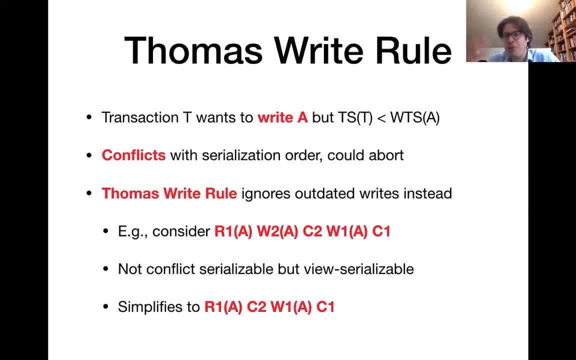 where writes don't really matter. So that is an optimization to the simple handling strategy that we have discussed before. But what if w to a affected different rows in a than w1 of a? And the thing I think there's a misunderstanding about, like, basically, which types of objects we are granting those locks for. 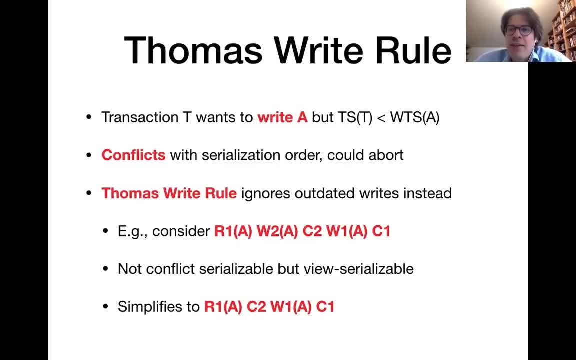 So that's a great question. So here we essentially assume that those objects- a- they refer to things like that- could for instance refer to one's single row. So here we are not considering multigranularity locking, We're only considering atomic objects in our database, which typically are rows. So here a that could for instance be: 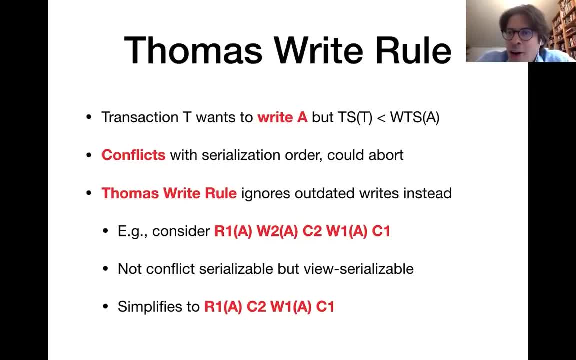 the row in your accounts table which represents the account of one specific customer, of Alice, for instance. right? So we don't consider multigranularity locking So each if we have two operations on the same object a, it means that they refer to exactly the same object in the database. 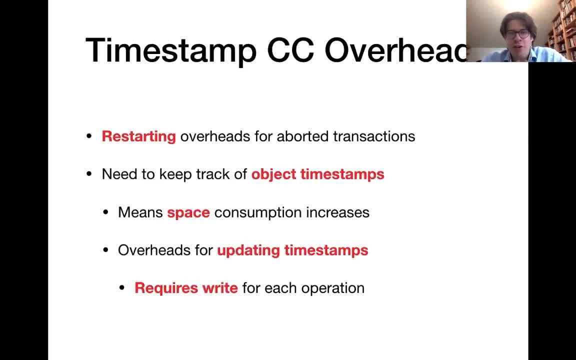 All right, good. So for timestamp concurrency control we also have a couple of overheads. like for the optimistic concurrency control, we also might have overheads due to restarting and aborting transactions in case of conflict. Also here we need to keep track of object timestamps. 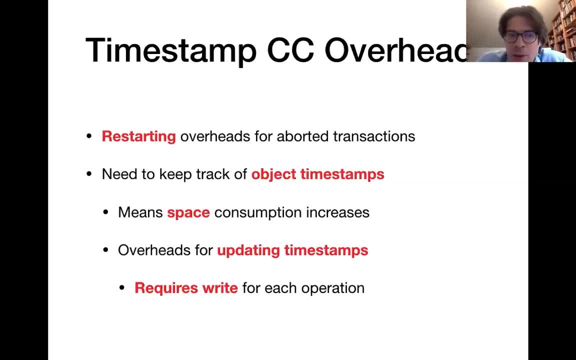 We need to keep track of the read and the write timestamp for all objects in my database and, depending on the granularity- if you're talking, for instance, about a single rows, which is typical, then having to store some values to timestamps for each of those rows. 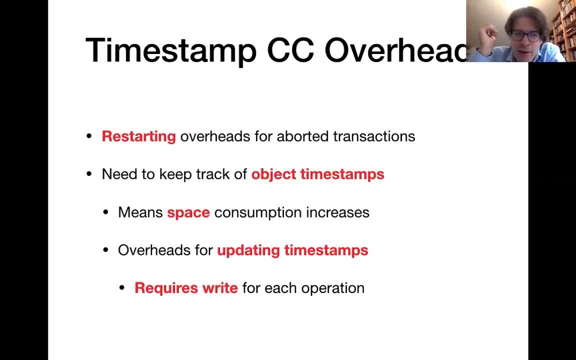 that could actually mean a little bit of space overhead. also, there is the overhead of updating those object timestamps, because for everything to work correctly, we actually we need to keep track of those timestamps, might have to recover them, for instance, during a recovery operation, which we will discuss, uh, quite soon, um, and also 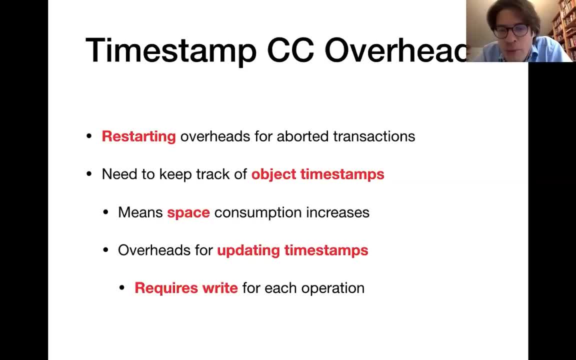 if you're just reading an object, if a transaction is just reading an object, then still we have an associated light operation because we need to update the corresponding timestamp and that means that we have quite a bit of additional overheads. um, especially because of the last point, because 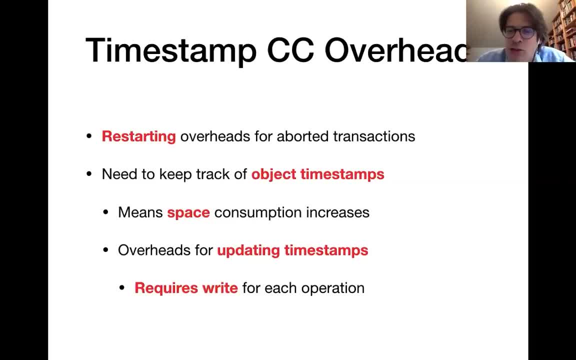 now every object axis essentially transforms into a right operation and better using this is a good idea. in practice it depends again on various factors. but, um, those overheads, they make it a little bit more complicated and they can also be more complicated. and, uh, people in the room can. 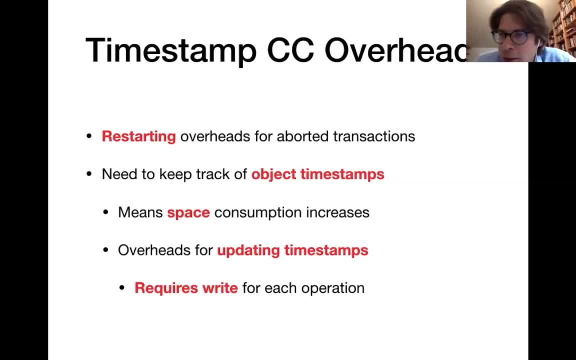 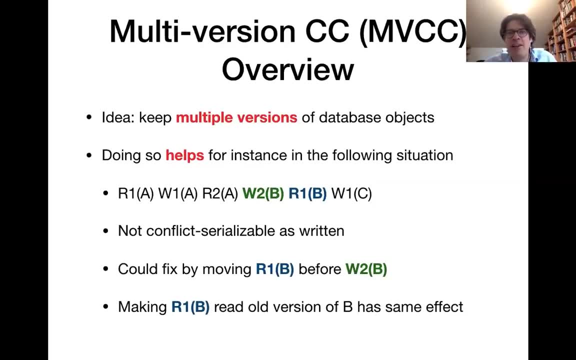 bit less attractive than some of the other concurrency control methods. All right, So we might not finish completely with multiversion concurrency control anymore, but I already want to give a little intro there. As the name suggests, the main idea of multiversion concurrency control is that we keep around. 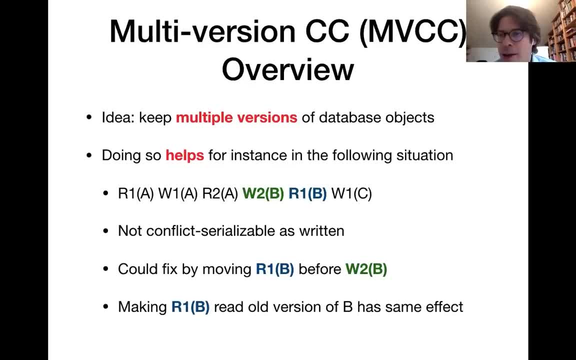 multiple versions of each object in the database. So the protocols that we have seen so far: they would assume one single value for an object in the database. Here we have multiple versions that are associated with different timestamps, And this example here shows why doing that can be a good idea. 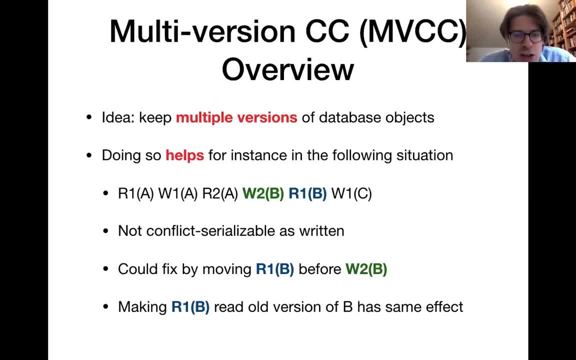 Here, for instance, we have a schedule which is not conflict-serializable in the way in which it is written. So we have an edge in the conflict graph from transaction one to transaction two because of the write to A, followed by the read of A by the second transaction. 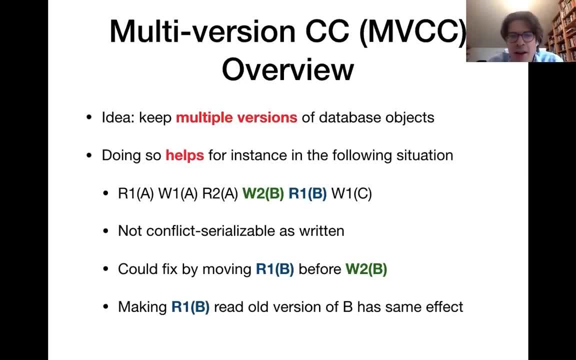 And we also have an edge from transaction two to transaction one because of those conflicting writes and reads on object B And those two are marked up in green and blue in this schedule. Now we could make- We would have- a conflict-serializable schedule had the read on object B happened before the 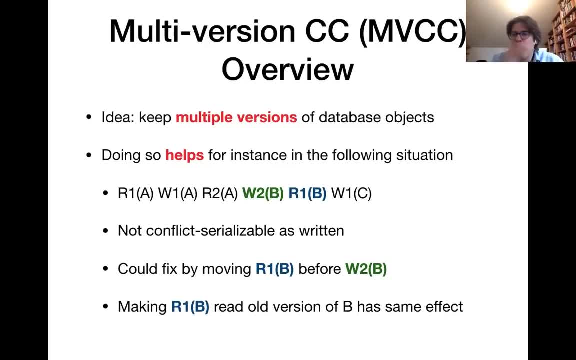 write to object B, So if those two would be swapped. So in order to essentially get there, what we could do is that, when having the read on object B, we just show to the requesting transaction an old version of object B, because the read: 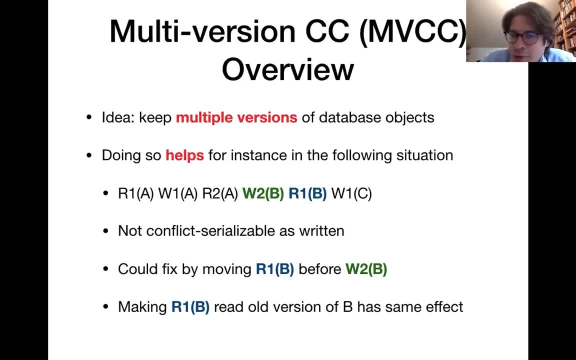 on object B is already there, And then we would have a conflict-serializable schedule in the way in which the read on object B happened before the write by the second transaction. So keeping around those multiple objects and choosing which version to show to a transaction. 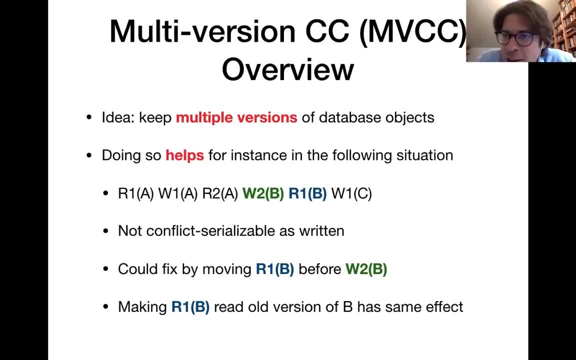 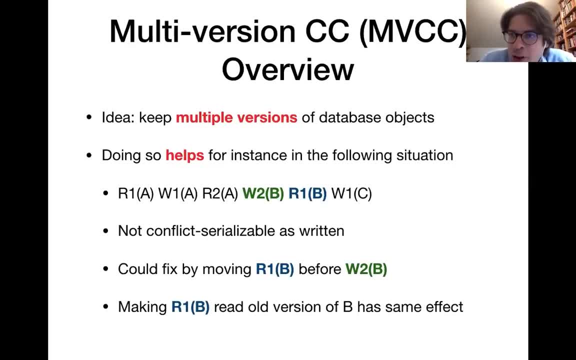 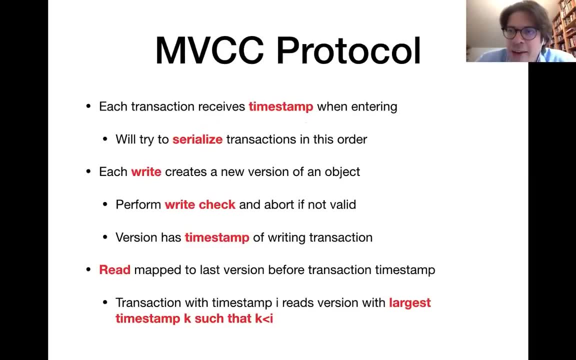 you have to include multiple version of an object B. So if we want to keep multiple versions of an object B, which is also associated with overheads, All right. So here again, we assign timestamps to the transactions once they enter the system. 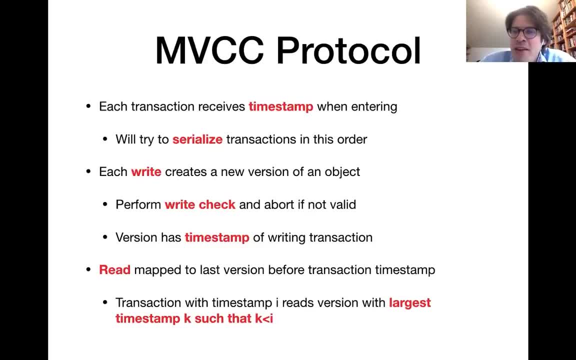 In the next time we will see in more detail how we check whether transactions can proceed and how we decide which version of an object B is needed, And I just wanted to tell you that that knowledge is very valuable of an object to show to a reading transaction. 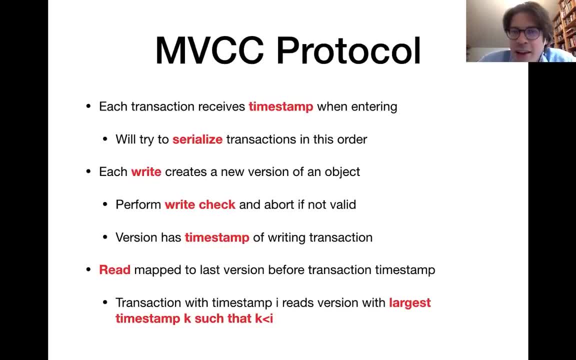 So we're gonna discuss that in more detail next time, But the main idea here is to keep around multiple versions of an object, and that can help to resolve certain conflicts where other protocols would have to abort the corresponding transaction. All right, thanks, And I see you again next week. 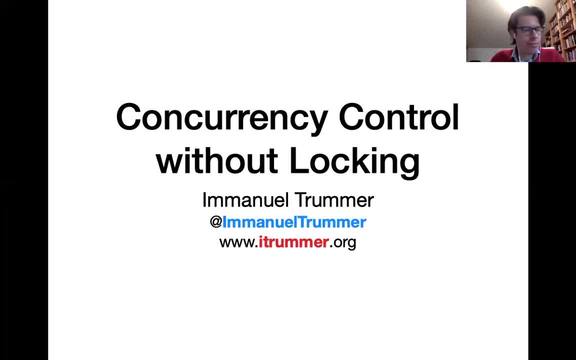 Have a great evening. All right, let's get started. So today we first of all gonna discuss a little bit more about concurrency control, And for the past couple of lectures we have been mostly discussing about concurrency control methods that use locking, And in the last lecture we have started discussing 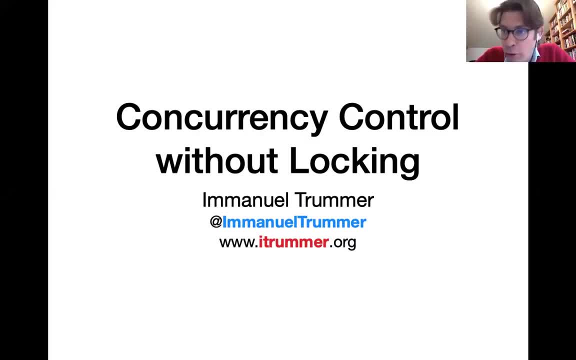 about a concurrency control methods that work without locks And, depending on the scenario, that can have performance advantages, because we saved the overhead for lock management The last time. we have already discussed two of them First of all- oops, I cannot advance the slides here. 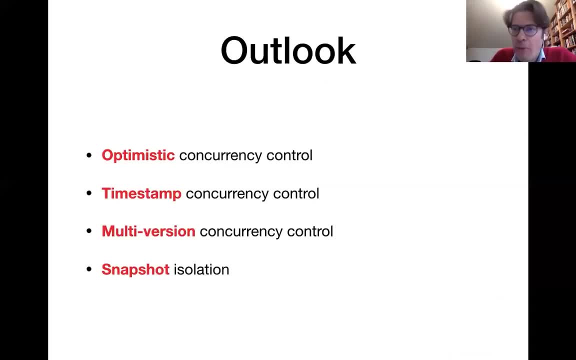 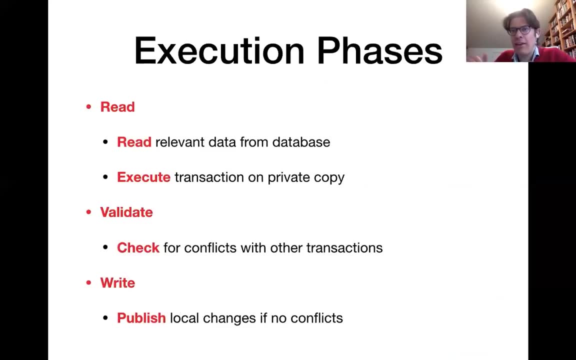 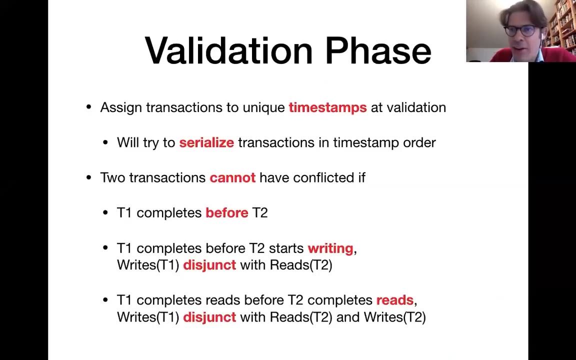 All right. so first of all, we have been discussing about optimistic concurrency control, which essentially assumes that everything goes well and then checks at the very end, And if it is wrong we have to abort and restart the transaction, but otherwise it is very efficient. 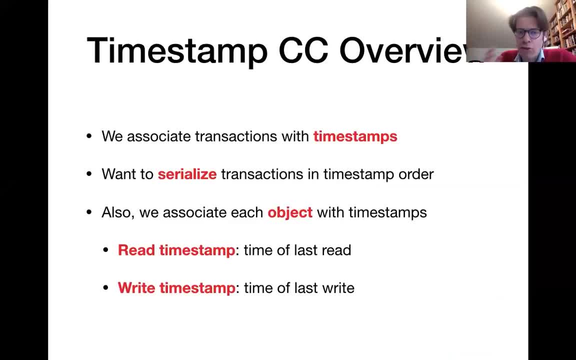 Then we have talked about timestamp based concurrency control, that we essentially associate objects with timestamps indicating when they were read or written for the last time And those object timestamps are based or are derived from the timestamps of the transactions. We assign them to timestamps at the beginning. 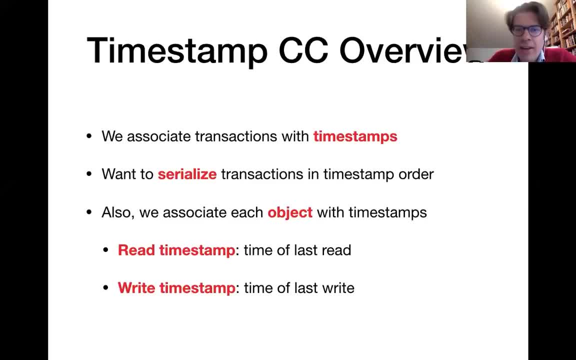 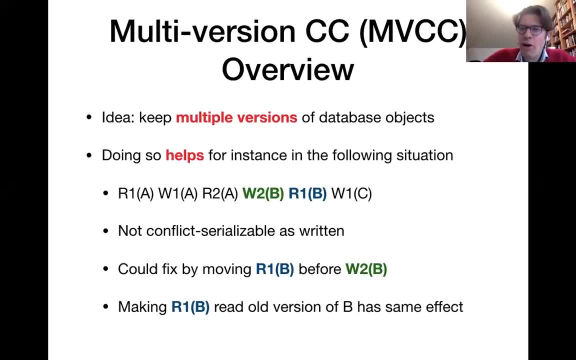 and then we try to simulate an execution In that timestamp order. Now, in the following we're gonna discuss about two more concurrency control methods that work without locking, And both of them actually use a different object versions. We have quickly discussed this slide last time. 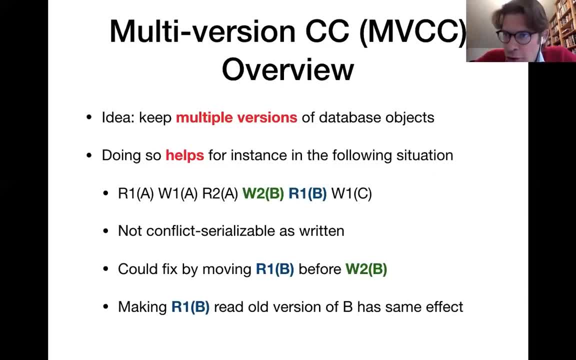 I'm gonna start here again, And the concurrency control method that we will discuss about is called multiversion concurrency control And, as the name suggests, the main idea is that instead of one version of an object, we might have a multiple. we will keep multiple versions of an object. 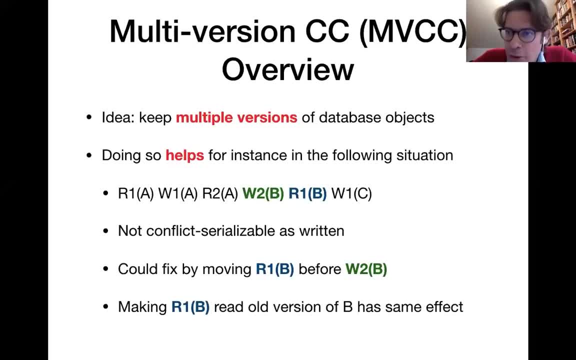 that are associated with timestamps And to see why that can be helpful. we have a little example over here. So if you look at the schedule, at the schedule that is marked here in the three line, in the third line we have a non. 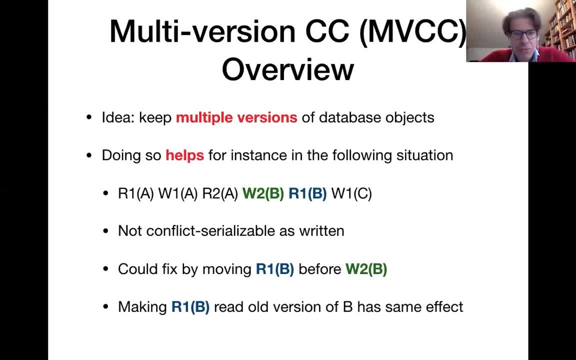 non-conflict, serializable as schedule. There is a conflict between transaction one and two on the A object at the beginning, So in the conflict graph you would have an edge from one to two, And later there is a conflict on B as well. 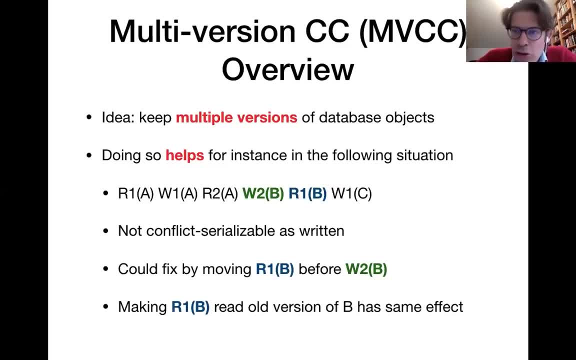 So in the conflict graph we also have an edge from transaction two to transaction one And that is why you have a cycle, So it is non-conflict serializable. Now, this would not happen had we read the B object a little bit earlier. 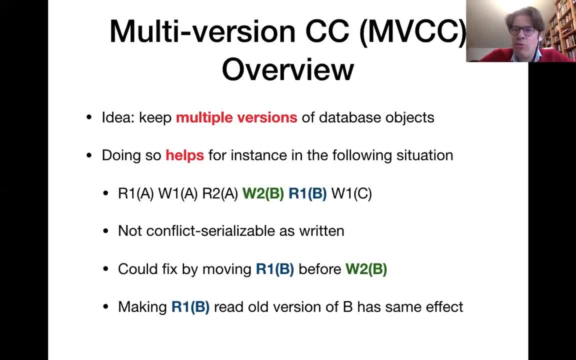 for the first transaction. So if you imagine that we are moving this read of B by transaction- one which is marked in blue a little bit earlier- then we wouldn't have the cycle in the conflict graph, And maintaining multiple versions of objects B gives you essentially that possibility. 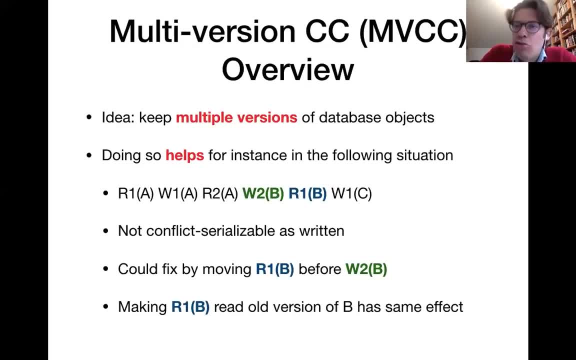 because once transaction one is requesting to read an object from B, in that case we could just serve it the previous version of object B before the write by transaction two has happened, And because this is the conflict that is causing the cycle in the conflict graph. 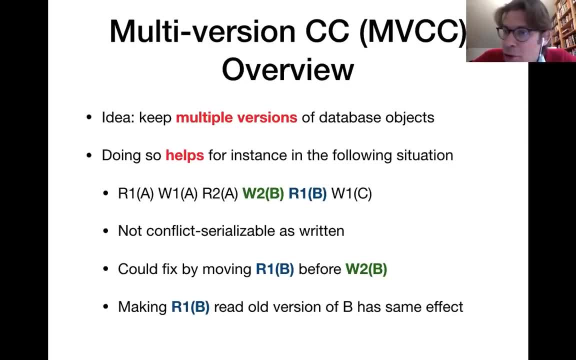 if we resolve it, we get a serializable conflict graph, And if we resolve it, we get a non-conflict serializable schedule again right? So that is the idea behind the multiversion concurrency control: We essentially eliminate conflicts by serving all the versions of an object. 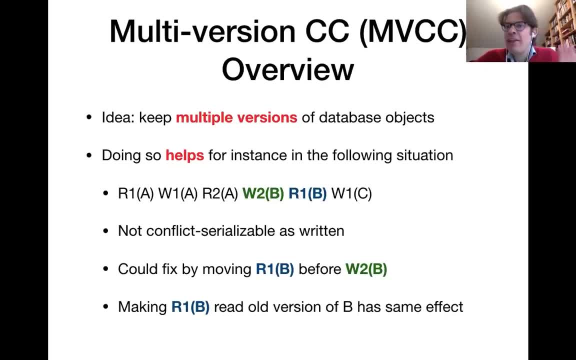 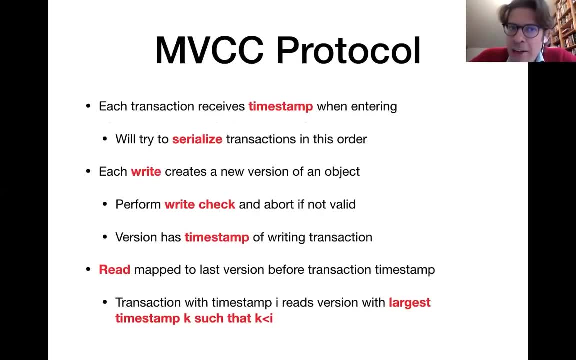 which of course requires us to keep around those multiple object versions. So this is the high level outline of the multiversion concurrency control protocol. First of all, each transaction gets a, B. This is a time stamp when entering the system. That's a unique time stamp. 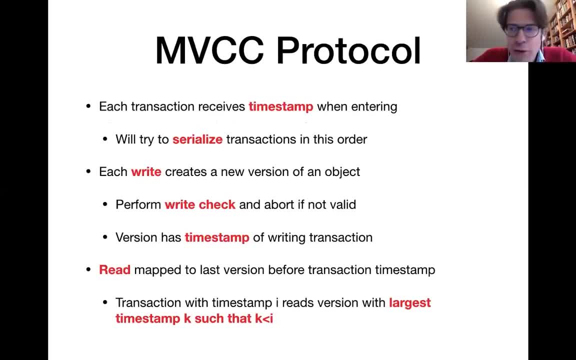 And we try to make everything look as if those transactions had executed in the order of those time stamps. Whenever a transaction writes an object in other concurrency control protocols, it means that the old value is overwritten by the new value. But in this case, here. 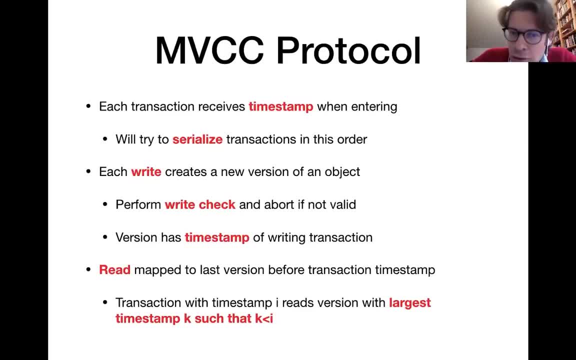 it means that a new write creates a new version of an object. First of all, before the transaction is actually allowed to write something, before we allow that to happen, we perform a check which I will describe in more detail on the next slide. 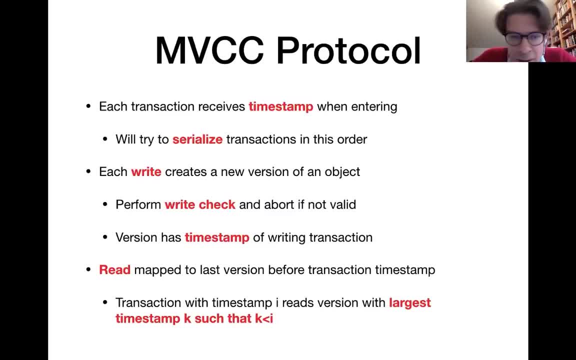 If the check fails then the transaction actually has to be aborted. But if the check succeeds, then the transaction proceeds and it creates a new version of the object And the creation time stamp of that version that is equal to the time stamp of the object. 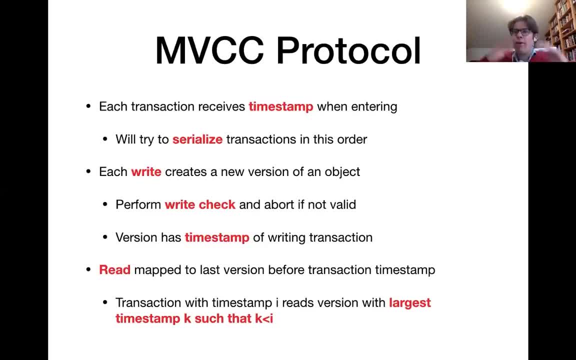 That is equal to the time stamp of the transaction Because, logically, we want to make everything look as if each transaction had executed precisely atomically at its timestamp And therefore, if the transaction had really created the object, then it should get the timestamp of the transaction. 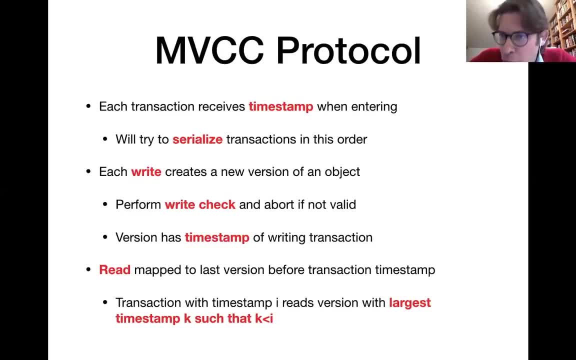 Whenever we have a read, we can exploit the fact that we have multiple versions, So we choose which version we want to show to the transaction. Whenever a transaction that has timestamp i tries to read an object, then we solve the version of the object. 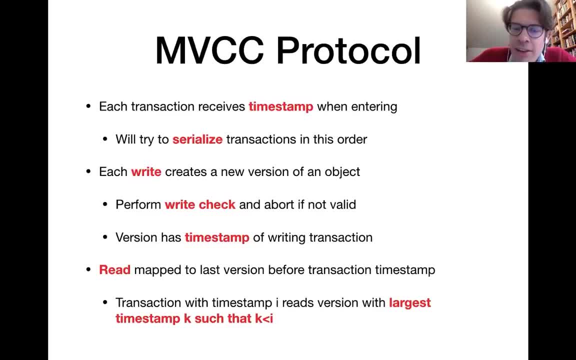 that has the largest timestamp, which is still smaller than i. And that is logical, because if transactions had really executed at their timestamps, then of course the transaction with timestamp, i would see the last written version of the object, And that is just the version of the largest timestamp. 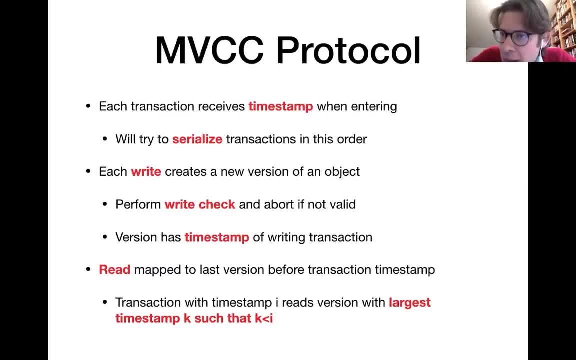 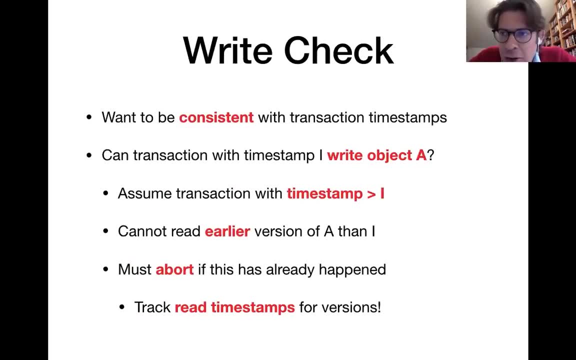 that is still smaller than the transaction timestamp. i All right Now. I have mentioned the write check on the last slide, And this is a test that we do whenever transaction tries to write an object. As always, we have to be consistent with the timestamp order. 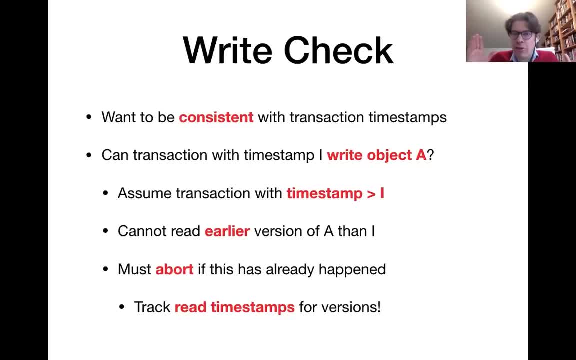 of the transactions. So now let's assume that a transaction with timestamp I wants to write to an object A. Now, logically, if there is another transaction with a higher timestamp than I, then that other transaction, when reading object A, should have read the version written by transaction I, or even a later version. 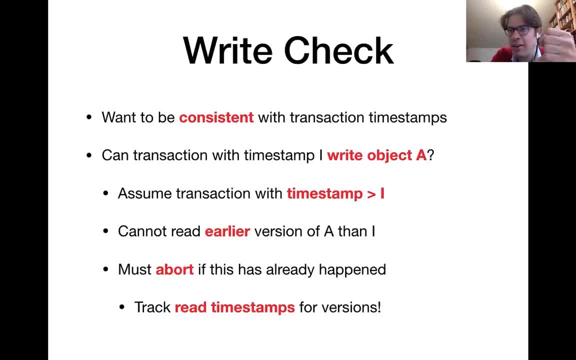 But for sure it wouldn't have read an earlier version because at the time I, the transaction which is currently being checked would have written the object with a timestamp of I right. So here, basically, if you find out that it is currently a transaction with a higher timestamp than I, 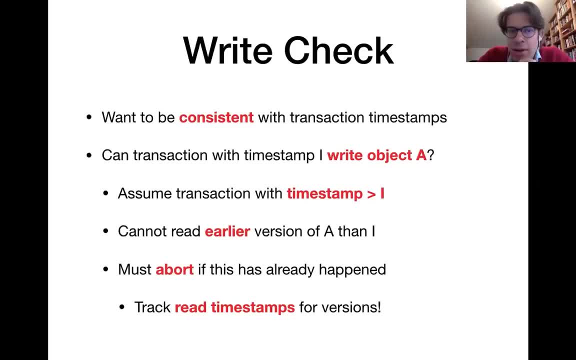 then that version has already read object A. Then we must abort the checked transaction, because if it had written the object at timestamp I, then the later transaction would have read that value or a later one. So if we would allow the transaction to proceed it creates an inconsistency. 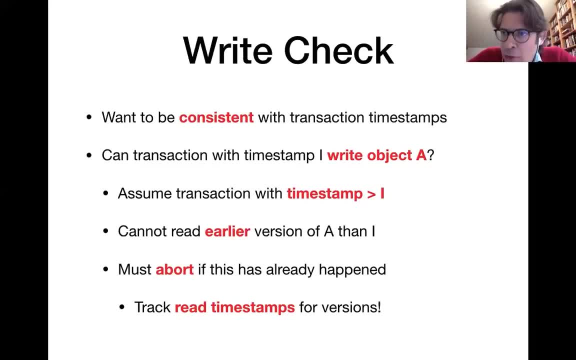 Alright, so that is the write check, and we perform it whenever a transaction tries to write an object. And in order to perform it, we need to not only keep track of the time at which objects are created, but also we have to keep track of the last read timestamp for an object. 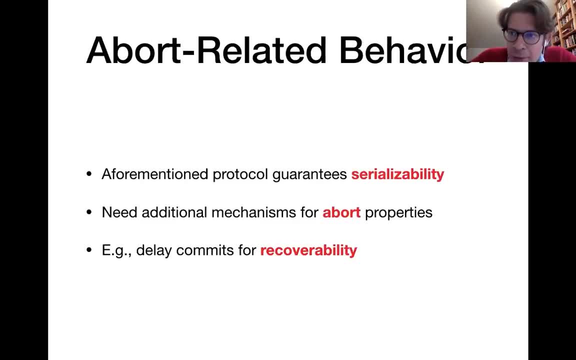 Alright, so what we have seen so far? it serves to create conflict-serializable schedules. We have seen in the last lectures those two hierarchies for schedules. The first one was about serializability, The second one was about abort-related properties. 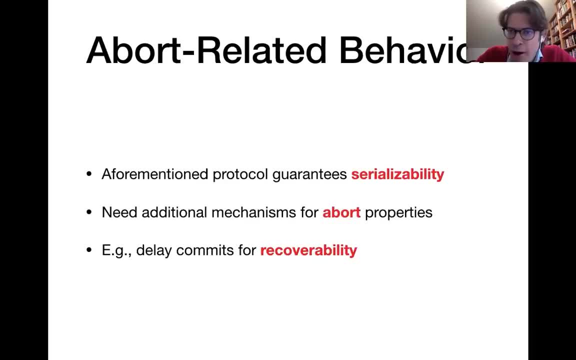 So what we have seen so far for multiversion concurrency control- essentially only this- deals with serializability, but it doesn't give you any abort-related properties, For instance. one important property is that the schedule is recoverable because we don't commit a transaction before other transactions. 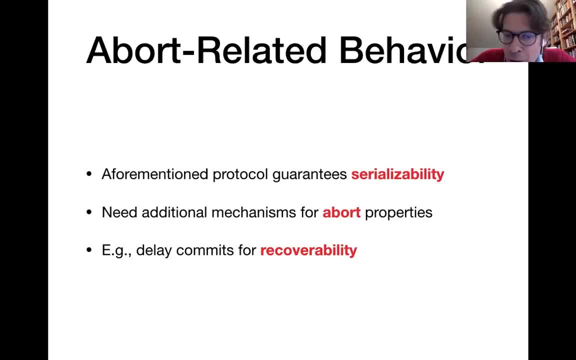 It has been. It has been influenced by have committed before, And the protocol we have seen so far does not yet take care of those properties. In order to get them, you can, however, extend the protocol and, for instance, delay commits until all influencing transactions have committed. 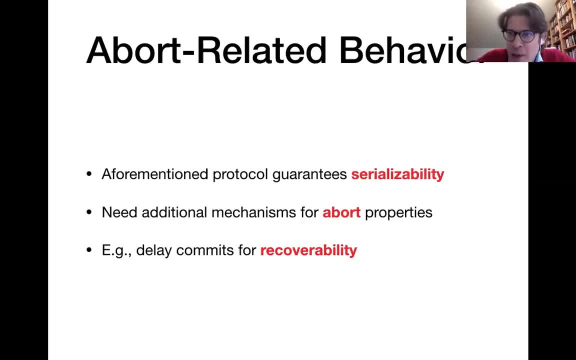 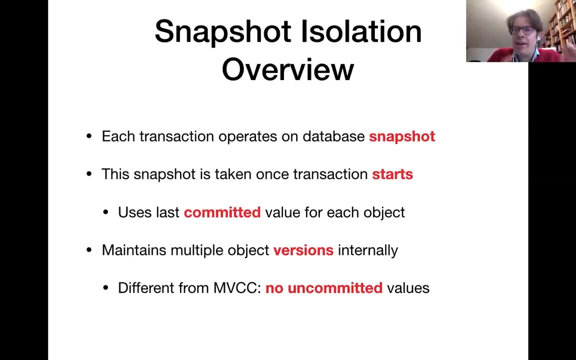 So just so you know, if you ever choose to implement it, then you probably want to take care of those properties as well, and that requires some extensions to the protocol. So that was a short overview of a multiversion concurrency control, And now we are going to see a little bit of a different variant of that. 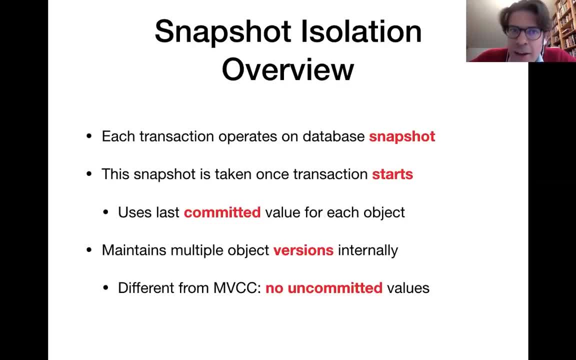 which is also very commonly used in practice, and that is called snapshot isolation. Now, snapshot isolation essentially means that whenever a transaction starts, we are conceptually taking a snapshot of the database which contains, for each object, the value of the last committed transaction. 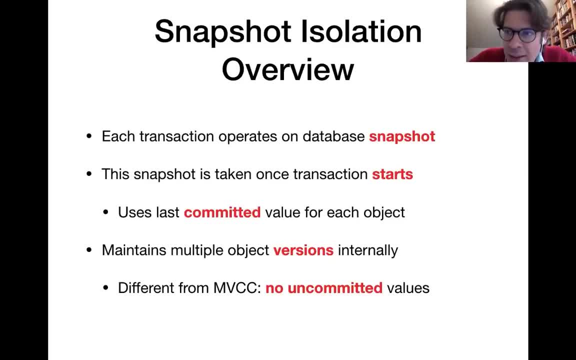 And then those transactions. they essentially operate on this frozen snapshot. So in a way here we also keep around multiple versions of the database, But whenever a transaction starts then it gets this frozen snapshot of the database, which doesn't change over time. 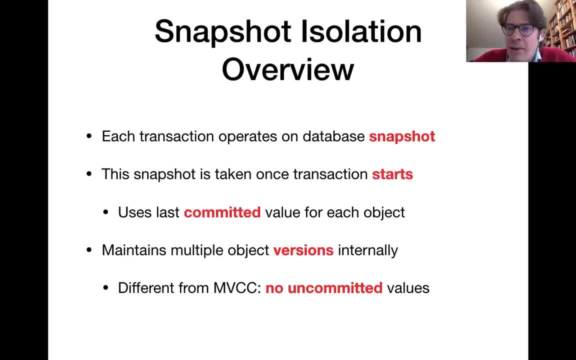 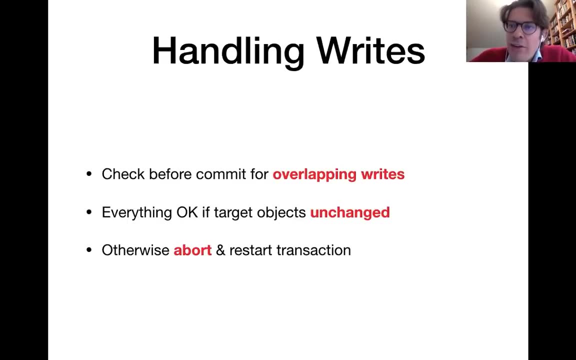 With multiversion concurrency control. in principle, while the transaction is executing, the values of different objects could change and new versions could be added. Here that cannot happen, So when reading data, transactions rely on the snapshot of the database that has been taken once they started executing. 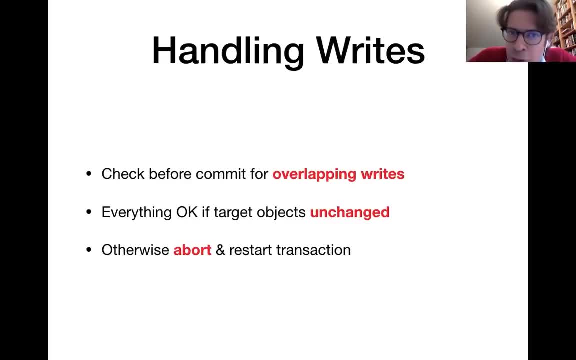 Then writing to objects. in this case we have to pay attention if multiple transactions are trying to write to the same object. If so, we could create conflict, so we cannot allow this to happen. So in this case, essentially after a transaction has executed, 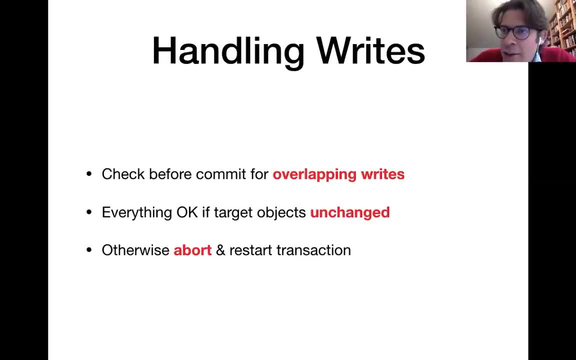 we are checking in order to make sure that no other transaction was already writing to objects that the current transaction is trying to write to. If that is the case, then the current transaction can go ahead and commit. But if there has been overlapping writes to the same object by a concurrent transaction. 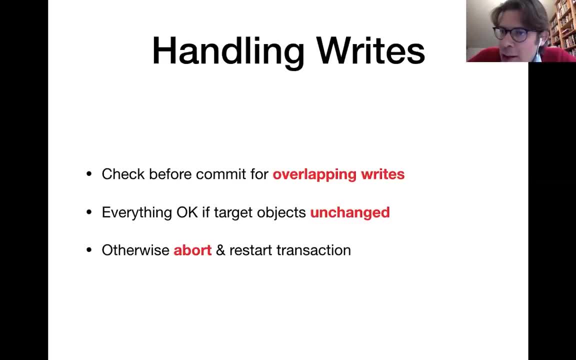 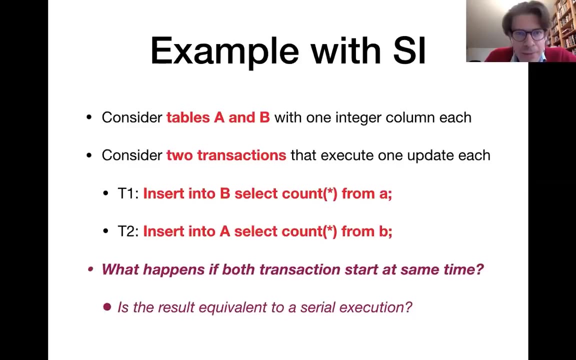 then, essentially, the first writer wins and the other transaction has to be aborted in order to avoid conflict. Now, this may sound great, but there is a catch to it. Let's make an example with two tables, A and B, which both have one integer column. 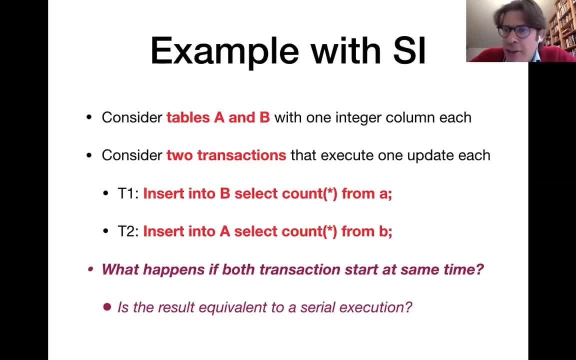 And now imagine those two transactions that we see here. The first transaction essentially tries to insert the count of rows in A as a value into B, And the second transaction tries to insert the count of rows from table B as a value into table A. 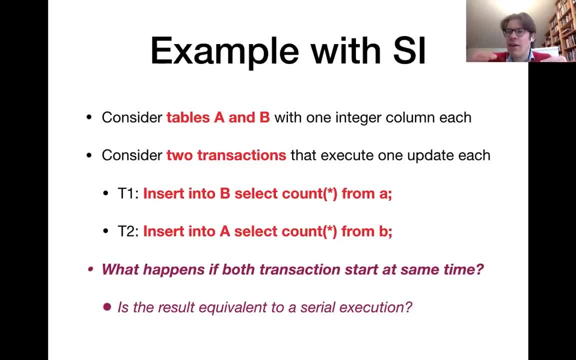 And now we assume that both of those transactions start at the same time, which means that they will operate on the same snapshot of the database. Now imagine that those transactions execute and insert their values. Does anyone have a suspicion about whether the result of that? 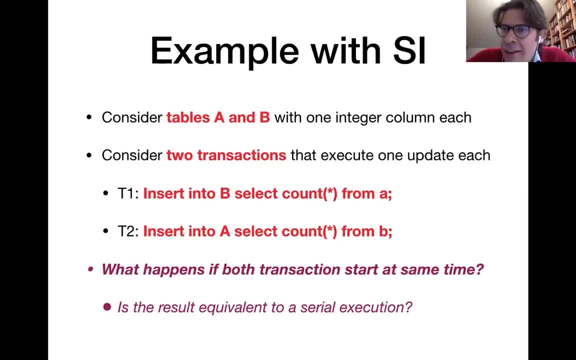 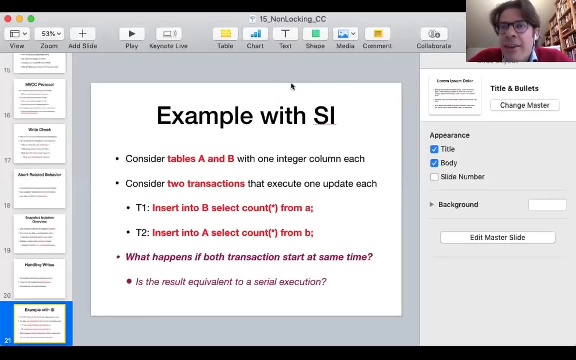 can be equivalent to a serial execution of those transactions. If you have an opinion, please put it into the chat. All right, And here we have the suggestion that one of the inserted values will be one less than it should be. Okay, very good. 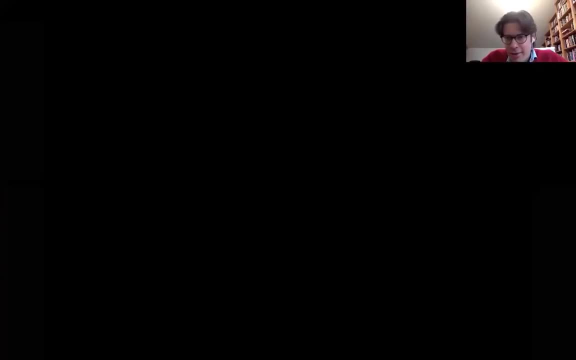 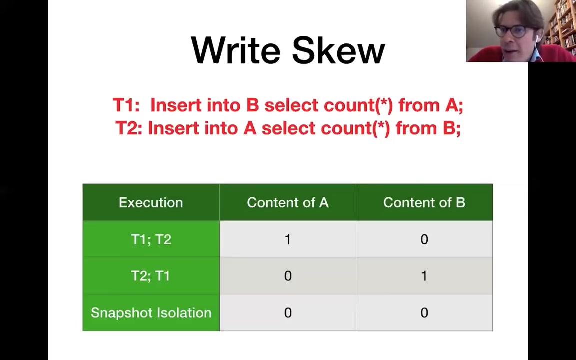 All right, Let's analyze that in a little bit more detail. Let me move this channel out, Okay. So if you want to find out whether we get to a result that could have been generated by a serial execution, then maybe first of all, 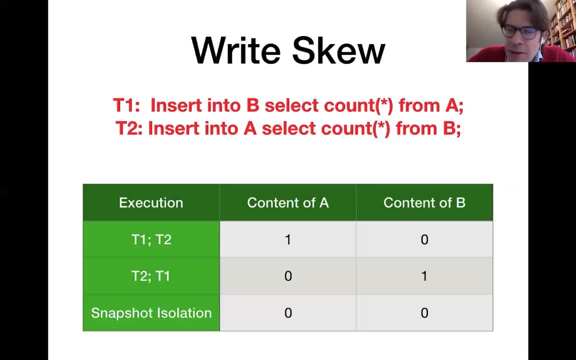 we want to think about all the possibilities for a serial execution. So here we have two transactions, So we have a choice about which of them we execute first, and that creates two possibilities. Now, for instance, we could start by executing the first transaction. 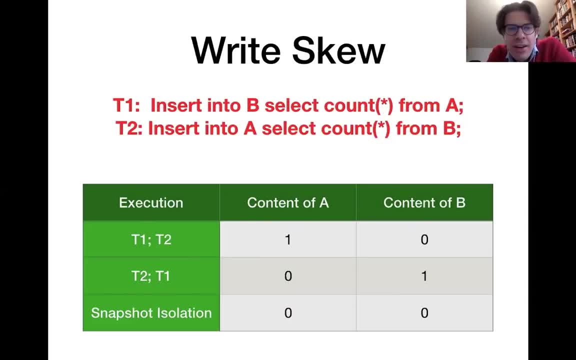 So the first transaction executes the query which inserts the count in A into table B And, assuming that at the start those two tables are empty, we would insert a zero into table B And now we have one row in table A. So if the second transaction runs, 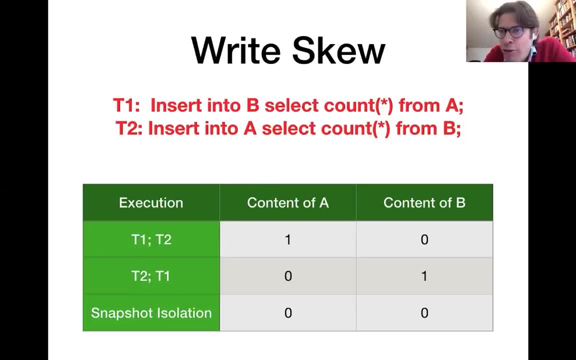 which inserts into table A the count of rows in table B. So since we just inserted a row into table B, it means that we would now insert a one instead of a zero into table A. If we do it the other way around, if we start with transaction two, 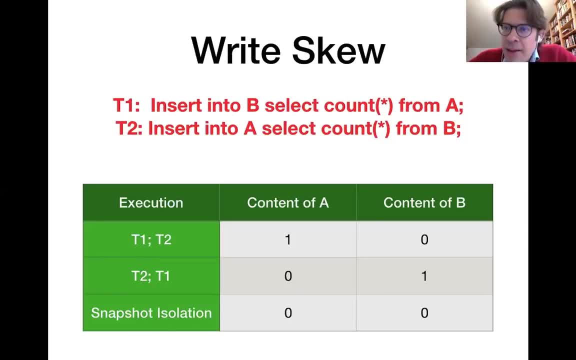 transaction two would first of all calculate the number of rows in B, which initially is zero, and insert that into A. So this is why in A we have now the zero. Now the first transaction runs and it inserts into table B the count of rows in table A. 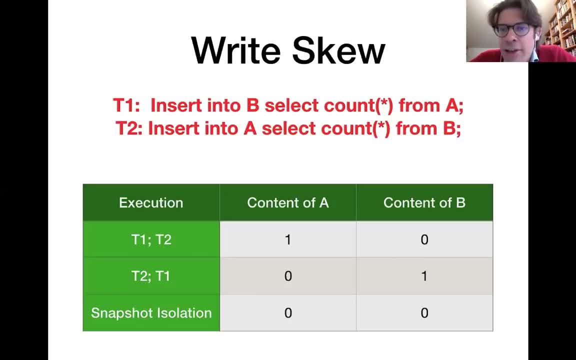 And since we have just inserted a row into table A, it would mean that we insert a one into table B. Now, if we use snapshot isolation, it means that both of those transactions start from the same snapshot of the database, and in this snapshot, 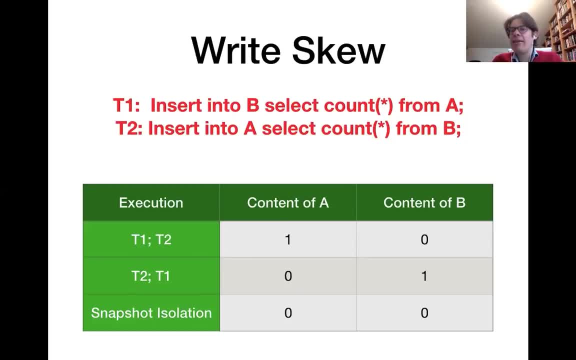 both of the tables are empty, And since both of them execute concurrently on the same snapshot, it means that both of them will account zero rows for both of the tables, and then they will insert the zero into those two tables, A and B. 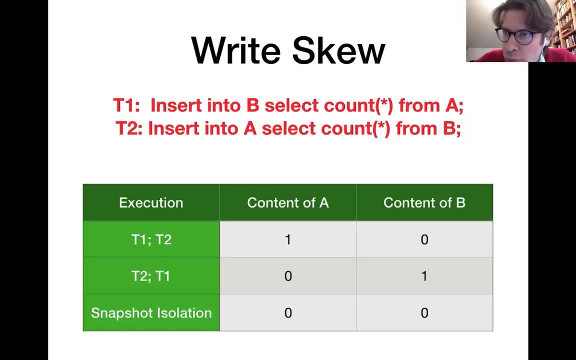 And that is an anomaly that is called right skew. All right, so this is maybe something that is worth having another look at if that seems strange. But here we have definitely a behavior that couldn't happen if executing transactions one after the other one. 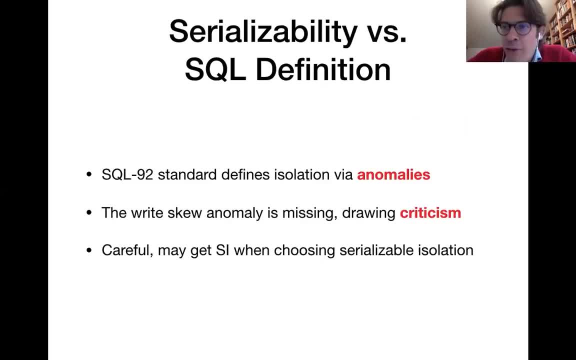 Now, right skew is one example for an anomaly that isn't really mentioned in those anomalies that we have seen initially. The anomalies that we have seen initially. they are based on the SQL standard And the fact that there is some concurrency control protocols which have anomalies that are not really mentioned. 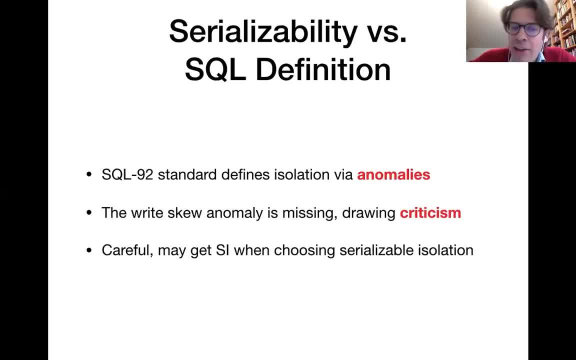 in the standard has actually led to criticism of the SQL standard. So that is maybe the last thing that I want you to know about concurrency control, that we have seen those different SQL isolation levels but depending on the system for some of those isolation levels, 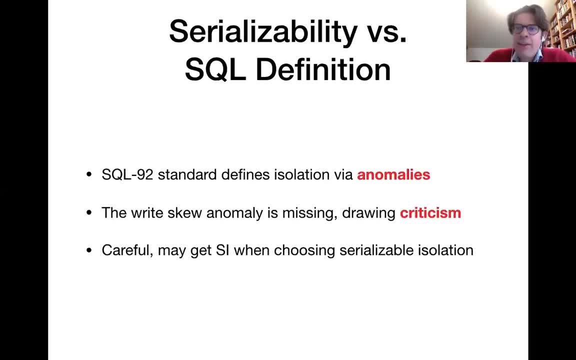 you might actually still have some anomalies, such as right skew, which are not mentioned in the SQL standard, But if you are running your database system with an important application, it might still lead to problems. So be very careful when using your database system. 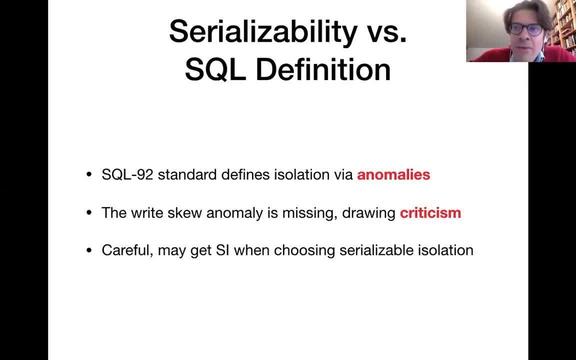 In fact, just make sure that you understand well not only which isolation levels you are dealing with, but also how precisely that isolation level is implemented, embedded. There might still be some anomalies that could appear All right. So that was concurrency control. 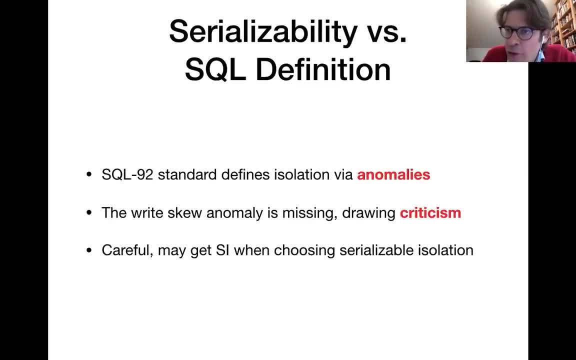 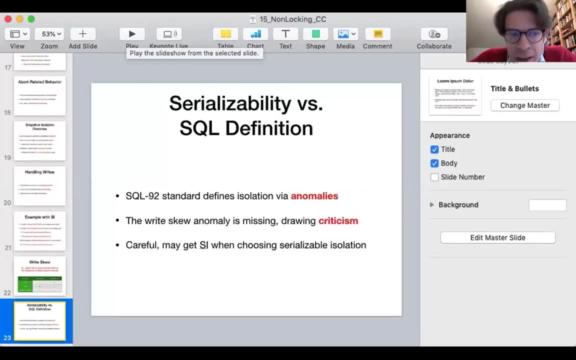 We have mostly been talking about locking-based concurrency control, And now we have also talked about a couple of alternatives without locking. In practice, locking-based concurrency control is very common. This is why we have spent more time discussing that. But as you have seen here, 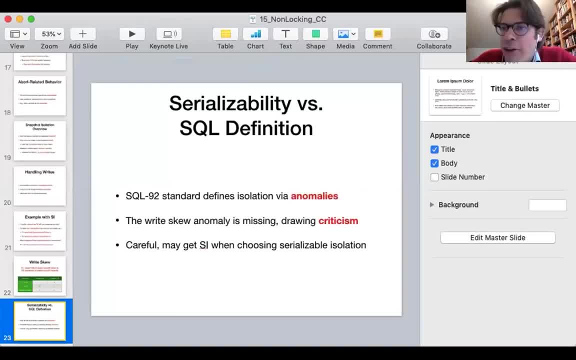 there's also many alternatives, And which one of them works best depends a lot on the particularities of the scenario. All right, So we will now switch to a different topic. I'm going to switch the slide set If you have any questions about concurrency control currently. 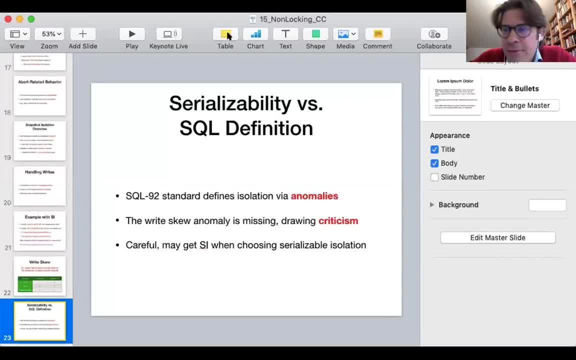 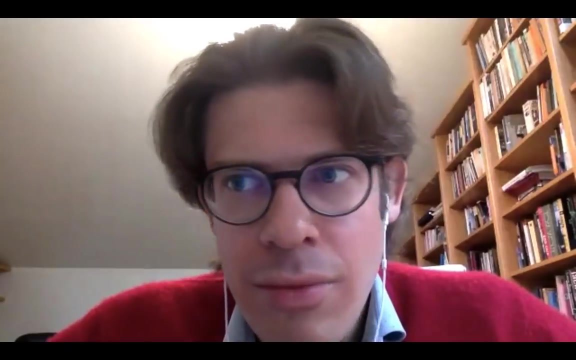 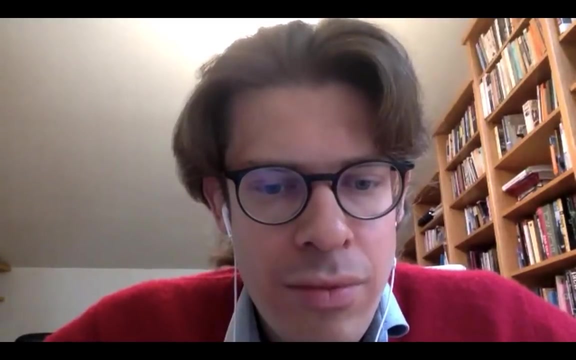 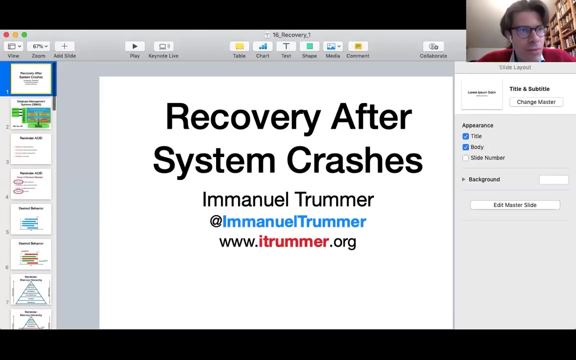 please feel free to put them into the chat And I'll give you a few quick links. Alright, thank you for listening and I hope you enjoyed the video. I hope you enjoyed the presentation. If you have any other questions, please feel free to put them in the chat. 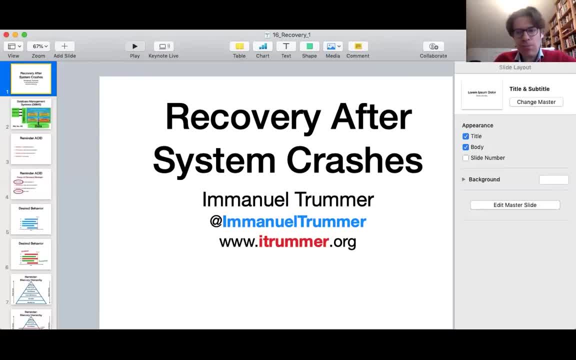 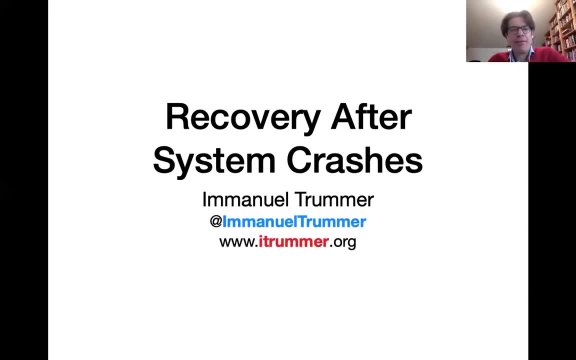 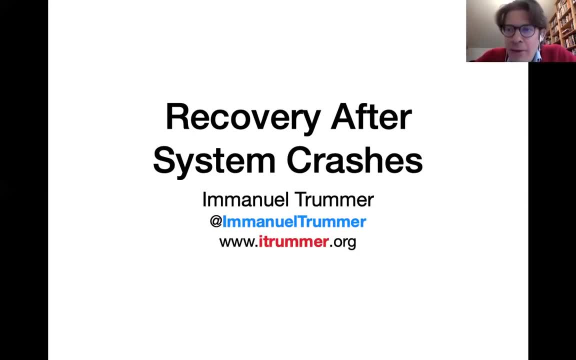 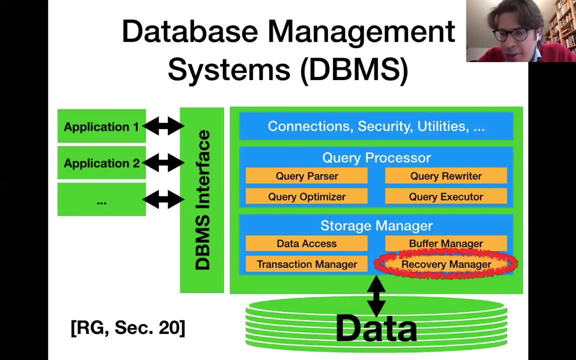 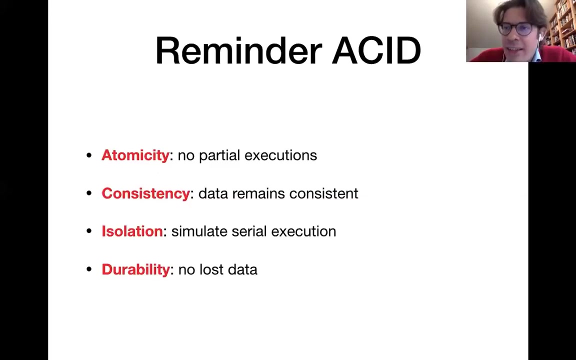 dive into the next topic, which is about recovery after system crashes. This is the component that we will be talking about, that is, the recovery manager marked up here and the relevant chapter in Ramakrishna and Gerke, that is chapter number 20.. So we have talked about the guarantees that database systems make. 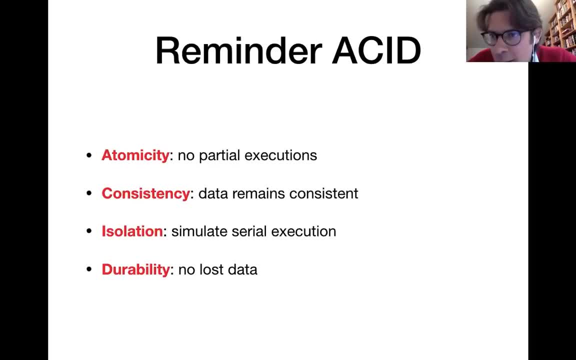 when it comes to transaction processing. Atomicity, which means no partial executions. Consistency, which means that your data remains consistent and satisfies all constraints. We have talked a lot about isolation, which means we simulate different transactions executing serially. and finally, we have durability, which means that we do not lose data that belongs to committed. 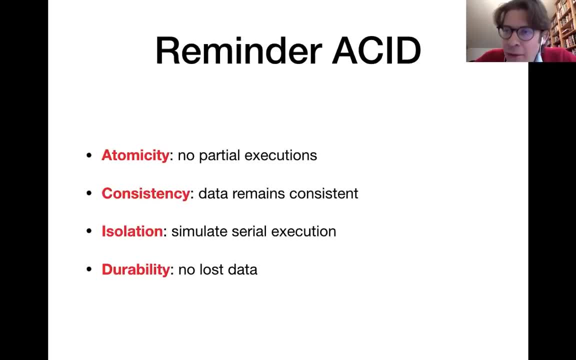 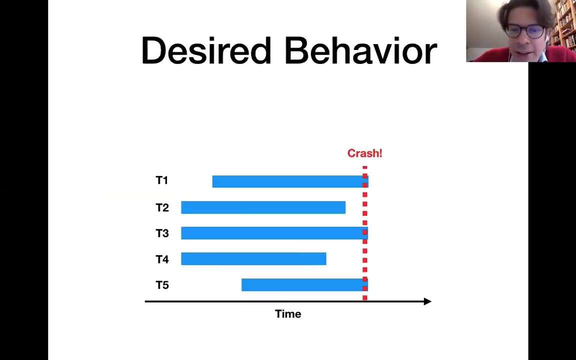 transactions. Now the recovery component essentially takes care of those two properties: First of all atomicity and then durability. So what we essentially want is this: So if you assume that we have multiple transactions executing in our system and then suddenly a crash happens, and the crash could happen for 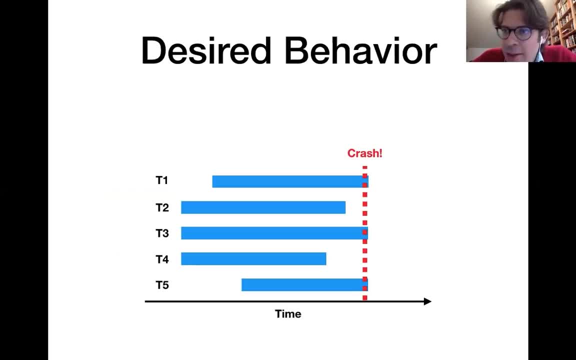 many reasons. One of the reasons, for instance, is a sudden power outage, But it could also be other things, such as a hardware fault or perhaps a software bug that suddenly makes the system crash. But in any case, we are currently executing lots of transactions and then suddenly 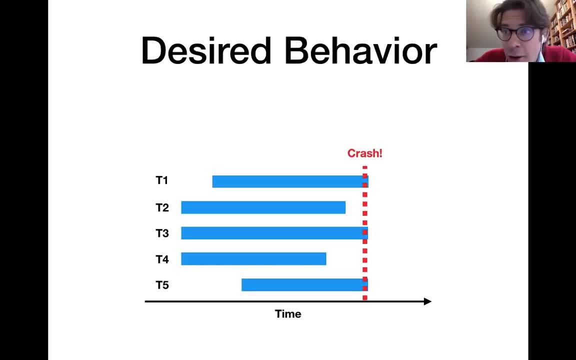 something happens and the database server has to shut down. Now in this graph, basically, we have some transactions that have already executed, by which I mean they have already committed. so we have informed the user, transaction has executed, you have nothing to worry about. and the effects? 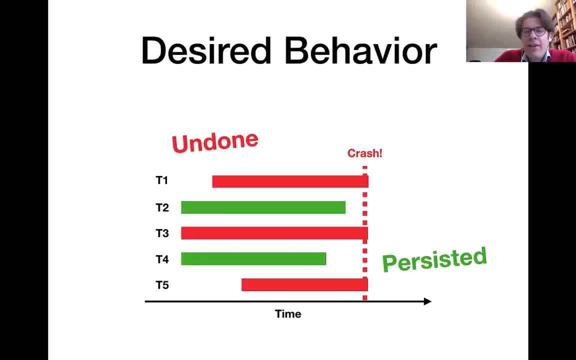 will be persisted And because of that, for those transactions that are now marked in green, we want to make sure that the effects of those transactions, they are actually persistent and they'll be recovered once the system comes back online. On the other side, for the transactions that are running during the 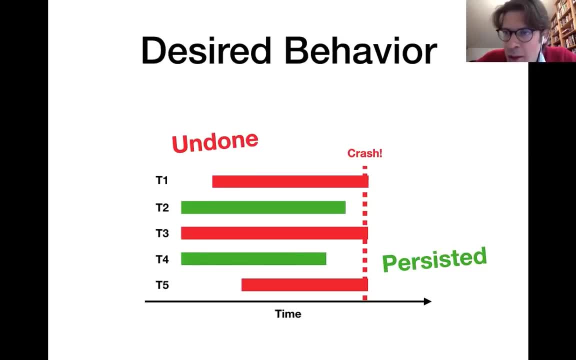 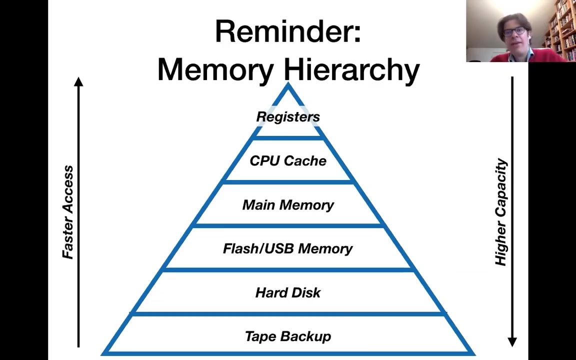 crash for those transactions, you want to abort them and we want to essentially undo them such that no traces of those transactions remains in the system. This refers back to the atomicity guarantee. So this is what we want to achieve once the system comes back online after the crash. This is a little 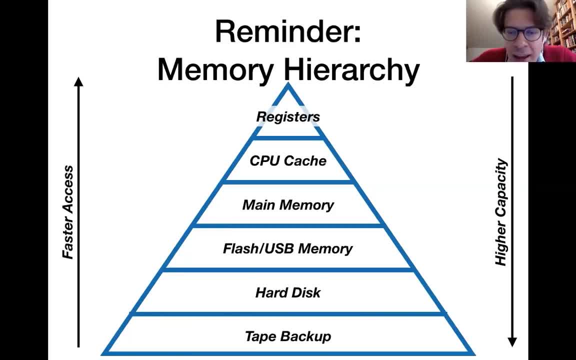 reminder here of the memory hierarchy, And this is the memory that comes after the crash. This is the memory that comes after the crash. This is a little reminder here of the memory hierarchy And this is memory hierarchy. makes it difficult to achieve the behavior that I have just shown, Because in 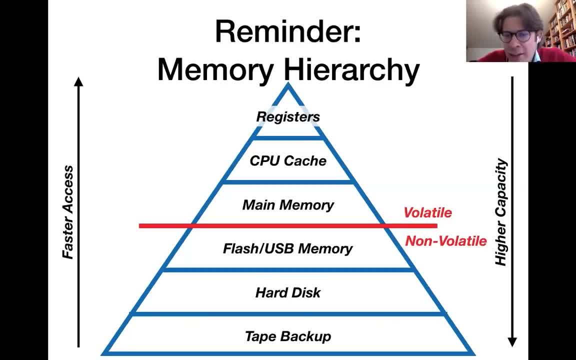 the memory hierarchy, we have essentially two parts. We have a volatile memory, which will be erased if there is a sudden power failure, for instance, and we have non-volatile memories, such as hard disk, which will remain where the content will remain, even during a system crash, Of course. 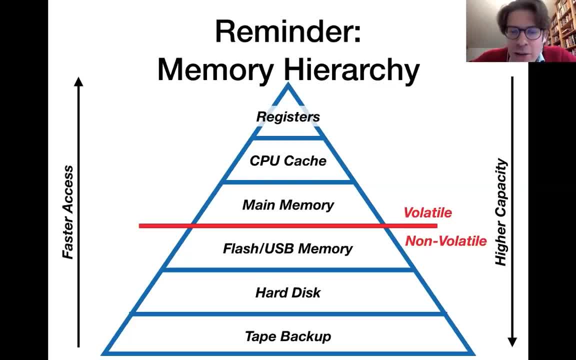 from the safety perspective, you might choose to always write to a non-volatile storage, but of course that would be very slow because, as the memory hierarchy shows, there is a higher level of the memory hierarchy which are volatile. They are, at the same time, much faster than the lower levels of the memory hierarchy and for 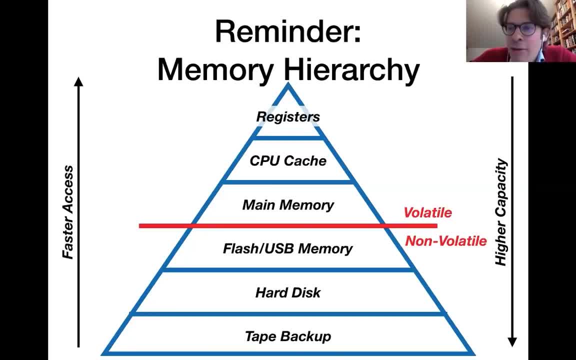 performance reasons. we therefore must work even with the volatile levels of the memory hierarchy, And that makes it challenging to guarantee that, even during a crash, we won't lose any important data or end up with the effects of half-finished transactions in our system. Let's first of all 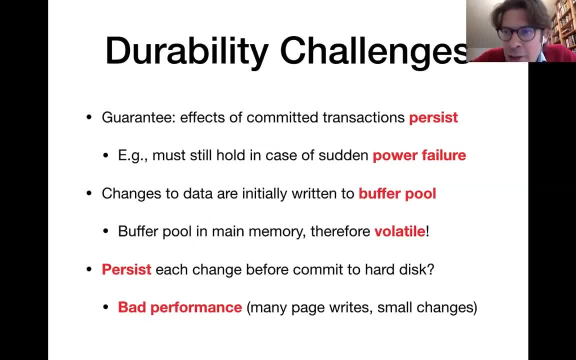 discuss about challenges related to durability, which essentially means we guarantee that the effects of all committed transactions persist even if there is a system crash. Essentially, once the transactions change data, their changes are written first of all to pages in the buffer pool and, as we have seen, the buffer pool that is the main memory portion, that is, 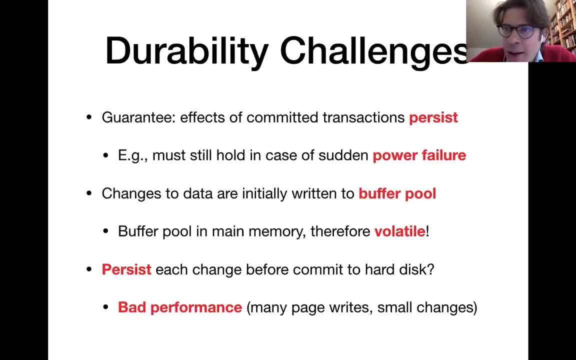 essentially reserved to the database system, and since it lives in main memory, it means it is volatile, and once the power cuts, all the content of the buffer pool will be lost. Now, one thing we could do, of course, is that every change is not only written into the buffer pool, but we also write it. 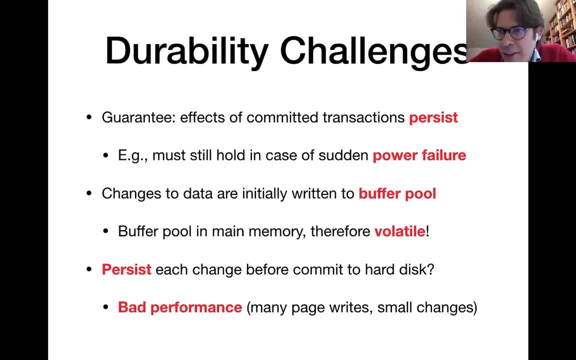 to hard disk, and if you do this immediately, or at least before the corresponding transaction commits, the problem is that we might get pretty bad performance because we have to write a lot of pages on hard disk and on most of those pages we actually have only very small changes because 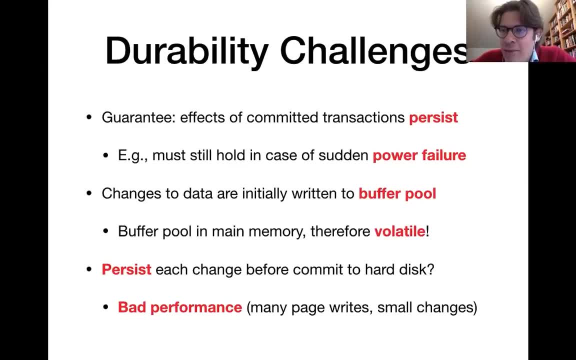 those transactions. they typically just the change the data maybe in one row of your table, while they leave the other rows in the table unchanged. and that means if you're trying to immediately write those data pages from the buffer pool onto hard disk, then you're writing a lot of bytes where most of them are actually. 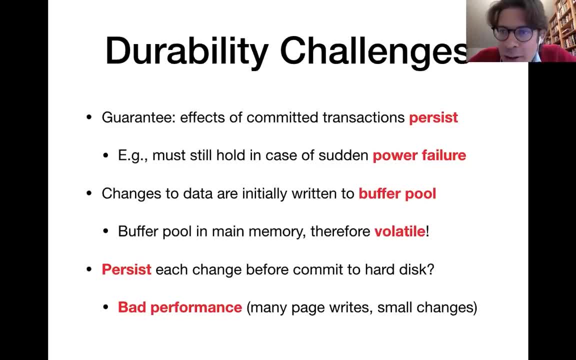 unchanged, but just a few bytes have changed, and for that, yes, actually performing a lot of page writes and that is very inefficient. So here the naive approaches don't work well. so in the following we're going to see a way to improve over that. First of all, let's discuss about 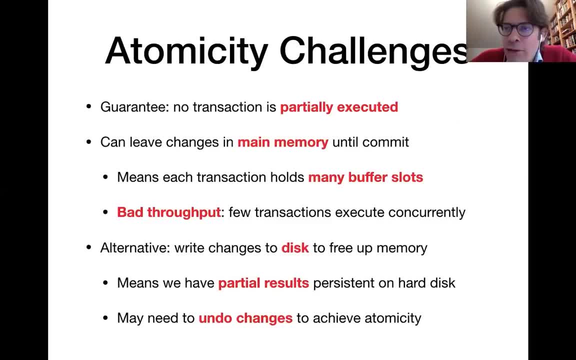 atomicity, which essentially means to guarantee that no transaction is partially executed. and one easy way to guarantee that, even during a crash, would be just to leave all those changes to the data of a transaction in main memory. So we only change things in the buffer pool. 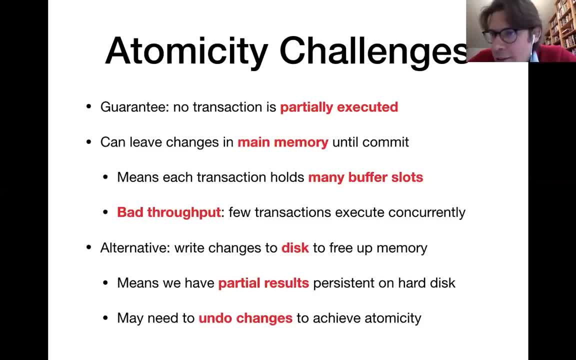 and then we know if there's a crash, then the buffer pool is erased, so automatically all the changes by the uncommitted transactions are erased, which is actually quite convenient, and that would be an easy way of getting atomicity. The problem with this approach is this: 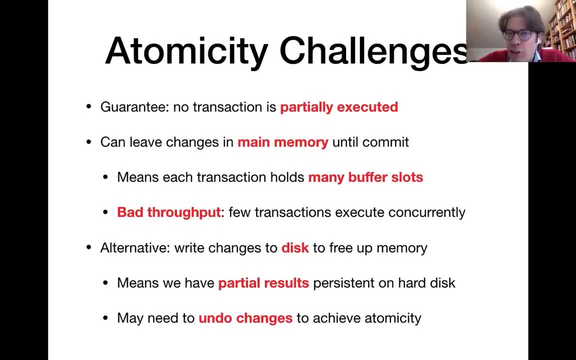 each transaction might change in the same way, So if you want to avoid that those changes get written to hard disk before the transaction commits, it means that a transaction has to hold on to all of those pages in main memory before it until it commits. That means that each concurrently executing 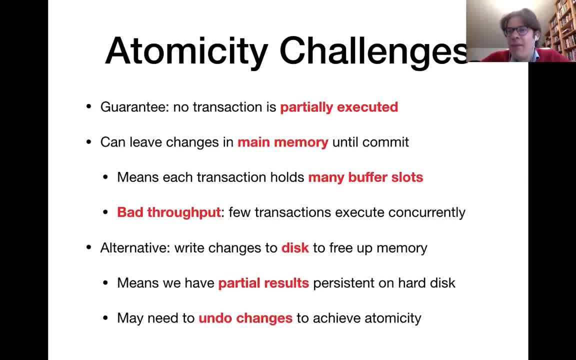 transaction might have to hold many pages in main memory at the same time, and that means we cannot execute too many transactions at the same time. All of those things that we discussed about concurrency control- a lot of it was exactly about allowing as many transactions as possible to execute at the same time in order to increase. 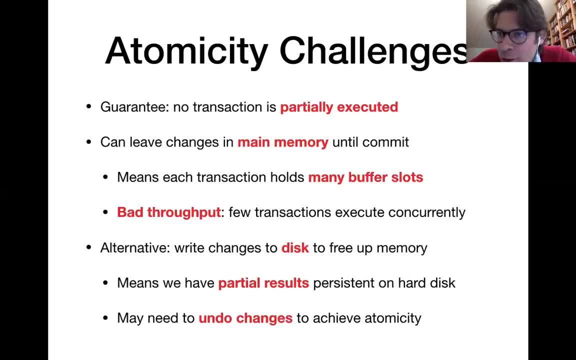 the throughput of your system, meaning the number of transactions that get finished per time unit. So if you would introduce a constraint that transactions have to reserve many pages in main memory- since the amount of main memory we have is typically limited- it would mean that the number of transactions that can execute at the same time and therefore our throughput, which is 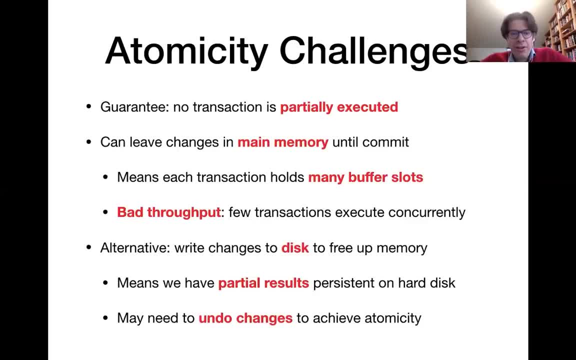 something that we want to avoid. So the alternative to that is, of course, that we allow transactions to let go of their pages in main memory and therefore we have more flexibility about how we use those precious pages in main memory. We essentially allow ourselves to swap. 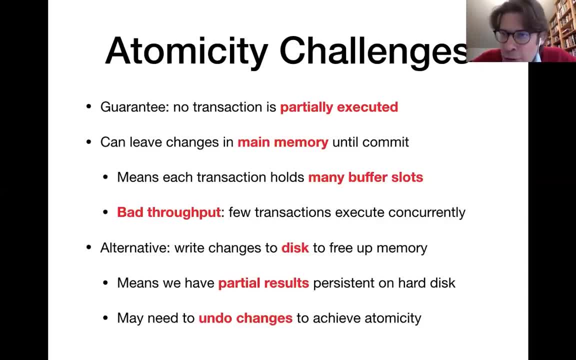 pages in main memory between different transactions. The problem with this is the following: so if a transaction has performed some changes on the data page in main memory and now we want to assign that page, we want to lend that page to a different transaction which needs to do something else. 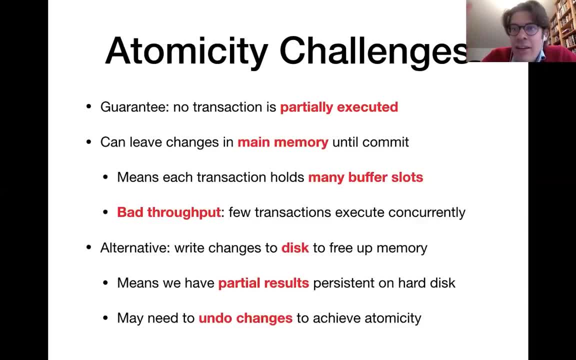 So at that point, of course, if we simply erase the current page in main memory, it would mean that we would lose the changes by the transaction, which, because of durability, we obviously don't want to do. On the other side, if you choose to keep the changes, and since we don't have that much main 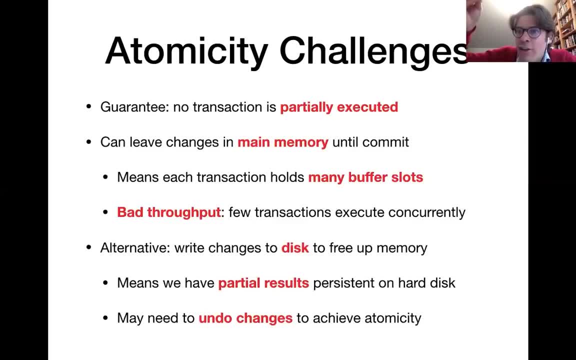 memory, we need to write those changes to a different layer in the memory hierarchy. so typically we would need to write those changes to hard disk. Here the changes are consistent. so if the current transaction successfully executes, then we are okay with writing those changes to hard disk. but if the current transaction suddenly aborts or if there 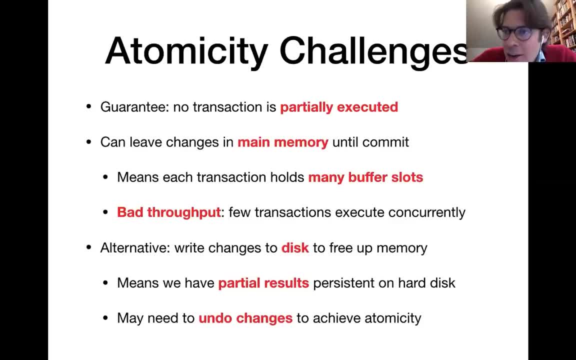 is a crash so that the current transaction is implicitly aborted, then it means that now suddenly on hard disk we have the changes by some half finished, by some aborted transaction and we will have the changes that we don't want to have due to atomicity. So again, there is different. 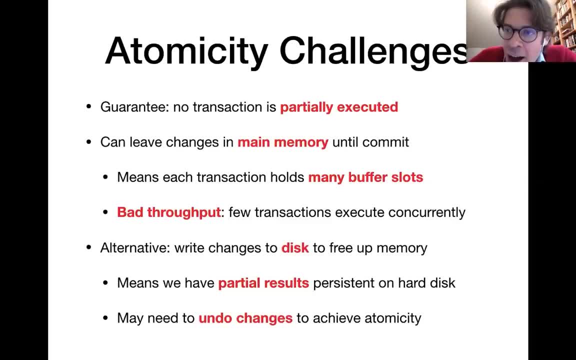 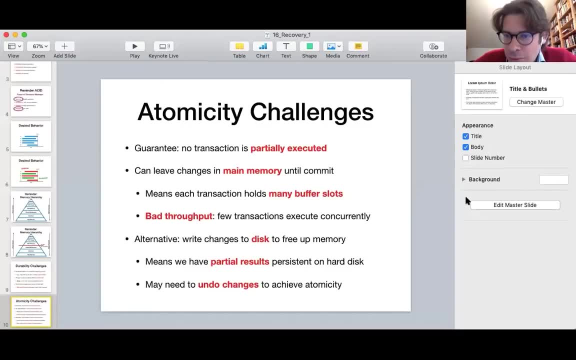 naive solutions, but all of them come with a serious drawback. so in the following we're going to see how we can improve over that. I think there might have been a question in the chat. Let me quickly check. So the question is whether, in the alternative, we are writing directly to the database data. So I have 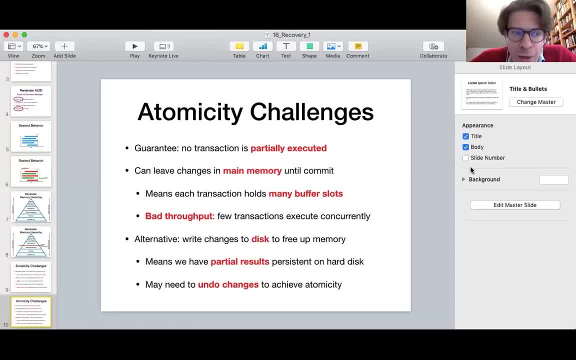 pointed out multiple alternatives for durability and for atomicity, and indeed one of them was that we essentially directly write changes to our database data, that so we directly can write changes to a hard disk, and that has the advantage that they per sist even after a system crash, which is good if the transaction is committed On the other side. 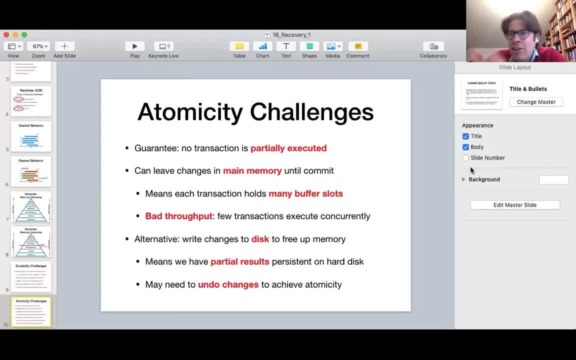 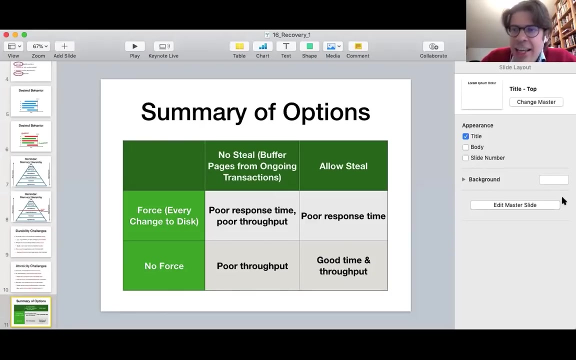 if the transaction doesn't finish before the crash and must be aborted. it means that we now have changes on hard disk that belong to a half finished transaction and we need to sooner or later undo those changes again. All right, So this here is a summary of the different options that we have, and that we have essentially. 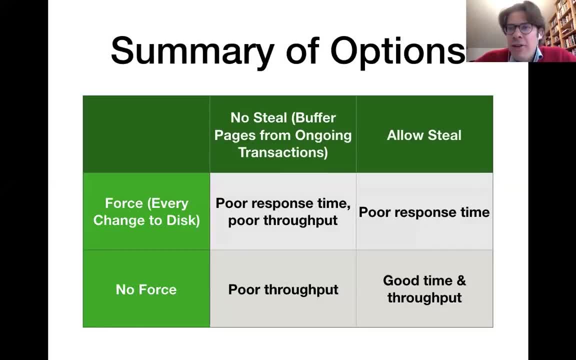 discussed in the previous slides. So we can choose to use a so-called a force policy, which means that we make all changes to the data persistent on hard disk before the corresponding transaction commits. The advantage of that is that we are safe If from losing data in the case of a system crash. the disadvantage of that is that we have a lot of page. 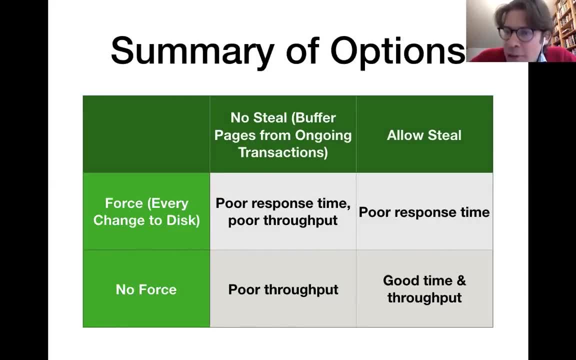 writes by each transaction and that leads to poor response time. The other thing, the other choice that we have is how flexible we are in assigning buffer paid buffer slots to transactions. A no steal policy essentially means that each transaction must hold on to its pages in the buffer. 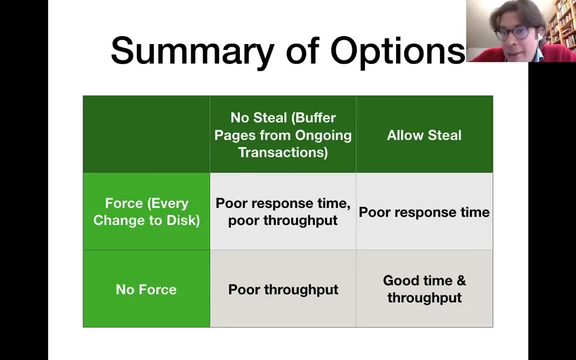 pool until it commits. The advantage of that is that we don't have to deal with undoing changes on hard disk by aborted transactions. The disadvantage of it is that each transaction will actually consume a lot of main memory pages, which severely limits our transaction throughput. 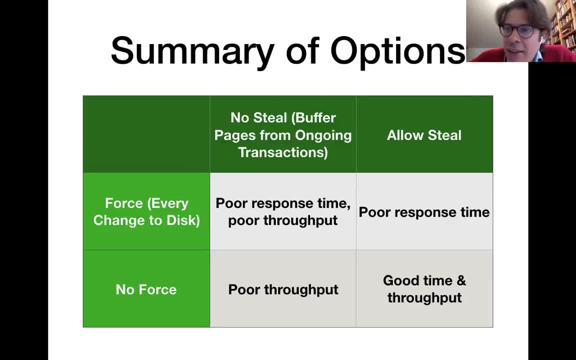 So, for performance reasons, what we want is a policy that allows a stealing, which essentially means that one transaction can steal a buffer slot from another transaction before the other transaction is actually committed. So allowing stealing leads to a higher throughput and having a no force policy. 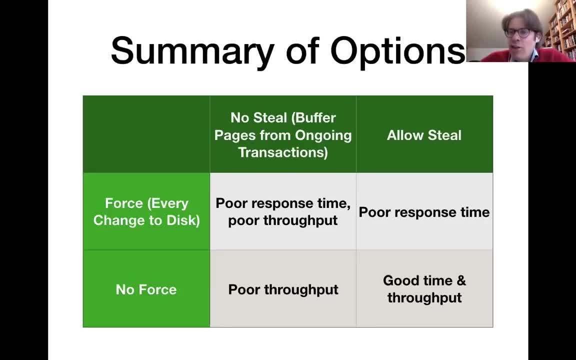 which means we do not force transactions to write all the changes to hard disk. that leads to better response time. So for performance reasons we want to allow stealing and we don't want to force writes to hard disk. The problem with that is, of course: what do we do about durability and atomicity guarantees? 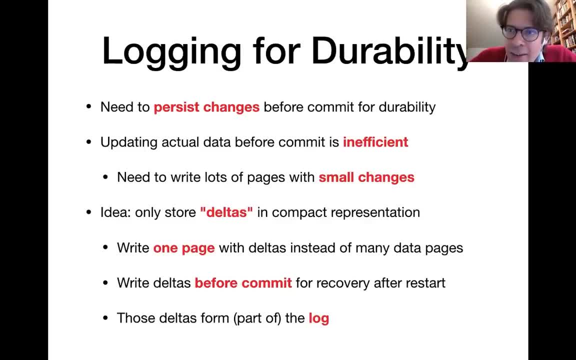 Now the high level solution that we will discuss in the following, that is, logging, which essentially means that we don't write the actual data on hard disk, But we write a highly compressed representation just of the deltas of the changes to the data to hard disk, and this is what we call a log. Now, in the following we're going to discuss, 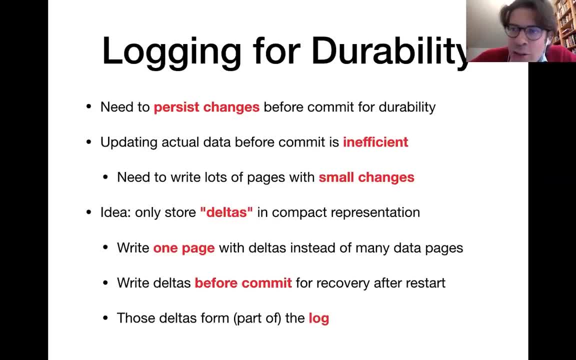 in more detail about how logging can help us to resolve those performance challenges that I have discussed on the last slides. Now, if we want to guarantee durability, it generally means that we have to make changes at precision. So, if we want to guarantee durability, it generally means that we have to make changes at precision. 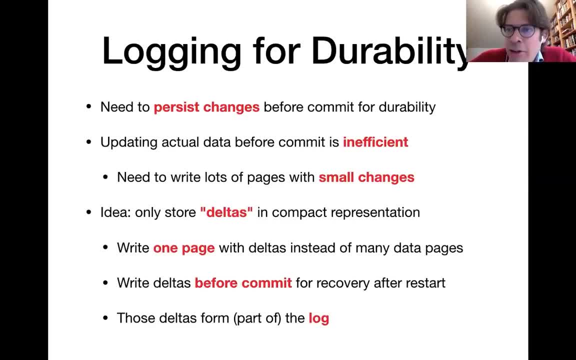 Now, if we want to guarantee durability, it generally means that we have to make changes at precision of a transaction before the transaction commits, because durability means that after the transaction commits, it is guaranteed to stay in the system even if there is a crash. And very clearly, since everything in volatile memory is lost during a crash, we must make changes. 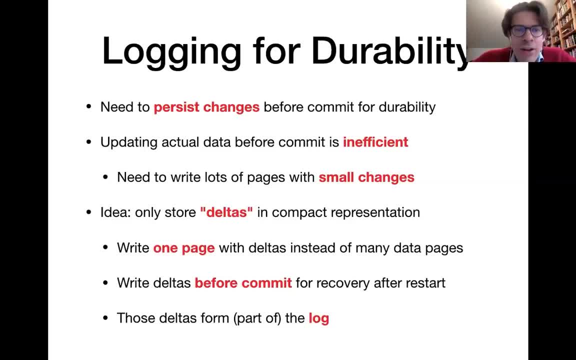 persistent on hard disk before we allow a transaction to commit. We have already discussed the possibility to update the actual data before the transaction commits commit, which is what we call the force policy. the reason why that is inefficient is that the changes that a transaction needs to make they're typically distributed over many different data. 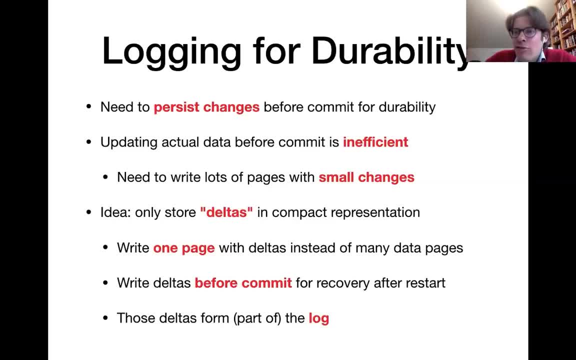 pages, and this means that we would actually have a lot of page rights just for making persistent a lot of small changes in the data. the idea behind logging is that we don't do that, but instead we just collect all those updates to the data in a very compressed representation. so for one. 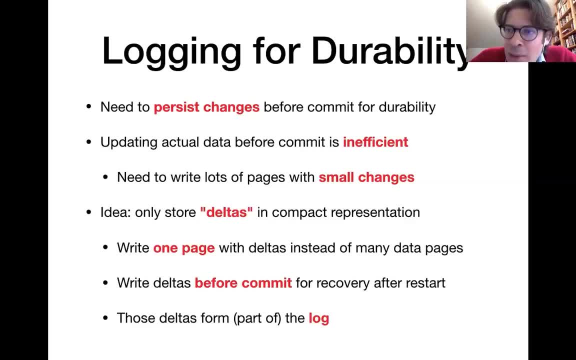 transaction, you typically can collect all its updates in compressed representation on one single log data page, and if you want to make that persistent, we can just write the log data to hard disk, typically with one single page right, and that is much more efficient than writing all those different data pages that the transaction has changed and then we just have to. 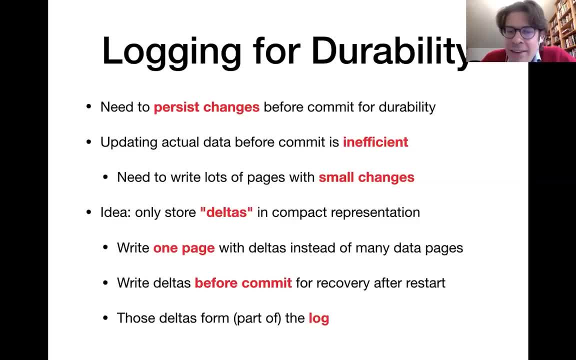 make sure that those this logging related data are written to hard disk before the transaction commits. and so, even if we haven't changed the actual data, since we have a list of the updates to the data, that is sufficient in order to recover the data if there's a crash once the system comes back online. 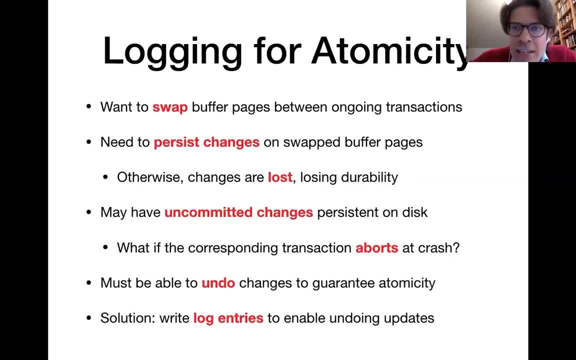 now let's see how logging can help us to deal with atomicity. now we have already discussed why we want to swap the pages in the buffer pool between different transactions, and once we swap ownership of one slot in the buffer pool from one transaction to another one, we first of all have to 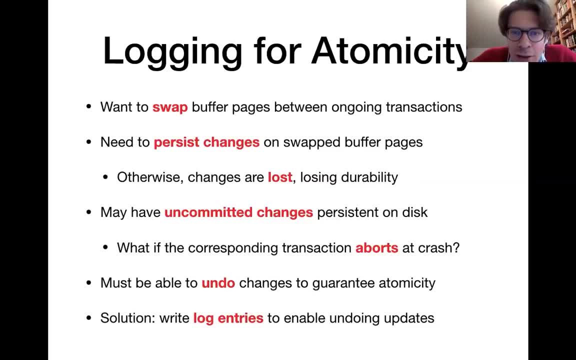 preserve the changes of the first transaction, and that means that we need to write the current content of the buffer pool slot at two hard disk, because otherwise the changes would be lost and that is incompatible with the durability requirement. so the thing is this: if we swap pages and we write changes to the current page by the current 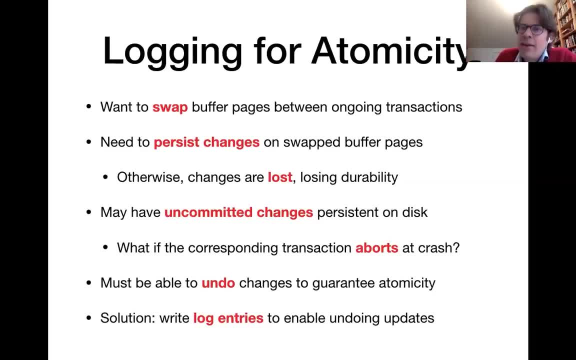 transaction on hard disk. if the current transaction later aborts, which could, for instance, be because the system crashes, but also because of a different reason, In that case we need to take care of those changes to the data that we now have already written to hard disk, because we need to undo those. 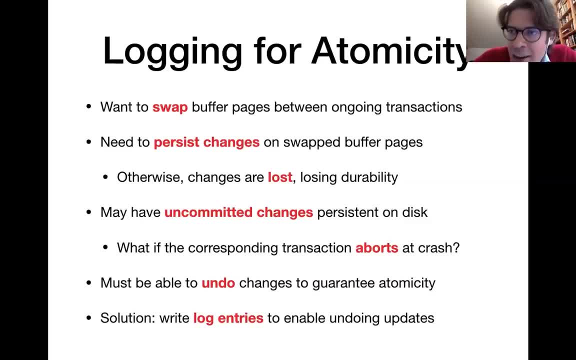 changes in order to guarantee that the database looks as if the aborted transaction had never happened, And in order to enable this, we will expand our log with information that allows us to undo each change to the data in case the corresponding transaction aborts, And we just have to make sure. 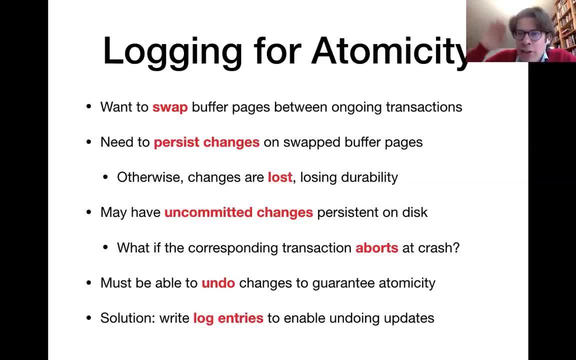 that we write those log entries for a specific page to hard disk, which means that if the system crashes immediately after we have written the current page content from the buffer slot to hard disk, then we still have the required information in order to undo the changes by the current transaction. 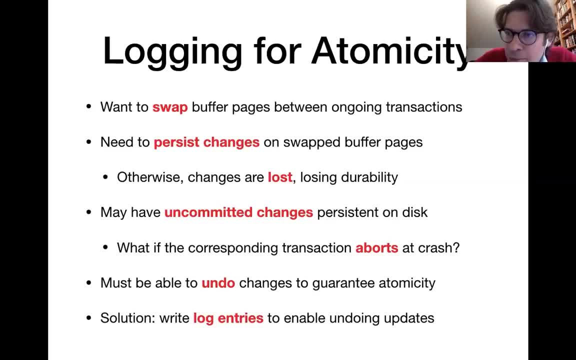 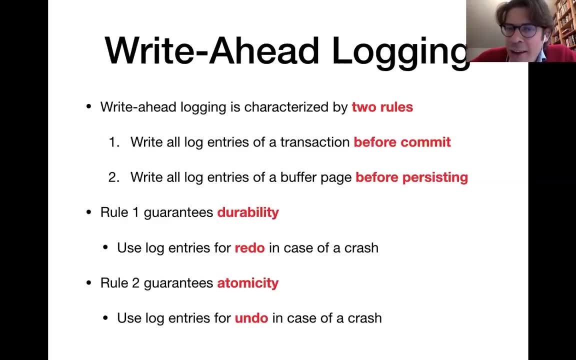 in order to bring the data back into a consistent state. So now we have discussed how logging can help with durability and atomicity. The general term for the class of logging algorithms that we will discuss about in the following slides is write ahead logging, And write ahead logging is essentially 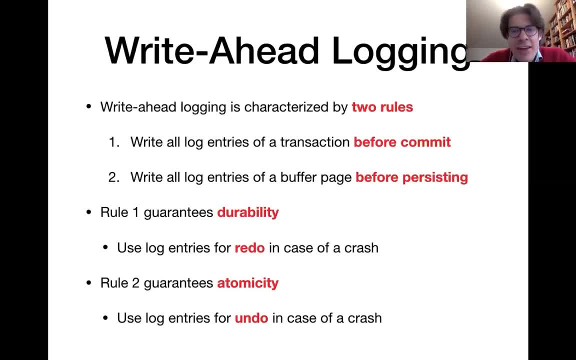 characterized by the two rules that you see here. First of all, we have to write all the log entries that relate to a transaction before the transaction commits. And the second rule is we have to write all log entries that concern a page in the buffer pool to hard disk before that a page is written to hard disk. 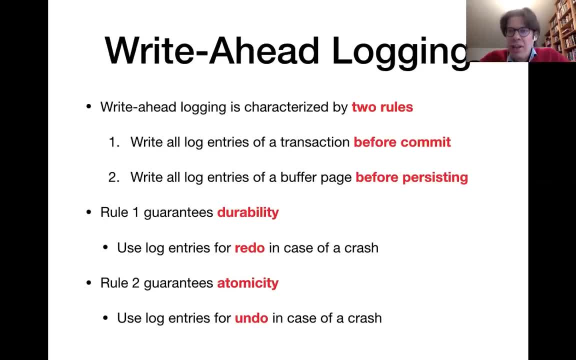 Rule number one is important to guarantee durability, because if a transaction commits and we have the log entries from that transaction on hard disk, then we can use that in order to redo the changes of the transaction, even if the system immediately crashes after the transaction commit. Rule number two is important for atomicity. 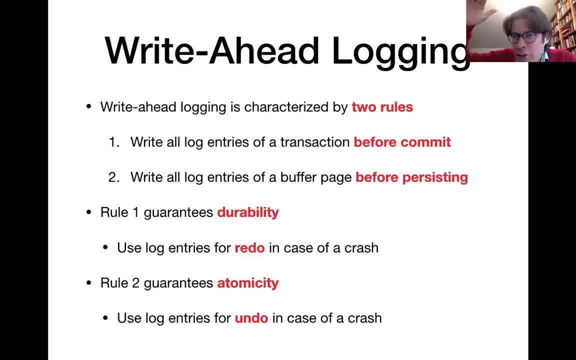 Because if you write a change data page to hard disk and those changes have been made by a transaction that will later abort, If we have the log entries about that page on hard disk already, then we can undo the changes in order to erase the effects of the aborted transaction. So this is the two rules of write ahead. 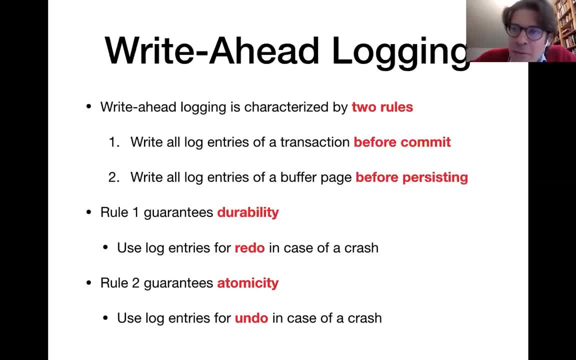 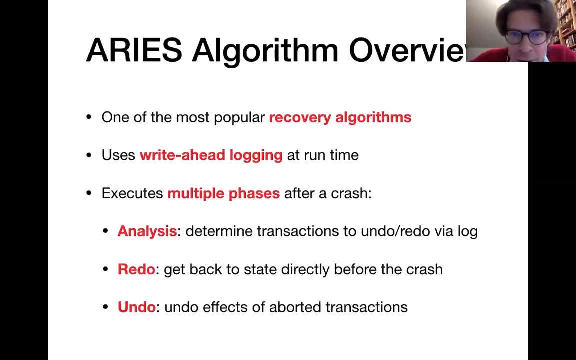 logging, And in the following slides we will also see one specific algorithm that uses write ahead logging. This algorithm is called the Arias algorithm. It is a very classical algorithm. It has been proposed decades ago, but the variants of it are still quite popular. 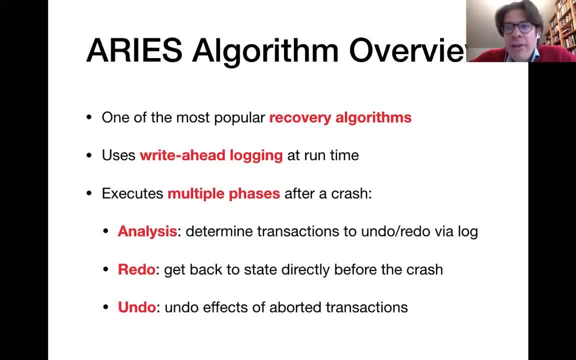 in a database as systems. Now this algorithm uses a write ahead logging and we will see in the following how precisely it implements it And after we boot the system up again after a crash. this Arias algorithm will perform three recovery phases. It first of all will analyze the last log entries that 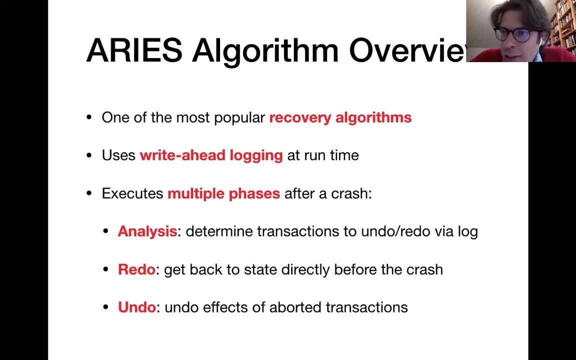 it finds in hard disk in order to decide which transactions need to be undone and for which transactions we need to redo data changes. Then it will have the redo phase, in which we redo the changes of committed transactions that were lost due to the crash, And finally we have the undo phase. 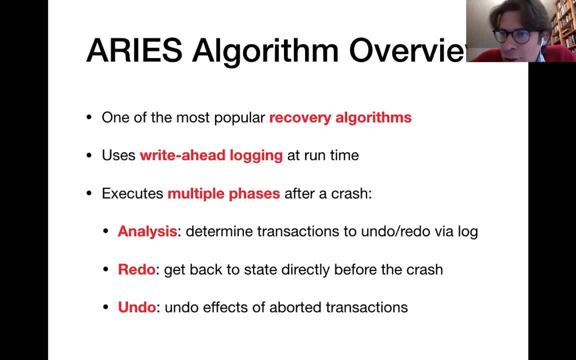 in which we undo the changes of all transactions that have still been active during the crash and must be aborted. So we are gonna see that in much more detail in the following. It is an algorithm that has quite a few moving parts, so we will take some time. 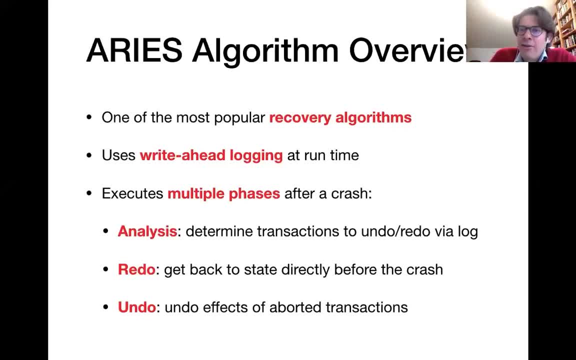 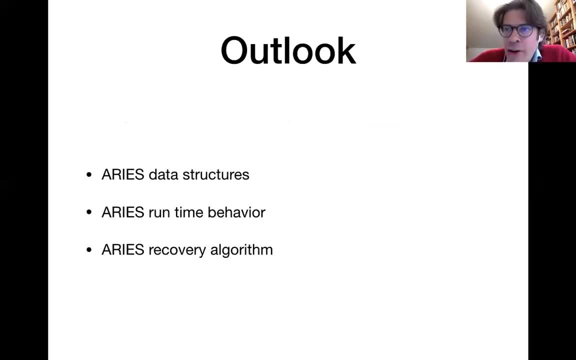 to discuss the different parts of the algorithm and the different data structures in this lecture and also still in the next lecture. In general, we're going to break it down into three phases. First of all, we're going to discuss about the data structures of the algorithm. Then we're going to talk about the 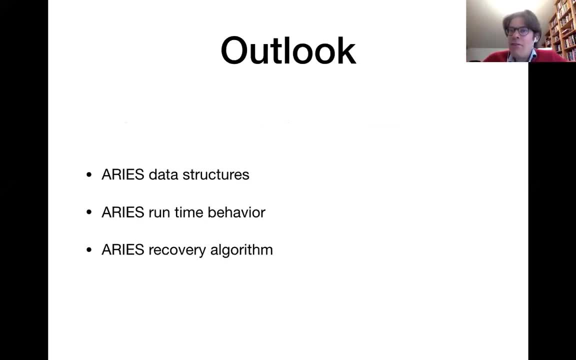 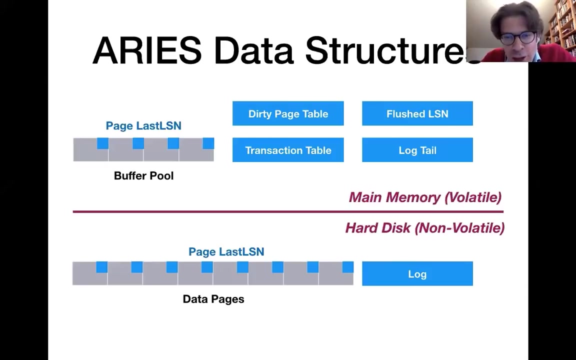 behavior that it has at one time where it generates log entries that help with recovery later. And finally, we're going to discuss in detail how the recovery proceeds precisely Now. in the following we still have a little bit of time to talk about the different data structures of the ARIES algorithm And all of those different data. 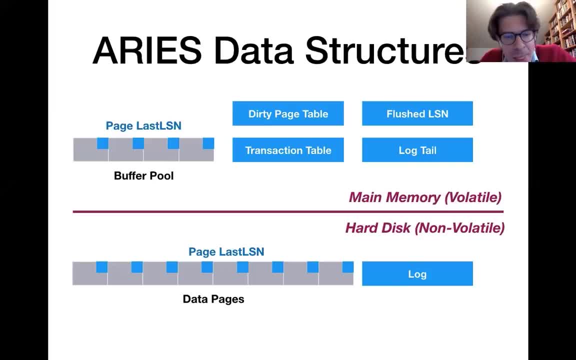 structures. I have them represented here. So here we have some data structures in gray and those are the data structures that do not directly relate to the ARIES algorithm. So here we have, of course, the data pages on a hard disk and we have the buffer pool pages in main memory. So you see the 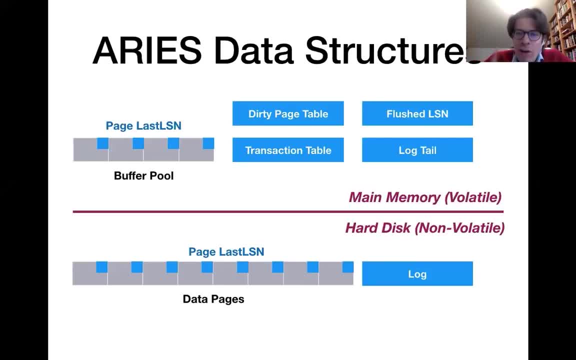 divider in the middle of the screen. Everything on top of it is stored in main memory, which means it is volatile and will be lost during a crash. Everything below the divider is stored on hard disk. It is non-volatile and will persist after a crash. So here we have. 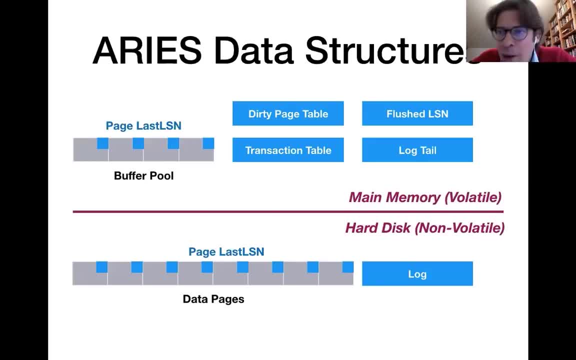 data pages on hard disk in gray and we have buffer pool pages in main memory in gray. Now the first thing that I want to discuss here is: you see those little blue rectangles for the buffer pool and for the data pages. Those are essentially timestamps, that. 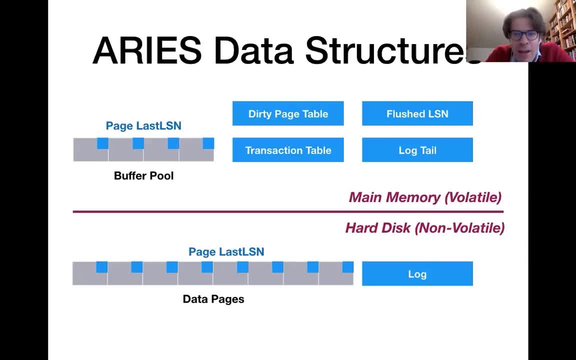 tell the ARIES algorithm when those pages have changed for the last time. Beyond that, there's a couple of specific data structures of the ARIES algorithm. here drawn in blue, The following: we're gonna go over all of those different data structures and explain at a high level. 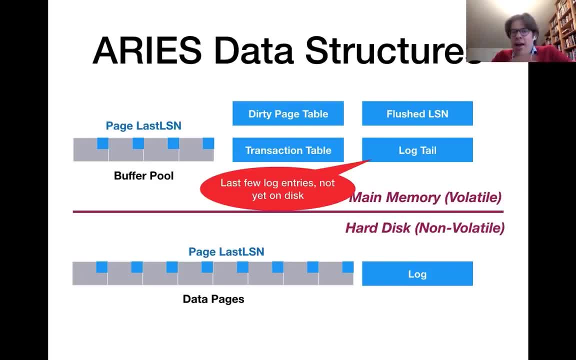 what they are about Now. first of all, log entries are first written not to hard disk but into main memory. We postpone writing them to hard disk for as long as possible and the log tail is stored in main memory. and those are essentially the most recent log entries which have been generated but which 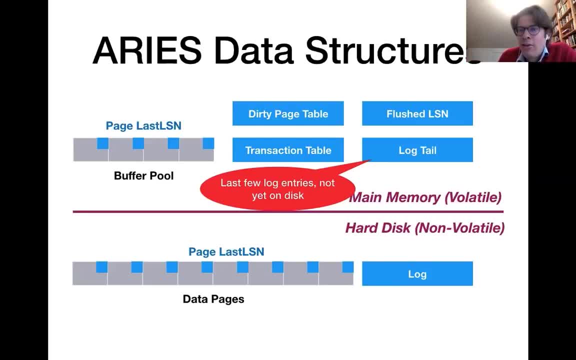 haven't made it to hard disk yet. So this log tail, those are log entries which are eventually written to hard disk, unless there's a crash, because in that case the log tail is essentially lost. The flushed lsn keeps track essentially of where the log tail starts. so 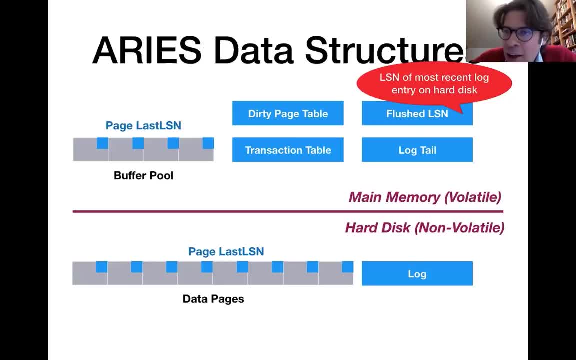 using the flushed lsn we keep track of which log entries have already made per se, have already been made, persistent on hard disk. So this essentially captures the lsn, which stands for the log sequence number, and that is a unique identifier for the line In the log file, essentially, and the flushed lsn. 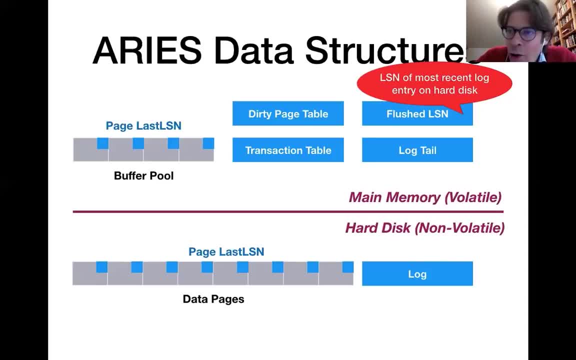 that is essentially the last log line that made it already to hard disk. So in several cases it is important to verify whether log entries, for instance about a transaction, have already made it to hard disk, because then we can allow that transaction to commit and the flushed lsn essentially keeps track of which log. 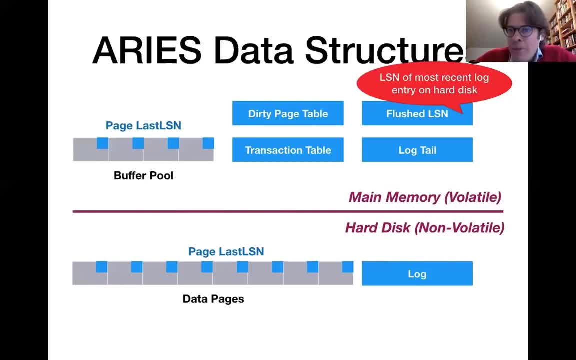 entries have already been made persistent. Now, the log tail is essentially a buffer, and in the context of buffers, we often use the word flushed in order to say that we essentially write the buffer content to a persistent storage and then we erase it to make it available again and enable it to receive more data. 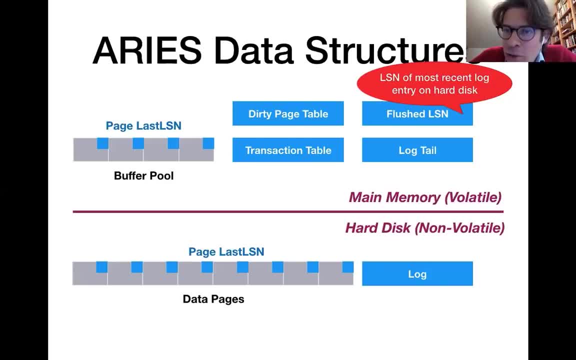 And this is why we use this terminology here when it comes to the log. So the log tail is a buffer And every once in a while we flush it, meaning we write its content to hard disk and flushed. lsn keeps track of when that has happened for the last time. 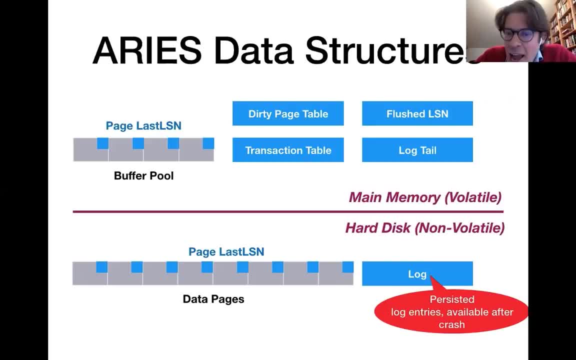 Now here on hard disk we have the act2.log that will be used for recovery. It is stored on persistent storage so after we come back online after a crash we will be able to access those entries here and the recovery phase of the ARIES algorithm. 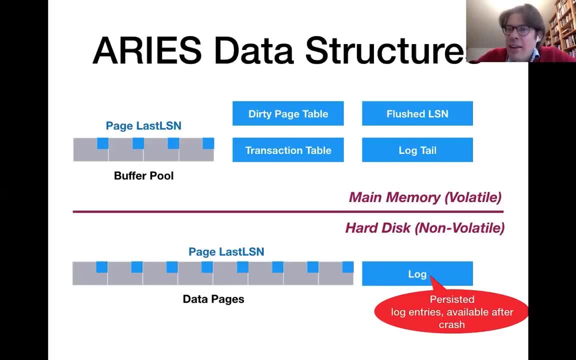 uses exactly this log in order to bring the data back into a consistent state. The transaction table is an auxiliary data structure which keeps track of transactions that are currently active. for each transaction, It stores the current status, whether transaction is currently running or whether it has already decided to commit. 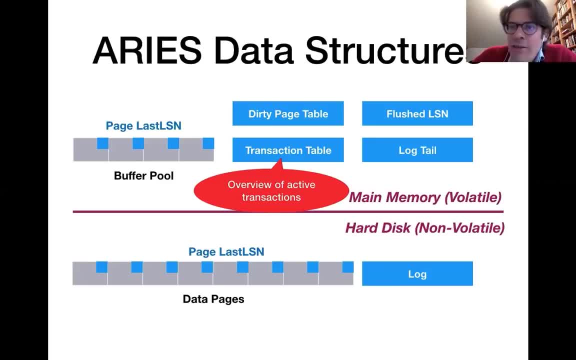 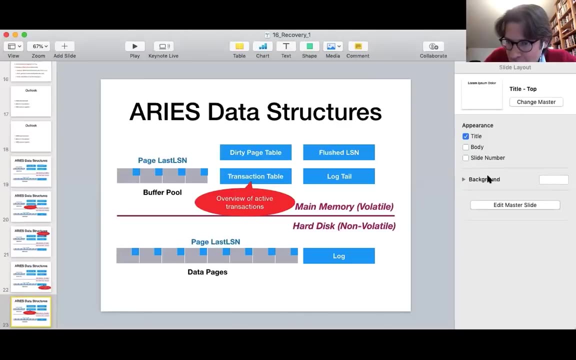 for instance, and also for each transaction, they keep track of the last log line, of the last log sequence number that this transaction has generated. I see there's a couple of questions in the chat. let me quickly bring the chat back. Okay, very good, okay, so here. 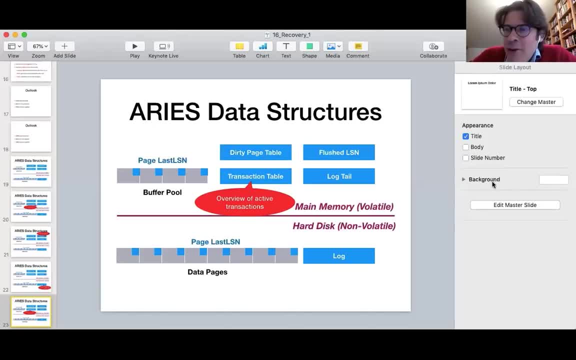 there was a great question and already the answer. so lsn stands for log sequence number. so you can imagine that all those log entries, they are numbered. essentially each log entry has a unique number. This number is monotonically increasing. so if you imagine your entire log as a text file, for instance, 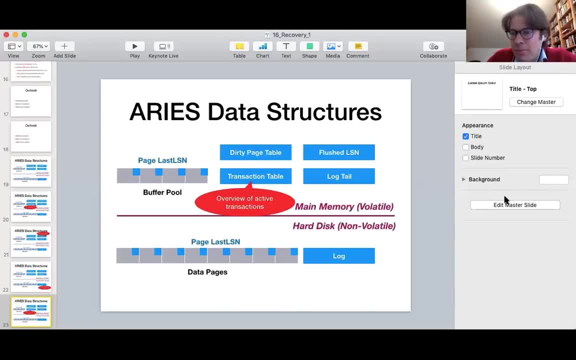 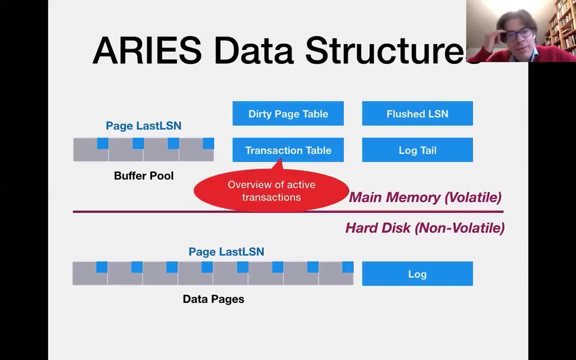 then the lsn would essentially be the line number, and you keep appending lines to the end of that file. All right, so that is the transaction table, and you also have a so-called dirty page table and that essentially keep track of the pages which are currently loaded into the. 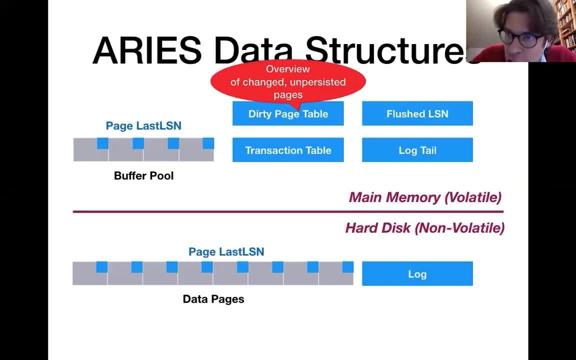 buffer pool in main memory and they have been changed in some way and those changes have not yet made it to hard disk. So this essentially keeps track of pages. that might be potentially problematic because I might lose changes to those pages, which have only been made in main memory. but 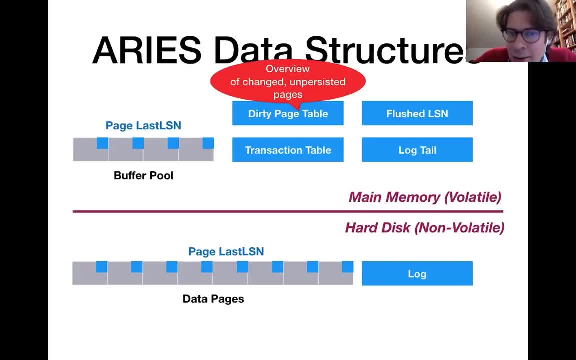 haven't been persisted on hard disk yet. All right, and as I have already said here, associated with each slot in the buffer pool we have the log sequence number of the last log entry which changed the corresponding page, and we also have the same on hard disk. 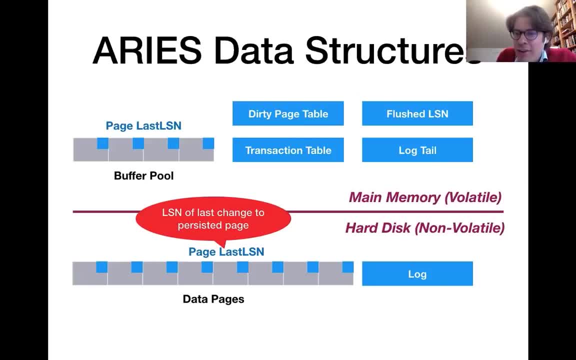 So this is a high level overview of the different data structures that the algorithm uses. so here you see. already there's quite a few different data structures, And in the following we're going to see in more detail how the algorithm updates those data structures at runtime. 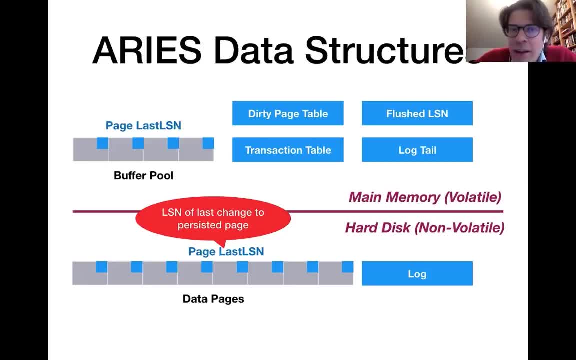 and how it will exploit those data structures during a recovery. So this is what we are going to do next time and in the following- probably the following two lectures, we will keep discussing about this idea. Have a nice day, and then I'll see you again on Wednesday. 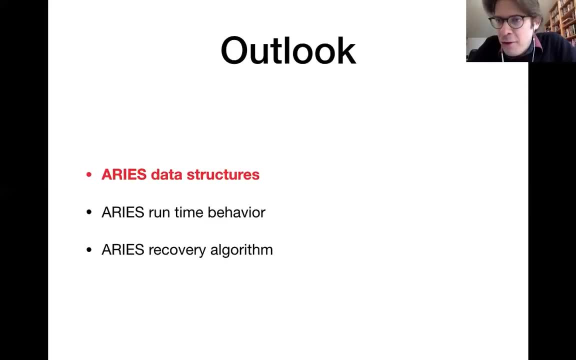 Good, all right. so today we're going to continue discussing about recovery, and that essentially means that, after the system crashes, we want to restore the database into a consistent state. We want to guarantee durability, which means that the changes of committed transactions persist, and atomicity, which means that we 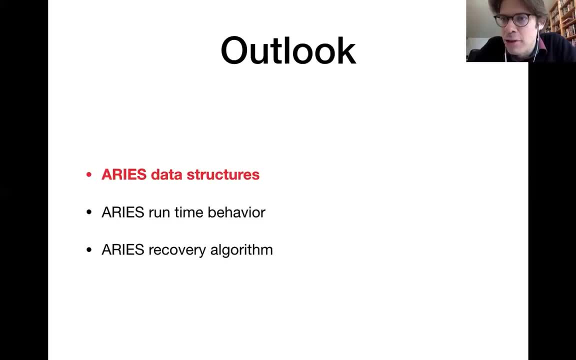 won't have the effects of any partially executed transactions. Now, the component which guarantees that is the recovery manager. and the last time we have started discussing about one of the most popular algorithms for recovery, which is the areas algorithm, And in the following we're going to discuss: 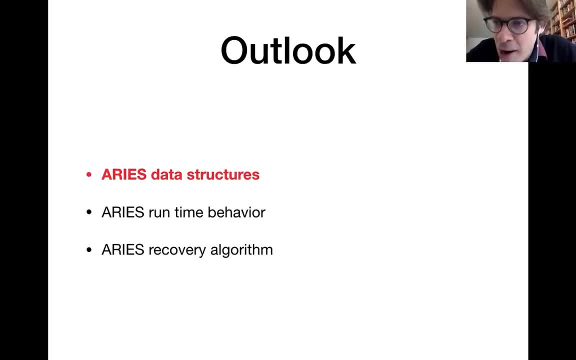 this algorithm in detail. it has quite a few moving parts, so it will take a lot of time. So let's get started. First, we'll discuss the data structures- we already talked about that a little bit last time- and we're gonna discuss about the runtime. 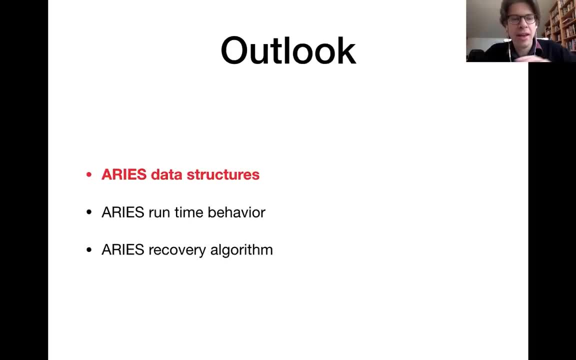 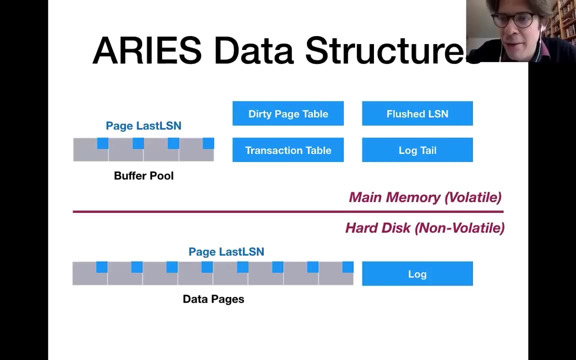 phase of the algorithm, as long as everything is going well, and then, finally, we will talk about the recovery phase, so how we bring the database back into a consistent state after we had a crash. So this over here is a high level overview of all the data structures that the areas algorithm uses. 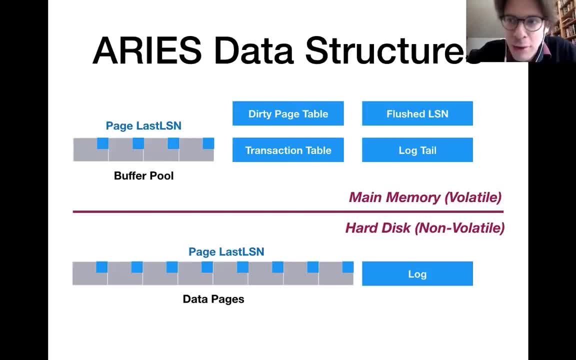 You can see, it's a couple of different data structures. Some of them are stored in main memory and some are stored on hard disk, and everything which is in main memory will be lost during a crash by the things on hard disk persist. Now here, first of all, two components that we have seen before. 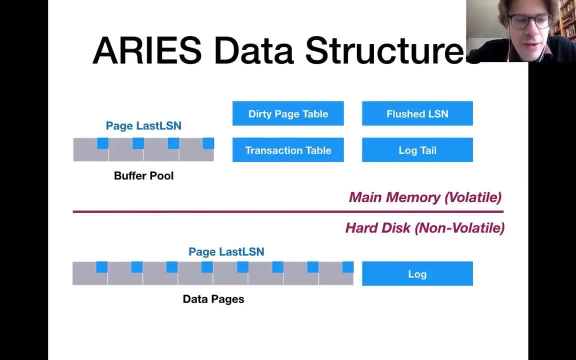 which are not directly part of the areas algorithm. We have the buffer pool, which is the data structure of the areas algorithm. We have a portion of main memory reserved for the database system and we have slots in order to store pages of data, and on hard disk, we have, of course, the data. 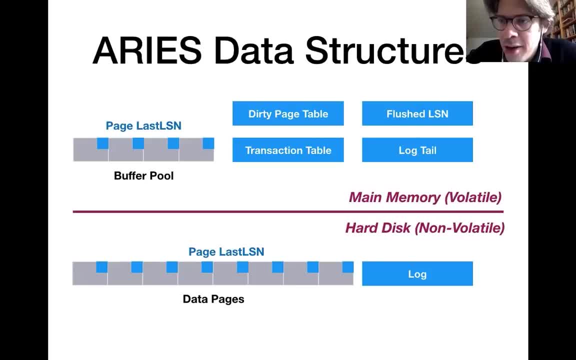 pages themselves. Everything marked in blue is specific to the areas algorithm and in the following we're going to quickly go over those different data structures and say what they are all about. First of all, we have seen that the idea, in order to be efficient and still 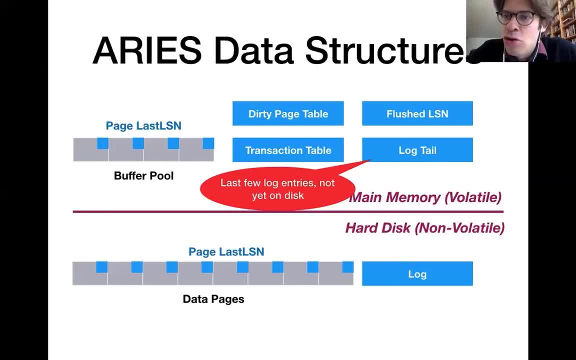 allow a recovery after a crash is to do logging. So we produce small entries that essentially describe what changed and when. we generate those entries. first of all they are stored in main memory in the log tail buffer, So the last few log entries will always be buffered here. 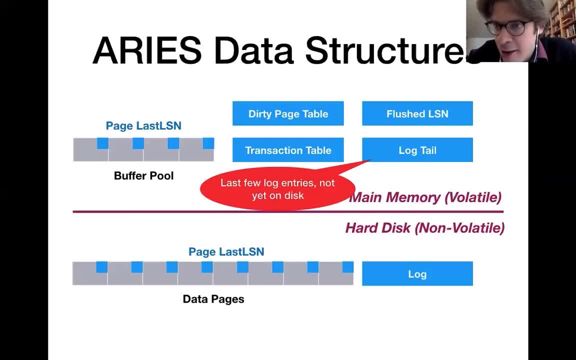 in main memory. That means, of course, that they are not yet persistent. so if the system crashes then we would lose this last part of the log. The flushed lsn essentially tells us until which log entry the log has been persistent. So each log entry is associated with a. 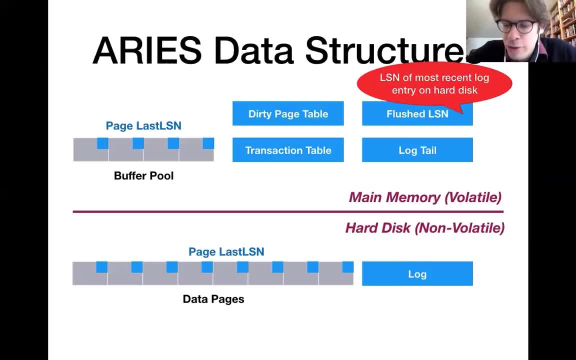 so-called lsn, which means a log sequence number, which is just some monotonically increasing id number for those log entries. If you imagine the log as a text file, then it could for instance be the line number And the flushed lsn essentially tells us. 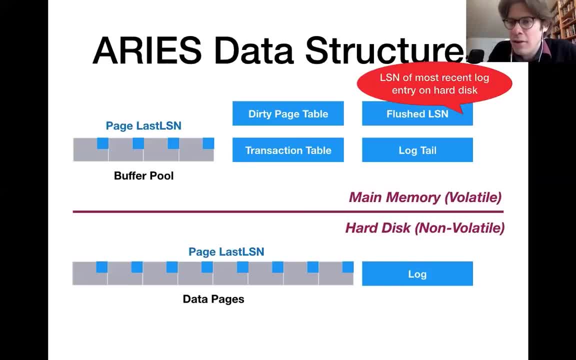 up to which line. we have written the log to hard disk already, where it will be safe in case of a crash, And in order to make certain guarantees, it's very important that we keep track which part of the log is currently safe and which part of the log is currently. 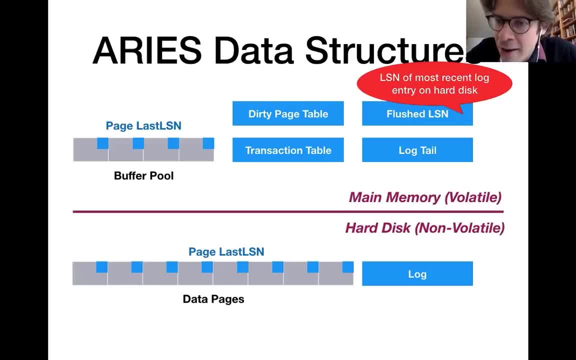 in volatile storage And this flushed lsn that keeps track of that last log entry that was written to hard disk And that here, as already discussed, is the hard disk portion of the log. So those are the log entries that will be used during the recovery. Every once in a while we are writing out. 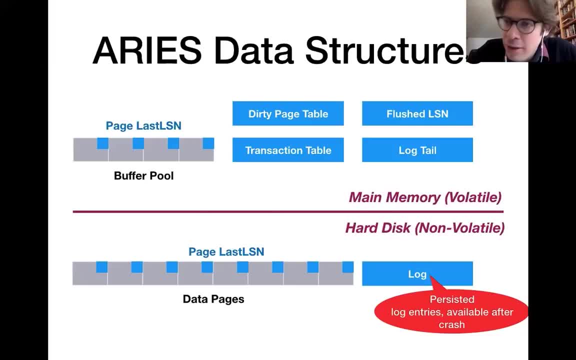 the content of this log tail buffer to a hard disk. We say that we flush it and here on hard disk we have the persistent portion of the log. We have a transaction table data structure which essentially gives an overview of active transactions, So it's stored for each transaction that is currently. 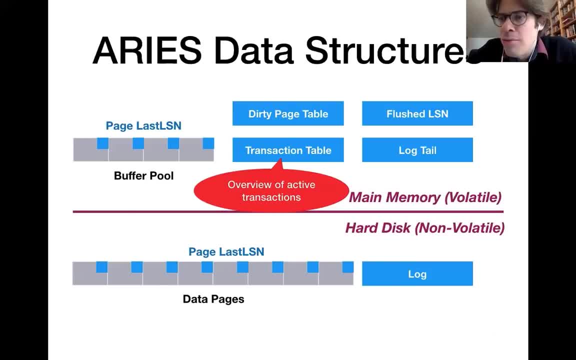 executing some additional information which makes it easier to recover operations from that transaction. So we have a dirty page table that keeps track, essentially, of pages that are currently on hard disk and in memory, And the in memory version differs from the hard disk version, So that happens if we have loaded one of 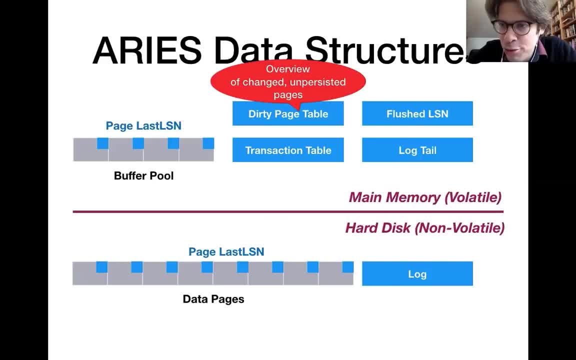 those data pages from hard disk into the buffer pool and then we changed it. at that point it becomes a dirty page because we have two different versions And if we had a crash at this point then the main memory version would be lost and along with it all the associated changes. 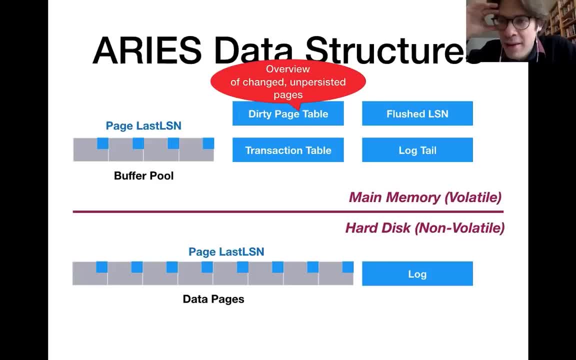 So dirty pages. these are pages where we might have problems in case of a sudden crash. For other pages we still have the most recent version on hard disk and that version will still be available after the system comes back online. Then, for each of the pages in our buffer pool, we now introduce: 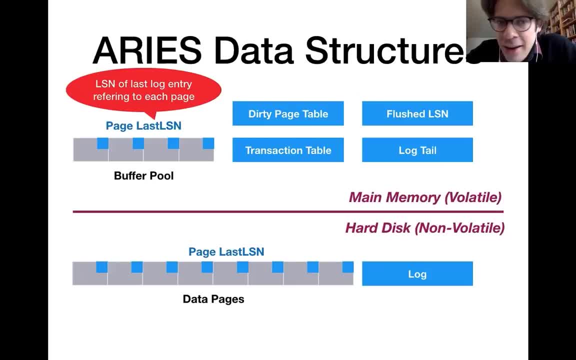 the page last, lsn, or page lsn, which essentially indicates, for each of the currently loaded pages in the buffer pool, what was the last log entry that changed this page. So when we are keeping track of log entries, we are always referring to them by the log sequence number lsn. and here we 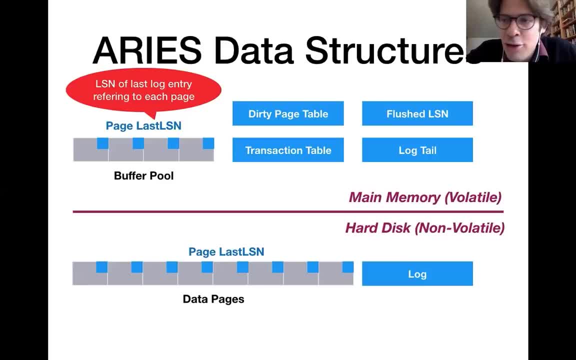 keep track of the last lsn that affected each of those buffer pages. And we don't only have this in memory but we also have this on a hard disk. so the on disk version also captures the last lsn that affected this on disk version. And if we have a page in a version on hard disk and in a 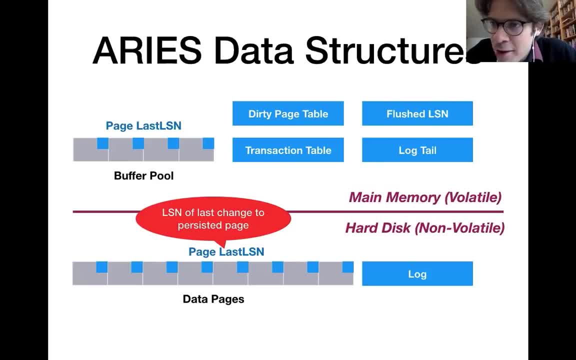 version in memory. then we can use this page lsn to decide in certain situations how much those two pages differ, for instance. So basically this is like a timestamp of the last change All right now. so in the following I'm gonna discuss those data structures in more detail. That was now the 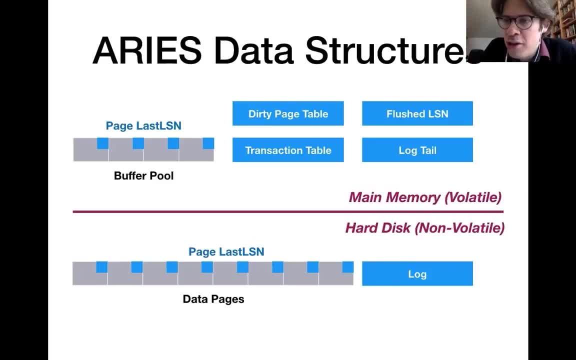 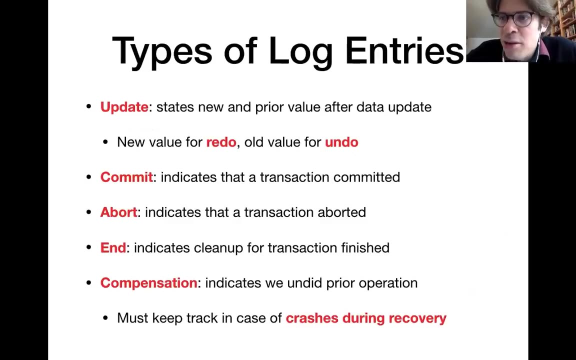 high level overview. We are now gonna go more into detail, Starting with the structure of the log. So far, I've generically talked about log entries, So let's see how they actually look. So, first of all, there's multiple types of log entries, depending on the event that they are describing. So 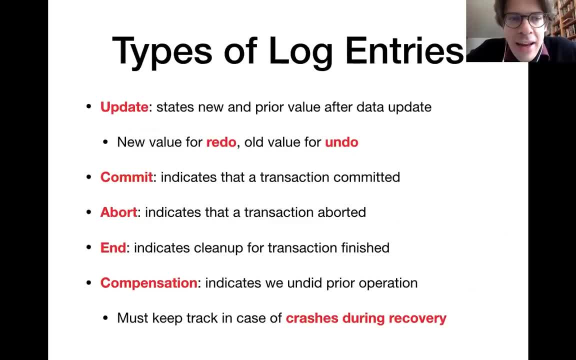 for instance, if we are updating data, then associated with that, we generate an update log record. This log record contains fields to store the value before and after an update, which is important because we might have to redo operations whose effects were lost due to a crash. But 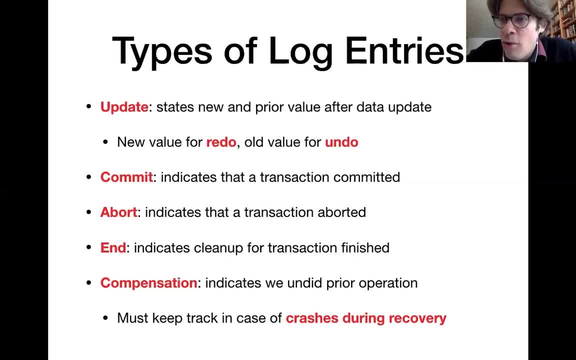 we also might have to undo operations of transactions that have only partially executed once the crash comes in, And in order to make an undo we also need the old value before the corresponding change. That's why the update log records store both the old and the new version of the value. If a transaction commits, then we also 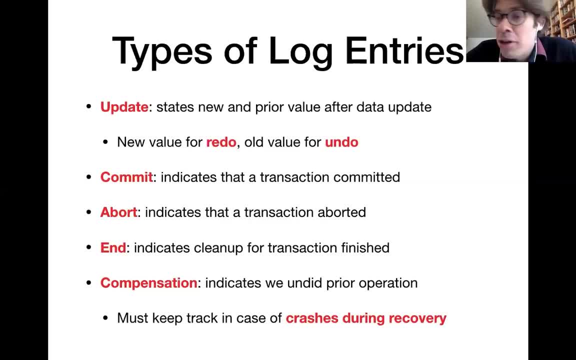 need to keep track of that in the log. During recovery, we essentially need to decide for each transaction: is this a transaction that had already committed once we crashed, or is this a transaction which was still running during the crash? In that case, we want to abort it. So it's. 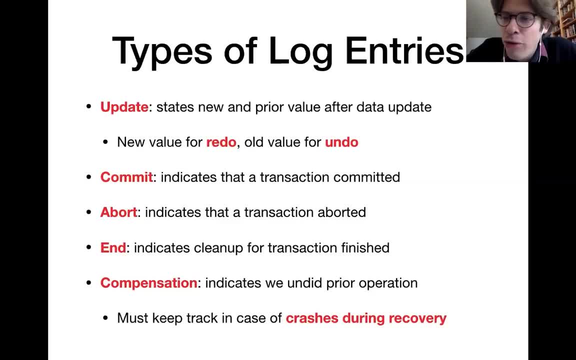 very important that we keep track in our log of those transaction commits. The other side transaction might also abort. We also keep track of that with the corresponding log entry. And so far we always have talked only about transaction commit and transaction abort. Here we 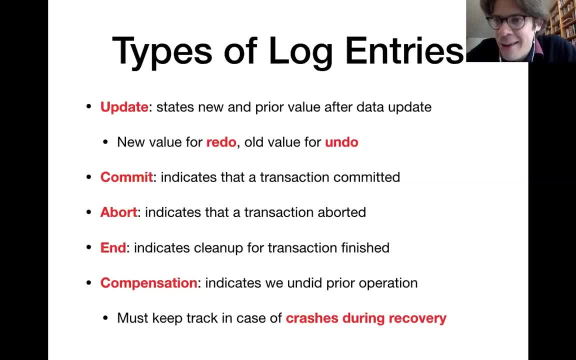 additionally have the transaction end, And that is something which happens after the commit and after the abort. It is essentially indicating that the recovery manager has now done everything that it needs to for a transaction, For instance, for an aborted transaction. that would mean that we have a 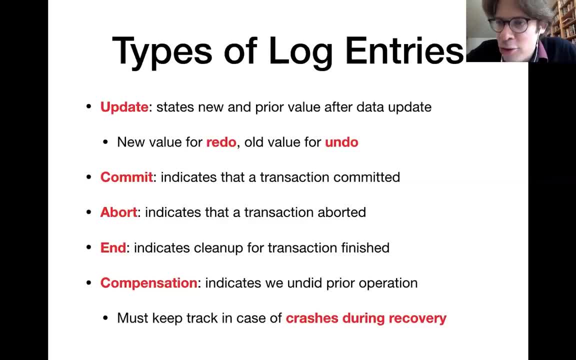 undone all of the associated changes, And so essentially the end log record for transaction means that everything is done and we can now forget about this transaction. One final type of a log record is the compensation log record, And that essentially keeps track of when we 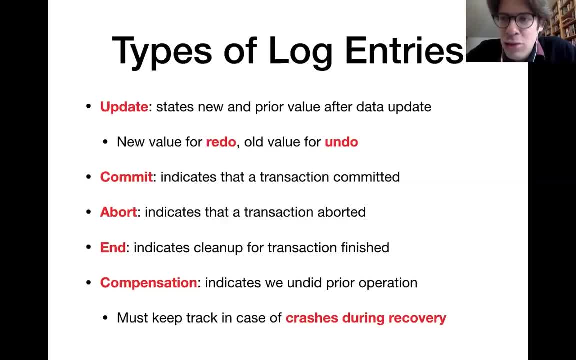 undo the operations of transactions. Doing that is important already because while you are recovering your data base system after a crash, in some cases, if you're really unlucky, you might have another crash while you are recovering your database. Perhaps the reason for the first crash is that. 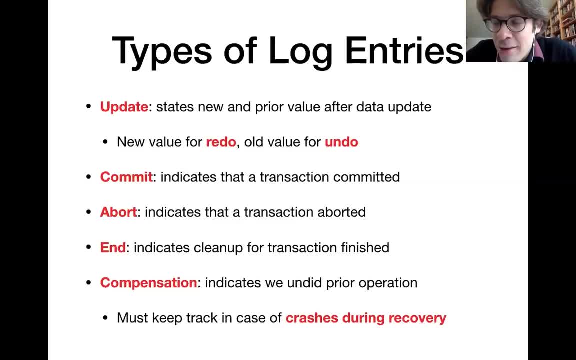 the power supply is currently unstable and maybe it remains unstable for a certain amount of time, So then it might actually increase the chances that you have another crash while you're currently recovering things And those compensations or log records, among other things they allow us. 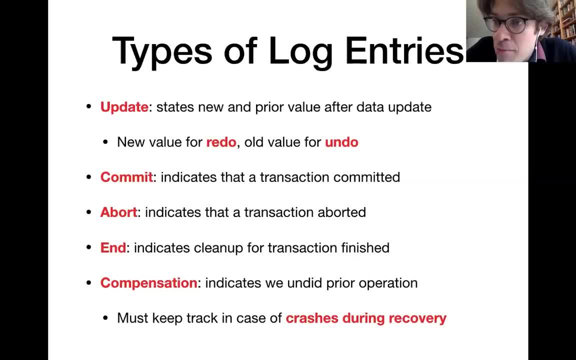 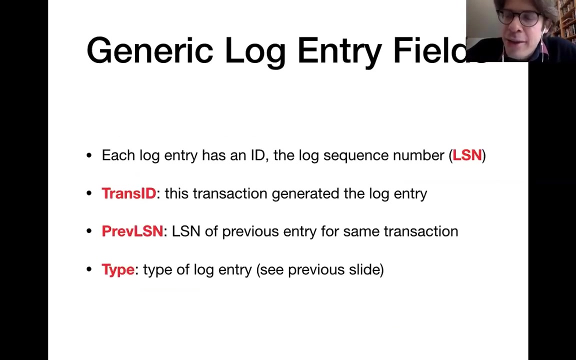 to keep track of which operations have already been undone, such that we don't try to undo the same thing multiple times if we can avoid it. So compensation log records essentially keep track of which undo operations. we have already done Now the structure of a generic log entry that applies to all of those different. 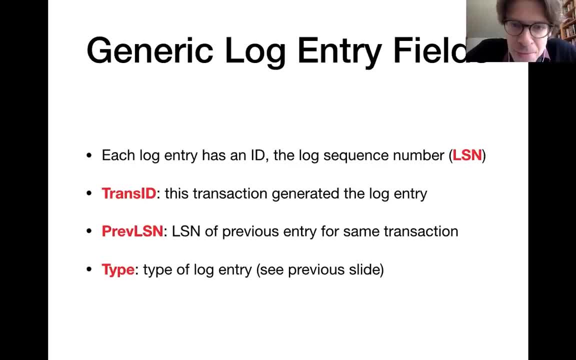 types of log entries that we have seen. First of all, a log entry has a log sequence number. of course, that is the id by which we reference specific log entries. Then log entries always relate to specific transactions, which can, for instance, be the transaction which updated the data And the transaction id in the log entry. 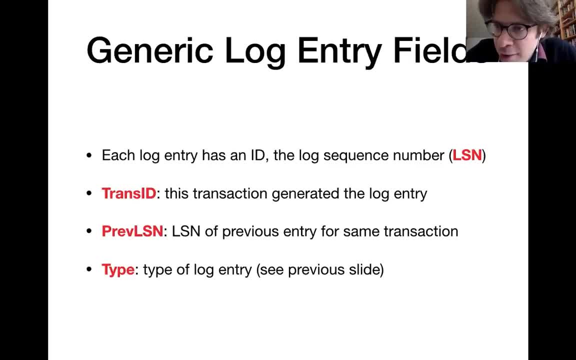 is the log entry of the transaction, So it keeps track of which transaction is associated with the event that we are logging. There's also a field named pref lsn, and that is essentially a pointer back to the last log entry that was generated by the same. 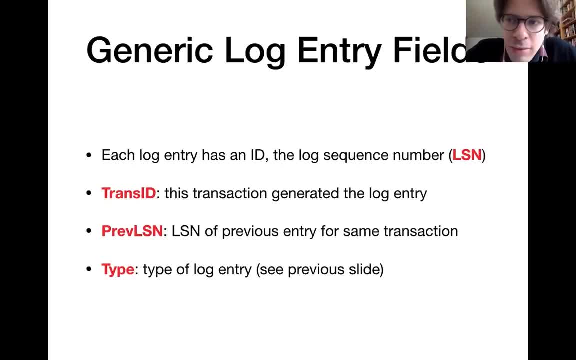 transaction. Now, very strictly speaking, that would not be required, but it often makes things more efficient because, for instance, if you want to undo the operations of one transaction, you undo them in reverse order, and this is when you want to jump ideally through your log only to the operations by that specific transaction. 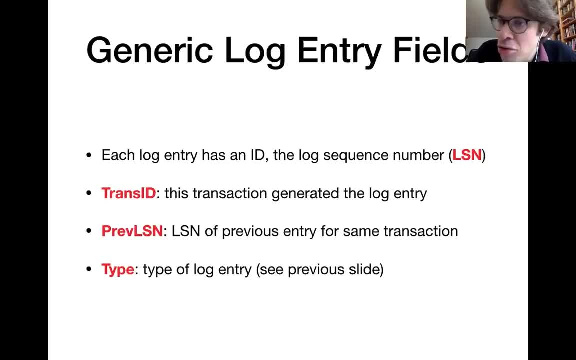 And this pref lsn field essentially allows you to do that. So this is for efficiency reasons. And then, of course, since we have seen there's multiple types of log entries, we need to keep track of which type we currently have. So we have also a field in order to store the type of the log entry. 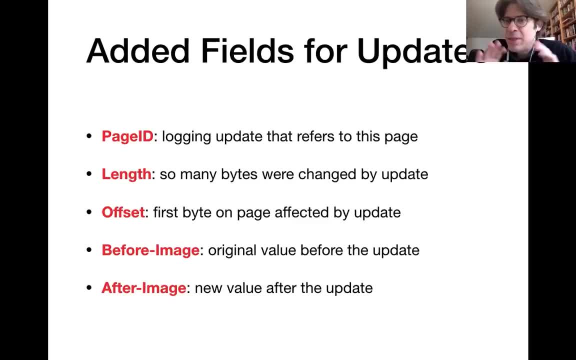 Specifically for update log records there is a couple of additional fields. If you have an update, it always refers to specific bytes on a specific page. So in that log entry we additionally store the page id to which the update refers. The length indicates how many bytes were changed. 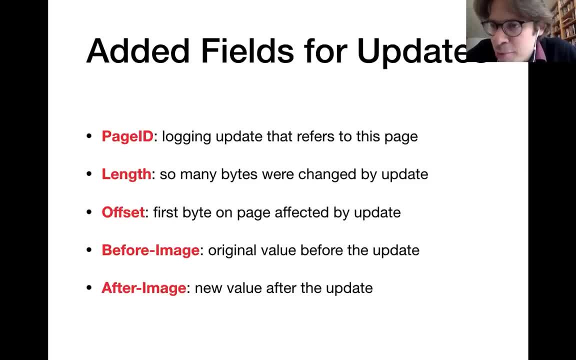 and we assume it's a consecutive bytes for one specific log entry, An offset indicating what was the first byte that we changed on the page. And then, as discussed, we need the before image and the after image, which means essentially the value before and after the update, such that we can. 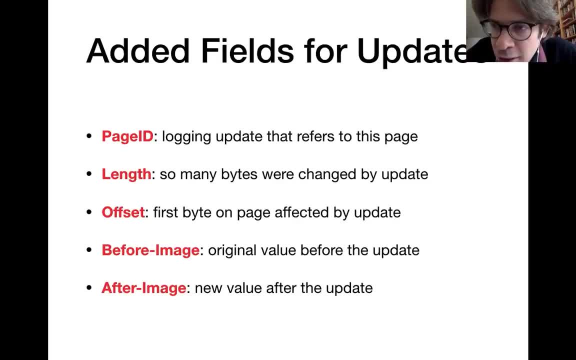 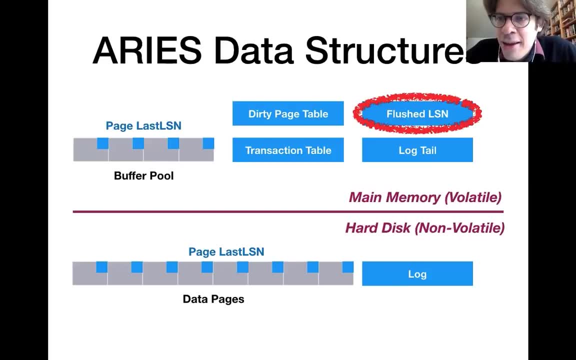 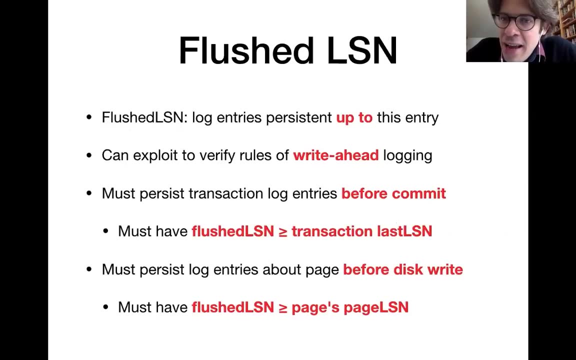 redo the operations or undo the operation if we need to. So that was the log. The flushed lsn is relatively quick to explain. It essentially just indicates up to which log sequence number we have already written log entries to hard disk. And as a little reminder, 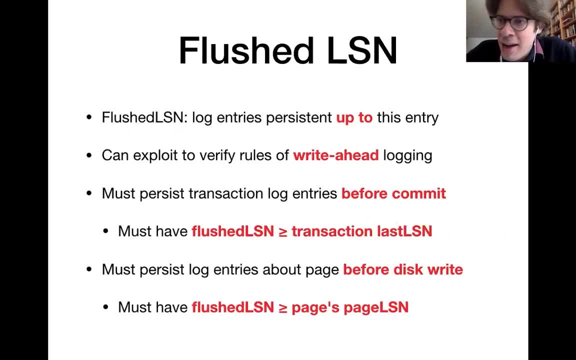 we have started last time the recovery chapter by discussing about right ahead logging And that generally means that the following two rules: when we do logging, Before a transaction commits, we write all the log entries about a transaction to permanent, to persistent storage, And before we write some page from our buffer pool to hard disk, which 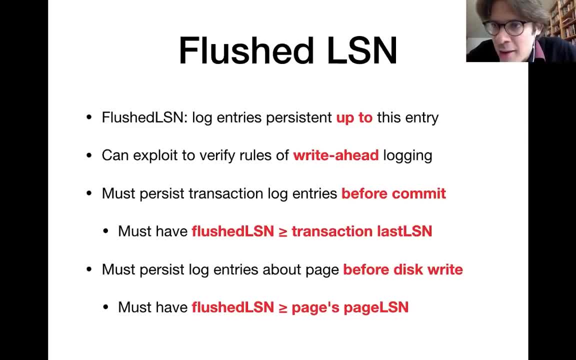 might contain changes by transactions that are currently not committed yet. Whenever we do that, we first should write to hard disk all the log entries that we have already written. should write to hard disk all the log entries which concern the page that we are about to write to hard disk. 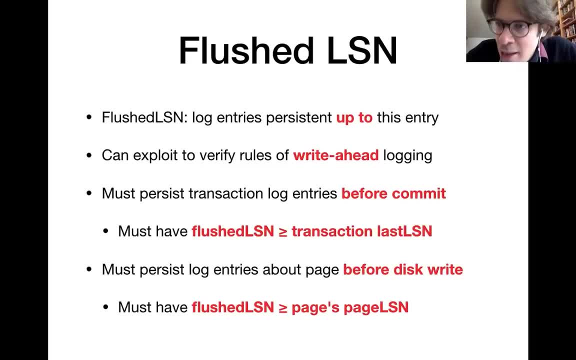 And the flushed LSN essentially allows us to keep track whether those two conditions are satisfied, And if they're not satisfied, then we can react by writing more log entries from monetized storage to hard disk. So first of all, we need to persist. 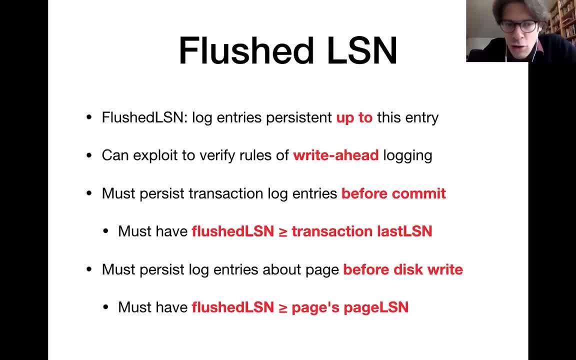 log entries that refer to a transaction before a transaction commits, And we can test that by looking whether the flushed LSN is greater or equal to the last LSN of the corresponding transaction, The last LSN of the transaction which is stored in the transaction table. 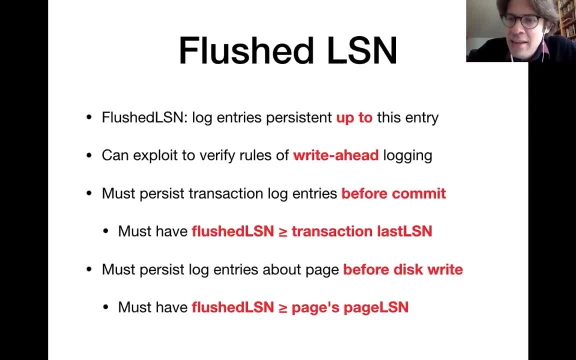 that I'm going to discuss in more detail in a minute indicates essentially The last log entry generated by that transaction, And if flushed LSN is at least as large as that last log entry, we know that all log entries related to the transaction must have been written to hard disk. 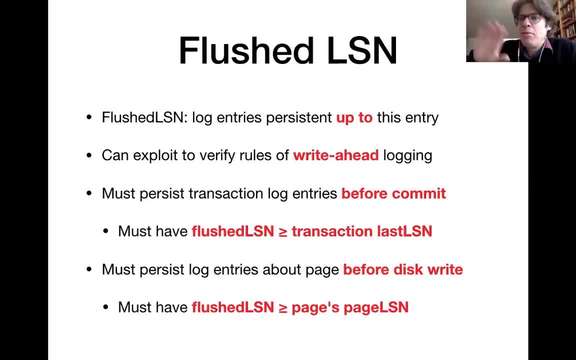 Now the other rule refers to the case where we write one data page from our buffer pool onto hard disk And for those pages we store the page LSN, Which was essentially the last log entry that affected the page, And if we can make sure that the flushed LSN is greater or equal. 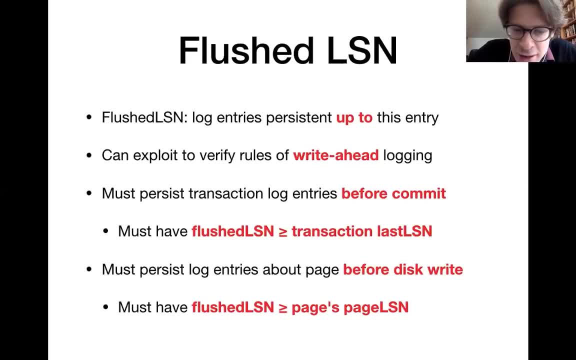 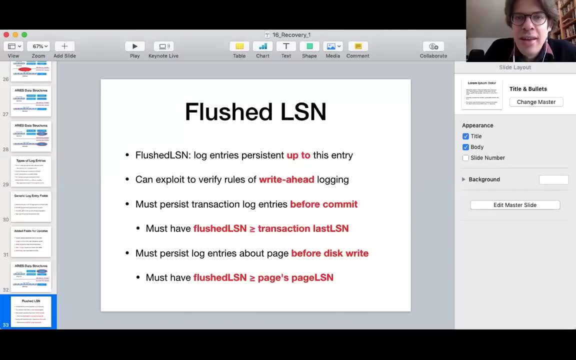 to the page LSN of the page that we want to write to hard disk. then we can be sure that all the log entries which refer to that page they have been made persistent. So the rules of write-ahead logging are satisfied. There might be a question in the chat. 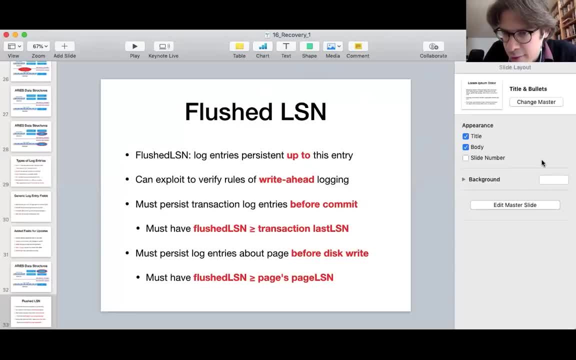 Yes, Yes, exactly. So a flushed LSN essentially gives you the last log sequence number that was written to hard disk And after that, since the log entries are in volatile memory, so if there's a crash then they will be lost- 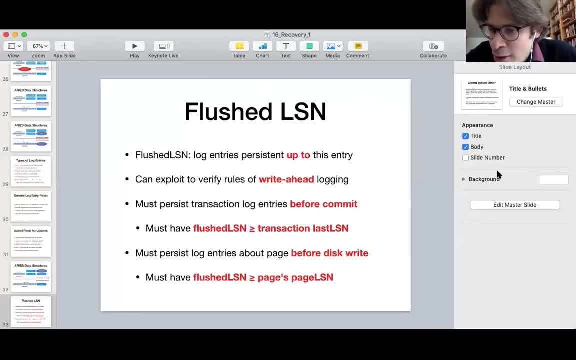 And the question here Is whether the flushed LSN data structure is just a single entry And that is correct. So the flushed LSN- that is the simplest data structure that we have seen on the screen- essentially is just one single number. 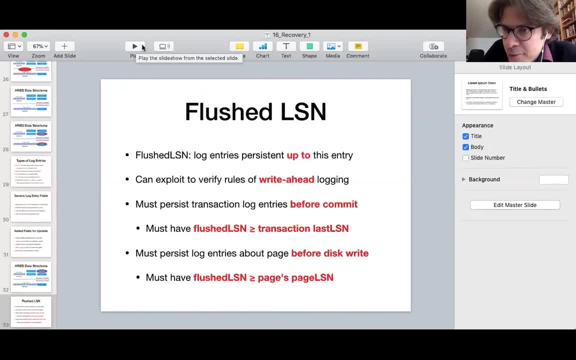 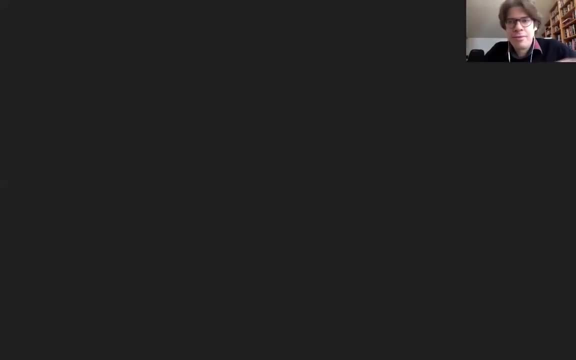 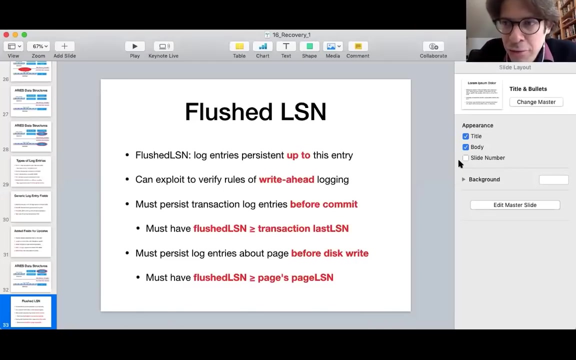 Very good question. Is there any other questions at this point about the data structures? No, No, No, Any other questions that we have discussed so far? All right, And yes, in general, with this algorithm, I encourage you to ask questions once something is unclear. 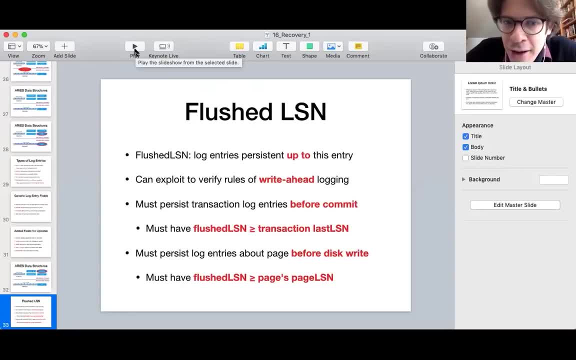 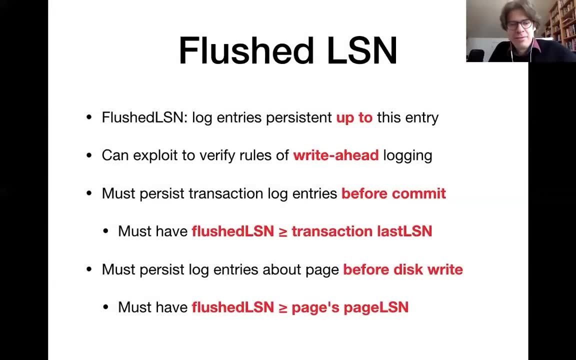 Because it has lots of moving parts that build on each other. So, yes, don't hesitate to ask questions in the chat. Good, So this is the purpose of the flushed LSN, which essentially is just one single number stored in main memory. 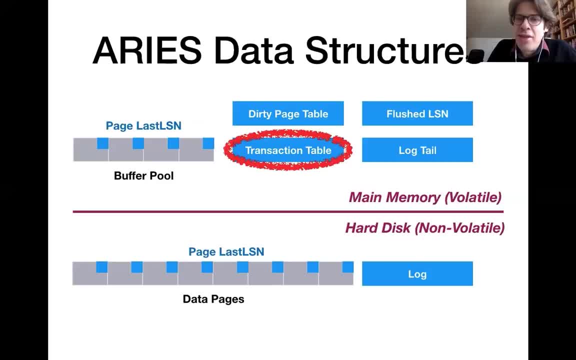 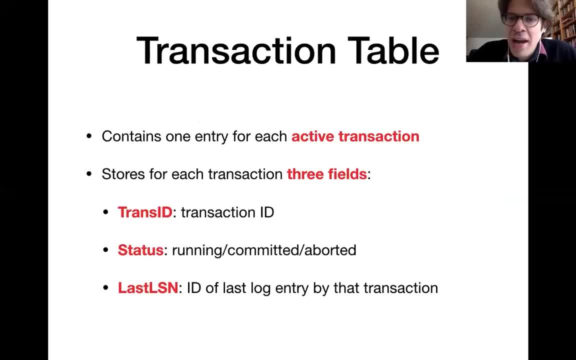 All right, now let's discuss a little bit about the transaction table. So the transaction table contains entries for active transactions And for each of those transactions it essentially stores three fields. First of all, it stores the transaction ID. Then it stores the status of the transaction, which can be running, committed or aborted. 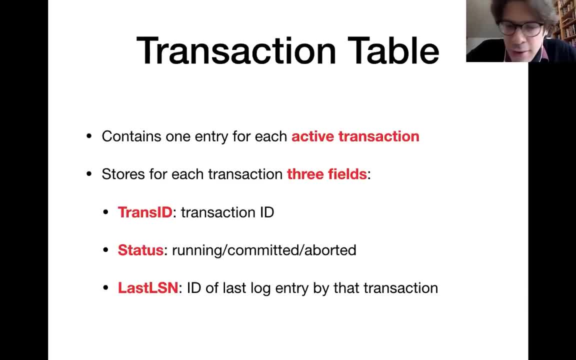 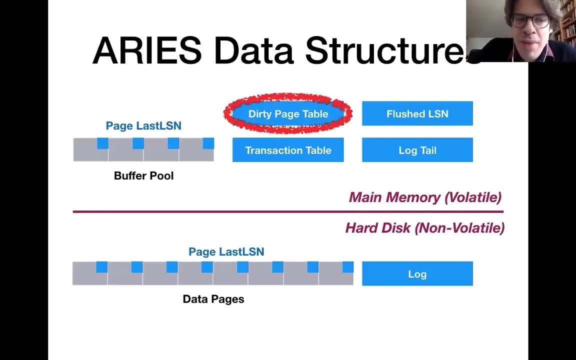 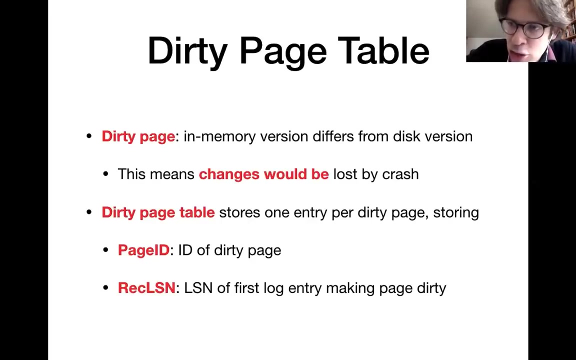 And then it stores the last LSN of that transaction And that is essentially the last log entry generated by that transaction. That is the transaction table. The dirty page table stores information about pages that are currently loaded on the LSN. A dirty page is generally a page where the in-memory version differs from the hard disk. 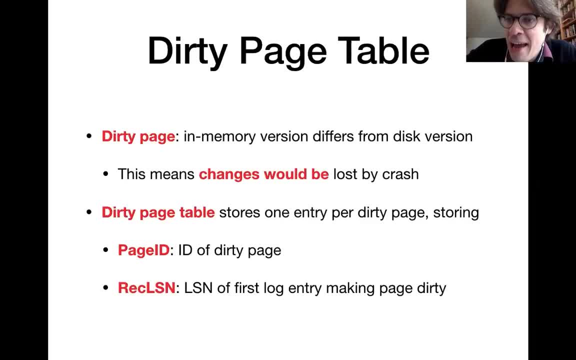 version, which means that the changes that we currently have in the in-memory version would be lost in case of a crash. So the dirty page table stores one entry for each of those dirty pages. First of all, of course, the page ID. 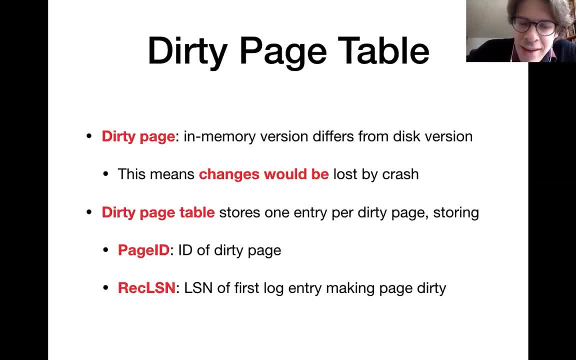 And then the so-called rec LSN, And that is the, The earliest log entry which made the page dirty basically. So, starting from that log entry, the on-disk version starts deviating from the in-memory version, And that is very useful knowledge during recovery, because we know when it comes to the changes. 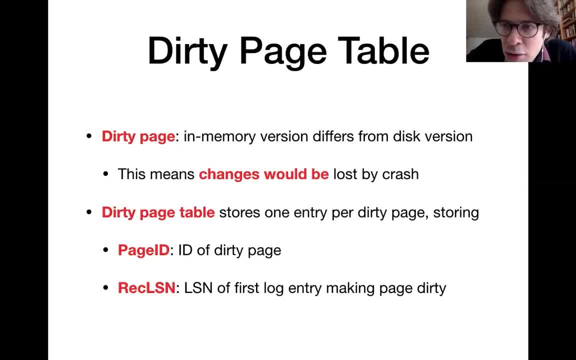 of a specific page, you only need to redo those changes, starting from the back LSN. All right. One source of confusion in my experience when it comes to this data structure- that's why I'm proactively pointing it out- is what happens if you have multiple updates to the same page. 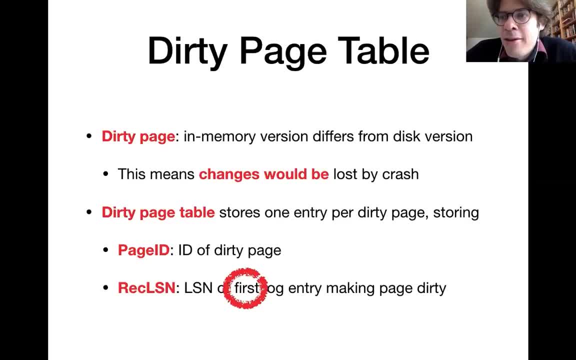 It is easy to make the mistake to believe that the rec LSN, for instance, changes if you have multiple updates to the same page. That's tempting, But actually the rec LSN is set only once a page becomes dirty for the first time. 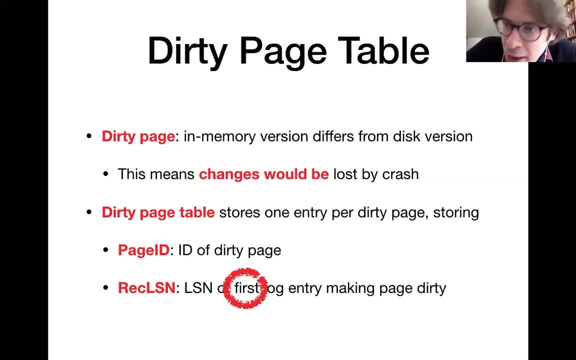 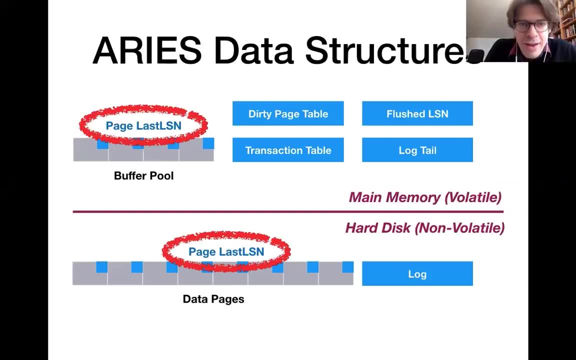 Once there's further updates to the same page, we don't change the rec LSN anymore. Just pointing out one possible source of confusion there. All right, That was the dirty page table Now. finally, let's discuss a little bit about the page LSN, or page-last LSN. 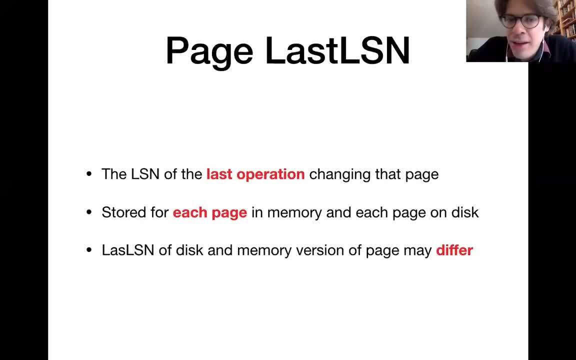 We just Essentially, you see. Okay, So the page that changes the last operation has been changed. It's actually just the block sequence number of the last operation that changed the page. This is stored in memory and on hard disk. If I have the same page on hard disk and also in an in-memory version, then those two might. actually differ, So we always adapt the one in main memory. if there's updates and if at some point one of those pages get written to hard disk, we can still add it. We don't have to do that right now disk. then we essentially override the old page lsn on hard disk. 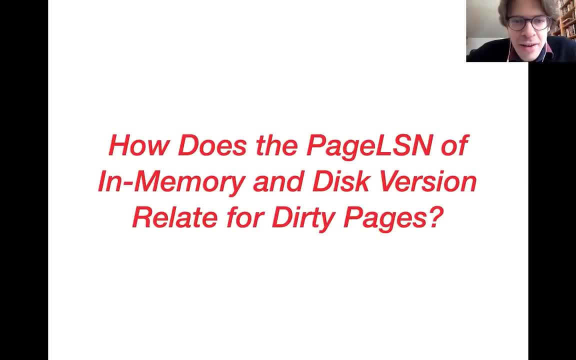 one little question, um, to test your understanding. so, um, if we consider the page lsn of the in memory and of the disk version of the same page, um, what can we say about the two, about how they relate to each other, if we know that the page is dirty? 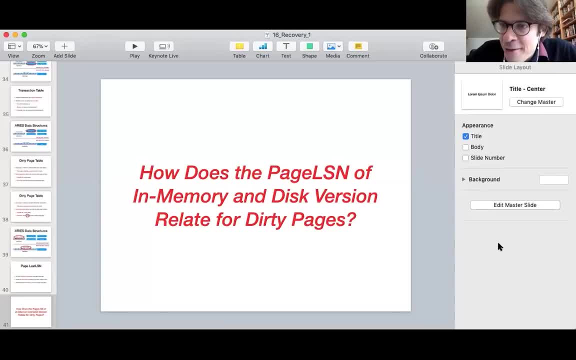 exactly, so the last lsn for the page in memory will be a strictly greater um than the last lsn or page lsn of the corresponding disk page. exactly, yeah, good. so now we have discussed all the data structures of the aries algorithm. in the following we're going to discuss: 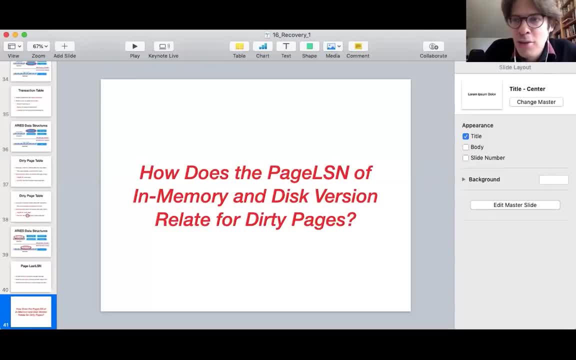 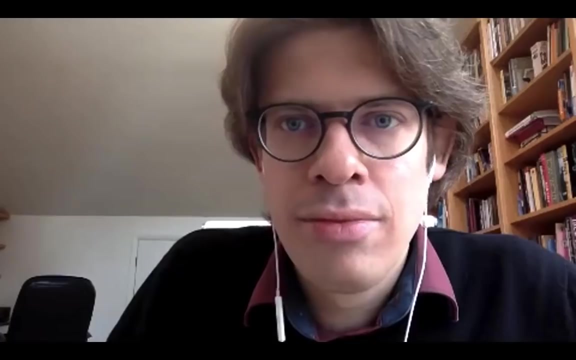 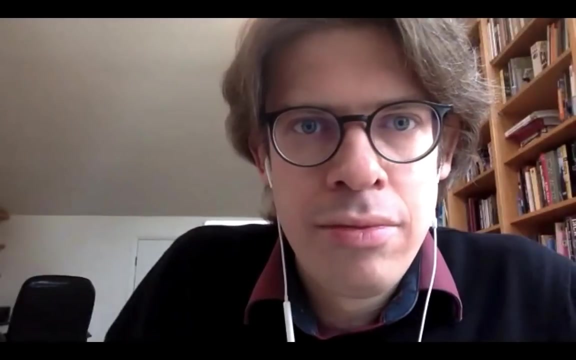 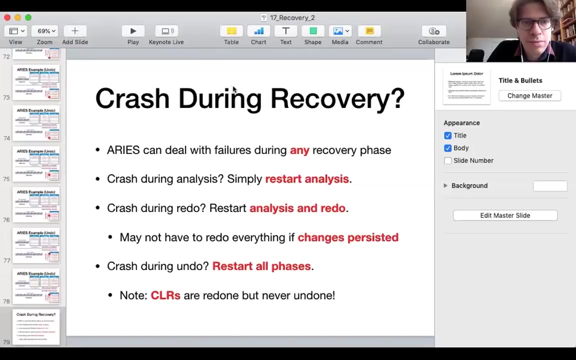 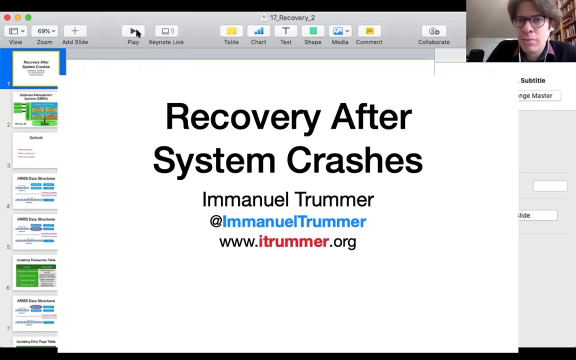 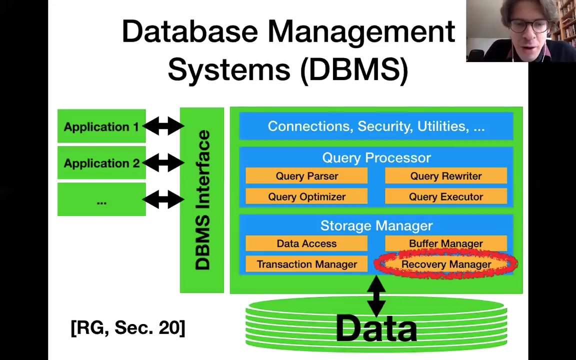 about how they are updated, so i'm quickly changing my slide deck here. um, let me know if there's any questions. so far okay, so all right. so we continue discussing about the ARIES algorithm. so we are still talking about the recovery manager and the relevant chapter in Ramakrishna and Ikyaki is still 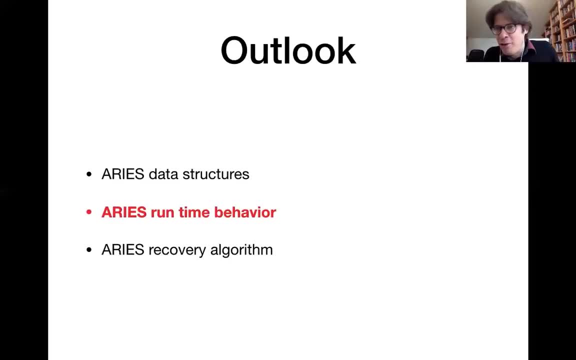 number 20.. So we have discussed about the data structures of the ARIES algorithm. now, in the following, we're going to discuss about the runtime behavior. so when I discuss about how we update those data structures under normal conditions until there is a crash, and once we have a crash then we enter the last phase- 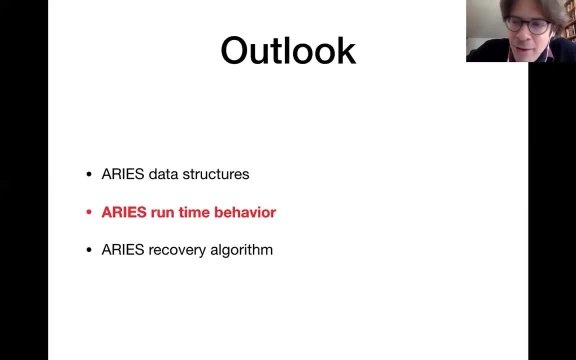 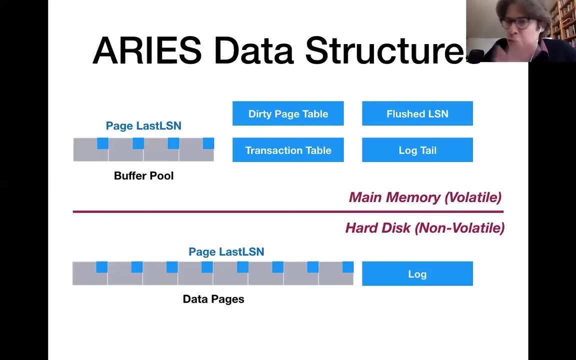 which we will discuss later, which is when the ARIES algorithm uses the log in order to recover the database. Alright, so those are the data structures that we have seen and on the following, we're going to discuss about how they are being updated, starting with the transaction table. So the transaction table. 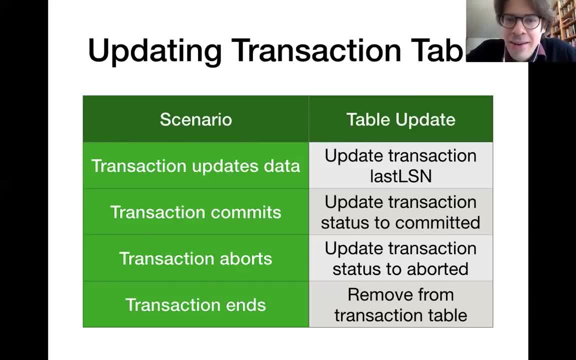 keeps track of which transactions are currently active and when they have last done generated any log entries. So we have four possible scenarios when it comes to the transaction table. So on the left side you see an event and on the right side you see how we need to update the transaction table in case of that event. 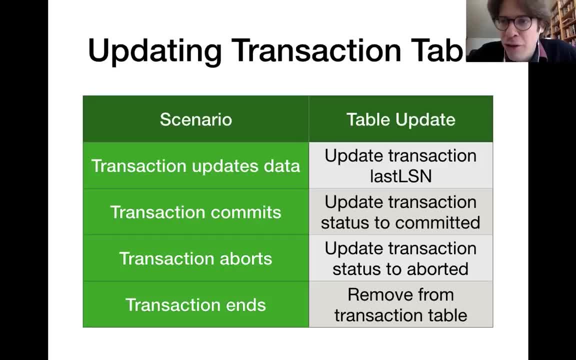 So, first of all, it might happen that a transaction updates data, so in that case we simply have to update the last at its end of the corresponding transaction. That's the kind of event, look, we're looking for in a log entry, since at the other end, the conversion today will end at. 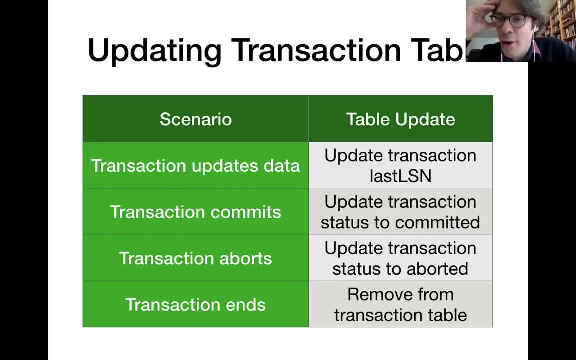 end of that period. So you can basically look at the transaction. only month. ELSI also shows that at the end there is a log entry away and for those given sex family symbols you get a brought back date small. then we have problems. If a transaction commits, we would update the status of the transaction to a one time Done for могifiable connection. 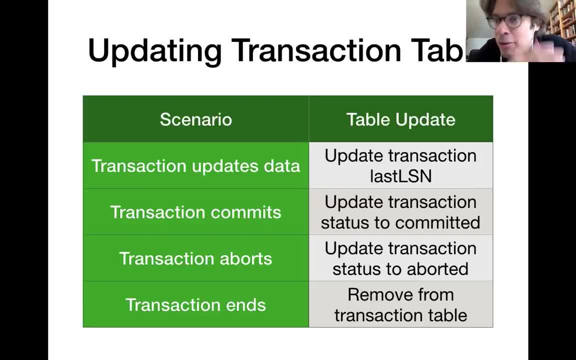 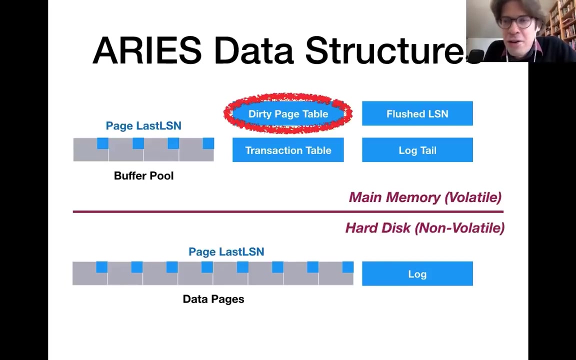 all the clean up we need to do for this transaction after the commit or after the abort. if that happens, at that point we reconsider the transaction as finished and we can remove it from the transaction table. that is how we update the transaction table all right. now for the dirty page table. there is the 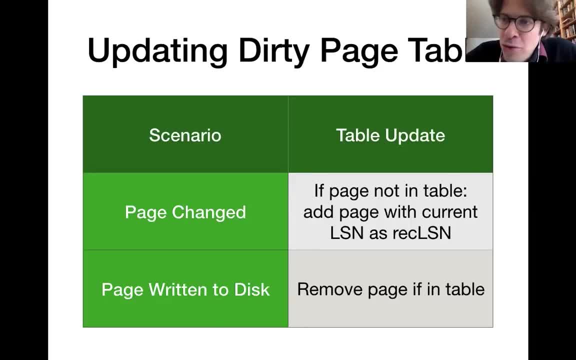 scenario that a page changes, then what we do is that we first of all check in the dirty page table whether the page is already in the table. if that is the case, we don't actually need to do anything because, as I quickly mentioned before the reg lsn, which is the earliest time at which the page became dirty, that 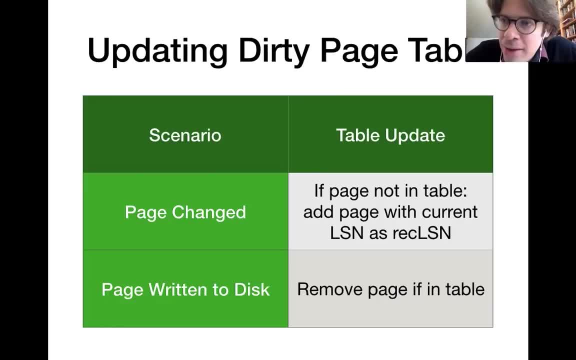 doesn't change in case of further updates, but if the page is not in the dirty page table, then we have to insert it and the vsept. it's a rec lsn to the current log sequence number, because this is when the page became dirty. the. 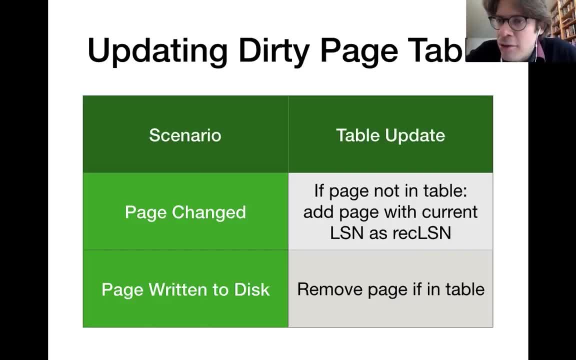 other side of it is a page gets written to hard disk. so a dirty page by definition was always a page where the in-memory version differs from the hard disk version. and if you write one of those pages back to hard disk then essentially the current in-memory version overrides the on. 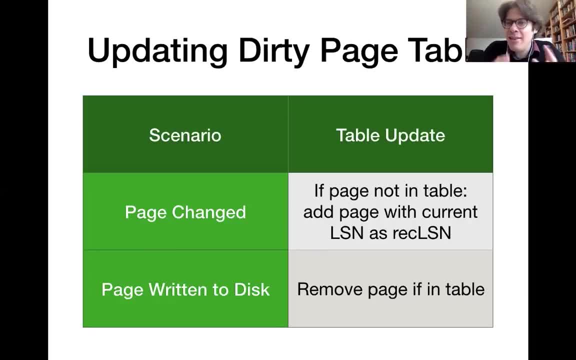 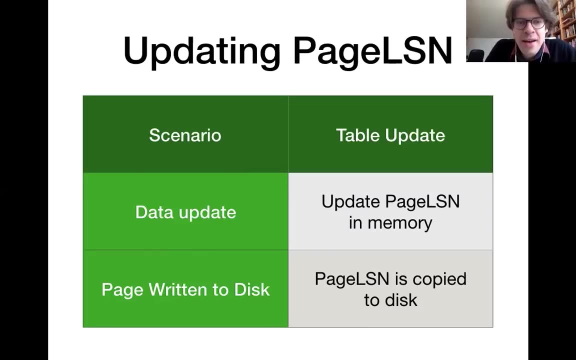 disk version. it means that now there is no difference anymore between the two. this is why we take out the corresponding page from the dirty page table. now for the page last, that is an or page lsn. here we need to keep track of the data update, so whenever we have, 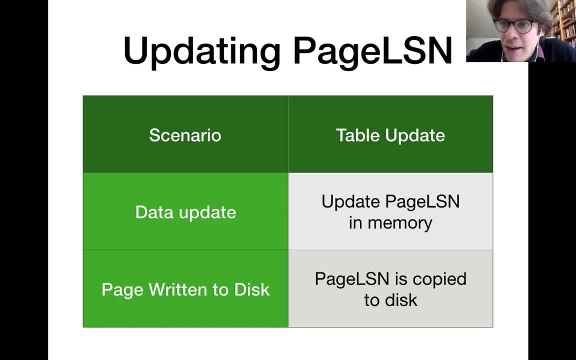 a data update, we need to keep track of the data update. so whenever we have a data update, we need to keep track of the data update. we need to keep track of the data update. we need to update the page at us and in main memory- so important- we don't update the page at us and on hard disk that 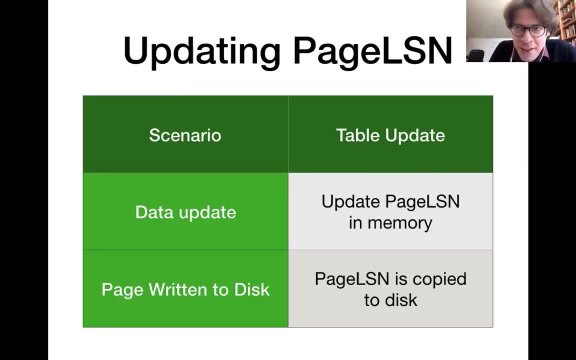 would be bad for performance because we would have a disk writes. instead, you only update it in main memory and then every once in a while one of those in-memory pages overrides the disk version and then that happens the corresponding page at us and also overrides the on disk page. 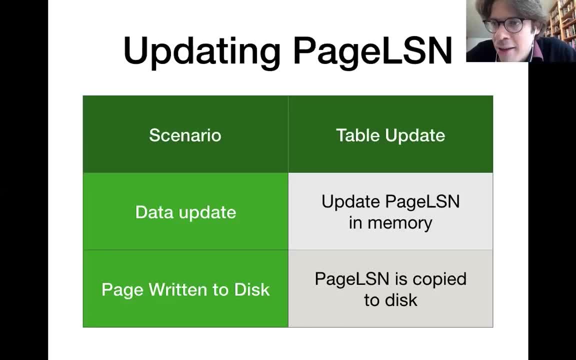 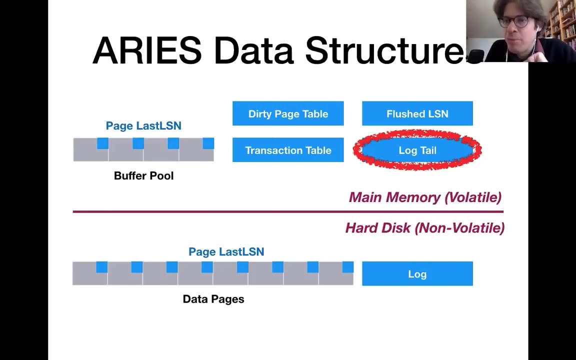 Edison right, so those a disk page. Edison right, so those a disk page at us, and the only updated than ever, the right one of those at us and the only updated than ever, the right one of those pages in our buffer pool back to hard disk. pages in our buffer pool back to hard disk. all right now. the noctail is the portion of the log. 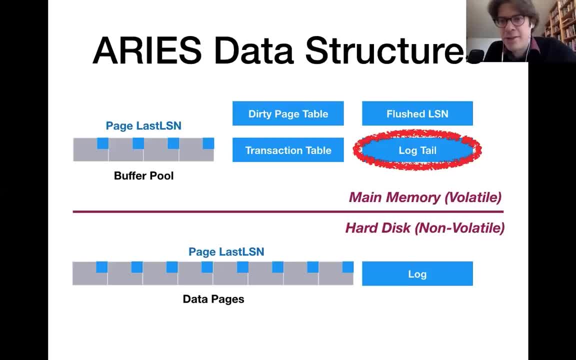 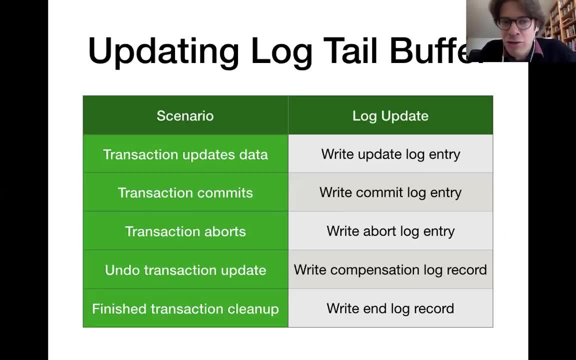 all right now the noctail is the portion of the log which has not been made persistent yet. so this which has not been made persistent yet, so this is still in a main memory and in general we have is still in a main memory and in general we have to generate log entries essentially whenever one. 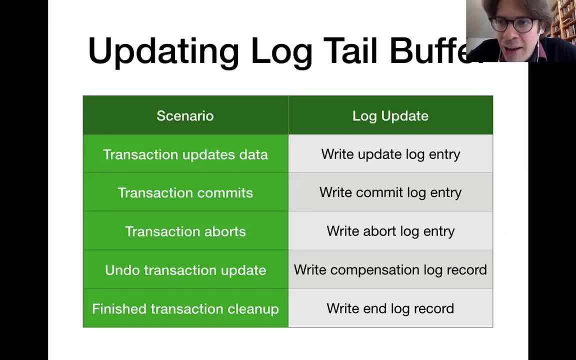 to generate log entries, essentially whenever one of the event of the event occurred that we have lock entries associated with. we have seen those different occurred that we have lock entries associated with. we have seen those different types of log entries, types of log entries and, essentially, whenever a transaction updates data, we generate an update. 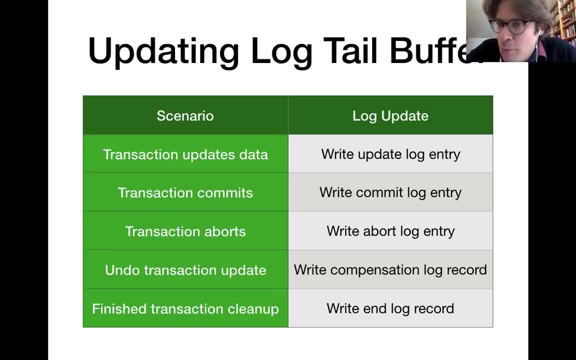 and, essentially, whenever a transaction updates data, we generate an update log entry. whenever transaction log entry, whenever transaction commits, we generate a commit log record. whenever one transaction commits, we generate a commit log record. whenever one transaction aborts, we generate an abort log. aborts, we generate an abort log record. and whenever we undo something, we generate a compensation log. 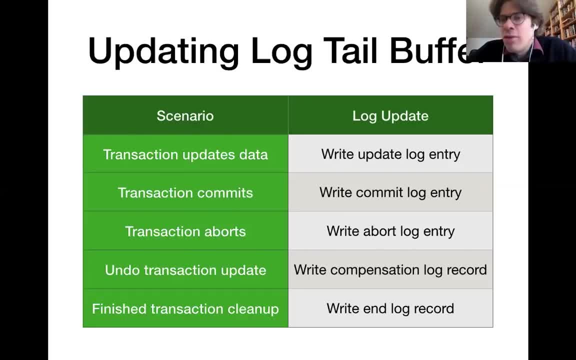 record. and whenever we undo something, we generate a compensation log record. um, whenever we finish, um, whenever we finish clean up for a transaction, we write the clean up for a transaction. we write the clean up for a transaction, we write the end block record. so essentially: end block record. so essentially. 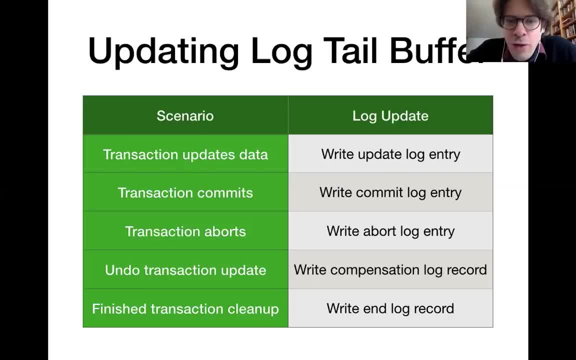 end block record. so essentially, we write log records for the different, we write log records for the different. we write log records for the different events, that we have specific types of log events, that we have specific types of log events, that we have specific types of log entries for. 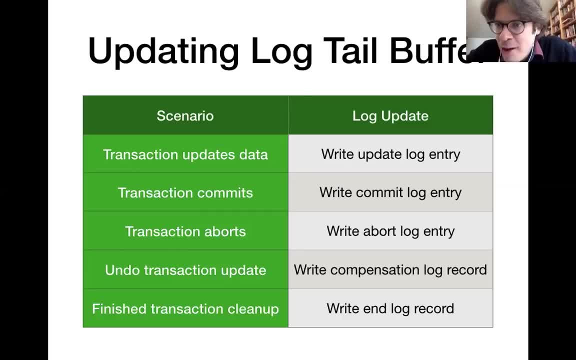 entries for, entries for: and first of all, we write them into this, and first of all, we write them into this, and first of all, we write them into this. lock tail buffer in a main memory. lock tail buffer in a main memory. lock tail buffer in a main memory every once in a while. uh, that buffer. 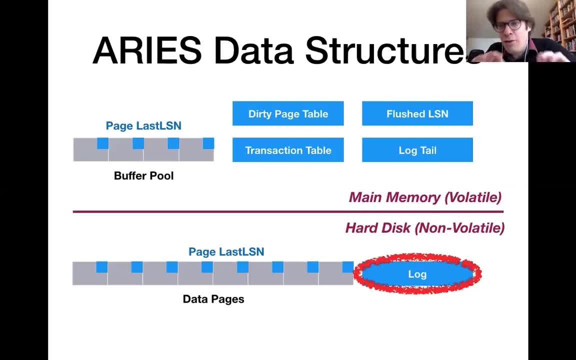 every once in a while, uh, that buffer, every once in a while, uh, that buffer gets written to hard disk, gets written to hard disk, gets written to hard disk, all right. so now, finally, let's come to all right. so now, finally, let's come to all right. so now, finally, let's come to the hard disk version of the lock. 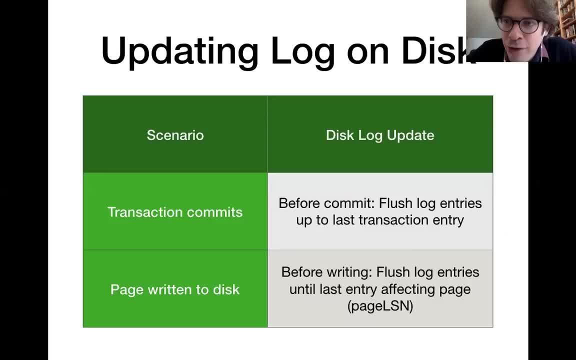 the hard disk version of the lock. the hard disk version of the lock. so um here generally. we need to follow so um here generally. we need to follow so um here generally we need to follow the rules of um, the rules of um, the rules of um of uh right ahead logging so whenever. 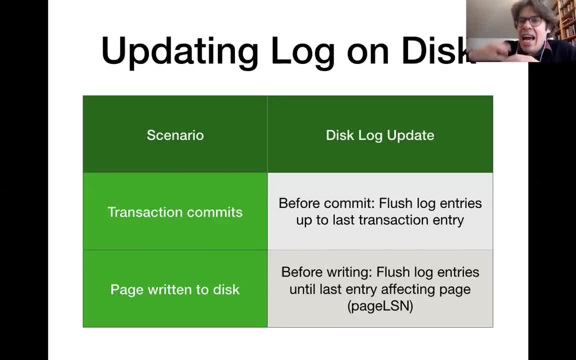 of uh right ahead logging, so whenever. of uh right ahead logging, so whenever transaction commits. we need to make transaction commits. we need to make transaction commits. we need to make sure, sure, sure, that we add to the lock on hard disk, that we add to the lock on hard disk. 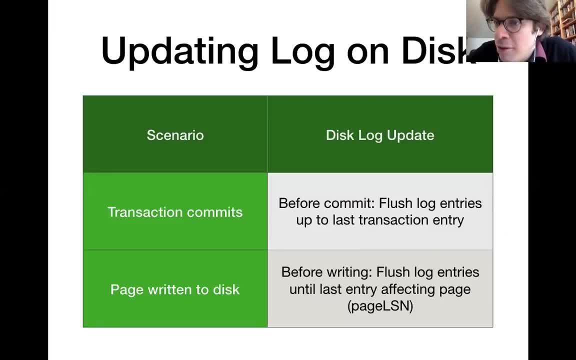 that we add to the lock on hard disk all the log entries that relate to this, all the log entries that relate to this, all the log entries that relate to this transaction, transaction, transaction, and in order to proactively avoid another, and in order to proactively avoid another. 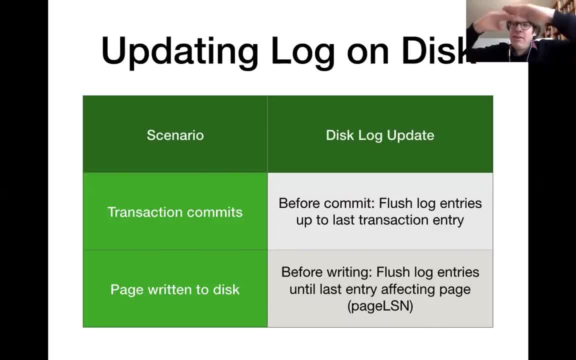 and in order to proactively avoid another possible source of misunderstandings. possible source of misunderstandings. possible source of misunderstandings. so those log entries, they are generated. so those log entries, they are generated. so those log entries, they are generated in a sequence, and the log entries 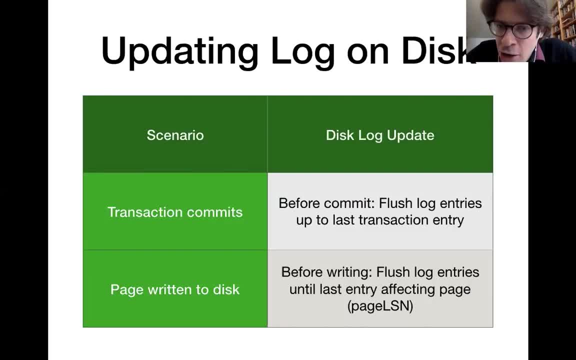 in a sequence and the log entries in a sequence and the log entries generated by different transactions. they generated by different transactions. they generated by different transactions. they might might, might alternate. so if a transaction commits, alternate. so if a transaction commits, alternate. so if a transaction commits, we're not writing only the log entries. 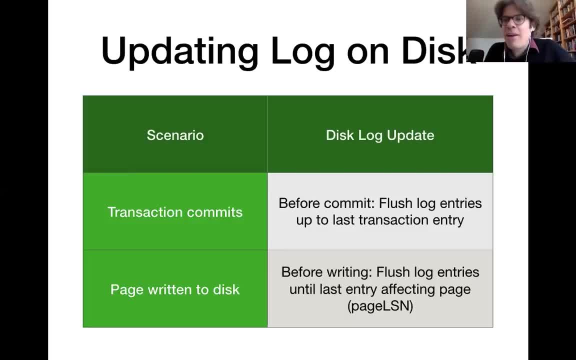 we're not writing only the log entries, we're not writing only the log entries to hard disk which connects to that, to hard disk which connects to that, to hard disk which connects to that specific transaction, specific transaction, specific transaction. but we just write um sequentially. but we just write um sequentially. 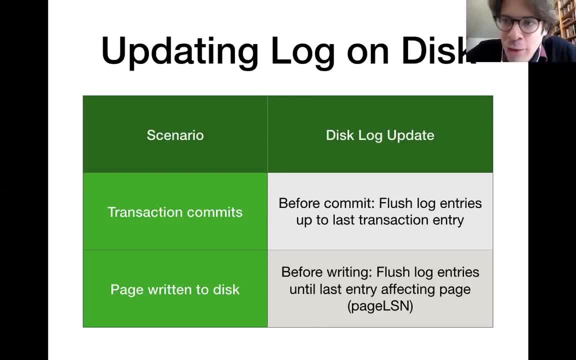 but we just write um sequentially: all log entries up to the last log, all log entries up to the last log. all log entries up to the last log entry from the transaction to hard disk. entry from the transaction to hard disk. entry from the transaction to hard disk. so 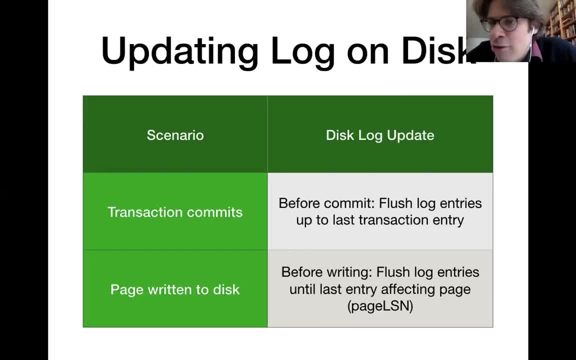 so. so in passing, we will also make log entries in passing, we will also make log entries in passing, we will also make log entries from other transactions persistent once from other transactions persistent once from other transactions persistent. once we do that, we do that, we do that um also before we write some of our in. 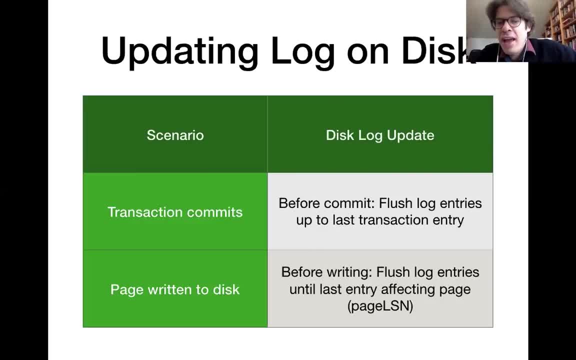 um. also, before we write some of our in um also, before we write some of our in memory pages, memory pages, memory pages to hard disk, we need to make sure that to hard disk. we need to make sure that to hard disk. we need to make sure that we have all required information. 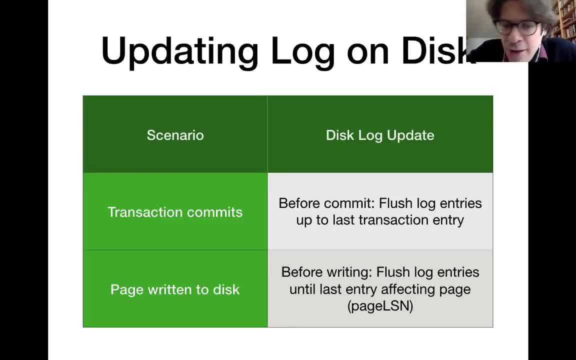 we have all required information. we have all required information in order to undo changes on that page, in order to undo changes on that page, in order to undo changes on that page later, later, later. so we require that all the log entries. so we require that all the log entries. 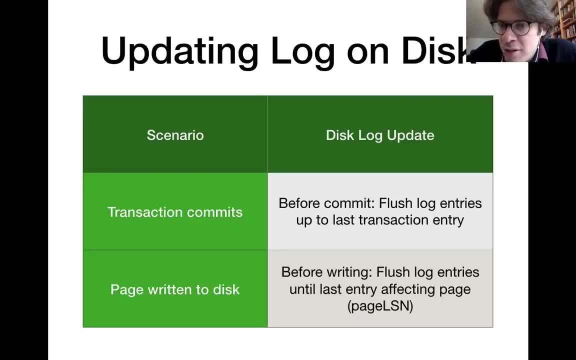 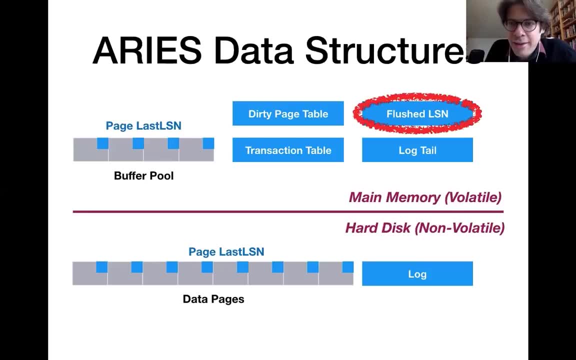 so we require that all the log entries that relate to this page are made, that relate to this page are made, that relate to this page are made persistent, persistent, persistent on hard disk. all right, and all right, and all right, and yes, quickly the flashed lsn. so and 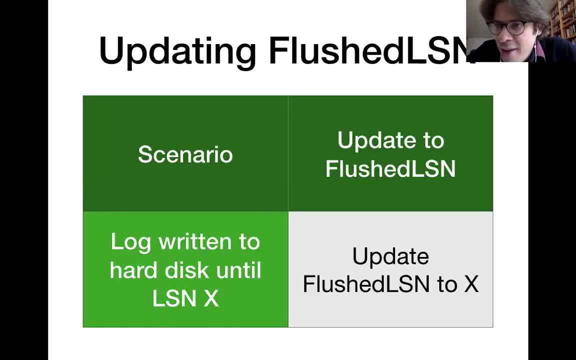 yes, quickly the flashed lsn. so and yes, quickly the flashed lsn. so, and here there is here. there is here. there is pretty much on the one scenario, pretty much on the one scenario, pretty much on the one scenario. if we write more log entries to hard, 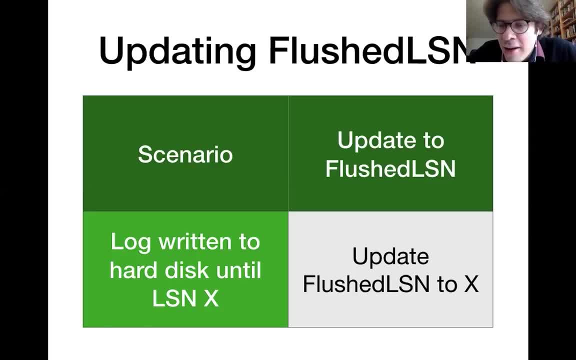 if we write more log entries to hard, if we write more log entries to hard disk, disk, disk, then we also have to update the flashed. then we also have to update the flashed, then we also have to update the flashed ls, ls, ls and accordingly and set it to the last. 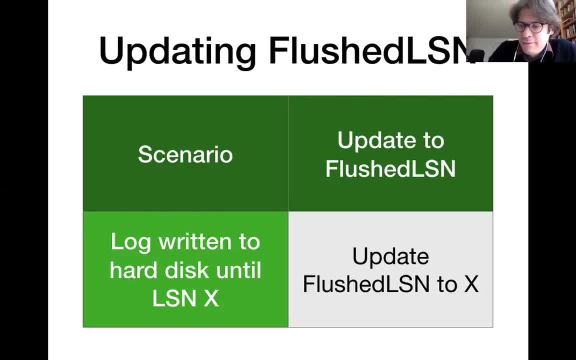 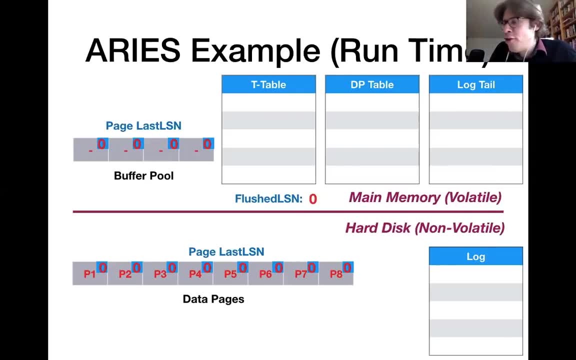 and accordingly, and set it to the last and accordingly, and set it to the last log entry that was written to hard disk. all right, so this was all right. so this was all right. so this was an overview of how those different data, an overview of how those different data. 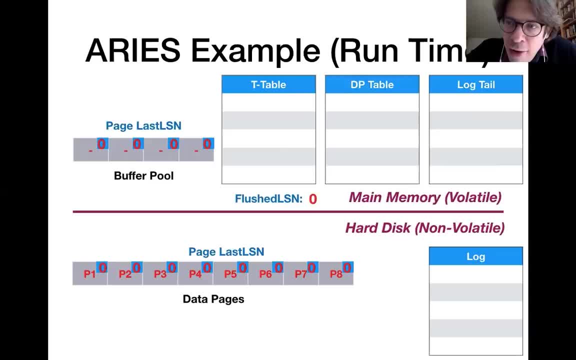 an overview of how those different data structures, structures, structures are updated before i pass on to the are updated before i pass on to the are updated before i pass on to the recovery part. recovery part, recovery part. i'm gonna make a little example here. i'm gonna make a little example here. 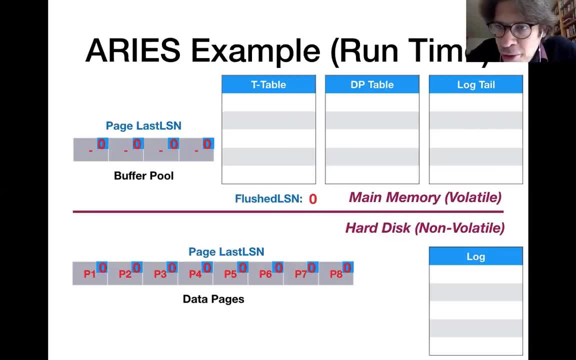 i'm gonna make a little example here. so what you see here again is the. so what you see here again is the. so what you see here again is the expanded version of those different, expanded version of those different, expanded version of those different data structures that we have seen. 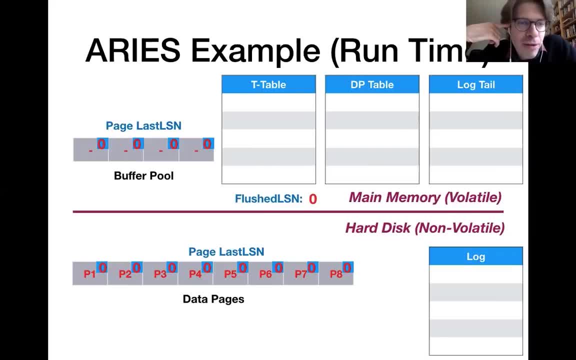 data structures that we have seen. data structures that we have seen. we have pages stored on hard disk. we have pages stored on hard disk. we have pages stored on hard disk. currently our buffer pool, currently our buffer pool, currently our buffer pool is empty and currently all of our 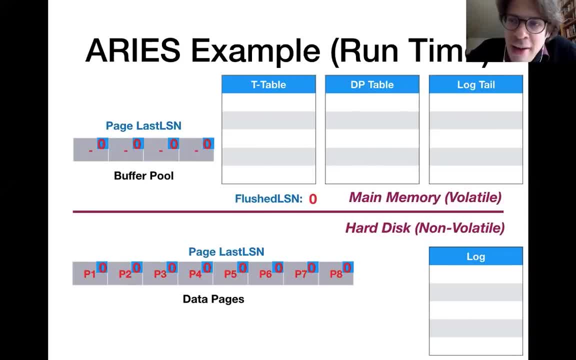 is empty and currently all of our is empty, and currently all of our data structures here are empty as well. data structures here are empty as well. data structures here are empty as well. so, in the following, so in the following, so in the following, we're gonna, um, we're gonna simulate a. 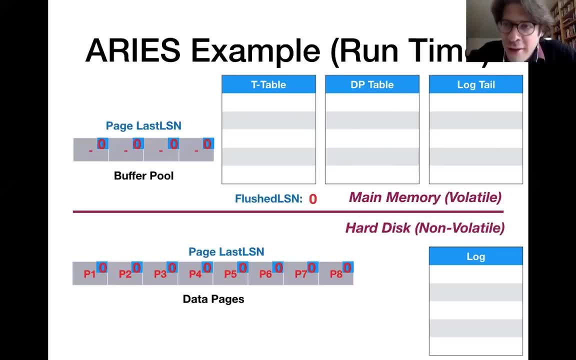 we're gonna, um, we're gonna, simulate a. we're gonna, um, we're gonna, simulate a couple of execution steps and see how couple of execution steps and see how couple of execution steps and see how those different data structures, those different data structures are updated by doing that. so, um, 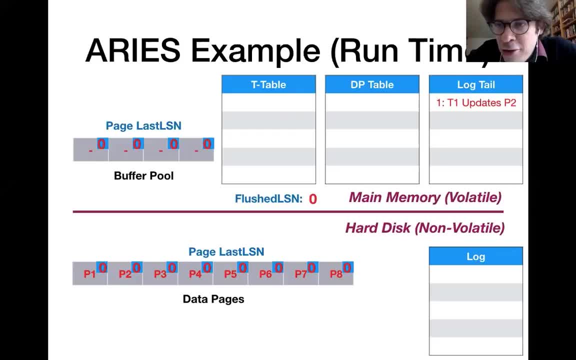 are updated by doing that. so um are updated by doing that. so, um, first of all, first of all, first of all, the half a transaction, one which updates the half a transaction, one which updates the half a transaction, one which updates page number two, page number two, page number two. so, um then, 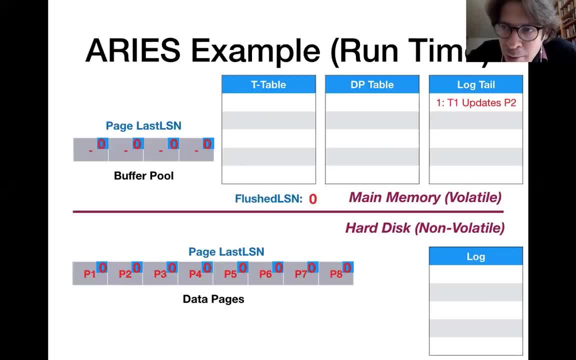 so, um, then, so, um, then, then writing those log entries in the, then writing those log entries in the, then writing those log entries in the examples, examples, examples. then of course i'm not gonna try to, then of course i'm not gonna try to, then of course i'm not gonna try to represent the entire. 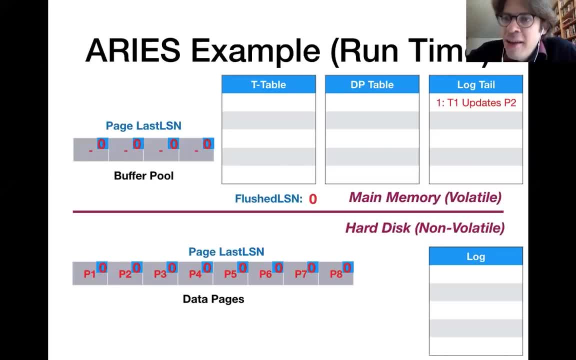 represent the entire, represent the entire log entry, but i am focusing on the log entry, but i am focusing on the log entry, but i am focusing on the essentials and the following essentials and the following essentials and the following: i'm gonna just report which transaction, i'm gonna just report which transaction. 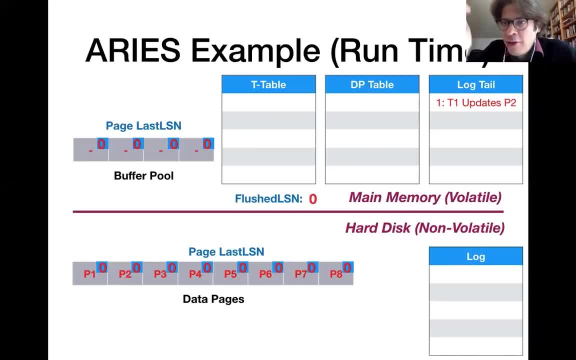 i'm gonna just report which transaction number and on which page the update number and on which page the update number and on which page the update occurred. but just so you know, of course occurred. but just so you know, of course occurred. but just so you know. of course, the real log entry would contain many. 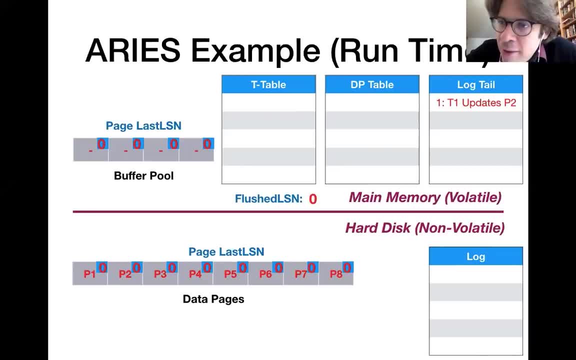 the real log entry would contain many. the real log entry would contain many more fields, as we have seen on more fields, as we have seen on more fields, as we have seen on one of the past slides, one of the past slides, one of the past slides, and this initial number, the one in this, 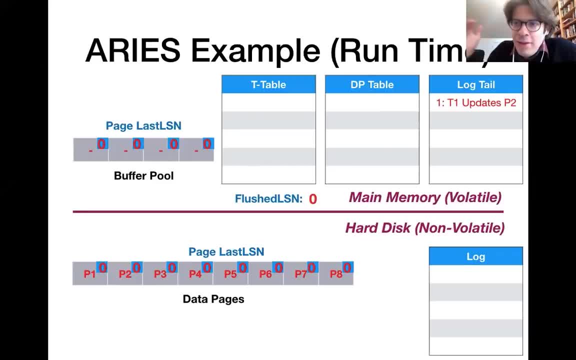 and this initial number, the one in this and this initial number, the one in this case, case, case, that is essentially the log sequence, that is essentially the log sequence, that is essentially the log sequence number and, as you will see, number and as you will see, number and as you will see, it will keep monotonically increasing. 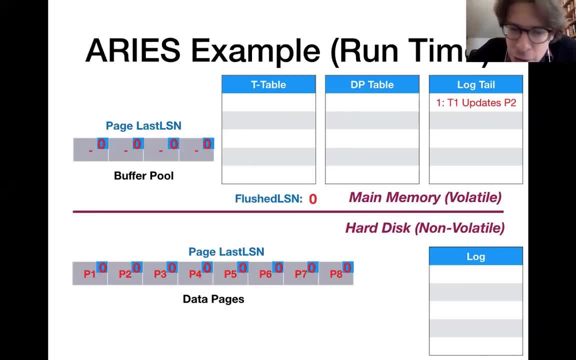 it will keep monotonically increasing. it will keep monotonically increasing. so here transaction number one wants to. so here. transaction number one wants to. so here transaction number one wants to update page number two. update page number two, update page number two. that means first of all we need to load. 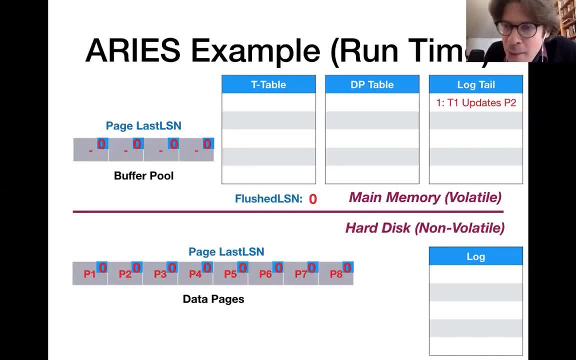 that means first of all, we need to load. that means first of all we need to load. page number two, page number two, page number two: from hard disk into main memory needs to. from hard disk into main memory. needs to. from hard disk into main memory needs to come. 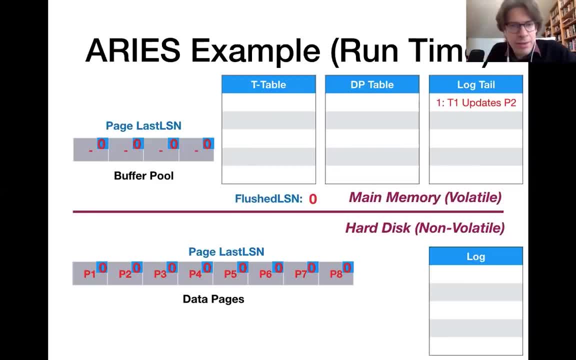 come, come into our buffer pool, that is into our buffer pool, that is into our buffer pool. that is one of the changes. let me just make the one of the changes. let me just make the one of the changes. let me just make the step and now explain. 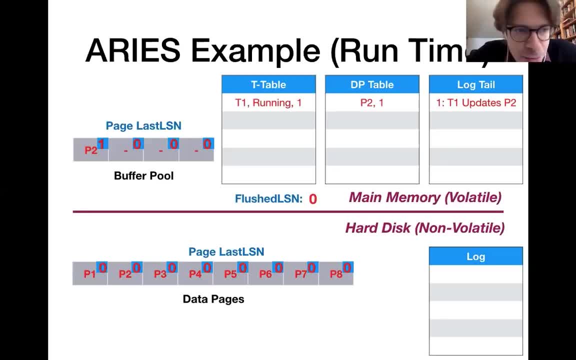 step and now explain, step and now explain what happened here. so you see here first what happened here. so you see here first what happened here. so you see here, first of all of all of all, as promised, a page number two has moved. as promised, a page number two has moved. 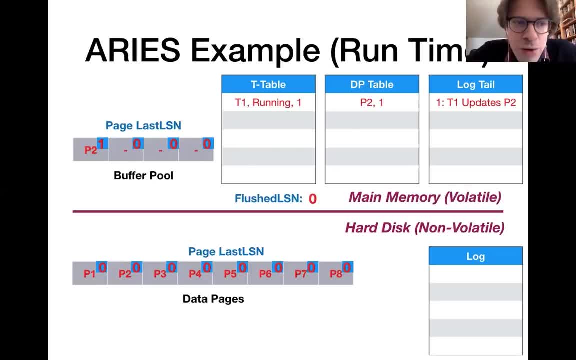 as promised, a page number two has moved into. has been copied into the buffer into. has been copied into the buffer into. has been copied into the buffer: pool, pool, pool in main memory. um, now the first thing in main memory. um, now the first thing in main memory. um, now the first thing that you see. 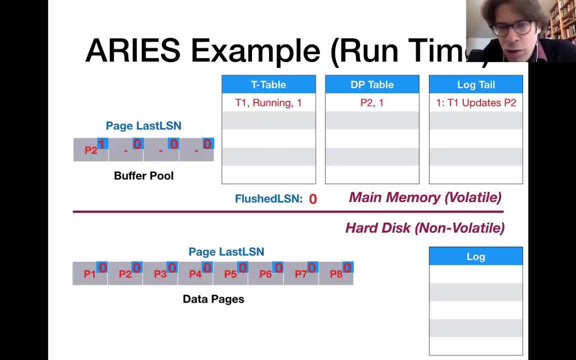 that you see that. you see the page lsn of the in memory version of the page lsn of the. in memory version of the page lsn of the in memory version of page number two, page number two. page number two has been updated to one because here we. 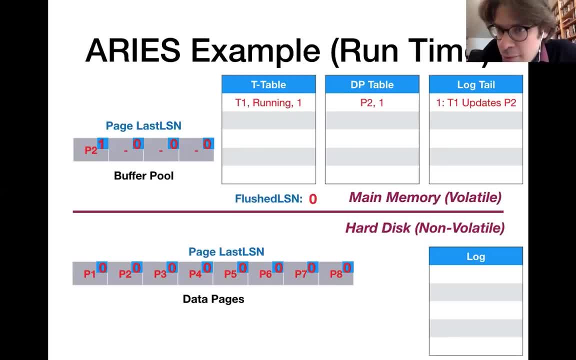 has been updated to one because here we has been updated to one because here we are processing, are processing, are processing- number two, so we keep track of that. i also number two, so we keep track of that. i also number two, so we keep track of that. i also note that. 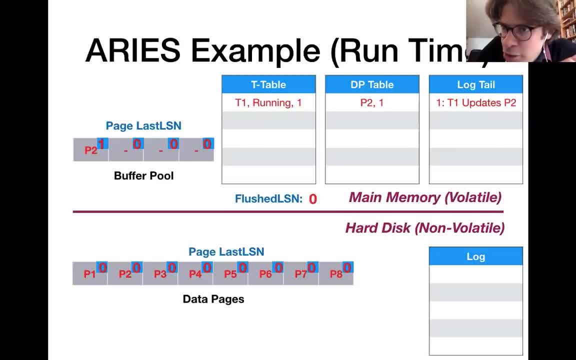 note that, note that for the on disk version of the page, which for the on disk version of the page, which for the on disk version of the page, which has not been changed yet, has not been changed yet, has not been changed yet, here we still have a page at us and of 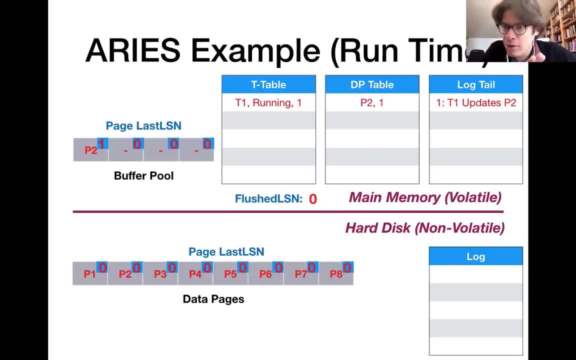 here we still have a page at us, and of here we still have a page at us. and of zero, because the news changes are not zero, because the news changes are not zero, because the news changes are not yet reflected, yet reflected, yet reflected on the hardest version. 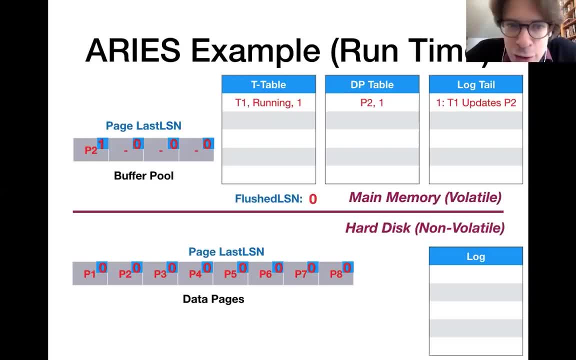 also. we have to enter the transaction also, we have to enter the transaction also. we have to enter the transaction into our transaction table, into our transaction table, into our transaction table. you see here the first entry we are. you see here the first entry we are. you see here the first entry we are. we are noting down transaction one as 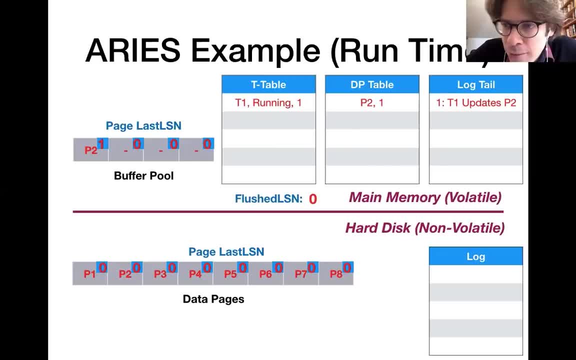 we are noting down transaction one as we are noting down transaction one as running with a last lsn of one. running with a last lsn of one. running with a last lsn of one: last lsn is always the last, last lsn is always the last. 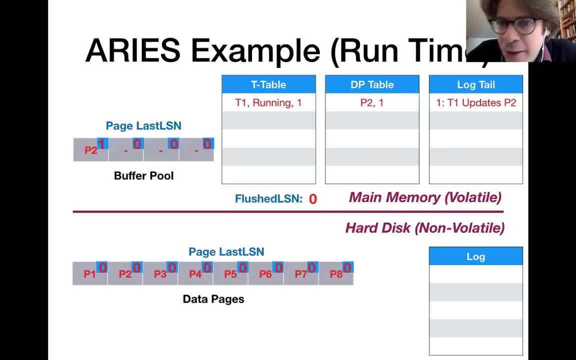 last lsn is always the last log entry generated by this transaction, log entry generated by this transaction, log entry generated by this transaction, and that is number one, and that is number one, and that is number one also. page number two has become dirty also, page number two has become dirty. 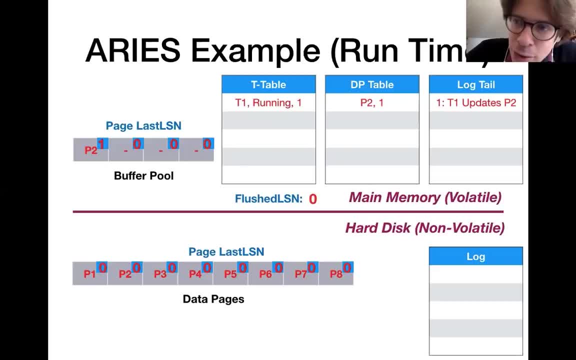 also, page number two has become dirty because, um, we have now diverging in, because, um, we have now diverging in, because, um, we have now diverging in memory and hard disk versions, memory and hard disk versions, memory and hard disk versions. that is why we enter it into our dirty. 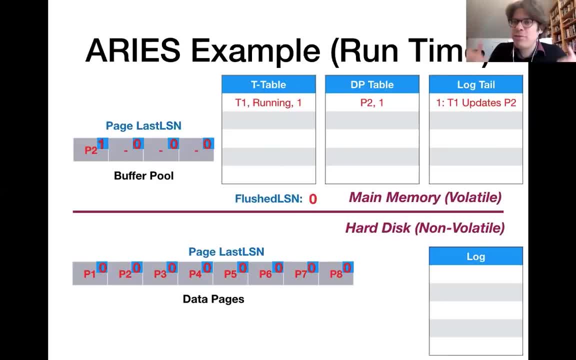 that is why we enter it into our dirty. that is why we enter it into our dirty page table page table page table with a direct lsn. the most recent block with a direct lsn. the most recent block with a direct lsn. the most recent block entry. 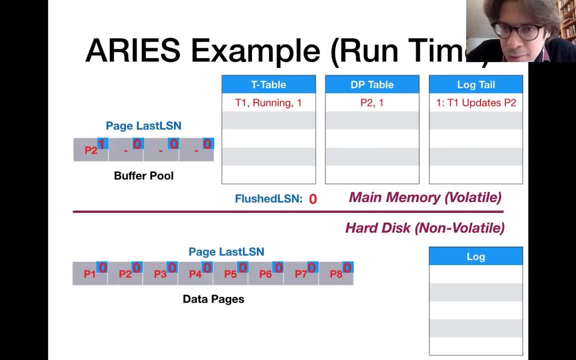 entry. entry: making the page page dirty set to one. making the page page dirty set to one. making the page page dirty set to one. right, so, um, right, so, um, right, so, um, that covers everything. let's process that covers everything. let's process that covers everything. let's process the next operation, and here there is. 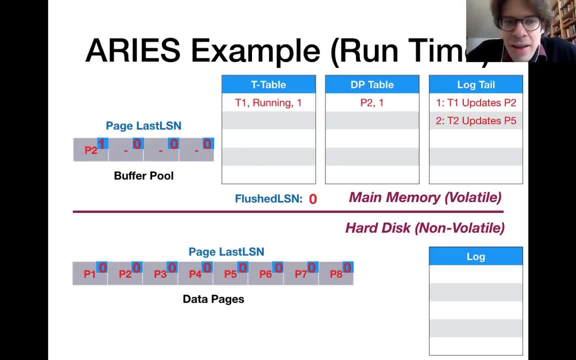 the next operation. and here there is the next operation. and here there is another transaction transaction number, another transaction transaction number, another transaction transaction number two, which updates a page two. which updates a page two. which updates a page: number five, all right, number five, all right, number five, all right, maybe i'm actually before continuing, i 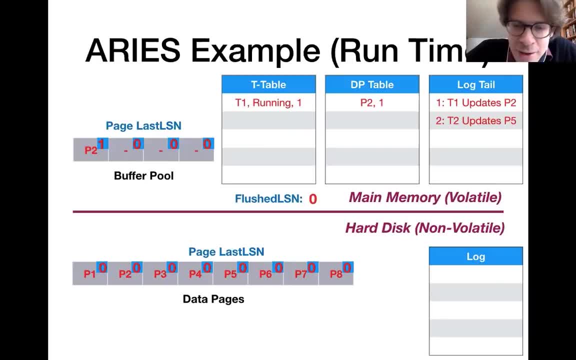 maybe i'm actually before continuing. i maybe i'm actually before continuing. i give you a second to think about what. give you a second to think about what. give you a second to think about what you expect to happen in those different. you expect to happen in those different. 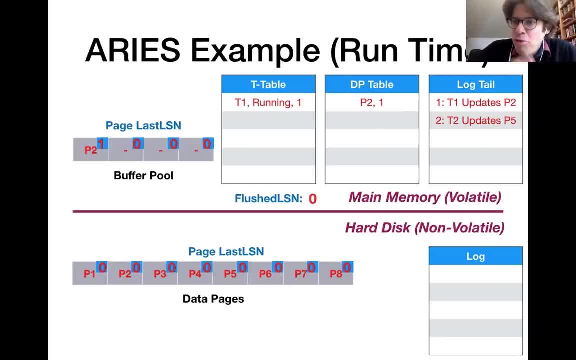 you expect to happen in those different data structures, and perhaps somebody data structures and perhaps somebody data structures and perhaps somebody can make a little proposition. can make a little proposition. can make a little proposition in the chat. does anyone have a in the chat? does anyone have a? 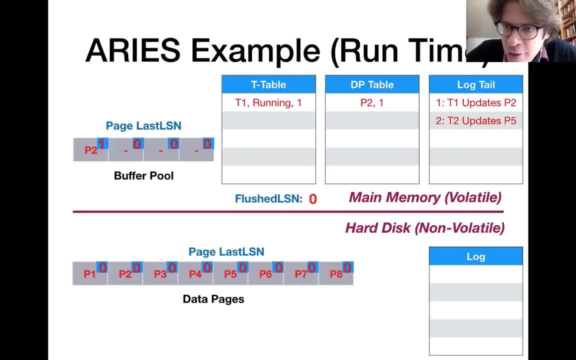 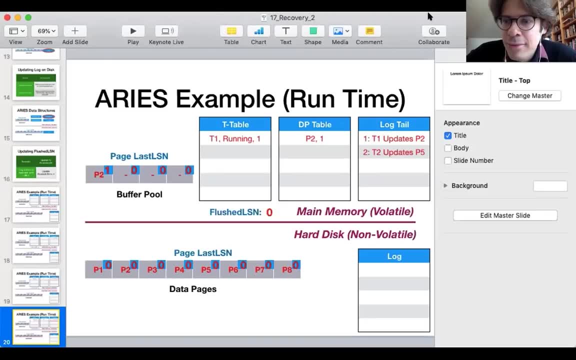 in the chat. does anyone have a proposition about how? the different proposition about how the different proposition about how the different data structures change due to this entry? data structures change due to this entry. data structures change due to this entry. all right, very good. okay, so i have a. 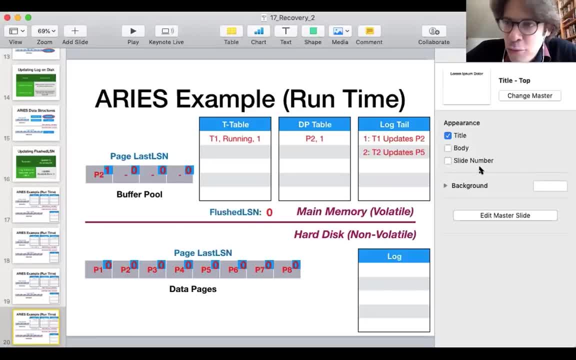 all right, very good, okay, so i have a. all right, very good, okay. so i have a first proposition, first proposition, first proposition: that page five will get moved into the. that page five will get moved into the. that page five will get moved into the buffer pool in the memory. 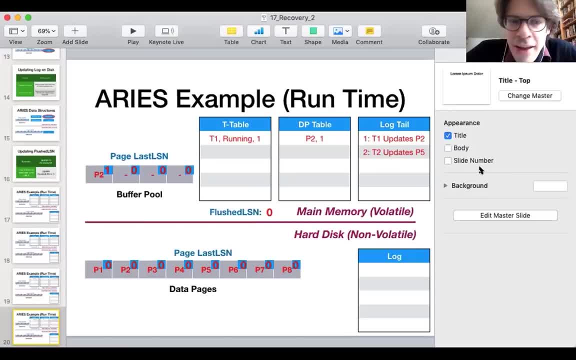 buffer pool in the memory, buffer pool in the memory. and the page lsn the page last, that is, and the page lsn the page last, that is, and the page lsn the page last that is. n n n will be set to two. okay, very good. 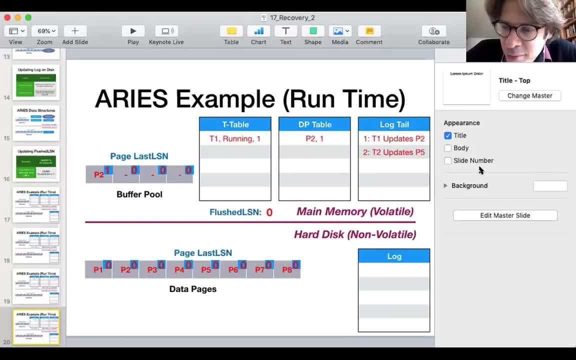 will be set to two. okay, very good, will be set to two. okay, very good. is there anything else that happens? ah, very good, okay, very good. so uh, p5. ah, very good, okay, very good. so uh, p5. ah, very good, okay, very good. so uh, p5 gets added the page number five that we 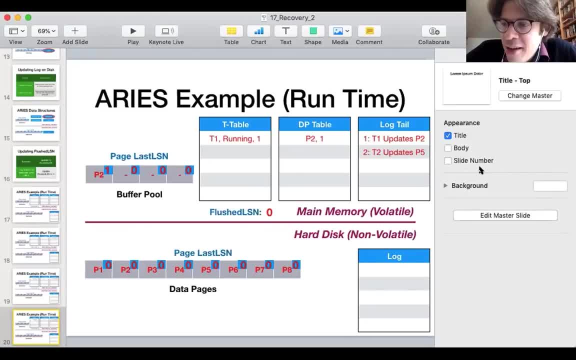 gets added. the page number five that we gets added. the page number five that we are updating. gets added to the dirty are updating. gets added to the dirty are updating. gets added to the dirty page table page, table page table. and the last lsn and the last lsn. 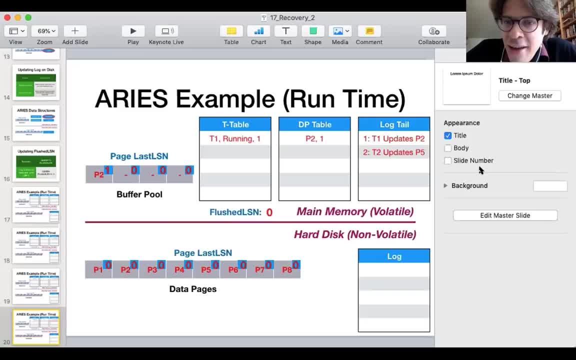 and the last lsn, the rec lsn in this case, uh exactly. the rec lsn in this case, uh, exactly. the rec lsn in this case, uh exactly, will be set to two, because this is when will be set to two, because this is when will be set to two, because this is when the page became dirty. 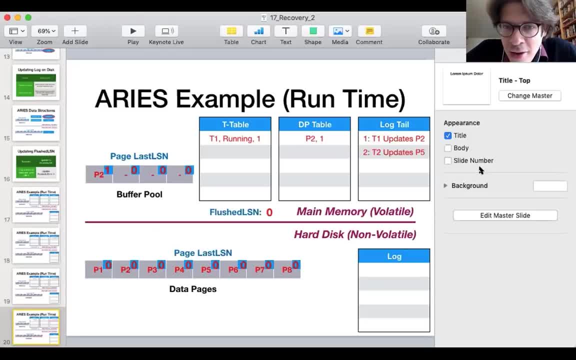 the page became dirty. the page became dirty, and somebody else is proposing here also, and somebody else is proposing here also, and somebody else is proposing here also that we insert, that we insert, that we insert into the transaction table the entry into the transaction table, the entry into the transaction table, the entry transaction tool. 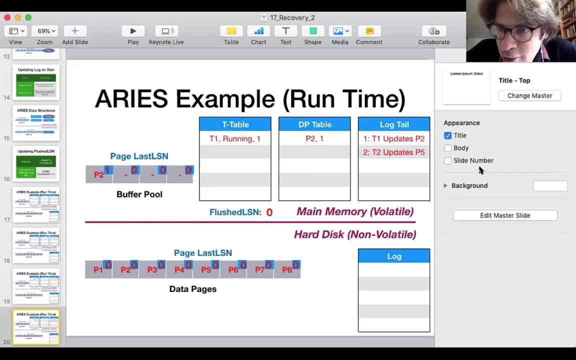 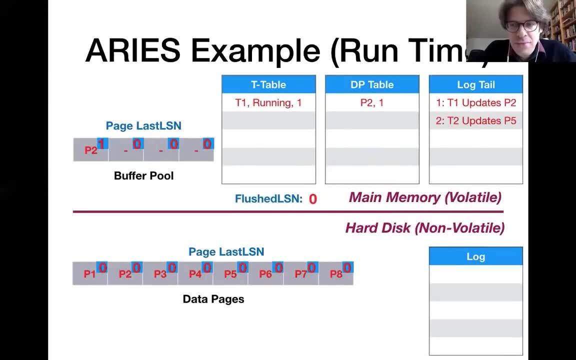 transaction tool. transaction tool running um last at us, and two running um last at us, and two running um last at us, and two absolutely correct. yes, so those are the absolutely correct. yes, so those are the absolutely correct. yes, so those are the changes that we make in this case here. 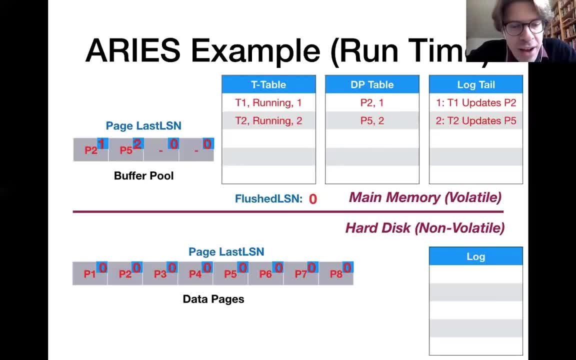 very good, exactly so. now we have moved. very good, exactly so, now we have moved. very good, exactly so. now we have moved page five, page five, page five: um from hard disk copied it into main. um from hard disk copied it into main. um from hard disk copied it into main memory. 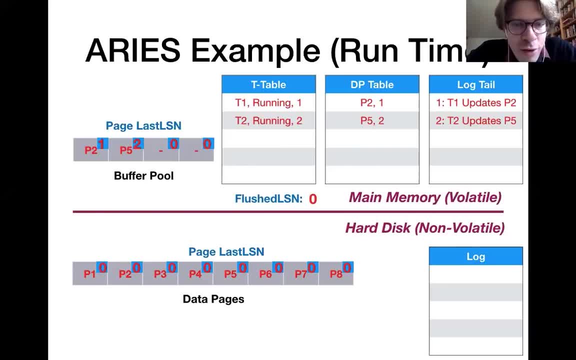 memory, memory. we have changed it and kept track of that. we have changed it and kept track of that. we have changed it and kept track of that. change, change, change with the page at its end and with the page at its end, and with the page at its end, and we have inserted p5 into the dirty page. 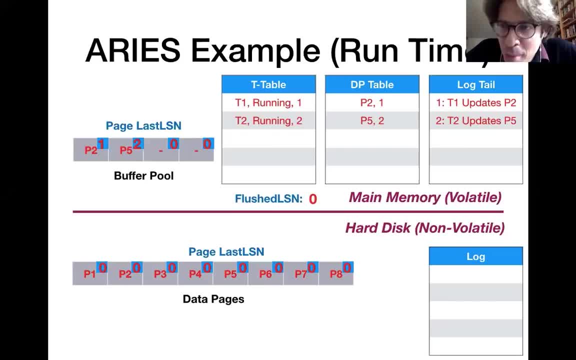 we have inserted p5 into the dirty page. we have inserted p5 into the dirty page table with a rack lsn2 and we have mark table with a rack lsn2 and we have mark table with a rack lsn2 and we have mark. transaction two is running. 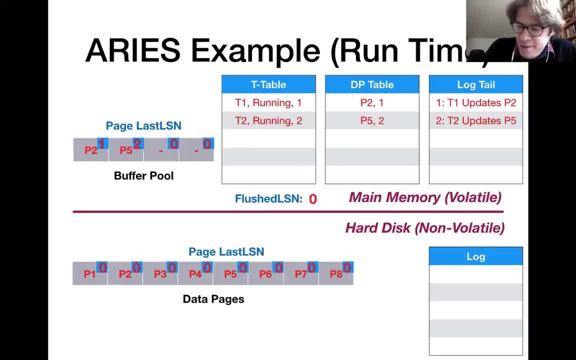 transaction two is running. transaction two is running with last lsn2. all right with last lsn2. all right with last lsn2, all right. next operation is an update by a next operation is an update by. a next operation is an update by a transaction one. 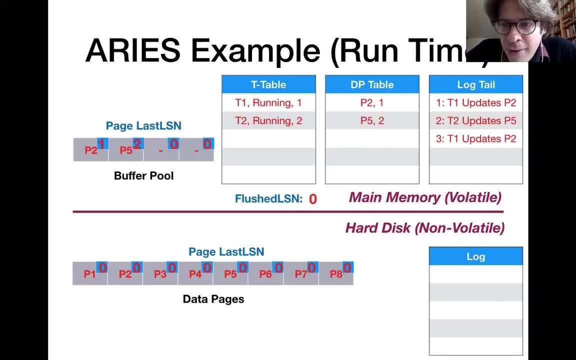 transaction one, transaction one of page two again. um, all right of page two again. um, all right of page two again. um, all right, so what happens here? so what happens here, so what happens here, is that we already have page number two, is that we already have page number two. 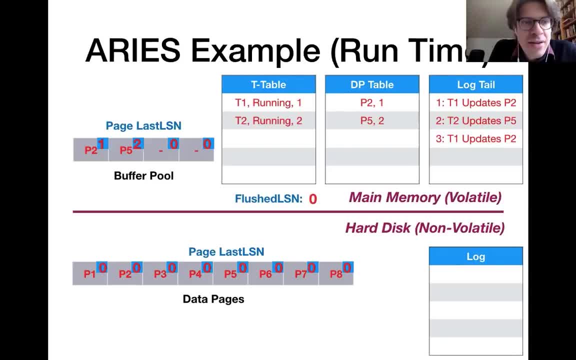 is that we already have page number two in main memory. so we still change it in main memory. so we still change it in main memory. so we still change it and have to update the page lsn and have to update the page lsn and have to update the page lsn here in memory to three. 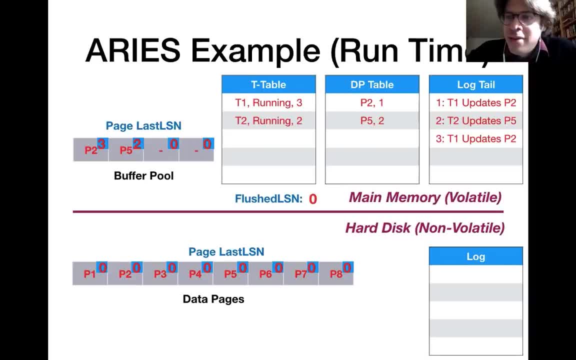 here in memory to three here in memory to three. and for the other changes. so now some. and for the other changes. so now some. and for the other changes. so now some. temptation might be to update something, temptation might be to update something, temptation might be to update something in the dirty page table, but that is not. 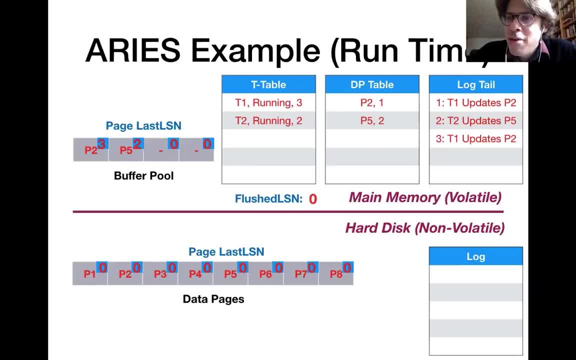 in the dirty page table, but that is not in the dirty page table. but that is not necessary, necessary. necessary because a page number two is already in, because a page number two is already in, because a page number two is already in the dirty page table. the dirty page table. 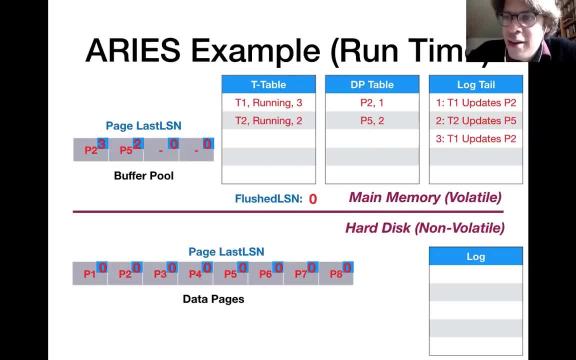 the dirty page table, and we only keep track of the first log. and we only keep track of the first log, and we only keep track of the first log entry by which the page entry, by which the page entry, by which the page became dirty. so here the dirty page table. 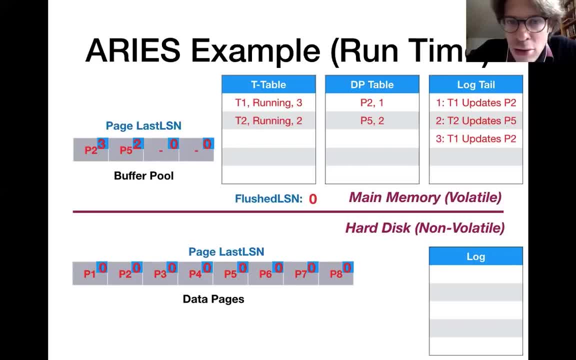 became dirty. so here the dirty page table became dirty. so here the dirty page table. nothing changes. even if we have another, nothing changes. even if we have another, nothing changes, even if we have another. update to page number two. update to page number two. update to page number two on the transaction table in this. 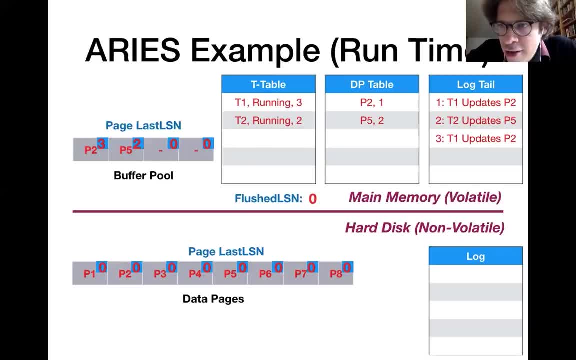 on the transaction table in this on the transaction table. in this transaction table on the other side, transaction table on the other side. transaction table on the other side. we have a change for transaction one. it is. we have a change for transaction one. it is. we have a change for transaction one. it is still. 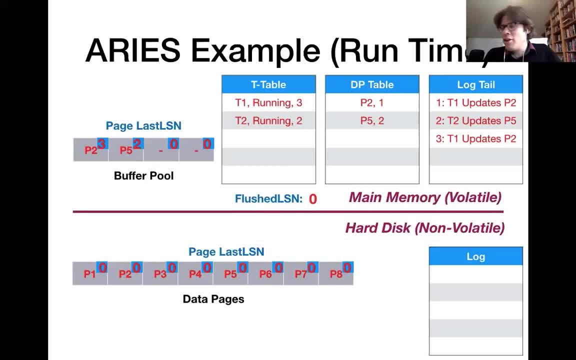 still still running, but now the last lsm, the last running. but now the last lsm, the last running, but now the last lsm, the last log entry is generated. log entry is generated. log entry is generated. must be set to three, because that is the. must be set to three because that is the. 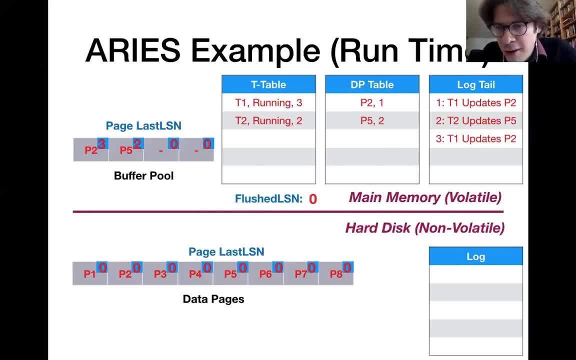 must be set to three, because that is the current, current, current log sequence number. all right, log sequence number. all right, log sequence number. all right, let's continue. and at this point a. let's continue. and at this point a. let's continue. and at this point, a transaction. 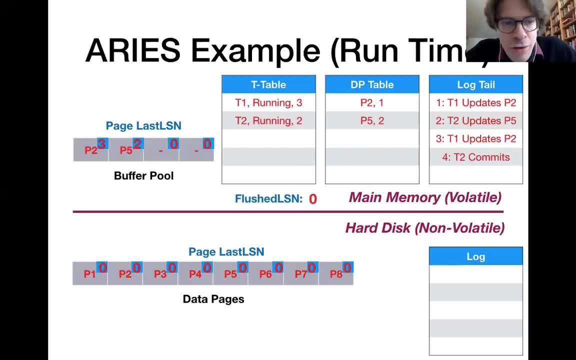 transaction transaction two: uh must commit two, uh must commit two, uh must commit. all right, so all right, so all right. so now let's uh see what changes here. that now let's uh see what changes here. that now let's uh see what changes here. that is actually an interesting case, so maybe 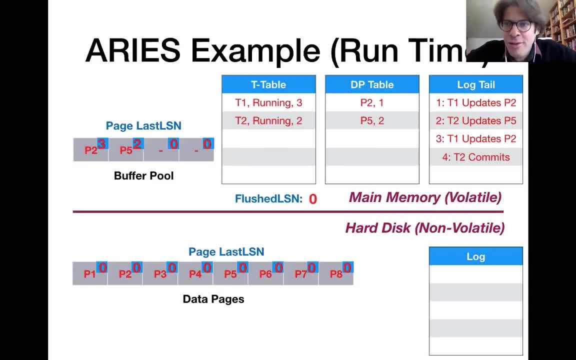 is actually an interesting case. so maybe is actually an interesting case. so maybe let me just ask you that question again. let me just ask you that question again. let me just ask you that question again. i give you a couple of, i give you a couple of, i give you a couple of seconds to think about it, and maybe 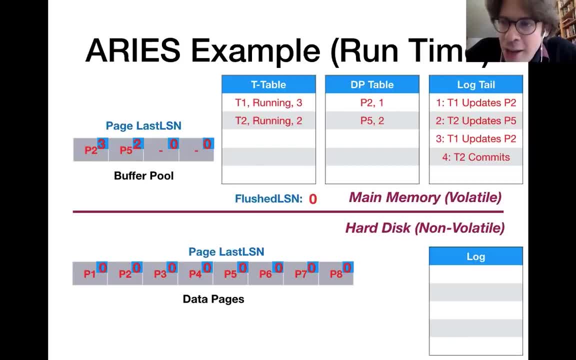 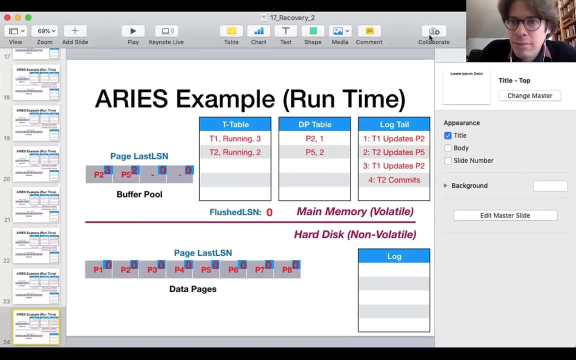 seconds to think about it and maybe seconds to think about it, and maybe anyone can make a suggestion about what anyone can make a suggestion about what anyone can make a suggestion about what could change in those data structures. if you think about the rules of, if you think about the rules of. 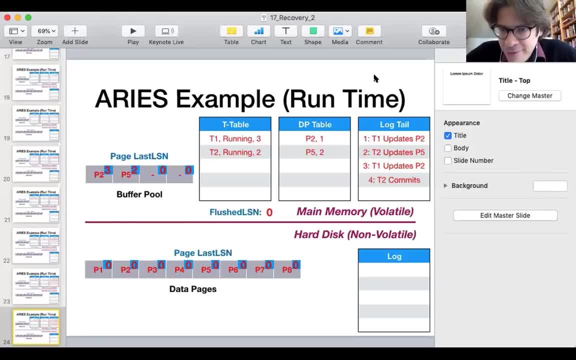 if you think about the rules of writerhead logging, writerhead logging, writerhead logging, okay, okay, okay, great proposition here. so people start great proposition here. so people start great proposition here. so people start talking about, talking about, talking about flushing the log, which is probably what: flushing the log, which is probably what. 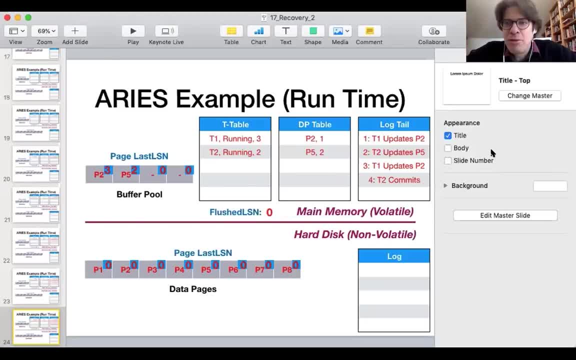 flushing the log, which is probably what you want to do because for you want to do, because for you want to do, because, for right-ahead locking, if you remember the right-ahead locking, if you remember the right-ahead locking, if you remember the rules, there was something that had to. 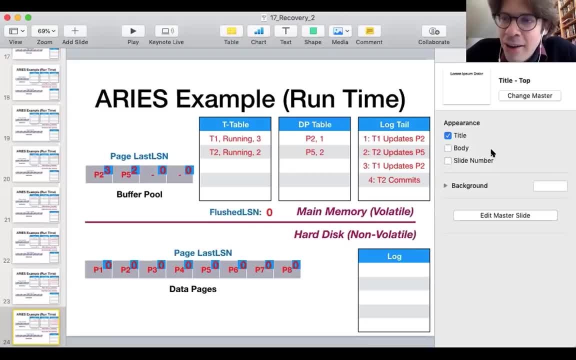 rules. there was something that had to rules. there was something that had to happen when transactions commit and happen when transactions commit and happen when transactions commit. and something that had to happen, something that had to happen, something that had to happen. when i try, when we write pages to hard. 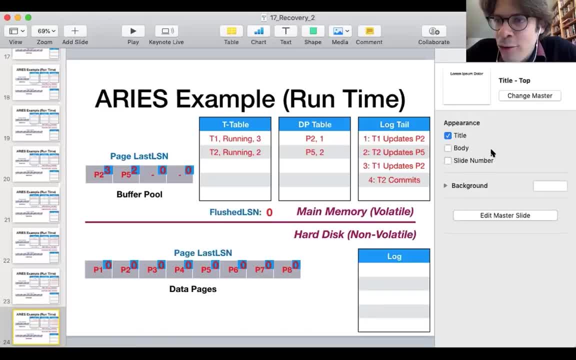 when i try, when we write pages to hard, when i try when we write pages to hard disk and both related to we have to disk and both related to we have to disk and both related to we have to write log entries to hard disk. write log entries to hard disk. 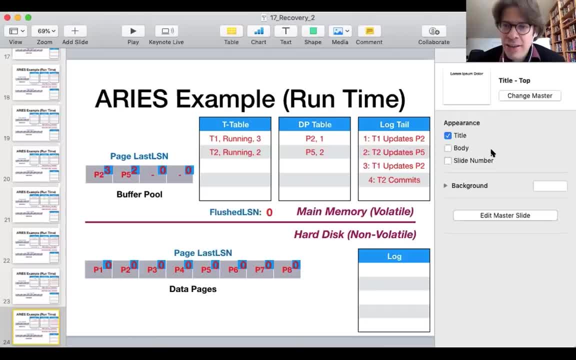 write log entries to hard disk. and so here the suggestion is that we, and so here the suggestion is that we, and so here the suggestion is that we flush um the first two uh log entries, flush um the first two uh log entries, flush um the first two uh log entries, and that is definitely required. 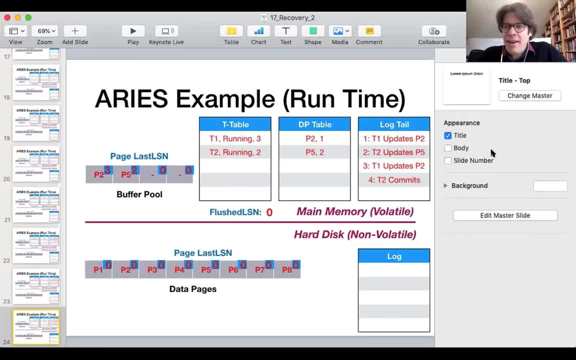 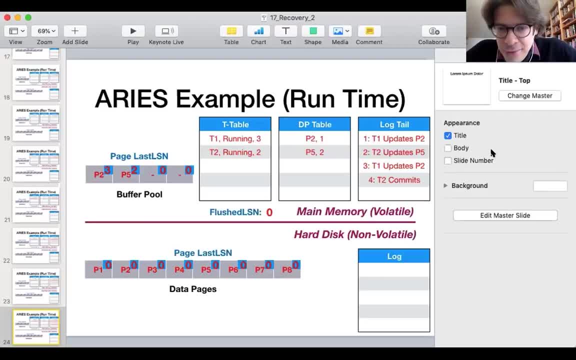 flush more, perhaps, or suggest to change some of the other data structures as some of the other data structures, as some of the other data structures as well. so when we come back online, so when we come back online, so when we come back online after the crash, after the crash, 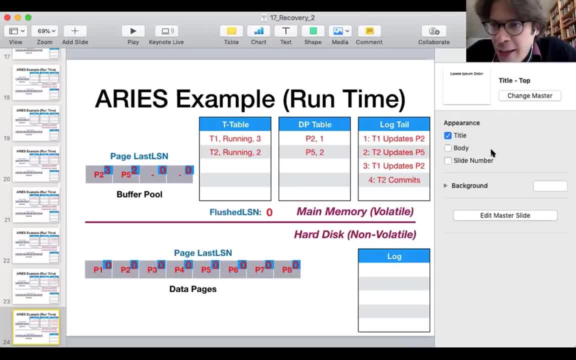 after the crash. we want to know, we want to know. we want to know um which transactions have been running, um which transactions have been running, um which transactions have been running during the crash. so we will abort those during the crash. so we will abort those during the crash. so we will abort those transactions. 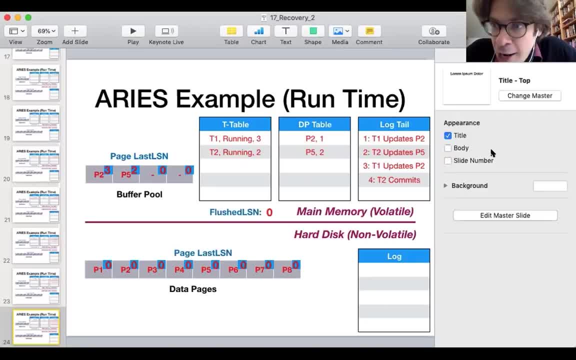 transactions, transactions, and which transactions have already, and which transactions have already, and which transactions have already committed before the crash, committed before the crash, committed before the crash. so it's very important that we, so it's very important that we, so it's very important that we are aware um that which transactions. 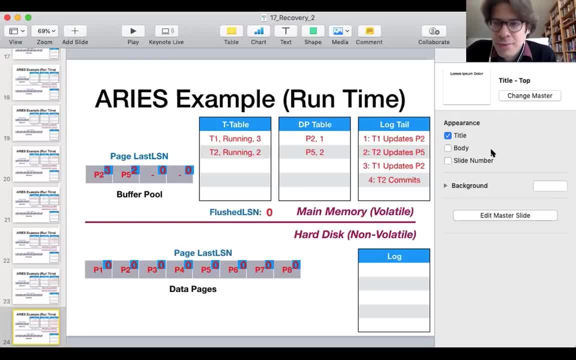 are aware um that, which transactions are aware um that which transactions have already committed before the crash, have already committed before the crash, have already committed before the crash, and there's also some, and there's also some, and there's also some. um, okay, the transaction table. yeah, it is. 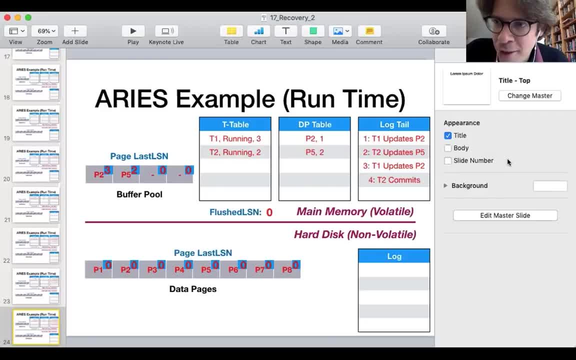 okay, the transaction table. yeah, it is okay the transaction table. yeah, it is updated with, updated with updated with information about the commits and information about the commits and information about the commits. and here that is a little bit tricky. because here that is a little bit tricky because 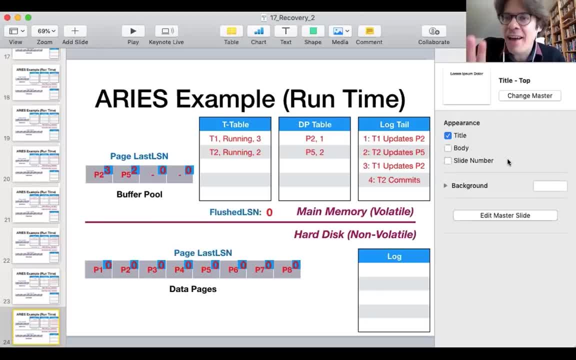 here that is a little bit tricky, because um, um, um, a priori um. it is unclear in which order a priori um it is unclear in which order a priori um it is unclear in which order those different data structures, those different data structures, those different data structures are updated. so 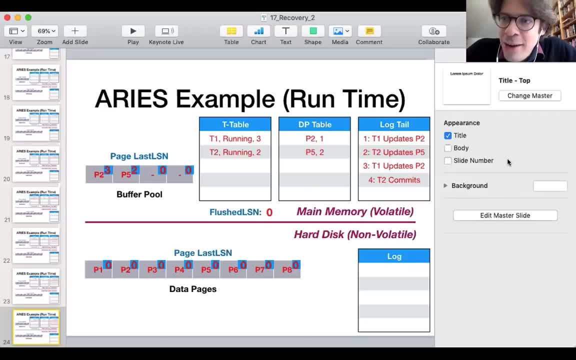 are updated, so are updated. so, for the um, what needs to happen for commit? for the um, what needs to happen for commit? for the um, what needs to happen for commit? we generally said that, uh, the. we generally said that, uh, the. we generally said that, uh, the transaction needs, that we need to write. 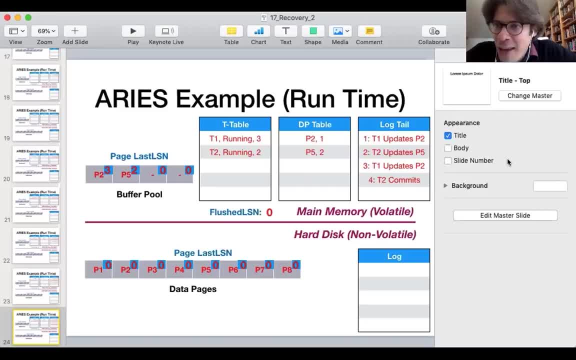 transaction needs that we need to write transaction needs that we need to write log entries to hard disk up to the last log entries to hard disk, up to the last log entries to hard disk, up to the last log entry of that transaction. so log entry of that transaction. so 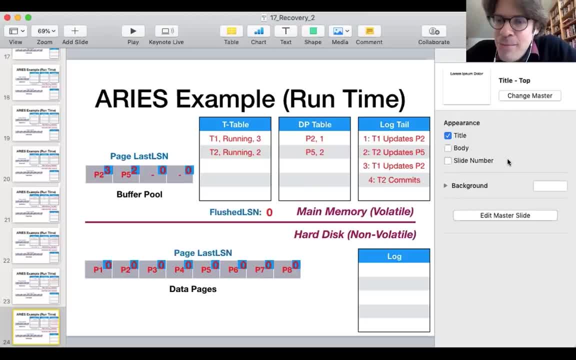 log entry of that transaction. so in this drawing here right now, i have in this drawing here right now, i have in this drawing here right now, i have only put, the only put, the only put, the commit log entry. but i have not yet commit log entry, but i have not yet. 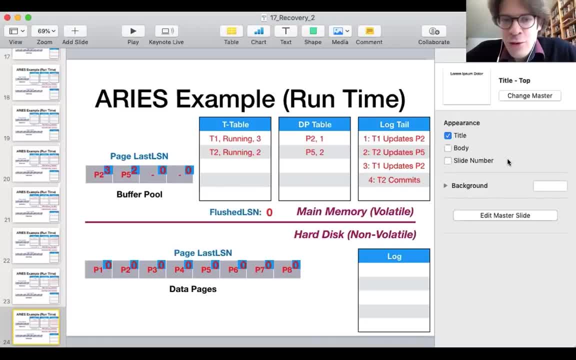 commit log entry, but i have not yet updated the associated data structures, updated the associated data structures, updated the associated data structures. so right now, transaction. so right now, transaction. so right now, transaction. two is still set to a last lsn of two. two is still set to a last lsn of two. 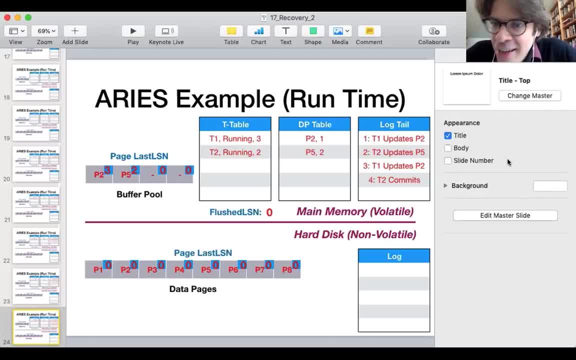 two is still set to a last lsn of two, but now that we have just but, now that we have just but, now that we have just added this log entry, the last lsn added this log entry. the last lsn added this log entry, the last lsn would be updated to a four, and then we 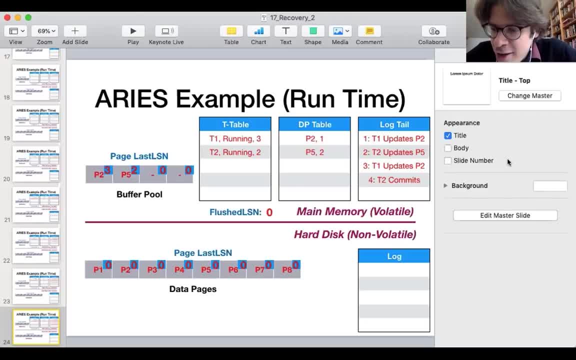 would be updated to a four, and then we would be updated to a four, and then we would want to write all of the associated, would want to write all of the associated, would want to write all of the associated log entries, log entries, log entries to hard disk, and indeed, um, we have to. 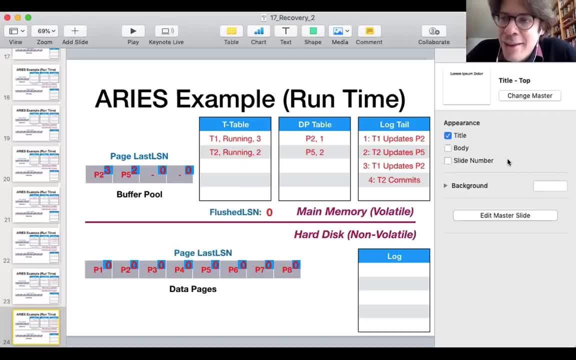 to hard disk, and indeed, um, we have to to hard disk and indeed, um we have to update the last lsn of the transaction. update the last lsn of the transaction. update the last lsn of the transaction. we also have to update the status of the. 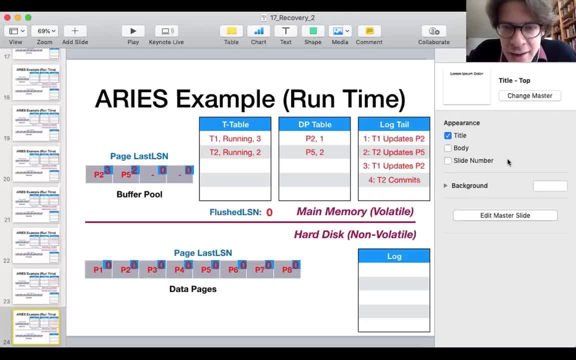 we also have to update the status of the. we also have to update the status of the transaction, transaction, transaction, and beyond that, the only other thing, and beyond that, the only other thing, and beyond that, the only other thing that changes, that changes, that changes is the flushed lsn in order to keep. 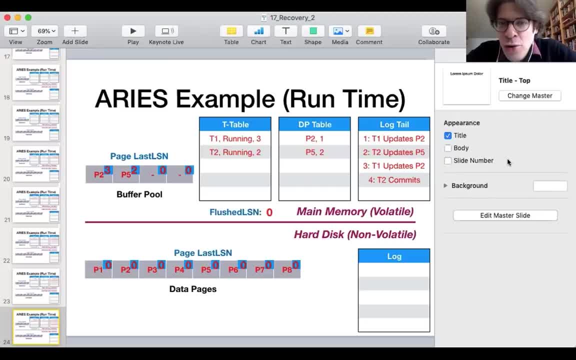 is the flushed lsn in order to keep? is the flushed lsn in order to keep track of which portion of the log? has track of which portion of the log? has track of which portion of the log has already been persisted, already been persisted, already been persisted? so this is, yeah, very good replies here. 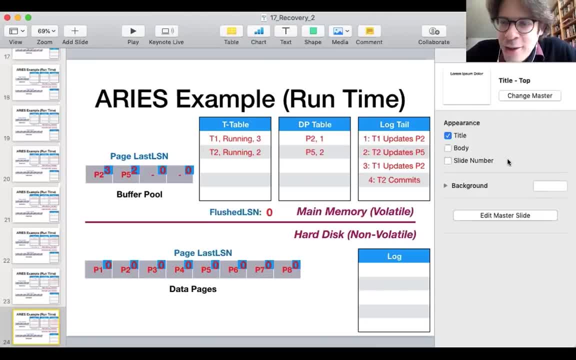 so this is, yeah, very good replies here. so this is, yeah, very good replies here. so, exactly this is what i wanted to. so, exactly this is what i wanted to. so exactly this is what i wanted to hear: that we have to write part of the hear. that we have to write part of the. 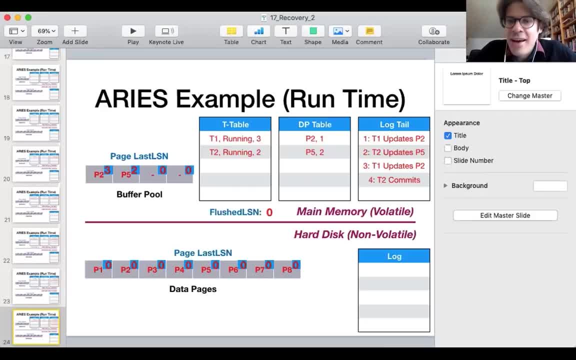 hear that we have to write part of the log- log log- back to hard disk in order to make those back to hard disk, in order to make those back to hard disk, in order to make those changes, changes, changes, uh, in order to persist uh those, uh, in order to persist uh, those. 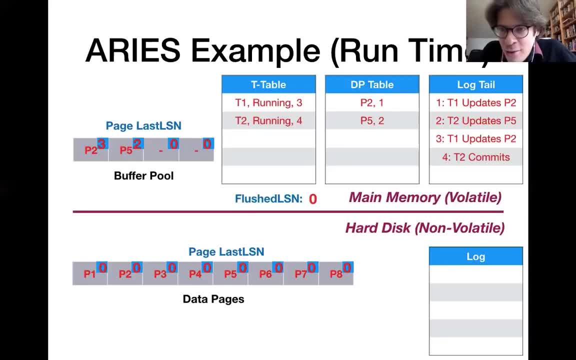 uh, in order to persist, uh, those changes. okay, let me changes, okay, let me changes okay. let me quickly show that here. chat away so you can see my slide um. chat away so you can see my slide um. chat away so you can see my slide um. all right, so now we have already. 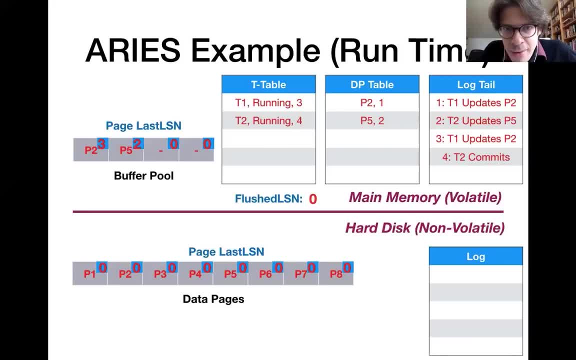 all right, so now we have already all right, so now we have already updated, updated, updated the um transaction table, the um transaction table, the um transaction table, and, and, and. all right, all right, all right, and, and, and. now we have written, now we have written, now we have written the block to hard disk. so here, multiple. 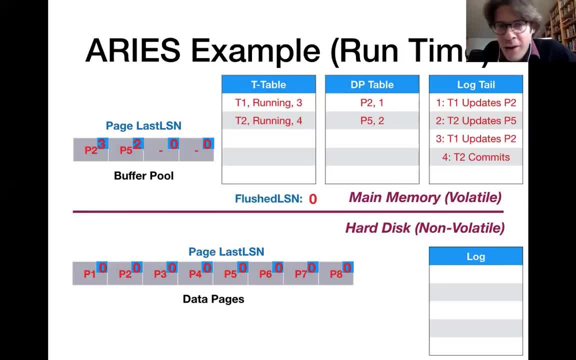 the block to hard disk. so here, multiple the block to hard disk. so here, multiple things have happened at the same time. things have happened at the same time. things have happened at the same time when going from one to the other one, when going from one to the other one. 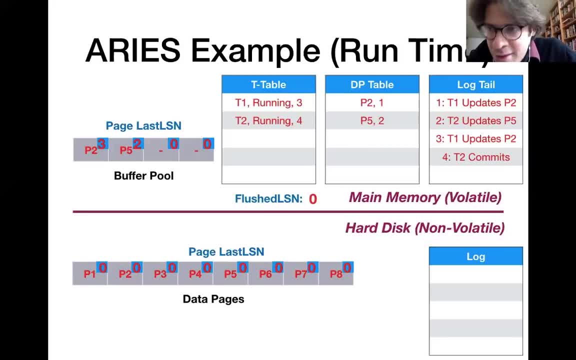 when going from one to the other, one. um strictly speaking, the um strictly speaking, the. um. strictly speaking, the status of transaction two should also be status of transaction. two should also be status of transaction. two should also be updated to the commit instead of updated to the commit instead of. 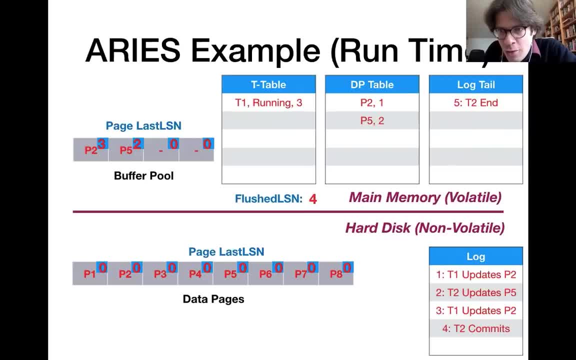 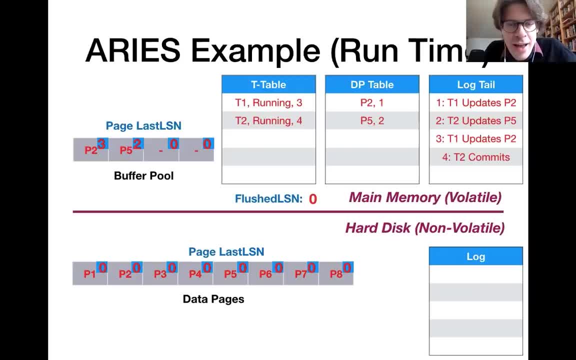 then it gets deleted out of the, then it gets deleted out of the transaction table anyway. transaction table anyway. transaction table anyway, but nevertheless, strictly speaking, uh, but nevertheless, strictly speaking, uh, but nevertheless, strictly speaking, uh, this running should actually be. this running should actually be this running, should actually be committed now in the transaction table. 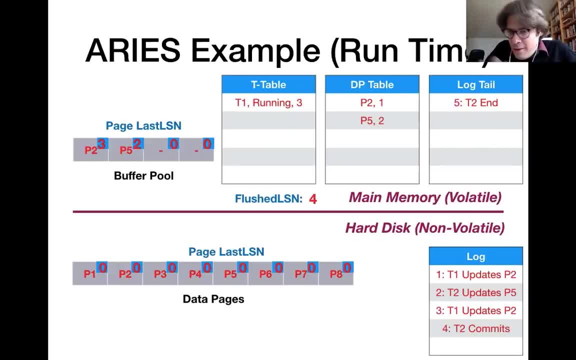 committed now in the transaction table. committed now in the transaction table for transaction for transaction for transaction, number two. beyond that: you see here number two. beyond that, you see here number two. beyond that, you see here that we have updated the flushed ls and that we have updated the flushed ls and 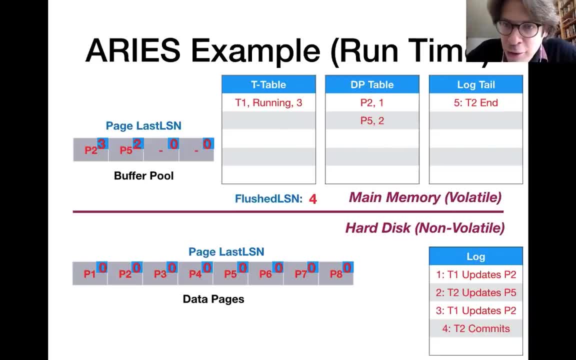 that we have updated the flushed ls and to force because now we have persisted to force, because now we have persisted to force, because now we have persisted the first four log entries. we have the the first four log entries. we have the the first four log entries. we have the end block record for transaction. 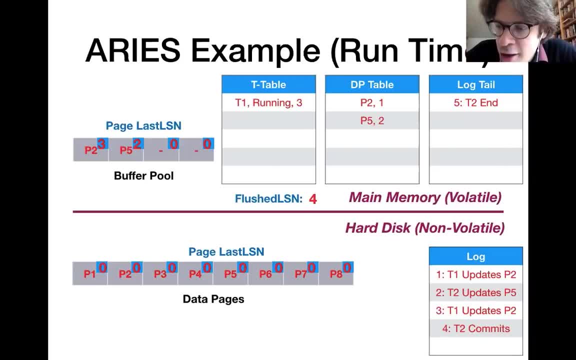 end block record for transaction. end block record for transaction five, which means that we can take out five, which means that we can take out five, which means that we can take out this transaction from the transaction, this transaction from the transaction, this transaction from the transaction table. and, of course, since we haven't, 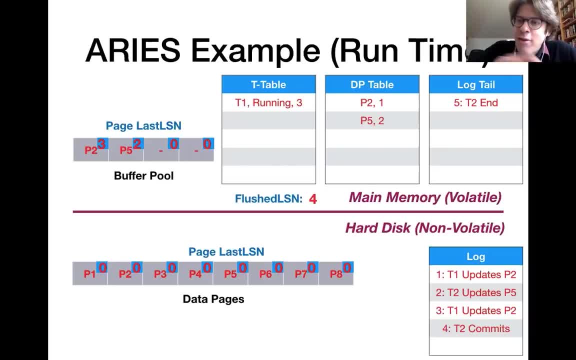 table. and, of course, since we haven't table, and of course, since we haven't written any written, any written, any pages to hard disk, we still have those pages to hard disk. we still have those pages to hard disk. we still have those entries in the dirty page table. 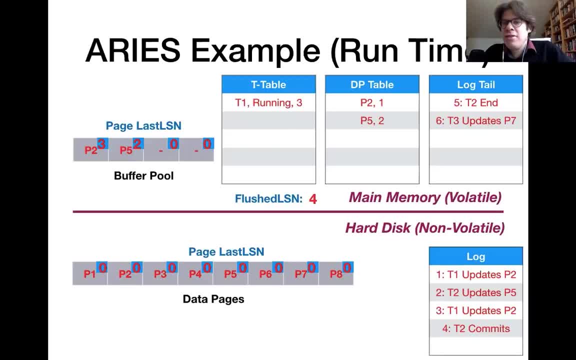 now, let's continue a little bit further now. let's continue a little bit further now. let's continue a little bit further now. we have a transaction. now we have a transaction. now we have a transaction, transaction number three which updates a. transaction number three which updates a. 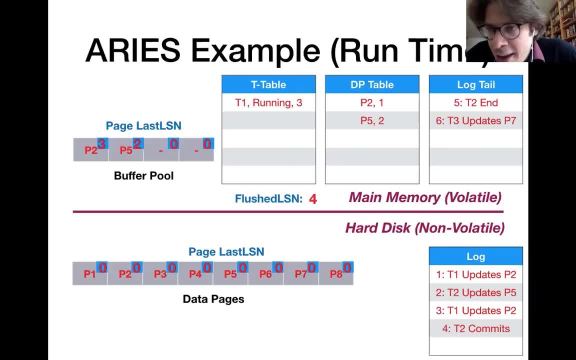 transaction number three, which updates a page page, page number seven. and again we have to move number seven. and again we have to move number seven. and again we have to move, for page number seven, for page number seven, for page number seven from hard disk into main memory. 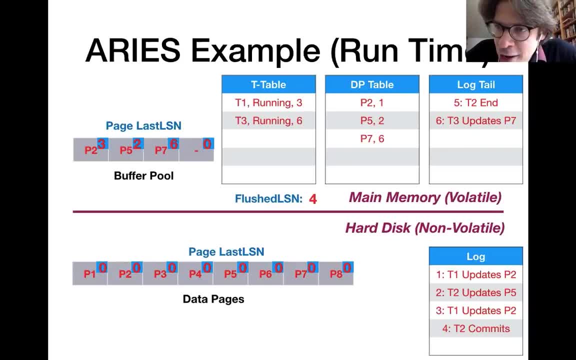 from hard disk into main memory. from hard disk into main memory. let me do that. here we have to update. let me do that. here we have to update. let me do that. here we have to update. the page lsn of page number seven. the page lsn of page number seven. 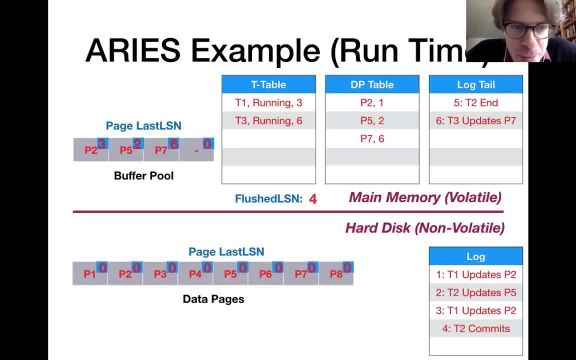 the page lsn of page number seven to a fix, because that is the current to a fix, because that is the current to a fix, because that is the current log sequence number. log sequence number. log sequence number. also transaction number three is fresh. so also transaction number three is fresh. so 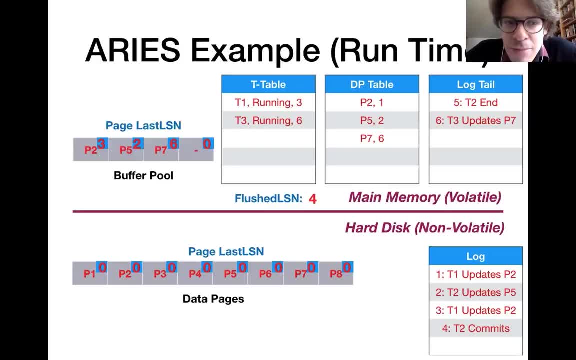 also transaction number three is fresh, so we have to add it to the transaction. we have to add it to the transaction. we have to add it to the transaction table. table table. enter page seven had been clean before. enter page seven had been clean before. enter page seven had been clean before. now it becomes dirty so we have to add. 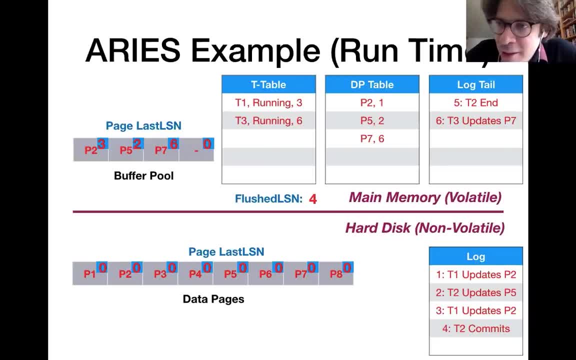 now it becomes dirty so we have to add. now it becomes dirty so we have to add it to the dirty page table it to the dirty page table it to the dirty page table with log sequence number six as the. with log sequence number six as the. with log sequence number six as the rack lsn. 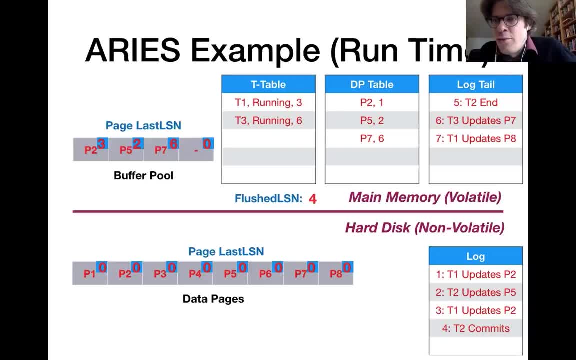 rack lsn, rack lsn. all right, so all right, so, all right. so one more transaction. one now updates a one more transaction. one now updates a one more transaction. one now updates a page page, page number eight. so we move page number eight into main memory. it also becomes dirty. 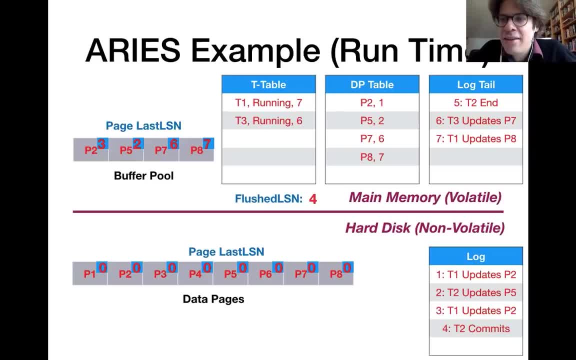 into main memory. it also becomes dirty. into main memory. it also becomes dirty. so we added, so we added, so we added with rack lsn 7 and transaction with rack lsn 7 and transaction with rack lsn 7 and transaction one gets updated in terms of last lsn. 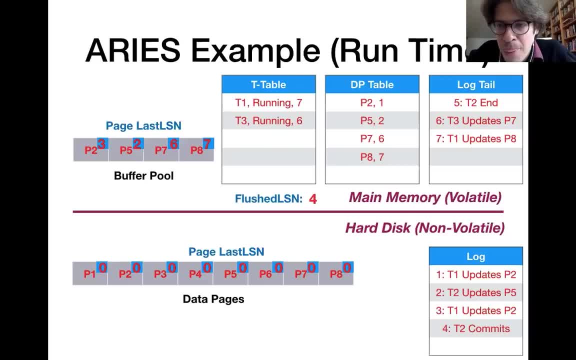 one gets updated in terms of last lsn. one gets updated in terms of last lsn and we set that to the current log. and we set that to the current log and we set that to the current log. sequence number: sequence number. sequence number as well. all right, so at this point to 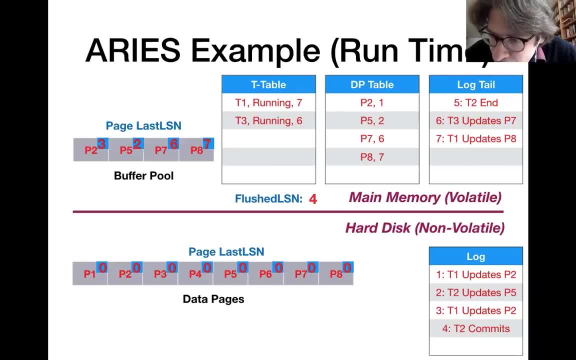 as well. all right. so at this point, to as well. all right. so at this point, to note that the note that the note that the buffer pool is filled up, buffer pool is filled up, buffer pool is filled up. so if we want to do any further, so if we want to do any further, 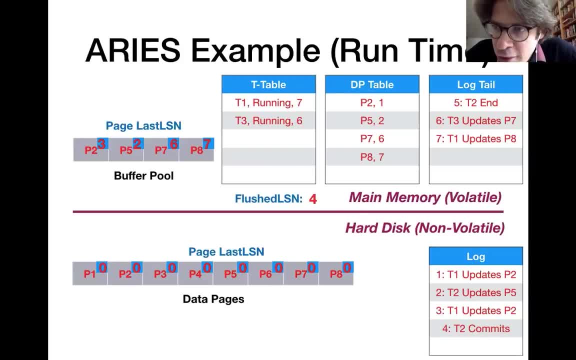 so if we want to do any further operations on different pages than what operations on different pages? than what operations on different pages than what we have in the buffer pool now we have in the buffer pool now, we have in the buffer pool now, then we first would have to write some. 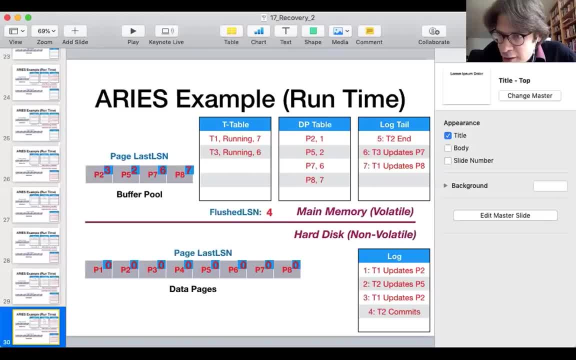 then we first would have to write some, then we first would have to write some of those pages to hard disk. of those pages to hard disk, of those pages to hard disk, you could check whether there's. you could check whether there's. you could check whether there's questions. 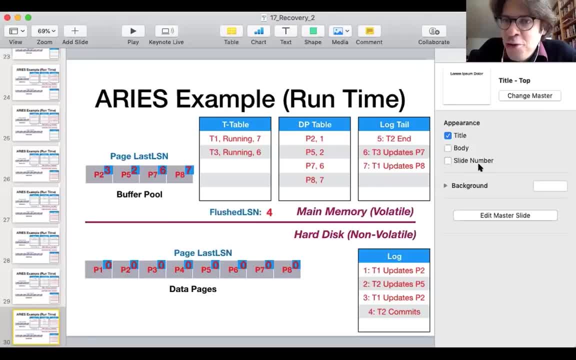 all right, and this is a great question. all right, and this is a great question. all right and this is a great question. so the question was: when transaction? so the question was when transaction. so the question was: when transaction number two finished, number two finished, number two finished, um, why didn't we? 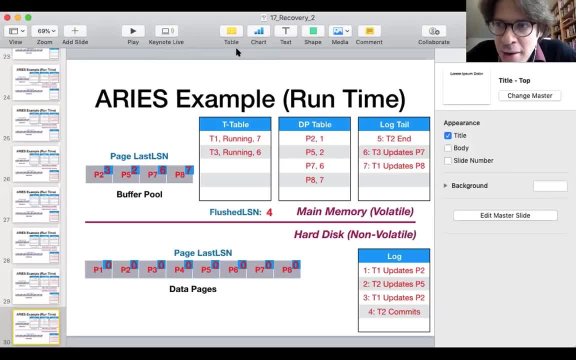 um, why didn't we, um, why didn't we write the associated pages? write the associated pages, write the associated pages, the pages that were changed by this, the pages that were changed by this, the pages that were changed by this transaction transaction, transaction to hard disk. so that's a great question. 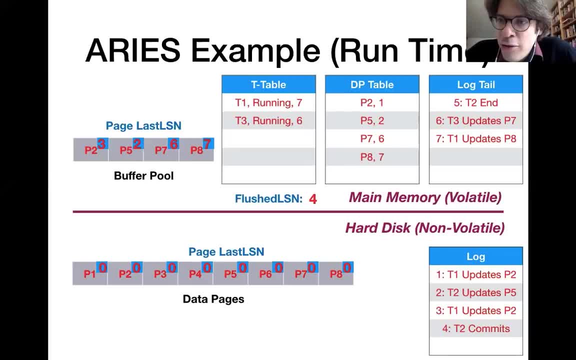 to hard disk, so that's a great question. to hard disk. so that's a great question, in fact, um, there is a policy which is, in fact, um, there is a policy which is, in fact, um, there is a policy which is called the force policy, called the force policy. 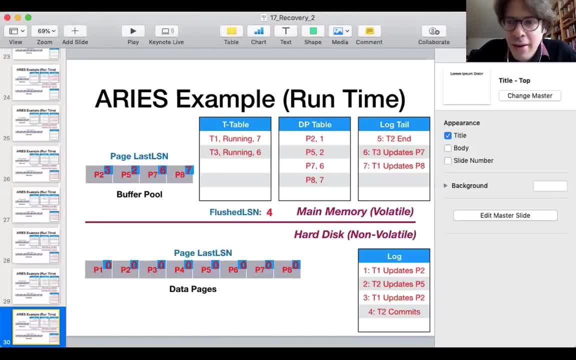 called the force policy. um, i can hear some noise here. um, i can hear some noise here. um, i can hear some noise here. we could be um, okay, all right, okay, all right, okay, all right, so um the question, so um. the question, so um. the question was: um, if a transaction commits, 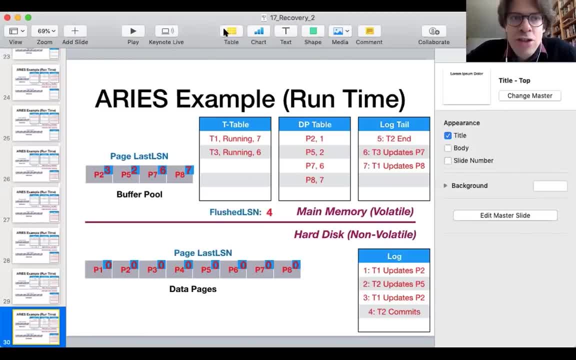 was um. if a transaction commits was um. if a transaction commits, why don't we write the pages that were? why don't we write the pages that were? why don't we write the pages that were changed by this transaction to hard disk, changed by this transaction to hard disk? 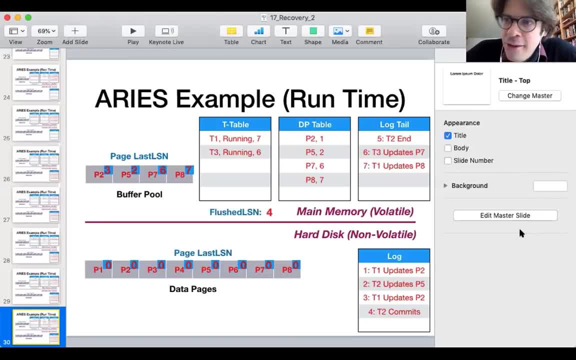 changed by this transaction to hard disk. and there's indeed a policy which does, and there's indeed a policy which does, and there's indeed a policy which does, exactly then, exactly then, exactly then. this is the first policy. um, we have it. this is the first policy, um, we have it. 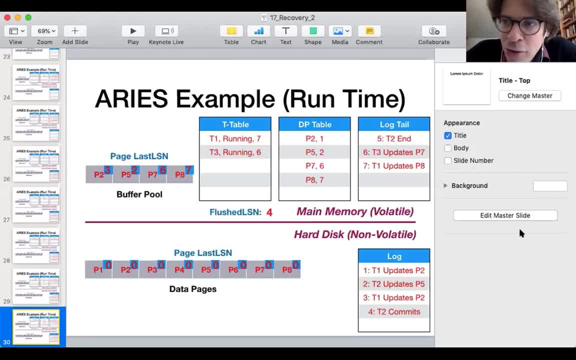 this is the first policy. um, we have it, discussed it very quickly, discussed it very quickly, discussed it very quickly. uh, last time we went over it. uh, last time we went over it. uh, last time we went over it relatively very fast, um it essentially relatively very fast, um it essentially. 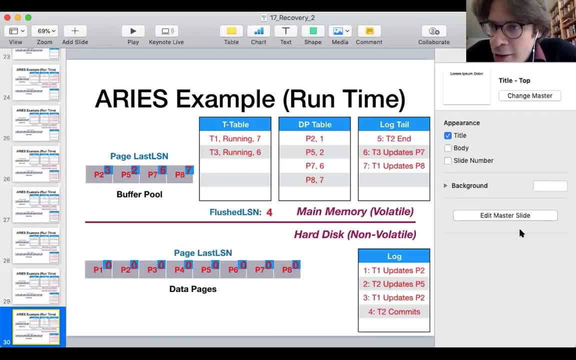 relatively very fast. um, it essentially means that before transaction commits, i means that before transaction commits, i means that before transaction commits i write all the associated changes to hard write, all the associated changes to hard write, all the associated changes to hard disk, disk disk. the problem with that is efficiency. 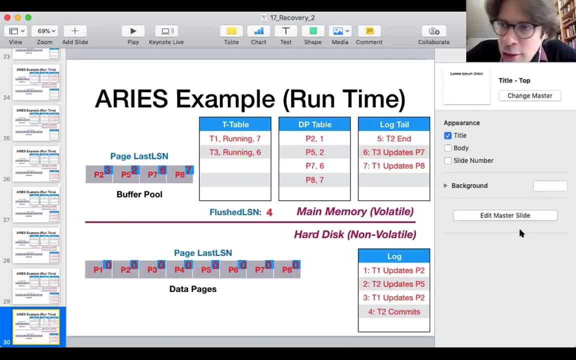 the problem with that is efficiency. the problem with that is efficiency, because if a transaction made lots of, because if a transaction made lots of, because if a transaction made lots of small changes on many different pages, small changes on many different pages, small changes on many different pages, then you would have to write all of. 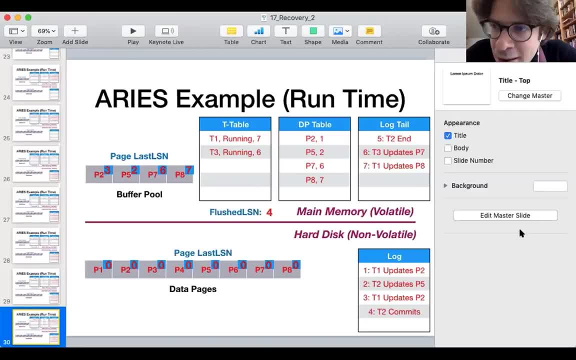 then you would have to write all of then. you would have to write all of those pages in the entirety to hard disk, those pages in the entirety to hard disk, those pages in the entirety to hard disk. they would have many, they would have many, they would have many page wide operations and it would 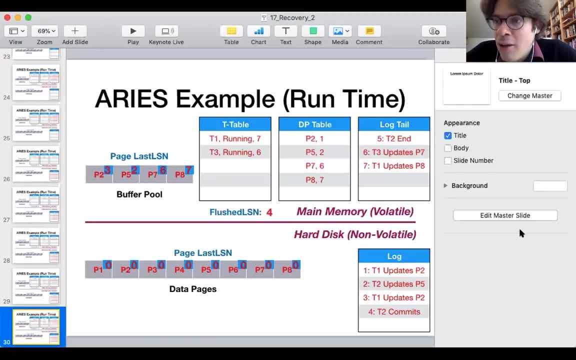 page wide operations and it would page wide operations and it would degrade. it would increase response time. degrade it would increase response time. degrade it would increase response time by quite a lot. so this is why people by quite a lot. so this is why people by quite a lot. so this is why people don't use it in practice, because of 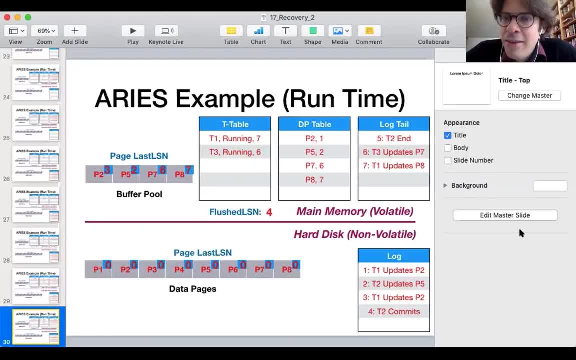 don't use it in practice because of. don't use it in practice because of performance reasons, performance reasons, performance reasons. the nice thing about logging is that the the nice thing about logging is that the the nice thing about logging is that the log essentially contains the same. 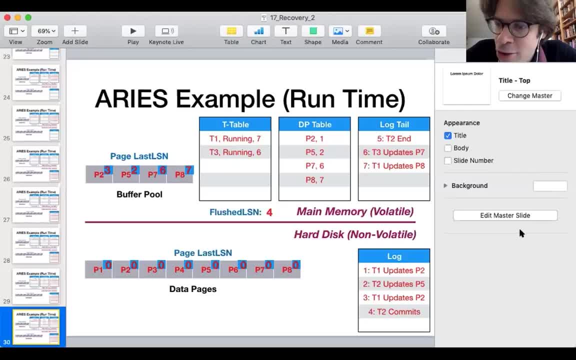 log essentially contains the same log essentially contains the same information, information, information. it also tells you which page pages were. it also tells you which page pages were. it also tells you which page pages were changed and how they were changed, changed and how they were changed, changed and how they were changed, and it allows you to compress those. 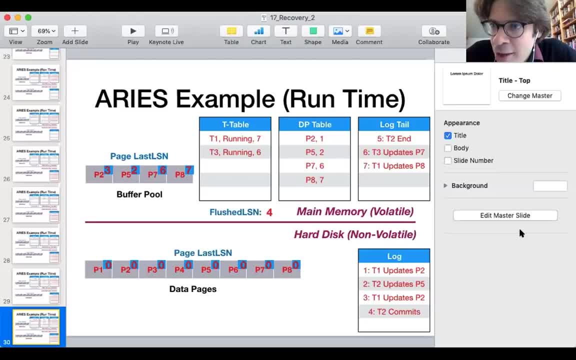 and it allows you to compress those, and it allows you to compress those changes into much fewer pages. so, instead, changes into much fewer pages. so instead, changes into much fewer pages. so, instead of writing, of writing, of writing, lots of data pages with small changes, you lots of data pages with small changes, you. 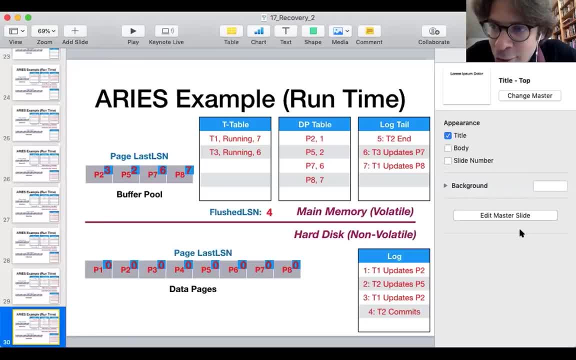 lots of data pages with small changes. you can just write at most one page, can just write at most one page, can just write at most one page with log entries which describe those with log entries, which describe those with log entries, which describe those changes, changes, changes in a very concise manner. so 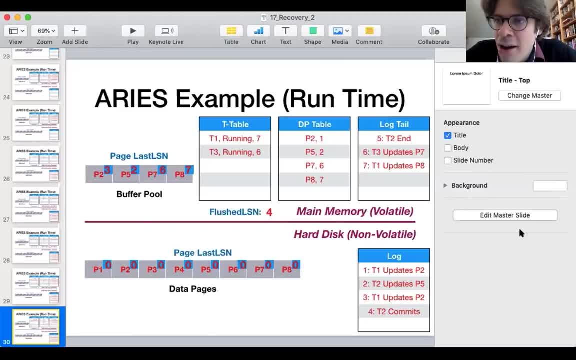 in a very concise manner. so in a very concise manner. so we avoid writing the pages, for we avoid writing the pages, for we avoid writing the pages for efficiency reasons, but instead we make efficiency reasons. but instead we make efficiency reasons, but instead we make sure that we write the log, which means 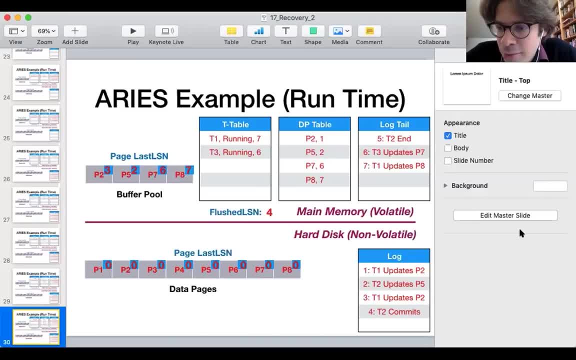 sure that we write the log, which means sure that we write the log, which means that we could redo those changes. if that, we could redo those changes, if that we could redo those changes. if there was a crash, otherwise, we just. there was a crash otherwise, we just. 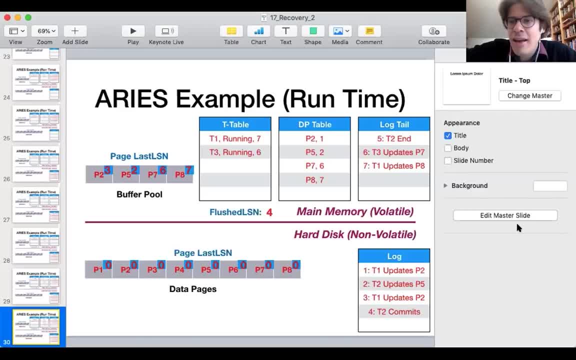 there was a crash. otherwise, we just rely on the changes to the data. that rely on the changes to the data. that rely on the changes to the data that they have written to disk. eventually they have written to disk. eventually they have written to disk, eventually. once we need more space in the buffer, 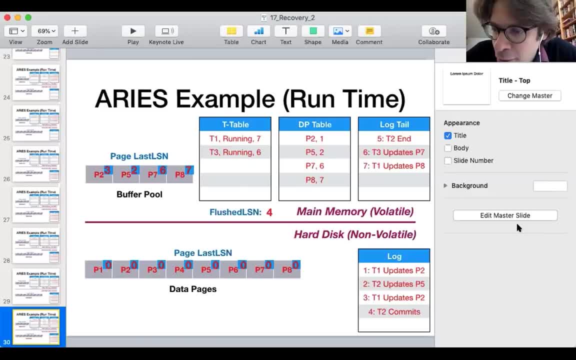 once we need more space in the buffer. once we need more space in the buffer, pool and pool and pool and need to free up one of the slots. need to free up one of the slots. need to free up one of the slots? great question, so that is why we do the. 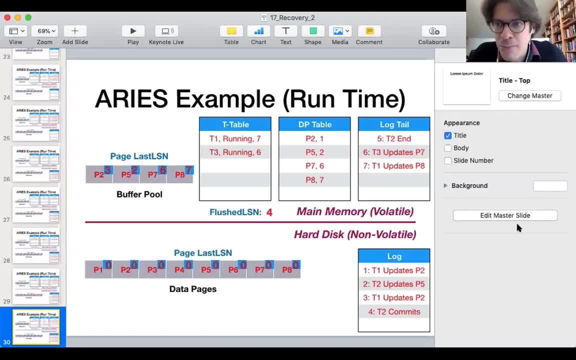 great question. so that is why we do the great question, so that is why we do the logging. so we don't need to logging, so we don't need to logging, so we don't need to write the corresponding data pages at. write the corresponding data pages at. 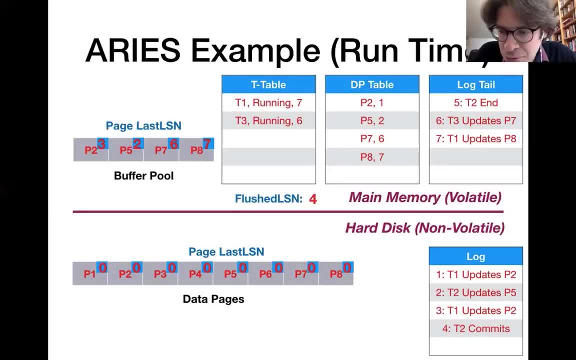 write the corresponding data pages at two hard disk. and now i already mentioned the case, and now i already mentioned the case, and now i already mentioned the case where we eventually write the pages to, where we eventually write the pages to, where we eventually write the pages to hard disk. if you need space in the 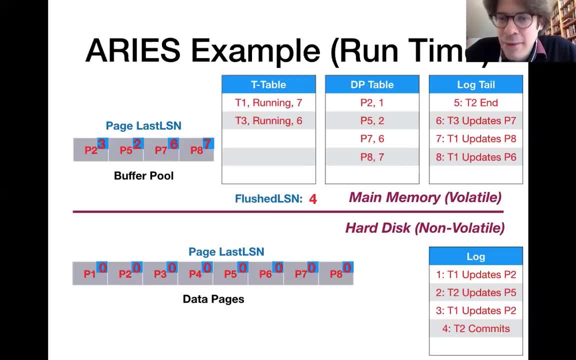 hard disk. if you need space in the hard disk, if you need space in the buffer pool- buffer pool, buffer pool- and with the next entry we have an, and with the next entry, we have an and with the next entry, we have an update to page number six by transaction. 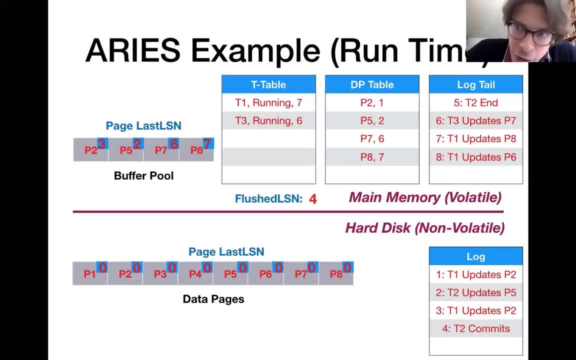 update to page number six by transaction. update to page number six by transaction one. and unfortunately we don't have page one, and unfortunately we don't have page one and unfortunately we don't have page number six in our buffer pool, number six in our buffer pool, number six in our buffer pool and we also don't have any space left in. 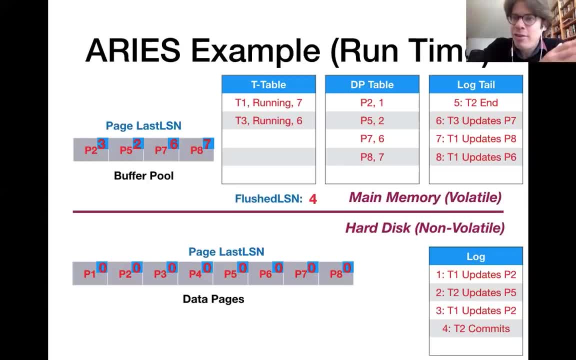 and we also don't have any space left in, and we also don't have any space left in our buffer pool, our buffer pool, our buffer pool. so we need to select one of those slots. so we need to select one of those slots. so we need to select one of those slots in a buffer pool in order to free it up. 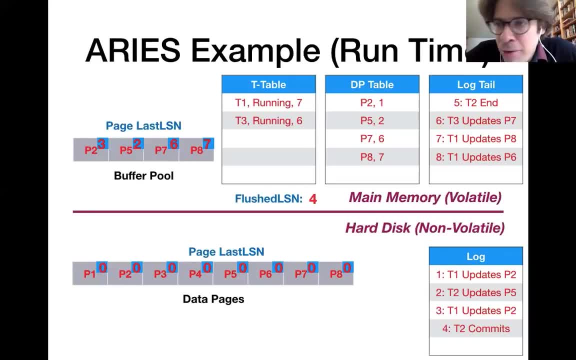 in a buffer pool in order to free it up, in a buffer pool in order to free it up. and since we currently have, and since we currently have, and since we currently have unpersistent changes in those buffer, unpersistent changes in those buffer, unpersistent changes in those buffer pool pages, 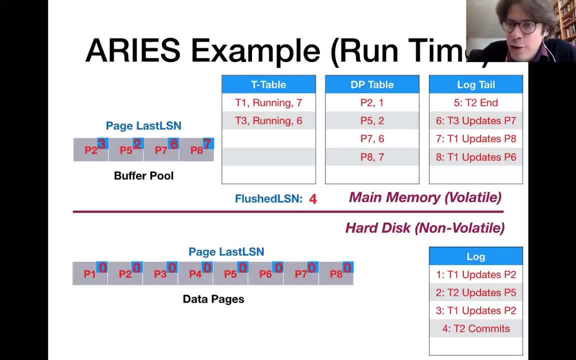 pool pages. pool pages. before i can free it up, i first need to. before i can free it up, i first need to. before i can free it up, i first need to back up the changes, back up the changes, back up the changes to hard disk we have discussed about. 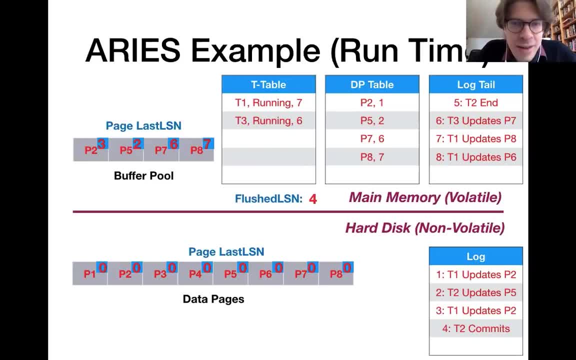 to hard disk. we have discussed about to hard disk. we have discussed about placement this one over here. so what i placement this one over here. so what i placement this one over here. so what i need to do is that i write the content. need to do is that i write the content. 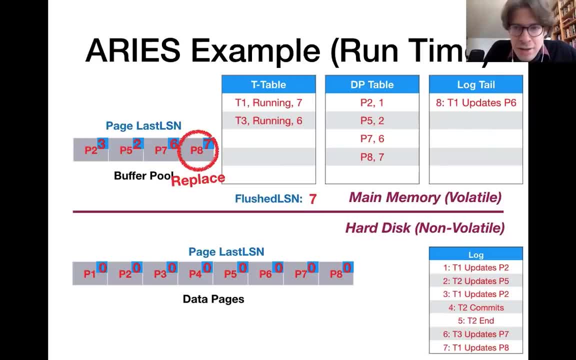 need to do is that i write the content of this page, of this page, of this page um back to a hard disk, and before i can um back to a hard disk and before i can um back to a hard disk, and before i can do that, do that. 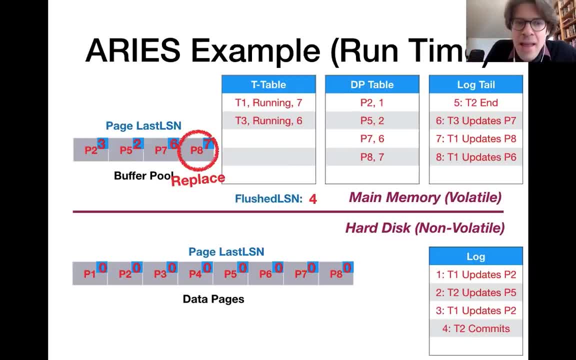 do that in order to follow the rules of a, in order to follow the rules of a, in order to follow the rules of a- right-ahead login. right-ahead login. right-ahead login- i need to make sure that i persist all. i need to make sure that i persist all. 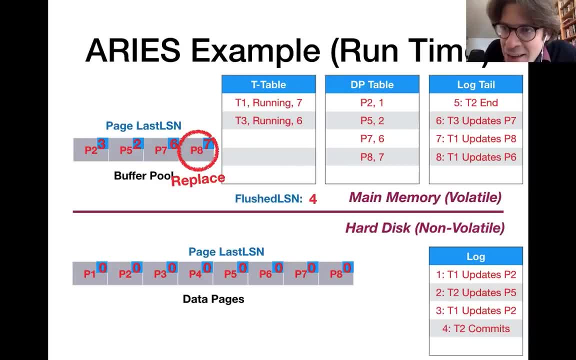 i need to make sure that i persist all the log entries that affect the page, the log entries that affect the page, the log entries that affect the page number eight to hard disk first number. eight to hard disk first number. eight to hard disk first. i need to do that if, for instance, the 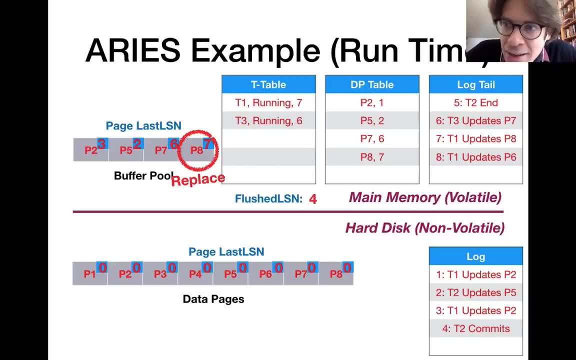 i need to do that if, for instance, the i need to do that if, for instance, the transaction transaction transaction that made the change to page number eight, that made the change to page number eight, that made the change to page number eight, later decides to abort, or if it is. 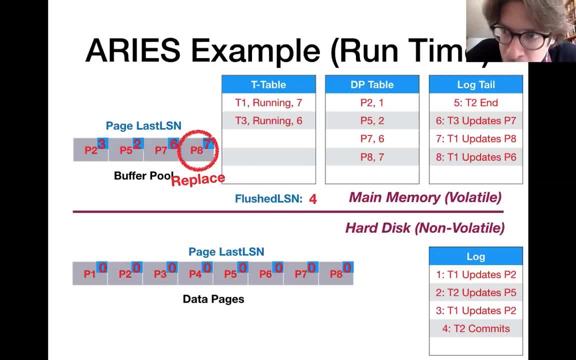 later decides to abort, or if it is later decides to abort, or if it is running and there's a crash which means running, and there's a crash which means running, and there's a crash which means that we want to abort it by default, that we want to abort it by default. 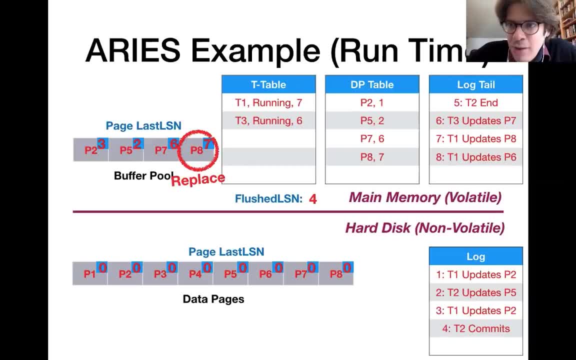 that we want to abort it by default? um then i need to be able to undo those. um then i need to be able to undo those? um then i need to be able to undo those changes. changes, changes of the partially executed transaction, of the partially executed transaction. 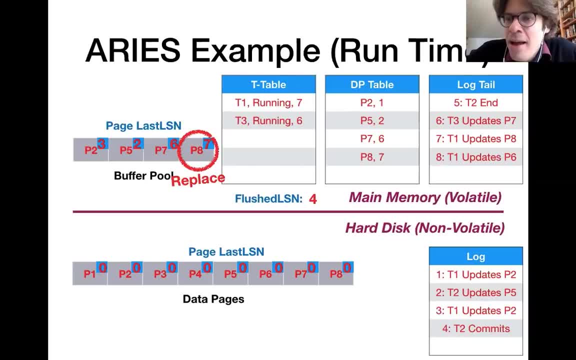 of the partially executed transaction that i am now about to write to hard, that i am now about to write to hard, that i am now about to write to hard disk, and this is why disk and this is why disk, and this is why i need to ensure that all the log entries 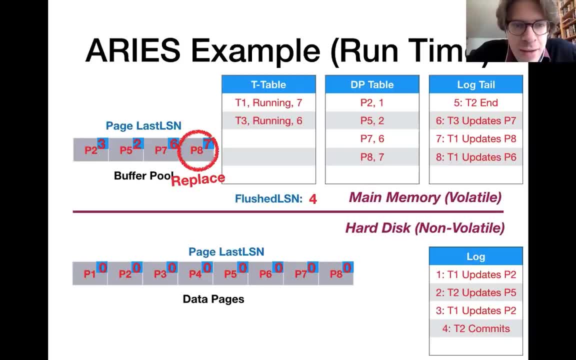 i need to ensure that all the log entries, i need to ensure that all the log entries that affected this page, that affected this page, that affected this page, are written to hard disk first. and here are written to hard disk first. and here are written to hard disk first. and here the page lsn of page eight. 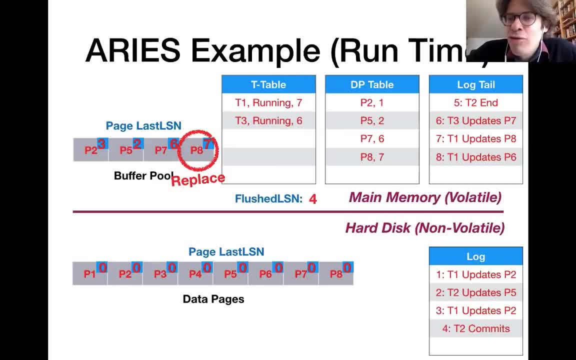 the page lsn of page eight. the page lsn of page eight is uh seven, so i have to write all. the is uh seven, so i have to write all. the is uh seven, so i have to write all the log entries after log entry seven. log entries after log entry seven. 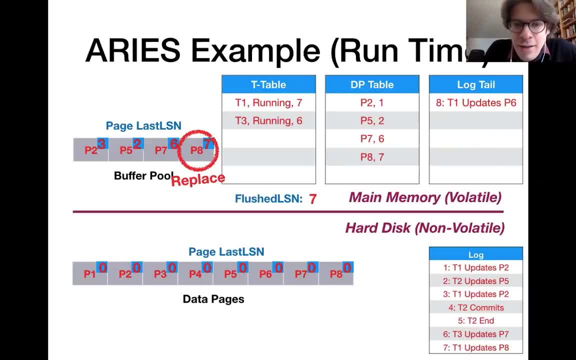 log entries. after log entry seven: uh from the log tail to hard disk and uh from the log tail to hard disk and uh from the log tail to hard disk. and i have to update, i have to update, i have to update the flashed at us and, and now i'm ready, 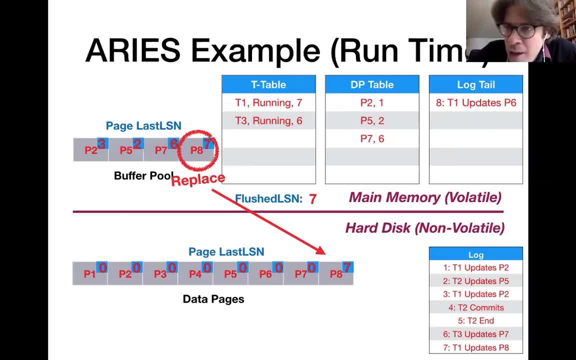 the flashed at us, and, and now i'm ready, the flashed at us, and, and now i'm ready to write. page number eight a two hard to write. page number eight, a two hard to write. page number eight a two hard disk. you see that the page it is. 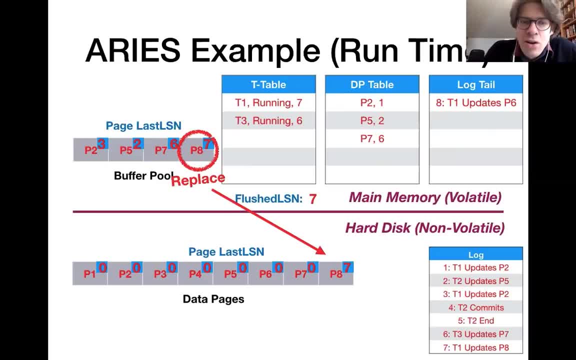 disk. you see that the page it is disk. you see that the page it is in one hard disk finally changes and in one hard disk finally changes. and in one hard disk finally changes and also um. now i want to also um. now i want to also um. now i want to take out the page number eight from the 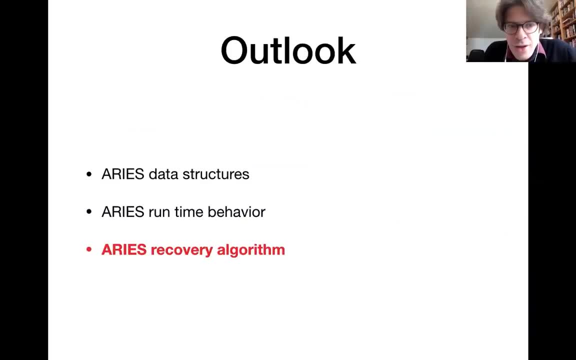 take out the page number eight from the. take out the page number eight from the dirty page table. all right, so that was a little example. all right, so that was a little example. all right, so that was a little example for the runtime phase. next time we're. 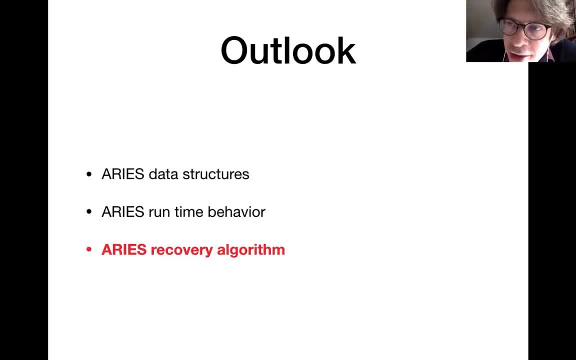 for the runtime phase. next time we're for the runtime phase, next time we're going to discuss about the recovery, going to discuss about the recovery, going to discuss about the recovery phase, which is invoked after the system phase, which is invoked after the system phase, which is invoked after the system comes back online after a crash. 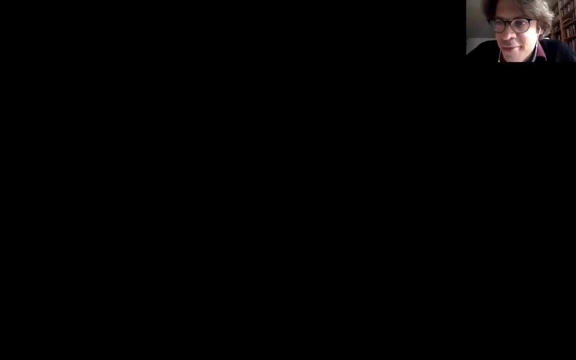 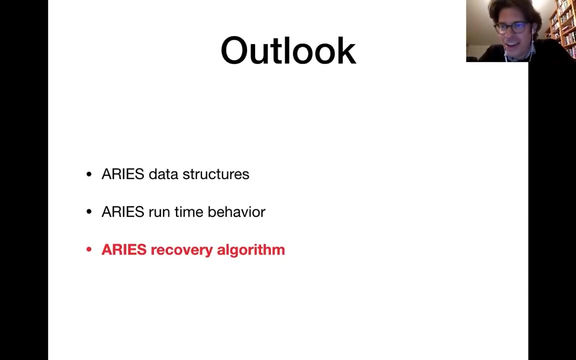 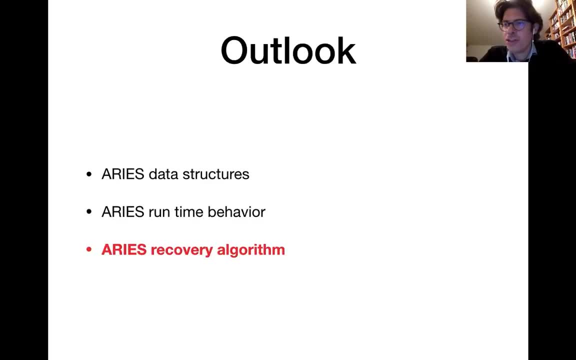 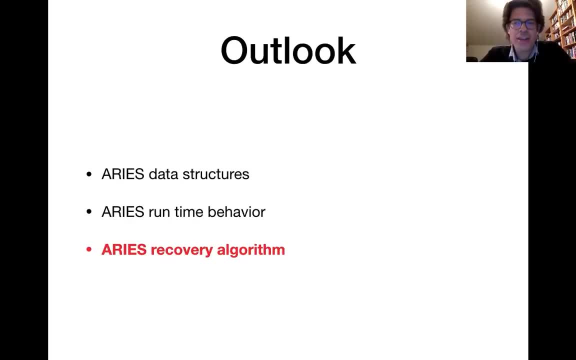 bring the database back into a. bring the database back into a consistent state after a system crash. consistent state after a system crash. consistent state after a system crash, and, and, and- the last time we have been discussing, the last time we have been discussing, the last time we have been discussing about one algorithm to do that. 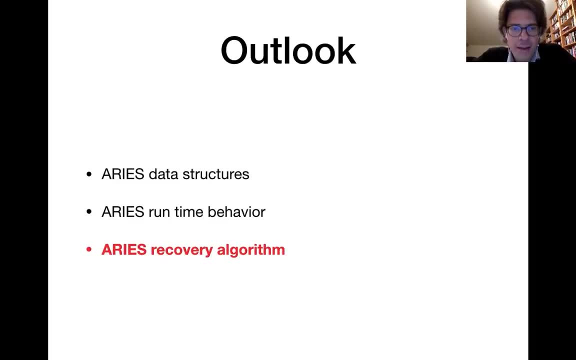 about one algorithm to do that, about one algorithm to do that, which is the arias algorithm, which is the arias algorithm, which is the arias algorithm. now for this algorithm, we have first of now for this algorithm. we have first of now for this algorithm, we have first of all discussed about the data structures. 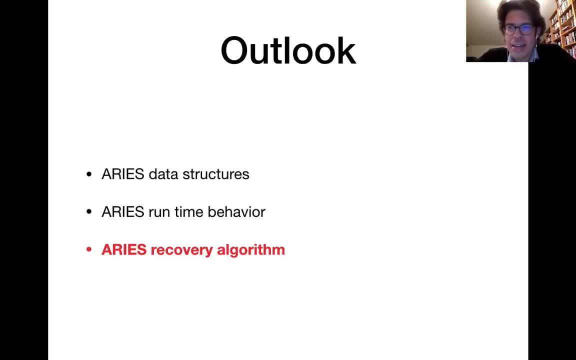 all discussed about the data structures, all discussed about the data structures it uses, which include some data it uses, which include some data it uses, which include some data structures in a main memory and some on structures in a main memory and some on structures in a main memory and some on hard disk. 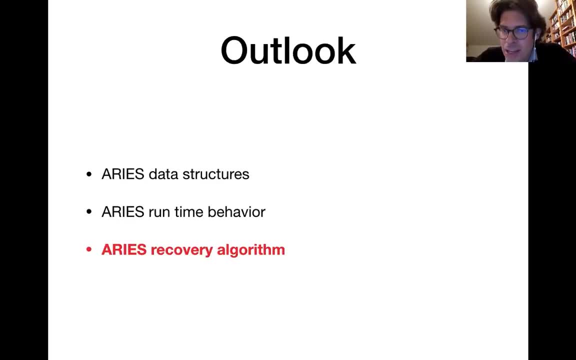 hard disk. hard disk. then we have discussed about how the. then we have discussed about how the. then we have discussed about how the algorithm, algorithm, algorithm behaves under normal circumstances, behaves under normal circumstances, behaves under normal circumstances. and now, in the following, we're going to: and now in the following we're going to: 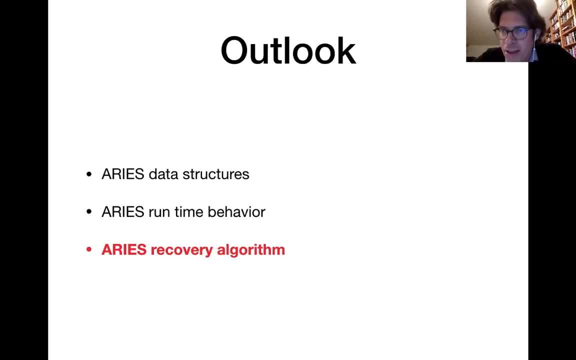 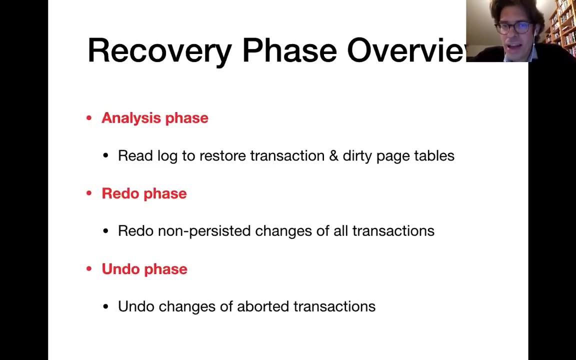 and now, in the following, we're going to discuss about, discuss about, discuss about how the algorithm does the recovery, how the algorithm does the recovery, how the algorithm does the recovery after a system crash. so the recovery has three phases. so the recovery has three phases. so the recovery has three phases. first of all, we have the 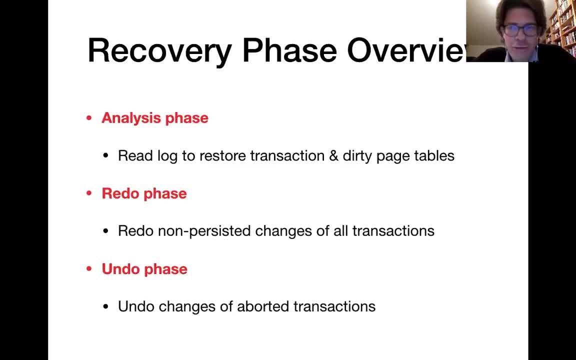 first of all we have the first of all, we have the analysis phase, then we have the redo analysis phase, then we have the redo analysis phase, then we have the redo phase and finally we have the undo phase phase and finally we have the undo phase phase and finally we have the undo phase. so, during the analysis phase, the 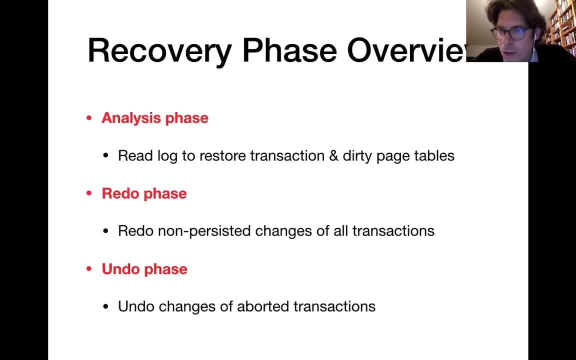 so during the analysis phase, the so, during the analysis phase, the algorithm restores a certain data algorithm restores a certain data algorithm, restores a certain data structures, which structures, which structures, which is the transaction table and the dirty is the transaction table and the dirty is the transaction table and the dirty page table, the transaction table. 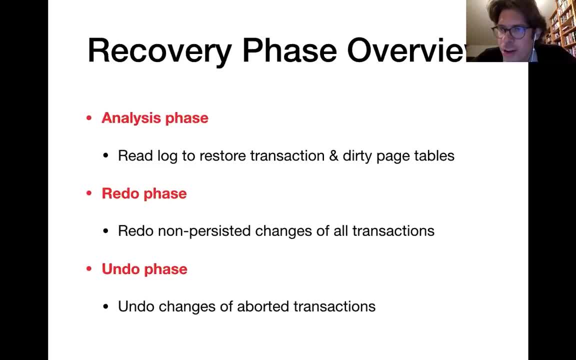 page table. the transaction table page table. the transaction table essentially gives an overview, essentially gives an overview, essentially gives an overview of the transactions that are currently of the transactions that are currently, of the transactions that are currently running, running, running and their status. the dirty page table and their status. the dirty page table. 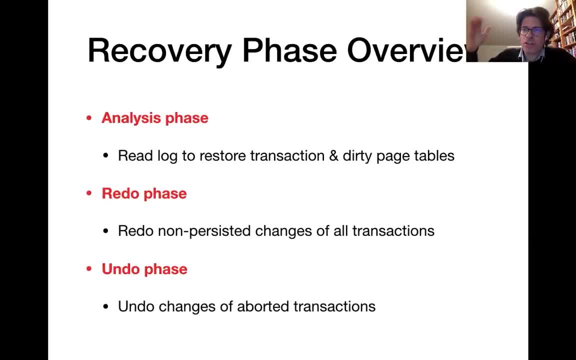 and their status. the dirty page table keeps track of pages. keeps track of pages. keeps track of pages where the in-memory version deviates, where the in-memory version deviates, where the in-memory version deviates from the hard disk version. so we have from the hard disk version. so we have. 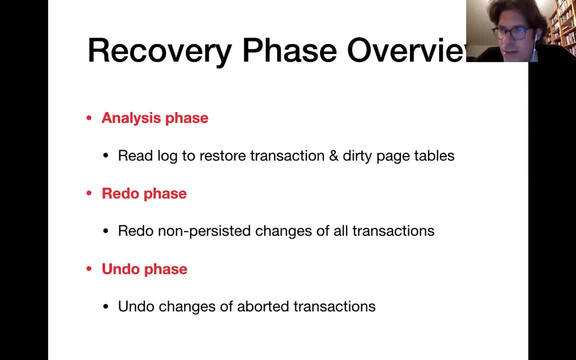 from the hard disk version. so we have changes in main memory, changes in main memory, changes in main memory that have not been made persistent yet, that have not been made persistent yet, that have not been made persistent yet, and with the dirty page table and with the dirty page table. 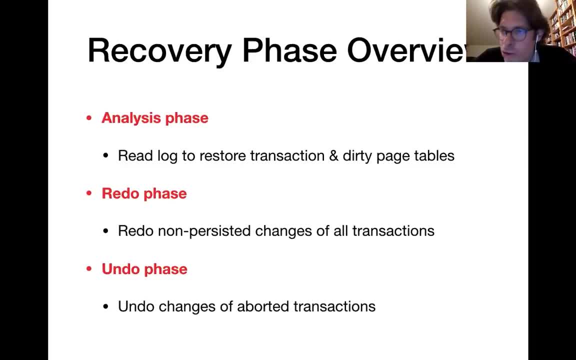 and with the dirty page table, we keep track of which pages are. we keep track of which pages are. we keep track of which pages are concerned by that concerned, by that concerned by that. during the redo phase, we are redoing. during the redo phase, we are redoing. 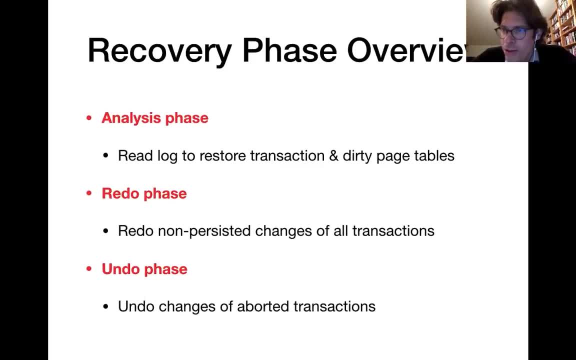 during the redo phase, we are redoing changes of committed transactions, or of changes of committed transactions, or of changes of committed transactions or of transactions in general that have not been transactions in general, that have not been transactions in general, that have not been made made made persistent yet during the undo phase. 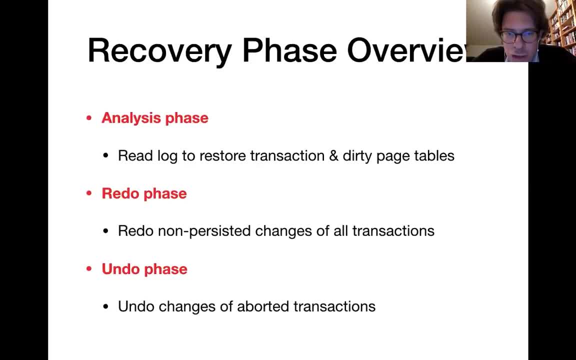 persistent yet during the undo phase. persistent yet during the undo phase. we are undoing the operations of. we are undoing the operations of. we are undoing the operations of transactions, transactions, transactions that are aborted, for instance, because that are aborted, for instance, because that are aborted, for instance, because they have been running. 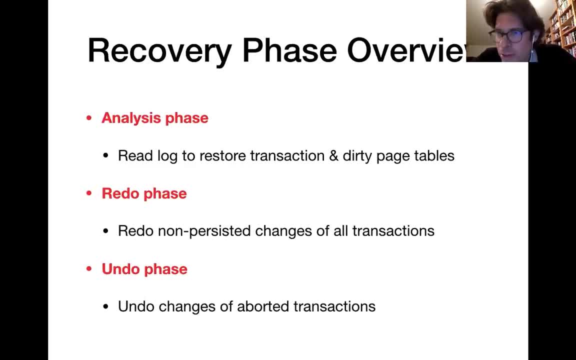 they have been running, they have been running at the point of the crash. so for those at the point of the crash, so for those at the point of the crash, so for those transactions, transactions, transactions- in the end the database should look as if. in the end, the database should look as if. 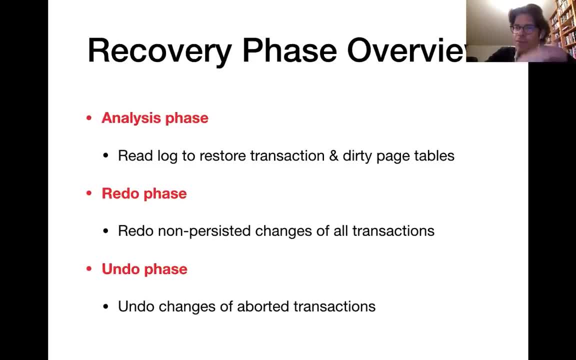 in the end, the database should look as if those transactions, those transactions, those transactions had never happened now in the following had never happened now in the following had never happened now in the following. we're gonna discuss those different faces. we're gonna discuss those different faces. we're gonna discuss those different faces in more detail. 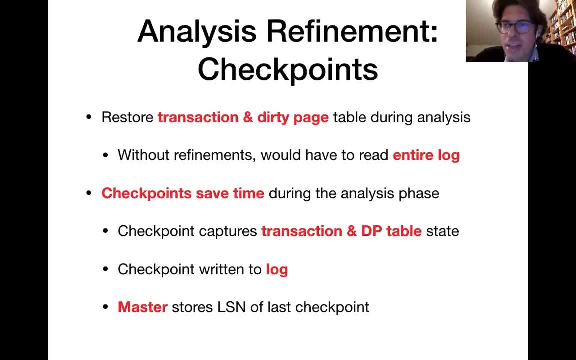 now one remark about the analysis phase. now one remark about the analysis phase. now one remark about the analysis phase. so i have already quickly mentioned that, so i have already quickly mentioned that. so i have already quickly mentioned that: during the analysis phase, our goal. during the analysis phase, our goal. 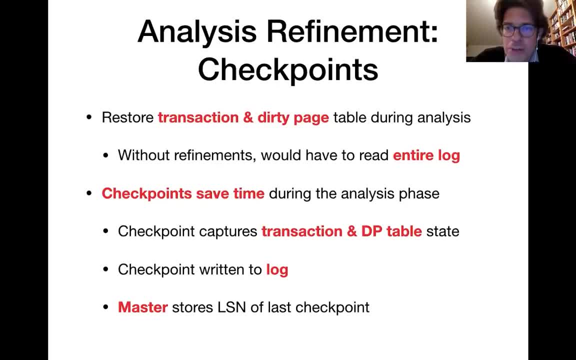 during the analysis phase. our goal is to restore the transaction table and is to restore the transaction table and is to restore the transaction table and the dirty page, the dirty page, the dirty page table. now we are restoring those data table. now we are restoring those data table. now we are restoring those data structures. 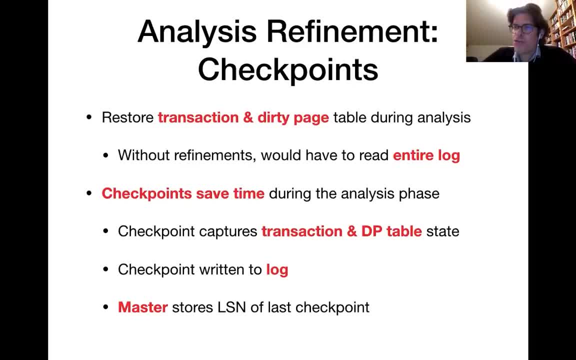 structures, structures by reading the log entries. which, by reading the log entries, which, by reading the log entries which describe the different, describe the different, describe the different, updates to the data transaction commits, updates to the data transaction commits, updates to the data transaction commits, and so on and so forth, and 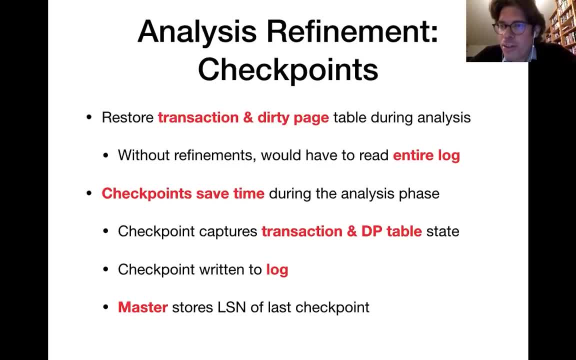 and so on and so forth, and and so on and so forth, and without any, without any, without any checkpoints, we would essentially have to checkpoints, we would essentially have to checkpoints, we would essentially have to read that log from the beginning of time. read that log from the beginning of time. 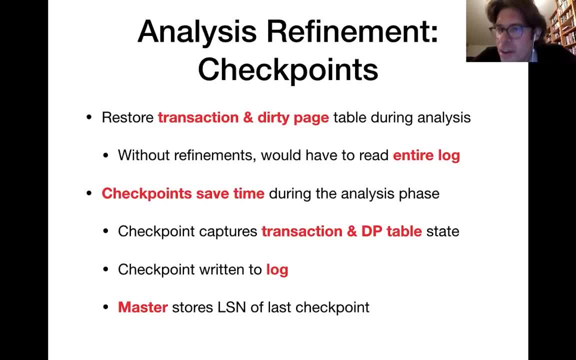 read that log from the beginning of time in order to restore our data structures, in order to restore our data structures, in order to restore our data structures, and of course that would be very, and of course that would be very and of course that would be very inefficient. so we 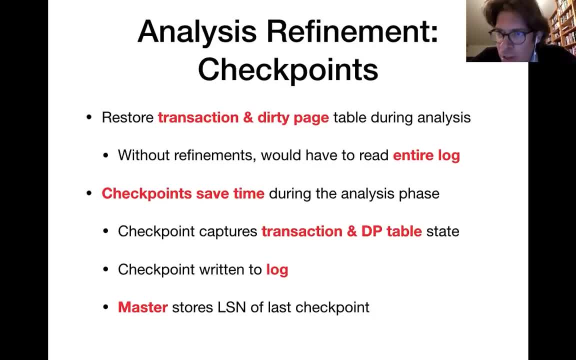 inefficient, so we inefficient, so we want to make the recovery as efficient, as want to make the recovery as efficient, as want to make the recovery as efficient as possible, and the checkpoints are a way possible, and the checkpoints are a way possible and the checkpoints are a way to make it more efficient. 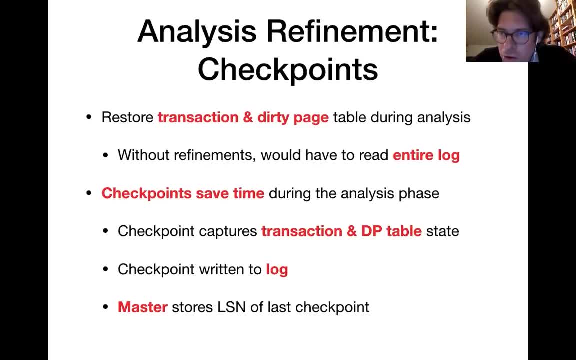 to make it more efficient. to make it more efficient. so during a checkpoint, they essentially so. during a checkpoint, they essentially so during a checkpoint, they essentially save the current state of the, save the current state of the, save the current state of the transaction table and dirty page table. 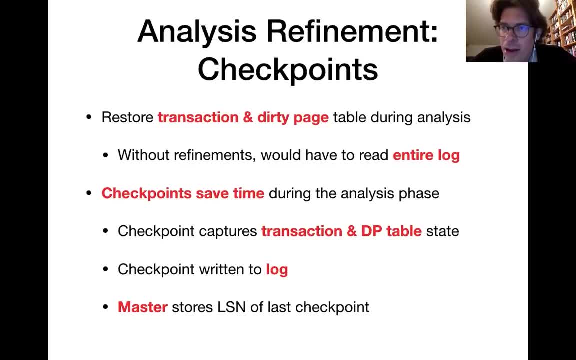 transaction table and dirty page table. transaction table and dirty page table. to hard disk, to hard disk to hard disk. and those checkpoints are also written, and those checkpoints are also written. and those checkpoints are also written to the log, to the log. to the log we have one so-called a master record. 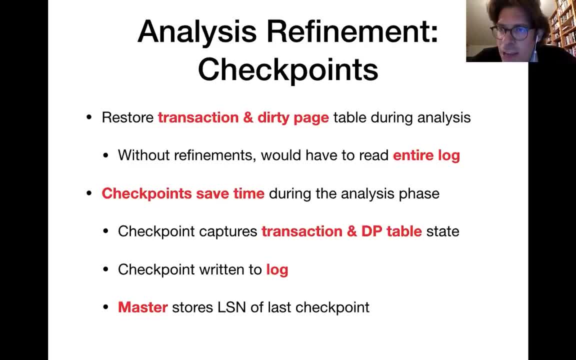 we have one so-called a master record. we have one so-called a master record stored, stored, stored on hard disk, which gives us the location on hard disk, which gives us the location on hard disk, which gives us the location within the log, within the log, within the log of the last checkpoint. so, because of that, 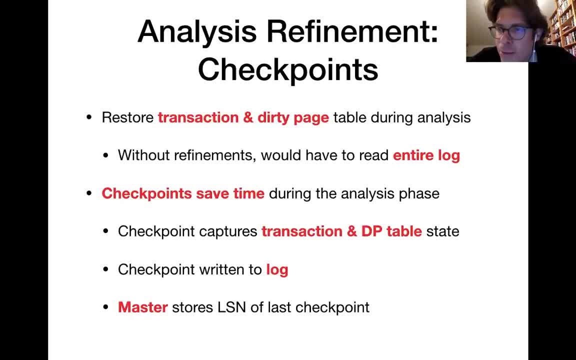 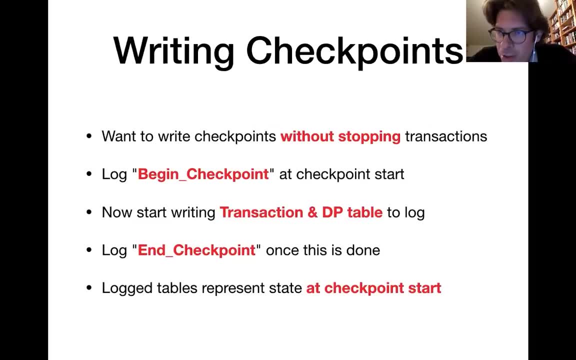 of the last checkpoint. so because of that of the last checkpoint, so because of that, we can avoid, we can avoid, we can avoid reading the log from the very beginning. now, this is how we write those. now, this is how we write those. now, this is how we write those checkpoints. uh, one important uh thing. 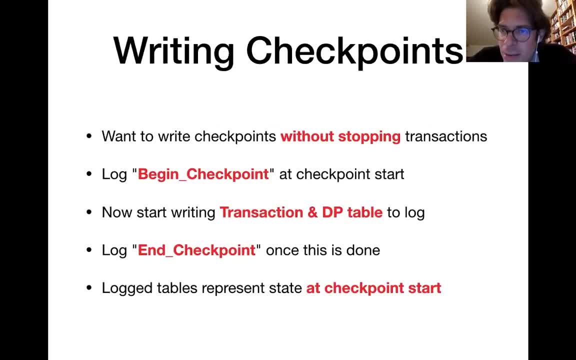 checkpoints, uh one important uh thing. checkpoints, uh one important uh thing that we want, that we want, that we want. we want to avoid having to stop the. we want to avoid having to stop the. we want to avoid having to stop the database in order to write out those. 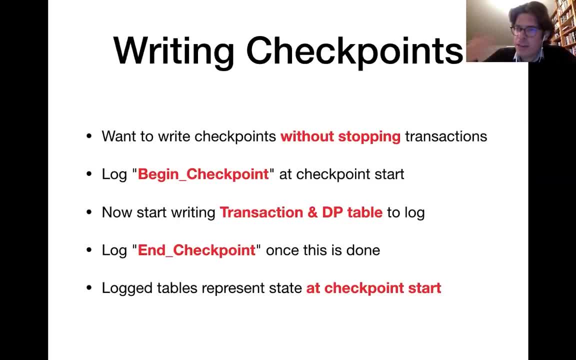 database in order to write out those database, in order to write out those checkpoints. so we want to continue checkpoints, so we want to continue checkpoints, so we want to continue processing transactions as they come in, processing transactions as they come in, processing transactions as they come in, while in the background, we are. 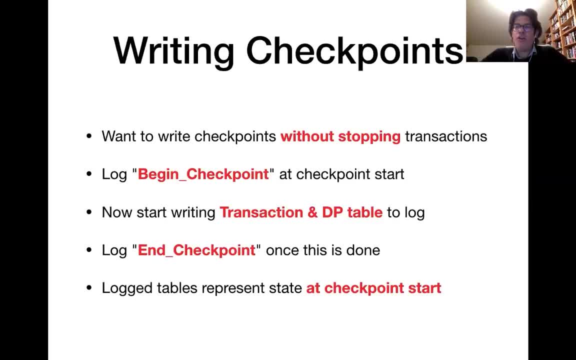 while in the background we are, while in the background we are processing the checkpoint, processing the checkpoint, processing the checkpoint now um writing out those data now, um writing out those data now, um writing out those data structures- the transaction table and structures, the transaction table and structures, the transaction table and the dirty page table. 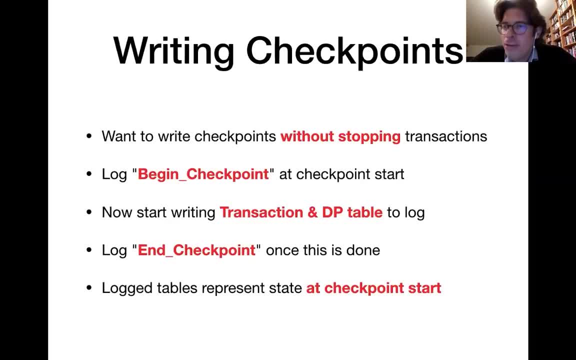 the dirty page table. the dirty page table, it takes a little bit of time. so it takes a little bit of time, so it takes a little bit of time. so, if we let the transactions continue, if we let the transactions continue, if we let the transactions continue, it means that the state of the 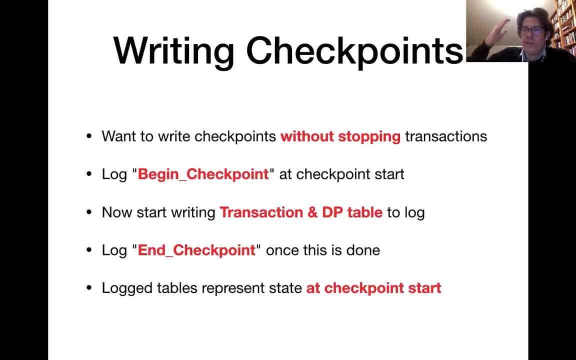 it means that the state of the. it means that the state of the transaction table and dirty page table. transaction table and dirty page table. transaction table and dirty page table. that we write out um to the lock. that we write out um to the lock. that we write out um to the lock. they will be probably outdated before we. 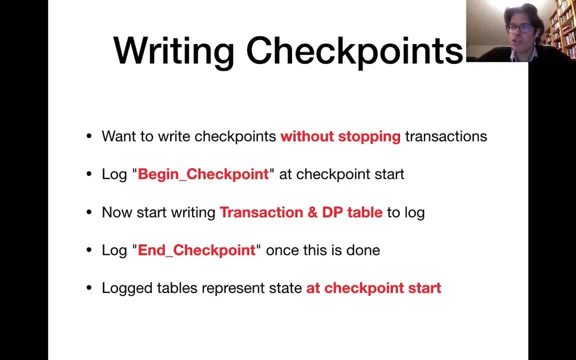 they will be probably outdated before we. they will be probably outdated before we even even even finish writing, and this is why it is very finish writing and this is why it is very finish writing, and this is why it is very important to mark up, important to mark up. 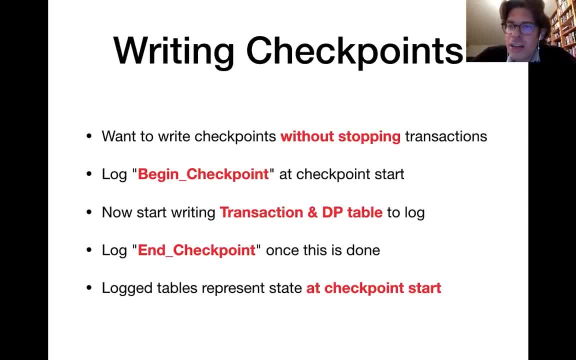 important to mark up in the log uh the point in time at which, in the log uh, the point in time at which, in the log uh, the point in time at which at this checkpoint is valid. at this checkpoint is valid. at this checkpoint is valid. so once we begin checkpointing, 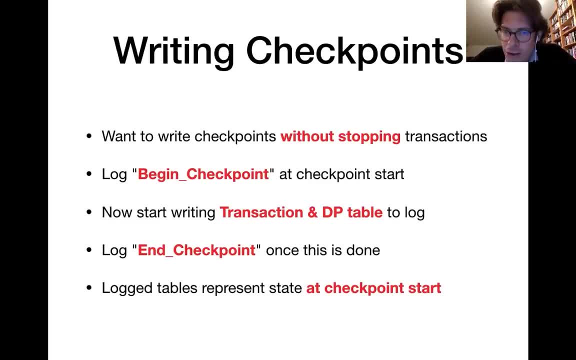 so once we begin checkpointing, so once we begin checkpointing, then we first of all write a begin, then we first of all write a begin, then we first of all write a begin checkpoint, a record into our log, and checkpoint a record into our log and checkpoint, a record into our log. and that essentially marks the point in. 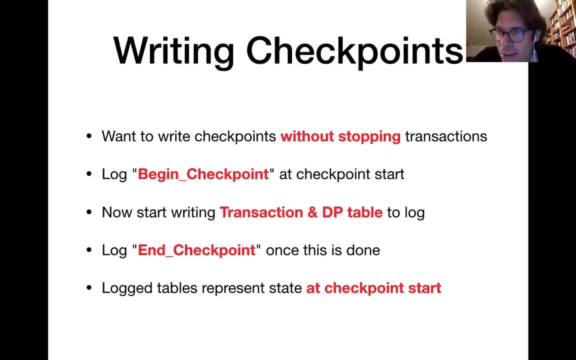 that essentially marks the point. in that essentially marks the point in time at which the checkpoint is valid, time at which the checkpoint is valid, time at which the checkpoint is valid and after writing this, begin checkpoint. and after writing this, begin checkpoint. and after writing this, begin checkpoint record. 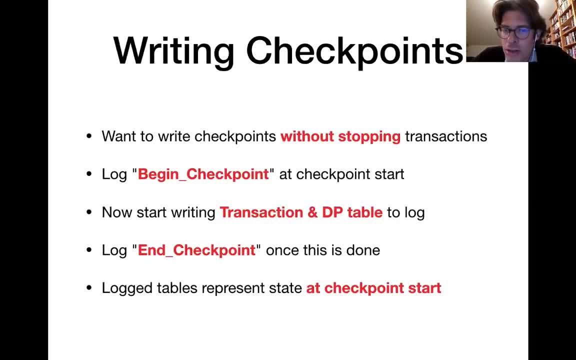 record record. we start writing the actual content of. we start writing the actual content of. we start writing the actual content of the transaction: the transaction, the transaction and a dirty page table while the and a dirty page table. while the and a dirty page table while the transactions. they keep. 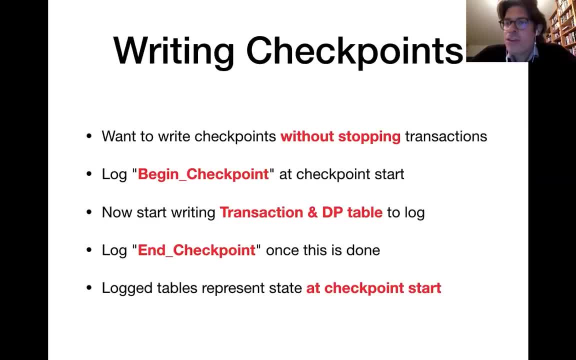 transactions. they keep transactions. they keep coming in and processing and thereby coming in and processing, and thereby coming in and processing, and thereby changing the transaction table and the changing the transaction table and the changing the transaction table and the dirty page table. dirty page table, dirty page table. so, once we have finished writing a 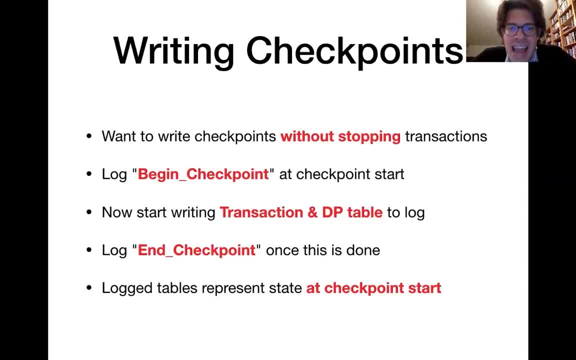 so once we have finished writing a, so once we have finished writing a transaction and dirty page table transaction and dirty page table transaction and dirty page table, then we write the end checkpoint, then we write the end checkpoint, then we write the end checkpoint, record, record, record. so, um, we know that checkpointing. 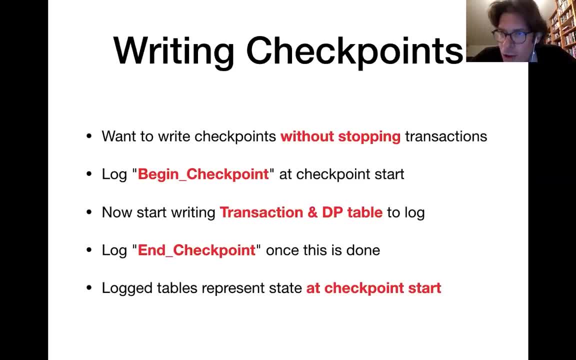 so, um, we know that checkpointing. so, um, we know that checkpointing has finished, but the has finished. but the has finished. but the state of the transaction and dirty page: state of the transaction and dirty page state of the transaction and dirty page table that we have written to hard disk. 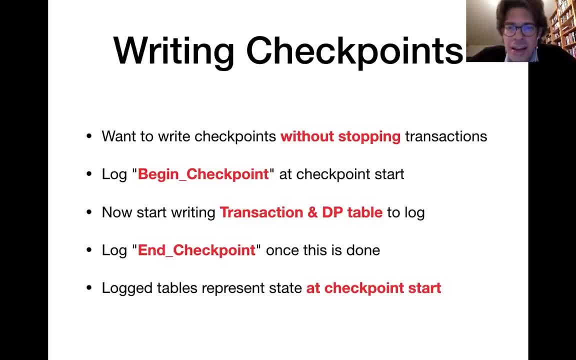 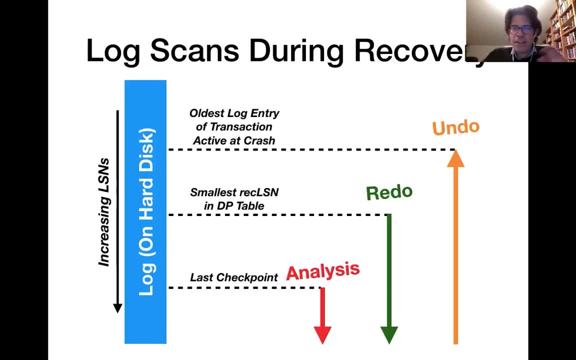 table that we have written to hard disk, table that we have written to hard disk is only valid at the begin. checkpoint is only valid at the begin. checkpoint is only valid at the begin. checkpoint: uh, record, uh, record, uh, record. all right, all right, all right, now now. 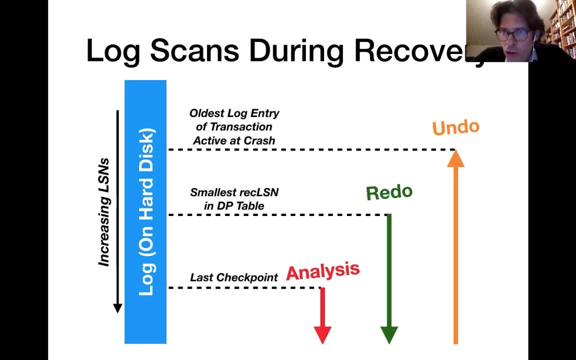 now, this is an overview of. which portion of this is an overview of? which portion of this is an overview of which portion of the log, the different phases, the log, the different phases, the log, the different phases. look at so, look at so, look at so. for the analysis phase, we start it. 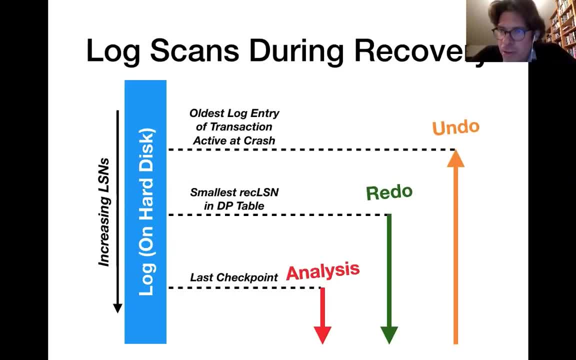 for the analysis phase. we start it for the analysis phase. we start it from the last checkpoint, from the last checkpoint, from the last checkpoint more precisely. we start looking at log more precisely. we start looking at log more precisely. we start looking at log entries, entries, entries at the begin, checkpoint, a record. 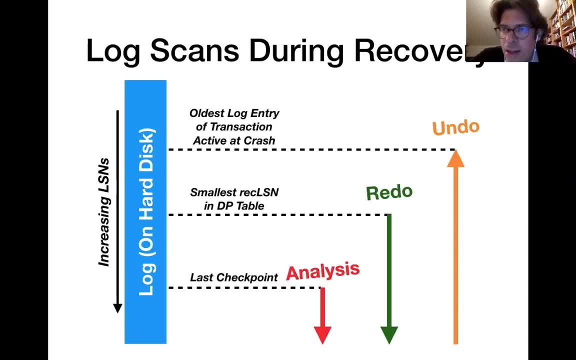 at the begin checkpoint, a record at the begin checkpoint, a record because, starting from there, because starting from there, because starting from there we might, we might, we might encounter log entries that are not encounter, log entries that are not encounter log entries that are not reflected in the transaction and dirty. 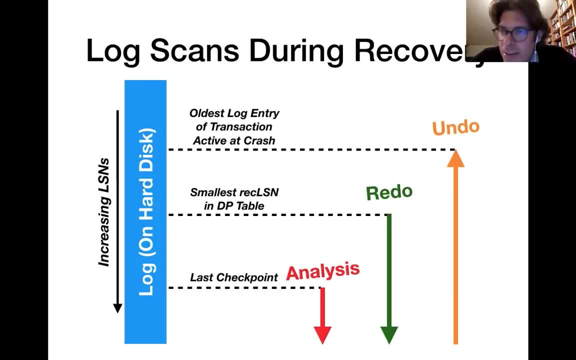 reflected in the transaction and dirty reflected in the transaction and dirty page table as it is page table, as it is page table, as it is represented in the checkpoint, represented in the checkpoint, represented in the checkpoint. so, starting from there, starting from the. so, starting from there, starting from the. 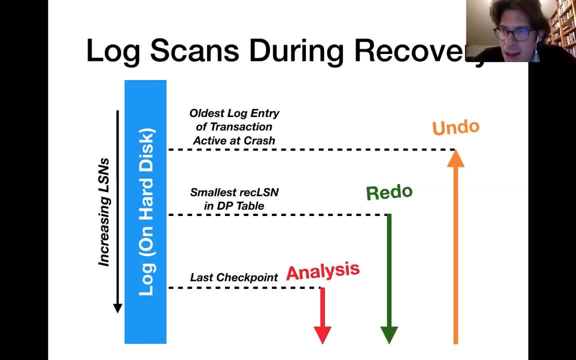 so, starting from there, starting from the checkpoint, we read checkpoint, we read checkpoint, we read the log um until we have reached the the log um, until we have reached the the log um, until we have reached the final entries before the system crash. final entries before the system crash. 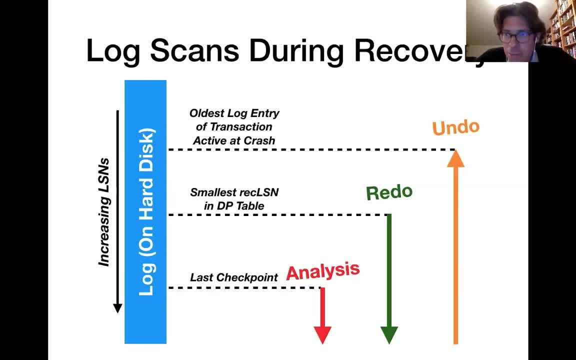 final entries before the system crash and and and in the redo phase. we start potentially in the redo phase. we start potentially in the redo phase. we start potentially even earlier, even earlier, even earlier. um, we essentially start with the um. we essentially start with the um. we essentially start with the earliest log entry. that 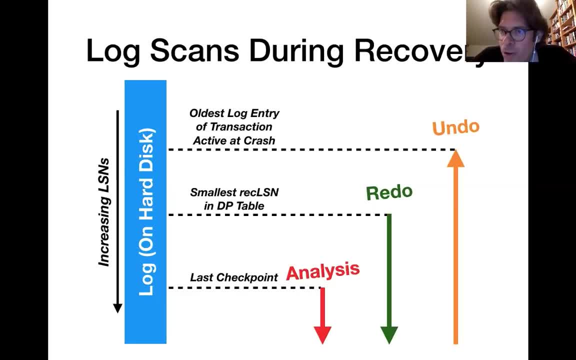 earliest log entry, that earliest log entry that might have changed one of our data, might have changed one of our data might have changed one of our data- pages, pages, pages- and is not yet persistent. and is not yet persistent and is not yet persistent on hard disk. so 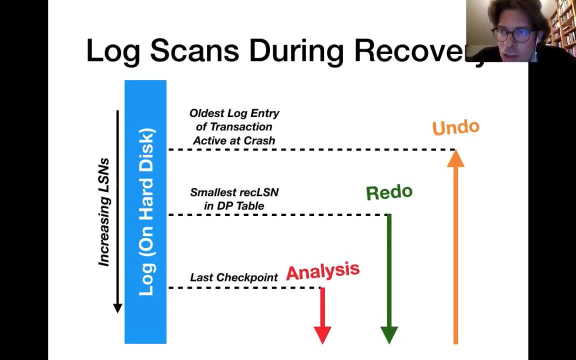 on hard disk, so on hard disk. so the dirty pages are those pages where the. the dirty pages are those pages where the. the dirty pages are those pages where the in-memory version, in-memory version, in-memory version deviates from the hardest version in the, deviates from the hardest version in the. 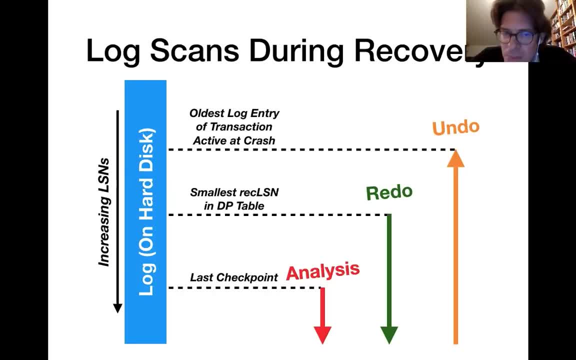 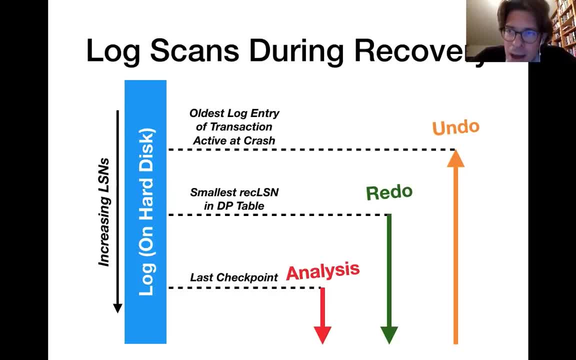 and we can use it in order to identify the log entry starting from which we, the log entry, starting from which we, the log entry starting from which we might have changes to the data that have, might have changes to the data that have, might have changes to the data that have not been made persistent yet. 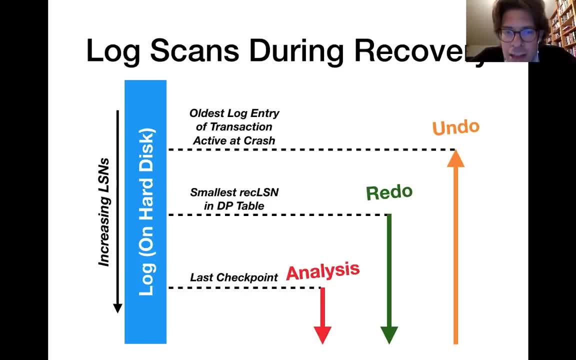 not been made persistent yet. not been made persistent yet. so we have to consider them during the. so we have to consider them during the. so we have to consider them during the redo phase. redo phase, redo phase. so in the dirty page table as a little. so in the dirty page table as a little. 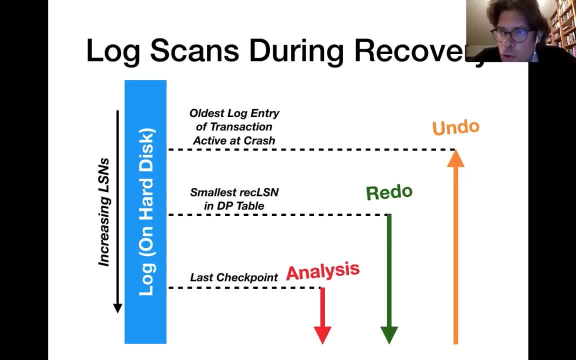 so in the dirty page table, as a little reminder, each page is associated with reminder. each page is associated with reminder. each page is associated with the so-called rack and is an entry, the so-called rack, and is an entry, the so-called rack, and is an entry. page dirty. 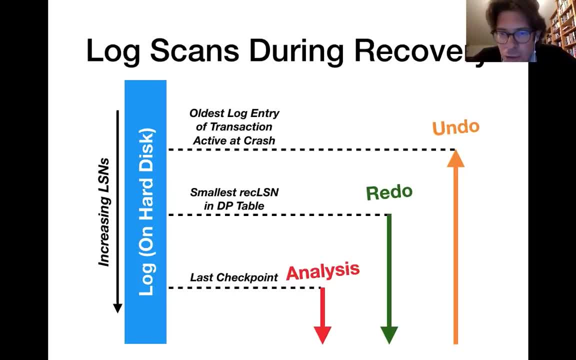 page dirty. page dirty meaning that the in-memory version, meaning that the in-memory version, meaning that the in-memory version deviates from the hard disk version, so deviates from the hard disk version, so deviates from the hard disk version. so, in order to know where to start the 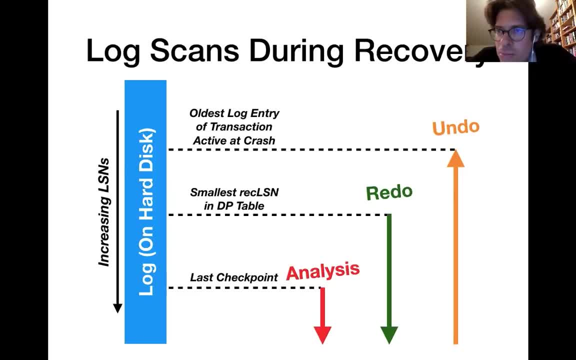 in order to know where to start the, in order to know where to start the redo phase from redo phase from. redo phase from, we just look at all the entries in the. we just look at all the entries in the. we just look at all the entries in the dirty page table. 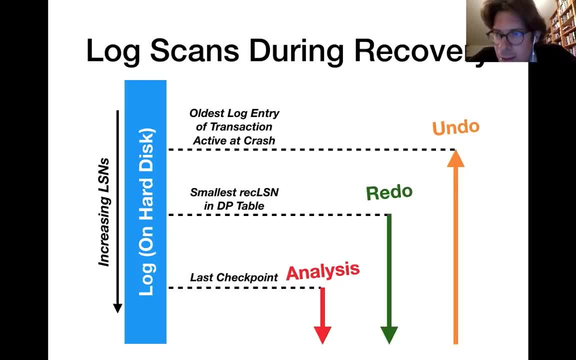 dirty page table. dirty page table: and identify the minimum rack lsn. this and identify the minimum rack lsn. this and identify the minimum rack lsn. this is where we start the redo phase, is where we start the redo phase, is where we start the redo phase from for the undo phase. 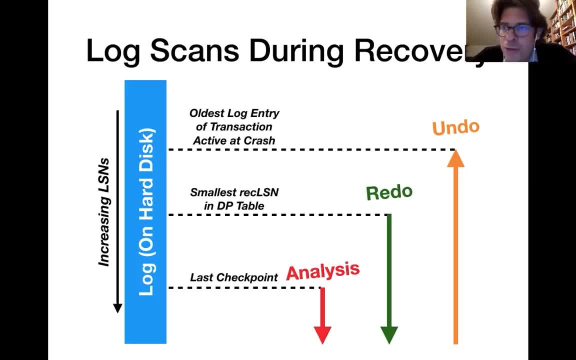 from for the undo phase. we are undoing the operations of. we are undoing the operations of. we are undoing the operations of aborted transactions or transactions. aborted transactions or transactions, aborted transactions or transactions that have been running at the point of, that have been running at the point of. 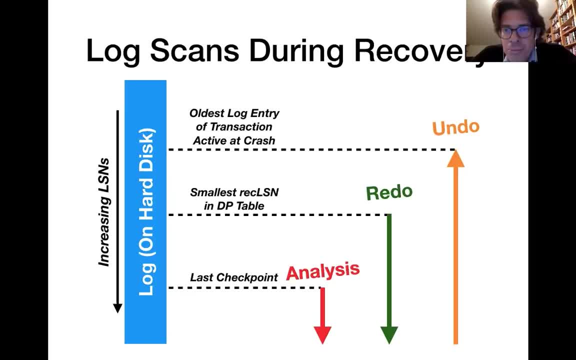 that have been running at the point of the crash. so we want to the crash, so we want to the crash, so we want to undo them, undo them, undo them, and here we want to undo the operations, and here we want to undo the operations and here we want to undo the operations of a transaction. 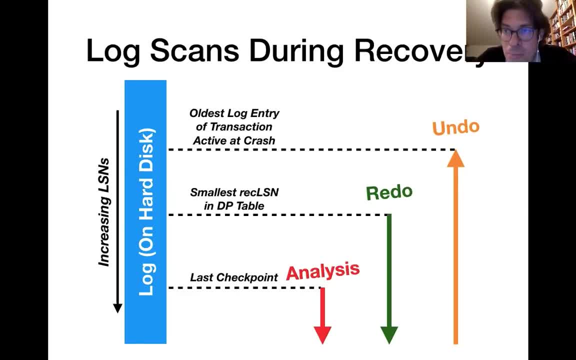 of a transaction, of a transaction in reverse order. so this is why we in reverse order. so this is why we in reverse order. so this is why we traverse the log, traverse the log, traverse the log backward, starting from the most recent backward, starting from the most recent. 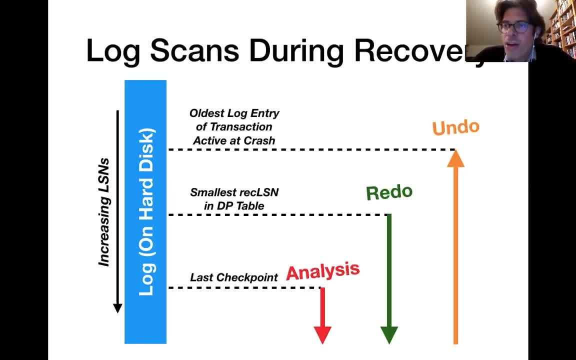 backward, starting from the most recent entries and going back to the earliest entries and going back to the earliest entries and going back to the earliest ones are no aborted ones are no aborted ones are no aborted. so this is the high level overview of. so this is the high level overview of. 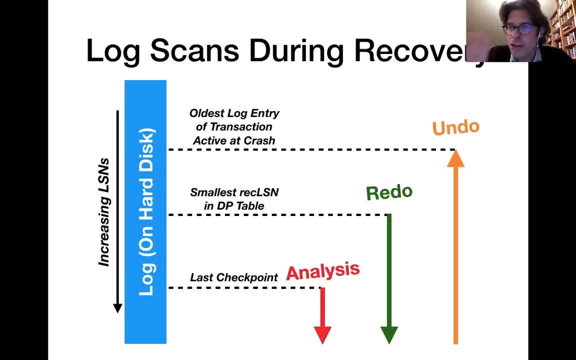 so this is the high level overview of how those different, how those different, how those different phases of recovery use the log phases of recovery, use the log phases of recovery, use the log. on the following we're going to discuss. on the following we're going to discuss: 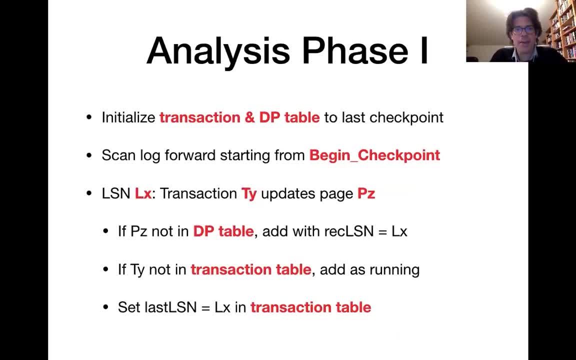 on the following. we're going to discuss them in a little bit more detail. so the analysis phase as discussed. so the analysis phase as discussed. so the analysis phase as discussed is about restoring the transaction, is about restoring the transaction, is about restoring the transaction and the dirty page table. 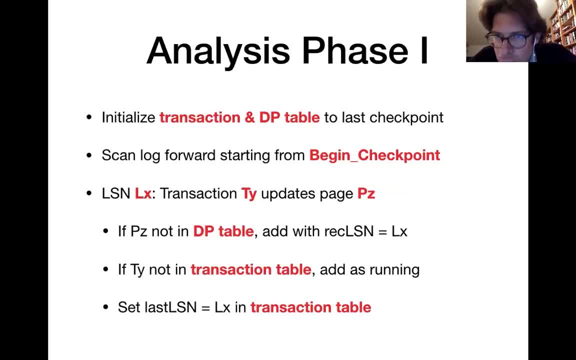 and the dirty page table and the dirty page table, so we start scanning from the last, so we start scanning from the last, so we start scanning from the last checkpoint. and if, for instance, we checkpoint, and if, for instance, we checkpoint, and if, for instance, we encounter a log entry stating that some 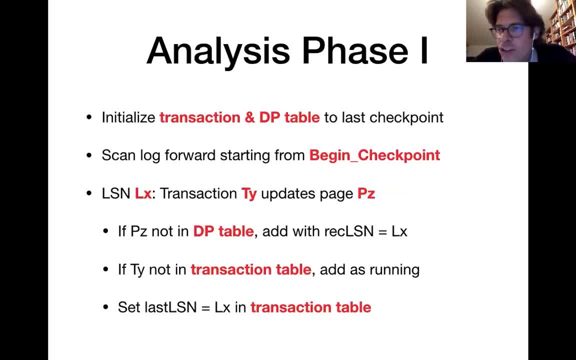 encounter a log entry stating that some encounter a log entry stating that some transaction ty has updated some page. transaction ty has updated some page. transaction ty has updated some page pset and the pset and the pset and the log entry has the log sequence number. 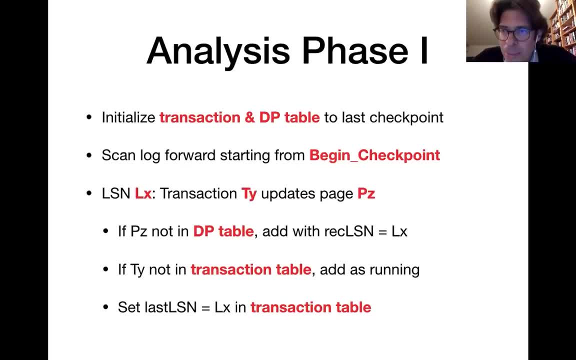 log entry has the log sequence number. log entry has the log sequence number lx. then we first of all lx, then we first of all lx, then we first of all update the dirty page table. we check: update the dirty page table. we check, update the dirty page table. we check whether the page 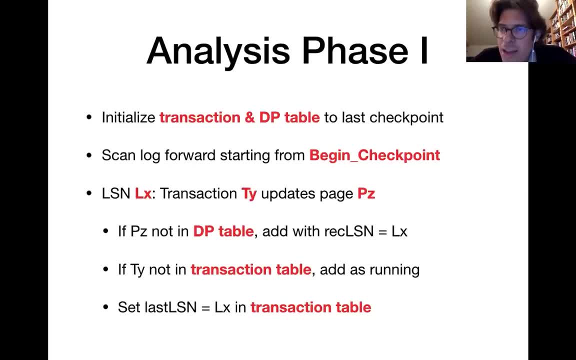 whether the page, whether the page pset is not in the dirty page table. pset is not in the dirty page table. pset is not in the dirty page table. if it is not included, then we insert it. if it is not included, then we insert it. 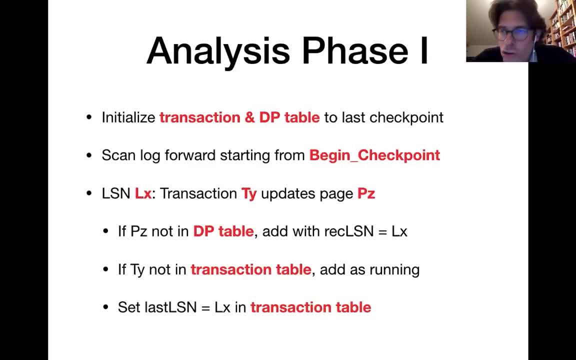 if it is not included, then we insert it with rack lsn set to the current log. with rack lsn set to the current log. with rack lsn set to the current log. entry number lx. because the rack lsn entry number lx. because the rack lsn. 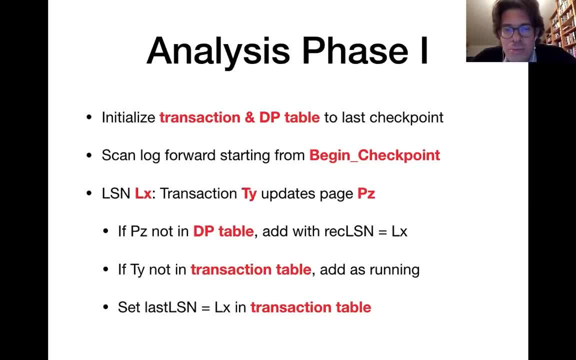 entry number lx, because the rack lsn always gives you the earliest log entry. always gives you the earliest log entry. always gives you the earliest log entry. that made a page dirty. that made a page dirty. that made a page dirty. if the transaction ty is and not in a 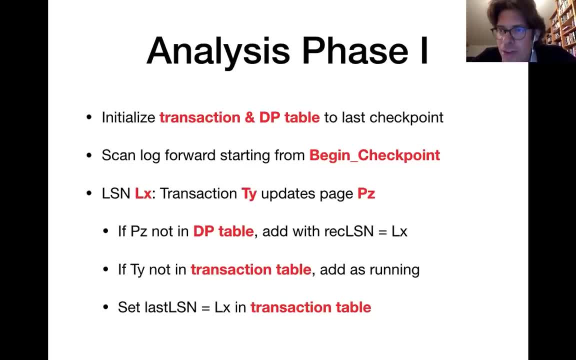 if the transaction ty is and not in a, if the transaction ty is and not in a transaction table- transaction table, transaction table- then we add it and we mark the status, then we add it. and we mark the status, then we add it and we mark the status as running. and if the transaction is. 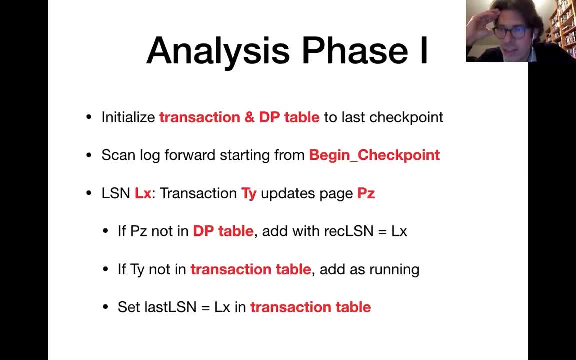 as running and if the transaction is as running and if the transaction is already in the transaction table, then already in the transaction table, then already in the transaction table, then we still need to update the last lsn. we still need to update the last lsn. we still need to update the last lsn, which always 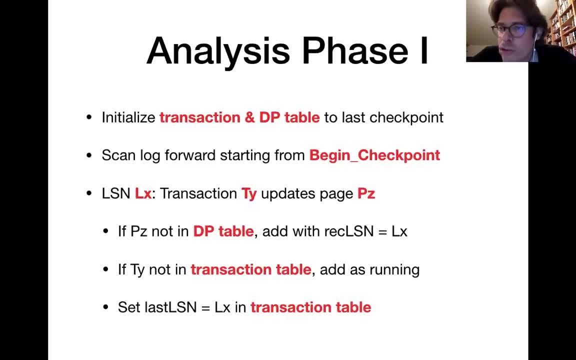 which always, which always gives the last log entry, gives the last log entry, gives the last log entry. created by a transaction, so we update. created by a transaction, so we update. created by a transaction, so we update that to the current log entry, that to the current log entry. 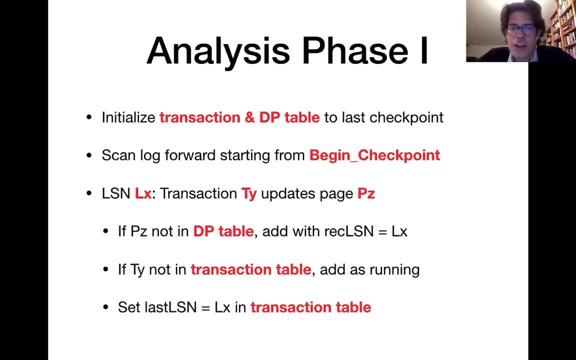 that to the current log entry and, and- and this is what we have to update if we- this is what we have to update if we, this is what we have to update if we encounter- encounter encounter one of those log entries that describe: one of those log entries that describe: 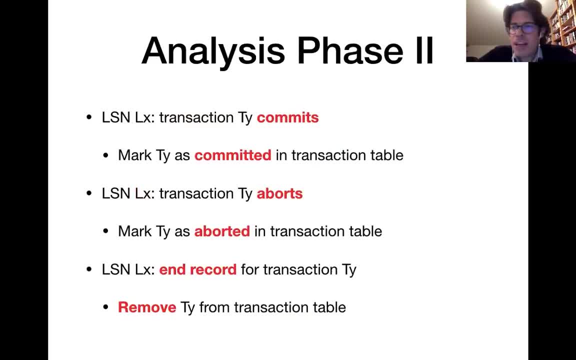 one of those log entries that describe an update, an update, an update to our data. now if a transaction to our data, now if a transaction to our data, now if a transaction commits and we see a corresponding log commits and we see a corresponding log commits and we see a corresponding log entry. 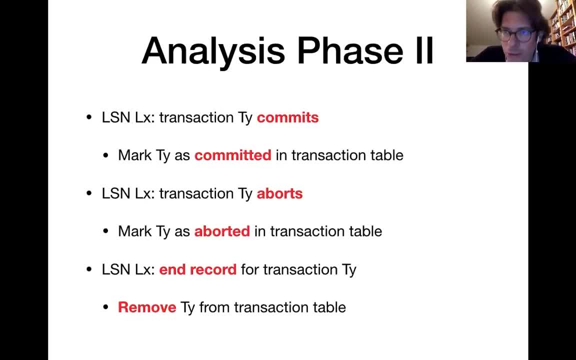 entry: entry. then we change in the transaction table. then we change in the transaction table. then we change in the transaction table the status of the transaction, the status of the transaction, the status of the transaction to committed and update the last lsn to committed and update the last lsn. 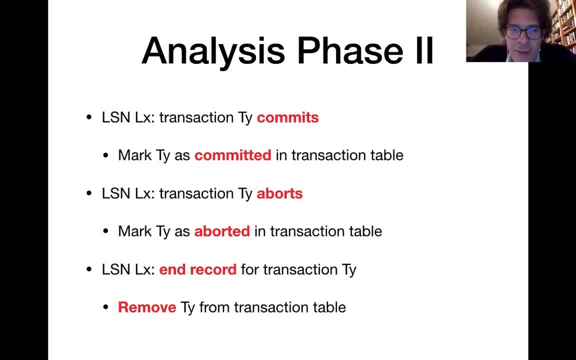 to committed and update the last lsn. if a transaction aborts, then if a transaction aborts, then if a transaction aborts, then correspondingly, we correspondingly, we correspondingly, we update the status to abort it, update the status to abort it, update the status to abort it and if we encounter an end log record. 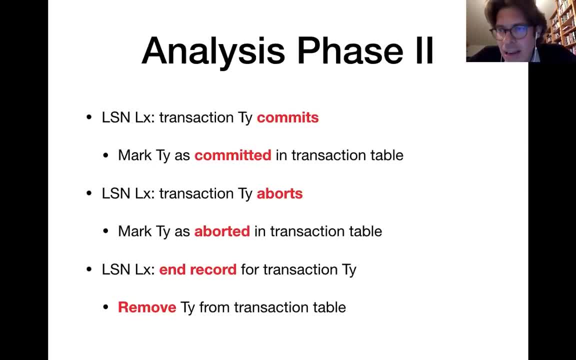 and if we encounter an end log record, and if we encounter an end log record for a transaction, for a transaction which essentially means that all the, which essentially means that all the which essentially means that all the cleanup for this transaction, cleanup for this transaction, cleanup for this transaction has been done, so we can forget about the 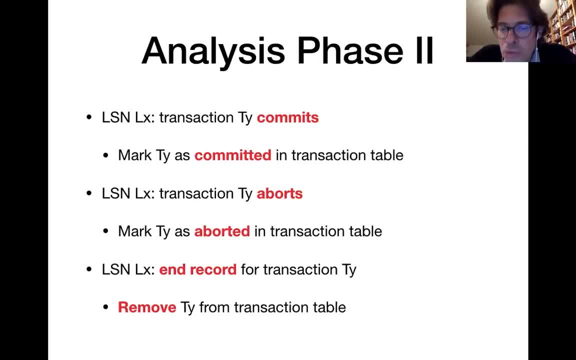 has been done, so we can forget about the has been done, so we can forget about the transaction. and this is why transaction and this is why transaction and this is why, in this case, we remove it from the. in this case, we remove it from the. in this case, we remove it from the transaction table. 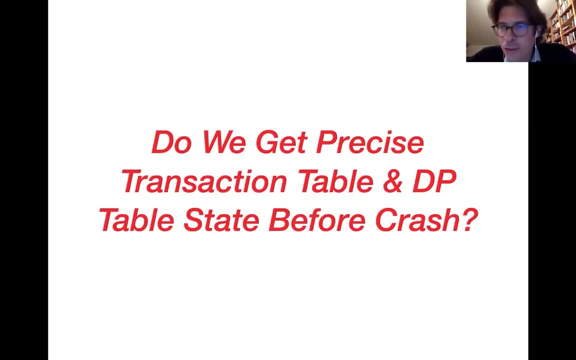 now one question to you and i give you a now one question to you and i give you a now one question to you and i give you a couple of seconds to think about it. couple of seconds to think about it. couple of seconds to think about it is whether we get a precise 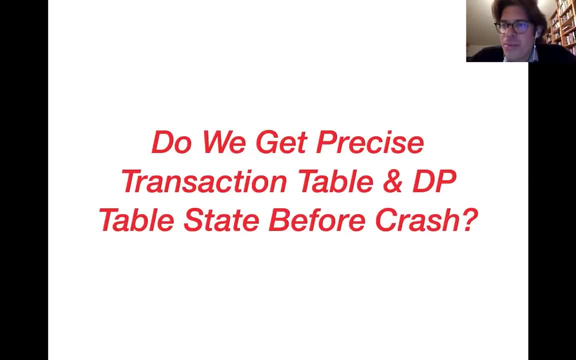 is whether we get a precise, is whether we get a precise transaction table and dirty page table transaction table and dirty page table, transaction table and dirty page table. that we had. that we had. that we had directly before the system crash after the. directly before the system crash after the. 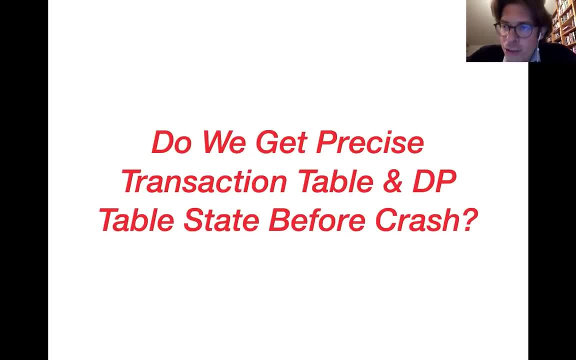 directly before the system crash. after the analysis phase. so basically, analysis phase, so basically analysis phase. so basically, will we always be successful in, will we always be successful in, will we always be successful in restoring the transaction table and restoring the transaction table and restoring the transaction table and dirty page table, precisely. 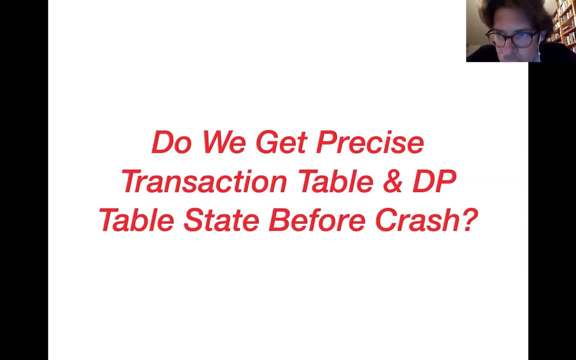 dirty page table, precisely dirty page table, precisely to their state, immediately before the, to their state immediately before the, to their state, immediately before the system crash. system crash, system crash because of the analysis phase, because of the analysis phase, because of the analysis phase. in the end, here we restore the. 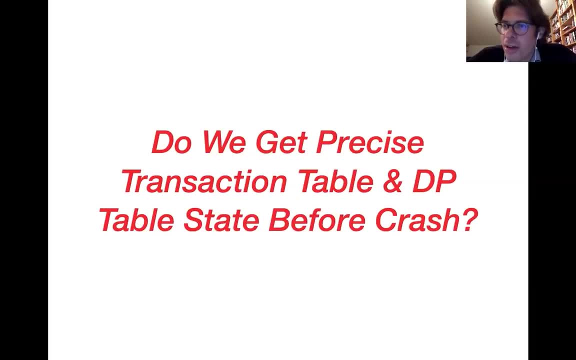 in the end, here we restore the. in the end, here we restore the transaction table and dirty page table. transaction table and dirty page table. transaction table and dirty page table based on log entries. based on log entries. based on log entries. and now, if you think about, and now if you think about, 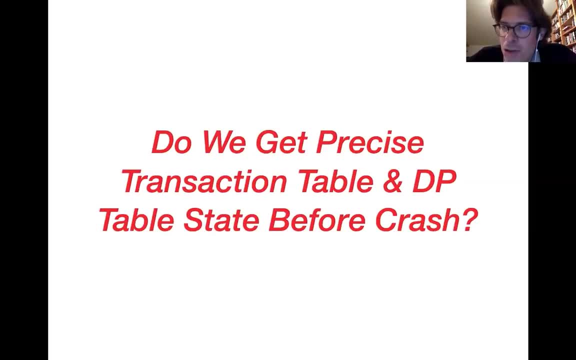 and now, if you think about the way that log entries have to make, the way that log entries have to make, the way that log entries have to make until they become persistent on hard, until they become persistent on hard, until they become persistent on hard disk disk, so the right answer here is that in some 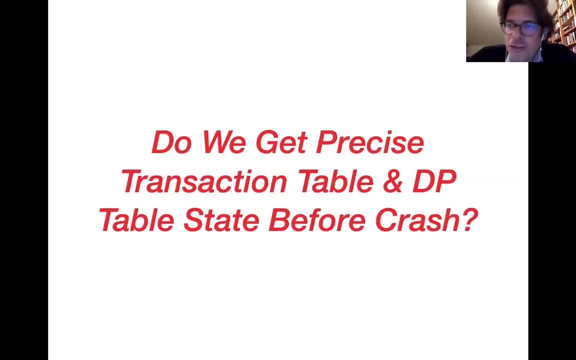 so the right answer here is that in some. so the right answer here is that in some cases we might not be able to restore the cases. we might not be able to restore the cases. we might not be able to restore the transaction table and dirty page table. 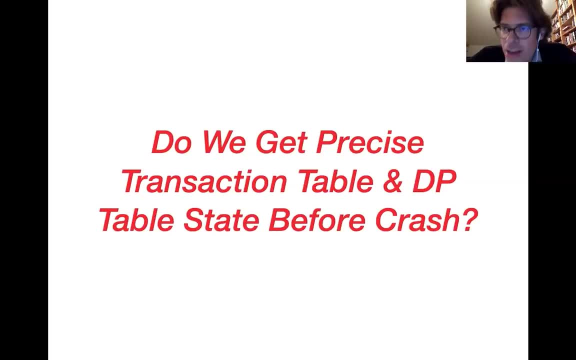 transaction table and dirty page table: transaction table and dirty page table: exactly into the state they were in, exactly into the state they were in, exactly into the state they were in before the system crash. because a log before the system crash, because a log before the system crash, because a log entries are first of all written into. 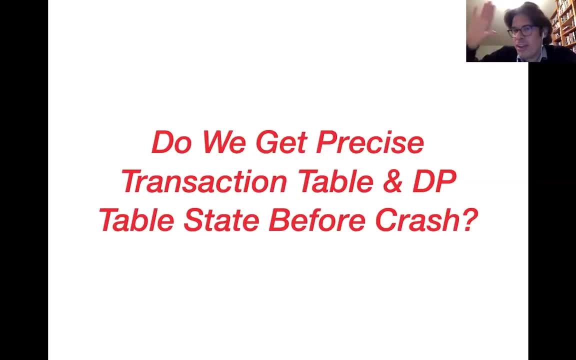 entries are first of all written into. entries are first of all written into the log tail in a main memory, which the log tail in a main memory, which the log tail in a main memory, which means that it will vanish if there is a means that it will vanish if there is a 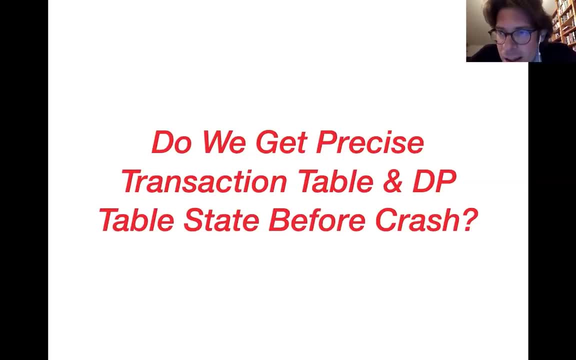 means that it will vanish if there is a system crash, and only every once in a system crash, and only every once in a system crash and only every once in a while we write the lock tail entries to. while we write the lock tail entries to. while we write the lock tail entries to hard disk, where they become persistent. 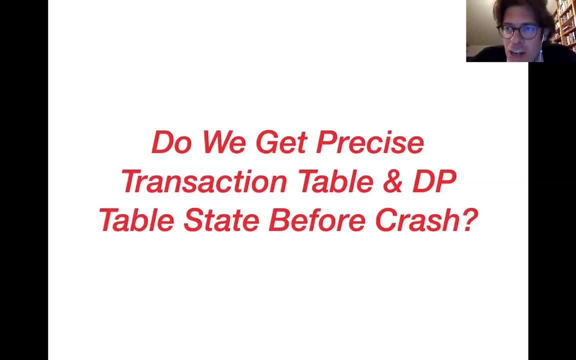 hard disk where they become persistent, hard disk where they become persistent. so the last few lock entries directly, so the last few lock entries directly, so the last few lock entries directly before the crash might get lost, which before the crash might get lost, which before the crash might get lost, which means that we might have a slightly 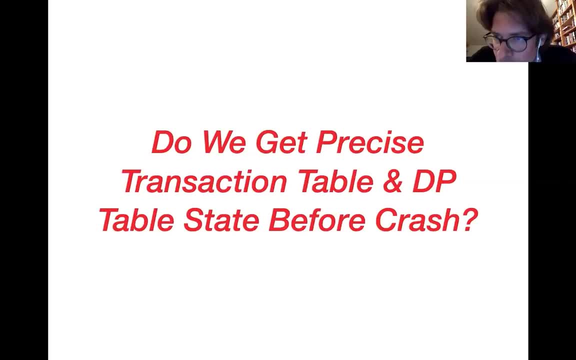 means that we might have a slightly means that we might have a slightly earlier state of the transaction and earlier state of the transaction and earlier state of the transaction and dirty page table. but a nice thing about dirty page table. but a nice thing about dirty page table. but a nice thing about this is that we can be sure that those 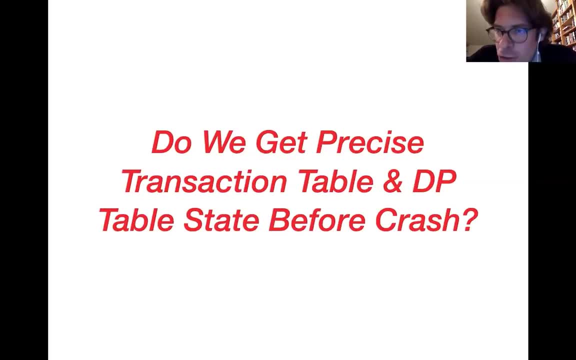 this is that we can be sure that those. this is that we can be sure that those lock entries that we lost. they don't lock entries that we lost. they don't lock entries that we lost. they don't refer to any transactions that have. refer to any transactions that have. 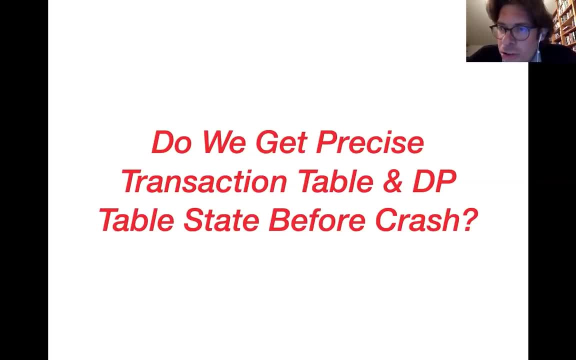 refer to any transactions that have already committed, for instance, because already committed. for instance, because already committed. for instance, because, due to the rules of right-ahead blocking, due to the rules of right-ahead blocking, due to the rules of right-ahead blocking that the areas algorithm is following. 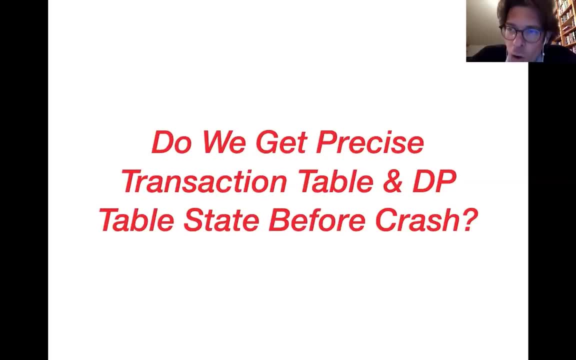 that the areas algorithm is following. that the areas algorithm is following. if a transaction commits, then we have to. if a transaction commits, then we have to. if a transaction commits, then we have to make all its lock entries persistent on. make all its lock entries persistent on. make all its lock entries persistent on hard disk. so in the following we're: 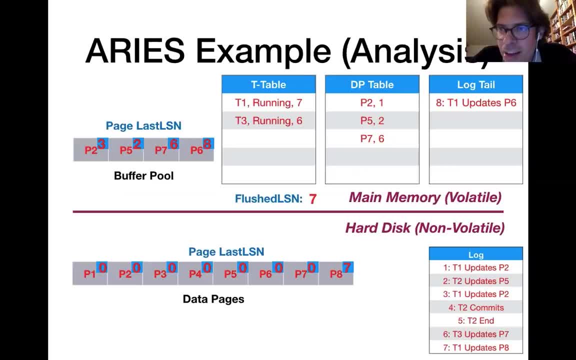 hard disk. so in the following we're hard disk. so in the following we're gonna make a little example about the, gonna make a little example about the, gonna make a little example about the analysis days. we continue with the analysis days. we continue with the analysis days. we continue with the example that we had before. and, by the way, 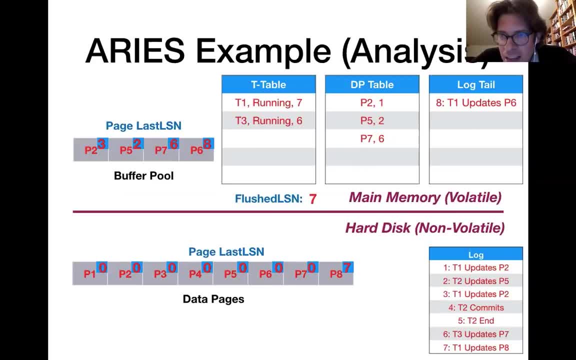 example that we had before and, by the way, example that we had before, and, by the way, here in this graphic, you also see here in this graphic, you also see here in this graphic, you also see again the a lock tail buffer on the right, again the a lock tail buffer on the right. 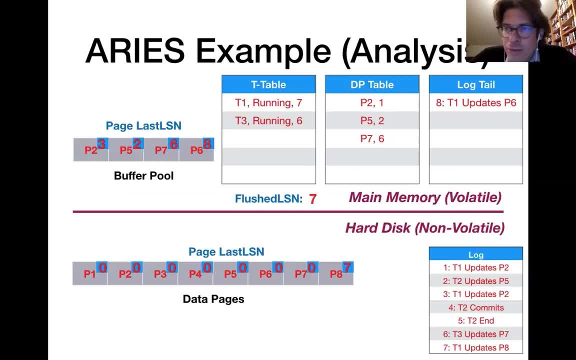 again the a lock tail buffer on the right upper corner, which is in main memory, upper corner, which is in main memory, upper corner, which is in main memory, which is volatile, and on the bottom you, which is volatile, and on the bottom you, which is volatile, and on the bottom you see the persistent part of the log which: 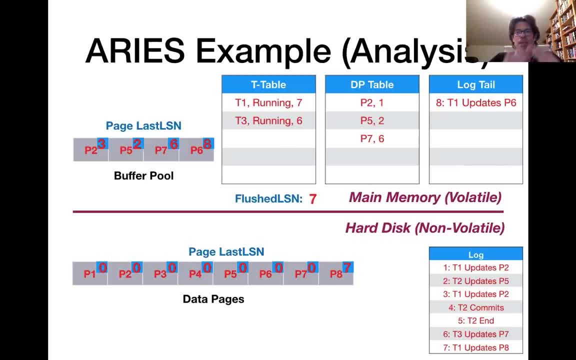 see the persistent part of the log which. see the persistent part of the log which is stored on hard disk. so let's assume is stored on hard disk. so let's assume is stored on hard disk. so let's assume that we have a crash in our system. for 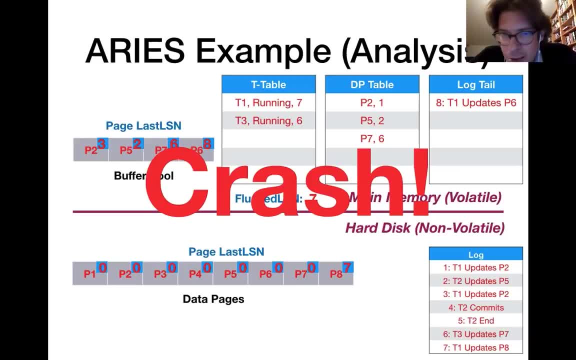 that we have a crash in our system for that we have a crash in our system. for instance, suddenly the power supply fails, instance, suddenly the power supply fails, instance, suddenly the power supply fails and the server is shut down because we, and the server is shut down because we. 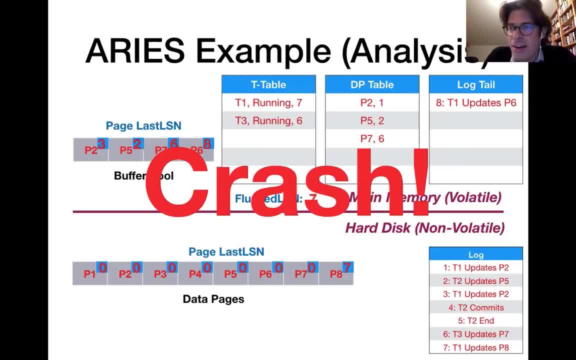 and the server is shut down because we don't have a power anymore. in that case, don't have a power anymore. in that case, don't have a power anymore. in that case, once the system comes back online, after once the system comes back online, after once the system comes back online after the crash, everything we have in main. 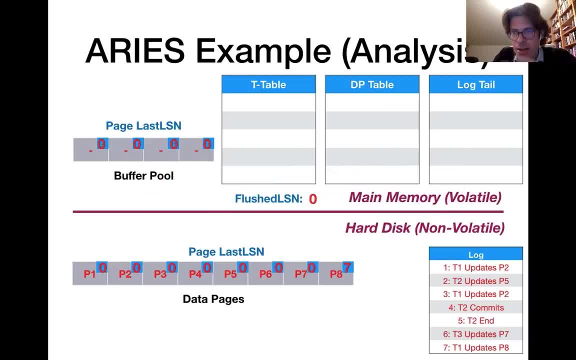 the crash everything we have in main, the crash, everything we have in main, erased of course here now. we don't have erased, of course here now. we don't have erased, of course here now. we don't have anything in our buffer pool and we don't anything in our buffer pool and we don't. 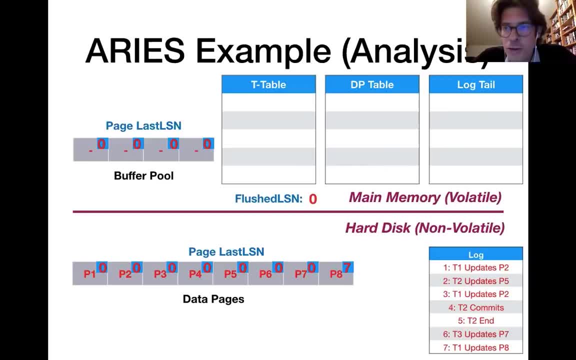 anything in our buffer pool and we don't have anything in the remaining data. have anything in the remaining data, have anything in the remaining data structures? so at this point, perhaps I'm structures, so at this point, perhaps I'm structures, so at this point, perhaps I'm quickly gonna remind you of the. 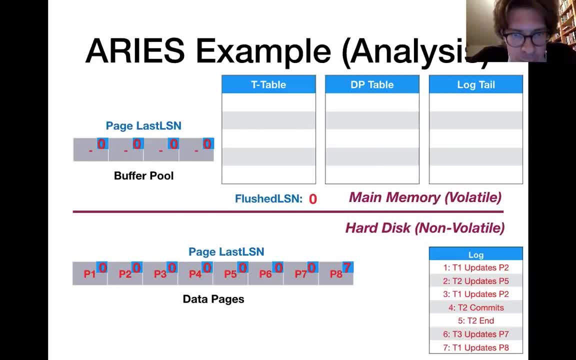 quickly gonna remind you of the quickly gonna remind you of the semantics of those different data semantics of those different data semantics of those different data structures that you see here, first of all, structures that you see here, first of all, structures that you see here, first of all, we have data structures that are not 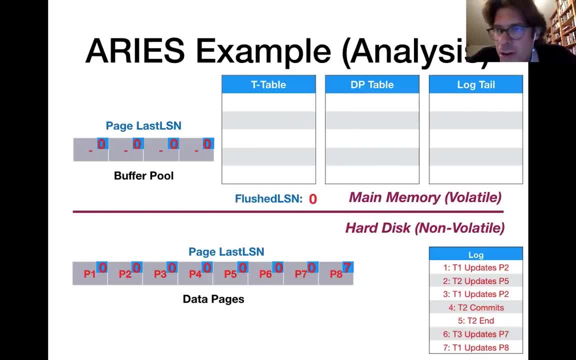 we have data structures that are not. we have data structures that are not specific to the areas algorithm but specific to the areas algorithm, but specific to the areas algorithm, but relates to a things that you've seen, relates to a things that you've seen, relates to a things that you've seen before in the course on hard disk of 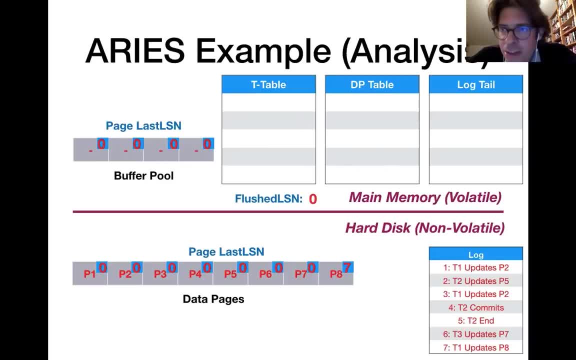 before, in the course on hard disk of before. in the course on hard disk, of course we have stored our actual data. at course we have stored our actual data. at course we have stored our actual data at the granularity of pages, and then in the granularity of pages, and then in. 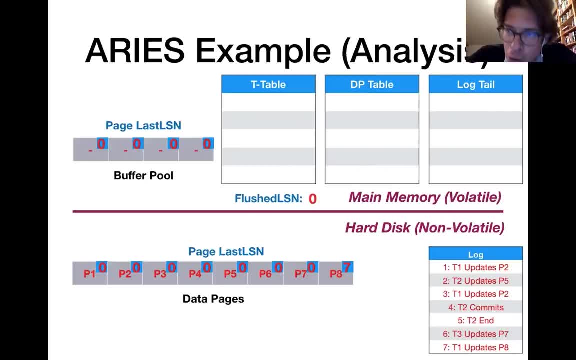 the granularity of pages, and then in main memory, you always have the buffer main memory. you always have the buffer main memory. you always have the buffer pool, which is the portion of main memory pool, which is the portion of main memory pool, which is the portion of main memory reserved for the database assistant and 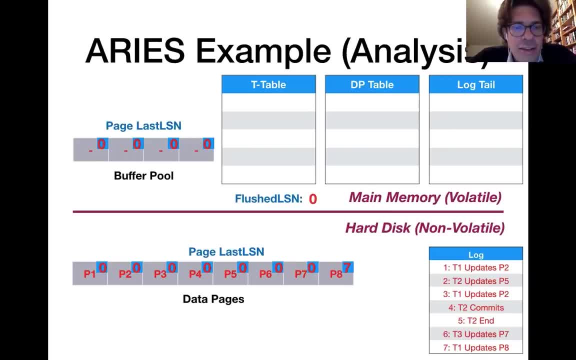 reserved for the database assistant and reserved for the database assistant, and also it is divided into slots, where also it is divided into slots, where also it is divided into slots where each of those slots can store one of the. each of those slots can store one of the. 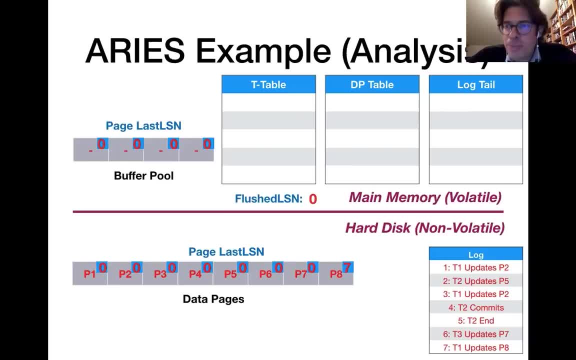 each of those slots can store one of the pages. now a first of all specific to pages. now a first of all specific to pages. now a first of all specific to the areas algorithm, the associate those, the areas algorithm, the associate those, the areas algorithm, the associate those, the pages on hard disk and in main. 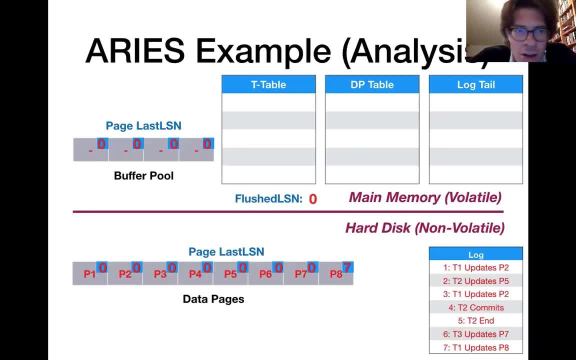 the pages on hard disk and in main the pages on hard disk and in main memory, with this page last and as n or memory with this page last, and as n or memory with this page last, and as n or simply page and as n, which essentially simply page, and as n, which essentially. 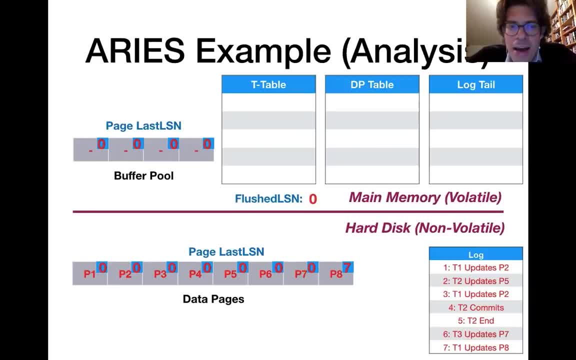 simply page and as n, which essentially gives you the last log sequence number, gives you the last log sequence number, gives you the last log sequence number that has changed the page. so the log that has changed the page, so the log that has changed the page. so the log entries are always associated with the 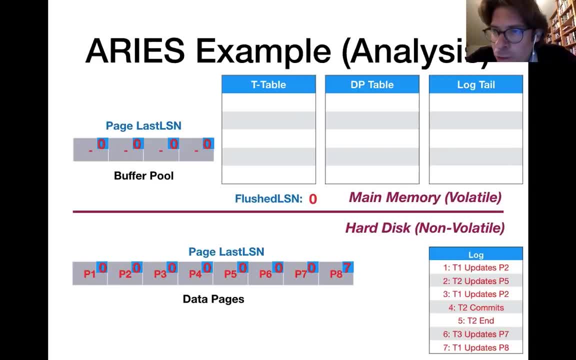 entries are always associated with. the entries are always associated with the log sequence number. it's an ID of the log sequence number. it's an ID of the log sequence number. it's an ID of the log entry. if you imagine the log as a log entry, if you imagine the log as a. 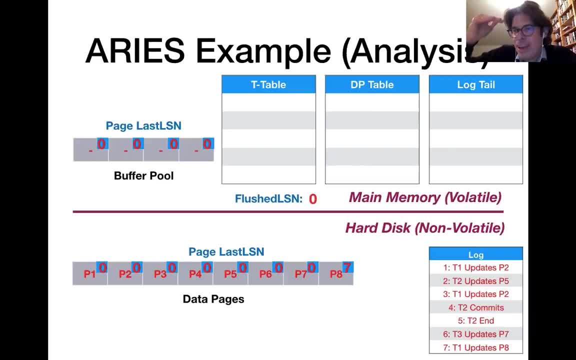 log entry. if you imagine the log as a text file, you can think of the log text file. you can think of the log text file. you can think of the log sequence number simply as the line sequence number, simply as the line sequence number, simply as the line number. and here for the in-memory. 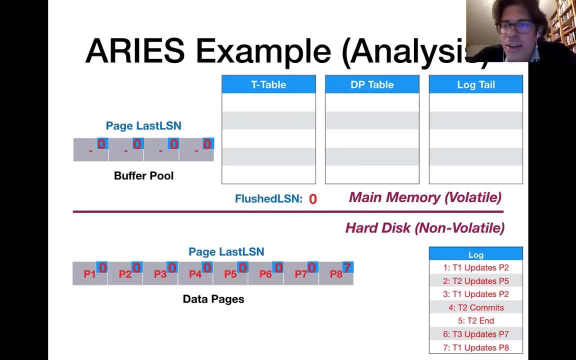 number and here for the in-memory number, and here for the in-memory version and for the hard disk version version and for the hard disk version version and for the hard disk version. we have the log sequence number that has. we have the log sequence number that has. 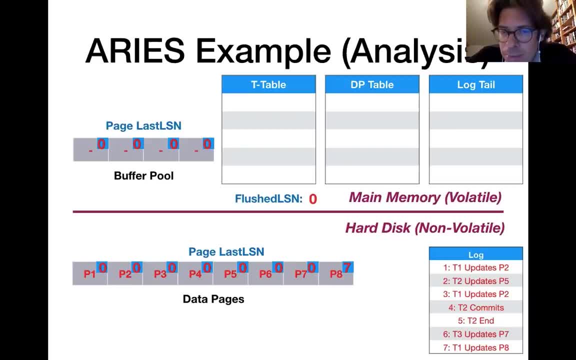 we have the log sequence number that has last changed the corresponding page, then last changed the corresponding page, then last changed the corresponding page. then we have the transaction table, which we have the transaction table which we have the transaction table which keeps track of the status of different. 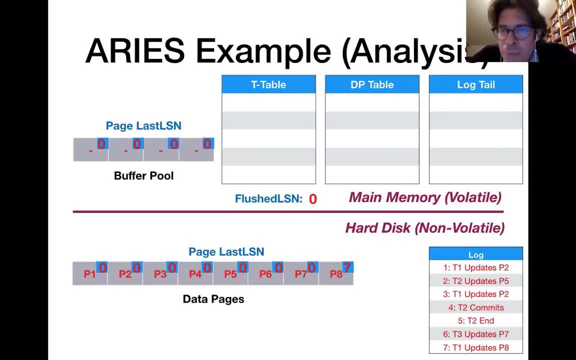 keeps track of the status of different. keeps track of the status of different transactions. we have the dirty page transactions. we have the dirty page transactions. we have the dirty page table which keeps track of pages where? table which keeps track of pages where? table which keeps track of pages where the in-memory version in the buffer pool. 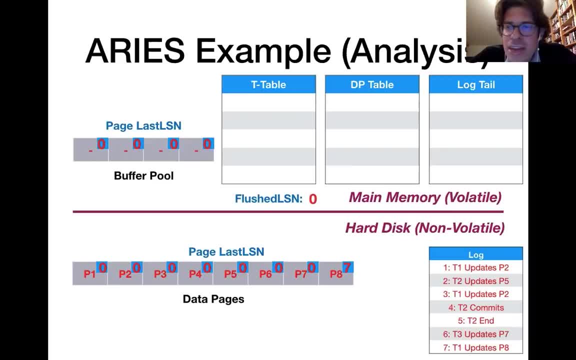 the in-memory version in the buffer pool. the in-memory version in the buffer pool on the left-hand side on top. deviates on the left-hand side on top. deviates on the left-hand side on top. deviates from the corresponding page on hearts. from the corresponding page on hearts. 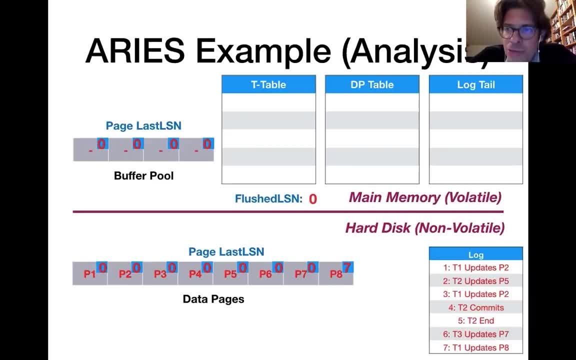 from the corresponding page on hearts disk on the bottom and keeps track of disk on the bottom and keeps track of disk on the bottom and keeps track of the log entry at which that happened. we the log entry at which that happened. we the log entry at which that happened. we have the lock tail buffer in main. have the lock tail buffer in main. have the lock tail buffer in main memory which stores the last few log memory. which stores the last few log memory. which stores the last few log entries that have made it too hard this entries that have made it too hard this. 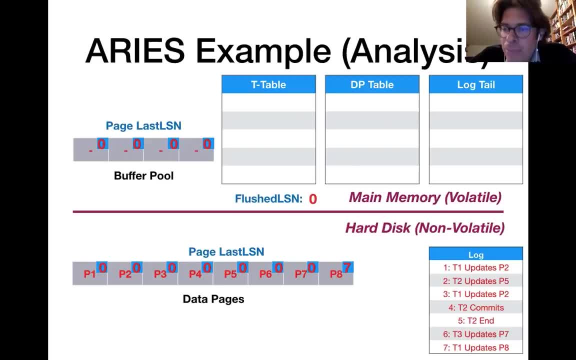 entries that have made it too hard. this get and we're the flushed Ellis and get and we're the flushed Ellis and get and we're the flushed Ellis. and which stores up to which log entry I which stores up to which log entry I which stores up to which log entry? I have already written them to hard disk. 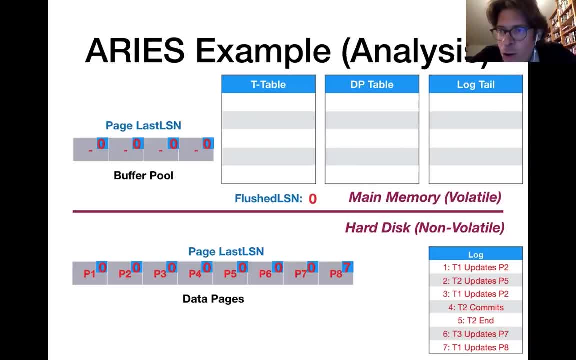 have already written them to hard disk, have already written them to hard disk and finally, here on hard disk, you have. and finally, here on hard disk, you have. and finally, here on hard disk, you have, the lock portion that has already made, the lock portion that has already made. 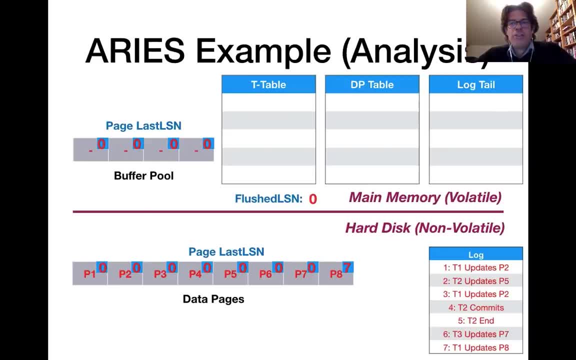 the lock portion that has already made it to persistent storage. so now we had it to persistent storage. so now we had it to persistent storage. so now we had to crash. we have to recover the to crash. we have to recover the to crash. we have to recover the transaction table and the dirty page. 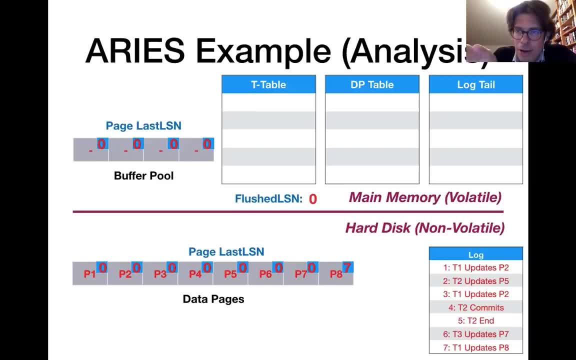 transaction table and the dirty page transaction table. and the dirty page table based on the entries that we find table. based on the entries that we find table. based on the entries that we find in the log on hard disk. so here in the log on hard disk. so here: 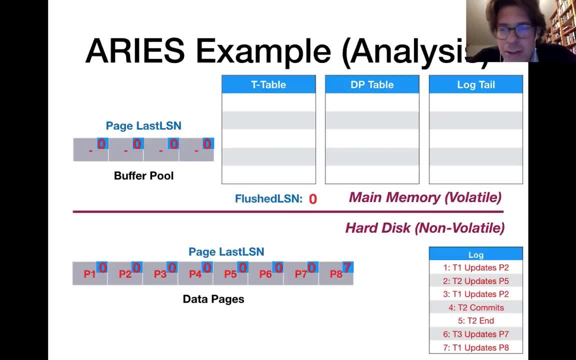 in the log on hard disk. so here, currently we don't have a checkpoint yet. currently we don't have a checkpoint yet. currently we don't have a checkpoint yet. so we simply start from the beginning of. so we simply start from the beginning of so we simply start from the beginning of the lock, starting with lock sequence. 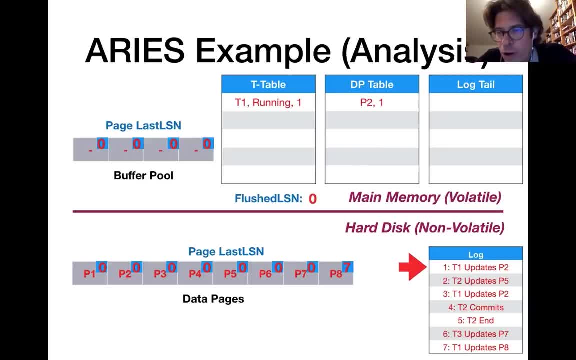 the lock starting with lock sequence: the lock starting with lock sequence number one. so here a transaction t1 number one. so here a transaction t1 number one. so here a transaction t1. updates a page p2. so first of all we updates a page p2. so first of all we 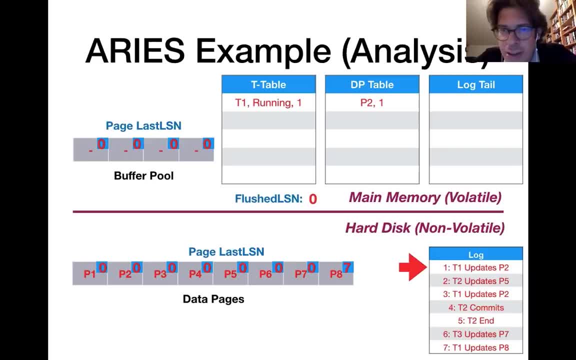 updates a page p2. so first of all, we have to insert a transaction into the, have to insert a transaction into the, have to insert a transaction into the transaction table. we mark it as running transaction table. we mark it as running transaction table. we mark it as running and the last L is n, which indicates the. 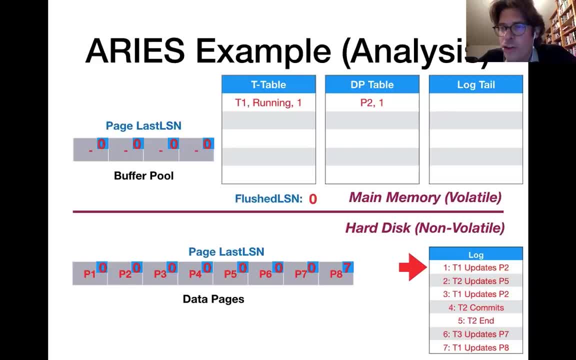 and the last L is n, which indicates the, and the last L is n, which indicates the last lock entry of that transaction. that last lock entry of that transaction, that last lock entry of that transaction that is currently set to one, so in the is currently set to one, so in the. 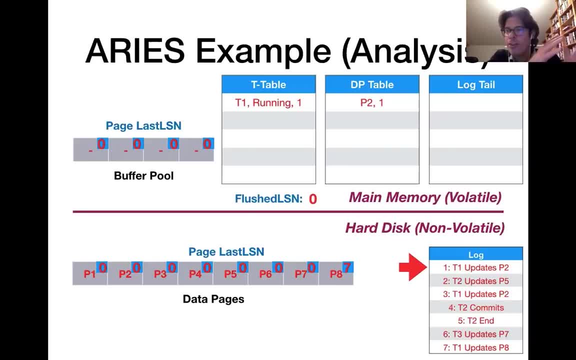 is currently set to one. so in the syntax that you see in the log, you always have syntax that you see in the log. you always have syntax that you see in the log. you always have the lock sequence number, then the lock sequence number, then the lock sequence number, then followed by the high level information about the. 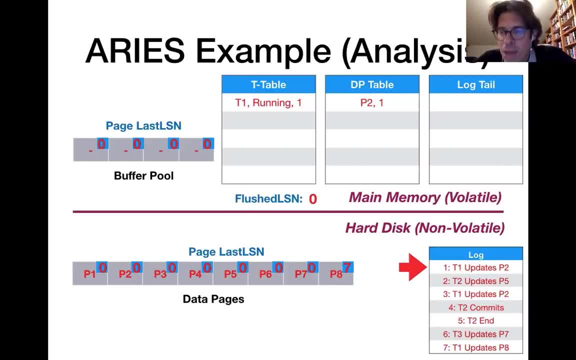 followed by the high level information about the, followed by the high level information about the lock entry. so here, t1 updates lock entry. so here, t1 updates lock entry. so here t1 updates the page a- p2 by changing something on the page a- p2 by changing something on. 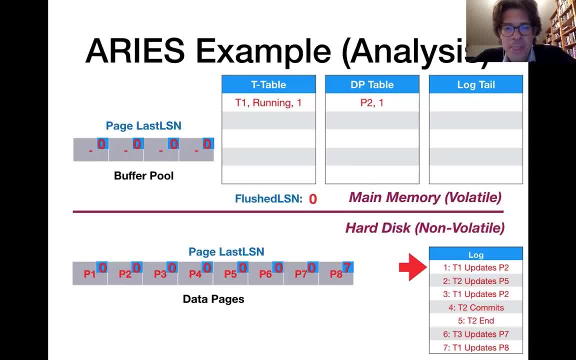 the page a p2 by changing something on that page and because of that, the page that page and because of that, the page that page and because of that the page now deviates from the main memory now deviates from the main memory now deviates from the main memory version of the page, deviates from the 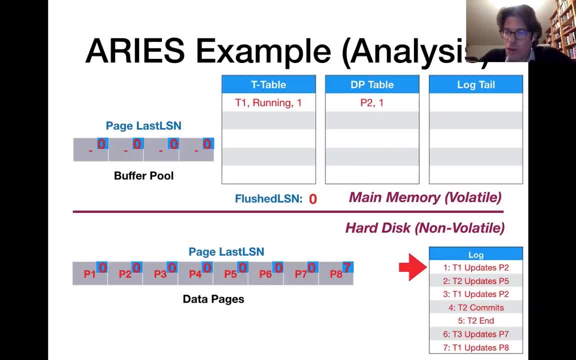 version of the page deviates from the version of the page, deviates from the hard disk version of the page and the hard disk version of the page and the hard disk version of the page and the earliest lock entry that has caused that earliest lock entry. that has caused that. 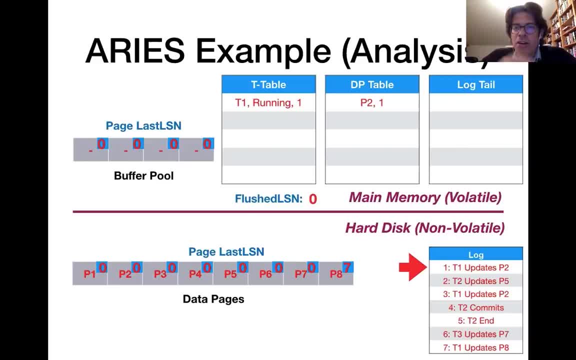 earliest lock entry that has caused. that is the current one number one. so we is the current one number one. so we is the current one number one. so we insert into the dirty page table page. insert into the dirty page table page. insert into the dirty page table page two with rec Alice and set to one now. 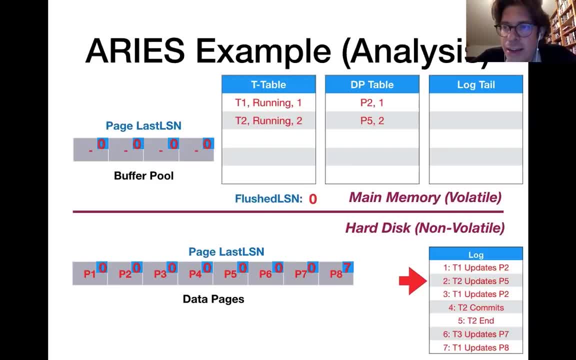 two with rec Alice and set to one. now. two with rec Alice and set to one. now. we continue here. we find a lock entry. we continue here. we find a lock entry. we continue here. we find a lock entry stating that transaction 2 has updated. stating that transaction 2 has updated. 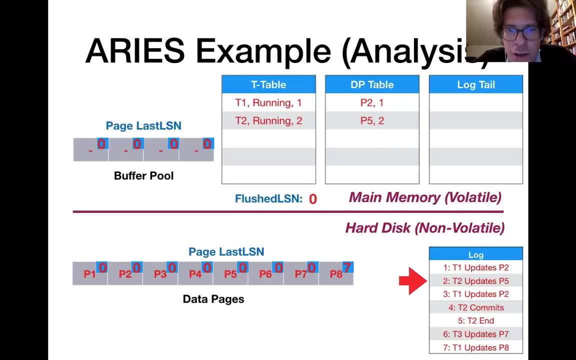 stating that transaction 2 has updated page 5, and that is a lock sequence, page 5, and that is a lock sequence, page 5, and that is a lock sequence, number 2. so we insert a transaction into number 2. so we insert a transaction into. 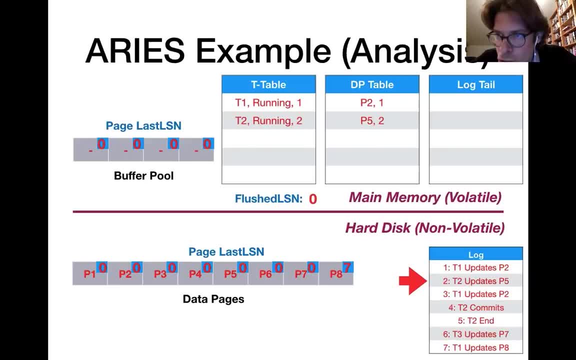 number 2, so we insert a transaction into the transaction table with last at us, the transaction table with last at us, the transaction table with last at us, and set to 2 and marked as running and in. and set to 2 and marked as running and in. 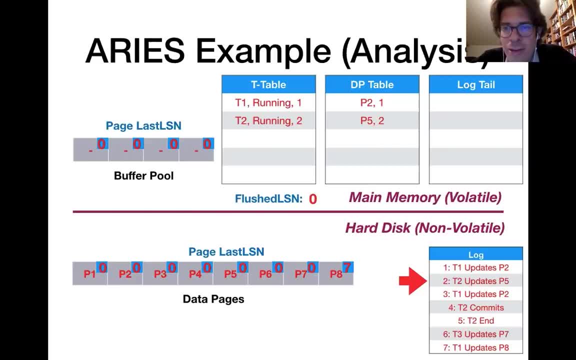 and set to 2 and marked as running. and in the dirty page table we insert page the dirty page table. we insert page the dirty page table. we insert page number 5 with the rack at us and set to number 5 with the rack at us and set to. 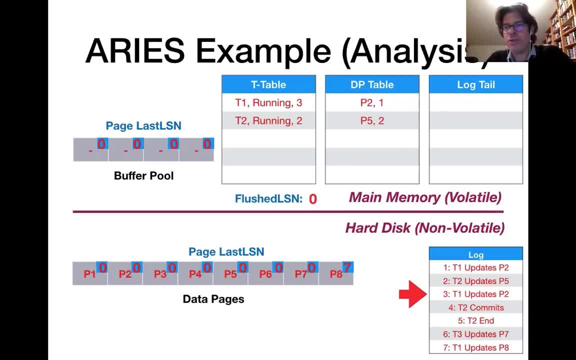 number 5 with the rack at us and set to 2. now transaction 1 decides again to 2. now transaction 1 decides again to 2. now transaction 1 decides again to all the update that transaction table, all the update that transaction table, all the update that transaction table and set the last at us and for. 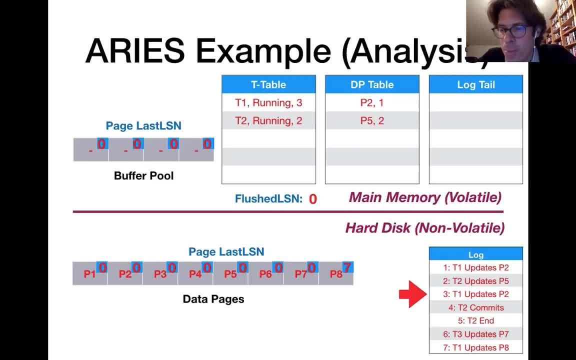 and set the last at us and for: and set the last at us and for: transaction 1, 2, 3, the current the lock transaction 1, 2, 3, the current the lock transaction 1, 2, 3, the current the lock sequence number. now, this is often a. 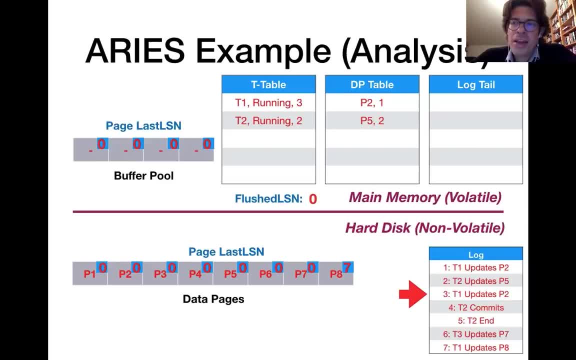 sequence number. now, this is often a sequence number. now. this is often a source of confusion. my experience don't source of confusion. my experience don't source of confusion, my experience: don't. update the dirty page table if you have. update the dirty page table if you have. 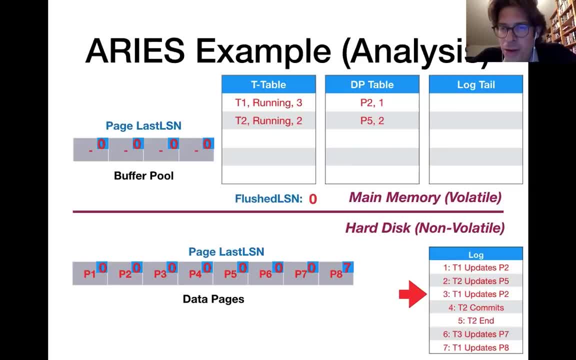 update the dirty page table if you have another update on the same page or the another update on the same page or the another update on the same page, or the dirty page table only stores the rack dirty page table only stores the rack dirty page table. only stores the rack LSN, which is the earliest log entry that 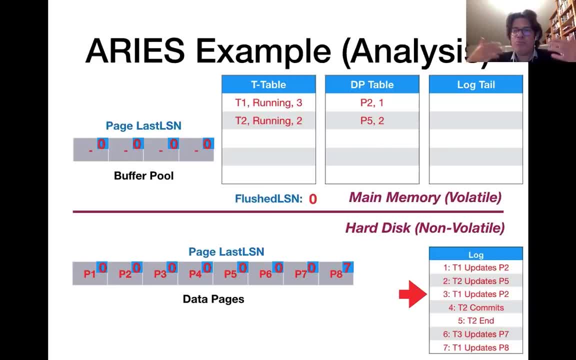 LSN, which is the earliest log entry, that LSN, which is the earliest log entry, that made the page dirty. so if we have made the page dirty, so if we have made the page dirty, so if we have repeated changes to the same page which repeated changes to the same page which 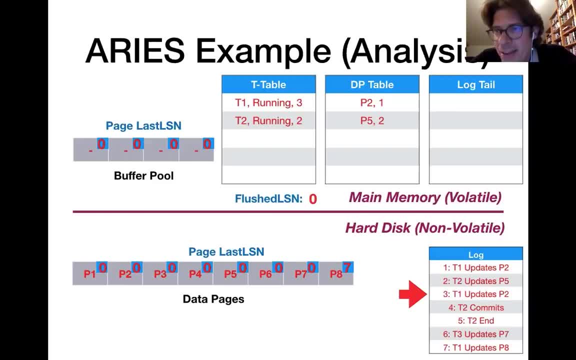 repeated changes to the same page. which is already dirty, then we don't need to. is already dirty, then we don't need to. is already dirty, then we don't need to change anything in the dirty page table. change anything in the dirty page table. change anything in the dirty page table. so we leave that one. the rack LSN of. 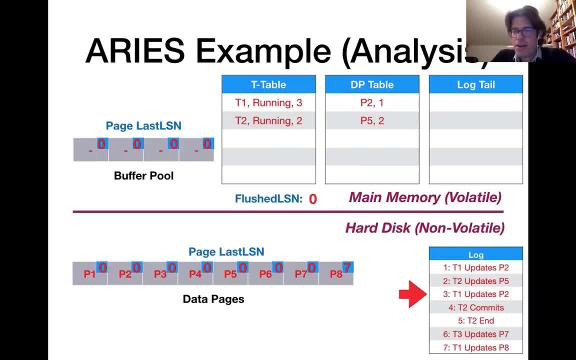 so we leave that one. the rack LSN of, so we leave that one. the rack LSN of page two sets to one, now here. page two sets to one, now here. page two sets to one, now here. transaction number to commit, so we set. transaction number to commit, so we set. 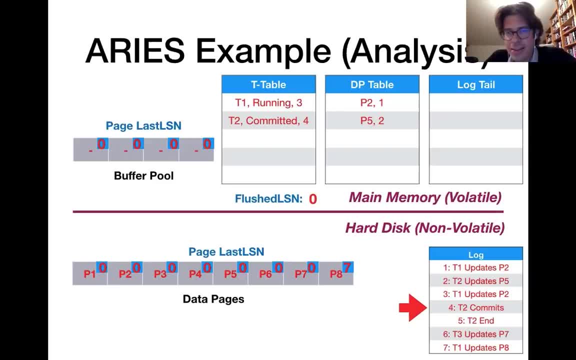 transaction number to commit. so we set the status to committed and update the, the status to committed and update the, the status to committed and update the last LSN, and now it even ends. which last LSN, and now it even ends which last LSN, and now it even ends, which means that we remove transaction two. 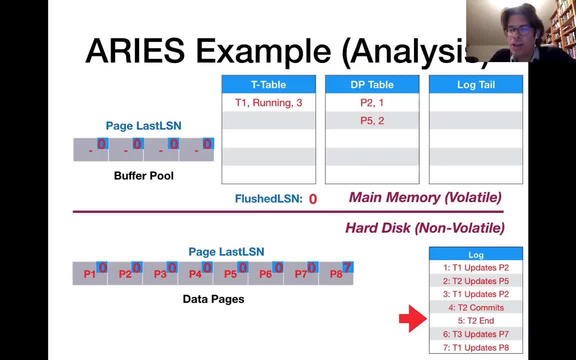 means that we remove transaction two means that we remove transaction two from the transaction table here now. we from the transaction table here now. we from the transaction table here. now we encounter a new transaction transactions, encounter a new transaction transactions, encounter a new transaction transactions, we, so we insert that into the. 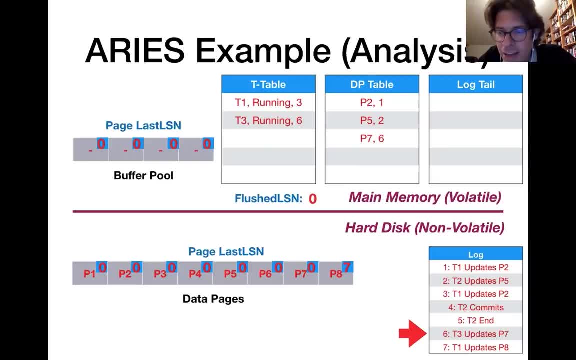 we so we insert that into the we so we insert that into the transaction table with a last LSN set transaction table with a last LSN set transaction table with a last LSN set to six. and it updates page number seven to six and it updates page number seven. 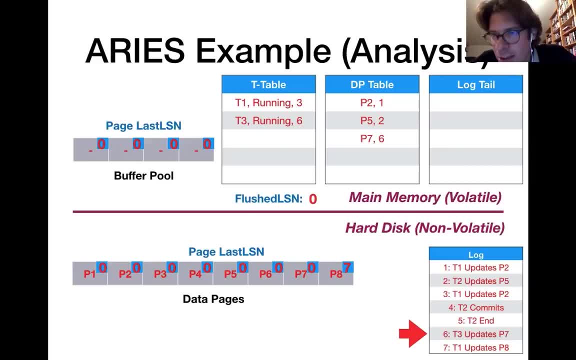 to six and it updates page number seven. so we insert page number seven with rec. so we insert page number seven with rec. so we insert page number seven with rec. LSN six into the dirty page table. LSN six into the dirty page table. LSN six into the dirty page table. finally, transaction one updates page. 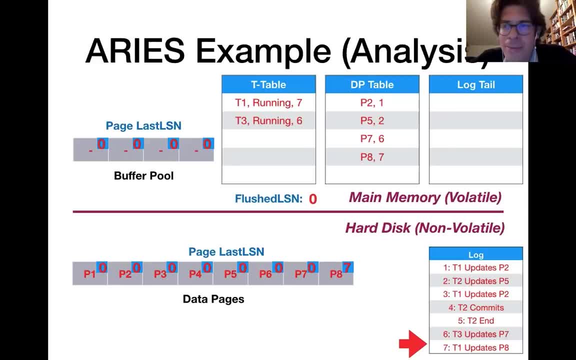 finally, transaction one updates page. finally, transaction one updates page eight as well. so here transaction one: we eight as well. so here transaction one, we eight as well. so here transaction one. we update the last that is in in the update, the last that is in in the update, the last that is in in the transaction table, and here we insert. 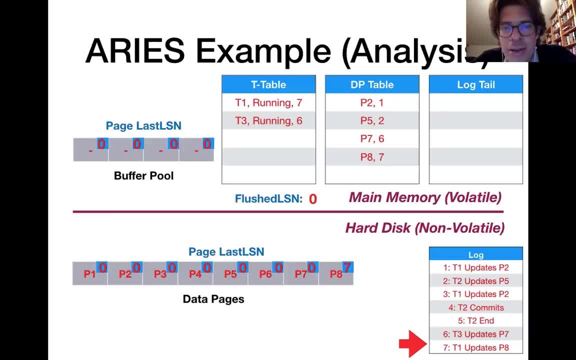 transaction table. and here we insert transaction table. and here we insert page number eight with rec errors and page number eight with rec errors and page number eight with rec errors and seven into the dirty page table. seven into the dirty page table, seven into the dirty page table. all right, so this is. 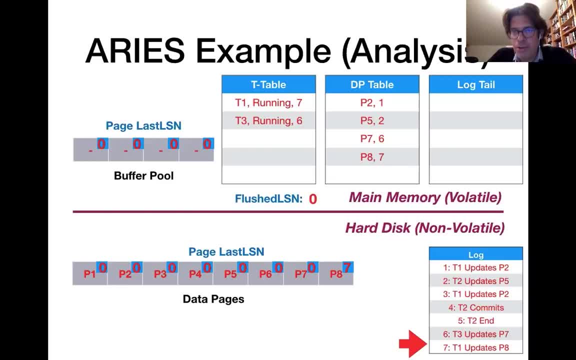 all right. so this is all right. so this is the analysis face in the simple example, the analysis face in the simple example, the analysis face in the simple example. we have restored the transaction table. we have restored the transaction table. we have restored the transaction table and dirty page table using the log. 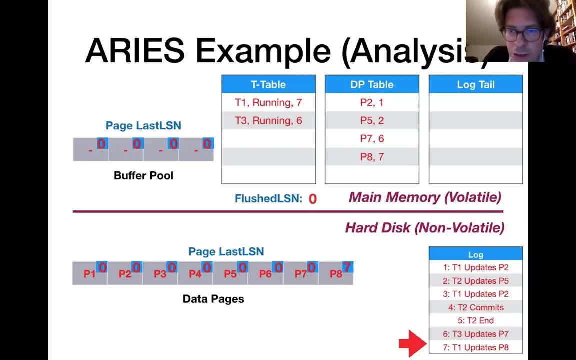 and dirty page table. using the log and dirty page table. using the log entries that we still find on hard disk. entries that we still find on hard disk. entries that we still find on hard disk after the crash. the next is the redo. after the crash: the next is the redo. after the crash. the next is the redo phase, and the redo phase needs to start phase and the redo phase needs to start phase and the redo phase needs to start from the earliest point at which changes, from the earliest point at which changes, from the earliest point at which changes occurred where that may not have made it. 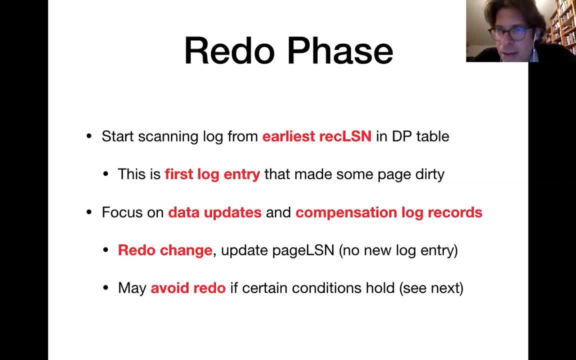 occurred where that may not have made it occurred where that may not have made it to hard disk. yet. in order to hard disk, yet, in order to hard disk, yet. in order to find that point, we analyze the dirty to find that point. we analyze the dirty to find that point. we analyze the dirty page table which contains, for each page. 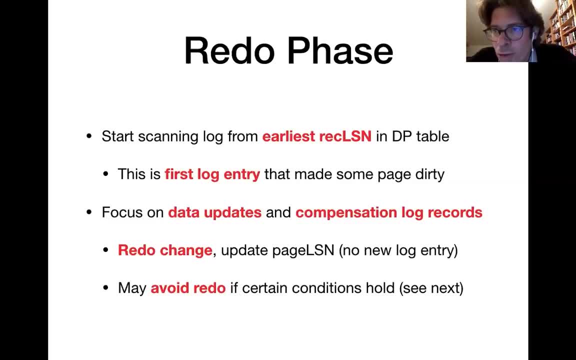 page table which contains, for each page page table which contains, for each page, the earliest stock entry that made it the earliest stock entry. that made it the earliest stock entry that made it dirty. so if we take the minimum over all dirty, so if we take the minimum over all, 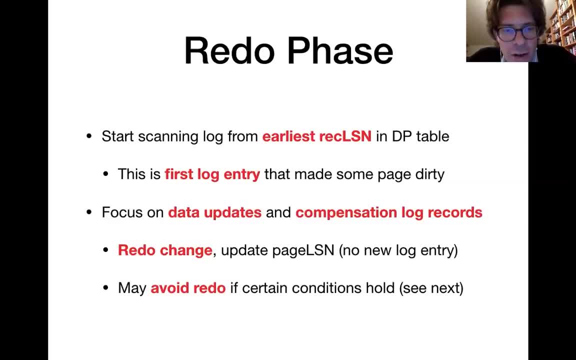 dirty. so if we take the minimum over all dirty pages, then we have the starting dirty pages, then we have the starting dirty pages, then we have the starting point for the redo phase and during the point for the redo phase. and during the point for the redo phase and during the redo phase, we focus on data updates and 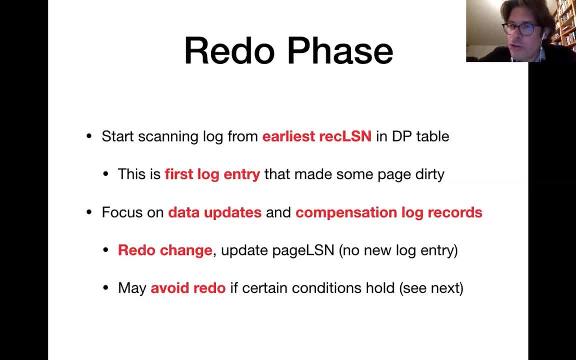 redo phase we focus on data updates. and redo phase we focus on data updates and compensation log records, which also compensation log records, which also compensation log records, which also correspond to data updates, but it is a correspond to data updates. but it is a correspond to data updates, but it is a specific type of update, because here 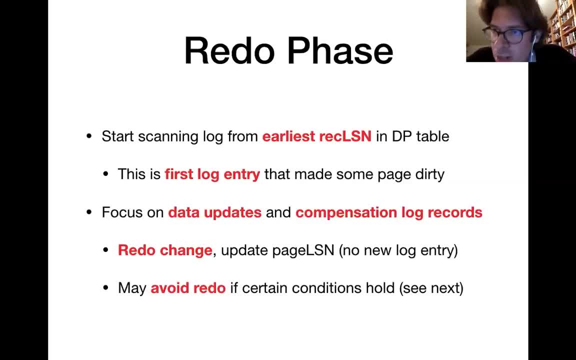 specific type of update. because here specific type of update? because here we're talking about updates that revert a. we're talking about updates that revert a. we're talking about updates that revert a previous update because the previous update, because the previous update, because the corresponding transaction has aborted. so 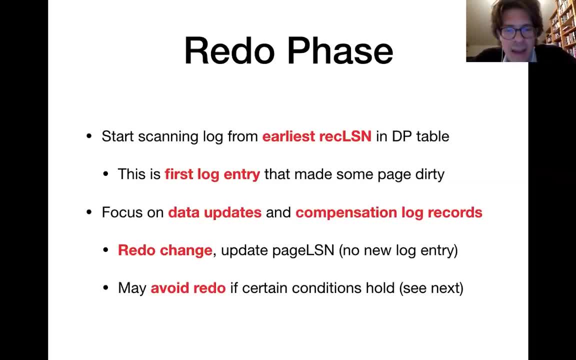 corresponding transaction has aborted. so corresponding transaction has aborted. so both are interesting for the redo phase, both are interesting for the redo phase, both are interesting for the redo phase and if you encounter one of those, and if you encounter one of those, and if you encounter one of those entries, then typically we have to, we do. 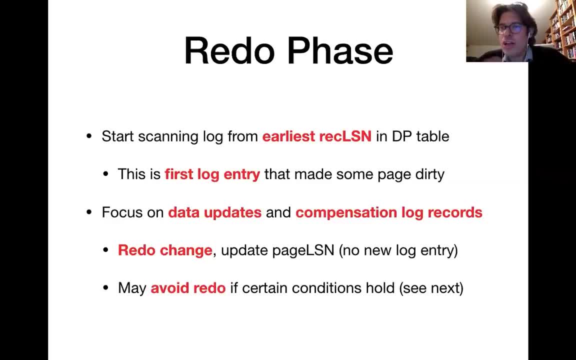 entries, then typically we have to we do entries, then typically we have to we do it, which means that we we do the course it, which means that we we do the course it, which means that we we do the course, whether we load the corresponding page, whether we load the corresponding page. 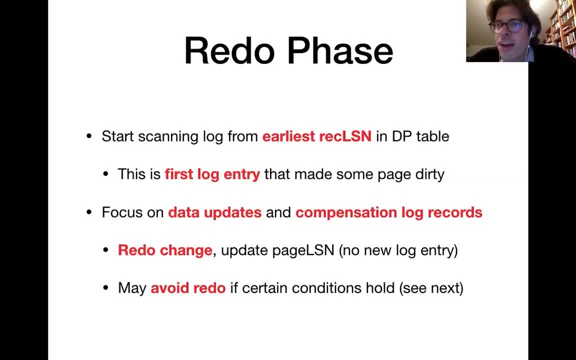 whether we load the corresponding page into main memory. we execute the change into main memory. we execute the change into main memory. we execute the change and we update the corresponding page and we update the corresponding page and we update the corresponding page. Edison of that in memory, a page there is. 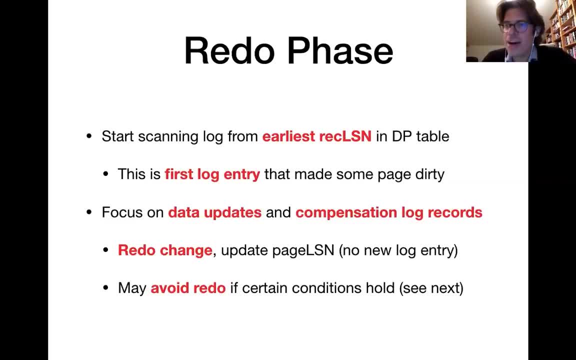 Edison of that in memory a page. there is Edison of that in memory a page. there is certain conditions and of which we can certain conditions and of which we can certain conditions and of which we can avoid redoing an operation, which of avoid redoing an operation, which of 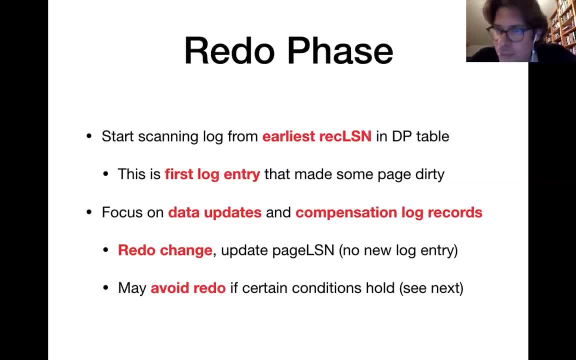 avoid redoing an operation, which of course we avoid if you can, because then course we avoid if you can, because then course we avoid if you can, because then things become more efficient. we can things become more efficient, we can things become more efficient. we can avoid to redo if one of the following: 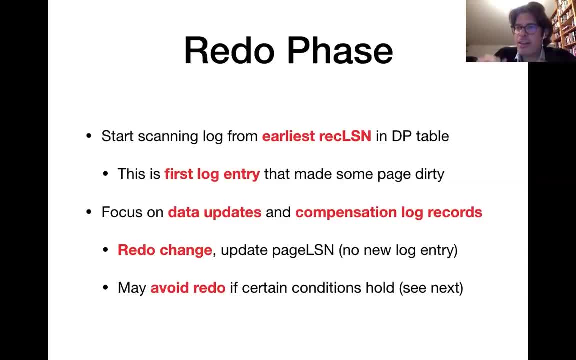 avoid to redo if one of the following: avoid to redo if one of the following three conditions is satisfied. so let's three conditions is satisfied. so let's three conditions is satisfied. so let's see under which conditions we can avoid, see under which conditions we can avoid. 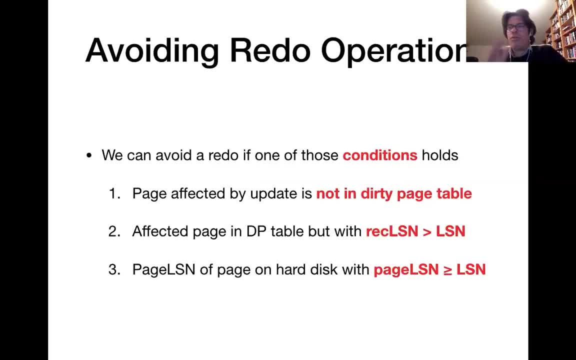 see under which conditions we can avoid the redo. so a first condition. if it the redo, so a first condition. if it the redo, so a first condition. if it holds, we can avoid the redo. it's the holds. we can avoid the redo. it's the holds. we can avoid the redo. it's the following: if the page affected by the 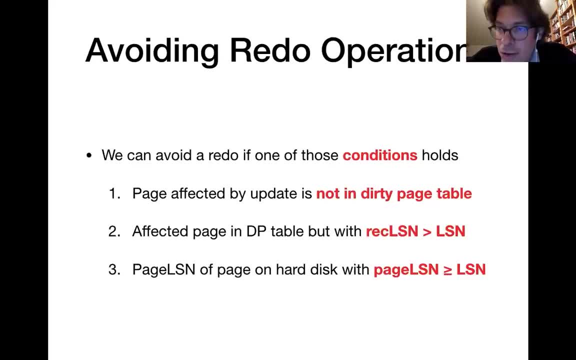 following: if the page affected by the following: if the page affected by the update we are currently looking at, is update we are currently looking at, is update we are currently looking at- is not in the dirty page table in not in the dirty page table in not in the dirty page table in anymore, then we know that the 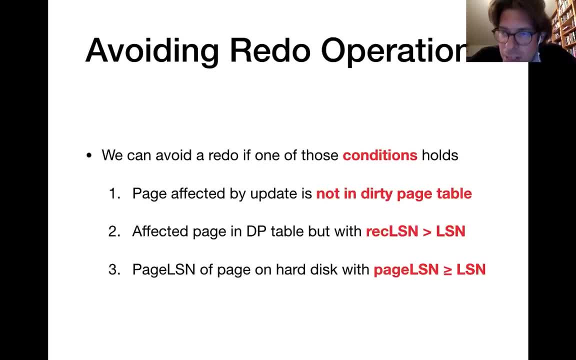 anymore then we know that, the anymore then we know that the corresponding log entry must already have corresponding log entry must already have corresponding log entry must already have been made persistent, so we don't need been made persistent. so we don't need been made persistent, so we don't need to redo the corresponding change also. 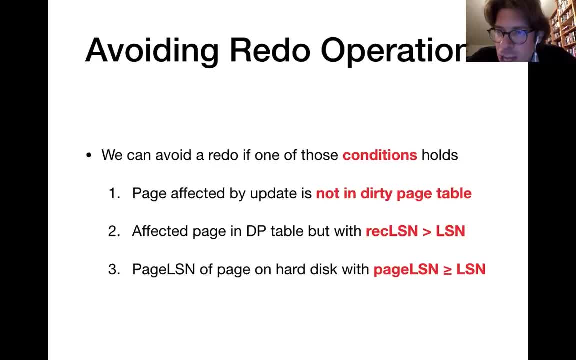 to redo the corresponding change. also. to redo the corresponding change, also assuming that a page is in the dirty. assuming that a page is in the dirty, assuming that a page is in the dirty page table, but the rec? LSN of that page page table, but the rec? LSN of that page. 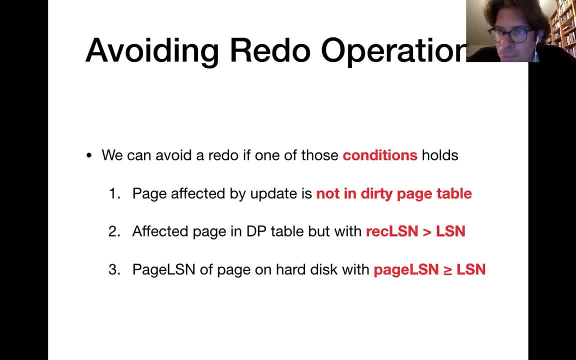 page table but the rec LSN of that page is greater than the current log sequence, is greater than the current log sequence, is greater than the current log sequence number. that essentially means that the number that essentially means that the number that essentially means that the page is dirty. 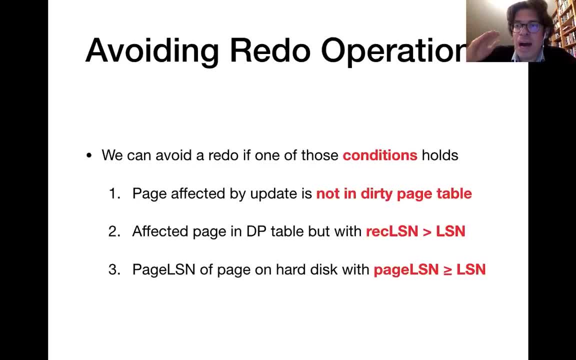 page is dirty. page is dirty, but it becomes dirty at by a later log. but it becomes dirty at by a later log, but it becomes dirty at by a later log entry than the current one. so also in entry than the current one. so also in entry than the current one. so also in this case we can avoid the redo and 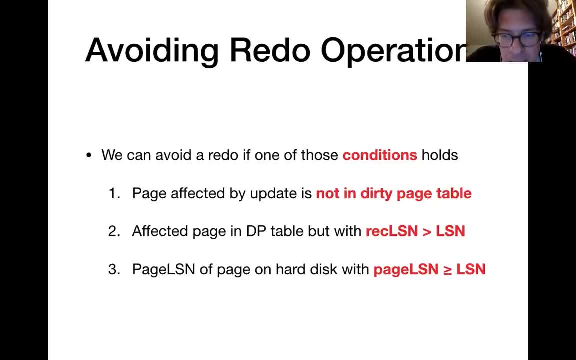 this case we can avoid the redo and this case we can avoid the redo. and, finally, we can avoid the redo as well. if, finally, we can avoid the redo as well, if, finally, we can avoid the redo as well, if the page LSN of the corresponding page. 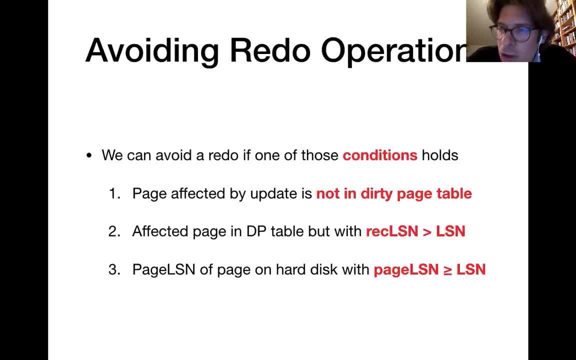 the page LSN of the corresponding page. the page LSN of the corresponding page on hard disk is greater or equal to the on hard disk is greater or equal to the on hard disk is greater or equal to the current log sequence number. so those are current log sequence number. so those are. 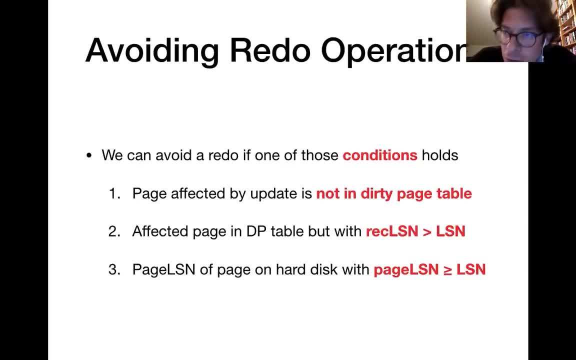 current log sequence number. so those are three conditions, three conditions, three conditions. if any of them holds, we don't have to. if any of them holds, we don't have to. if any of them holds, we don't have to redo the current update. we check those. redo the current update, we check those. 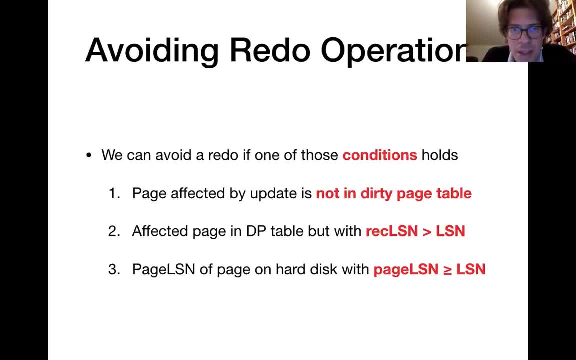 redo the current update. we check those three conditions in the order that you, three conditions in the order that you three conditions in the order that you see here. so one interesting question is see here. so one interesting question is see here. so one interesting question is: why do we check those conditions in? 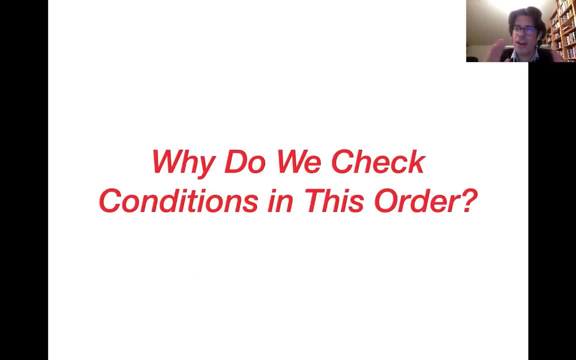 why do we check those conditions in? why do we check those conditions in precisely that order. so I give you a few precisely that order. so I give you a few, precisely that order. so I give you a few seconds to think about that, seconds to think about that. 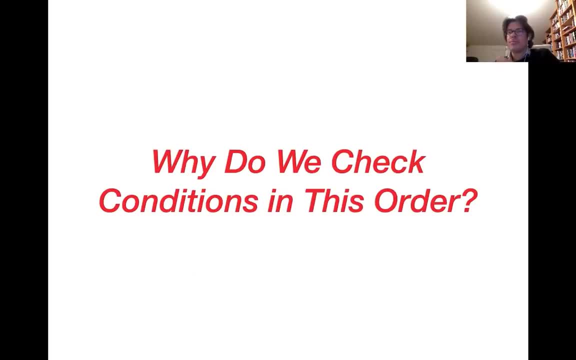 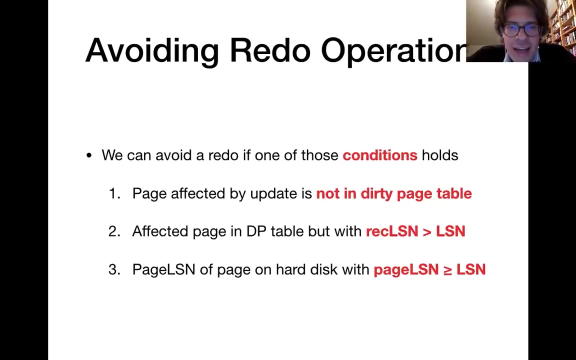 seconds to think about that, and I'm actually going to show you those, and I'm actually going to show you those, and I'm actually going to show you those conditions again and when thinking about conditions again, and when thinking about conditions again and when thinking about why we check them- in this order perhaps. 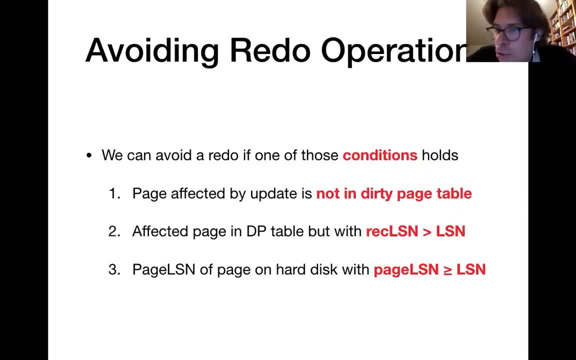 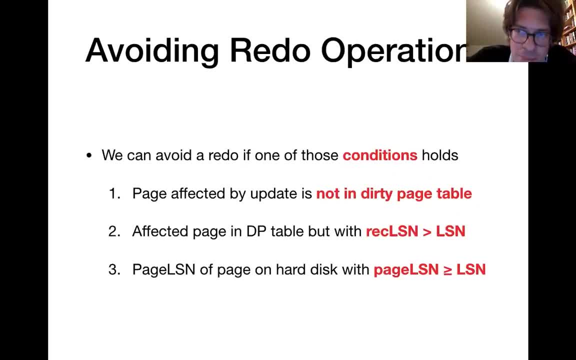 required to check those conditions, is required to check those conditions. is stored, but it's stored in main memory, or stored, but it's stored in main memory, or stored, but it's stored in main memory or on hard disk, and we know that accessing main memory, and we know that accessing main memory. 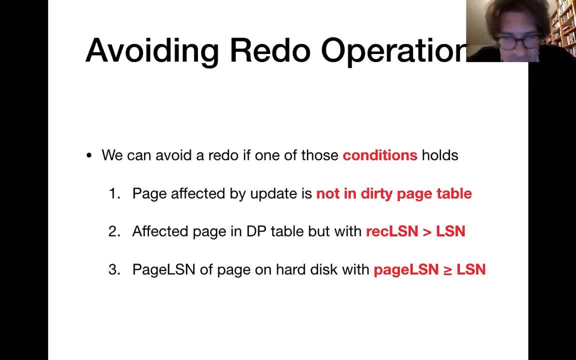 and we know that accessing main memory is more efficient than accessing hard, is more efficient than accessing hard, is more efficient than accessing hard disk, disk disk, and the right answer is that here the dirty page table is stored in main. and the right answer is that here the dirty page table is stored in main. 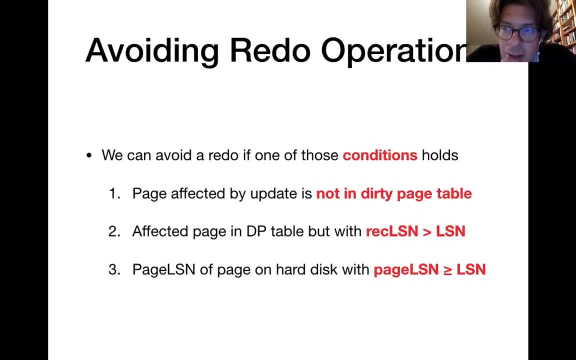 and the right answer is that here the dirty page table is stored in main memory. so the first two conditions can be memory. so the first two conditions can be memory. so the first two conditions can be verified relatively efficiently by the, verified relatively efficiently by the verified relatively efficiently by. the last condition refers to the page at us. 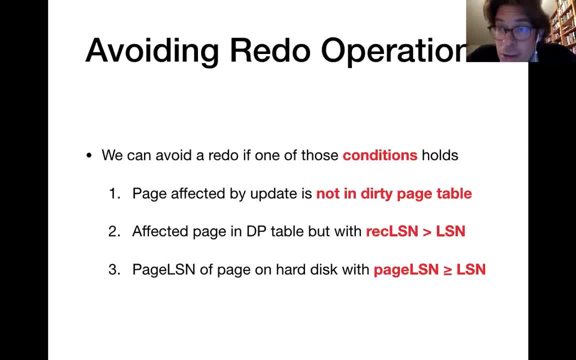 last condition refers to the page at us. last condition refers to the page at us in that is stored on hard disk and in in that is stored on hard disk and in in that is stored on hard disk and in order to get that, we already have to. 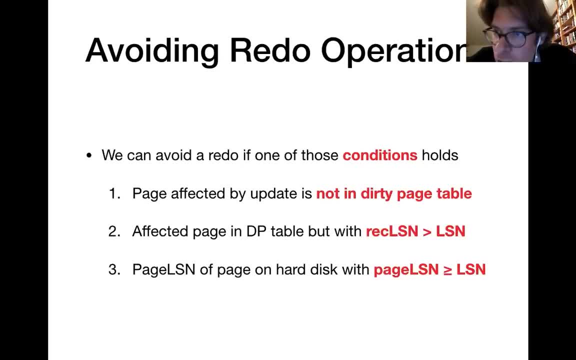 order to get that, we already have to order to get that, we already have to load that page from hard disk into main. load that page from hard disk into main. load that page from hard disk into main memory memory, which takes time. so this is why we, which takes time. so this is why we. 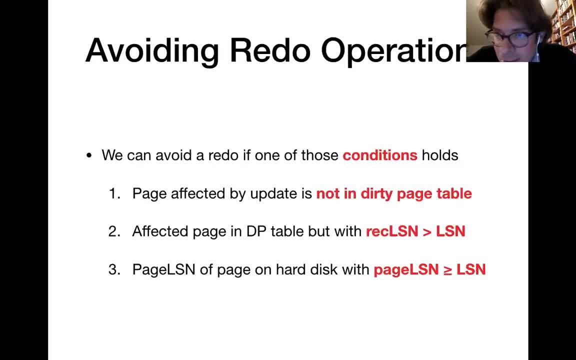 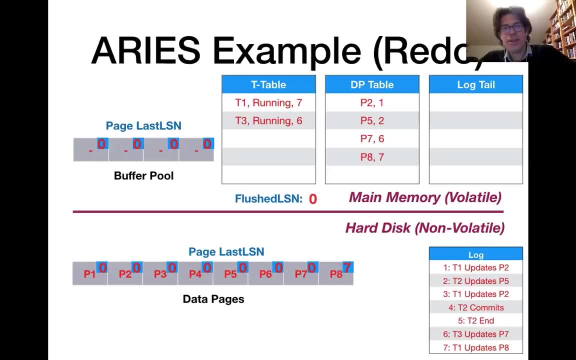 which takes time. so this is why we check the last condition, indeed, last the check. the last condition, indeed, last the check, the last condition, indeed, last the first two are much cheaper to verify first. two are much cheaper to verify first two are much cheaper to verify. all right, so now we continue with the. 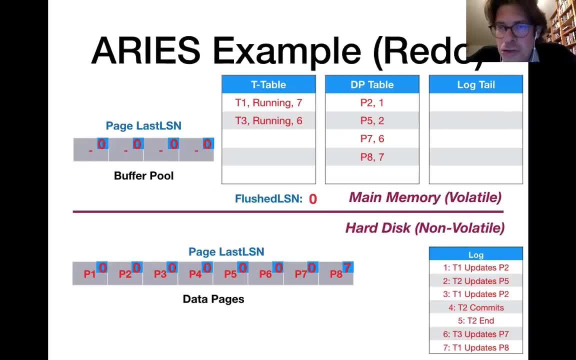 all right, so now we continue with the all right. so now we continue with the same running example, where we have just same running example, where we have just same running example where we have just executed the analysis phase, so now the. executed the analysis phase, so now the. 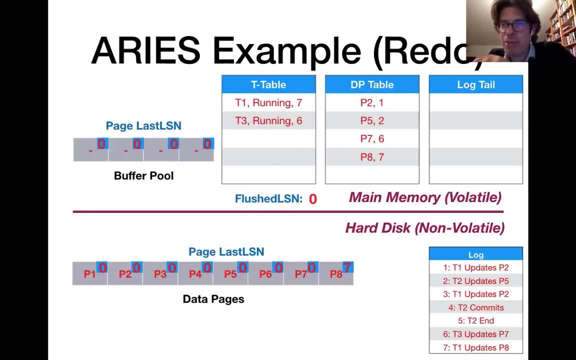 executed the analysis phase. so now the transaction table and the dirty page transaction table and the dirty page transaction table and the dirty page table. they have been restored as table. they have been restored as table. they have been restored as good as possible. so in the following we: 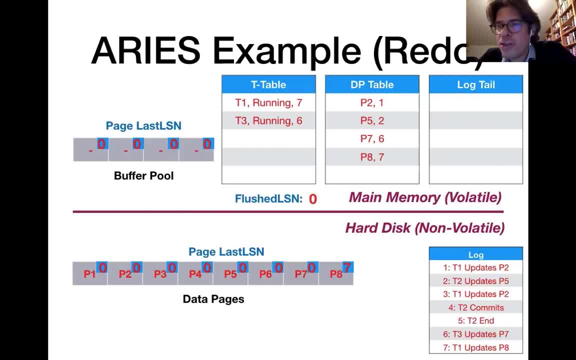 good as possible. so in the following, we good as possible. so in the following, we start the redo phase and first of all we start the redo phase. and first of all we start the redo phase and first of all we need to figure out starting from which, need to figure out starting from which. 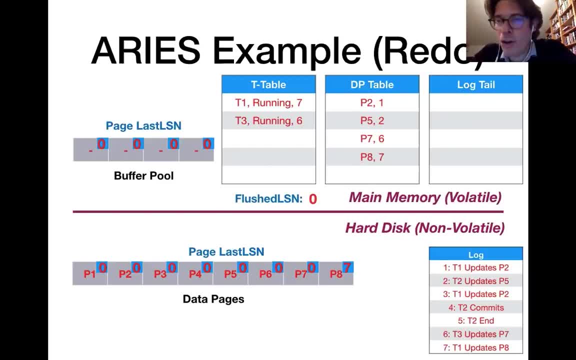 need to figure out starting from which log entry we need to read the log. and, in log entry, we need to read the log and in log entry, we need to read the log. and in order to find that out, we analyze the order to find that out, we analyze the. 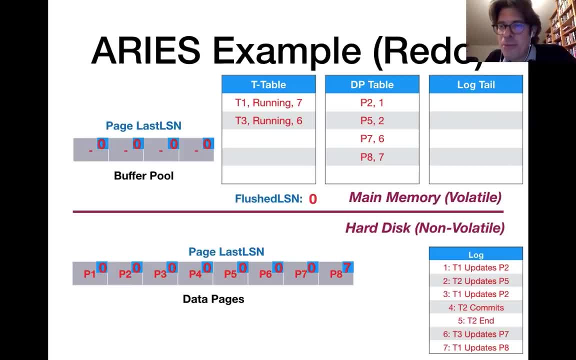 order to find that out, we analyze the dirty page table. we take the minimum dirty page table. we take the minimum dirty page table. we take the minimum rack at us and that we have stored there- rack at us and that we have stored there- rack at us and that we have stored there. that is the one that I have marked up. 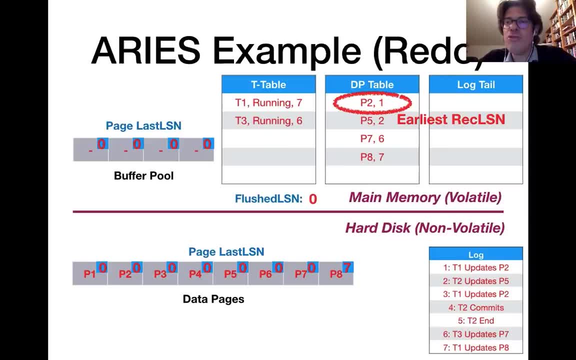 that is the one that I have marked up. that is the one that I have marked up here. so we do have to start the redo here. so we do have to start the redo here. so we do have to start the redo phase. indeed, from log entry number one: 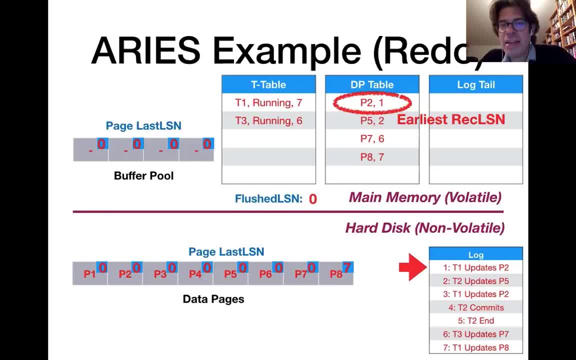 phase, indeed, from log entry number one. phase, indeed, from log entry number one. so let's start from log entry number one. so let's start from log entry number one. so let's start from log entry number one, which is a transaction one updating, which is a transaction one updating. 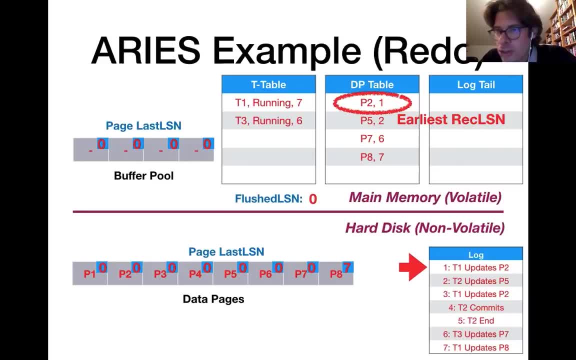 which is a transaction one updating page number two, and first of all we want to page number two and first of all we want to page number two and first of all we want to check whether we actually need to redo. check whether we actually need to redo, check whether we actually need to redo this, a log entry or not. 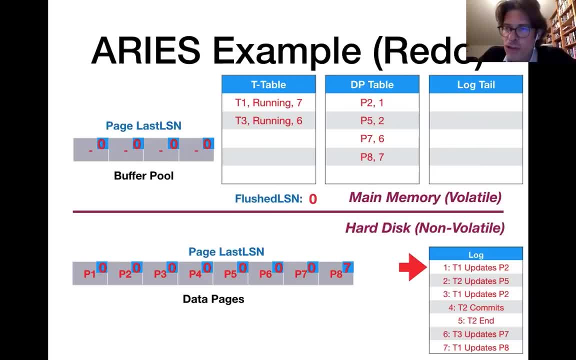 this a log entry or not? this a log entry or not? so first two conditions refer to the. so first two conditions refer to the. so first two conditions refer to the dirty page table. so let's first of all dirty page table. so let's first of all. 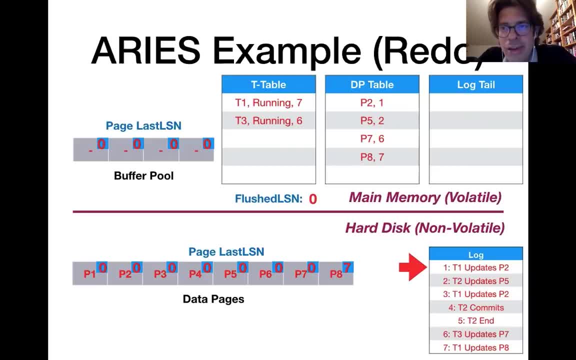 dirty page table. so let's first of all check page number two. is it in the dirty check page? number two: is it in the dirty check page? number two? is it in the dirty page table? and yes, indeed, it is in a page table and yes, indeed, it is in a. 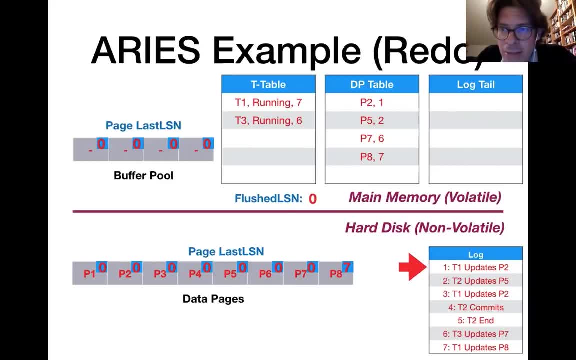 page table. and yes, indeed, it is in a dirty page table. and now we look at the dirty page table. and now we look at the dirty page table, and now we look at the record as n and, unfortunately, direct it record as n and, unfortunately, direct it record as n and, unfortunately, direct it is n, which is one in this case is not. 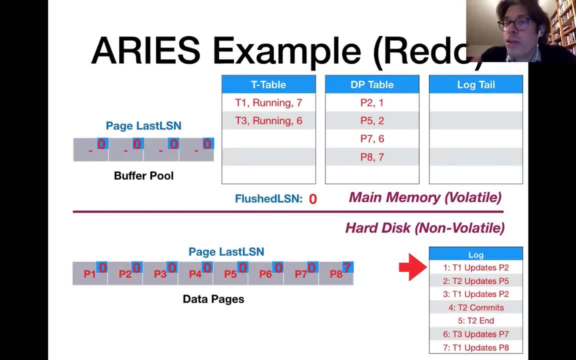 is n, which is one in this case, is not. is n, which is one in this case, is not greater than the current block sequence? greater than the current block sequence. greater than the current block sequence. addition: the page lsn on our disk. and. addition: the page lsn on our disk. and. 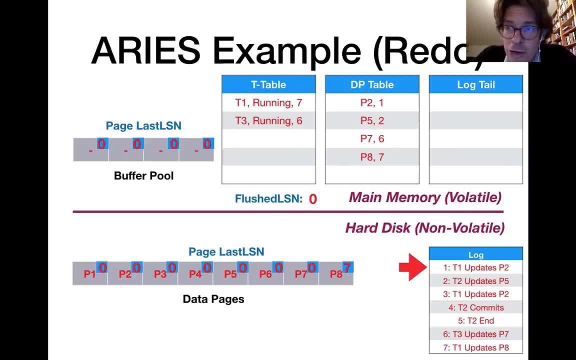 addition, the page lsn on our disk and for page number two that is zero, which for page number two that is zero, which for page number two that is zero, which is unfortunately not greater or equal to, is unfortunately not greater or equal to, is unfortunately not greater or equal to one, and this is why we have to probably 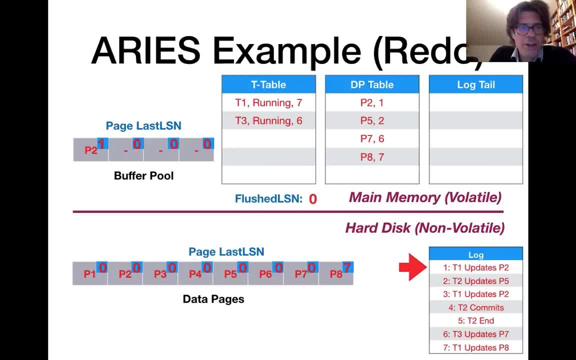 one, and this is why we have to probably one, and this is why we have to probably redo this change, redo this change, redo this change. so we are loading that page into main, so we are loading that page into main, so we are loading that page into main memory, we are executing the change in. 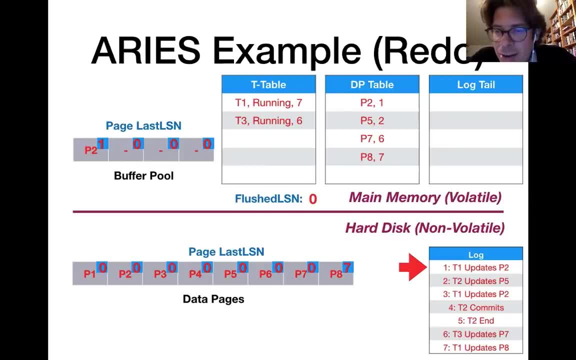 memory. we are executing the change in memory. we are executing the change in main memory and we are updating the page main memory. and we are updating the page main memory and we are updating the page lsn to one- all right. so in this case you lsn to one, all right. so in this case, you 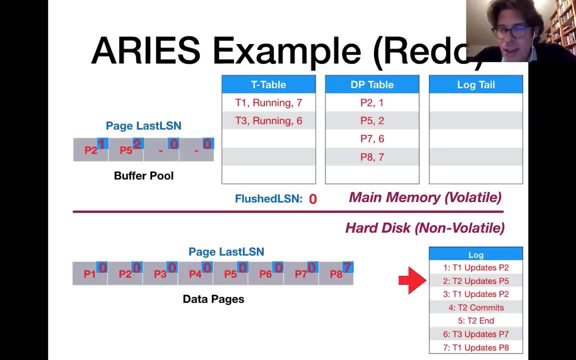 lsn to one, all right. so in this case, you had to redo, had to redo, had to redo the next. we encounter an update, by the next, we encounter an update, by the next. we encounter an update by transaction two, transaction two, transaction two of page number five, and here again, 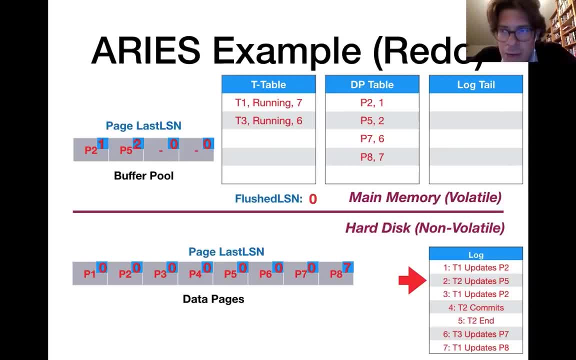 of page number five. and here again of page number five. and here again. page five is in the 30 page table. the page five is in the 30 page table. the page five is in the 30 page table. the rack lsn is not greater than a two. it. 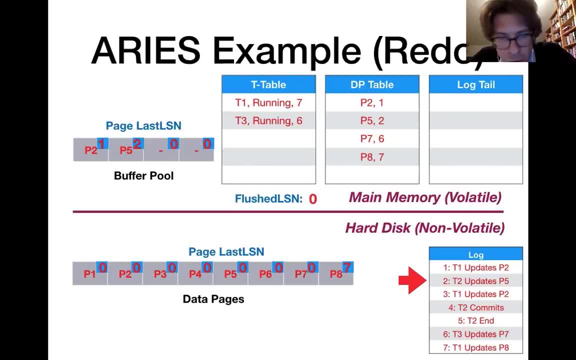 rack lsn is not greater than a two. it rack lsn is not greater than a two. it is exactly two, is exactly two, is exactly two, um. and if you look at the hard disk um, and if you look at the hard disk um, and if you look at the hard disk page lsn, then page five has a zero, which. 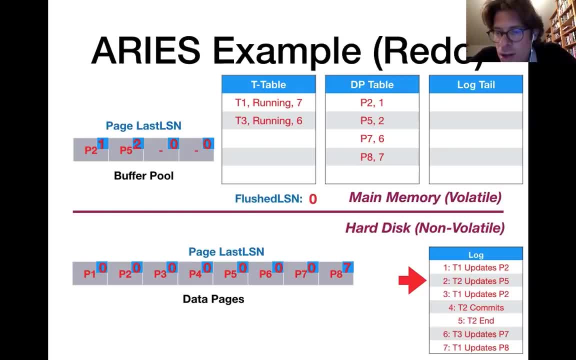 page lsn, then page five has a zero. which page lsn, then page five has a zero, which again is not the greater or equal to again is not the greater or equal to again is not the greater or equal to the current block sequence number which. the current block sequence number which 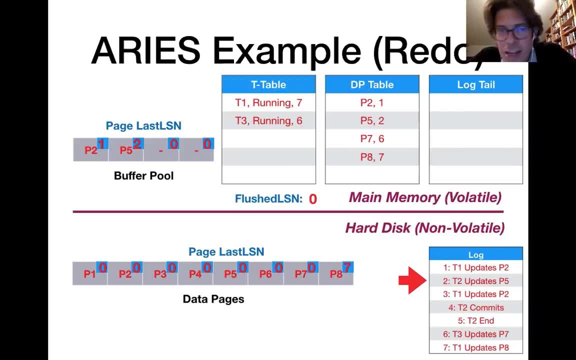 the current block sequence number, which is number two, is number two is number two. so we have to load it into the buffer. so we have to load it into the buffer. so we have to load it into the buffer pool. we update the page lsn to the. 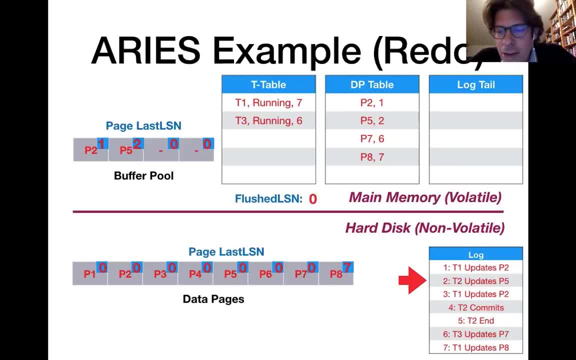 pool. we update the page lsn to the pool. we update the page lsn to the current block sequence number, which is current block sequence number, which is current block sequence number, which is two, two, two, and execute the associated change. and execute the associated change and execute the associated change. now, here again, t1 updates page two and. 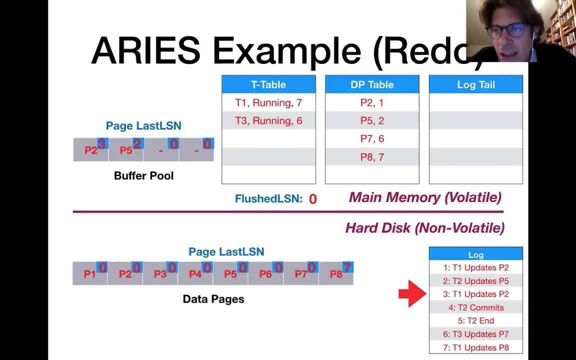 now here again. t1 updates page two. and now here again, t1 updates page two and page two is in the dirty page table with page two is in the dirty page table with page two is in the dirty page table with a lower rack: lsn. a lower rack: lsn. 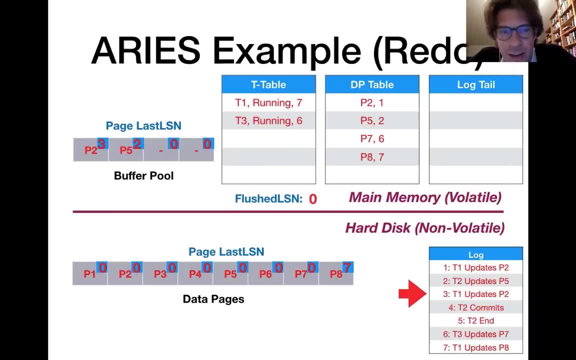 a lower rack lsn on disk on disk. on disk. page lsn is lower, we already have it. page lsn is lower, we already have it. page lsn is lower, we already have it loaded, loaded, loaded into main memory. so we just need to into main memory. so we just need to. 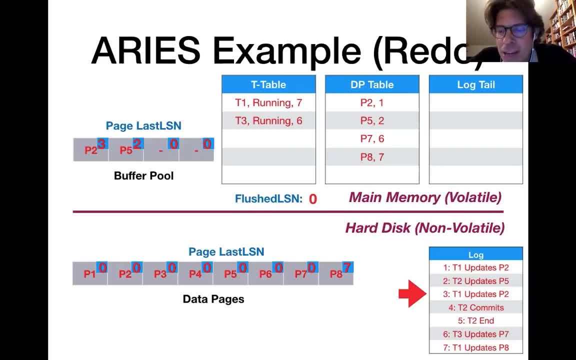 into main memory. so we just need to execute the corresponding change and execute the corresponding change and execute the corresponding change and update the page lsn to the current one. update the page lsn to the current one. update the page lsn to the current one, which is: 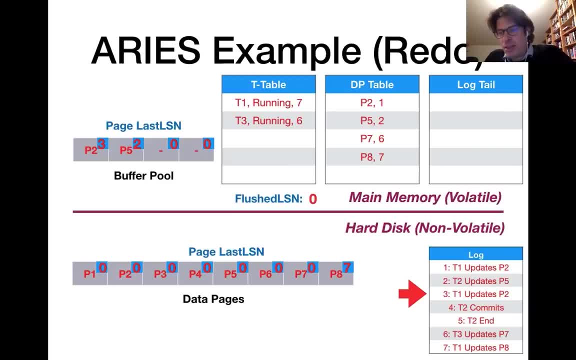 which is, which is three so commit and end block records. three so commit and end block records. three so commit and end block records. they are not interesting for redo. they are not interesting for redo. they are not interesting for redo. so we jump directly to the. so we jump directly to the. 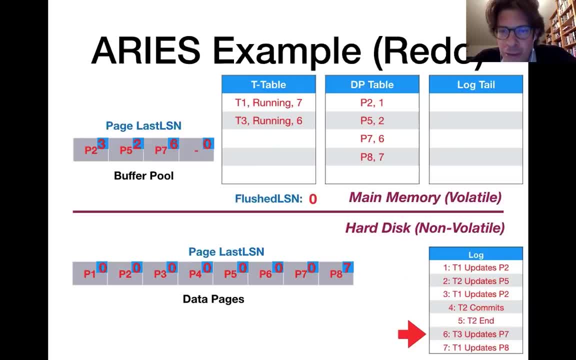 so we jump directly to the update of a page number seven by update of a page number seven, by update of a page number seven by transaction three, transaction three, transaction three. so here again um transact the page. so here again um transact the page. so here again um transact. the page number seven is in the dirty page table. number seven is in the dirty page table. number seven is in the dirty page table. it's a rack. lsn is not greater than the it's a rack. lsn is not greater than the it's a rack. lsn is not greater than the current one. 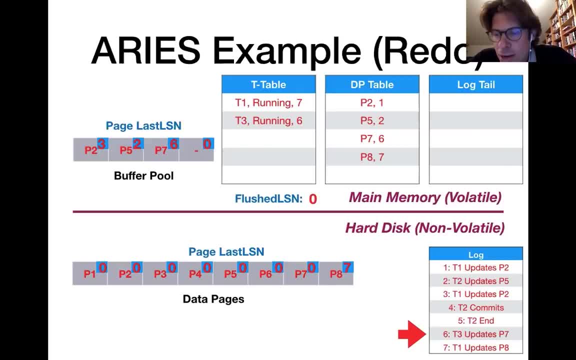 current one, current one. and looking at the page version on and looking at the page version on and looking at the page version on hard disk: uh, the page at this end is hard disk. uh, the page at this end is hard disk. uh, the page at this end is unfortunately lower than the current block. 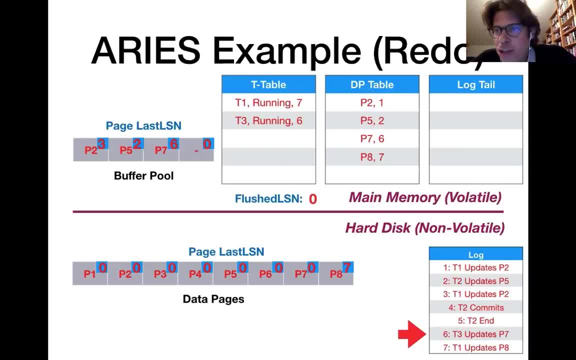 unfortunately lower than the current block. unfortunately lower than the current block sequence number. so we have to redo sequence number. so we have to redo sequence number. so we have to redo the operation. we load the page into main the operation. we load the page into main the operation. we load the page into main memory. 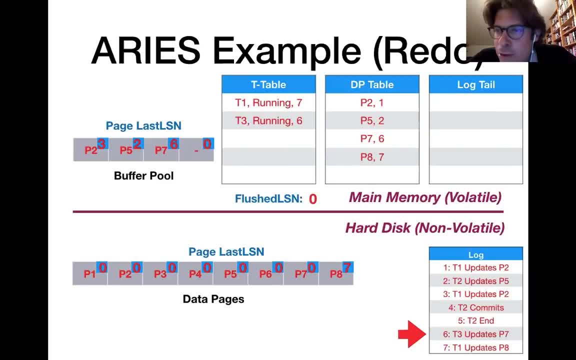 memory memory: execute the change and set the page at execute the change and set the page at execute the change and set the page at this end to six. so now let's look at the last um update. so now let's look at the last um update. so now let's look at the last um update transaction. one is updating page number. 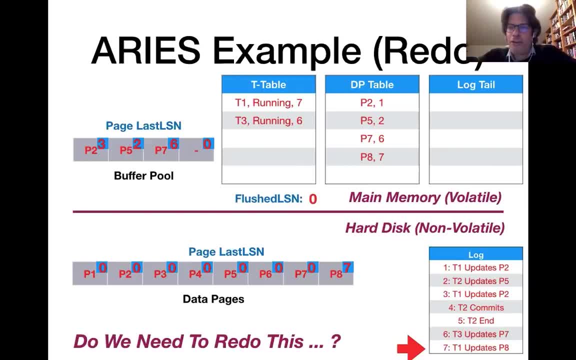 transaction one is updating page number. transaction one is updating page number eight, eight, eight. to think about whether we need to redo. to think about whether we need to redo. to think about whether we need to redo this change or not by verifying those, this change or not by verifying those. 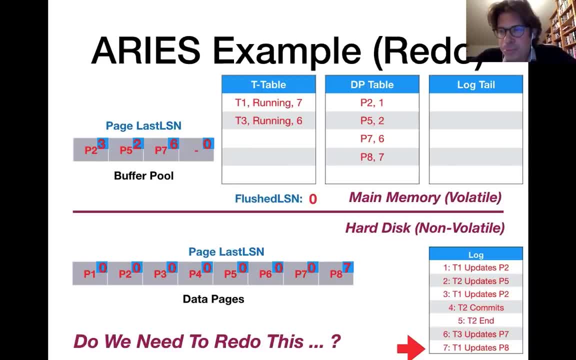 this change or not, by verifying those three conditions that we have seen, three conditions that we have seen, three conditions that we have seen before, but the first condition, but the first condition, but the first condition was checking. was checking, was checking better? the page is in the dirty page. 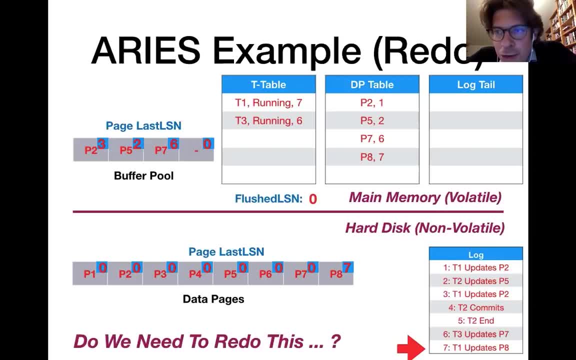 better the page is in the dirty page, better the page is in the dirty page table. then the second condition, then the second condition. then the second condition is looking at the rack lsn is looking at the rack lsn is looking at the rack lsn. third condition is looking at the hard. 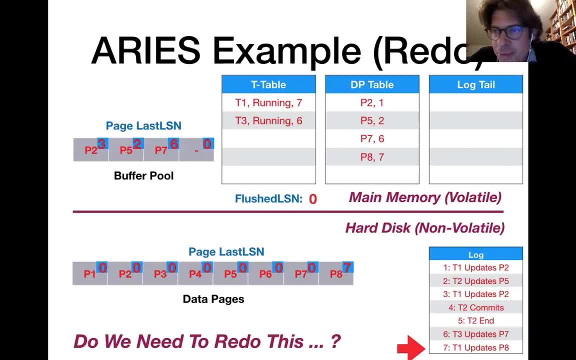 third condition is looking at the hard. third condition is looking at the hard disk version of the page disk version of the page disk version of the page, and in this case the page is in the dirty and in this case the page is in the dirty and in this case the page is in the dirty page table we find page number eight. 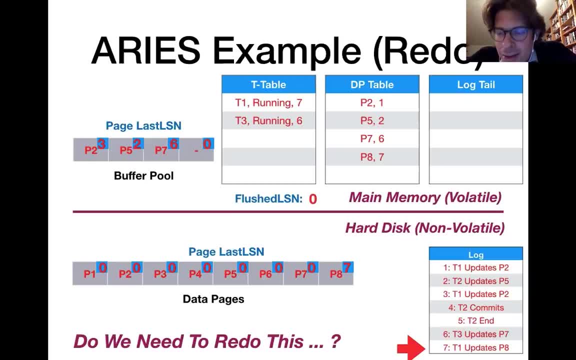 page table. we find page number eight page table. we find page number eight. so that condition is not verified. so that condition is not verified. so that condition is not verified, the the, the rack lsn of the page, rack lsn of the page, rack lsn of the page is not greater than the current one. so 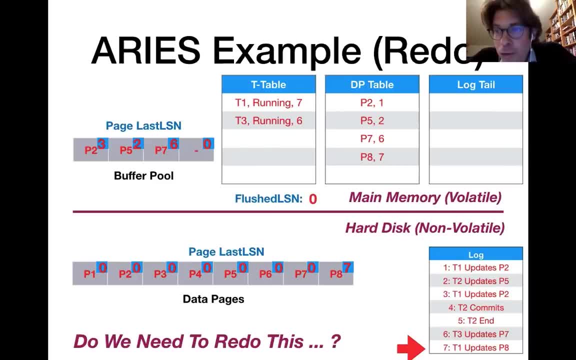 is not greater than the current one, so is not greater than the current one, so that condition is not verified. that condition is not verified. that condition is not verified either, either. either now. if you, however, look at the hardest now. if you, however, look at the hardest now. if you, however, look at the hardest version of the page. 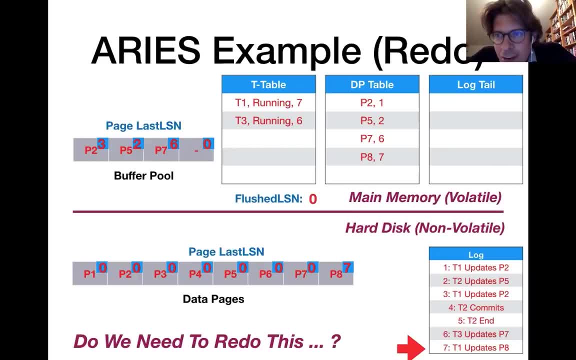 version of the page. version of the page. here for page number eight. we find that. here for page number eight. we find that. here for page number eight, we find that the page lsn is actually equal. the page lsn is actually equal. the page lsn is actually equal to seven. that means that all the changes 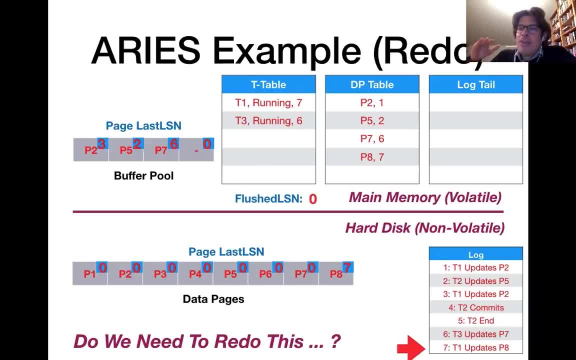 to seven. that means that all the changes to seven, that means that all the changes up to block sequence number seven have up to block sequence number seven have up to block sequence number seven have already been made. persistent on the already been made persistent on the already been made. persistent on the hard disk. 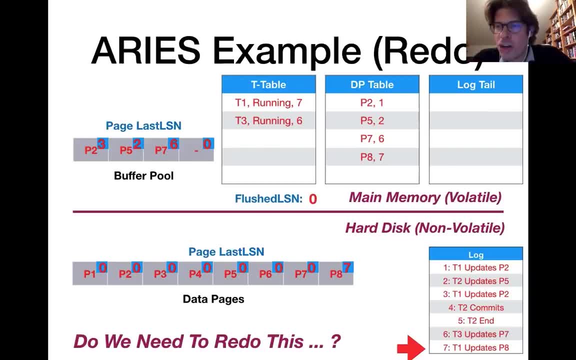 hard disk: hard disk. and this is why, in this case, we don't, and this is why, in this case, we don't, and this is why, in this case, we don't actually need to redo the corresponding actually need to redo the corresponding actually need to redo the corresponding change. 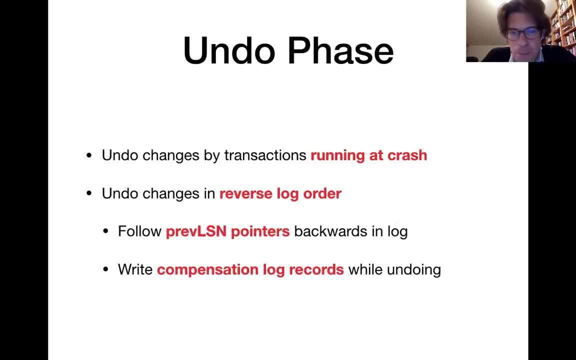 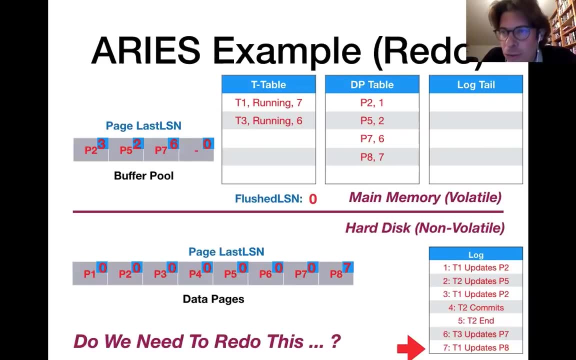 change, change. so here the final one does not need to. so here the final one does not need to. so here the final one does not need to be redone: be redone, be redone. that was the redo phase here. that was the redo phase here. that was the redo phase here. the next up is the undo phase. 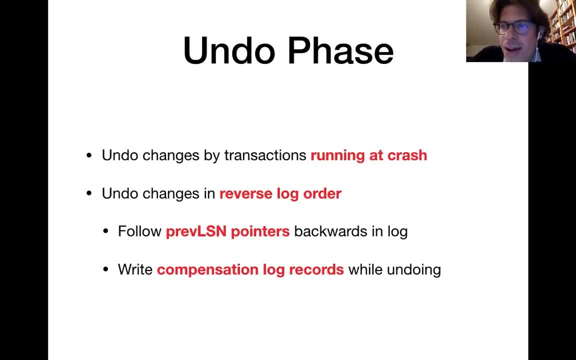 now here we want to undo transactions. now here. we want to undo transactions. now here. we want to undo transactions that we are running at the time of the, that we are running at the time of the, that we are running at the time of the crash, crash, crash. transactions that have not committed. 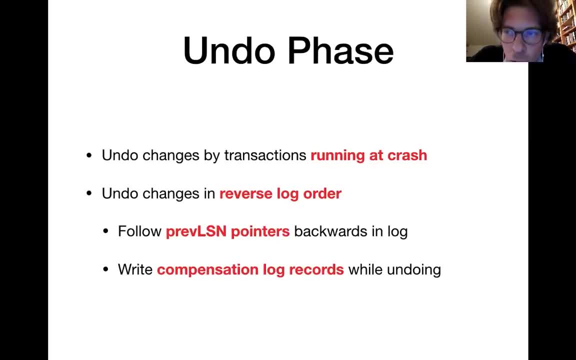 transactions that have not committed, transactions that have not committed before the crash and we want to undo before the crash and we want to undo before the crash and we want to undo those changes of those transactions, in those changes of those transactions, in those changes of those transactions in reverse order. 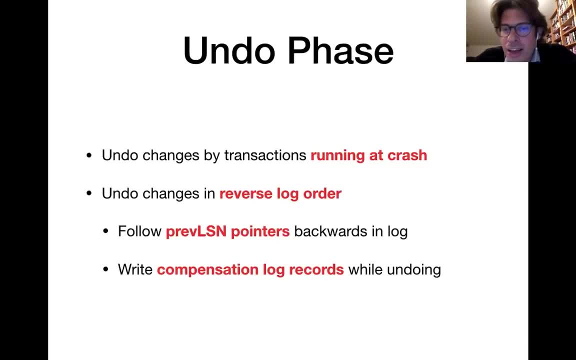 reverse order. reverse order. of course we could just keep reading. of course we could just keep reading. of course we could just keep reading log entries in a reverse order. log entries in a reverse order. log entries in a reverse order. but that would be inefficient, but that would be inefficient. 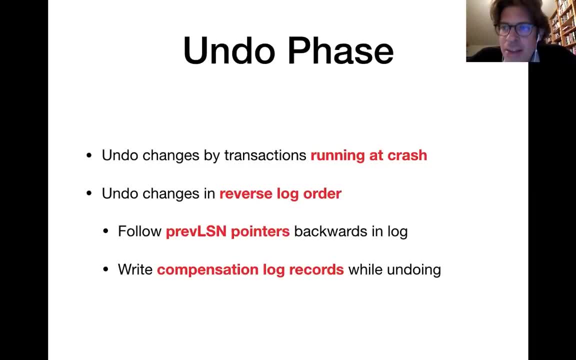 but that would be inefficient. some time ago, when discussing the. some time ago, when discussing the. some time ago, when discussing the structure of the log entries- structure of the log entries, structure of the log entries- i introduced the so-called prep lsn. i introduced the so-called prep lsn. 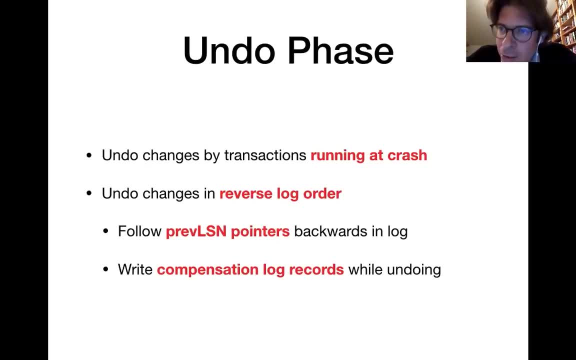 i introduced the so-called prep lsn field and for a given log entry. the field and for a given log entry. the field and for a given log entry. the prep lsn field essentially points. prep lsn field essentially points. prep lsn field essentially points to the last log entry generated by the. 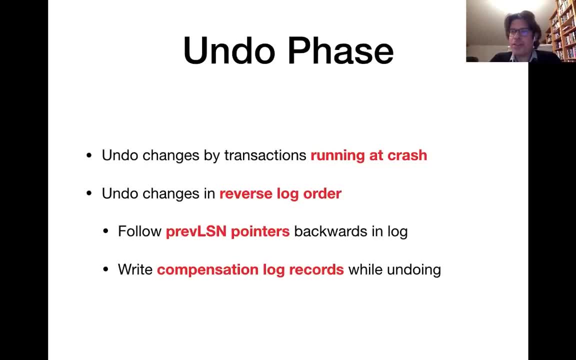 to the last log entry generated by the. to the last log entry generated by the same transaction. so here, this is same transaction. so here, this is same transaction. so here, this is essentially like a pointer. we just essentially like a pointer. we just essentially like a pointer. we just stored a log sequence number of the. 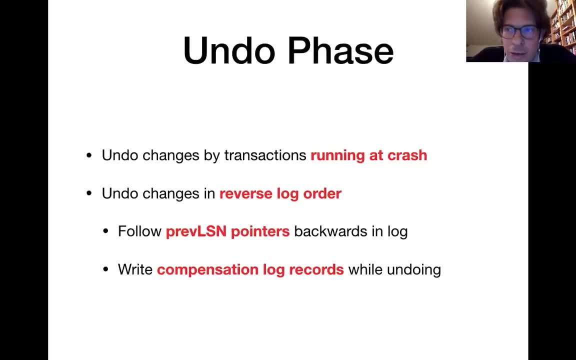 stored a log sequence number of the stored a log sequence number of the last log entry. last log entry, last log entry. so then going back through the log in. so then going back through the log in. so then going back through the log in order to undo. order to undo. 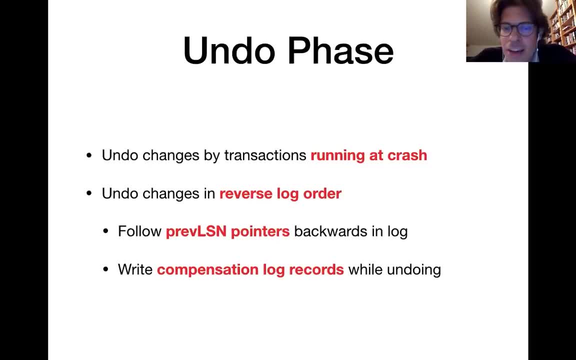 order to undo the changes of one specific transaction, the changes of one specific transaction, the changes of one specific transaction, then we use those pointers in order to, then we use those pointers in order to, then we use those pointers in order to efficiently, efficiently, efficiently jump through the lock along the. 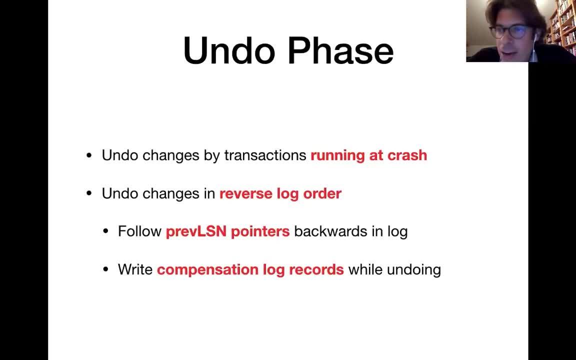 jump through the lock along the jump through the lock along the generated by the same transaction, generated by the same transaction, generated by the same transaction. and by we are undoing those changes, we, and by we are undoing those changes, we, and by we are undoing those changes, we also write those. 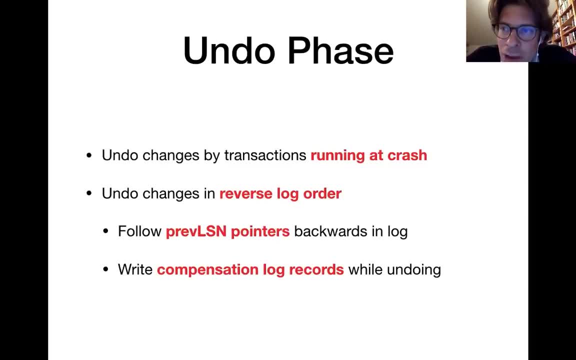 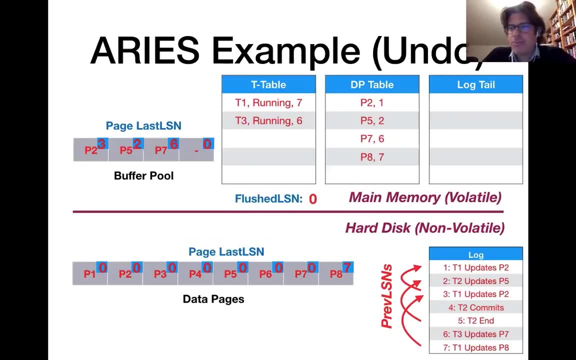 also write those, also write those compensation log records, which always compensation log records, which always compensation log records, which always keep track of changes that have already, keep track of changes that have already, keep track of changes that have already been undone. so let's again see how we do this in. 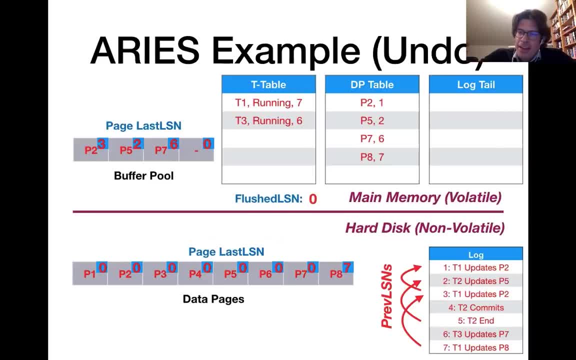 so let's again see how we do this in. so let's again see how we do this in the example, the example, the example here, so um here in the log on hard disk. here, so um here in the log on hard disk. here, so um here in the log on hard disk you can see: 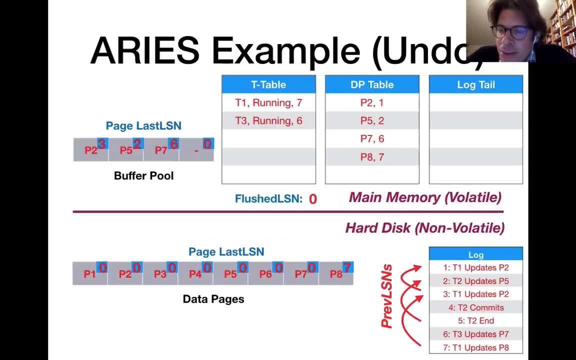 you can see. you can see that i symbolize those prep lsn, that i symbolize those prep lsn, that i symbolize those prep lsn pointers by those red arrows which are pointers, by those red arrows which are pointers, by those red arrows which are connecting. 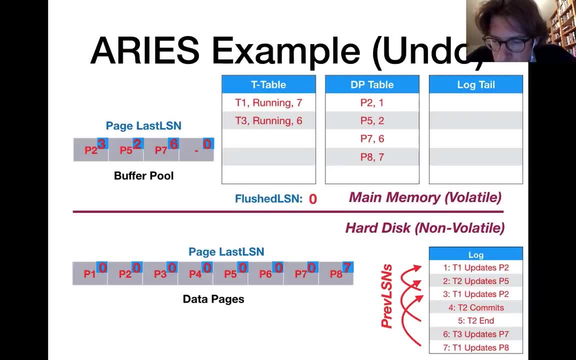 connecting, connecting log entries that belong to the same log entries that belong to the same log entries that belong to the same transaction, transaction, transaction. and we are undoing things in a reverse and we are undoing things in a reverse and we are undoing things in a reverse order. so here we have two transactions. 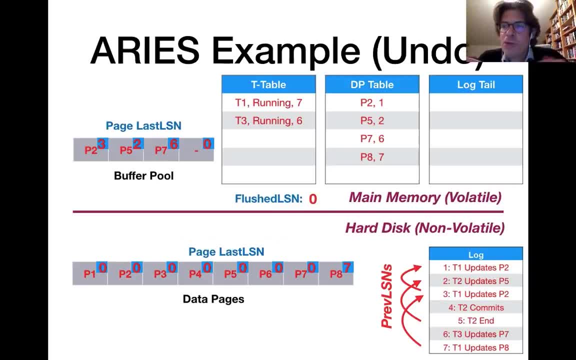 order. so here we have two transactions order. so here we have two transactions: running transaction one. running transaction one. running transaction one and transaction three. they were running and transaction three. they were running and transaction three. they were running at the time of the crash, so at the time of the crash. so 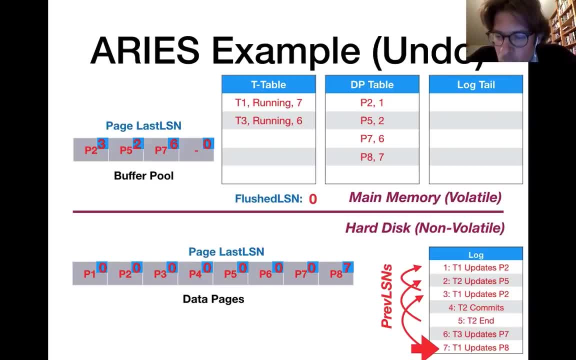 at the time of the crash. so we start undoing the last operation, we start undoing the last operation, we start undoing the last operation of a transaction, one which updated at, of a transaction one which updated at. of a transaction one which updated at page number eight. 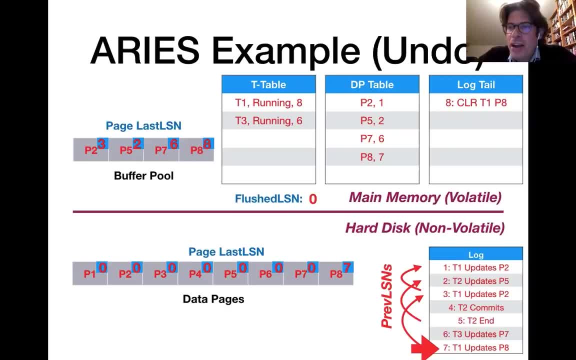 page number eight, page number eight. so, in order to undo this, so first of all, so, in order to undo this, so first of all, so, in order to undo this, so first of all, we write a compensation, we write a compensation, we write a compensation log record in our concise notation here. 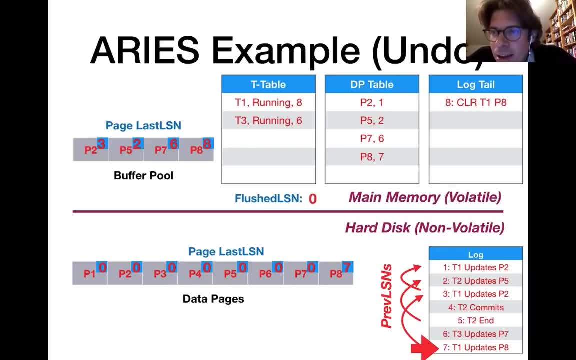 log record in our concise notation here. log record in our concise notation here for those examples. it is for those examples. it is for those examples. it is simply a clr, then the transaction simply a clr, then the transaction simply a clr, then the transaction identifier and then the page identifier. 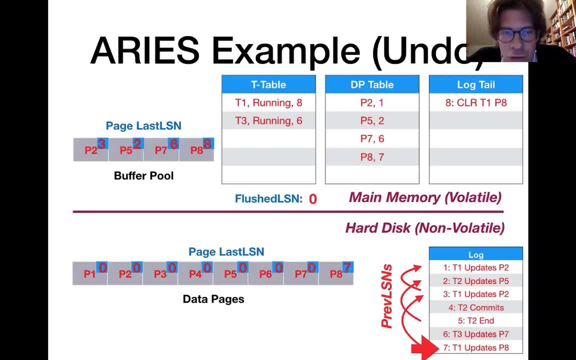 identifier and then the page identifier- identifier and then the page identifier. and in order to undo the change we have, and in order to undo the change we have, and in order to undo the change, we have to load the page from hard disk into. to load the page from hard disk into. 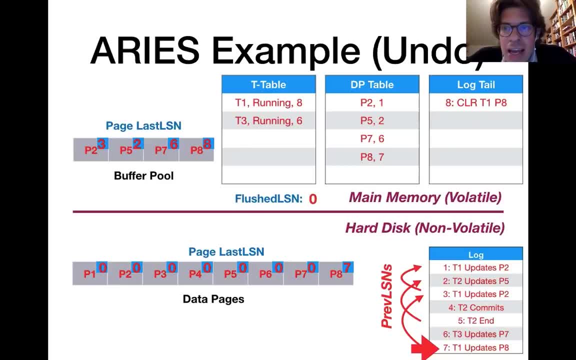 to load the page from hard disk into main memory, main memory, main memory. and we undo the change, and, and we undo the change, and and we undo the change. and undoing the change is also a change. so undoing the change is also a change. so undoing the change is also a change. so therefore, 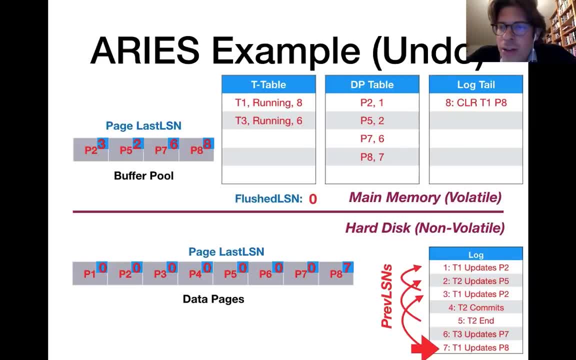 therefore, therefore, we also update the page lsn to. we also update the page lsn to. we also update the page lsn to the current log sequence number from the, the current log sequence number from the, the current log sequence number from the compensation compensation, compensation log record. so now, 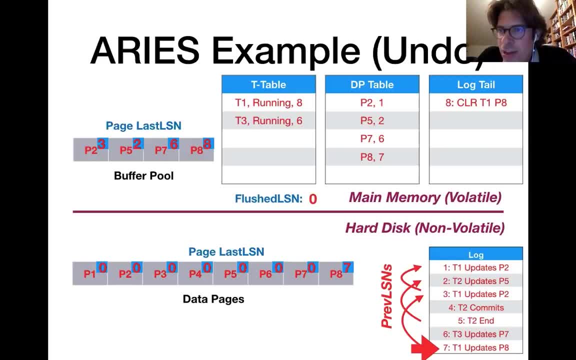 log record. so now log record. so now, um the next, um, the next, um, the next. log entry in reverse order would belong: log entry in reverse order would belong. log entry in reverse order would belong to a transaction, to a transaction, to a transaction s3, which also has to be. 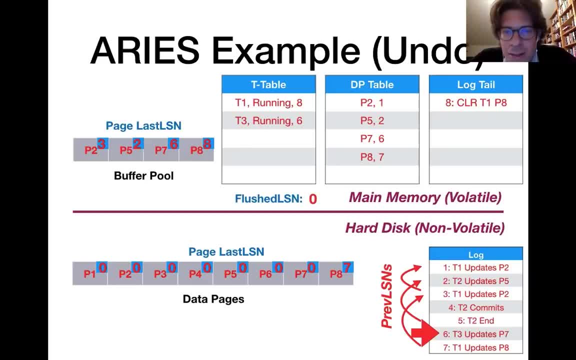 s3, which also has to be s3, which also has to be undone. so here, transactions, we updates undone. so here, transactions, we updates undone. so here, transactions, we updates. page number seven, page number seven, page number seven: so, uh, we write the compensation log. so, uh, we write the compensation log. 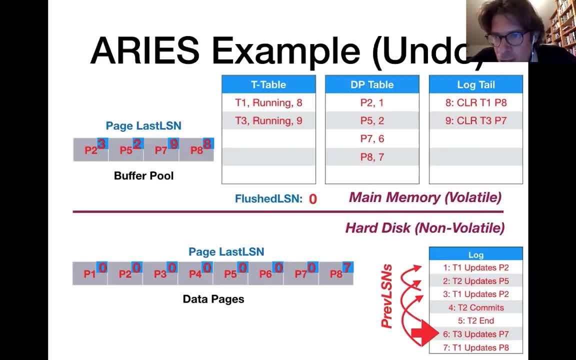 so, uh, we write the compensation log record record record again in order to undo this change, and again in order to undo this change, and again in order to undo this change. and the page number seven is already in our. the page number seven is already in our. the page number seven is already in our buffer pool, so we don't need to load it. 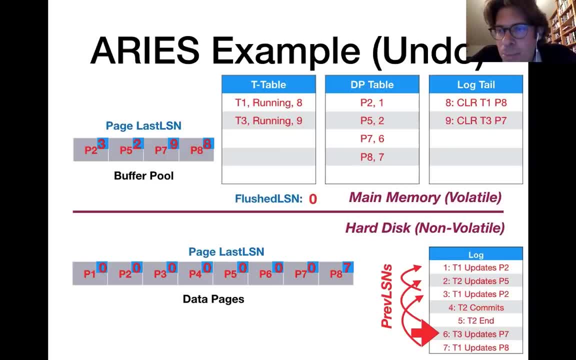 buffer pool, so we don't need to load it. buffer pool, so we don't need to load it anymore. we just anymore, we just anymore. we just undo the change and update the page lsm. undo the change and update the page lsm. undo the change and update the page lsm to number nine. 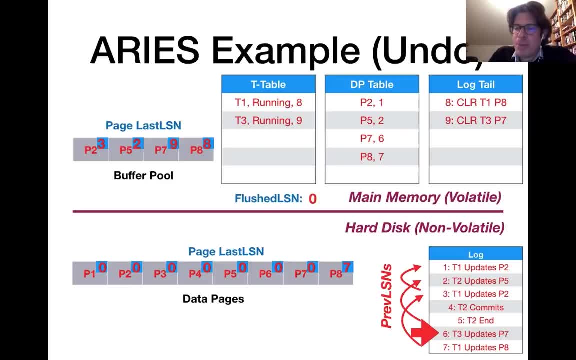 to number nine, to number nine. so now we use those pointers in order. so now we use those pointers in order. so now we use those pointers in order to to: to identify candidates for the next log. identify candidates for the next log. identify candidates for the next log entry that we might want to undo, which? 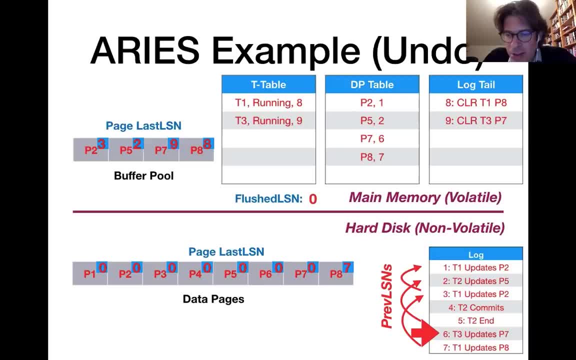 entry that we might want to undo. which entry that we might want to undo? which is one is one? is one changed by uh. one of the transactions changed by uh. one of the transactions changed by uh. one of the transactions that we are undoing, that we are undoing? 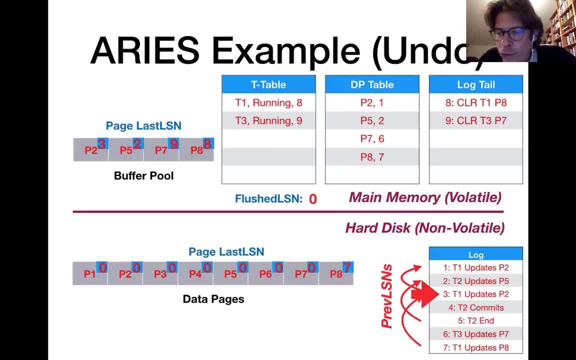 that we are undoing. so here we jump to the update of. so here we jump to the update of. so here we jump to the update of. transaction one to page number two. transaction one to page number two. transaction one to page number two. again, we write the corresponding. 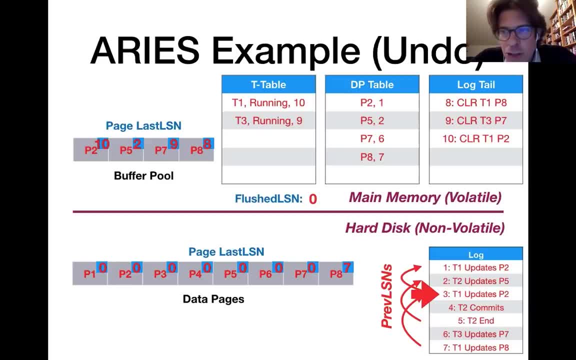 again. we write the corresponding again. we write the corresponding compensation compensation compensation log record and page number two log record. and page number two log record. and page number two: is um already in main memory, so we don't. is um already in main memory, so we don't. 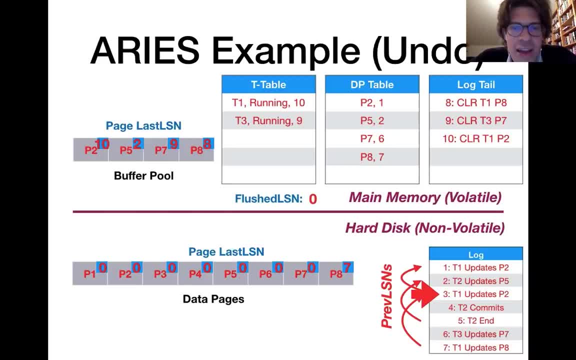 is um already in main memory, so we don't need to load it. we update the page. need to load it. we update the page. need to load it. we update the page lsn and we undo the corresponding change lsn and we undo the corresponding change lsn and we undo the corresponding change now. 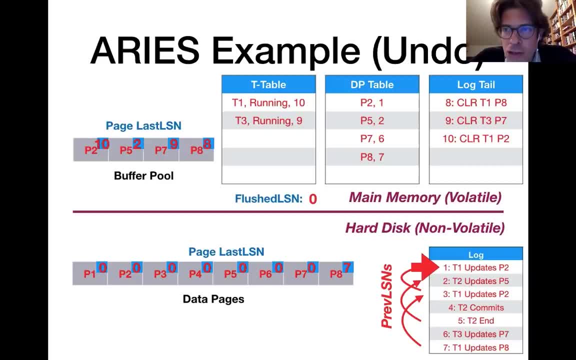 now. now we jump over the next one. because that we jump over the next one, because that we jump over the next one, because that one belongs to transaction two, which one belongs to transaction two, which one belongs to transaction two which committed. so we don't want to undo that. 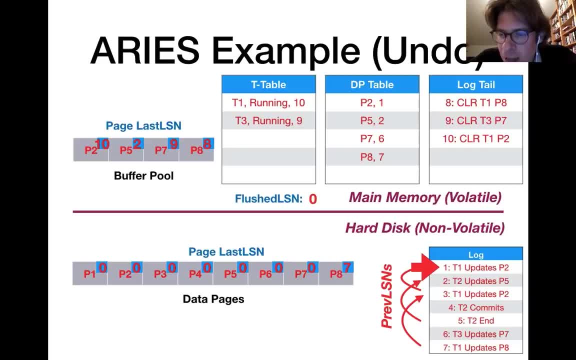 committed, so we don't want to undo that. committed, so we don't want to undo that. of course, of course, of course. so you're going directly to the first. so you're going directly to the first, so you're going directly to the first log entry by transaction, one which 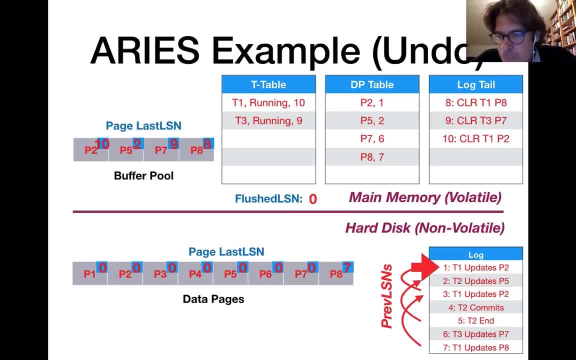 log entry by transaction one which log entry by transaction one which updated page number two and updated page number two and updated page number two. and here um page number two again. here um page number two again. here um page number two again is already in, uh, main memory. 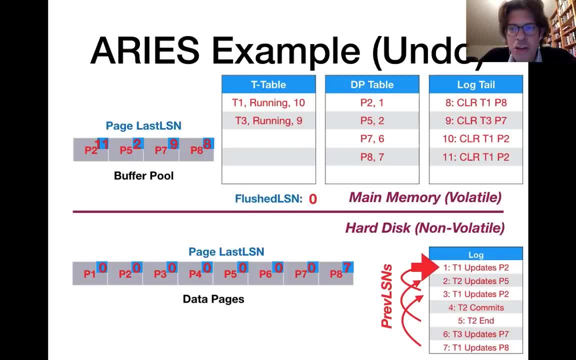 is already in uh main memory. is already in uh main memory um. we write the corresponding um. we write the corresponding um. we write the corresponding compensation log record. update compensation log record. update compensation log record. update. the page at this end and the page itself. the page at this end and the page itself. 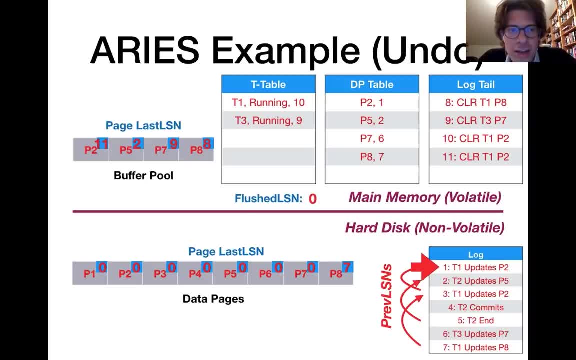 the page at this end and the page itself. and now we have undone all the and now we have undone all the and now we have undone all the associated um operations. so here we i associated um operations. so here we i associated um operations. so here we i could. 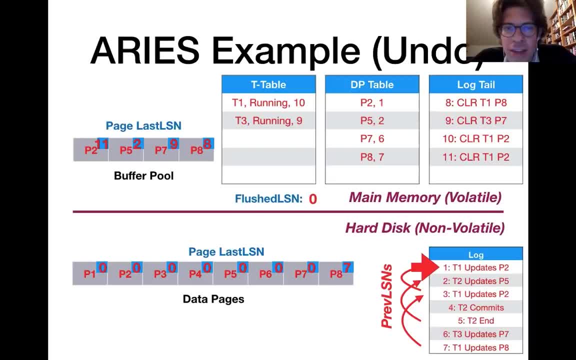 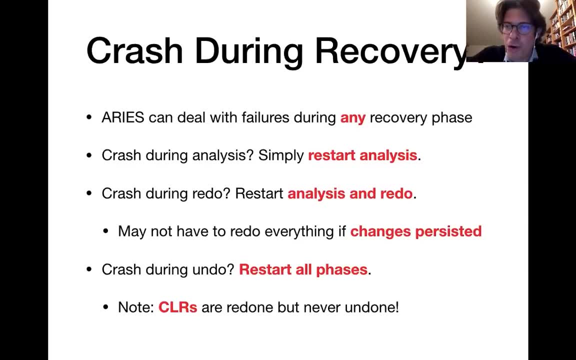 could, could, now, in the next steps, delete those now in the next steps. delete those now in the next steps. delete those transactions, for instance, from the transactions, for instance from the transactions, for instance from the transaction table, transaction table, transaction table. all right now, one last point. all right now, one last point. 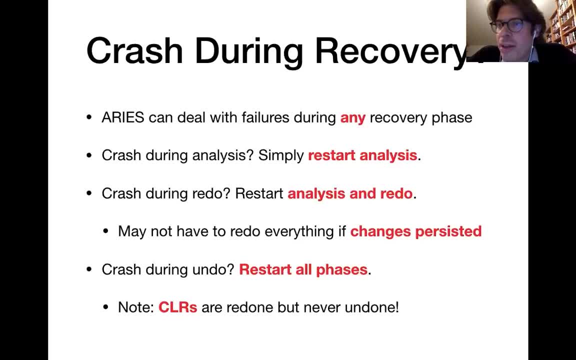 all right now. one last point that i want to discuss is a crashes that i want to discuss is a crashes that i want to discuss is a crashes doing recovery, doing recovery, doing recovery. now that might at first sound a little. now, that might at first sound a little. 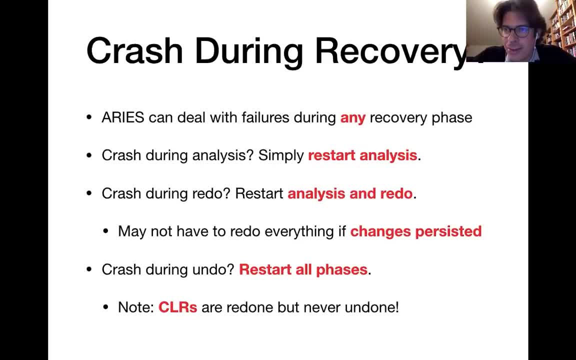 now that might at first sound a little bit unlikely. you just had a crash. what bit unlikely. you just had a crash. what bit unlikely. you just had a crash. what are the chances that it crashes while are the chances that it crashes while? are the chances that it crashes while you're in the process of recovering? but 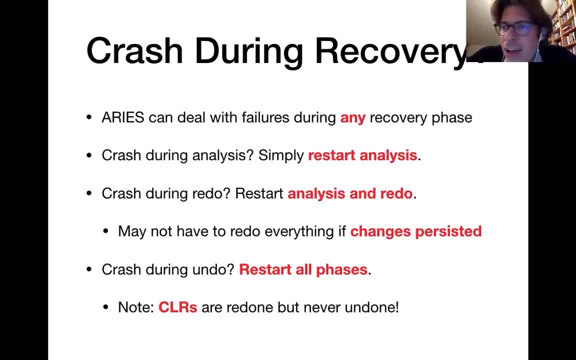 you're in the process of recovering. but you're in the process of recovering, but for instance, for instance, for instance, if you have an unreliable power supply, if you have an unreliable power supply, if you have an unreliable power supply and that has caused the first crash to 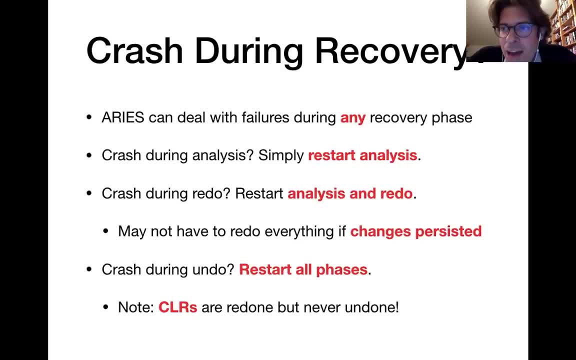 and that has caused the first crash to and that has caused the first crash to, maybe, maybe, maybe, um directly after it is still a little um directly after. it is still a little um directly after. it is still a little bit unreliable. so you might actually bit unreliable, so you might actually. 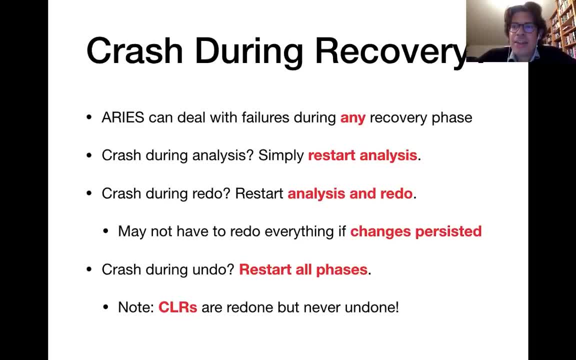 bit unreliable, so you might actually have increased chances for a second crash, have increased chances for a second crash, have increased chances for a second crash and in general, the aries algorithm and in general the aries algorithm and in general the aries algorithm has the nice property that it can deal. 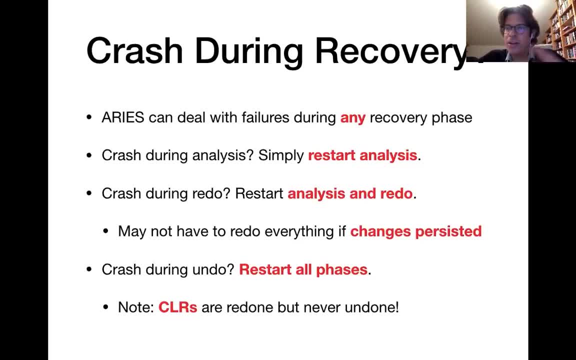 has the nice property that it can deal, has the nice property that it can deal with crashes during the recovery. so with crashes during the recovery, so with crashes during the recovery. so let's quickly, let's quickly, let's quickly go over the possibilities. so i mean, if 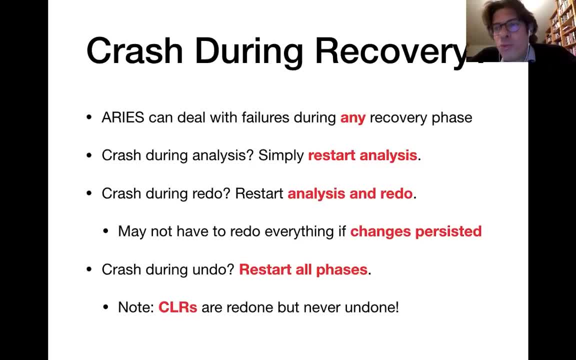 go over the possibilities. so i mean if go over the possibilities, so i mean if you have, you have, you have crash during the analysis phase, then you crash during the analysis phase. then you crash during the analysis phase, then you simply, simply, simply restart the analysis phase, restart the analysis phase. 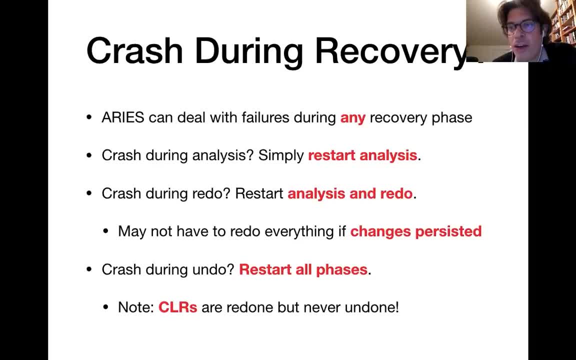 restart the analysis phase um. if you have a crash during the redo um, if you have a crash during the redo um, if you have a crash during the redo phase, then phase, then phase, then, of course, after the system comes back, of course, after the system comes back. 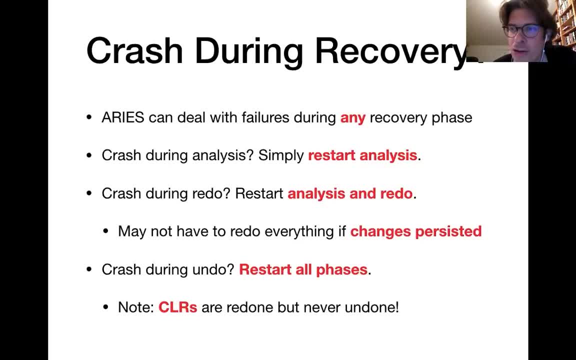 of course, after the system comes back online again after the second crash, you online again after the second crash. you online again after the second crash. you still have to re-execute, still have to re-execute, still have to re-execute the analysis phase and finally you have. 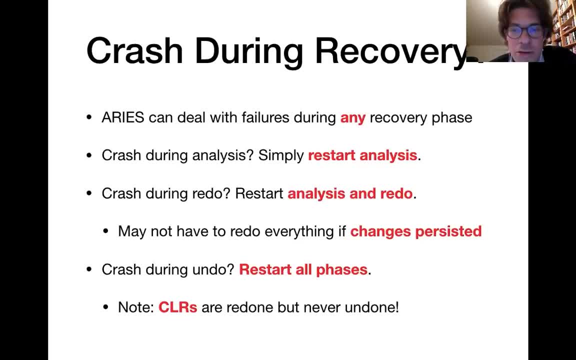 the analysis phase, and finally, you have the analysis phase and finally, you have to redo the, to redo the, to redo the, you have to restart the redo phase, as you have to restart the redo phase, as you have to restart the redo phase as well. now, perhaps, well now, perhaps. 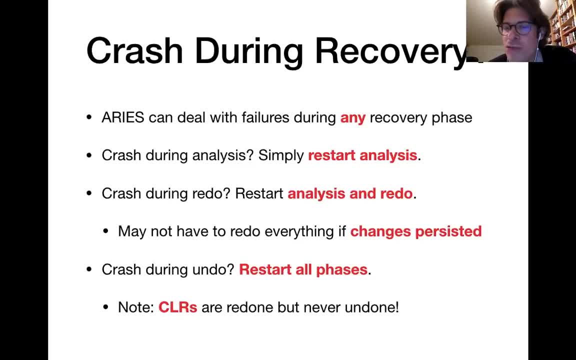 well, now, perhaps, if you're lucky, then some of the um, if you're lucky, then some of the um, if you're lucky, then some of the um redo operations. they have become redo operations. they have become redo operations. they have become unnecessary because during the first, unnecessary because during the first. 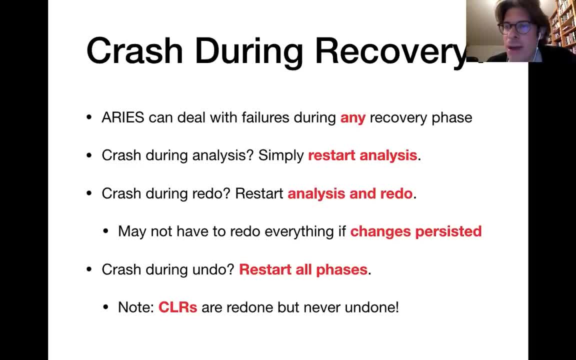 unnecessary because during the first recovery, a try you um manage to get recovery, a try you um manage to get recovery, a try you um manage to get some of those changes to hard disk, for some of those changes to hard disk. for some of those changes to hard disk, for instance, 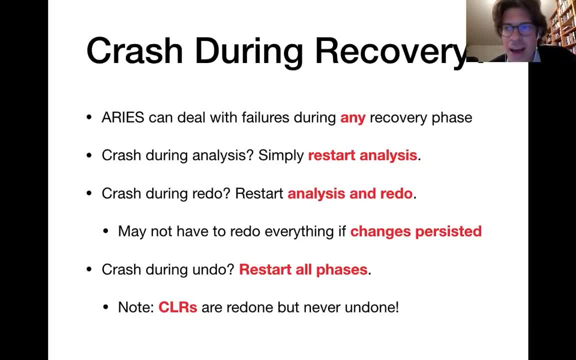 instance, instance, and similarly for the uh for the, and similarly for the uh for the, and similarly for the uh for the undo phase. if we have a crash there, then undo phase. if we have a crash there, then undo phase. if we have a crash there, then we again start. 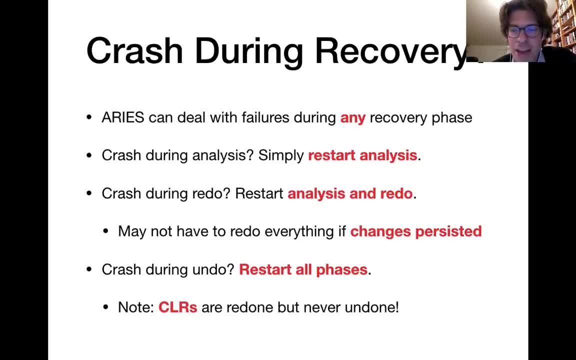 we again start, we again start. all faces from the analysis, all faces from the analysis, all faces from the analysis, phase um here, um, phase um, here, um phase um, here, um, we might already have started to and do we might already have started to and do we might already have started to and do some um operations, uh, from transactions. 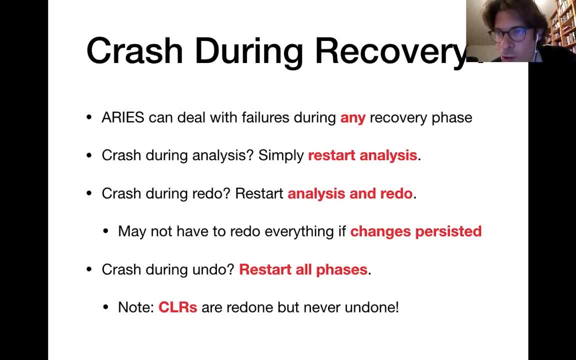 some um operations, uh from transactions. some um operations, uh from transactions. in that case, we have written the. in that case, we have written the. in that case we have written the corresponding compensation log records, corresponding compensation log records, corresponding compensation log records. so we would have redone those. 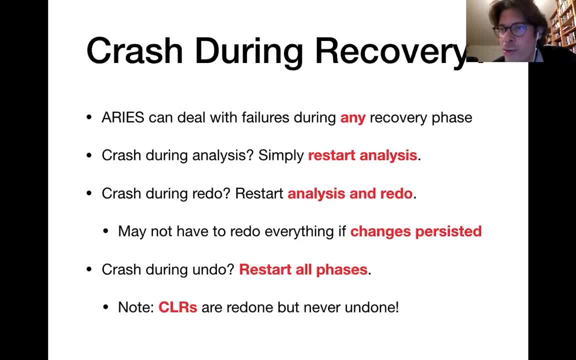 so we would have redone those. so we would have redone those compensation compensation, compensation log records during the redo phase, log records during the redo phase, log records during the redo phase. so um we can essentially so, um we can essentially so, um we can essentially start undo it. so some of the undo 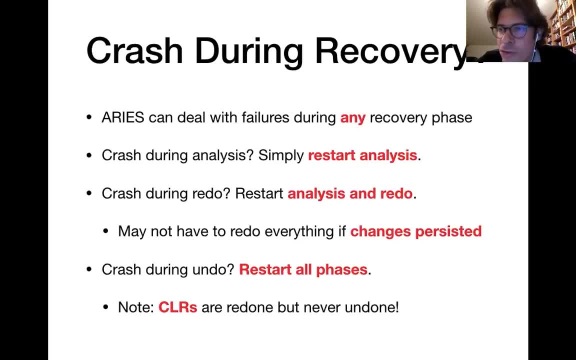 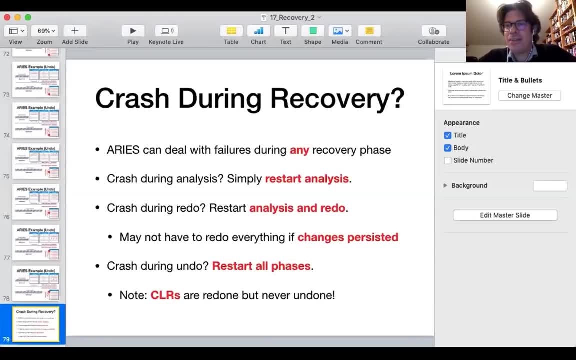 start undo it. so some of the undo. start undo it. so some of the undo operations, operations, operations. i have already happened in the redo, i have already happened in the redo, i have already happened in the redo: phase, phase, phase. all right, all right, all right. so that is the. 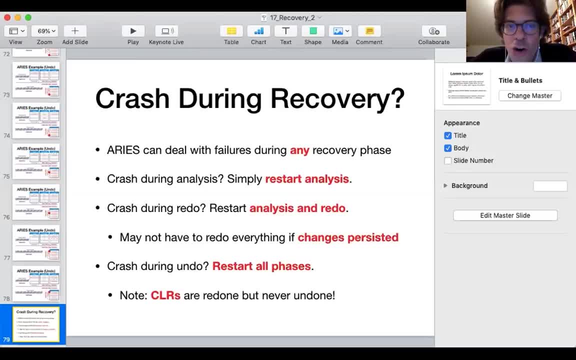 so that is the, so that is the aries algorithm and that concludes the aries algorithm and that concludes the aries algorithm and that concludes the chapter, chapter, chapter on a recovery. we have now essentially on a recovery. we have now essentially on a recovery. we have now essentially seen all the different. 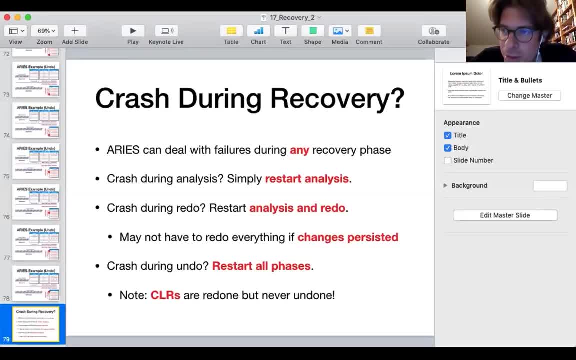 seen all the different, seen all the different components of a traditional relational components of a traditional relational components of a traditional relational database management system, database management system, database management system. in the next lecture we're gonna go in the next lecture we're gonna go in the next lecture we're gonna go a little bit over the material that we